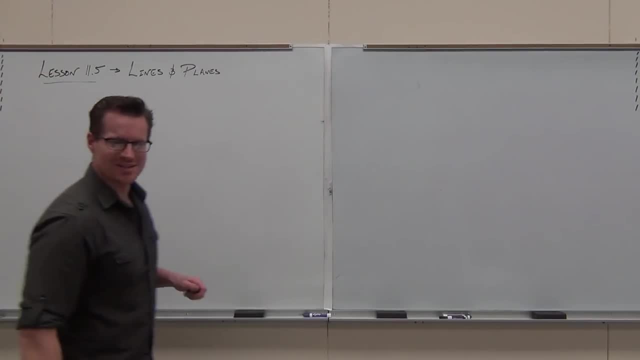 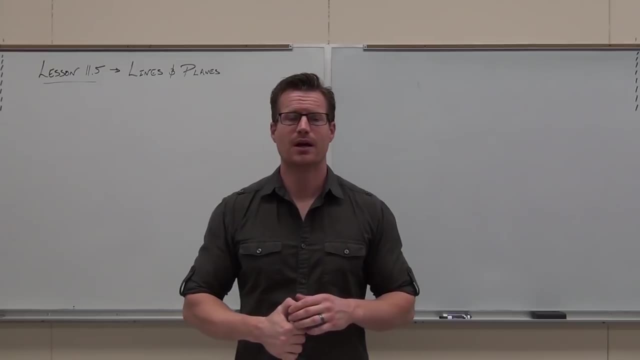 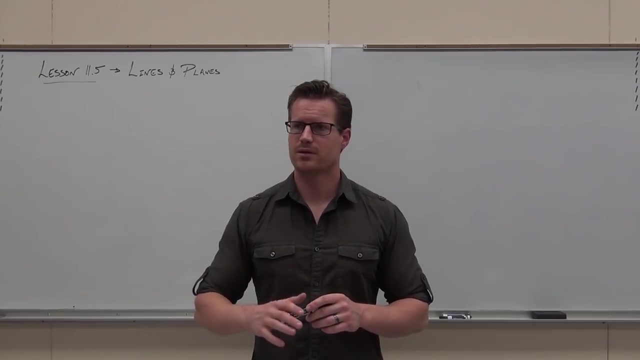 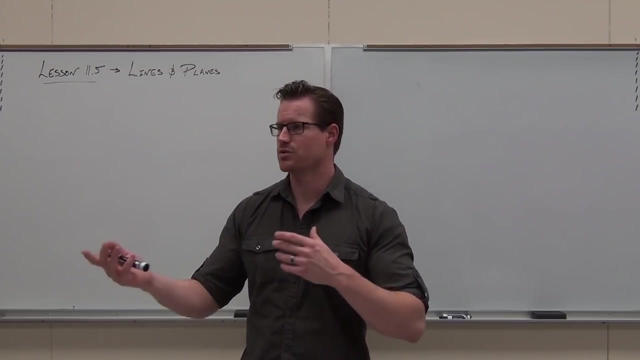 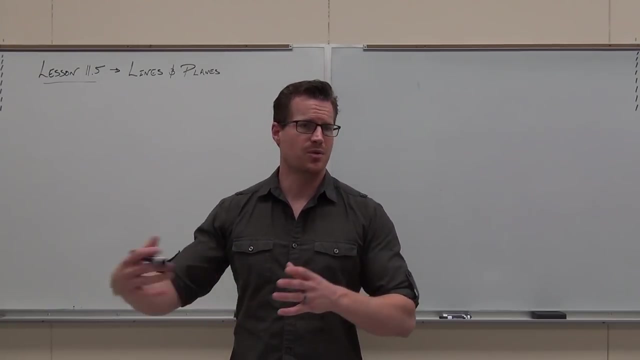 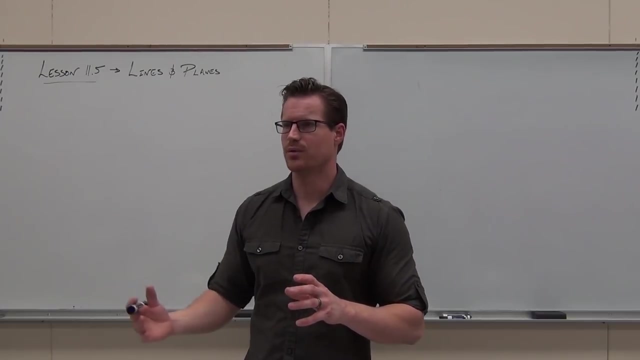 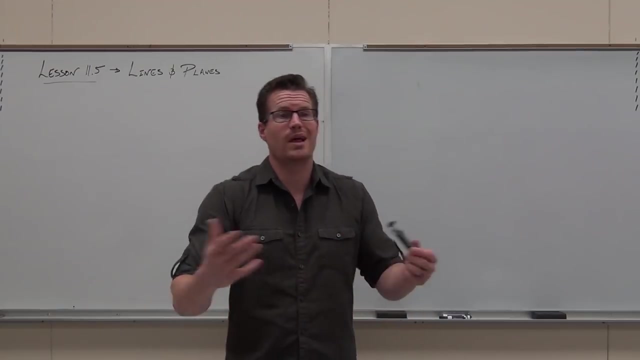 Thank you for watching. Be very careful when you're going through them so you later on, when you're done with the homework, you don't make those mistakes anymore. So we'll talk about those formulas. Honestly, it's probably enough to talk about the formulas- Hey, here's how it works. But we're going to spend the vast majority talking about the harder examples, like: how do you use this stuff? We'll make it through lines pretty quickly and then we'll talk about planes And then, as I said, the last thing we're going to do is talk about how to find the distance between a lot of these different things: A point in a plane, a point in a line, parallel planes, skew lines- What skew line even means? 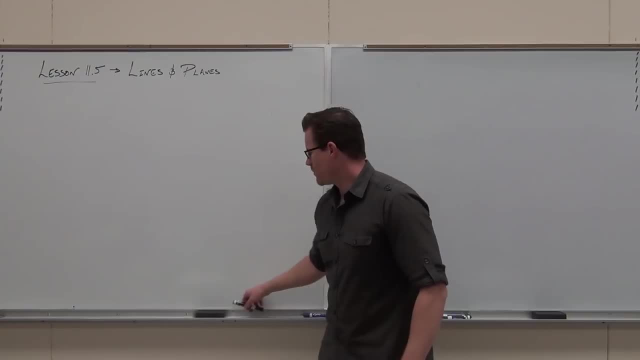 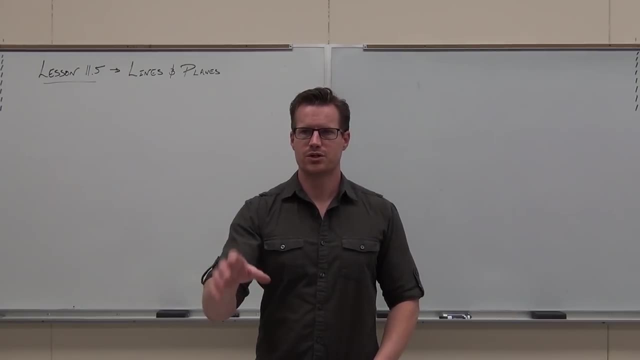 And how it all starts is really just an understanding. How would we define a line? How would we do that? Now, let's start here. What do you need in order to define a unique line? You need two points, Okay, great, In two dimensions, and that's still true. In two dimensions, we go. well, you need two points, or you need one point and good. 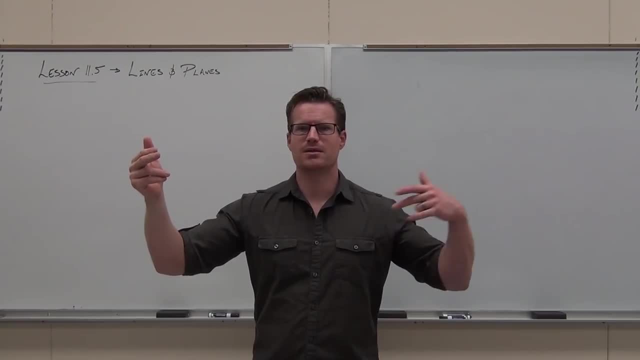 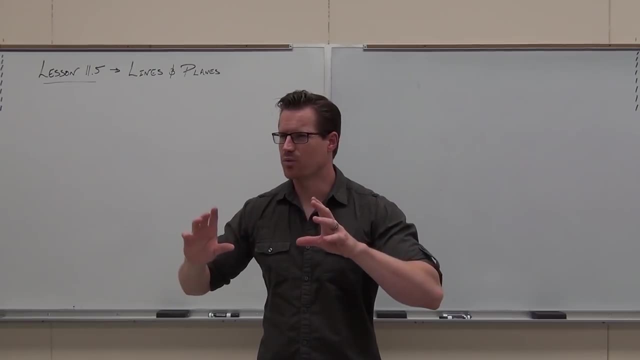 Well, in 3D we lose the slope idea But we gain the vector idea. So in 3D we go: yeah, you could do this with two points, Or, just like the point slope thing, we could do it with one point and a vector that has the same direction. 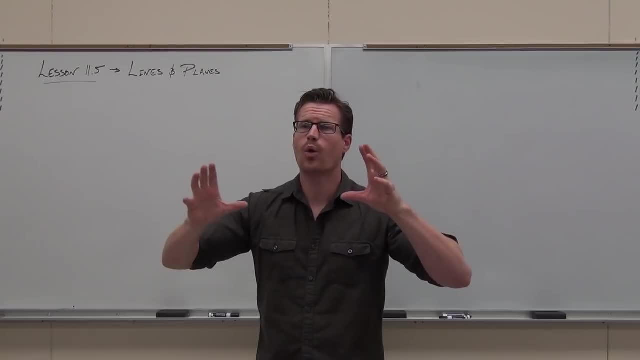 Okay, same direction. What's that mean? Same unit vector, Or it means that they are parallel, So we can do it with a point and a vector that's going in the same direction, just parallel to that line. That's the idea on how we're going to build the formula for a line. 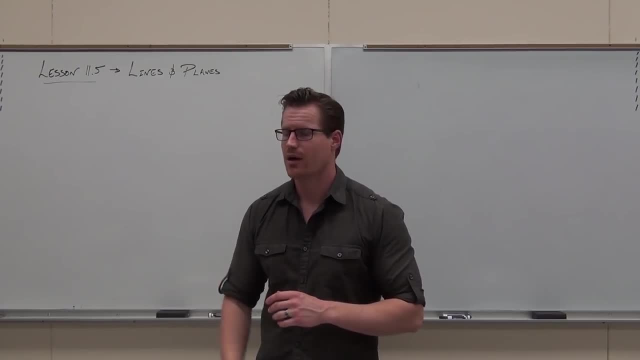 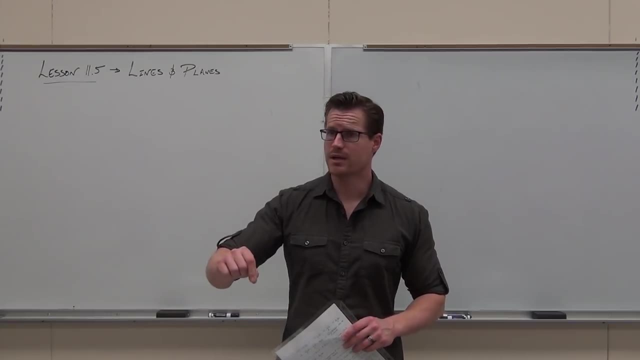 I'm going to give you, We're going to build it, We're going to do it from scratch, so you actually understand where everything's coming from. So let's write just a couple things out. In order to determine a line in space, you need a point and you need a vector in the same direction of that line. 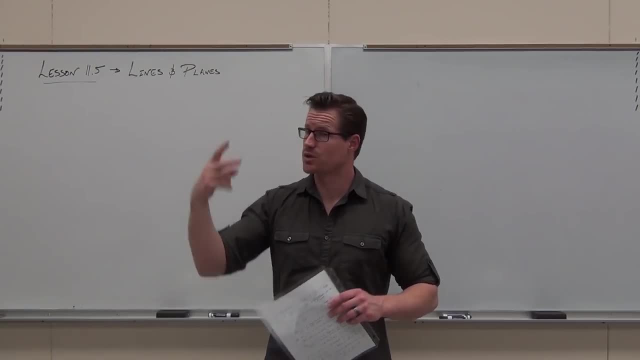 So you need to know where it's headed. That's the idea. So we could do this with two points, because, hey, between any two points you can find a vector right, Just like between any two points you can find a slope. 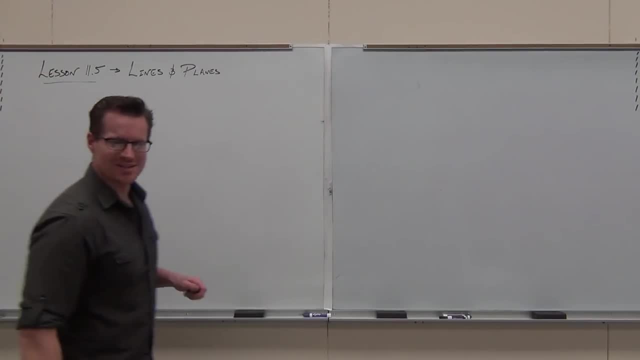 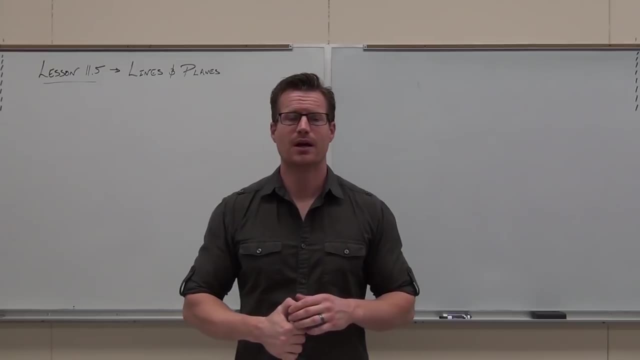 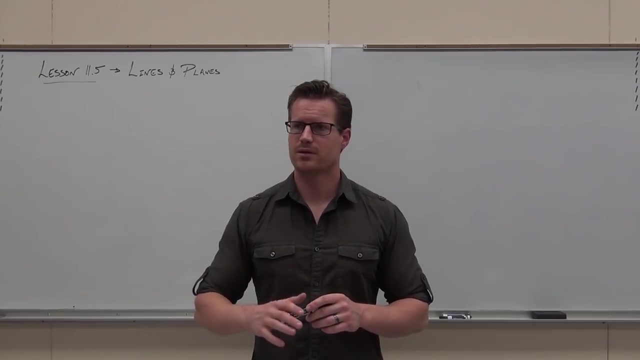 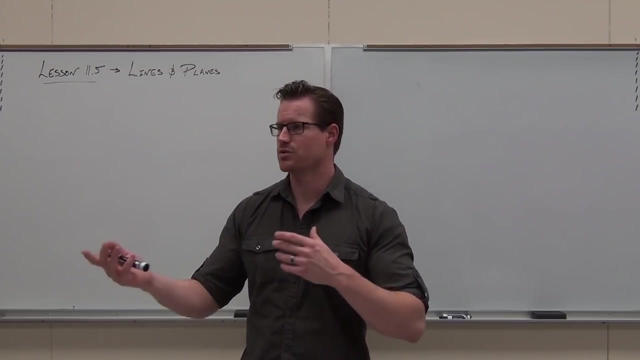 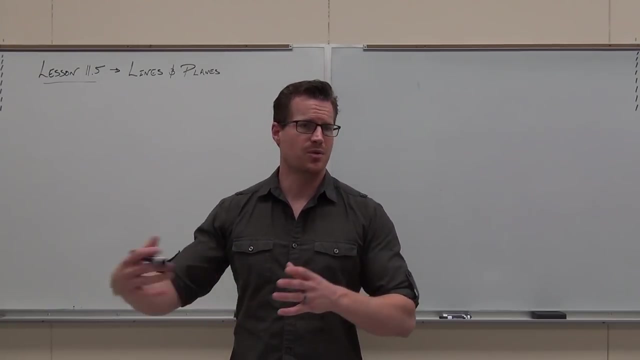 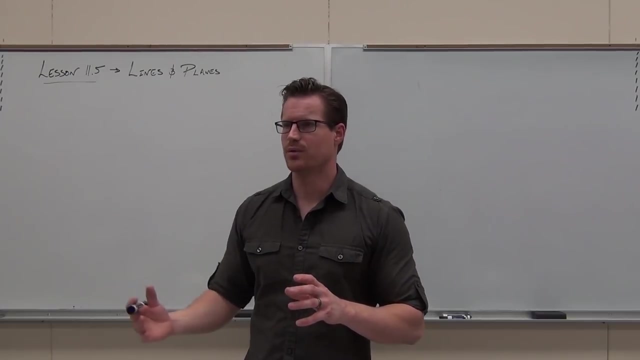 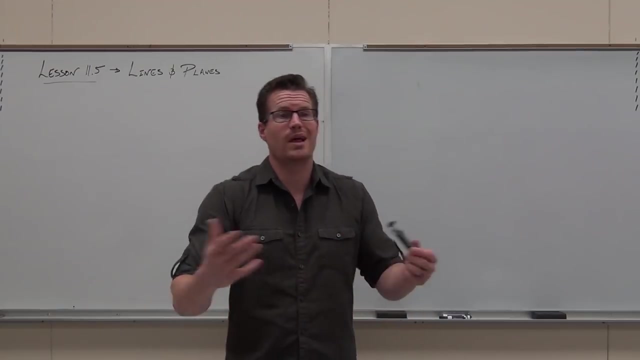 Thank you for watching. Be very careful when you're going through them so you later on, when you're done with the homework, you don't make those mistakes anymore. So we'll talk about those formulas. Honestly, it's probably enough to talk about the formulas- Hey, here's how it works. But we're going to spend the vast majority talking about the harder examples, like: how do you use this stuff? We'll make it through lines pretty quickly and then we'll talk about planes And then, as I said, the last thing we're going to do is talk about how to find the distance between a lot of these different things: A point in a plane, a point in a line, parallel planes, skew lines- What skew line even means? 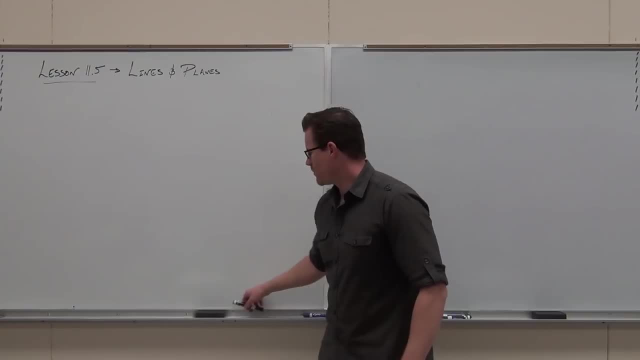 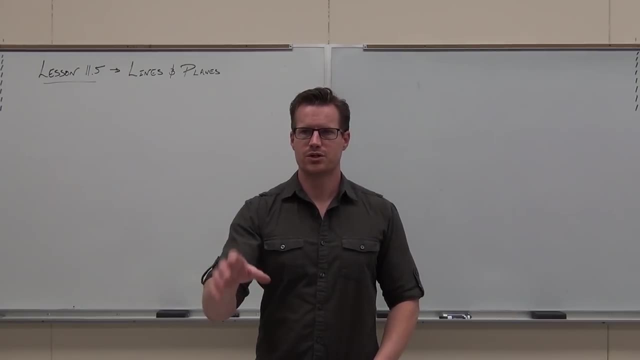 And how it all starts is really just an understanding. How would we define a line? How would we do that? Now, let's start here. What do you need in order to define a unique line? You need two points, Okay, great, In two dimensions, and that's still true. In two dimensions, we go. well, you need two points, or you need one point and good. 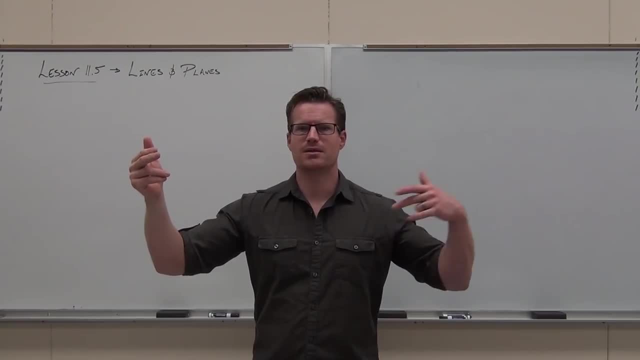 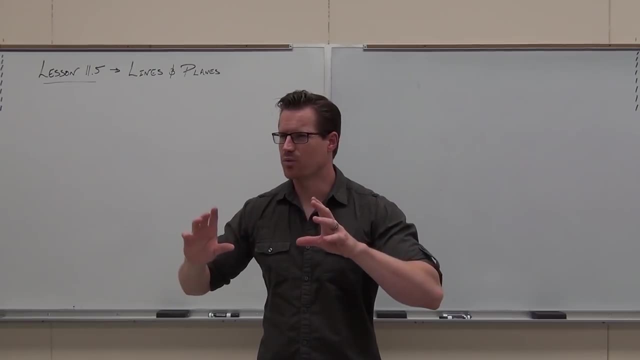 Well, in 3D we lose the slope idea But we gain the vector idea. So in 3D we go: yeah, you could do this with two points, Or, just like the point slope thing, we could do it with one point and a vector that has the same direction. 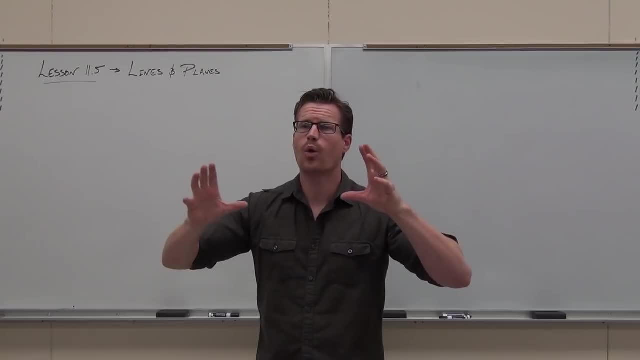 Okay, same direction. What's that mean? Same unit vector, Or it means that they are parallel, So we can do it with a point and a vector that's going in the same direction, just parallel to that line. That's the idea on how we're going to build the formula for a line. 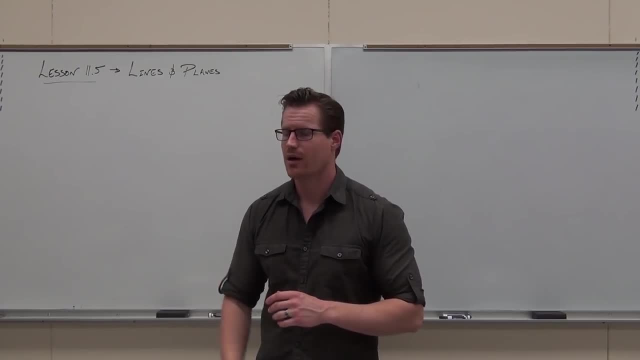 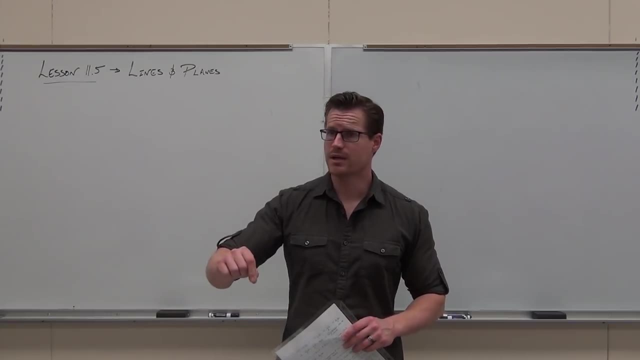 I'm going to give you, We're going to build it, We're going to do it from scratch, so you actually understand where everything's coming from. So let's write just a couple things out. In order to determine a line in space, you need a point and you need a vector in the same direction of that line. 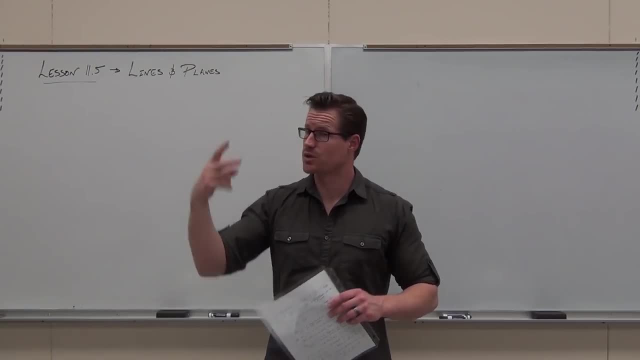 So you need to know where it's headed. That's the idea. So we could do this with two points, because, hey, between any two points you can find a vector right, Just like between any two points you can find a slope. 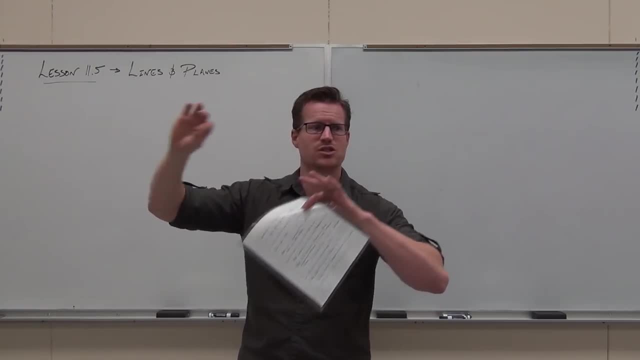 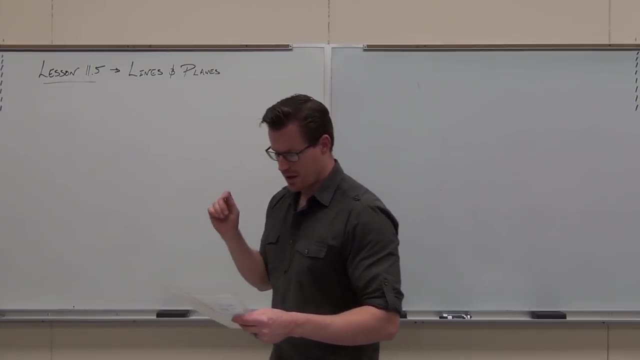 So the idea of a vector takes the idea of a slope and pushes it to 3D. That is what's happening. Head nod. if you're okay with the idea behind it, Let me draw you a little picture. Then we're going to do everything. 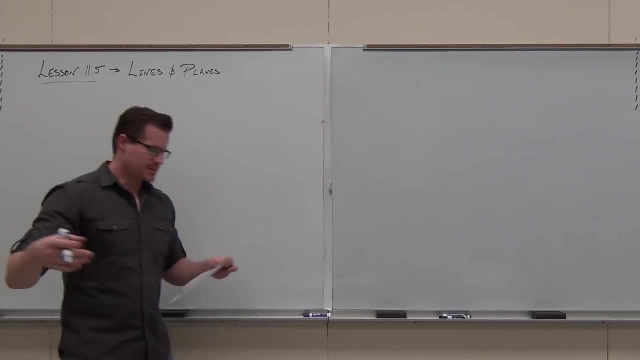 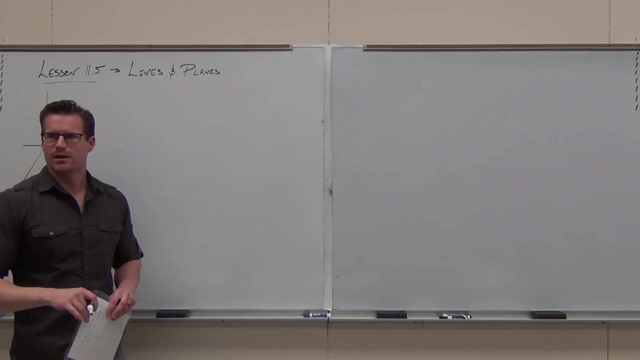 We'll do some examples. Basically, here's the idea. It says hey, in 3D. if I wanted to find a line through a random point, all I need is that point, that specific point. Okay, So I want to find a point. 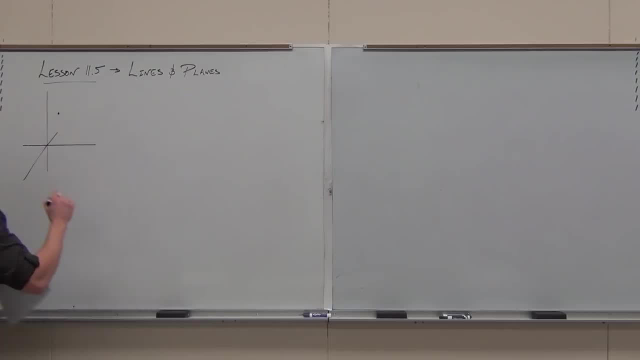 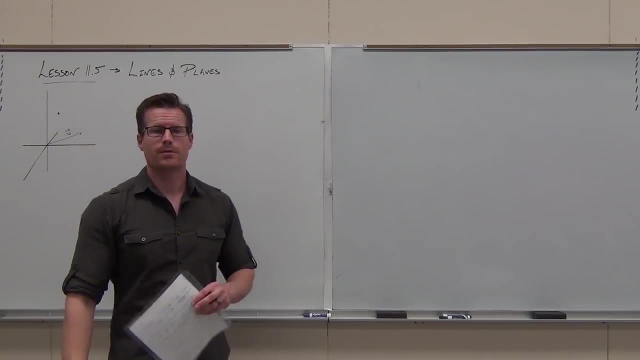 I want to go through. I don't know what point that is, but I want to go through that point and I want it in that direction. Well, that's all I really need. All I need is what direction I'm headed and what point I'm going through. 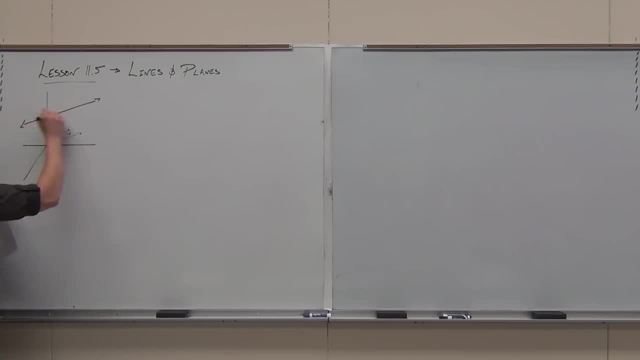 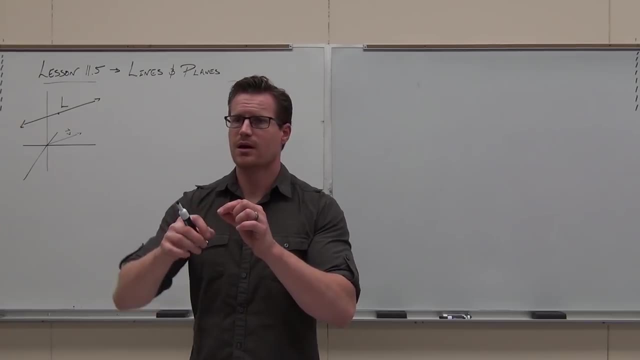 And if I can do that, then I know the line. It's going to be parallel to that vector. That's the whole idea. You have a point: Find a vector of the direction You want to go in, and then we can build this formula from it. 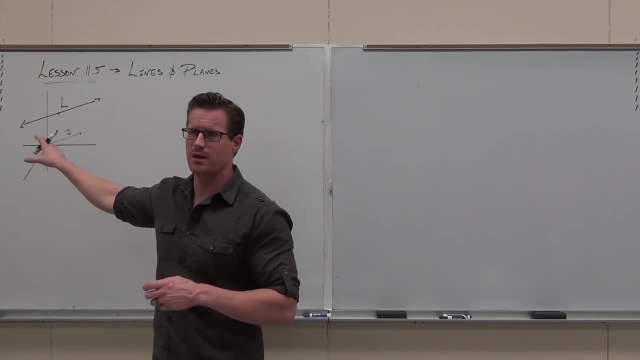 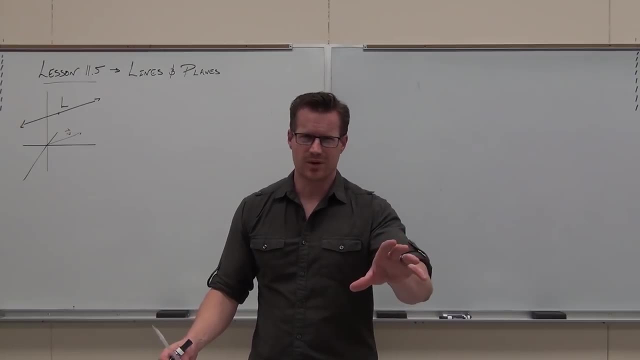 So keep this picture in your mind as we're coming up with the formula and you're going to be a lot better off for it. So this really acts like point slope. It's just we have now point vector. Notice, I already said it, but notice, if I give you two points, you can always find the vector between those two points. 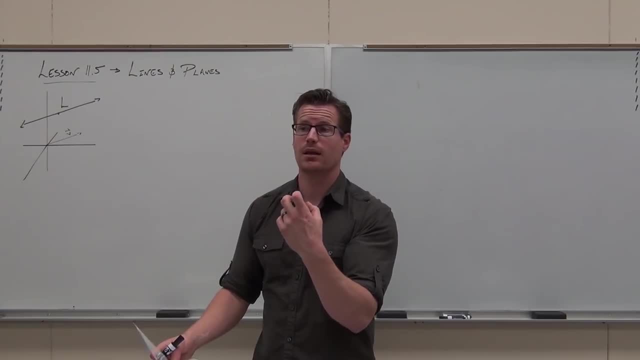 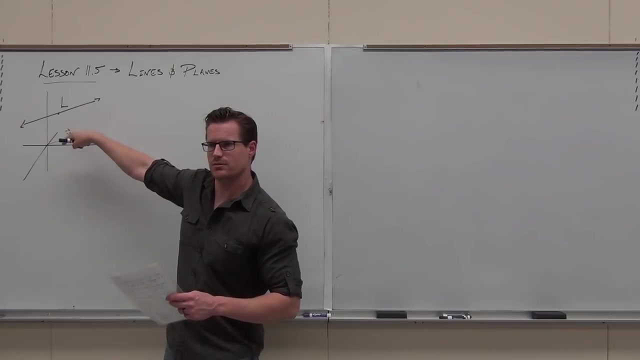 Does that make sense? So what two things do we need to make a line Now? point and vector, Direction, vector. That's all we need: The vector of the direction. So let's start building this. So, since the line is going to be parallel to the vector, so I'm going to write all this stuff out. 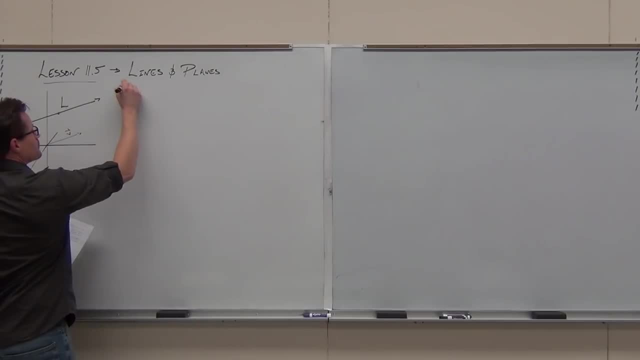 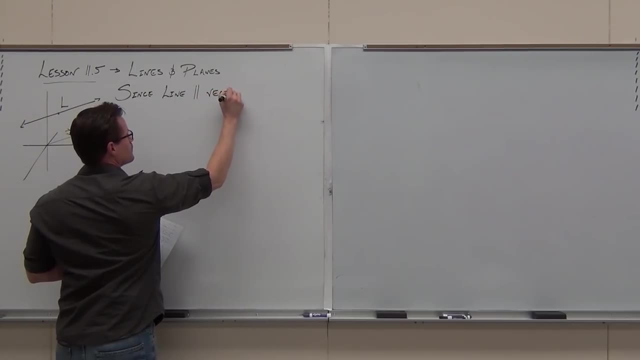 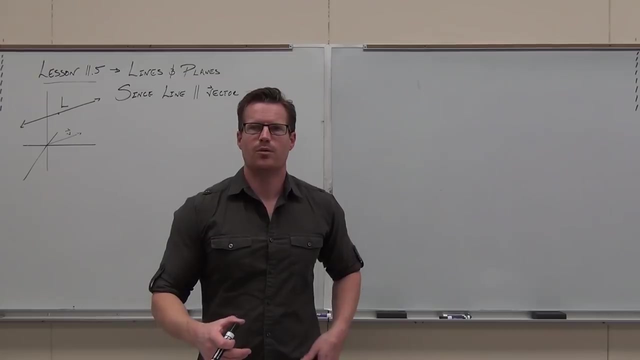 So the line is going to be parallel to the vector, Just for fun. Hey, what do you know about things that are parallel? And I know they have the same unit vector, but I want the other one. What They are? someone said it. 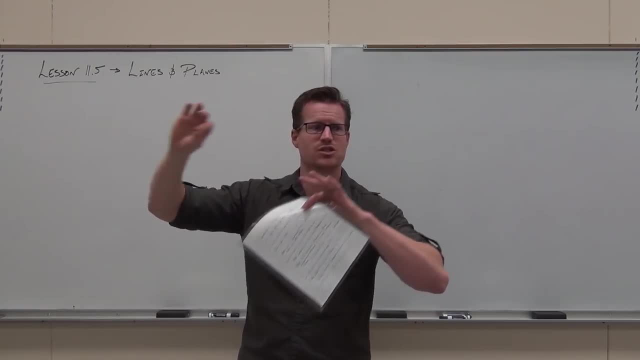 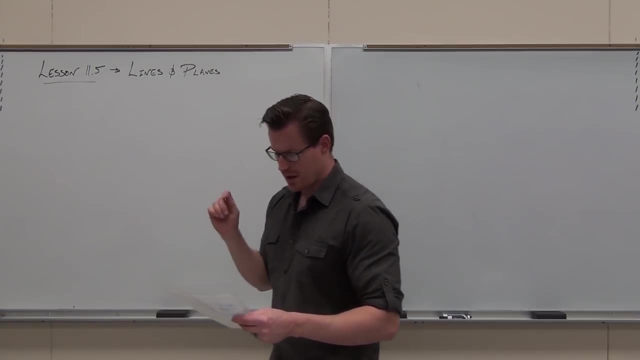 So the idea of a vector takes the idea of a slope and pushes it to 3D. That is what's happening. Head nod. if you're okay with the idea behind it, Let me draw you a little picture. Then we're going to do everything. 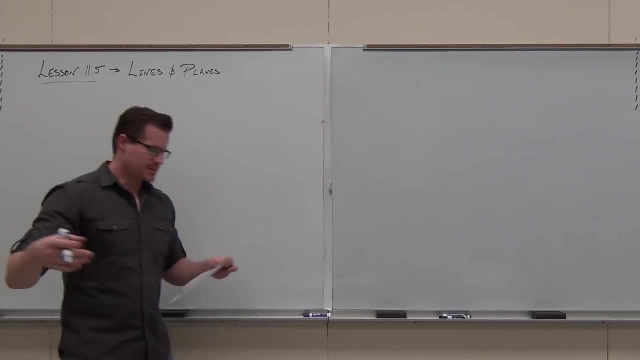 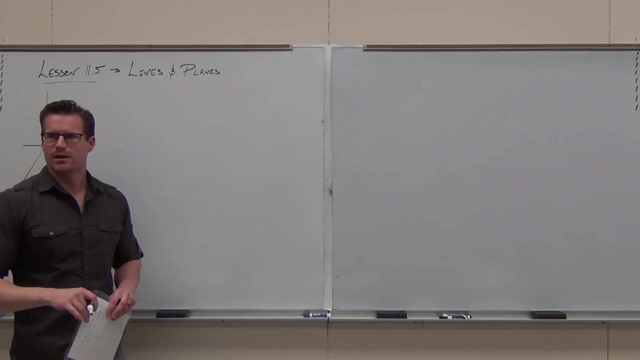 We'll do some examples. Basically, here's the idea. It says hey, in 3D. if I wanted to find a line through a random point, all I need is that point, that specific point. Okay, So I want to find a point. 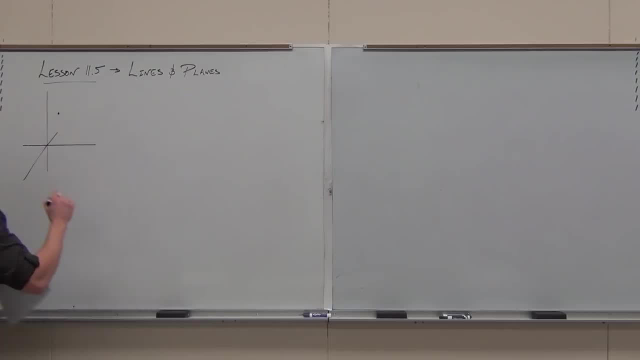 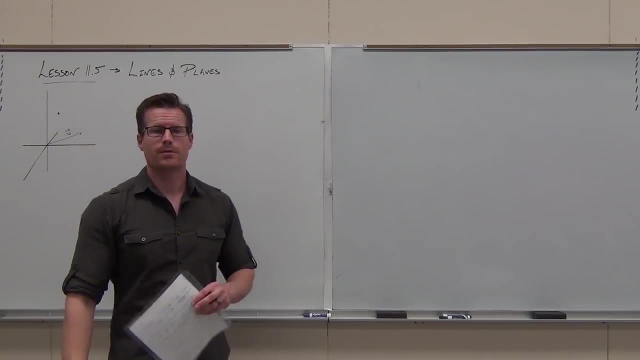 I want to go through. I don't know what point that is, but I want to go through that point and I want it in that direction. Well, that's all I really need. All I need is what direction I'm headed and what point I'm going through. 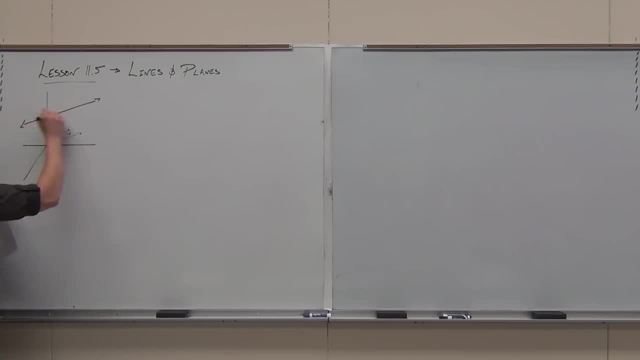 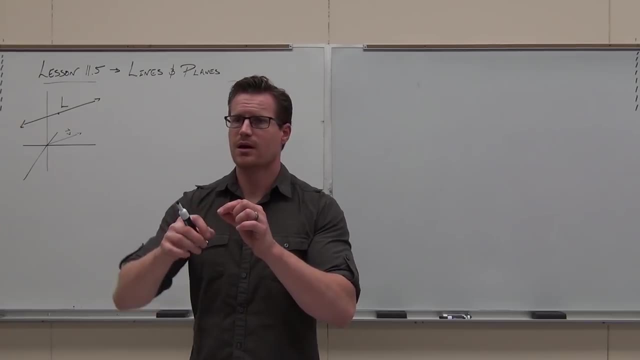 And if I can do that, then I know the line. It's going to be parallel to that vector. That's the whole idea. You have a point: Find a vector of the direction You want to go in, and then we can build this formula from it. 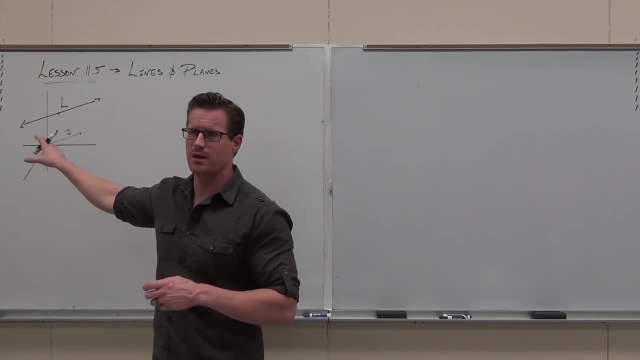 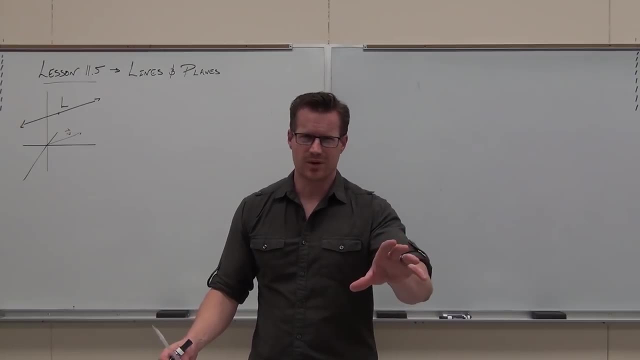 So keep this picture in your mind as we're coming up with the formula and you're going to be a lot better off for it. So this really acts like point slope. It's just we have now point vector. Notice, I already said it, but notice, if I give you two points, you can always find the vector between those two points. 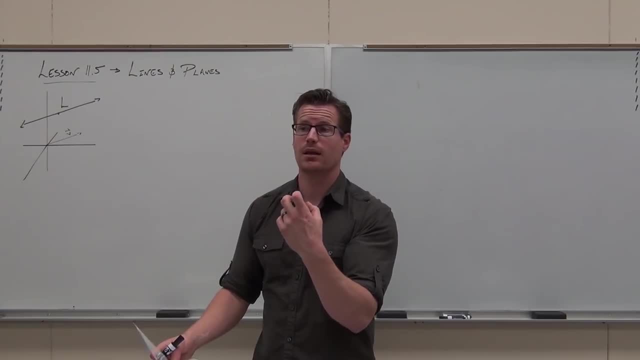 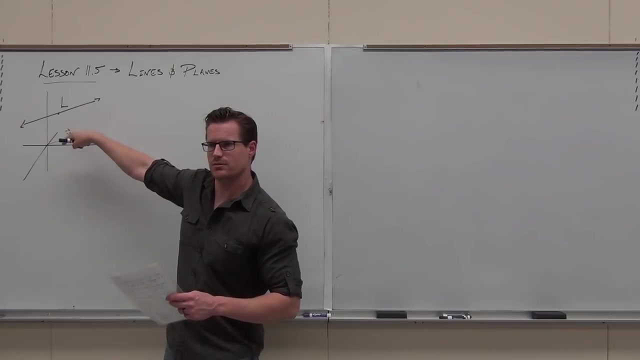 Does that make sense? So what two things do we need to make a line Now? point and vector, Direction, vector. That's all we need: The vector of the direction. So let's start building this. So, since the line is going to be parallel to the vector, so I'm going to write all this stuff out. 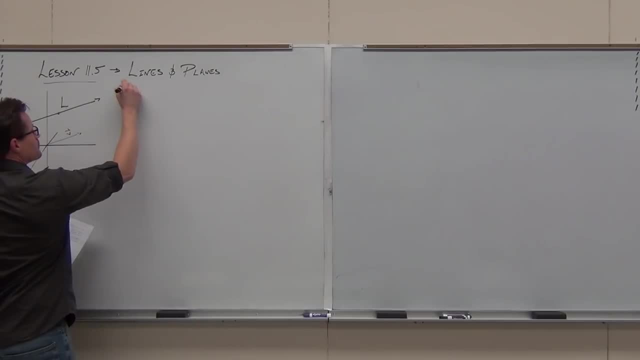 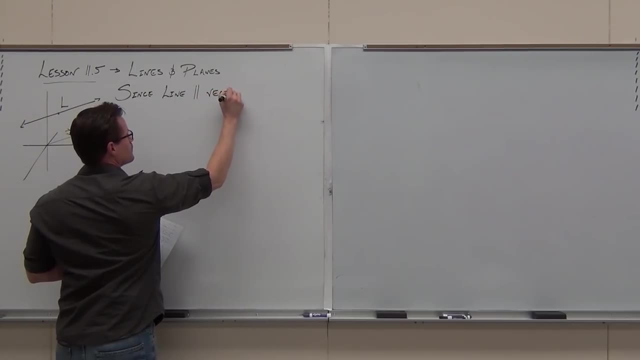 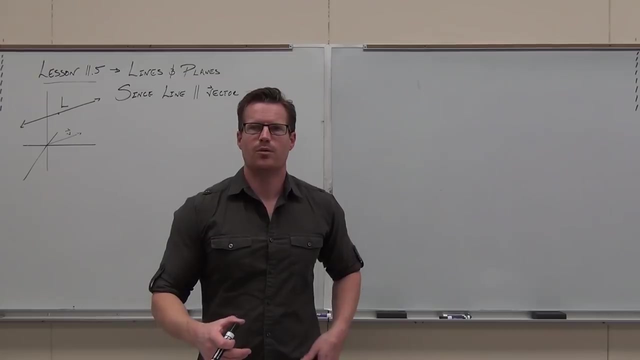 So the line is going to be parallel to the vector, Just for fun. Hey, what do you know about things that are parallel? And I know they have the same unit vector, but I want the other one. What They are? someone said it. 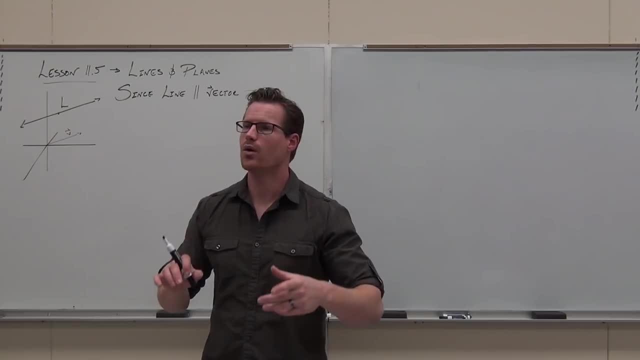 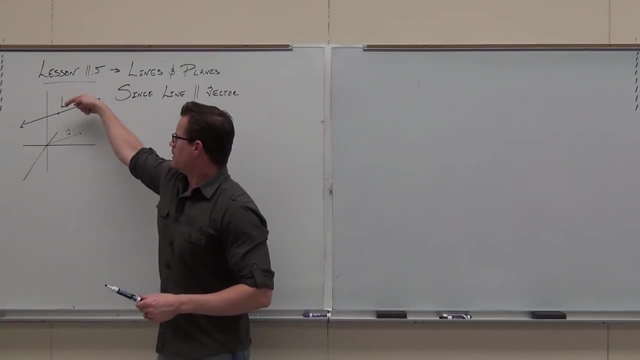 Say it louder: Scalar. They're scalar, Multiples, Multiples. Oh So okay. So stick with me here. This is the whole big deal, okay. And then everything flows from. algebraically, It's really easy. The vector of that line and the direction vector are parallel vectors. 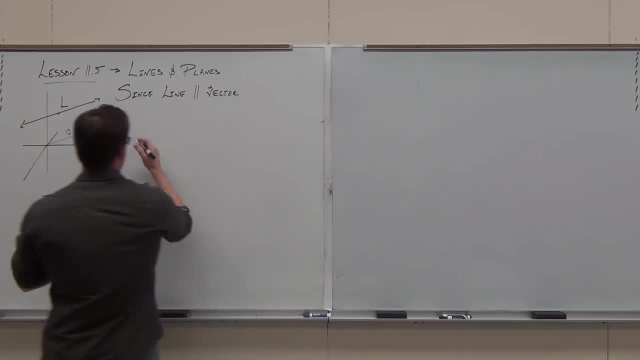 Yeah, Does that make sense If they are parallel vectors? So the vector of the line has to be a scalar multiple of the direction vector. 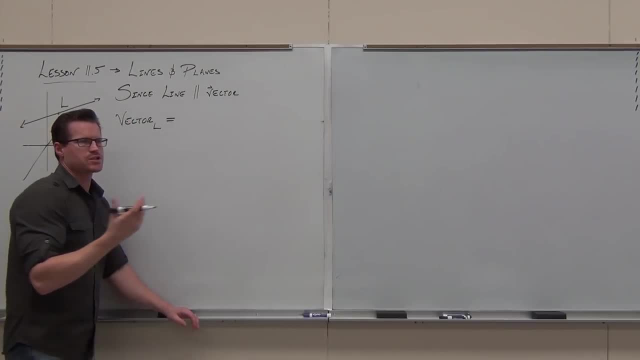 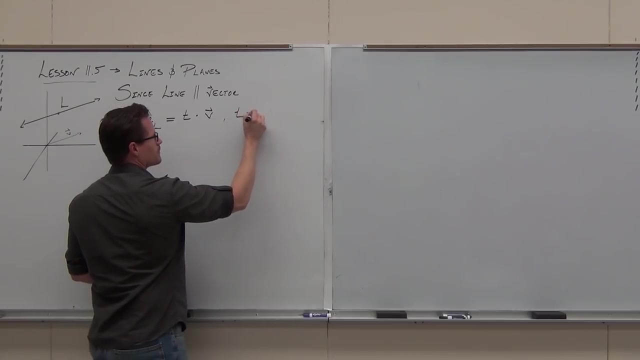 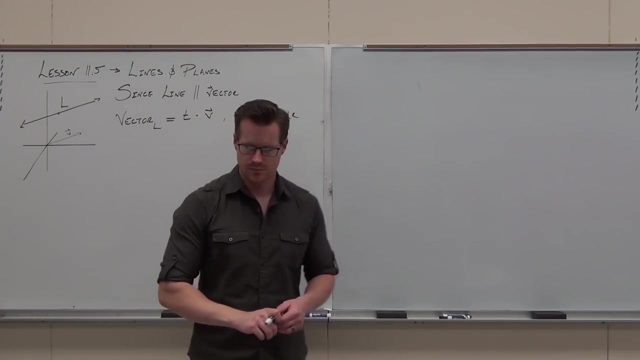 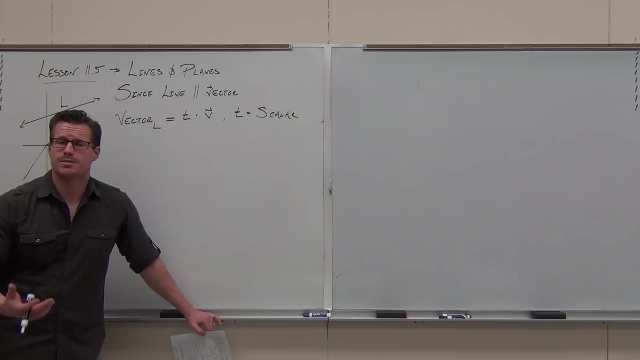 That's what we're going to call this thing: the direction vector. Well, if they're scalar multiples, let's just give it like a little letter to represent the scalar. Let's call it T Y. you'll see why. I know it's a. you know we've talked. I've talked it three times now, but I want to make sure you get this, because from this flows everything else. okay, 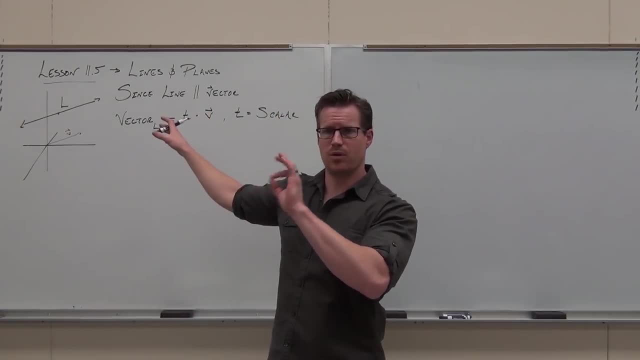 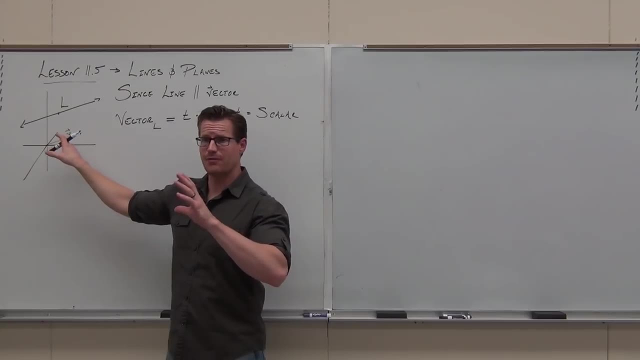 Do you understand the idea? We need a point, There's our point. We need a vector that says: I'm headed in this direction. There's our vector. If we have the line in the same direction as that vector- direction, vector- then the line is parallel to the vector and I'll be okay with that. 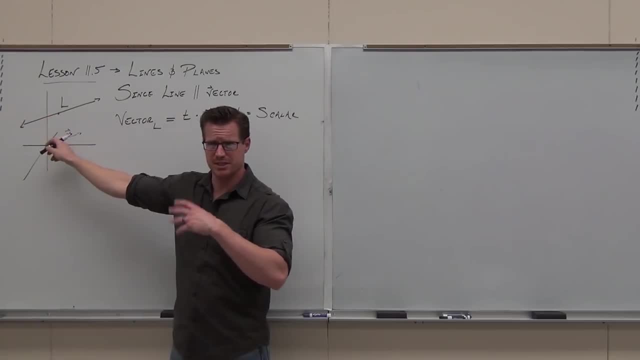 Any vector on this line is parallel to the vector. Any vector on this line is going to be parallel to this particular vector. that we're saying is in the same direction as the line. What that means is any vector on here- the vector of the line- is going to be a scalar multiple of this vector. 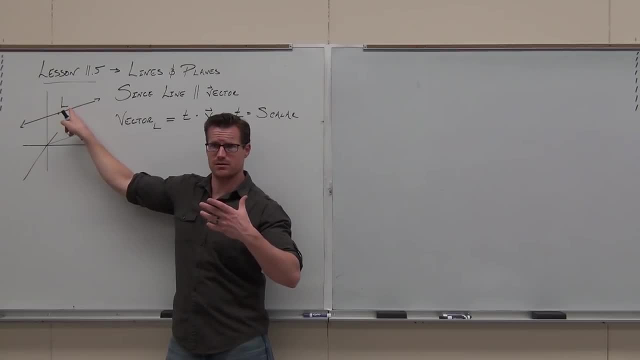 And that's all I'm saying. The vector on this line or of this line, any vector in there, is going to be a scalar multiple of this direction vector. That's the idea. I don't know if you're okay with that one. 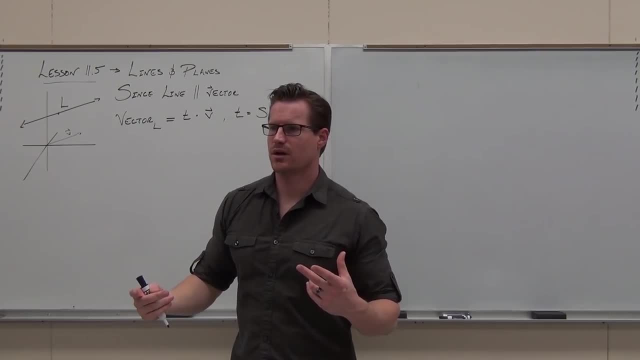 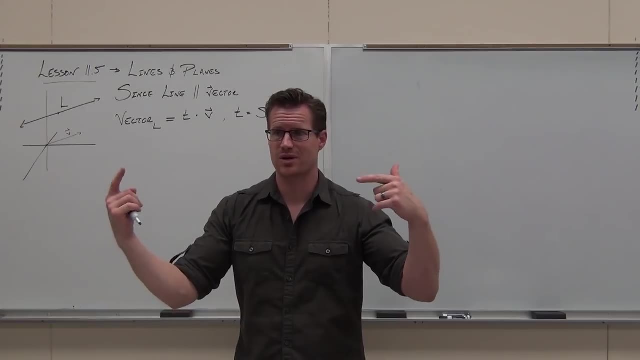 We also said something else. We said: given any two points on a line, You can always find the vector between them. Do you remember doing that? Just subtract the values of X, subtract the values of Y, subtract the values of Z. you get a position vector. 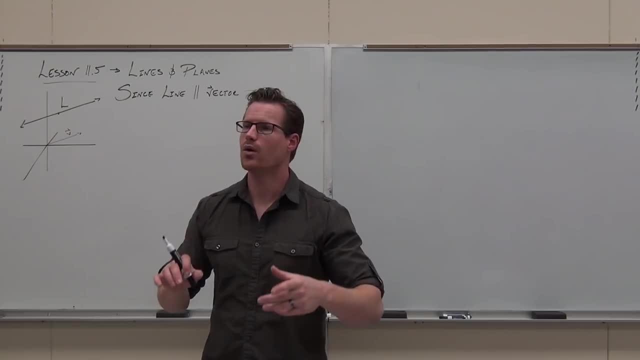 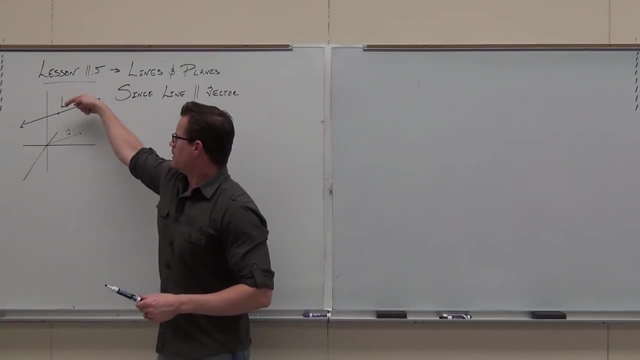 Say it louder: Scalar. They're scalar, Multiples, Multiples. Oh So okay. So stick with me here. This is the whole big deal, okay. And then everything flows from. algebraically, It's really easy. The vector of that line and the direction vector are parallel vectors. 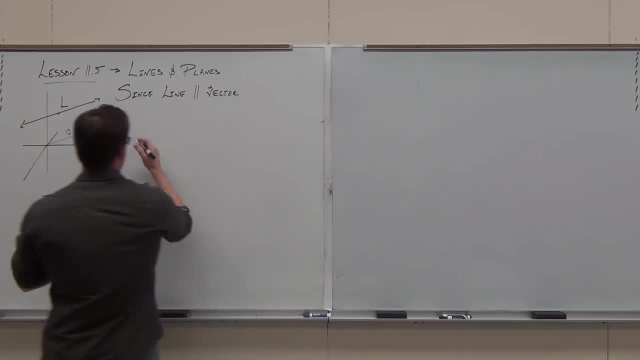 Yeah, Does that make sense If they are parallel vectors? So the vector of the line has to be a scalar multiple of the direction vector. 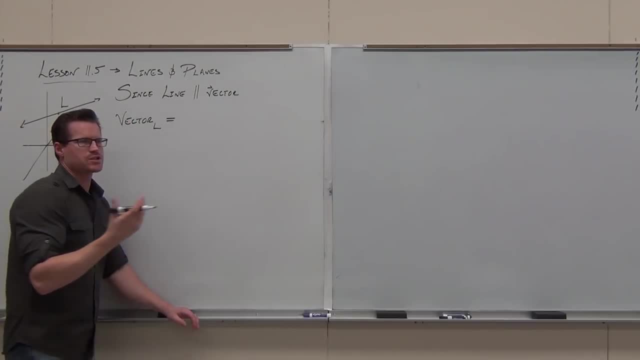 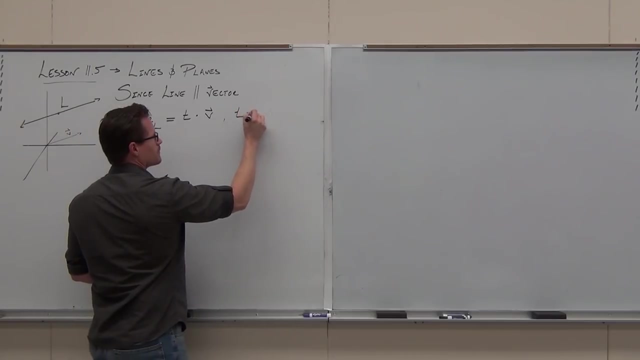 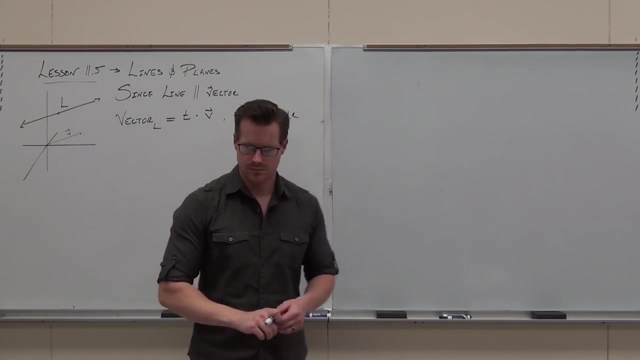 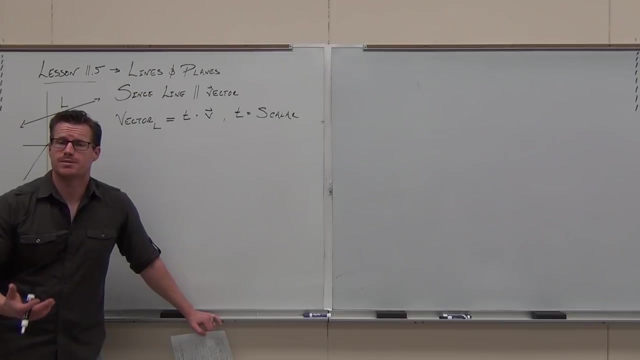 That's what we're going to call this thing: the direction vector. Well, if they're scalar multiples, let's just give it like a little letter to represent the scalar. Let's call it T Y. you'll see why. I know it said. you know we've talked. I've talked it three times now, but I want to make sure you get this, because from this flows everything else. okay. 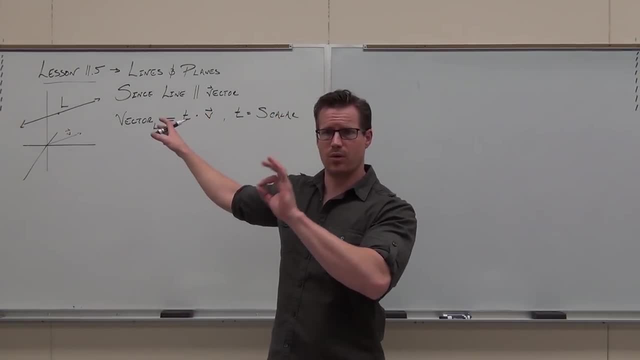 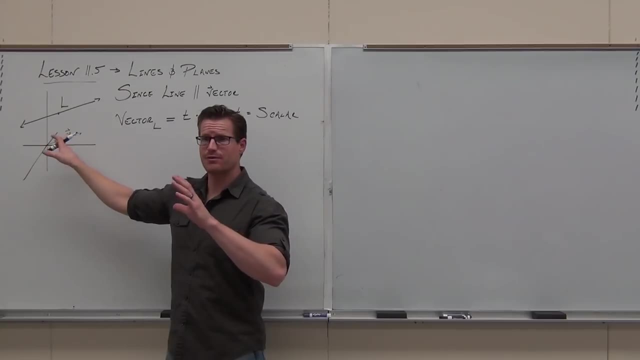 Do you understand the idea? We need a point, There's our point. We need a vector that says: I'm headed in this direction. There's our vector. If we have the line in the same direction as that vector- direction, vector- then the line is parallel to the vector and I'll be okay with that. 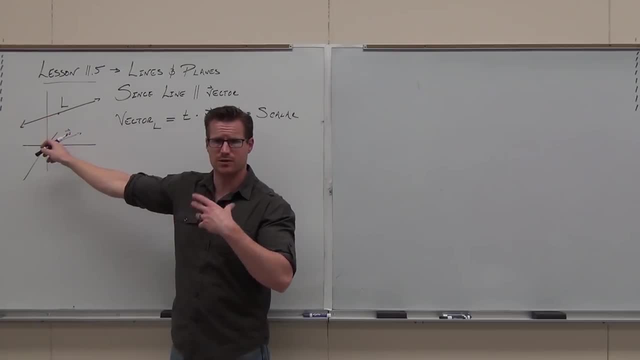 Any vector on this line. This line is going to be parallel to this particular vector that we're saying is in the same direction as the line. What that means is any vector on here. the vector of the line is going to be a scalar multiple of this vector. 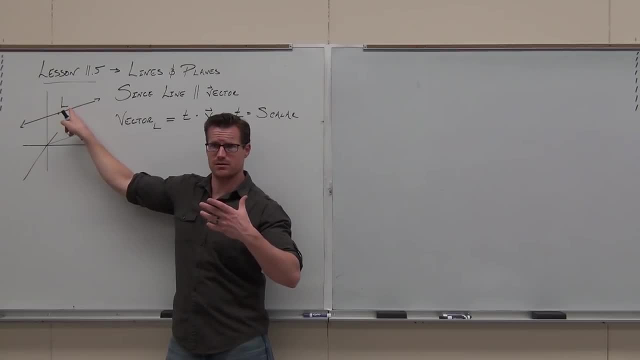 And that's all I'm saying. The vector on this line or of this line, any vector in there, is going to be a scalar multiple of this direction vector. That's the idea. I don't know if you're okay with that one. 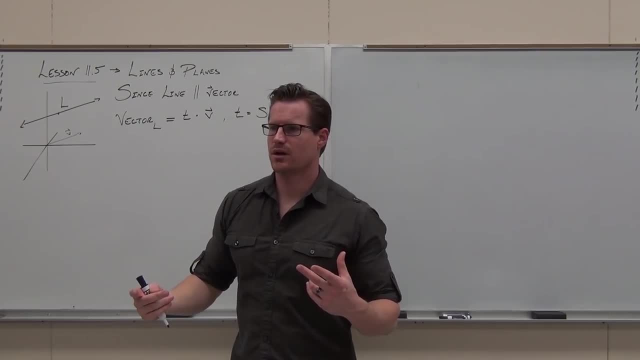 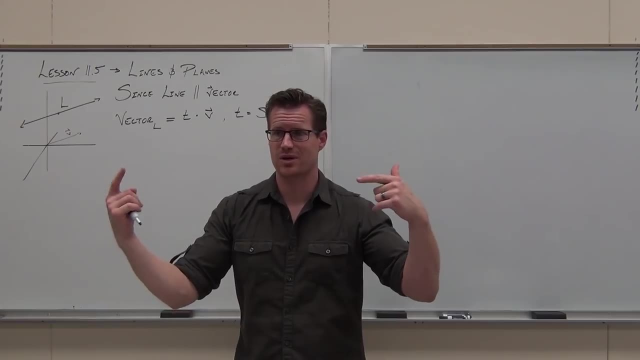 We also said something else. We said: given any two points on a line, You can always find the vector between them. Do you remember doing that? Just subtract the values of X, subtract the values of Y, subtract the values of Z. you get a position vector. 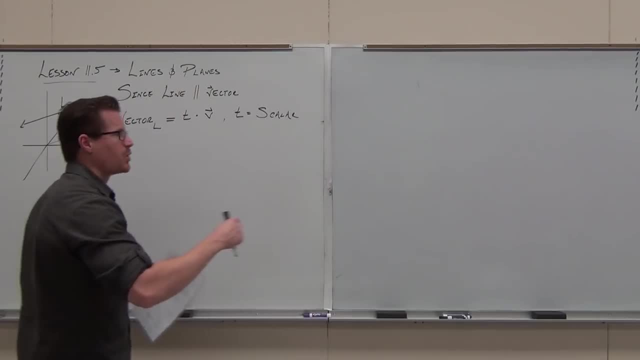 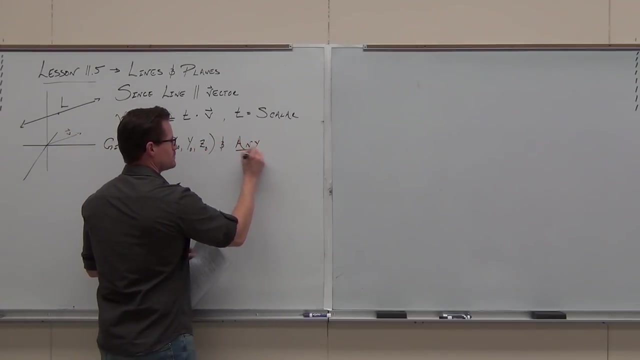 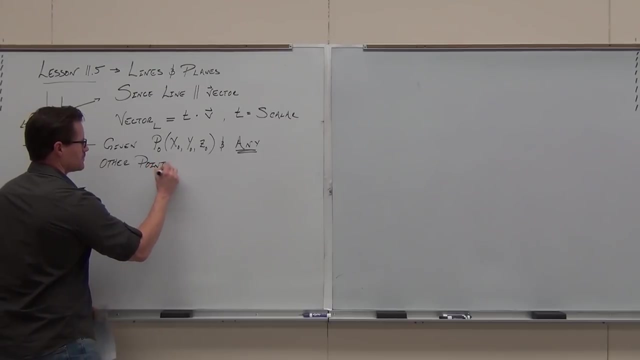 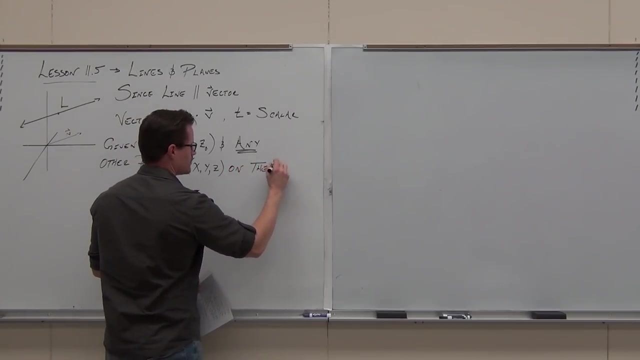 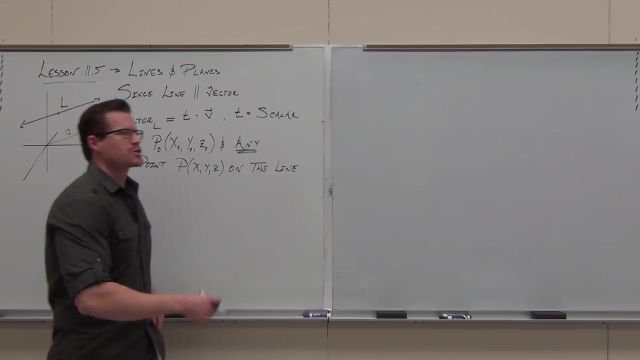 Pretty, not so bad, So let's talk about this. So, given a point, We call the actual points the piece of zero, like a specified point on a line And any other point. So if I give us a point, just a specified point, 3, 1,, 2.. 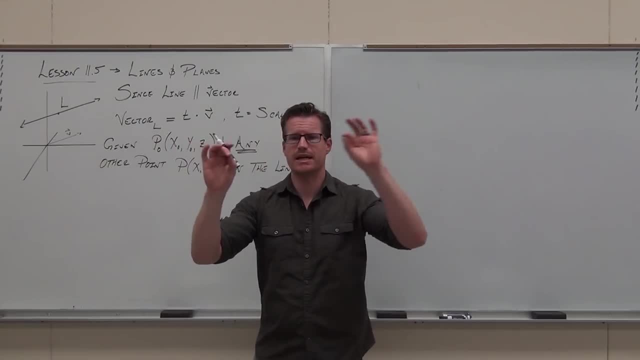 And any other point: X, Y Z. So we're letting that float, But it's any point on that line. Do you guys understand what I'm talking about? Where we're going to get our variable is from this: X, Y Z. 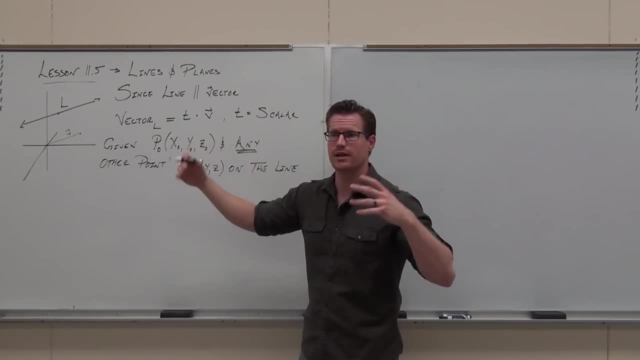 So I have a point on the line And any other point it just has to be on the line, I don't care what it is. We can always find a vector between this point and this point. We can always find that vector. 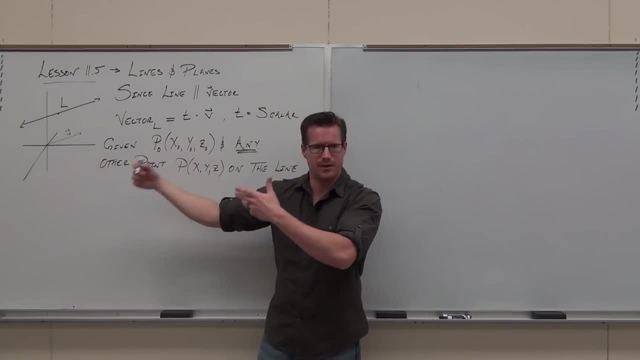 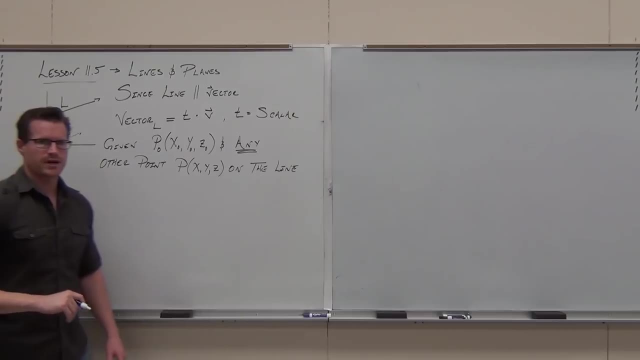 And it's going to be a vector on that line, because these two points are on that line, It's got to be there. So the vector of the line That's that little dot, That little L there. So the vector of the line is going to be- let's call it the same. 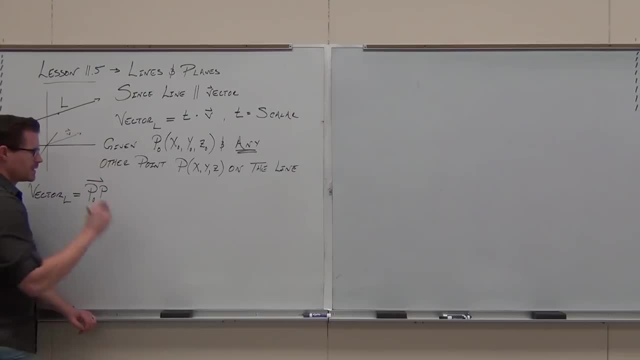 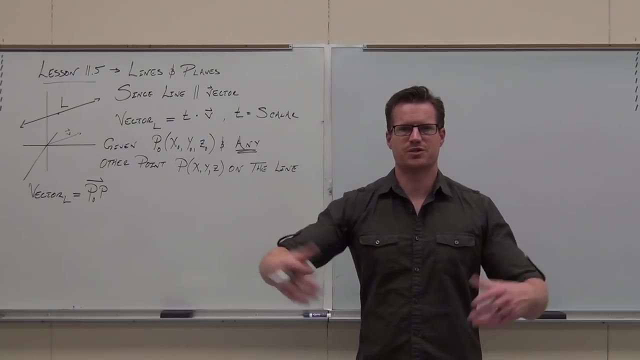 It's going to be the same as the vector between P sub zero and P. Any other point, We'll do a 20-second recap, because then it's pure algebra. You guys, we already talked about it, But you get the idea. 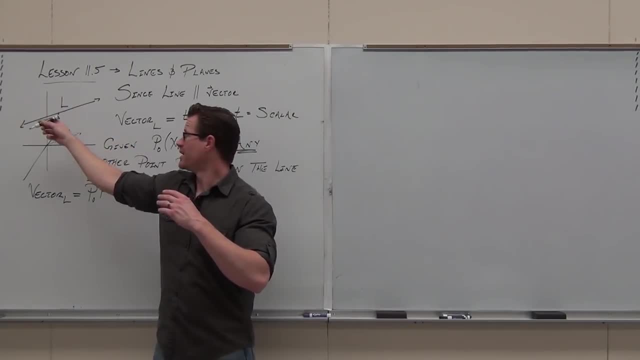 This line. hey, it's parallel to the vector. If it's parallel to the vector, any vector on that line is a scalar multiple of the direction vector. That's the idea. More than that, If I give you a point, we can always find the vector of that line between a point and any other one. 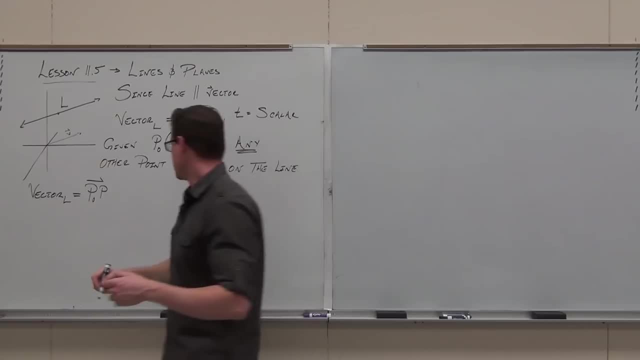 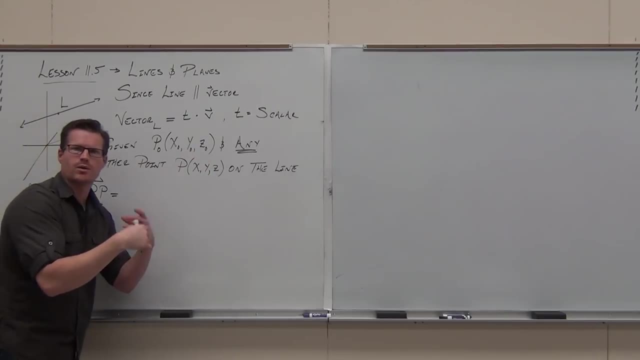 Between a point and any other one And, in fact, the way that we do that- this minus this, this minus this, this minus this- this is how we always find the vector between two points. So the vector of the line, if these two points are on that line, says: well, yeah, just subtract them. 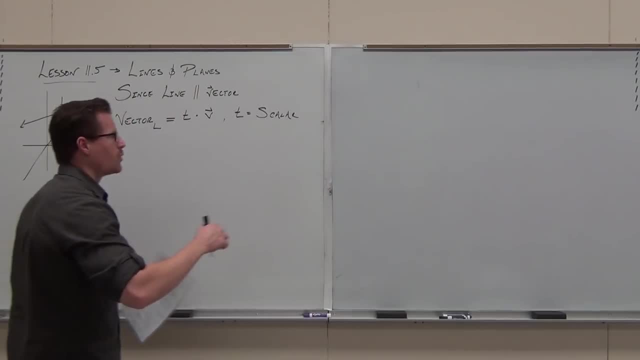 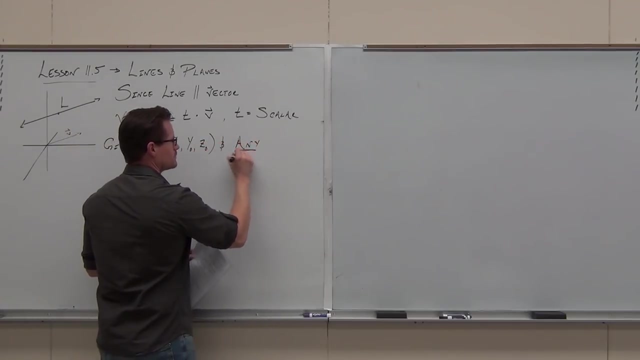 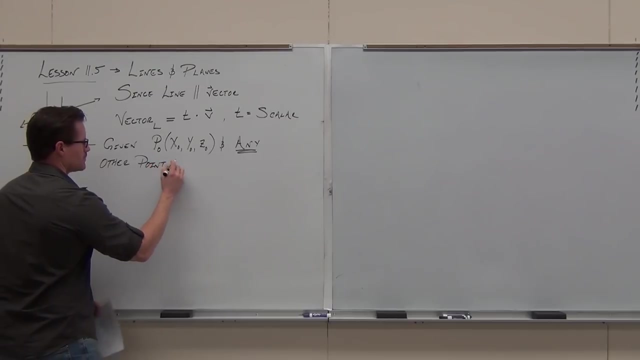 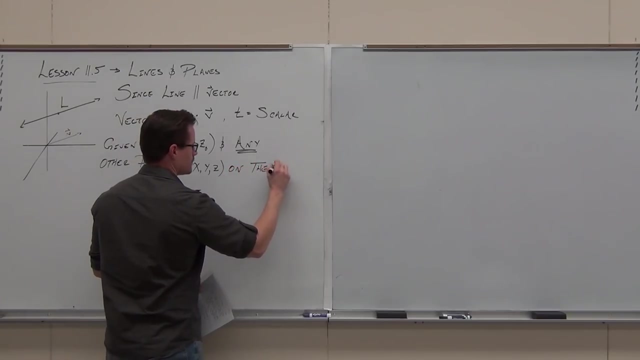 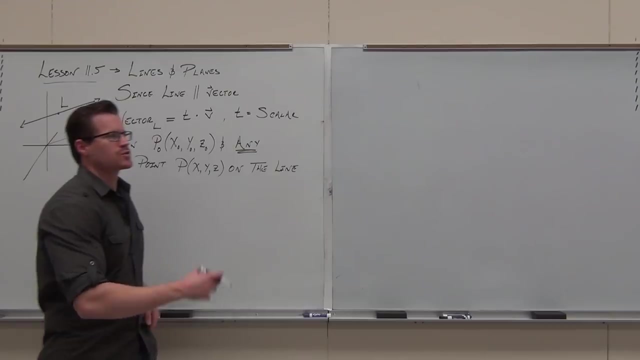 Pretty, not so bad, So let's talk about this. So, given a point, we call the actual points the piece of zero, like a specified point on a line And any other point. So if I give us a point, just a specified point, 3, 1,, 2.. 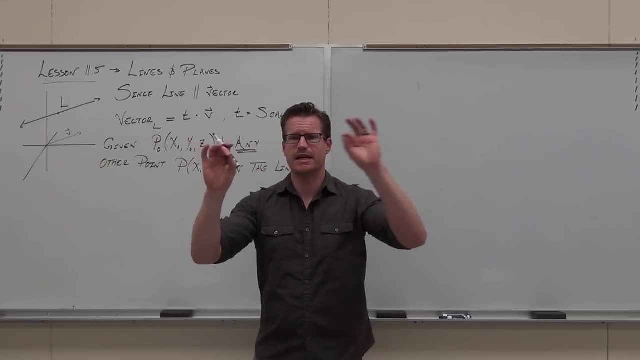 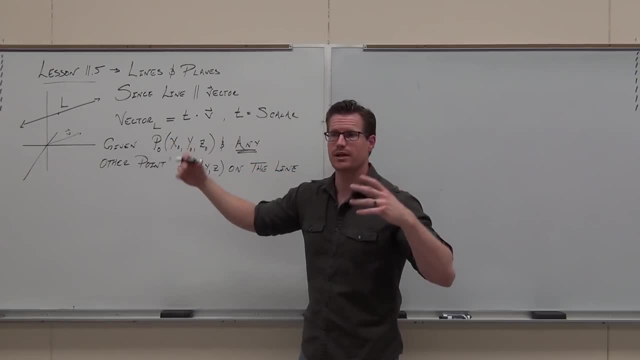 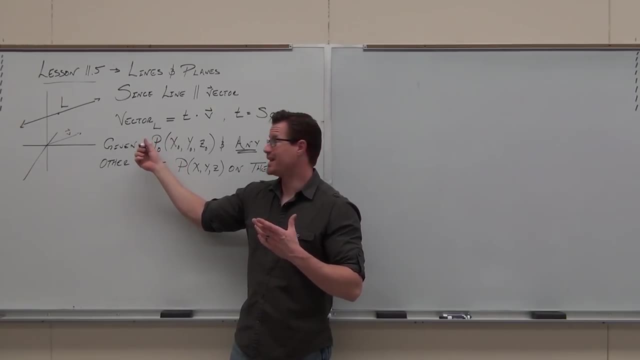 So I have a point on the line and any other point it just has to be on the line, I don't care what it is. We can always find a vector between this point and this point. We can always find that vector, And it's going to be a vector on that line because these two points are on that line. 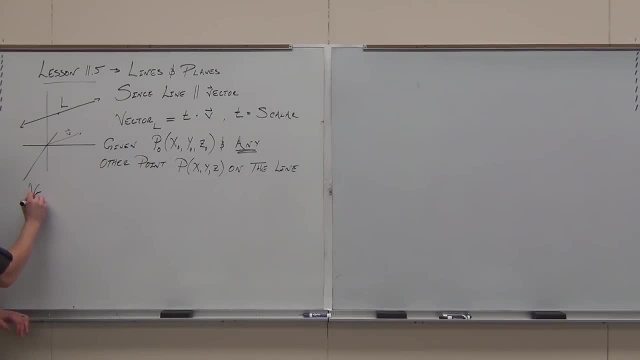 It's got to be there. So the vector of the line, that's that little L. So the vector of the line is going to be- let's call it the same. it's going to be the same as the vector between P, sub 0 and P. 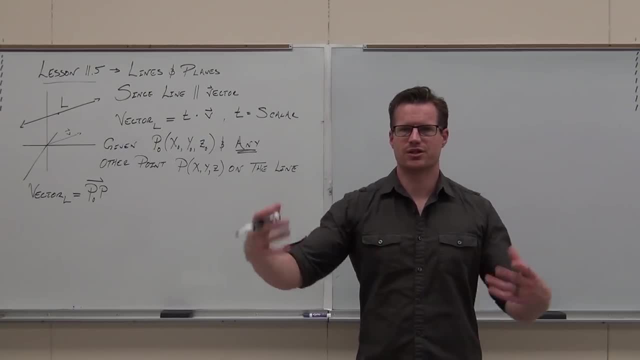 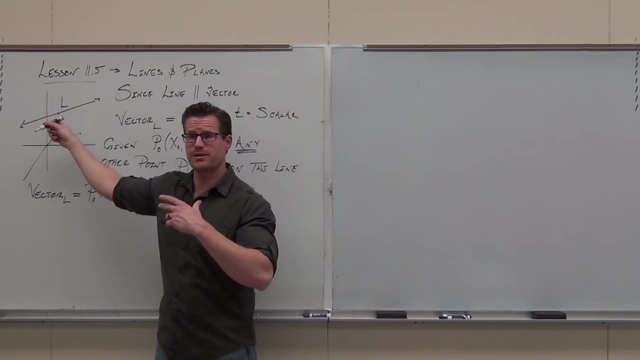 Any other point, We'll do a 20 second recap, because then it's pure algebra. You guys, we already talked about it, but you get the idea. This line, hey, it's parallel to the vector. If it's parallel to the vector, any vector on that line is a scalar multiple of the direction vector. 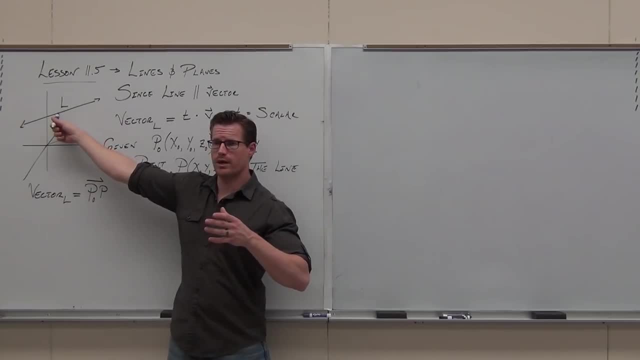 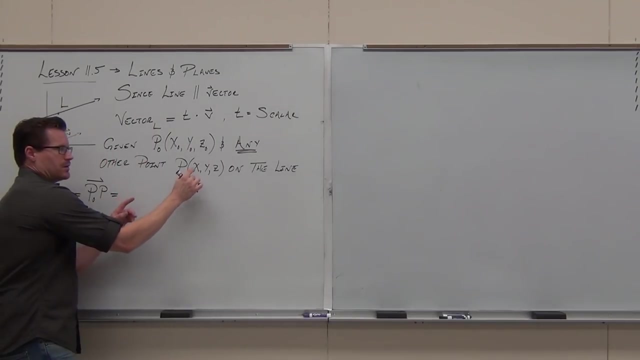 That's the idea. More than that, If I give you a point, we can always find the vector of that line between a point and any other one, Between a point and any other one. And in fact, the way that we do that, this minus this, this minus this, this minus this. 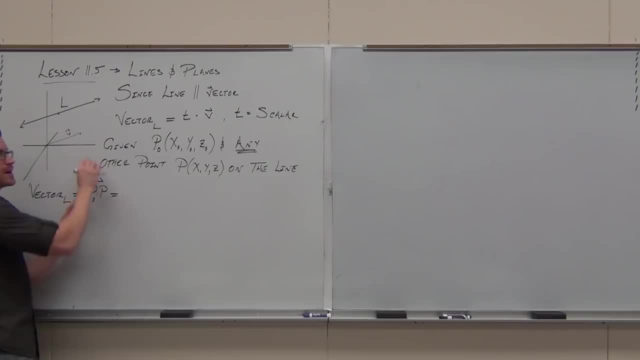 this is how we always find the vector between two points. So the vector of the line, if these two points are on that line, says: well, yeah, just subtract them, And that's what we use to represent the vector of that line. 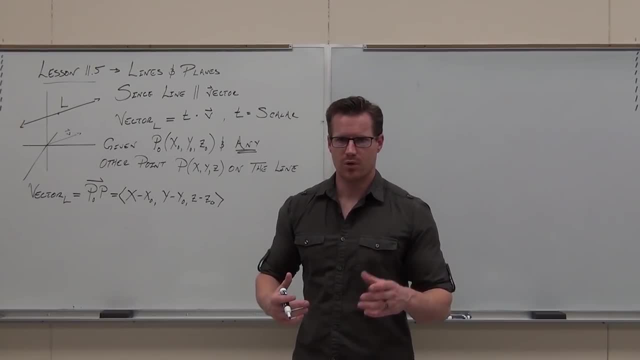 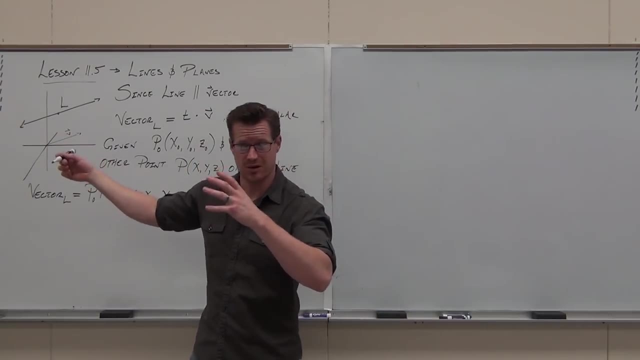 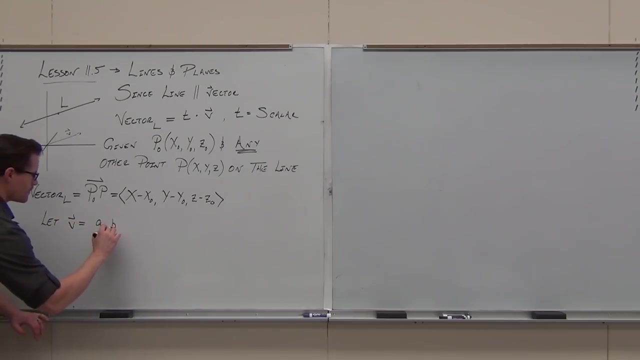 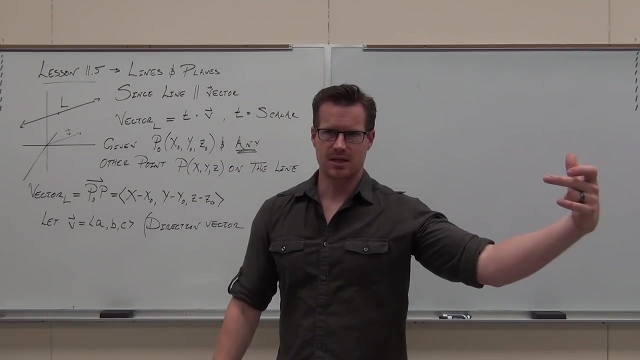 Are you sure you're okay with this? We got one more thing. We do have to identify this direction vector, so the direction of our line. These things are parallel. here We call this the direction vector and A, B and C the components of the direction vector. 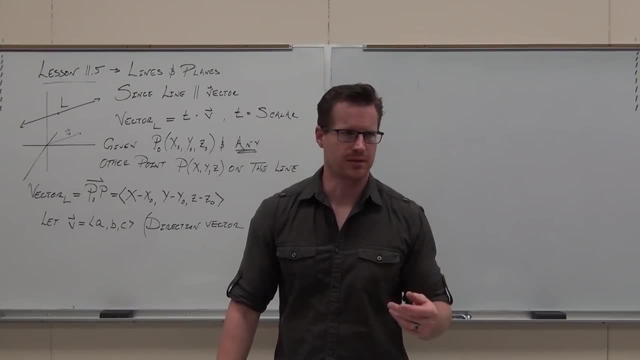 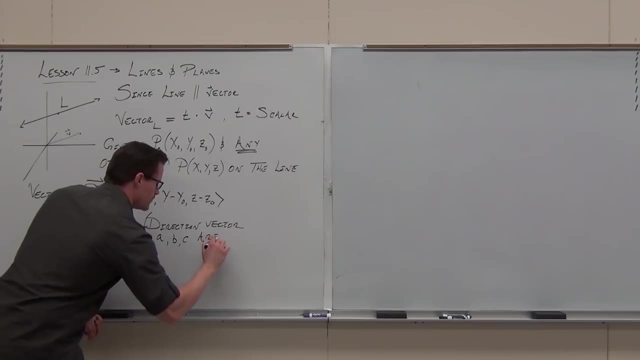 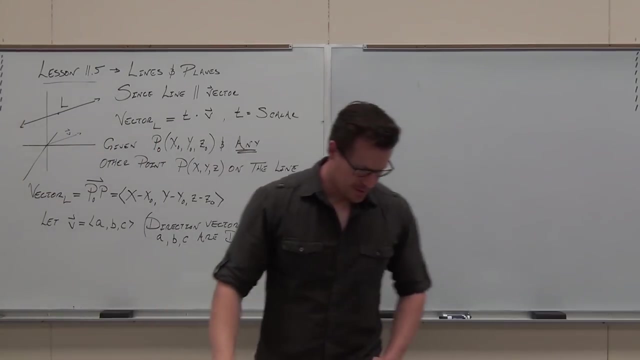 we call this direction numbers. Why? Because they give us the direction. That's why, Of the X, Y and Z, Okay, we're almost done. It doesn't even look like we're almost done, but we're almost done. 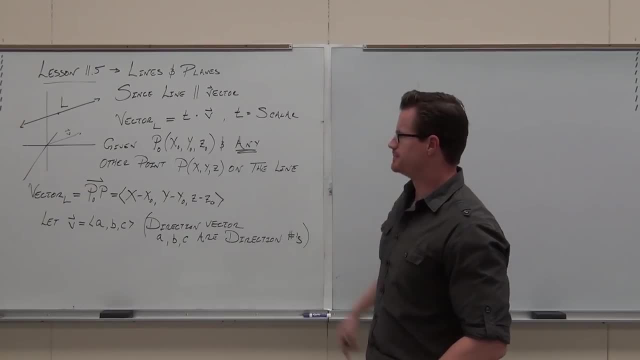 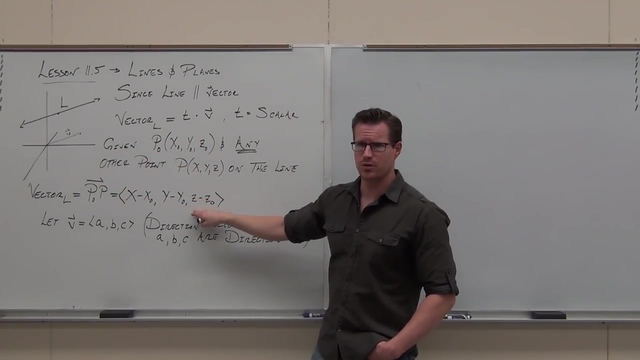 Here's the whole punchline of this. I'm going to do it over here. You guys have it written down. I've got two points on the line. I can always find the vector between them. In fact, here it is. Here's the whole point. 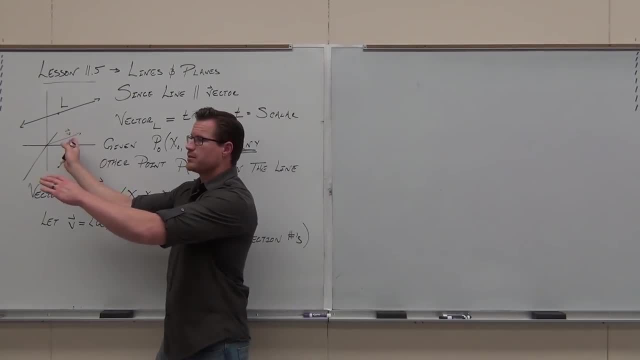 I know. I know that if this vector is in the same direction as my line, that they are parallel. If they are parallel, then they are scalar multiples. If they're scalar multiples, let's use T as the scalar. then here's what I know. 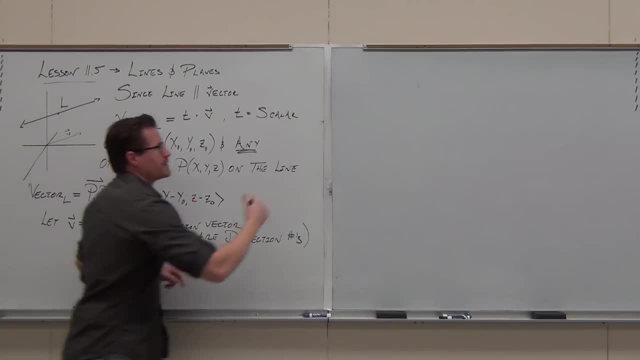 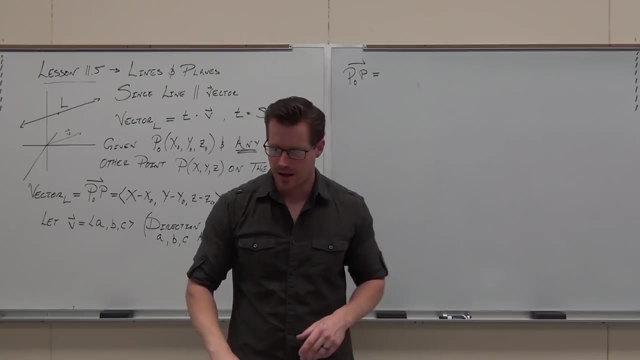 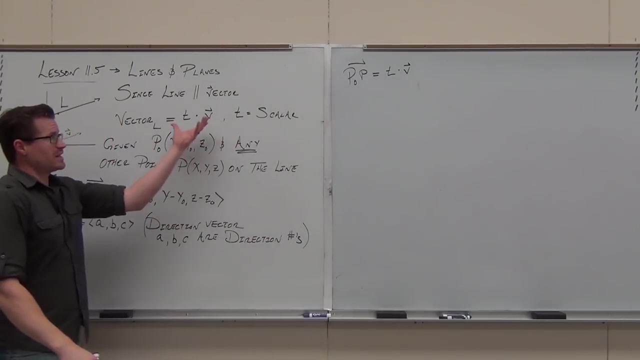 I know the direction of my line, That's, the vector of my line has to be this. We literally have it right here. Here's the vector of my line. Here's the vector of my line. I did it, man. There's two points. 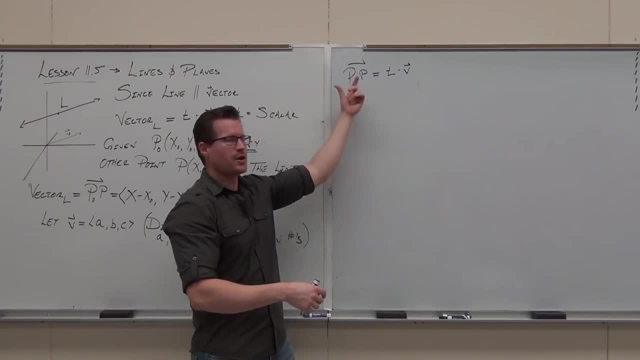 It's a vector. That's the vector of my line. I know they're parallel. Therefore, I know that the vector of my line is a scalar multiple of the direction vector. What's telling me the direction of my line? It's almost trivial. 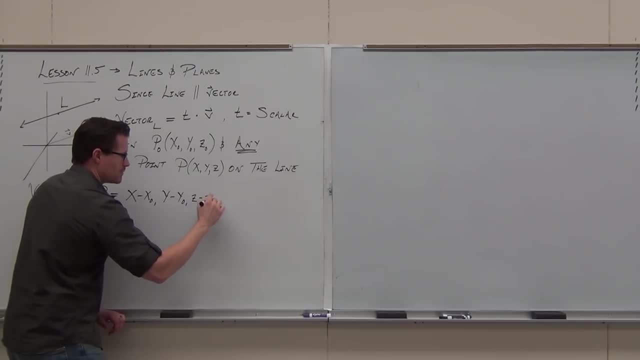 So we're going to do a 20-second recap of that line and then we're going to do a 20-second recap of that line. So we're going to do a 20-second recap of that line and then we're going to do a 20-second recap of that line. 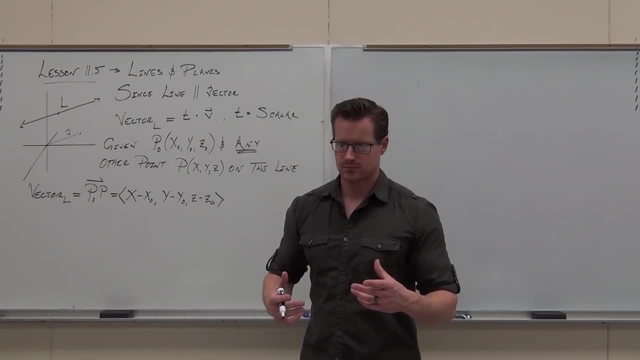 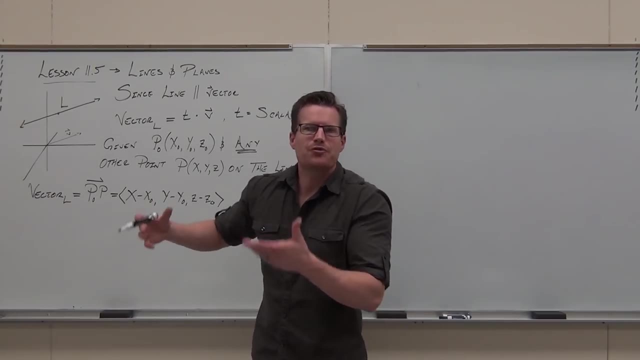 And that's what we use to represent the vector of that line. Are you sure you're okay with this? We've got one more thing. We do have to identify this direction vector, so the direction of our line. These things are parallel here. 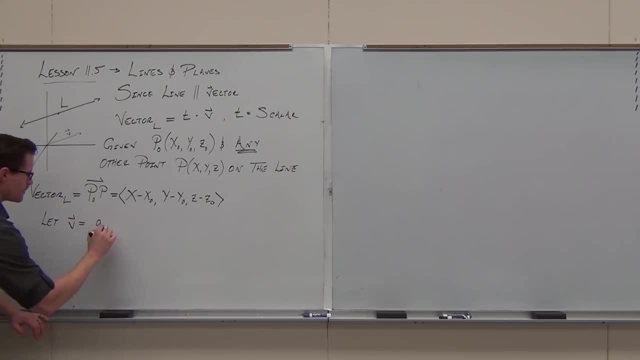 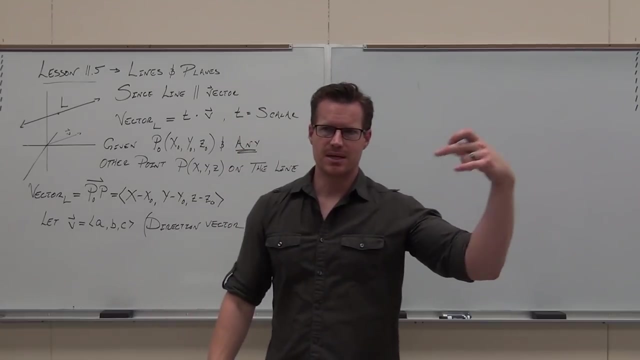 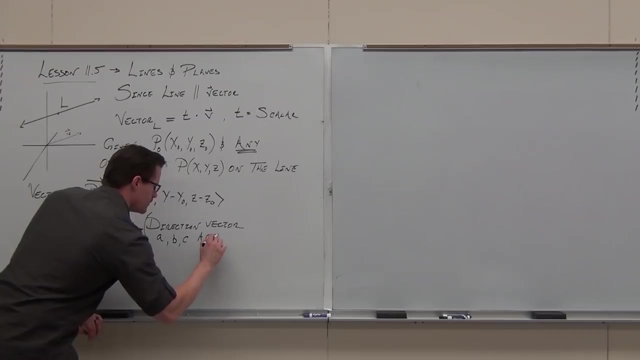 We call this the direction vector and a, b and c the components of the direction vector. we call this direction numbers. Why? Because they give us the direction. That's why Of the x, y and z. Okay, we're almost done. 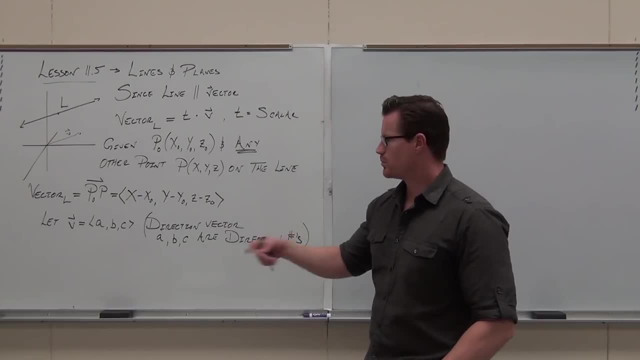 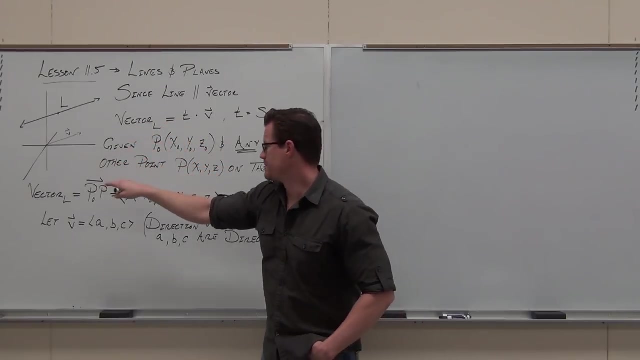 It doesn't even look like we're almost done, but we're almost done. Here's the whole punchline of this. I'm going to do it over here. You guys have it written down. I got two points on the line. I can always find the vector between them. 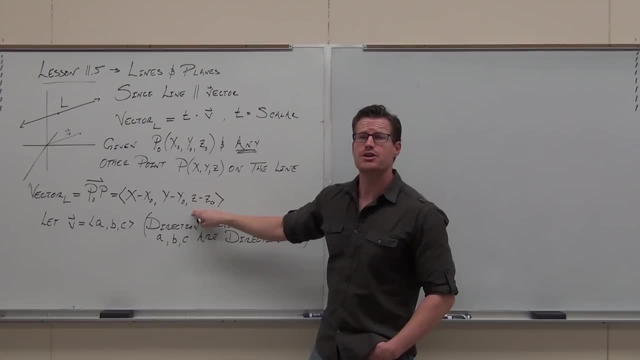 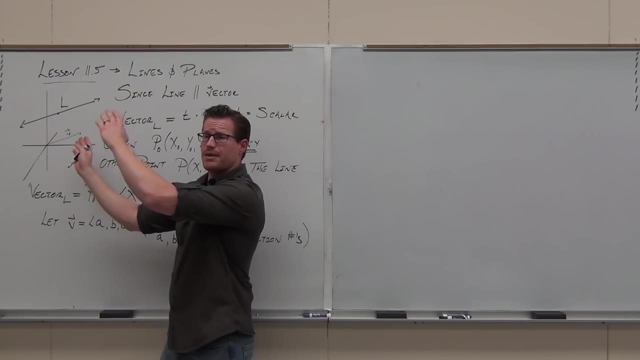 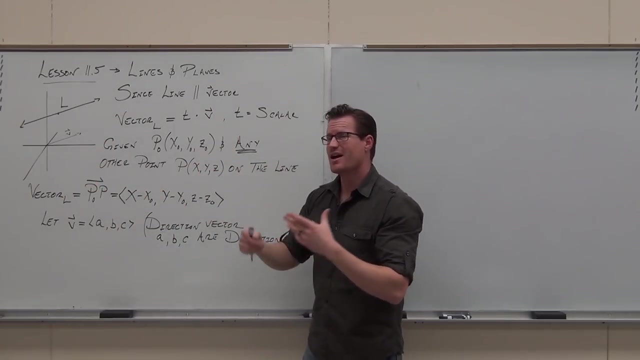 In fact, here it is. Here's the whole point. I know, I know that if this vector is in the same direction as my line, that they are parallel. If they are parallel, then they are scalar multiples. If they're scalar multiples, let's use t as the scalar. then here's what I know. 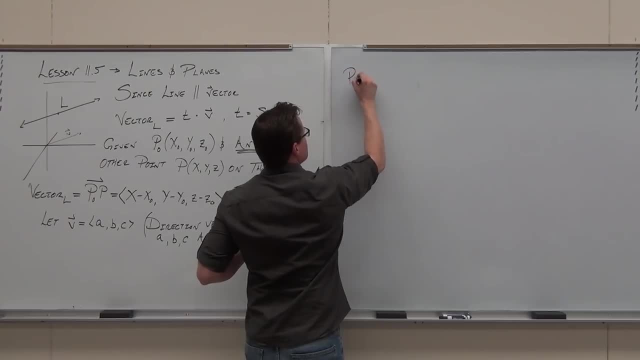 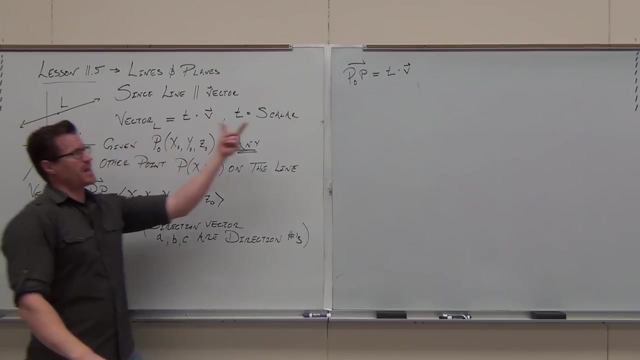 The direction of my line, That's the. the vector of my line has to be this: We. we literally have it right here. Here's the vector of my line. Here's the vector of my line. I did it, man. 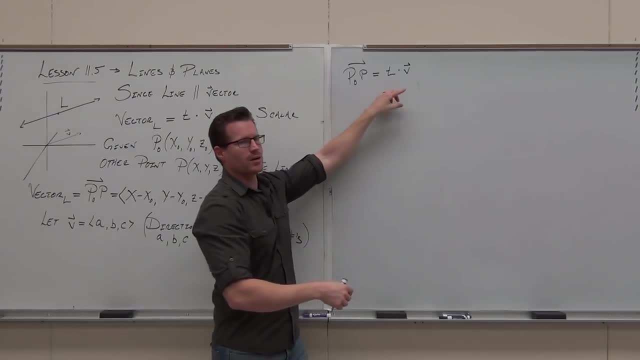 There's. there's two points. It's a fraction. That's the vector of my line. I know they're parallel. Therefore, I know that the direct, the vector of my line, is a scalar multiple of the direction vector. What's telling me the direction of my line? 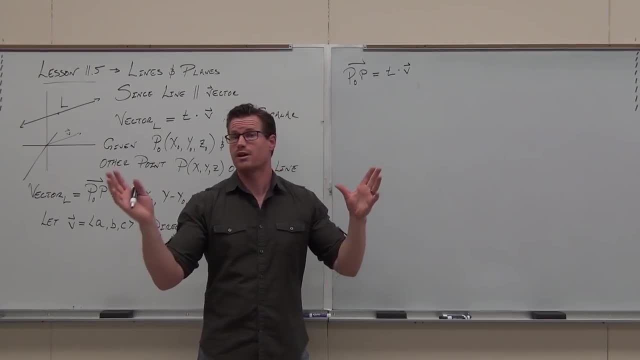 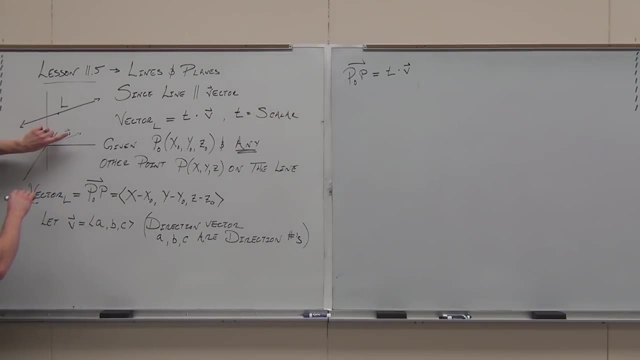 It's almost trivial. It's like, yeah, they're parallel. There's, you're going to just multiply by whatever number it takes to get you from this one. multiply by a, a multiply by a scalar, It's just going to move your vector somewhere. 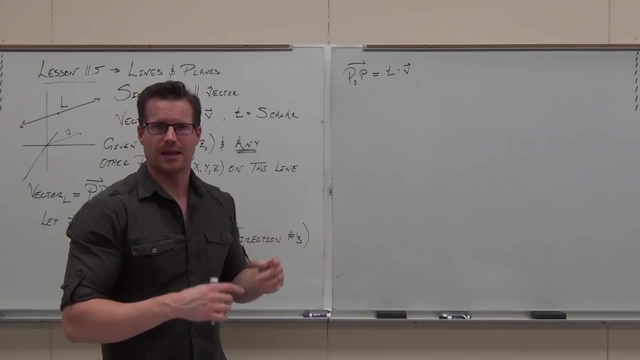 It's not going to alter the direction. It's going to move it so that it matches up with that line. That's, that's what this says. That's all it says. So, if anything, you'll be okay with what it says. 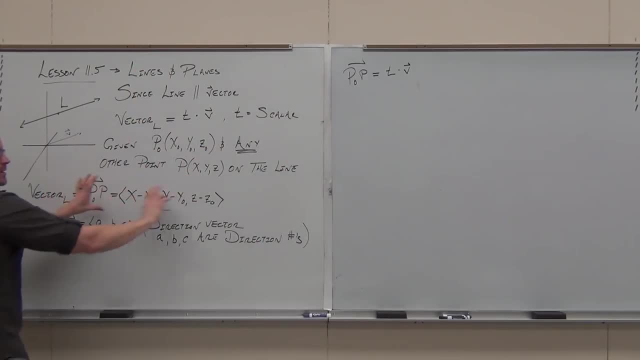 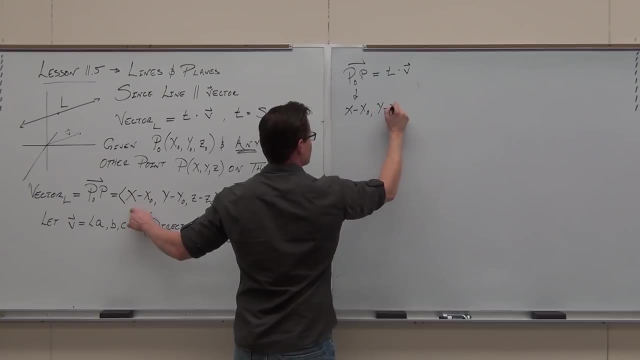 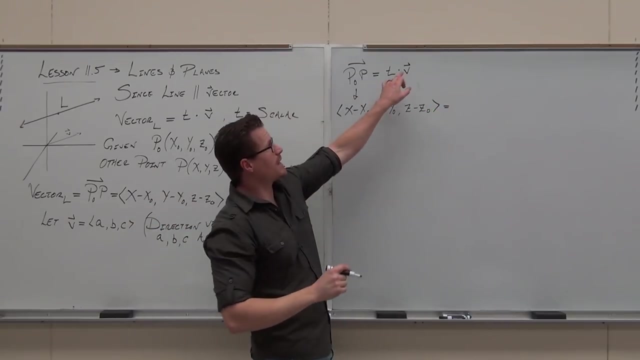 And now comes algebra. Since we found that vector And since we gave this one some letters, what are the letters for that vector? What are those? A, B, C? Yeah, those are my direction numbers, because that's my direction vector. 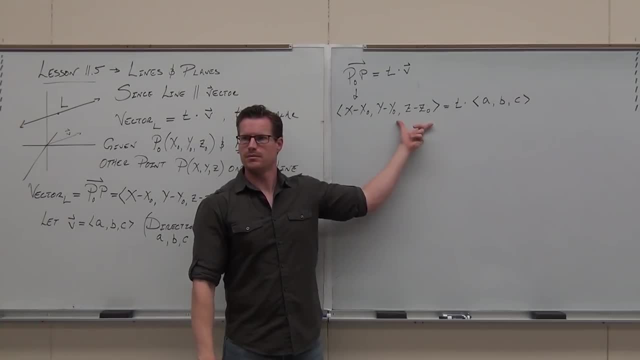 See if you can make the jump. Do you guys see where these things are coming from? Hello, yes, no, Yes. What vector is this? The two-point vector? Any vector on The line? The line What? what? what's this? 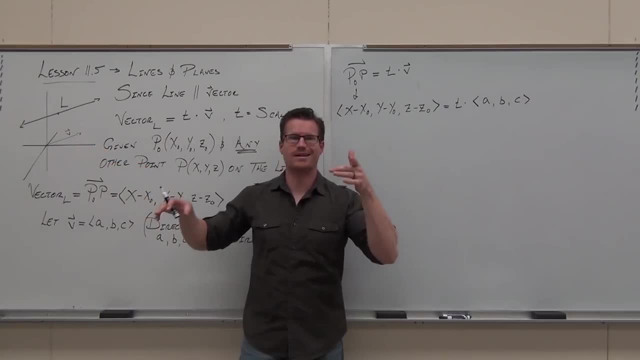 The direction. Good, That's this one saying: hey, I'm headed in this direction. It's just a position vector which is nice to deal with, But you know what This vector has to be: a scalar multiple of this vector. 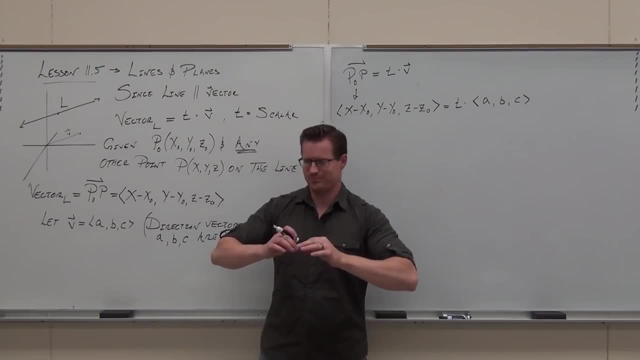 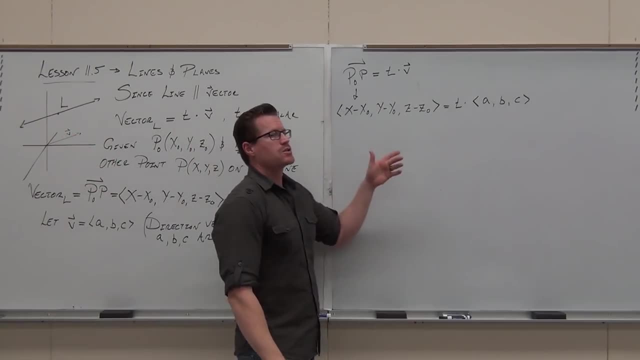 because they're in the same direction. That means that they are parallel. I'm just kind of moving it somewhere so it matches up through some point. That's, that's essentially what I'm doing. Let's do a couple things here. Let's distribute a scalar, because I can. 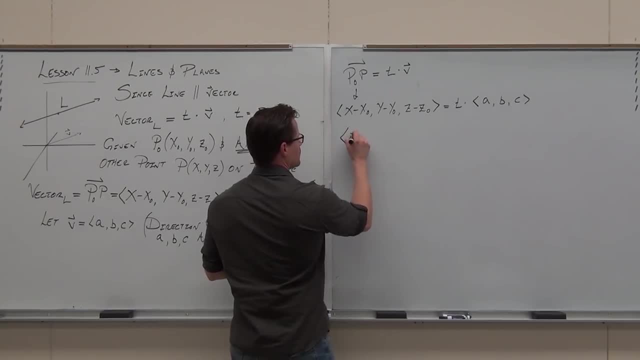 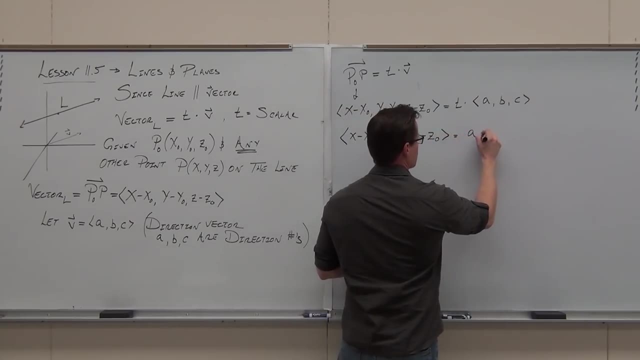 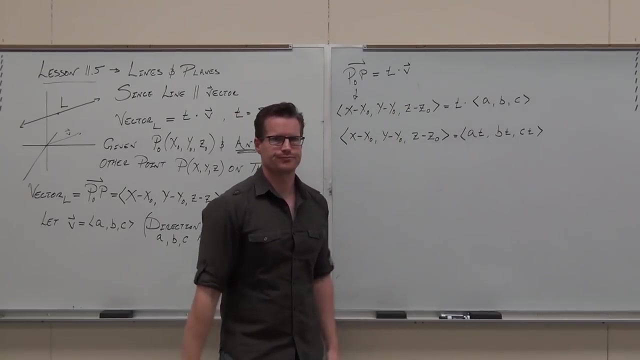 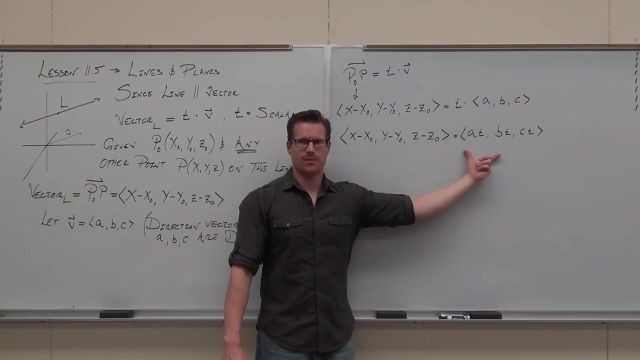 It's not a dot product, It's just a number. So he's sitting on the first point here, right? Let's go back and see It's: You've got a vector equal to a vector. If vectors are equal, their components must be equal. 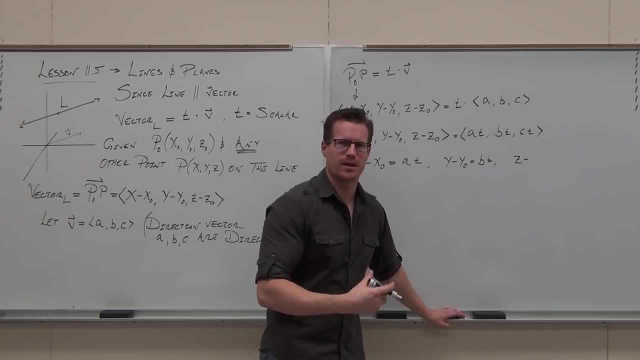 I hope you're not getting bored. It's not hard, but it's important to see where it comes from. I don't want to just give it to you, because otherwise I'm going to give you the formula to go. what are these pieces? 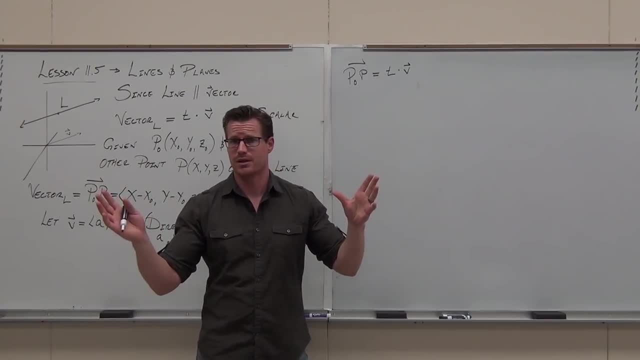 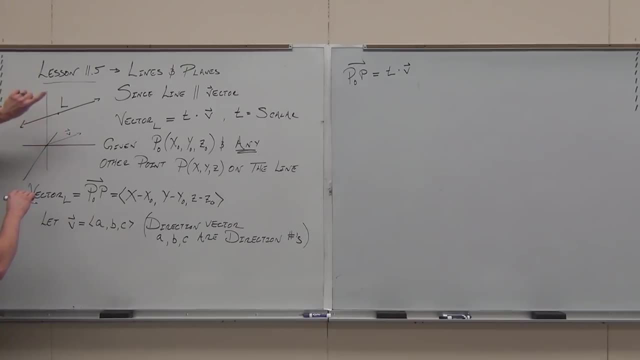 It's like, yeah, they're parallel. You're going to just multiply by whatever number it takes to get you from this one. multiply by a scalar. It's just going to move your vector somewhere, It's not going to alter the direction. 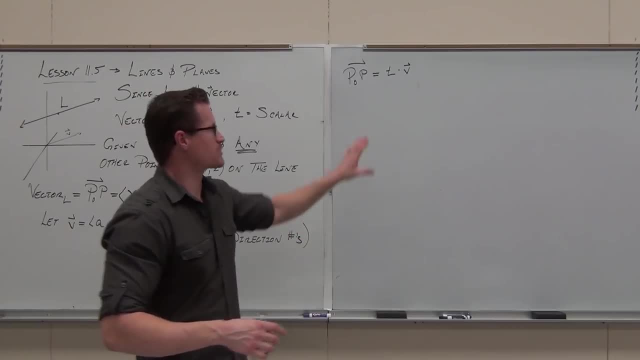 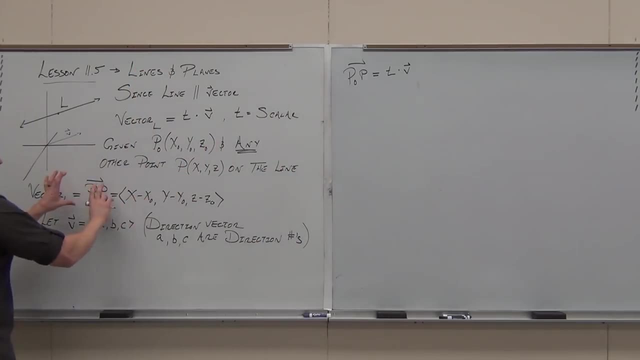 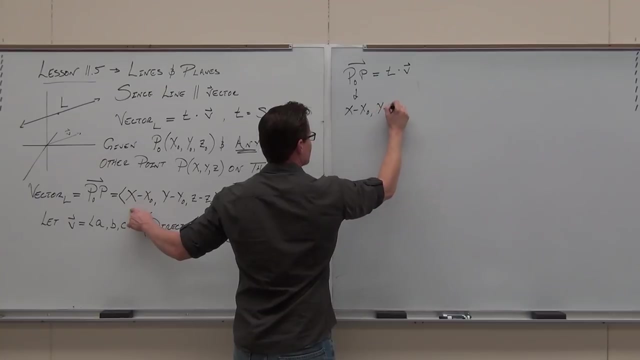 It's going to move it so that it matches up with that line. That's what this says, That's all it says. So if this feels okay with what it says, And now comes algebra: Since we found that vector And since we gave this one some letters, what are the letters for that vector? 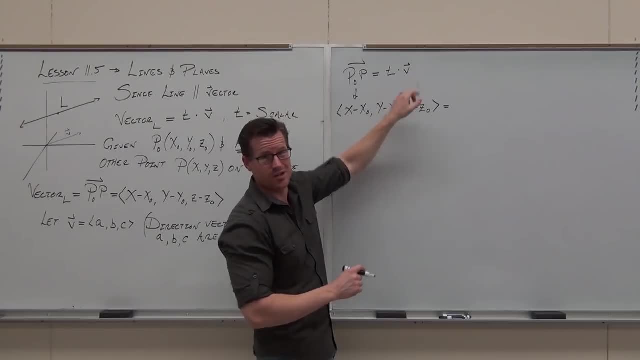 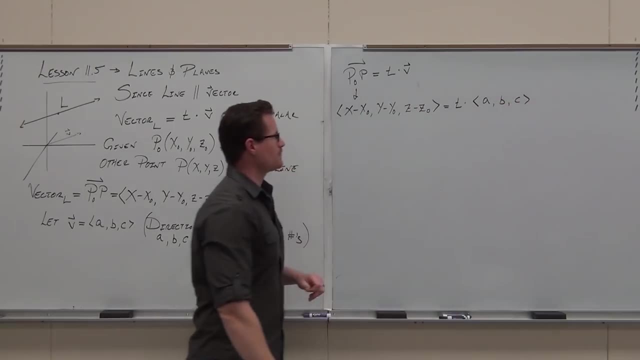 What are those? A, B, C? Yeah, those are my direction numbers, because that's my direction vector. See if you can make the jump. Do you guys see where these things are coming from? Hello, yes, no, Yes. 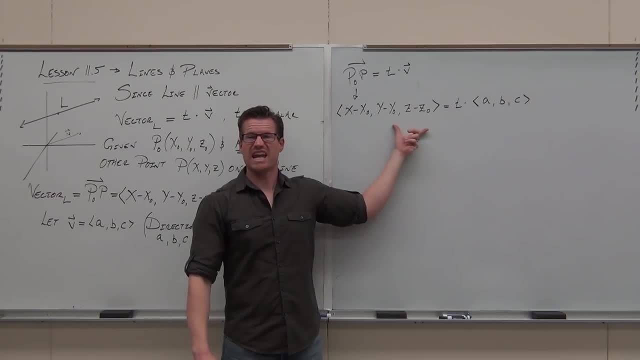 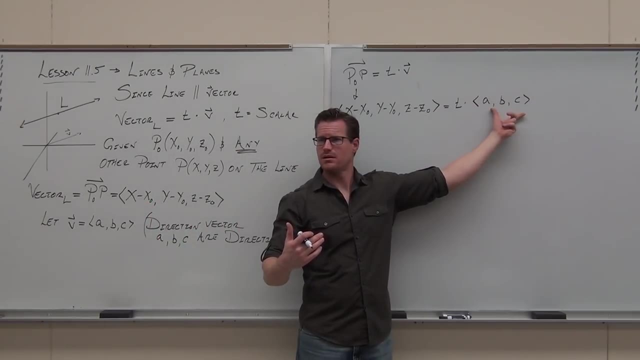 What vector is this? 22. Any vector on the line. What? what's this? Good? That's this one saying, hey, I'm headed in this direction. It's just a position vector which is nice to deal with. 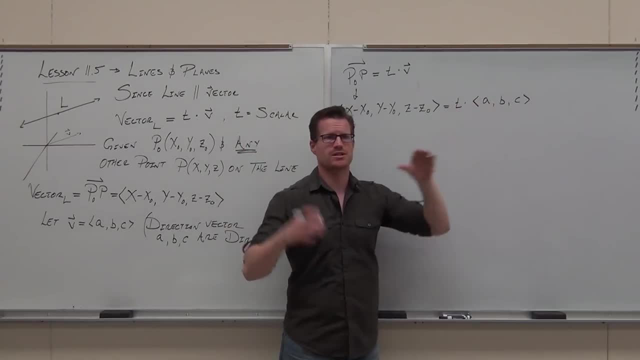 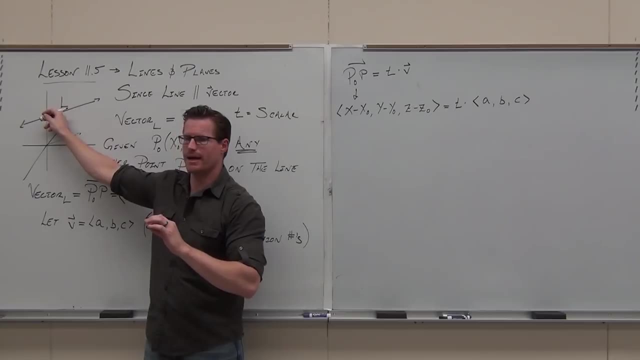 But you know what? This vector has to be a scalar multiple of this vector, because they're in the same direction. That means that they are parallel. I'm just kind of moving it somewhere so it matches up through some point. That's. that's essentially what I'm doing. 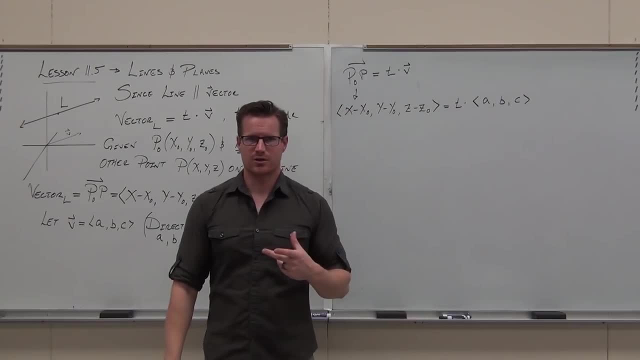 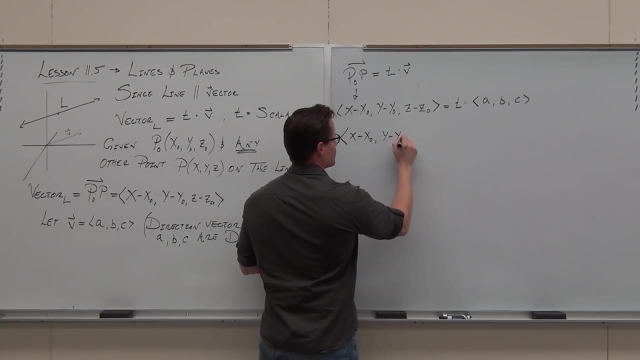 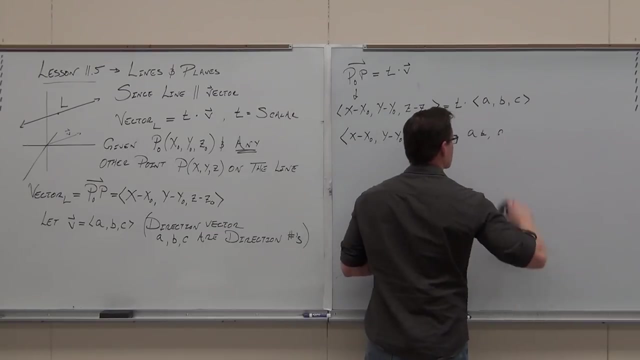 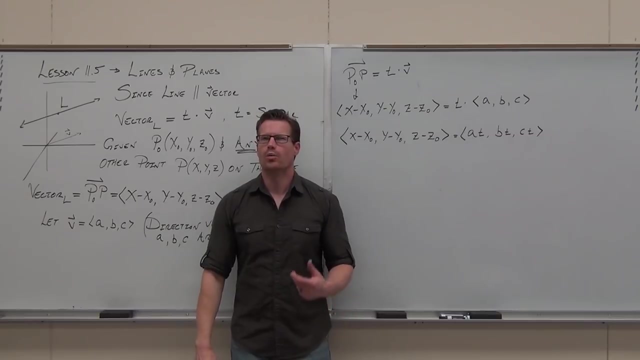 Let's do a couple things here. Let's distribute a scalar, because I can. It's not a dot product, It's just a number. Let's try it. Awesome, What do you have Here? Once again, I'm going to pray. 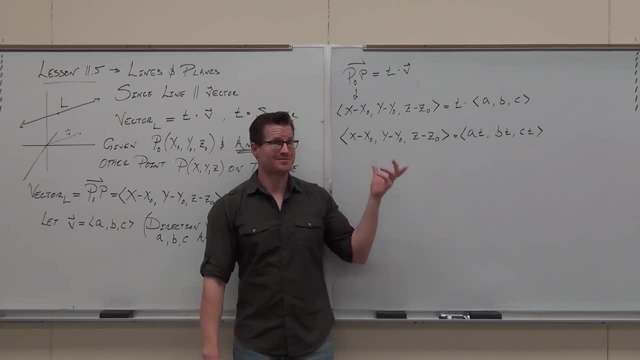 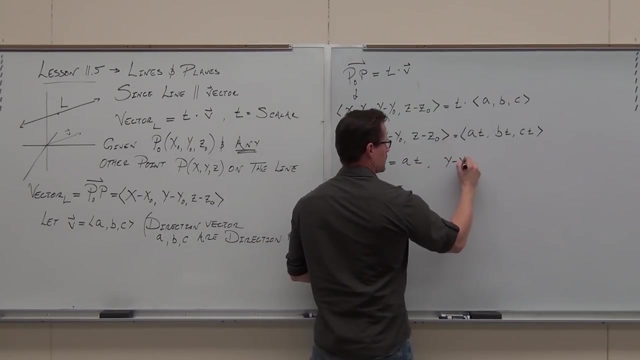 Again, You've got a vector equal to a vector. If vectors are equal, their components must be equal. I hope you're not getting bored. It's not hard, but it's important to see where it comes from. I don't want to just give it to you because otherwise 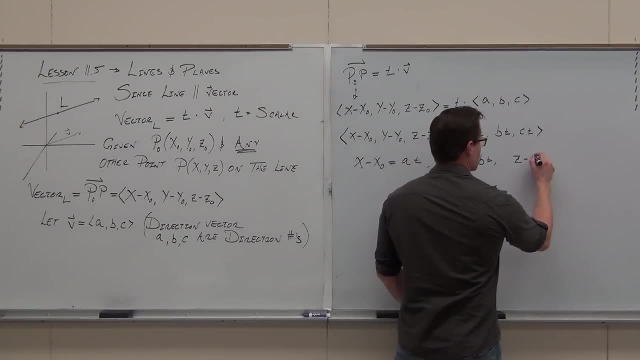 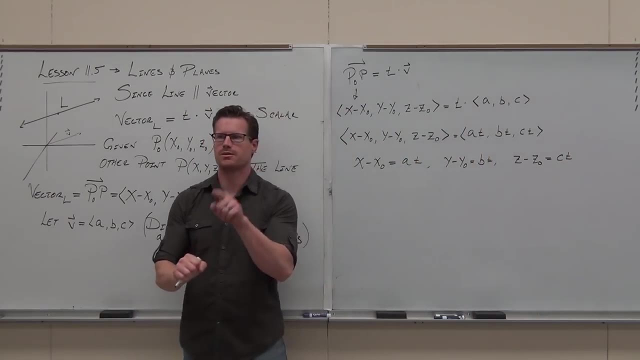 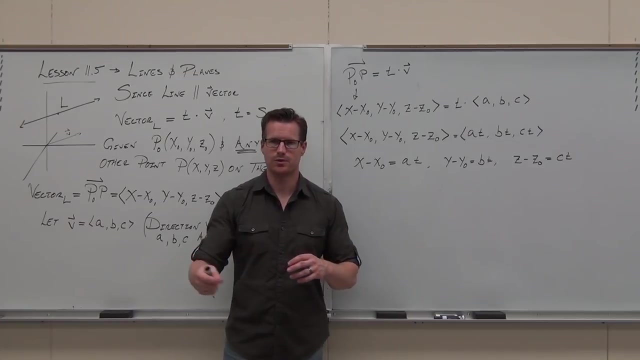 I'm going to give you the formula to go. what are these pieces? That's silly, You guys. okay with that one. Now, the way that equations of lines and such usually work is we like to solve for variables. Is that a variable? 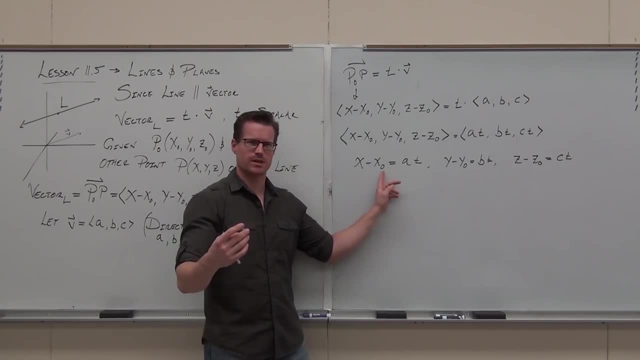 No, No, What is it? Come on, put it. what is that? What is that The x-coordinate of that specific point that I have to give you? Does that make sense, Or do you have to be able to find it? 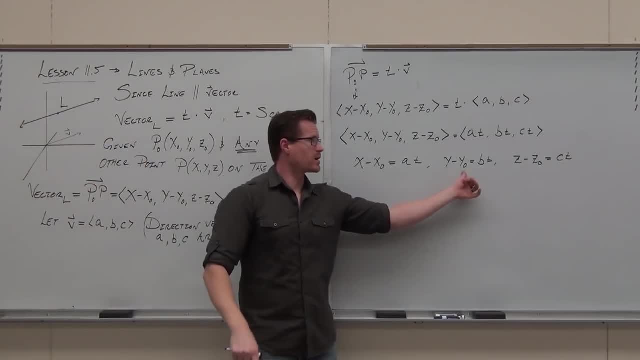 It's the. it's on a. it's a point. It's the x-coordinate point. That's the y-coordinate, That's the z-coordinate. What is the a and the b and the c? Where is that coming from? Unit vector. 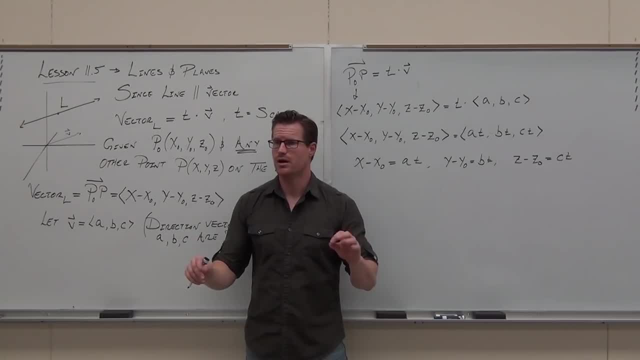 The not necessarily unit vector. In fact, I don't want you to think of unit vector. The direction vector does not have to be a unit vector. These are those variables. Let's solve for them. Let's solve for the variables. 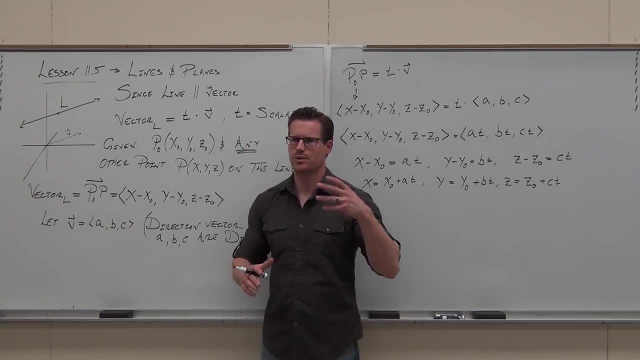 Take. take about 10 seconds and let's see if we can absorb this. okay, What I want to do, what I want you to do in your head, is work your way through this, Think about: Okay, I have a line and it's the same direction. 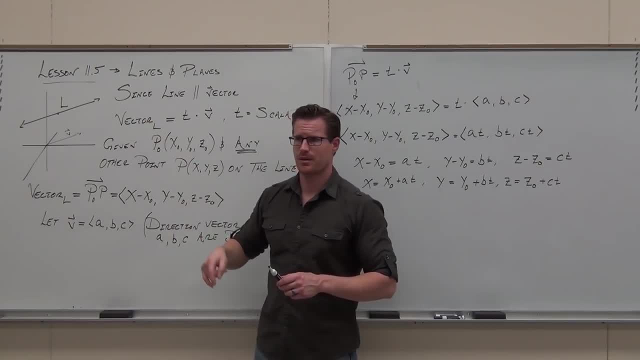 as some other position vector, no problem, That means they're parallel. Parallel means scalar multiples. Any vector between two points, easy to do, just subtract them, We got. we got a vector, If this vector is in the same direction as this vector. 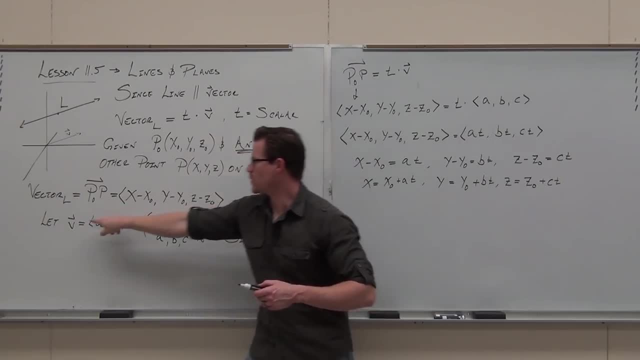 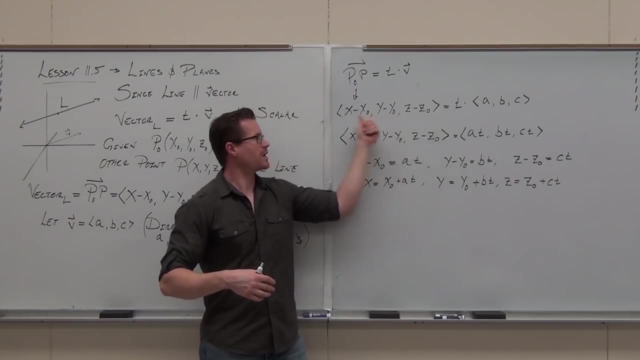 then this equals a scalar multiple of this. That's, that's this. Let's drop it down. Here's the vector we found between two points, one specific and one. just so you know, It's somewhere else on the line. This one was given to you as ABC. 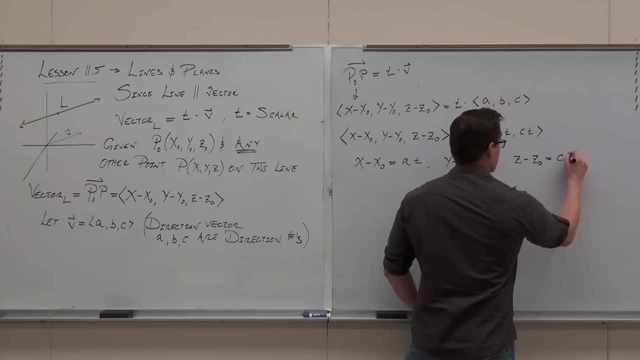 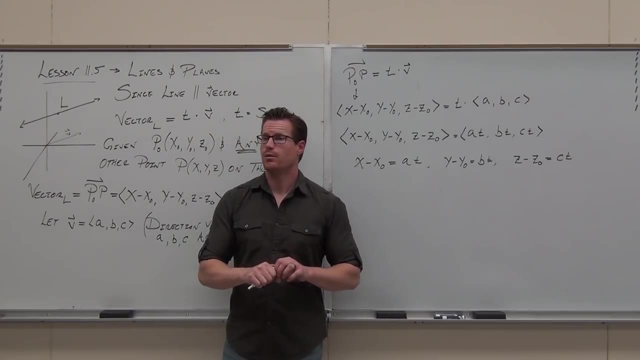 That's silly, You guys. okay with that one. Now, the way that equations of lines and such usually work, is we like to solve for variables. Is that a variable? No, No, What is it? Come on, put it. what is that? 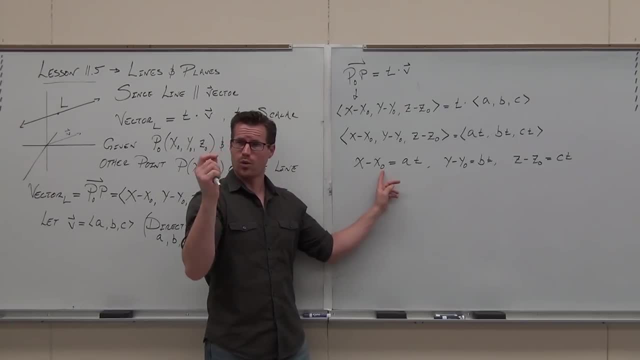 What is that? The x-coordinate of that specific point that I have to give you? Does that make sense Or do you have to be able to find it? It's on a, it's a point. It's the x-coordinate point. 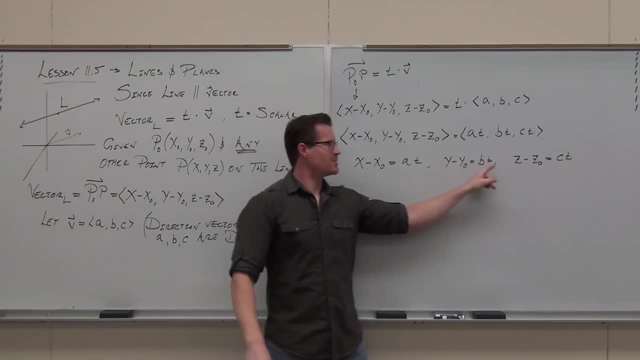 That's the y-coordinate, That's the z-coordinate. What is the a and the b and the c? Where is that coming from? Unit vector- The not necessarily unit vector, In fact, I don't want you to think of unit vector. 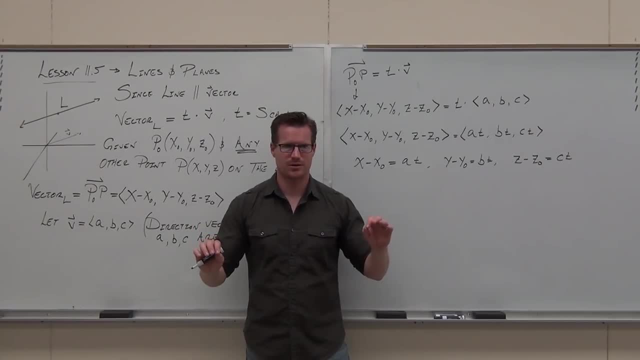 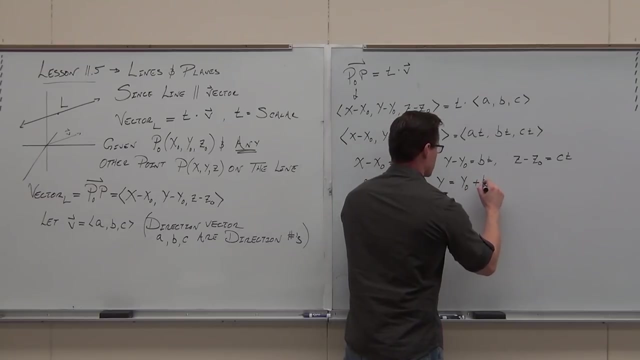 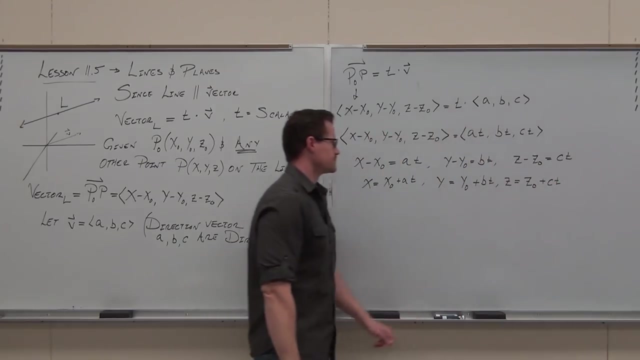 The direction vector does not have to be a unit vector. These are those variables. Let's solve for them. Let's solve for the variables. Take, take about 10 seconds and let's see if we can absorb this. OK, What I want to do, what I want you to do, 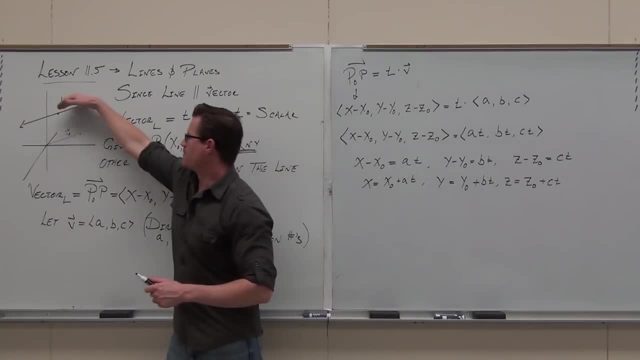 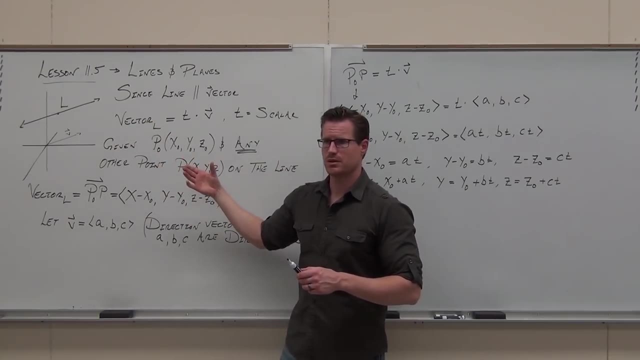 in your head is: work your way through this. Think about: Okay, I have a line and it's the same direction as some other position vector, no problem, That means they're parallel. Parallel means scalar, multiples, Any vector between two points. easy to do. 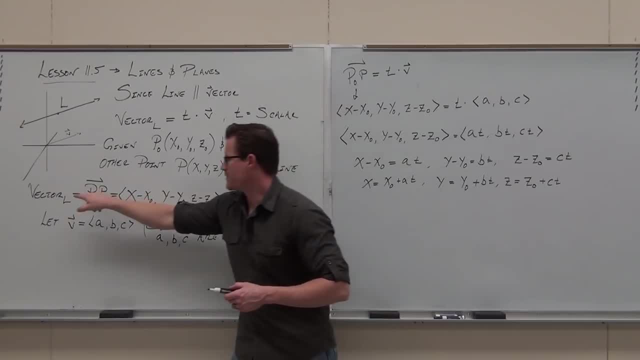 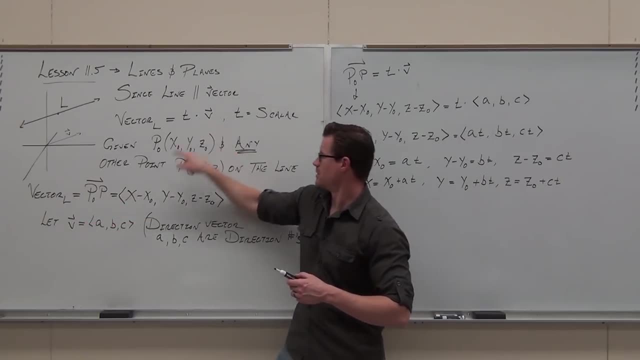 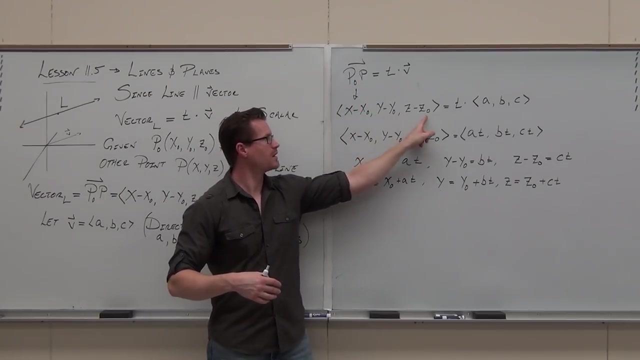 just subtract and we got a vector. If this vector is in the same direction as this vector, then this equals a scalar multiple of this. That's this. Let's drop it down. Here's the vector we found between two points, one specific and one just somewhere else on the line. 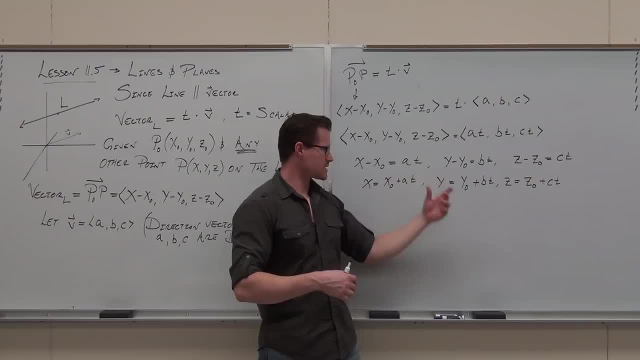 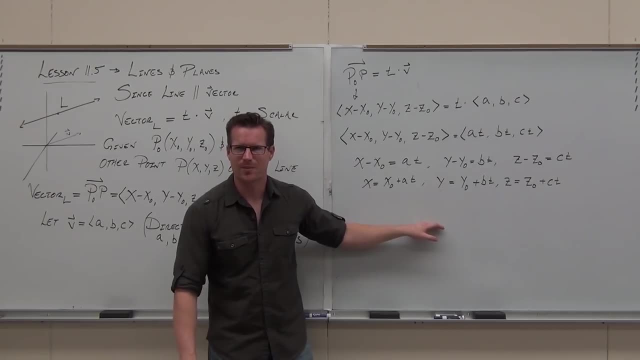 This one was given to you as ABC Distribute. do all this stuff? work it down. This is the equation of a line in three dimensions. Why does it look weird? You know why we use the T. Do you remember calculus two? 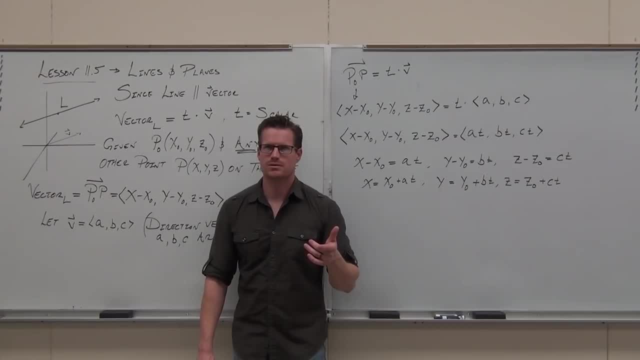 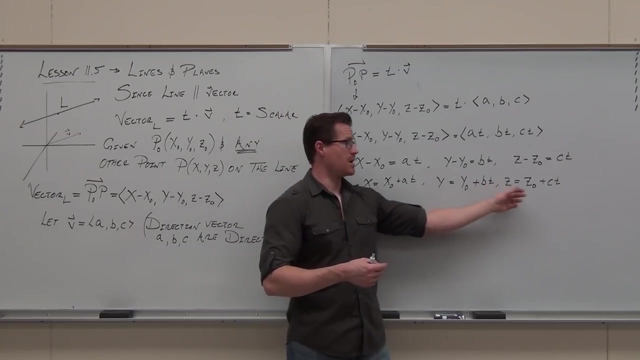 Remember section 10.3? When you did parametric equations? Yeah, In 3D lines are parametric equations. They have to be because we have to tell it: okay, at a certain time, same time, same T. 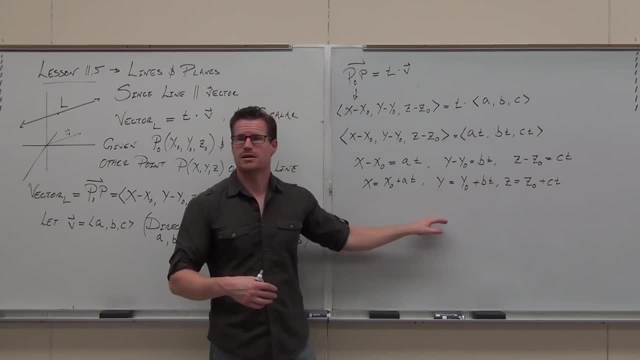 Distribute. you know, do all this stuff. work it down. This is the equation of a line in three dimensions. Why does it look weird? You know why we use the T. Do you remember Calculus 2?? Remember section 10.3.2, when you did parametric equations? 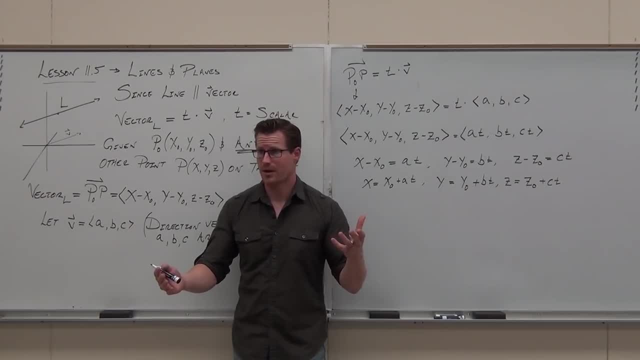 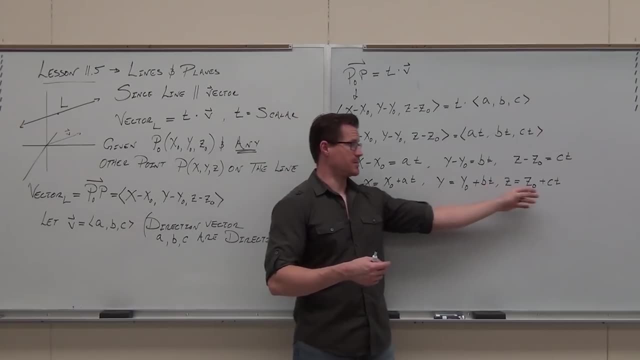 Yeah, In 3D lines are parametric equations. They have to be, because we we have to tell it. okay, at a certain time, same time, same T, you're taking a vector ABC and you're pushing it up until it goes through. 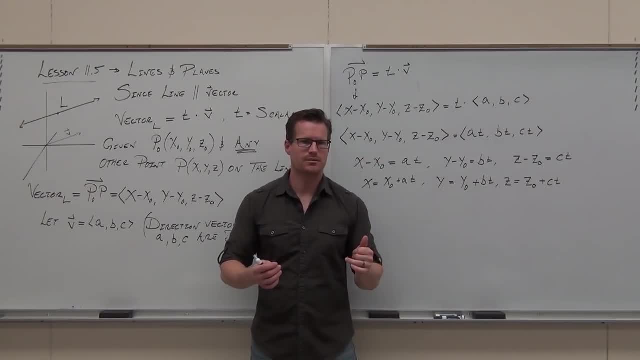 or down until it goes through that point. That is what is happening, That's. that's the idea. You're multiplying by a number to push the vector up until it goes through the point. It's kind of cool, right? And you have to do that with parametric. 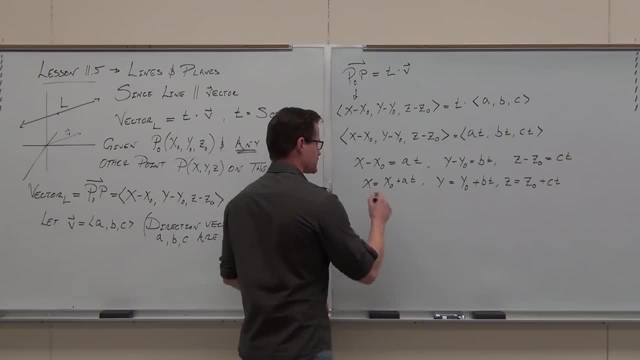 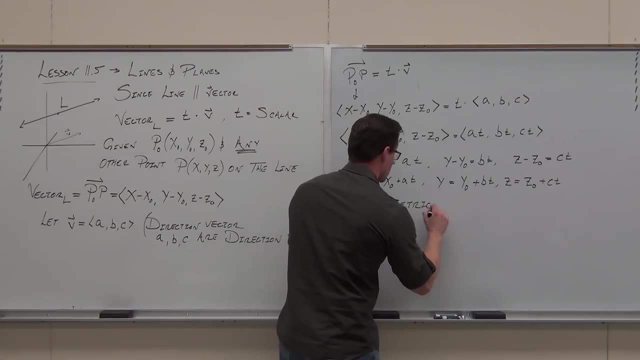 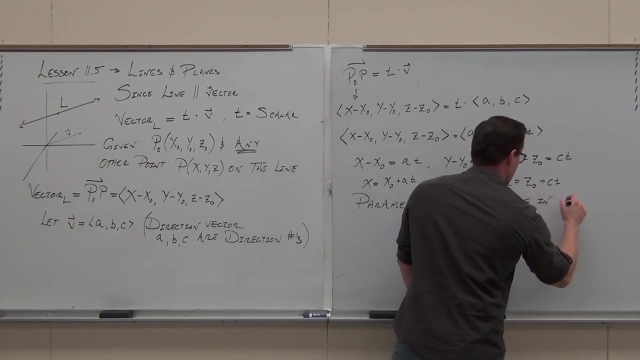 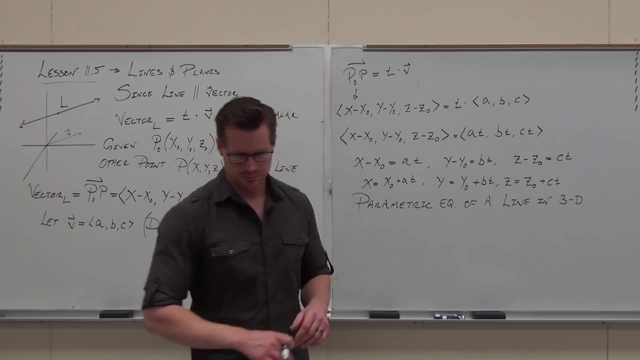 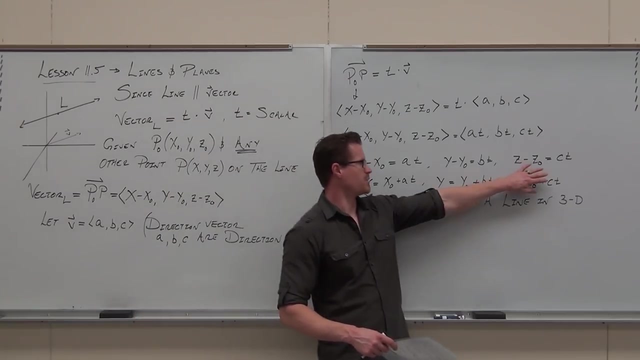 So this right here. this is the parametric equation for a line In 3 space R3, 3D. By the way, if you cover that up, you might have seen that in 2D in parametric. 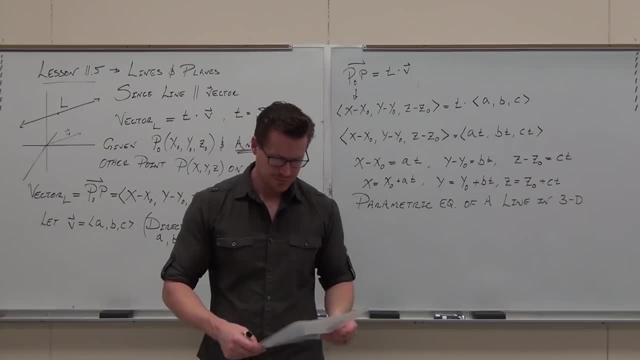 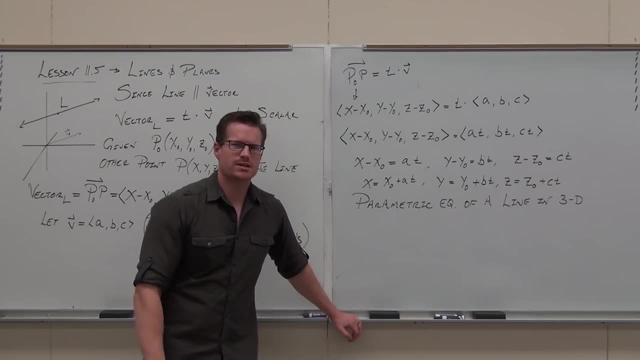 Okay, I've seen this, this stuff before. How about this one, though? How about this? Firstly, what? what is T going from what? what's the interval of T? What is it If you have a line? how far do lines go? 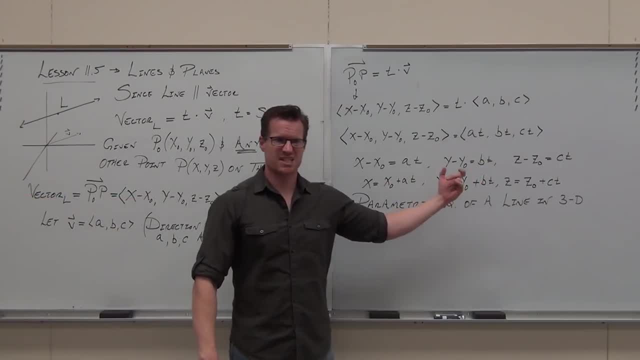 Forever, Forever. So this parameter, this T, goes typically from negative infinity to positive infinity. unless you have problems with your T, like domain issues or something or you, you stop it, You say I'm just talking about this, this interval. 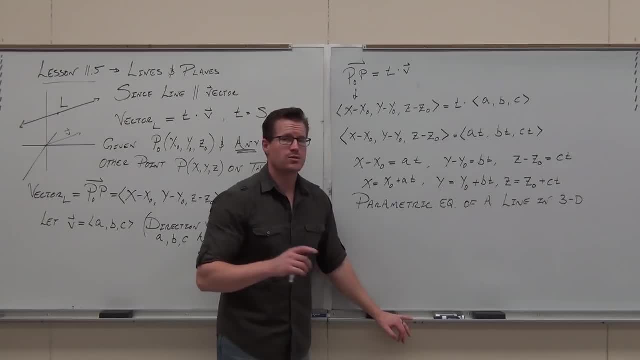 This T goes forever. Now here's my next question. Can you take, since it's the same T, can you solve each of these for T? Yes, Let's try that. I'm going to do it real quick, real quick, like so. T equals X minus X0 over 8.. 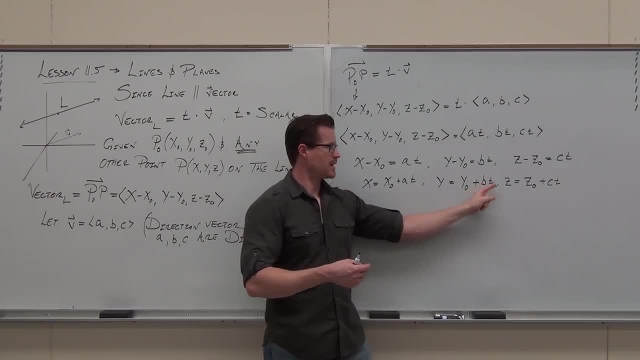 you're taking a vector ABC and you're pushing it up until it goes through or down until it goes through that point. That is what is happening. That's the idea. You're multiplying by a number to push the vector up. 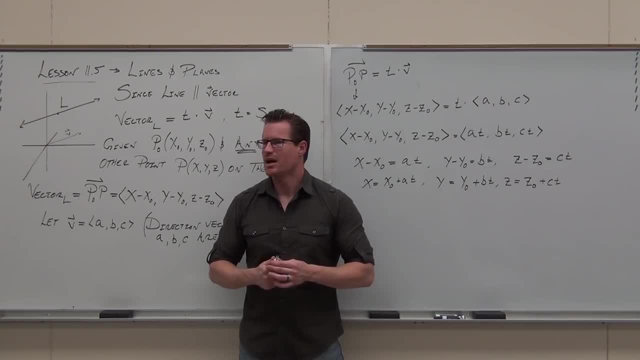 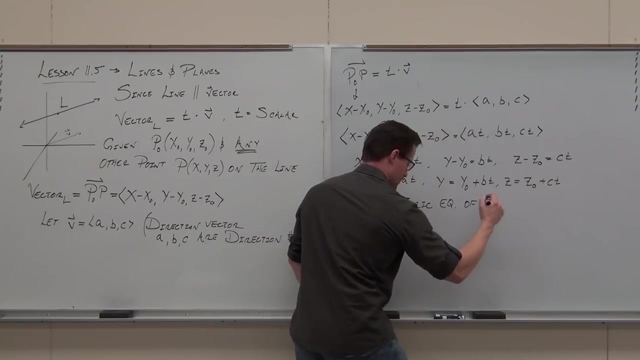 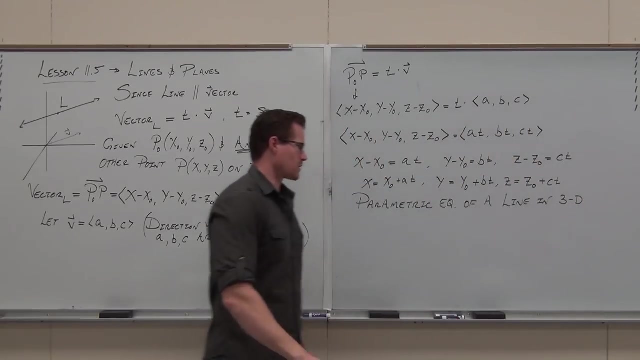 until it goes through the point. It's kind of cool, right, And you have to do that with parametric. So this right here. this is the parametric equation. This is a parametric equation for a line In three space: R3, 3D. 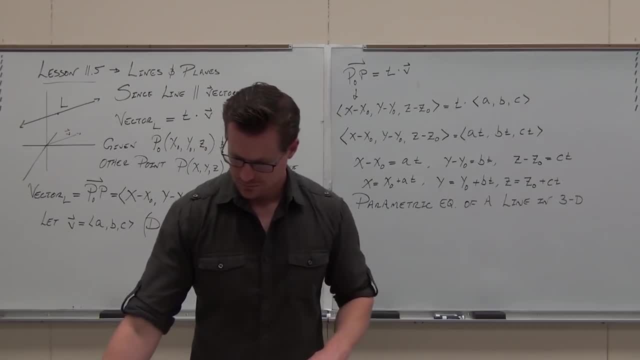 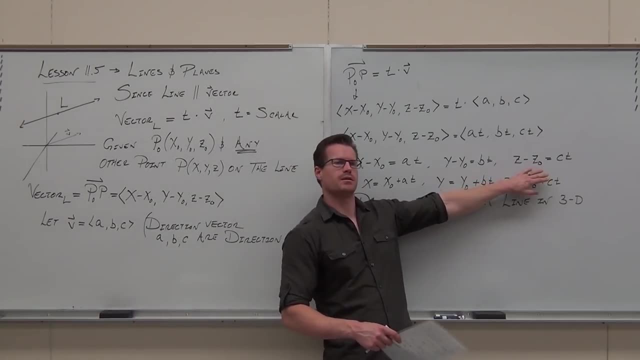 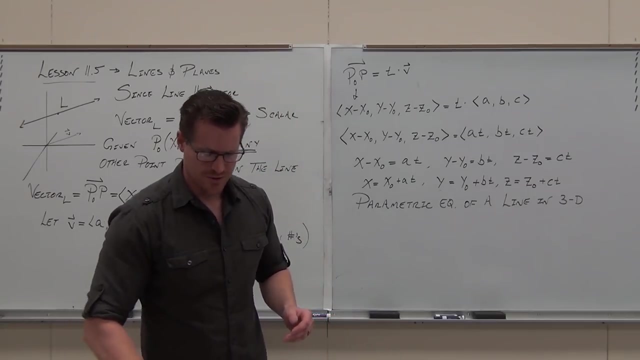 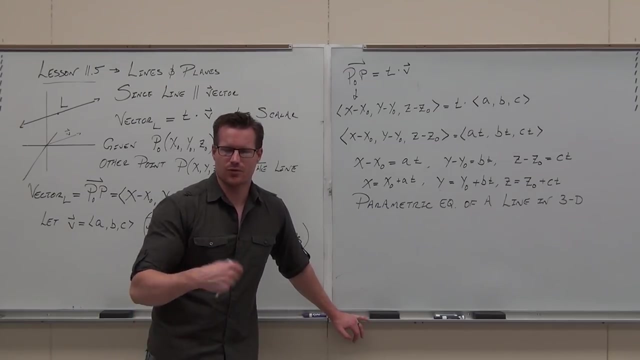 By the way, if you cover that up, you might have seen that in 2D, in parametric. You might have seen this stuff before. How about this one, though? How about this? Firstly, what is T going from? what's the interval of T? 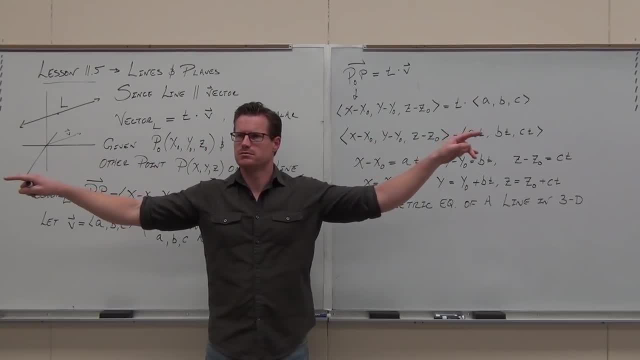 What is it if you have a line? how far do lines go? Forever, Forever. So this parameter, this T, goes typically from negative infinity to positive infinity, unless you have problems with your T, like domain issues or something, or you, yes, yes, 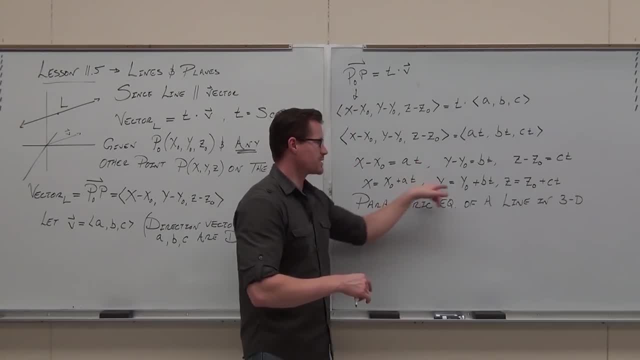 You stop it. You say I'm just talking about this interval. So typically this T goes forever. Now here's my next question: Can you take, since it's the same T, can you solve each of these for T? 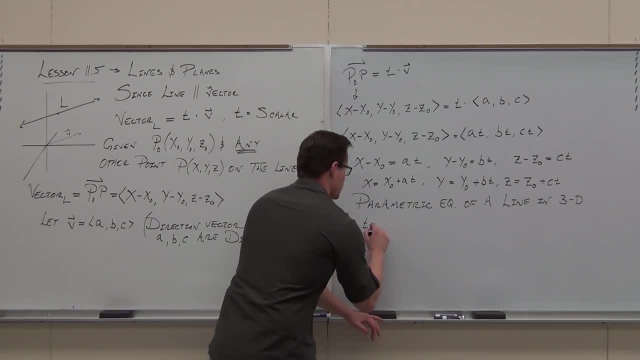 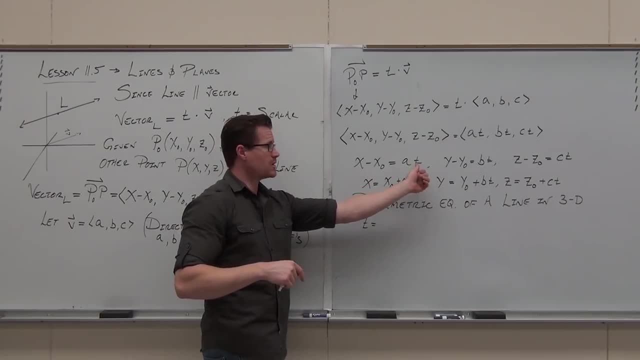 Yes, Let's try that. I'm gonna do it real quick, real quick-like. So T equals X minus X, zero over A. You could actually do it from here. This is probably easier Solve for T here, here and here. 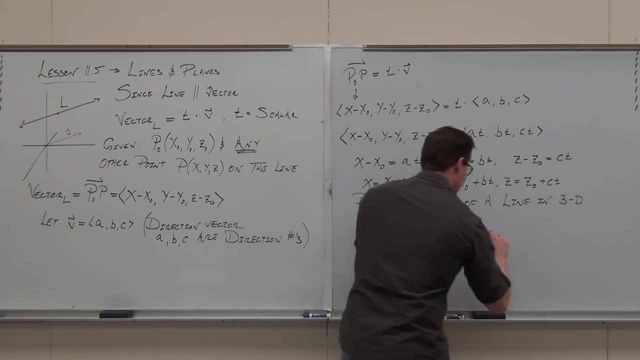 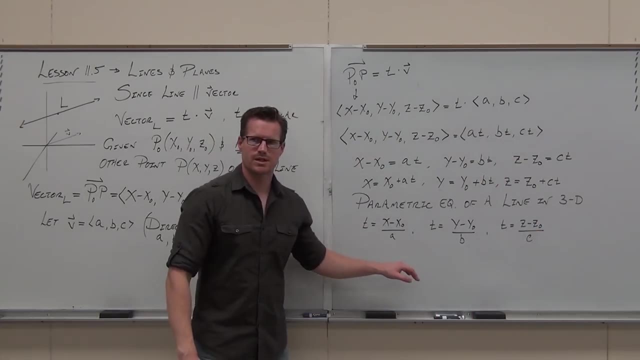 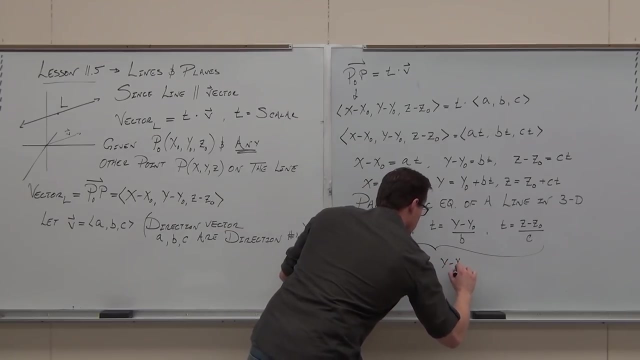 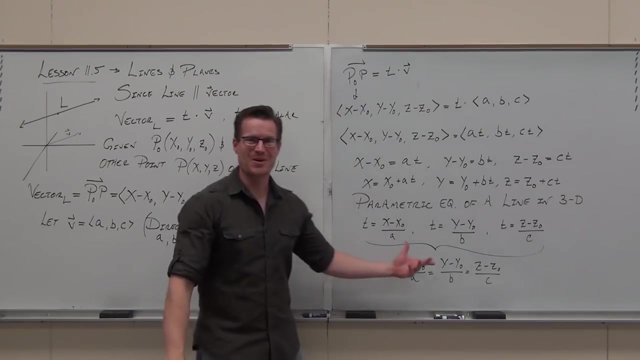 One more little step here. Notice it's the same T. So if this is the same T that we have solved for, combine all this stuff down. That's weird. Does it make sense? on how we get that? Come on, look at the board here real quick. 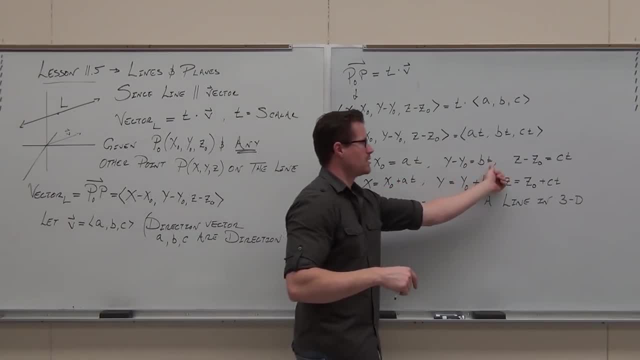 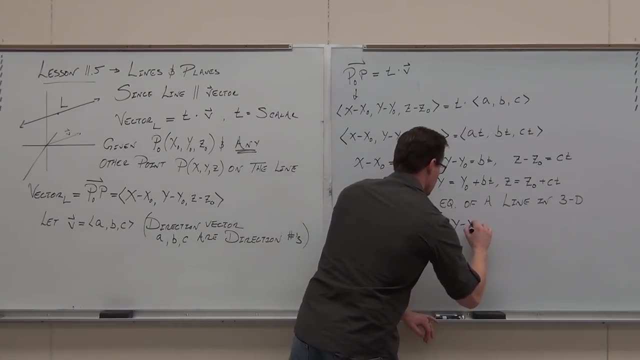 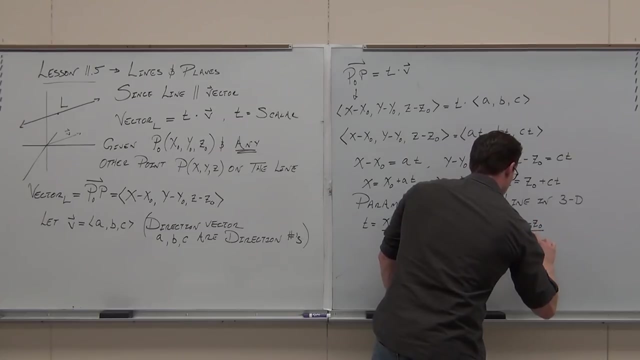 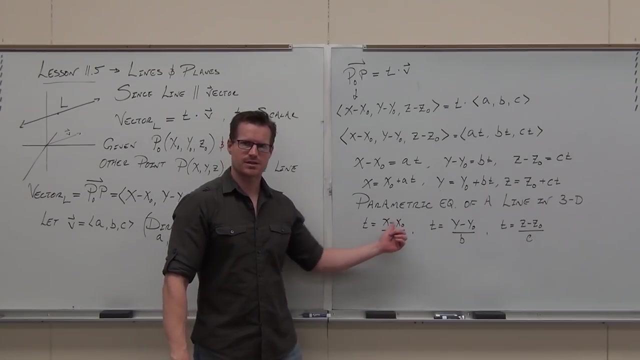 You could actually do it from here. This is probably easier Solve for T here, here and here. One more little step here. notice it's the same T. So if this is the same T that we have solved for, combine all this stuff down. 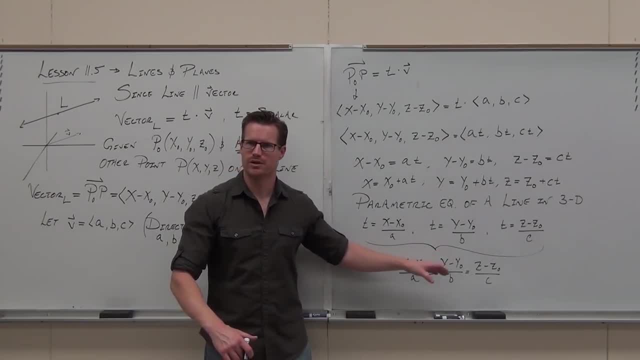 That's weird. It doesn't make sense on how we can do this. It's the same T. Yeah, Come on, look at the board here real quick. Does it make sense on how we get to that We can solve for T. solve for T, solve for T. 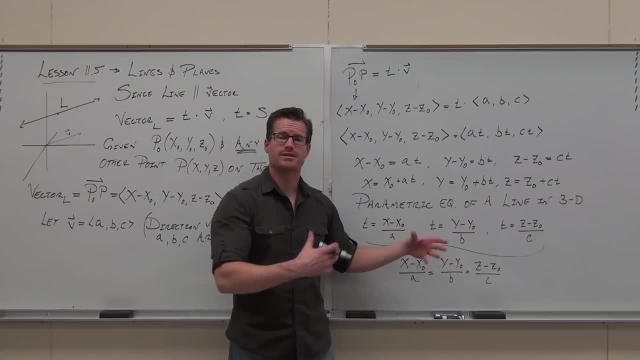 Then these things have to be equal. This is a different way to write the same thing. So there's two ways to write the equation of a line. Two ways for us: This one, which I. I actually like this one a whole lot. 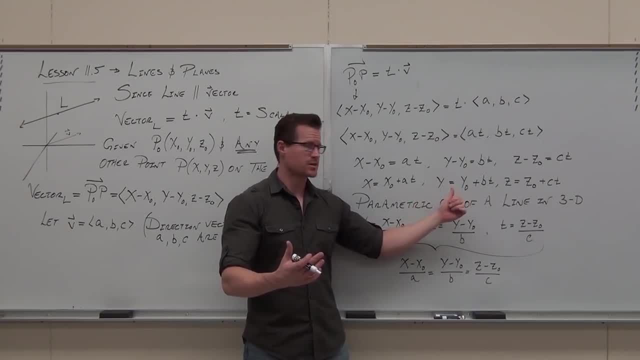 This one. this is the parametric equation for a line, because you're given the parameter T. That's the only variable that you have is that T. Plug in T gives you X coordinate. Plug in T gives you Y coordinate. Plug in T gives you Z coordinate. 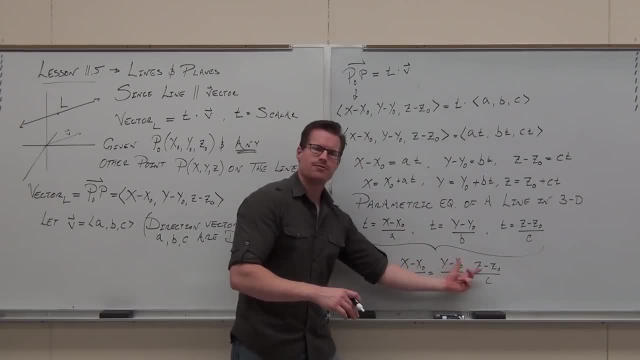 That's the parameter. Or if you solve for T, you have this form. This is called the symmetric equation of a line. Either one, we're going to use both. It's very much like the vector notation IJK or vector brackets- same junk, okay. 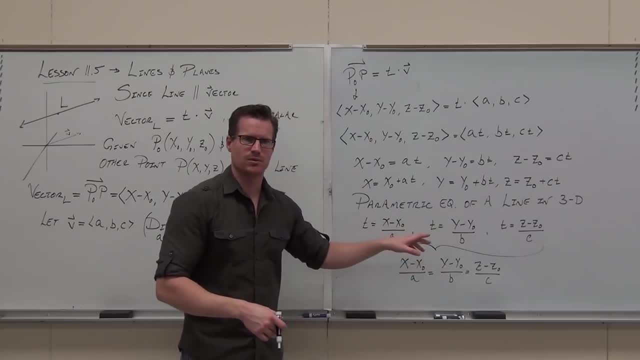 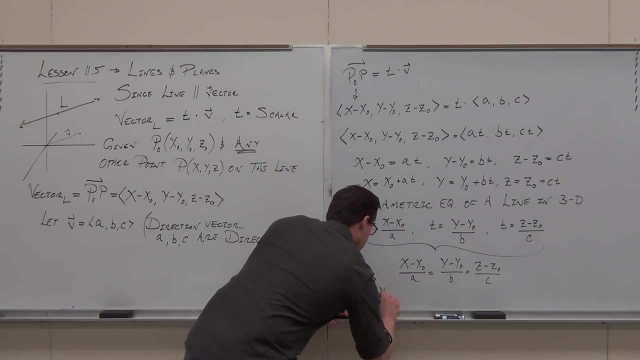 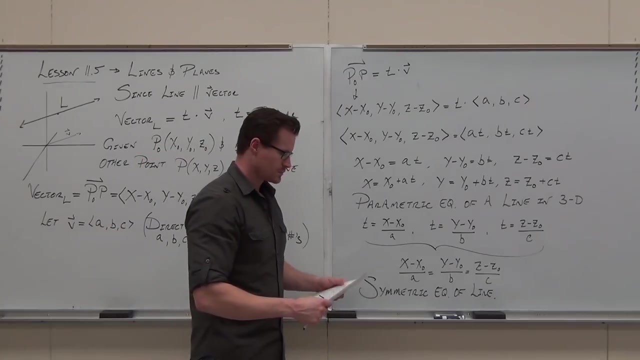 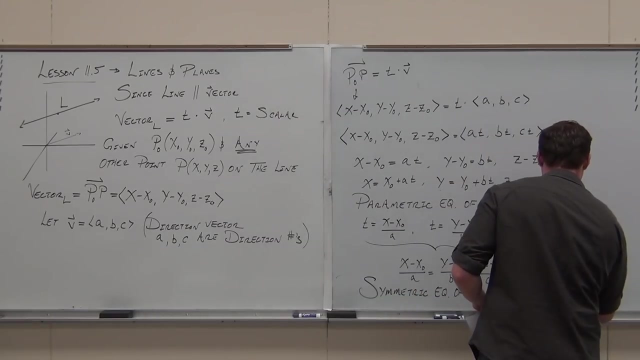 The real things I want you to know is what the pieces do. all right, So we're going to write down what this is and then we'll talk about what all these things are. These two things say the same thing. I'm sorry I missed it. 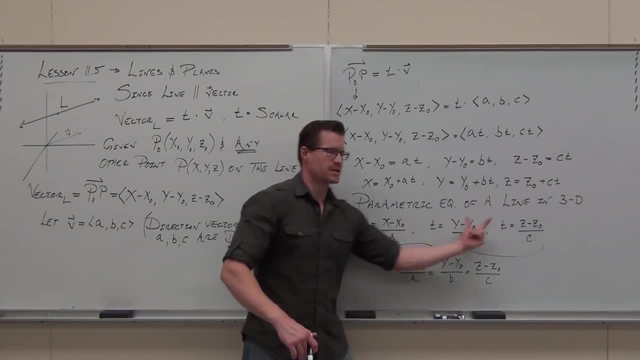 Does it make sense on how we get that? If we can solve for T, solve for T, solve for T, then these things have to be equal. This is a different way to write the same thing, So there's two ways to write the equation of a line. 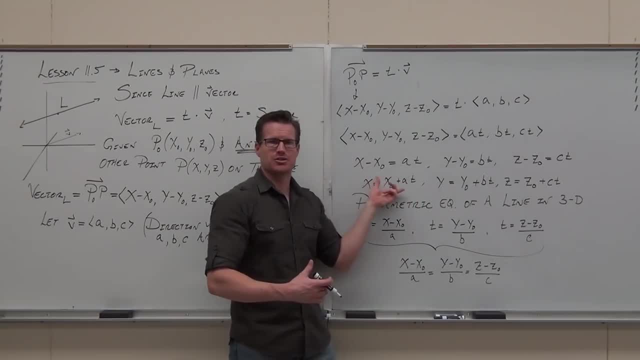 Two ways for us. This one, which I actually like. this one a whole lot. This one: this is the parametric equation for a line, because you're given the parameter T, That's the only variable that you have is that T. Plug in T gives you X coordinate. 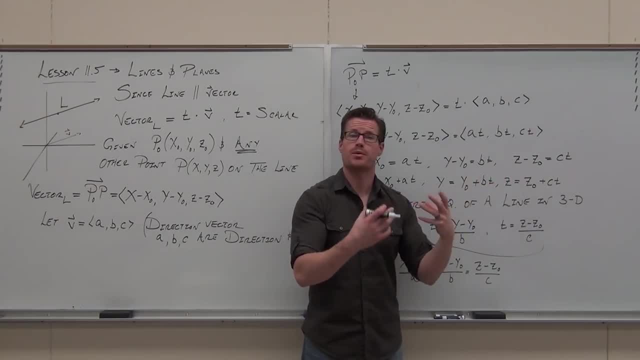 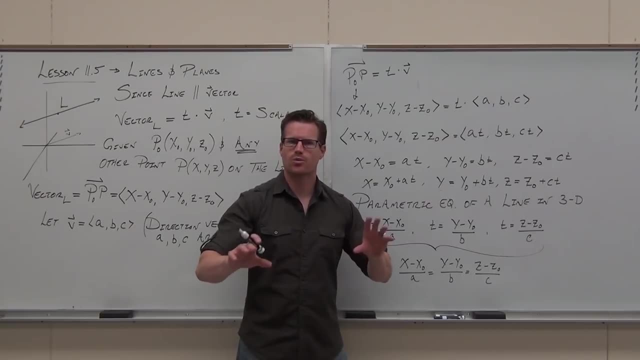 Plug in T gives you Y coordinate. Plug in T gives you Z coordinate. That's the parameter. Or if you solve for T, you have this form. This is called the symmetric equation of a line. Either one, we're gonna use both. 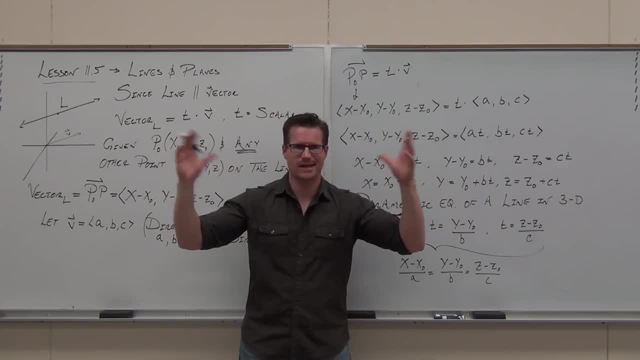 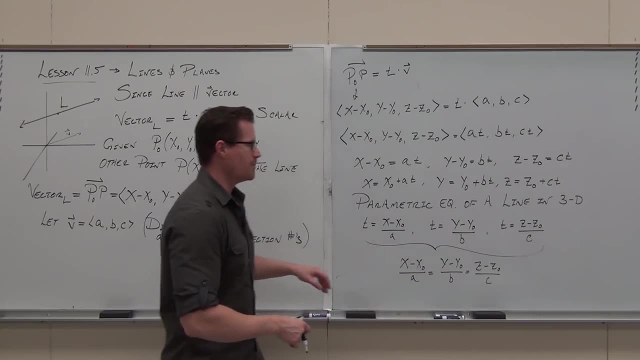 It's very much like the vector notation I, J, K or vector brackets- same junk. okay, The real things I want you to know is what the pieces do. All right, so we're gonna write down what this is. 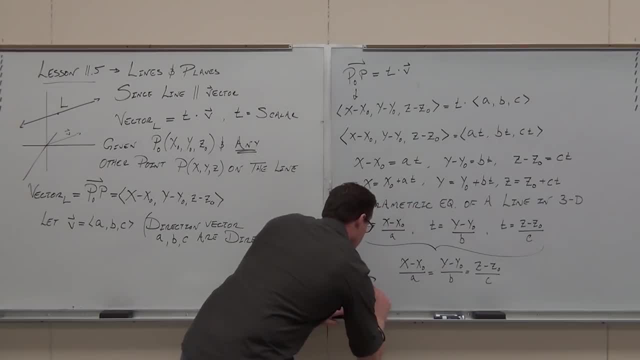 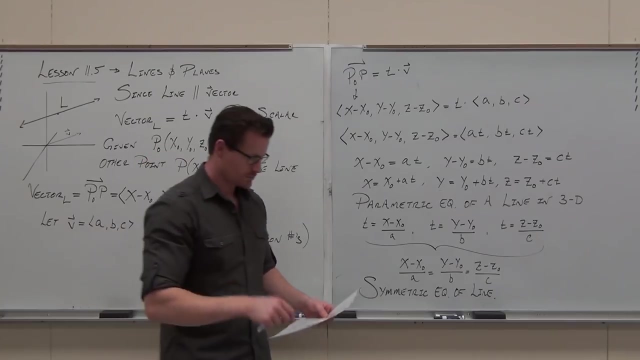 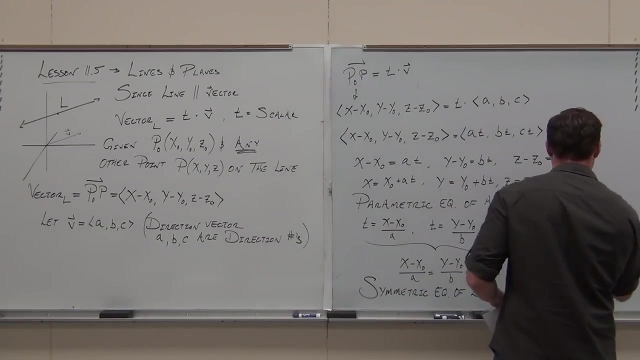 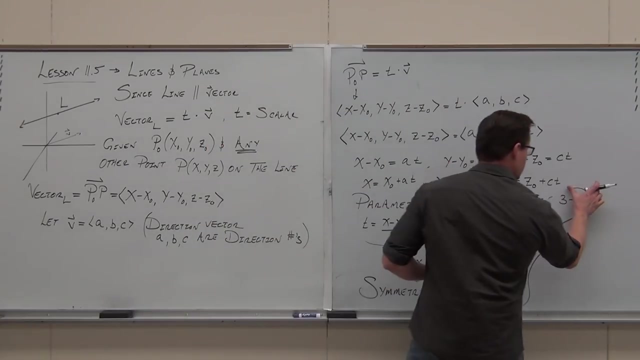 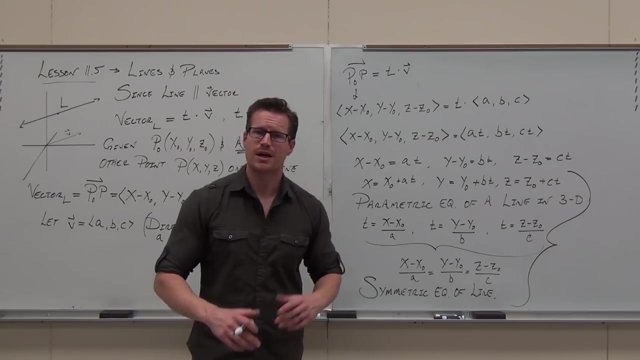 and then we'll talk about what all these things are. All right, These two things say the same thing. I'm sorry I missed it. These two things say the same thing. I want you to use them universally. First thing, I want you to see what goes on. 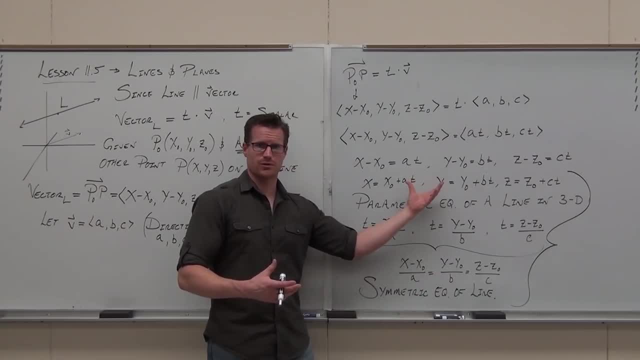 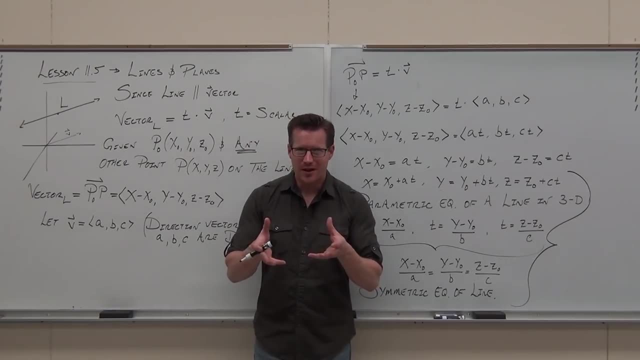 Do you understand that these are equivalent, This one and this one's equivalent. We got the parametric or we got the symmetric. They say the same thing. What they say is: hey, what two things do you need to make the equation of a line in 3D? 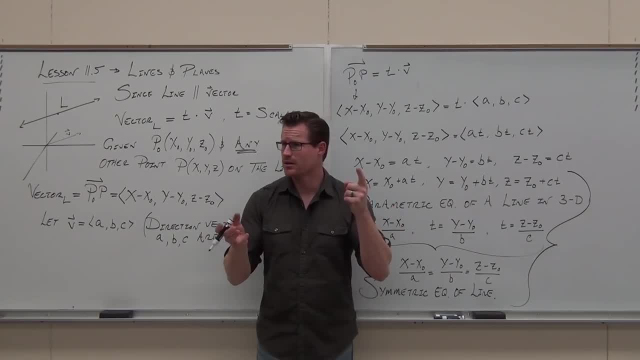 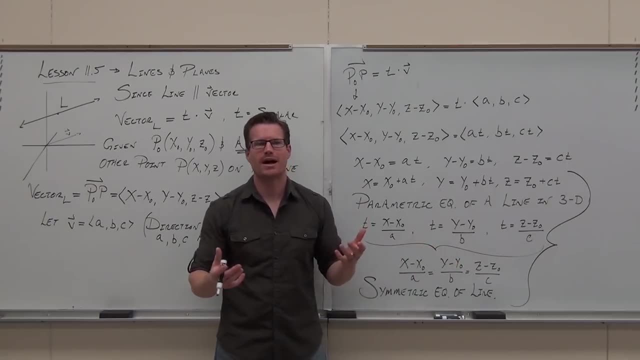 What two things? A point and a direction vector. Does this have a point and a direction vector in it? So this is for hey, if I give you a point. no, wait a minute, Let's see if you're really paying attention. 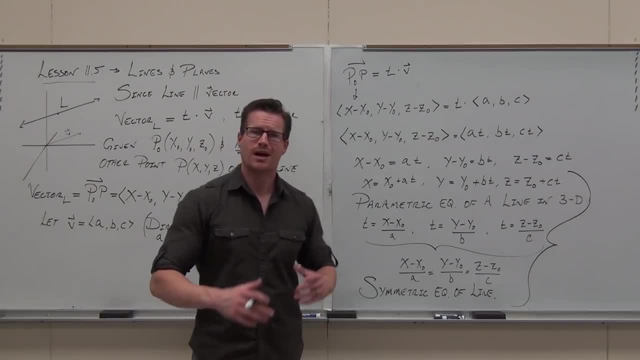 These two things say the same thing. I want you to use them universally. First thing, I want you to see what goes on. Do you understand that? these are equivalent, this one and this one's equivalent. We got the parametric, oh, we got the symmetric. they say the same thing. 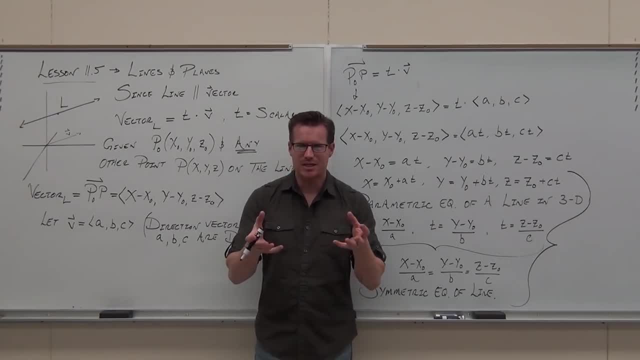 What they say is: hey, what two things do you need to make the equation of a line in 3D? What two things? A point and a direction vector. Does this have a point and a direction vector in it? So this is for hey, if I give you a point. no, wait a minute, let's see if you're really paying attention. 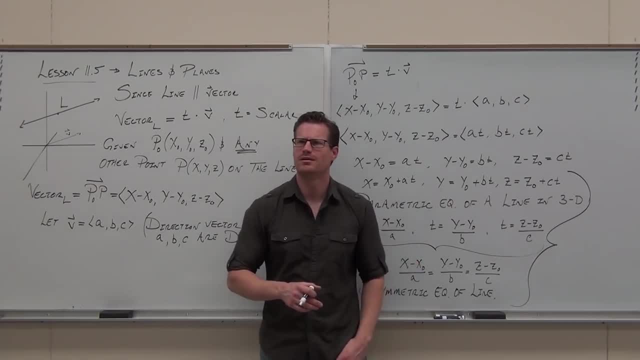 What's the point? Some of you guys are wondering that right now. What is the point, Man? What is the point in both of these, this or this? what's the point? Exactly what we started with the given point, So this works for any point. 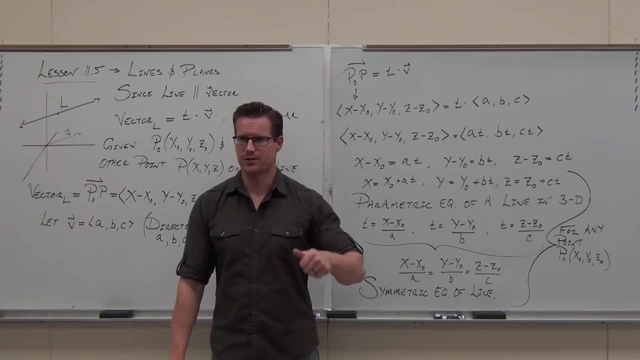 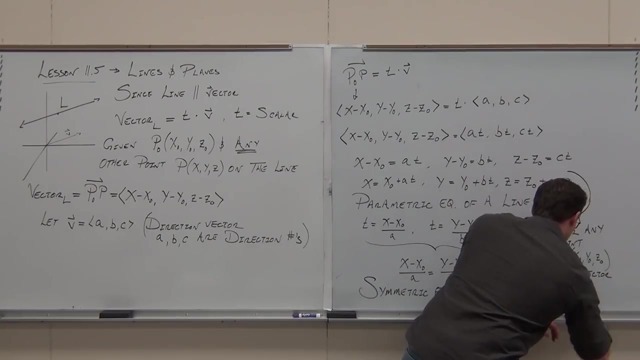 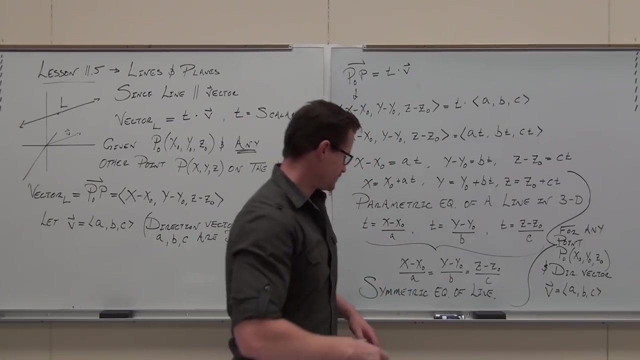 You need a point, you need a vector point and direction vector And, oh my gosh, what's the vector Vector ABC. Now let's see 20 minutes. Talk for 20 minutes about the equation of a line. 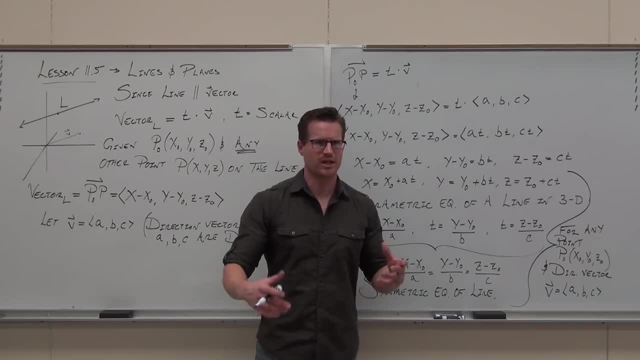 Is it super hard? No, No, it's not. It's really really easy. But I want you to get where it comes from. I could have started the class right here and said: oh, this is the equation of a line. 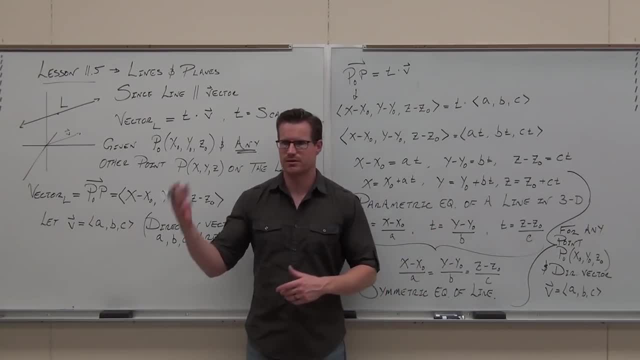 Start with a point: X0,, Y0, you just put it here And you take a vector in the same direction and you put it here And you know what You can do it that way, But I want you to understand the idea of why this is the way it is. 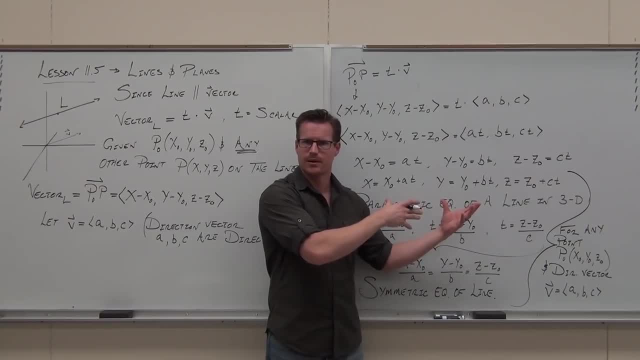 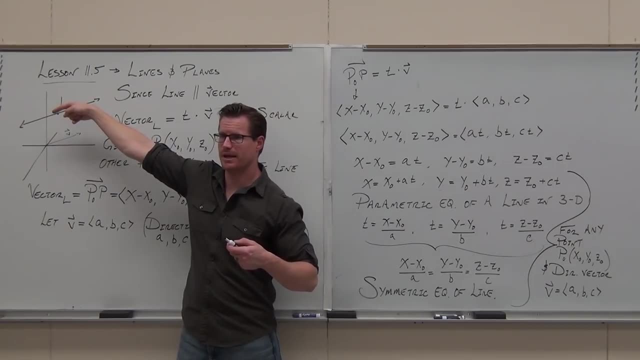 Have I explained it well enough for you to understand where it comes from. You're taking a direction vector. you're pushing it up by multiplying by a scalar multiple until it actually goes through your point. That's what you're doing. You go okay. well, how do I do that? 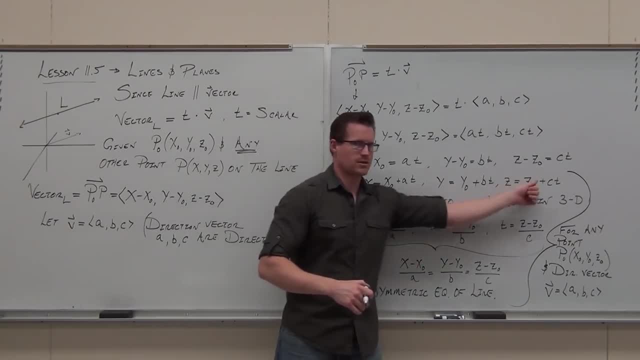 Take the point, take the vector, add some crap to it until it hits the point. That's what we're doing really. We're taking a vector, multiplying scalar, raising it and going through that point. That's the idea. 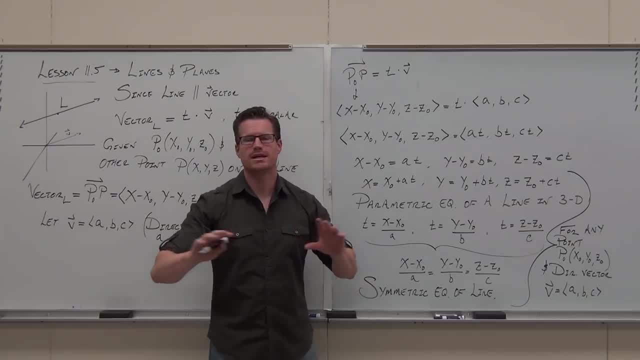 I don't know if you're okay with the idea Now how we use it. it's really, it's honestly really easy, As long as you're given the two things you need. If I give you a point and a vector, you can fill out either one of these things: X0, Y0.. 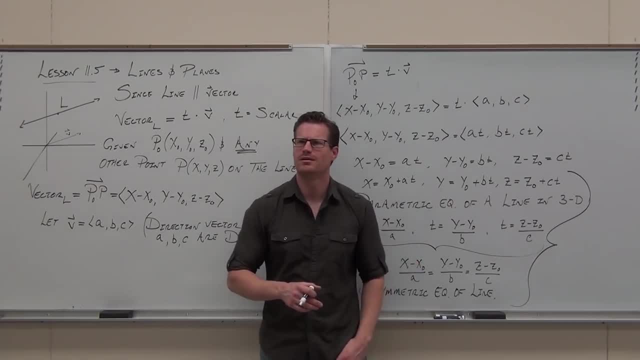 What's the point? Some of you guys are wondering that right now. What is the point, Man? What is the point in both of these, this or this? What's the point? Exactly what we started with the given point. So this works for any point. 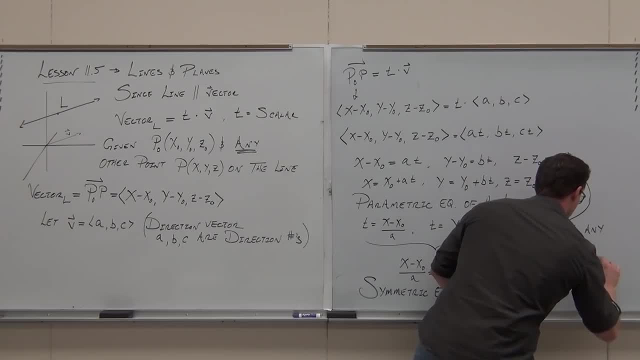 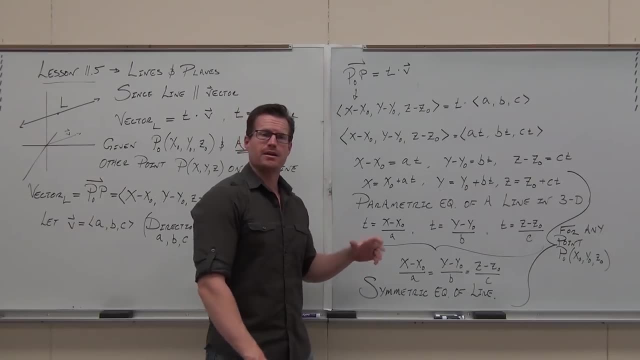 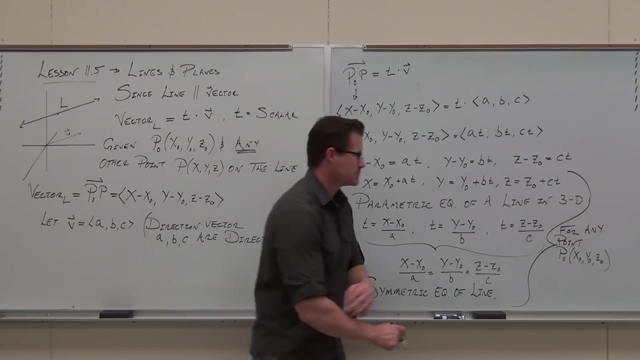 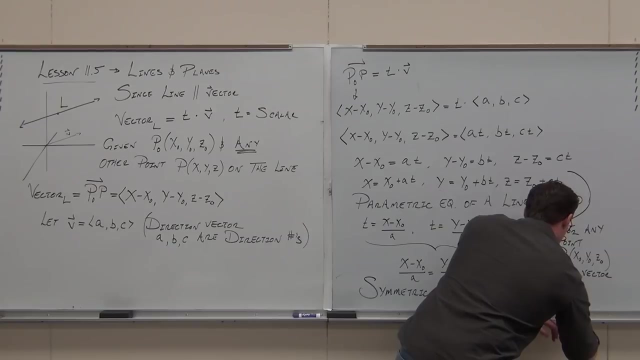 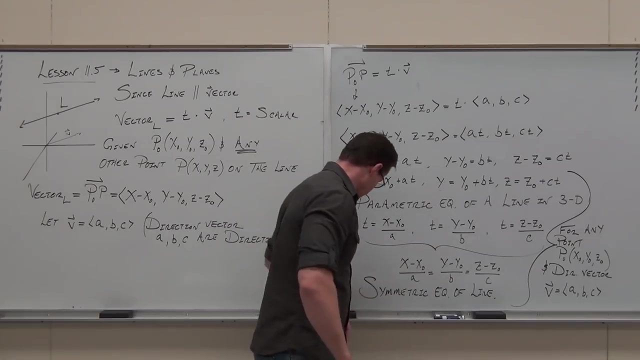 You need a point, you need a vector point and direction vector And, oh my gosh, what's the vector Vector ABC. Now let's see 20 minutes. Talk for 20 minutes about the equation of a line. 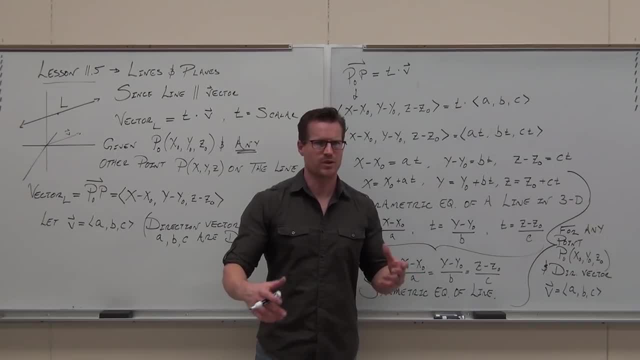 Is it super hard? No, No, it's not. It's really really easy. But I want you to get where it comes from. I could have started the class right here and said: oh, this is the equation of a line. 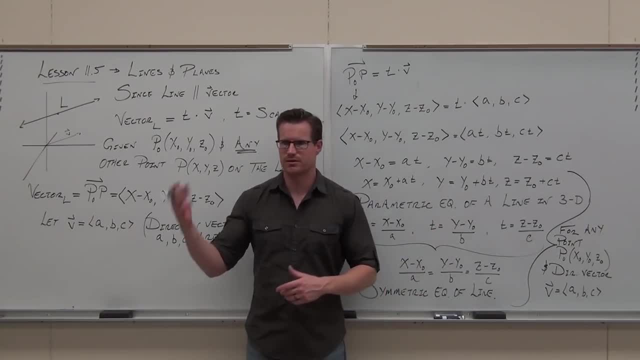 Start with a point: X0,, Y0, you should put it here. And you take a vector in the same direction and you put it here And you know what. You can do it that way, But I want you to understand the idea of why this is the way it is. 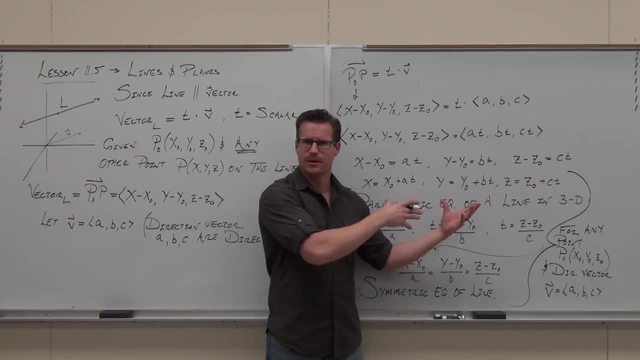 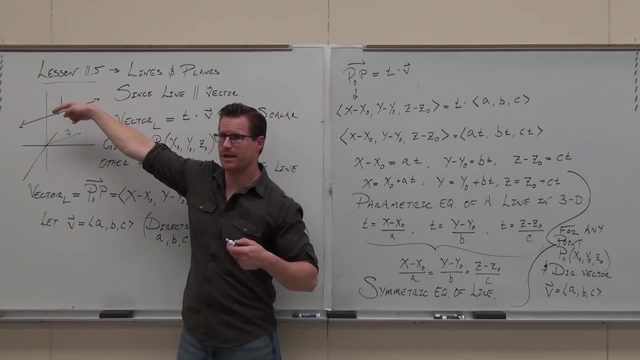 Have I explained it well enough for you to understand where it comes from. You're taking a direction vector, You're pushing it up by multiplying, by scalar multiplying. That's what you're doing. You go okay. well, how do I do that? 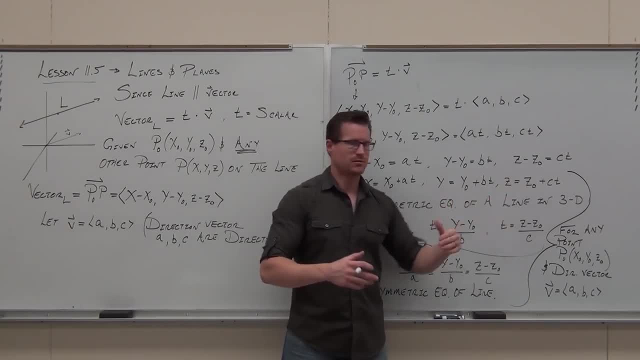 Take the point, take the vector, add some crap to it until it hits the point. That's what we're doing really. We're taking a vector, multiplying scalar, raising it and going through that point. That's the idea. 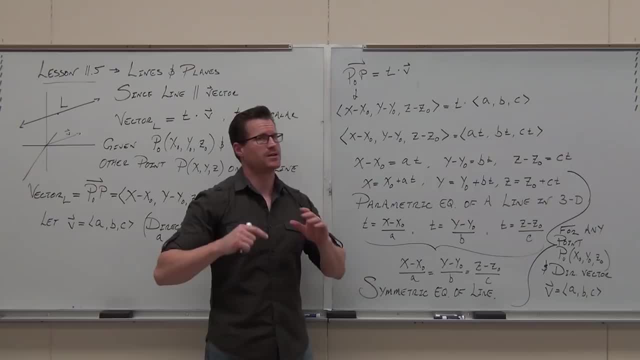 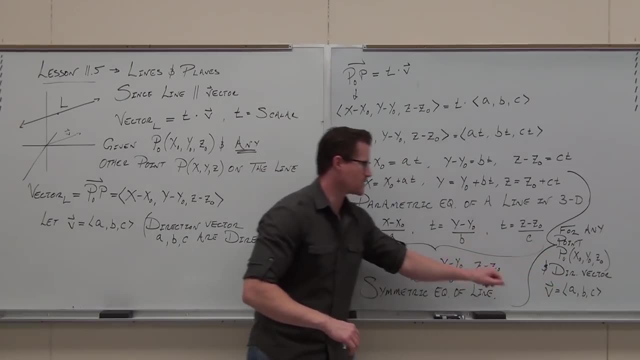 I don't know if you're okay with the idea Now how we use it. it's really, it's honestly really easy, As long as you're given the two things you need. If I give you a point, Okay, If I give you a point and a vector, you can fill out either one. 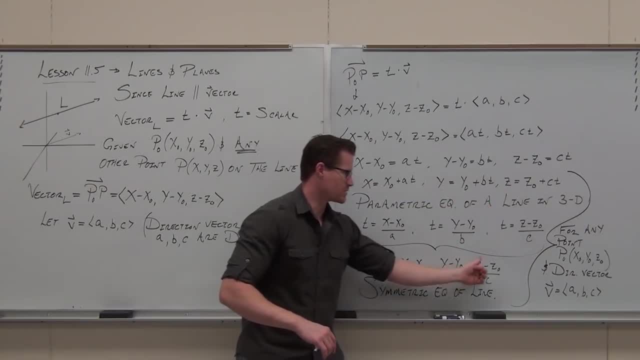 of these things: x sub 0,, y sub 0, or x sub 0,, y sub 0,, z sub 0, and then the direction numbers a, b, c in the same order. It's really nice. 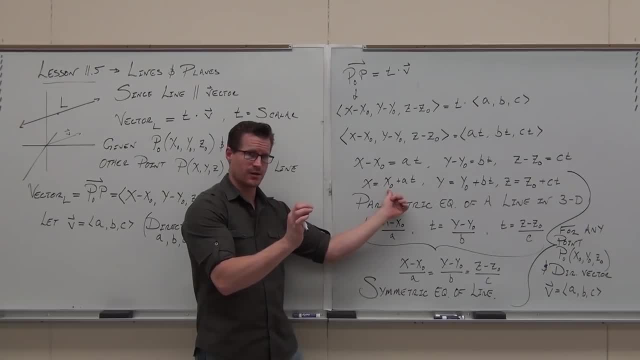 X goes with x and x. the x coordinate of the point goes with x. The x component of the vector goes with x. Please just don't get these confused. It's really easy for students to be given this thing that has three numbers and this thing that has three numbers. 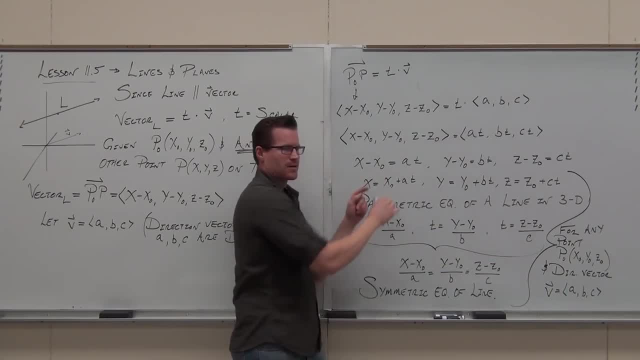 and put them in all the wrong spots, And put this here and this here, and then you don't have the same thing. Does that make sense? Be careful on what these are. Also, what's really cool. anytime I give you one of these lines and I say, hey, 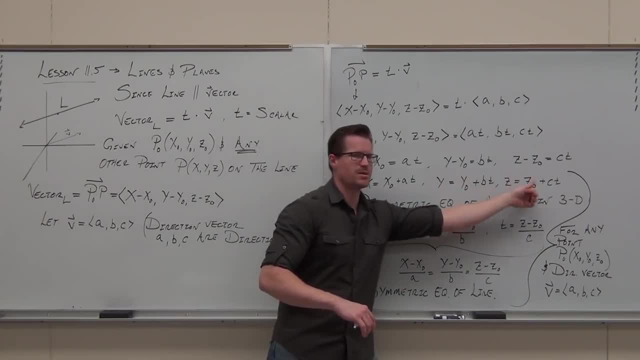 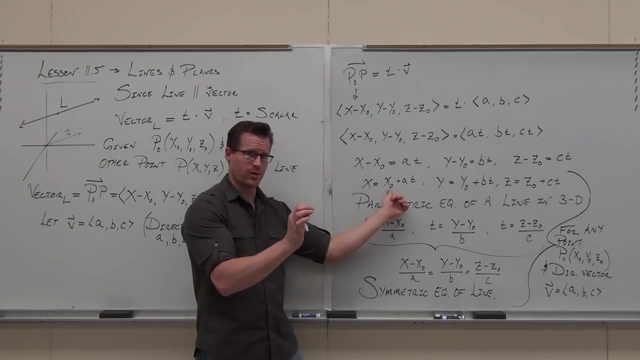 Or X0,, Y0, Z0, and then the direction numbers A, B, C in the same order. It's really nice. X goes with X and X. the X coordinate of the point goes with X. The X component of the vector goes with X. Please just don't get these confused. 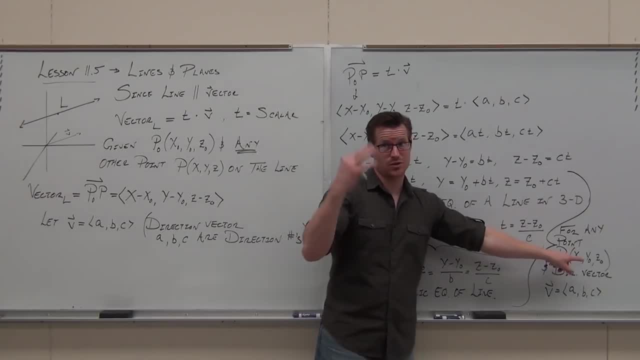 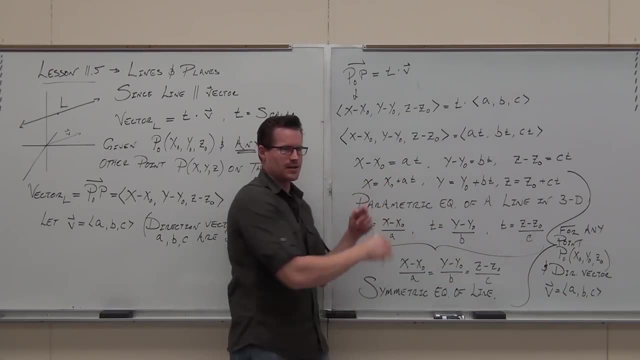 It's really easy for students to be given this thing that has three numbers and this thing that has three numbers and put them in all the wrong spots, And put this here and this here, and then you don't have the same thing. 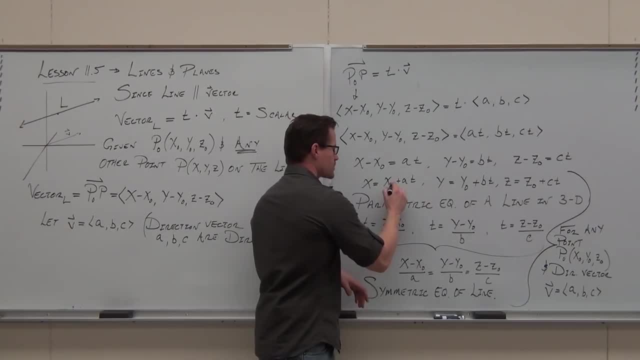 Does that make sense? Be careful on what these are. Also, what's really cool: any time I give you one of these lines and I say, hey, can you find the vector that's parallel to that line? Can you find a vector that's parallel to this? 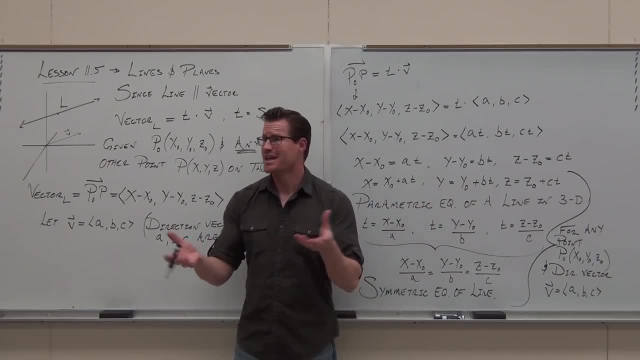 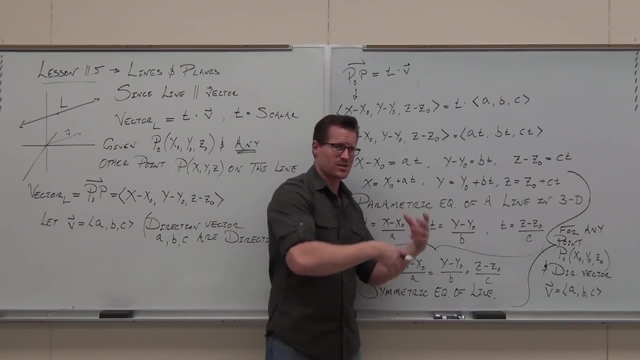 Yeah, As long as you have A, B and C, you automatically have the vector. Can you find a point on the line? Yeah, Automatically, you have a point on the line. It's pretty cool. It literally gives us the two things we need to make the equation of line. 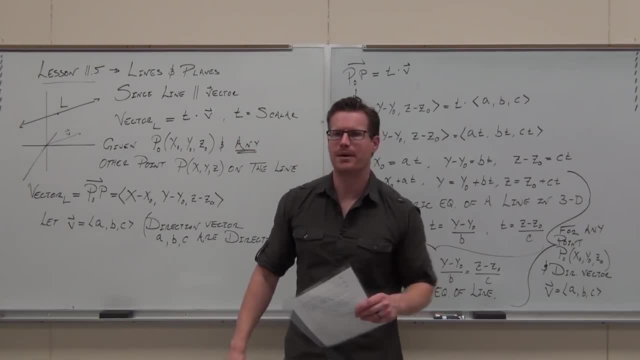 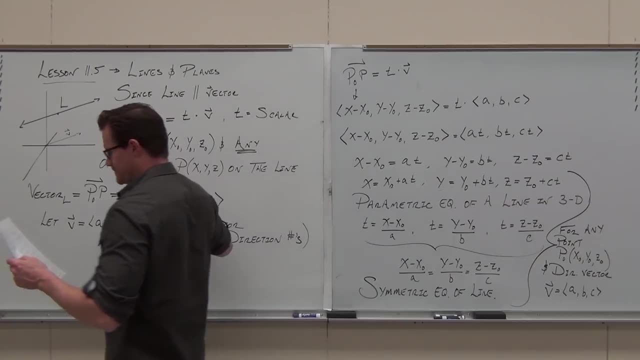 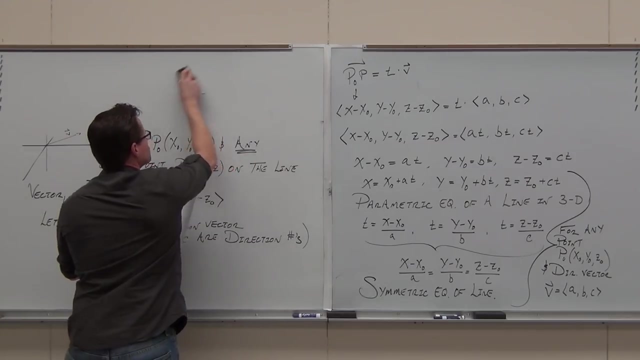 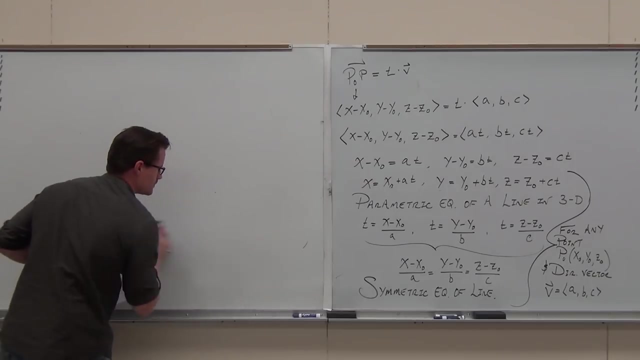 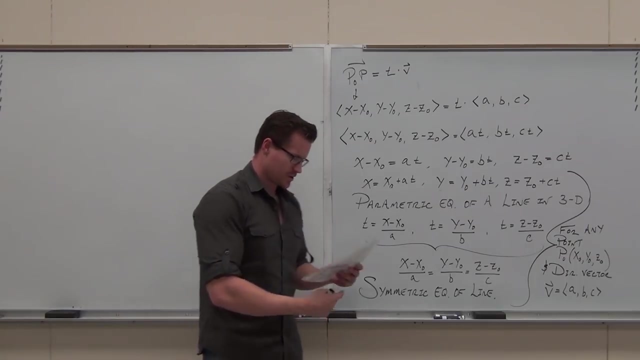 Now let's practice some, because I know I've probably bored the crap out of you Just a little bit Just right now with all the- I hope I didn't. I wanted you to understand it. You know what, Actually, I'm going to write a couple notes before I do that. 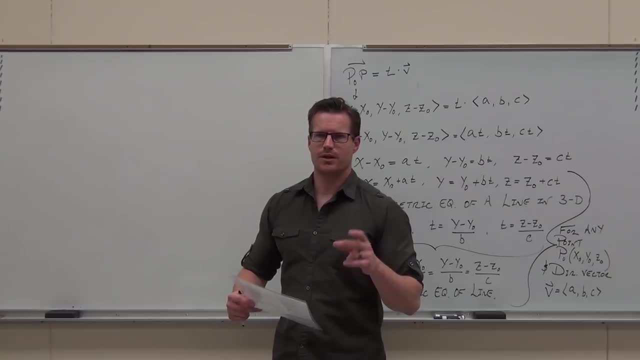 I know I'm going to forget if I don't do this. I want you to know that if a direction number, what's a direction number? X, zero, Y sub zero, Z sub zero or A, B, C, What are direction numbers? quickly, 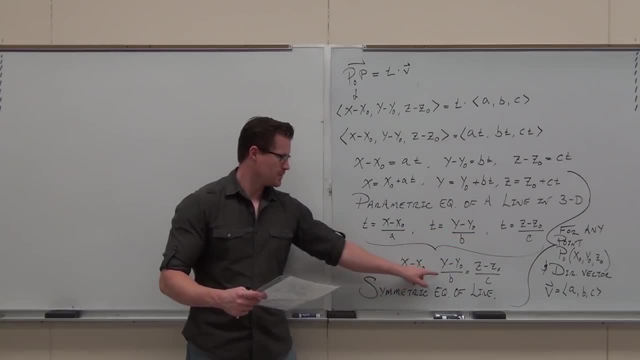 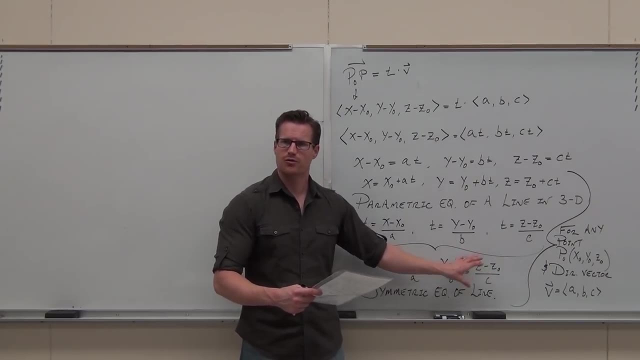 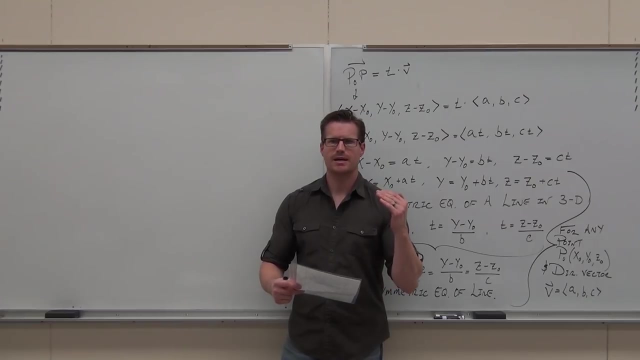 If one of those is zero. if one of those is zero, it's possible This: you lose the equation because you have this undefined thing: If one of those is zero, so here or here or here, If one of those is zero, then what that means is that the line is actually bound. 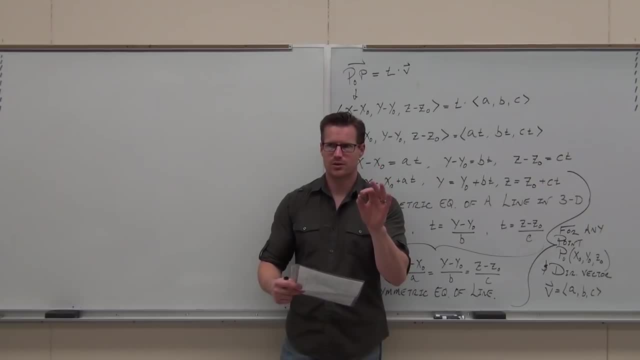 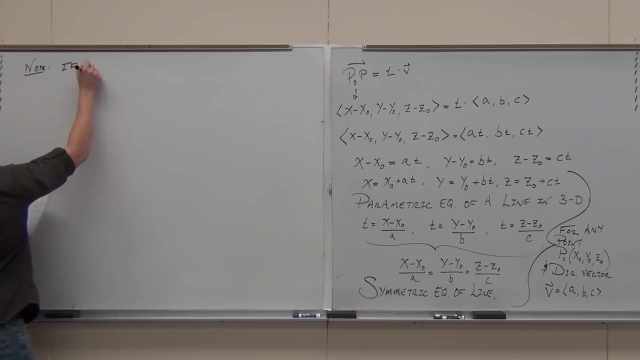 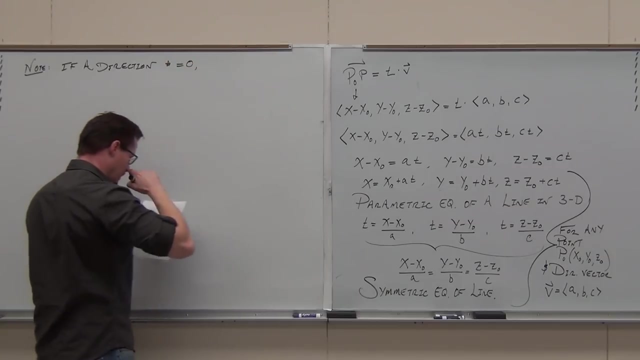 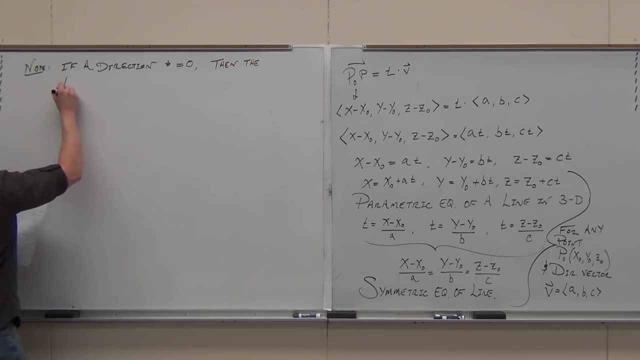 in a plane. if a direction number is zero, your line is actually in a plane that's parallel to the YZ axis, the XZ axis or the XY axis. I'm going to write that out here real quick. Let's just say that A is zero, okay. 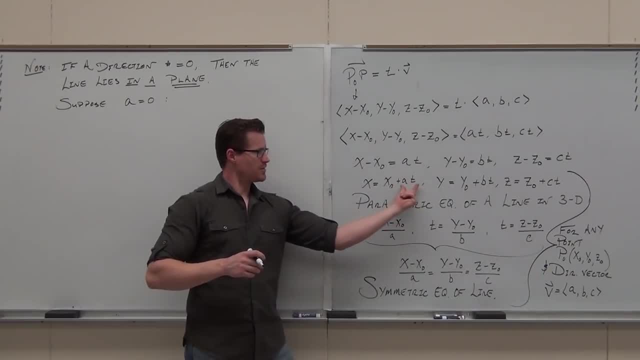 So zero means zero. This piece is zero Zero times a number. I don't care what it is is zero. So what that means is that X would equal X sub zero. You can do it here, but this is easier. 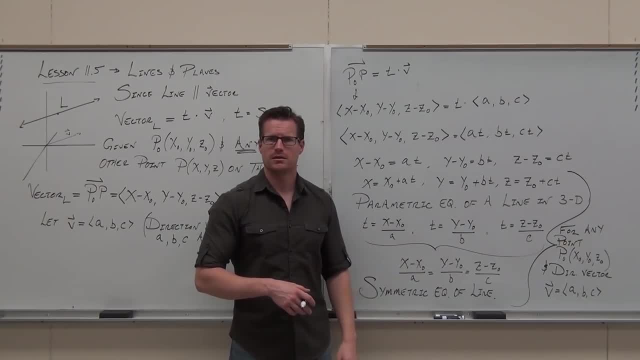 can you find the vector that's parallel to that line? Can you find a vector that's parallel to this? Yeah, As long as you have a, b and c, you automatically have the vector. Can you find a point on the line? 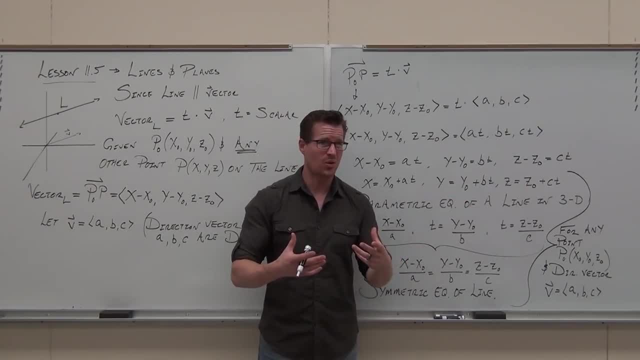 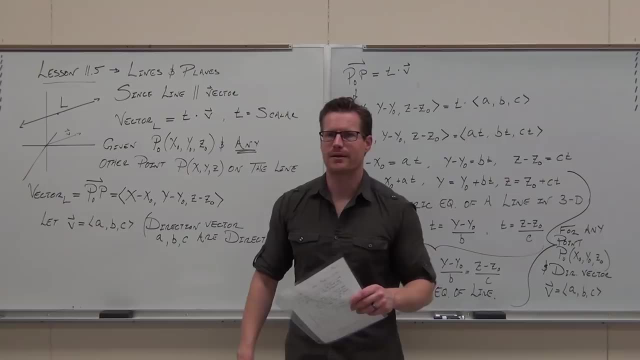 Yeah, Automatically you have a point on the line. It's pretty cool. It literally gives us the two things we need to make the equation work. Now let's practice some, because I know I've probably bored the crap out of you just right now with all the I hope I didn't. I wanted you to understand it. 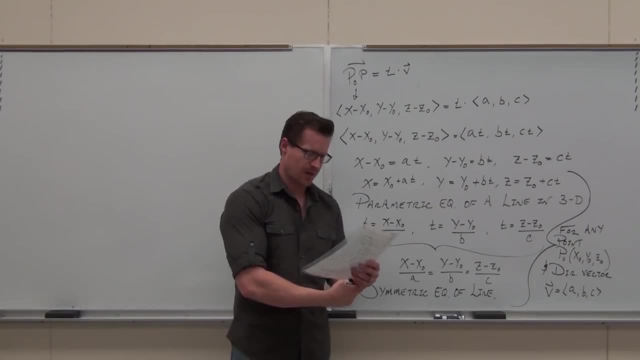 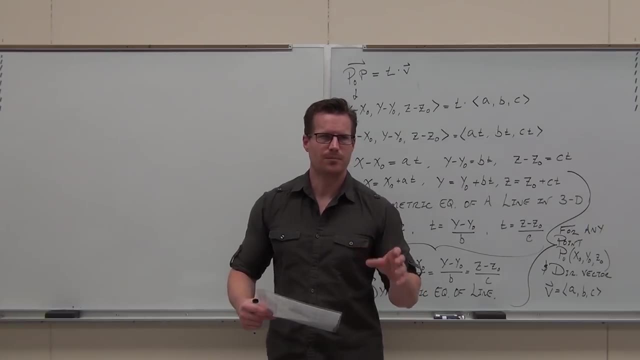 You know what actually? I'm going to write a couple notes before I do that. I know I'm going to forget if I don't do this. I want you to know that if a direction number, what's a direction number? X, zero, Y, sub zero, Z sub zero or ABC? 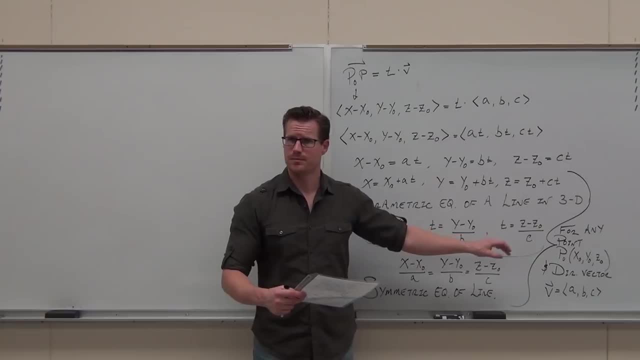 What are direction numbers quickly, If one of those is zero? if one of those is zero, it's possible This: you lose the equation because you have this undefined thing If one of those is zero. so here or here or here. 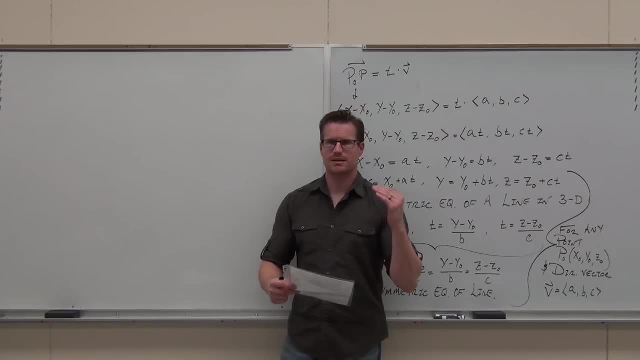 If one of those is zero, it's possible. If one of those is zero, then what that means is that the line is actually bound in a plane. If a direction number is zero, your line is actually in a plane that's parallel to the YZ axis, the XZ axis or the XY axis. 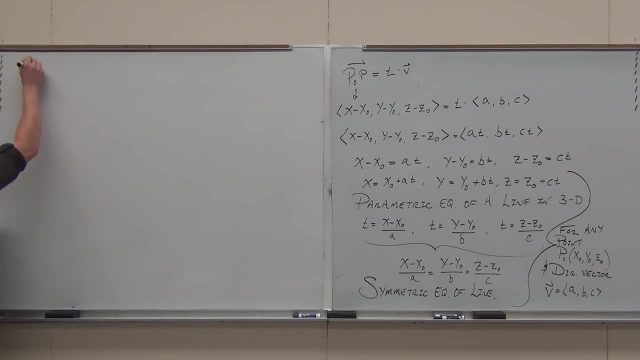 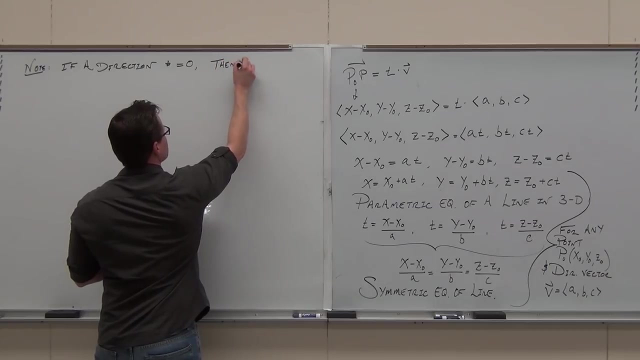 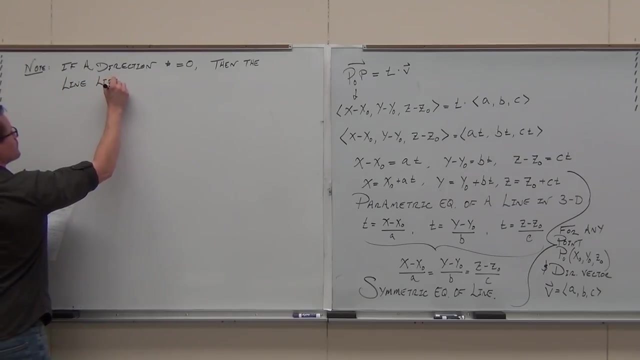 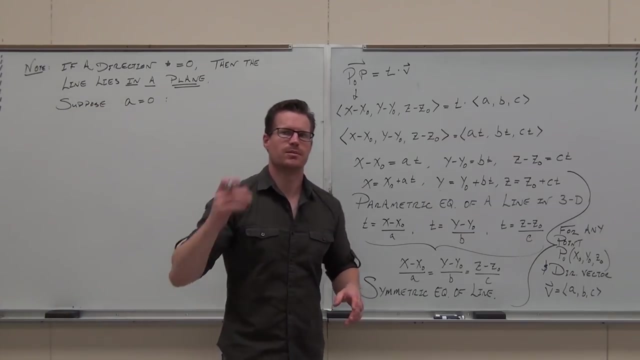 I'm going to write that out here real quick. I'm going to write that out here real quick: Specifically, Specifically, Specifically. Let's just say that A is zero. okay, so zero means this piece is zero. Zero times a number- I don't care what it is- is zero. 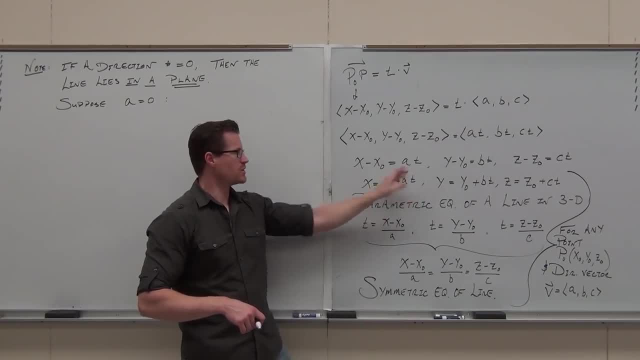 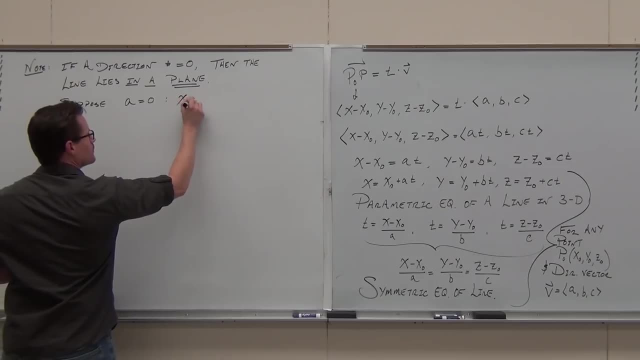 So what that means is that x would equal x sub zero. You can do it here, but this is easier: X would equal x sub zero. Does that make sense to you? What this means here? ladies and gentlemen, please focus. I know there's not a lot of numbers, okay. 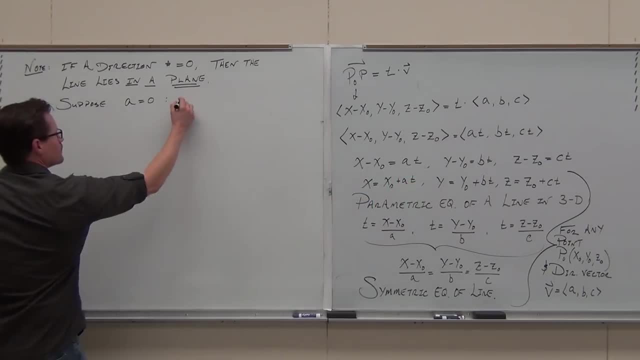 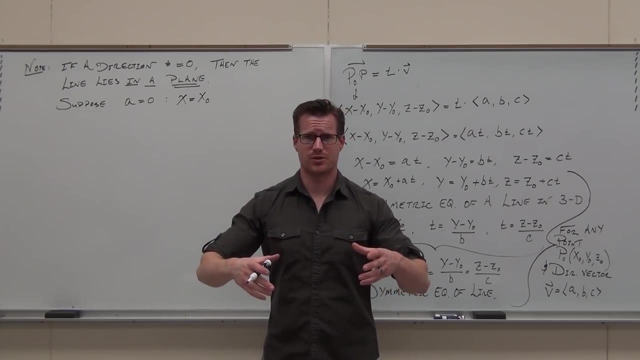 X would equal X sub zero. Does that make sense to you? What this means here? ladies and gentlemen, please focus. I know there's not a lot of numbers, okay, But that's going to be a number. It's going to be a point like three or negative five. 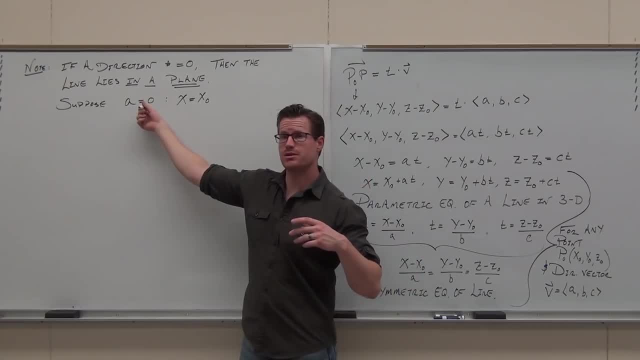 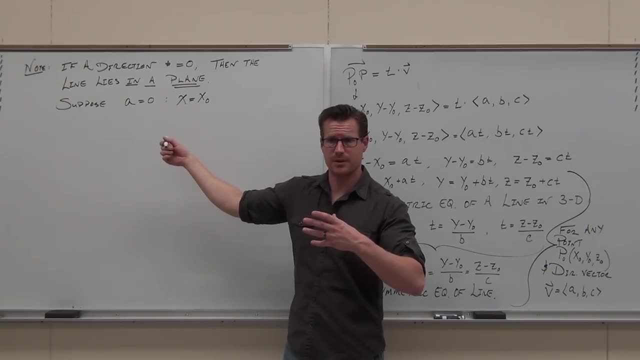 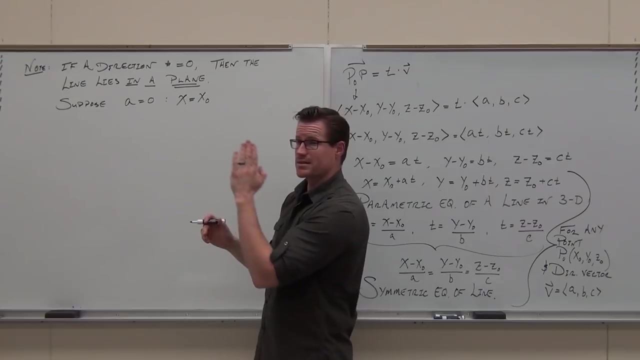 Does that make sense? What this means. if that number is zero, the line is going to lie in the X equals X sub zero plane. So if that's three, it's going to lie in that plane. Remember drawing planes. The plane would go through that X equal three or X sub zero, whatever that is. 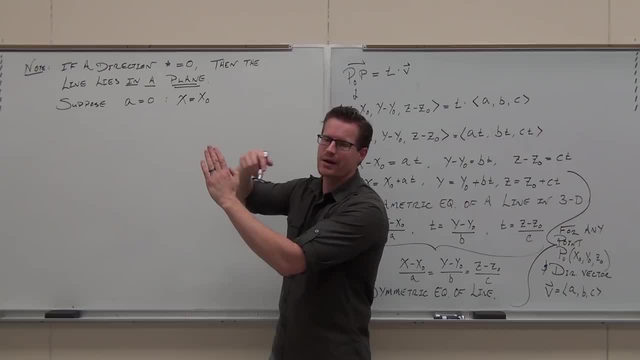 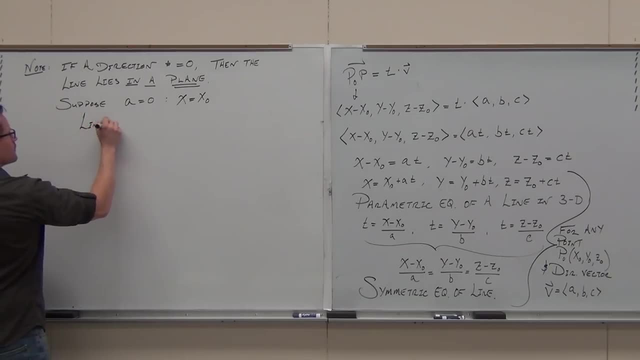 It's going to lie in that plane somewhere. It's actually kind of 2D. It'll be parallel to the YZ plane. That's what would happen here. 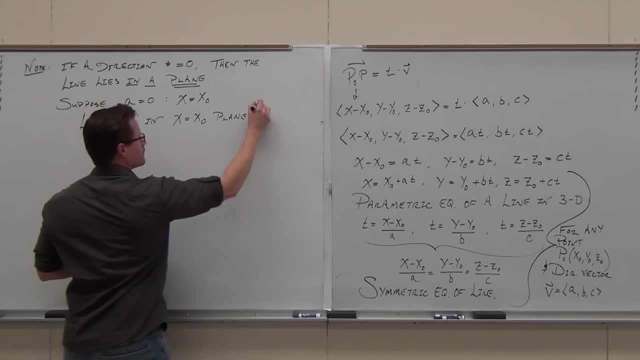 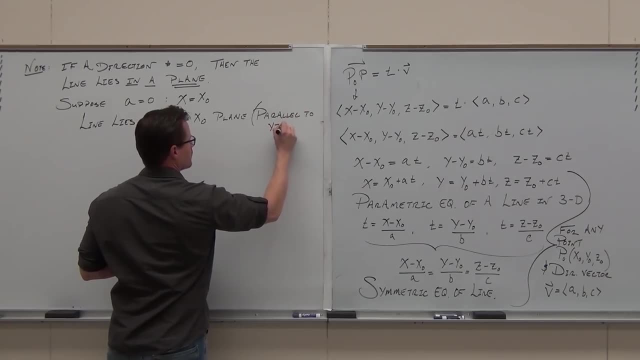 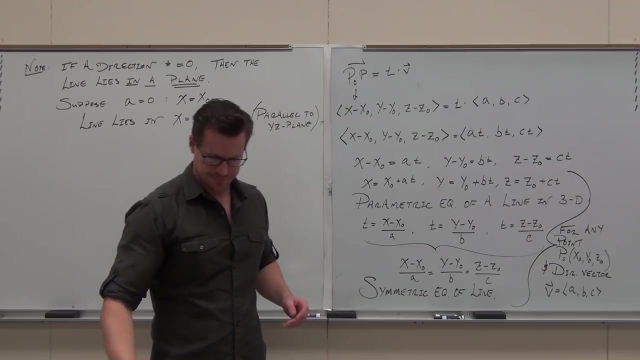 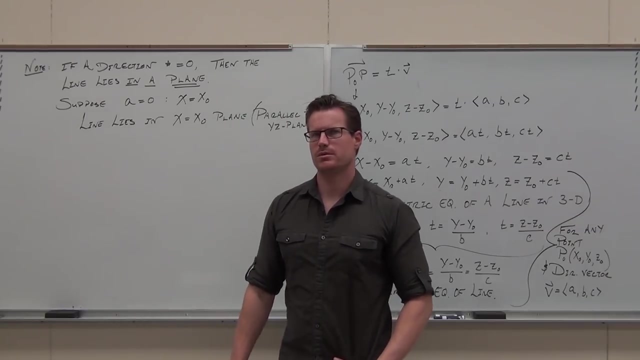 Last little note: How would you tell two lines are parallel In 2D? Not a straight question. You should know this. They never cross. 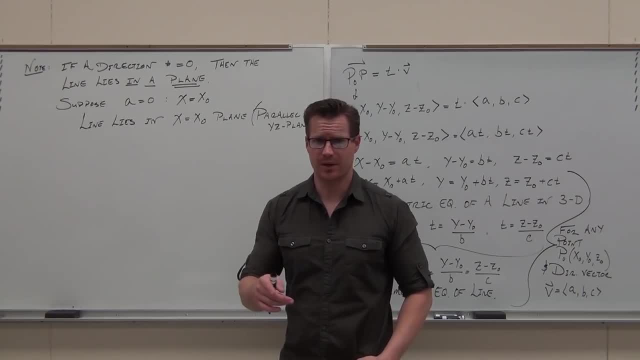 They never cross. Okay, yeah, that's true. How do you tell if they're parallel, though? Like really easy, You've got y equals m. How do you tell if the two lines are parallel? Same slope: Do we have slope in 3D? 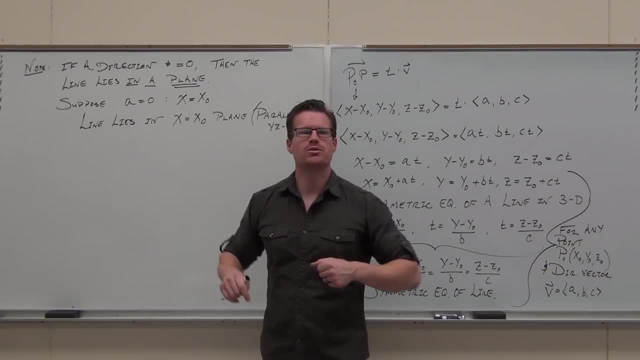 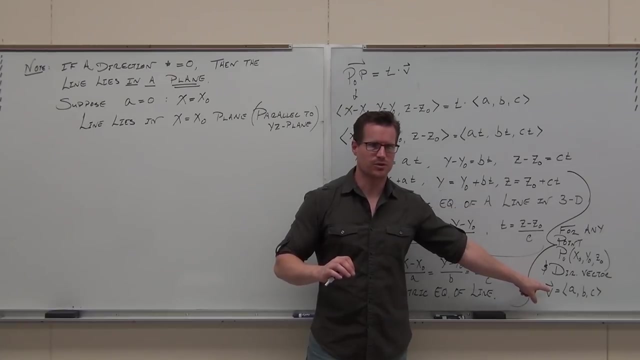 Not. yet What do we have in 3D? How do you tell that two lines will be parallel in 3D? Same direction, Same unit vector or scalar multiples? If they're direction vectors or scalar multiples, Just like we always check for parallel vectors? 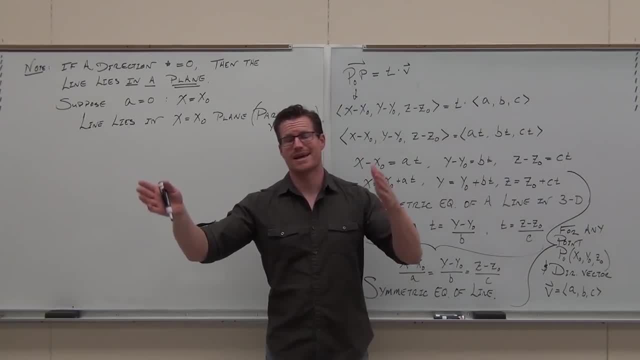 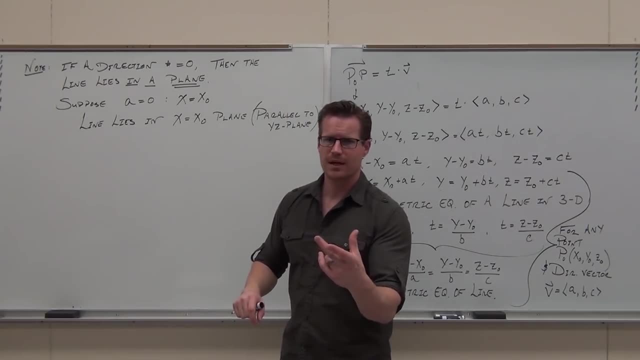 Remember talking about parallel vectors? right? Same stuff, man. Look at the vector lines. Hey, if they're scalar multiples, the lines are parallel. Does that make sense to you? That's how we always check. So two lines are parallel if their direction vectors. 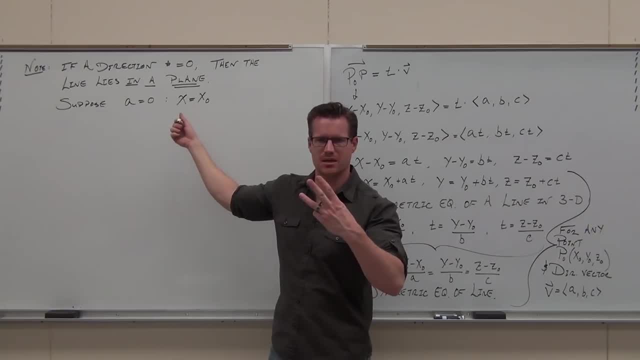 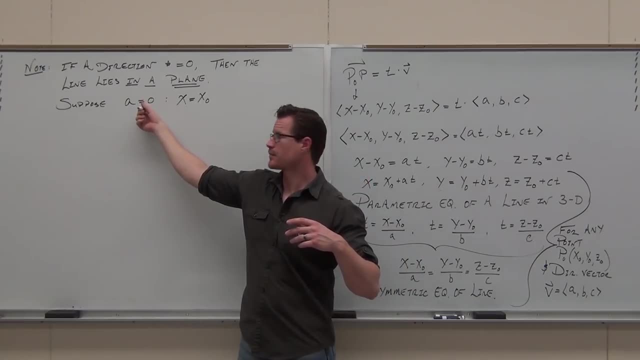 but that's going to be a number. It's going to be a point like three or negative five. Does that make sense What this means? if that number is zero, the line is going to lie in the x equals x sub zero plane. 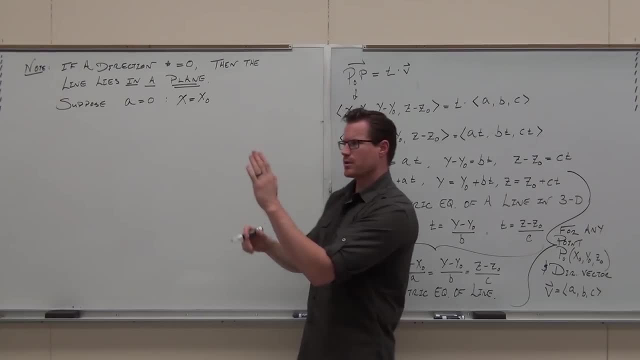 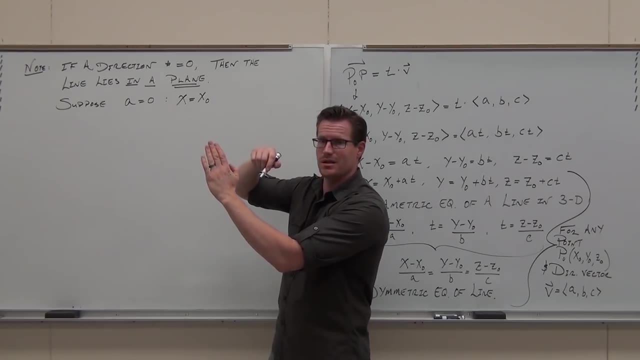 So if that's three, it's going to lie in that plane. Remember drawing planes. The plane would go through that x equal three or x sub zero, whatever that is, It's going to lie in that plane somewhere. It's actually kind of 2D. 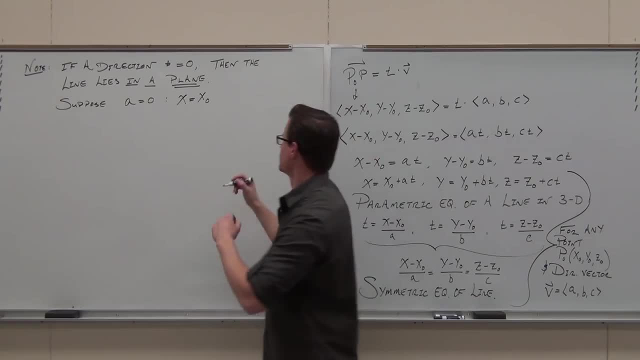 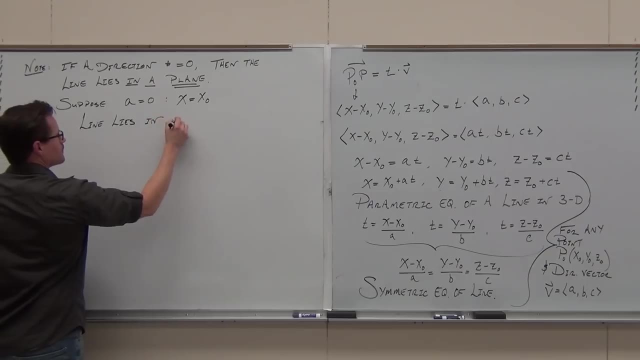 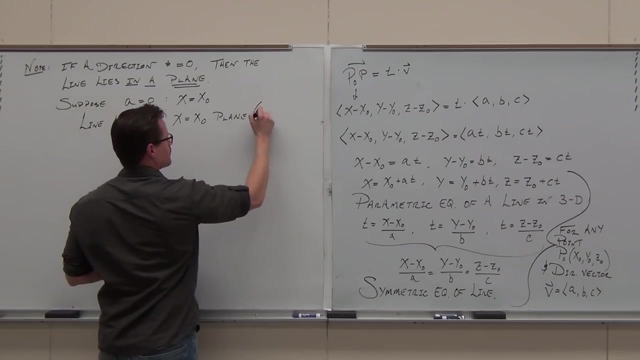 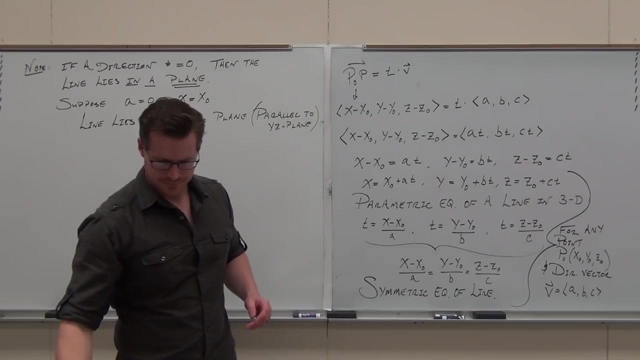 It'll be parallel to the yz plane. That's what would happen here. It's going to be a quantum plane and the competition is going to be one. It's going to be one. It's actually Spencer. It's going to be Spencer again. 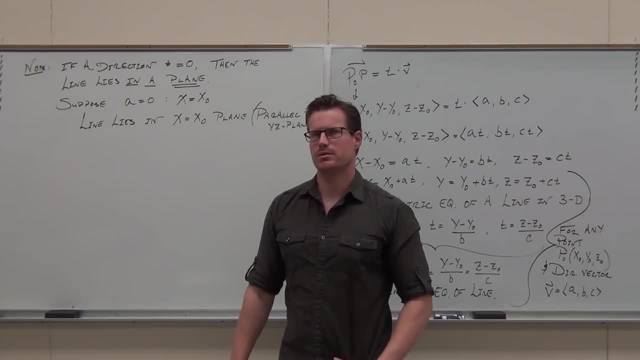 Never mind. Last little note: how would you tell? how would you tell two lines are parallel in 2D. Not a straight question. you should know this. They never cross, They never cross. okay, yeah, that's true. 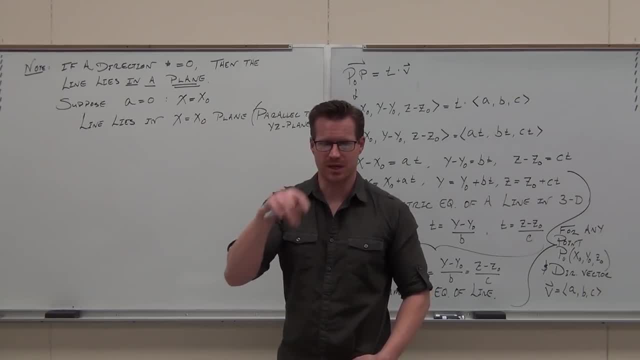 How do you tell if they're parallel though? Like really easy, you've got y equals m. How do you tell if the two lines are parallel? Same slope, Same slope. Do we have slope in 3D? Not yet, Not yet. 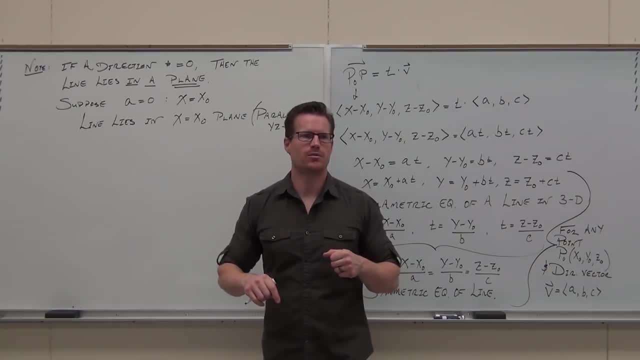 What do we have in 3D Perfect? How do you tell that two lines will be parallel in 3D? Same direction? Same direction, Same direction, same unit, vector or scalar multiples? If they're direction, vectors are scalar multiples. 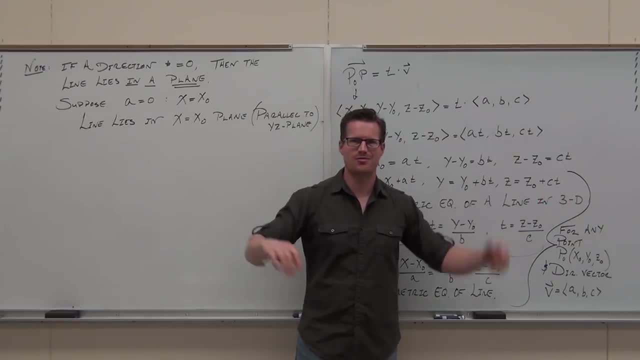 Just like we always check for parallel vectors. Remember, we're talking about parallel vectors, right? Same stuff, man. Look at the vector lines. Hey, if they're scalar multiples, the lines are parallel. Does that make sense to you? That's how we always check. 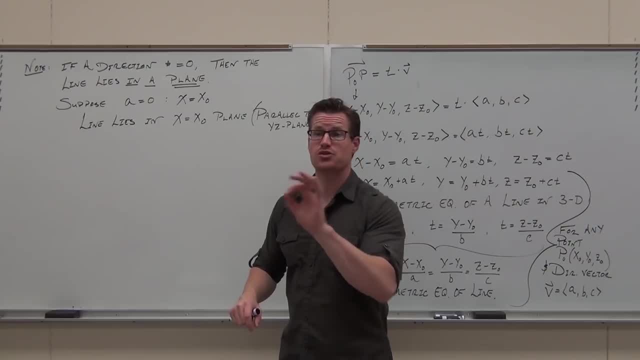 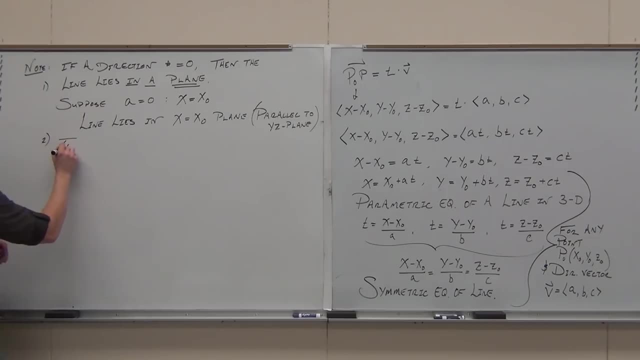 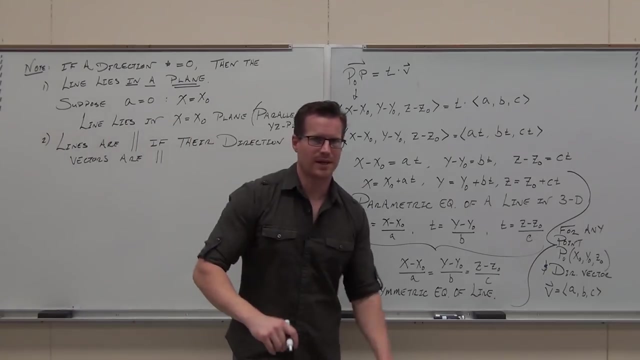 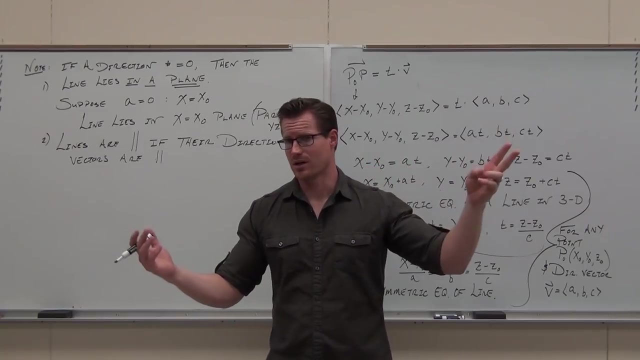 So two lines are parallel if their direction vectors are parallel. Okay, Lines are parallel If the direction vectors are parallel. Okay, now pop quiz. pop quiz notes. How do you tell when two vectors are parallel? Do you use a cross product? 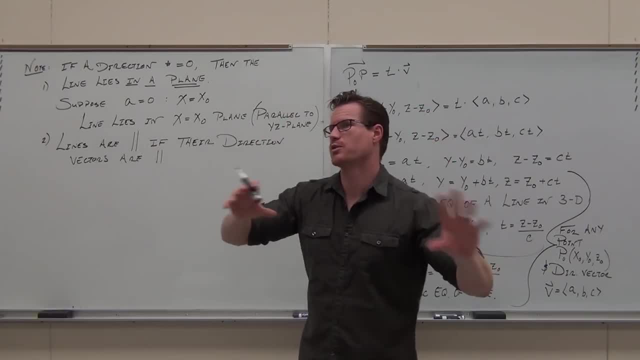 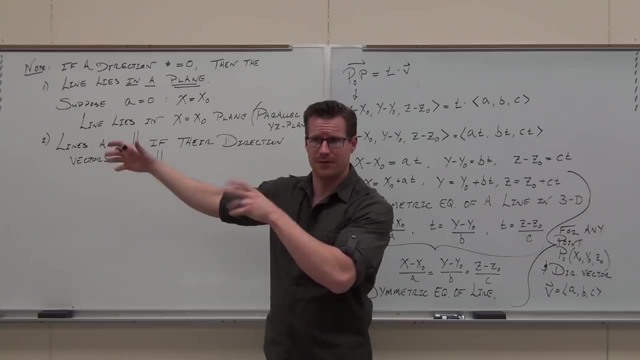 Do you find unit vectors or do you look for scalar multiples? Scalar multiples, Because that's so freaking fast. Okay, do that. So what this means is: hey, yeah, two lines are parallel If the direction vectors of those lines are scalar multiples. that makes a parallel. 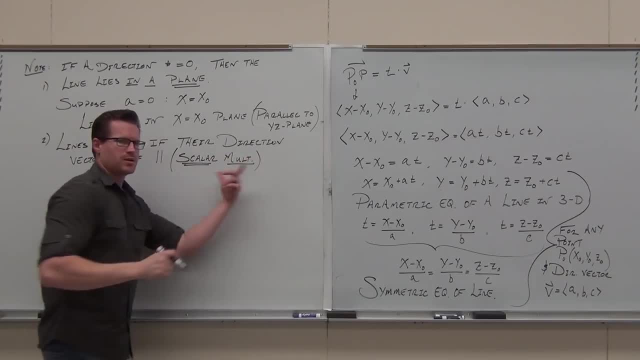 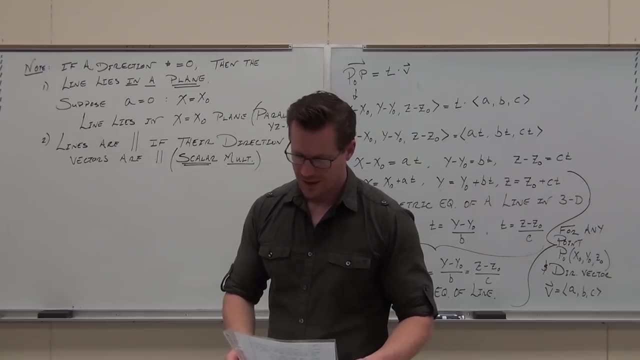 This should be the only thing in the world you ever do: to figure out whether two vectors are parallel. Look for scalar multiples, because it's fast, It's really nice. Now we're ready, man. Now we're ready to go. We've talked about a lot of stuff. 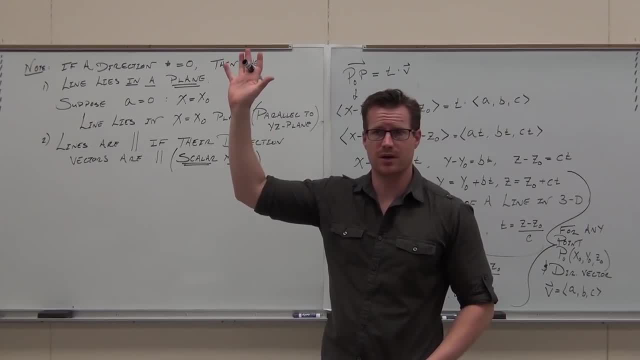 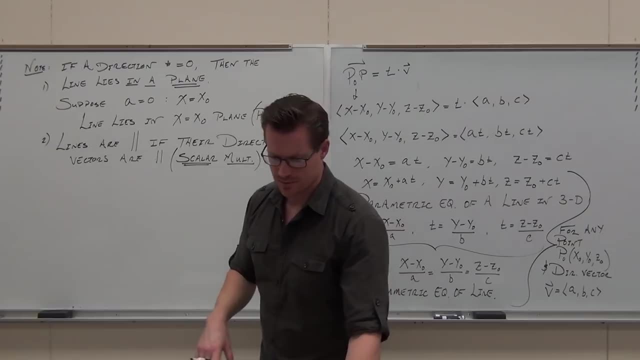 I need to make sure it makes absolute sense. Show if you feel okay with what we've talked about Now. I know it's very. hopefully it's not vague, but it's not concrete yet because we haven't done much. Well, let's start that right now. 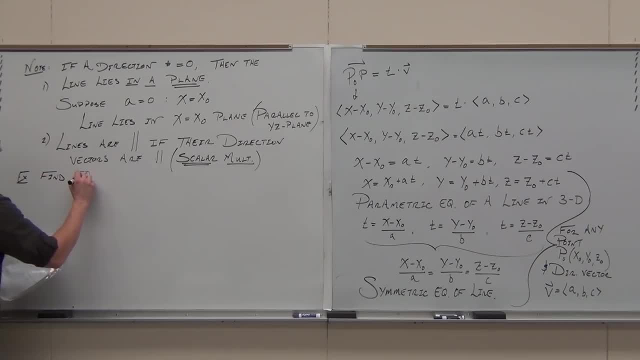 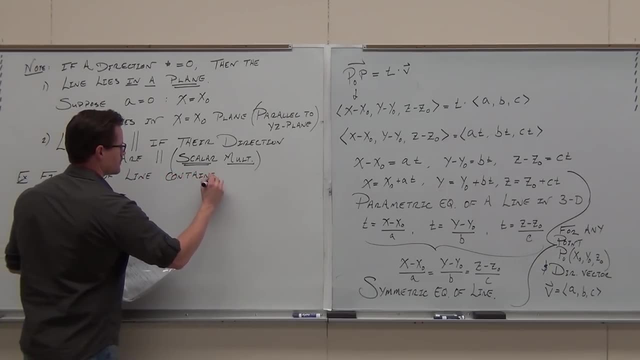 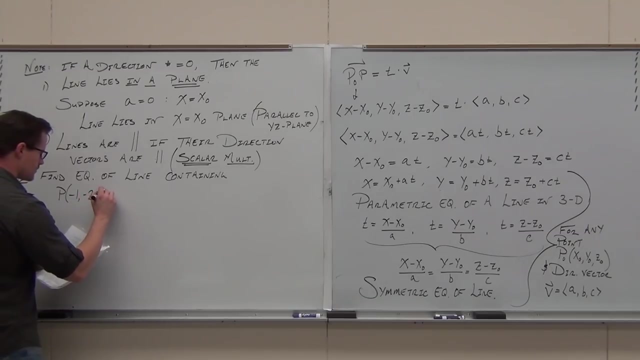 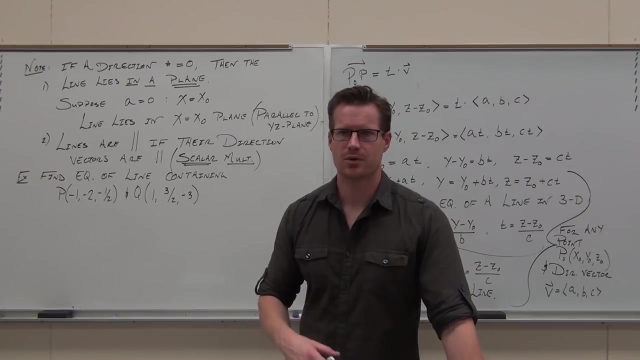 Please don't zone out as I'm going through these examples, because you're going to get stuck. Okay, All right, Because like halfway through a lot of these examples, I start teaching you other things, like: oh, here's a note. 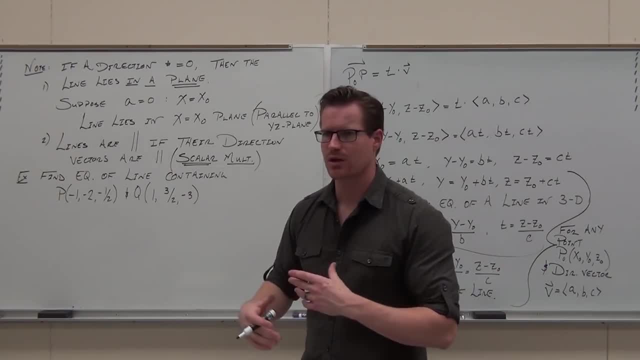 Watch what happens, all right. So if we just kind of gloss this over, you're going to miss some things. So please stick with me here. Number one thing you all need to know: what do you need in order to find the equation of line in 3D? 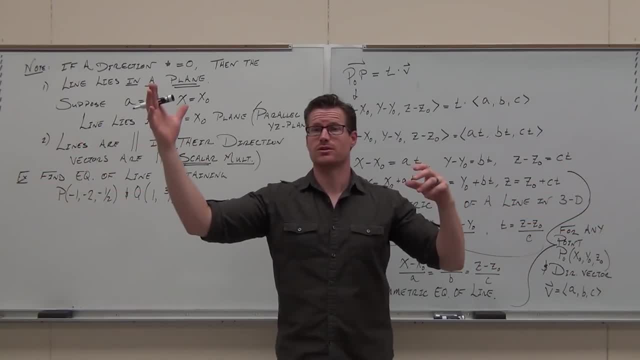 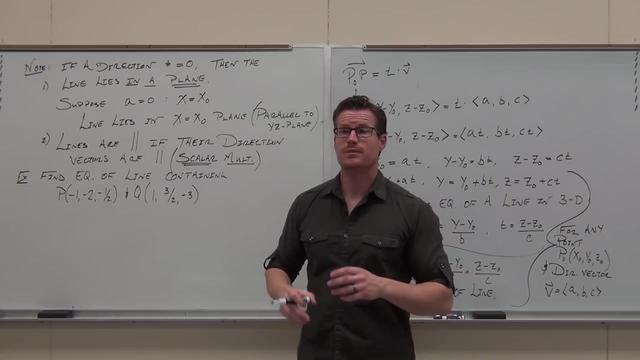 What do you need? Point Point and a vector Point and a vector Point and direction vector. Do we have a point? Yes, In fact we have two points. Pick one, It doesn't matter which one. Do we have a vector? 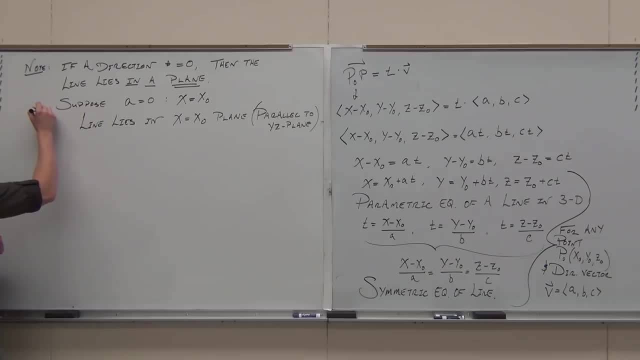 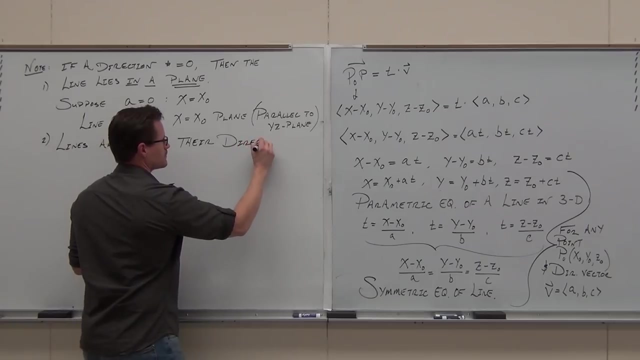 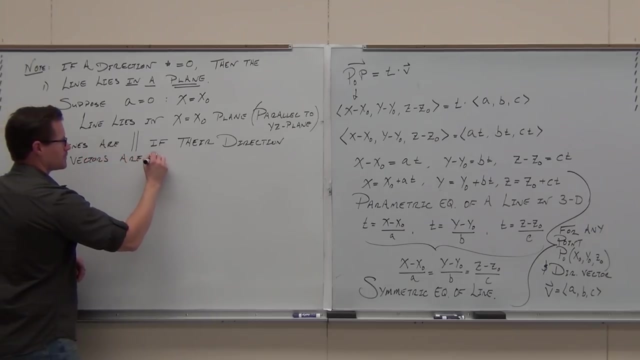 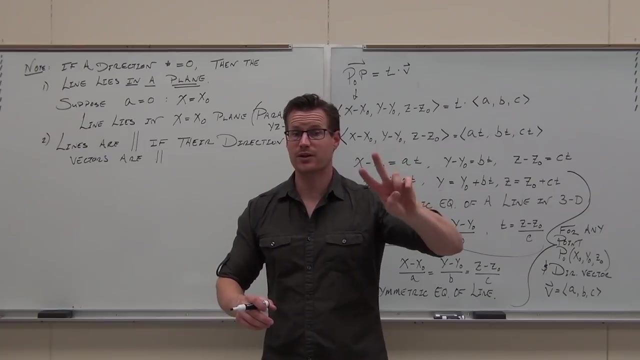 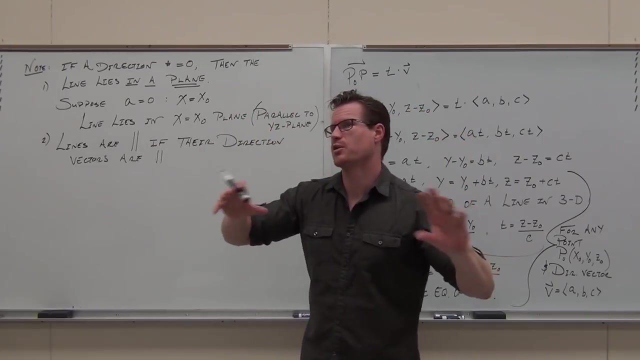 are parallel. Lines are parallel if their direction, vectors are parallel. Okay now, pop quiz, pop quiz, nose. How do you tell when two vectors are parallel? Do you use a cross product, Do you find unit vectors or do you look for scalar multiples? 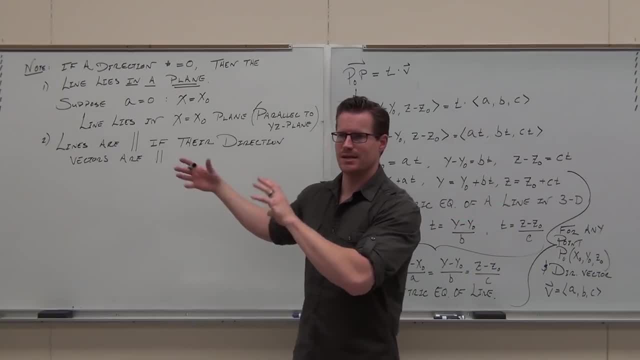 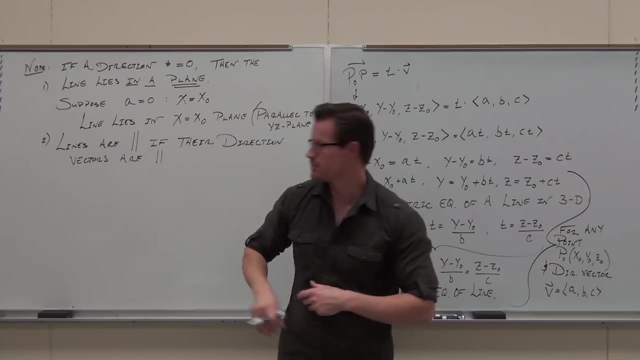 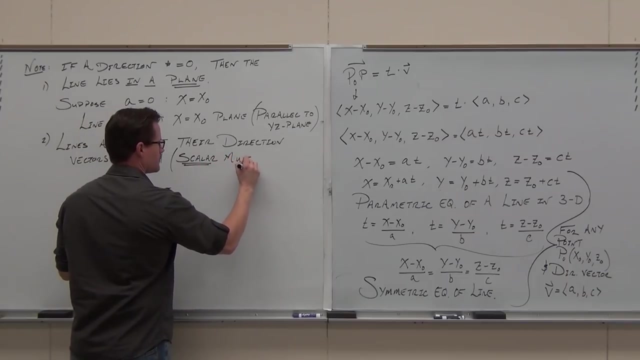 Scalar multiples, Because that's so freaking fast. Okay, do that. So what this means is: hey, yeah, two lines are parallel If the direction vectors of those lines are scalar multiples. that makes it parallel. This should be the only thing in the world you ever do to figure. 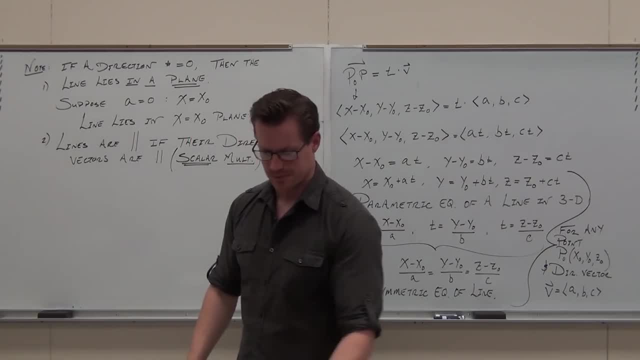 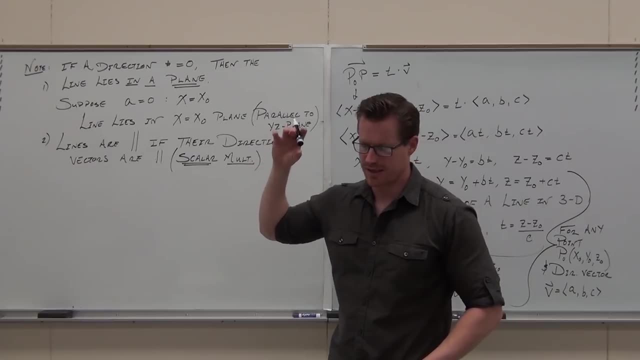 out whether two vectors are parallel. Look for scalar multiples, because it's fast, It's really nice. Now we're ready, man. Now we're ready to go. We've talked about a lot of stuff. I need to make sure it makes absolute sense. 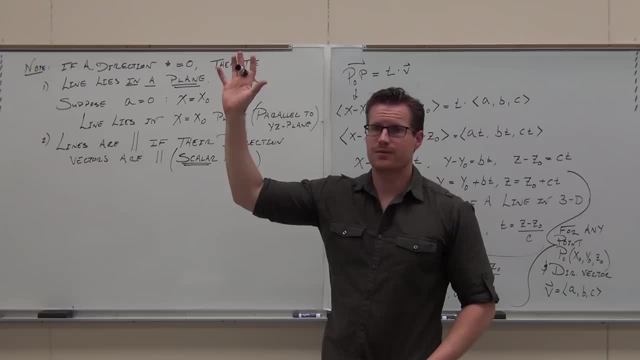 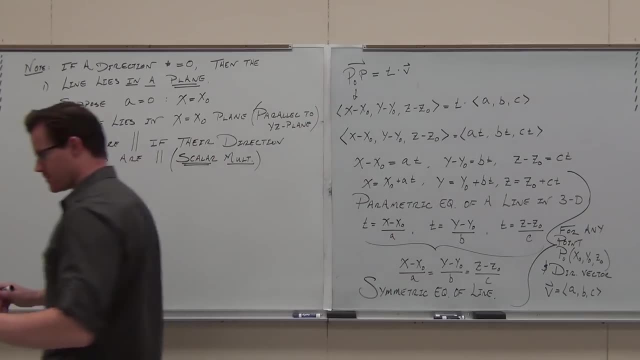 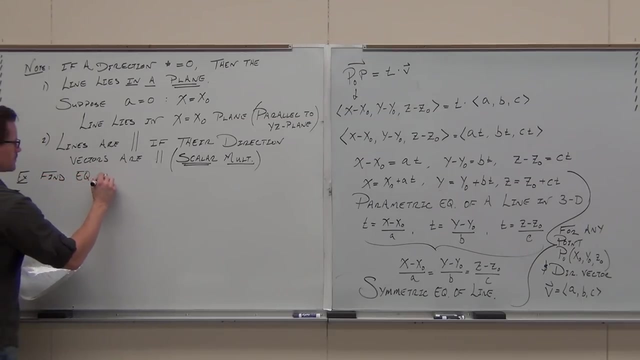 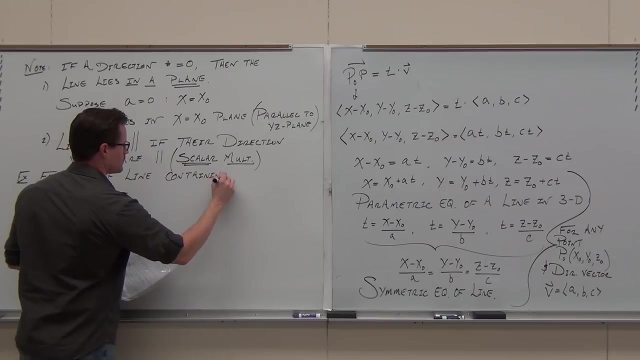 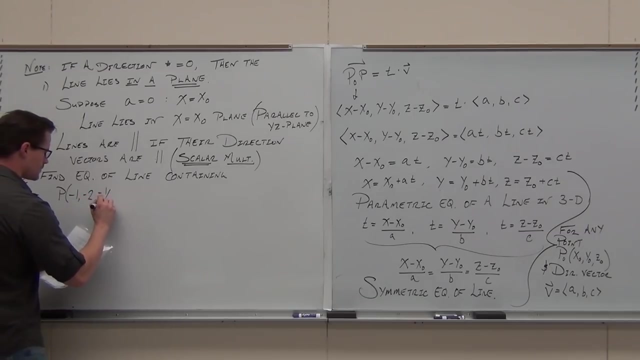 Show up hands if you feel okay with what we've talked about Now. I know it's very, hopefully it's not vague, but it's not concrete yet because we haven't done much. Let's start that right now. Please don't zone out as I'm going through these examples, because like halfway through a lot. 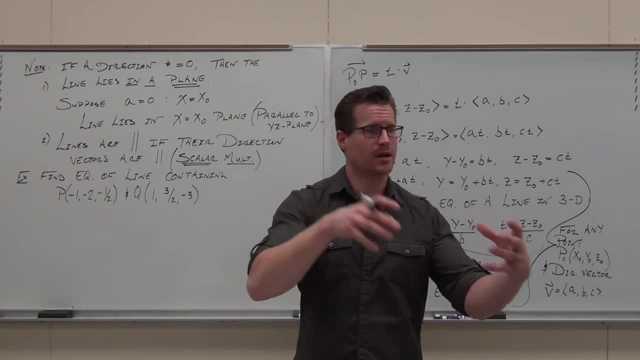 of these examples, I start teaching you other things like: oh, here's a note, Watch what happens, all right. So if we just kind of gloss this over, You're going to get it. You're going to get it, You're going to get it. 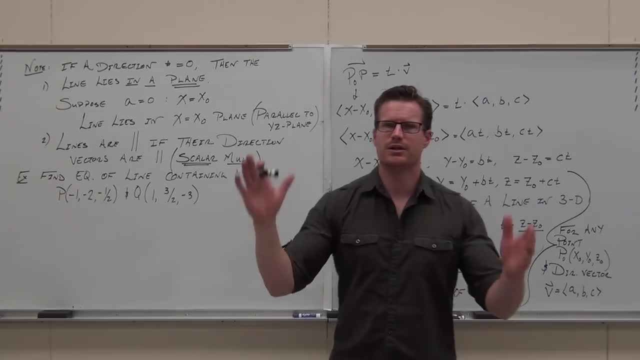 You're going to miss some things, so please stick with me here. Number one thing you all need to know: what do you need in order to find the equation of line in 3D? What do you need? A point and a vector. 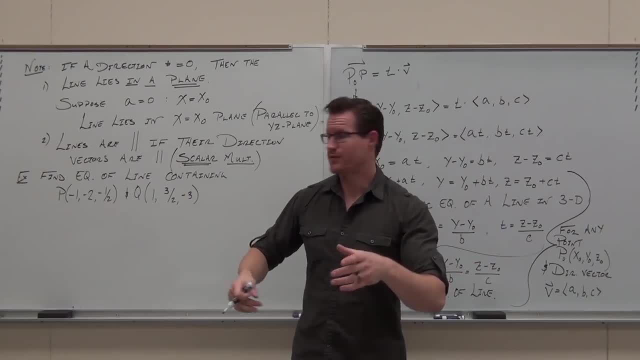 Point and a vector. Point and direction vector. Do we have a point? Yes, In fact, we have two points. Pick one, It doesn't matter which one. Do we have a vector? No, How do we find a vector? 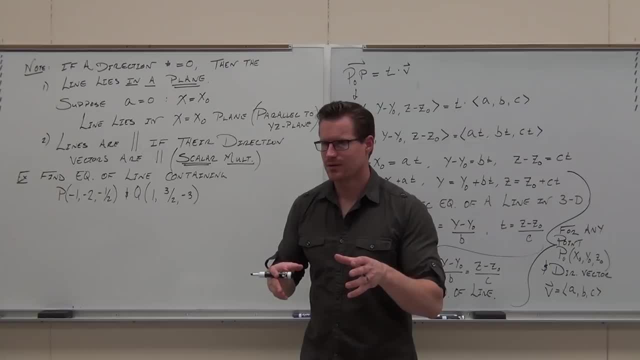 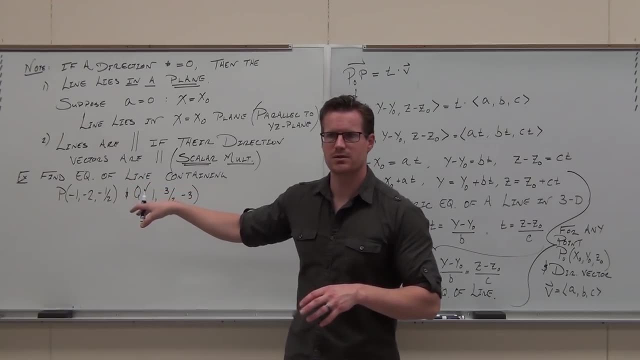 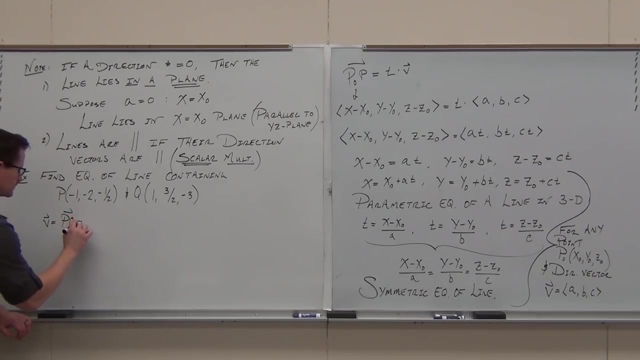 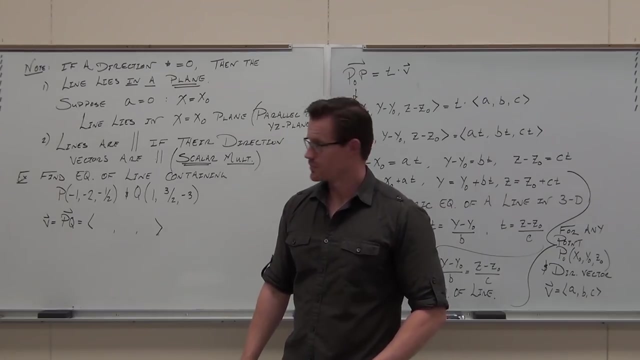 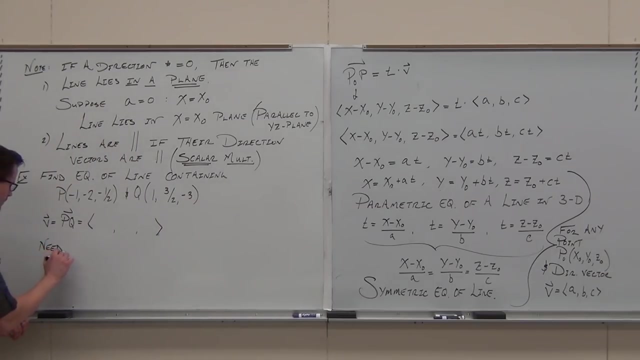 No, How do we find a vector? Just like we need two points to find a slope, we need two points to find a vector. Same stuff. Let's find the vector between p- cube. Go ahead and do that, All right. Did you find the direction vector for this line? 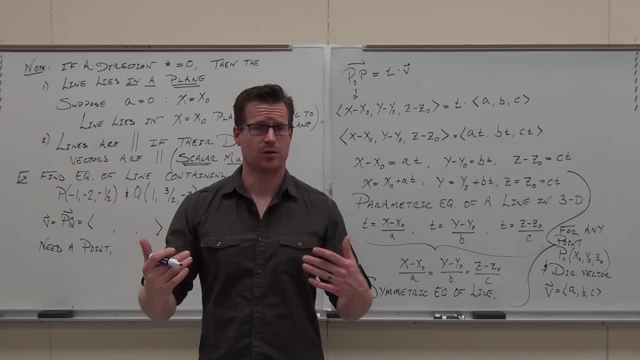 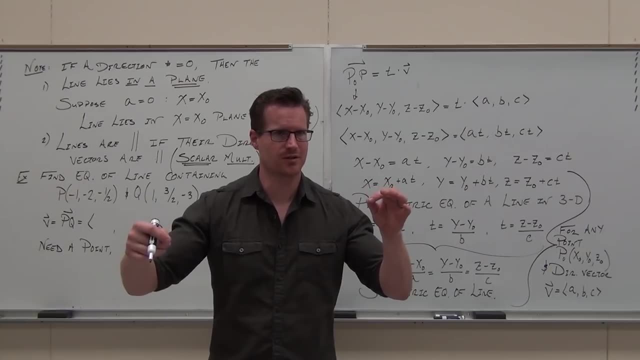 If you're like, wait a minute, that's a position vector. Yeah, that's the whole point. That's why we're taking this position vector and multiplying it by a scalar, because we never find a vector between two points. It's automatically a position vector. 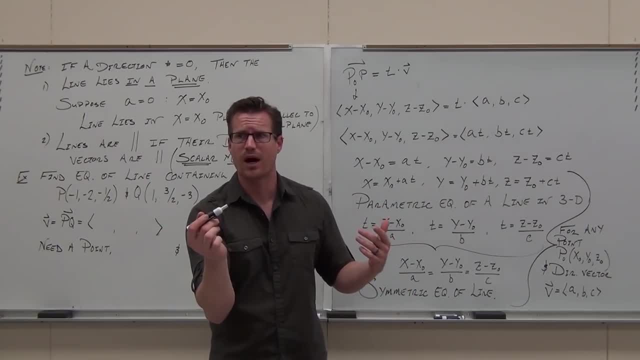 That's why the picture was relevant earlier. It said: yeah, you've got this vector starting at the origin. Why? Because every time we find a vector, it moves it there, And then we have to have that scalar multiple to move it through the point. 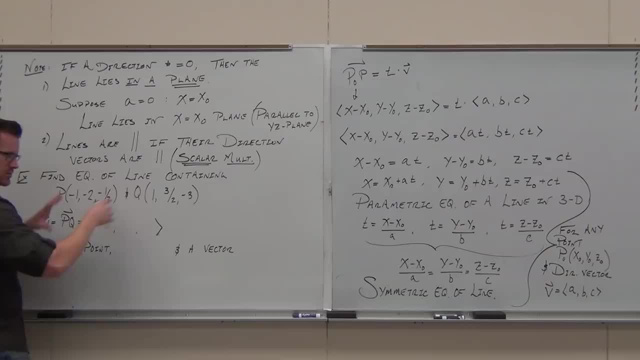 That's the plan here. So when you did this, how much did you get? Two, Two, Seven, Seven Negative five, Negative five. I'm going to believe you. Can I get a triple check on that though? Perfect. 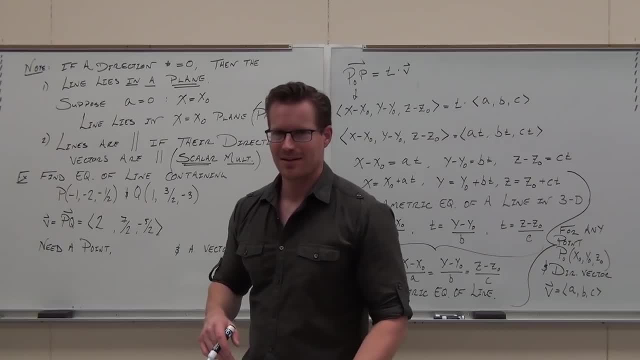 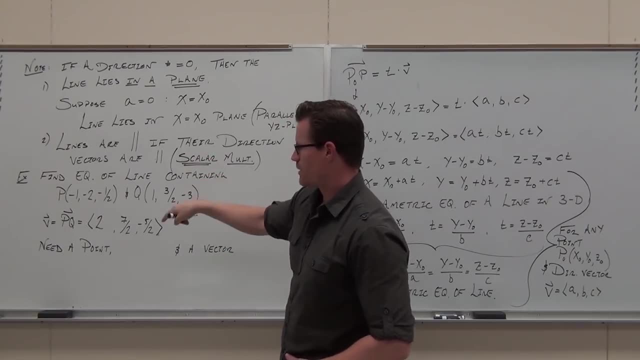 All right, See how much I believed you. Just kidding, Just kidding, It just happens, you know. Oh, So to find the equation of a line, we need a point vector. What point are you going to use? It doesn't matter. 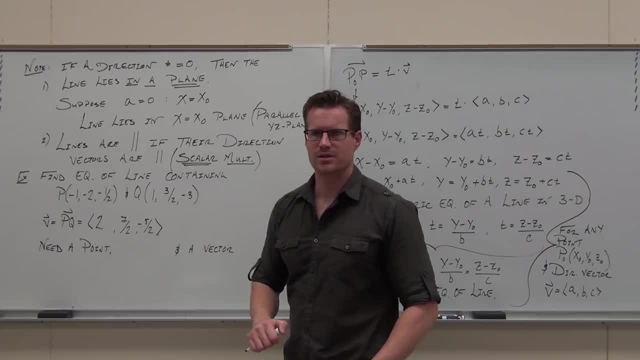 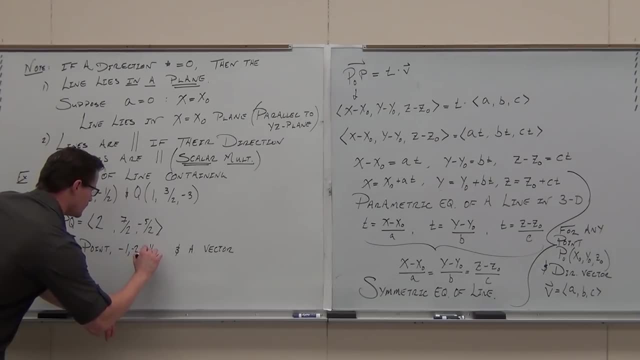 Pick one, It doesn't matter. Let's pick P, just so we all have the same thing in our notes here. Let's pick P. So I'll pick a point. And we need a vector. We already got one. We have it right now. 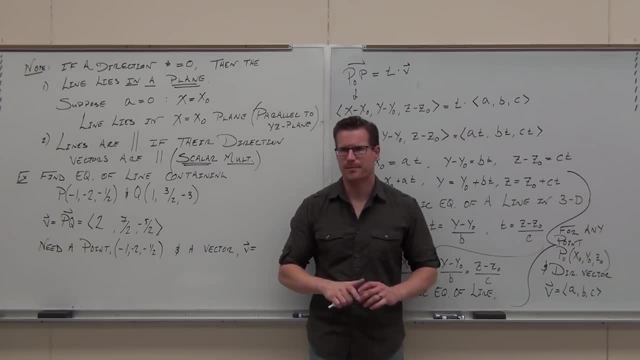 Oh, but wait a second. I want you to think this is one of those little things. OK, One of the little things I'm going to teach you right here. Don't write anything down, Change it. You guys agree with the idea we need a point and a vector. 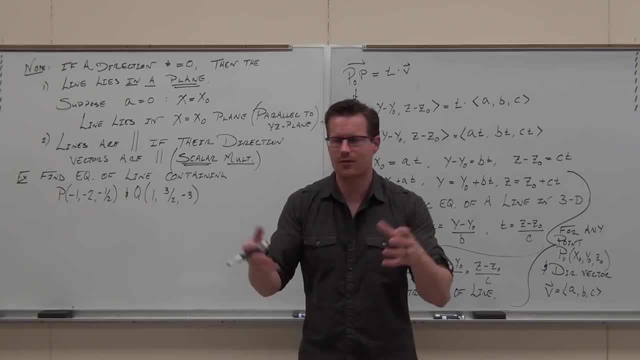 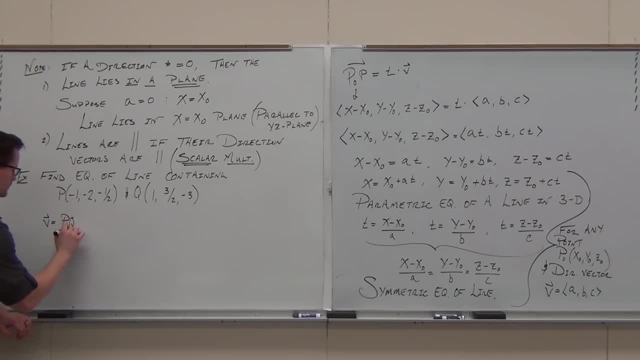 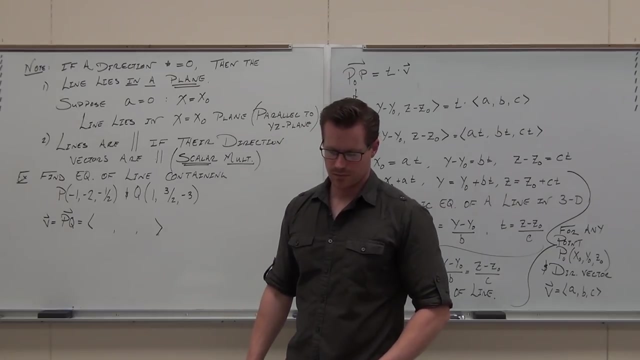 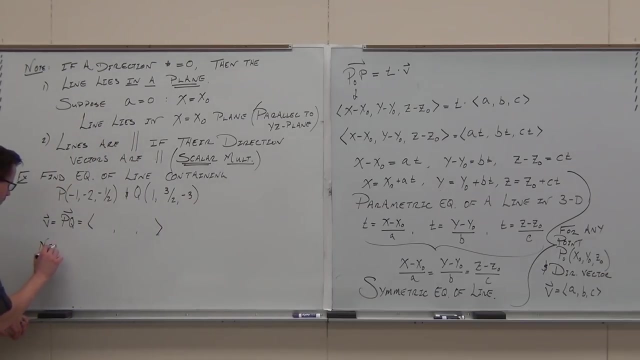 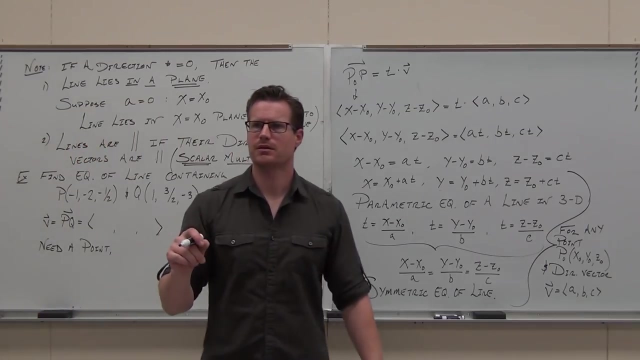 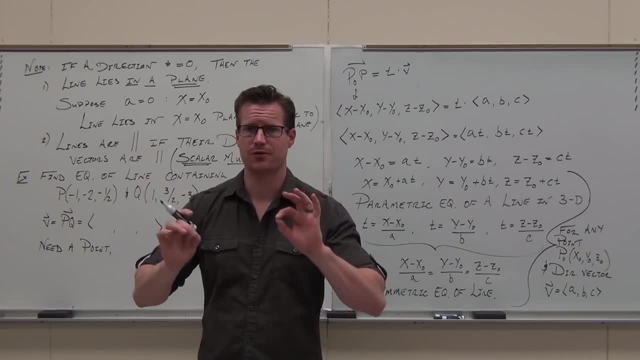 That's why we're taking this position vector and multiplying it by a scalar, because we never find a vector between two points. It's automatically a position vector. That's why the picture was relevant earlier. It said: yeah, you've got this vector starting at the origin. 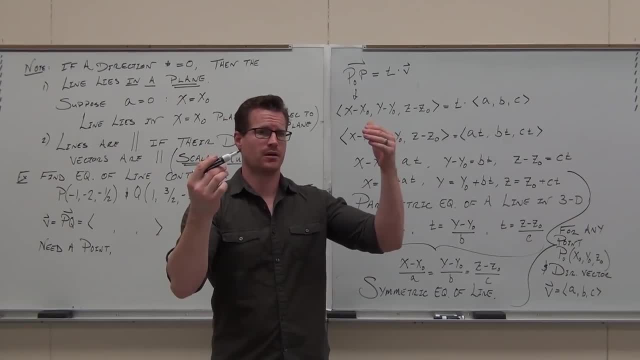 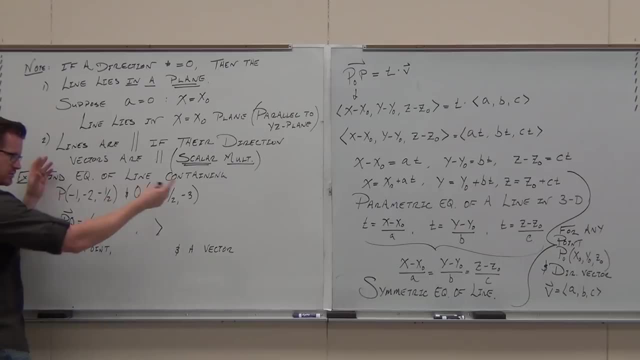 Why? Because every time we find a vector, it moves it there, And then we have to have that scalar multiple to move it there, And then we have to move it through the point. That's the plan here. So when you did this, how much did you get? 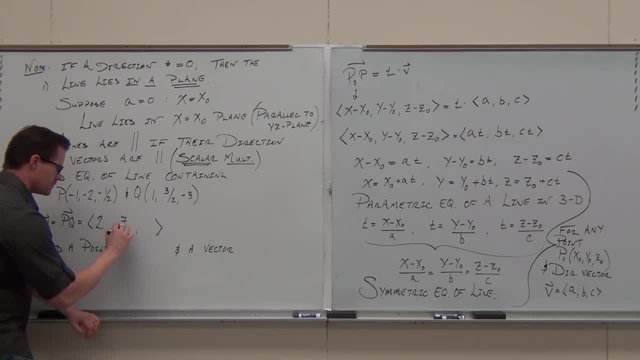 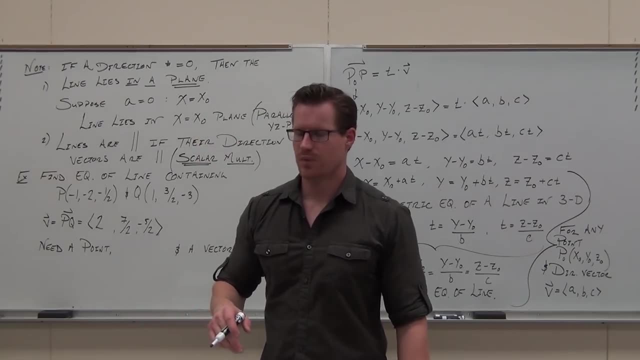 Two, Two, Seven, Seven, Seven Negative five, Negative five. I'm going to believe you. Can I get a triple check on that though? Perfect, All right, See how much I believed you. Just kidding, Just kidding. 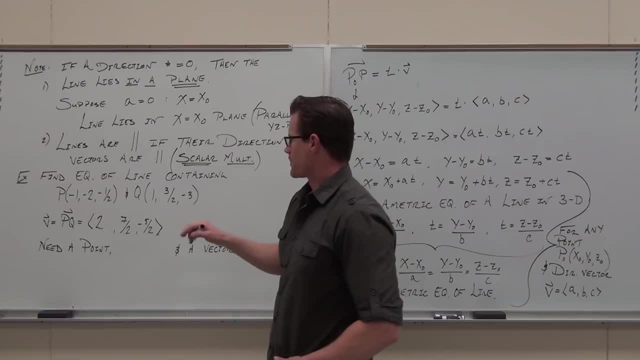 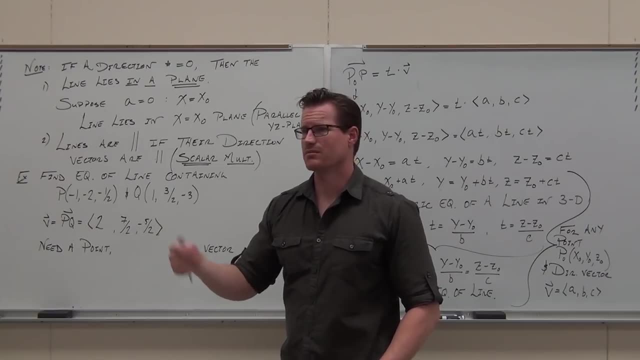 It just happens, you know. Oh, So to find the equation of a line, we need a point. What point are you going to use? It doesn't matter, Pick one, It doesn't matter, Let's pick P, just so we all have the same thing. 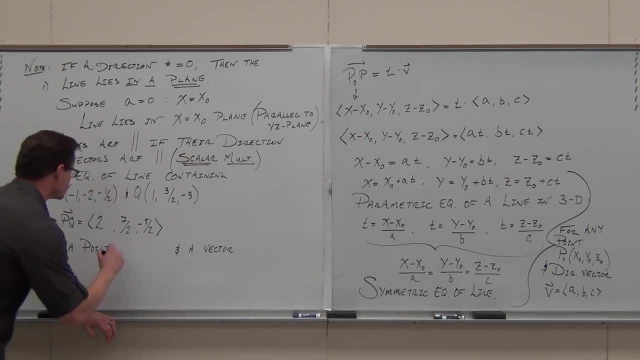 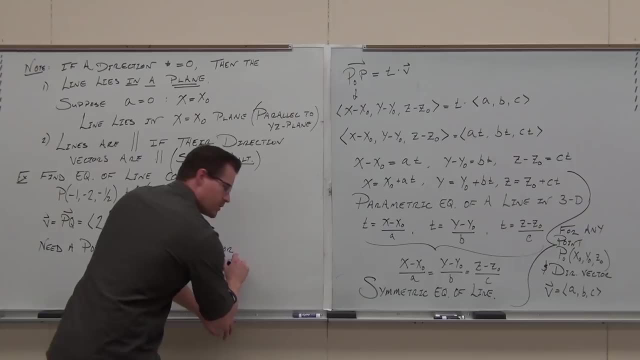 in our notes here, Let's pick P. So I'll pick a point. And we need a vector. We already got one. We have it right now. Oh, but wait a second. I want you to think this is one of those little things, OK. 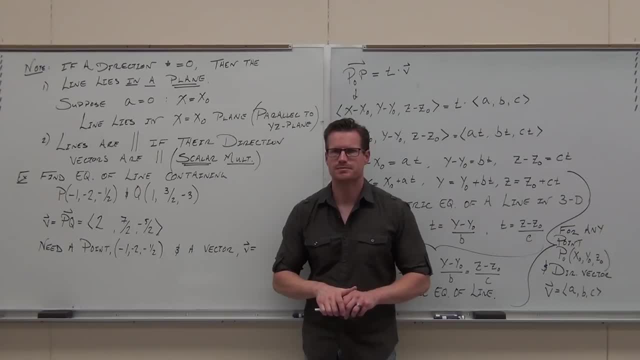 One of the little things I'm going to teach you right here. Don't write anything down, Change it All. right, You guys agree with the idea. we need a point and a vector. We got a point. We need a vector. We have a vector. 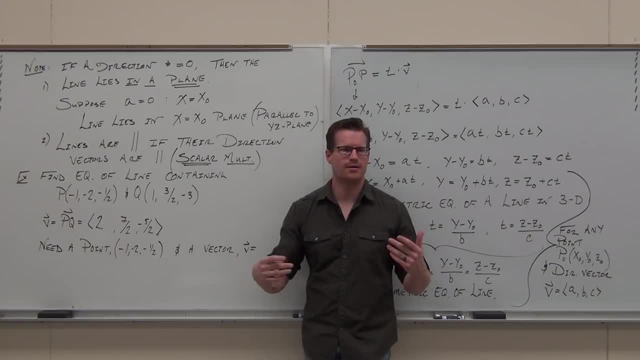 You can use that vector. But here's the whole point about that vector: It doesn't have to be a unit vector, It doesn't even have to be the vector you find right there. It just has to be the vector in the same direction. 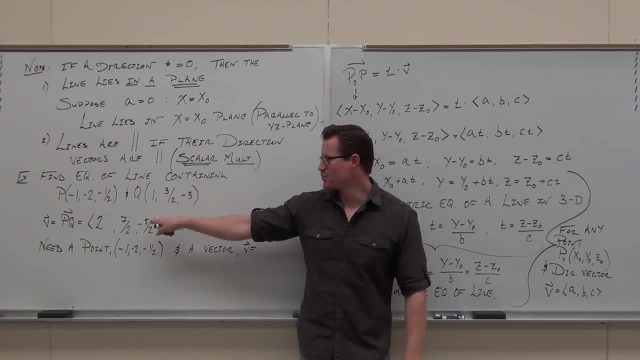 So make it nice on yourself. If you've got like those one-halves, here you go. no, I don't, that's silly. We can multiply any vector. Okay, scalar multiple- that's a number- And get a vector in the same direction, right. 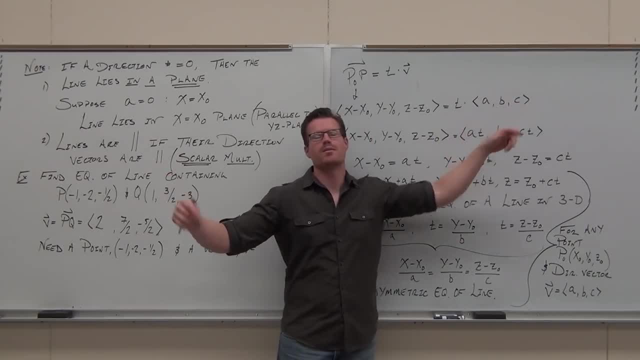 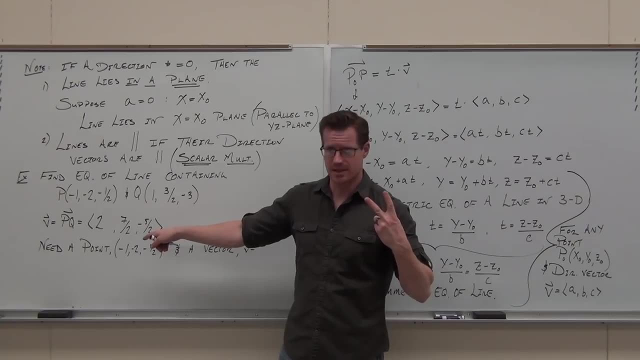 All this thing says it's in the direction we want. Multiply by whatever you want. I would multiply all this stuff by 2.. Is it going to be in the same direction? Yes. Is it going to be the same vector? No, Who cares. 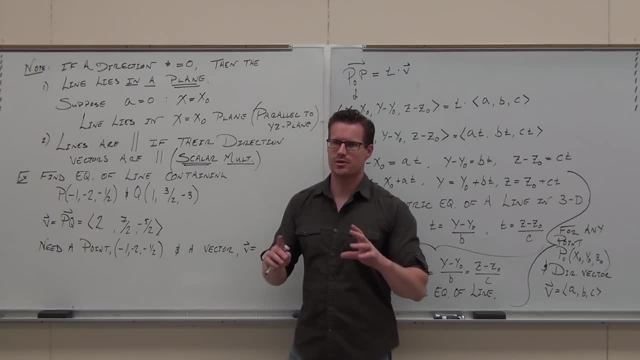 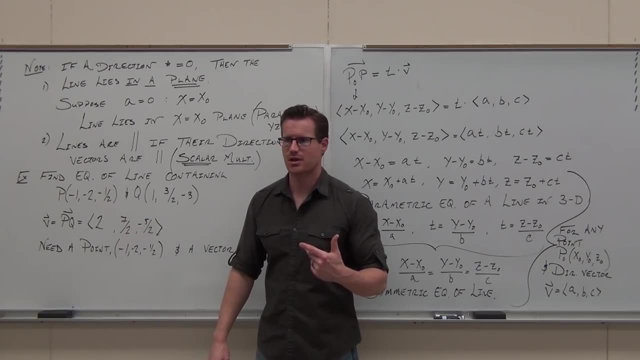 It's in the same direction. It's just a direction vector. So long story made short. if you have fractions, oh goodness, multiply by the LCD of your fractions. That's nice. okay, It gets rid of fractions If you have huge, huge vector numbers here. 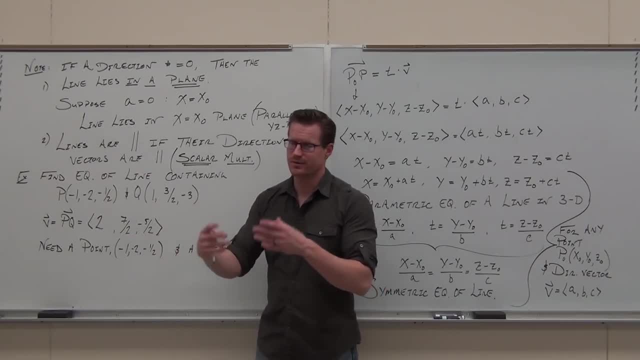 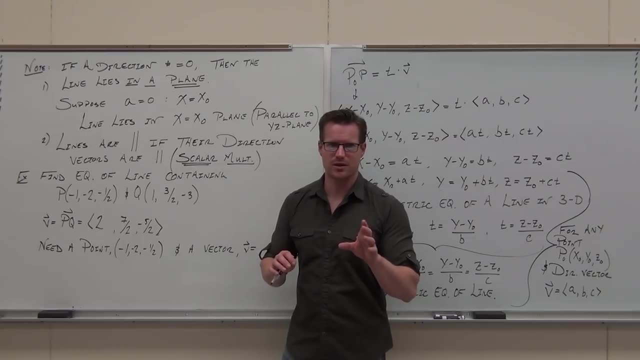 huge direction numbers. you can divide them all by a common denominator or, sorry, greatest common factor. You can change the sign, You multiply the negatives, You can basically do whatever you want. Please, please, make this mental note. I know some of you guys are writing, but stop. 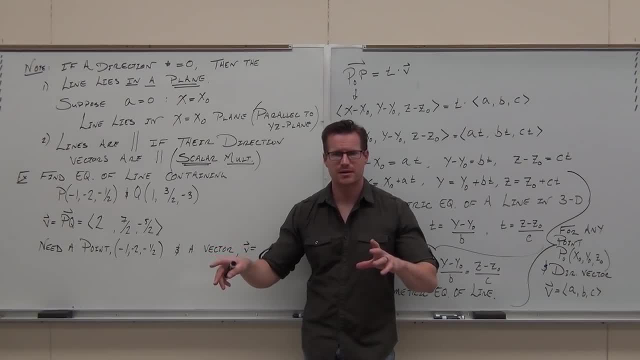 We got a point, We need a vector. We have a vector, You can use that vector. But here's the whole point about that vector: It doesn't have to be a unit vector, It doesn't even have to be the vector you find right there. 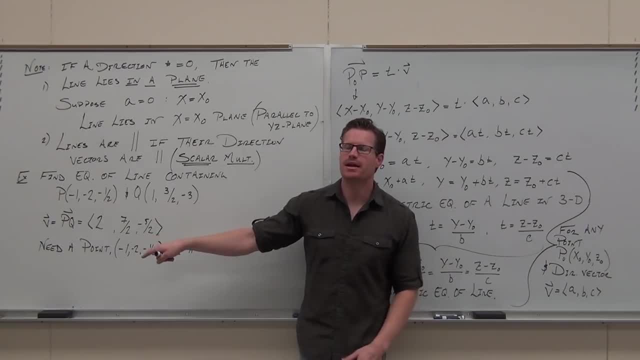 It just has to be the vector in the same direction. So make it nice on yourself. If you've got like those one-halves, here you go. no, I don't. that's silly. We can multiply any vector by a scalar multiple. that's a number. 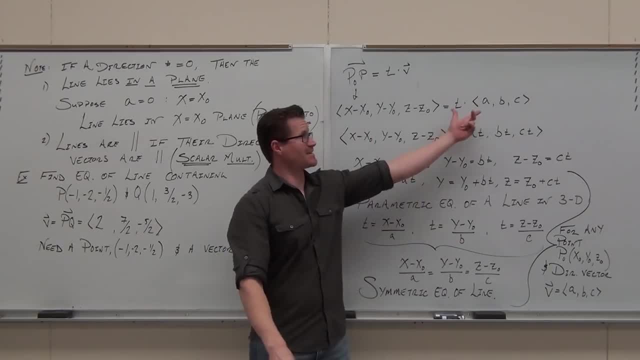 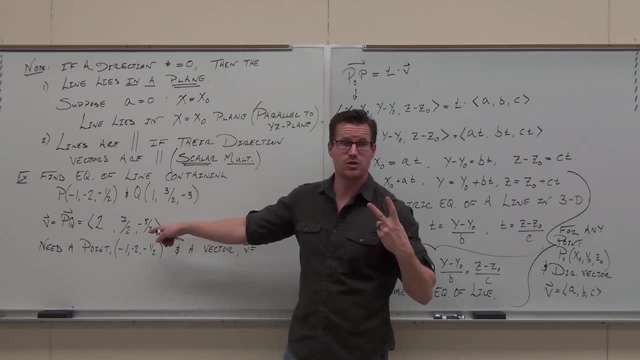 and get a vector in the same direction. right, All this thing says it's in the direction we want. Multiply by whatever you want. I would multiply all this stuff by 2.. Is it going to be in the same direction? Yes, Is it going to be the same vector? 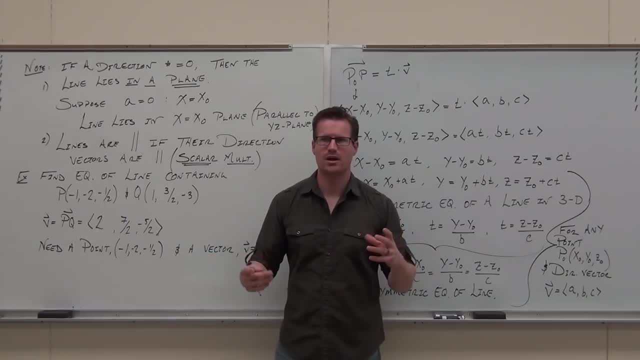 No, Who cares, It's in the same direction, It's just a direction vector. So long story made short. if you have fractions, oh goodness, multiply by the LCD of your fractions. That's nice. okay, It gets rid of fractions. 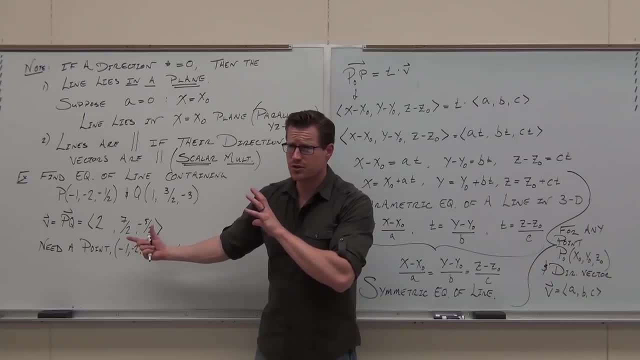 If you have huge, huge vector numbers here, huge direction numbers, you can divide them all by a common denominator or, sorry, greatest common factor. You can change the sign, You multiply the negatives. You can basically do whatever you want. Please, please, make this mental note. 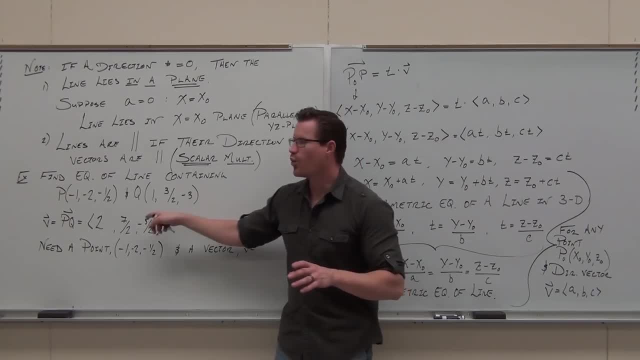 I know some of you guys are writing: but stop, You can't always do this unless you are talking about distances, Because distance is built into these numbers. okay, So as soon as we start talking about distances, can we do this junk? 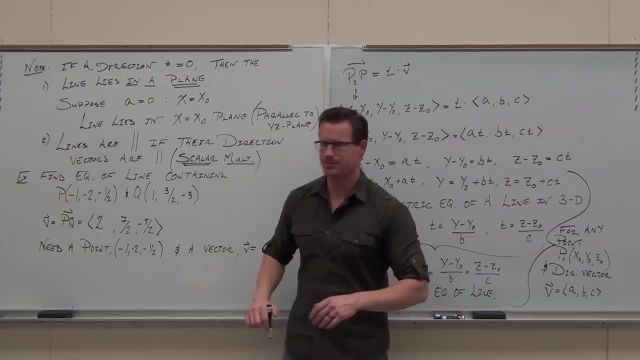 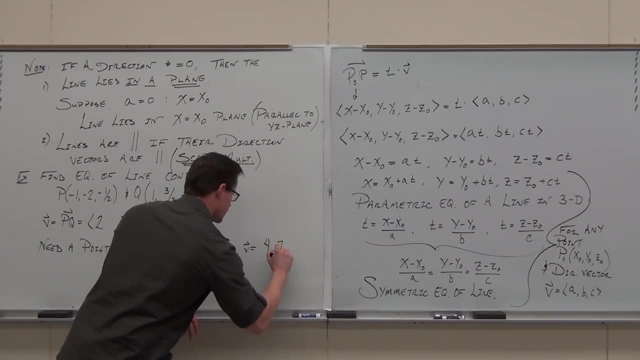 No, But if we're not, if we're just talking about direction, go for it. So I would for sure multiply this by 2 and change my vector. Now, what's easier, That's easier, That's a lot easier. 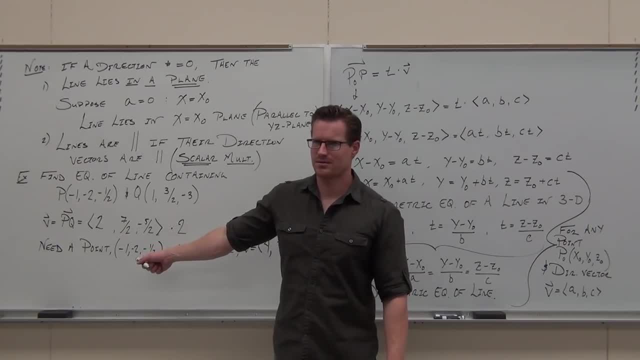 How about this one? Can I do that to the point? No, because the point is the actual spot in space. Okay, You can't do. unfortunately you can't do that, But you can do this with a vector. So modify your vectors, as long as you keep the same direction. 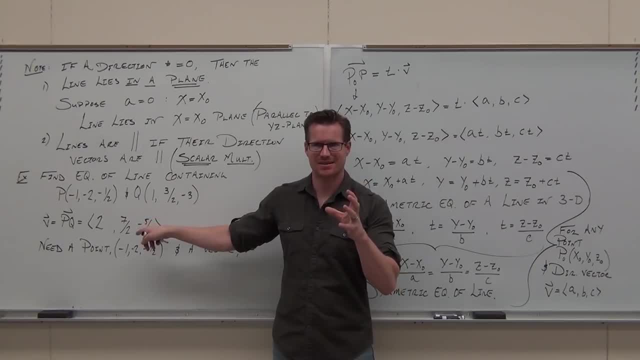 You can't always do this, unless you are talking about distances, Because distance is built into these numbers, okay, So stop. As soon as we start talking about distances, can we do this junk? No, But if we're not, if we're just talking about direction, go for it. 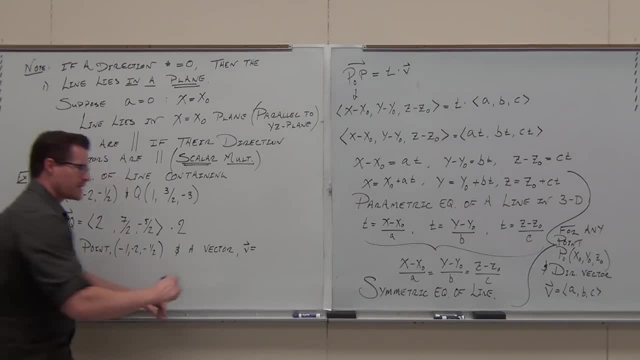 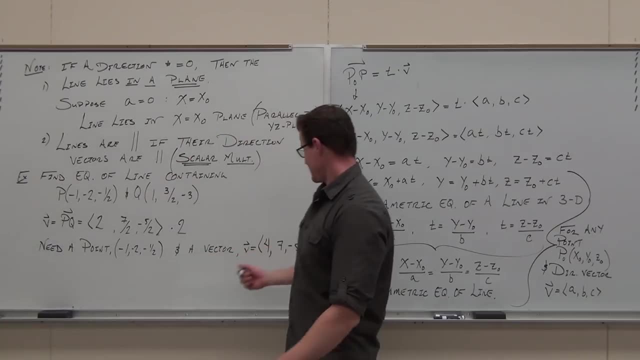 So I would for sure multiply this by 2 and change my vector. Now, what's easier? That's easier, That's a lot easier. How about this one? Can I do that to the point? No, because the point is the actual spot in space. 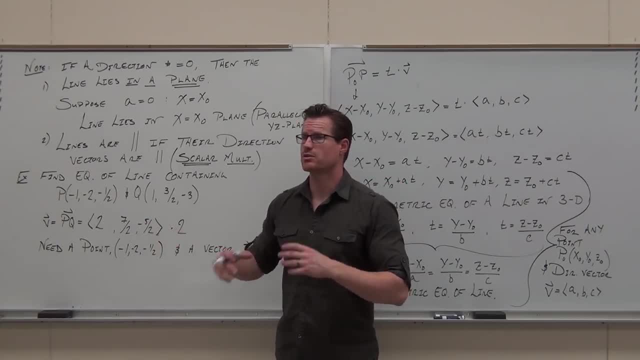 Okay, You can't do, unfortunately you can't do that, But you can do this. You can do this with a vector. So modify your vectors as long as you keep the same direction. And that means multiply by whatever number you want. 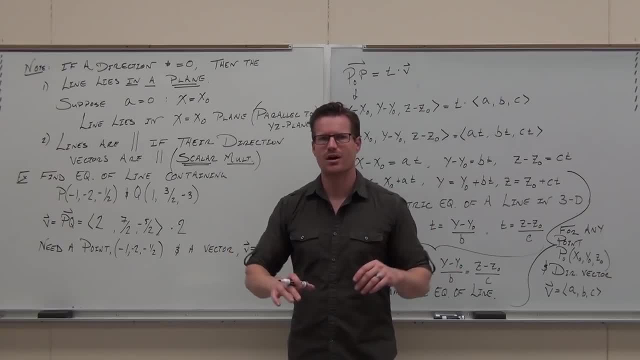 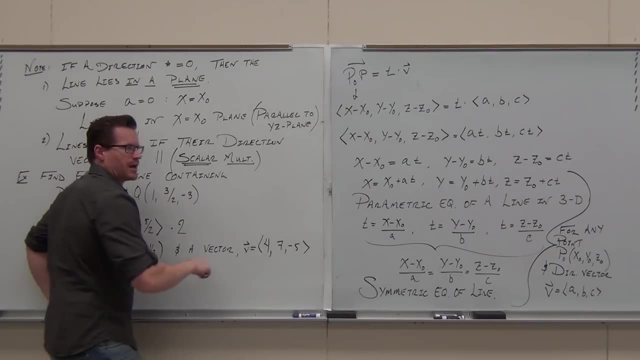 And that means multiply by whatever number you want, as long as it's a scalar, and you're good to go, Should fans feel okay with that one. Now I want to see if we can do this together. I'm going to write the equation of y. I'm going to start. 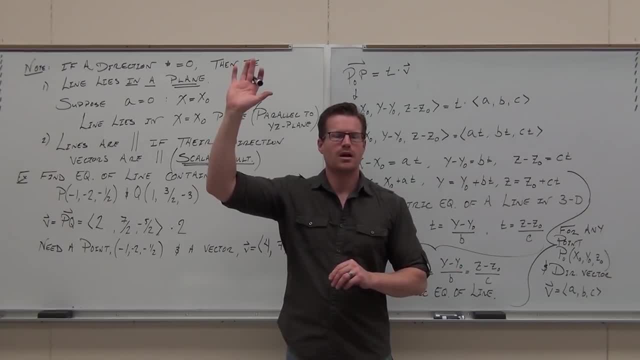 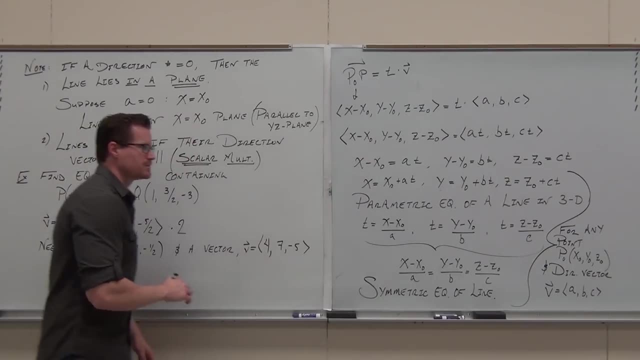 as long as it's a scalar and you're good to go, Should fans feel okay with that one. Now I want to see if we can do this together. I'm going to write the equation of line. I'm going to start with a parametric equation. 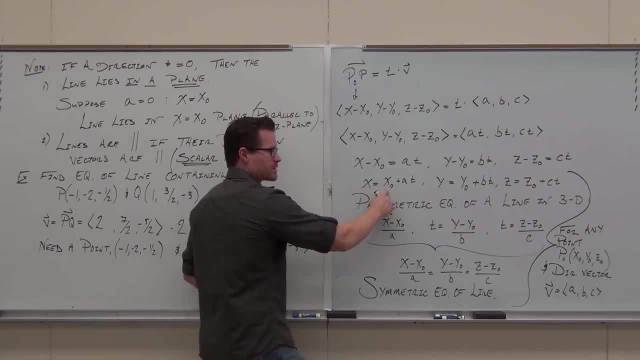 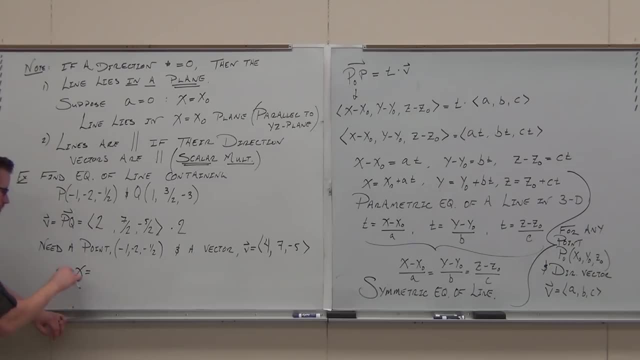 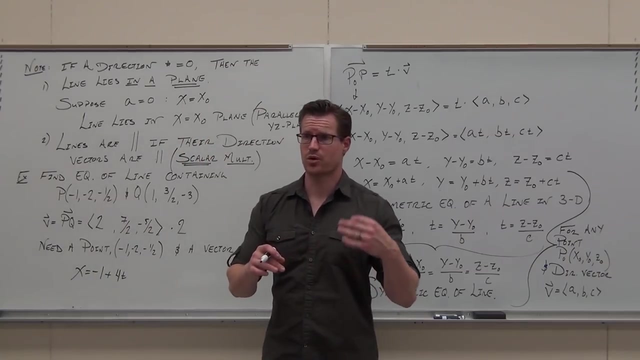 Literally all you do literally. put your x, y and z coordinates, put your direction numbers in the appropriate order. We need a x coordinate, a direction number and a parameter. That right there is the little equation for how the x coordinates work. 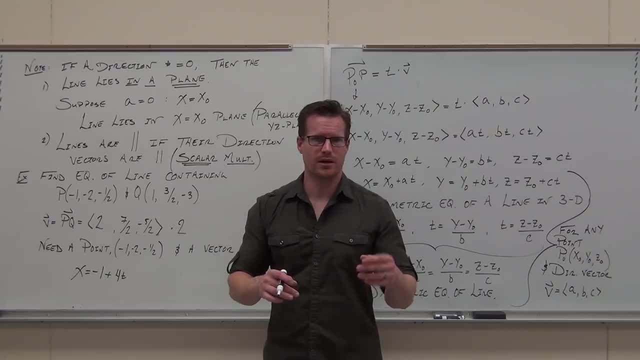 for any point on this line. That's pretty awesome. So say, you want to find an x coordinate for any points, plug in t, plug in all the values of t that you want, and you find these points in line. Well, at least x coordinates right now. 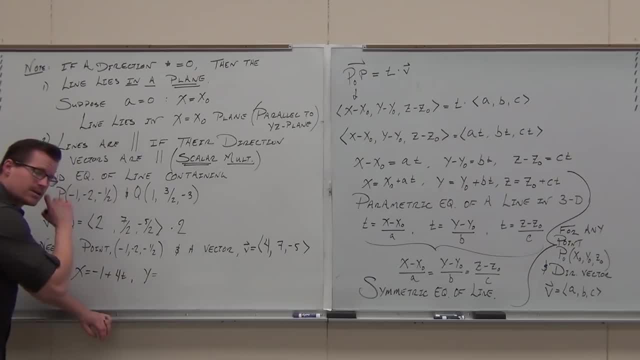 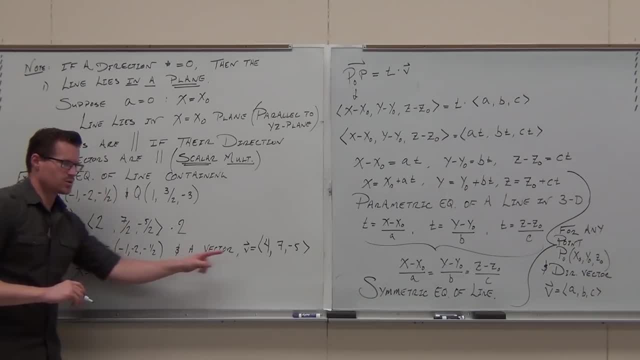 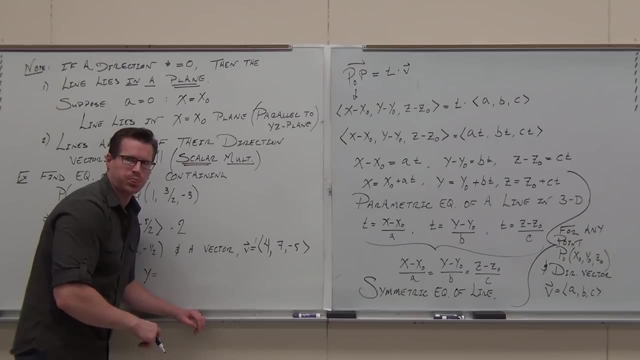 There you go. Do you understand how easy it is to get confused between these two numbers right now? Yeah, Especially if you're the one who likes to put commas for your vectors. That's why we have these things saying this is a vector. 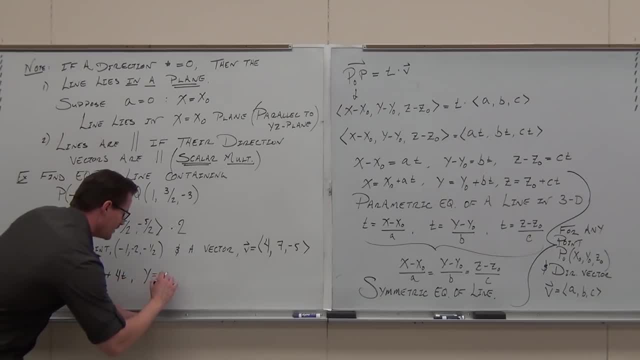 That's a point. You get the point. What's the next thing? Hopefully it's plus. It's going to be plus. We're going to use the sine appropriately. So on this, right here we have literal x, y and z coordinates. 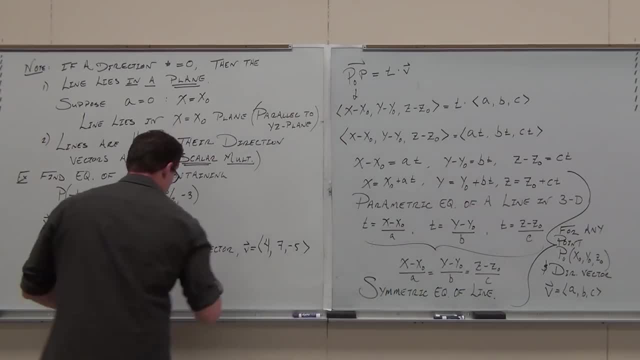 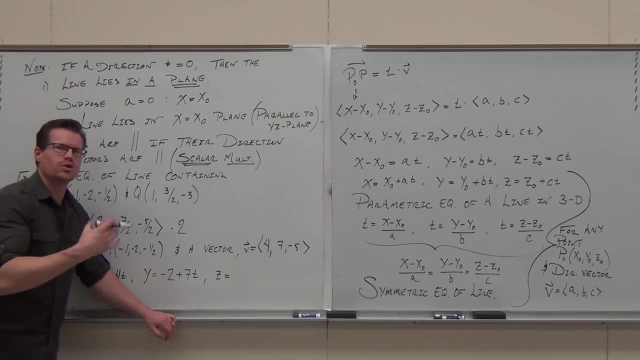 We have literal x, y and z components of the direction vector. Let's watch the z real careful Left-siders, you guys. what's the z coordinate of our point? What do we write first? Plus sine, minus sine. 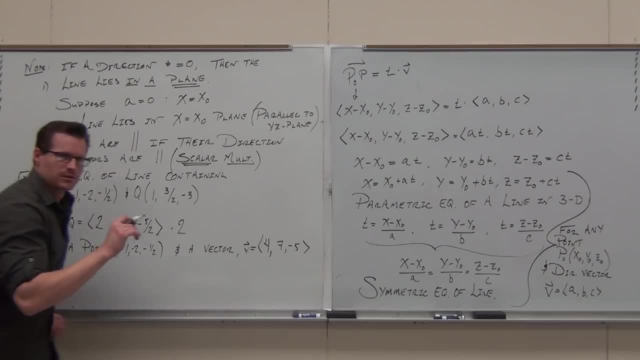 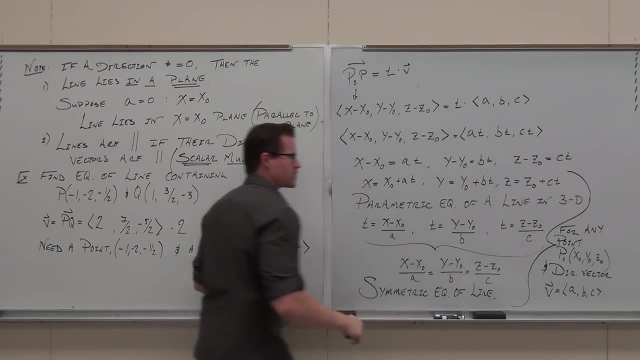 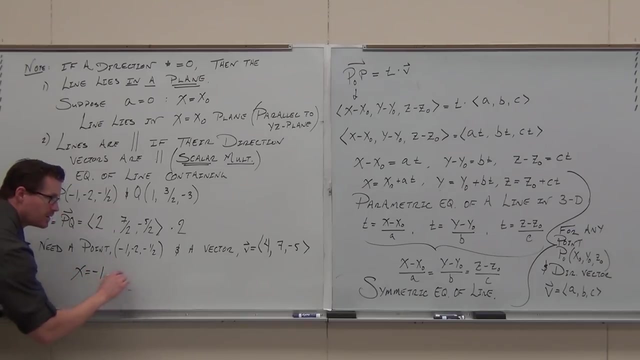 with a parametric equation. Literally all you do, literally put your x, y and z coordinates, put your direction numbers in the appropriate order. We need a x coordinate, a direction number and a parameter. That right, there is the little equation. 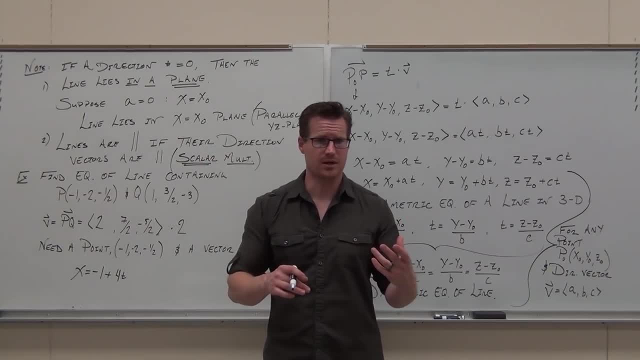 for how the x coordinates work for any point on this line. That's pretty awesome. So say you want to find an x coordinate for any points. plug in t. plug in all the values of t that you want, and you find these points in line. 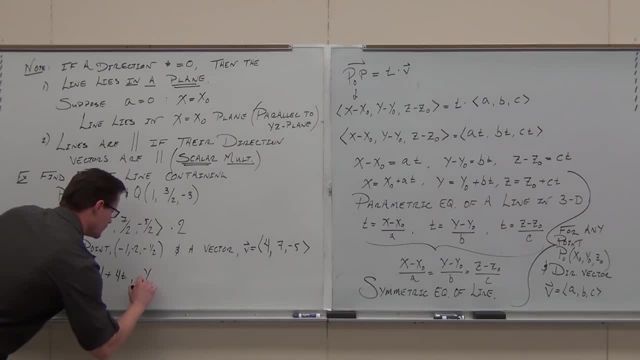 Well, at least x coordinates. right now, Let's do the y. What's the y start with? Come on right-siders. What's the y start with? Do you understand how easy it is to get confused between these two numbers? right now. 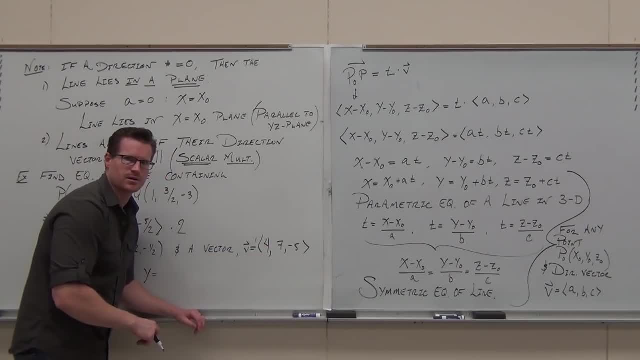 Yeah, Especially if you're the one who likes to put commas for your vectors. That's why we have these things saying this is a vector. That's a point. You get the point. What's the next thing? Hopefully it's plus. 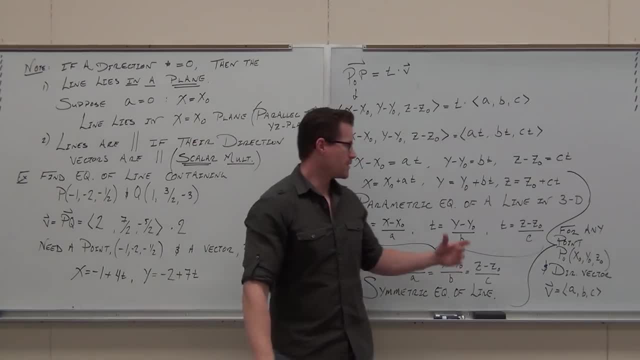 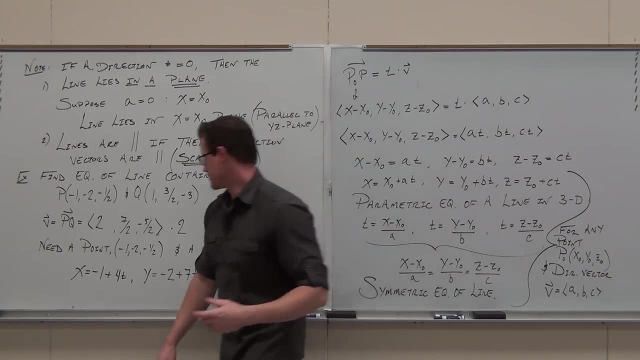 It's going to be plus, We're going to use the sign appropriately. So, on this, right here we have. We have literal x, y and z coordinates. We have literal x, y and z components of the direction vector. 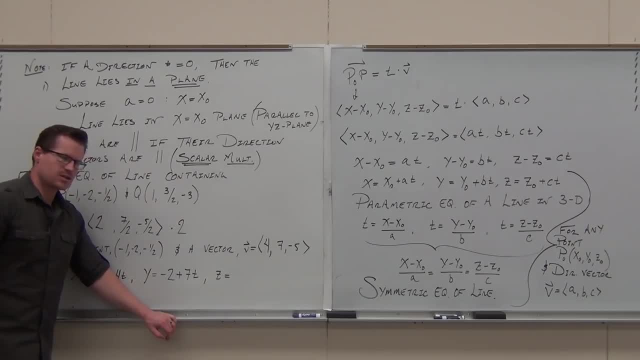 Let's watch the z, real careful Left-siders, you guys. what's the z coordinate of our point? What do we write first? Plus sign, minus, sign, What do you think? Minus what Pi? That's it, man. 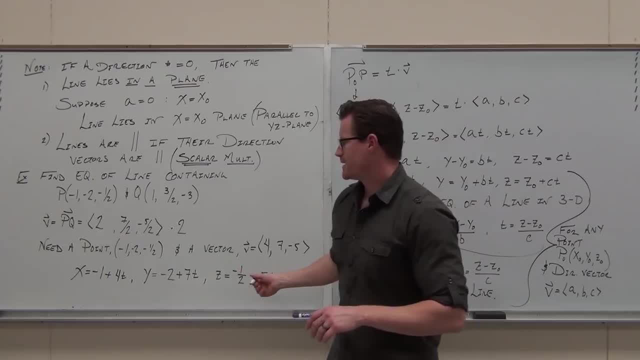 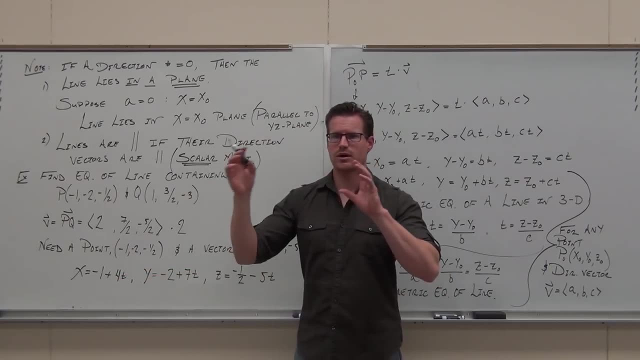 That's the parametric equation for a line and here's what it says: Given any value of t, same value for all three. you're going to get a point on that line Equations. plug it in and it'll give you an x coordinate. 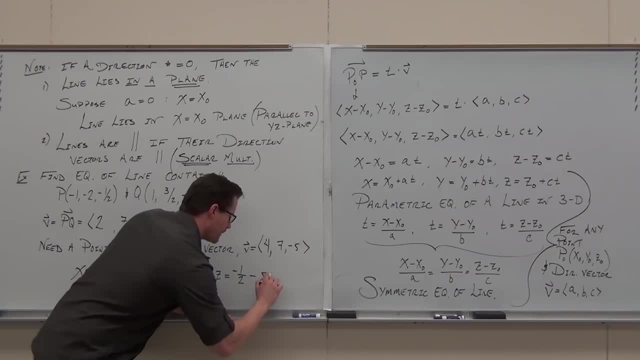 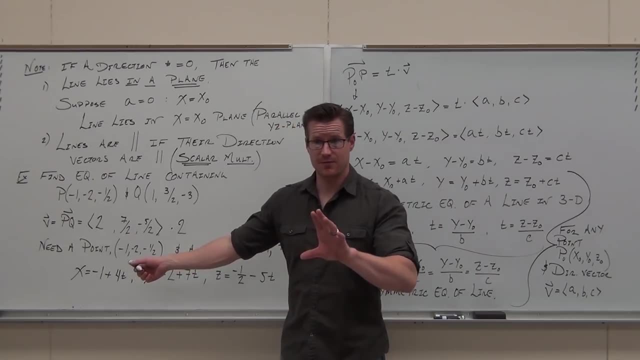 What do you think? Minus what, Minus what, Minus what? That's it, man. That's the parametric equation for a line, and here's what it says: Give any value, of t same value for all three equations. plug it in. 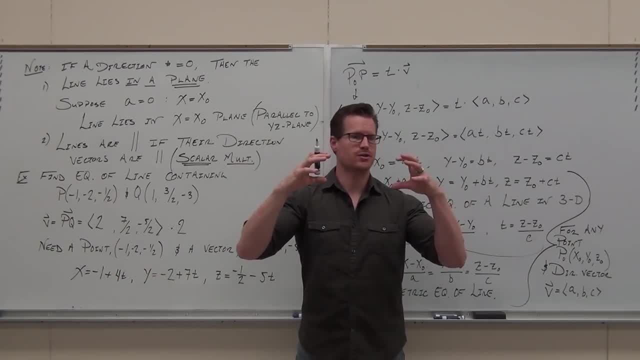 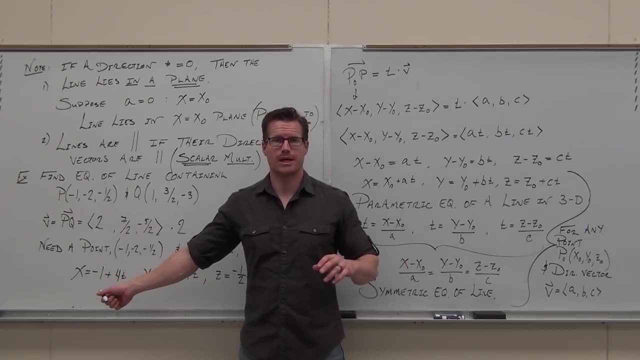 and it will give you an x coordinate, a y coordinate and a z coordinate. Put that together and you have yourself a point. That's how parametric equations work. That's the idea. Now, if I give you this, can you go backwards and tell me a point on that line? 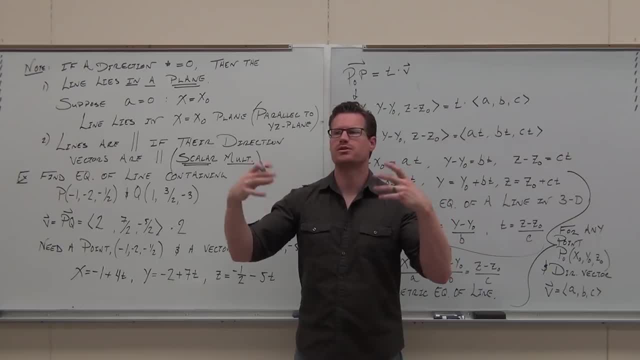 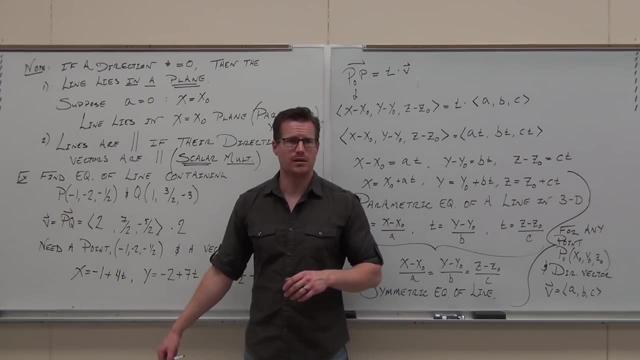 a y coordinate and a z coordinate. Put that together and you have yourself a point. That's how parametric equations work. That's the idea. Now, if I give you this, can you go backwards and tell me a point on that line? 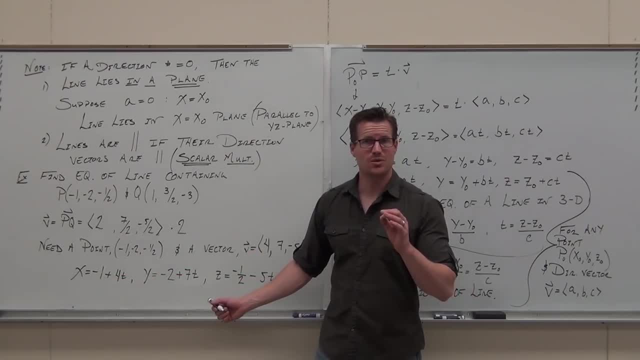 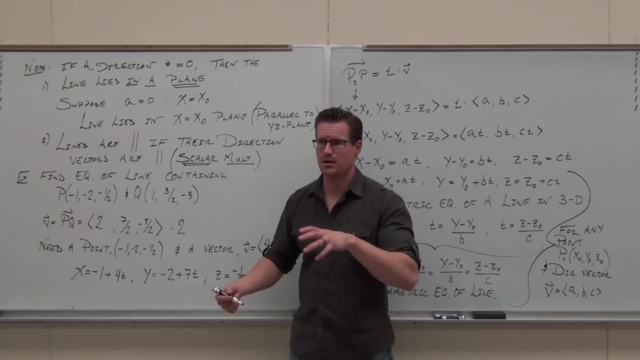 It's pretty easy. You plug in t equals zero, and that would give you that We'll call it the initial point, or something like that. It's pretty nice, So you can always find a point on a line by just plugging in t. 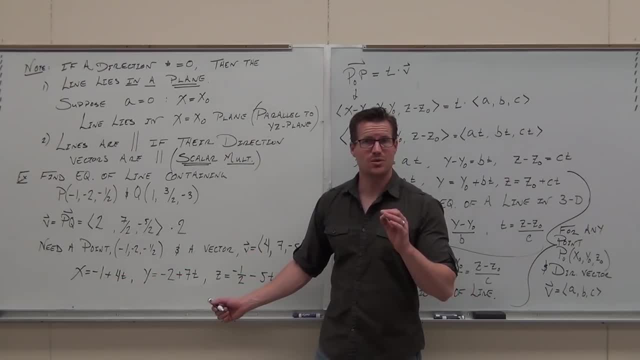 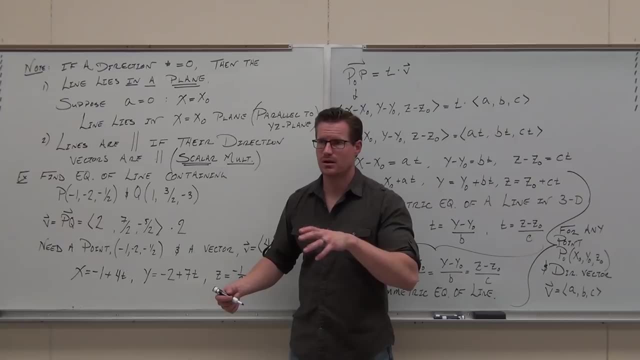 It's pretty easy. You plug in t equals zero and that would give you that We call it the initial point or something like that. so it's pretty nice. So you can always find a point. You can always find a point on a line by just plugging in t equals zero. 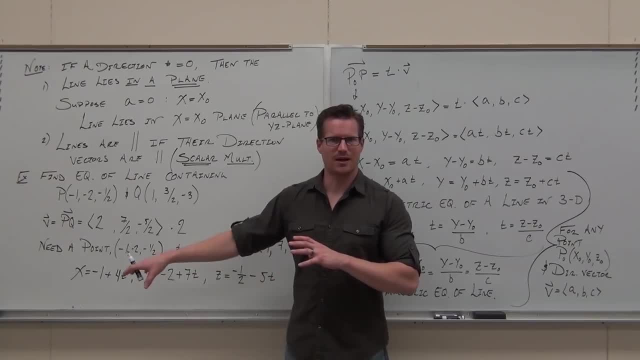 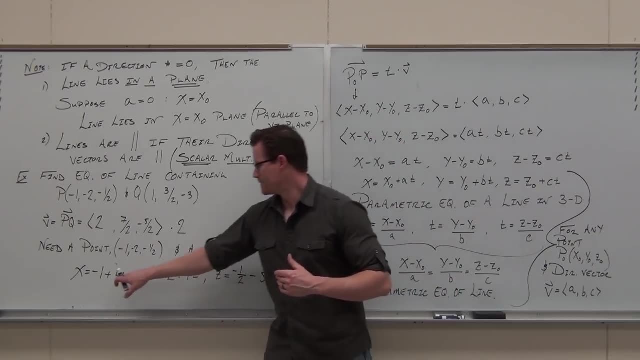 It's pretty nice. Can you always tell me a direction vector for that line? Yeah, Can you tell me the direction Just by looking at it? can you tell me the direction vector? Yeah, Four seven negative five. Can you tell me the original one? 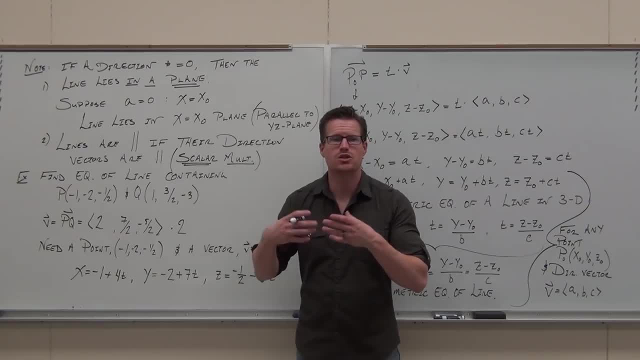 Who cares? I don't care, because it has the unit vector built in. I don't care that it's the one we got here or not, It's in the same direction. That's a lot of stuff. I'm probably over-talking. 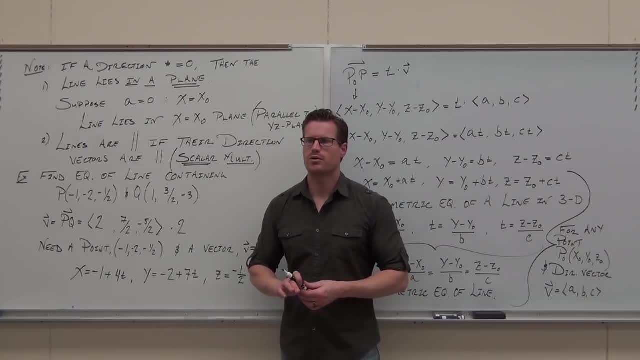 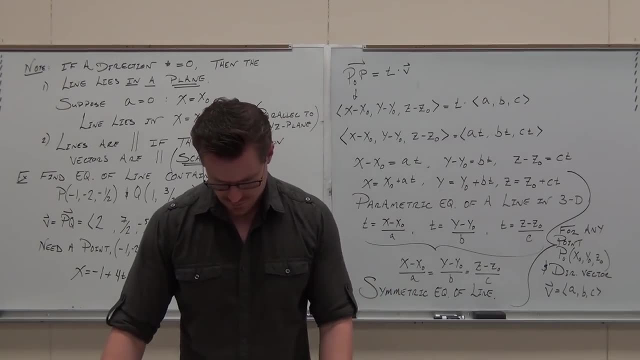 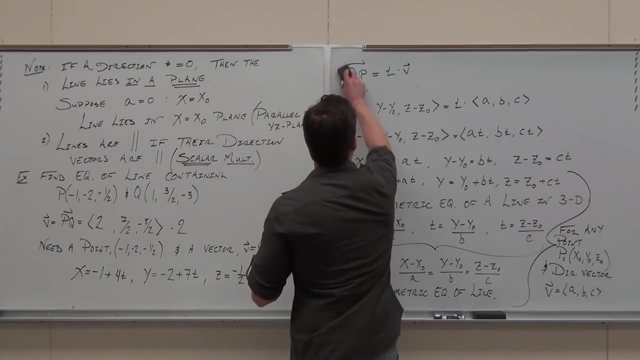 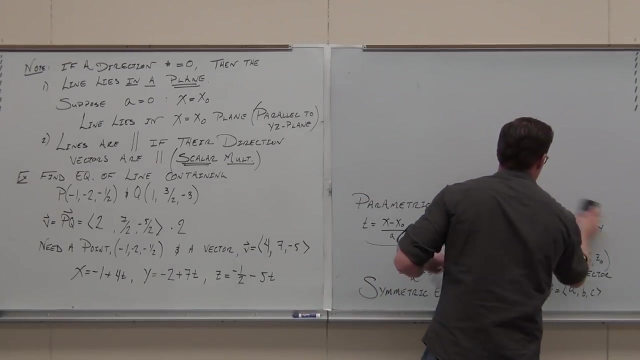 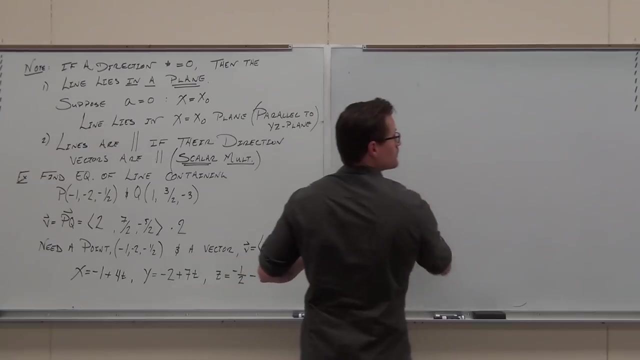 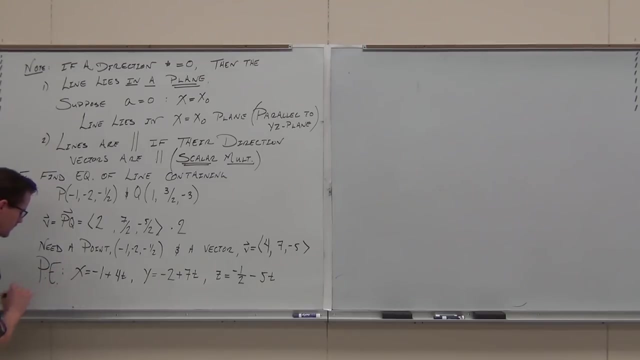 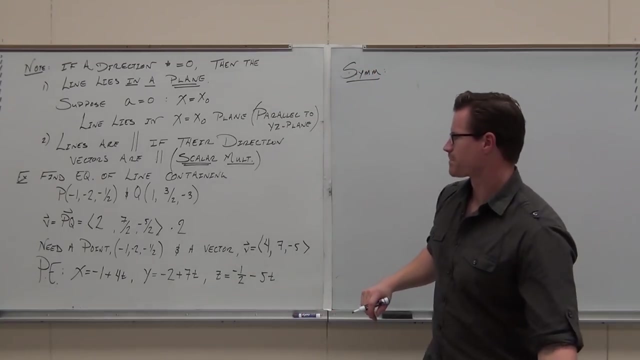 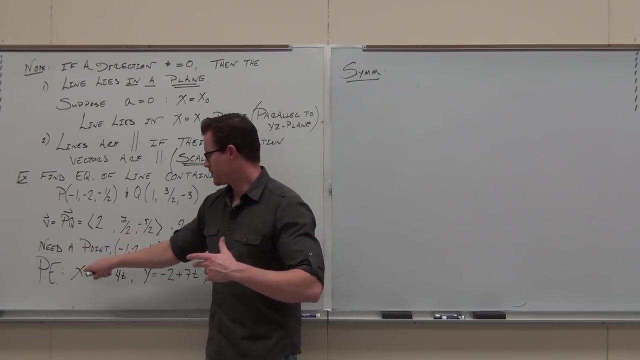 I'm over-talking it, but do you understand the concept here? Do one more thing: Change this into symmetric. See if you can do that. Whenever you're doing this, you've got to change back and forth. Change the sign of your x coordinates. add it over, subtract it over and divide by that number. 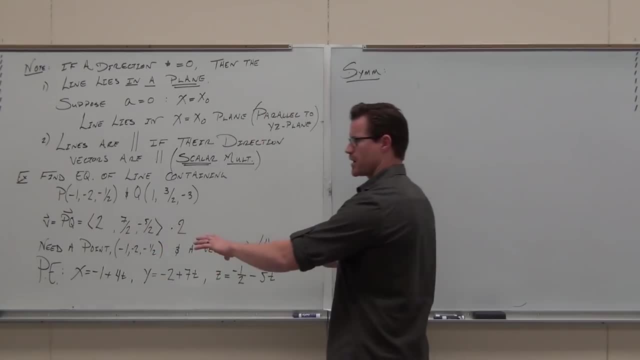 Don't change the sign of this number, please. So this is how this should look. So when I'm going to symmetric, I don't have any more x's, y's and z's. generally, There are specific cases. I'll show you that in just a second, when you do. 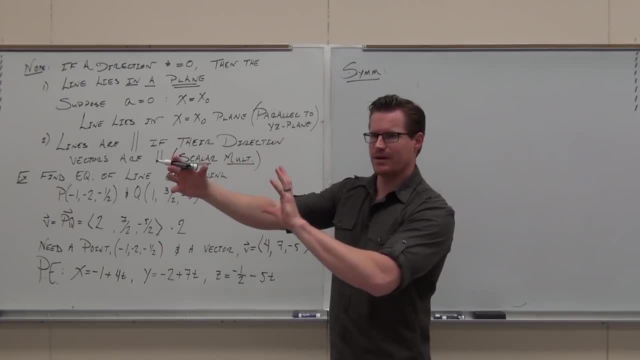 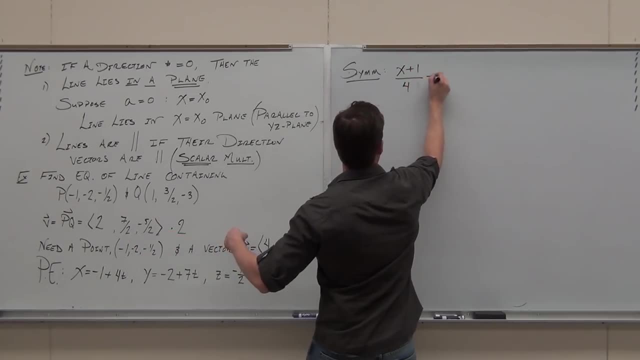 But generally here's how it looks: Like x equals. We don't have that anymore. It's kind of it's in that equation: So x plus 1 divided by 4.. Then we go to the y, Y plus. 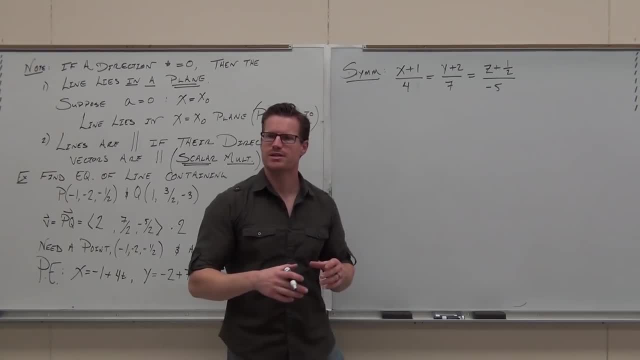 Yeah, just like that. that's it. Leave it just like that, and the reason is because it's easy to go back to parametric if you have to. It's easy to see what the point is and what the direction vector is. 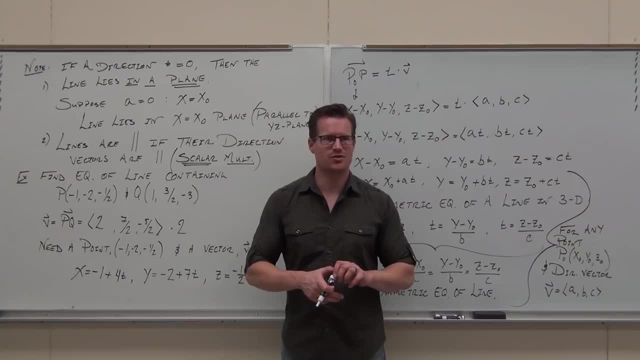 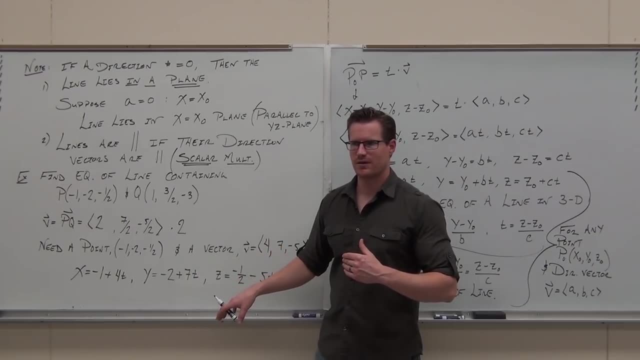 equals zero. It's pretty easy. All right, It's pretty nice. Can you always tell me a direction vector for that line? Can you tell me the direction Just by looking at it? can you tell me the direction vector Four, seven negative five? 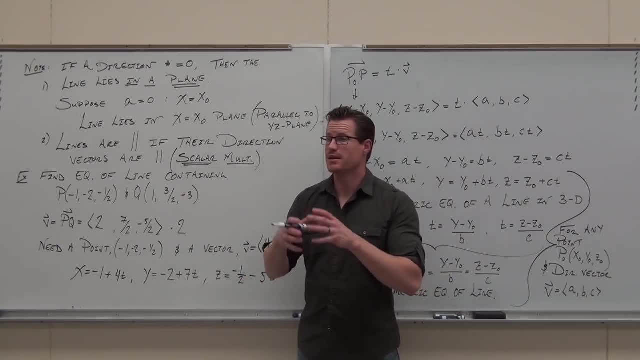 Can you tell me the original one? Who cares? I don't care, because it has the unit vector built in. I don't care that it's the one we got here or not, It's in the same direction. That's a lot of stuff and I'm probably over-talking it. 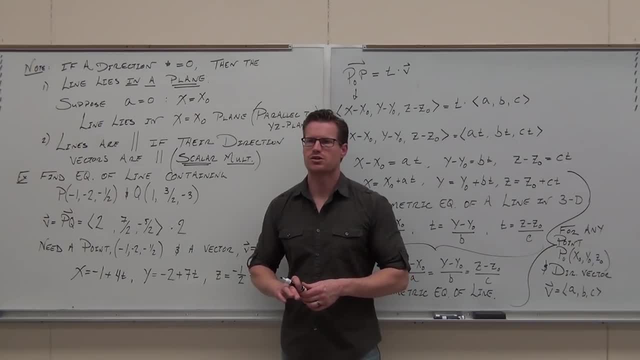 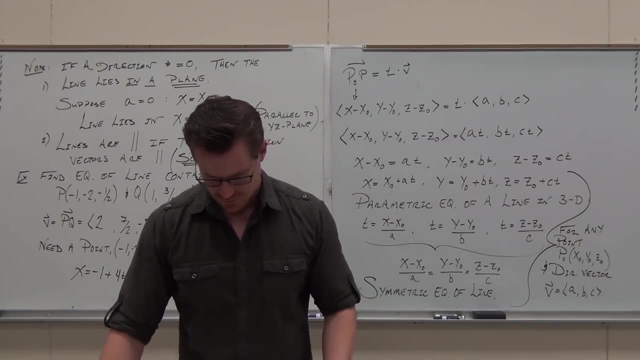 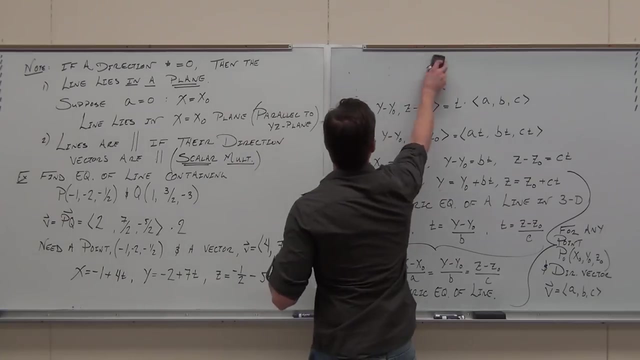 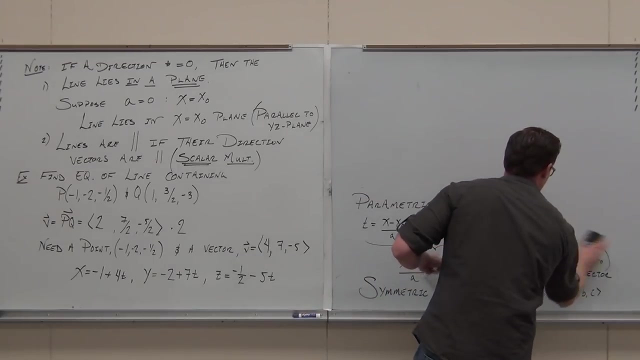 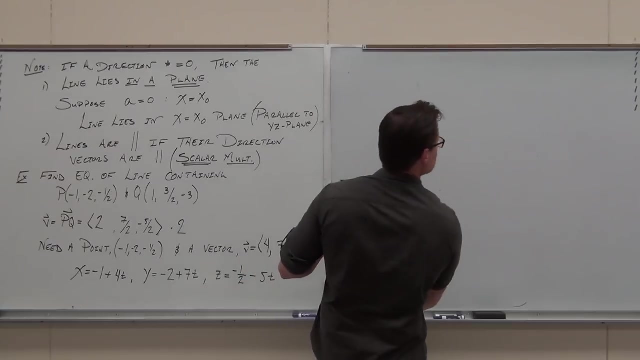 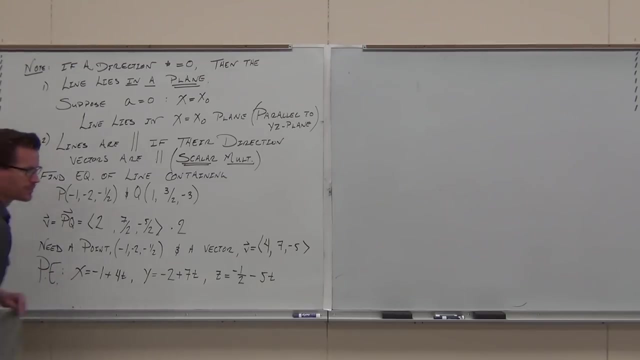 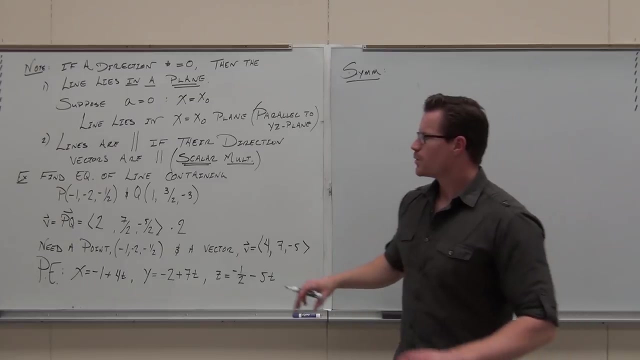 but do you understand the concept here? Do one more thing: Change this into symmetric. See if you can do that. Whenever you're doing this, you've got to change back and forth. Change the sign of your x coordinates, add it over. 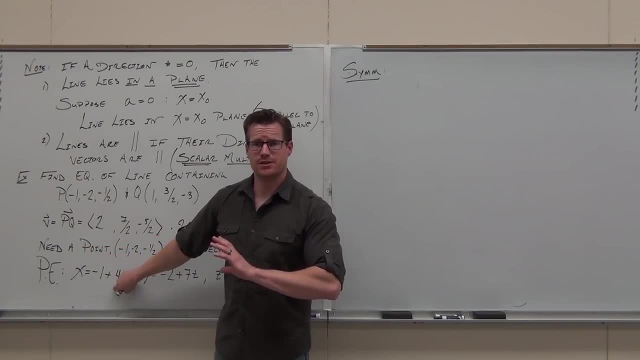 subtract it over and divide by that number. Don't change the sign of this number, please. So this is how this should look. So when I'm going to symmetric, I don't have any more x, y's and z's. 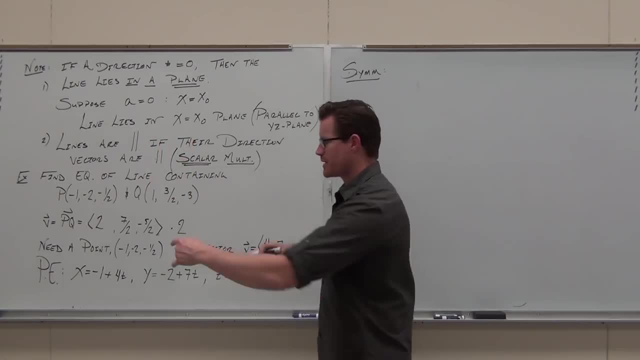 Generally. There are specific cases, I'll show you that in just a second when you do, But generally here's how it looks. Well, like x equals. We don't have that anymore. It's kind of it's in that equation. 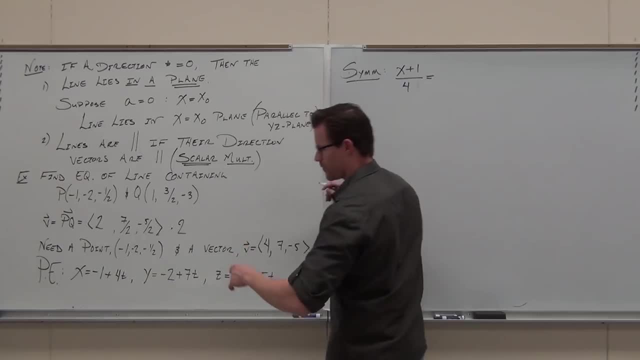 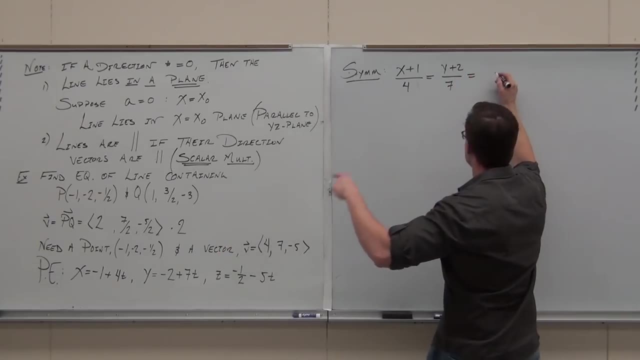 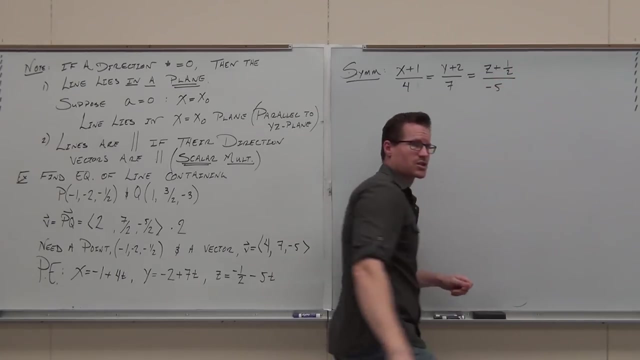 So x plus 1 divided by 4.. Then we go to the y. Yeah, just like that, That's it. Leave it just like that. And the reason is because it's easy to go back to parametric if you have to. 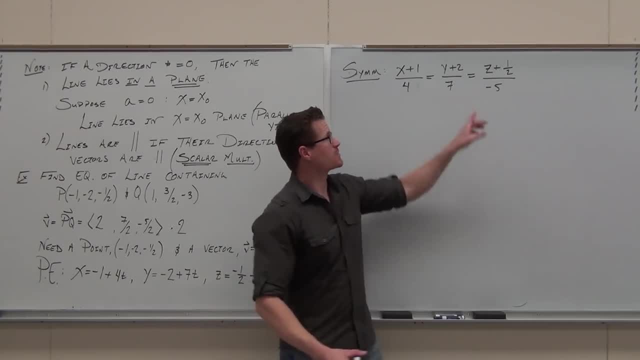 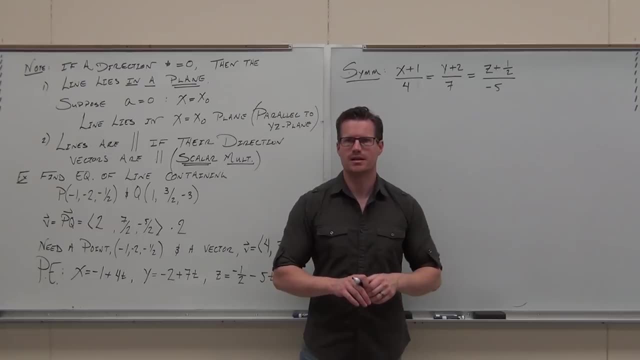 It's easy to see what the point is and what the direction vector is. You start messing with signs and then it doesn't work so well. You want positive x, positive y, positive z. Everything else, just hold it Head nod if you're okay with that one. 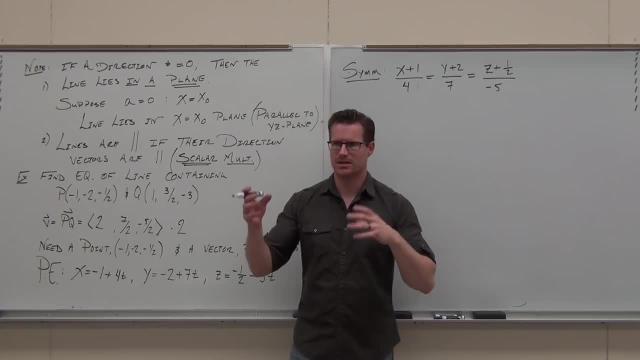 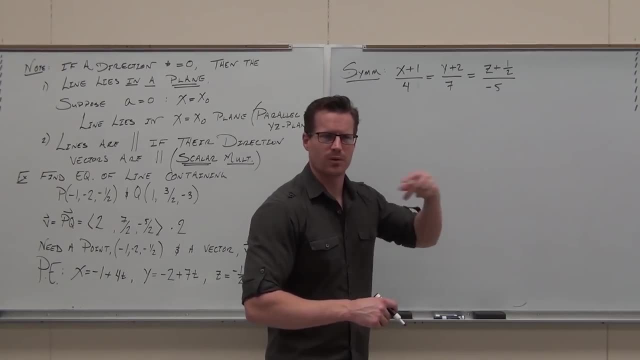 You start messing with signs and then it doesn't work so well. You want positive x, positive y, positive z. Everything else. just hold it Head, nod, if you're okay with that. one Backtrack. just a second. I don't want to move it fast, but I want you to get all of it quickly. 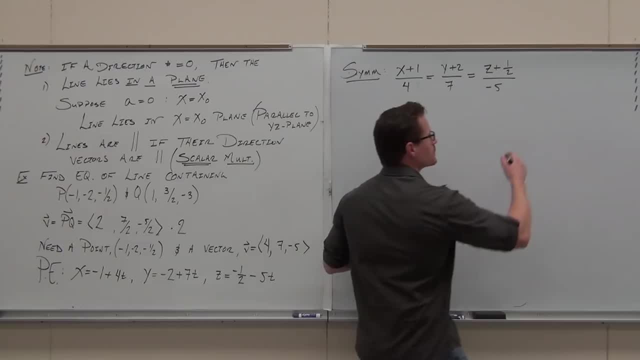 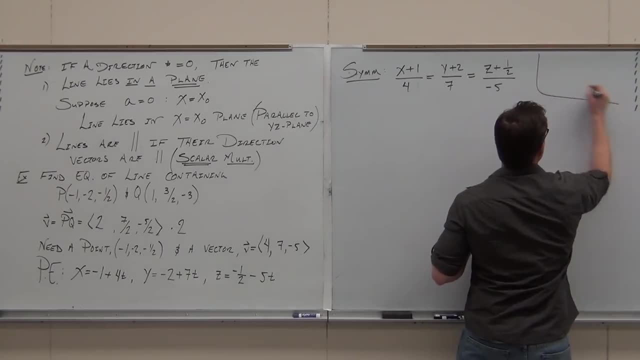 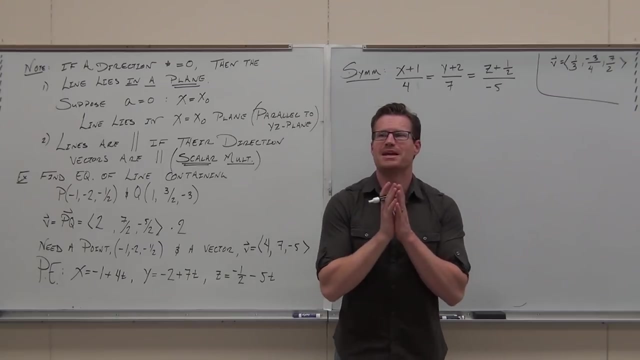 Backtrack. just a second. I don't want to move it fast, but I want you to get all of it quickly. If I were to give you this direction vector, Would you ever use that to build your line? I'm begging you. 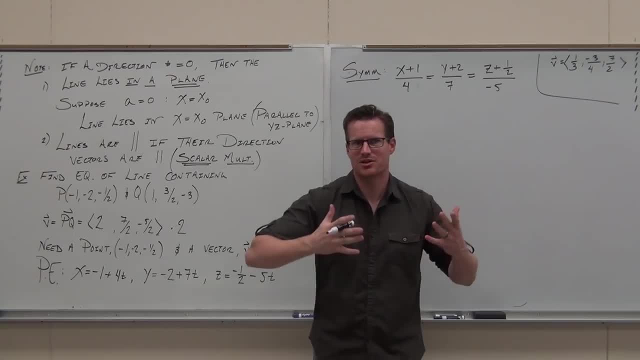 I don't want to grade that. okay, Please don't make me grade that, because you're probably going to be right. But I don't want to look at fractions. I don't like fractions. What would you multiply by 12.. 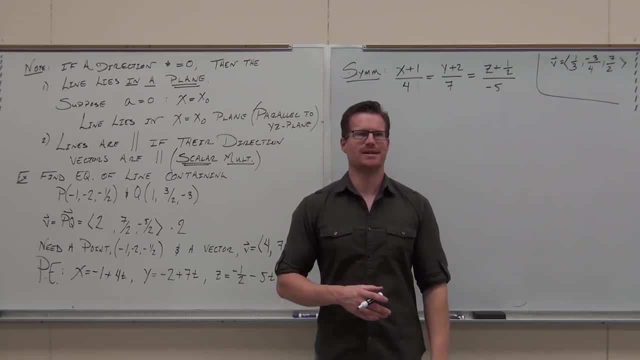 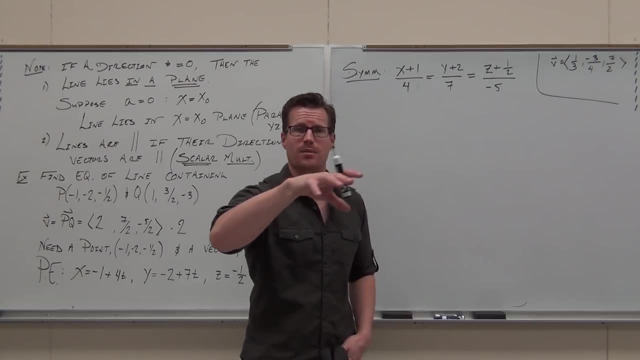 Good, How did you get 12? LCD Use that Done Real nice, Real nice stuff. Okay, How about this one? What would happen? So we're going to modify the problem. I'm going to do this a lot. 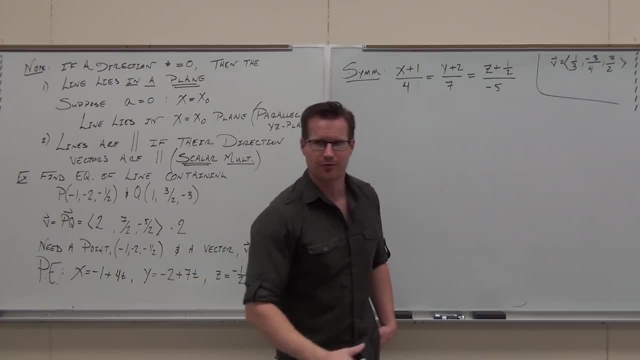 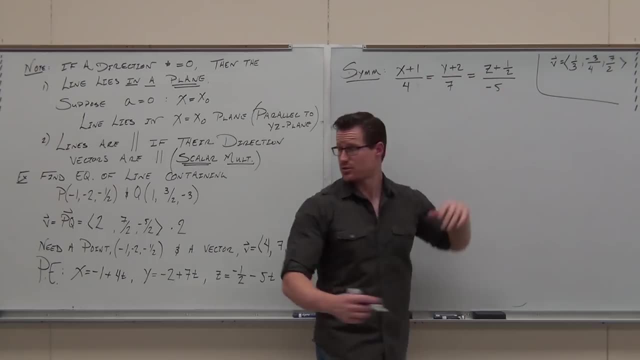 I don't have time for 50 examples, even though we're probably going to do like 50.. What if that number were zero? How would you write the symmetric equation? Because this would be pretty easy. If this is zero, you just have z equals negative 1 half, which you get what I'm talking about. 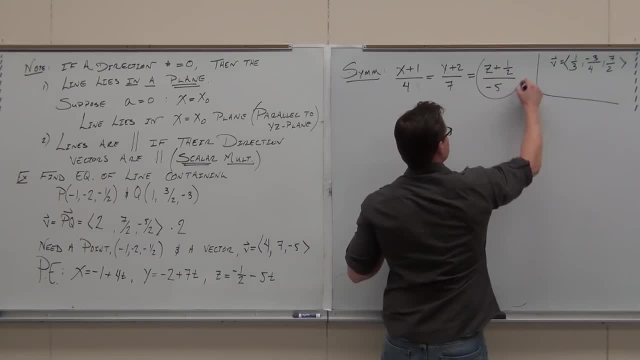 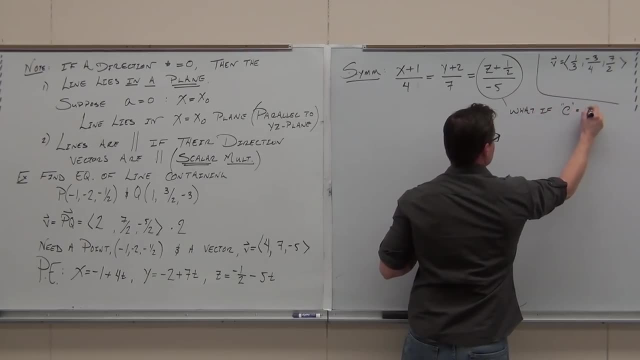 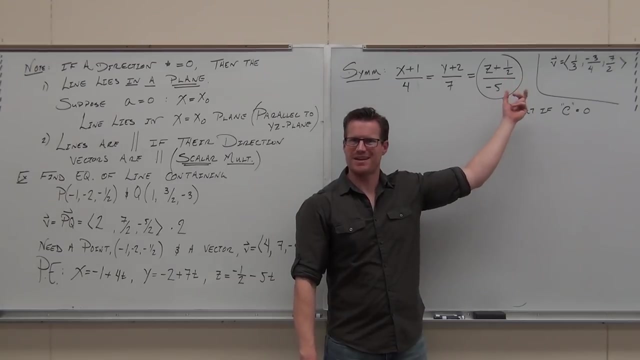 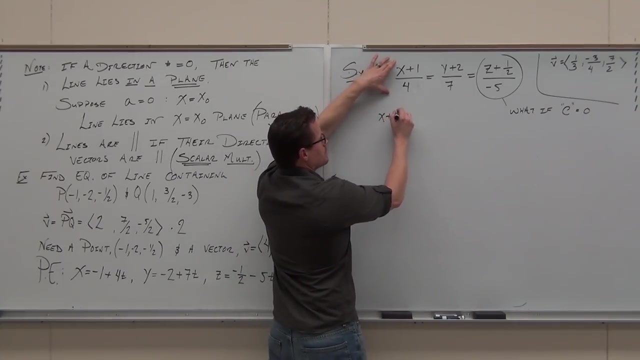 If this is zero? If that's the case, then we really can't write this format anymore, because we have that little undefined thing. So here's how it works: If that's zero, we keep these two, And then you put a comma, because we can't write it like this. 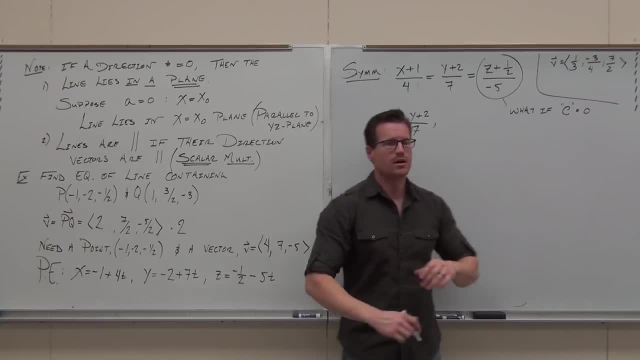 and you wrap it up with the same format over here, this being zero. So it would be. It would be the z equals negative 1 half. That's how you would write that If you ever have a direction number that's zero. parametric doesn't change. 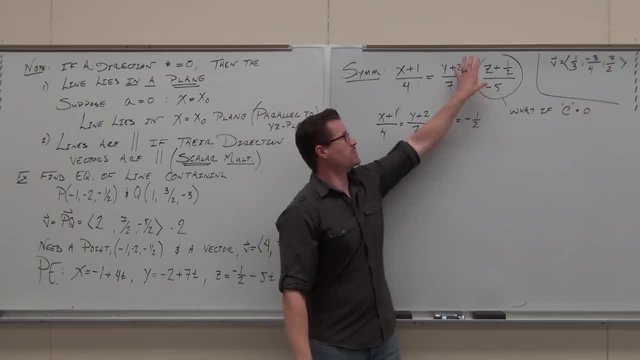 You just have a zero there. times t, That's zero Symmetric. you drop out one of those symmetric equations. leave the two, You have one that's equal to a constant. Now stop and think about this. If you have a variable equal to a constant in 3D, what's it mean? 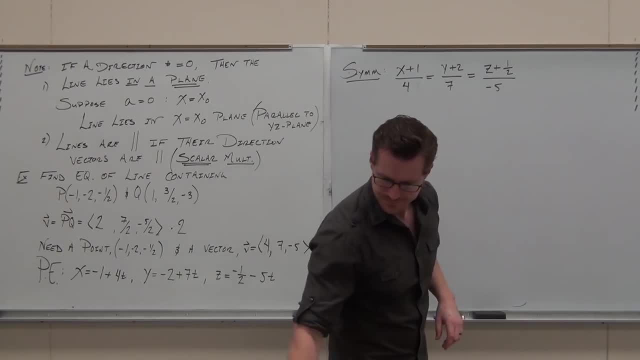 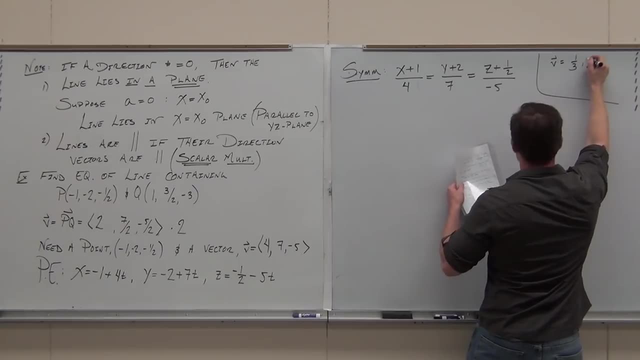 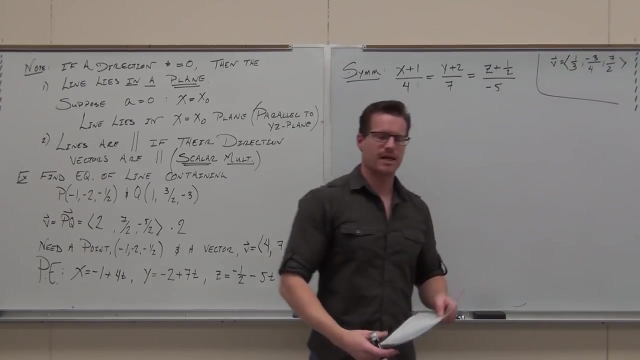 If I were to give you this direction vector, Would you ever use that to build your line? I'm begging you, I don't want to grade that. okay, Please don't make me grade that, because you're probably going to be right. 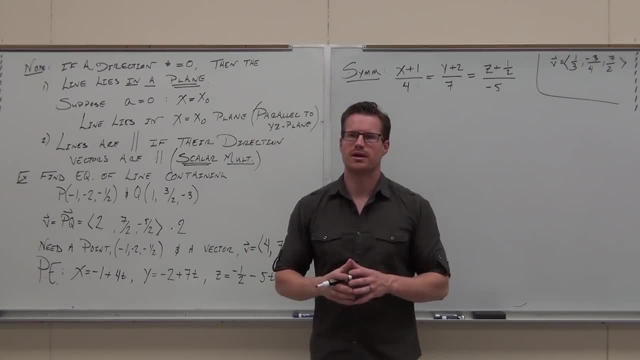 But I don't want to look at fractions. I don't like fractions. What would you multiply by 12.? Good, How'd you get 12?? LCD Use that Done Real nice, Real nice stuff. Okay, how about this one? 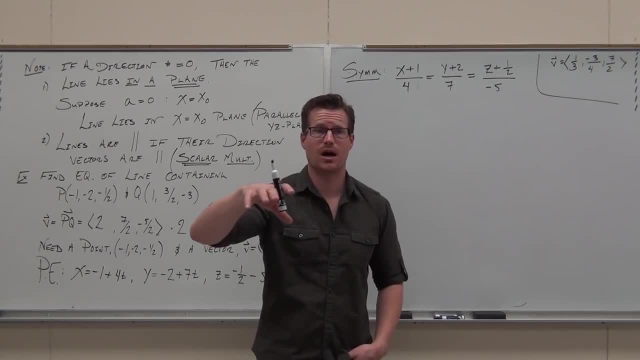 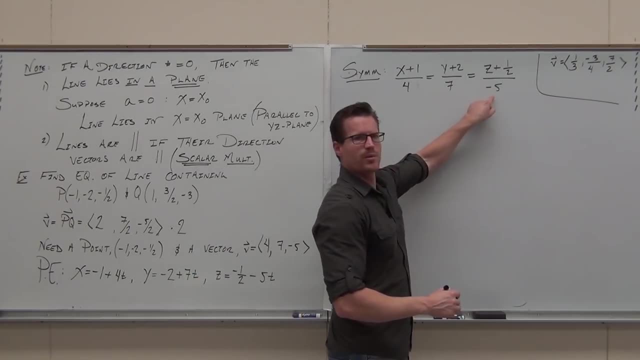 What would happen? so we're going to modify the problem. I'm going to do this a lot. I don't have time for 50 examples, even though we're probably going to do like 50.. What if that number were zero? 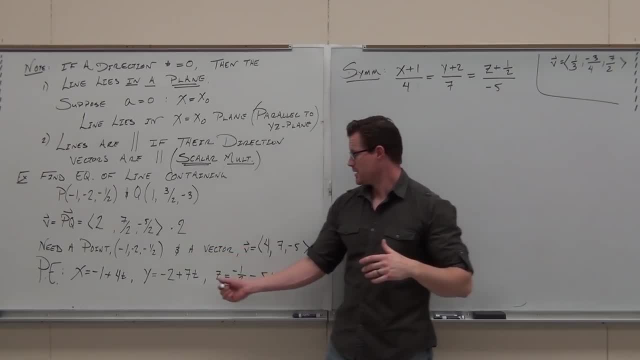 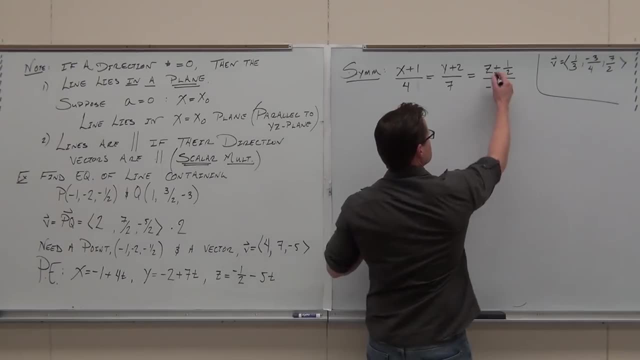 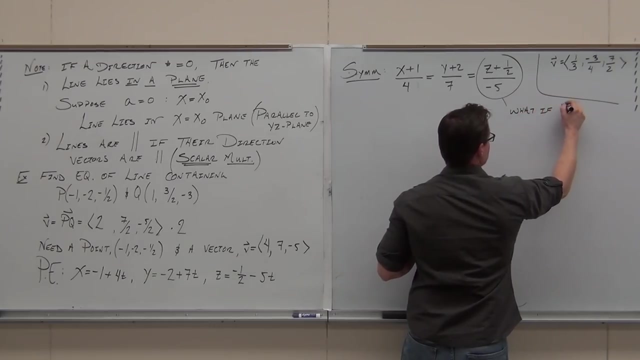 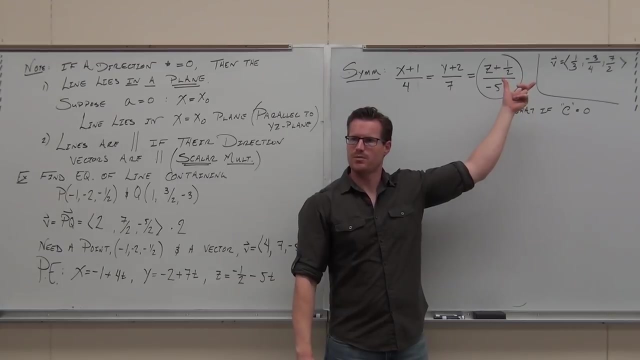 How would you write the symmetric equation, Because this would be pretty easy. If this is zero, you just have z equals negative one-half. Did you get what I'm talking about If this is zero? If that's the case, then we really can't write this format anymore. 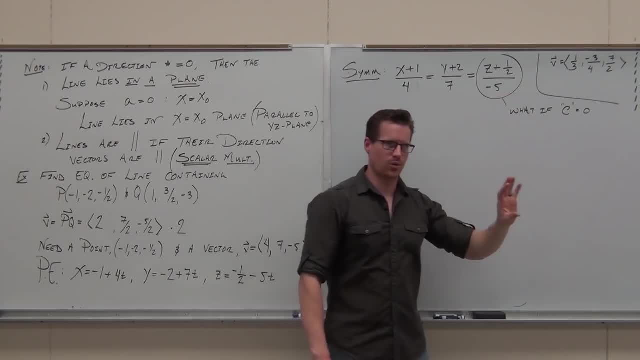 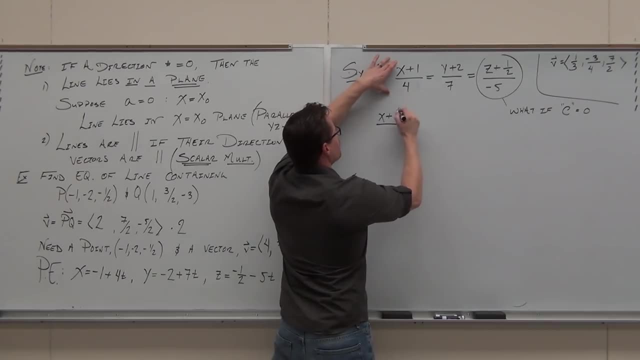 because we have that little undefined thing. So here's how it works: If that's zero, we keep these two, And then you put a comma, because we can't write it like this, and you wrap it up with the same format over here. 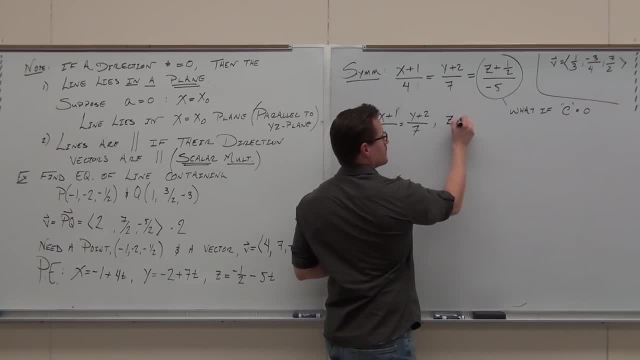 Here, this being zero, So it would be the z equals negative one-half. That's how you would write that If you ever have a direction number that's zero, parametric doesn't change. You just have a zero there times t, that's zero. 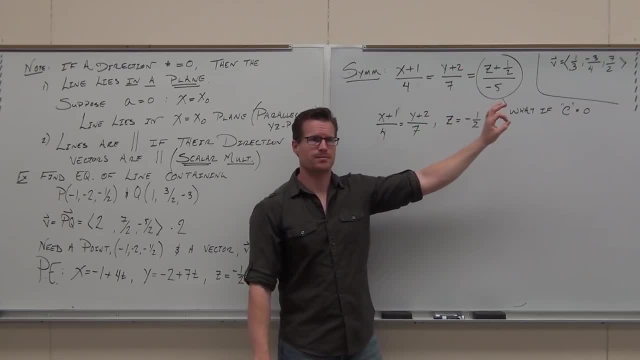 Symmetric. you drop out one of those symmetric equations. leave the two, You have one that's equal to a constant. Now stop and think about this. If you have a variable equal to a constant in 3D, what's it mean? 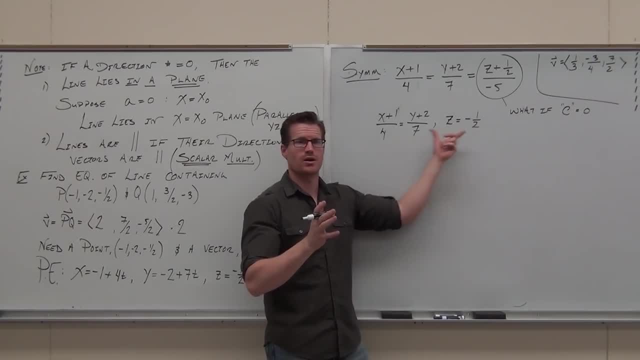 It's on a. this line is on a plane. Look at this happening. X, Y and Z are changing right on this problem, But if it's here, is Z changing Negative one-half on a plane. This is lying on a plane that's parallel to the X- Y plane, just a half step below. 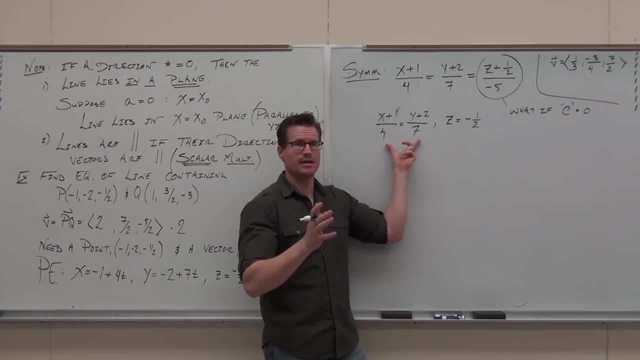 It's on a plane. It's on a plane. This line is on a plane. Look at this happening. x, y and z are changing right on this problem, But if it's here, is z changing No. 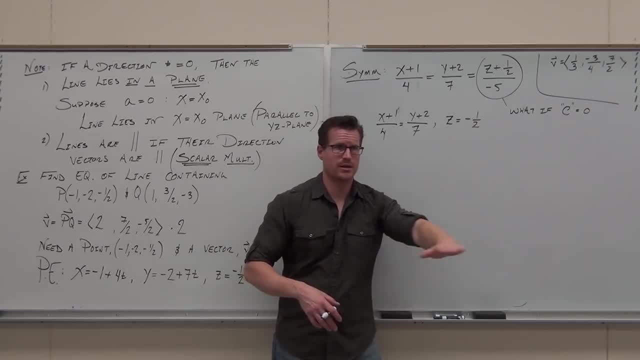 Negative 1 half on a plane. This is lying on a plane that's parallel to the xy plane, just a half step below, and this is the only crap that's changing xy. Do you guys see what I'm talking about? It's kind of cool, right. 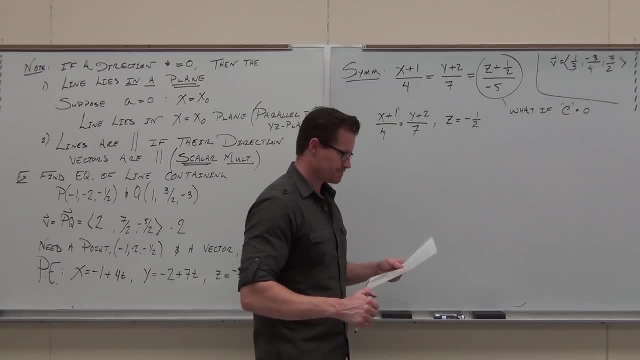 That's what's happening here. Let's extend it. I'm going to go back to our original. Do you guys have this written down, Because I'm about to erase it? Are you guys okay with that one? Okay, Because I don't want to confuse you with the next one. 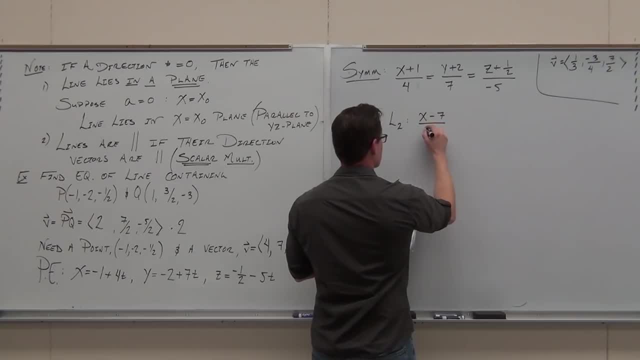 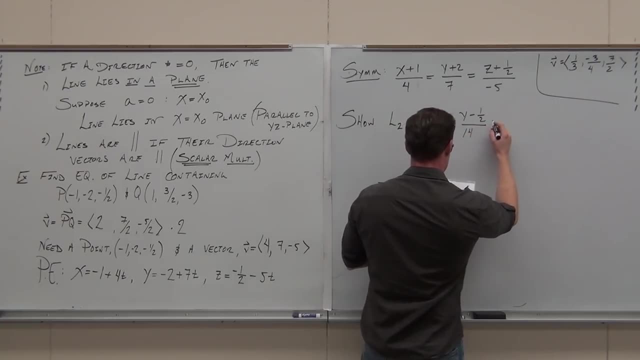 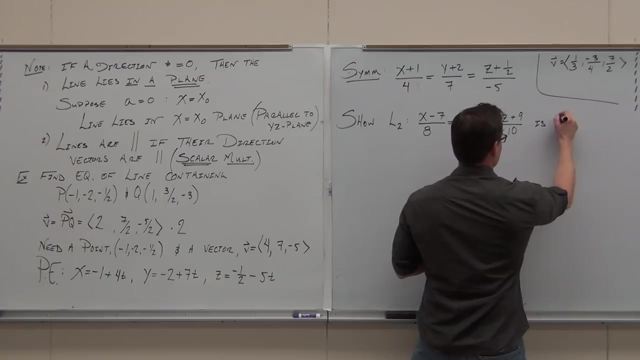 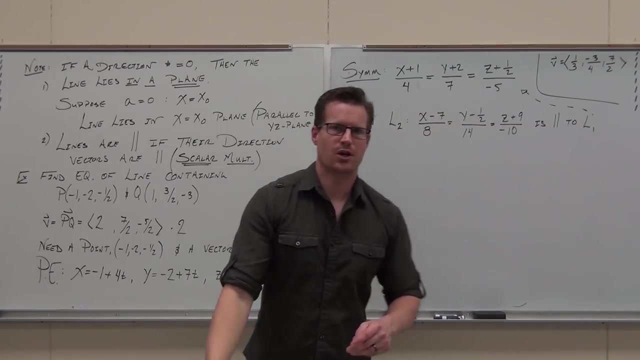 Can you show line 2?? Let's say this is line 2.. Can you show line 2 is parallel to line 1? Can you show? I can show it. I know what I'm doing, man. Can you guys show it? 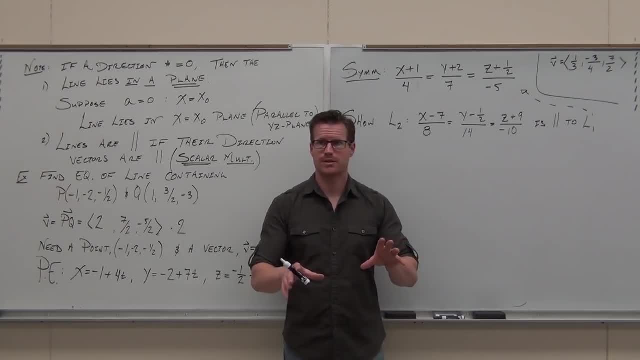 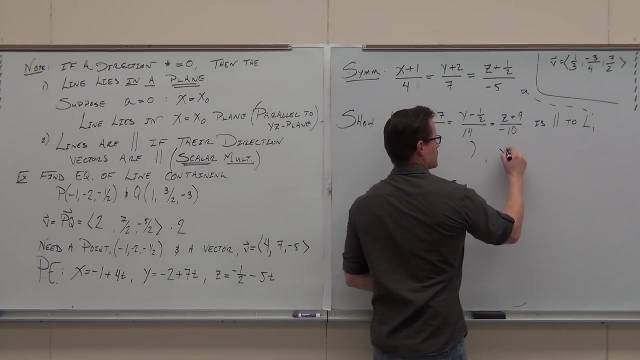 Yes, No, Yeah, Okay, Here I'm going to give you 10 seconds. What I want in 10 seconds is from this line: I want you to find me a point on that line And I want you to find me the direction vector from that line. 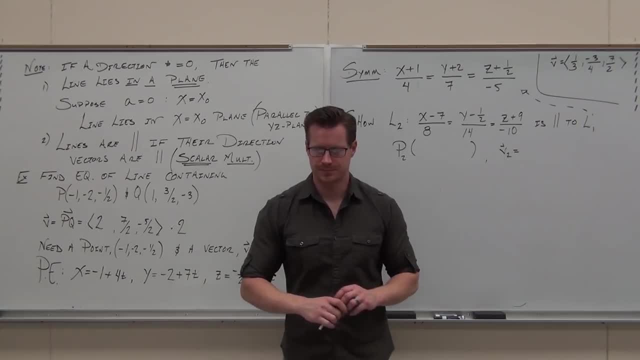 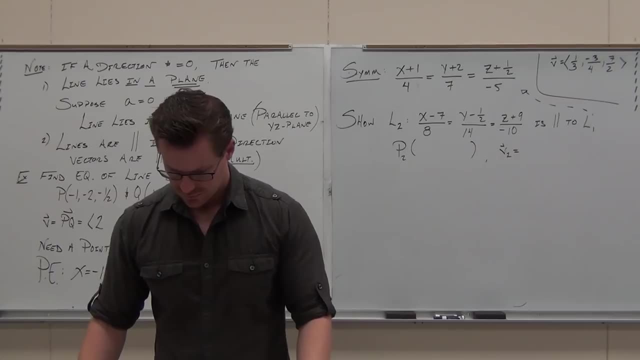 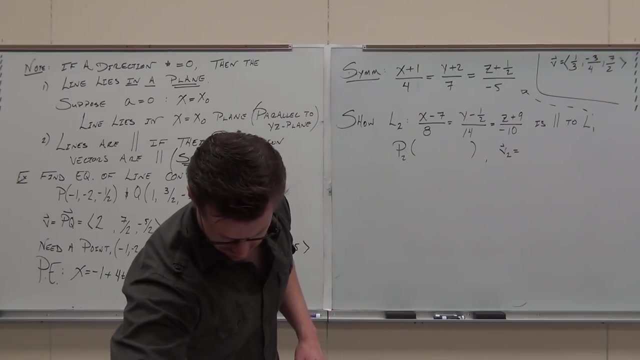 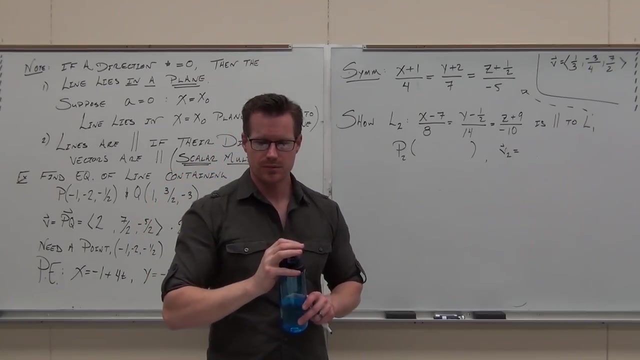 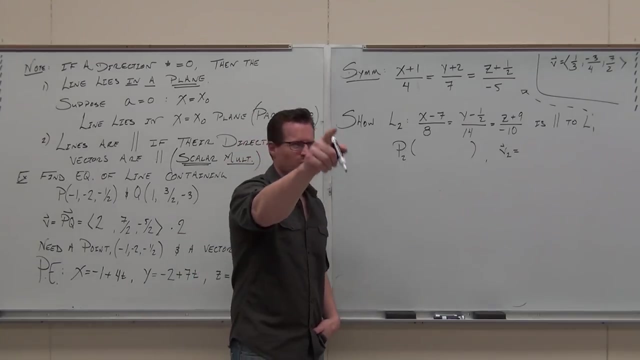 Can you do it? Go for it, Go for it, Go for it. Can you find me the point? You guys got the point. You guys are going to get the vector Point. Oh, what's the point to start with? 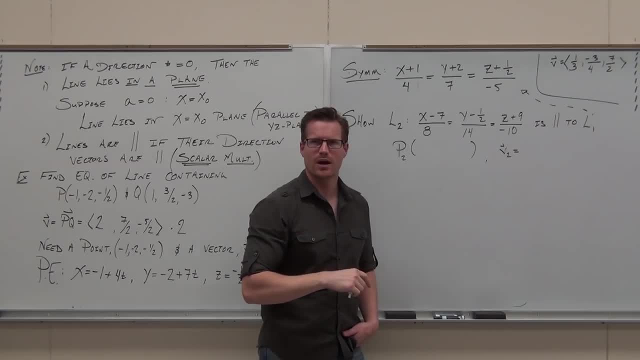 7? Or negative, 7? Positive, 7. Why? Why the opposite sign? The equation. Because on the symmetric equation it's x minus that. So we're changing signs here. So this is 7.. What's the y? 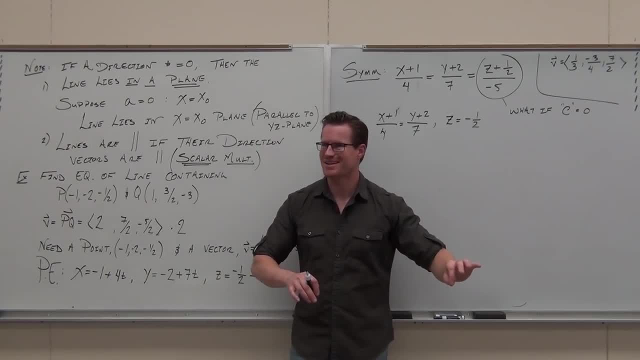 and this is the only crap that's changing X- Y. Do you guys see what I'm talking about? It's kind of cool, right? That's what's happening here. Let's extend it. I'm going to go back to our original. 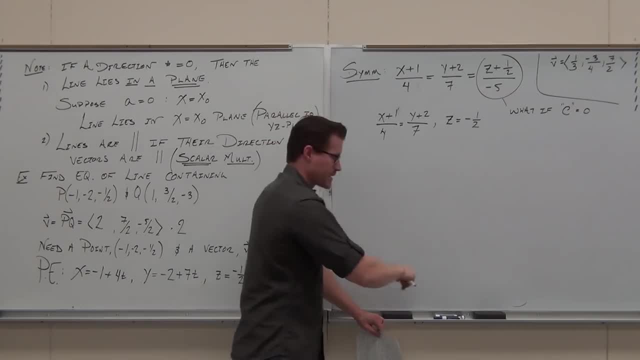 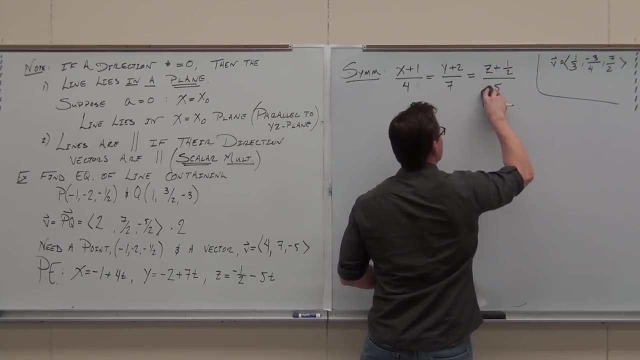 Do you guys have this written down? Because I'm about to erase it. Are you guys okay with that one? Okay, because I don't want to confuse you with the next one. Okay, Okay, Okay, Okay, Okay Okay. 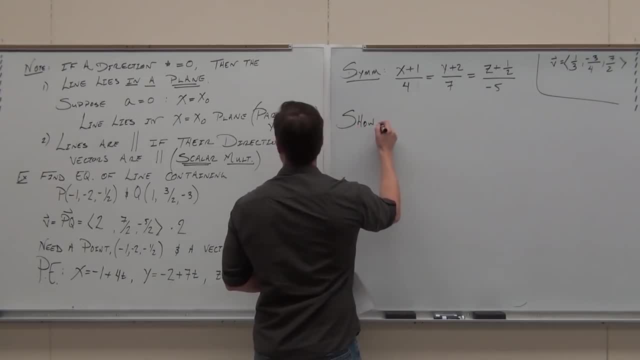 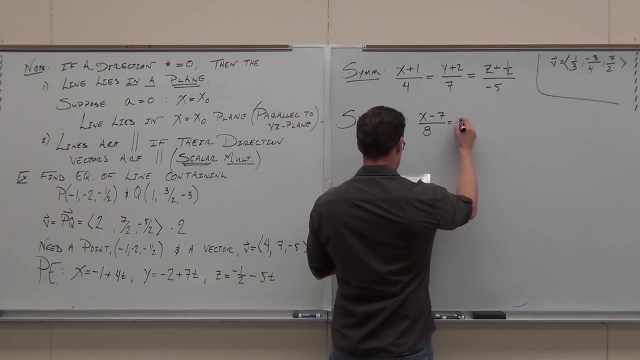 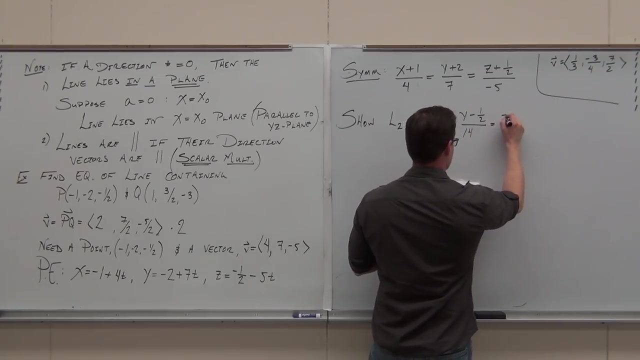 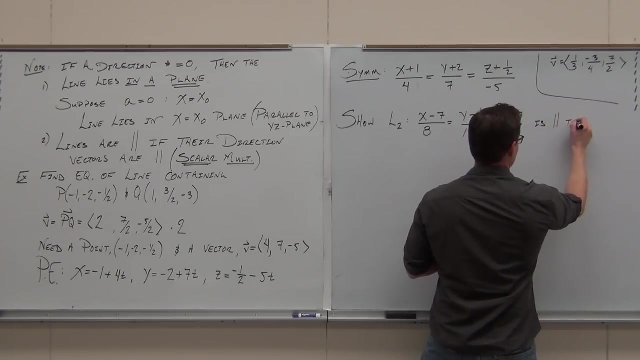 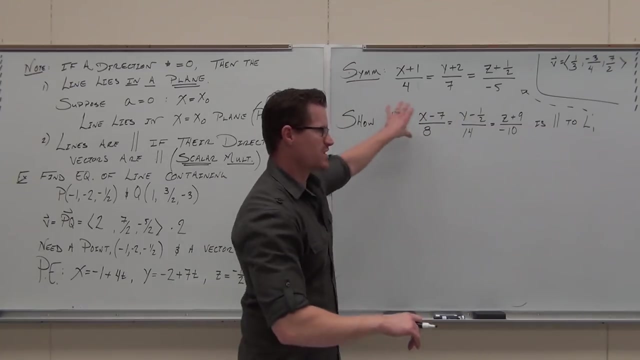 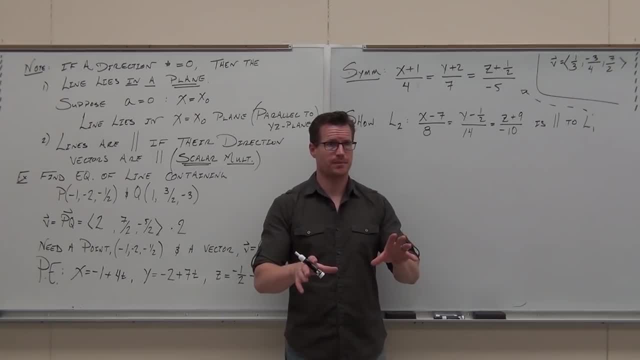 Can you show? I can show it. I know what I'm doing, man. Can you guys show it? Yes, no, Okay, I'm going to give you ten seconds. What I want in ten seconds is from this line: I want you to find me a point on that line. 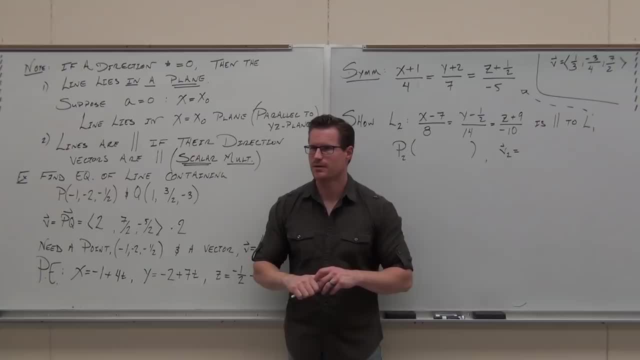 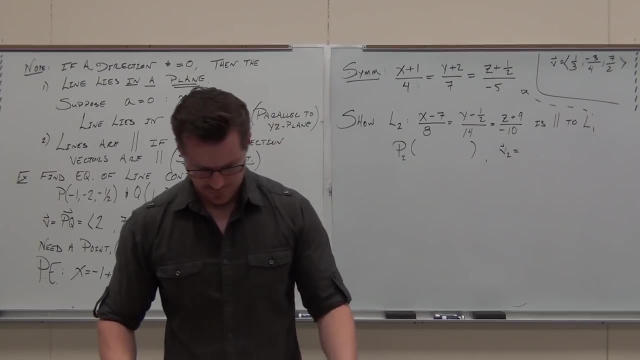 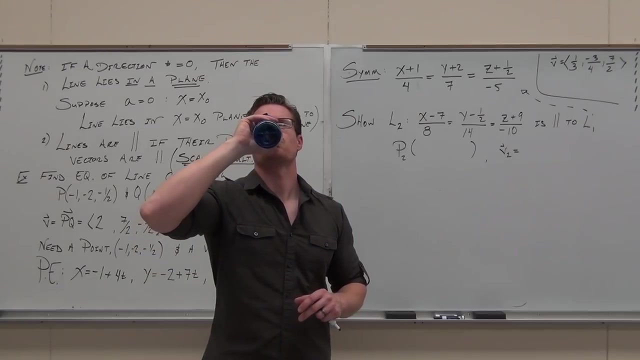 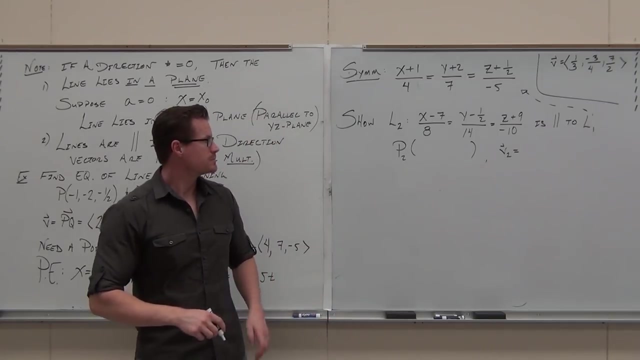 And I want you to find me the direction vector from that line. Can you do it? Go for it, Go for it. Can you find me the point? You guys got the point. You guys are going to get the vector Point. 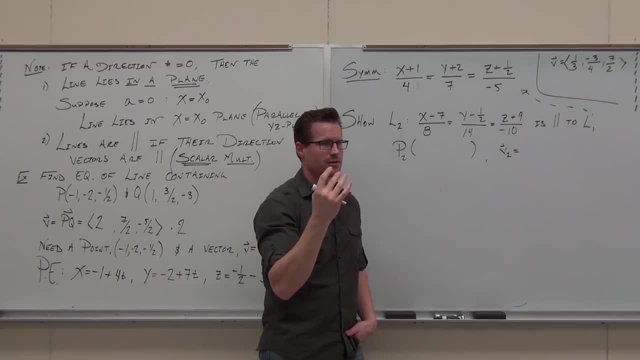 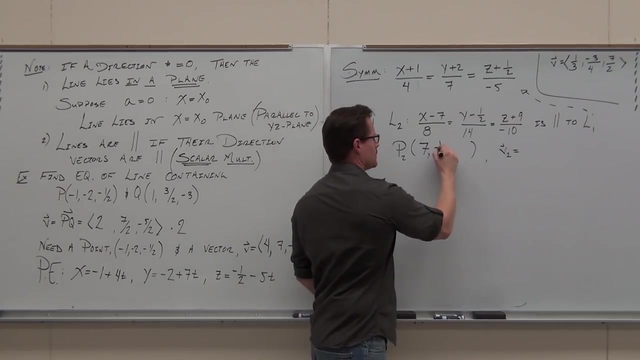 Oh, what's the point? start with Seven Negative seven. Why? Why the opposite sign? Because on the symmetric equation it's x minus that. So we're changing signs here. So this is seven. What's the y And the z? 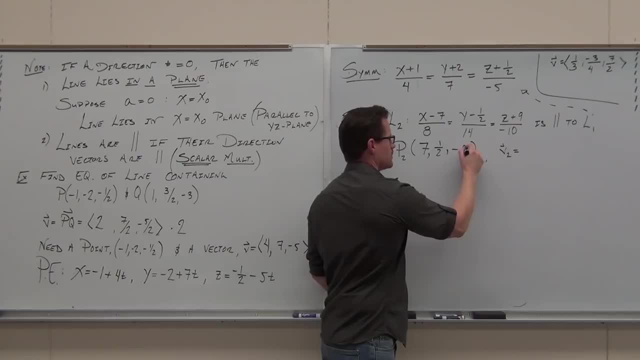 Positive y And the z Negative z. I didn't actually hear you. I kind of imagined you said negative 9.. Did you say negative 9?? Yes, I hope so. I should have said: you guys huh Slackers. 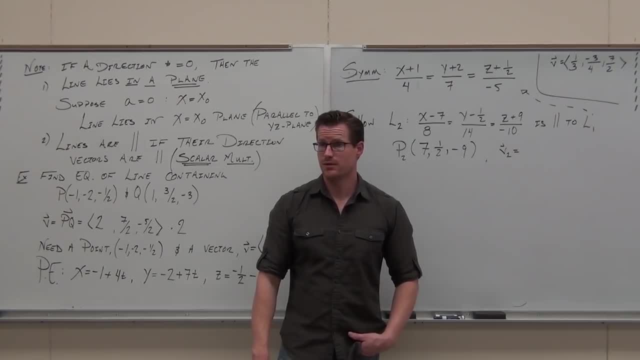 Come on now, Left-siders y'all. Can you find the vector, the direction vector? Yes, This is the easy part with this. This is why this format really shines. It's really nice. You know what it is? Denometers. 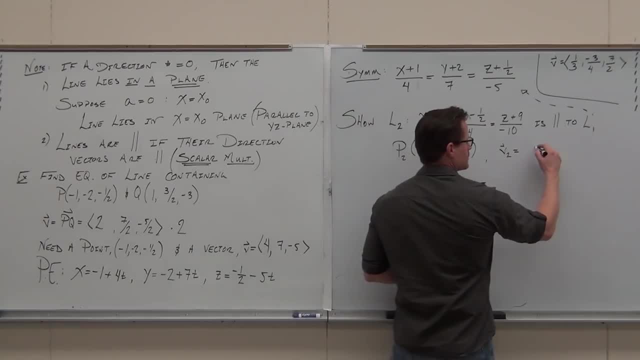 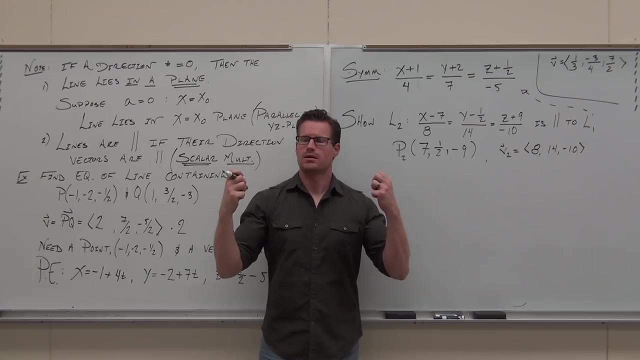 That's all it is, And it's even matched up X, y, z. So this is parentheses or vector bracket. Yes, And they're important. Now next question: Come on, Stick with me here. Are these two lines parallel? 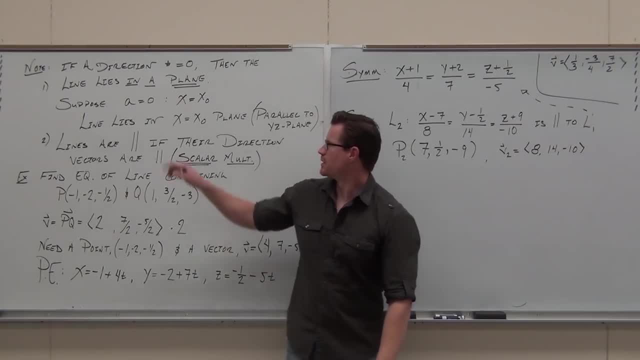 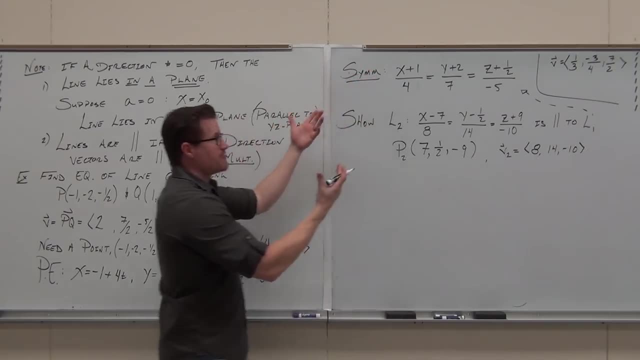 Yes, We talked about it earlier. We had a statement up here. Lines are parallel if the direction vectors are scalar or multiple, So we're going to write out vector 1.. We already have that, man. This is what we used. 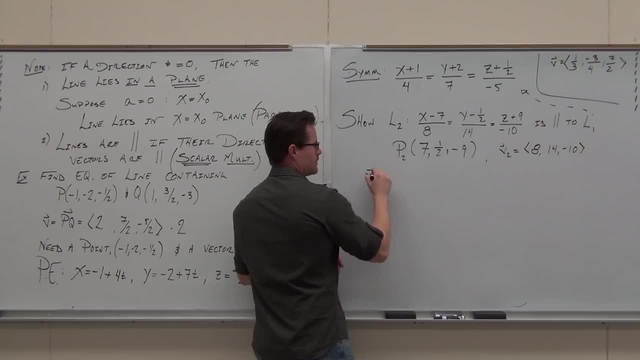 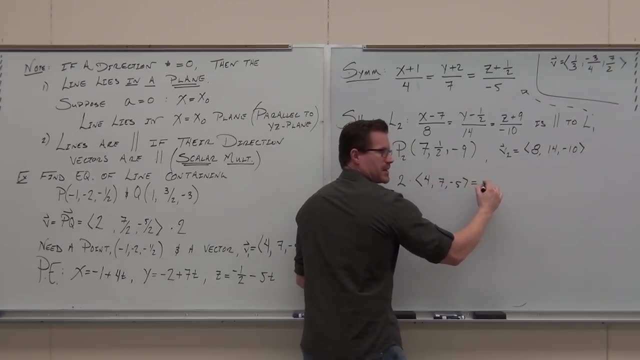 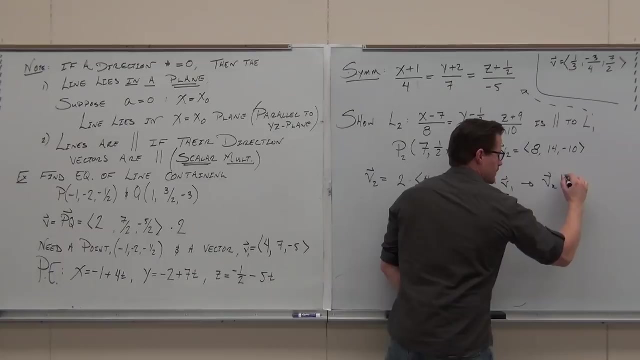 So if we call that vector 1. Vector 2, this vector is 2 times. It's 2 times 4, 7, negative 5. That means it's 2 times vector 1, which means that vector 2 is parallel to vector 1.. 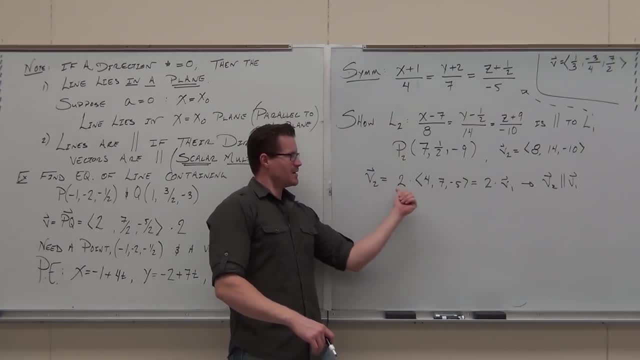 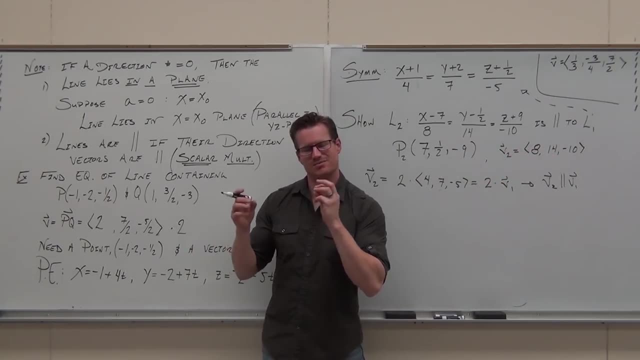 What's that say to you? What's this all say to you? It says, hey, did you catch that? first thing, by the way, It's pretty easy to see. You know, we divide by the 2. That's why this scalar multiple thing is kind of nice, because it's pretty obvious. 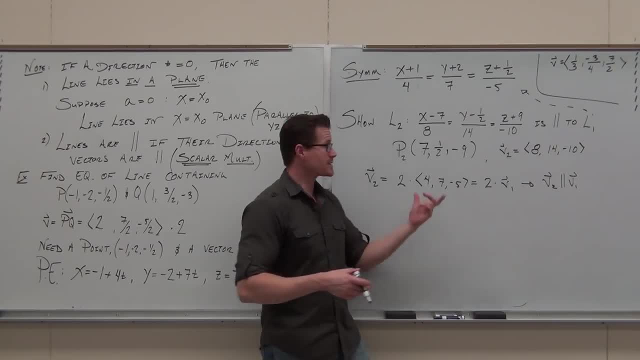 You go. well, that looks like it's 2 times every number. Huh, What's that say? Well, it says that it's literally 2 times every number. It says it's 2 times that vector. It says these vectors are parallel. 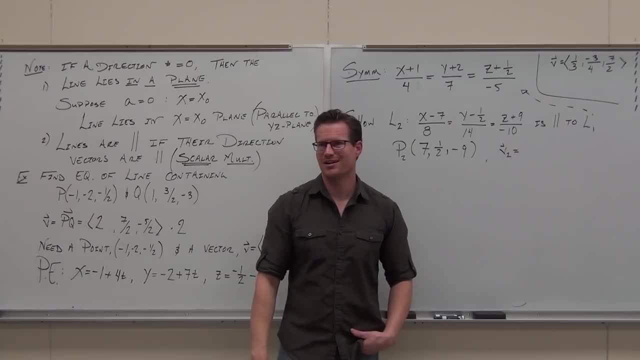 I didn't actually hear you. I just kind of imagined you said negative nine. Did you say negative nine? Yes, I hope so. I should have said: you guys, huh Slackers, Come on now, Left-siders y'all, can you find the vector, the direction vector? 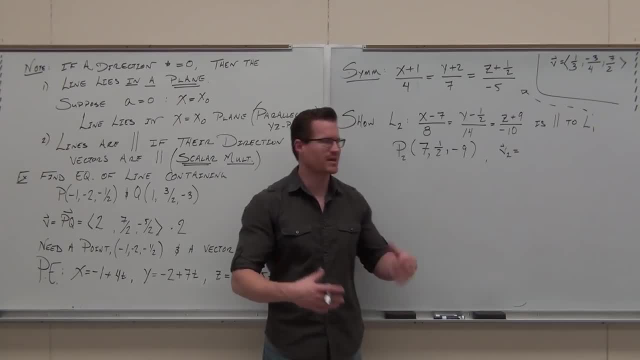 Yes, This is the easy part with this. This is why this format really shines. It's really nice. You know what it is? Denometers, That's all it is, And it's even matched up x, y, z. 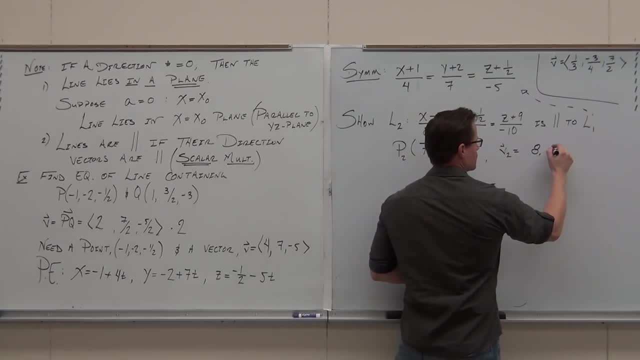 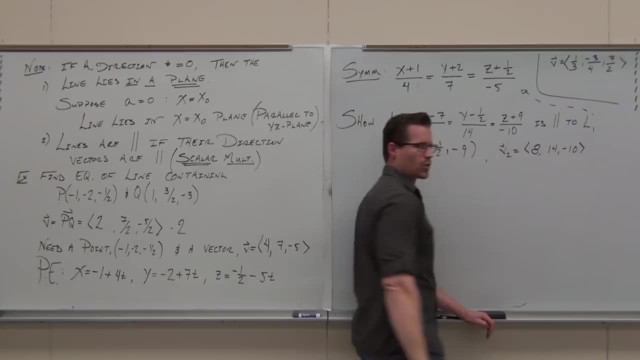 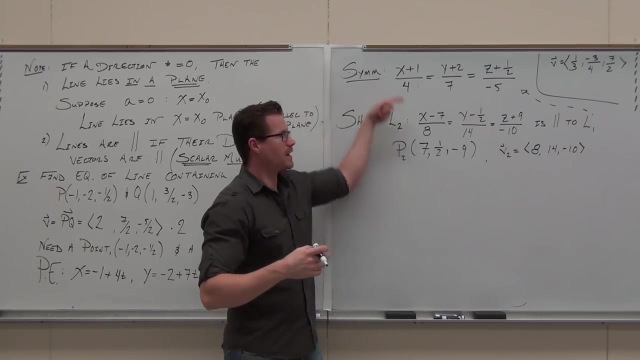 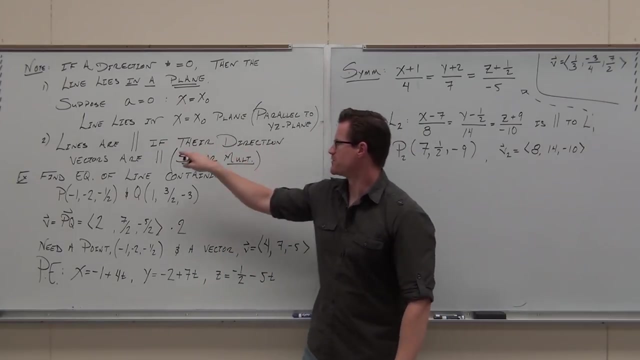 So this is parentheses or vector bracket. They're important. Now next question: Come on, Stick with me here. Are these two lines parallel? Yes, We talked about it earlier. We have a statement up here. Lines are parallel if the direction vectors are scalar multiple. 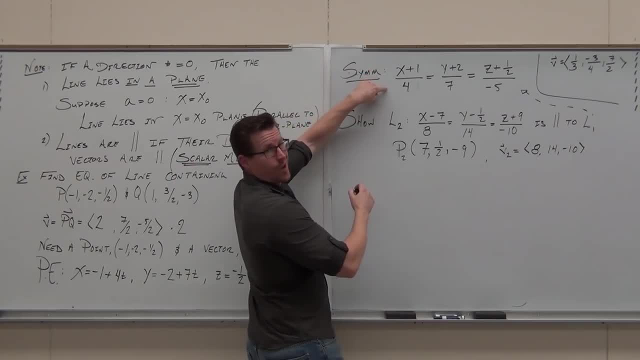 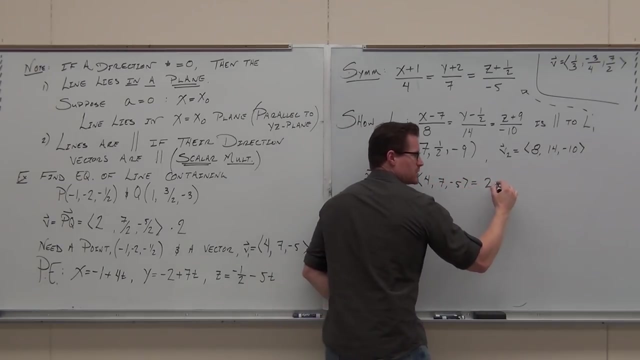 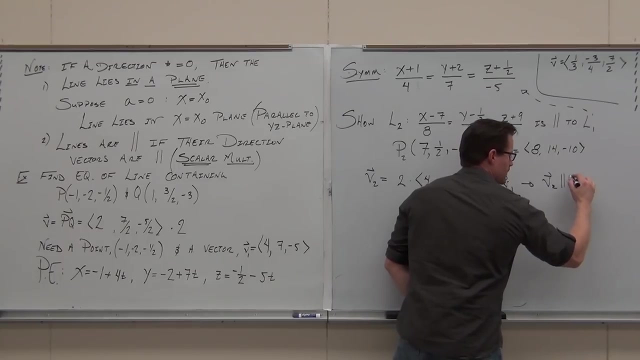 So we're going to write out vector one. We already have that man, It's what we used. So if we call that vector one vector two, this vector is two times four seven negative five. That means it's two times vector one, which means that vector two is parallel to vector one. 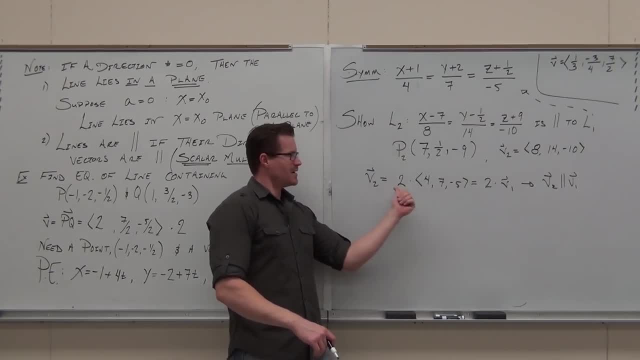 What's that say to you? What's this all say to you? It says, hey, did you catch that first thing? by the way, It's pretty easy to see. You know, we divide by the two. That's why this scalar multiple thing is kind of nice. 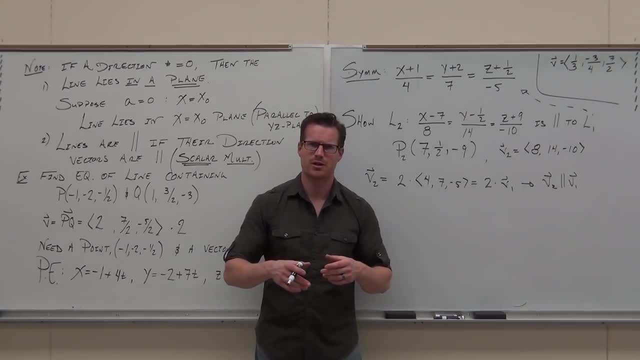 It's pretty obvious. You go: well, that looks like it's two times every number. Huh, What's that say? Well, it says that it's literally two times every number. It says it's two times that vector. It says these vectors are parallel. 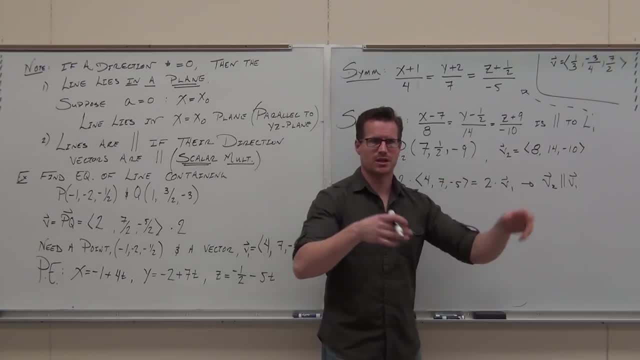 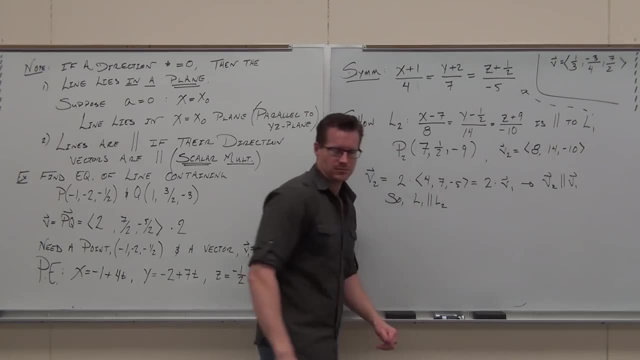 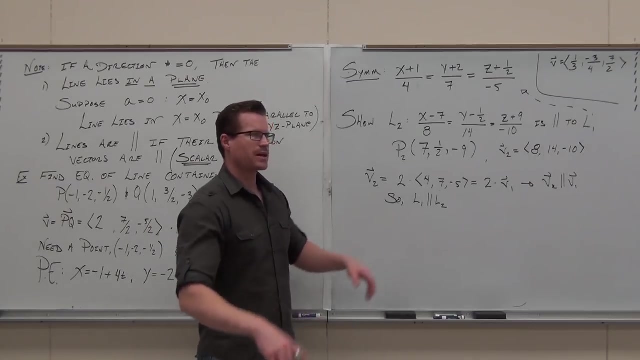 What's it say about the lines? This proves that line 1 is parallel to line 2 or vice versa. I'm not going to ask you to, but if I asked you to, could you take this equation and write it as a parametric equation for the line? 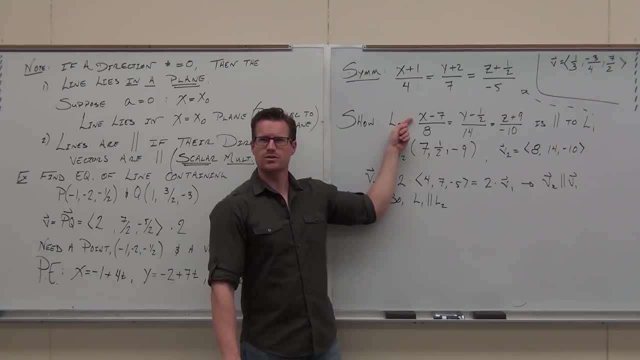 Could you do that? Yes, It would be. x equals 18, 0, 7,. Oh boy, we've got to do it. Okay, well, we're going to do it, We're going to do it. 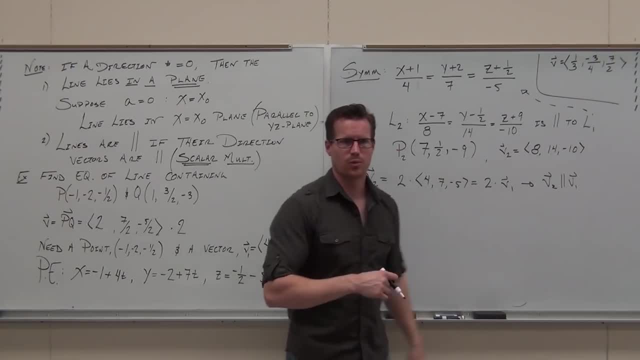 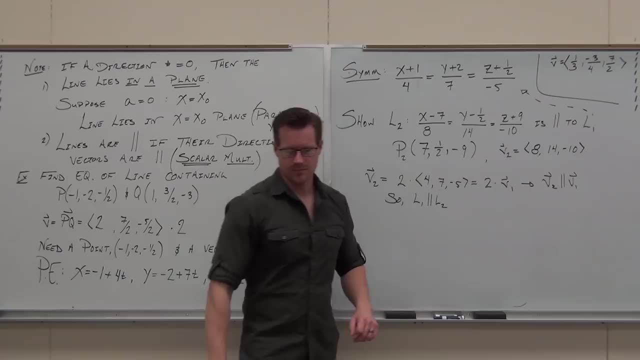 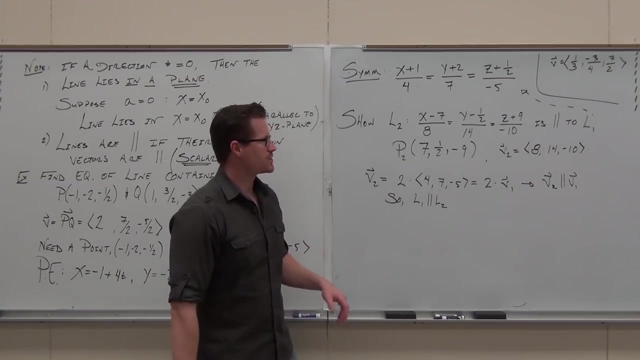 What's it say about the lines? This proves that line one is parallel to line two, or vice versa. Could you go- if I I'm not going to ask you to, but if I asked you to, could you take this equation and write it as a parametric equation for the line? 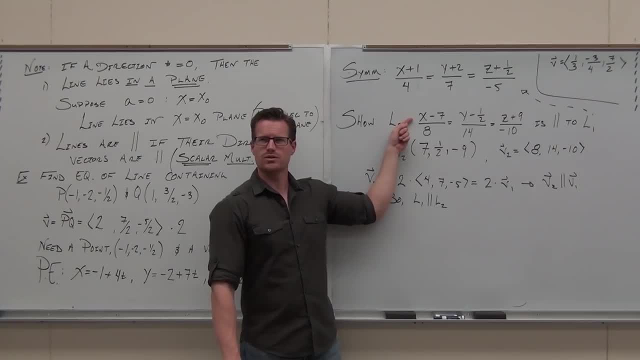 Could you do that? Yes, It would be x equals. Oh boy, we better do it. Okay, we're going to do it. We're going to do it. If you wrote this as a parametric. Sorry, my board work's getting a little sloppy here. 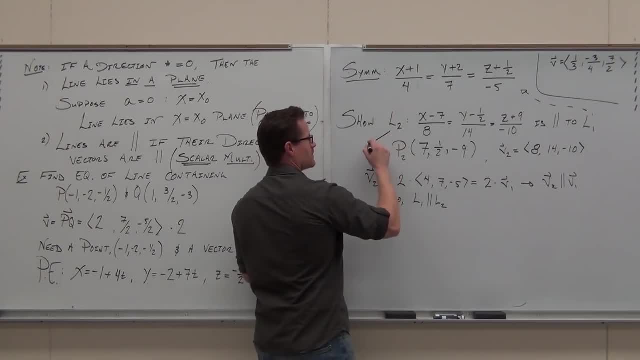 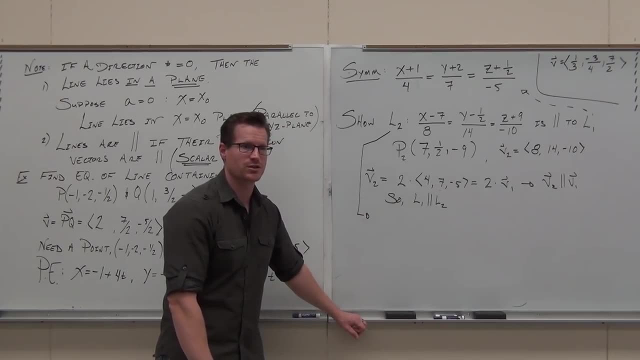 If you wrote this as a parametric. Sorry, my board work is getting a little sloppy here, So I'm kind of thinking about these things on the top of my head. make sure you can actually do them. If you wrote this as a parametric. 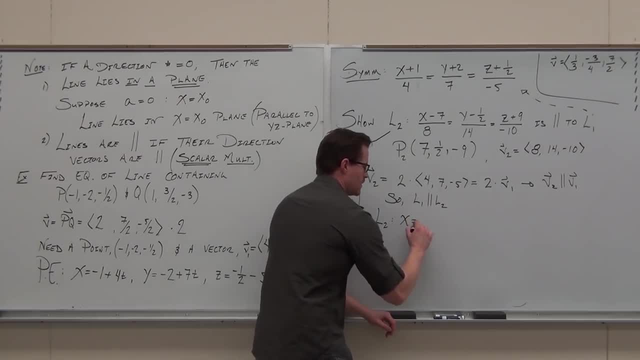 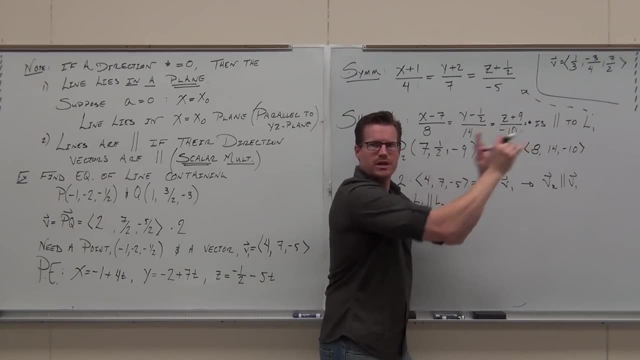 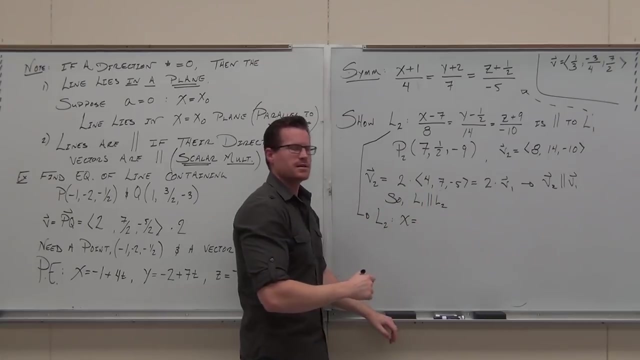 1. You're basically solving for X, and these all equal T. So each individual one, you're equaling that to T and solving for X. So we multiply by 8. Oh, that's 18.. And then we would add the 7.. 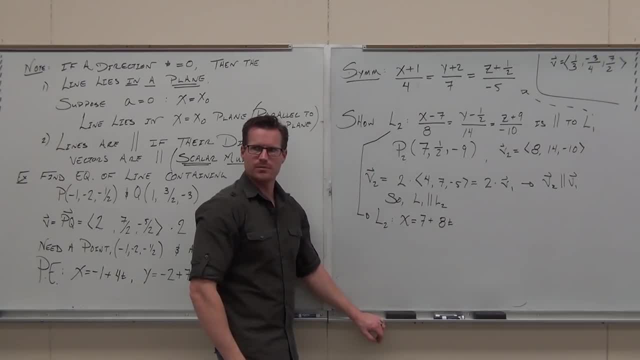 7 plus 18, in that order, You guys. okay with that one. If you didn't catch it the first time, here it is again. You're equaling each of these things to T, because that's how we built this equation. 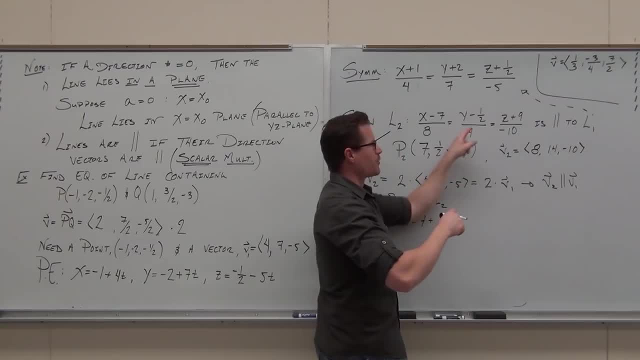 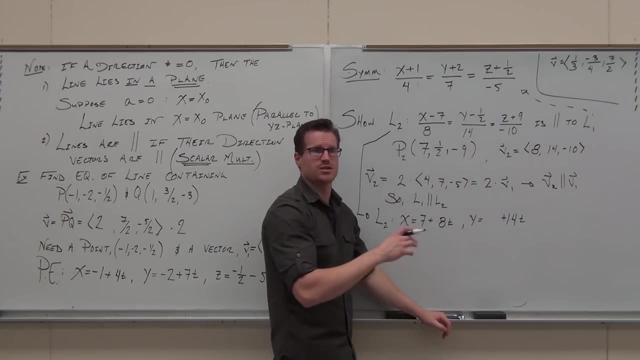 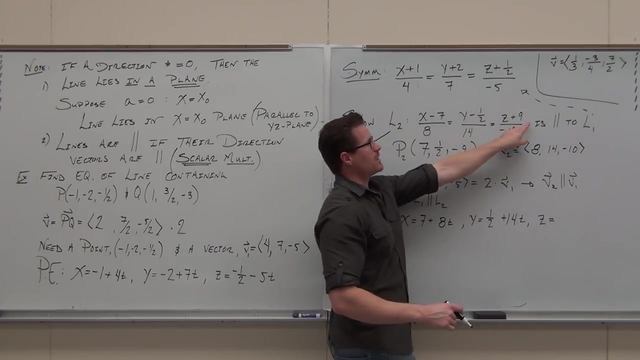 So we multiply 14 times. just imagine the T 14 times T. It's positive, so we're going to have a plus. It's written in this order. And then we would add the 1 half Z, imagine equal to a T. We multiply by negative 10.. 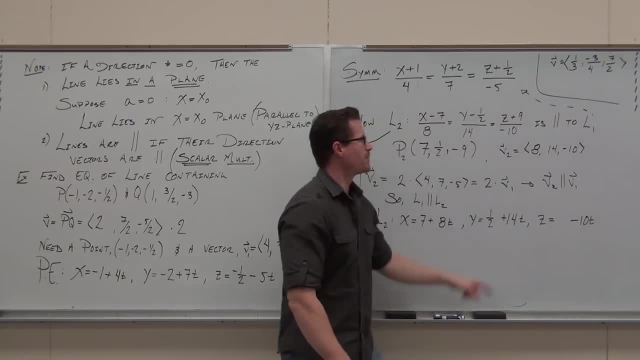 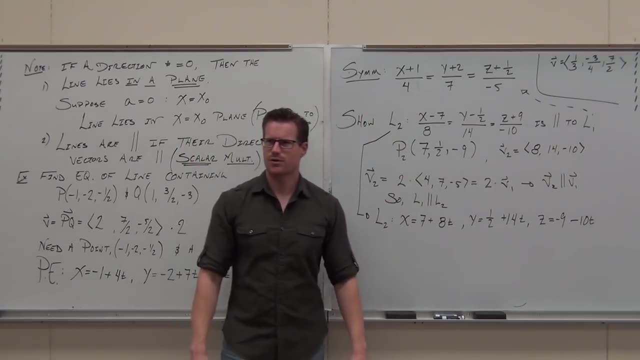 We're going to have a minus 10 T, We subtract the 9. Negative: 9 minus 10 T. Head nod, if you're okay with that one. Are you sometimes going to get different looking lines based on the direction vector that you're using? 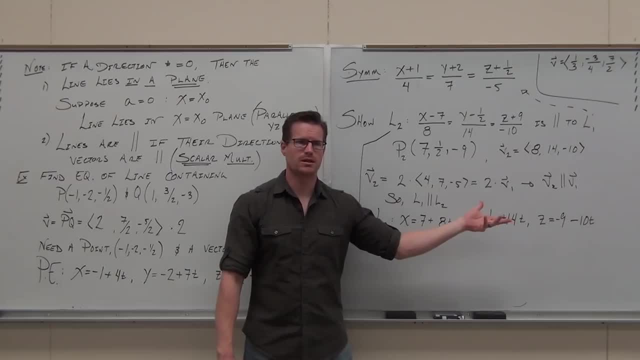 If I chose to use this vector right here, I'd have a different looking line, even though it's the same line, because the direction vector scale, the multiple, is still parallel, still to the same point. We can get different looking stuff If we always simplify our direction vectors. 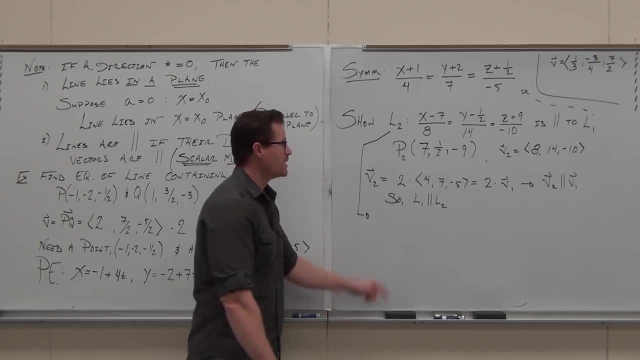 I'm kind of thinking of these things off the top of my head. Make sure you can actually do them. If you wrote this as a parametric, you're basically solving for x and these all equal t. All right, All right, All right. 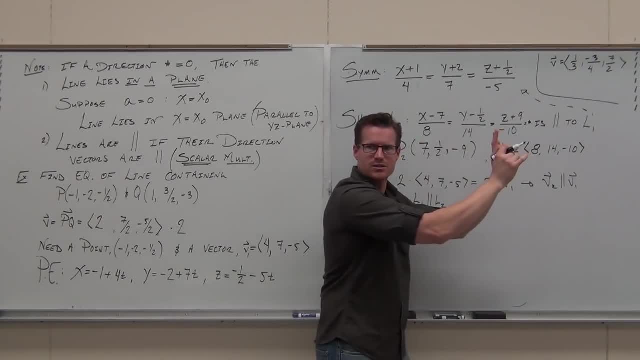 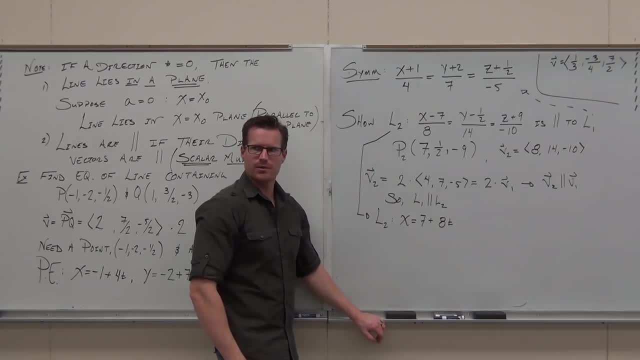 7 plus 18, in that order, You guys? okay with that one. If you didn't catch the first time, here it is again. You're equaling each of these things to t, because that's how we built this equation. So we multiplied 14 times. 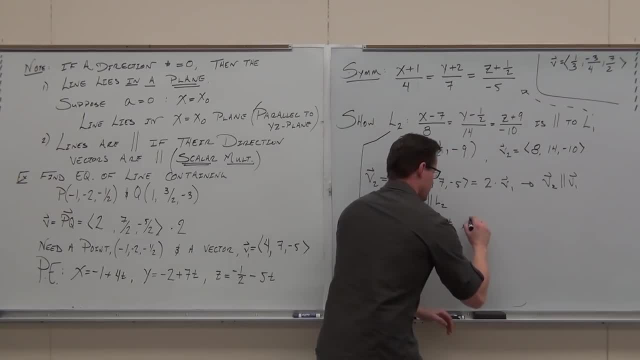 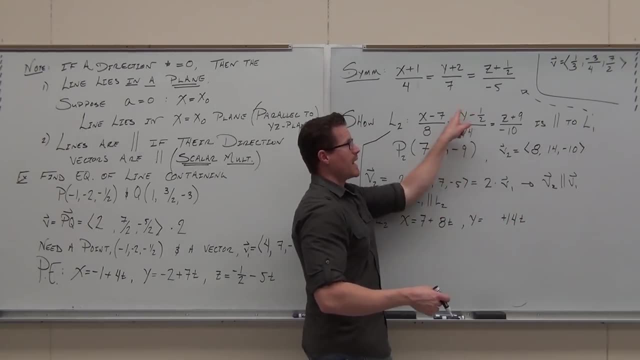 Just imagine the t 14 times times t. It's positive, so we're going to have a plus. It's written in this order. And then we would add the 1 half Z, imagine equal to a t. We'd multiply by negative 10.. We're. 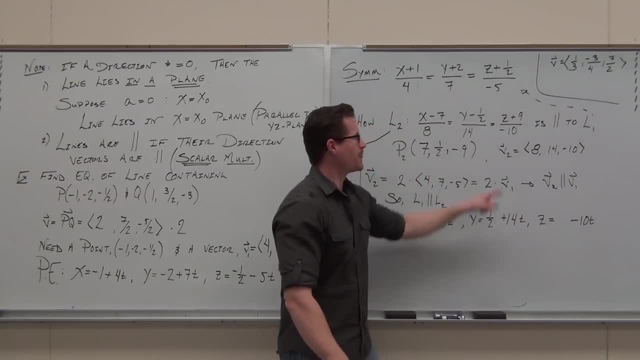 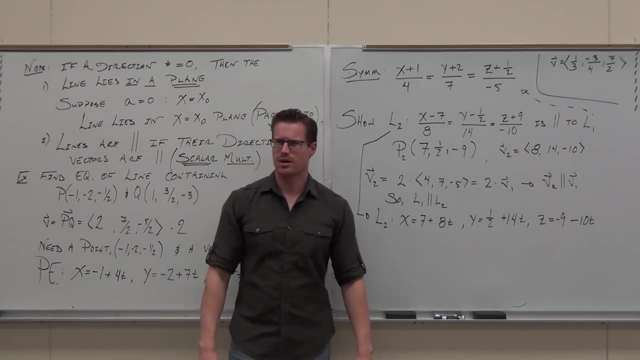 going to have a minus 10 t, We'd subtract the 9. Negative 9 minus 10 t. Head nod, if you're okay with that one. Are you sometimes going to get different looking lines based on the direction vector that you're using? If I chose to use this vector right here, 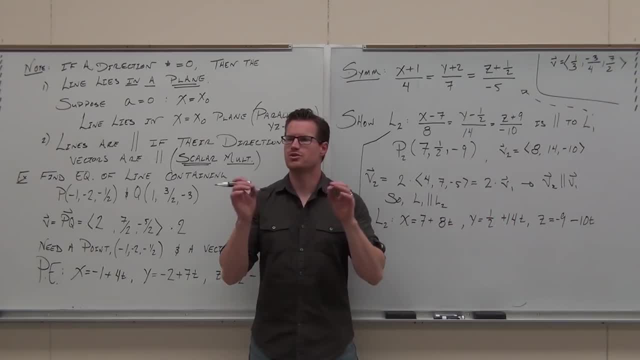 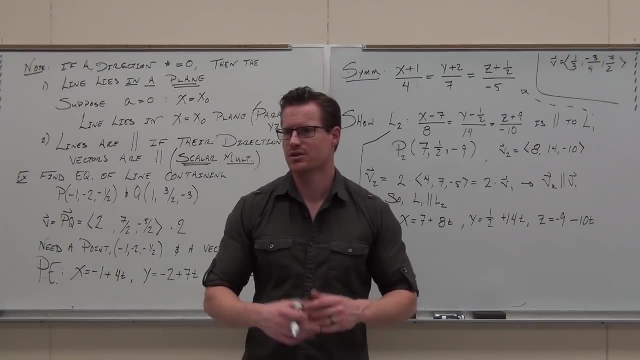 I'd have a different looking line, even though it's the same line, because the direction vector is still parallel, still to the same point. We can get different looking stuff. If we always simplify our direction vectors, then we get the same stuff. Okay, for real, we. 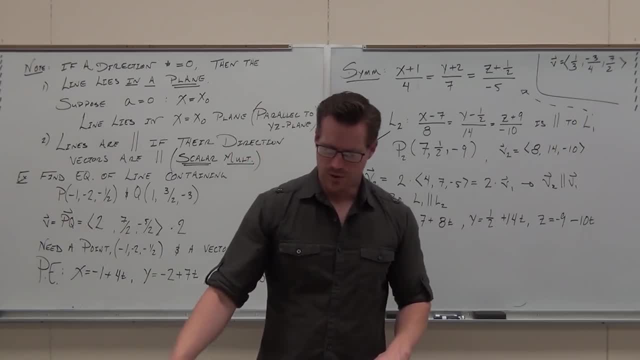 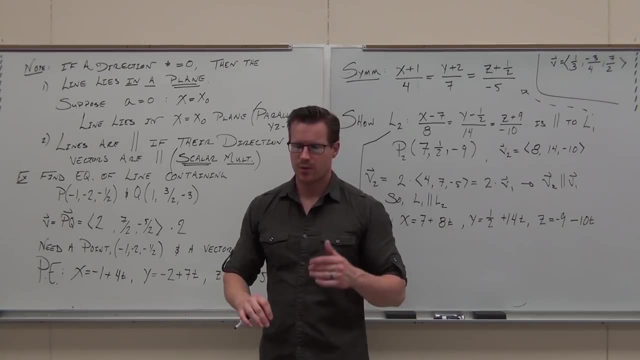 then we get the same. We can get different looking stuff. Okay, for real, we covered a lot. Okay, yes, no, maybe Head nod, if you are What I'd like to do. to wrap all this up, I want to show you one more example. 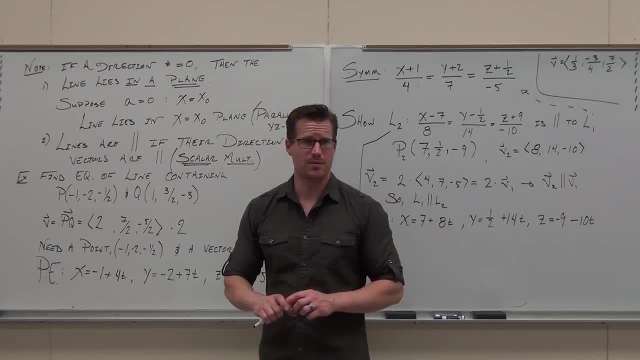 I'm going to put one on the board for our break that I want you to think about, and then we're going to come back and pretty much crush it. It'll be a very similar example. I know we're going to go past our break a little bit. 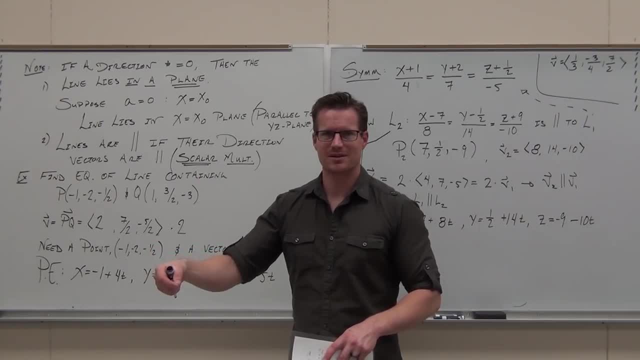 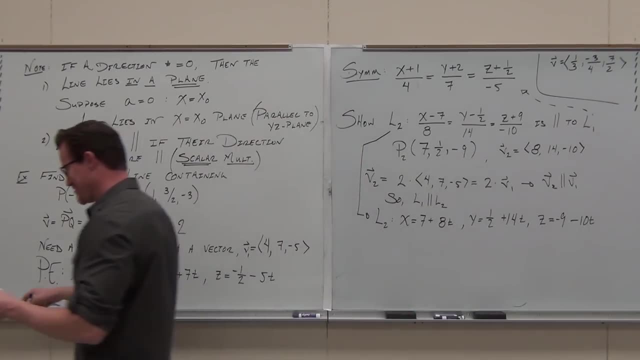 but right now I think it's fresh and I really want to do it. You guys with me May as well just say yes, because we're going to anyway. So yeah, I trust you, Professor Leonard, Let's do it. 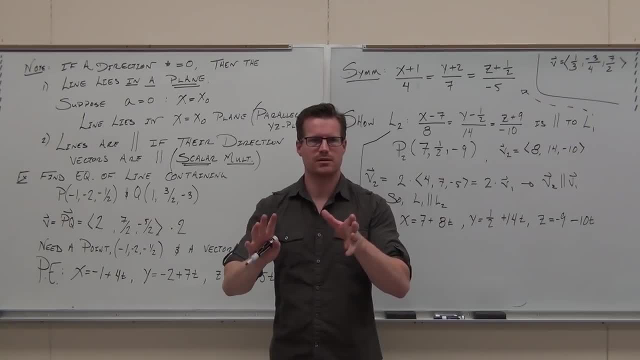 covered a lot. Okay, yes, no, maybe Head nod if you are. What I'd like to do to wrap all this up, I want to show you one more example. I'm going to put one on the board for our break that I want you to think. 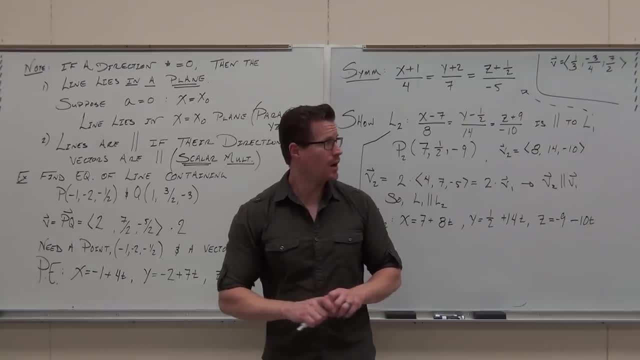 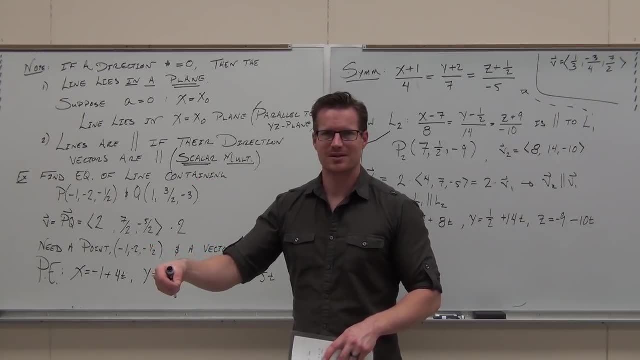 about and then we're going to come back and pretty much crush it. It'll be a very similar example. I know we're going to go past our break a little bit, but right now I think it's fresh and I really want to do it. You guys with me May as well just say yes, because 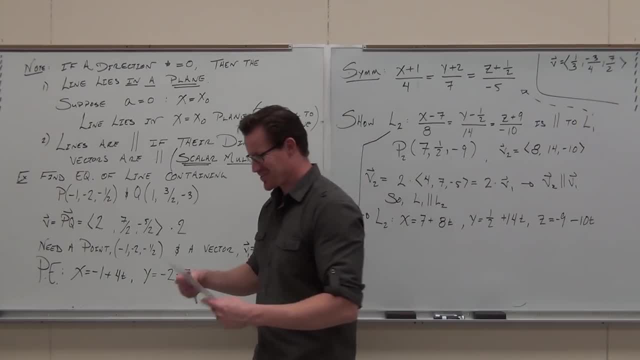 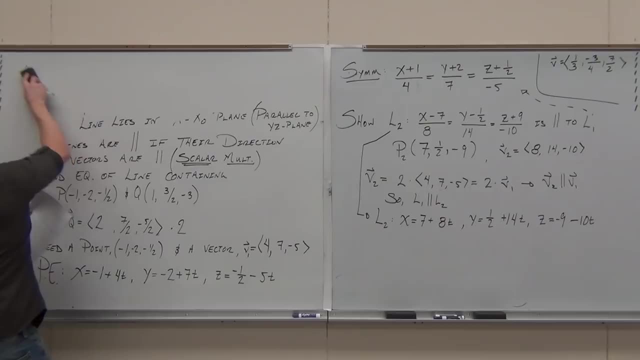 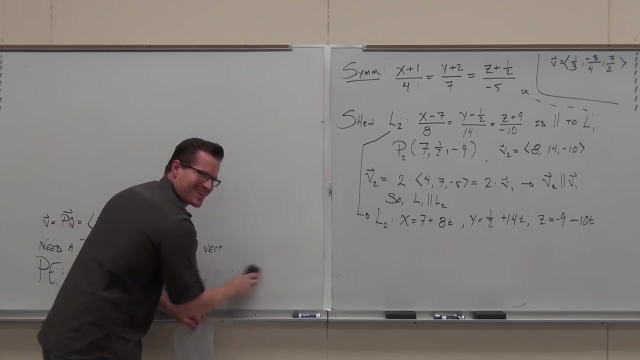 we're going to anyway. Yeah, I trust you. Professor Leonard, Let's do it Now. I'm putting words in your mouth. I love Calculus 3. Best class ever. I even got a woo Woo. That was the lamest woo I've ever heard. You go for Space Mountain, you end. 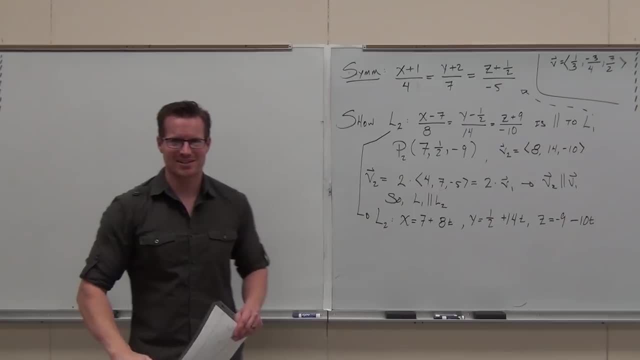 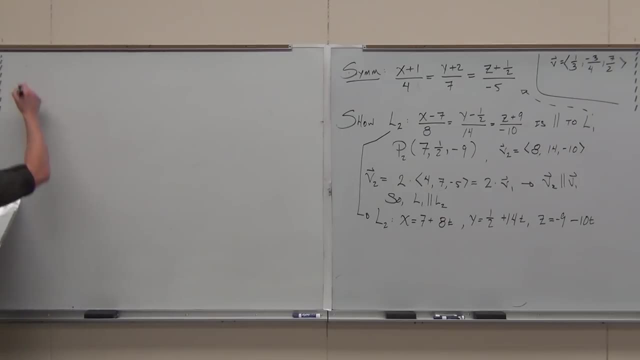 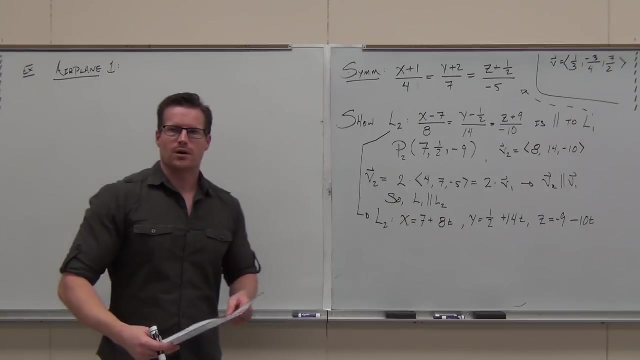 up on the teacups. That was the woo I just got. Yeah, Thanks a lot. All right, I love the teacups. actually, I think they're amazing. For a period of time we're going to imagine these airplanes are flying in a straight line. 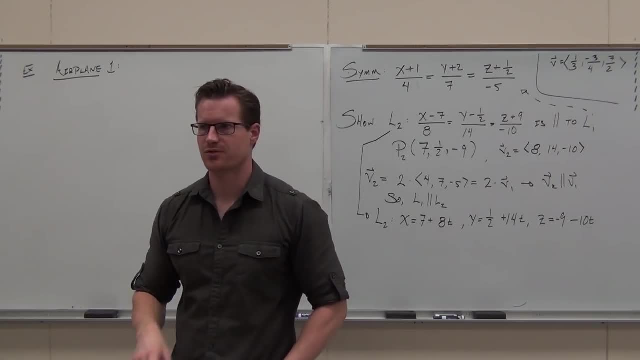 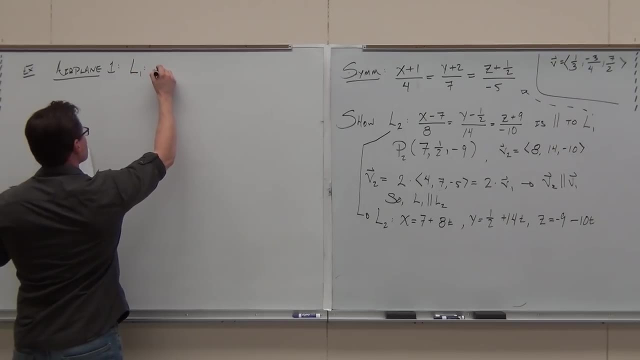 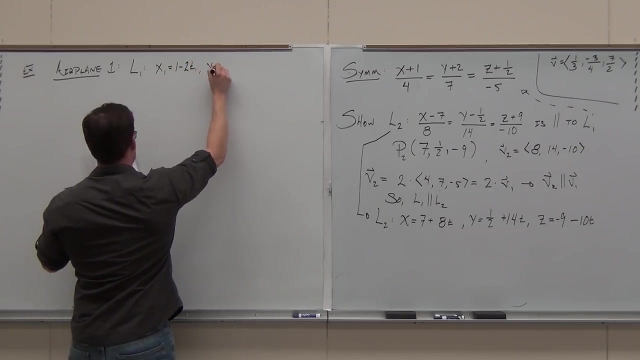 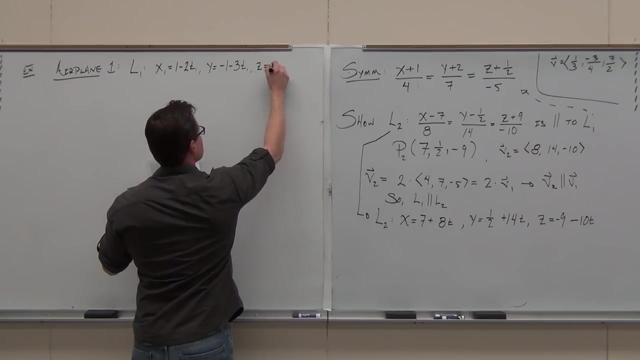 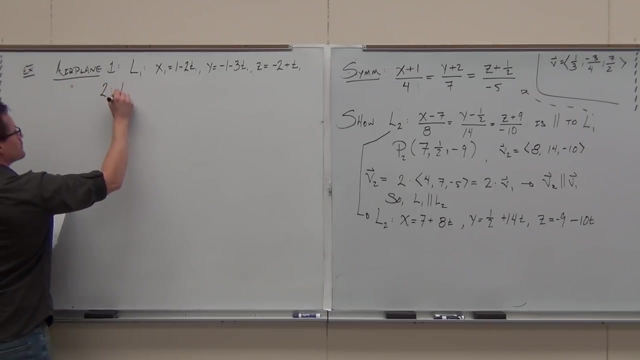 Of course they go around the Earth right, But for a period of time we're going to imagine them flying on a straight line. All right, All right. Now were going to do the one on the left, but you're on the right, so I'm just going. 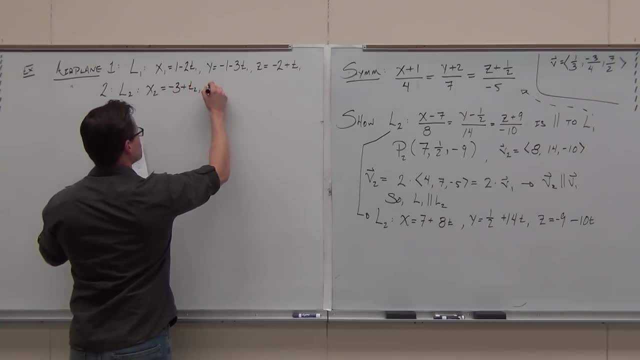 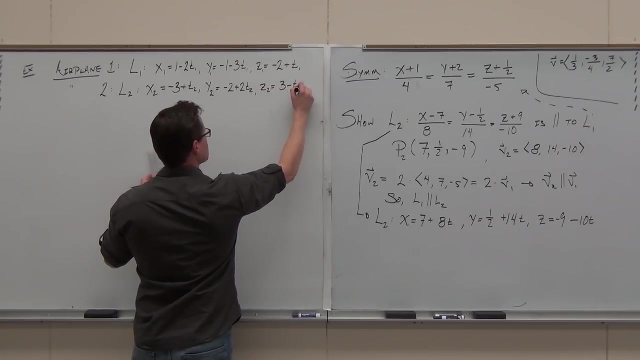 to move these and put them in your face. Needle out. Oh, wow, Yeah, Wow, All right, All right, A couple more questions. A couple more questions, Okay, All right, Okay. One is: what does the moon's red light look like on us at noon? 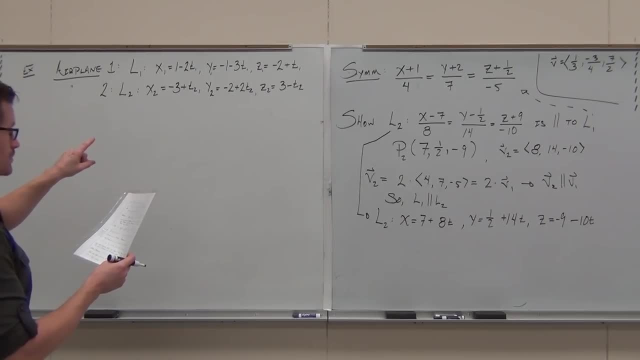 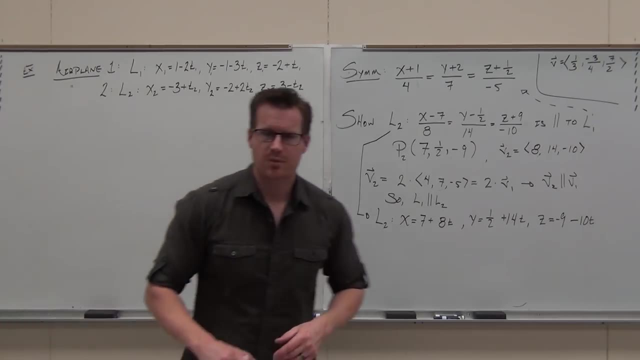 Well, for a moment I'd say the moon. I like the way it looks. What's going on, Okay? Okay, so two airplanes. These airplanes are going to go through certain points, They're going to have certain direction. vectors: 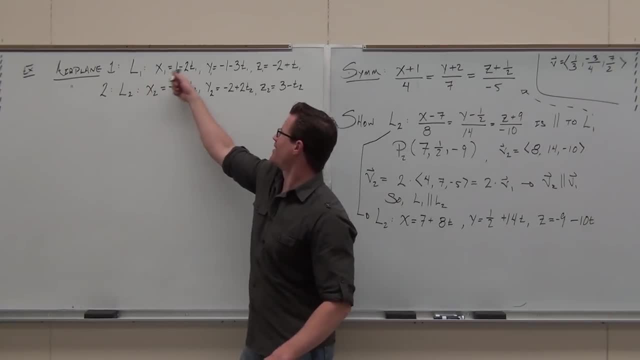 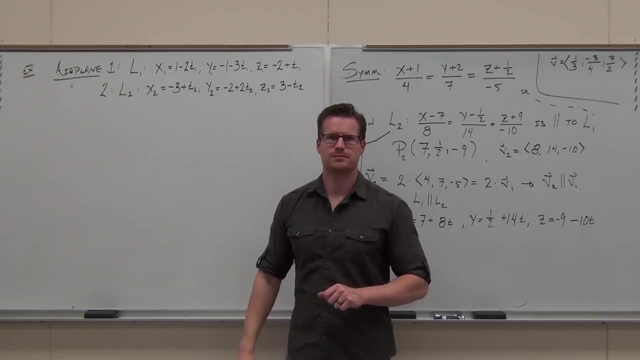 They're going to be flying in a certain direction. So we have plane one, all the little ones. Plane two, all the little twos With me. yes, no, Here's a question: Do they crash? It's a pretty pertinent question. 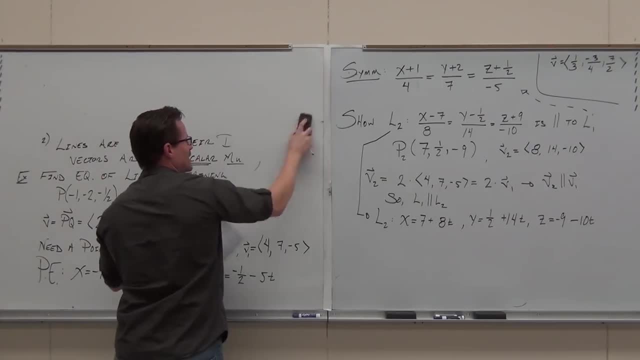 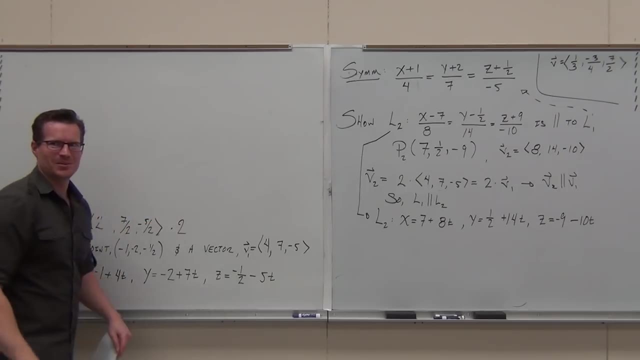 Now I'm putting words in your mouth. I love Calculus 3. Best class ever. I even got a woo Woo. That was the lamest woo I've ever heard. You go for Space Mountain, you end up on Space Mountain. 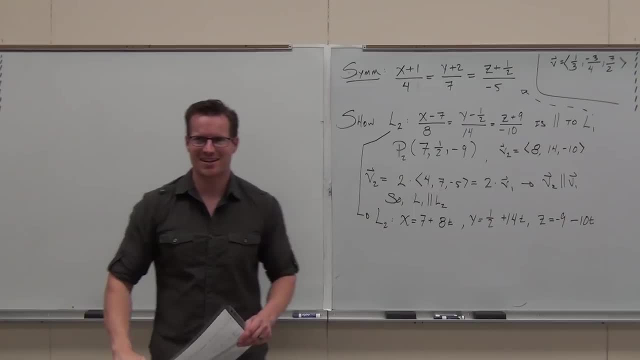 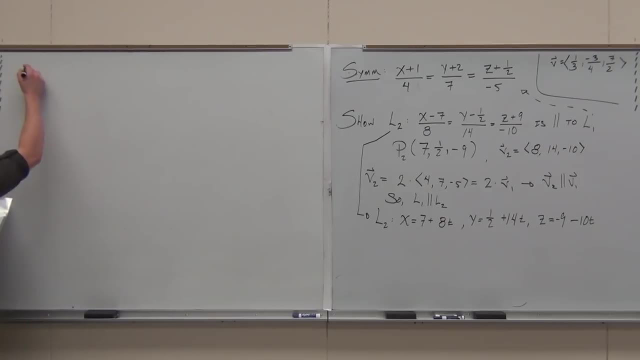 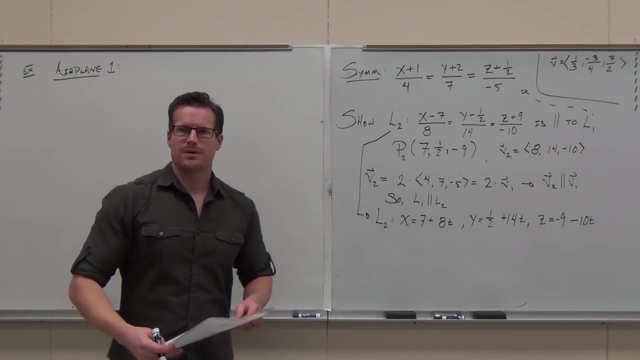 You end up on the teacups. That was the woo I just got. Yeah, Thanks a lot. All right, I love the teacups. actually, I think they're amazing. For a period of time, we're going to imagine these airplanes. 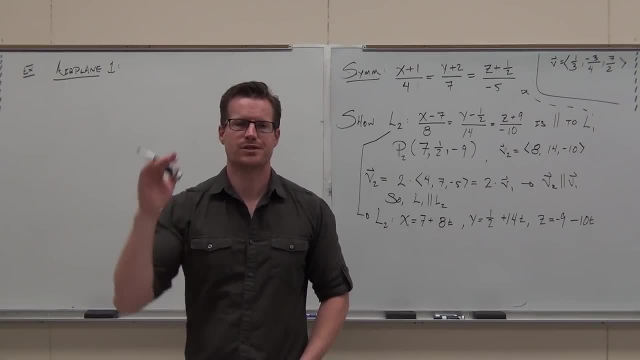 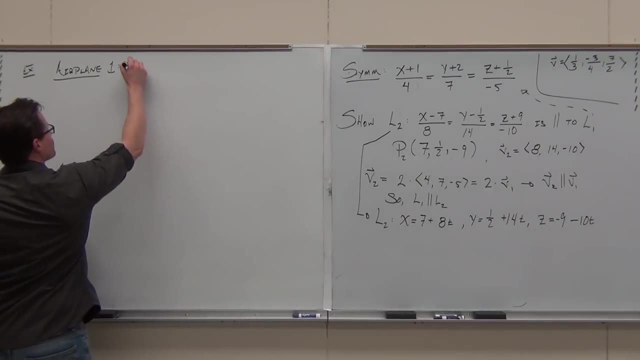 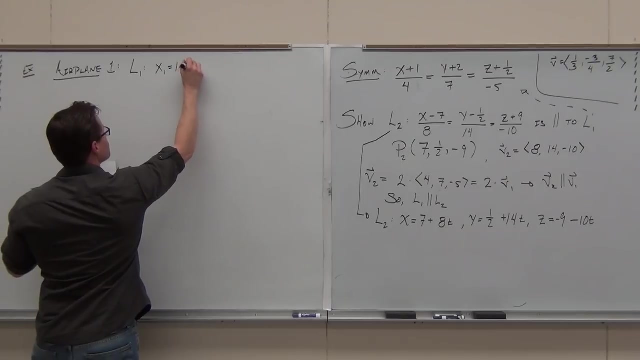 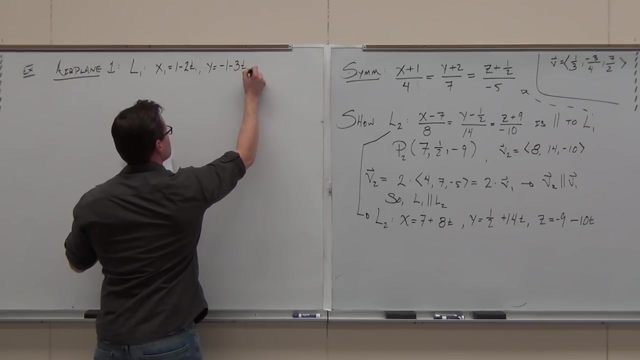 are flying in a straight line. Of course the go around the Earth, right, But for a period of time we're going to imagine flying in a straight line. Okay, Can you guys see? I'm going to show you how to do it. 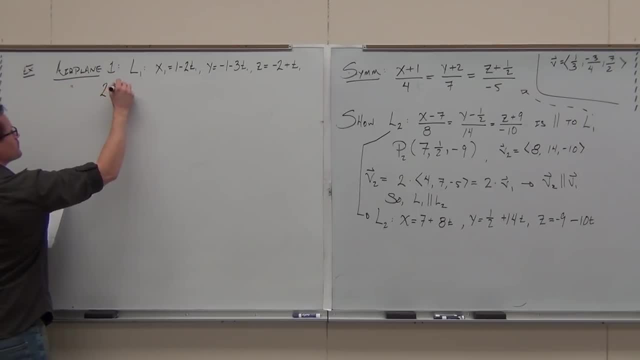 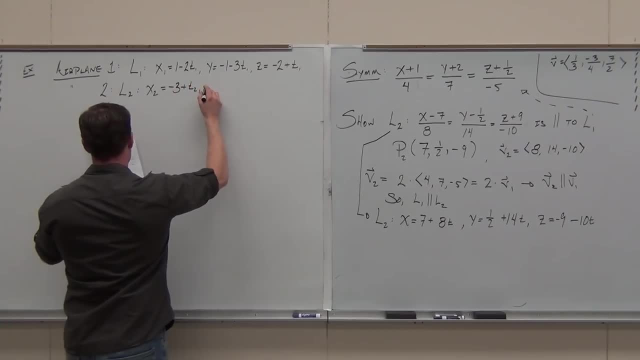 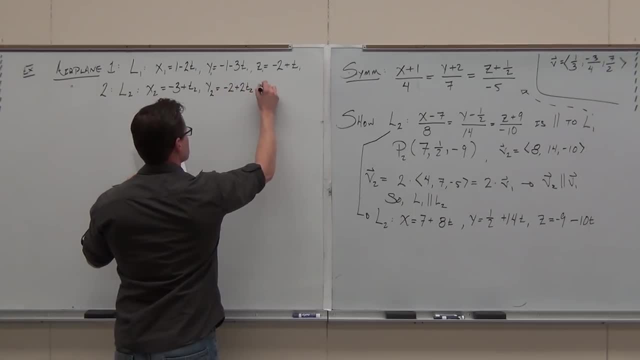 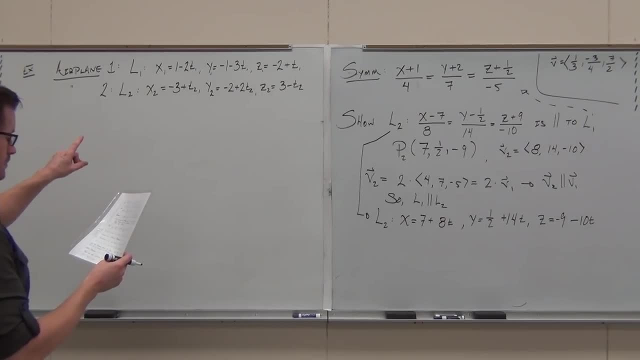 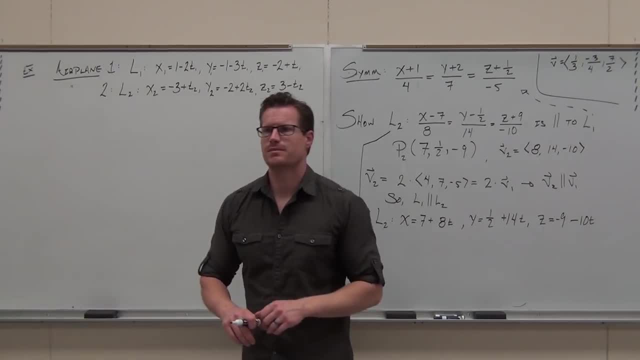 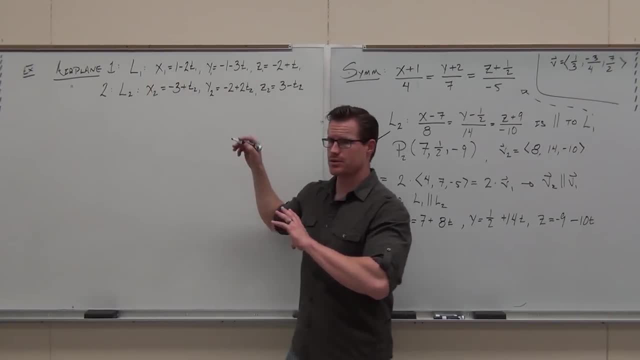 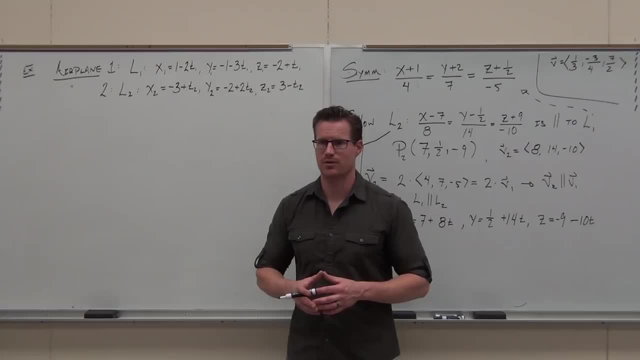 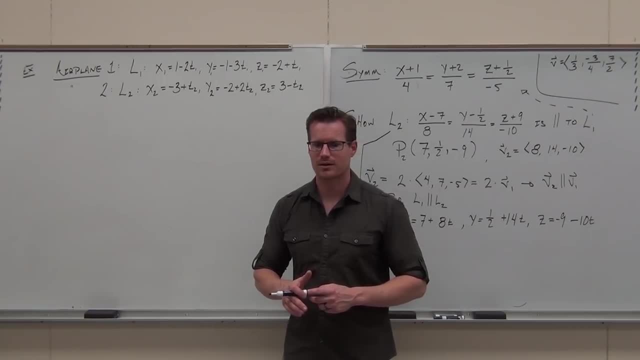 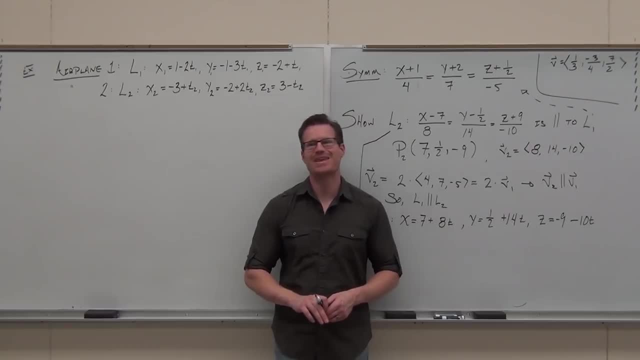 I'm going to show you how to do it. I'm going to show you how to do it. have to hate each other, That's eye roll, My wife awesome eye rolls Like seriously. I see them every day. Love you, baby, Three times a day: Morning, twice at night, Anyhow. 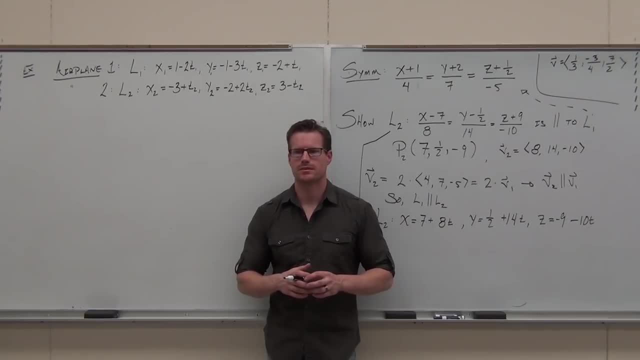 No, seriously, though, What has to happen for planes to crash? They have to intersect, Of course. What's that mean? It cannot be parallel, Okay, that's true. Are non-parallel planes, for sure, intersecting? If that happened, none of you would ever fly, ever. Or if you. 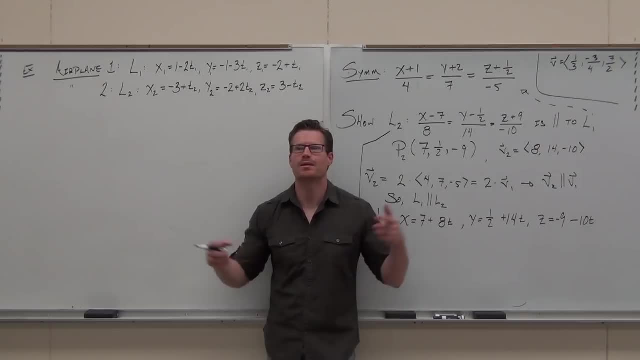 did, it'd only be once, Because a lot of planes do this Seventh favorite dance move. This is why we get to do disco, because our arms don't all the time Really hurt. actually, No, not necessarily parallel, Even. even. what if they did this? 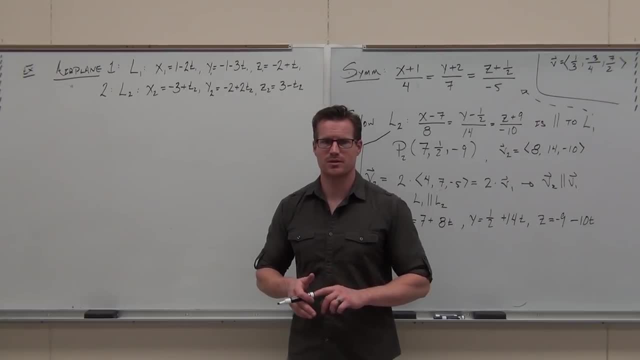 I don't want to be on a freaking plane and have it crash. You guys are going to buy me a ticket to Disneyland so I can go on the teacups right, Probably going to fly. I'm going to drive all the way down there. 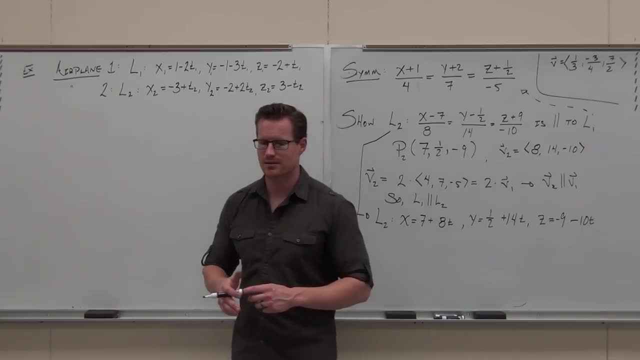 So I don't want to crash. Hello Goodness, Sickos, Don't you want to know, Are they going to crash? What has to happen for two planes to crash, They do have to hit each other. Yeah, That's eye roll. 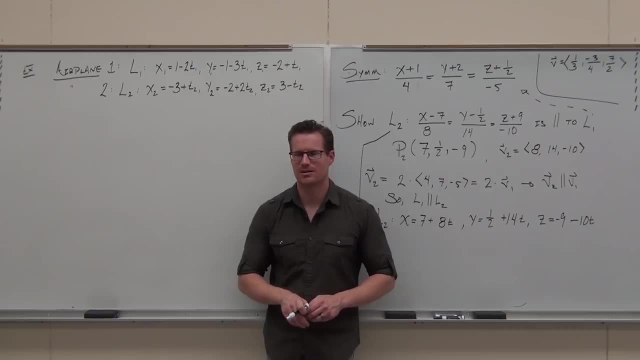 My wife awesome eye rolls Like seriously. I see them every day. Love you, Love you, baby, Three times a day, Morning, twice at night, Anyhow, no. seriously, though, What has to happen for planes to crash? 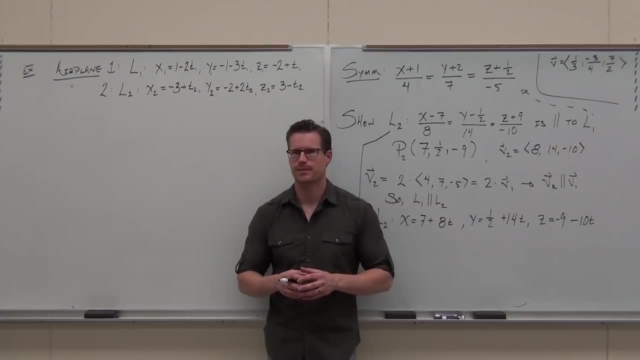 Intersect. They have to intersect, Of course. What's that mean? It cannot be parallel. Okay, That's true. Are non-parallel planes for sure intersecting? I have a point of view: If that happened, None of you would ever fly, ever. Or if you did, it would only be once. Yeah, Well, it depends, Because a lot of planes do this. It depends on the thyroid Seventh favorite dance move, Mm-hmm. This is why we get to do disco, because our arms don't all the time. 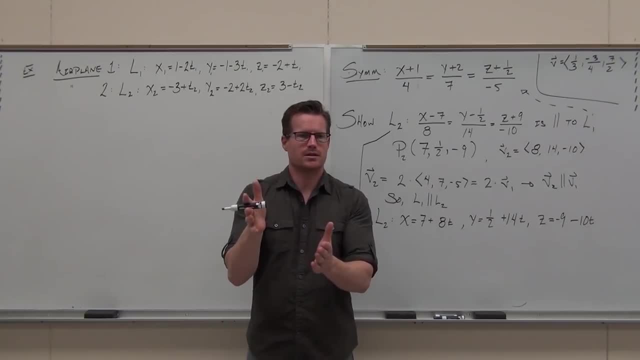 They really hurt, actually, No, not necessarily parallel, Even even. what if they did this? Woo Woo, Woo, Woo Woo, Just like that? Same point, They're crossing, a same point, Are they hitting? So, in order for us to intersect an actual crash? 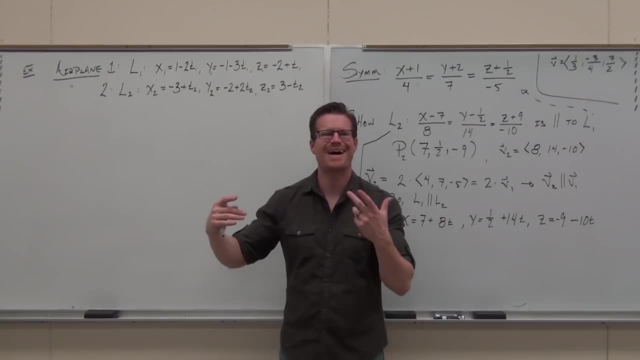 like an intersection in three space. with parametric, there's a time associated with it. It's like our times are different. This one took off. It's traveling at a certain, after a certain period of time from its takeoff. This one's taking off later or sooner. who care? 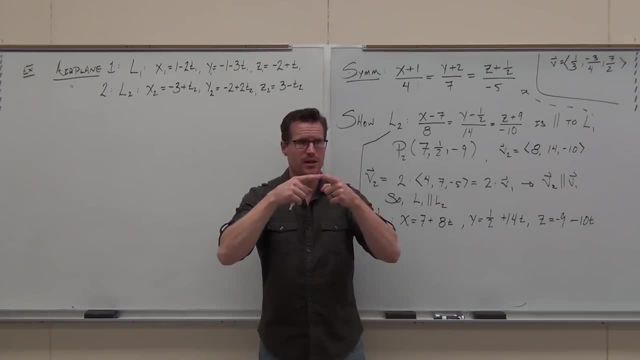 But at a certain time. So we need the things to hit the certain point at the exact same time. Does that make sense? That's an aspect of it that we don't have in 2D, really, unless we're talking about parallelism. 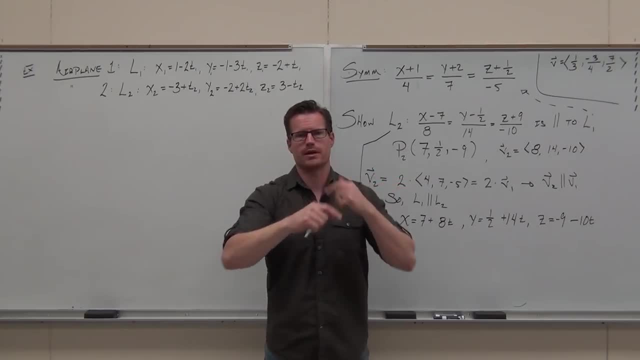 Same point, They're crossing a same point Are they hitting? So in order for us to intersect an actual crash, like an intersection of three space with parametric, there's a time associated with it. That's why our times are different. This one took off, It's traveling for, at a certain 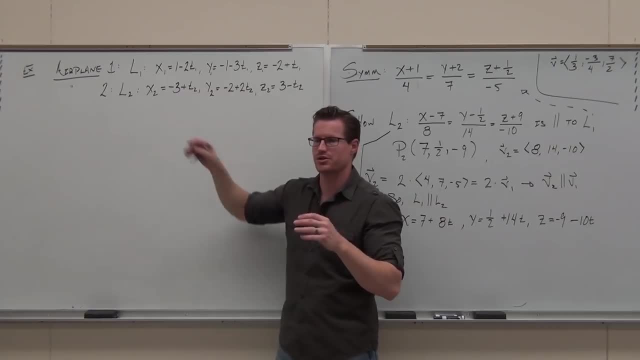 after a certain period of time from its takeoff. This one's taking off later or sooner, who cares- But at a certain time. So we need these things to hit a certain point at the exact same time. Does that make sense? That's an aspect of it that we don't have in 2D, really. 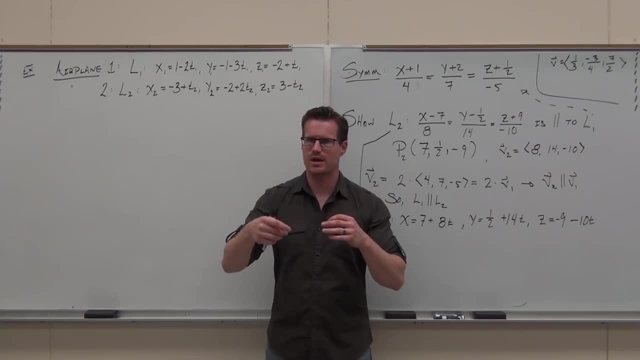 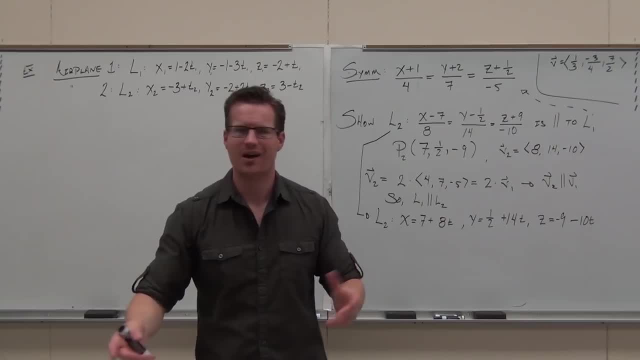 let's figure it out. This is where our, our practice comes in. You have lines Done, But let's think about intersections now. Let's think about how do we tell when they cross a, a, a coordinate plane, How do we do that stuff? So number one thing. so, in order for 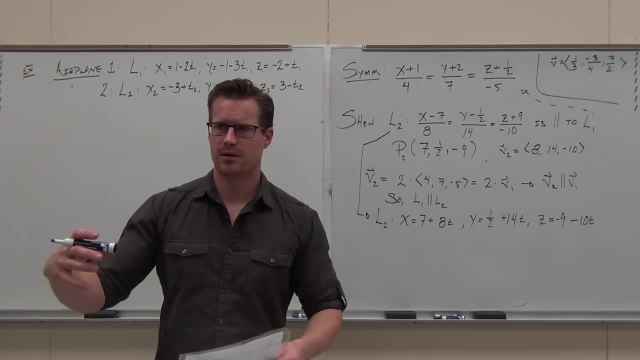 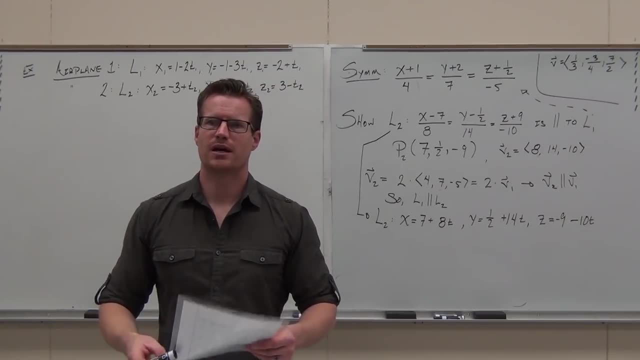 them to to intersect. they have to cross the same point, They have to cross at the same time. Do I understand what I'm, what I'm talking about? Okay, First thing you want to check? let's check if they're parallel, because I do know. 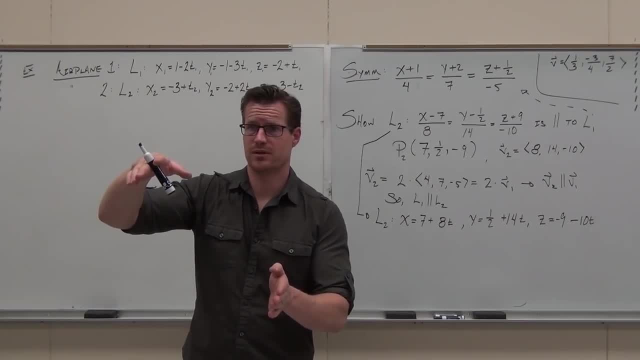 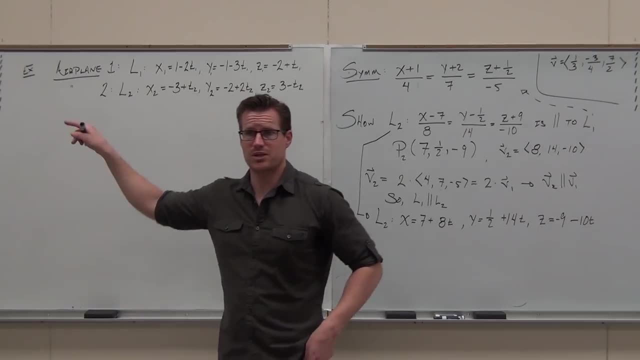 this: If our planes are parallel, we don't have to bother with the rest of it, Because if our planes are parallel, they are not crossing. Does that make sense? Check parallel right now. What I want you to do: write down the direction vector for plane one. I want you. 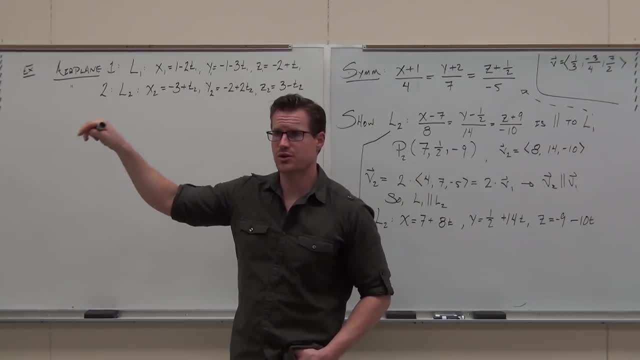 to write down the direction vector for plane two. This is not just trivial. Make sure you can write down the direction vector for plane one and the direction vector for plane two, And I want you to check whether the lines are parallel right now. Go for it, I'm going. 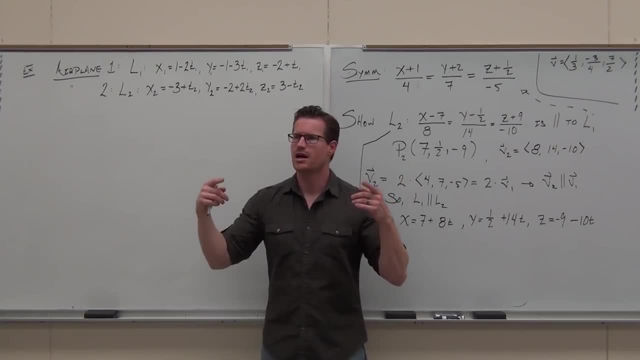 parametric in 2d, and then we do. but with parametric we have this: in order to get an intersection, you have to have same point at the same time. how in the world do we do that? well, let's, let's figure it out. this is where our practice comes in. 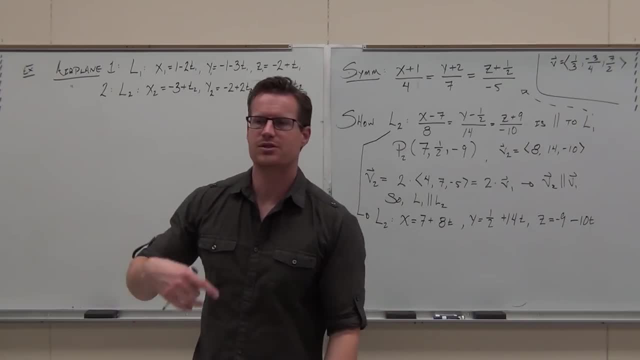 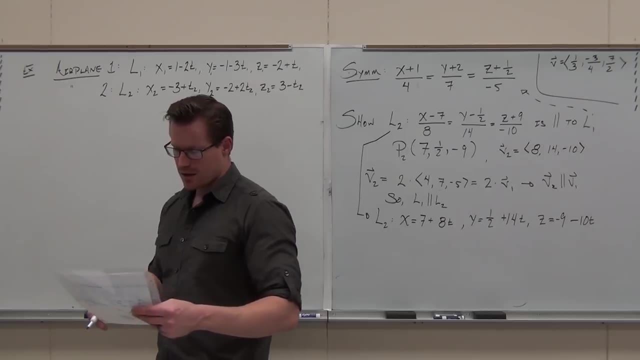 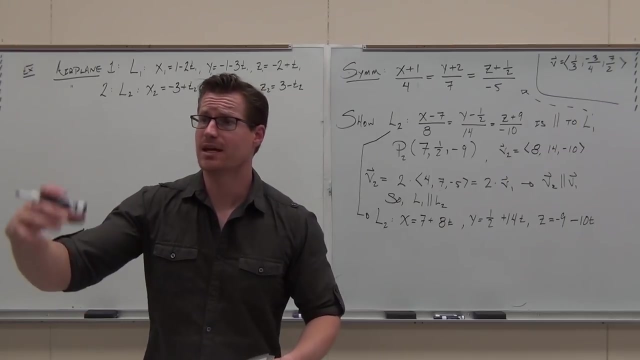 you have lines done, but let's think about intersections now. let's think about how do we tell when they cross a coordinate plane, how do we do that stuff? so number one thing: so remember them to intersect. they have to cross the same point, they have to cross at the same time. I understand what I'm talking about. 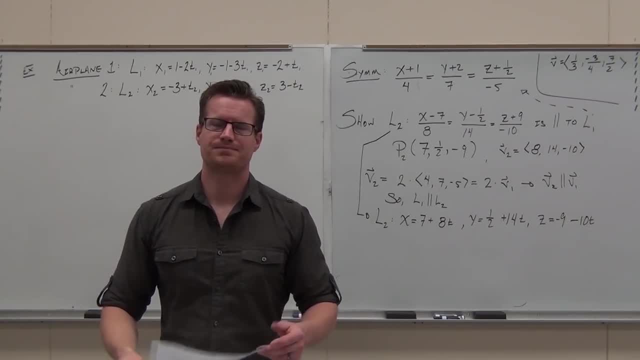 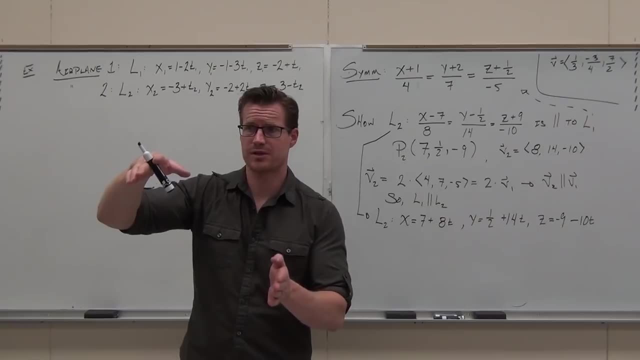 okay, first thing you want to check, let's check if they're parallel, because I do know this: if our planes are parallel, we don't have to bother with the rest of it, because if our planes are parallel, they are not crossing. does that make sense? check parallel right now. what I want you to do: write down the direction vector. 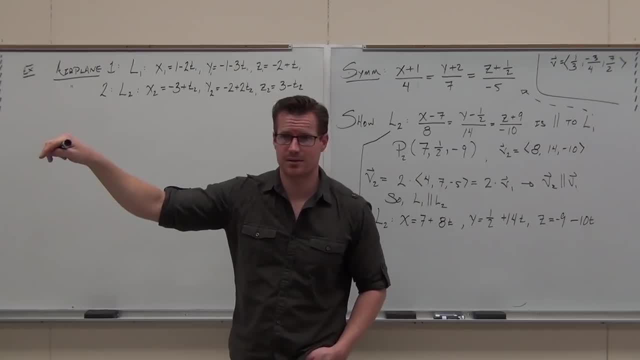 for plane one. I want you to write down the direction vector plane. this is not just trivial. make sure you can write down the direction vector for plane one and the direction vector for plane two and the direction vector for plane three. plane two and I want to check whether the lines are parallel right now. go for. 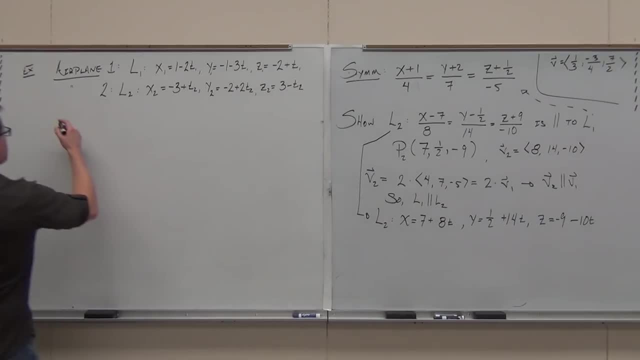 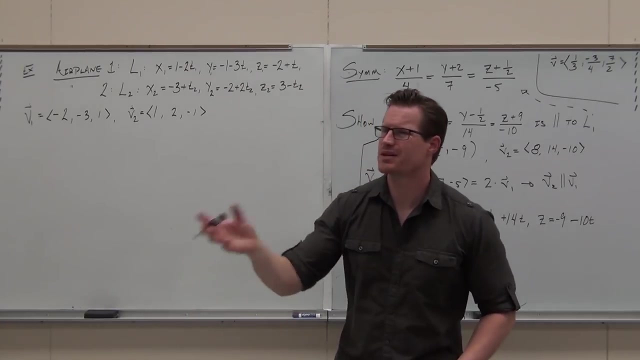 it. I'm gonna do on the board as you're doing it, because you shall be doing on your own. lines are super nice because they have the points and they have the direction vectors built in. just don't mix them up. okay, don't use points for direction. 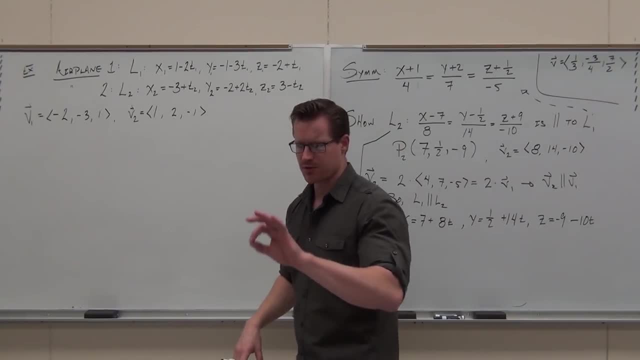 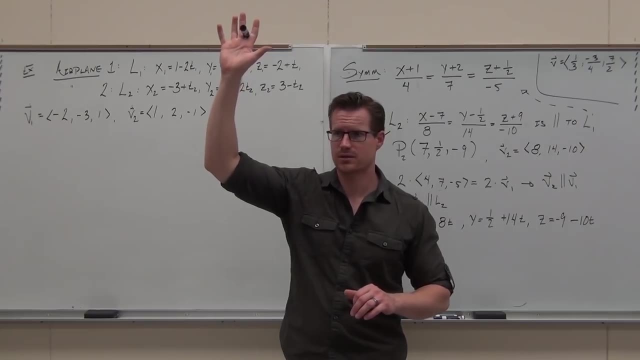 vectors and vice versa. in our case, the the ones I got was negative, two negative three, one for plane one and one, two negative one for plane two. show of hands: if you get the same thing I got, yes, no, that's fantastic. now it's pretty easy to see whether. 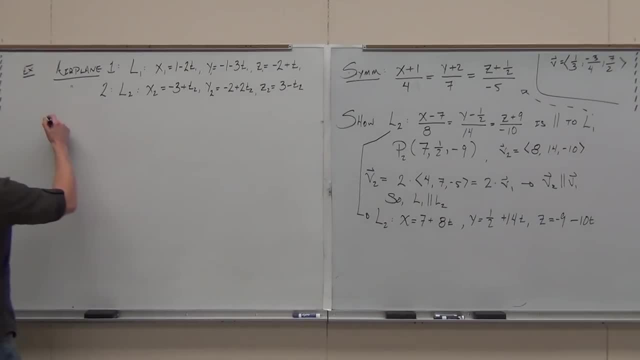 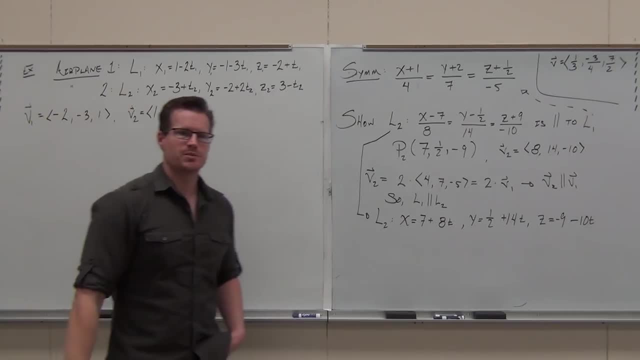 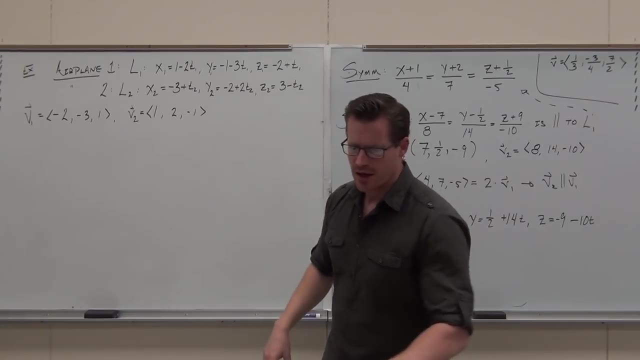 Okay, Lines are super nice because they have the points and they have the direction vectors built in. Just don't mix em up. Okay, Don't use points for direction vectors, and vice versa. In our case, the ones I got was negative two negative three, one for plane one and 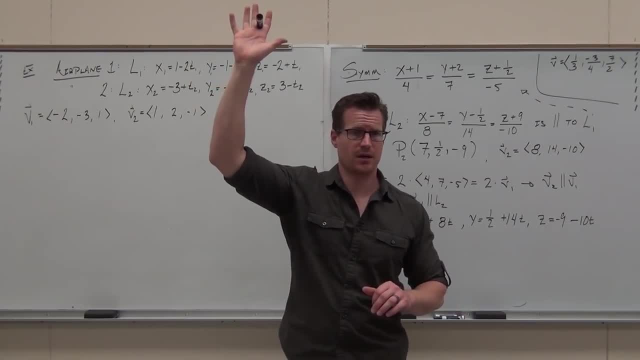 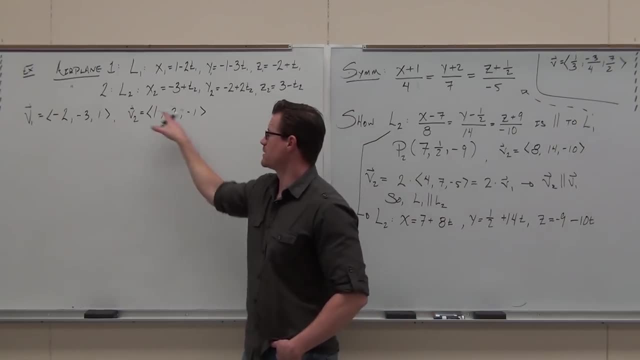 one, two negative one for plane, two Show of hands: if you got the same thing, I got. Yes, That's fantastic. Now it's pretty easy to see whether they're parallel or not. Are these two things, two vectors, parallel? 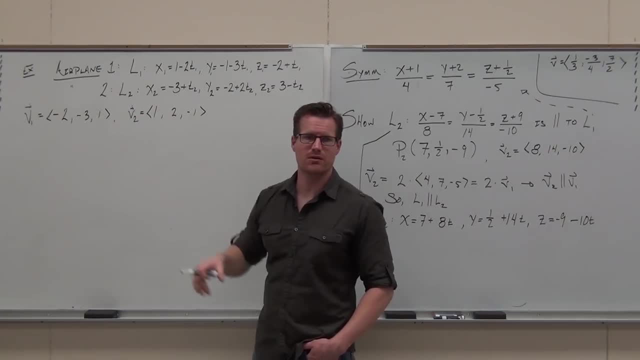 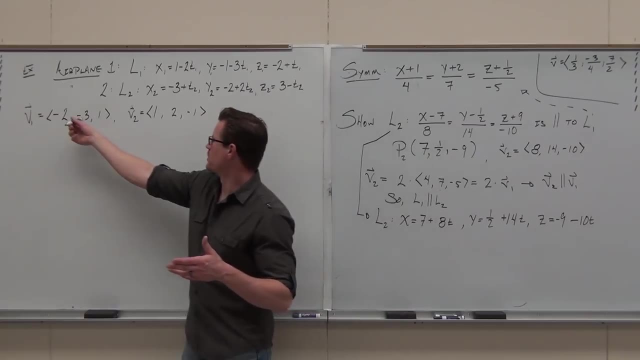 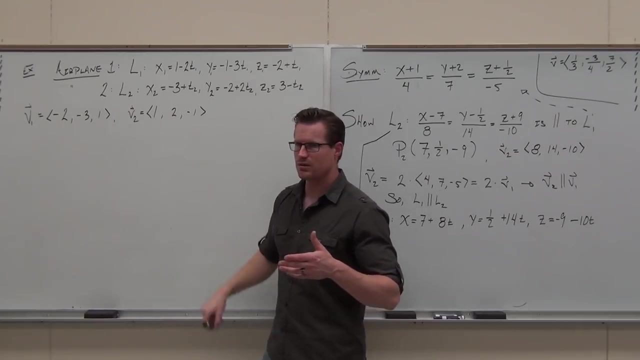 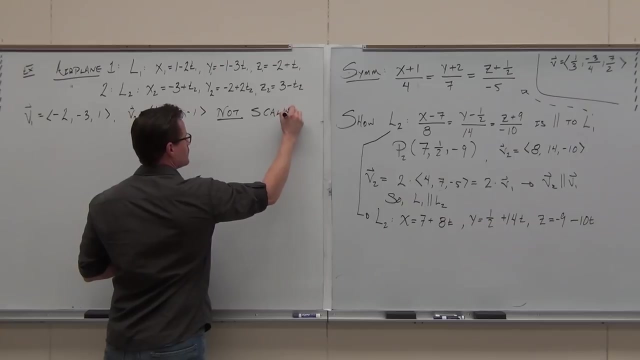 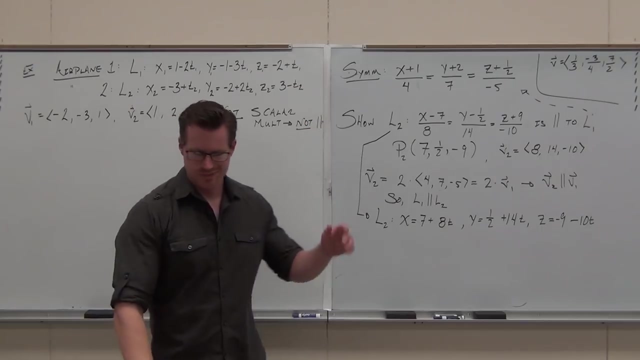 they're parallel or not. are these two things, two vectors, parallel? they're not parallel. why not, since they're not scalar? it's pretty easy to see. you'd have to multiply it by one half. now, not scalar, multiples, not parallel. we talked about it, though does that? 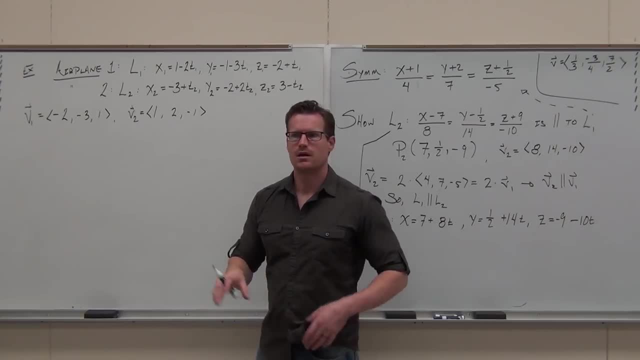 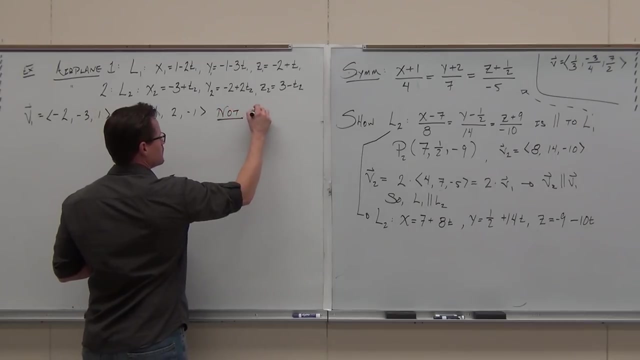 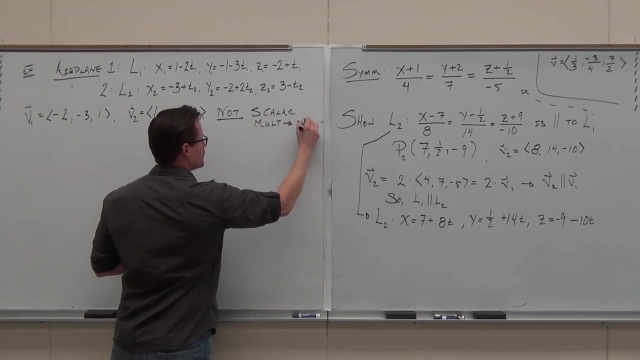 No, They're not parallel. Why not They don't, Since they're not scalar, and it's pretty easy to see, you'd have to multiply it by 1 half. No, No, Not scalar. multiples, not parallel. We talked about it, though. 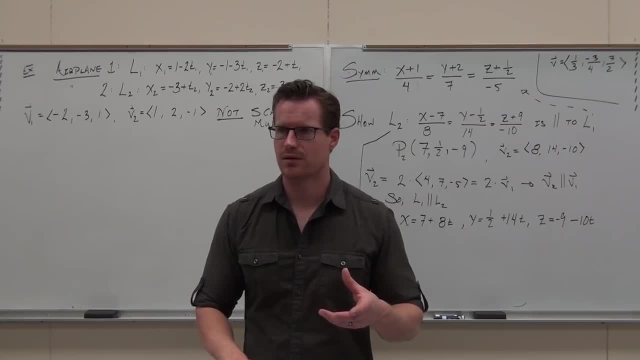 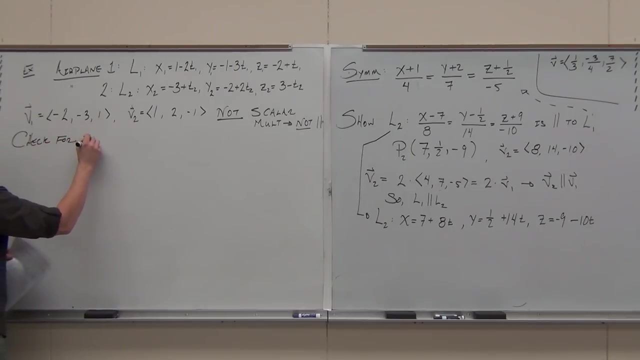 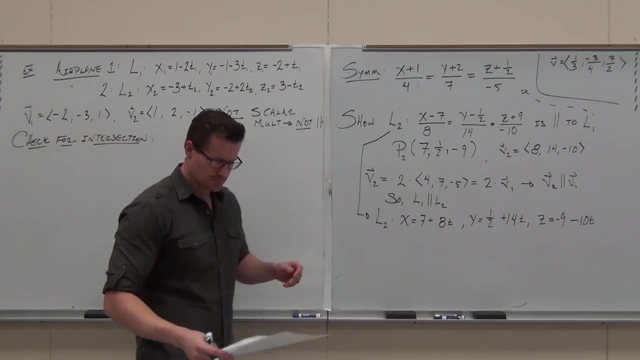 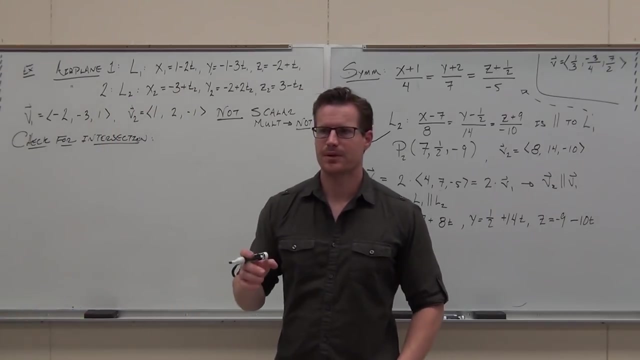 Does that necessarily mean that these planes are crashing Same point, same time? Here's how you check that. Here's how you check. If we want to check for an intersection, What has to happen? what has to happen is this: Our x1 coordinate. look at the board here. 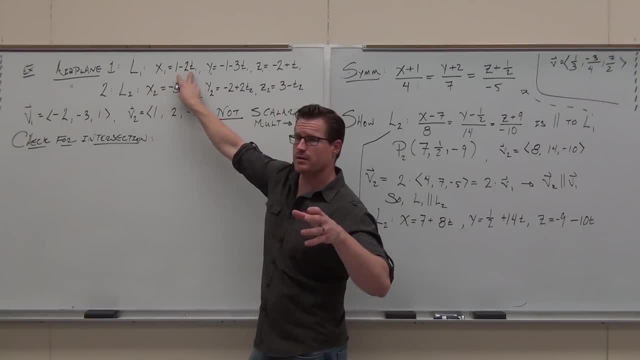 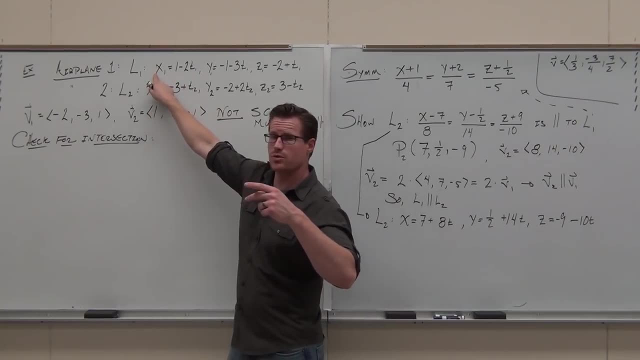 Look, stop whatever you're doing with the board. This is our x coordinate. It's given by when I plug in a time for us and I get out an x value. I plug in a time, I get an x value. In order for this to work, this has to equal this. 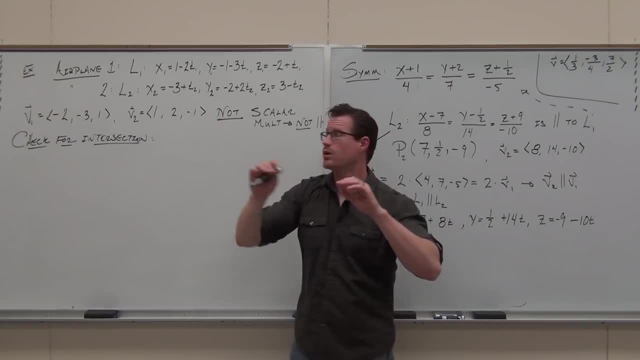 This is: This has to equal this. Our x coordinates have to equal, Our y coordinates have to equal, Our z coordinates have to equal, and they have to all equal at the same exact time. Does that make sense to you? So we set them equal. 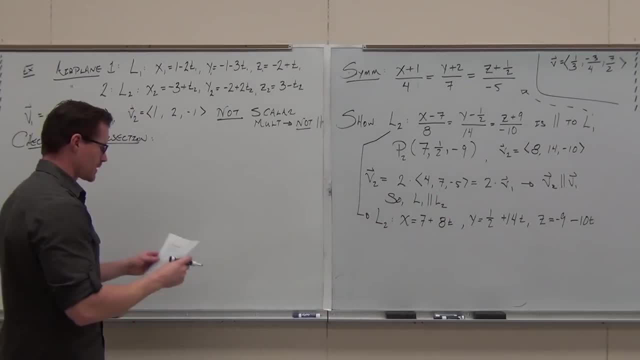 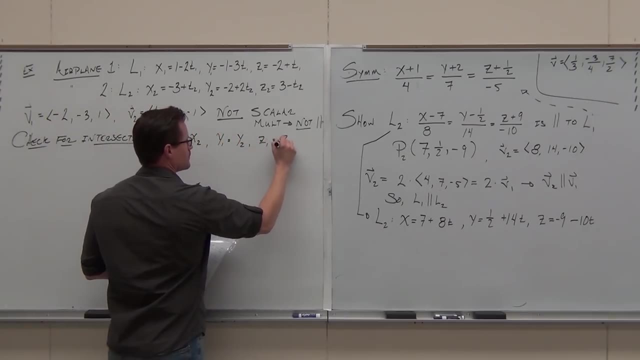 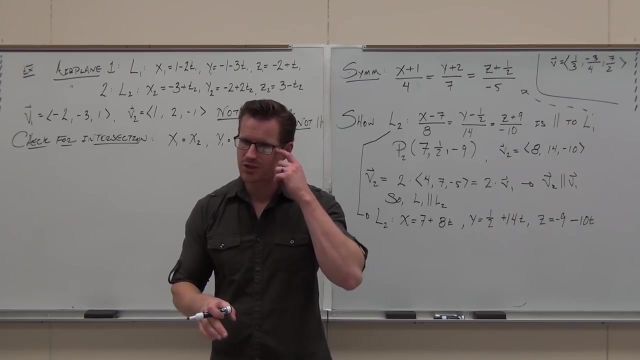 Okay, well, let's let that happen. I want you to set those equal. Do it. Do it now. Don't just wait for me to write on the board. I want you to try it. I'm trying to get you to kind of internalize this. 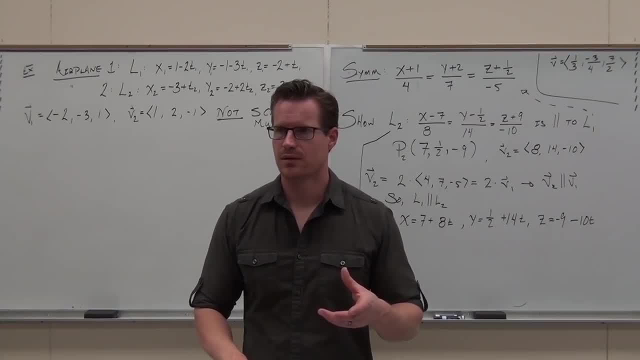 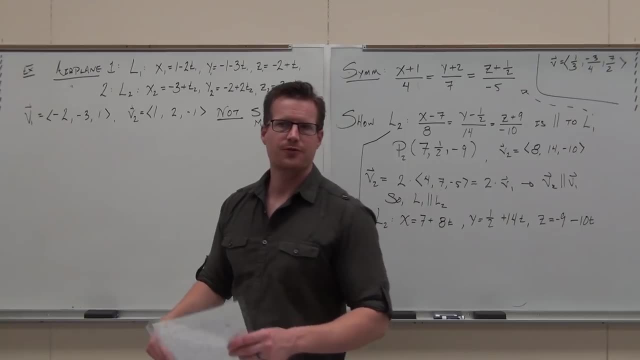 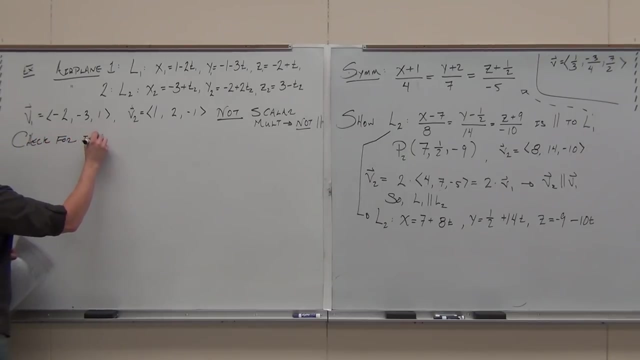 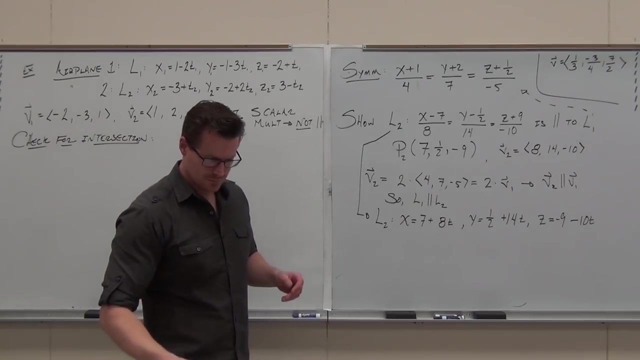 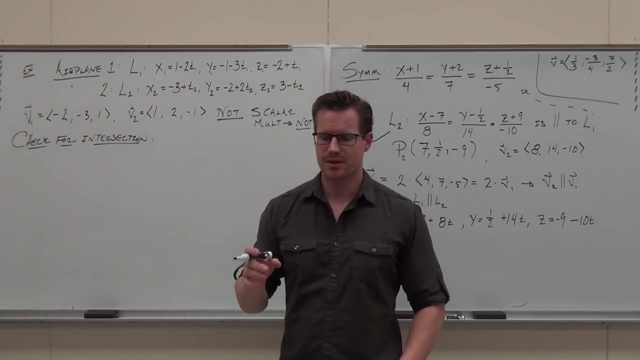 necessarily mean that these planes are crashing. same point, same time. here's how you check that. here's how you check. if we want to check for an intersection, here's how you check for the intersection. what has to happen? what has to happen is that's our X 1 coordinate. look at the look at the board here a little. look WOW. 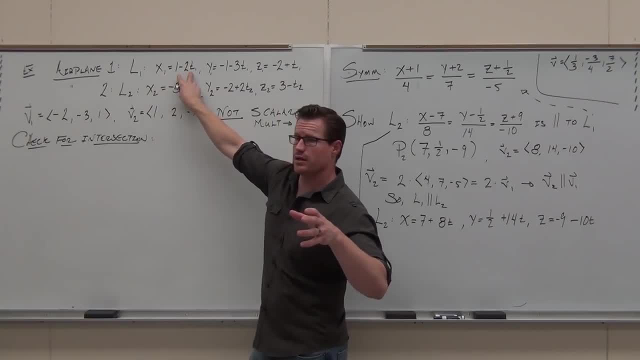 stop whatever you're doing. this is our X coordinate. I can just use this to do just for straight. you have to keep it straight until I get to the one point of thexyanknown It's given by when I plug in a time for us and I get out an x value. 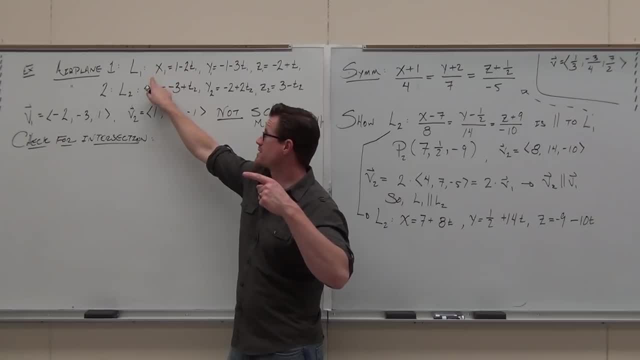 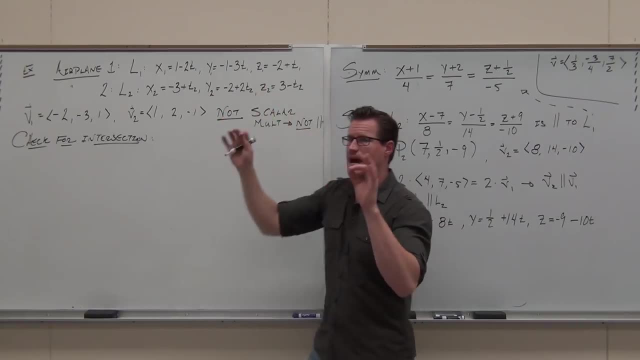 Plug in a time I get an x value. In order for this to work, this has to equal this, This has to equal this. Our x coordinates have to equal, Our y coordinates have to equal, Our z coordinates have to equal and they have to all equal at the same exact time. 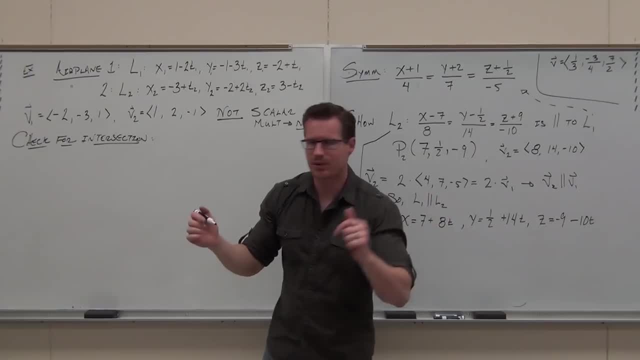 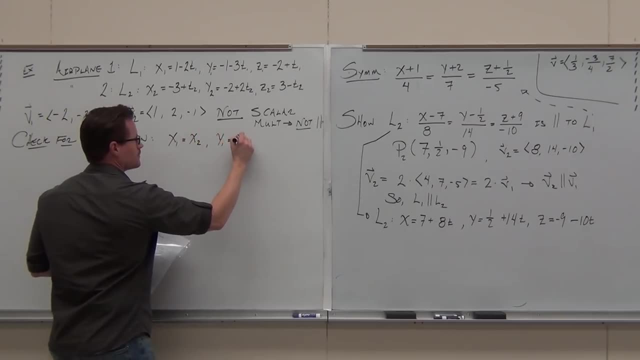 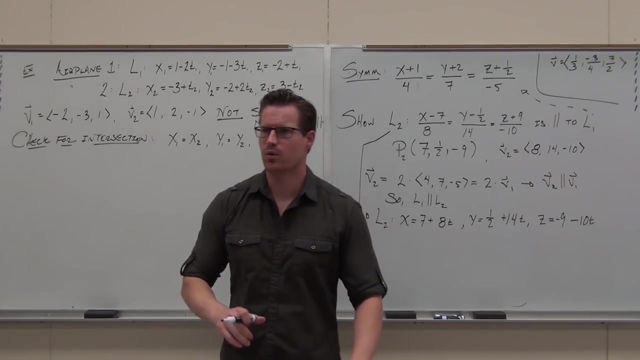 Does that make sense to you? So we set them equal? Okay, well, let's let that happen. I want you to set those equal. Do it now, Don't just wait for me to write on the board. I want you to try it. 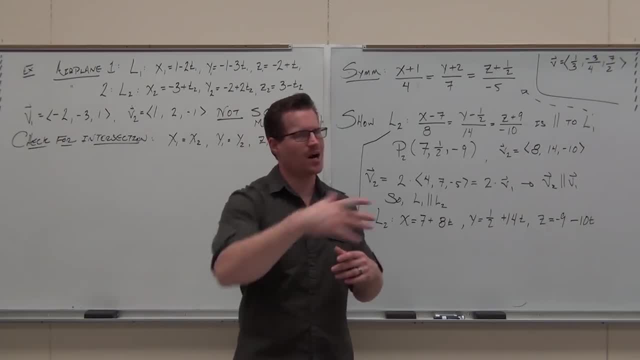 I'm trying to get you to kind of internalize this. When you start just copying stuff down, yeah, that's great, but I know what I'm doing, so you're always going to get it right. I want you to actually do it on your own and go: oh, I did get it right. 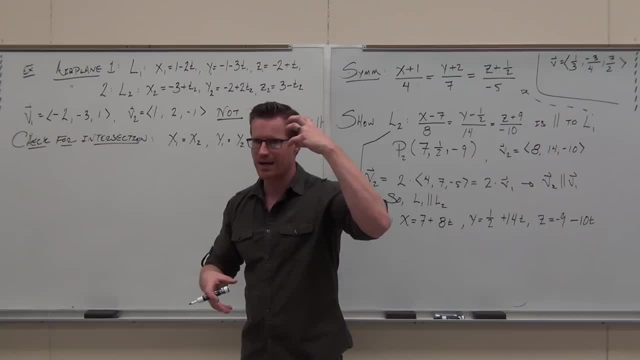 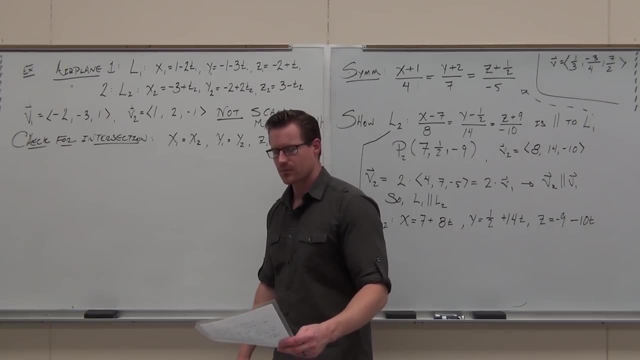 or I really don't get this. yet That's part of trying to grasp the concept: moving beyond just absorbing to participating. I want you to be doing that in this class. What is our F X, sub 1.. What are you writing down right now? 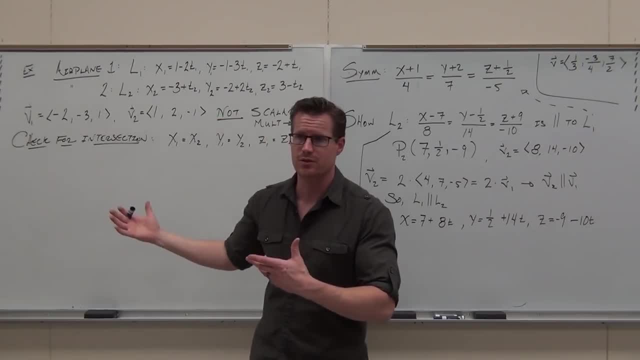 When you start just kind of I'm just copying stuff down, Yeah, that's great, but I know what I'm doing, so you're always going to get it right. I want you to actually do it on your own and go: oh, I did get it right. 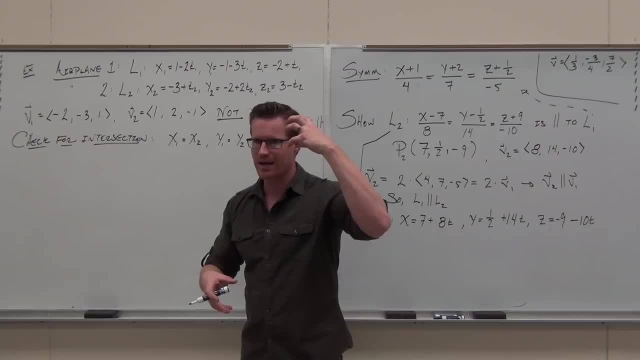 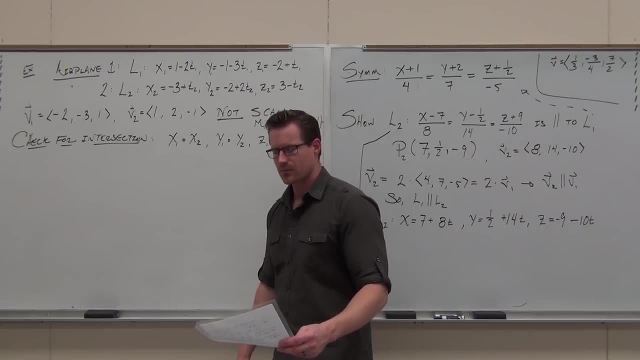 or I really don't get this. yet That's part of trying to grasp the concept, moving beyond just absorbing to participating, and I want you to be doing that in this class. What is our x sub 1?? What are you writing down right now? 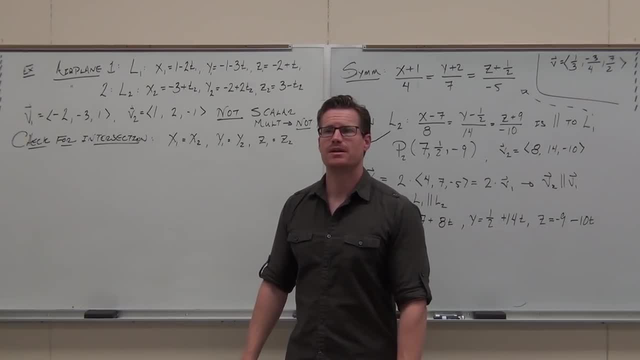 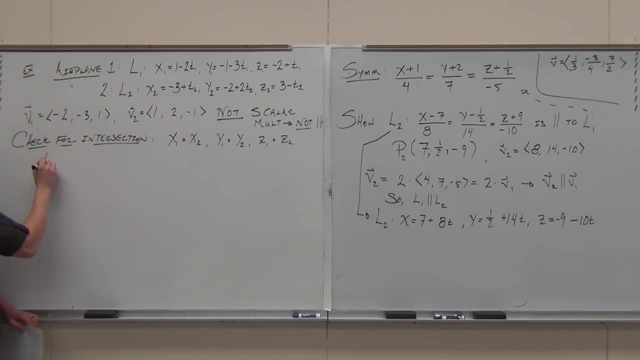 What would you write down? See it in the back ladder. That's where it's from. yeah, X sub 1 is 1.. X sub 1 is 1 minus 2t, but it's 2t sub 1.. 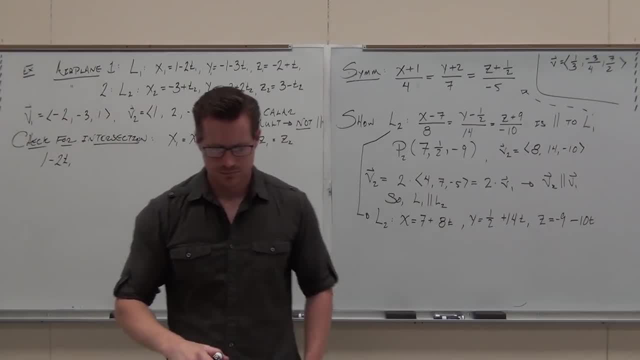 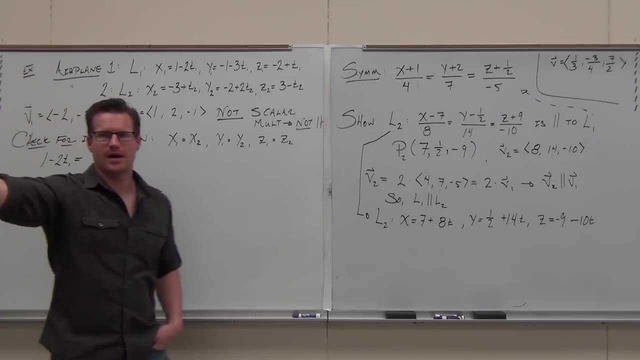 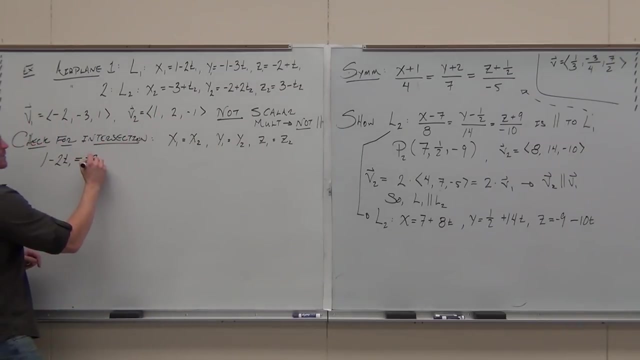 Make sure you have that little 1.. Okay, back people got that one. Front guys. what's that supposed to equal? Come on, Come on quickly. 3 plus t sub 1. Perfect, What else has to happen? 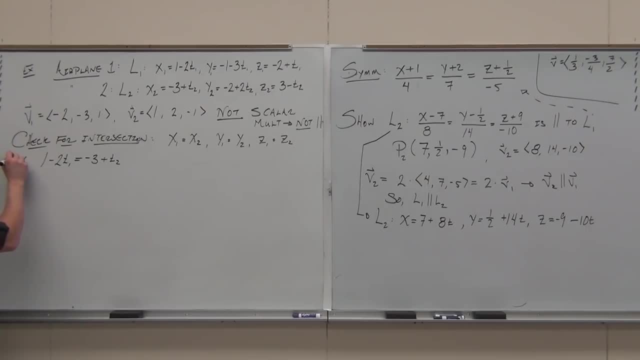 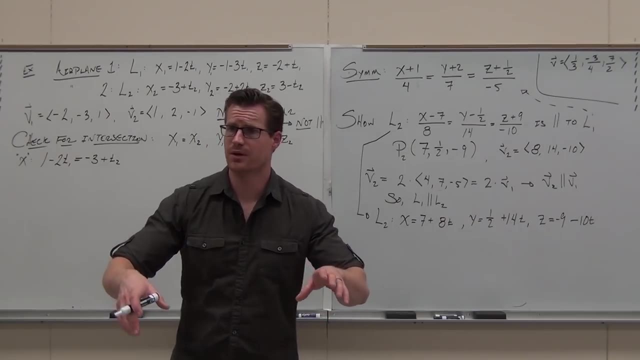 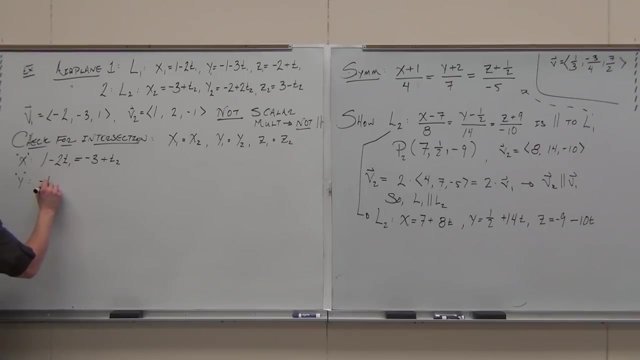 Well, this would be our. That would be our x. That's from our x. Let's write the other ones. Write them down on your own, as I'm writing them down up here. I also need the y's and the z's. 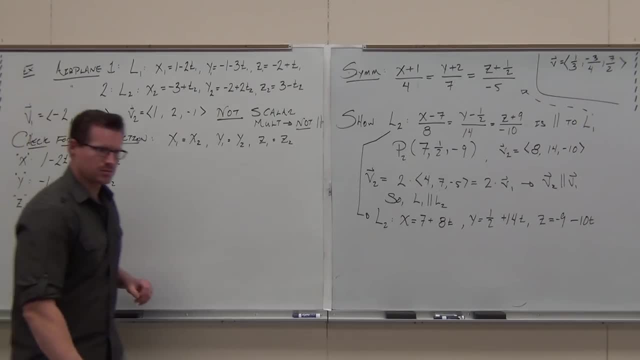 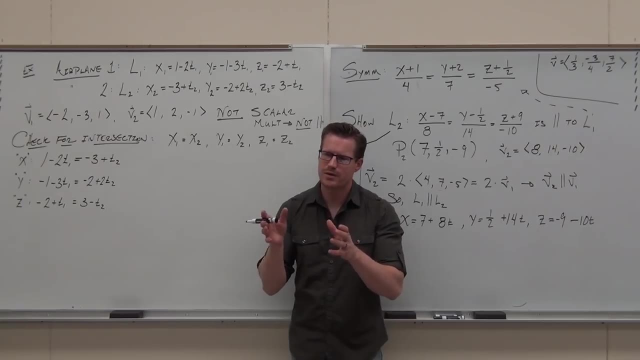 I want to ask you if you guys understand where all this stuff is coming from. Right now, what we're doing is we're we know that they're not parallel, so they might intersect, they might not, I don't know. This is how you check. 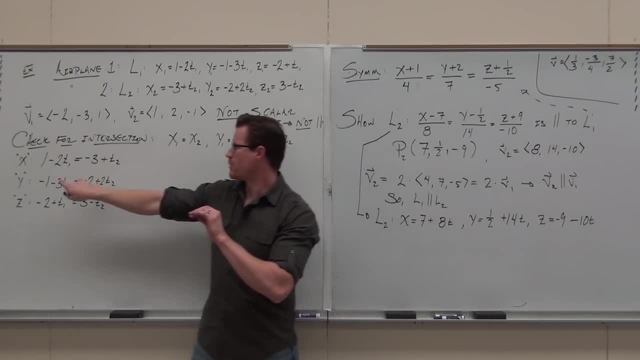 You check whether the x coordinates are going to be equal, Whether the y coordinates are going to be equal and the z coordinates are going to be equal, and they all better be exactly equal on from both equations that we have in order for them to intersect. 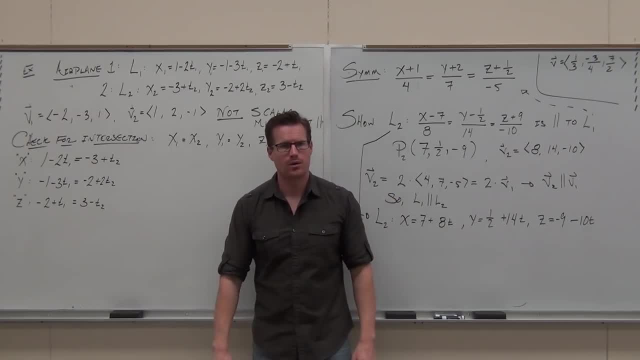 So Okay, What in the world are we going to do now? Solve How Systems, Systems. How many equations do we have? Three, How many variables do we got? Three, Two, T1, T2.. Parameters have the t's as the variables. 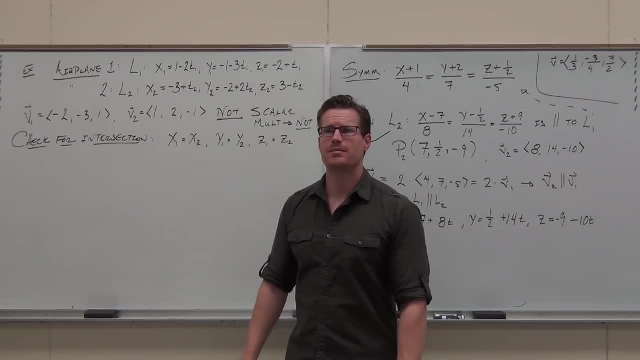 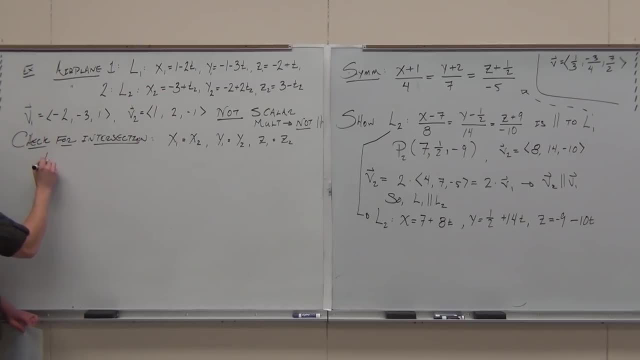 What would you write down? See it in the back letter. That's where it's from. yeah, X sub 1 is 1 minus 2T, but it's 2T sub 1.. Make sure you have that little 1.. 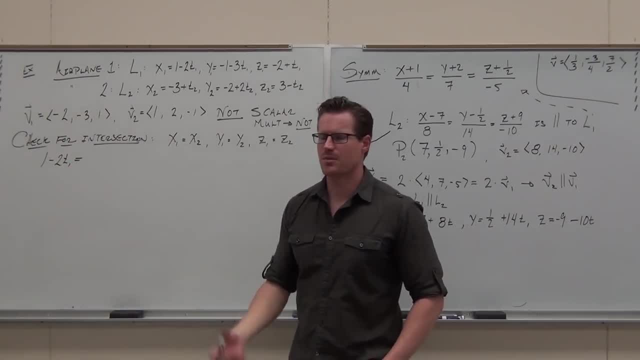 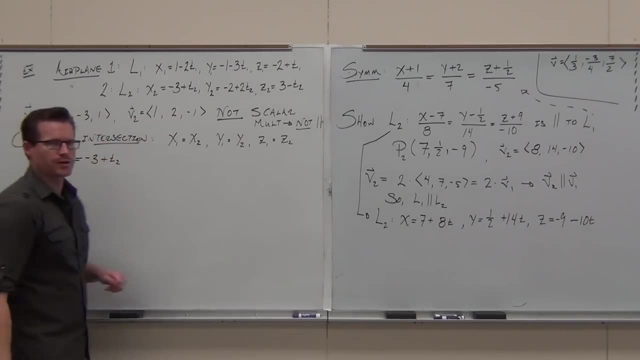 Okay, back, people got that one Front guys. what's that supposed to equal? Come on, Come on quickly. We're good: 3 plus 2T sub 1. Perfect. What else has to happen? Well, this would be our. that would be our X. 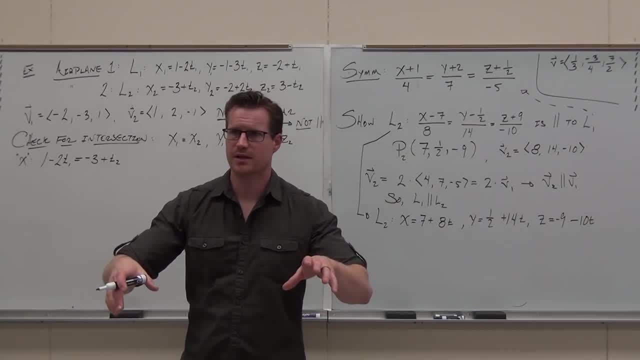 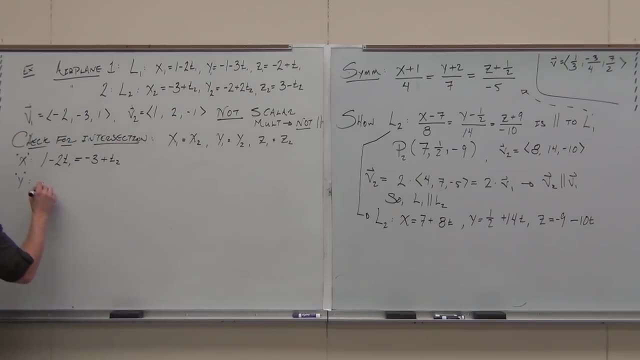 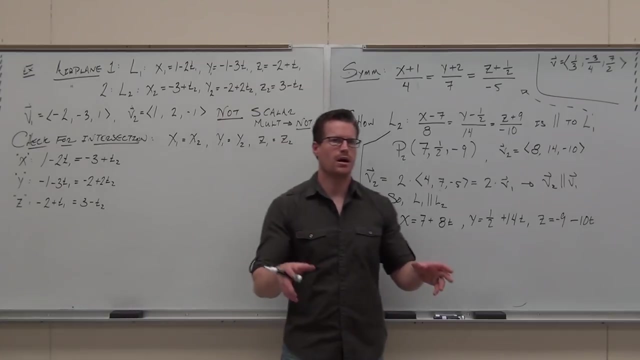 That's from our X. Let's write the other ones. Write them down on your own, as I'm writing them down up here. I also need the Y's And the Z's. I want to ask you if you guys understand where a lot of this stuff is coming from. 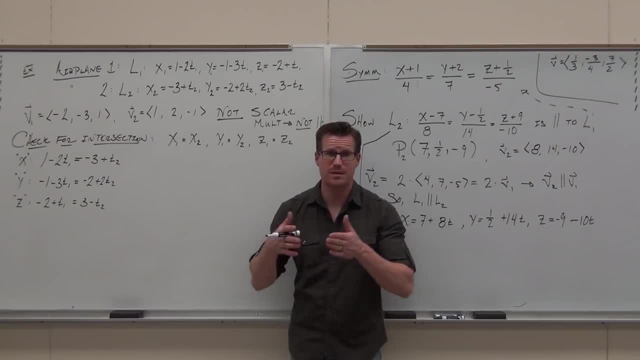 Right now what we're doing is we're check. we know that they're not parallel, so they might intersect, They might not, I don't know. This is how you check. You check whether the X coordinates are going to be equal. 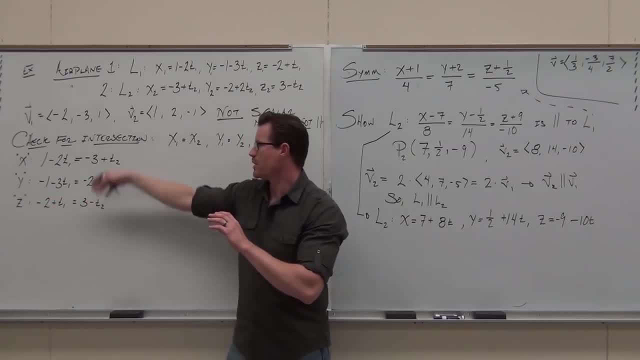 Whether the Y coordinates are going to be equal, are going to be equal and the Z components are going to be equal, and they all better be exactly equal from both equations that we have in order for them to intersect. So what in the world are we going to do now? 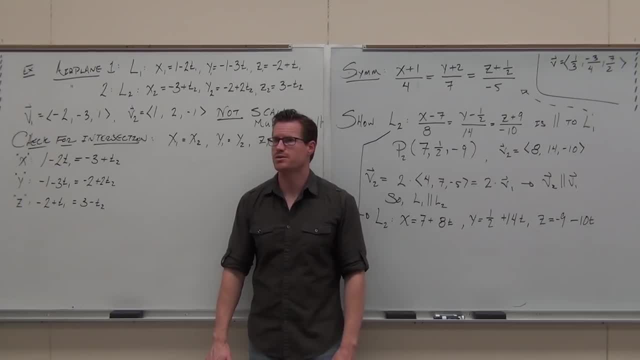 Solve How? Systems, Systems. How many equations do we have Three? How many variables do we have Three? Two, T1, T2.. Parameters have the T's as the variables. There's only two variables With three equations. that means we have one too many. 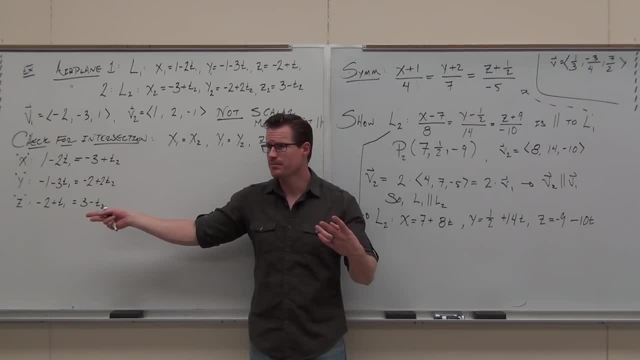 There's only two variables With three equations, that means we have one too many. That's the one you test. Listen carefully, Pick any two that you want. I pick the easiest ones to make a nice system of. I will make you a promise if you do it right. 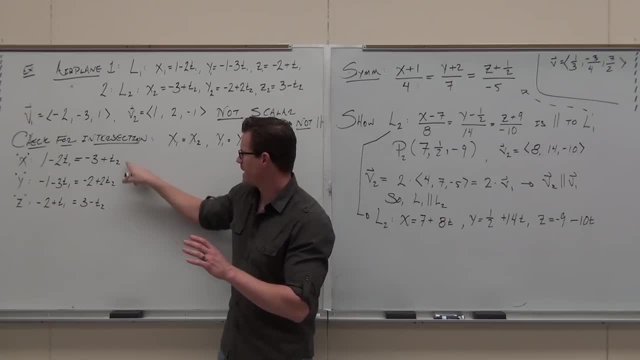 Pick any two. I'm going to pick these two because I like the fact that I can just add them together and get rid of T2.. Do you see what I'm talking about? That's really easy. So I'm going to pick these two. 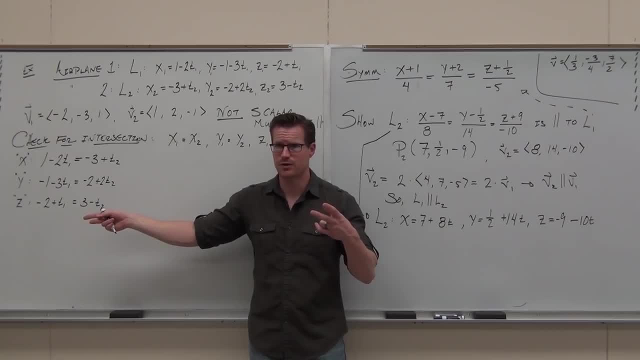 That's the one you test. Listen carefully, Pick any two that you want. I pick the easiest ones to make a nice system of. I will make you a promise if you do it right, Pick any two. I'm going to pick these two because I like the fact. 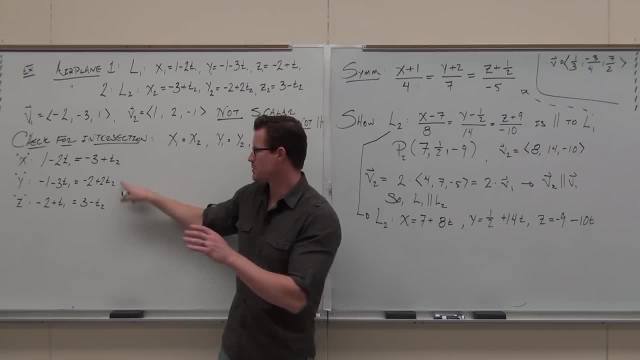 that I can just add them together and get rid of T2.. Do you see what I'm talking about? That's really easy. So I'm going to pick these two. The two that you pick are always going to work. It has to. 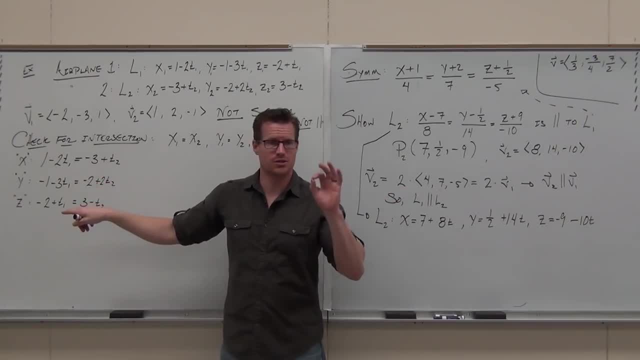 It's a system. It's the one that you don't pick. that determines the system. It determines whether you actually intersect or whether you do not. Did you catch that? That's what's going to happen. So these two, they're going to be the same. 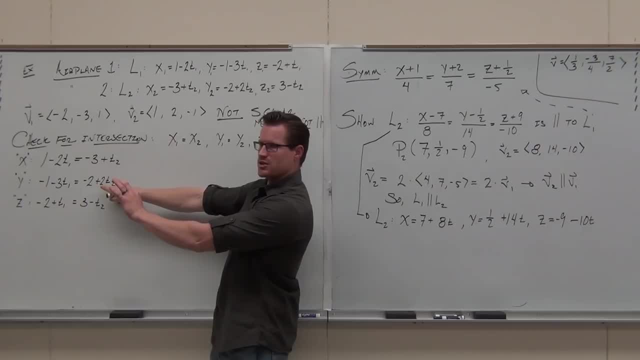 I know what it's going to be. It's going to be the same, But the one I don't pick, this one, This is the one that's going to get you approved to you. I just want you to see that I'm going to talk ahead of it. 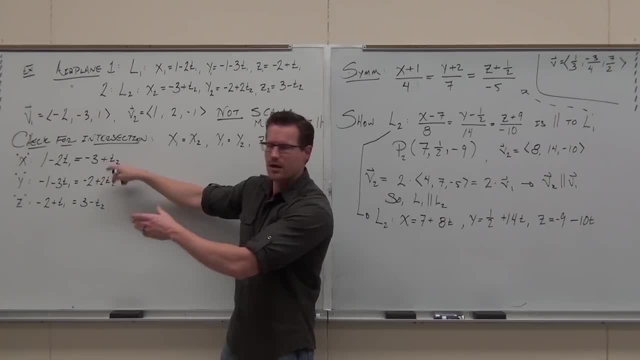 That way you're like: oh, that's what's happening here, Why You pick the equations in the system They will be equal. You're solving for the place where those are equal. The one you don't pick is the one that determines whether you 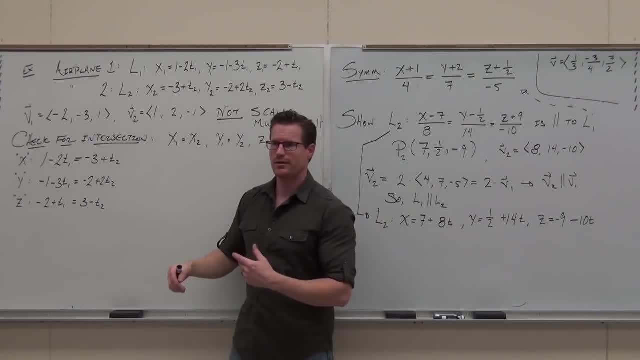 The two that you pick are always going to work. It has to. It's a system. It's the one that you don't pick that determines whether you actually intersect or whether you do not. Did you catch that? That's what's going to happen. 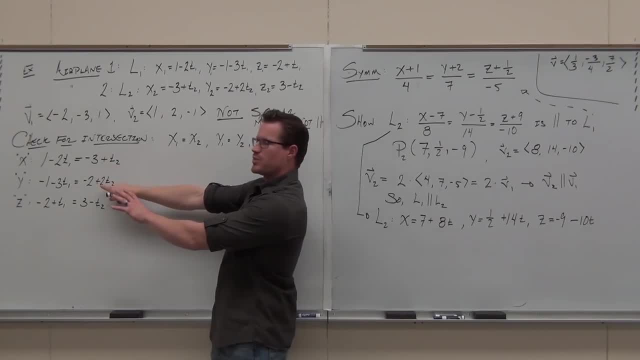 So these two, they're going to be the same. I know what it's going to be. It's going to be the same. But the one I don't pick, this one, this is the one that's going to get you all pruned to you. 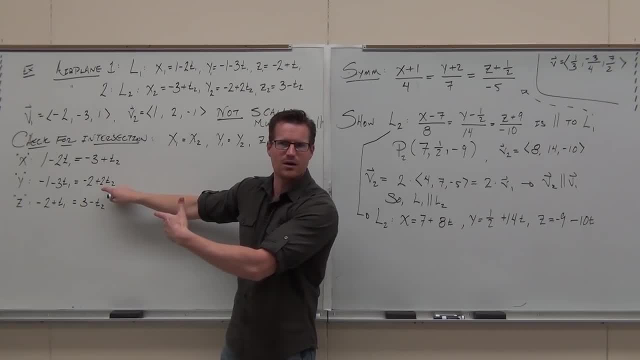 I just want you to see that I'm going to talk ahead of it. That way you're like: oh, that's what's happening here, Why You pick the equations in the system They will be equal. You're solving for the place where those are equal. 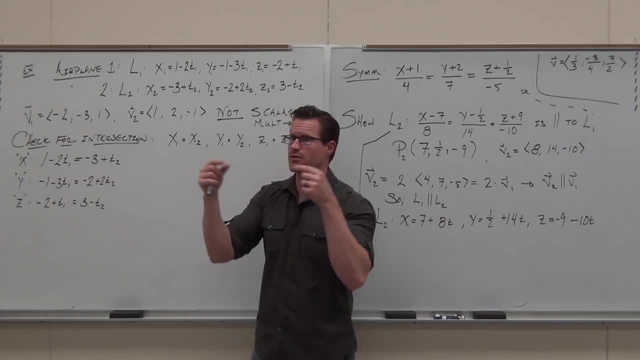 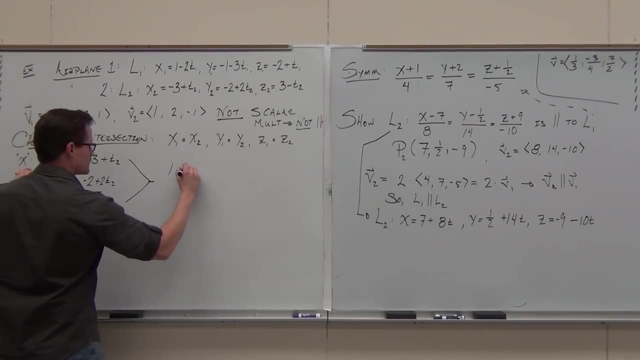 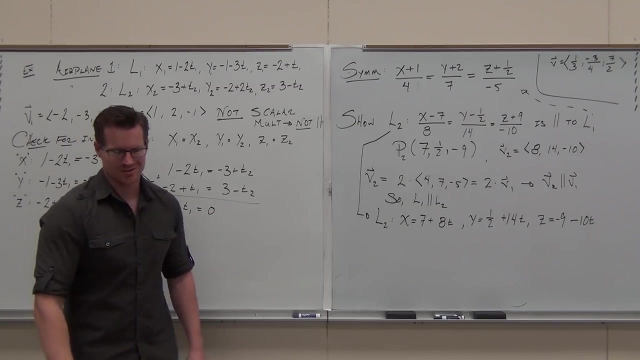 The one you don't pick is the one that determines whether you actually intersect or if you get different numbers, then you don't. So pick any two. Let's pick these. I like this one. I can just add them Zero, I'll get zero. 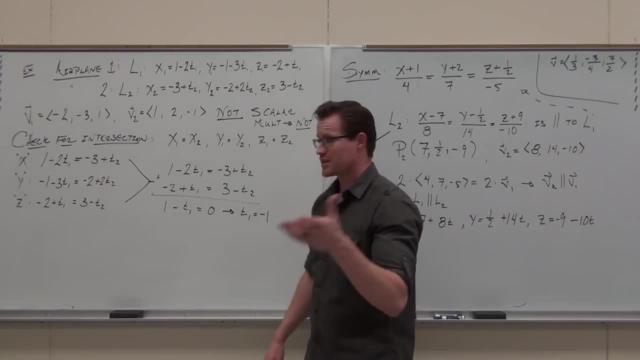 I know right now the t1 is negative 1.. In 3D world we think t is time, but it's really not exactly time. It's negative 1 as well. it doesn't really matter. Negative 1, maybe an hour before 12 o'clock. 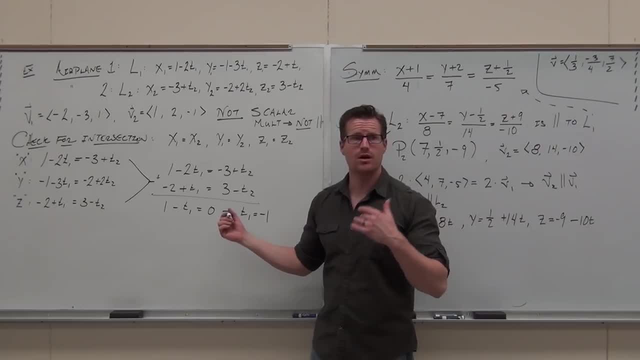 Who cares? But that's what's happening here. This is going to cross into this point at. t equals negative 1 for airplane number 1.. Now can you find t sub 2? Shouldn't that be a negative 1 at the beginning there? 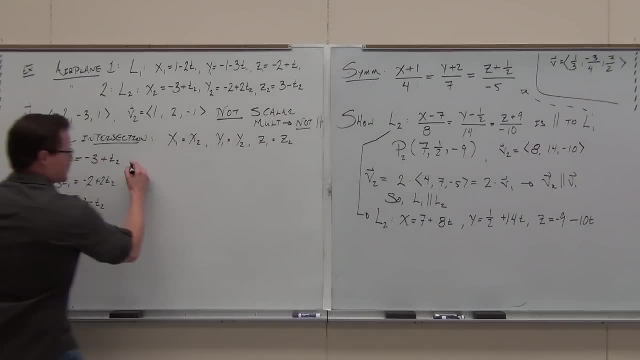 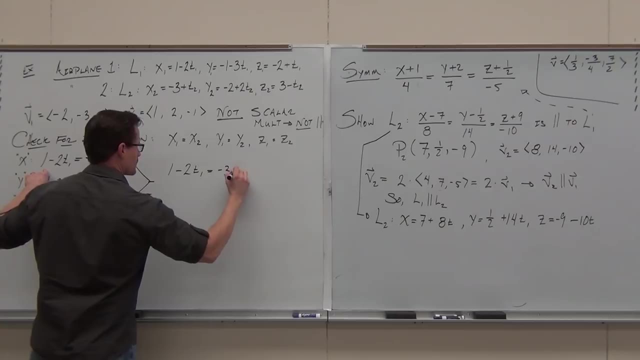 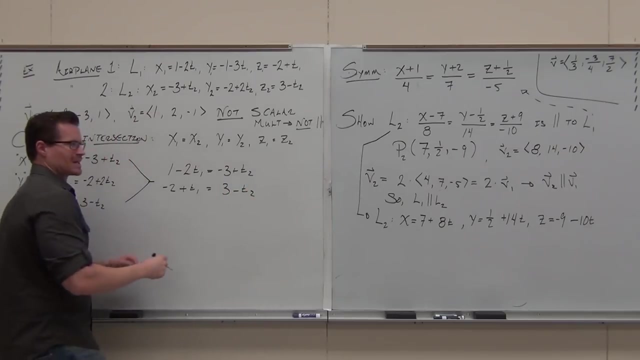 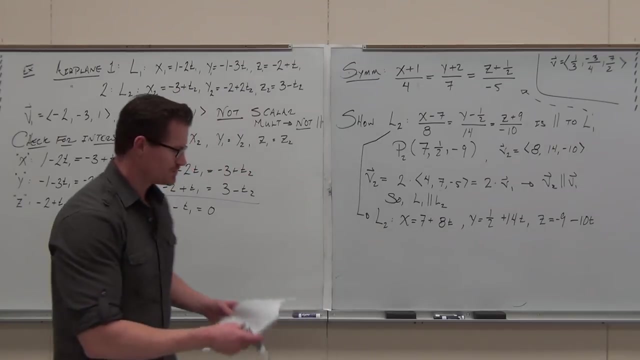 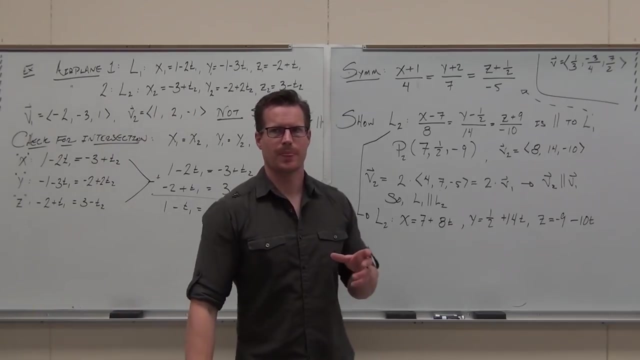 actually intersect, or if you get different numbers, then you don't. So pick one, Pick any two. Let's pick these. I like this one. I can just add them Zero. I'm not getting zero. I know right now the T1 is negative 1.. 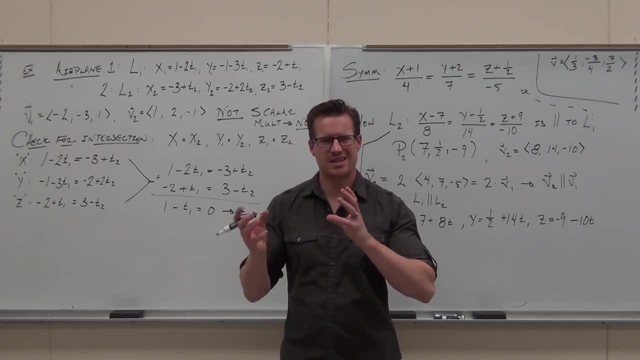 In 3D world. we think T is time, but it's really not exactly time. It's negative 1 as well. it doesn't really matter. Negative 1, maybe an hour before 12 o'clock- Who cares? 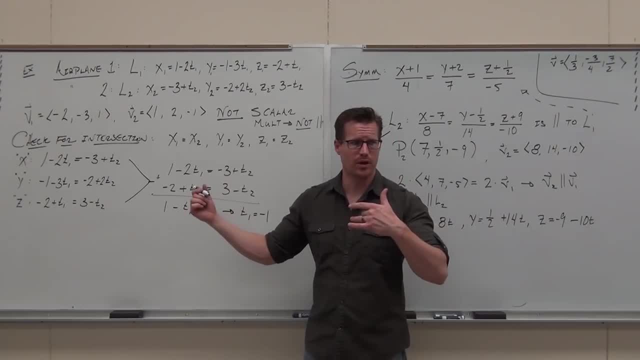 But that's what's happening here. This is going to cross into this point at. T equals negative 1 for airplane number 1.. Now Can you find T sub 2? Shouldn't that be a negative 1 in the beginning there? 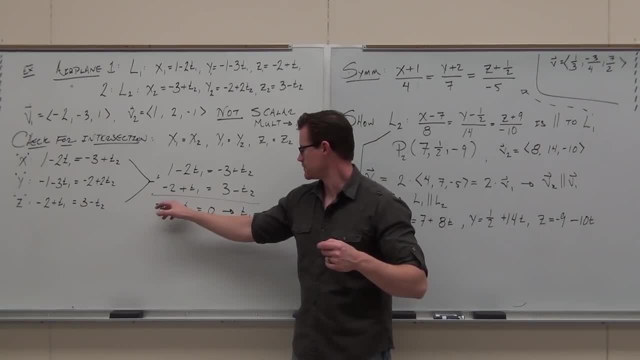 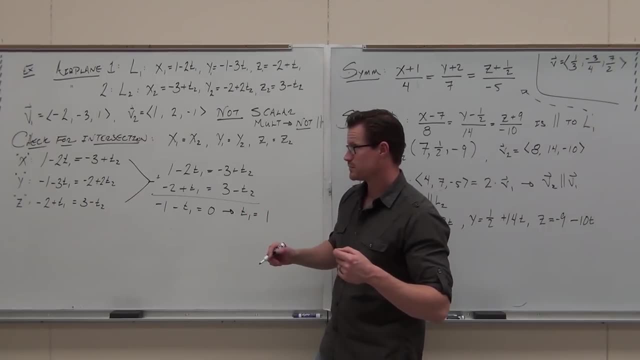 Negative: 1 minus 2.. Oh yeah, Okay Sorry, It is negative 1.. I like this better. This is why I have you guys here. Catch my errors. I told you, it's the little things that get you. 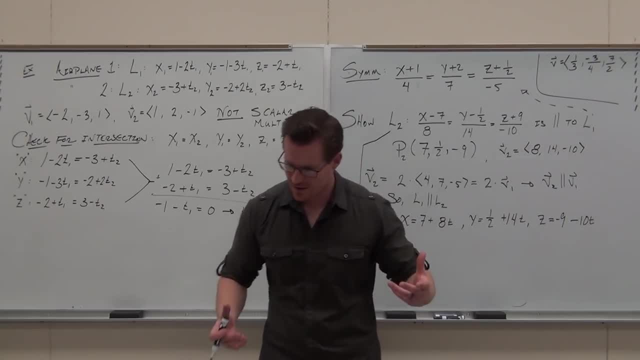 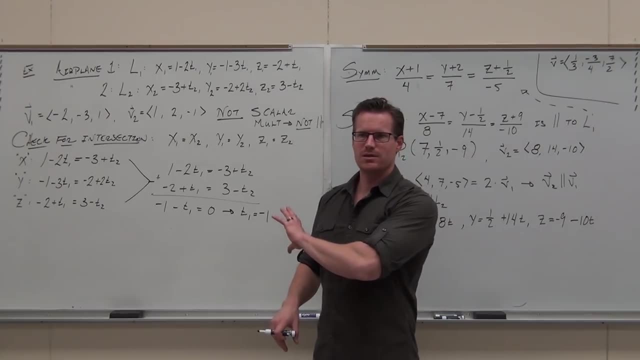 For me it is. at least It's those. I even have an answer right here. I guess I could just look at it right and negative 1.. Hey, there you go. Hmm, From that can you find T2?. 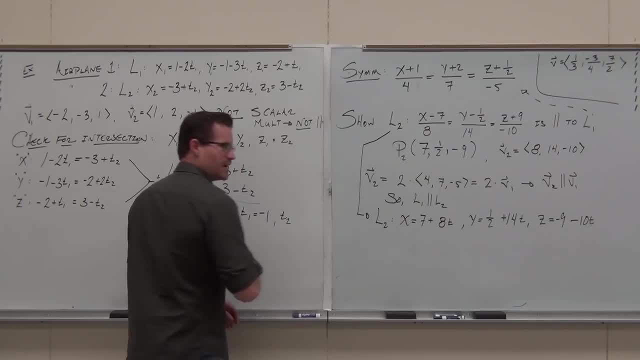 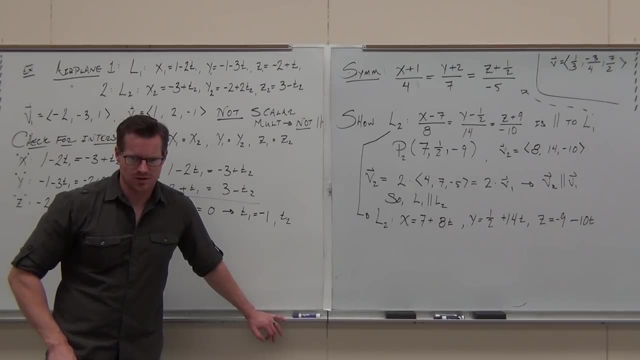 Yes, Yes, Have you all done it, Since I obviously can't do any math today, Have you found it? Yeah, What is it? 2. Really, Six, Six? I don't think it's 2. No, 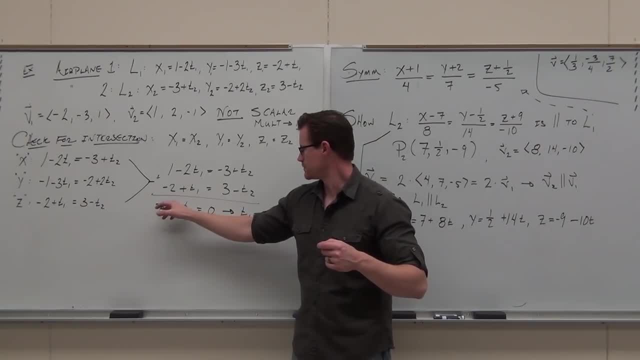 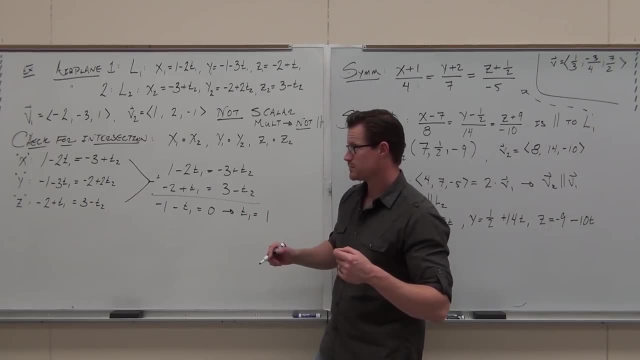 Negative 1 minus 2.. Oh yeah, Sorry, I like this better. This is why I have you guys here. Catch my errors. I told you it's the little things that get you. For me it is at least. 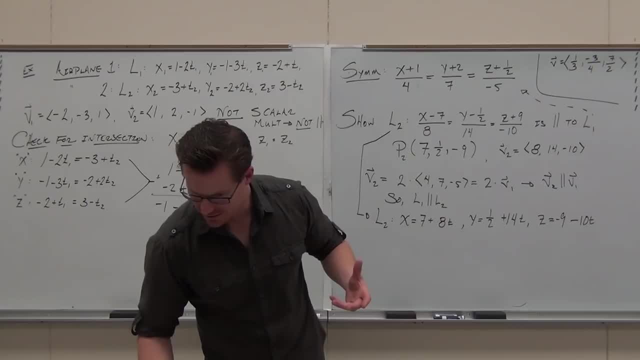 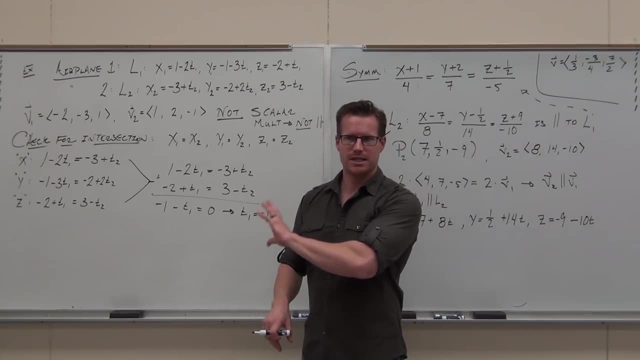 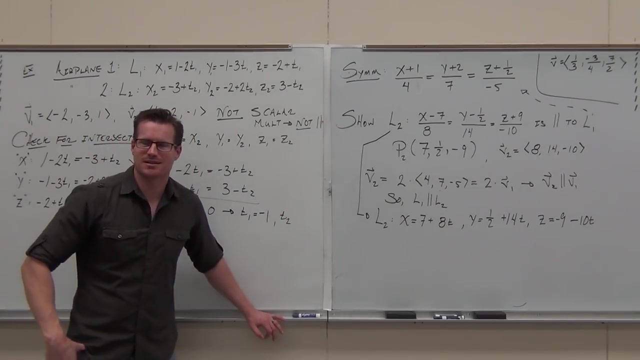 It's those. I even have an answer right here. I guess I could just look at it right. Negative 1. Negative 1. From that can you find t2?? Yes, Have you all done it, Since I obviously can't do any math today? have you found it? 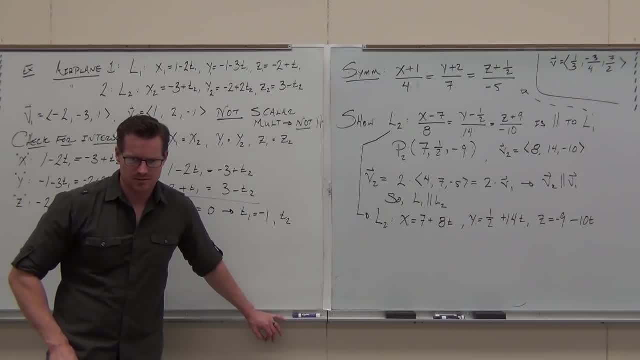 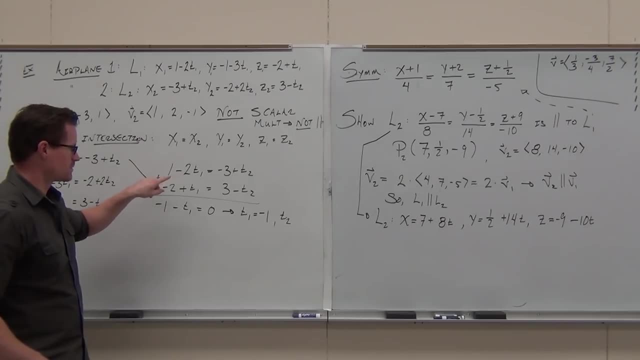 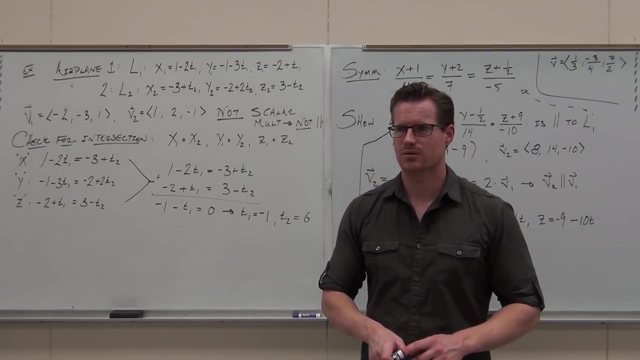 What is it? 2. Really 6. I don't think it's 2. 6. I think it's 6. I'm pretty sure Did you get 6?. Triple check. Quadruple check. Quintuple check. 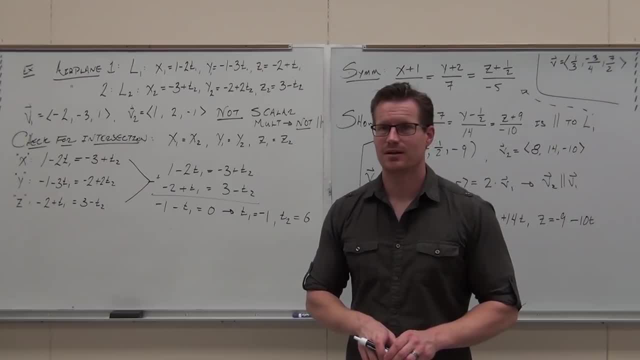 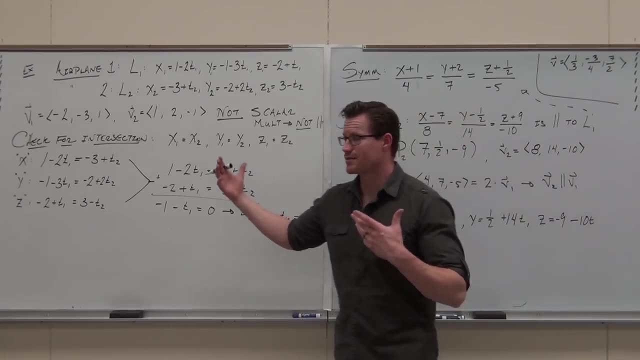 I don't know any higher than that, so hopefully that's enough. Listen carefully, I don't want to lose you. Honestly, we've done zero calculus in this class so far. None, None. We're just working with 3D stuff. 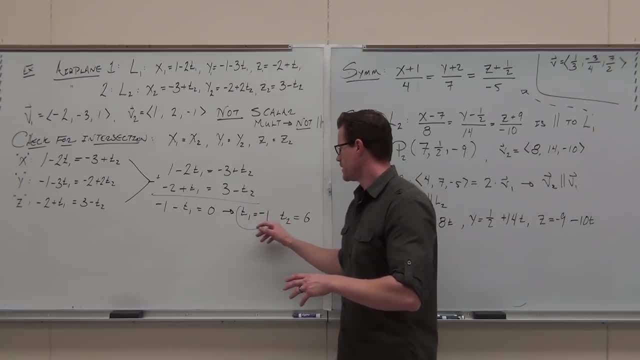 Here's what's happening. We solve the system. Airplane 1 is going to cross this point. at t equals negative 1.. Airplane 2: at t equals t2 equals positive 6. That doesn't tell you anything right now. 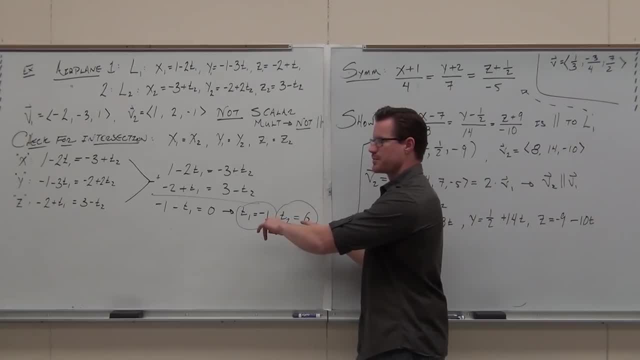 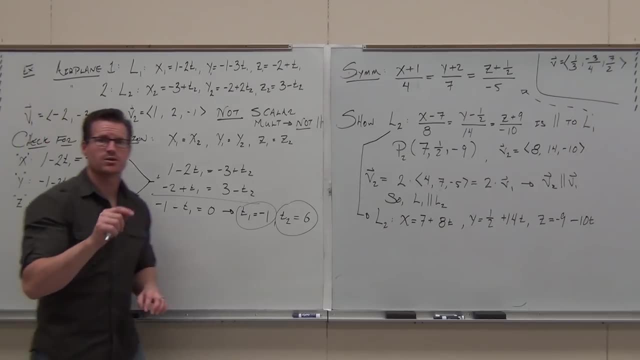 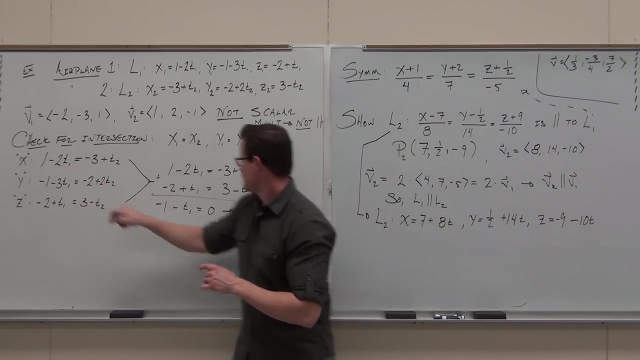 That doesn't tell you. Here's how you tell. Take these numbers, Plug them in respectively for each of these three. Now here's where the promise comes in. I guarantee you that when you plug in negative 1 here and positive 6 here, 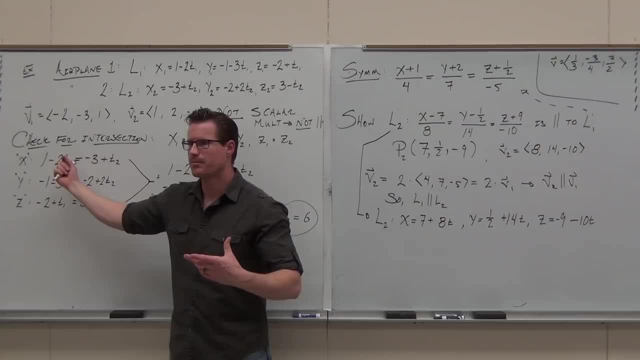 which you should. that's what those numbers mean. it's going to equal the same number. I guarantee you that when you plug in negative 1 here and you plug in positive 6 here, it's going to equal the same number. Why? 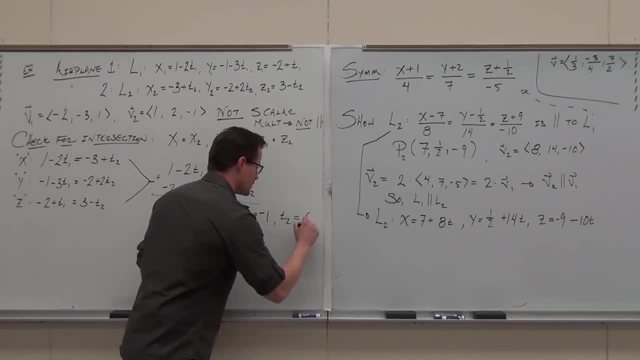 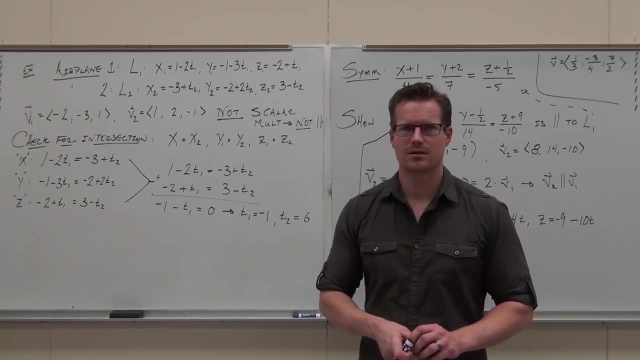 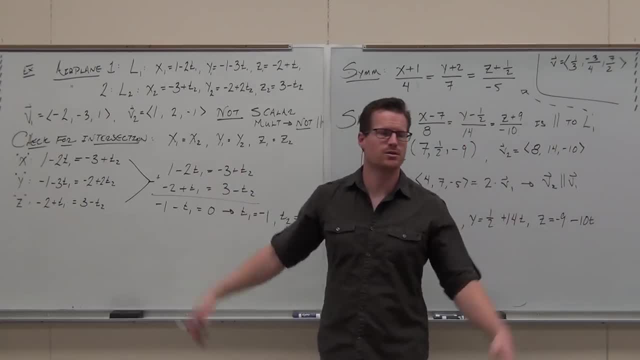 Listen carefully. I don't want to lose you It honestly. this is: we've done zero calculus in this class so far. none, none. We're just working with 3D stuff. Here's what's happening. We solve the system. 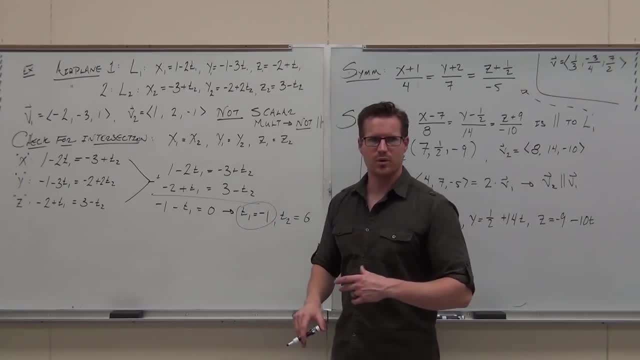 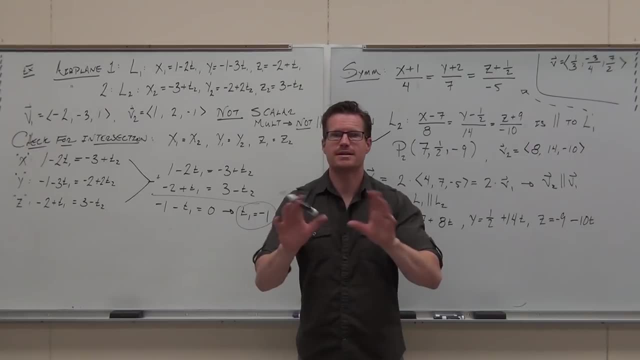 Airplane 1 is going to cross this point: at t equals negative 1. Airplane 2: at t equals t2. equals negative, equals positive 6.. That doesn't tell you anything right now. That doesn't tell you. Here's how you tell. 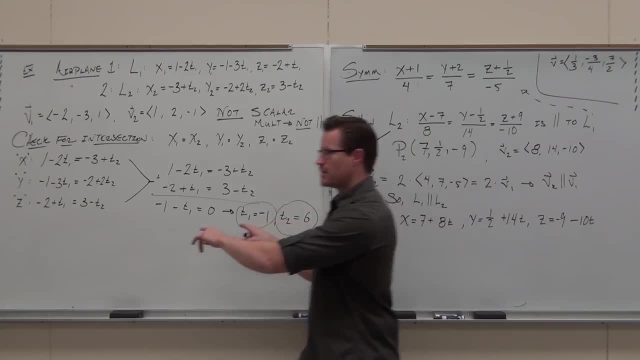 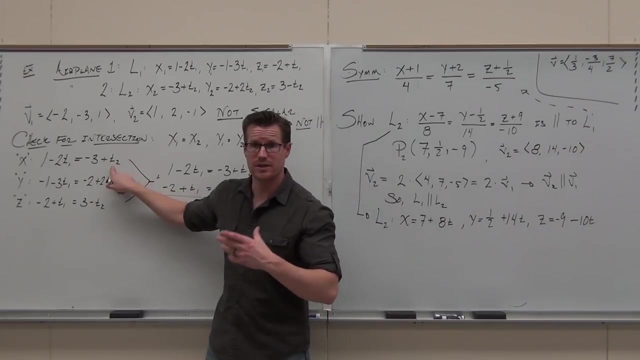 Take these numbers, plug them in respectively for each of these three. Now here's where the promise comes in. I guarantee you that when you plug in negative 1 here and positive 6 here- which you should, that's what those numbers mean- it's going to equal the same number. 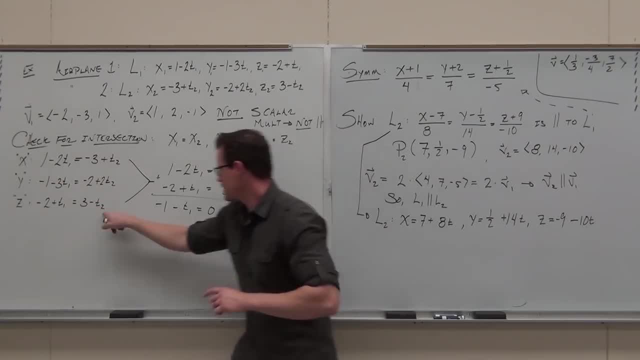 I guarantee you that when you plug in negative 1 here and you plug in positive 6 here, it's going to equal the same number. Why? That's where I got this system from. It has to. This is the only one that can, so if you're on time on a test. 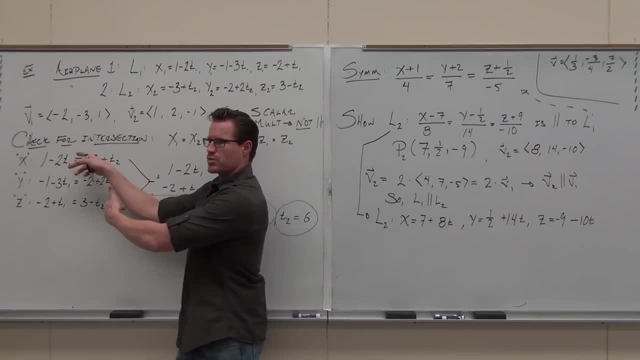 and you're like, oh my gosh, I don't know, I don't know, I don't know. don't worry about these two, It's going to work out. What about this one? If these two sides, when you plug in negative 1 and positive 6,? 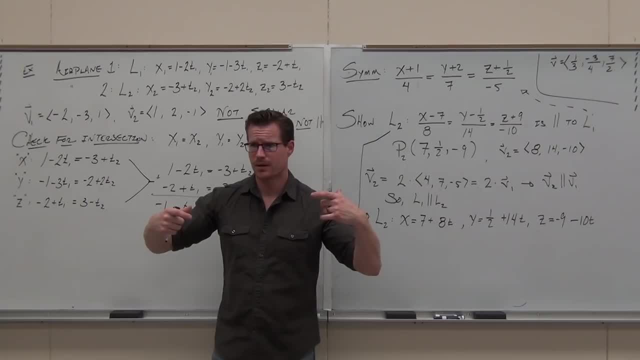 if it works out to the same number, these planes crash. If it works out to different numbers, these planes do not crash. Does that make sense to you? Are you sure I'm getting kind of looks? Yes, Plug it in. 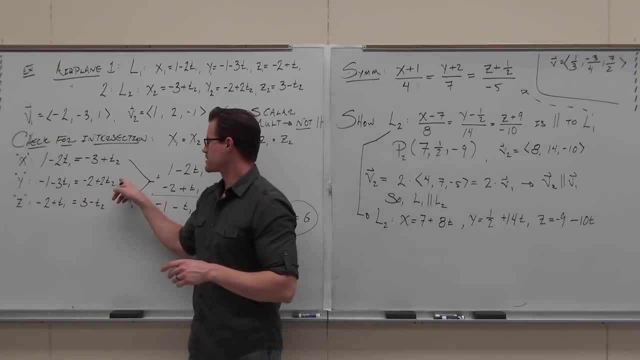 That's where I got this system from. It has to. This is the only one that can. So if you're I don't have time on a test and you're like, oh my gosh, I don't know, I don't know, I don't know, 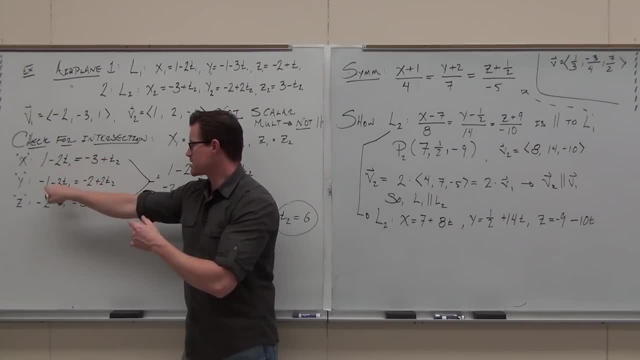 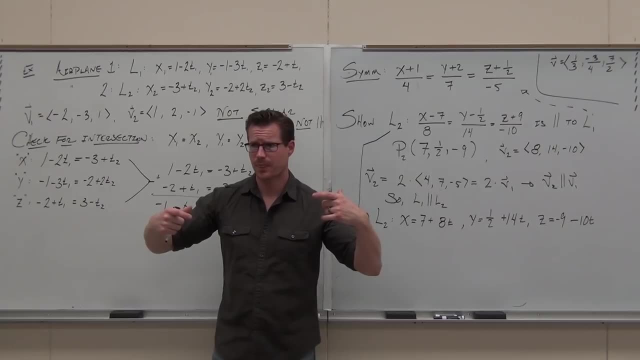 Don't worry about these two, It's going to work out. What about this one? If these two sides? when you plug in negative 1 and positive 6, if it works out to the same number, these planes crash. If it works out to different numbers, these planes do not crash. 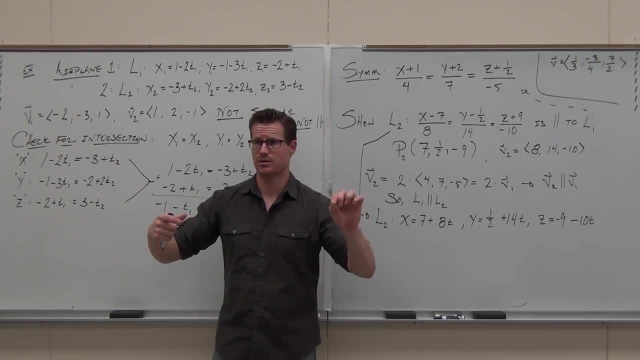 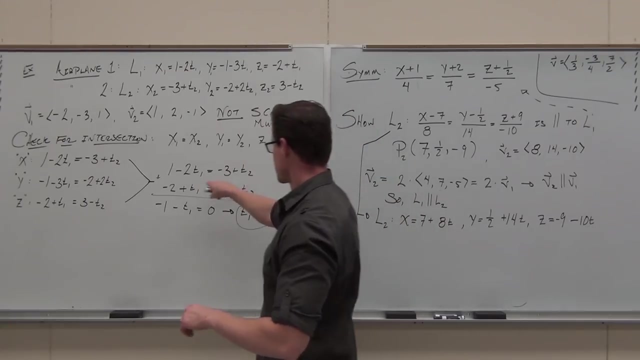 Does that make sense to you? Are you sure I'm getting kind of looks: Yes, Plug it in, Plug this into your system and solve for T2.. Yeah, I did, I used this one, So let's try it. 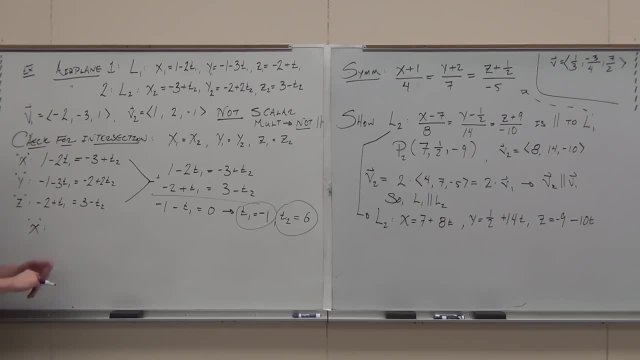 So far X's. If I plug in negative 1 here, come on, stick with me here. If I plug in negative 1 here, how much is this? Oh boy, How much Let's plug in negative 1 here. 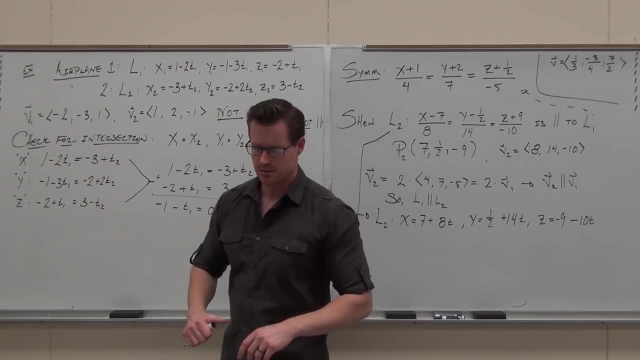 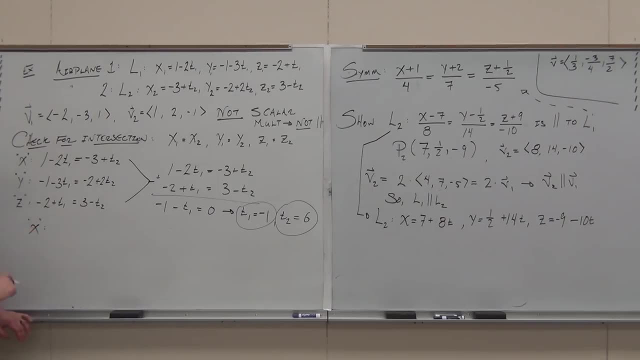 Plug this into your system and solve for T2.. No, I did. I used this one, So let's try it. So far X's If I plug in negative 1 here. come on, stick with me here. 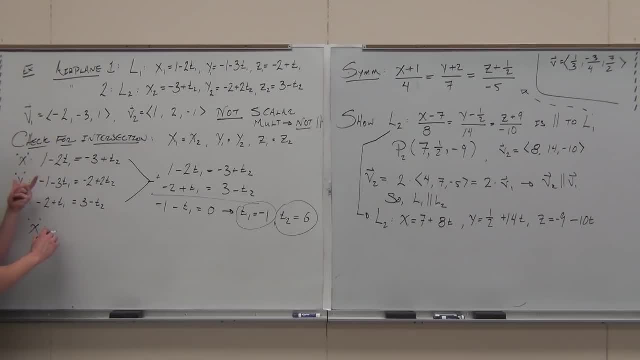 If I plug in negative 1 here, how much is this? Oh boy, How much. Let's plug in negative 1 here. Three, Three. Let's plug in positive 6 here. Is it the same? Yes, Let's plug in negative 1.. 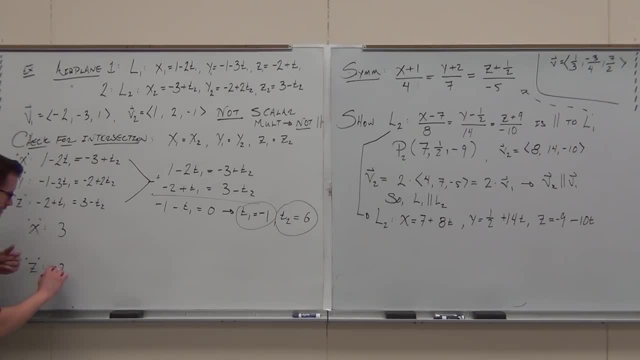 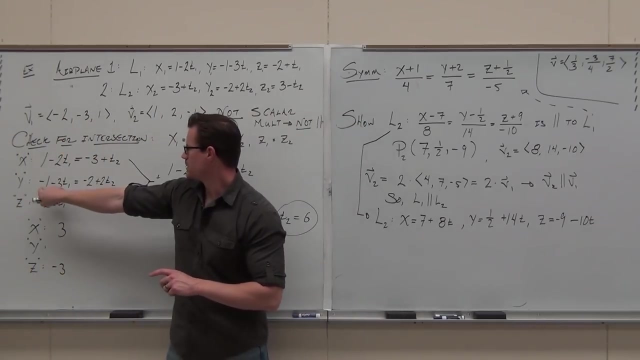 Here. What is it Negative? 3. Let's plug in positive 6 here. What is it Negative? 3. They're the same I promised you. I'm mad at my work. Let's plug in negative 1 here. 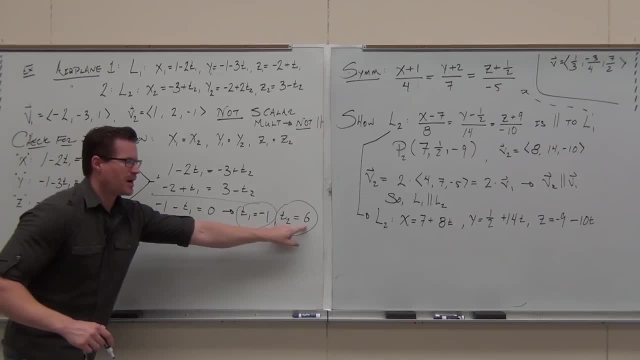 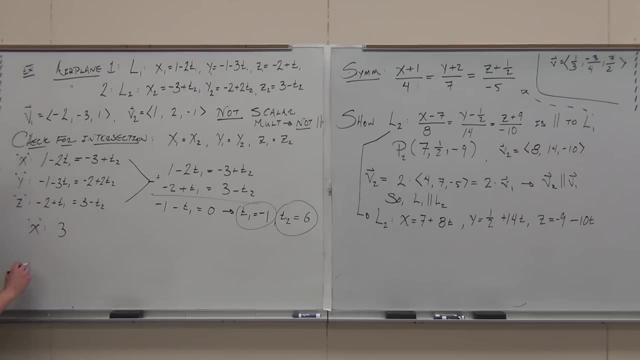 Three, Three. Let's plug in positive 6 here, Is it the same? Yes, Let's plug in negative 1 here, What is it? Let's plug in positive 6 here, What is it? Negative 3. They're the same. 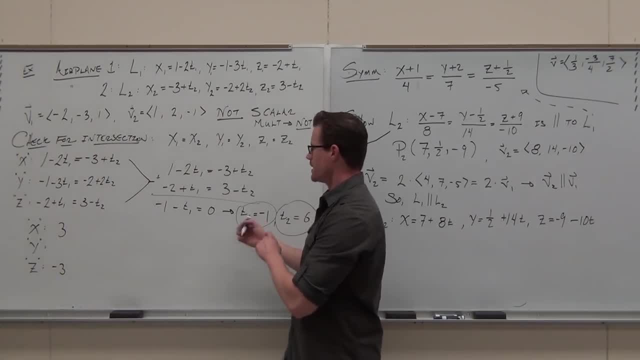 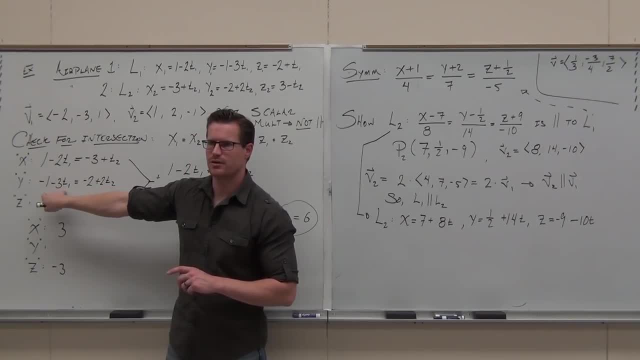 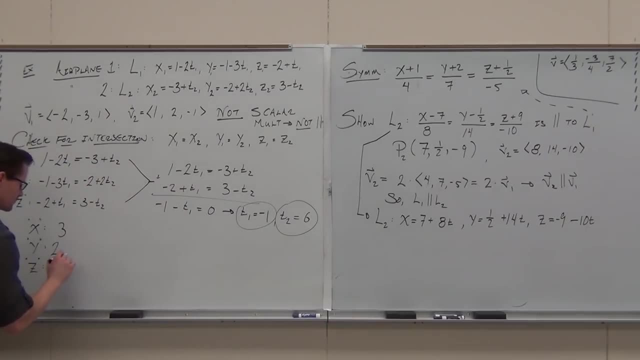 How much do you get? You should calculate it if I ask you. I don't care. How much do you get? Two, Two, Two, Two. Okay, Plug in 6.. are they the same? Here we plugged in this. 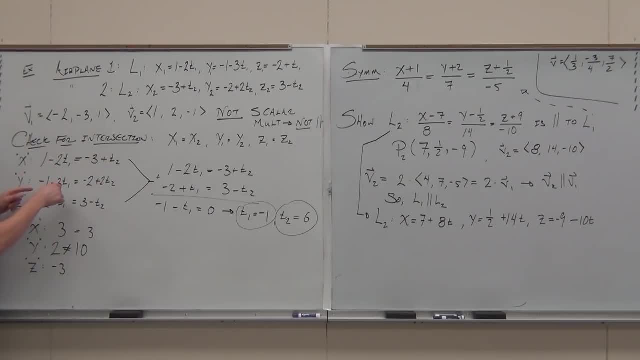 We got 3.. It equaled 3 when we plugged in here, Here we got it: We got negative 3.. It equaled negative 3.. We got 2.. We got 10.. That says that these planes do not intersect. 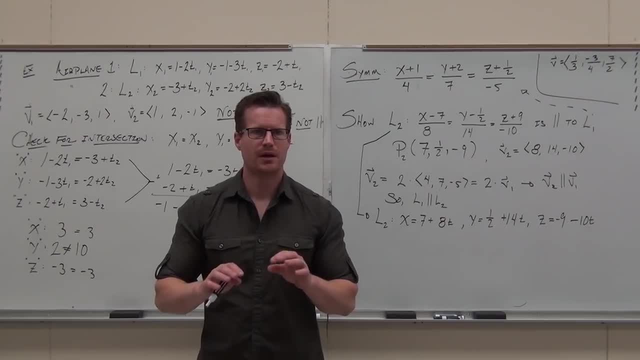 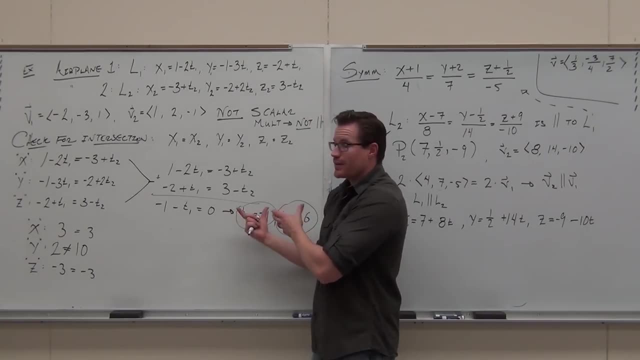 They don't intersect, They're missing at that time. That's what's happening. Do you guys get the idea? It's not this. These times are often different. It's well. they could take off at different times, couldn't they? 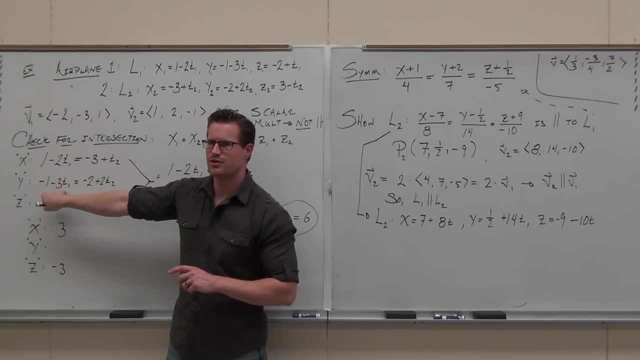 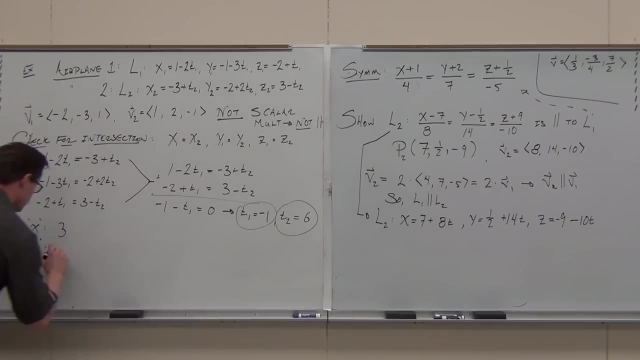 Be careful with it. How much do you get? You should calculate it for me. actually, I don't care. How much do you get? Two, Two, Two, Two. Okay, Let's plug in negative 6.. These two right here. 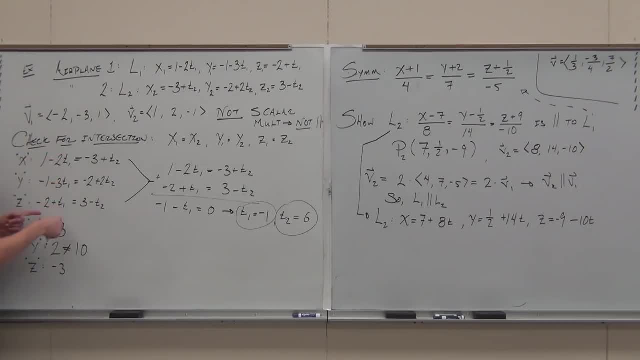 Plug in 6.. Plug in 6.. Are they the same? adults don't know. Here we plugged in this, We got 3.. It equals 3 when we plugged it in here. Here we got it. We got negative 3.. 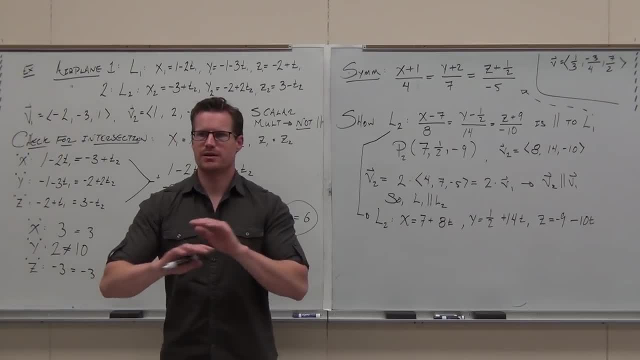 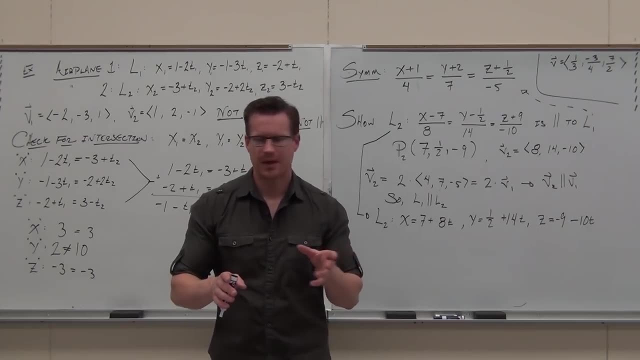 It equals negative 3. We got 2.. We got 10. That says if these planes do not intersect, they don't intersect, They're missing at that time. That's what's happening. Do you guys get the idea? It's not this. 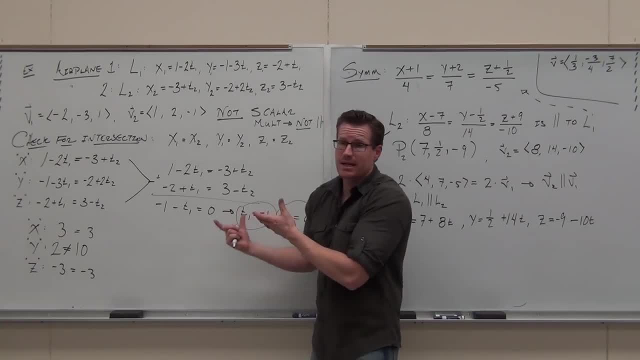 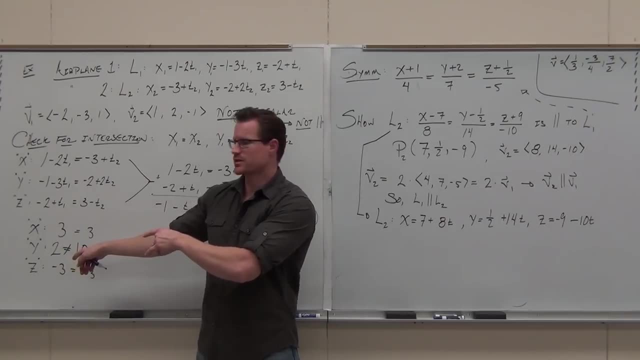 These times are often typically different. It's well, they could take off at different times, couldn't they? So they're different times of the day. That's the one that I'm talking about. It's always the one that you didn't pick for your systems. That's the plan. So if you guys feel okay with that, 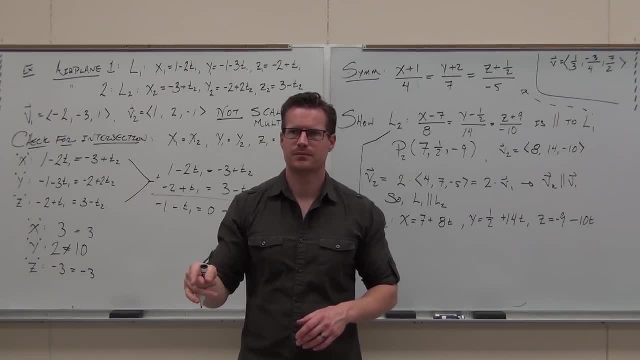 idea. Would you like to try another one? Would you like to do that? I'm going to put one on the board. I want you thinking about it, See if you can do it. Test yourself. I know we have a break. I'm going to give you a couple extra minutes. You're welcome, See. 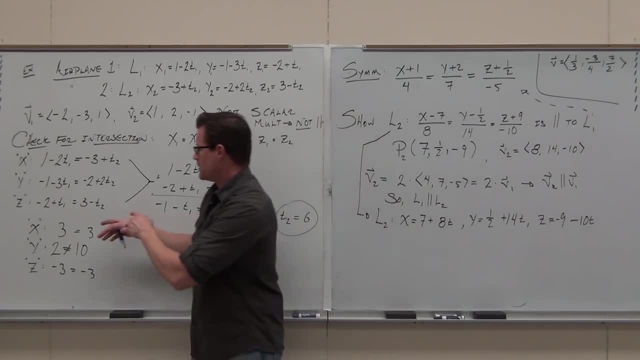 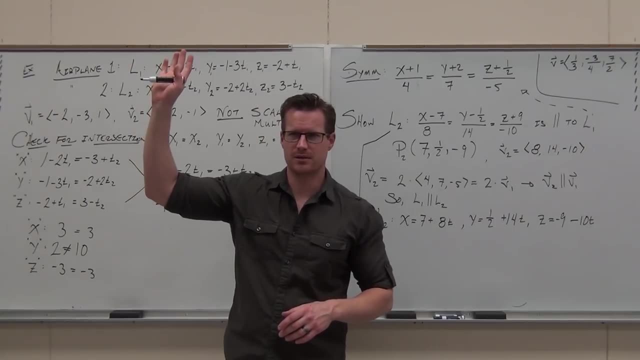 So they're different times of the day. That's the one that I'm talking about. It's always the one that you didn't pick for your systems. That's the plan. So if you guys feel okay with that idea, Would you like to try another one? 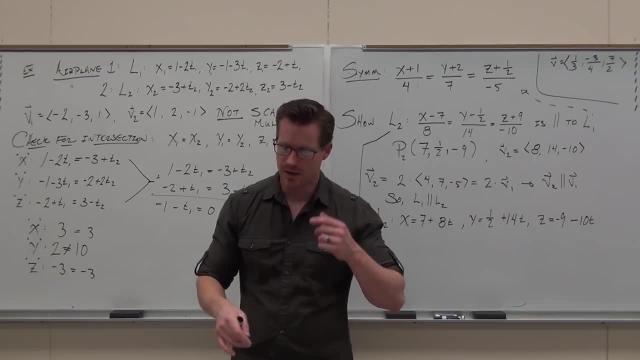 Would you like to do that? I'm going to put one on the board. I want you thinking about it, See if you can do it, Test yourself. I know we have a break. I'm going to give you a couple extra minutes. 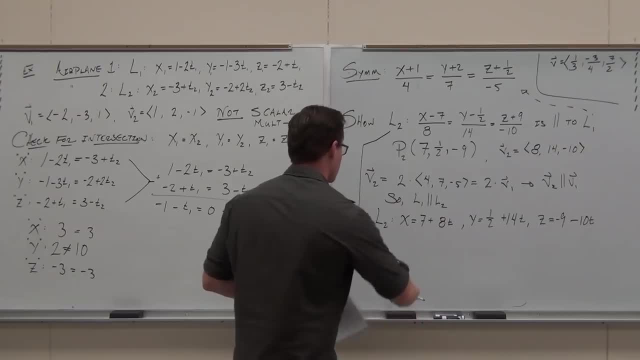 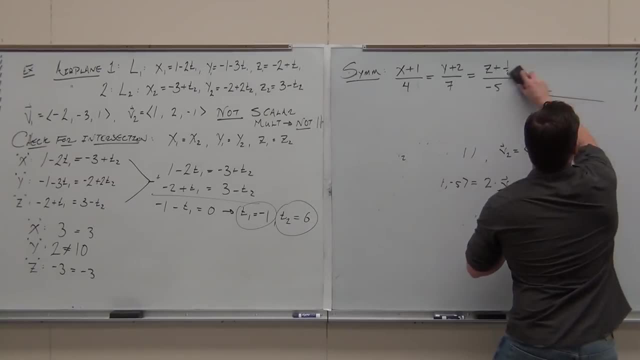 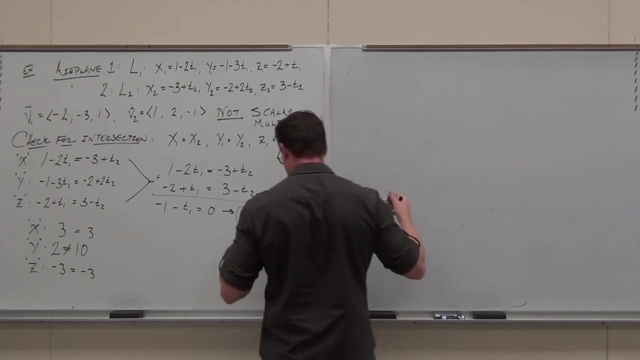 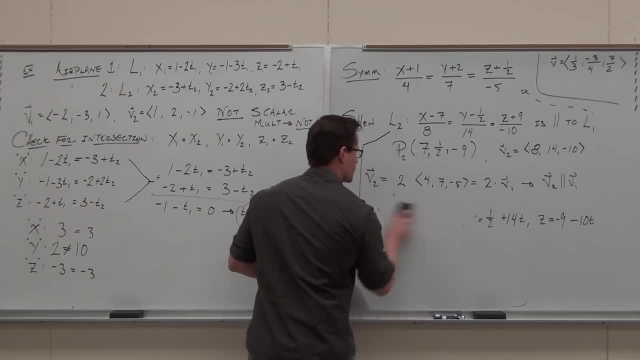 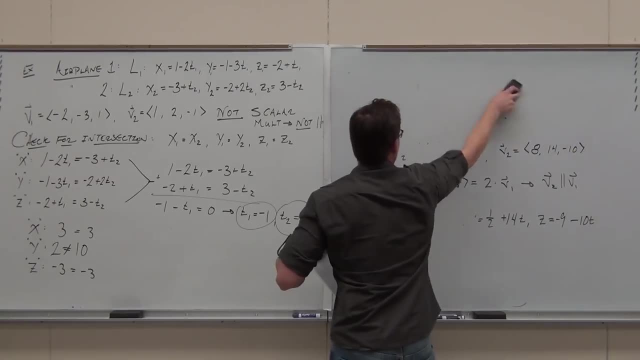 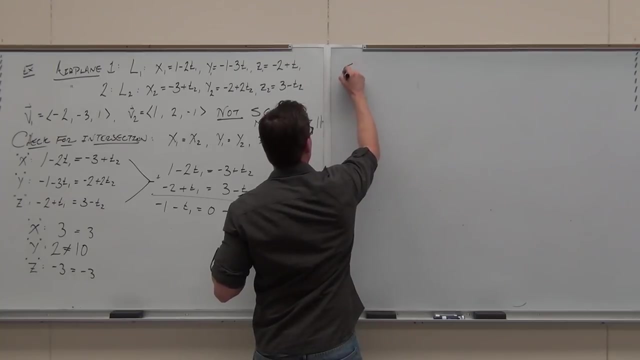 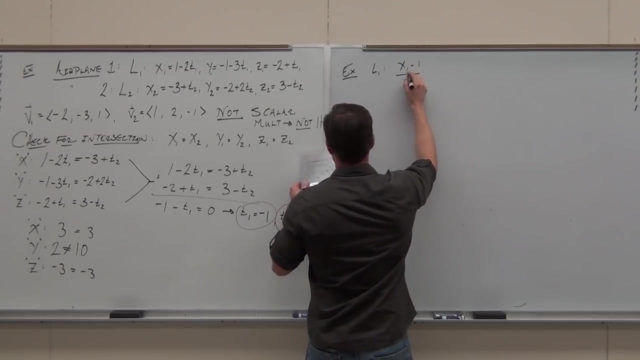 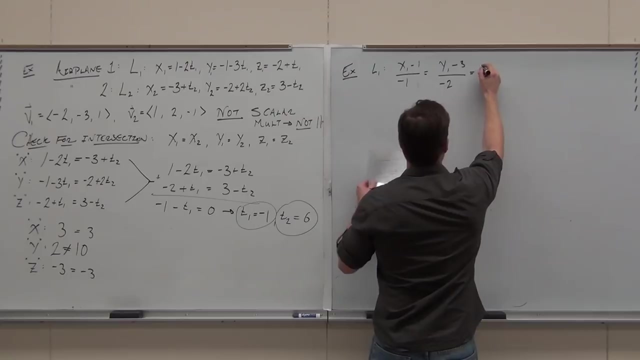 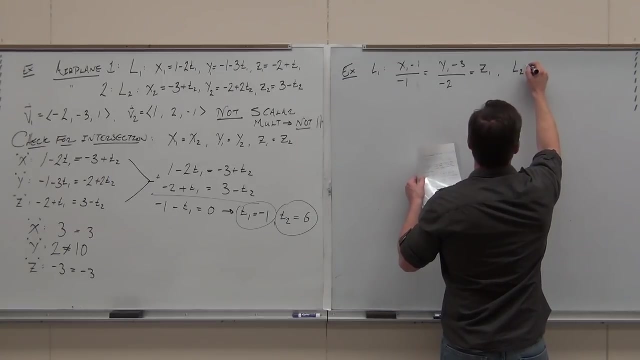 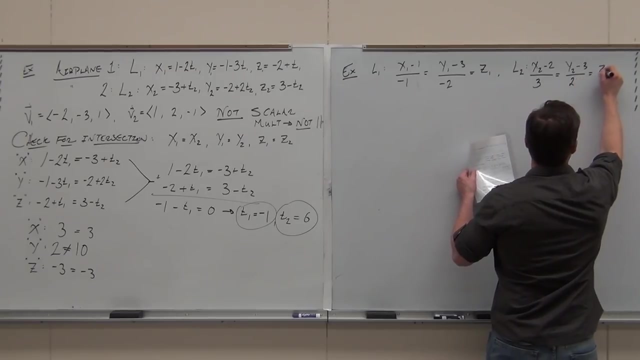 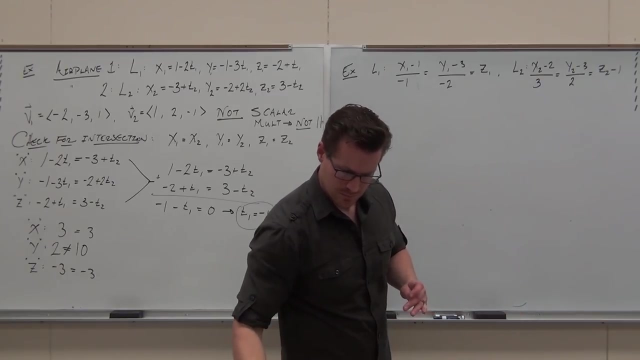 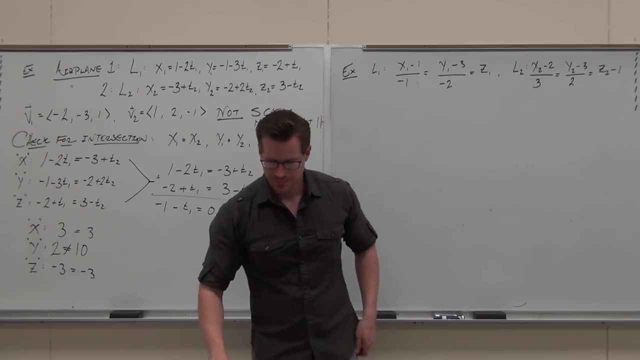 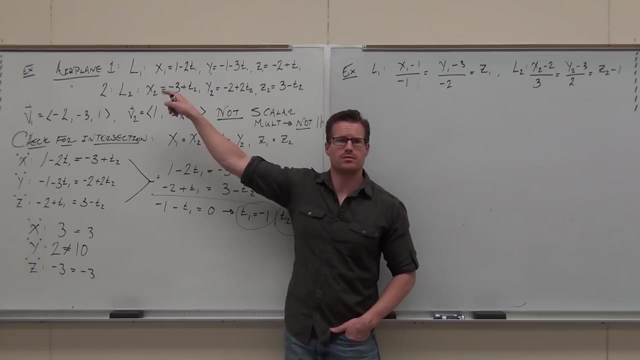 if you can do it. Thank you Right down. I'm going to say just a little blurb and then I promise that I'm going to break us, Probably breaking you right now. Number one thing: were these lines parallel? No, they're not. 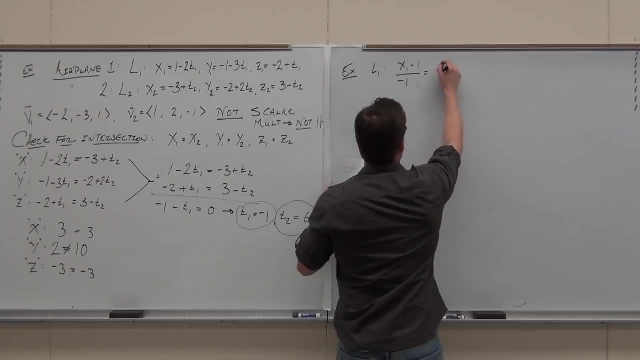 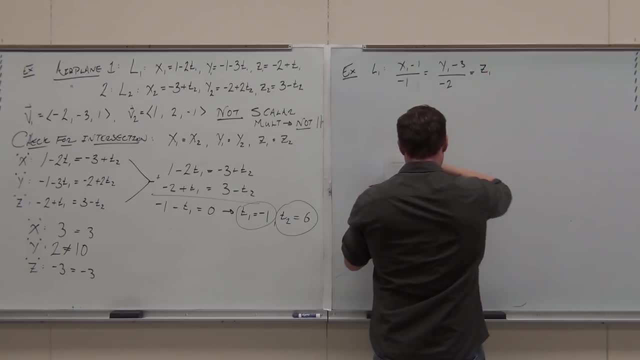 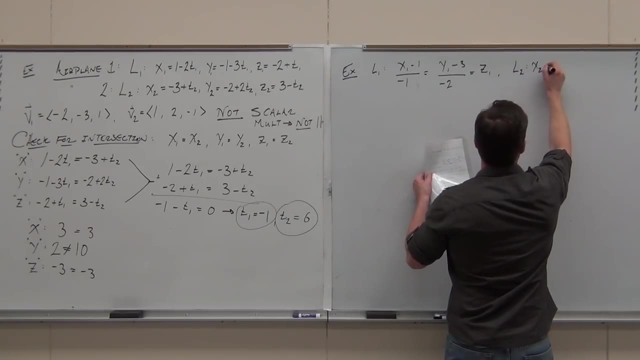 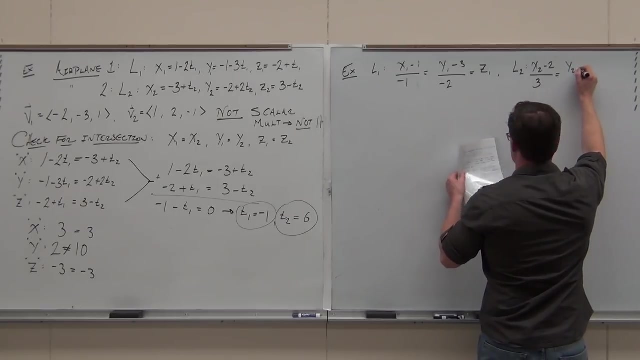 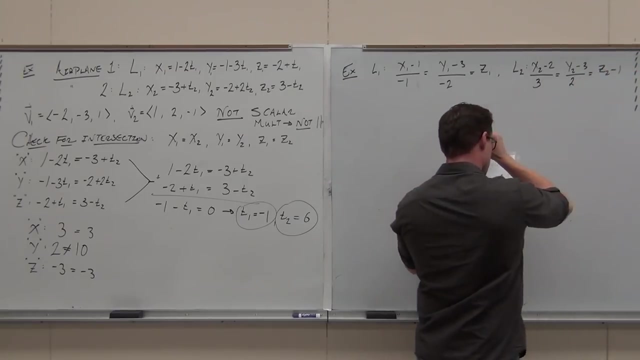 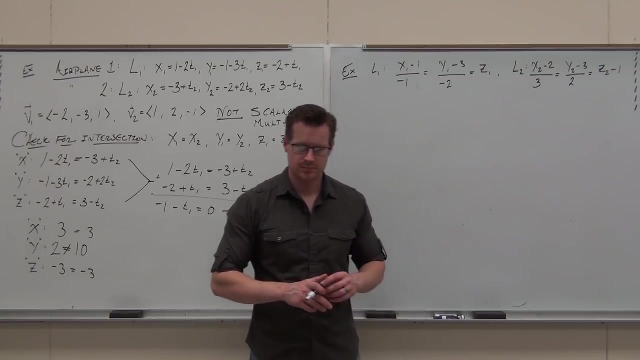 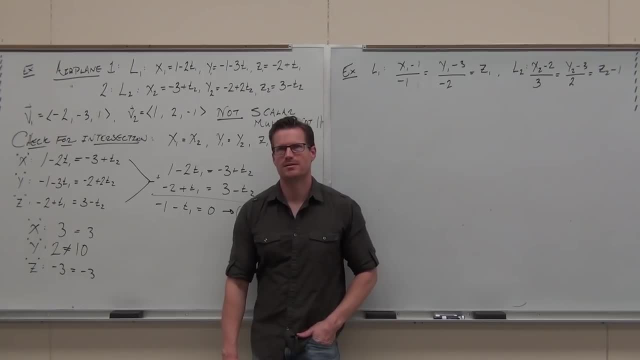 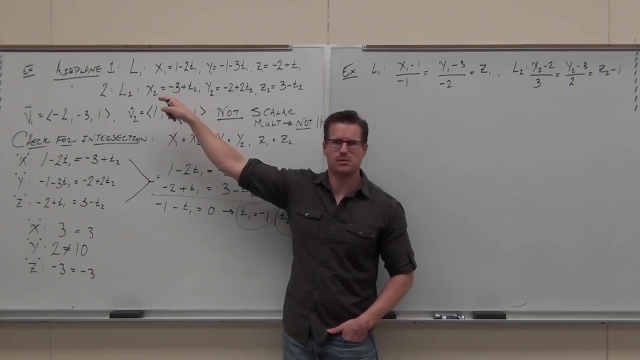 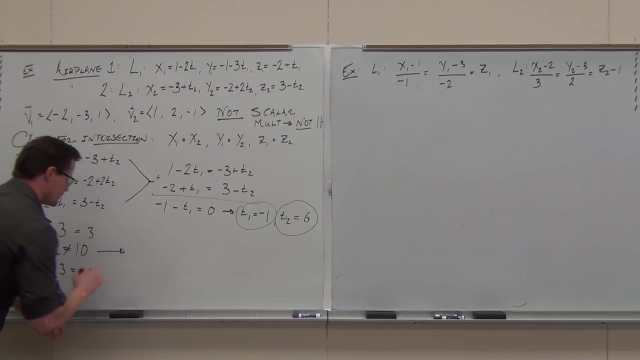 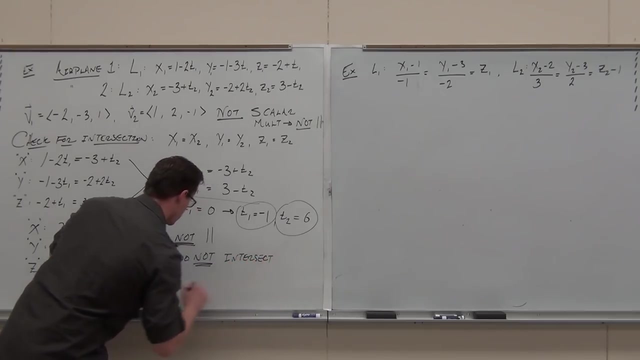 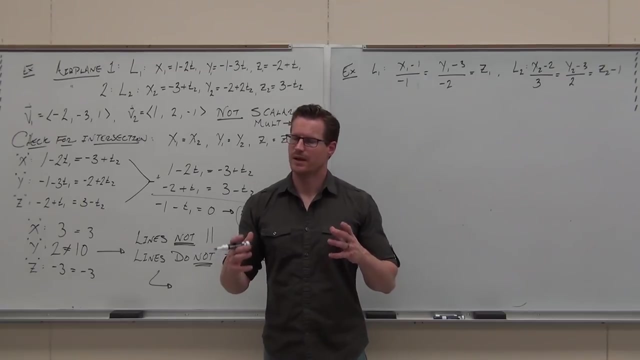 break us. I'm probably breaking you right now. Number one thing: were these lines parallel? Did they intersect? Did they intersect? When you have lines that are not parallel and they don't intersect, they look like this: These aren't parallel, they're not the same direction, they're not crossing. 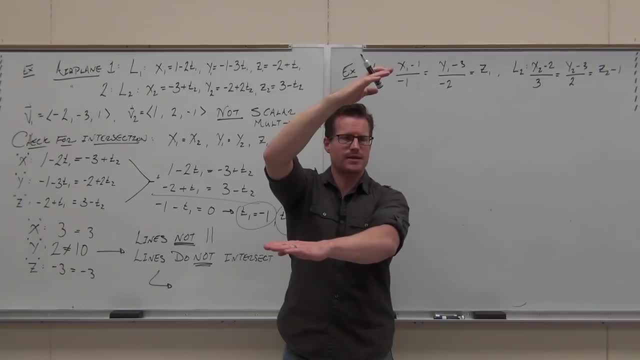 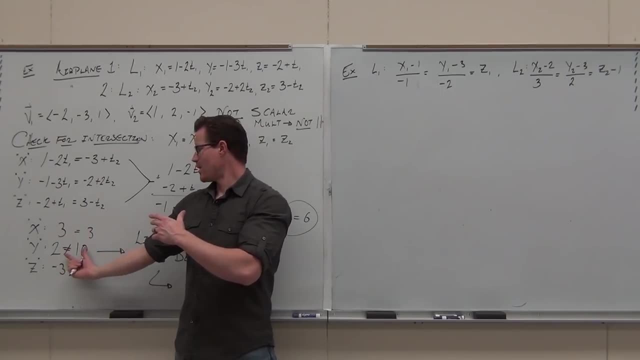 Those are called skew. Skew lines happen a lot. That's what this tells you. It says at these times: I have x equals 3, I got z equals negative 3, I got y equals 2 and y equals 10.. 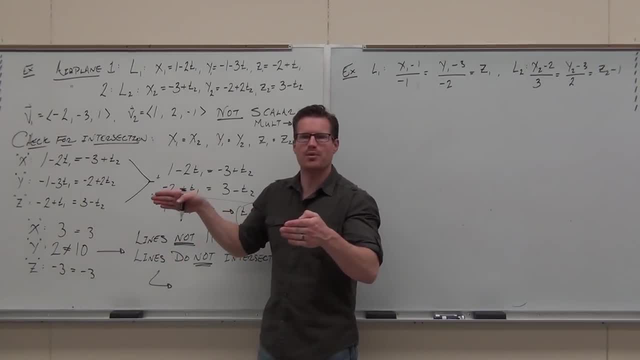 Think about that. You got y equals 2 and y equals 10.. They're separated, They're not intersecting. Even if your x and your z coordinates are the same, your y's are not. when I have those times, The only place they could possibly intersect would be at these times, with the planes respectively. 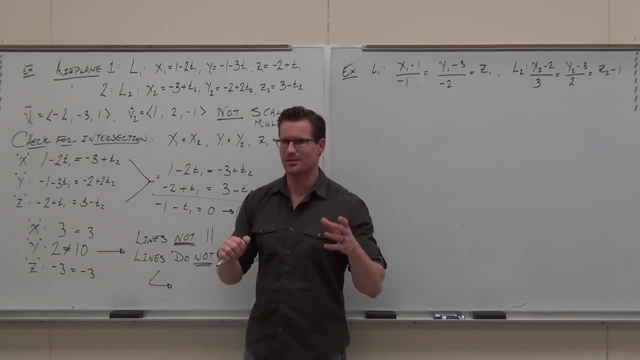 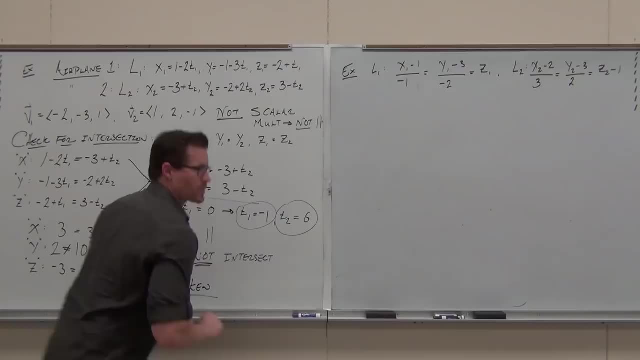 If they're not the same, they're not intersecting. Verify they're not intersecting. Not intersecting. That's called skew. These are skew lines. Here's what I want from us before we take a break, What I want for you to do. number one thing: these two lines I'm going to ask you are: 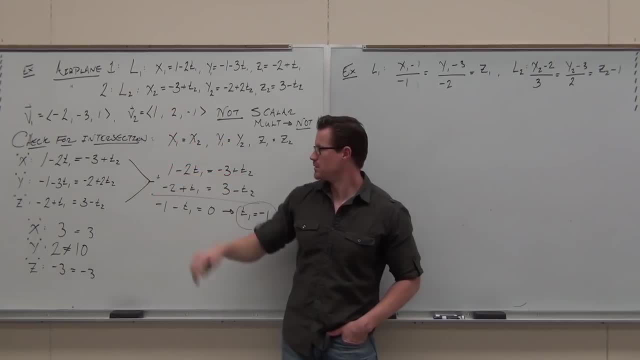 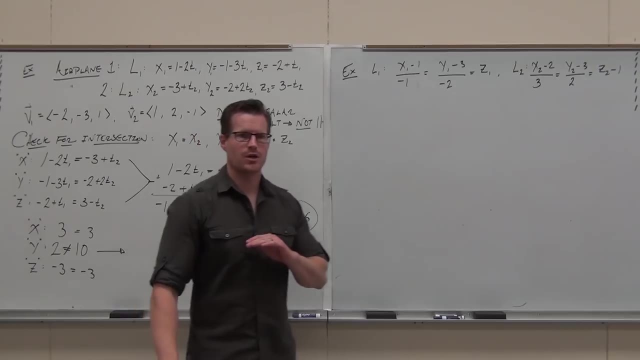 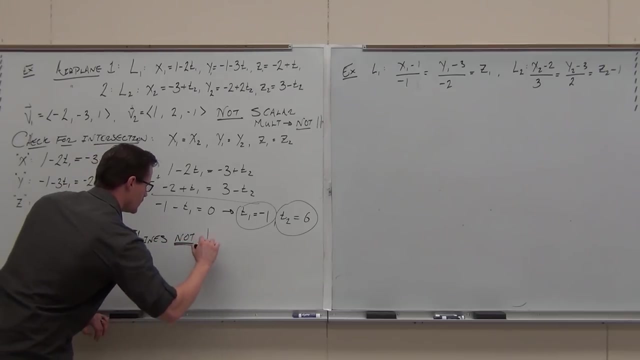 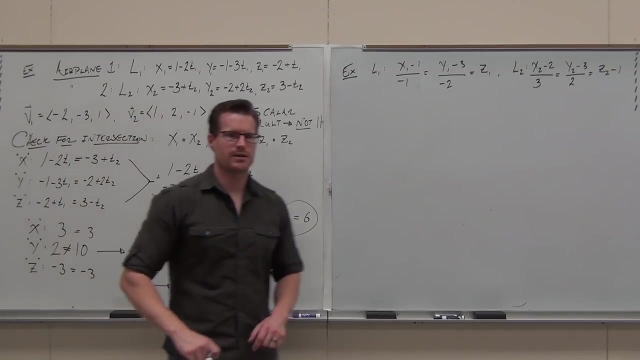 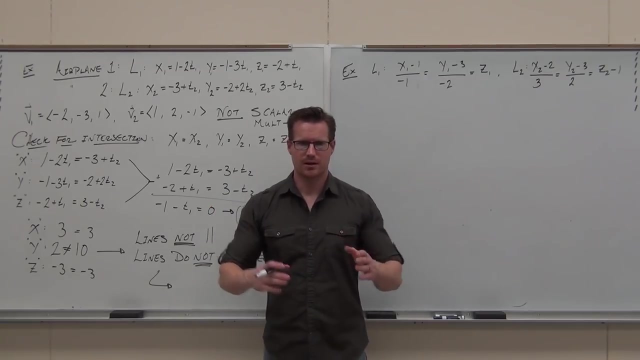 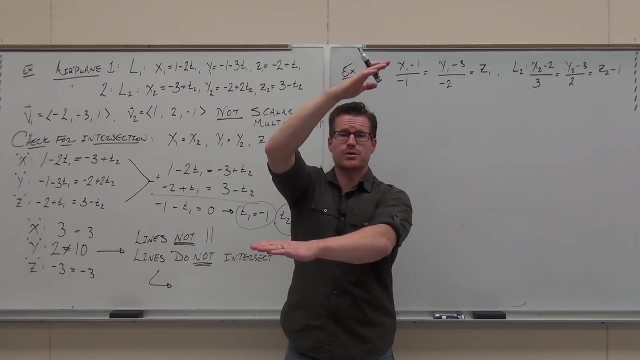 Did they intersect? Yes, Did they intersect? No. How did they intersect When you have lines that do not, that are not parallel and they don't intersect? they look like this: These aren't parallel, They're not in the same direction. 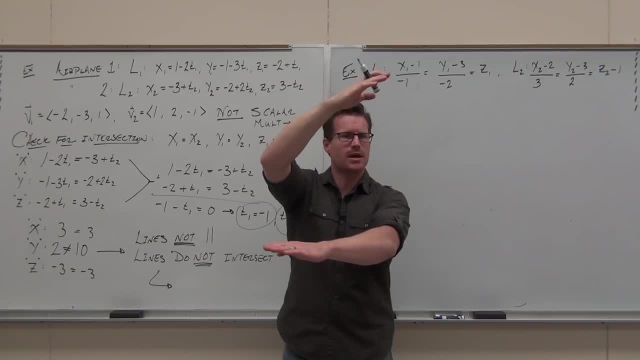 They're not crossing. Those are called skew. Skew lines happen a lot. All right, that's what this tells you. It says at these times: I have X equals 3.. I got Z equals negative 3.. I got Y equals 2 and Y equals 10.. Think about that. You've got Y equals 2 and Y equals. 10. This is new. Think about that. This is how you look. You look at, this is a nice bezel, isn't it? You look at two lines in supreme, not one left and one in right, just like two ways. You're like: look at what are those Right? These lines go in this way. 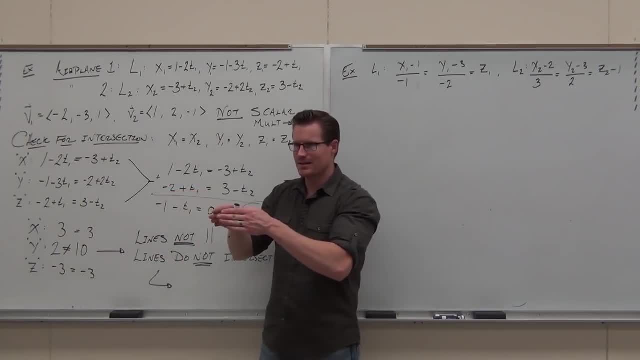 Think about that. you got y equals 2 and y equals 10, they're separated, they're not intersecting. even if your x and your z coordinates are the same, Your y's are not. when I have those times, The only place they could possibly intersect would be at these times. 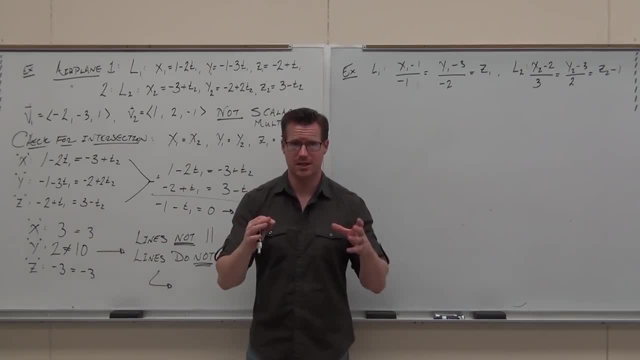 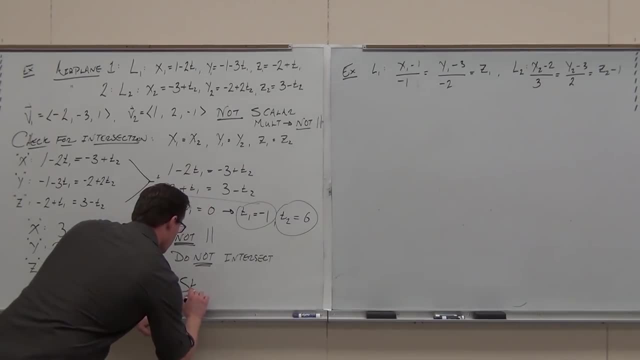 with the planes respectively. If they're not the same, they're not intersecting. Verify: they're not intersecting. not intersecting. That's called skew. these are skew lines. Here's what I want from us before we take a break. 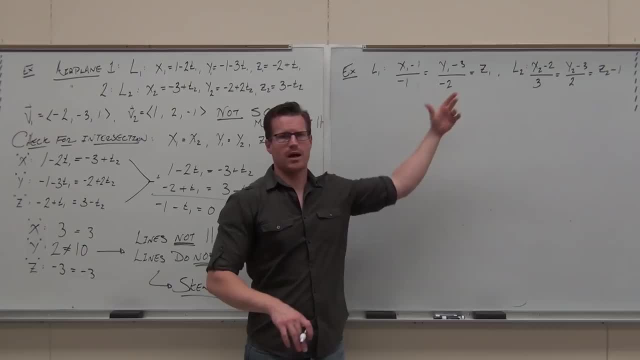 What I want for you to do. number one thing: these two lines I'm going to ask you: are they parallel, are they skew or do they intersect? I want all three answers. Are they parallel? That's talking about the vectors. 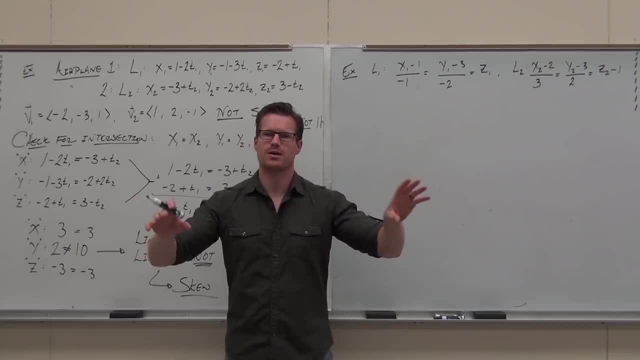 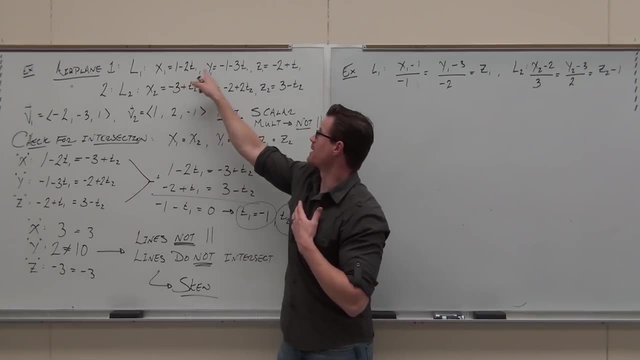 Find the direction vectors, see if they're scale multiples. that's the easiest question. okay, Find out if they're parallel. After that, check for the intersection, just like this. If it helps you- and it does, it helps me to write them out like this: 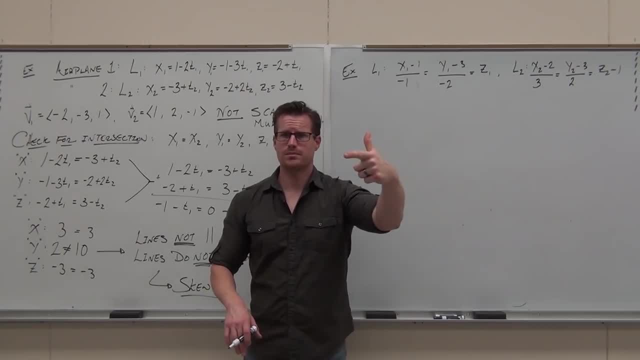 they parallel, Are they skew Or do they intersect? I want all three answers. Are they parallel? That's talking about the vectors. Find the direction vectors. See if they're scaling multiples. That's the easiest question. Okay, Find out if they're parallel. 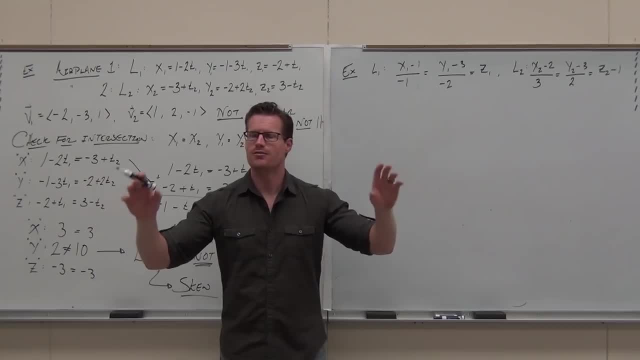 After that, check for the intersection, Just like this. If it helps you- and it does, it helps me- to write them out like this, because it makes checking really easy. This is awkward because they're the symmetric equation. Ah, I don't, it's hard. 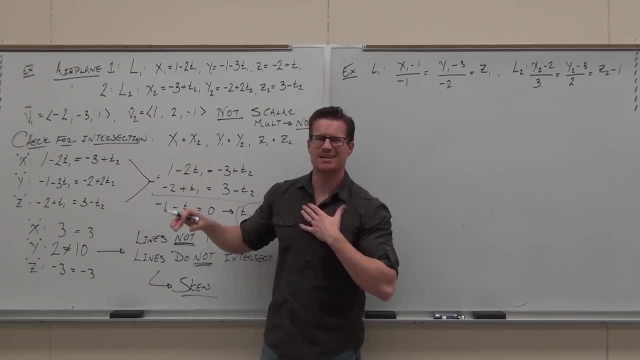 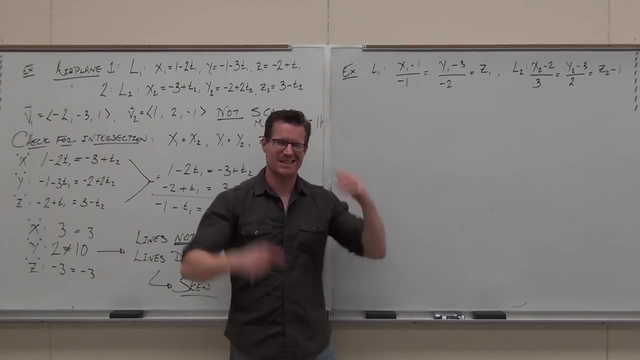 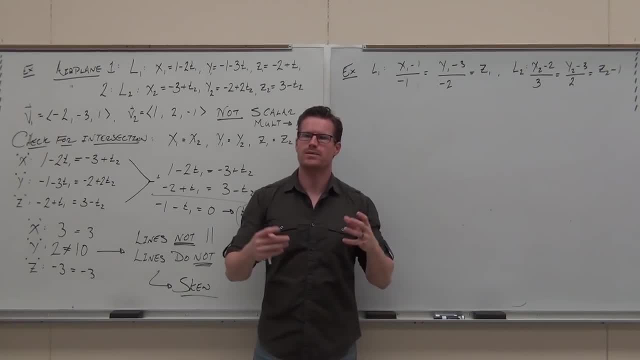 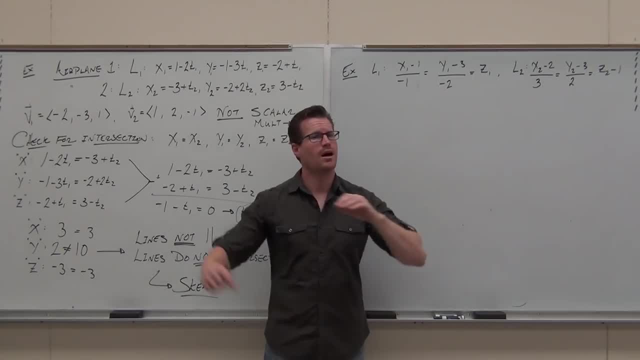 So when I come back, I'm going to crush the problem, but I'm going to do parametric, I'm going to check the direction vectors, I'll check parallel, I'll check intersections And then we're going to go from there. 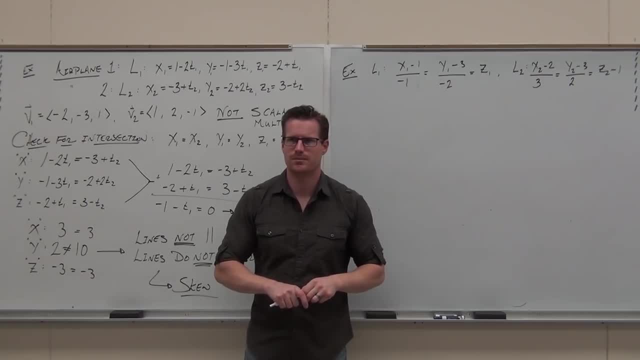 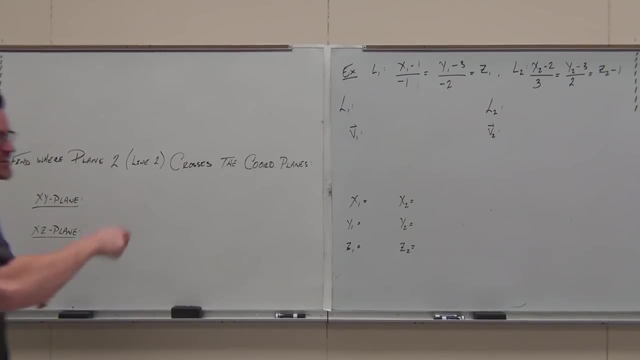 Do you guys understand what I want you to do? Okay, we'll be back in a second. I told you we were going to crush the problem. We're going to go through it really, really fast. Listen, this is just. this is actually a really really really, really, really, really really. 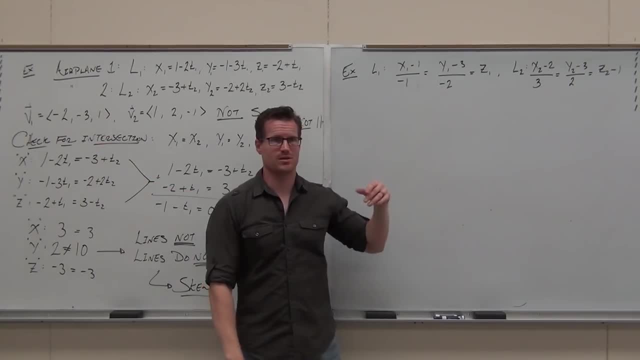 because it makes checking really easy. This is awkward. Is there the symmetric equation? ah, I don't, it's hard. ehh, Maybe set them up as parametric. That's what I'm going to be doing, the first thing. 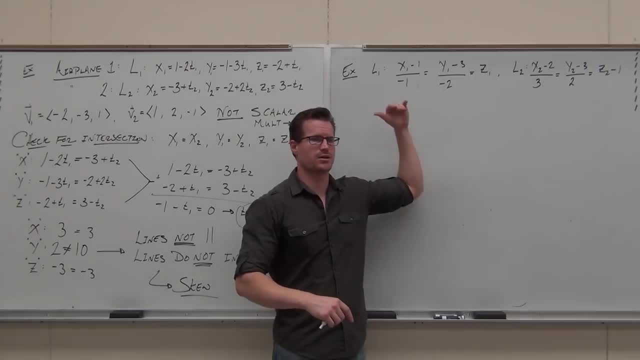 So when I come back, I'm going to crush the problem, but I'm going to do parametric, I'm going to check the direction vectors, I'll check parallel, I'll check intersections and then we're going to go from there. 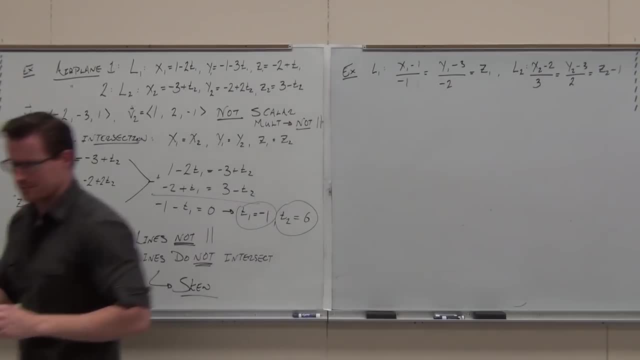 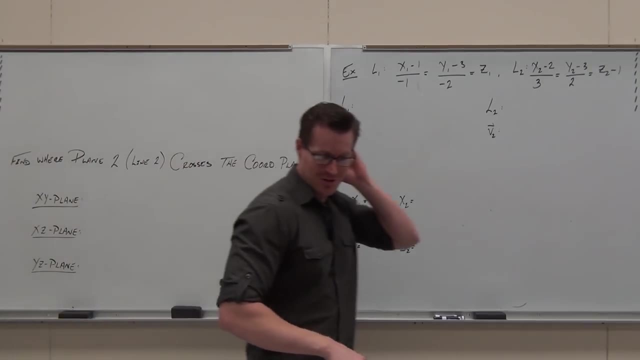 Do you guys understand what I want you to do? Okay, we'll be back in a second. I told you we're going to crush the problem. We're going to go through it really, really quickly. Listen, this is just. this is an extra. 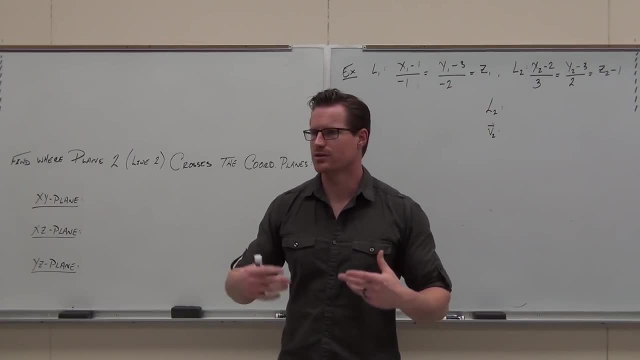 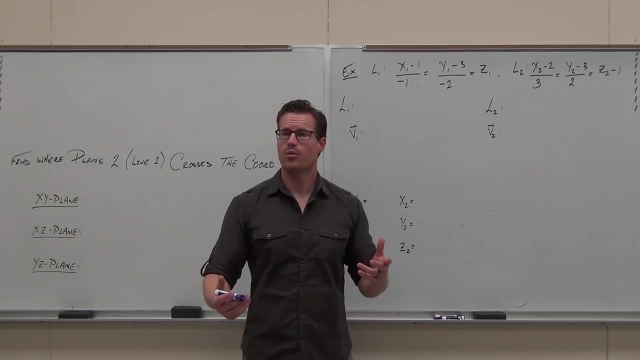 I want to tell you how to do it, but we're going to go through because I know it takes a while to absorb this stuff. So here's the idea. Let's suppose these are planes. Do the planes crash? Number one: the easiest way to check this is: are they parallel? 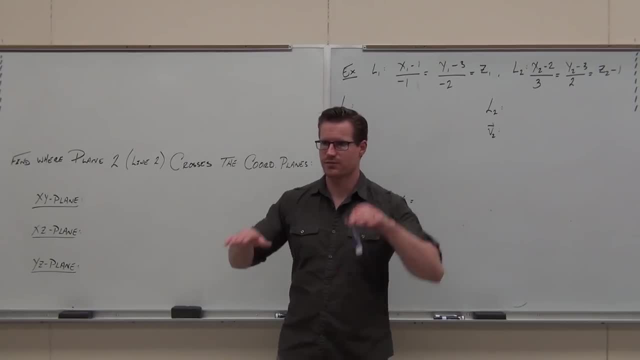 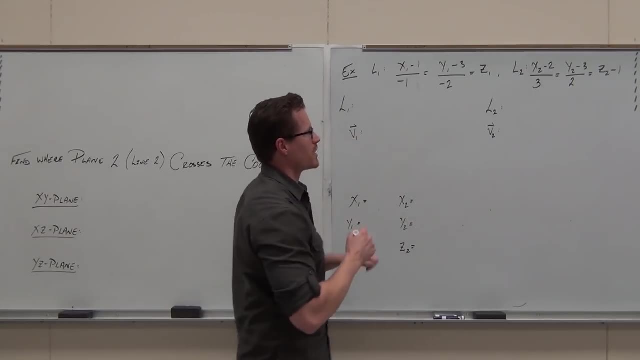 If they are parallel, they don't crash, They do not intersect. Think of planes landing: One lands first, the other lands second. They those things cannot crash In in the air. they're flying the same direction. Now, number one thing: if you ever get: 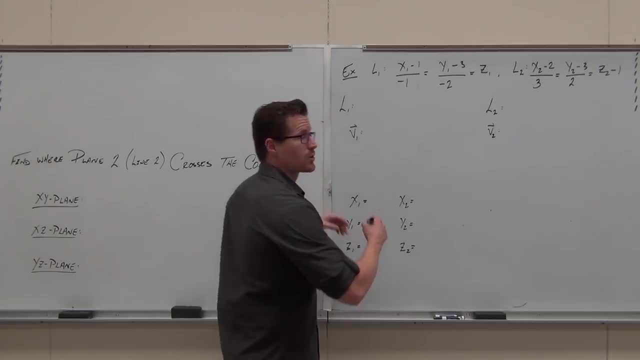 a plane that's symmetric and you don't like it. learn how to change to parametric equations of these lines. So when we do this, just give yourself a little T1, though. That way you know that you're talking about plane number one. 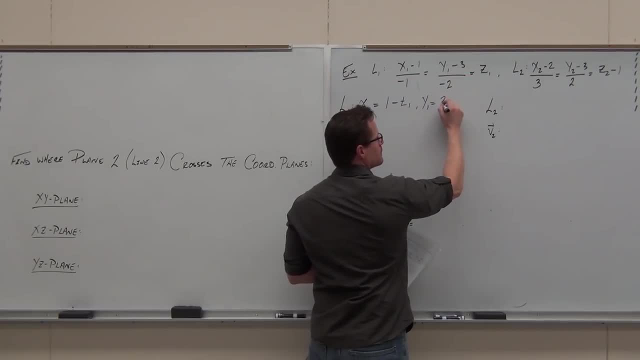 Multiply an imaginary T1 by negative 1.. Negative 2, add the 3. Oh, Z1.. That's weird When you get that that Z1, there's nothing around there. Well, there is. It's still divided by 1.. 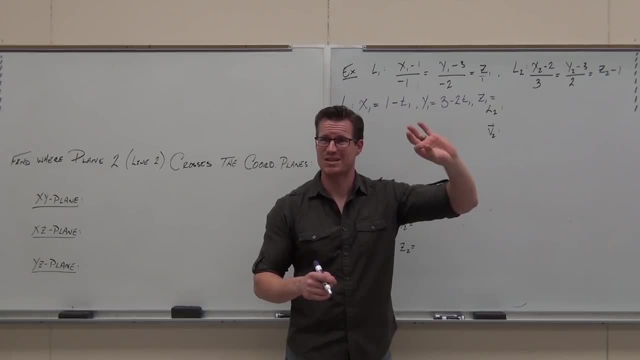 So in this case, when you have that Z1 divided by 1 equals T1, that's what it is: Z1 equals T1.. There's just no X. sorry, there's no Z coordinate on the point. That's. that's the idea. 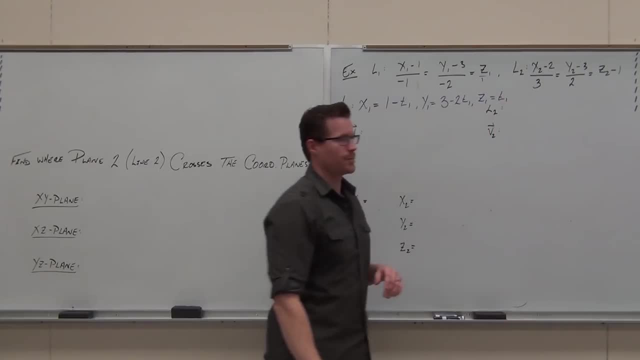 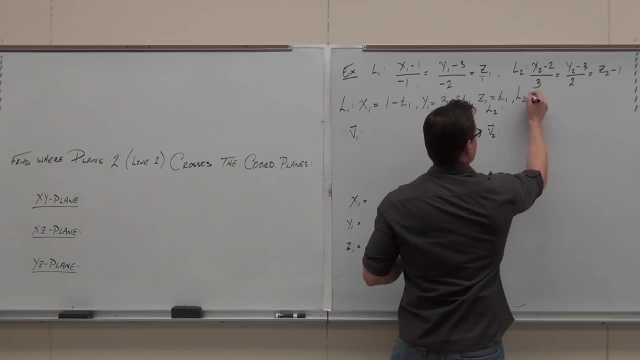 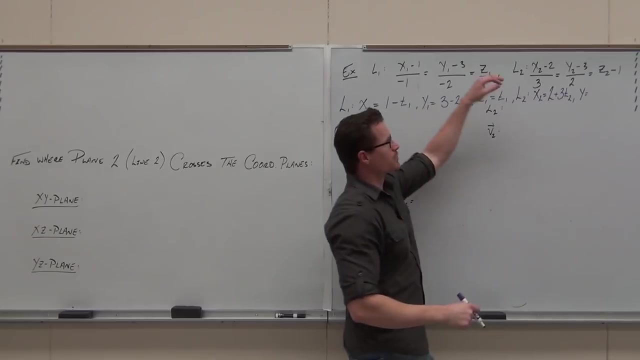 So this would equal T1, you guys okay with the the idea here? L2, same stuff. multiply the T2 times 3, add the 2.. Multiply the imaginary T2 times 2, add the 3.. 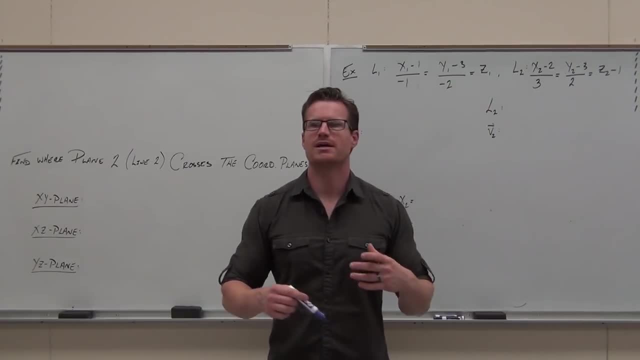 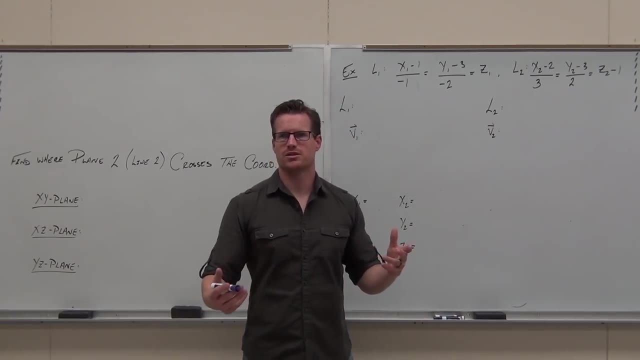 This is just. this is extra. I already taught you how to do it, But we're going to go through because I know it takes a while to absorb this stuff. So here's the idea. Let's suppose these are planes. Do the planes crash? 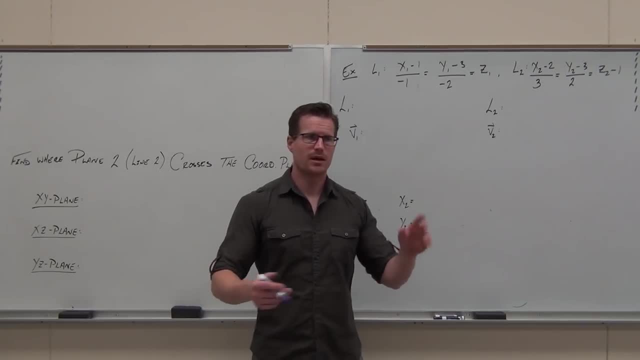 Number one. the easiest way to check this is: are they parallel? If they are parallel, they don't crash. They do not intersect. Think of planes landing One lands first, the other lands second. Those things cannot crash In the air. they're flying in the same direction. 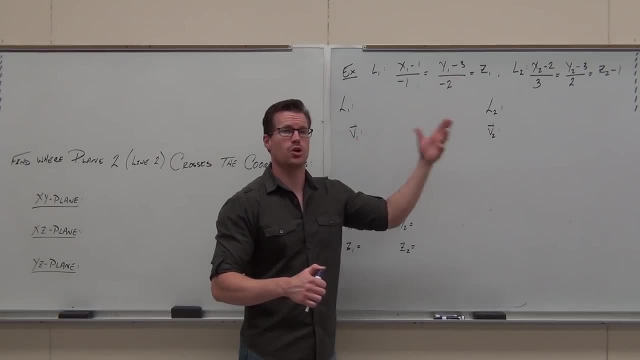 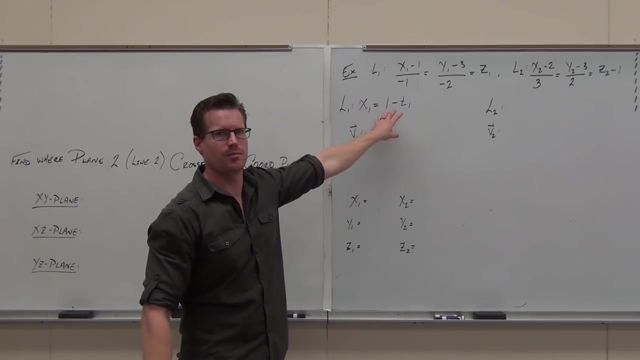 Now number one thing: if you ever get symmetric and you don't like it, learn how to change to parametric equations of these lines. So when we do this, just give yourself a little T1 though. That way you know that you're talking about plane number one. 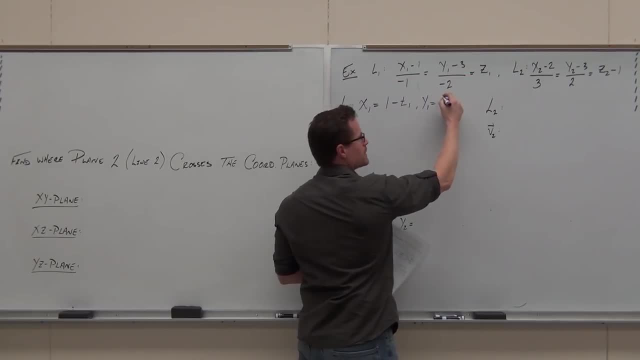 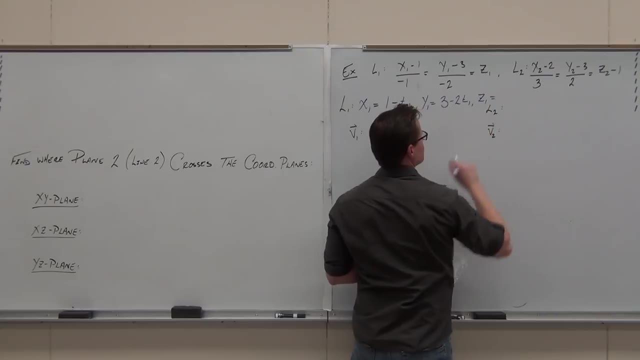 Multiply an imaginary T1 by negative 2, add the 3.. Oh, Z1.. That's weird. When you get that, that Z1, there's nothing around there. Well, there is. It's still divided by 1.. 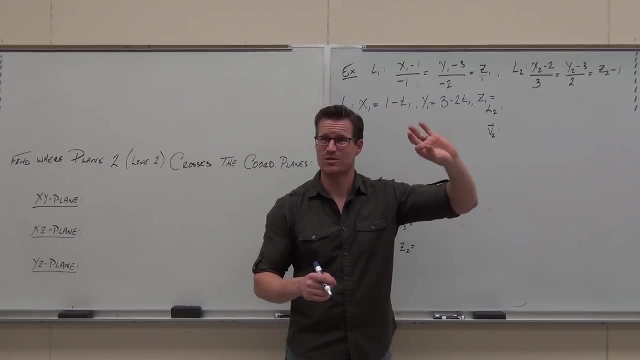 So in this case, when you have that Z1 divided by 1 equals T1, that's what it is: Z1 equals T1.. There's just no X. sorry, there's no Z coordinate on the point. That's the idea. 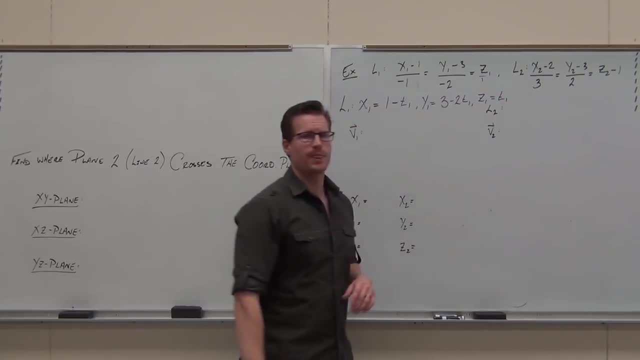 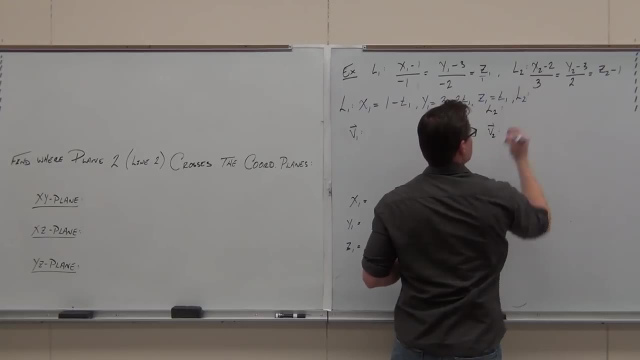 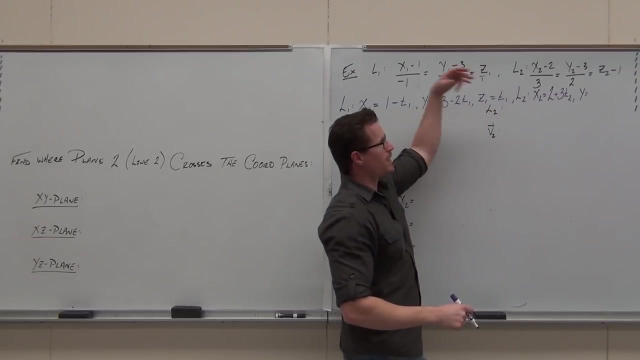 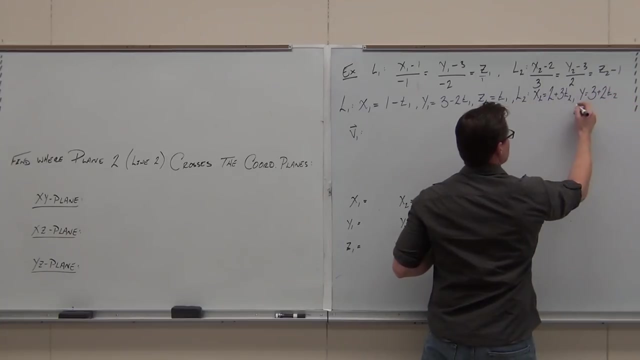 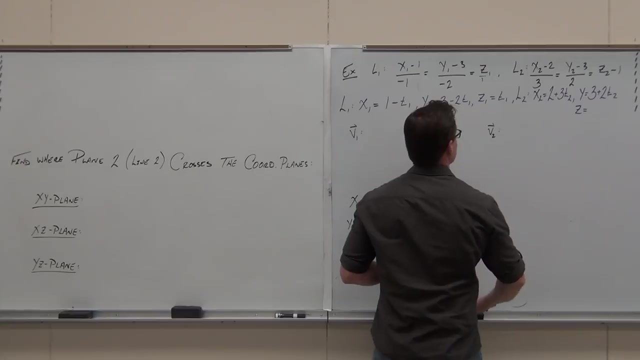 So this would equal T1.. You guys okay with the idea here? L2, same stuff. Multiply the T2 times 3, add the 2.. Multiply the imaginary T2 times 2, add the 3.. It's about 1 plus T for Z2.. 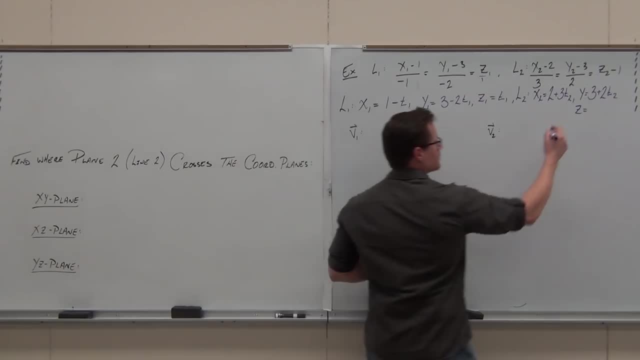 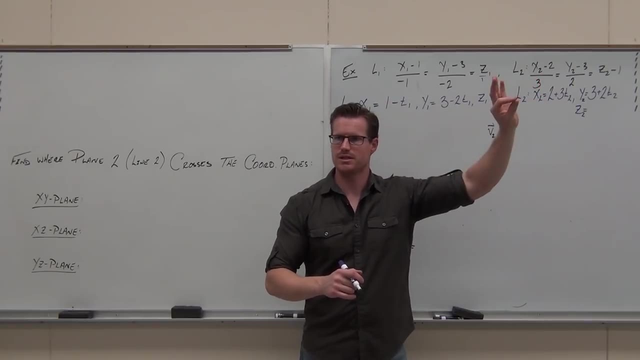 Say that again. Is that 1 plus T for Z2? For Z2.. Well, imagine the T2,. okay, what's the denominator? Well, 1.. So 1 times the T2, add the 1. So you said 1 plus. 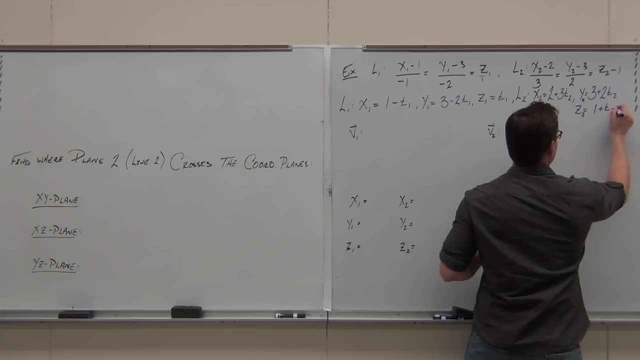 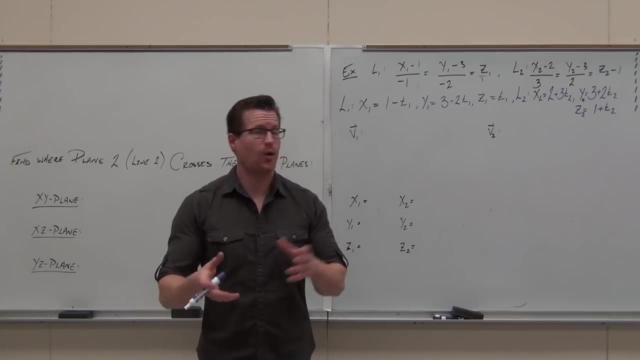 Z2.. Yeah, I need a head nod if you're okay with those things. Now, as soon as you've done that, or from here, it doesn't matter folks, whatever you feel comfortable with. That's why I'm giving you both so we get comfortable with them, because you need to be. 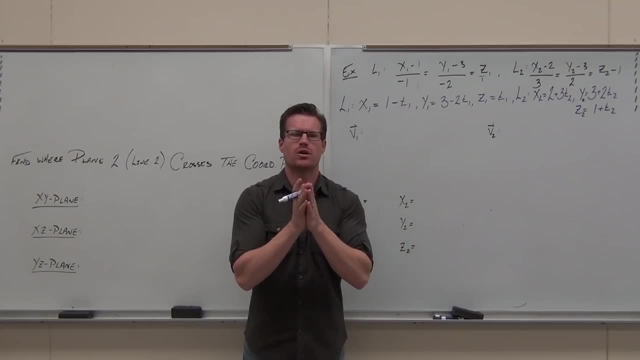 Next thing: check parallel. What's going to tell you whether these planes are parallel? What's going to tell you Scales, Scales. Oh, So you need the vectors. Let's find the vectors. Vectors are often easiest from here. 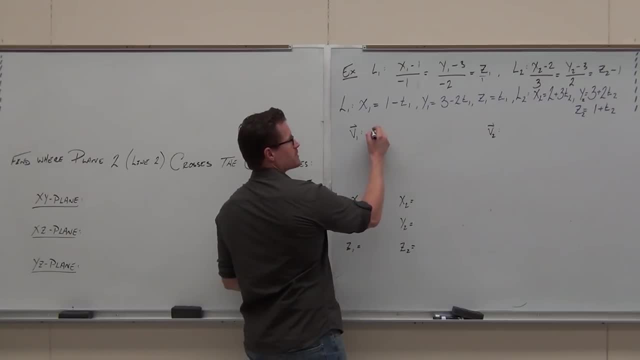 You can still find them from here. Vector for plane 1 and direction 1.. The direction vector is negative 1,, negative 2, and 1.. Don't forget the 1.. It's not 0 because there's a Z1 being equal. 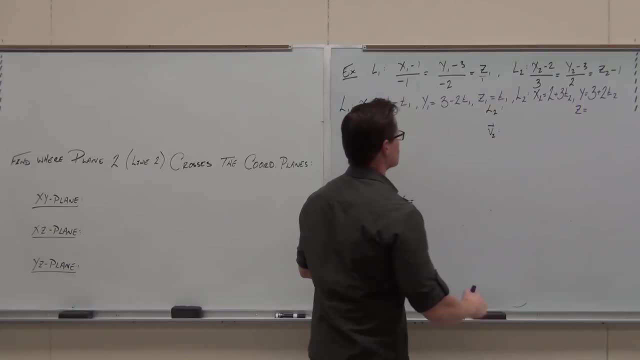 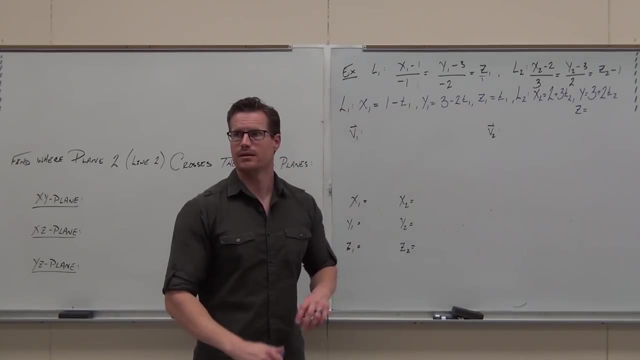 That's how you do it. That's how you do it. That's how you do it. So you're going to have 1 plus T for Z2.. Say that again. Is that 1 plus T for Z2? For Z2.? 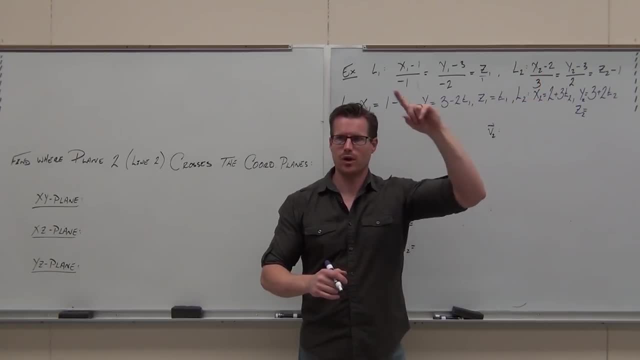 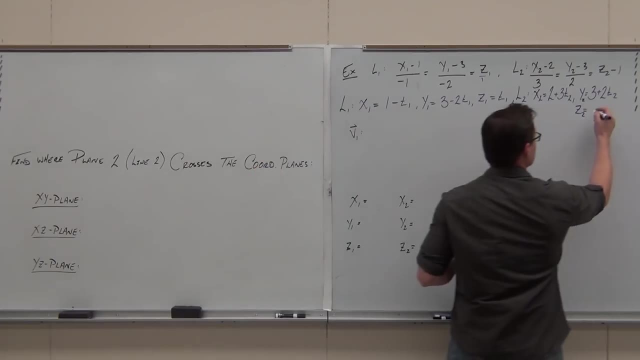 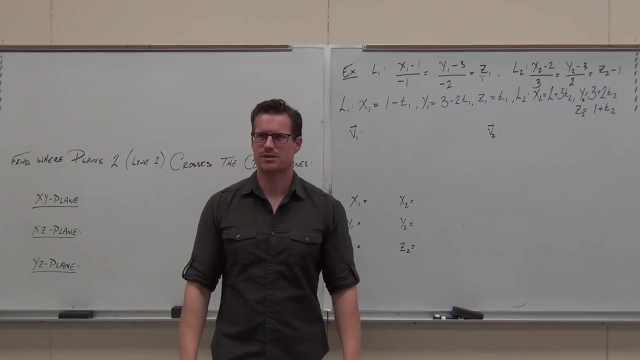 Well, imagine, imagine the T2.. Okay, what's? what's the denominator? Well, 1.. So 1 times the T2, add the 1.. So you said 1 plus. Yeah, I need a head nod if you're okay with those things. 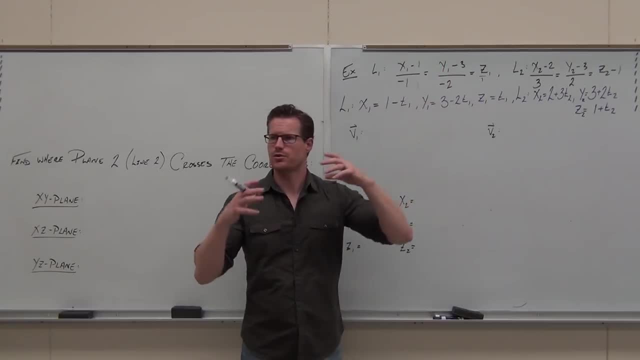 Now, as soon as you've done that, or from here, it doesn't matter folks, whatever you feel comfortable with. that's why I'm giving you both, so we get comfortable with them, because you need to be Next thing check parallel. 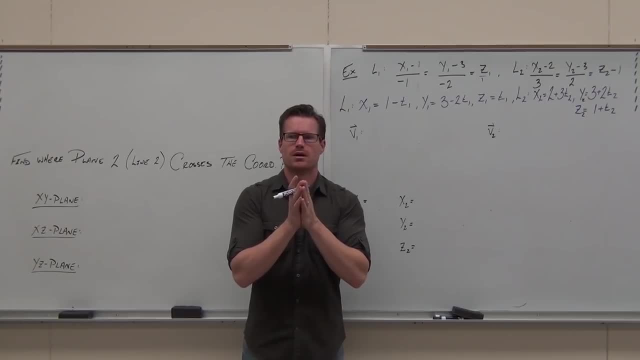 What's going to tell you whether these planes are parallel? What's going to tell you Scalable, Scalable. Oh, So you need the vectors. Let's find the vectors. Vectors are often easiest from here. You can still find them from here. 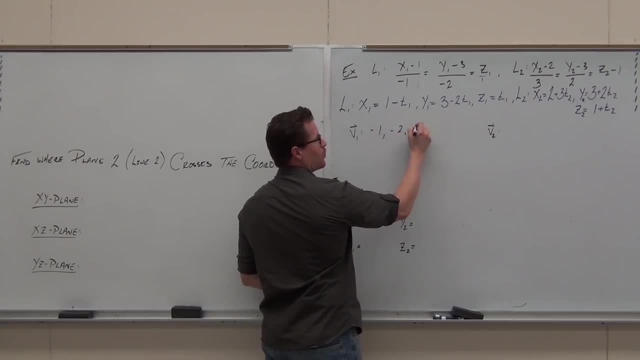 Vector for plane one. the direction vector is negative one. negative two and one. Don't forget the one. It's not zero, because there's a Z1 being equal, It's one. in that case, Same thing. right there, You guys are okay with the negative one, negative two, one. 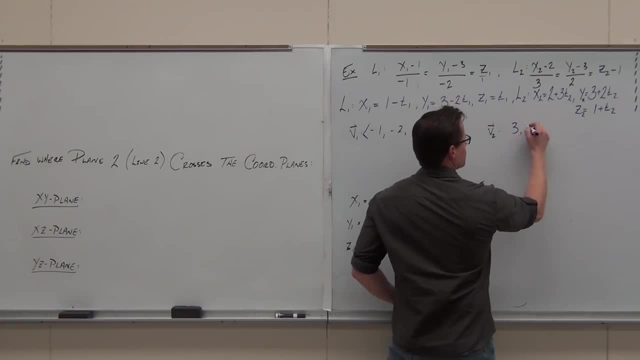 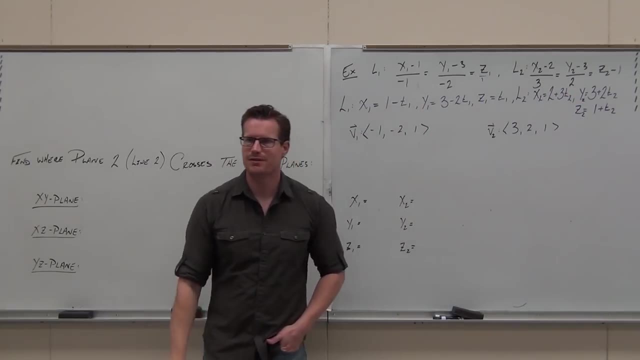 What's the other direction vector? Quickly, please. Yep, here or here, either way. three, two, one Man. this is about the easiest one I've ever given you to check a parallel. Are these things parallel? Parallel? 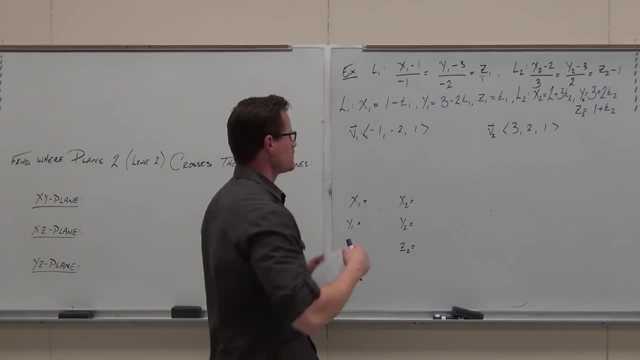 There's no way. They're not scalar multiples. so these are not parallel. Not parallel because they're not scalar multiples and it's pretty obvious. You don't even have to show that, okay, It's obvious, they're not scalar multiples. 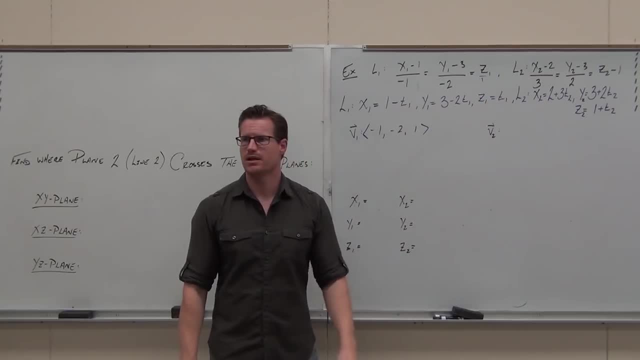 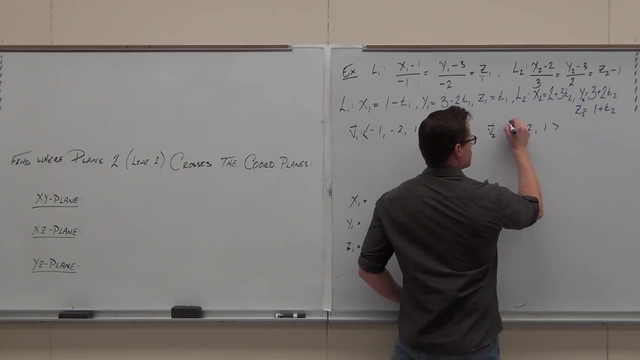 It's 1 in that case, Same thing. right there, You guys. okay with the negative 1, negative 2, 1?. What's the other direction vector? Quickly, please: 3, 2, 1.. Yep. 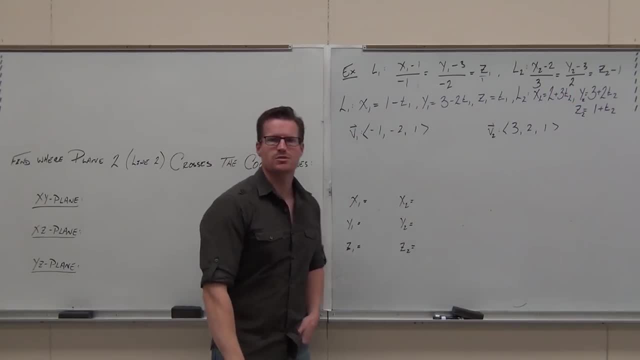 Here or here either way: 3,, 2, 1.. Matt, this is about the easiest one I've ever given you to check a parallel. Are these things parallel Parallel? There's no way. They're not scalar multiples, so these are not parallel. 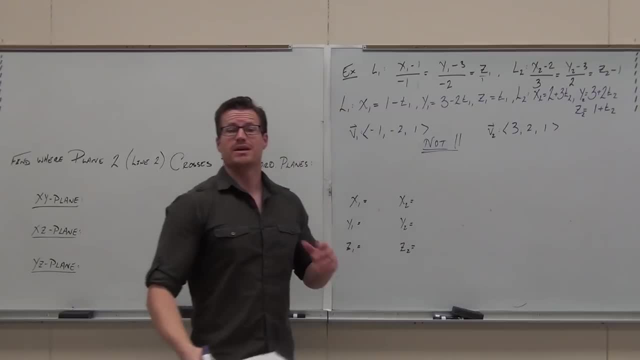 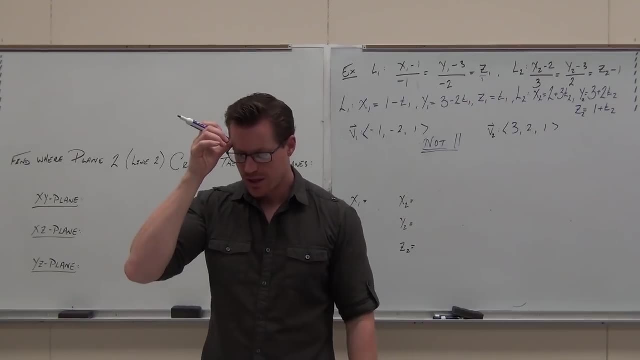 Not parallel because they're not scalar multiples and it's pretty obvious. You don't even have to show that. okay, It's obvious, they're not scalar multiples. Next question: If they're not parallel, do they necessarily intersect? Not necessarily. 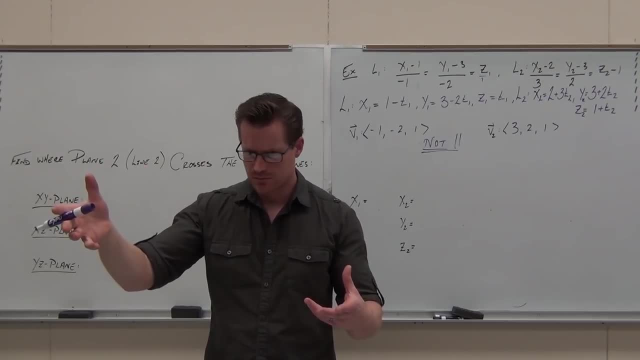 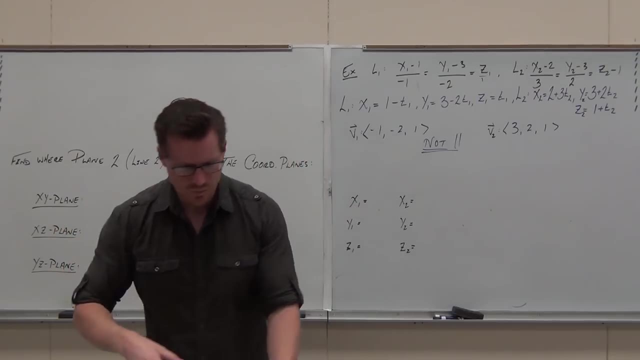 Next question: if they're not parallel, do they necessarily intersect? Not necessarily, They could be skew. So then we're going to check for the intersection. So the next part, we go: okay, let's see, Can we check for the intersection? 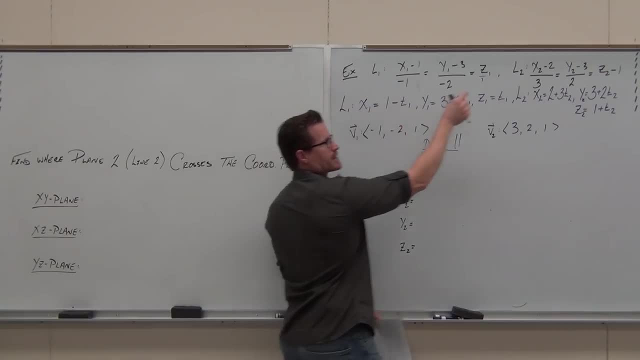 If we check for the intersection, it means that the X1 has to equal the X2, Y2, and I'm sorry, Y1 and Y2 have to be the same and Z1 and Z2 have to be the same. 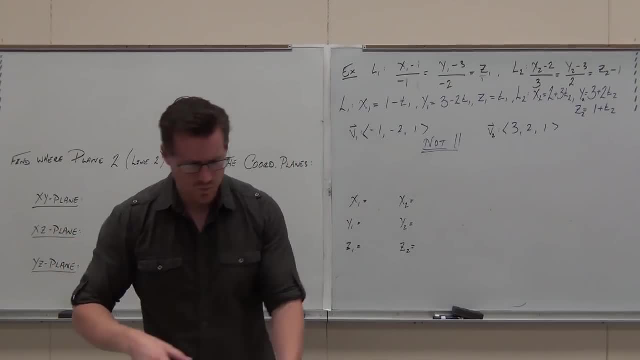 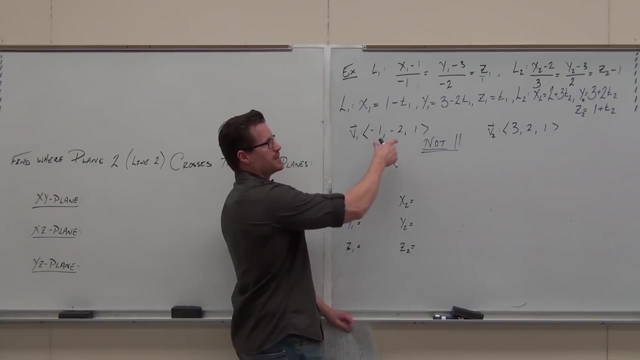 They could be skewed. so then we're going to check for the intersection. So the next part, we go: okay, let's see, Can we check for the intersection? If we check for the intersection, it means that the X1 has to intersect with the X2.. 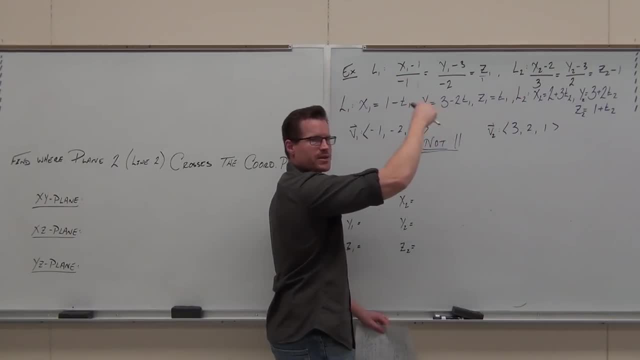 Okay, X1 has to equal to X2, Y2, and I'm sorry, Y1 and Y2 have to be the same and Z1 and Z2 have to be the same, So we set these coordinates equal, Okay. 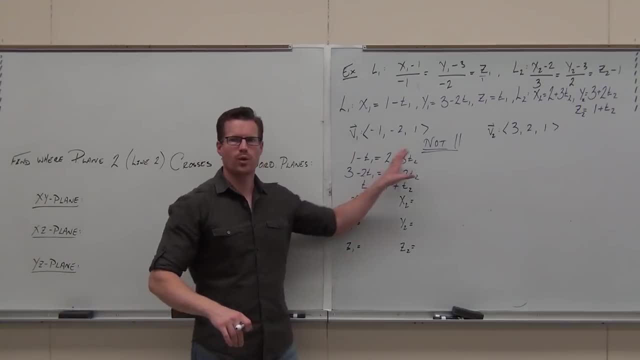 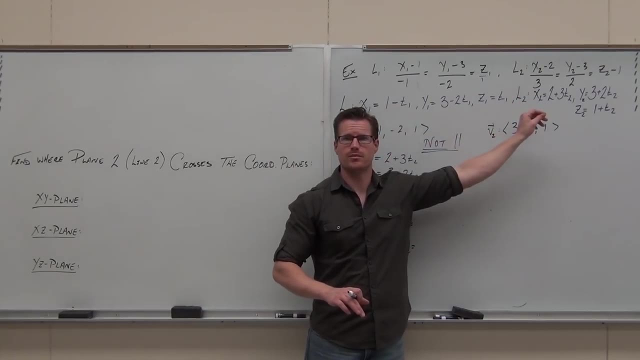 If you can tell where I got these things from, I'll be very pleased. Can you tell where those things came from? Can you tell where these lines came from So you can make it from symmetric to parametric- Sweet Back and forth. 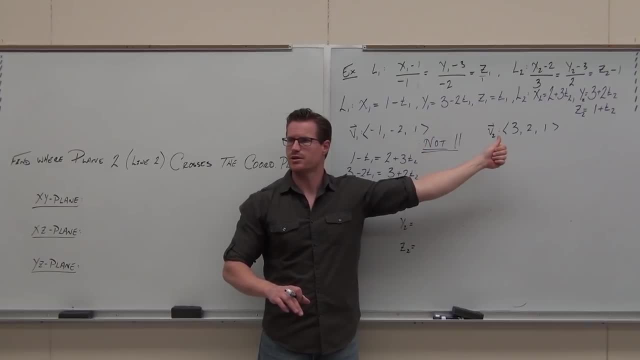 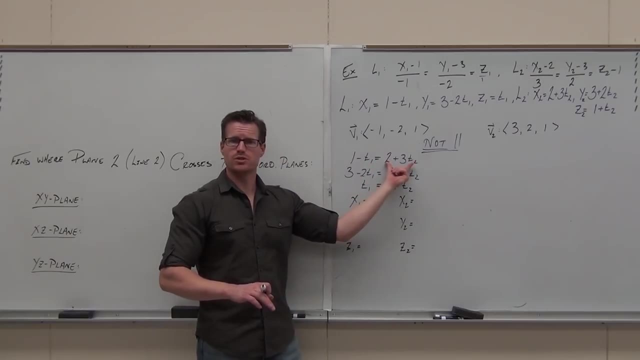 Can you make it from either one to the vectors, the direction vectors. Is it readily apparent that these are not parallel? Yes, Okay, Is it okay that we got these things equal? Do you see where those come from? So, once we have our line X, coordinates have to be equal. 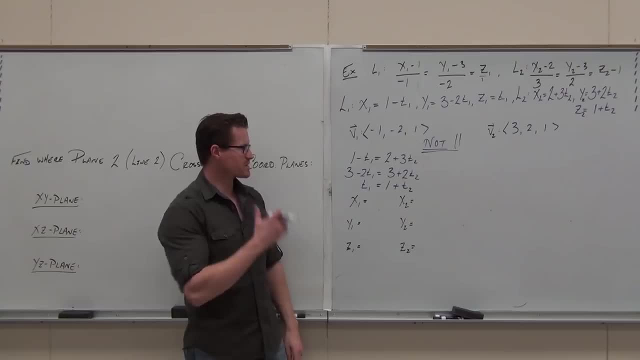 and Y and Z and it gives you a system. What's the best ones to pick? It doesn't really matter, You can pick any one, but I would pick those two again because that T1 is real nice. That's why I picked that. 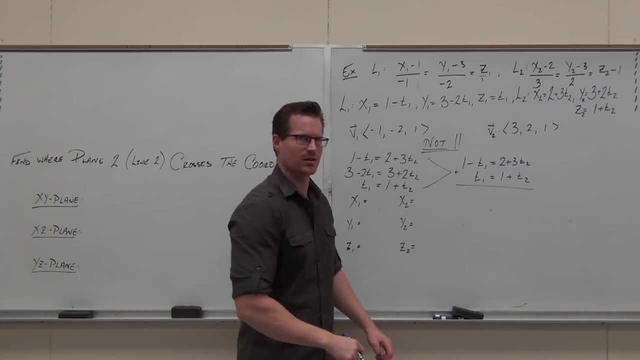 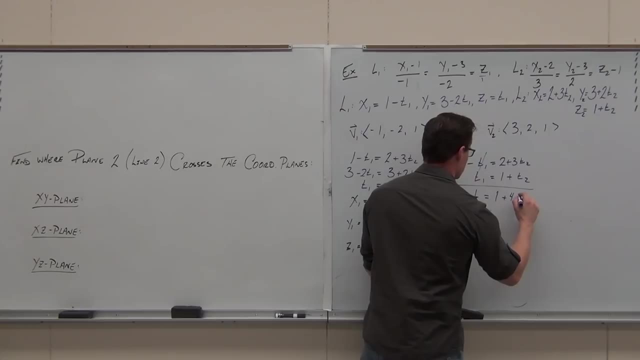 If I add these and get my signs correct, I'm going to be able to solve for T2, and that's going to be negative 1 and a half. So if I add them together, 1,, 0,, 4, T2, and that 3.. 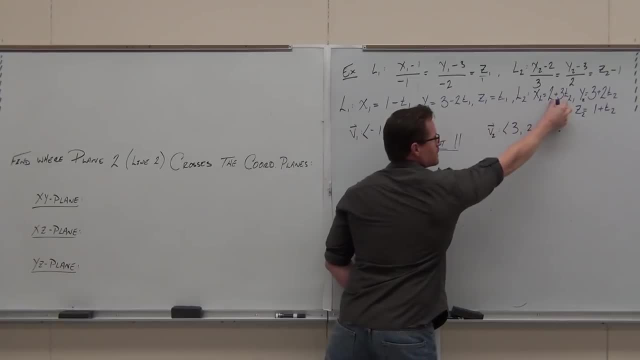 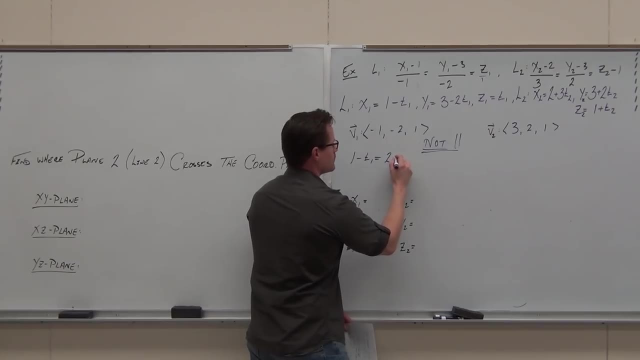 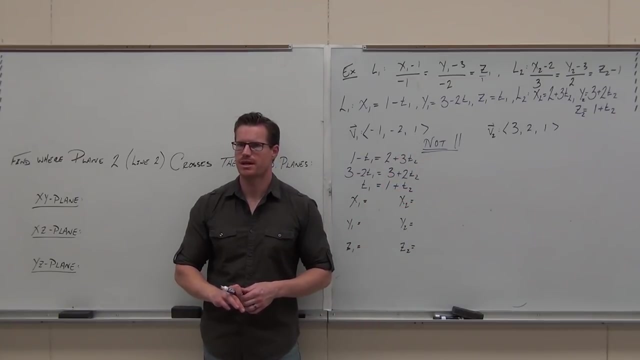 So we set these coordinates equal. If you can tell where I got these things from, I'll be very pleased. Can you tell where those things came from? Can you tell where these lines came from, So you can make it from symmetric to parametric? 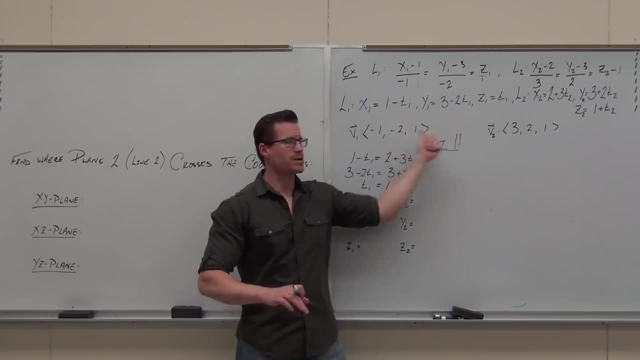 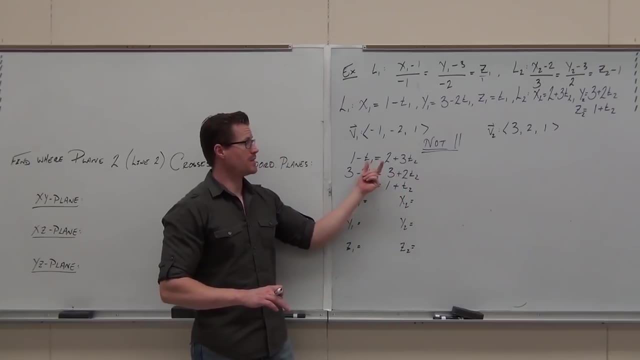 Sweet Back and forth. Can you make it from either one to the vectors, the direction vectors. Is it readily apparent that these are not parallel? Yes, Okay, Is it okay that we got these things equal? Do you see where those come from? 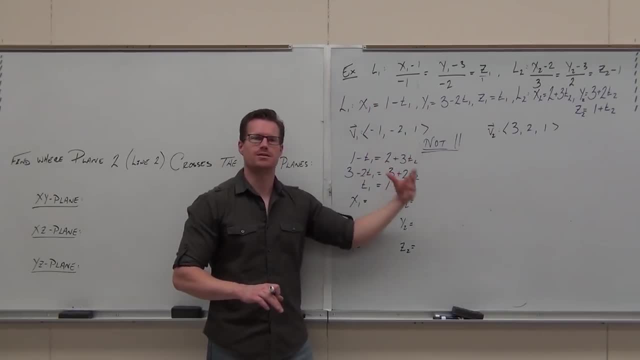 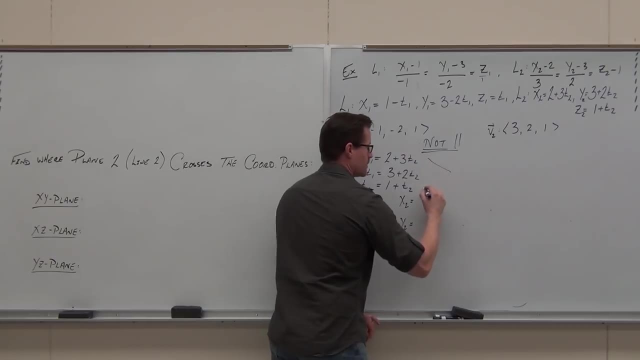 So once we have our line, X coordinates have to be equal, and Y and Z, and it gives parallel. It gives you a system. What's the best ones to pick? It doesn't really matter, You can pick any one, but I would pick those two again, because that T1 is real nice. 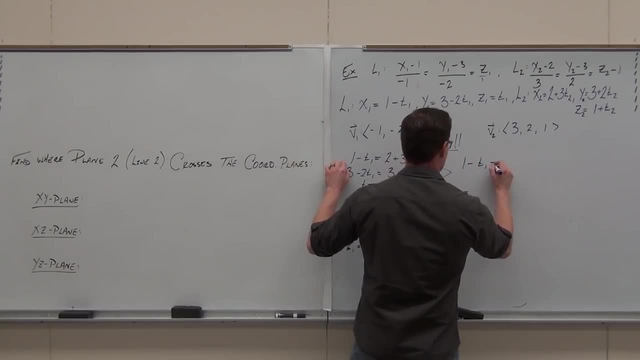 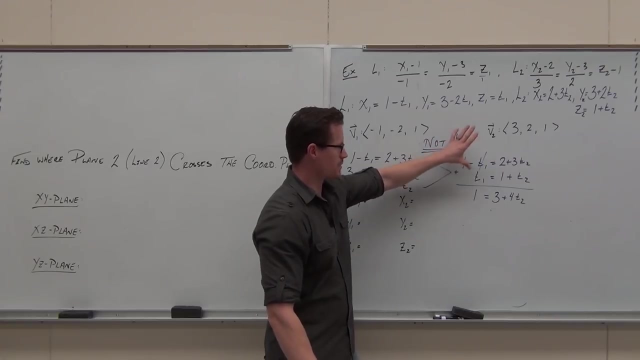 That's why I picked that If I add these and get my signs correct, I get a negative 1.5.. So if I add them together, 1, 0,, 4,, T2 and that 3.. You guys, all right with that one. 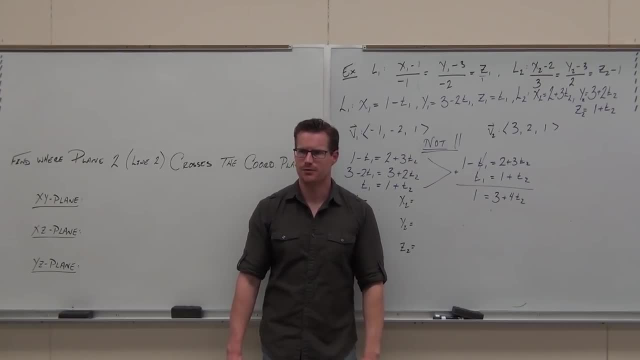 What am I going to get when I solve for T2?? Negative, Negative: 1.5. 1.5. 1.5. 1.5. 1.5. 1.5. 1.5.. 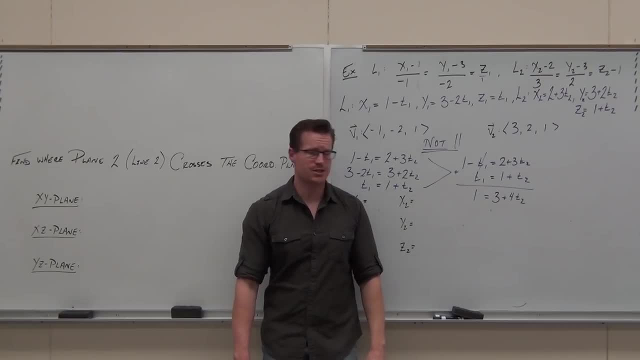 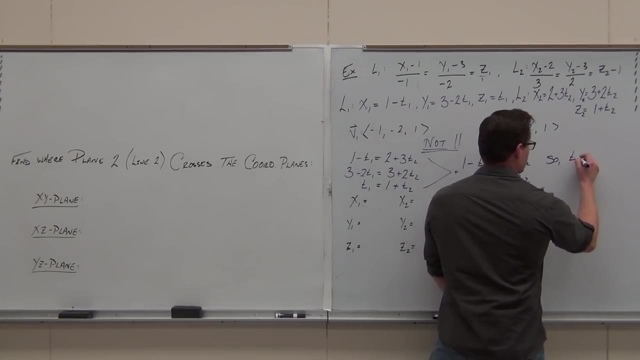 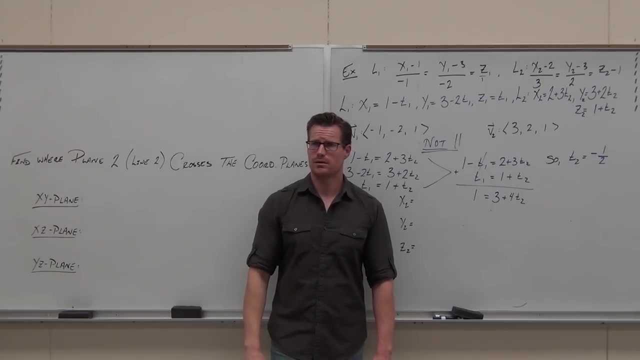 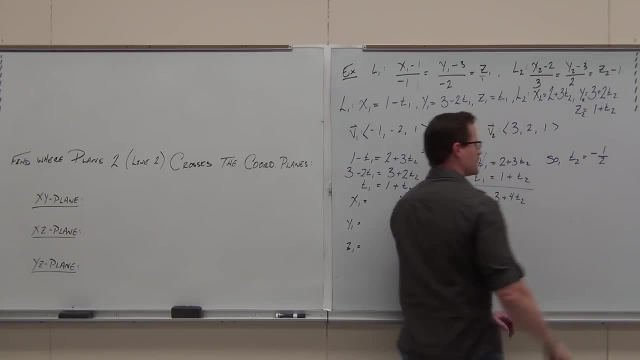 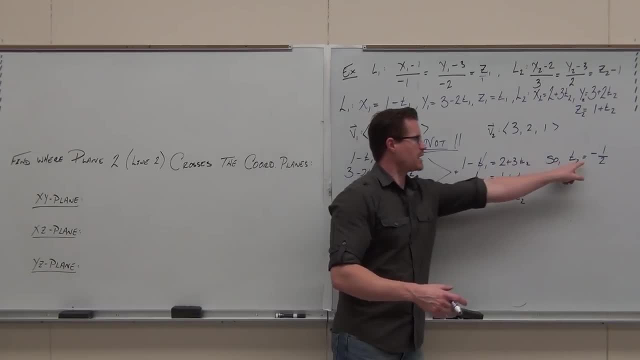 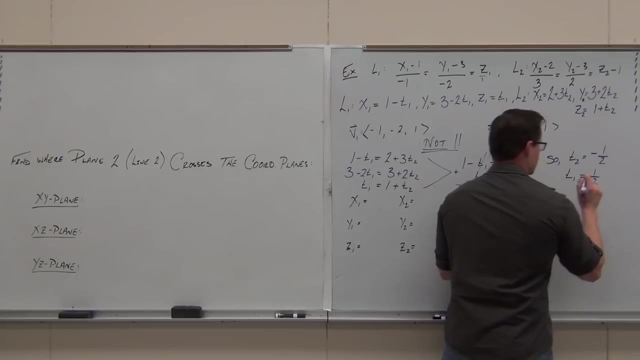 It doesn't. that's not what I'm asking. They're not going to be the same in general. If I plug in this here, 1 plus negative 1.5 is positive 1.5.. Okay, now, if you're out with that one, it's a lot of work. 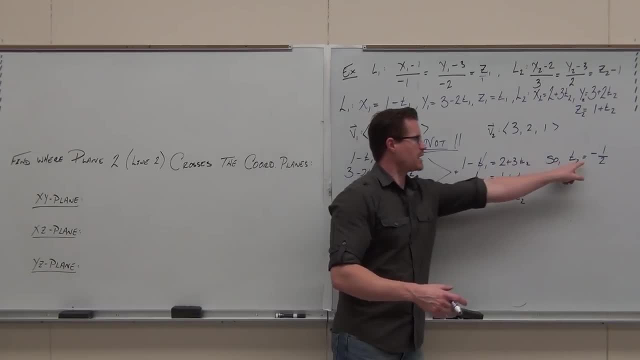 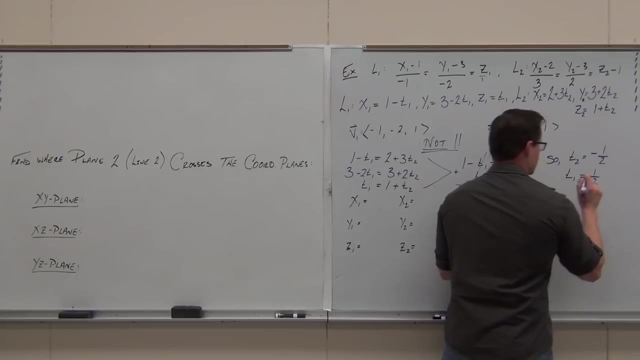 It doesn't. that's not what I'm asking. They're not going to be the same in general. If I plug in this here, 1 plus negative 1 and a half is positive 1 and a half. Okay, now, if you're out with that one, it's a lot of work. 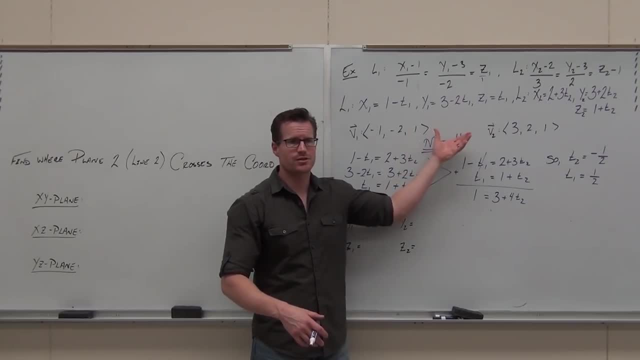 There's a lot of steps here. It starts with: hey, find vectors, See if they're parallel. If they aren't parallel, you've got to check intersection. Intersection is set all the x, y and z coordinates equal respectively. 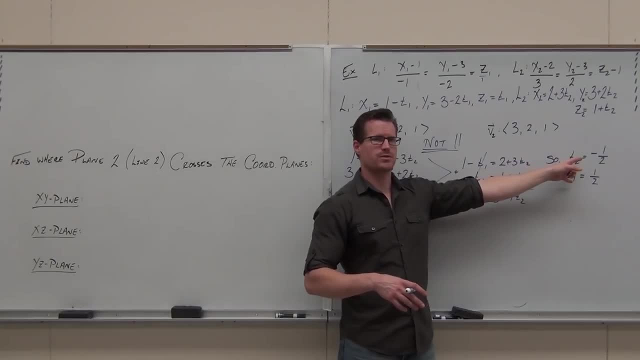 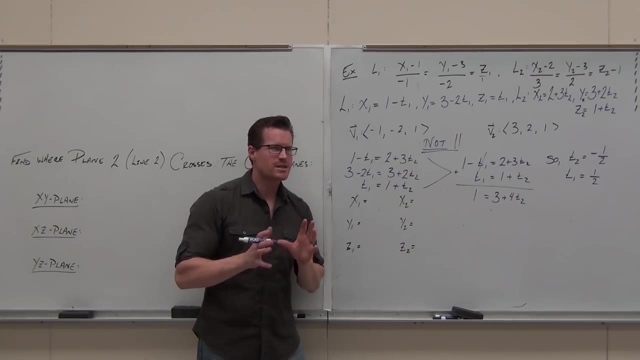 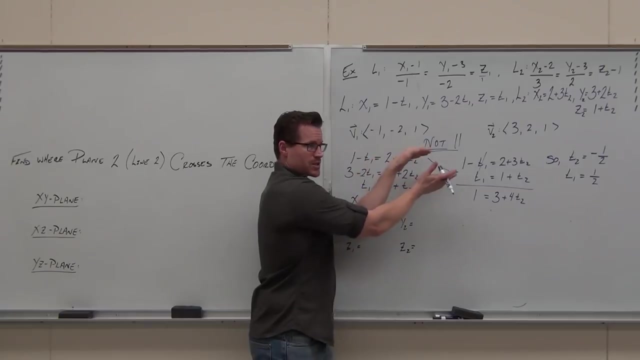 You've got to system, solve that system, and then take these values, plug them in on both sides and see what happens. What's the only one that could potentially not be equal- Top, middle, bottom- Because that's where we've got our system from- is the top and the bottom. 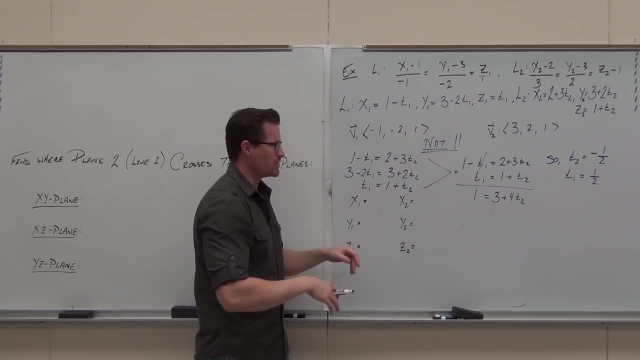 They're going to be the same. I guarantee it. Guarantee, I'll show you, though I'm going to give you the other way Baby sides. I erased it The other way, so setting them each independently equal. that seems easier for some people. 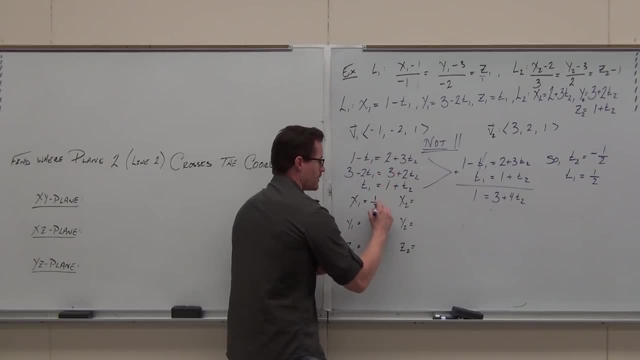 So if I take T1, plug it in here, I get 1 half. If I take T2, plug it in here, I also get, looks like, 1 half. Are they the same? Yes, They have to be. 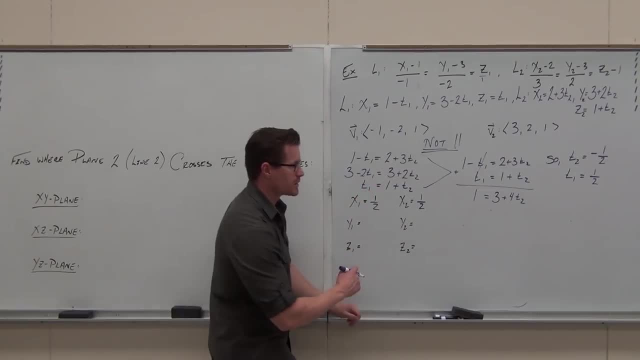 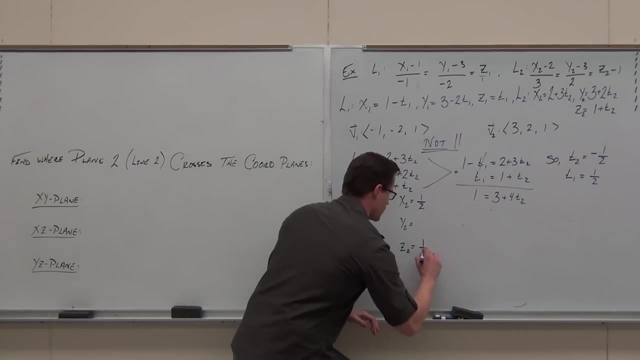 Let's do it down here. Take T1, put it here. Oh, let's see that's 1 half. Take T2, put it here. Looks like 1 half. Hey, they're the same. We already talked about that. 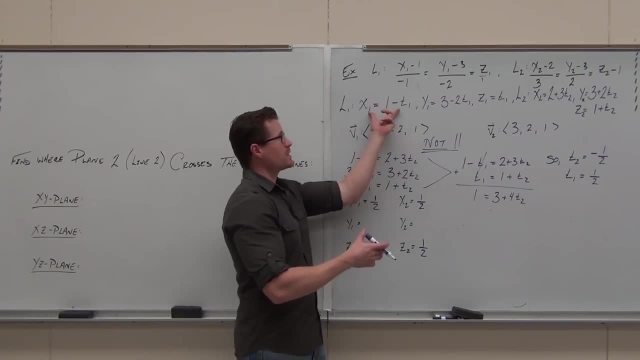 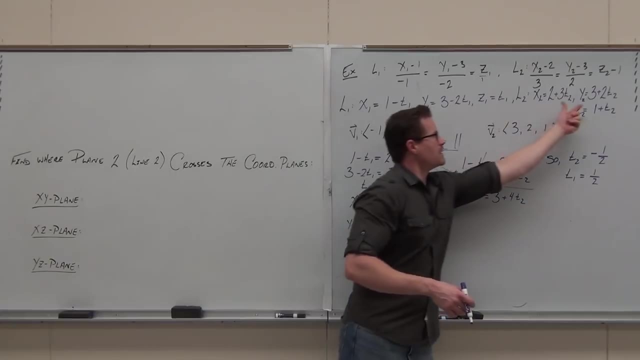 They are going to be the same And not. if you're okay with that one, You can even do it up here. It doesn't matter, They're the same. jump Now take these two and plug them in to the middle one, or plug them in here. 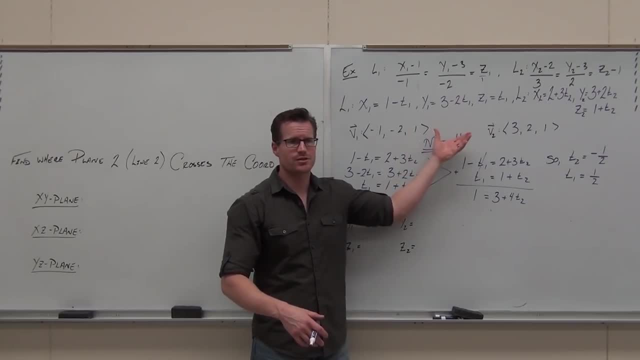 There's a lot of steps here. It starts with: hey, find vectors if they're parallel. If they aren't parallel, you've got to check intersection. Intersection is set. all the X, Y and Z coordinates equal respectively. You've got to system, solve that system and then take these values. 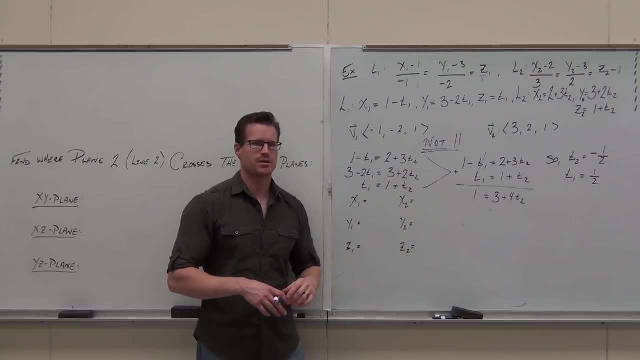 plug them in on both sides and see what happens. What's the only one that could potentially not be equal- Top, middle, bottom, Because that's where we've got our system from- is the top and the bottom. They're going to be the same, I guarantee it. 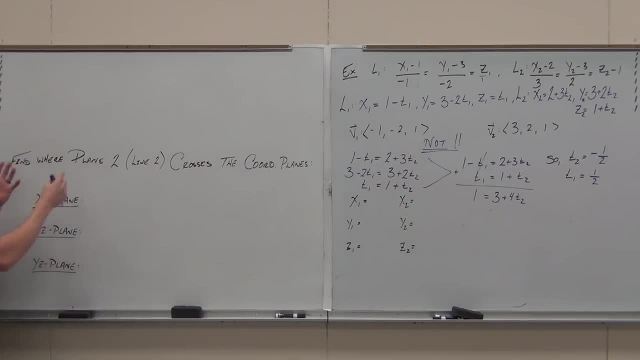 Guarantee I'll show you, though I'm going to give you the other way besides. all right, I erased it the other way. So setting them each independently equal, that seems easier for some people. So if I take T1, plug it in here, I get 1.5.. 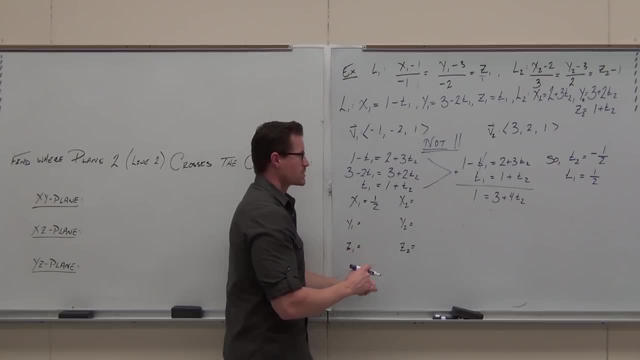 If I take T2, plug it in here, I also get looks like 1.5.. Are they the same? Yes, They have to be. Let's do it down here. Take T1, put it here. Oh, let's see, that's 1.5.. 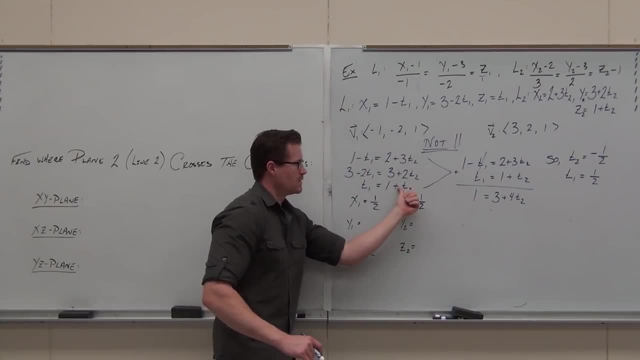 Take T2, put it here, It looks like 1.5.. Hey, they're the same. We already talked about that. They are going to be the same. I don't know. if you're okay with that one, You can even do it up here. 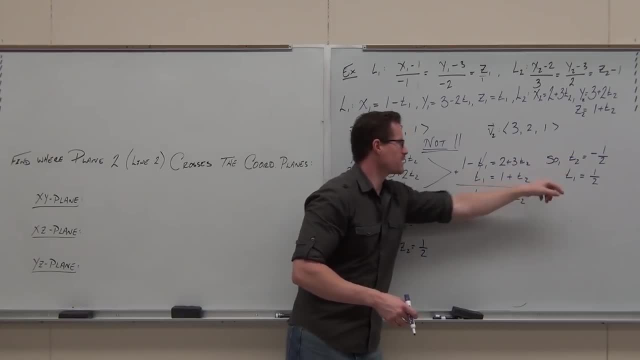 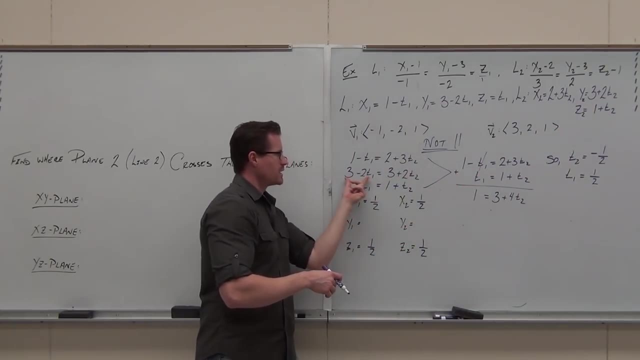 It doesn't matter, They're the same same jump. Now take these two and plug them in to the middle one, or plug them in here. That's where we got it from in the first place. Take T1, plug it in here. 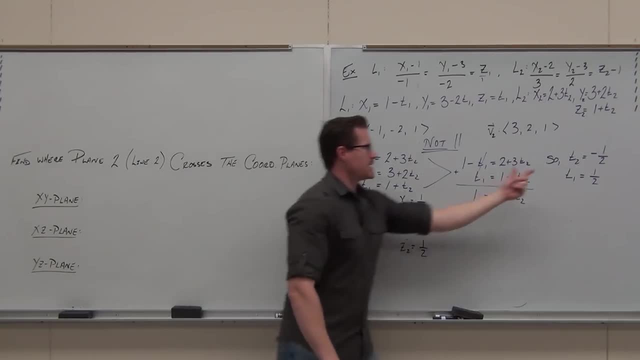 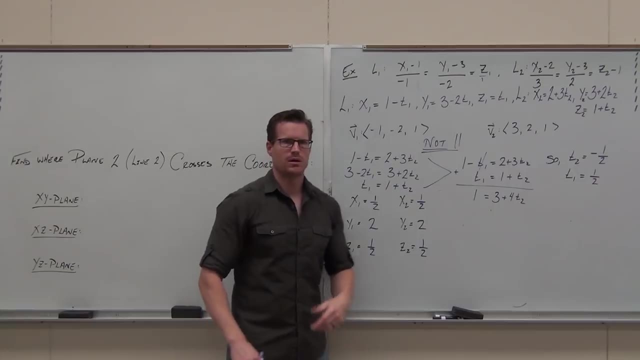 It looks like I'm going to get 2.. Take T2, plug it in here. Looks like I'm going to get O. Do the planes intersect? Yes, They do. Why? Good, Because when I have that time I get the same exact point. 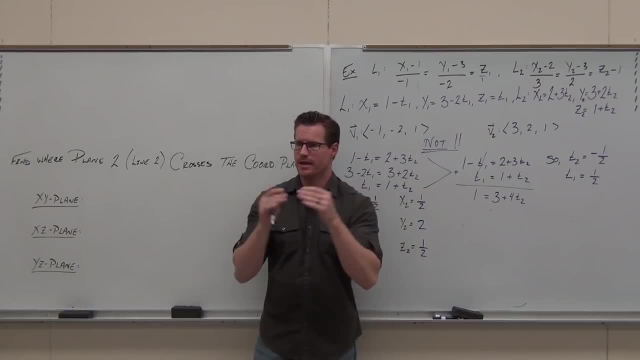 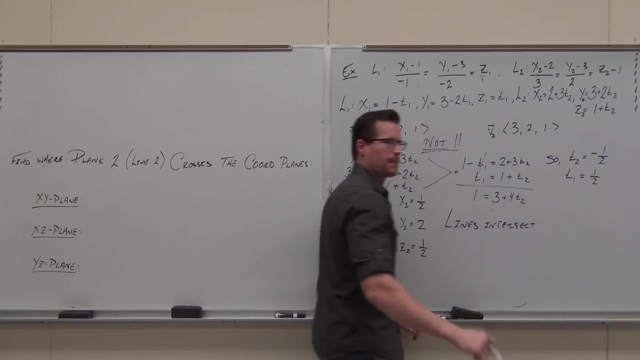 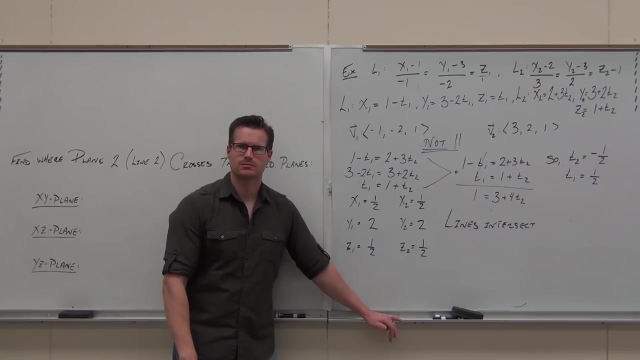 They're not off at any point, at any coordinate. They do intersect, They crash. That's a bad thing. I'm sure you understand the bad thing. So these lines intersect. At what point You found the point X1, X2, sorry, X1, Y1, Z1, or X2, Y2, Z2.. 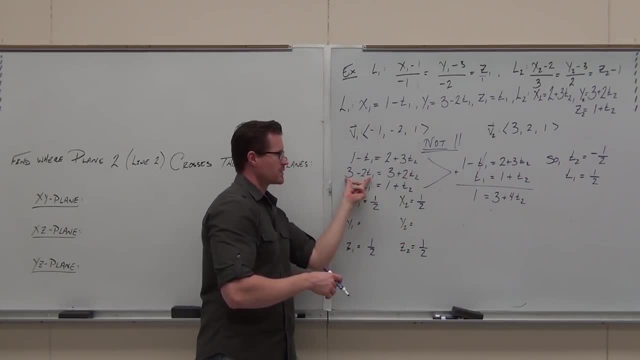 That's where we got it from in the first place. Take T1, plug it in here. Looks like I'm going to get 2.. Take T2, plug it in here. Looks like I'm going to get O. Do the planes intersect? 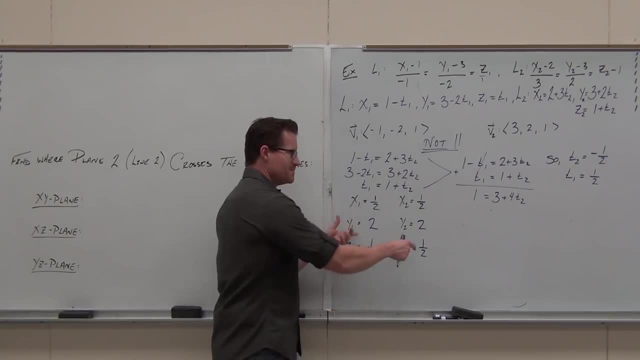 Yes, They do. Why? Because when I have that time, I get the same exact point. They're not off at any point, at any coordinate. They do intersect, They crash. That's a bad thing. I'm sure you understand the bad thing. 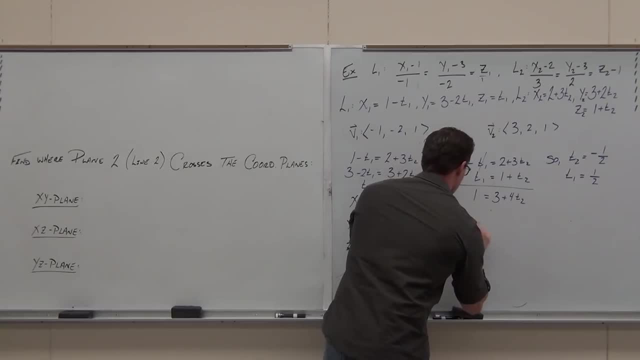 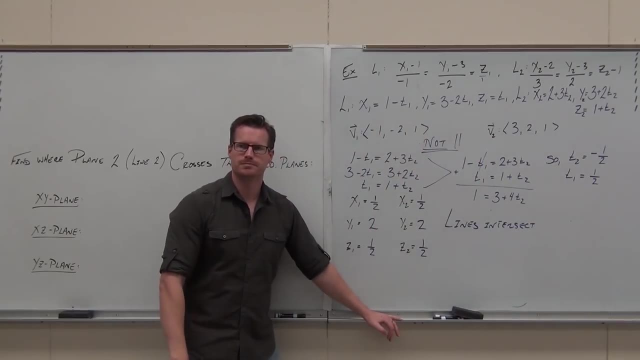 So these lines intersect. They intersect at what point? Find You found the point X1, X2, sorry, X1, Y1, Z1, or X2, Y2, Z2, this is the same thing. 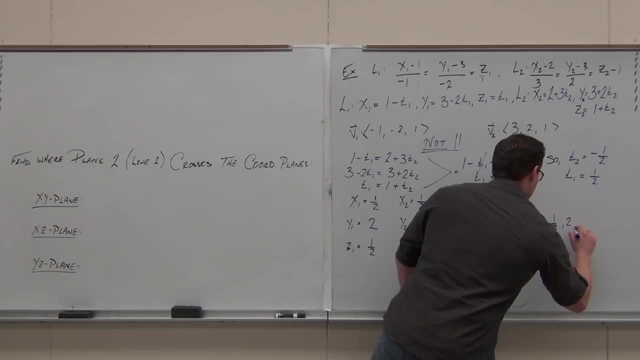 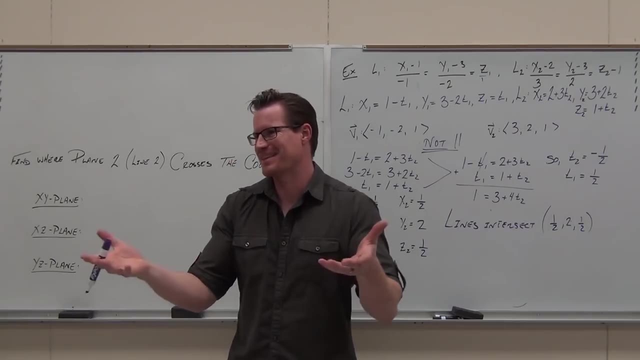 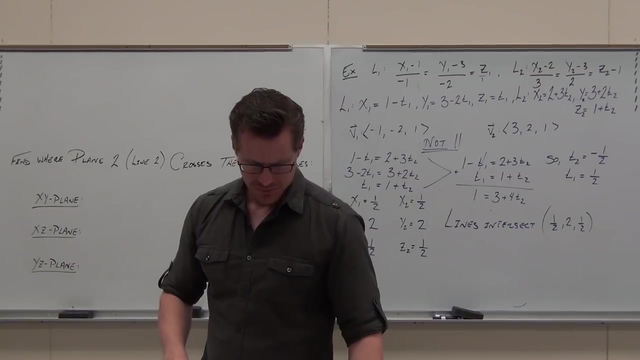 They intersect at the point that we just found. That's why we said they intersect. They intersect because it was at that point. It seems trivial, but you know, you need to understand that. Are you okay with it? Can you find the angle at which these planes will collide? 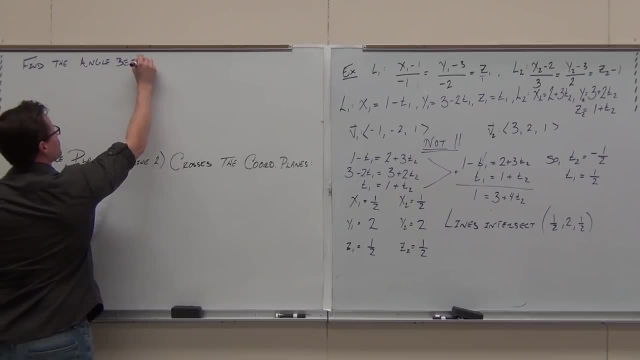 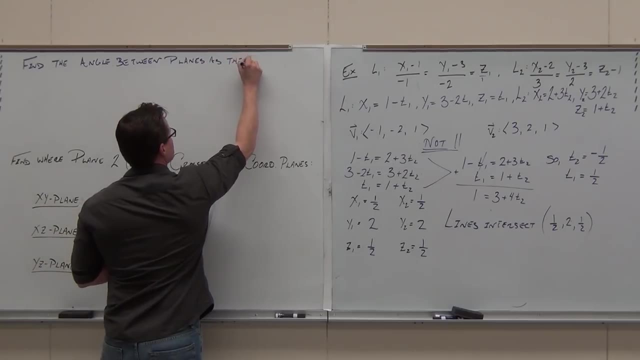 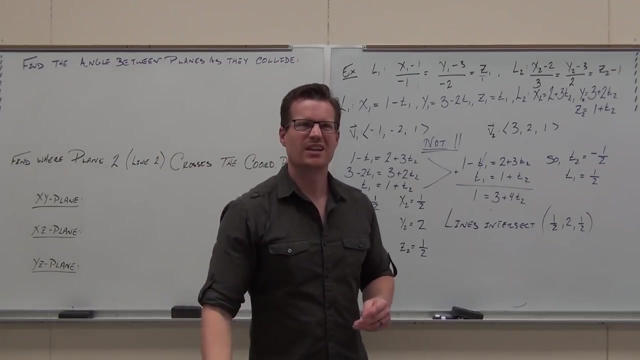 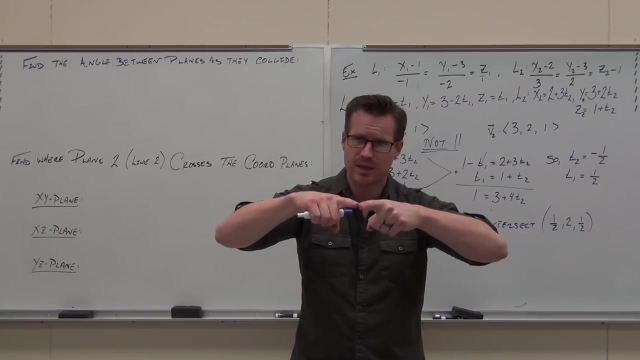 Well, you need a little note for that. How can we find that? Think about it. How can we find the angle between lines? Lines are given by their Direction, Direction vectors. How can we find the angle between two lines? Come on, put it together. 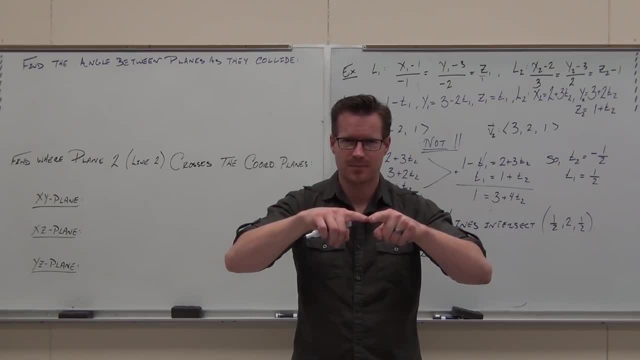 How can we find the angle between two lines? Do you use like the 1A cosine inverse or something or a line? Do lines have vectors? Do lines have vectors? Yes, Can you find the angle between two vectors? Yes, Are those vectors kind of like in the lines somewhere? 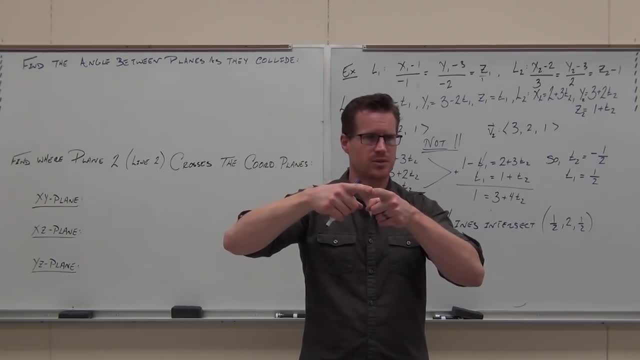 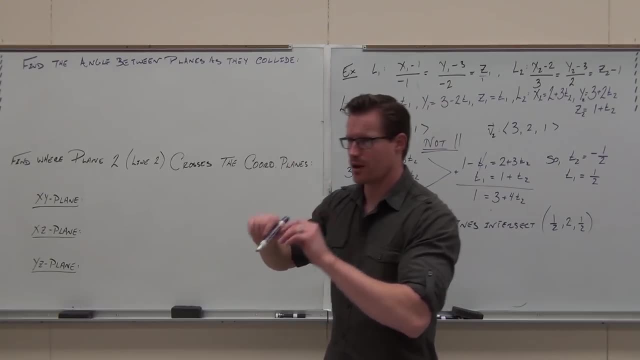 If you find the angle between the direction vectors, you will have found the angle between the lines. Does that make sense? So it's not hard. You've probably done it So in order to find the angle between the planes, which are the lines here. that's a horrible thing. 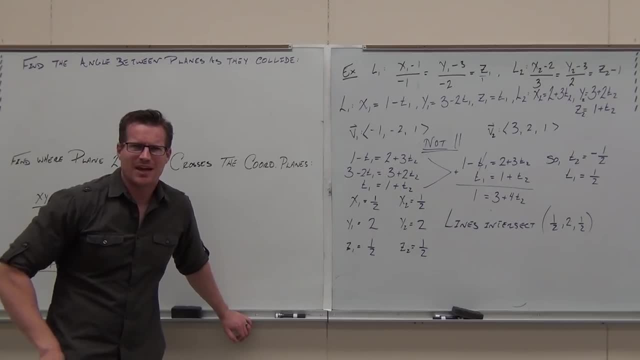 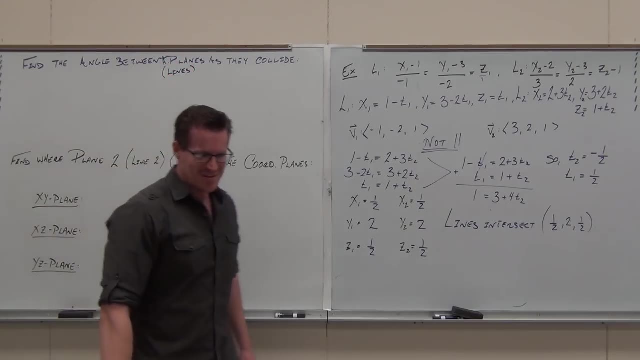 I shouldn't have done that to you, huh, Because we're going to be talking about planes in a little bit: Airplanes. Are you still going to go to the internet? That is not relevant right now. Probably not. I can't afford it. 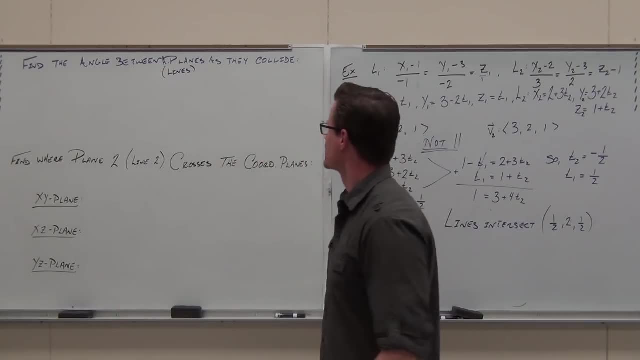 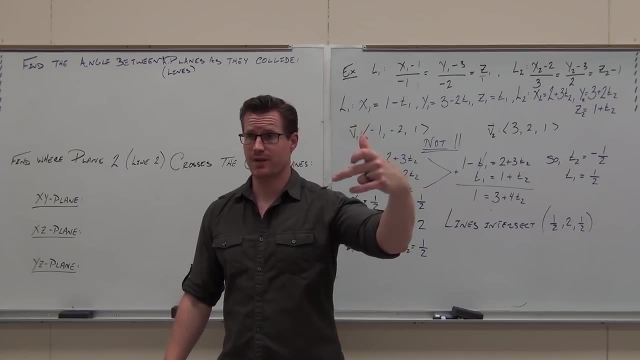 It's too expensive- Find the angle between the airplanes, the lines as they collide. The angle between the lines is the same as the angle between the vectors. So if you can find the angle between vectors, you can find the angle between the lines. 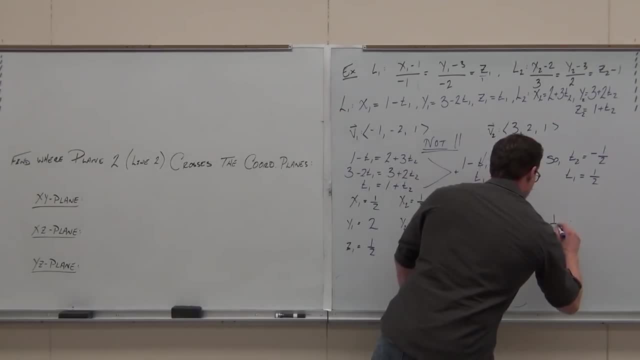 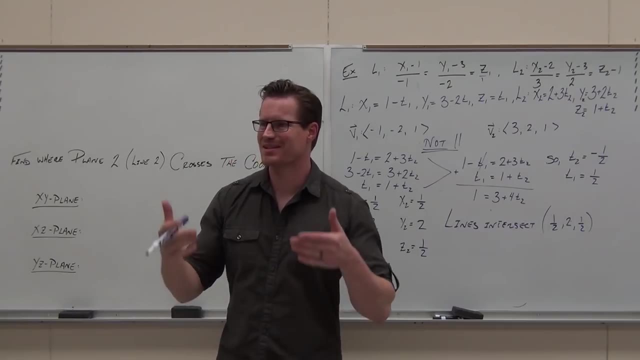 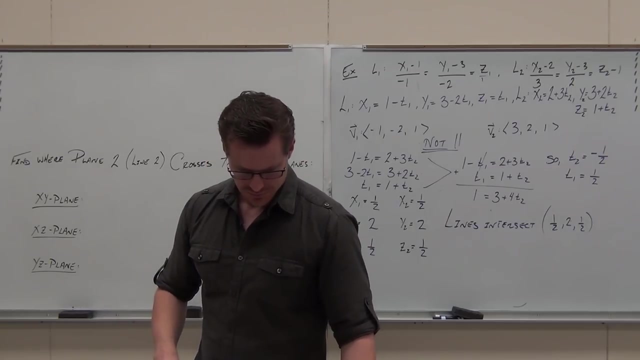 This is the same thing. They intersect at the point that we just found. That's why we said they intersect, Because it was at the point. It's at that point. It seems trivial, but you need to understand that. Are you okay with it? 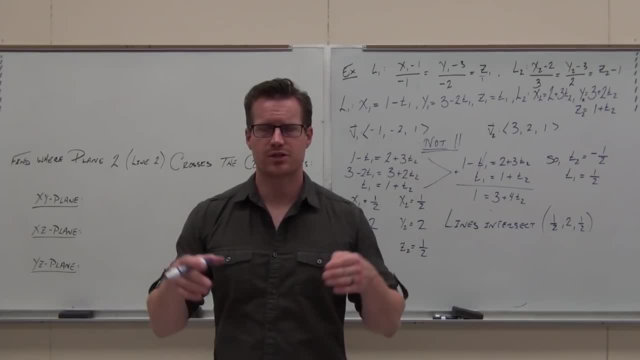 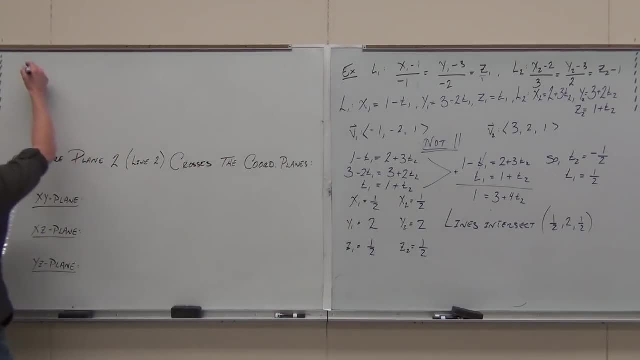 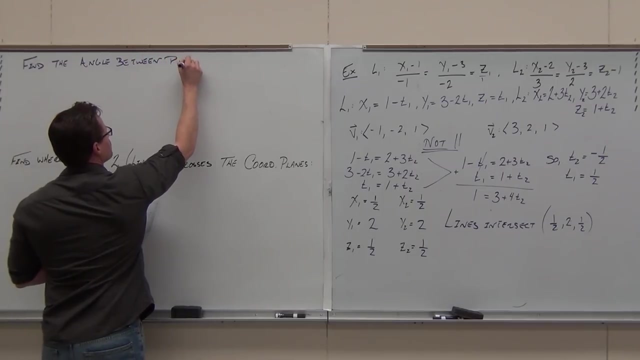 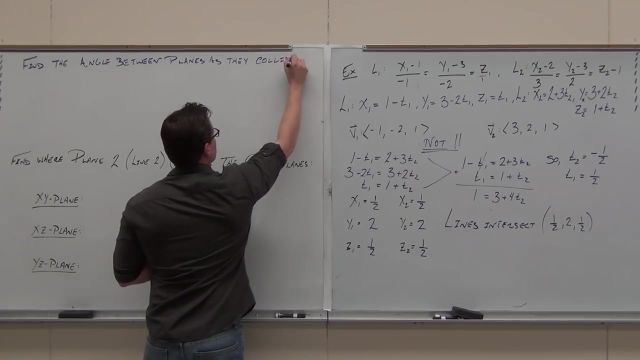 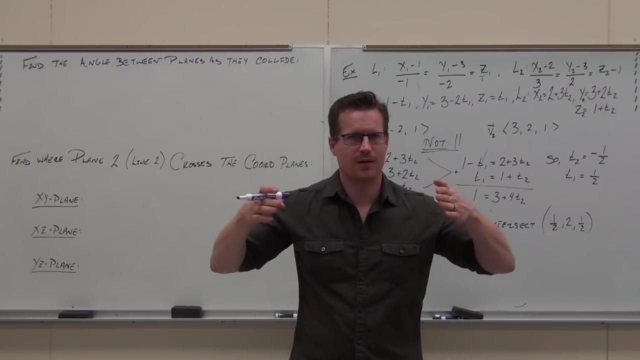 Can you find the angle at which these planes will collide? Well, you need a little note for that. Think about it. How can we find the angle between lines? Lines are given by their Direction Direction vectors. How can we find the angle between two lines? 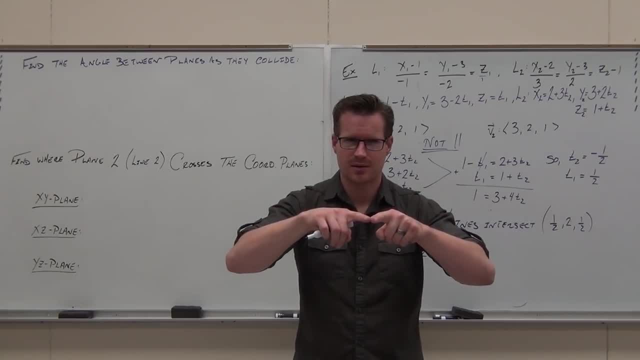 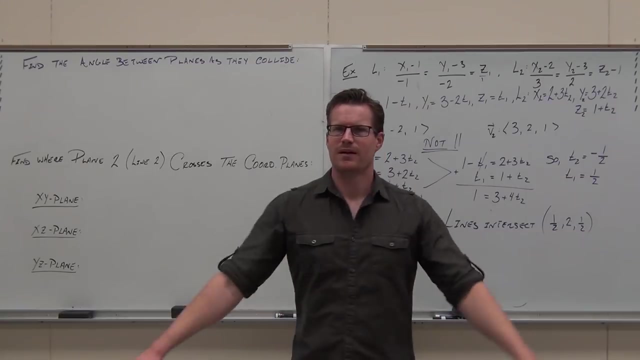 Come on, put it together. How can we find the angle between two lines? Do you use the 180 cosine inverse? Do lines have vectors? Do lines have vectors? Yes, Can you find the angle between two vectors? Yes, Are those vectors kind of like in the lines somewhere? 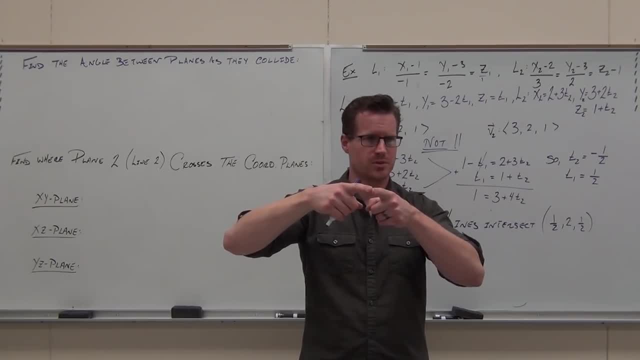 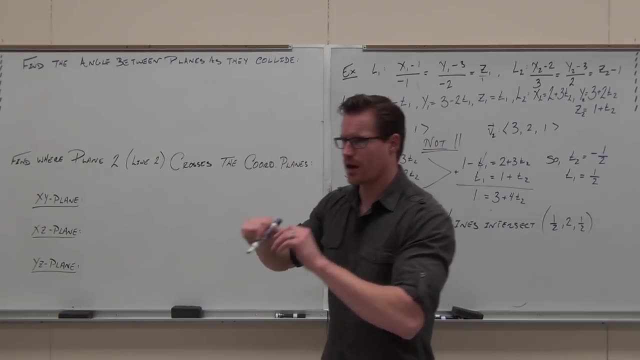 If you find the angle between the direction vectors, you will have found the angle between the lines. So it's not hard, You've probably done it. So, in order to find the angle between the planes, which are the lines here, that's a. 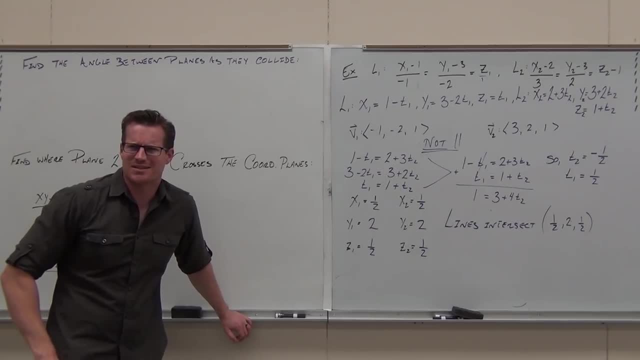 horrible thing. I shouldn't have done that to you, huh, Because we're going to be talking about planes in a little bit: Airplanes. Are you still going to go to the internet? That is not relevant right now, Probably not. 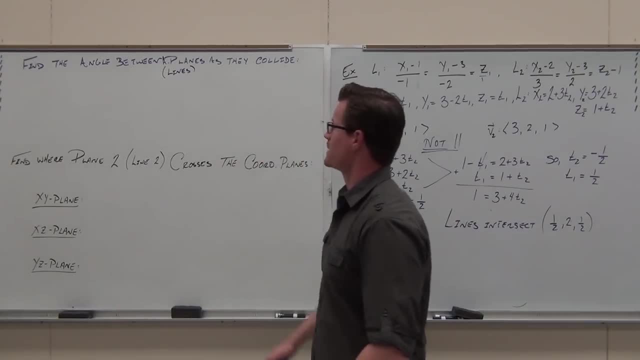 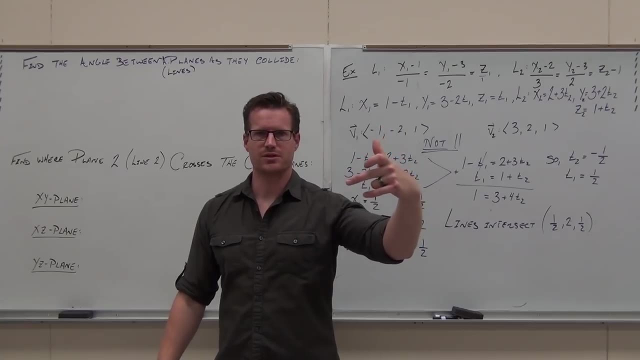 I can't afford it. It's too expensive. Find the angle between the airplanes, the lines as they collide. The angle between the lines is the same as the angle between the vectors. So if you can find the angle between the vectors, you can find the angle between the lines. 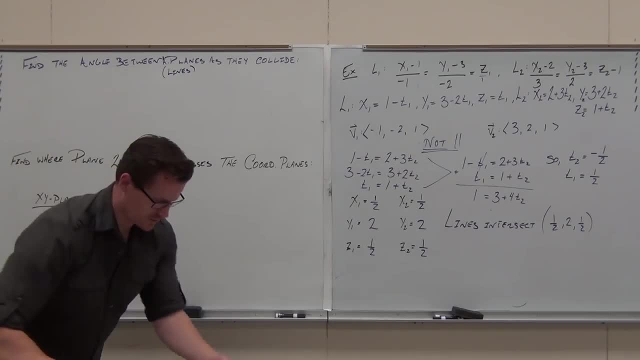 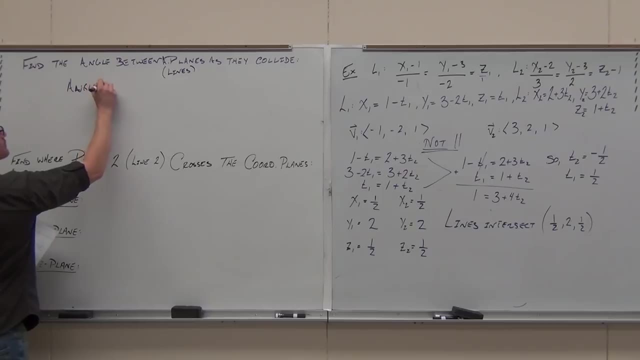 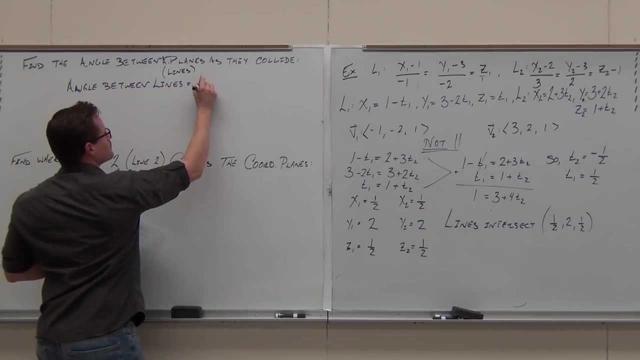 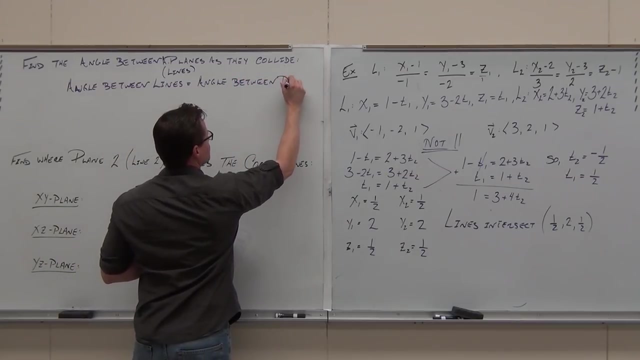 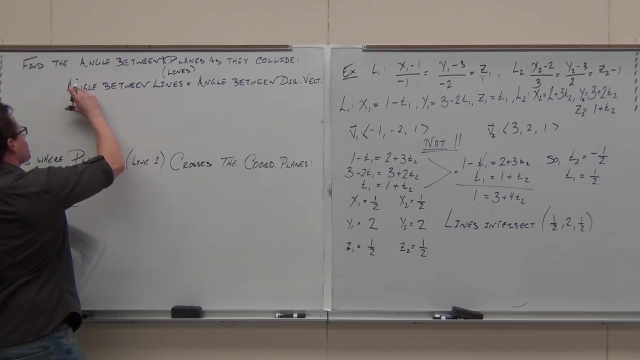 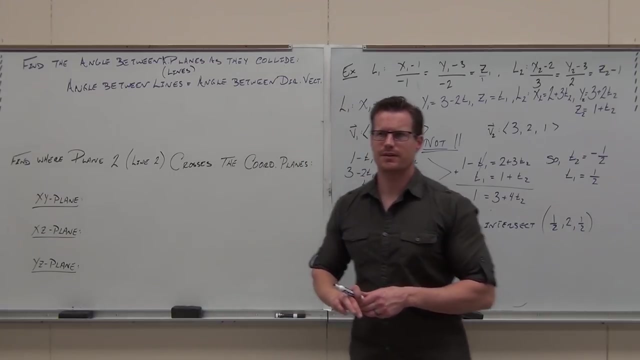 Do I have it written down better than this? Yeah, Okay, Great, Okay, Great. How many of you right now, given that these lines? well, let's see, can you tell me the vectors that give us the direction of these lines? 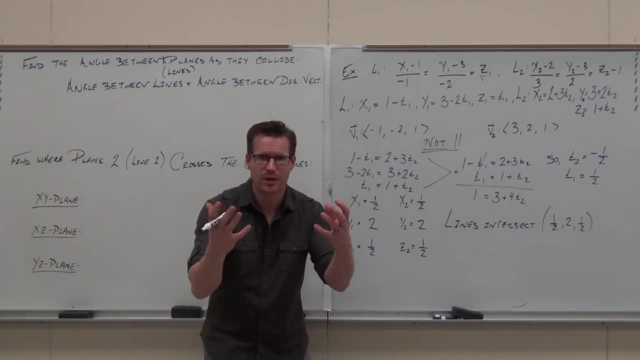 Can you tell me the vectors Specifically? come on quickly. what's one vector? The angle? Can you tell me the other vector? Can you find the angle between those two vectors? Yes, Then you will have found the angle between these two lines as they intersect. 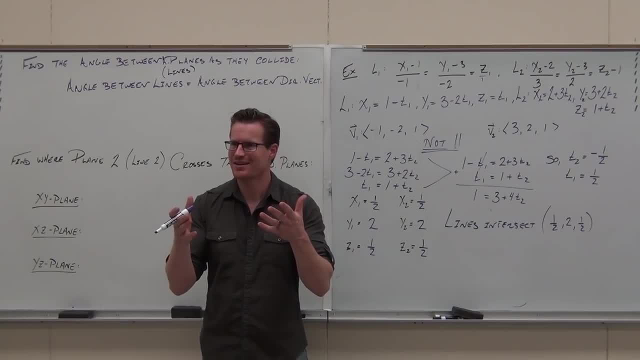 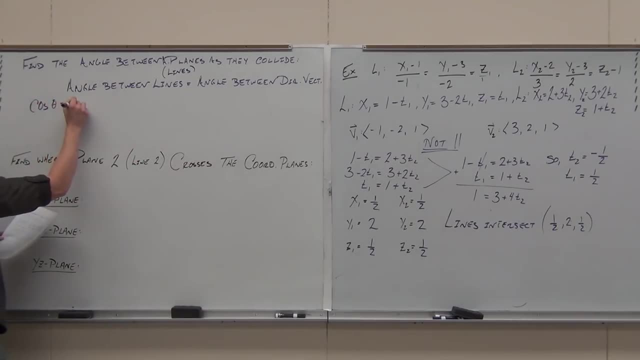 Let's go: oh, what does that for you? Do you remember the formula? Do you know how to do that? The vector or the angle between any of the lines is given by this. So for us, specifically, we go: okay, well, let's do this. 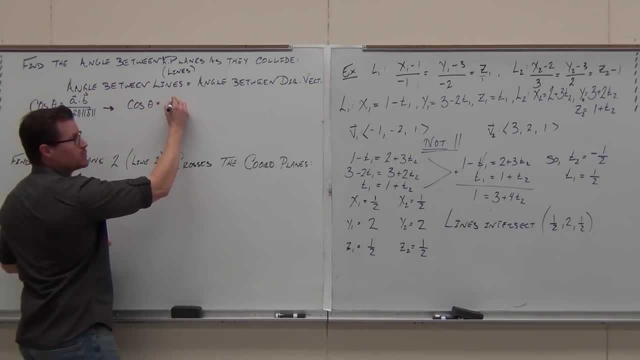 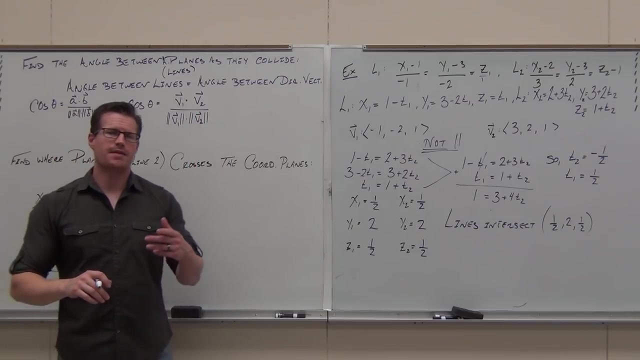 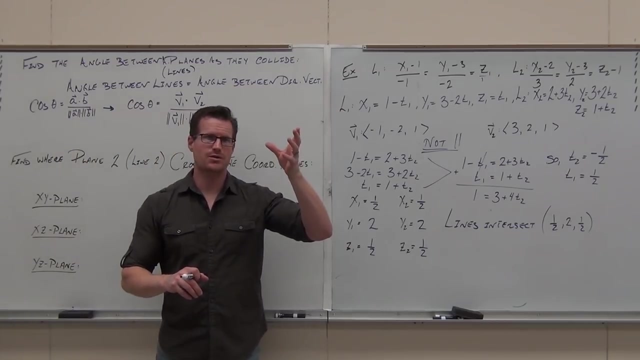 Let's take V1, dot with V2.. We go T1, dot with V2.. What we do is we're going to divide the F by F prime. So that's a zero and it's going to be zero. 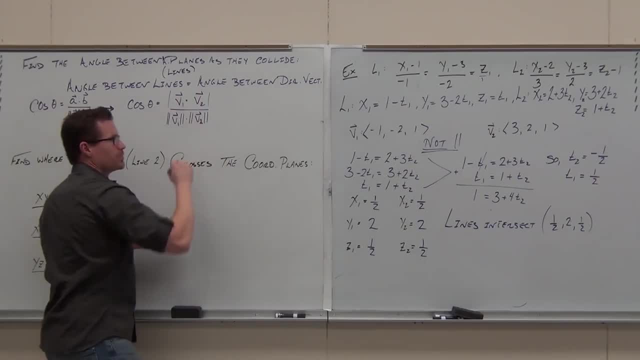 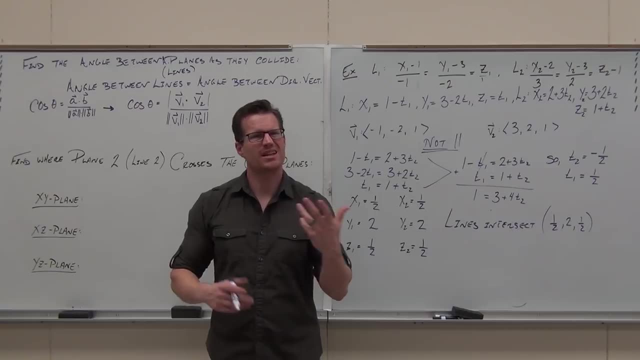 minus one 3.. Now I'm going to go ahead and do a little math here to see what's going on here. I'm going to divide by the magnitude and then I'm going to put one more thing up here so you don't get confused, please listen. 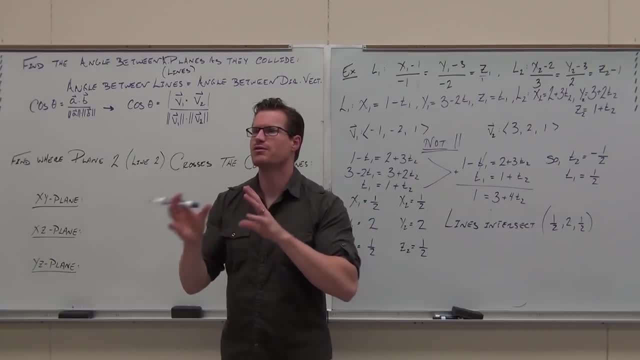 Let's do that. Let's keep it an acute angle. That way we don't get two different answers. Does that make sense to you? We're going to keep it acute. It's a cute little angle, Anyway. so do it. 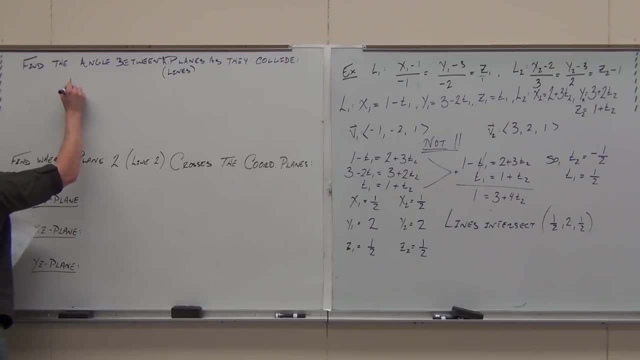 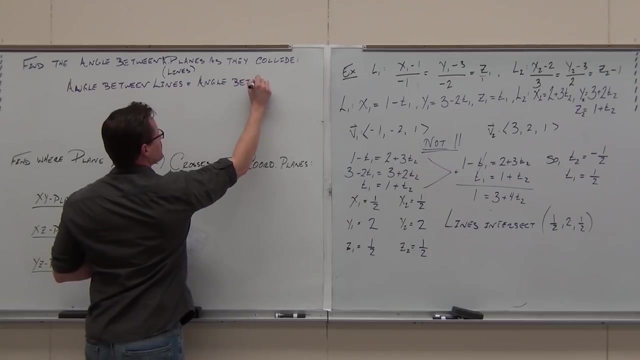 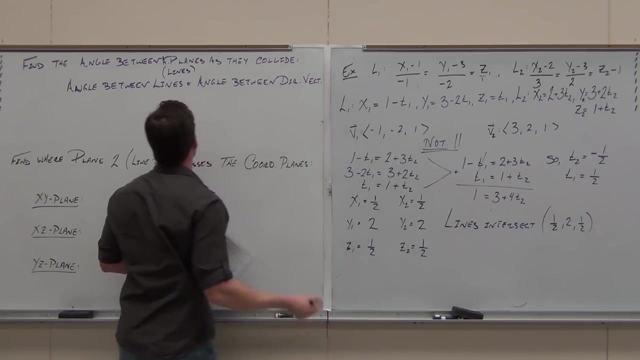 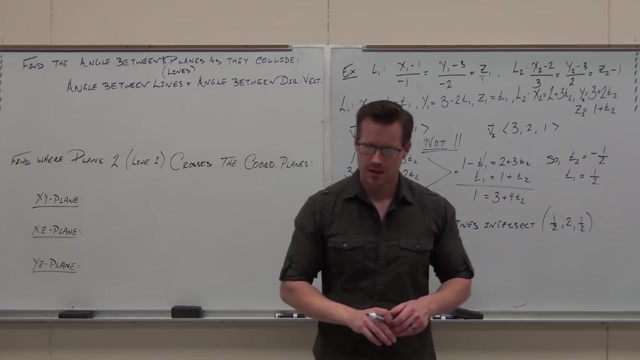 Have it written down better than you should, Bill. Thank you so much. Thank you. Does it work? It does. You're welcome. that's great, Thank you. Thank you. How many of you right now, given that these lines well, 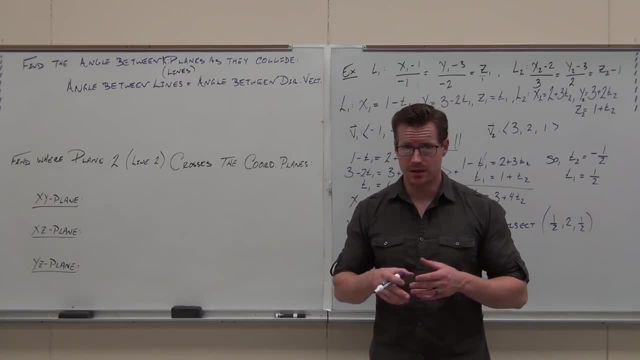 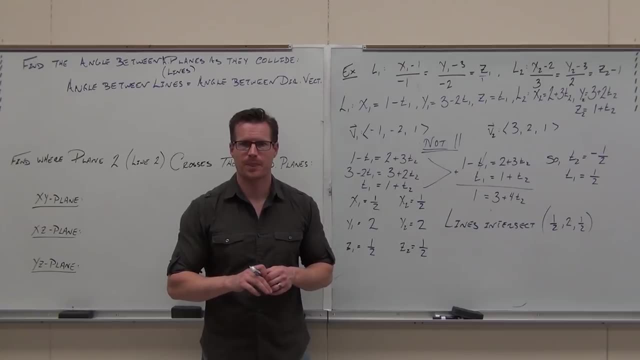 let's see. can you tell me the vectors that give us the direction of these lines? Can you tell me the vectors Specifically? come on quickly. what's one vector, The other one? Can you tell me the other vector, The other one? 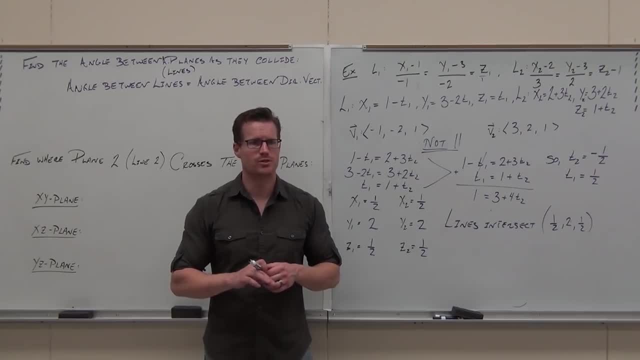 Can you find the angle between those two vectors? Yes, Then you will have found the angle between these two lines as they intersect. Let's go. oh, what does that for you? Do you remember the formula? Do you know how to do that? 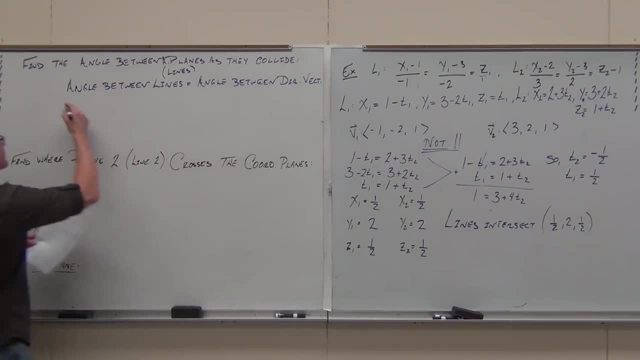 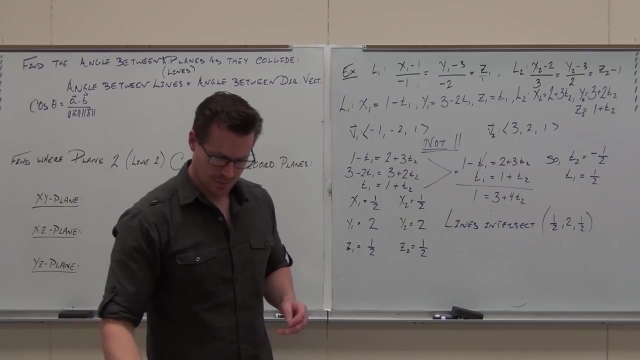 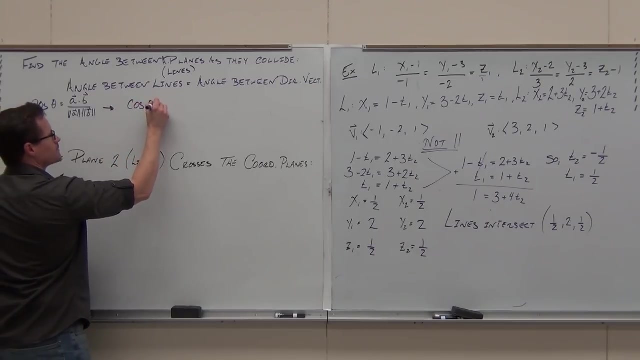 The vector or the angle between any of the lines is given by this. So for us specifically, we go: okay, well, let's do this. Let's take V1,, dot with V2, divide by their magnitudes, and then I'm going to put one more thing up here. 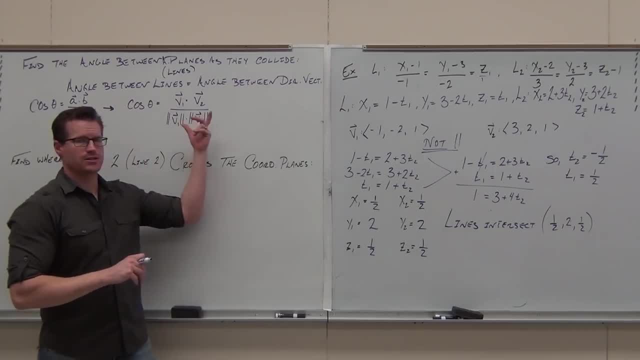 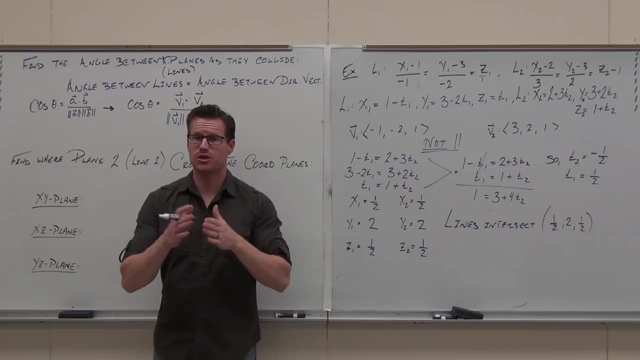 so you don't get confused, please listen. This right here has the chance to give us either an acute angle or an obtuse angle. If you always want to make this the acute angle, put an absolute value there around that scalar, because dot product gives you a scalar. 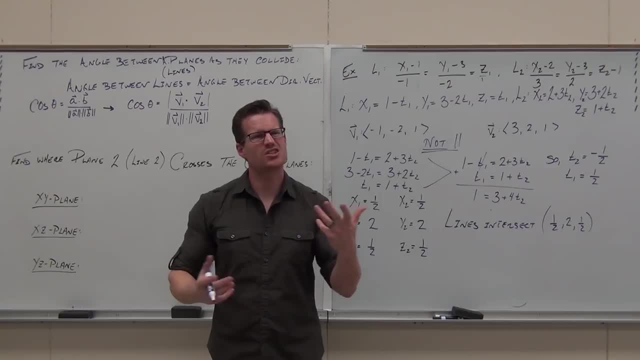 and that will always give you the acute angle between your lines. Let's do that. Let's keep it an acute angle. That way we don't get two different answers. Does that make sense to you? We're going to keep it acute. 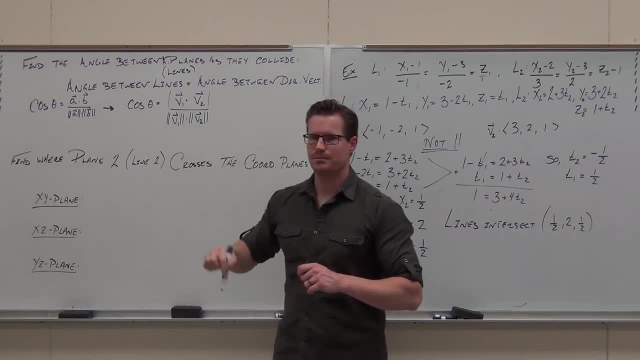 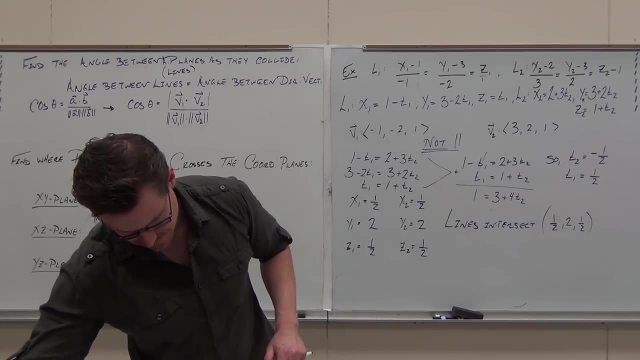 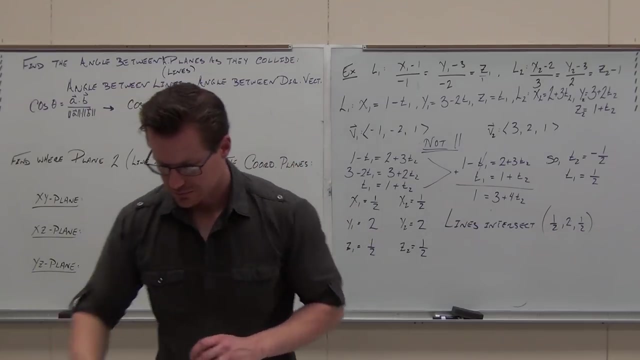 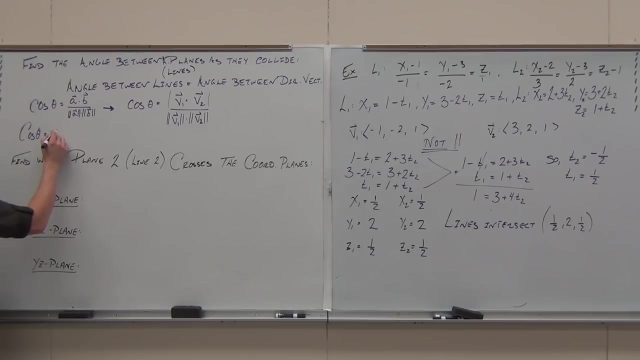 It's a cute little angle Anyway, so do it, Go for it. Find me the angle between those two direction vectors. Find me the angle between the lines. what I'm asking you: Do you remember how to do a dot product? 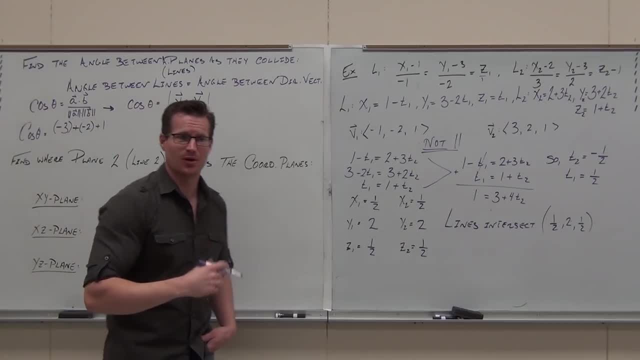 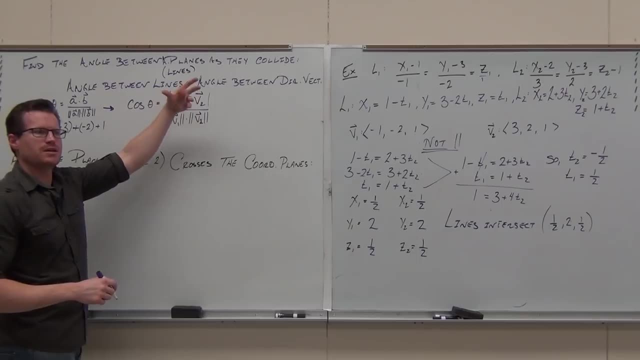 Do you remember that at all? Yeah, I hope that you do. We've done a lot since then, but hopefully you do. Take the components, Multiply them, Add them Here. also, take an absolute value so you get the acute angle. 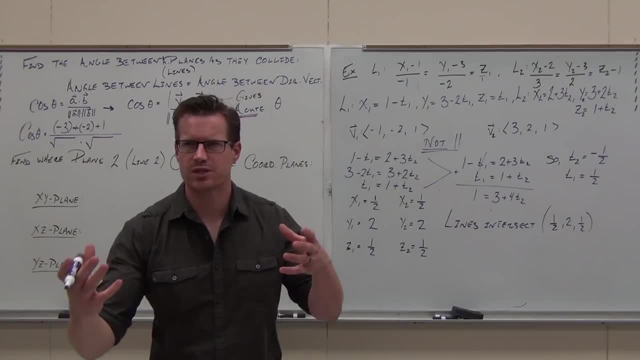 Do you remember how to find a magnitude? I know it's got square root. Explain to me in your own words how to find a magnitude of a vector. Come on quickly. What do you do? Square them, Add them. What's the square root of a vector? 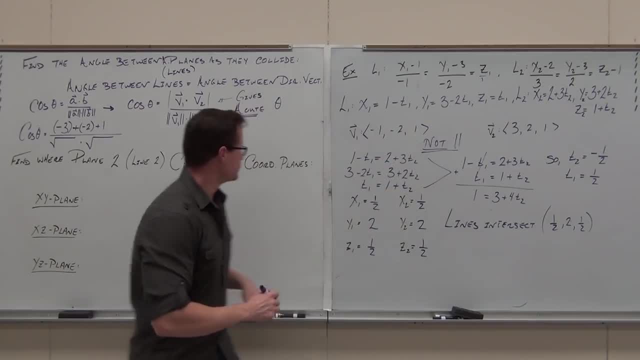 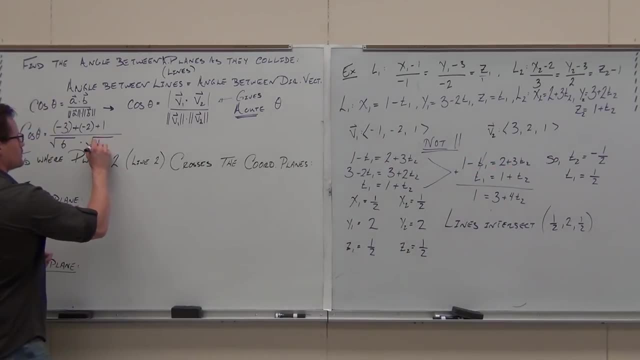 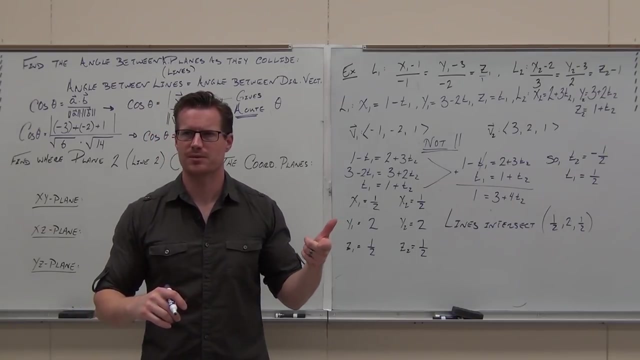 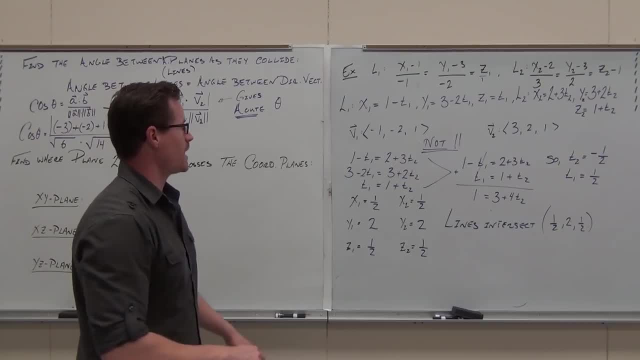 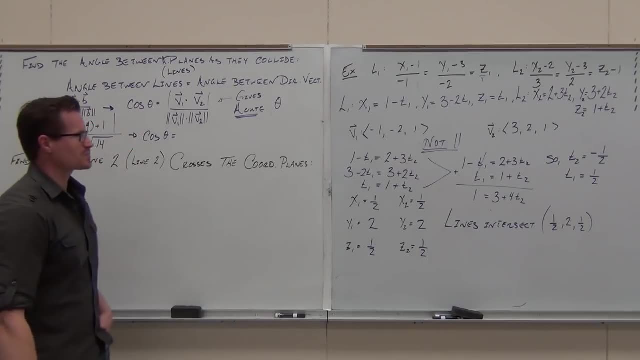 1, 4, 1.. Oh Snap, I made a mistake. Negative 4? I just saw that. I was like: wait a minute, That doesn't look right. Negative 4.. Better checking the work again. 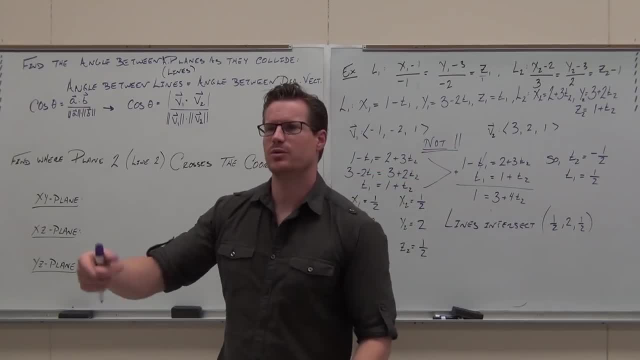 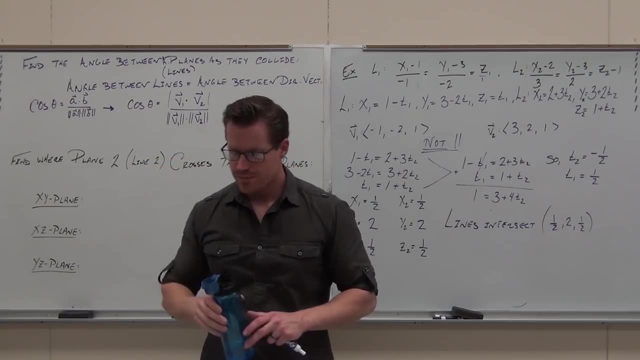 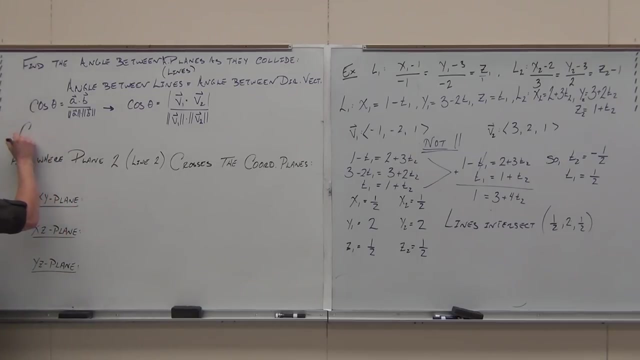 Find me the angle between those two direction vectors. Find me the angle between the lines. what I'm asking you, Man, do you remember how to do a dot product? Do you remember that at all? Yeah, I hope that you do. 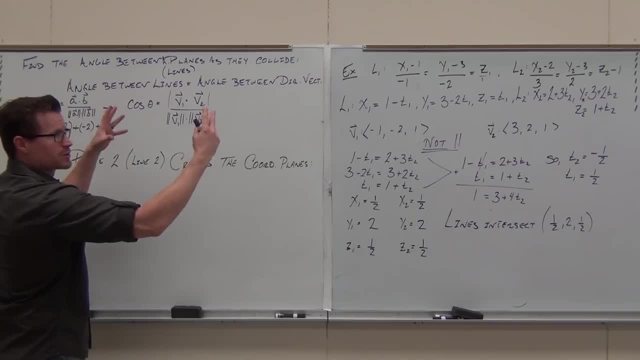 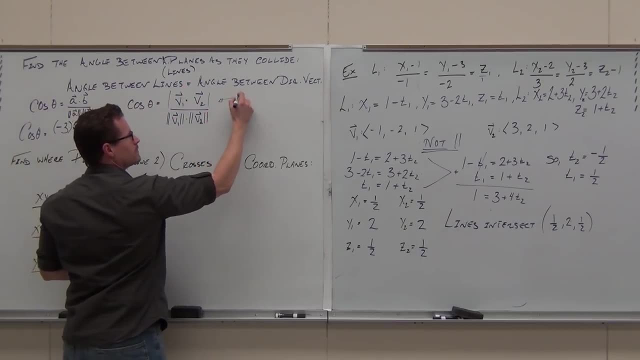 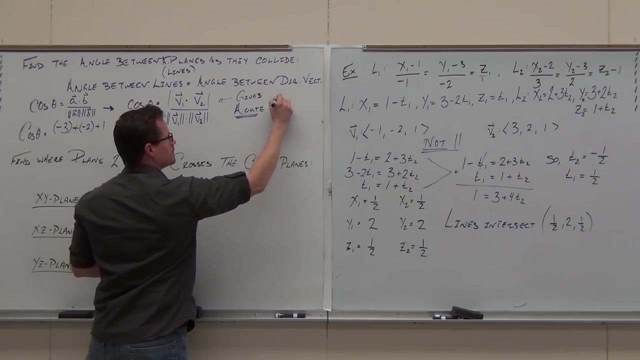 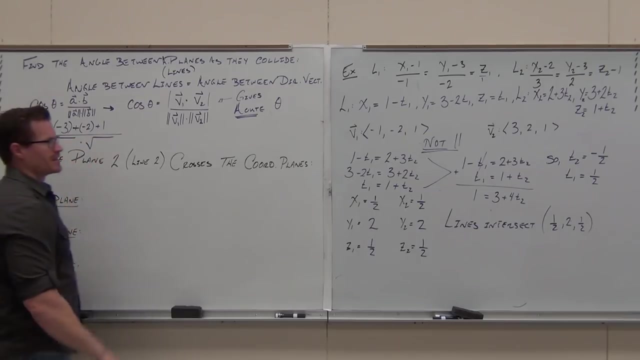 We've done a lot since then, but hopefully you do. Take the components, multiply them, add them Here. also, take an absolute value so you get the acute angle. Do you remember how to find a magnitude? I know it's got square root. 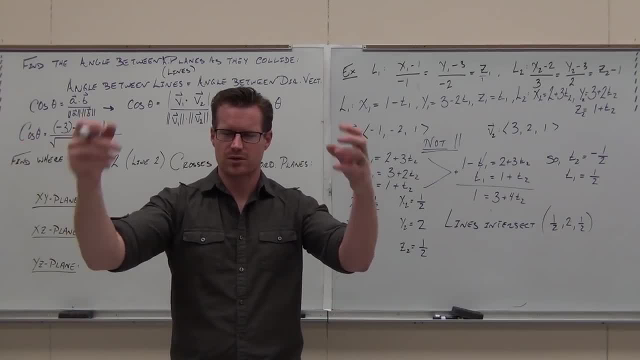 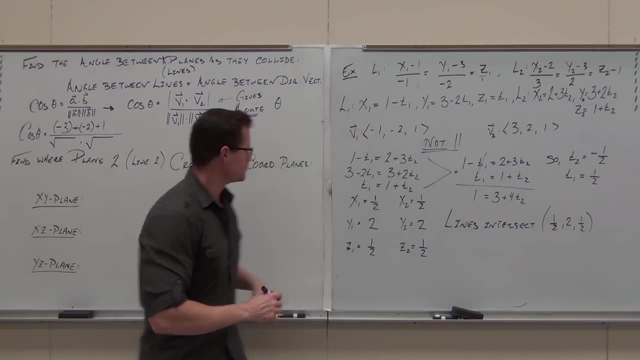 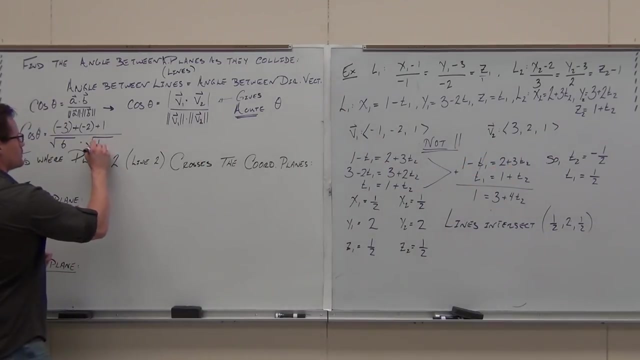 Explain to me in your own words how to find a magnitude of a vector. Come on quickly. What do you do? Square them, Add them One, four, one, Nine, Nine, four, one. Oh, what did you get on that one? 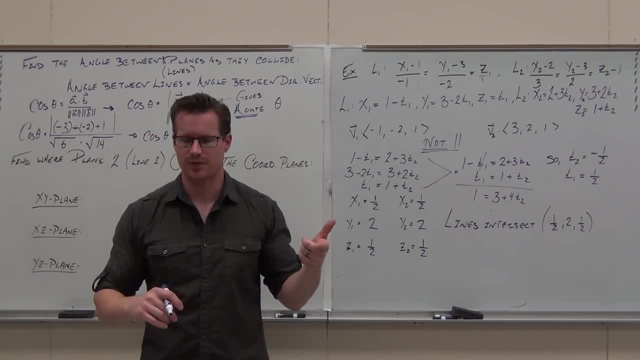 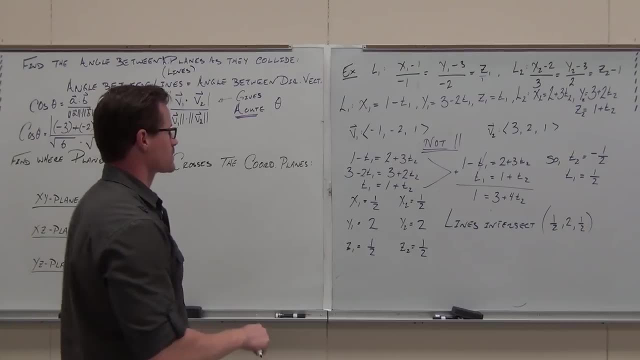 So it's negative three, negative two. that's negative five. that's one negative four. but absolute value. Hopefully we're getting. oh snap, I made a mistake. I just saw that. I was like wait a minute, that doesn't look right. 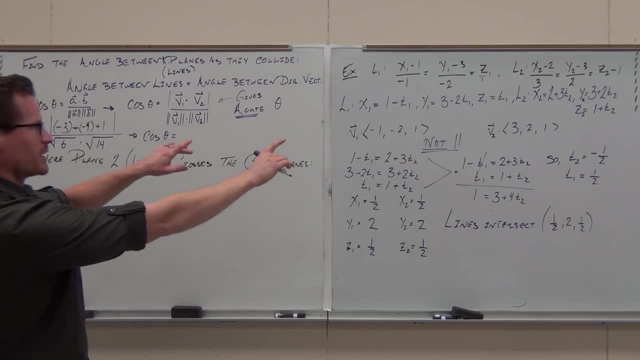 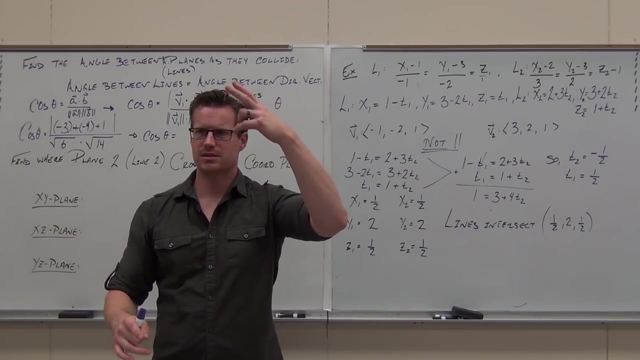 Negative four- Better check my work again- Negative three, negative one, sorry, positive three. negative one is negative three, Two. negative two that's negative. four, One one that's one. So if I combine those I'm getting negative six and absolute value would be positive six. 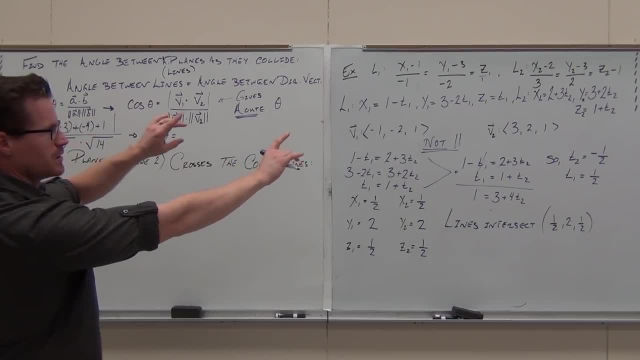 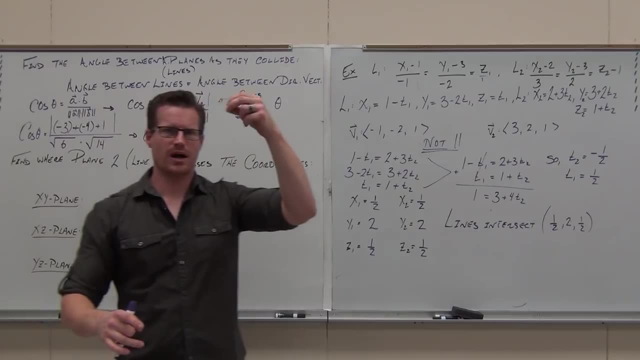 Negative, 3, negative 1.. Sorry, positive 3, negative 1 is negative 3. 2, negative 2, that's negative 4.. 1, 1,, that's 1.. So if I combine those, I'm getting negative 6. 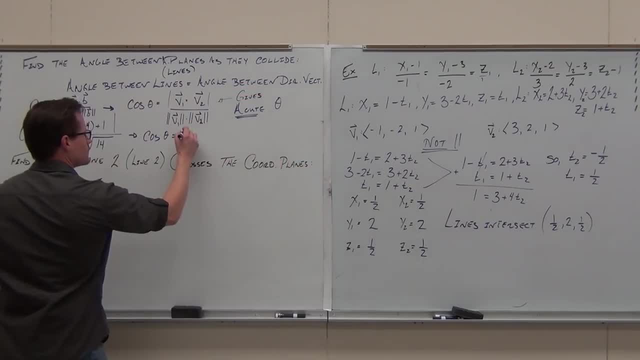 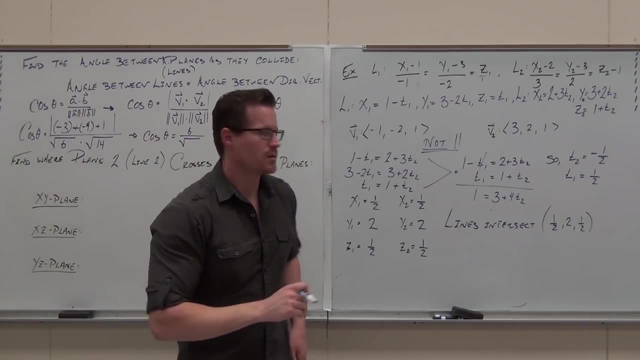 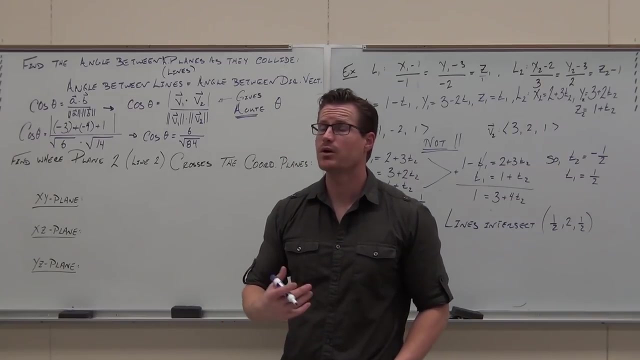 and absolute value would be positive 6.. Can you give me 6 times 14,, if you would? Now we're in real-world land, okay, So I don't care if you rationalize this right now. I want you to give me an approximation for the angle. 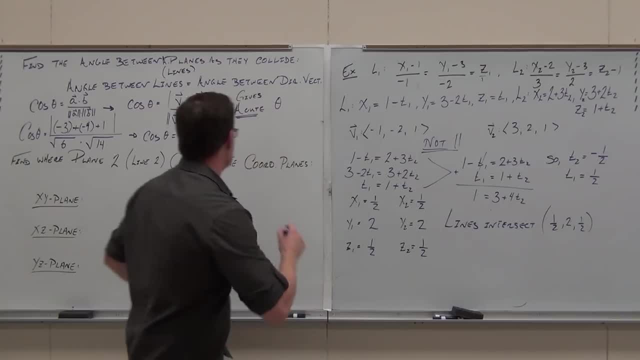 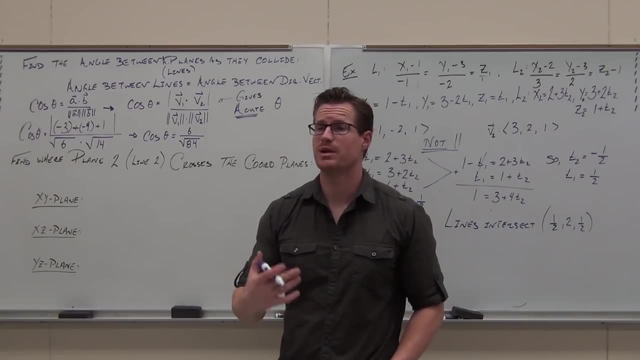 Can you give me six times 14, if you would Negative four, Now we're in real-world land, okay, So I don't care if you rationalize this right now. I want you to give me an approximation for the angle. 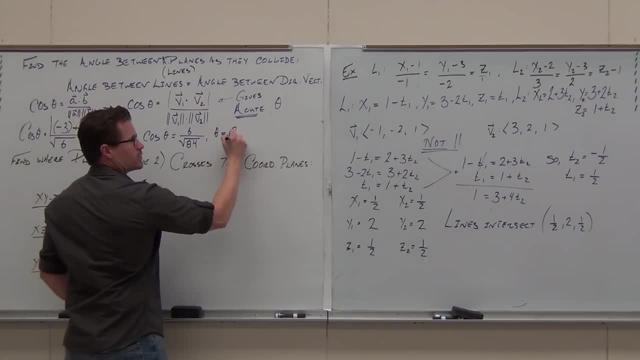 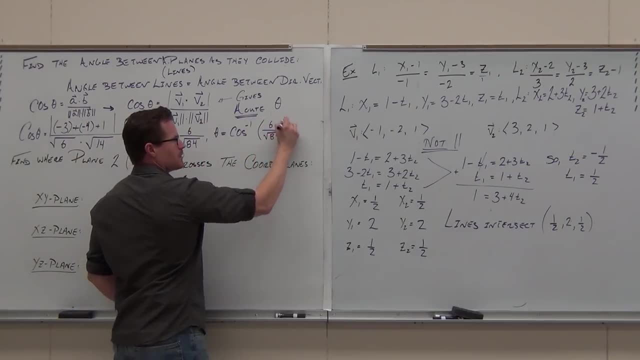 So for us we go okay. theta would be cosine inverse of. however you want to write this, You can rationalize and simplify for the equation. So this is the exact angle. but this is going to be about how much. I think I get something in the 40s. 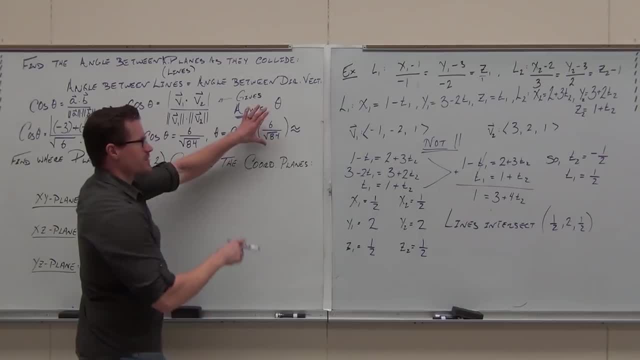 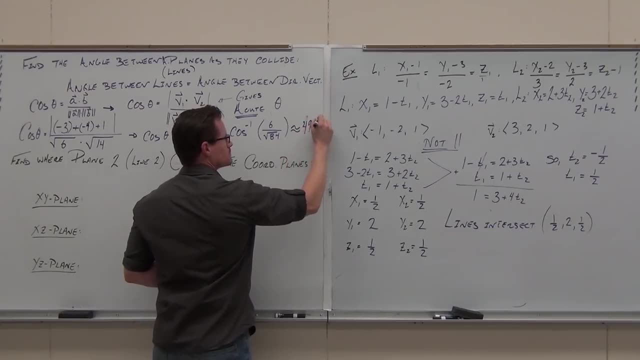 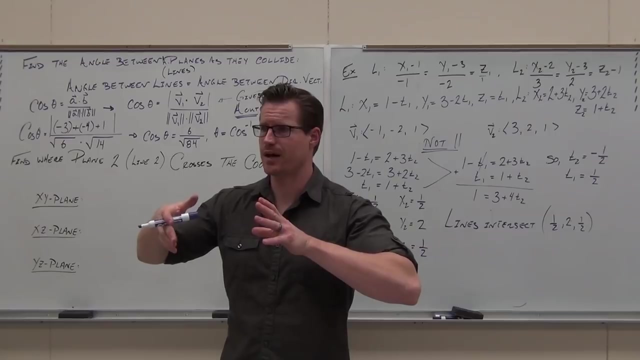 49.1.. 49.1.. So cosine inverse of this 49.1 degrees. We just found the angle that these planes are going to crash at the acute angle because we picked the absolute value. The other one would give us the obtuse angle. 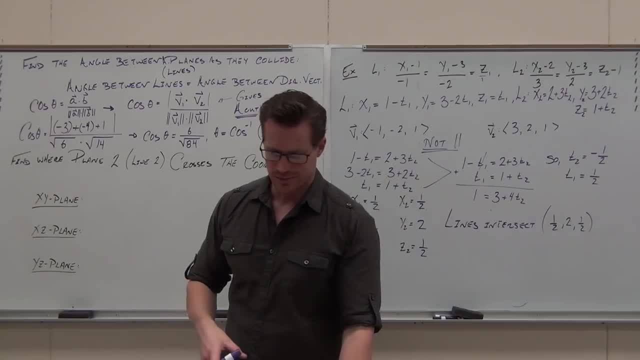 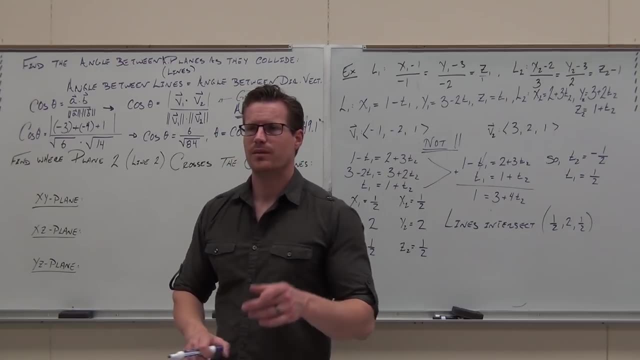 Are you understanding? That's what we're talking about. We want the acute angle Generally. why That's our convention? Now, I don't really want these planes to crash. Oh wait, wait, Pop quiz, pop quiz. 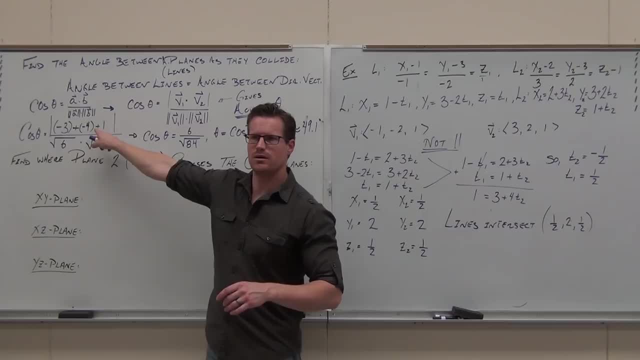 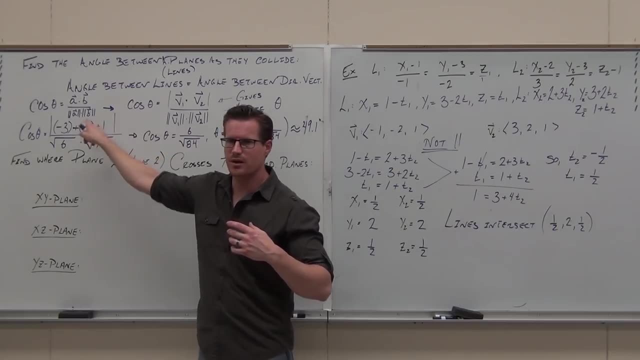 What if this worked out to be zero? Come on, stick with me. Come on, I know we have a lot. okay. What if this worked out to be zero? What if the dot product worked out the numerator, the dot product worked out to be zero? 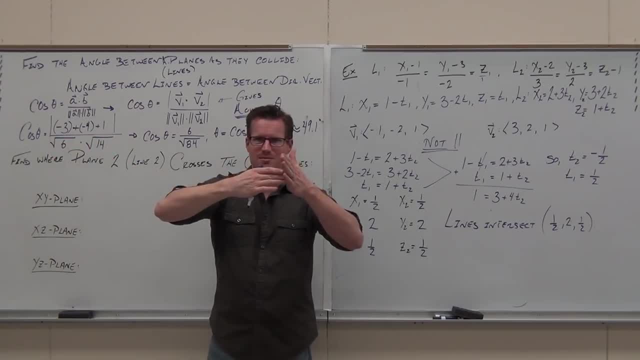 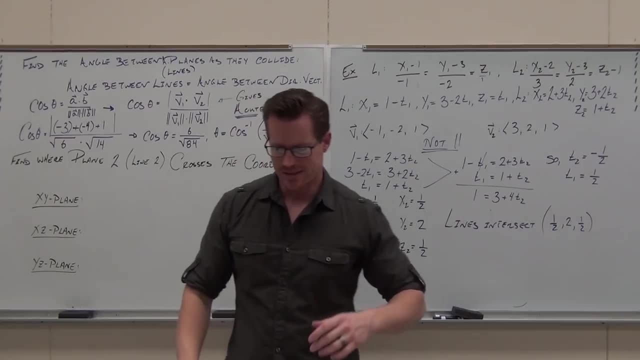 What would you know about these Plane? Orthogonal, Orthogonal, Orthogonal. Meet right at 90 degrees perpendicular, orthogonal. That's what would be happening. Kind of cool, All right. So it's, that's not, but I want to test you on it. 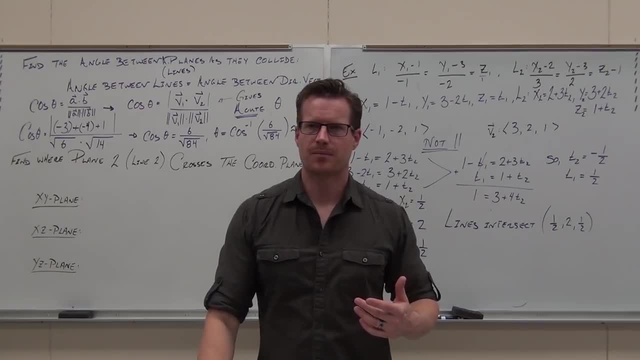 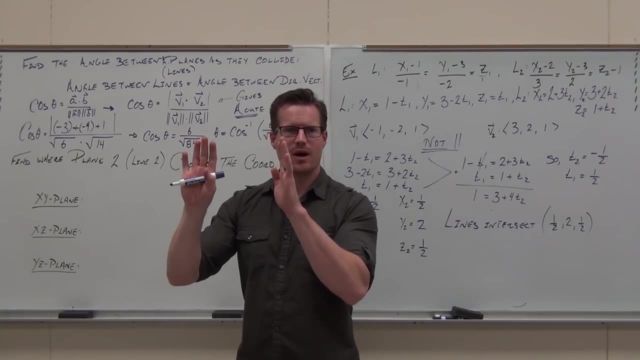 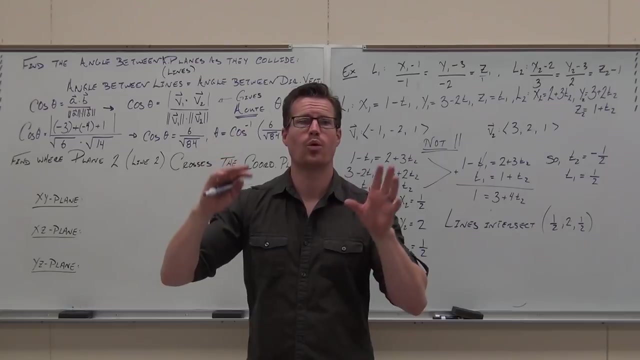 I don't want these planes to intersect, So I'm going to develop a warning system As soon as plane number two enters my little octant here. so my octant is the xy, the yz and the xz planes. As soon as it crosses those things, I'm going to send warnings. 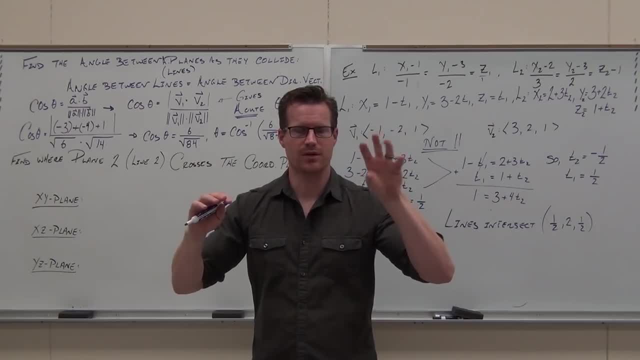 And I'm going to say, hey, You're on a collision course because I don't want these things to happen. if I'm the whatever people that control airplanes, do you know? I don't know, I'm not that guy. 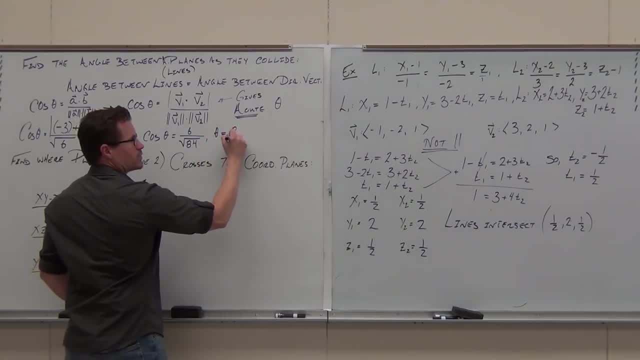 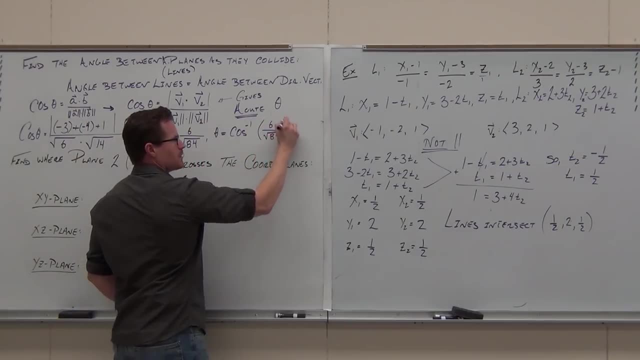 So for us we go okay. theta would be cosine inverse of. however you want to write this, You can rationalize and simplify for the exact angle. but this is going to be about how much I think I get something in the 40s. 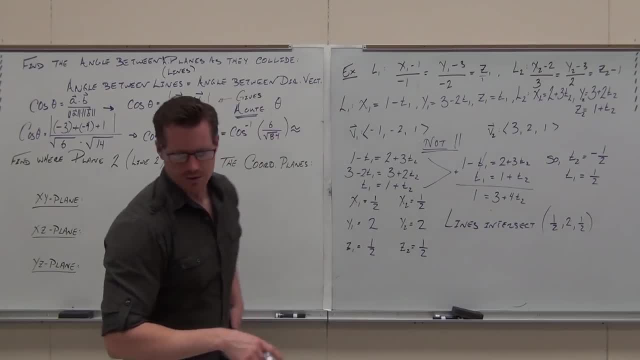 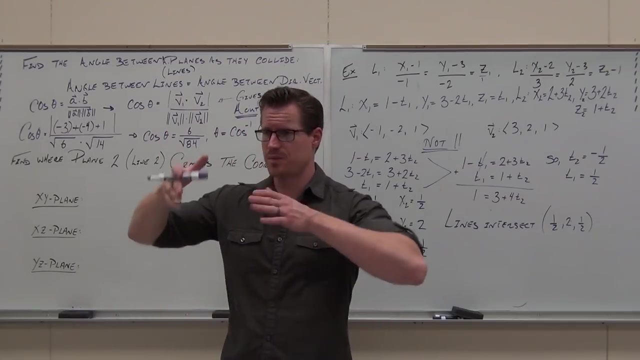 Forty-nine point one, Forty-nine point one, So cosine inverse of this Forty-nine point one degrees. We just found the angle that these planes are going to crash at the acute angle because we picked the absolute value. The other one would give us the obtuse angle. 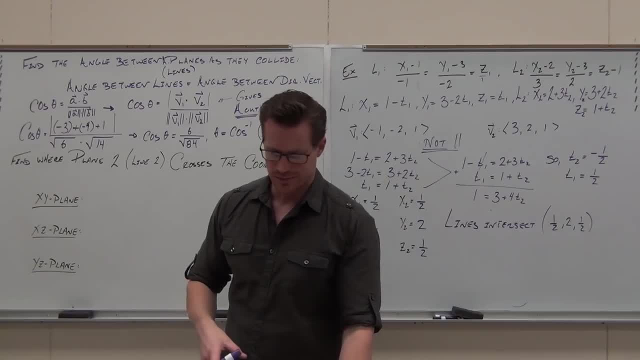 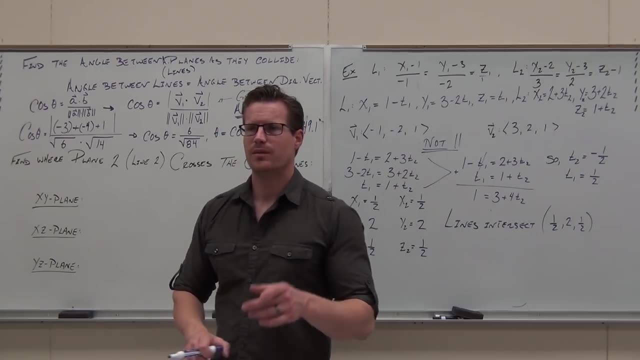 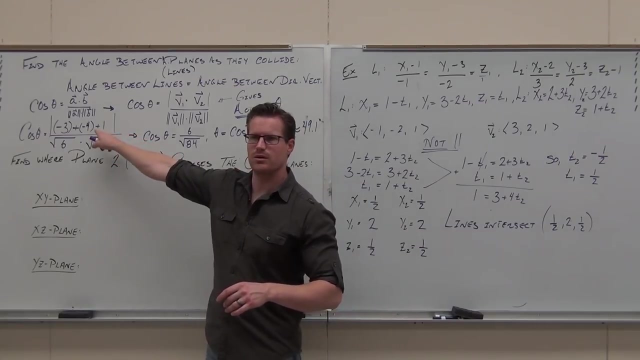 You understand what I'm talking about. We want the acute angle Generally. why that's our convention? Now, I don't really want these planes to crash. How about? oh wait, wait, pop quiz, pop quiz. What if this worked out to be zero? 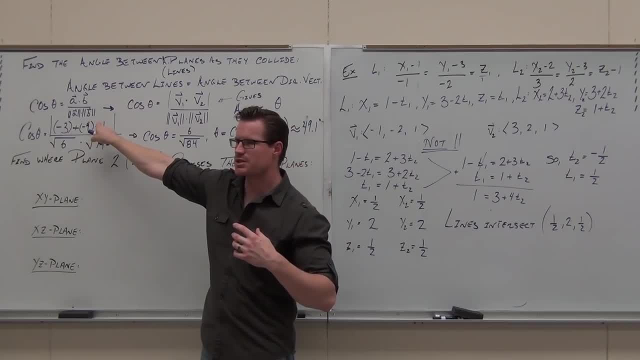 Come on, stick with me. Come on, I know, I know we have a lot. okay, What if this worked out to be zero? What if the dot product worked out the numerator, the dot product, worked out to be zero? 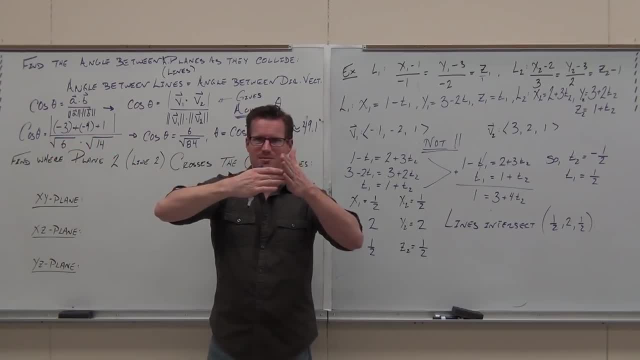 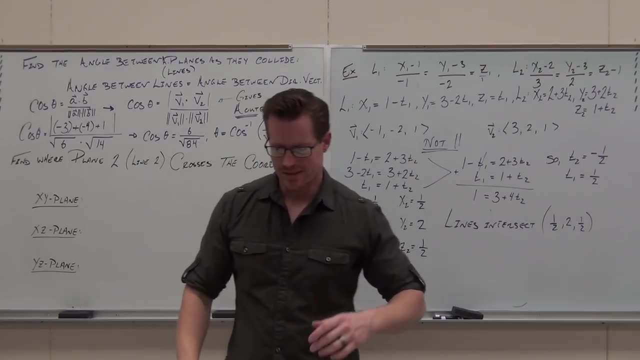 What would you know about these planes? Orthogonal, Orthogonal, Eating right, meeting right at 90 degrees perpendicular orthogonal. That's what would be happening. Kind of cool, all right. So it's, that's not, but I want to test you on it. 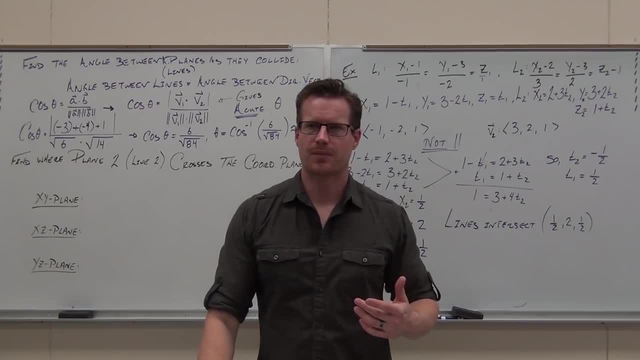 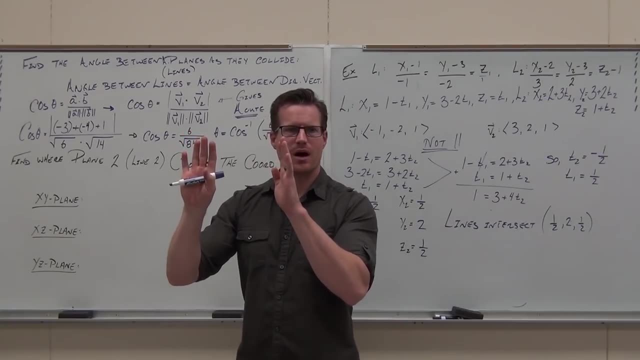 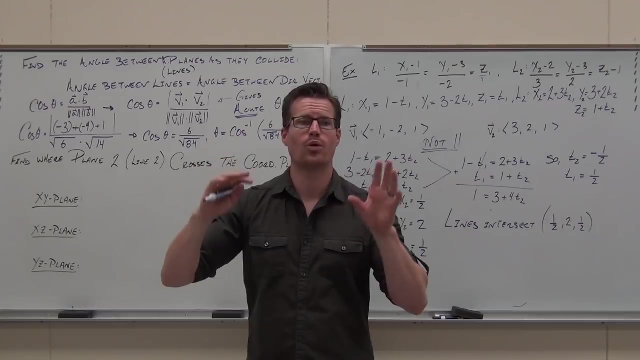 I don't want these planes to intersect, So I'm going to develop a warning system As soon as plane number two enters my little octant here. so my octant is the xy, the yz and the xz planes. as soon as it crosses those things, I'm going to send warnings. 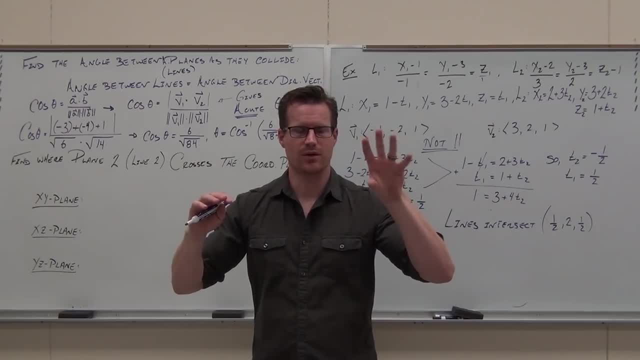 And I'm going to say, hey, you're on a collision course Because I don't want these things to happen. if I'm the whatever people that control airplanes, do you know? I don't know, I'm not going to do that. 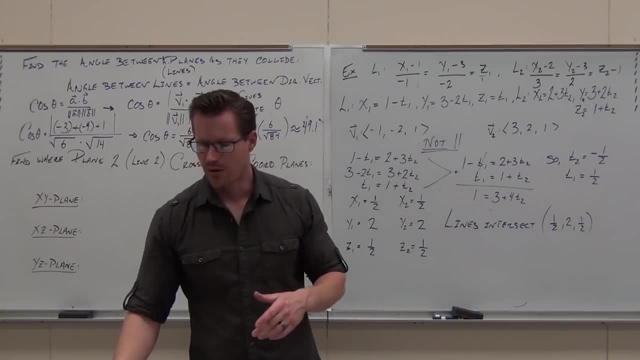 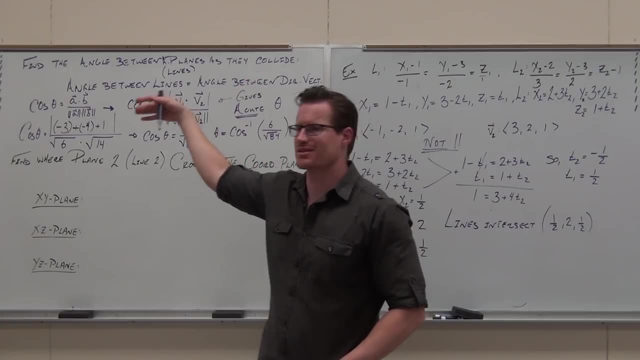 I'm not that guy, I teach math. But what I want to happen? I want to figure out when and where they're going to cross my coordinate planes. Here's how you do that. Now, naturally I'm making airplanes, but this is just lines intersecting stuff, okay. 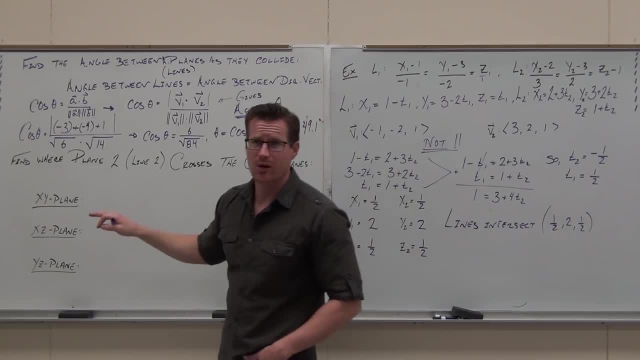 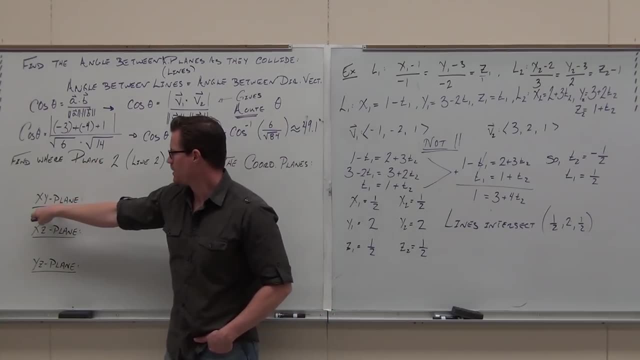 That's what's going on. So how you figure out where and when we cross the yz plane, how to do that? Just set the component that gives you that plane equal to zero. So basically set the component, not less. 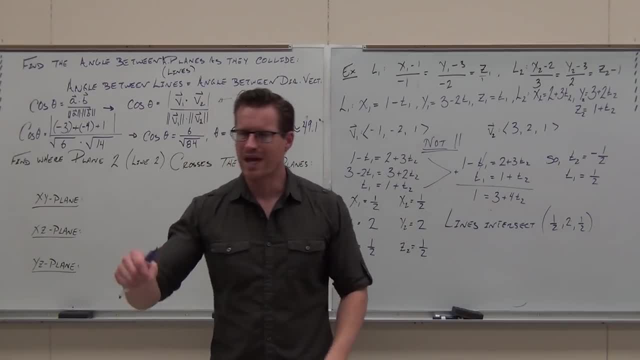 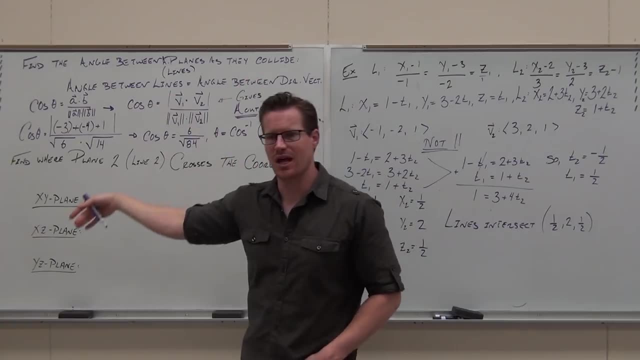 I teach math. But what I want to happen? I want to figure out when and where they're going to cross my coordinate planes. Here's how you do that. Now, naturally, I'm making airplanes, but this is just lines intersecting stuff, okay. 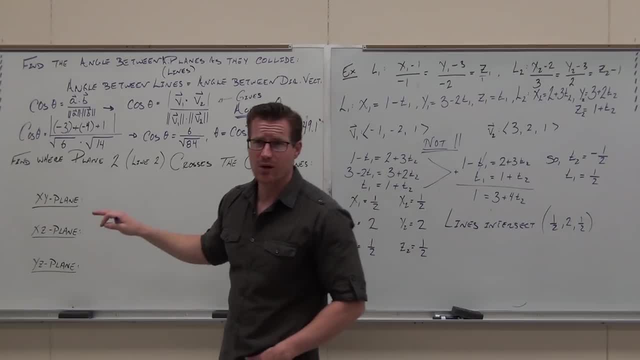 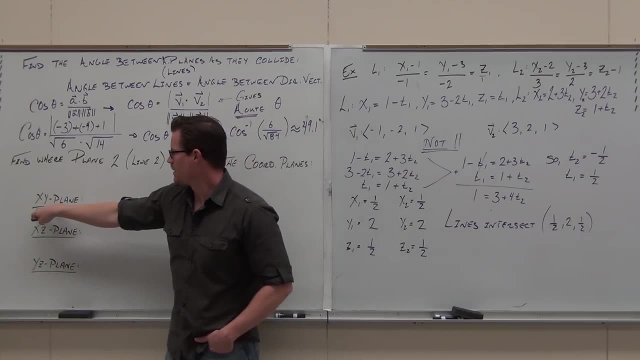 That's what's going on. So how you figure out where and when we cross the yz plane. how to do that? Just set the component that gives you that plane equal to zero. So basically, set the component not listed equal to zero. 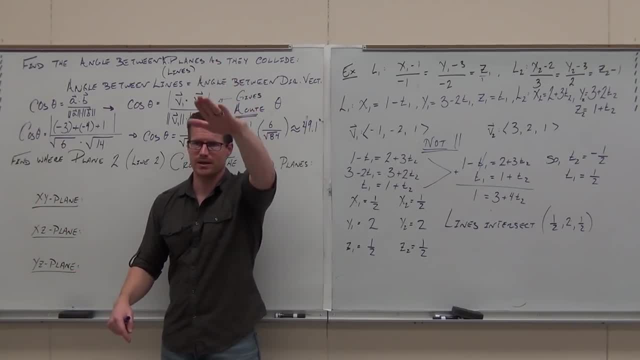 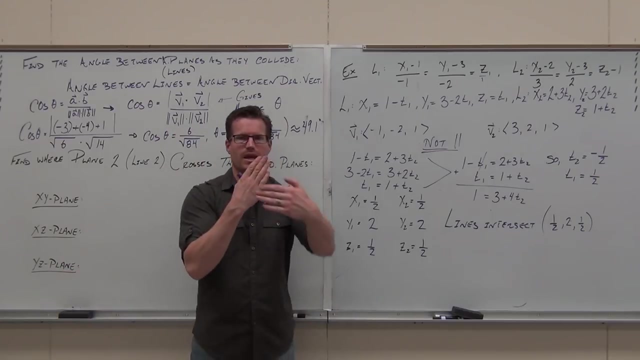 Not listed equal to zero. If I'm crossing the xz plane, that's when- sorry xy plane, that's when z is zero. If I'm crossing the xz plane, that's when y is zero. If I'm crossing the yz plane, that's this one, that's when x is zero. 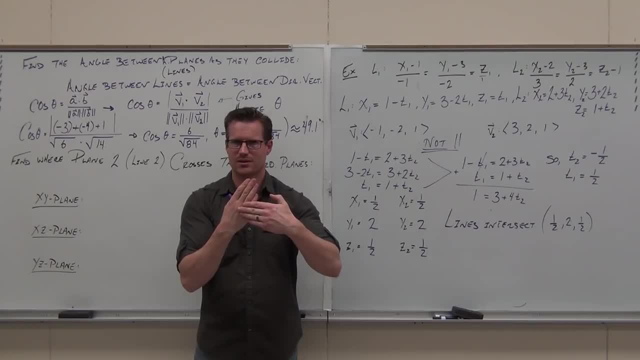 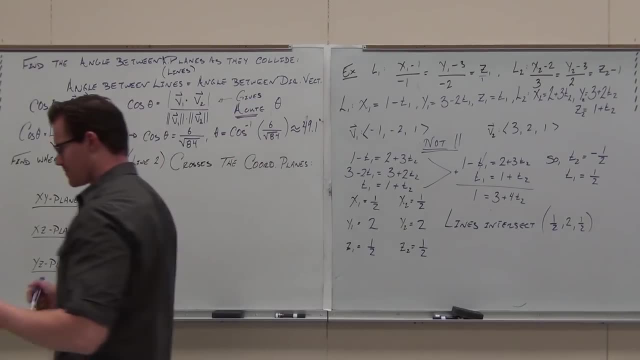 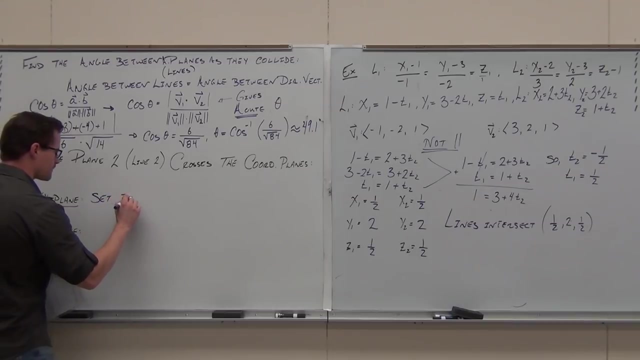 Does that make sense? Are you sure? Or are you just nodding your head? so I'll shut up and keep on doing this math, you know All right. So whatever plane you want, whatever variable is not listed, set it equal to zero. 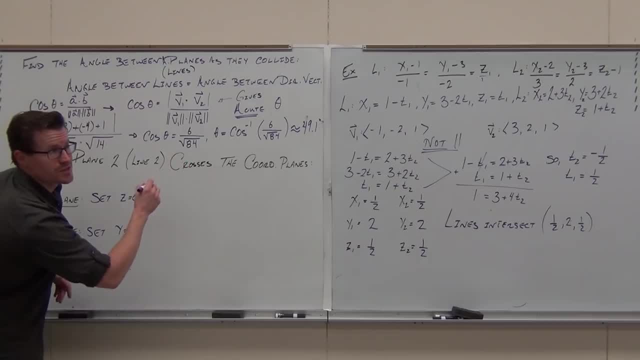 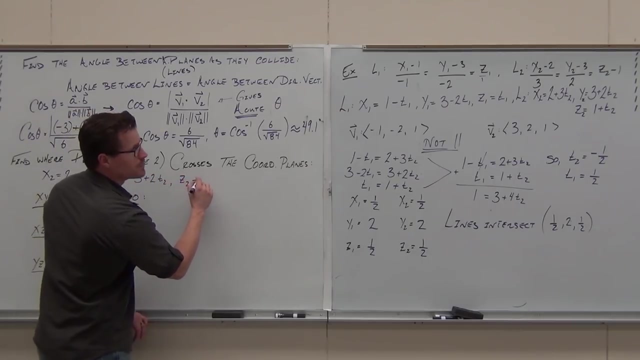 Now I'm talking about plane two, line two. So line two was this one. If I set z equal to zero, I'm only looking here. this is all I'm looking at. If I'm going to set there's no z, there's no z, there's the z. 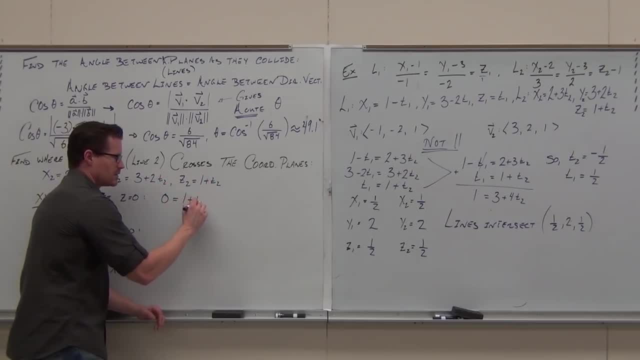 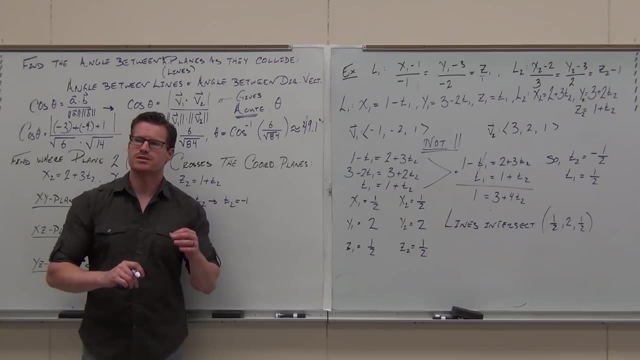 If I set z equal to zero, Then t two, t sub two, equals negative one. This is the when. When I'm going to cross the xy plane is when t is negative one. Now, can you figure out the point to that? 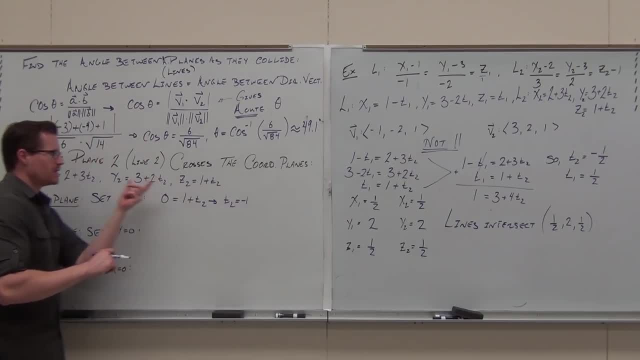 Well, yeah, Now that you've got a t sub two equals negative one. just plug it in. If I plug that in, then I'm going to get the point. So if I plug in negative one here, well, let's see negative three. 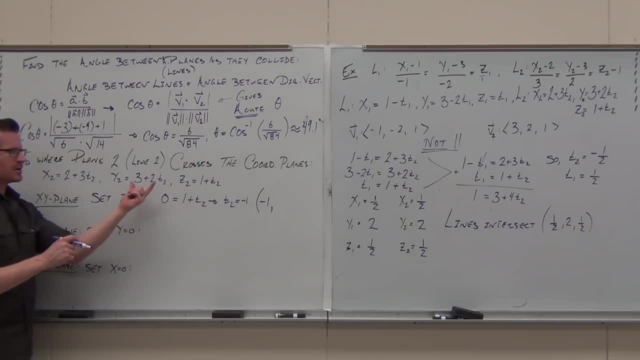 That looks like a negative one If I plug in negative one to me. if I plug in negative one here, that looks like a positive one to me. If I plug in negative one here, why would I do that? I just set z equal to zero. 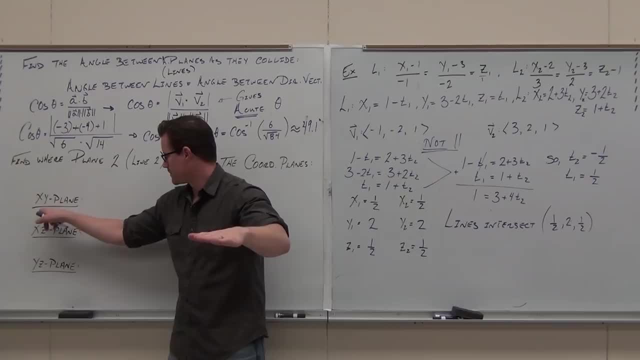 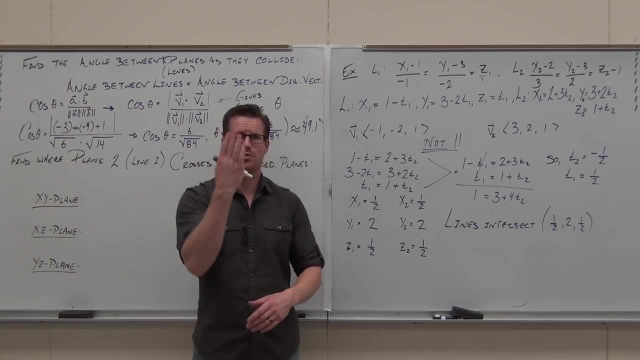 If I'm crossing the xz plane, that's when- sorry xy plane, that's when z is zero. If I'm crossing the xz plane, that's when y is zero. If I'm crossing the yz plane, that's this one, that's when x is zero. 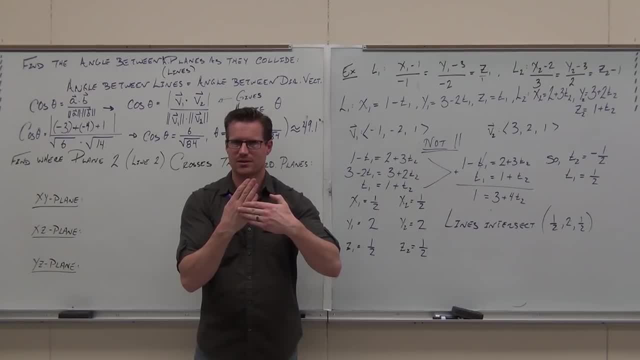 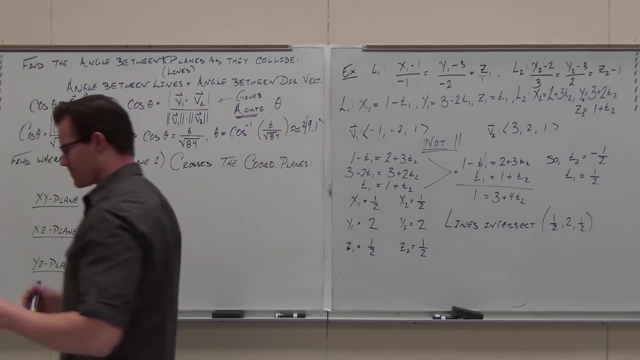 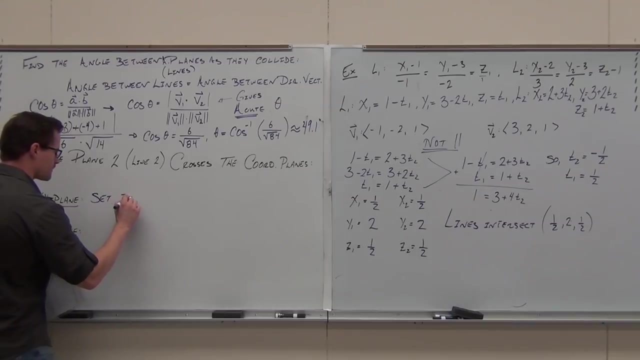 Does that make sense? Are you sure? Or are you just nodding your head? so I'll shut up and keep on doing this math, you know All right. So whatever plane you want, whatever variable is not listed, set it equal to zero. 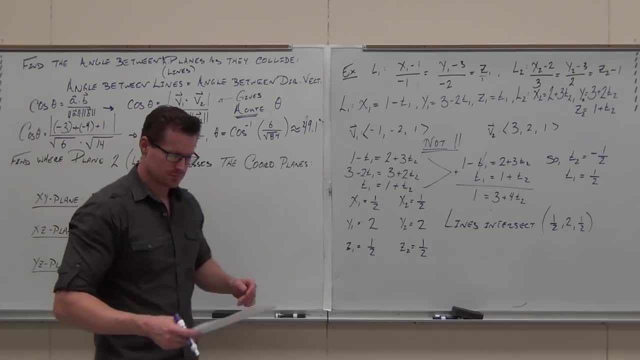 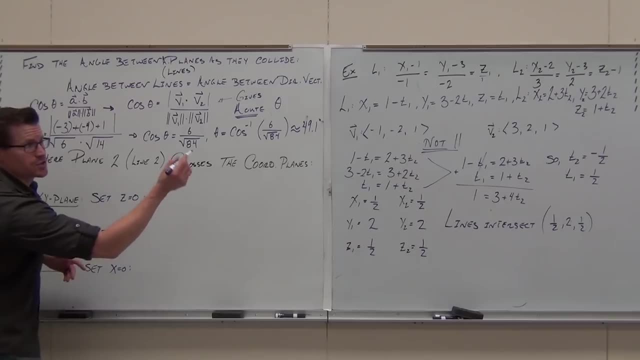 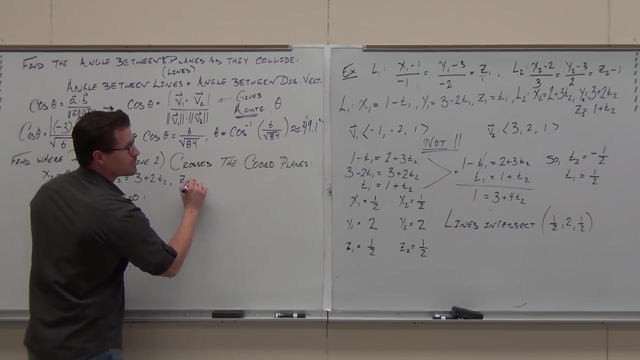 Now I'm talking about plane two, line two. So line two was this one. If I set z equal to zero, I'm I'm only looking here. this is all I'm looking at. If I'm going to set there's no z, there's no z, there's the z. 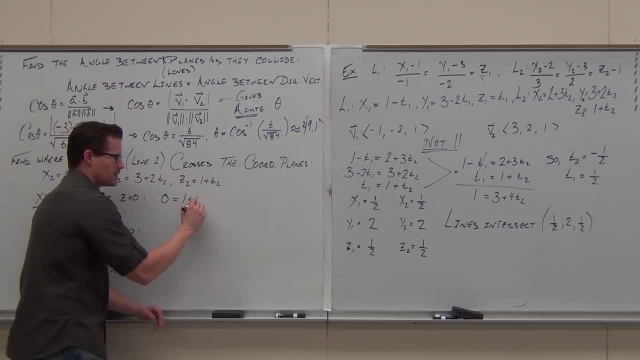 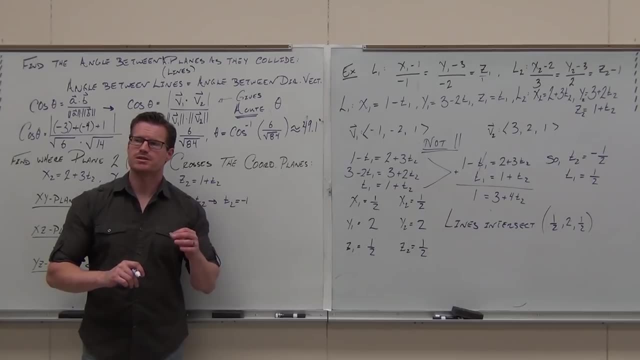 If I set z equal to zero, then t two, t sub two, equals negative one. This is the when. when I'm going to cross the xy plane is when t is negative one. Now, can you figure out the point to that? 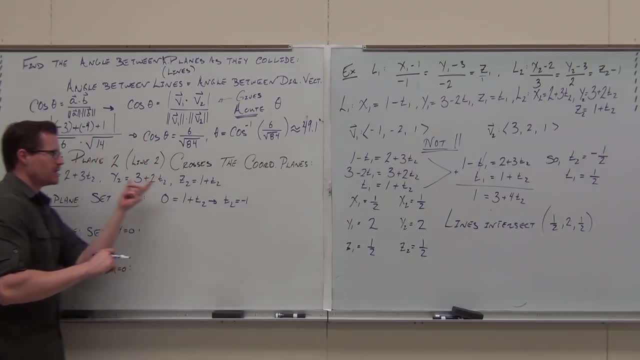 Well, yeah, Now that you got a t sub two, If I set t sub two equals negative one, just plug it in. If I plug that in, then I'm going to get the point. So if I plug in negative one here, well, let's see, that looks like negative one to me. 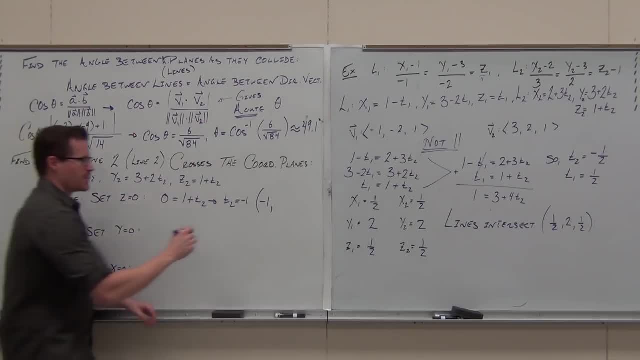 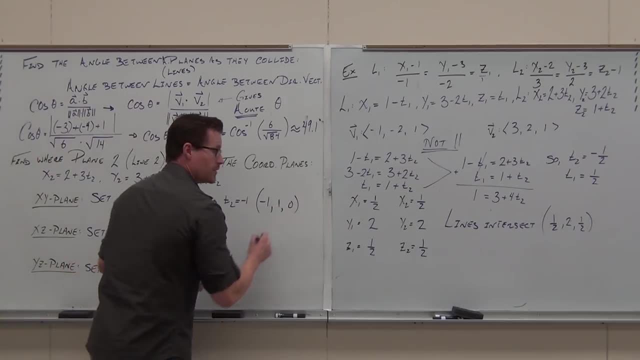 If I plug in negative one here, that looks like positive one to me. If I plug in negative one here, why would I do that? I just set z equal to zero. It's obviously going to be zero. Verify that that point is actually on the xy plane, because your z is zero. 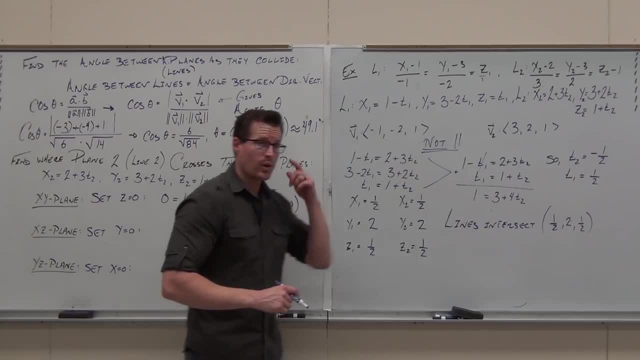 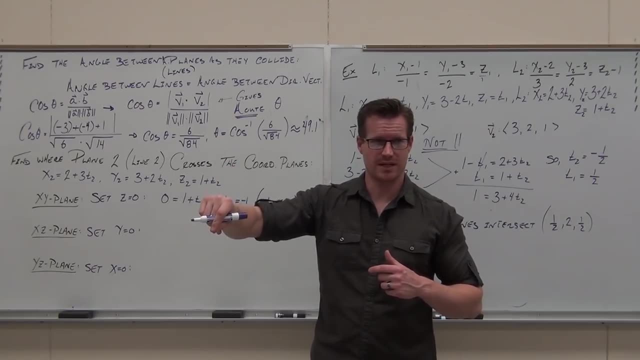 It's obviously going to be zero. Verify that that point is actually on the xy plane, because your z is zero. That was the whole idea. Does that make sense? Can you do the next two? Can you do that? Try it, Try it. 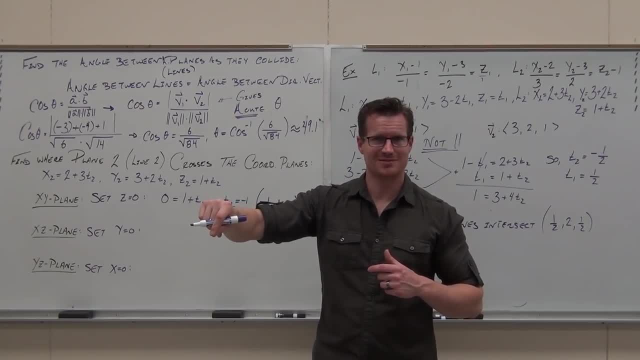 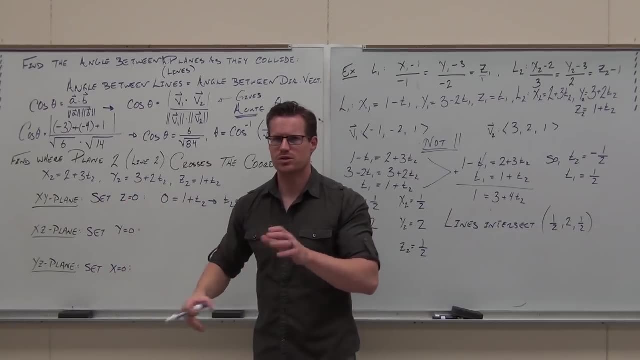 That was the whole idea. Does that make sense? Can you do the next two? Can you do that? Try it, Try it. Set y equals zero. Go through it on your own, Don't just wait for me to do it. 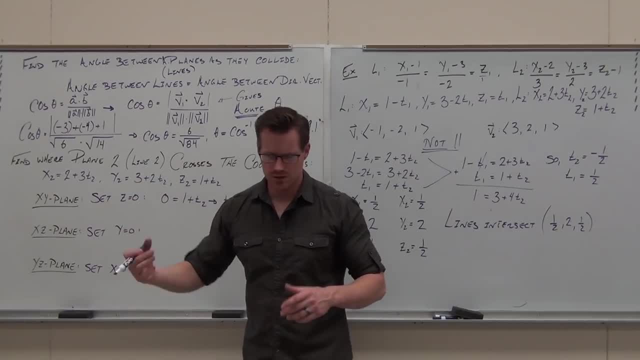 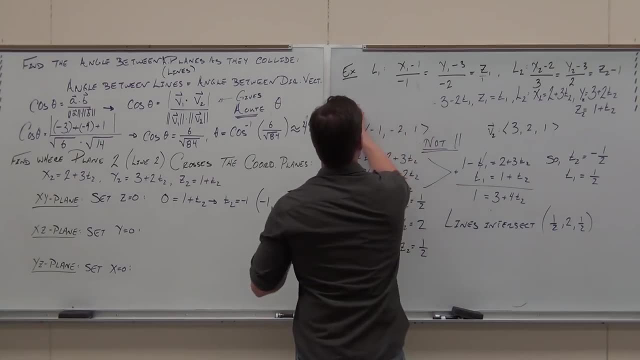 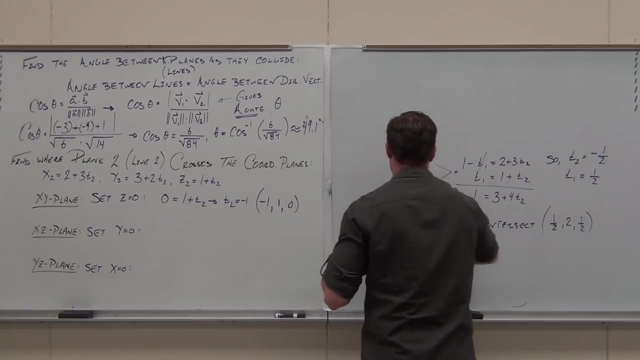 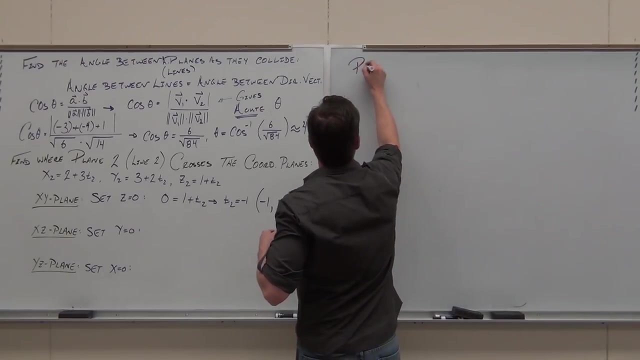 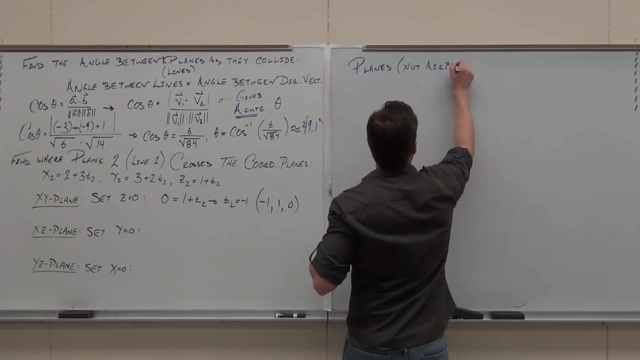 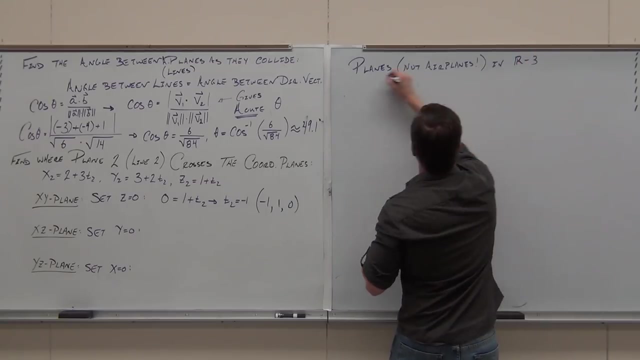 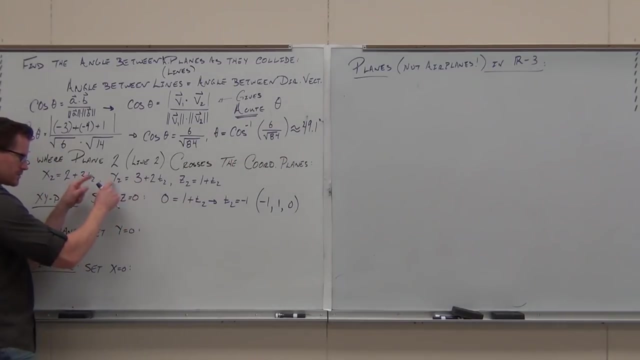 Set y equal to zero. Go through it on your own. Don't just wait for me to do it. I'm going to do it in just a minute. Just a minute, Just a minute. One, Two, One, Two, Three. 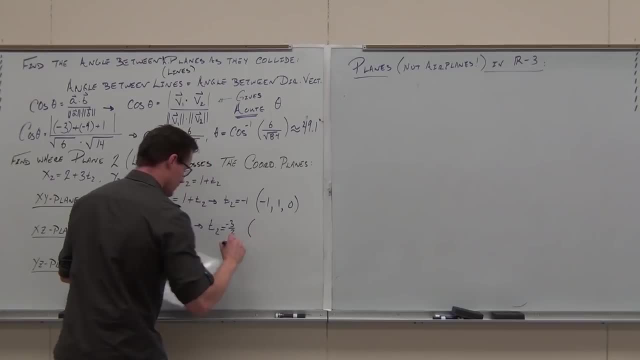 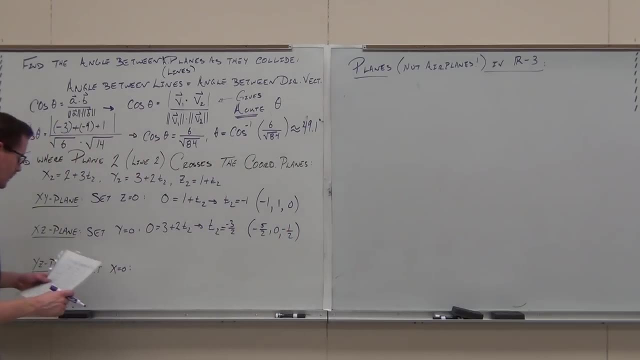 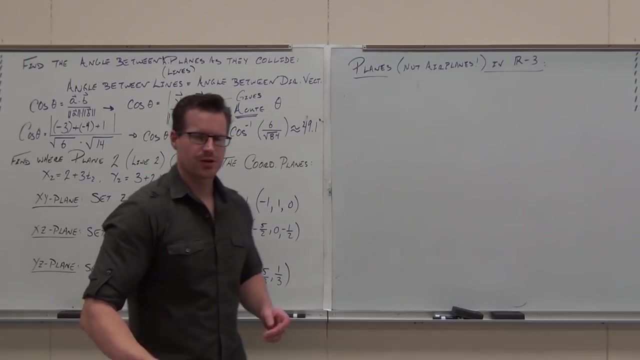 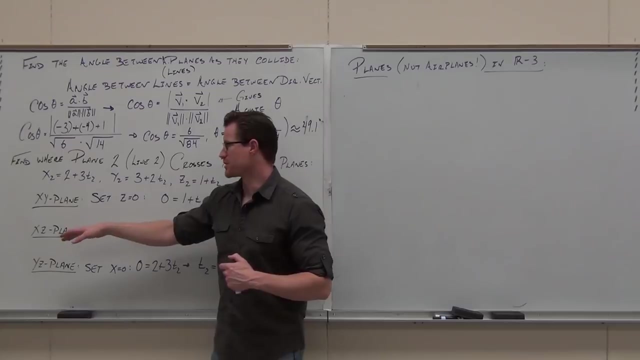 Four, Five, Six, Seven, Eight, Nine, 10., 11. 12. 23.. If you did it on your own, that's excellent. I at least want the idea understood. If I'm going to cross the XZ plane, Y has to be zero. 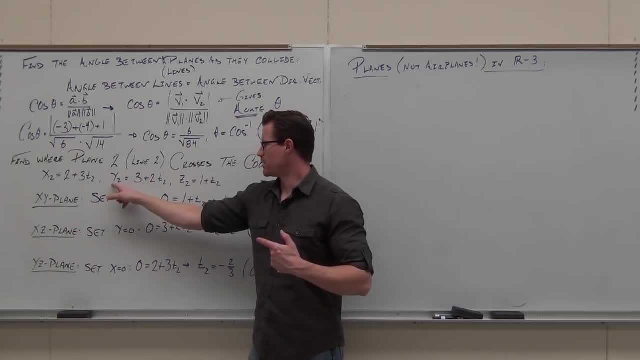 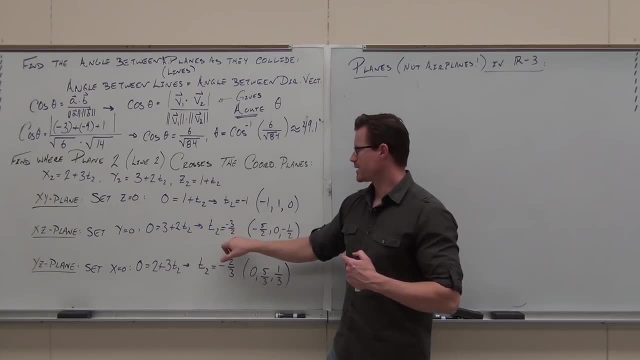 Go to the Y coordinate. that formula zero, Y has to be zero. If we solve, this is the, when I'm going to cross the XZ plane, Take it and plug it in. Of course Y is going to be zero. 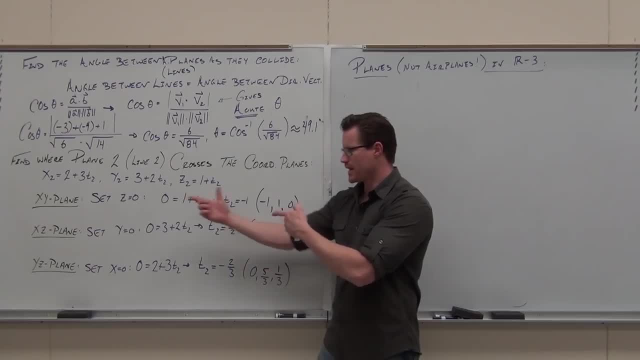 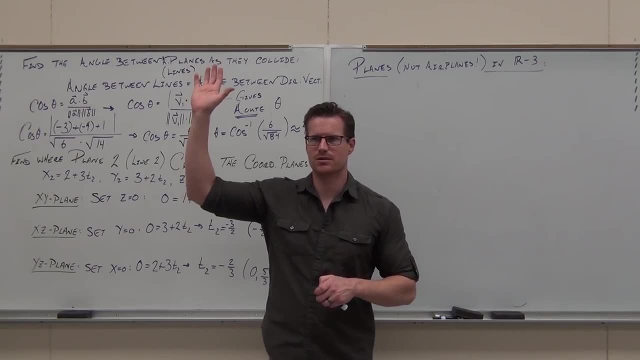 That's literally how we got it And you got a point. That's a point on the XZ plane. Same thing happens with the YZ plane and that's the point that we have. I need to show fans the concept here. 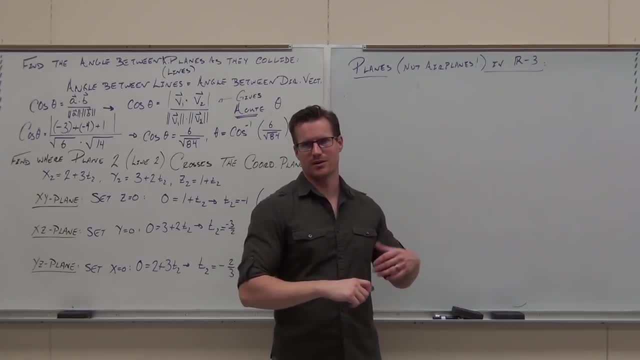 Okay Now planes. Planes are not just planes, Planes are not airplanes. all right, Planes are really cool and they're really easy. What we're going to do is I'm going to make it through the formula and the rest of it's just practice. 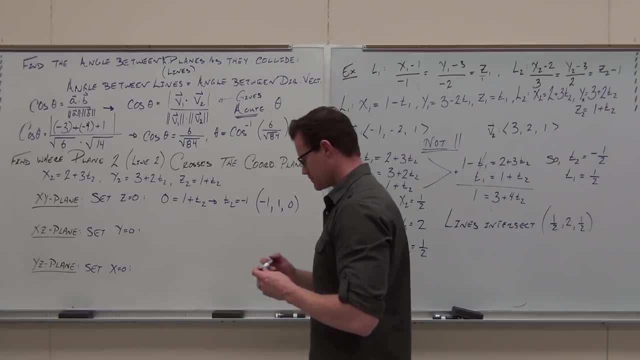 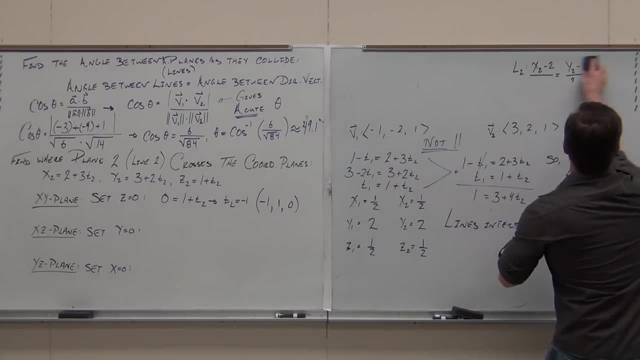 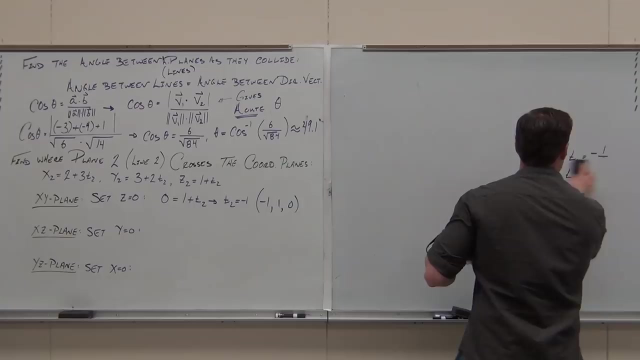 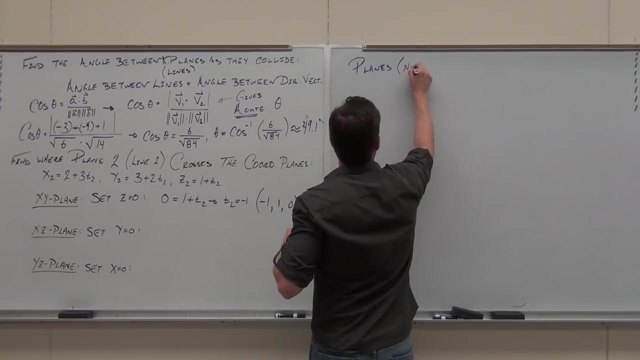 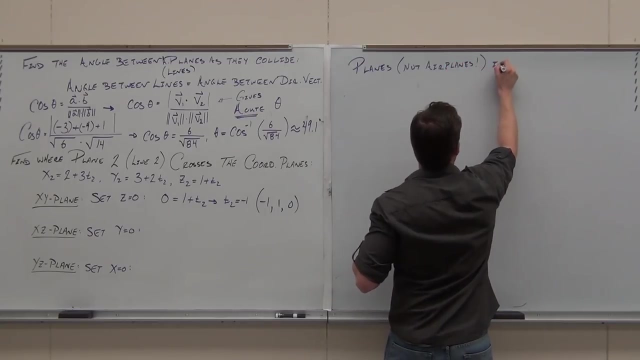 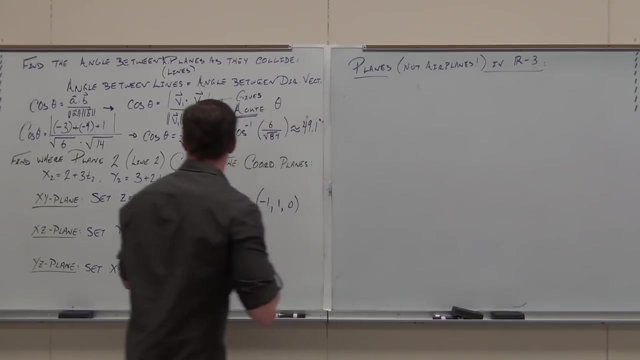 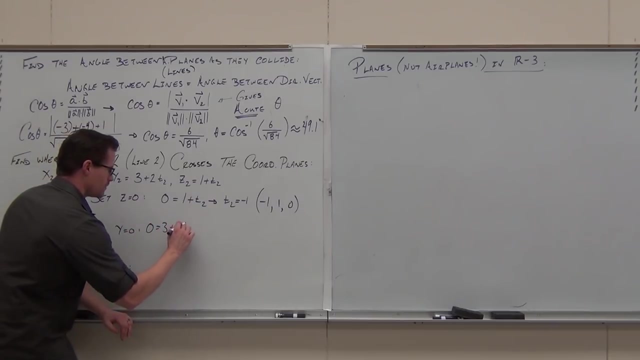 I'm going to do it in just a minute And then you do the other side. Sorry, You can funny Give three TV це. Okay, so is the point minus z equal extra to what? Yes, All right, Anyways, that's the test to verify if that's what you're saying. 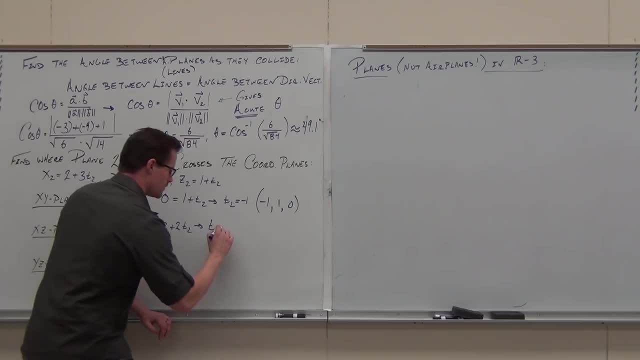 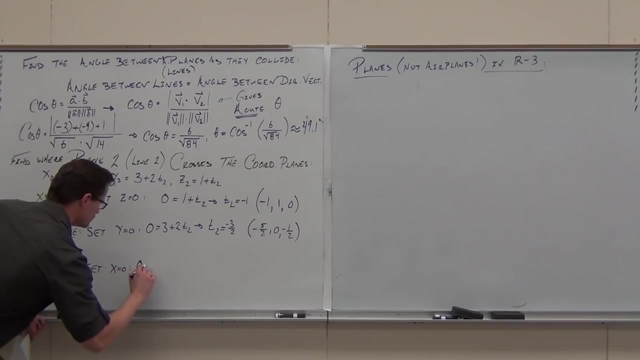 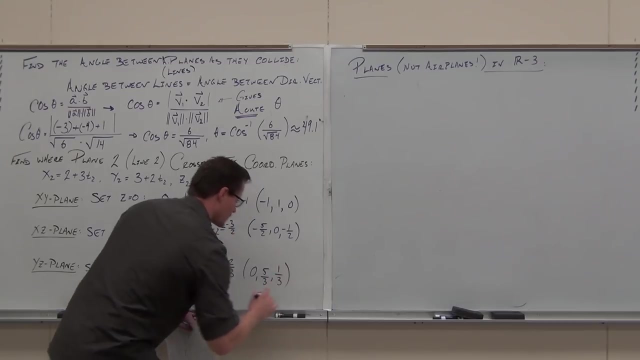 I'm sure that we're going to do that. That was awesome, Yep, Okay, guys, We're doing it All right, Bye, Bye, Bye, Bye. Thank you, If you did it on your own, that's excellent. 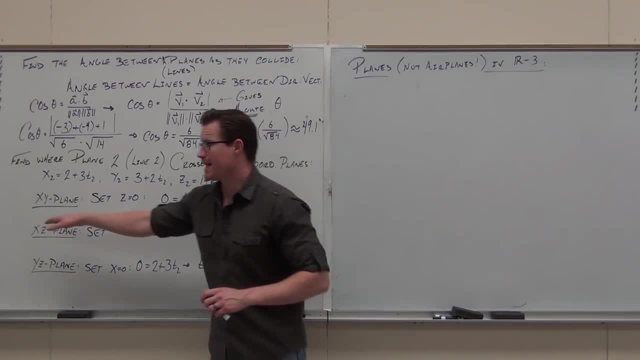 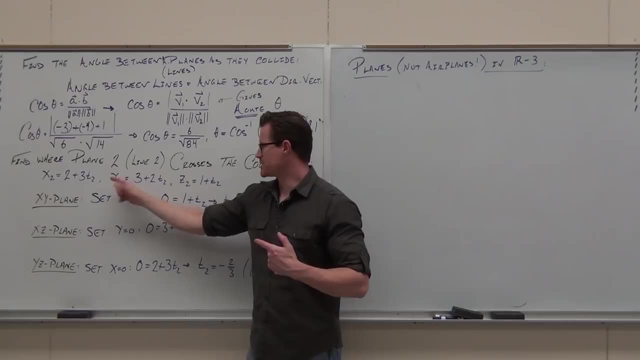 I at least want the idea understood. If I'm going to cross the xz plane, y has to be 0. Go to the y coordinate. that formula 0, y has to be 0. If we solve this is the when I'm going to cross the xz plane. 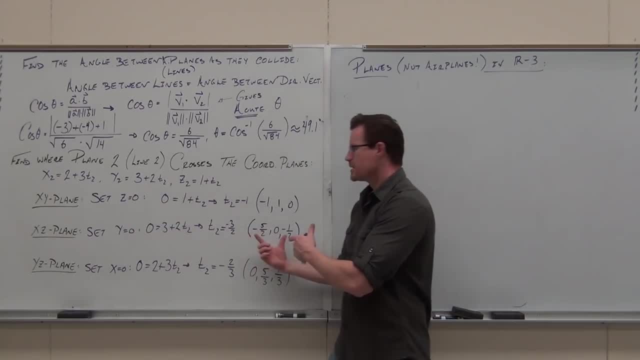 Take it and plug it in. Of course, y is going to be 0. That's literally how we got it And you got a point. That's a point on the xz plane. Same thing happens with the yz plane and that's the point that we have. 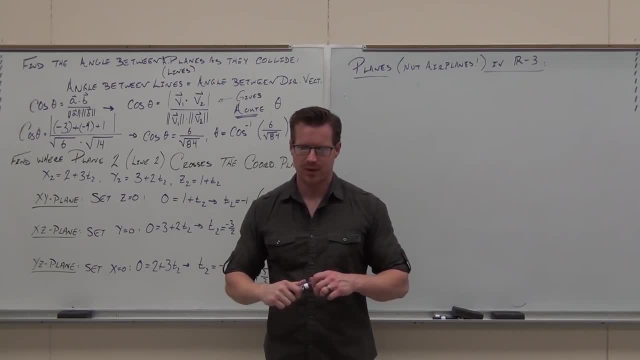 I need to show fans the concept here. Okay now, planes. Planes are not airplanes. all right, Planes are really cool and they're really easy. What we're going to do is I'm going to make it through the formula. 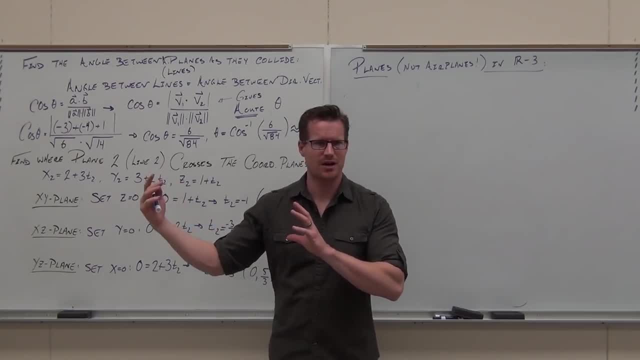 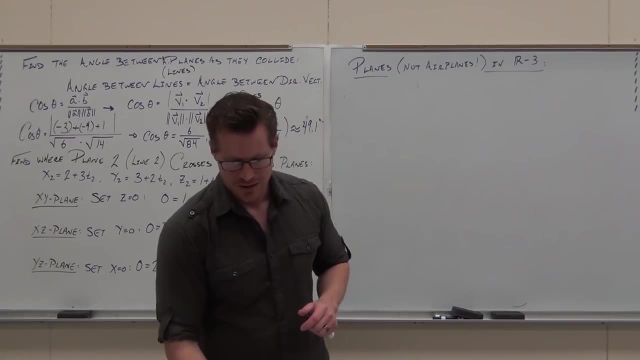 and the rest of it's just practice. It works very similar to this stuff. There's just one thing that we need to understand about planes before we really get into the nitty-gritty. I'm going to define something that we've talked about. 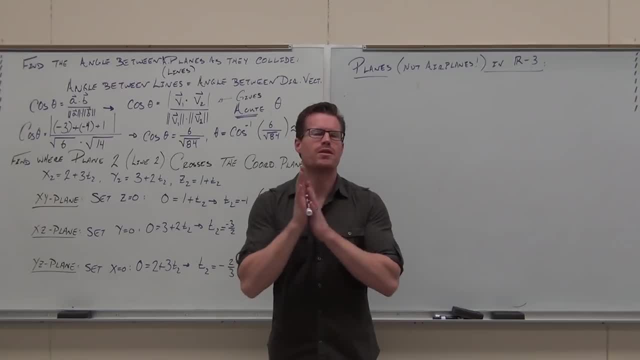 It works very similar to this stuff. There's just one thing that we need to understand about planes before we really get into the nitty-gritty. I'm going to define something that we've talked about. we haven't actually defined yet: It's called a normal. 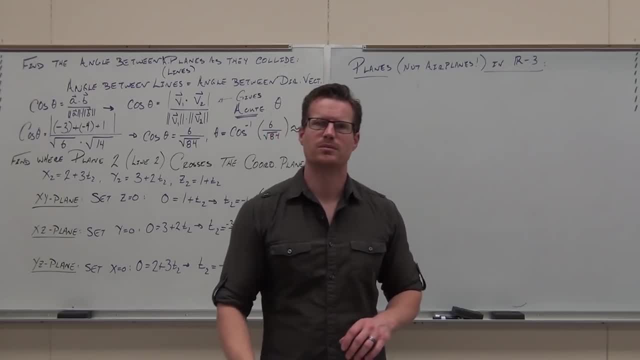 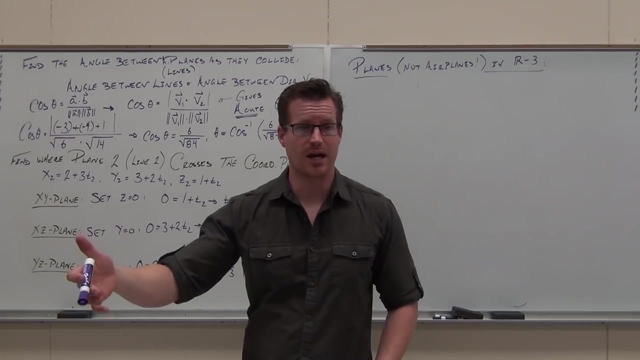 we haven't actually defined yet. It's called a normal. Here's what a normal I told you about it. What's a normal mean? An idea of perpendicular. Normal specifically means orthogonal or perpendicular to a plane. That's what we say here. 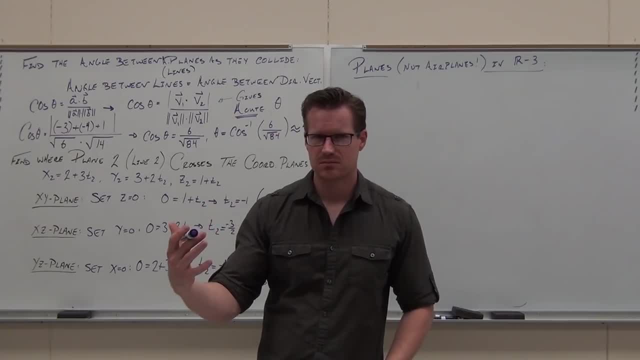 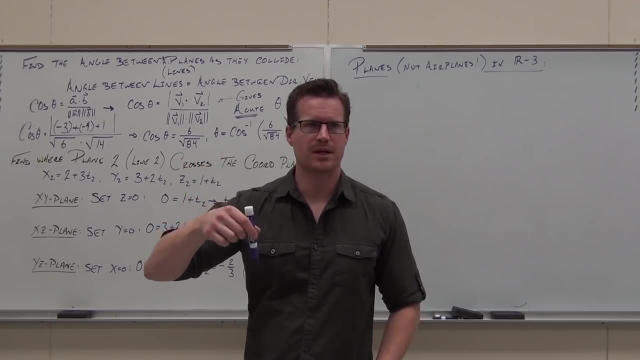 Here's what a normal I told you about it. What's a normal mean? It's an idea of perpendicular. Normal specifically means orthogonal or perpendicular to a plane. That's what we say here Now, because we said, well, normal is two vectors. 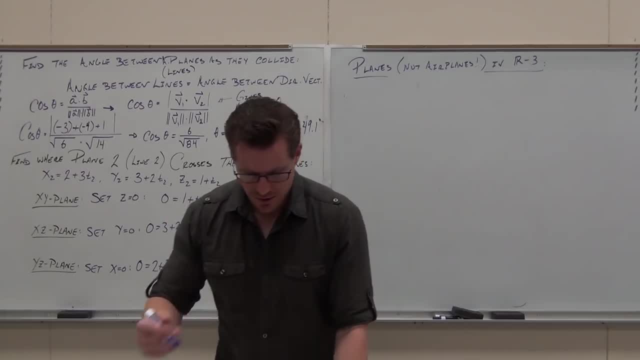 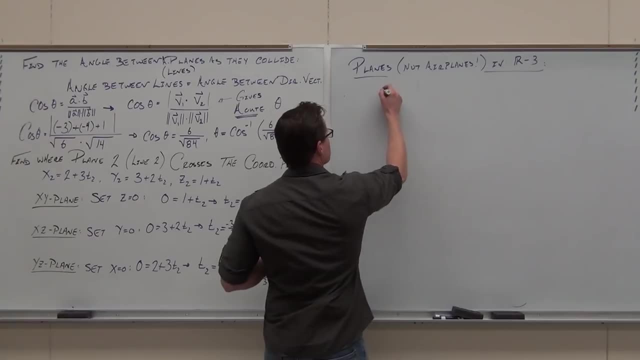 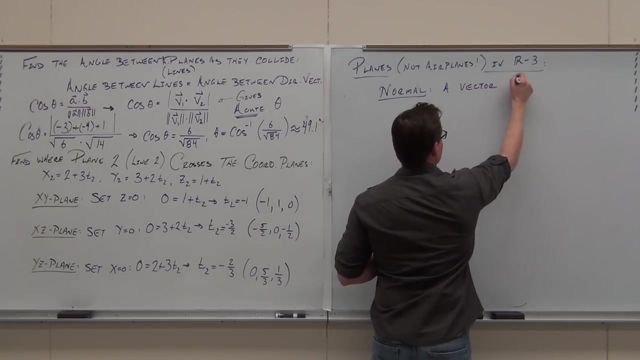 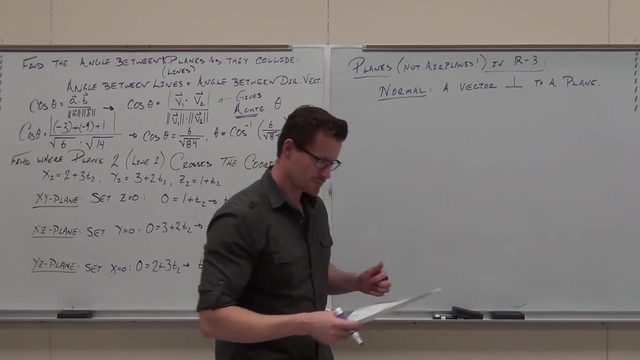 Well, a vector can be contained in a plane. so technically, yes, But when we say a normal, a normal vector is a vector perpendicular to a plane. Now, how about this? we're going to build the formula and then we'll take our break. 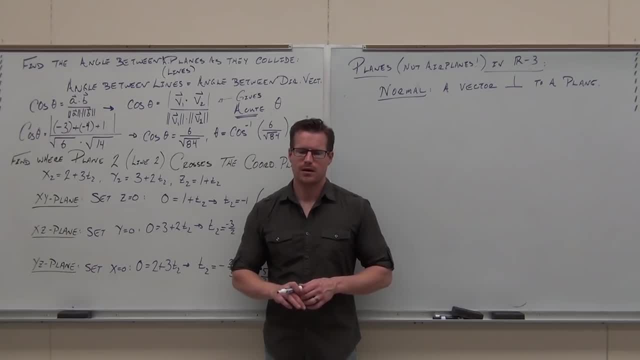 How about this? how many normal vectors are there to a plane? Here's a plane. How many normal vectors come off of that thing? Infinite, Infinite, Infinite. Are those normal vectors all parallel? Yes, Which means they're all scalar multiples. 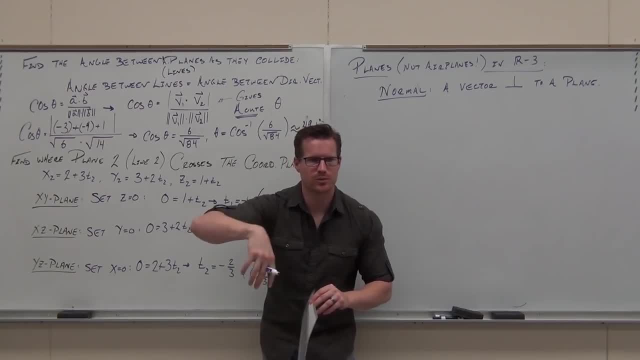 So while there are infinitely many normal vectors, they're all scalar multiples of the same unit normal. Now we don't need a unit normal, but I'm trying to get to understand that it doesn't matter. One normal vector is enough to define a plane. 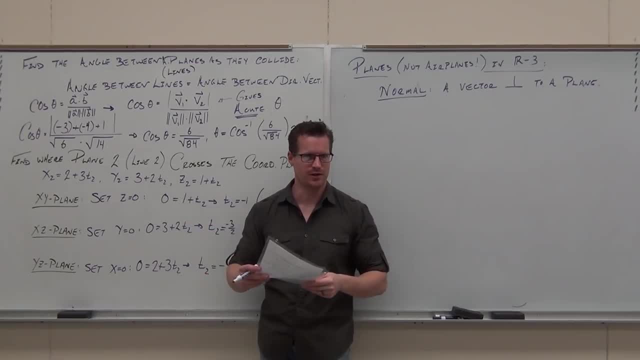 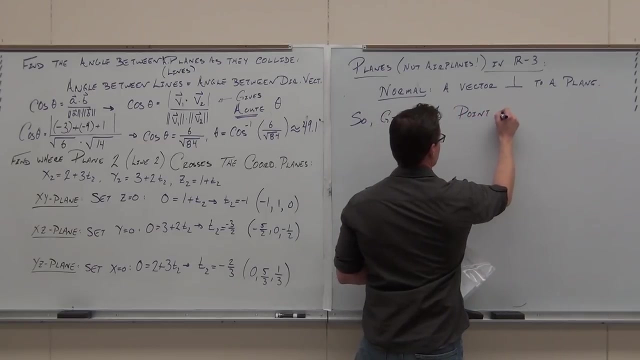 Do you understand what I'm talking about? It's all the other ones. All these other ones are just scalar multiples of it, You with me. So, given one point on a plane. 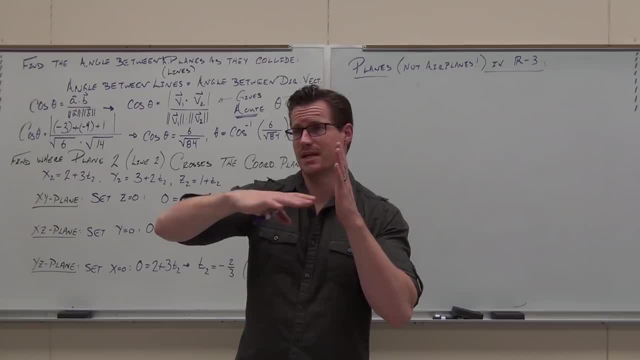 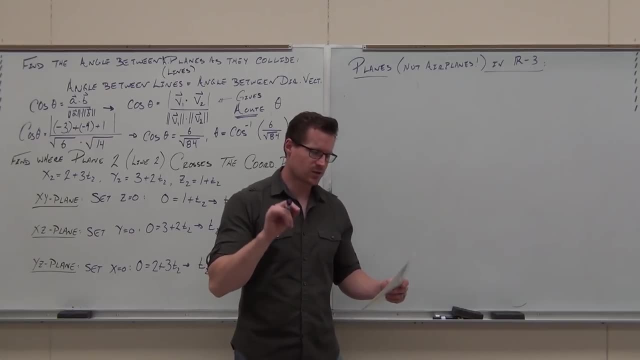 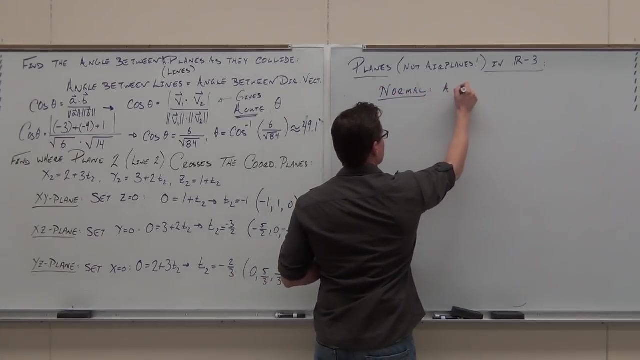 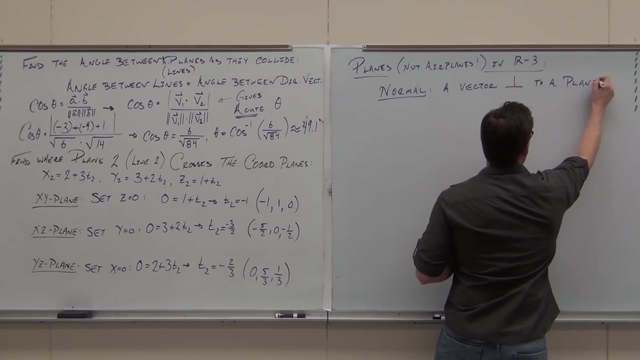 Now, because we said: well, normal is two vectors. Well, a vector can be contained in a plane, so technically, yes, but when we say a normal, a normal vector Is a vector perpendicular to a plane. Now, how about this? 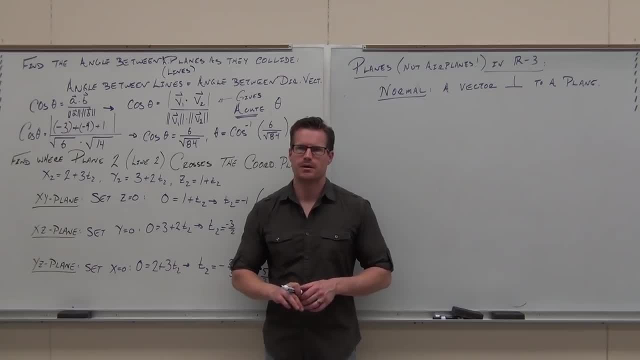 We're going to build the formula and then we'll take our break. How about this? How many normal vectors are there to a plane? Here's a plane. How many normal vectors come off that thing? Infantly many Are those normal vectors all parallel? 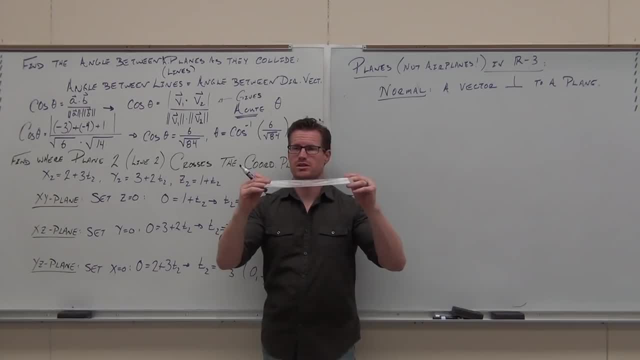 Yes, Which means they're all scalar multiples. So while there are infinitely many normal vectors, they're all scalar multiples. Now we don't need a unit normal, but I'm trying to get you to understand that it doesn't matter. 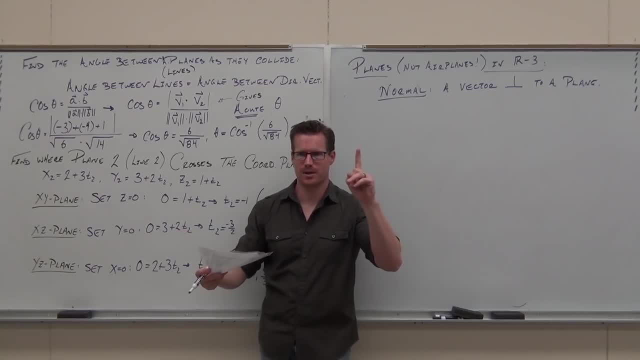 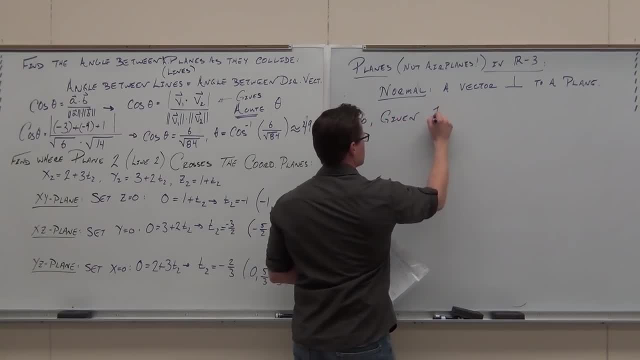 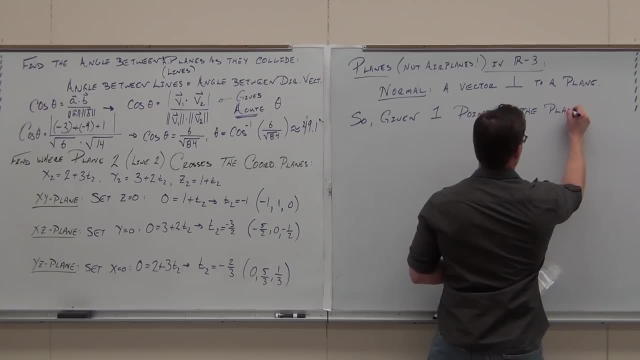 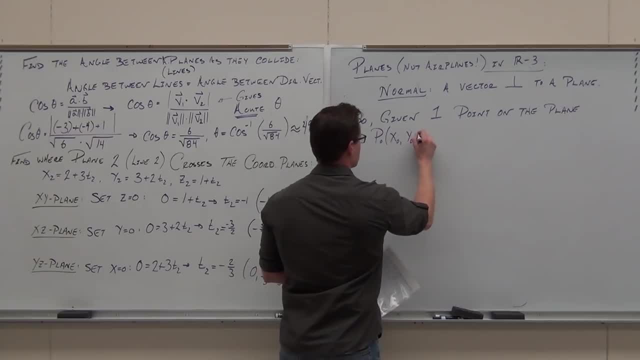 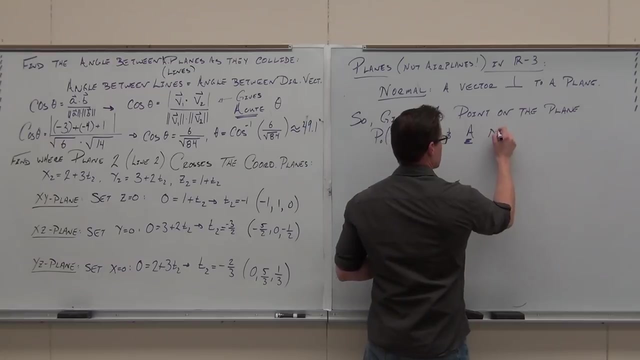 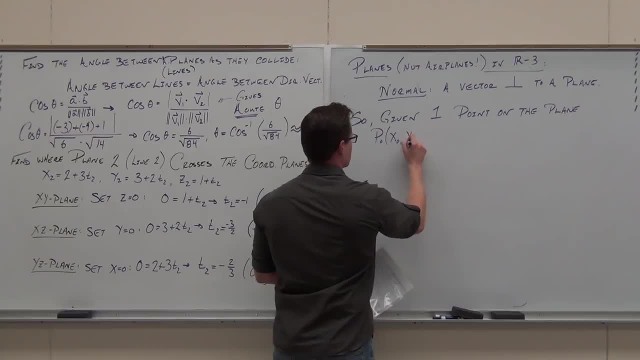 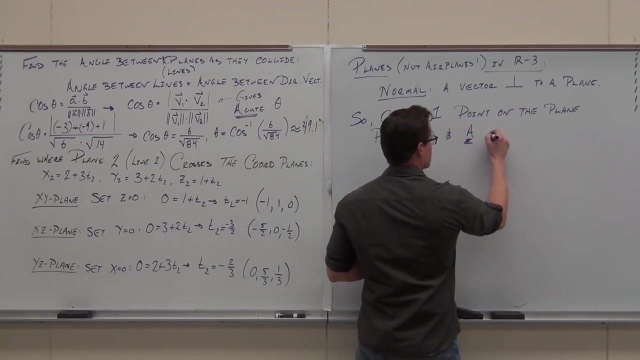 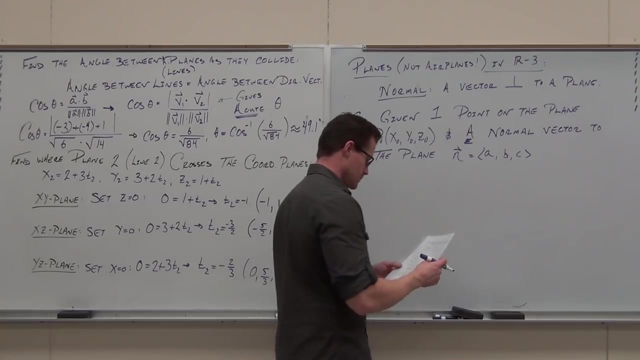 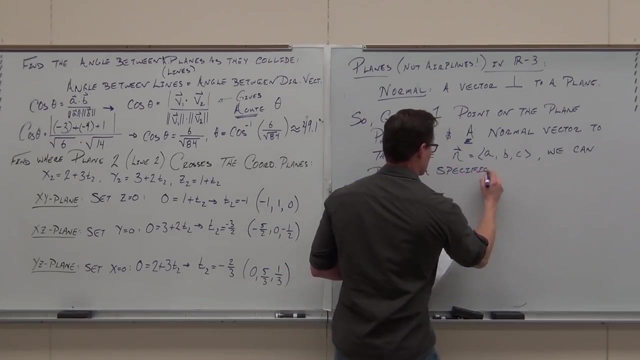 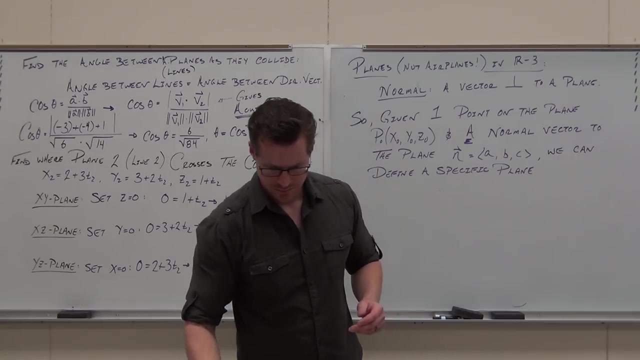 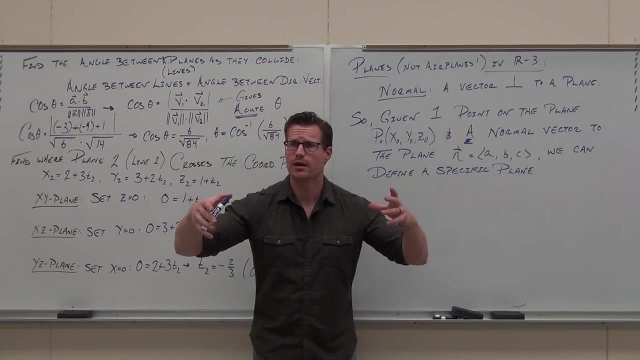 and a- I'm not going to say the, I'm going to say a- a normal vector to the plane. We can define a specific plane. Here's the idea, like a, just a, a rundown of it. 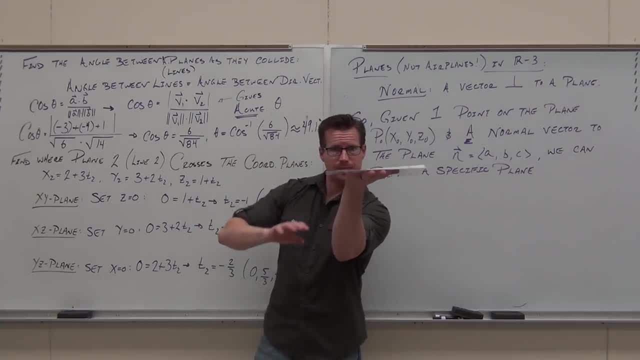 Look, You can't define a plane by the vectors that are in it, because there are infinitely many vectors in that, in that plane. Does that make sense? You go okay. how am I supposed to do that? I don't know. 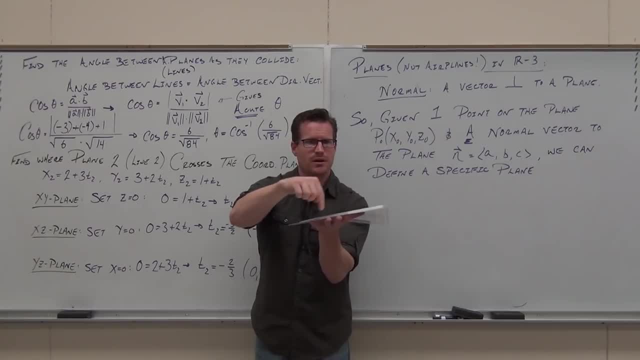 I don't know either. You just can't. There's infinitely many vectors in there, But there's only one normal, only one normal vector, or scalar multiples of that normal vector. Does that make sense? So a point, something that solidifies where a plane's at. 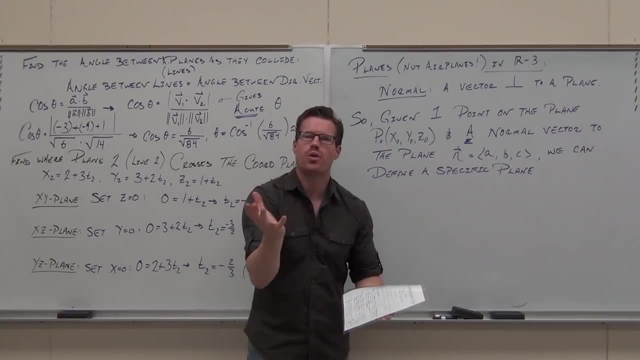 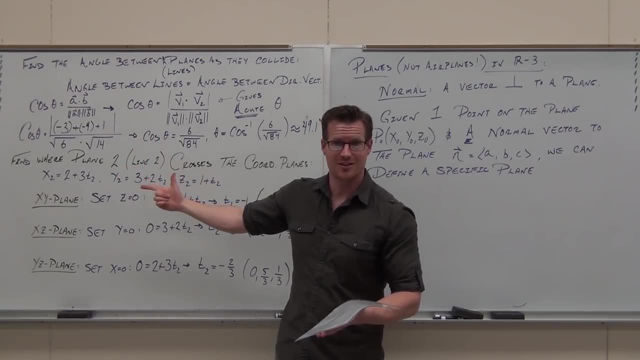 and a normal vector, it's enough to do this stuff. Now, this is what. This is why it gets confusing for you people. Look at what you need for a line. You need a point and a vector. Look what you need for a plane. 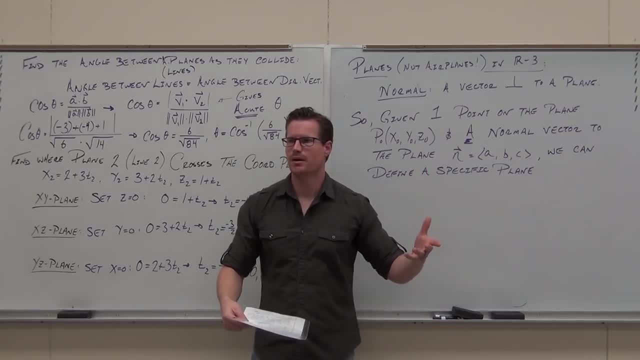 You need a point and a vector. It's the same crap. It's just the type of vector you have which makes all the difference in the world. We're talking about lines. You need a point and a vector in the same direction. If you want a plane, you need a point. 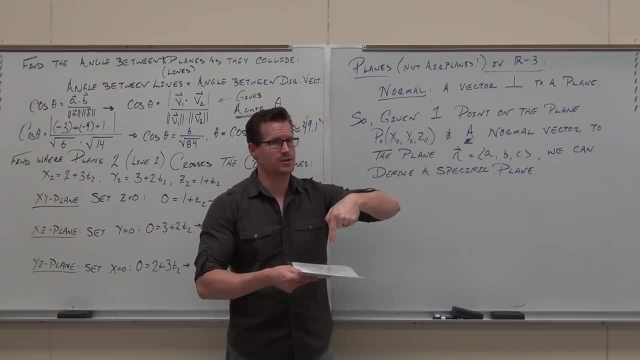 and a vector. that is normal. That's the difference. The formulas look very, very like. You see it? same stuff. it's just the way that we organize that stuff that makes all the difference. you understand, You're going to make some mistakes at it. 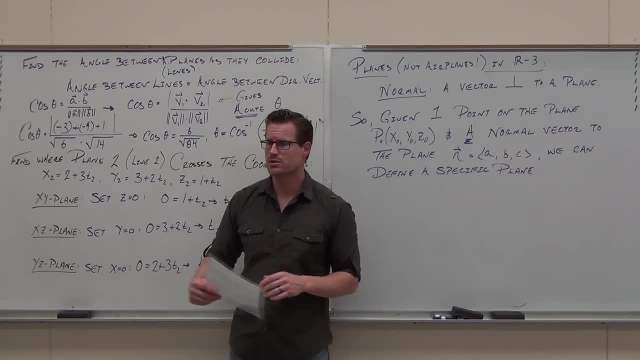 You're going to use the formula for a plane when I want a line and you're going to use the formula for a line when I want a plane, sometimes Just when it happens go, oh crap, I can't do that. 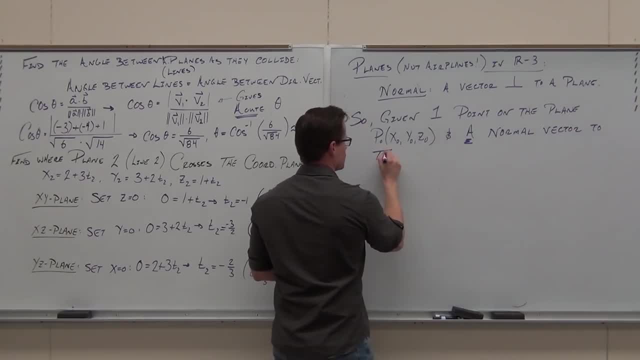 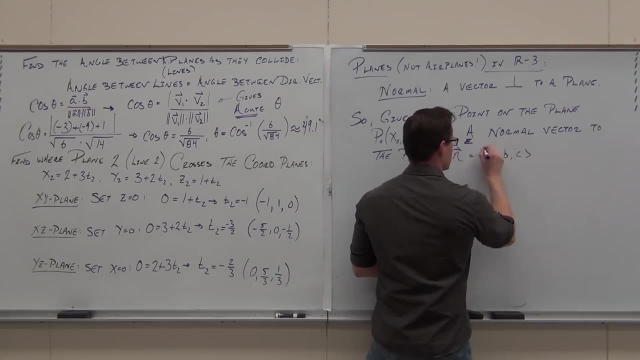 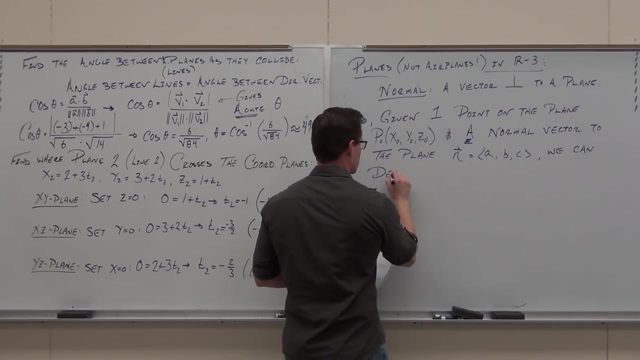 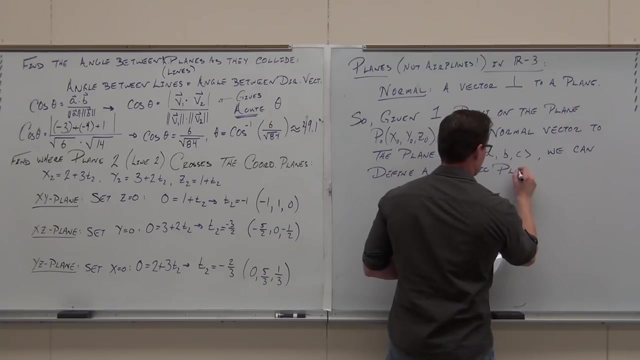 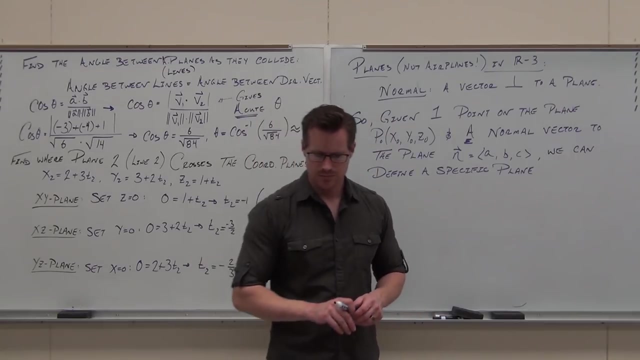 So we just do one more ellipse. Here's one log of One log of One log of Two log of One log of One log of we can define a specific plane. Here's the idea, like just a rundown of it. 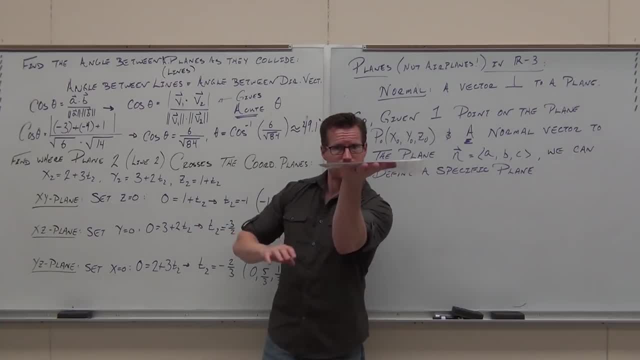 Look, you can't define a plane by the vectors that are in it, because there are infinitely many vectors in that plane. Does that make sense? You go, okay, how am I supposed to do that? I don't know. I don't know either. 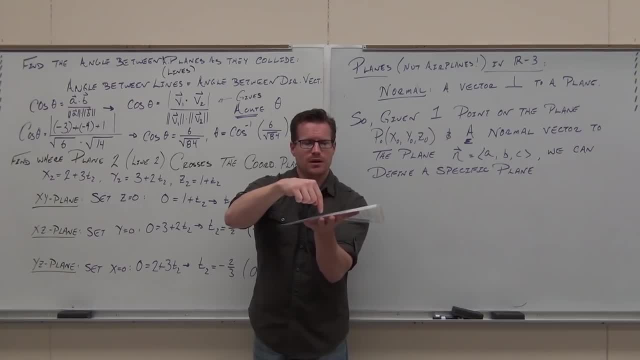 You just can't. There's infinitely many vectors in there, But there's only one normal, Only one normal plane. There's only one normal vector or scalar multiples of that normal vector. Does that make sense? So a point, something that solidifies where a plane's at. 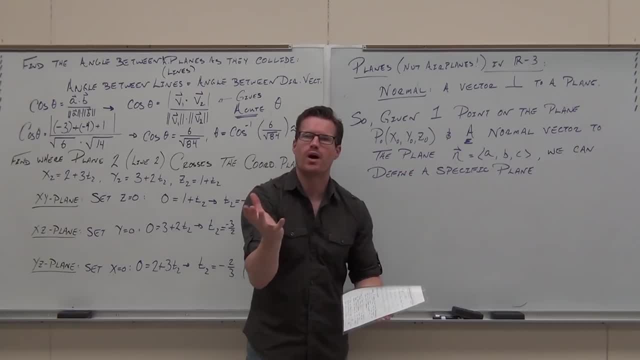 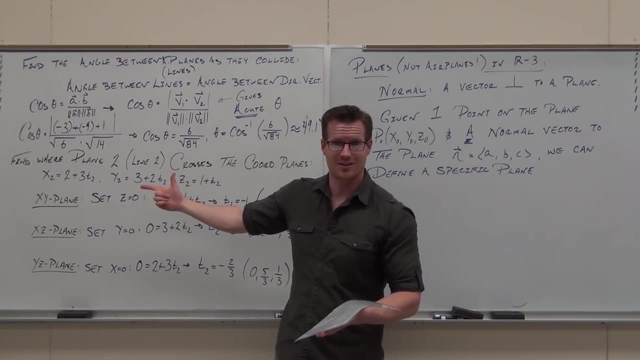 and a normal vector. it's enough to do this stuff. Now, this is why it gets confusing for you people. Look at what you need for a line: You need a point and a vector. Look what you need for a plane: You need a point and a vector. 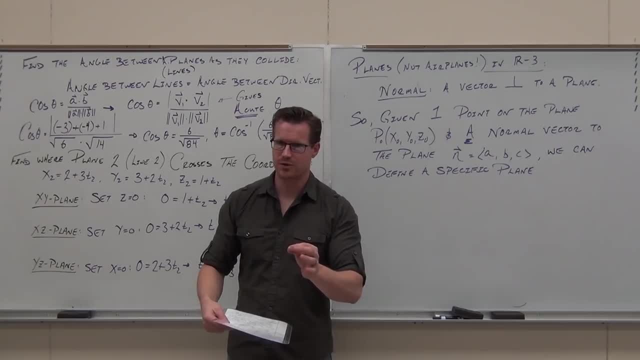 It's the same crap. It's just the type of vector you have which makes all the difference in the world. We're talking about lines. You need a point. You need a point and a vector in the same direction. If you want a plane, you need a point and a vector. that is normal. 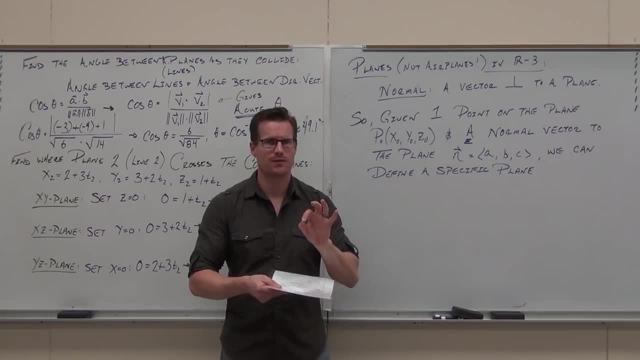 That's the difference. The formulas look very, very similar. You see it: same stuff. It's just the way that we organize that stuff that makes all the difference. You understand, You're going to make some mistakes at it. You're going to use the formula for a plane when I want a line. 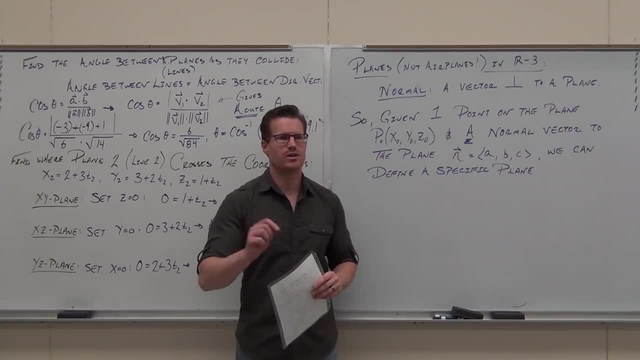 and you're going to use the formula for a line when I want a plane, sometimes Just when it happens: go, oh crap, I can't do that. Think it through very carefully. What am I actually doing? Do I want to find the equation for a line or for a plane? 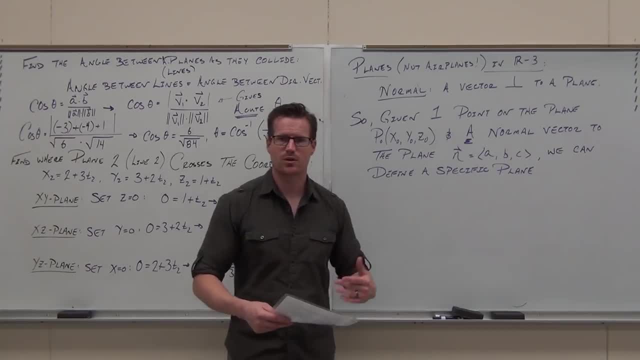 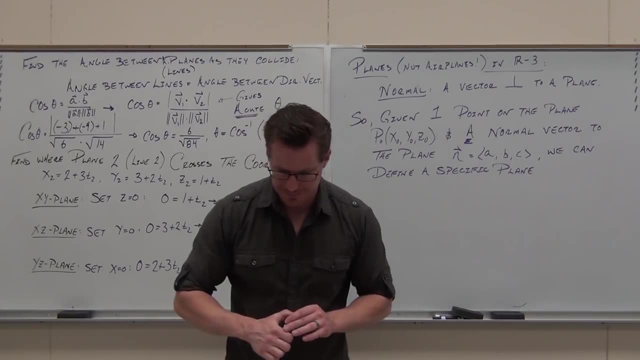 and do the appropriate thing with that. Does that make sense? So let's build the equation. We'll run through a very quick example. It's not going to be hard. You just need to use the appropriate thing in the appropriate spot. So we're going to take any vector in the plane. 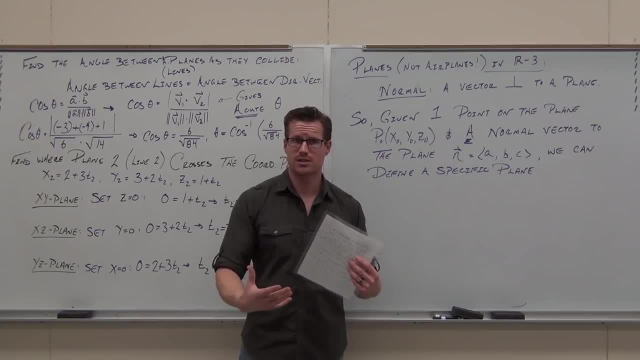 Think it through very carefully. What am I actually doing? Do I want to find the equation for a line or for a plane and do the appropriate thing with that? Does that make sense? So let's build the equation. We'll run through a very quick example. 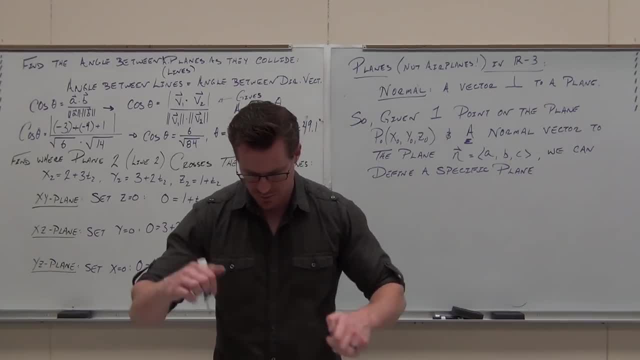 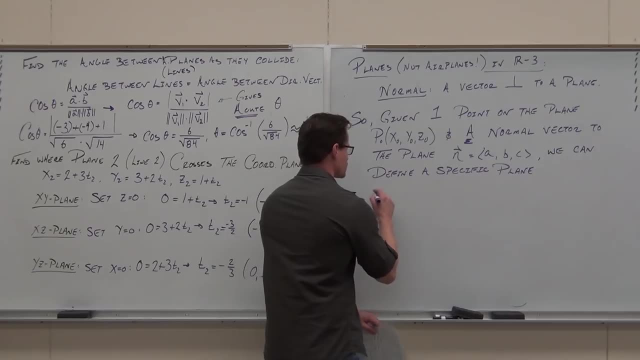 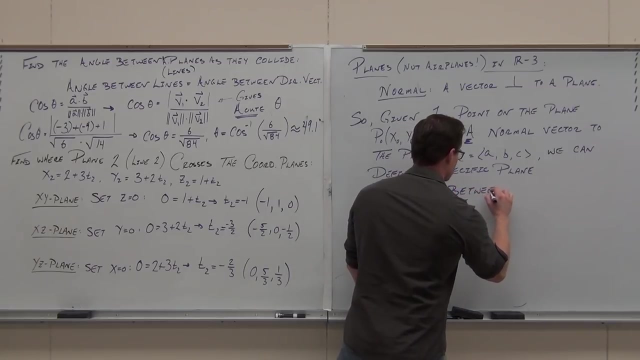 It's not going to be hard. You just need to use the appropriate thing in the appropriate spot. So we're going to take any vector in the plane. It's going to look a lot like the line, so I'm going to move a lot quicker through it. 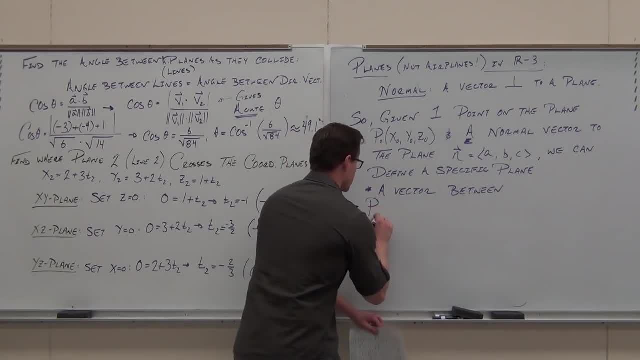 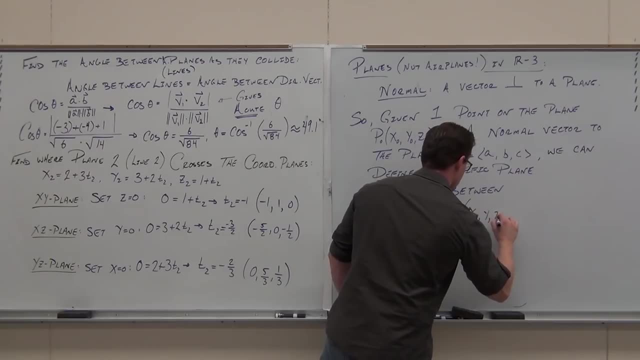 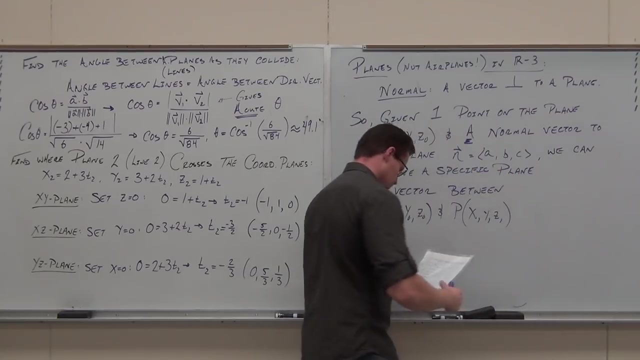 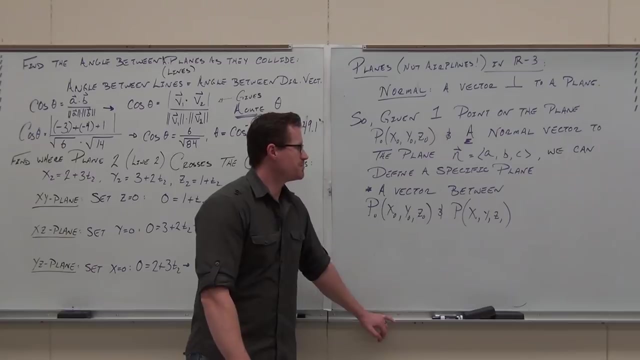 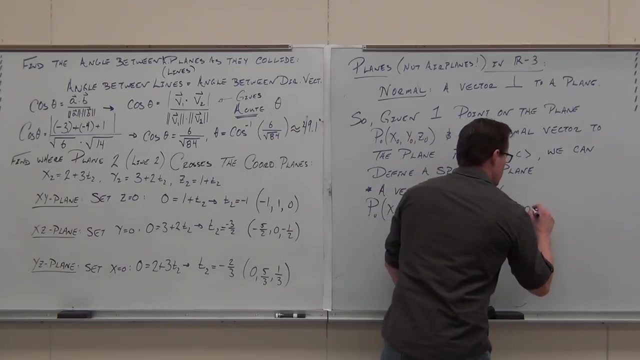 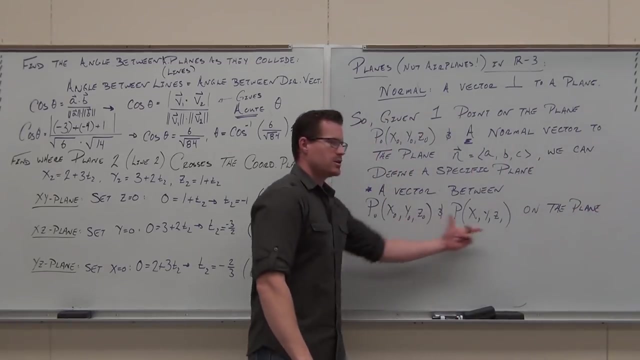 but it's going to look very, very similar. So here you go. Let's start with a vector between two points. These points are going to be on the plane, So a vector between two points. Can you give me the vector between two points? 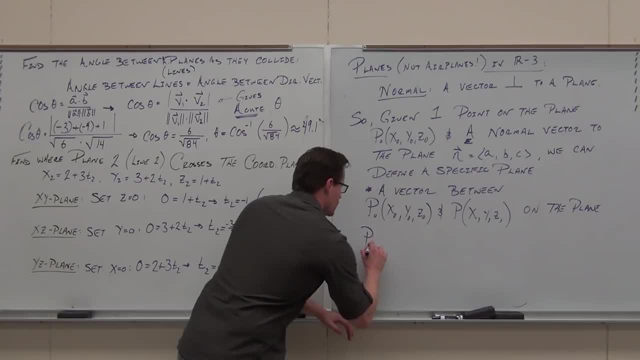 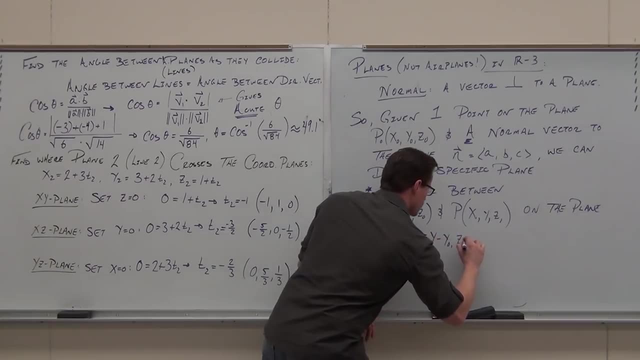 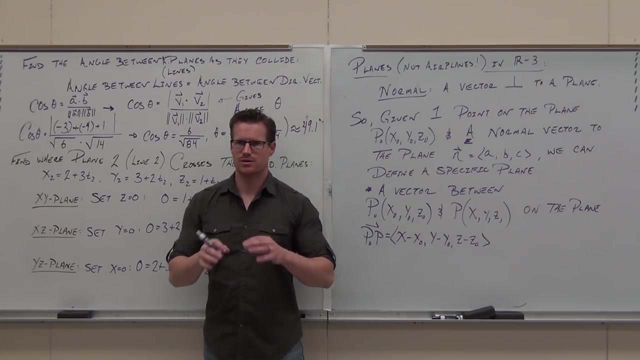 Of course, We've already done that. So that vector is the same thing we started with You guys. all right with what I'm talking about. So this is two points in the plane, Hey, you find the vector. This vector lies in that plane, lies on the plane. 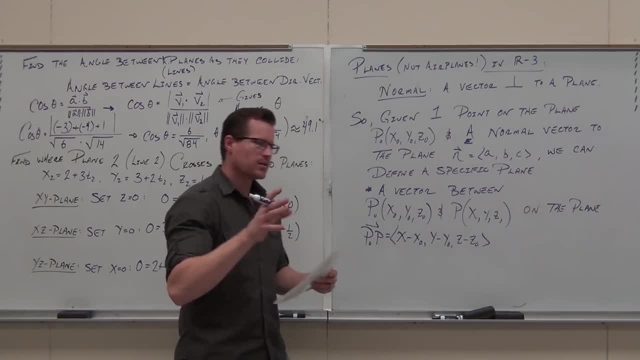 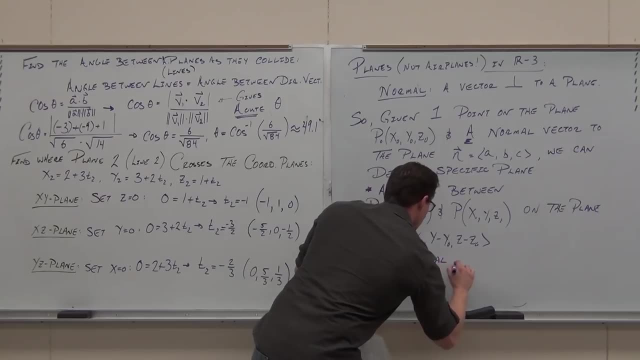 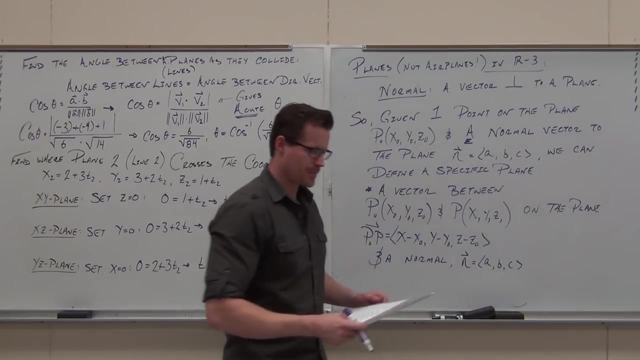 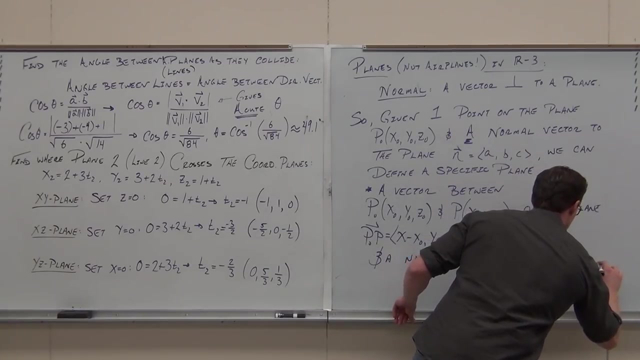 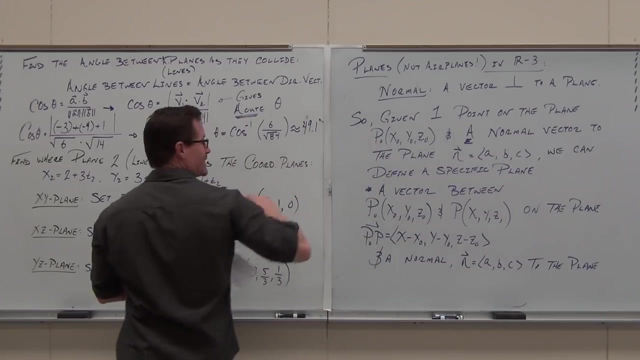 Head nod if you're okay with that one. Now let's continue. We go right. Let's also take a normal To the plane. Here's the match You're actually going to. I hope that you like this. The proof part is kind of interesting. 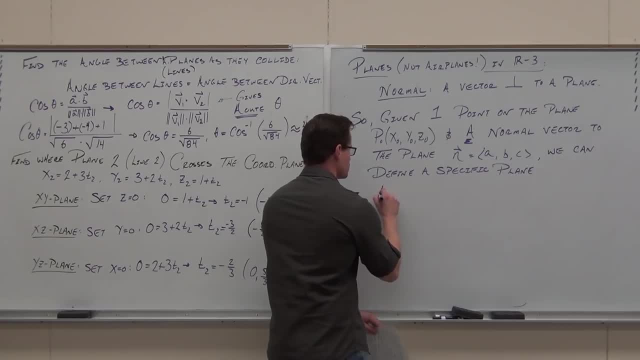 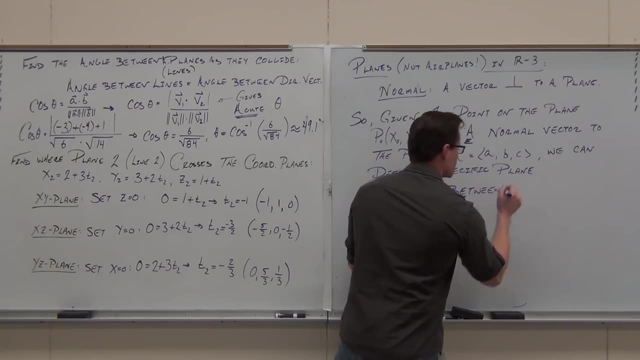 We just want it to be small this time. That's a point we're going to set. It's going to look a lot like the line, so I'm going to move a lot quicker through it, but it's going to look very, very similar. 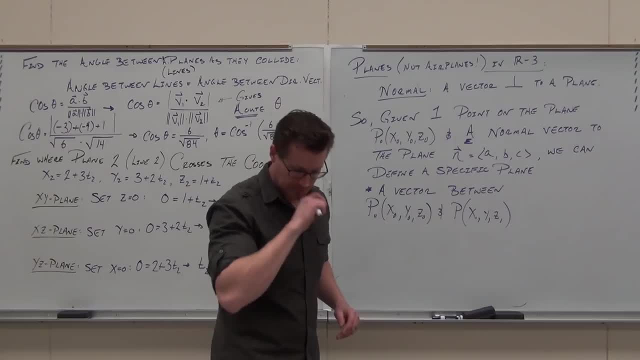 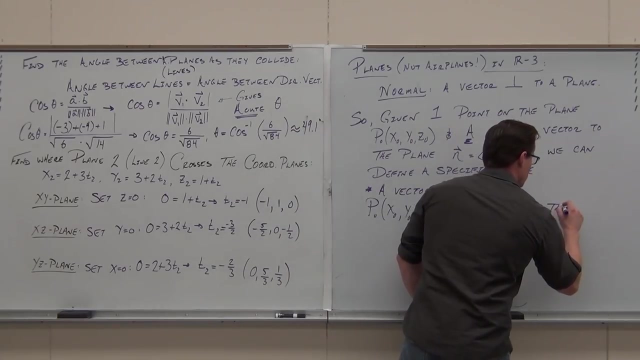 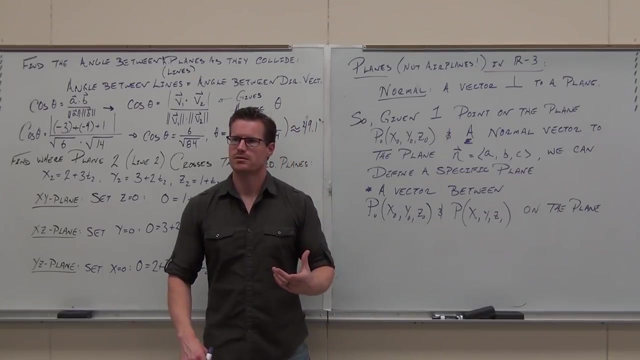 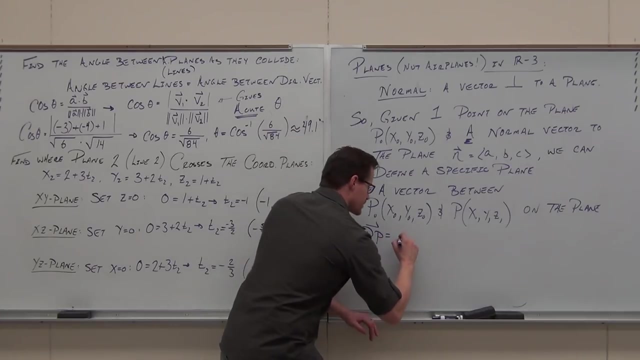 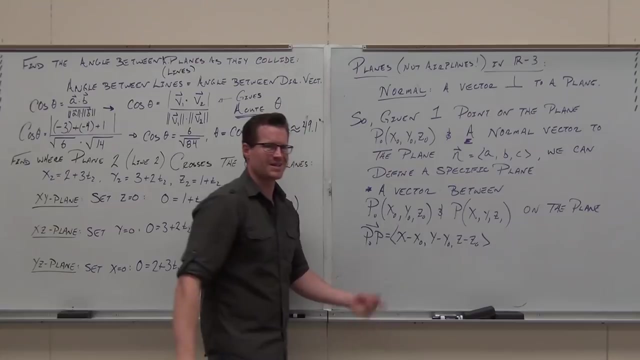 Let's start with a vector between two points. These points are going to be on the plane, So a vector between two points on the plane. Can you give me the vector between two points? Of course We've already done that, So that vector is the same thing we started with. 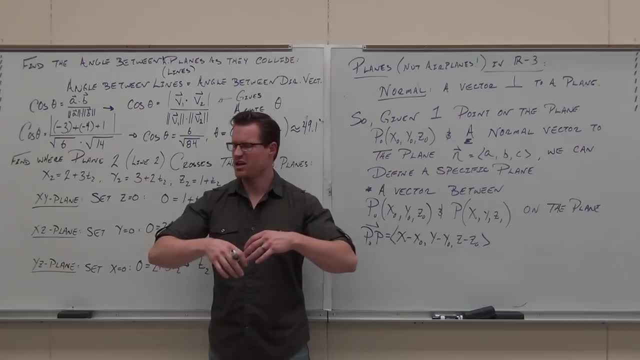 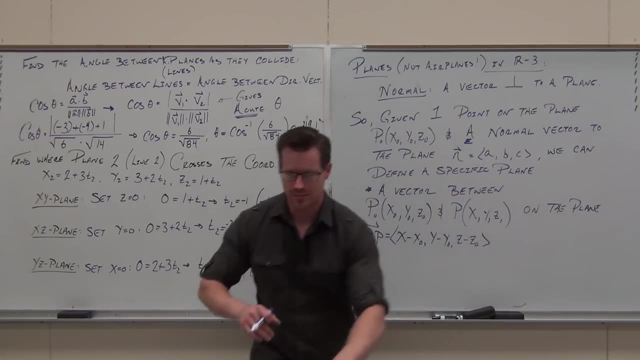 You guys all right with what I'm talking about. So there's two points on the plane. Hey, you find the vector. This vector lies in that plane, lies on the plane Head. nod, if you're OK with that one. Now let's continue. 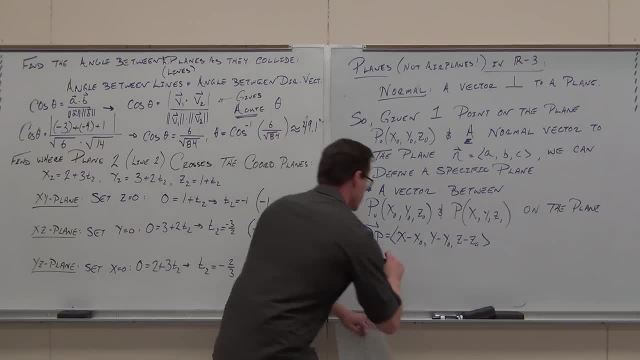 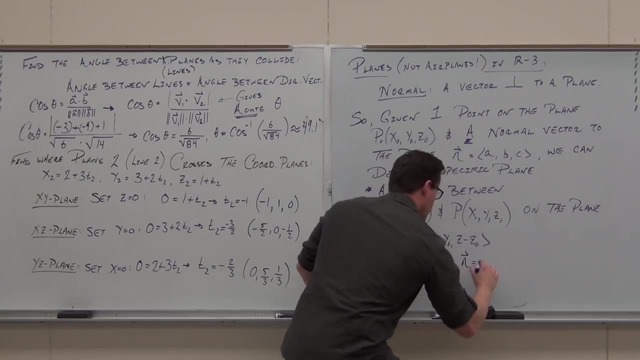 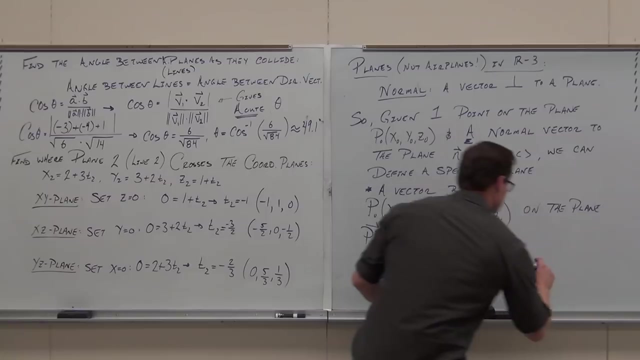 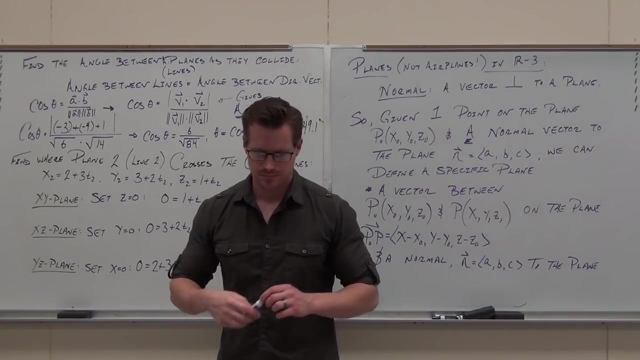 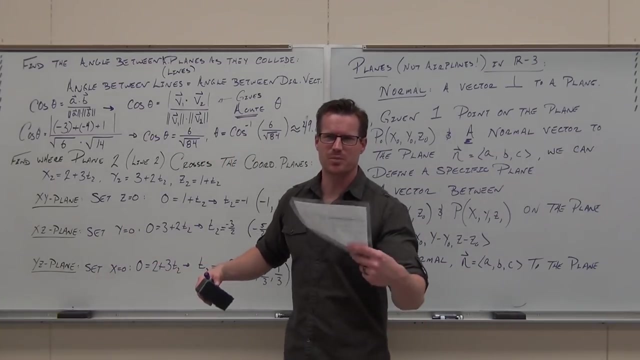 We go: all right, let's also take a normal. Let's take a normal vector to the plane. Here's the match You're actually going to. I hope that you like this, that the proof part's kind of interesting Form part, working with it. OK. 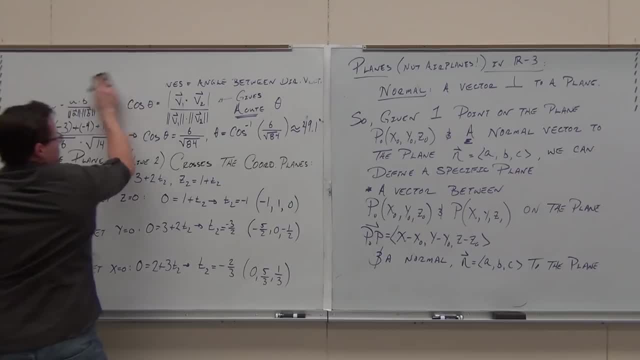 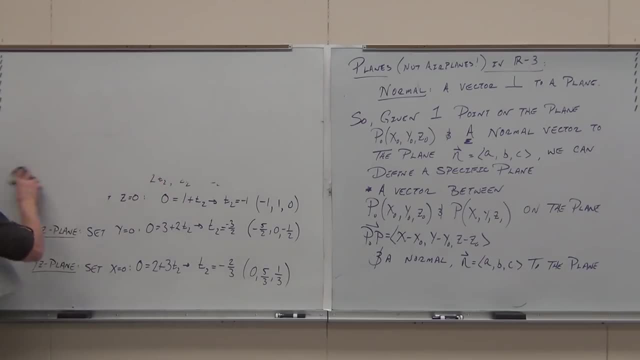 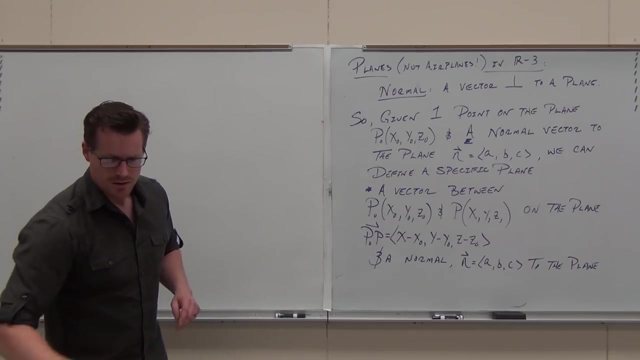 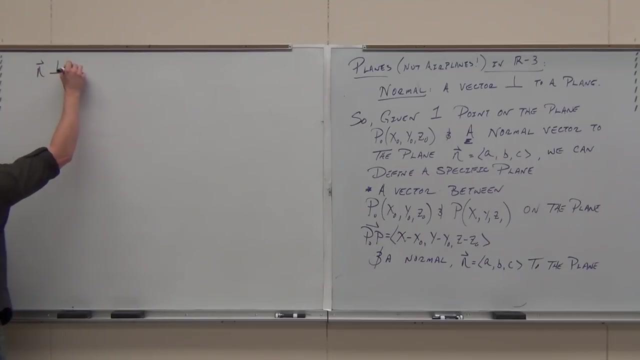 The proof part's kind of interesting. It's kind of cool to me, but that's super dorky. so you know, cool is relative, I guess. All right, True or false. True or false N, a normal vector. 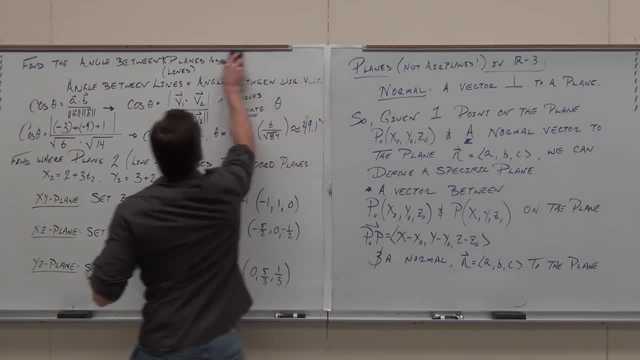 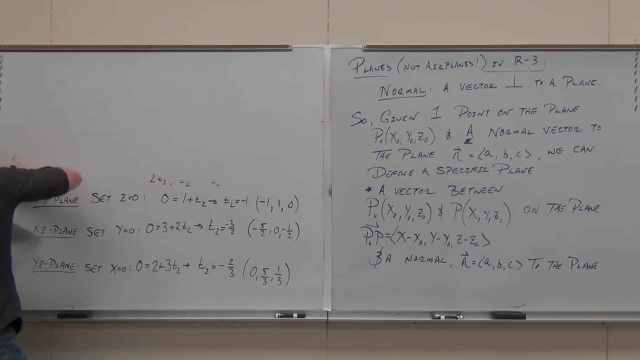 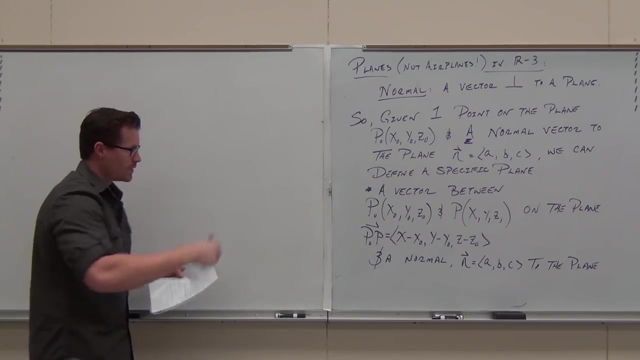 Forming part working with it. okay, The proof part is kind of cool to me. Well, that's super dorky. so you know, cool is relative, I guess. All right, True or false. True or false. 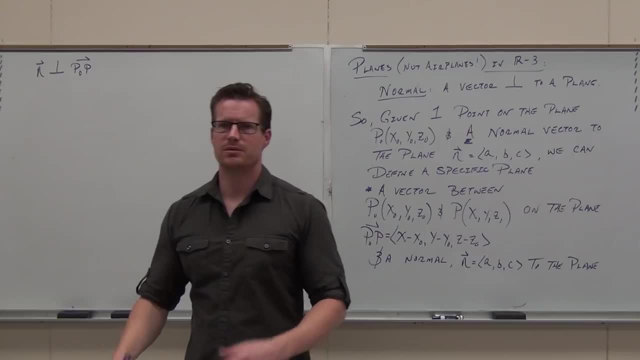 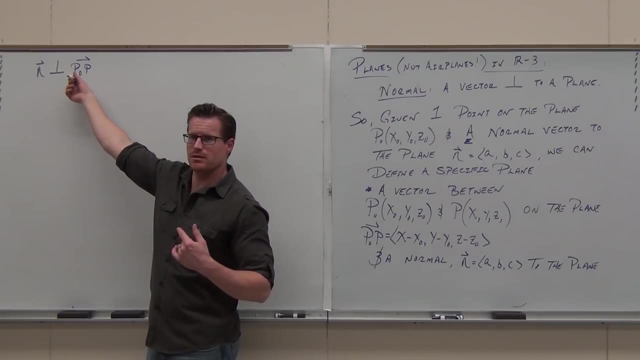 N. the normal vector has got to be perpendicular to P0, to P, to P. True or false? True, Is this in the plane? Yes, Yeah, that's why we built it that way. Is this perpendicular to the plane? 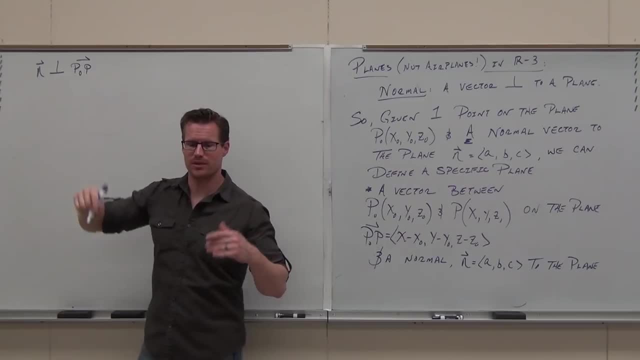 Yes, Yes. Therefore, it's got to be perpendicular to every vector in that plane. Here's the magic. You know it Because this is in the plane. ends the magic. So you know it Because this is in the plane. ends the magic. 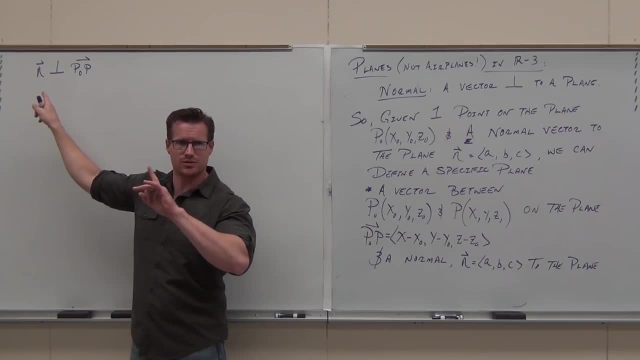 It's normal, it's perpendicular to this, because that's in the plane And that's your. you're actually with me. I can write that down. How about this one? What do you know about two vectors that are perpendicular? What do you know about that? 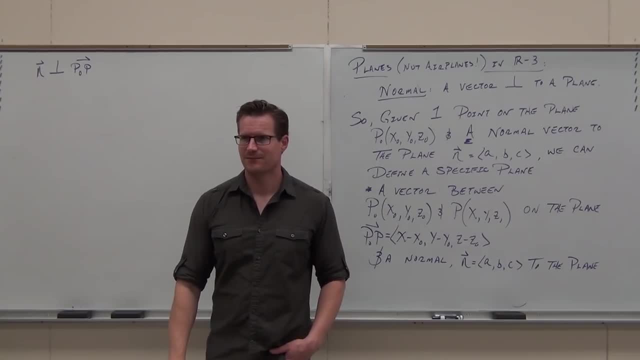 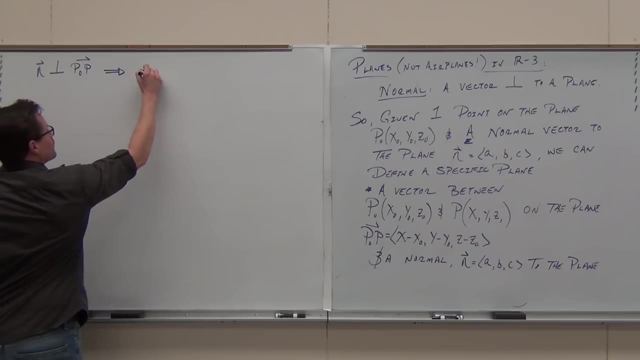 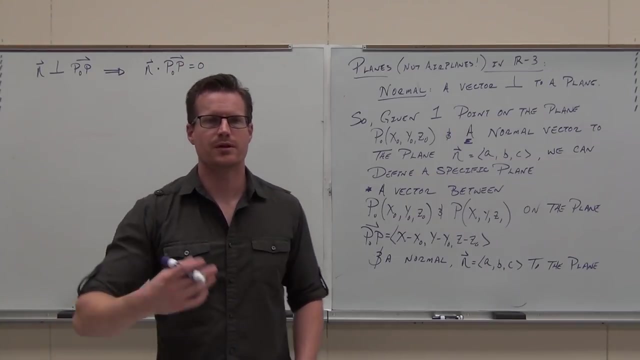 How do you test for perpendicular vectors? They're which product? Dot product. They're dot product. Which way do I want to do it? Yeah, If two vectors are perpendicular, orthogonal, their dot products have to be zero. That's it. 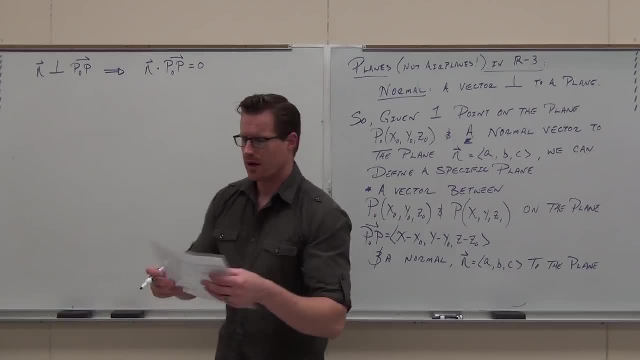 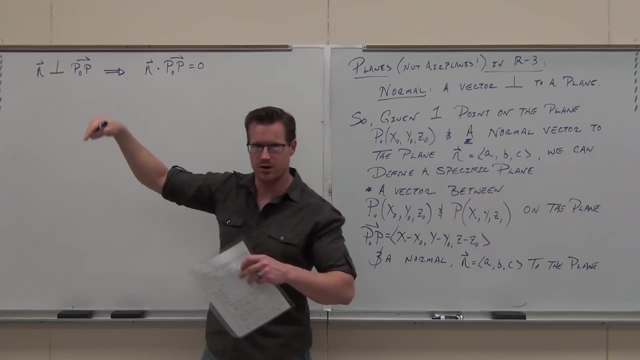 That's literally, like essentially it. Remember that this happened if, and only if, these things were perpendicular. That was the only way it happened. So if we have perpendicular, we have to have the dot product equal to zero. But I have that vector and I have that vector. 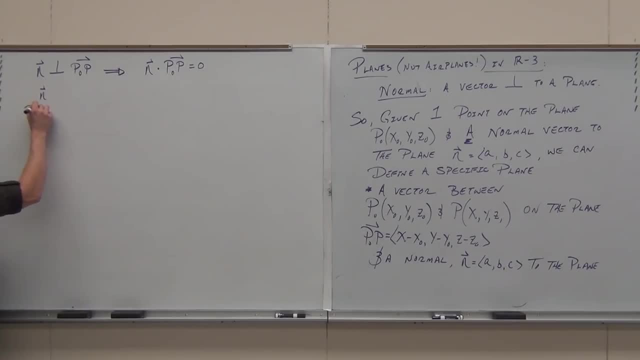 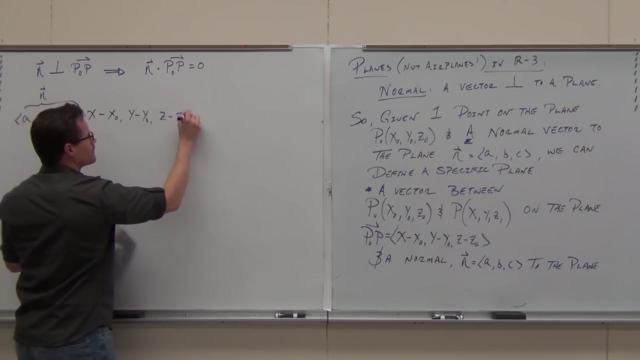 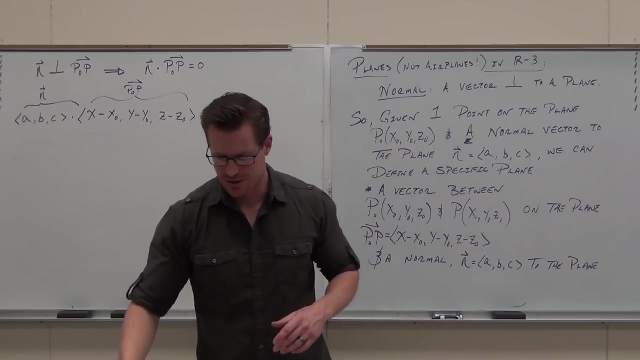 This vector, Dot with this vector. It's got to be zero. It's got to be Here's n, Here's this. I know they're orthogonal. I know the dot product's got to be zero. That's pretty cool. 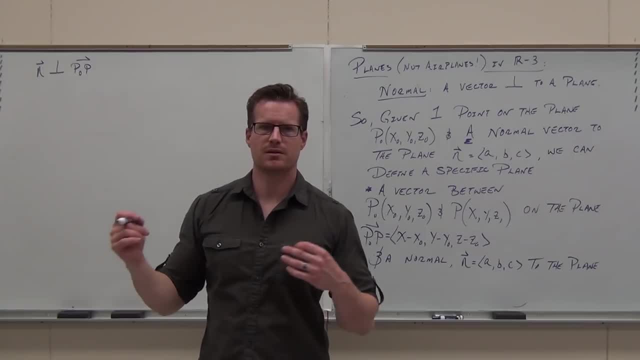 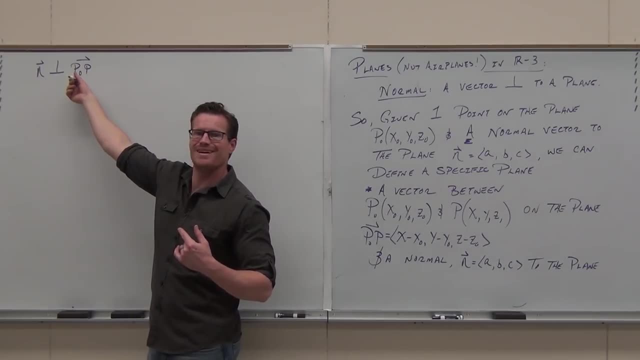 A normal vector has got to be perpendicular to p0 to p, True or false? True or false? Is this in the plane? Yes, Yeah, so we built it that way. Is this perpendicular to the plane? Yes, Therefore, it's got to be perpendicular to every vector in that plane. 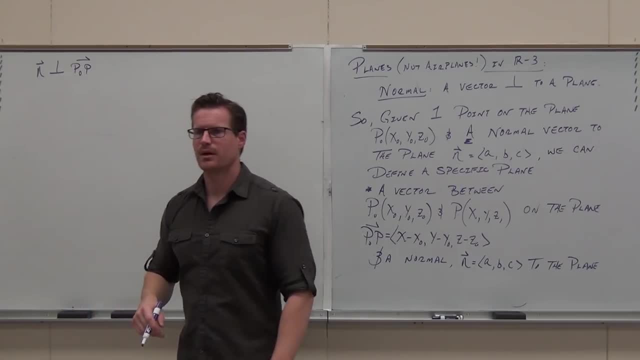 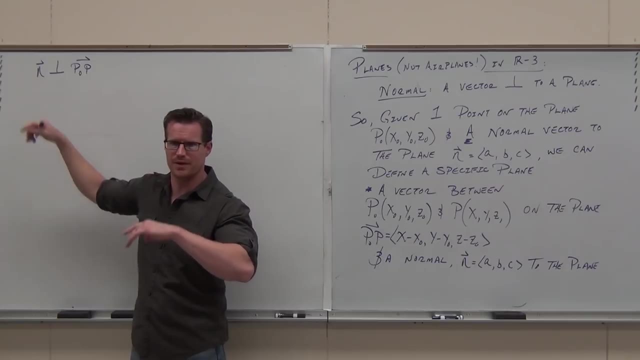 Now, here's the magic. You know it Because this is in the plane and it's a normal, it's perpendicular to this, because that's in the plane And that's your. you're actually with me. I can write that down. 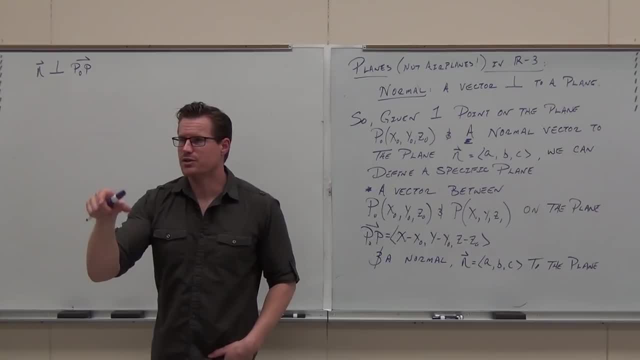 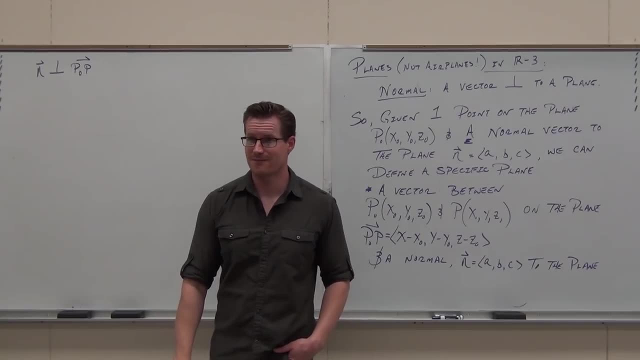 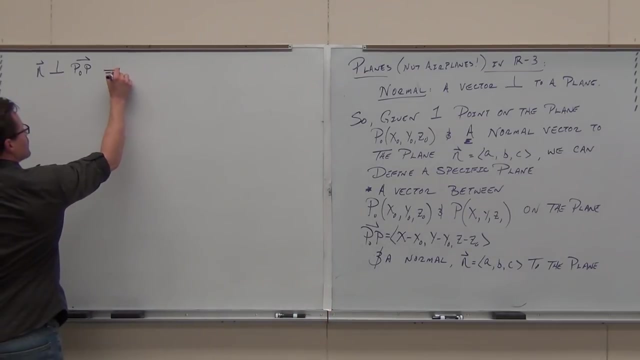 How about this one? What do you know about two vectors that are perpendicular? What do you know about that? How do you test for perpendicular vectors? They're which product? Dot product. They're dot product. Which way do I want to do it? 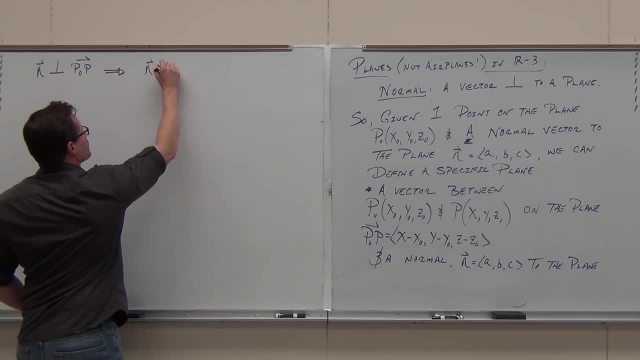 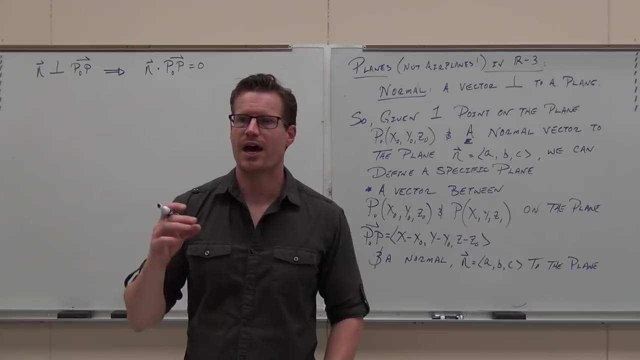 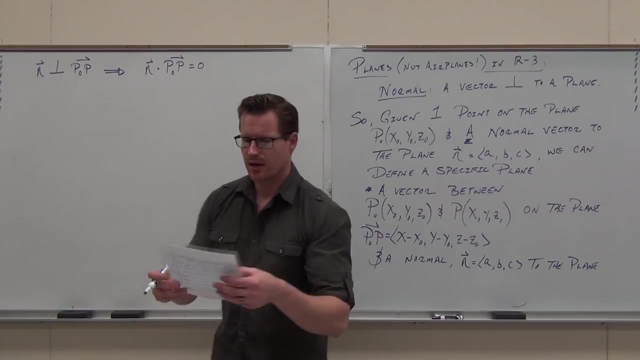 Yeah, Do that. Yeah, Yeah, Yeah, Yeah, Yeah. If two vectors are perpendicular, orthogonal, their dot products have to be zero. That's it. That's literally, like essentially it. Remember that this happened if, and only if, these things were perpendicular. 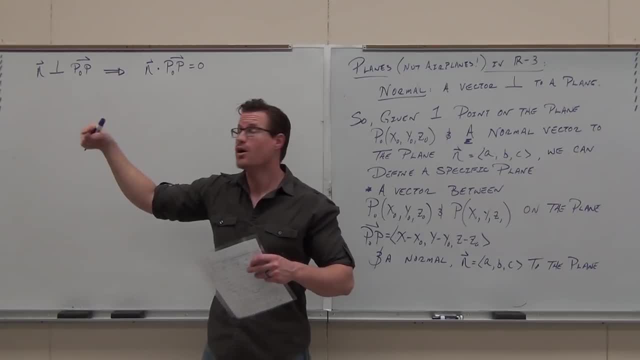 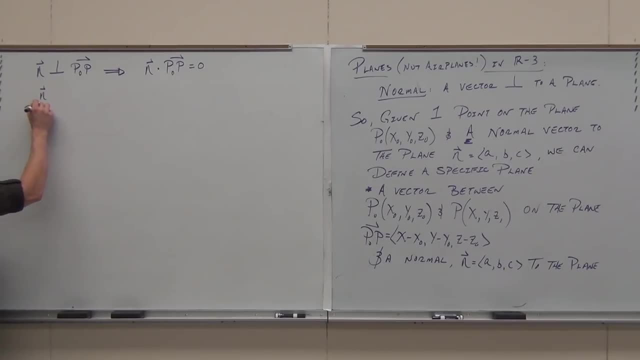 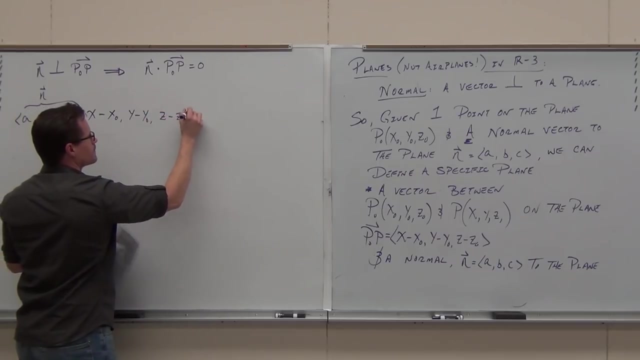 That was the only way it happened. So if we have perpendicular, we have to have the dot product equal to zero. But I have that vector and I have that vector, This vector. Dot with this vector has got to be zero. It's got to be. 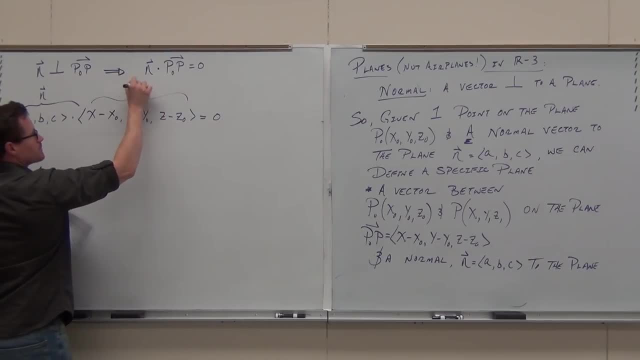 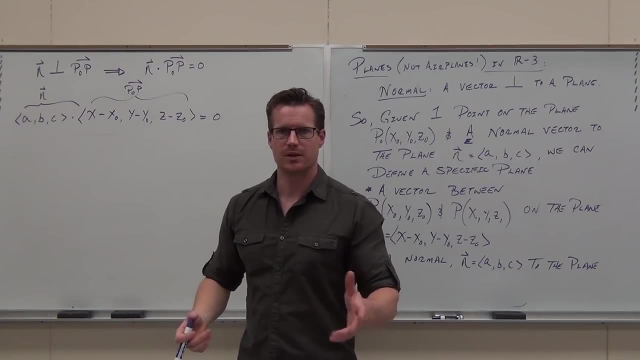 Here's n, Here's this. I know they're orthogonal. I know the dot product's got to be zero. That's pretty cool. Can we do some work with it? Let's see X component, Y component, Z component. 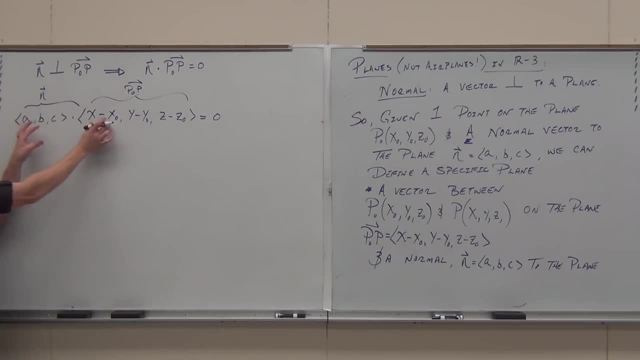 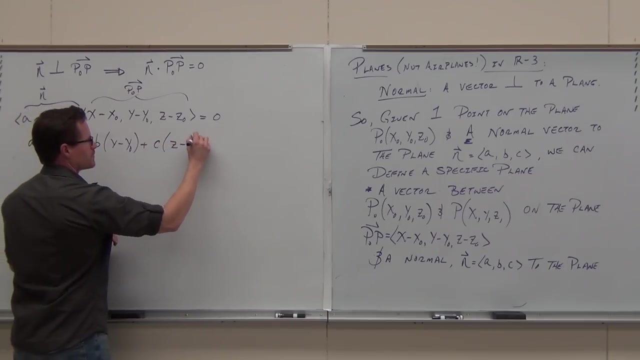 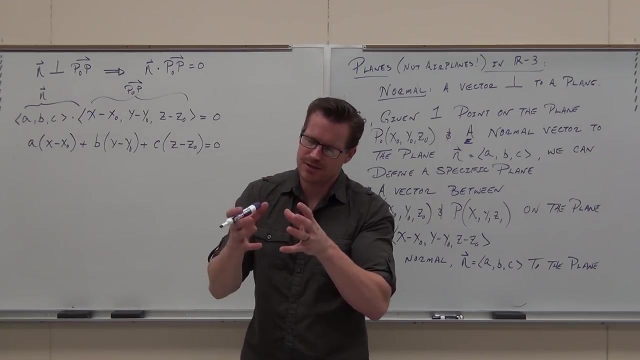 X component, Y component, Z component. They're just vectors. I can dot product them. So if I do, We get that. Follow along with me. Do you see that? we get the scalar function? It has variables in it, So we're going to call it a function. 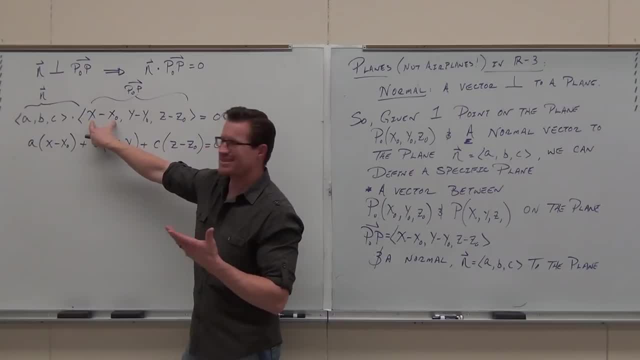 But it's a scalar function. It has number. That's just a number. There, No vector Number. Y components. Multiply them together. Add That's what it is. Take X, Take Y, Take Z. Multiply the components. 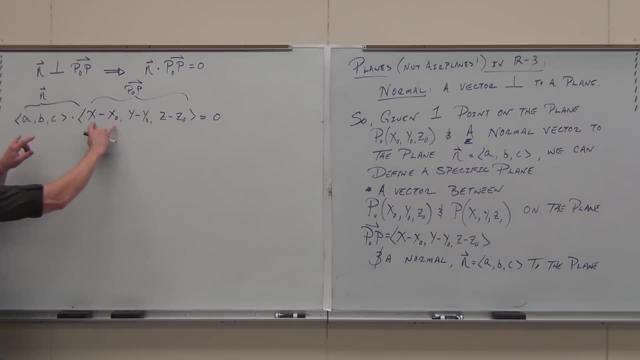 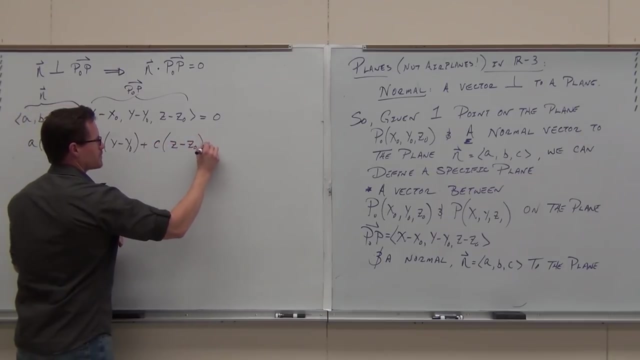 Can we do some work with it? Let's see X component, Y component, Z component, X component, Y component, Z component. They're just vectors. I can dot, product them. So if I do, We get that. 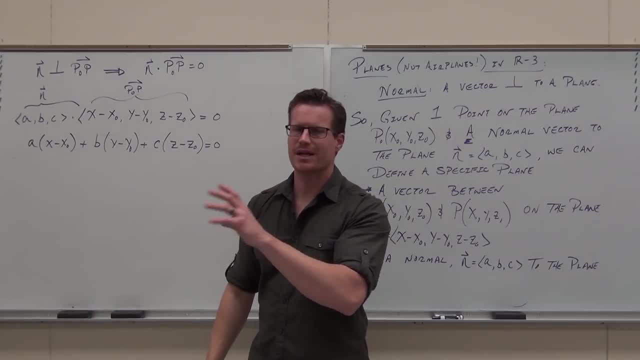 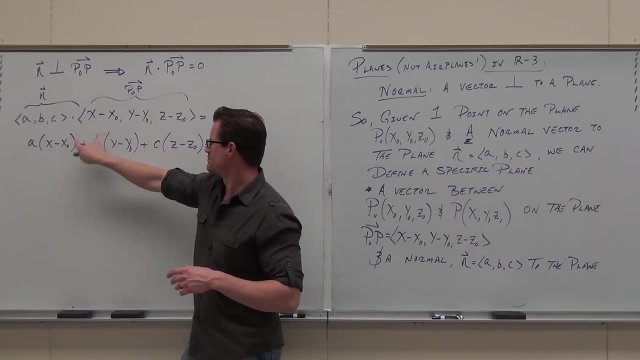 Follow along with me. Do you see that we get the scalar function? It has variables in it, So we're going to call it a function, But it's a scalar function. It has number. That's just a number. There, No vector. 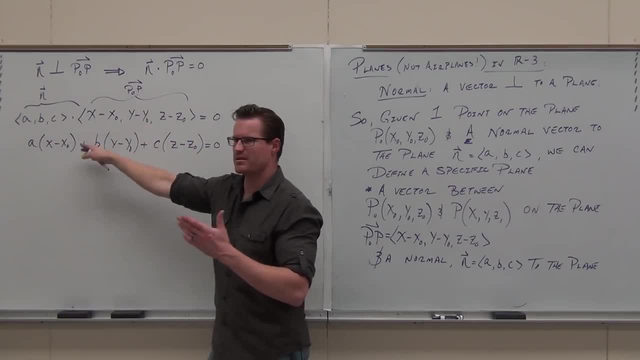 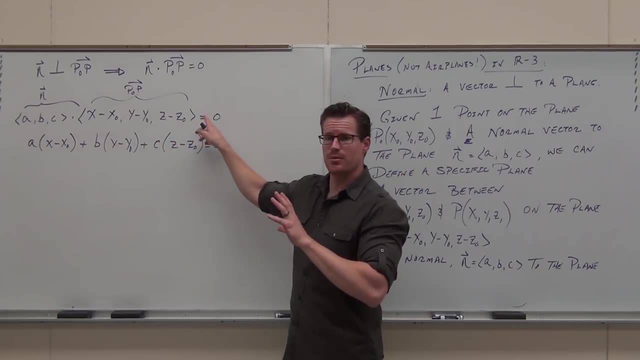 Number Y components. multiply them together, add. That's what it is. Take X, take Y, take Z. Multiply the components, add them together. It's just we know that that dot product has to be equal. Why Everyone in class right now? why do we know that dot product has to be equal to zero? 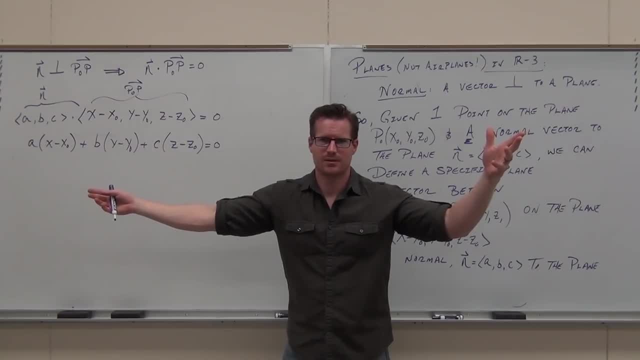 That's good enough for me, man. 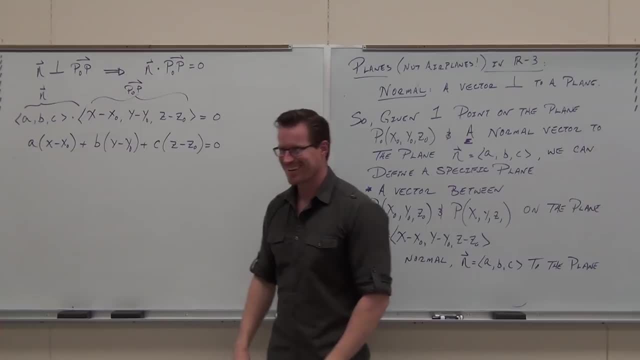 They're orthogonal. Dot product zero: Done Orthogonal, Sweet, Cut That. right. there is the standard form equation of a plane. That's literally it. Look at it. If I give you a point, could you plug in the point? 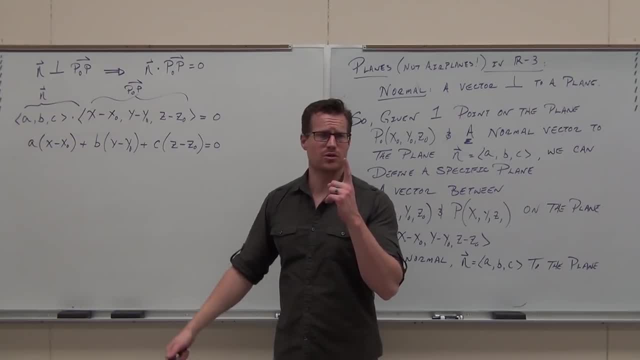 If I give you a normal vector, could you plug in the normal vector? Yeah, That's it Now what I said: standard, Do you remember? like the Y minus Y1 equals M, X minus X1 thing? Do you remember that? 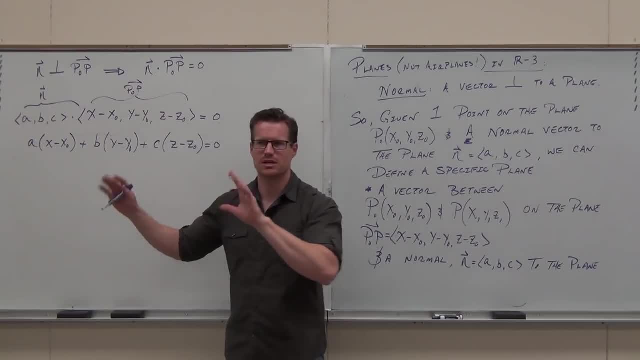 You always start there with a point and a slope. You always start there with a point and a vector, same stuff. And then you like, distribute and you add to one side and you get it into the Y, the slope intercept form. Do you remember that? 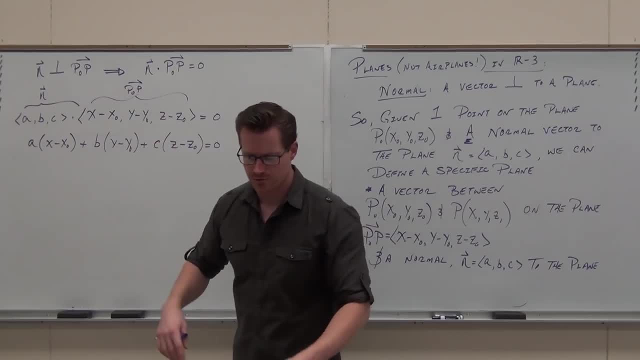 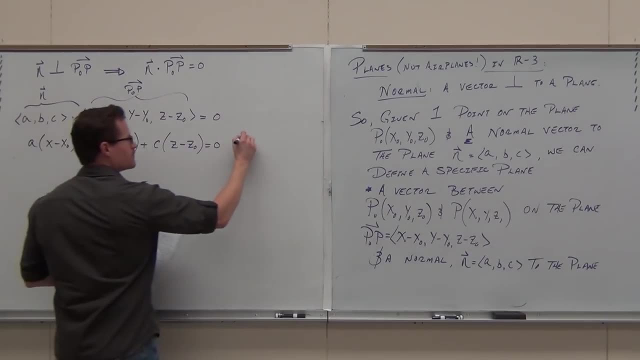 We do the same thing here, So this is called the standard form. It's what we use to get to the next thing. I was a little bad. They say health class. all right, It means standard form, so don't whatever. 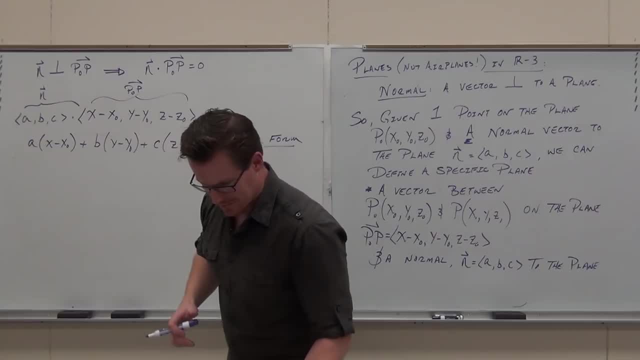 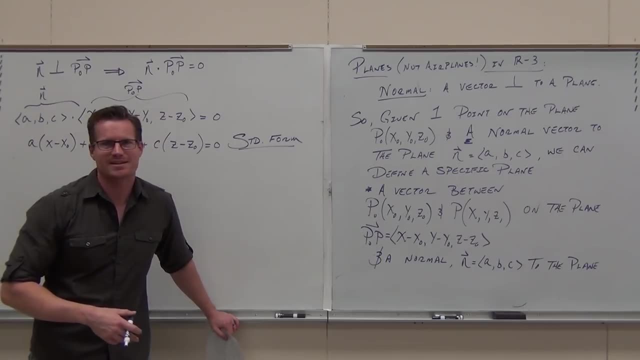 Can I get a little clap? Don't answer that. that's wrong. Sorry, that's a bad joke. I'm ashamed. I'm a little ashamed of that one. That was funny. That was funny. That does not get better. 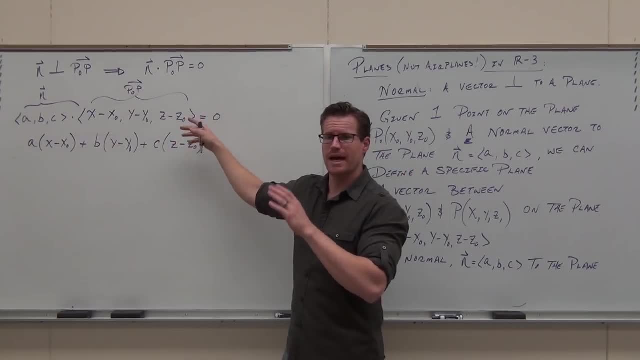 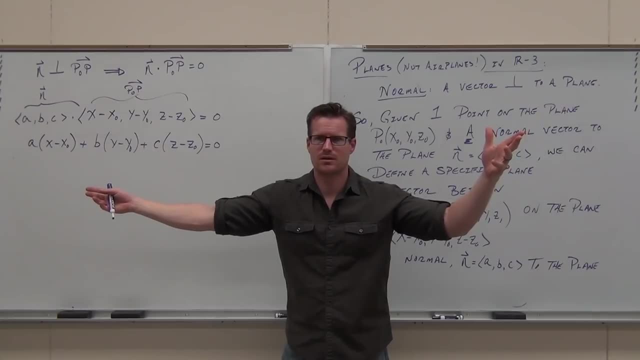 Add them together. It's just we know that that dot product has to be equal. Why Everyone in class right now? Why do we know that dot product has to be equal to zero? Cosines? All I heard was orthogonal. OK. 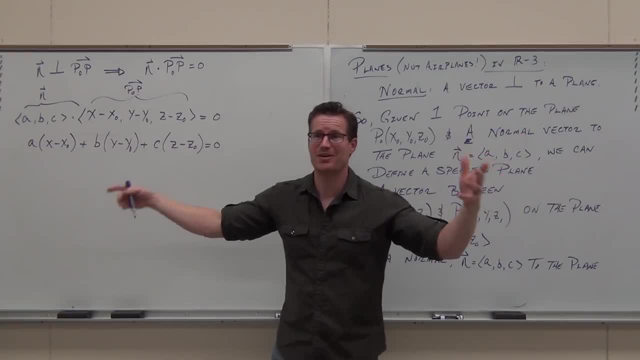 That's good enough for me, man, They're orthogonal. They're orthogonal Dot product Zero Done Orthogonal Sweet. Got it That right. there is the standard form equation of a plane. That's literally it. Look at it. 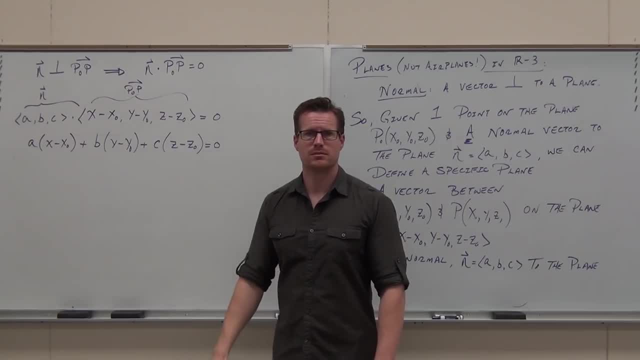 If I give you a point, could you plug in the point. If I give you a normal vector, could you plug in the normal vector? Yeah, That's it Now what I said. standard formula is this: Do you remember like the Y minus Y1 equals M, X minus Y2?? 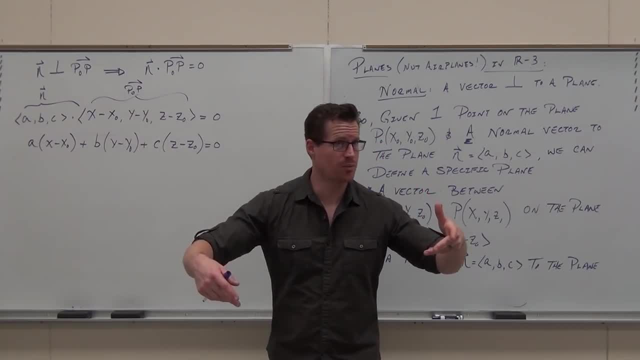 M minus X1 thing. Remember that You always start there with a point and a slope. You always start here with a point and a vector, Same stuff, And then you like, distribute and you add to one side and you get it into the slope. 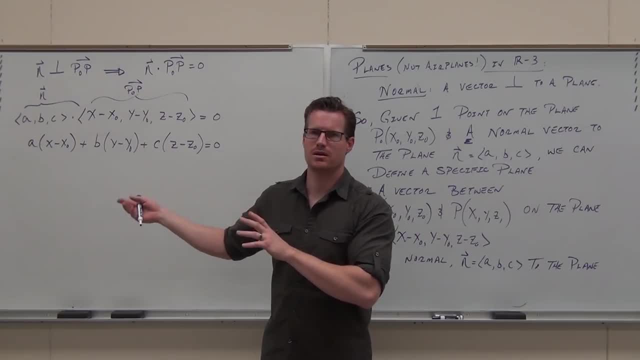 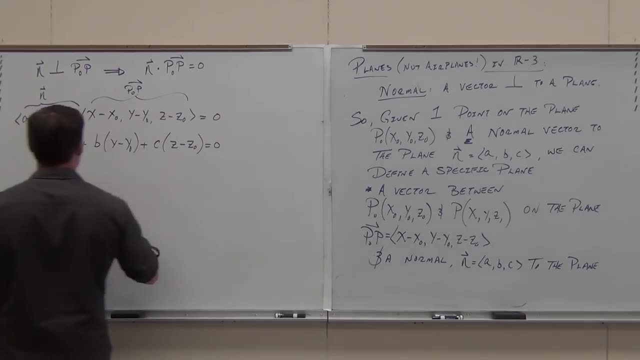 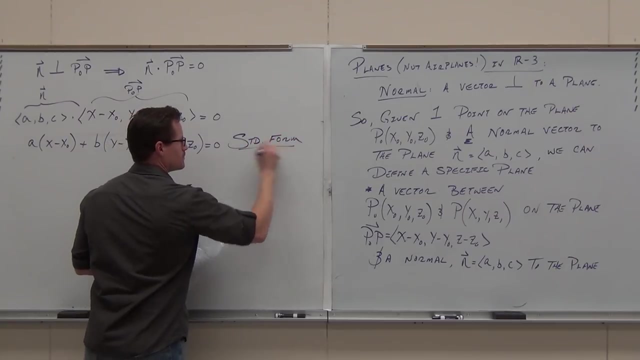 intercept form. Remember that We do the same thing here, So this is called the standard form. It's what we use to get to the next thing. That looks a little bad. They say it in health class. alright, It means standard form. 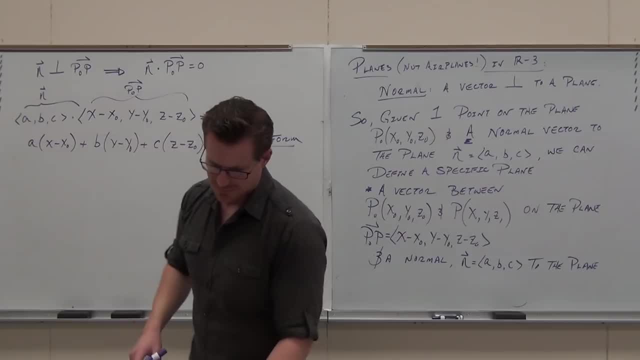 So don't whatever. Can I give you a little clap? Don't answer that. That's wrong. Sorry, That's bad joke. I'm ashamed. I'm a little ashamed of that one. That was funny. that was funny. 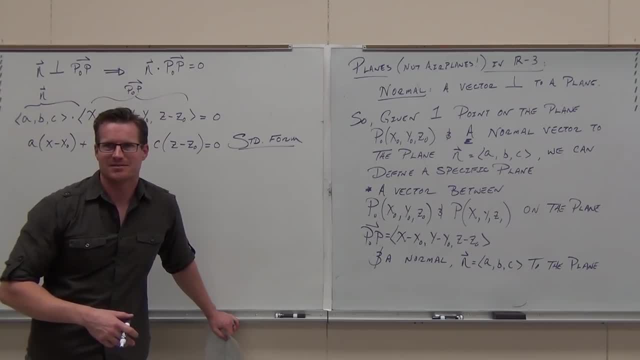 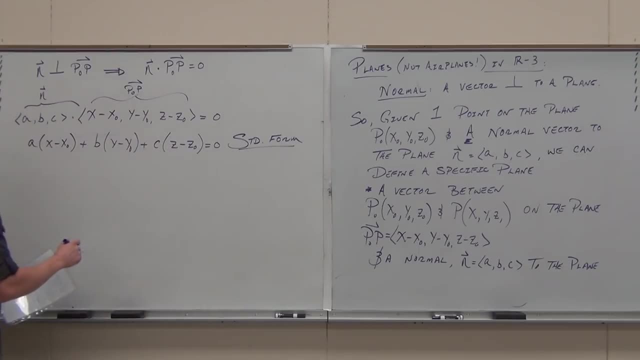 That does not get better. There's a lot better than that. I'm not going to edit it. Enjoy that. Okay, friends, If you distribute all the things that you saw, all the things that I said earlier, If you distribute all this junk, I want you to jump down to here. 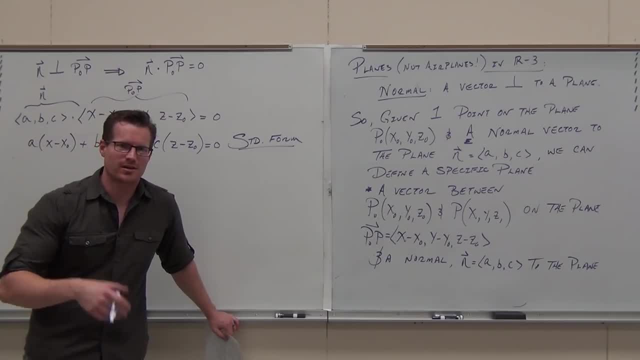 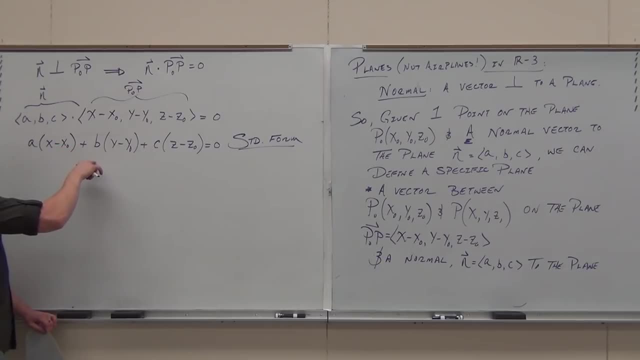 There's a lot better than that. I'm not going to edit it. Enjoy that. Okay, friends, If you distribute all this junk, I want you to jump down to here. What happens is we get this AX, we get an actual number. 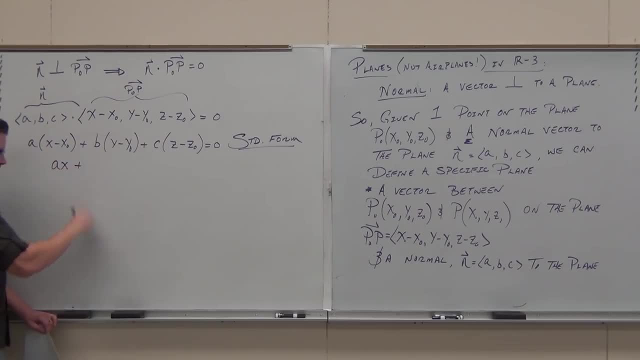 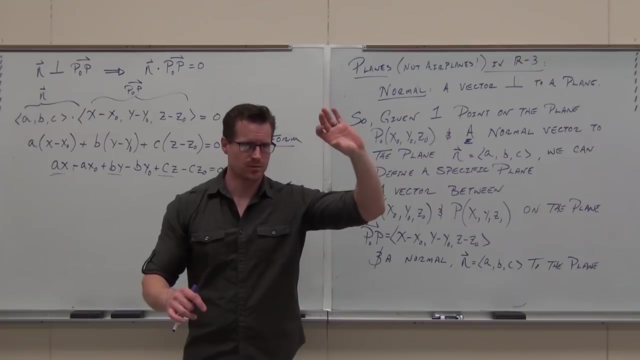 Do you see it? We get you know. I'll show you. Keep this, this, this, and you are going to have three numbers Direction. well, the normal vector components times the actual piece of what do you call those things? 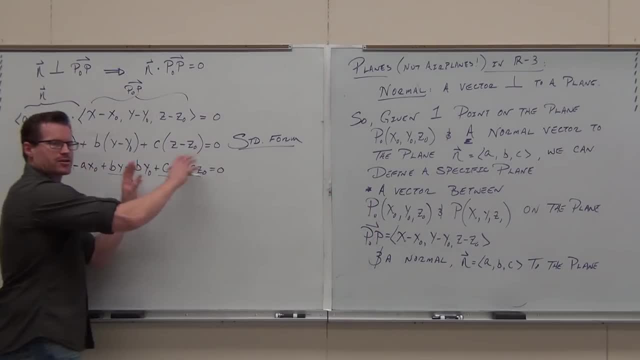 Coordinates of our point And they're going to be numbers. If you add or subtract or whatever, get them all to one side. we end up getting this. Now. this all looks very fancy. I don't want you to worry about the fancy. 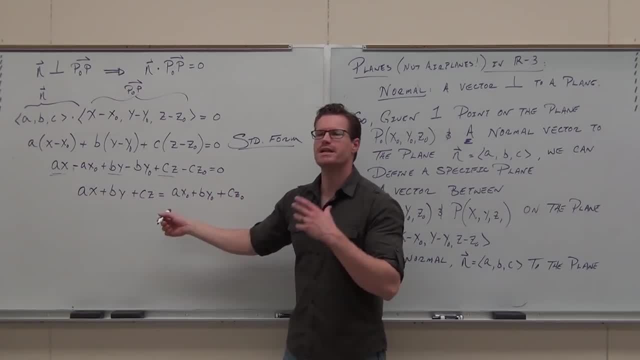 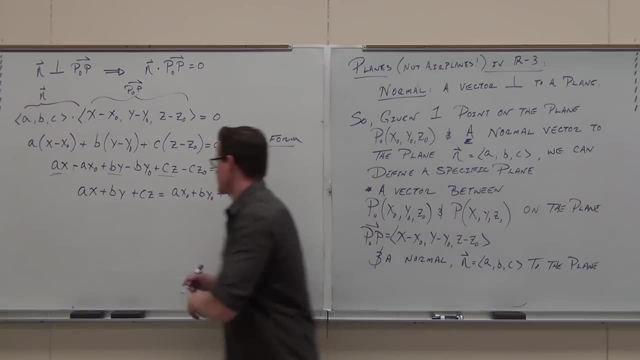 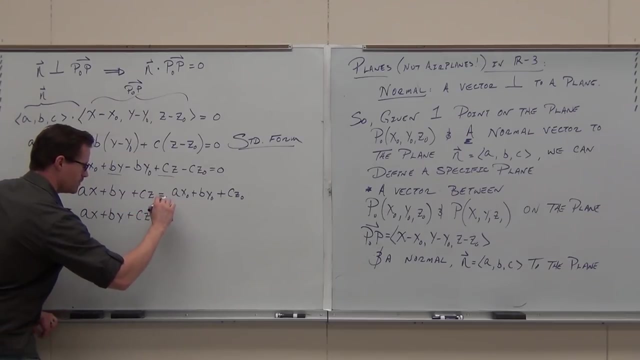 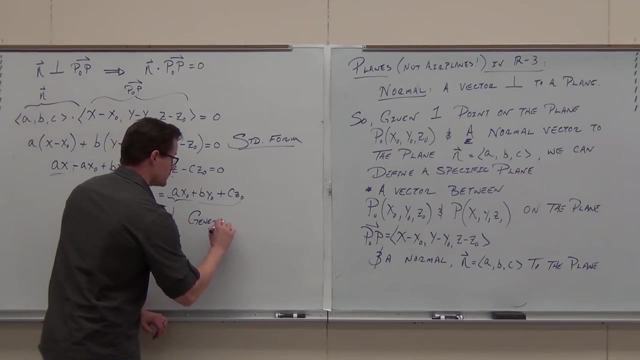 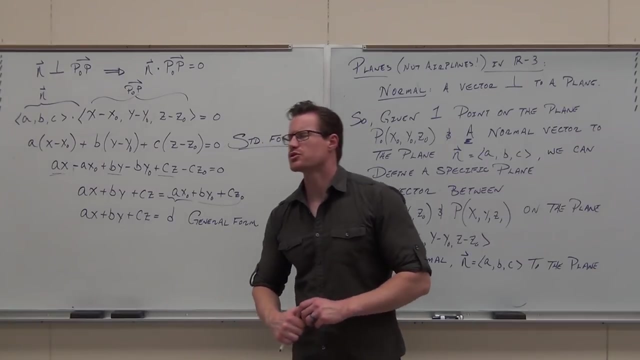 I want you to worry about the next thing. Do you see that this is all going to be one number? Yes, Just a number. We call that number D. That number D is just all the junk. That's general form. This works so much like point slope and the slope intercept. 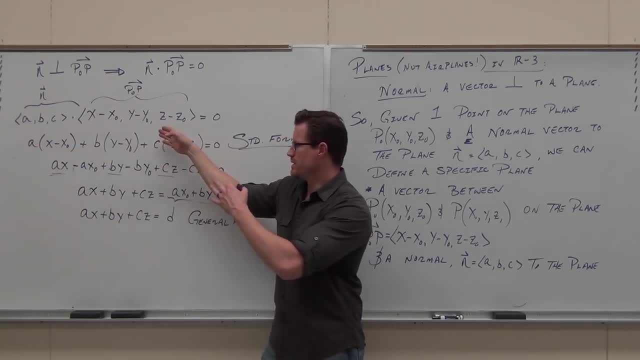 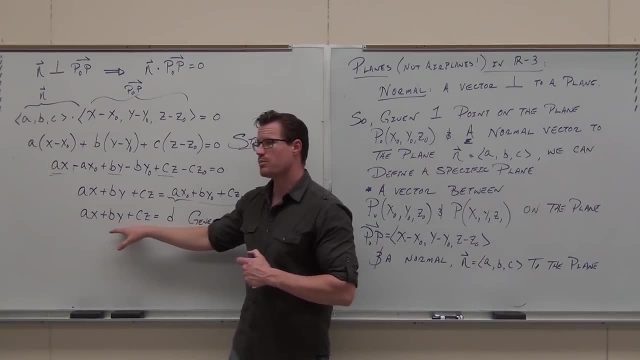 We use a point and a normal to get down to this sort of thing. It's not really slope intercept, but it's a lot easier to work with. This right there doesn't quite give you a point, but it definitely gives you a normal vector. really, really easy. 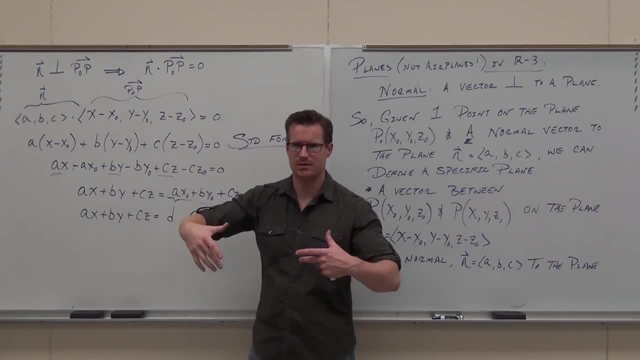 Show of hands. if you look here, Okay with what I'm talking about. Are you really getting this? Tell you what? can we do an example here real fast, Before we do well, we're going to do a lot more examples. 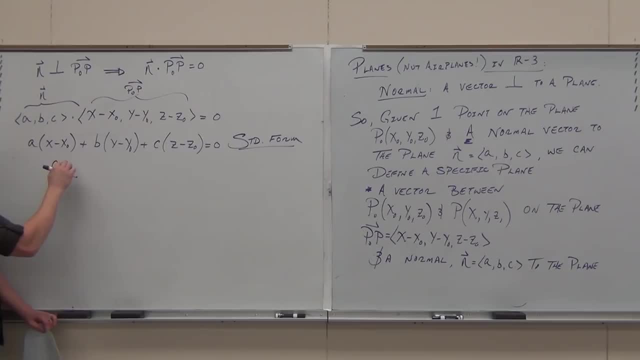 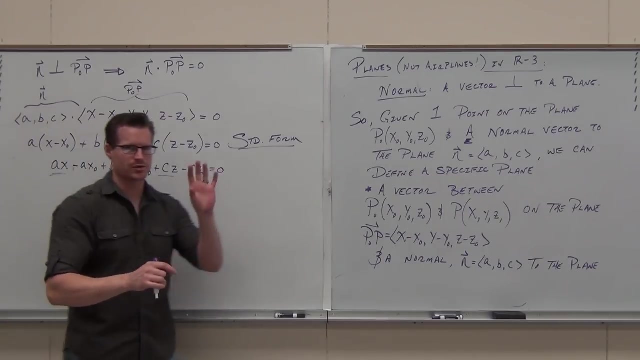 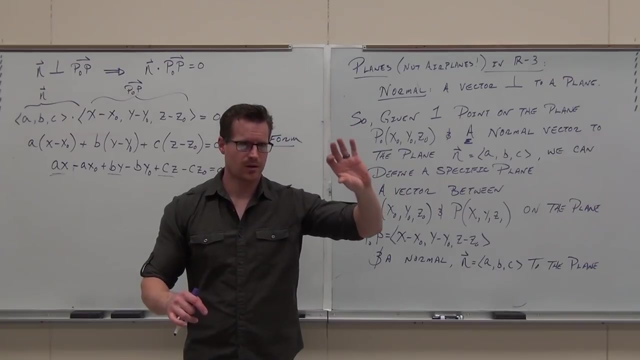 What happens is we get this AX, We get an actual number. Do you see it? We get you know. I'll show you. Keep this, this, this, and you are going to have three numbers. direction: well, the normal vector components times the actual piece of what do you call those things? coordinates of our point. 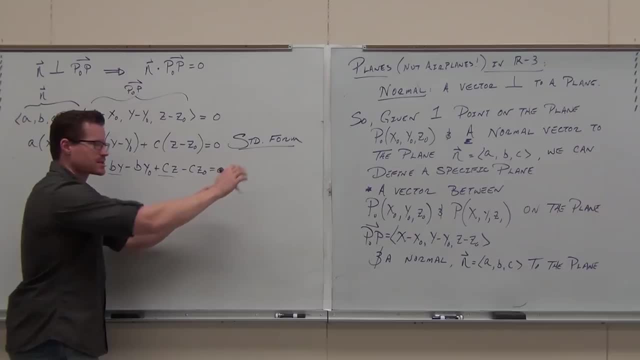 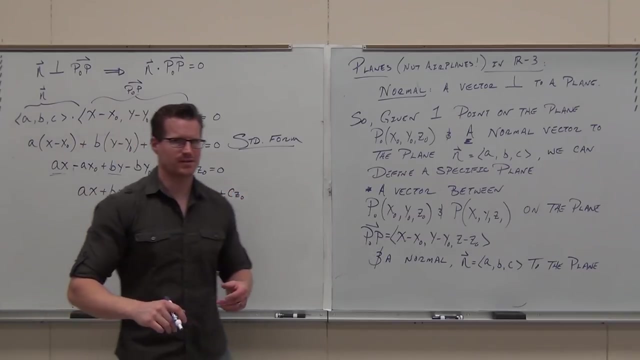 And they're going to be numbers. If you add or subtract or whatever, get them all to one side, we end up getting this. Now, this all looks very fancy. I don't want you to worry about the fancy. I want you to worry about the next thing. 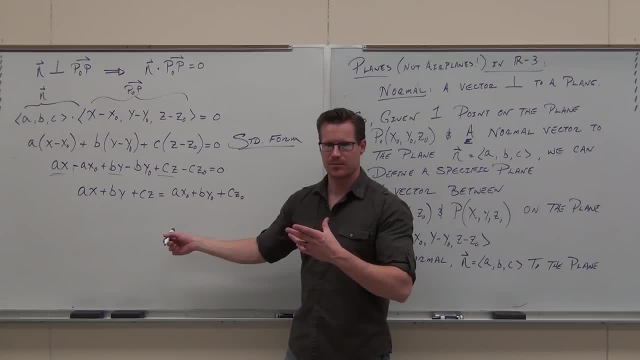 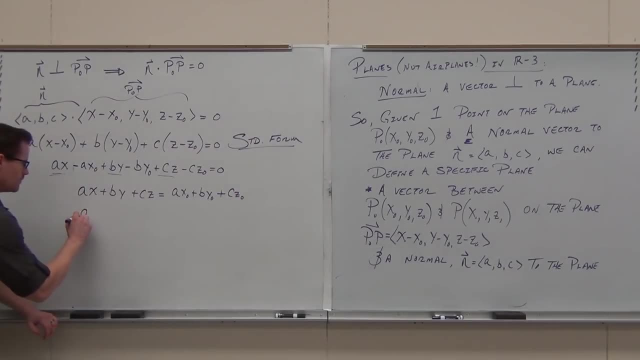 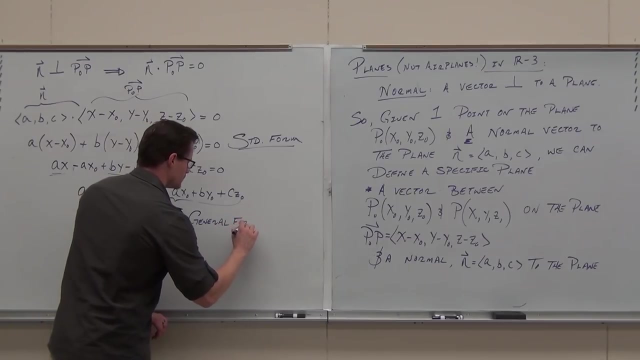 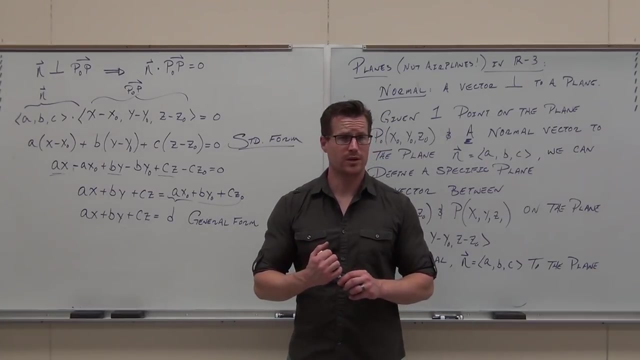 Do you see that this is all going to be one number? Yes, Just a number. We call that number D. That number D is just all the junk. That's general form. This works so much like point slope into slope intercept. 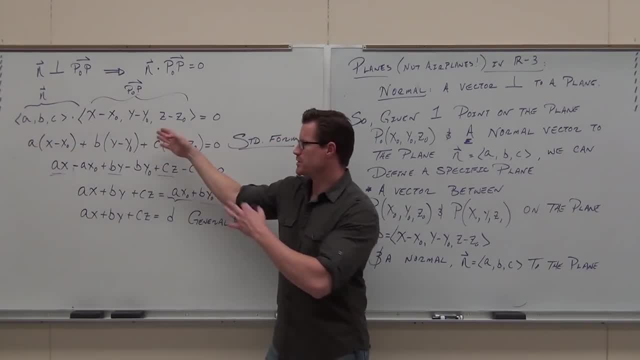 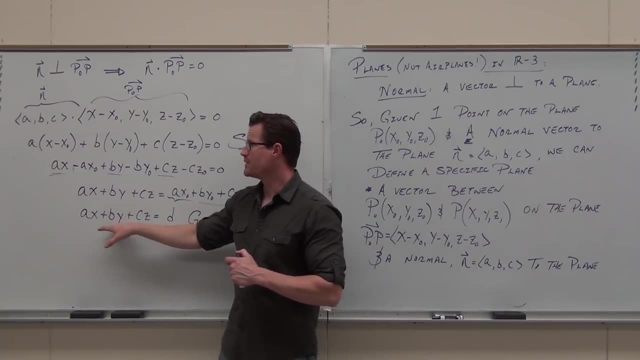 We use a point and a normal to get down to this sort of thing. It's not really slope intercept, but it's a lot easier to work with. This right there doesn't quite give you a point, but it definitely gives you a normal vector. really, really easy. 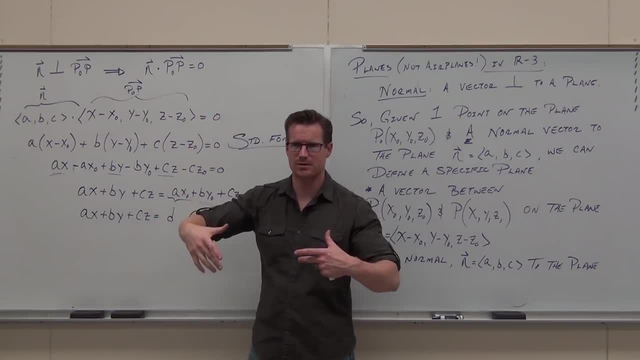 So, if you feel okay with what I'm talking about, Are you really getting this? Tell you what. Can we do an example here real fast Before we do? well, we're going to do a lot more examples when we come back. 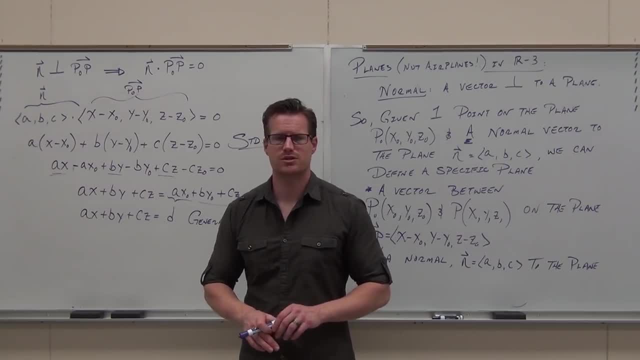 We're going to go through everything Before we do, though, in case anyone just needs to take off. just hope you don't. But if I had two vectors, imagine three points in a plane. Here's my plane: Vector here. vector here. 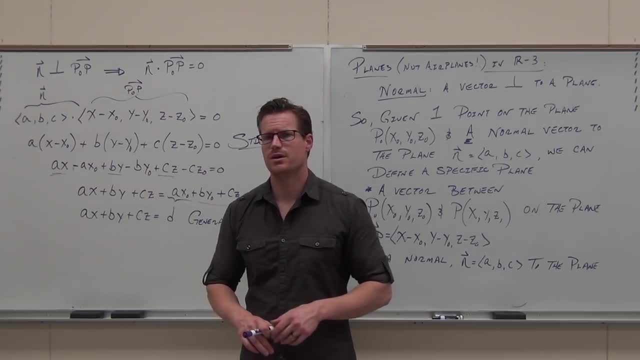 when we come back and we're going to go through everything Before we do. though, in case anyone just needs to take off, which I hope don't, but if I had two vectors, imagine three points in a plane. Here's my plane. 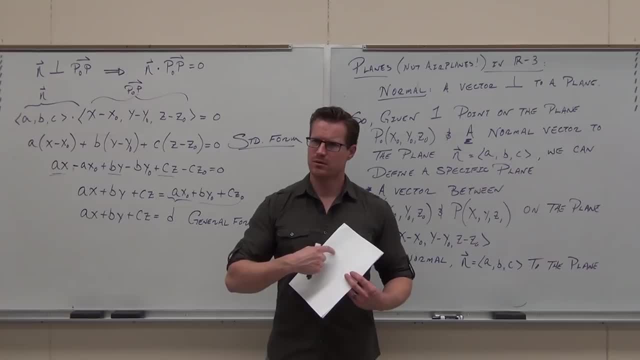 Vector here. vector here. Would you know how to find a normal given two vectors in a plane? What would give you a mutually orthogonal vector to two vectors in a plane? If you have two vectors in a plane, you can always get a normal vector by a what's everybody. 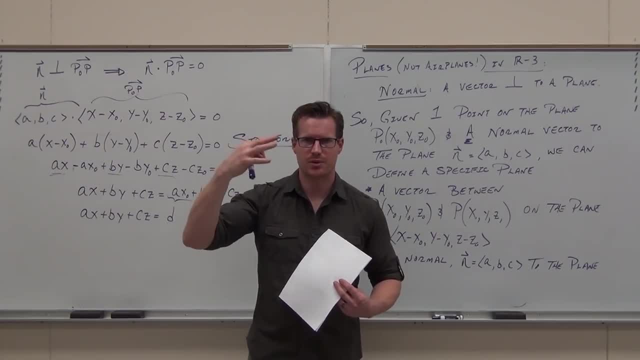 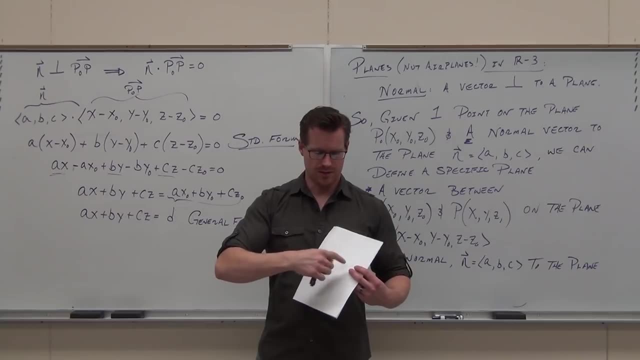 A cross-part, A cross-part. This is why you need three points to define a plane, Because if I have three points, I can go .1, .2, .3.. Vector- I'm going to draw on my paper. I got a white board. 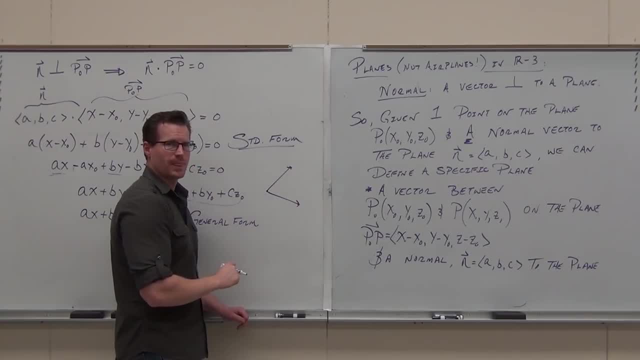 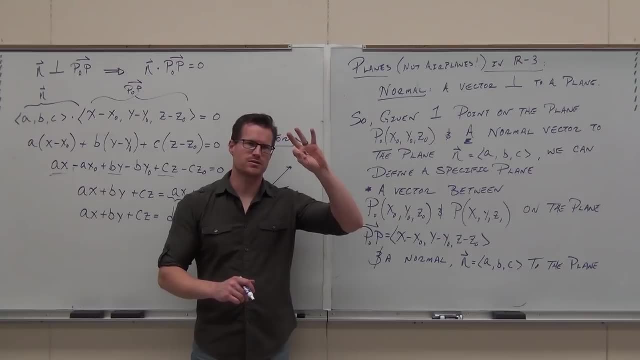 Three points, Vector one, vector two: If I do a cross-product, that's my normal. That's why you need three points, because three points defines two vectors And two vectors, you can cross-product, And you can cross-product, you get a normal. 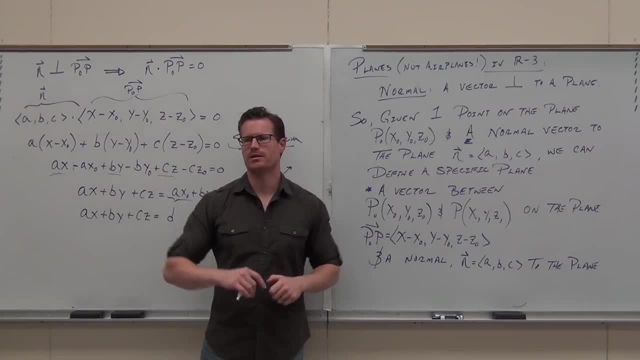 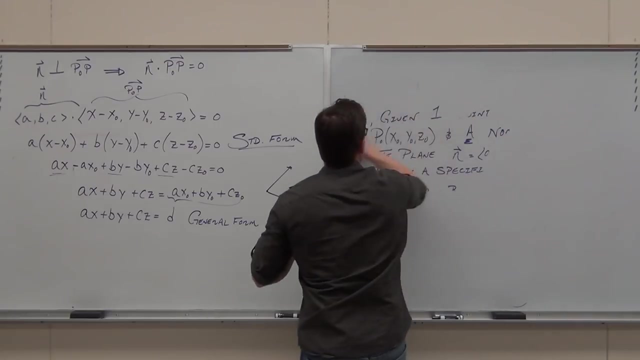 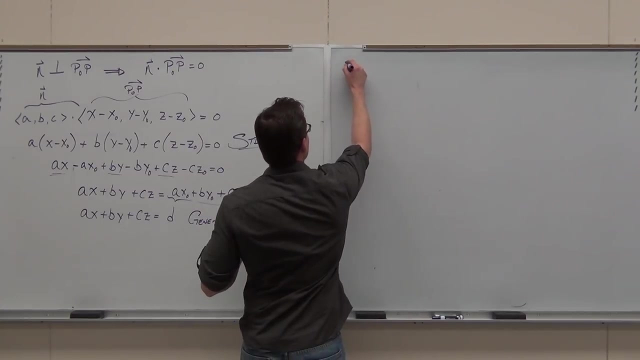 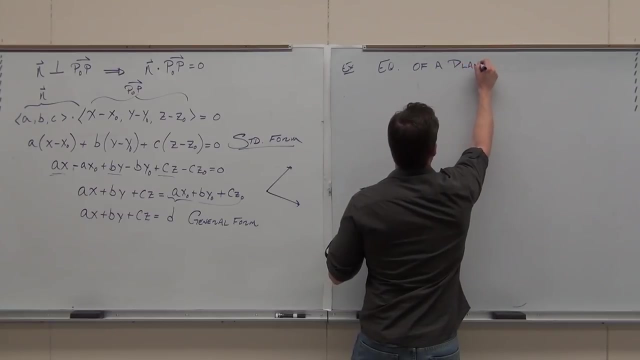 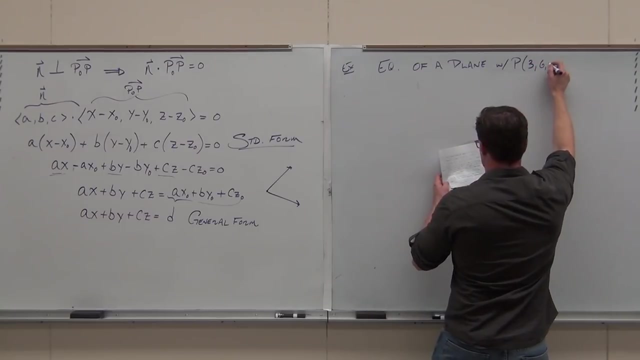 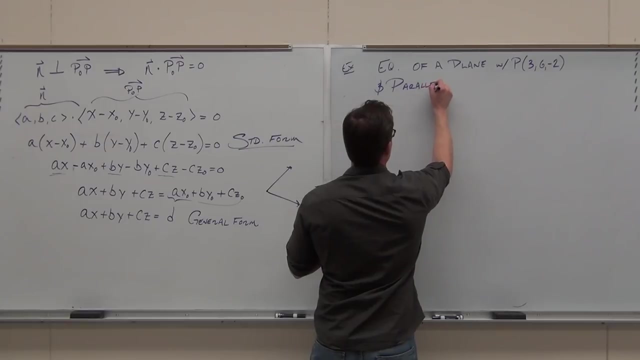 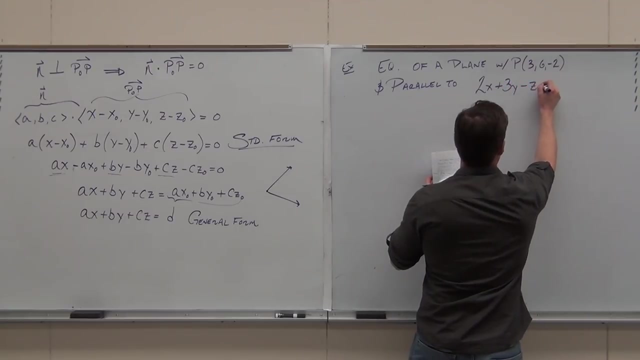 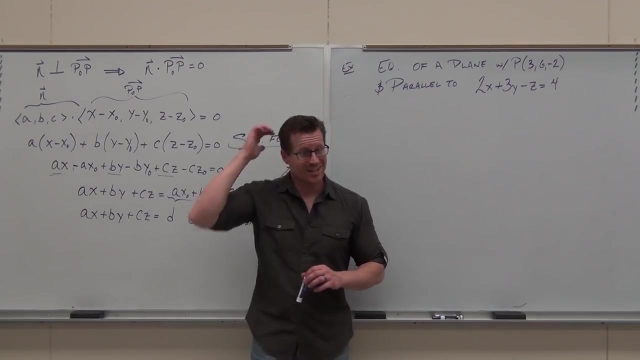 And if you have a point and now a normal, we have a plane. That's the idea. That's pretty darn cool. Let's do our one example, then we're going to take our break. Pretty basic example. You know, a lot of times, a lot of times, people get equations of lines. 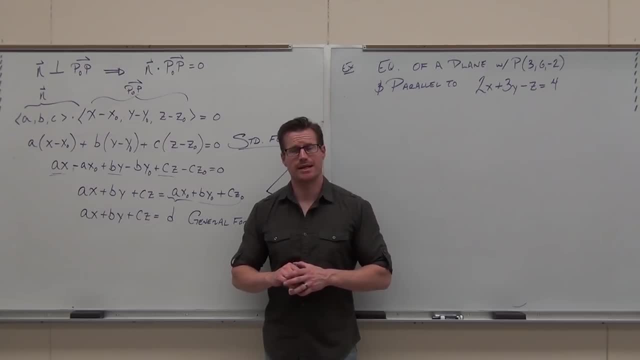 and equations of planes really jacked up. So I need you to be really good at that. I want to find the equation for planes. so we're going to be using this stuff- equations of planes- But I want it through a point and I want it parallel to this thing that I've given you. 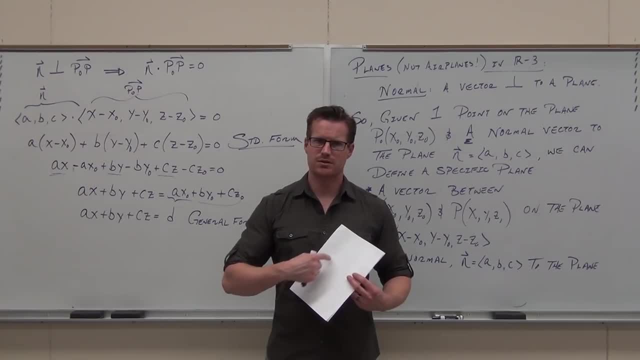 Would you know how to find a normal given two vectors in a plane? What would give you a mutually orthogonal vector to two vectors in a plane? If you have two vectors in a plane, you can always get a normal vector by a what's everybody. 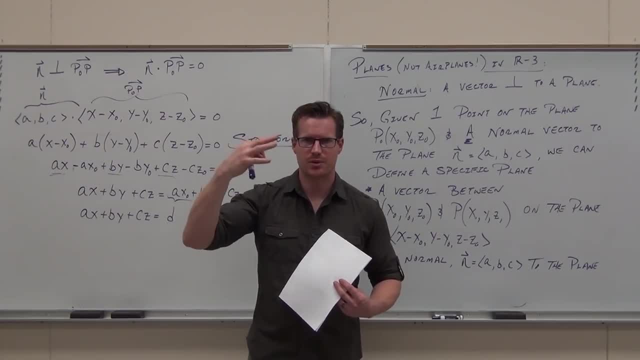 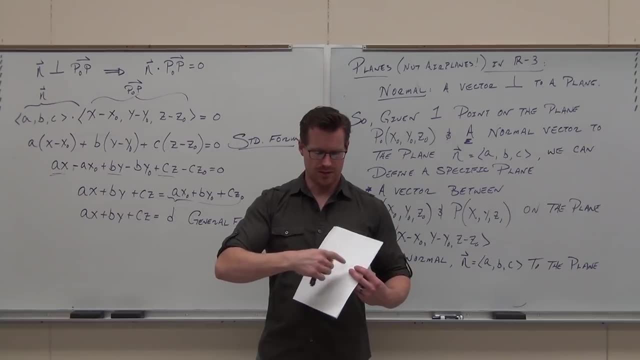 Cross-part, Cross-part. This is why you need three points to define a plane, Because if I have three points I can go. point one, point two, point three: Vector. I'm going to draw my paper. I've got a whiteboard. 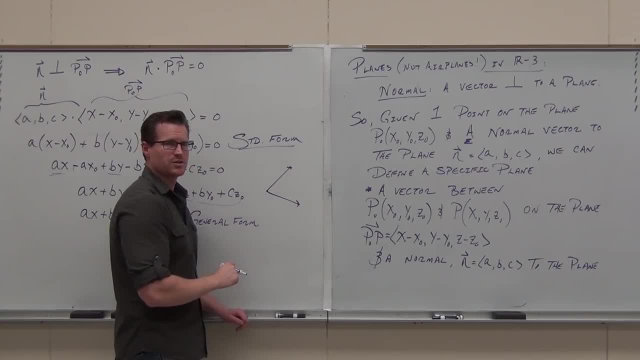 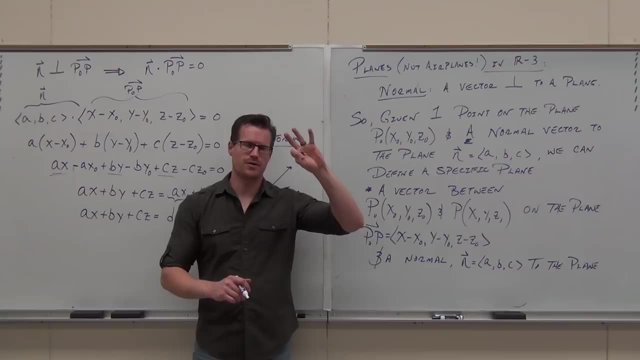 Three points, Vector one, vector two: If I do a cross-product, that's my normal. That's why you need three points, because three points defines two vectors And two vectors, you can cross-product, And you can cross-product, you get a normal. 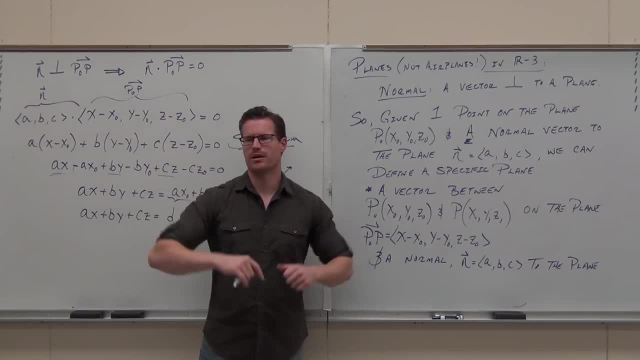 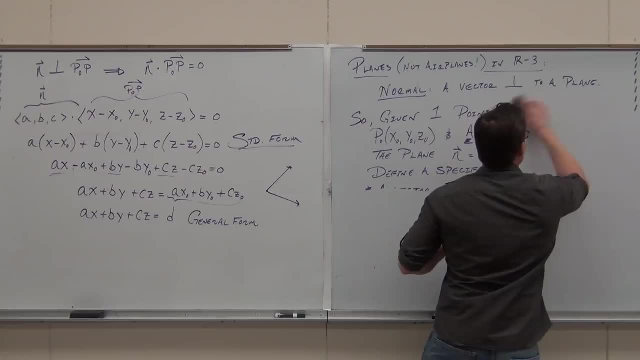 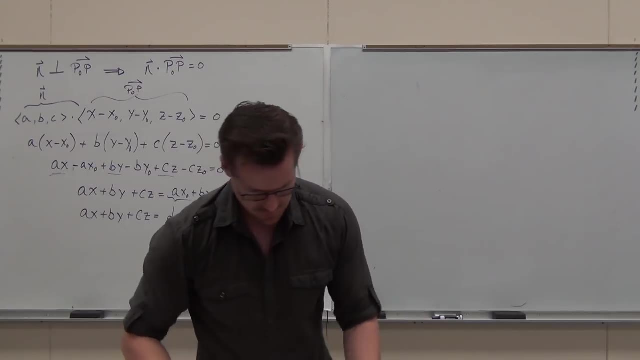 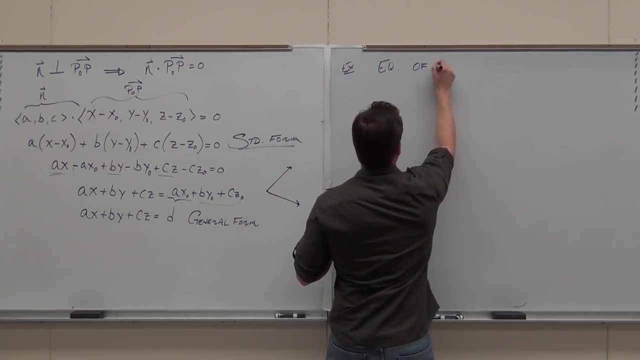 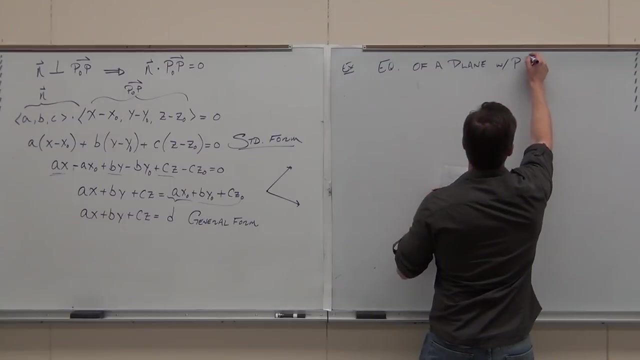 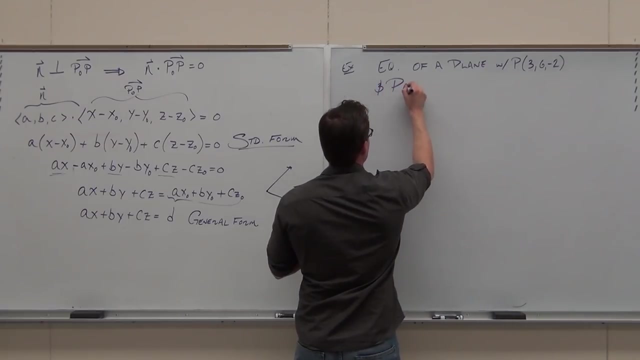 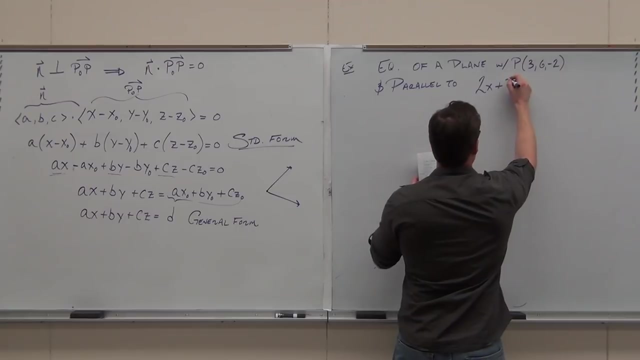 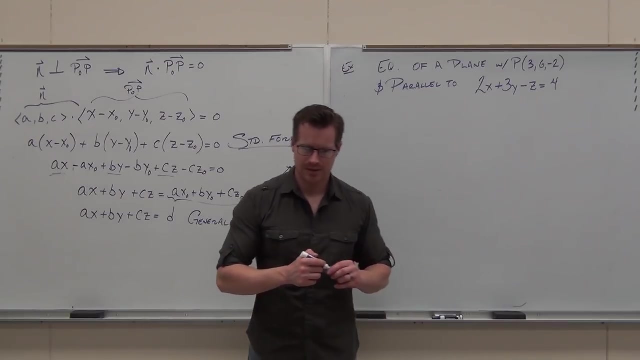 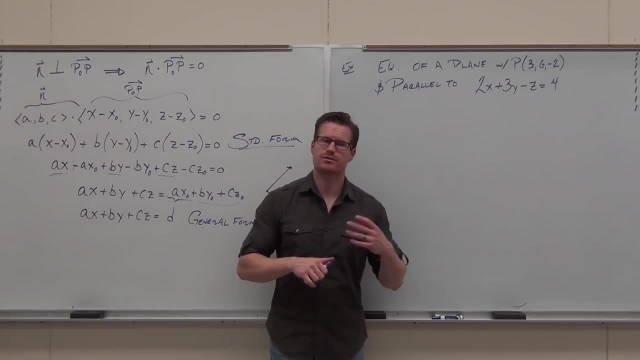 You know, a lot of times, a lot of times, people get equations of lines and equations of planes really jacked up. So I need you to be really good at that. I want to find the equation of a plane. so we're going to be using this stuff: equations of planes. 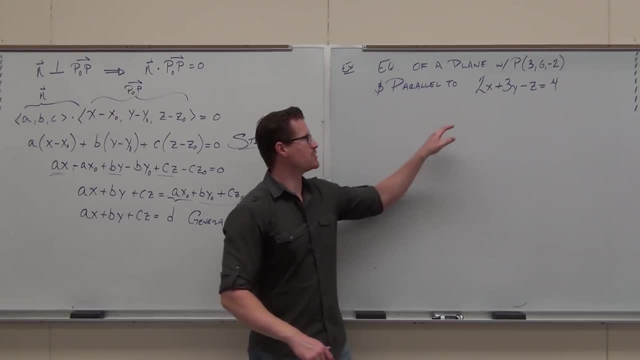 But I want it through a point and I want it parallel to this thing that I've given you. Now, what two things do you need to find the equation of a plane? What two things: A point, A point And A normal vector. 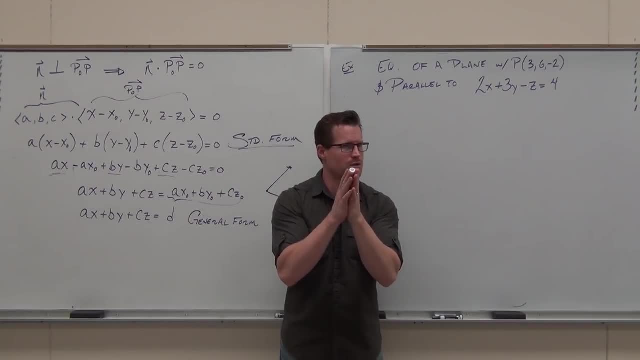 Now, what two things do you need to find the equation of a plane? What two things? A point, A point. And what type of vector? Normal, Normal vector for a plane. What have I given you here? Is this a line or is this a plane? 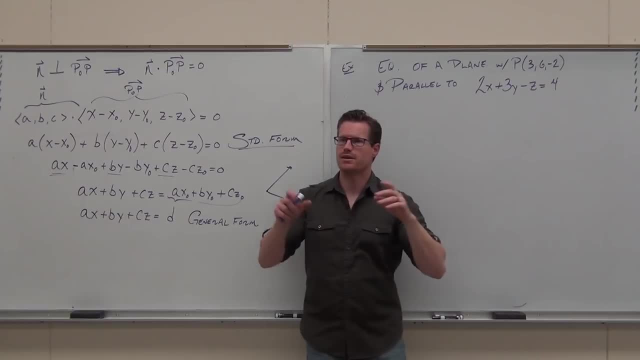 What is that? Lines have this: the X equals, Y equals, Z equals. Do you see that They have equal signs everywhere, like everywhere, They're either fractions equal or X, Y and Z equal. Do I have that? What is this thing then? 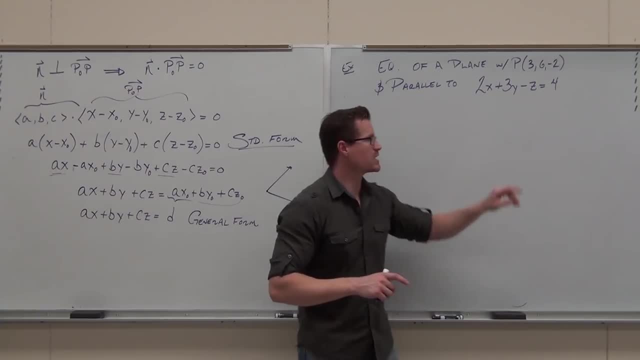 This is a plane for sure. Can you right now tell me the normal vector to that plane? Can you tell me right now- Don't say it out loud, Just write it down- if you can Write down what the normal vector to that plane is. 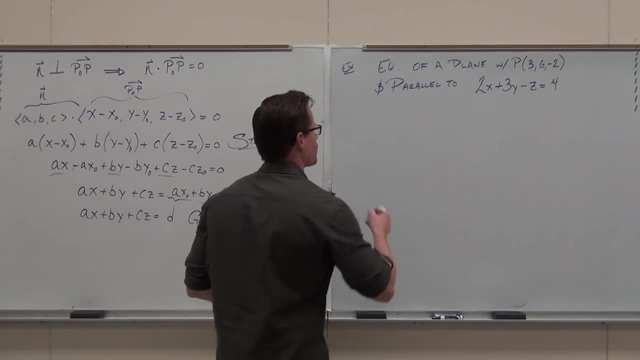 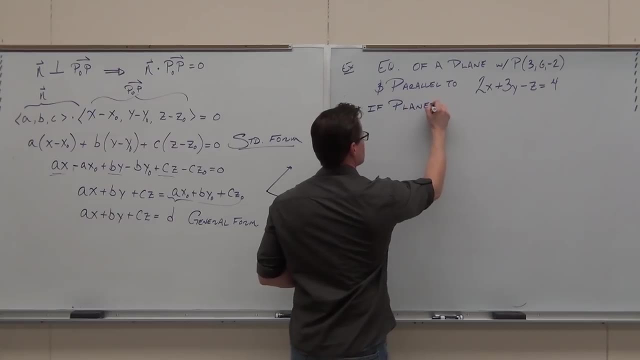 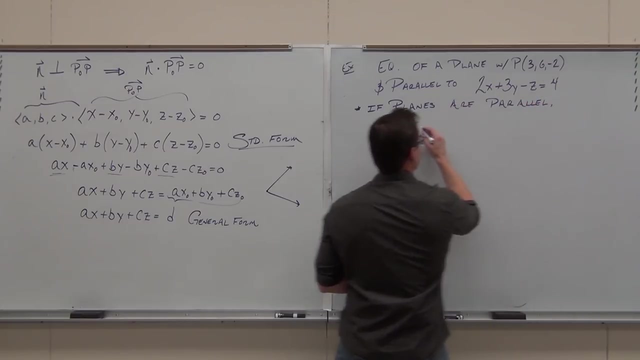 Go. Normal vector to that plane equals Y, squared. What is this thing called? It's thegest vector. What vector to find No weight? What vector just minus this value? The της vector to that plane? Yeah, Р KEVIN, What vector do you mean? 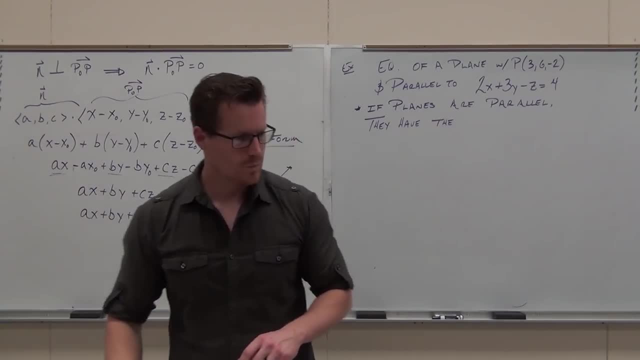 Monster vector to that plane. What vector? just minus that value, Those are VIC is the equals sign. Who are you looking at? Am I looking at someone? Absolutely, Those areges are shoutings. What else am I looking at? Life is like that. 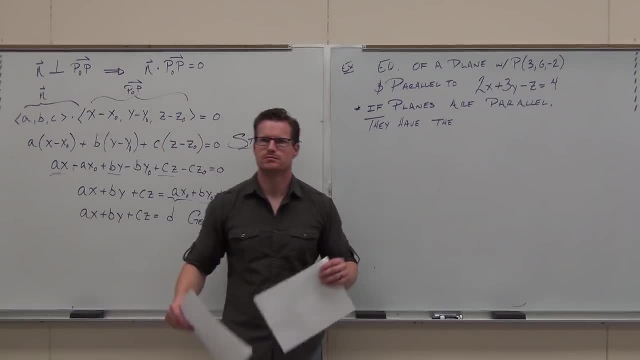 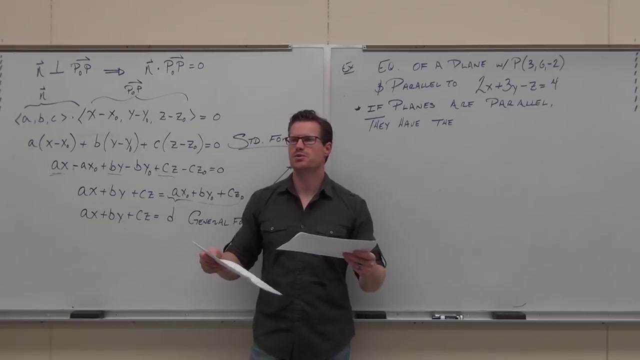 What vector do you find? It's a plane. it's a plane. These planes are parallel. I can't do it. it's a loop paper. These planes are parallel. Tell me something about their normal vectors. Tell me something about two lines that are parallel. 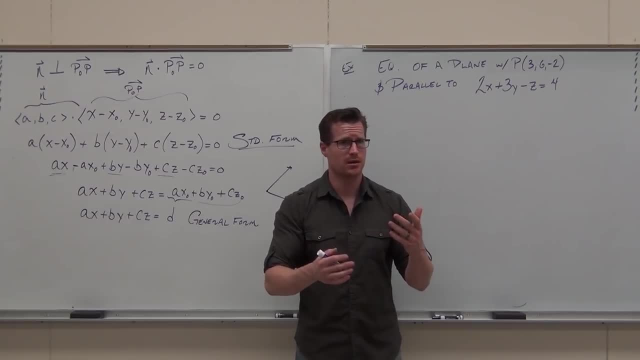 What type of vector? Normal vector, Normal vector for a plane. What have I given you here? Is this a line or is this a plane? What is that? A plane? A plane, A plane Lines? have this: the X equals, Y equals, Z equals. 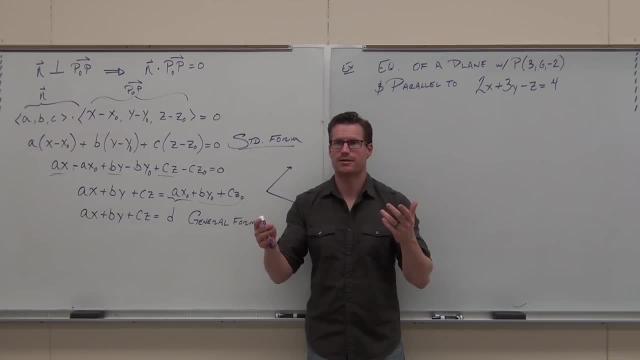 Do you see that They have equal signs everywhere, like everywhere, They're either fractions equal or X, Y and Z equal. Do I have that? What is this thing then? This is a plane, for sure. Can you right now, can you right now tell me the normal vector? 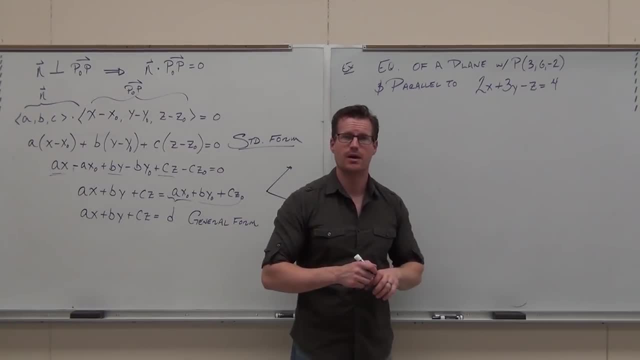 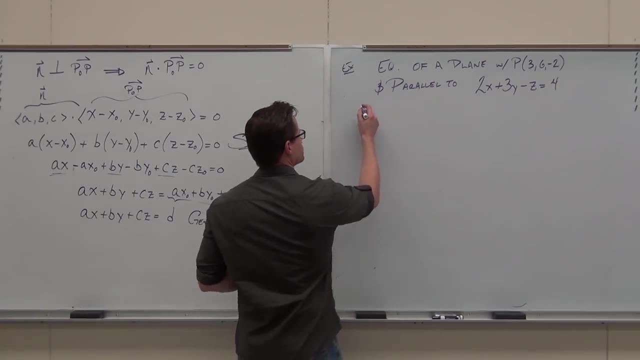 to that plane. Can you tell me right now? Don't say it out loud, just write it down. if you can Write down what the normal vector to that plane is, Go. It's the normal vector for the F to the zeros of one word. 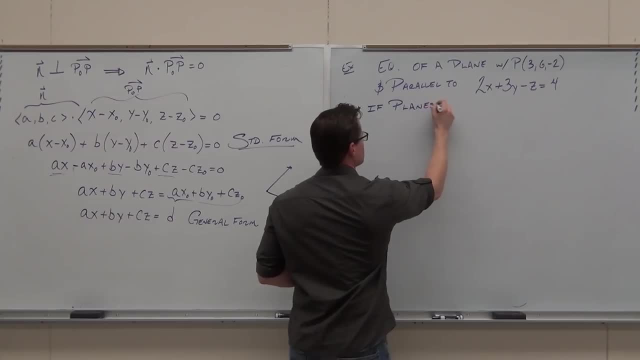 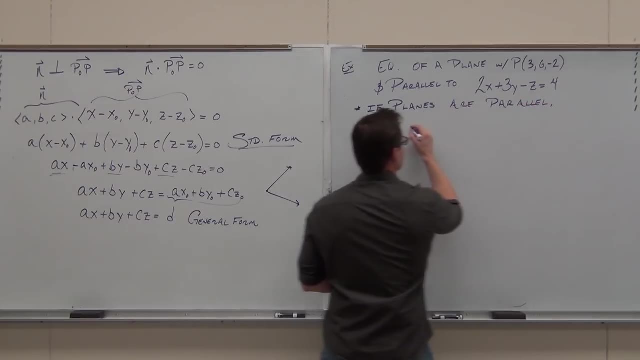 Right, OK, So you'll write it down. Sorry, You can see it's a nice square element, right? So the dignity of that vector is one string out of three. What equals it? It's the on the H, you mean. 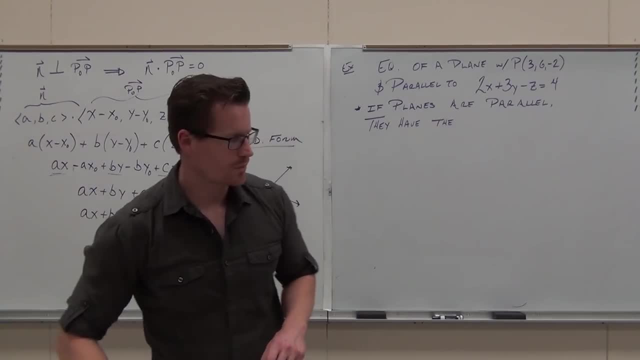 Five and six goes to the갖 Five Three. That was very important Big number. Yep, OK. And now you have the two things equalなので you just need to minus the positive Right. Yes, Okay. 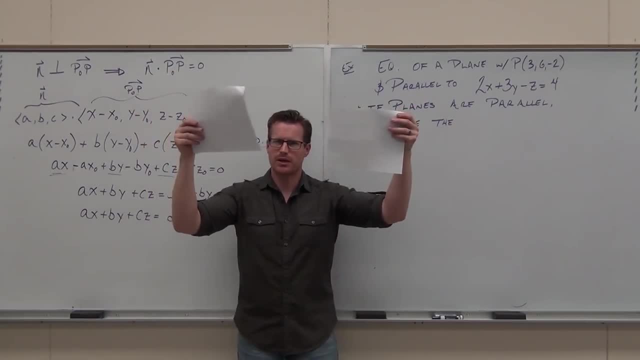 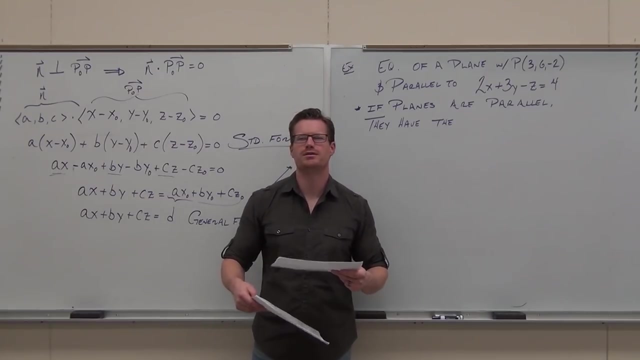 It's a plane. it's a plane. These planes are parallel. I can't do it. it's a root paper. These planes are parallel. Tell me something about their normal vectors. Tell me something about two lines that are parallel. Tell me something about two lines that are parallel. 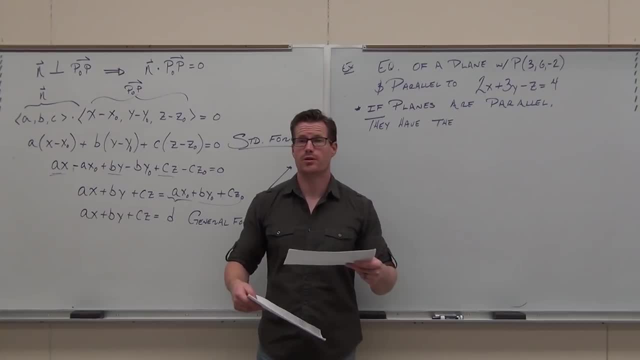 Tell me something about two lines that are parallel: Same slope, Same slope or, in 3D, same vector, same direction, scalar multiples. So if these two planes are parallel to each other, tell me something about their normal vectors. 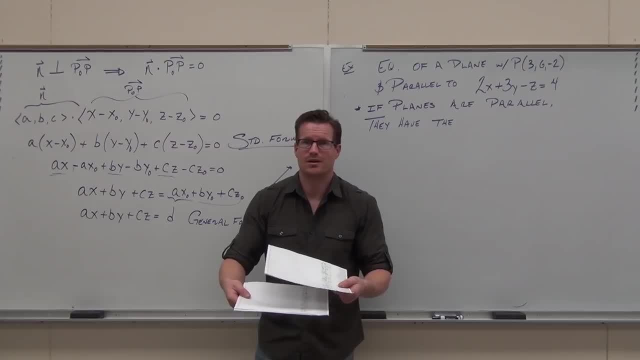 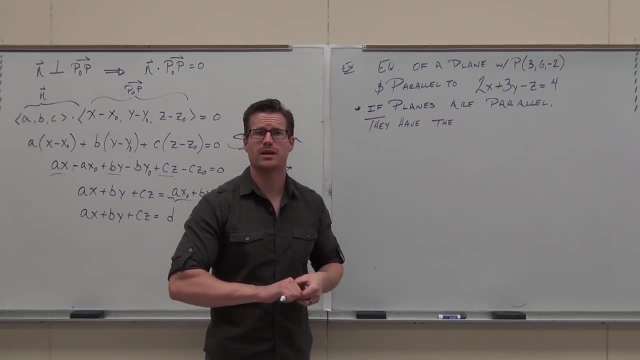 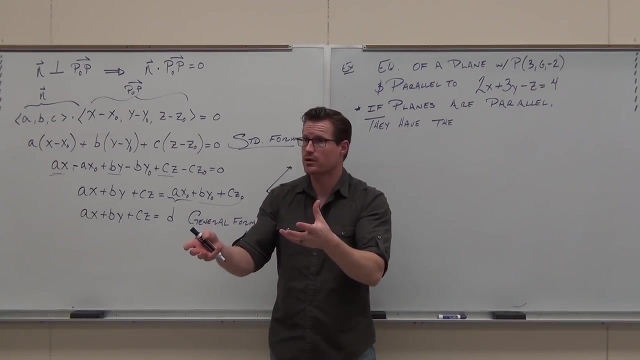 Can they be anything else but the same vector? No, So whenever I ask you, hey, find the equation of a plane that's parallel to another plane, if you can find the normal vector to a parallel plane, you have found the normal vector that we are looking for. 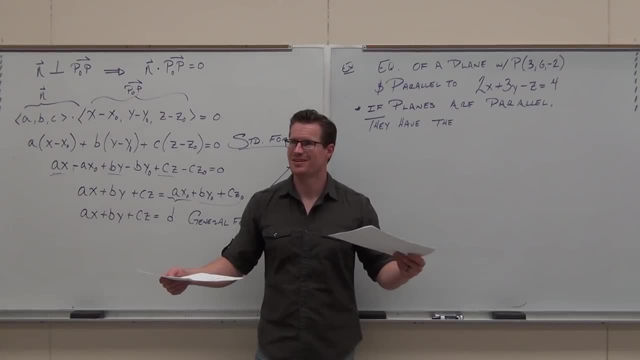 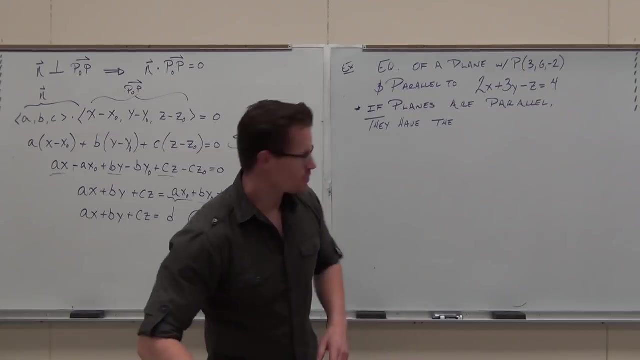 Same slope, Same slope or, in 3D, same vector, same direction, scalar multiples. So if these two planes are parallel to each other, tell me something about their normal vectors. Can there be anything else but the same vector? No, So whenever I ask you: hey, find the equation. 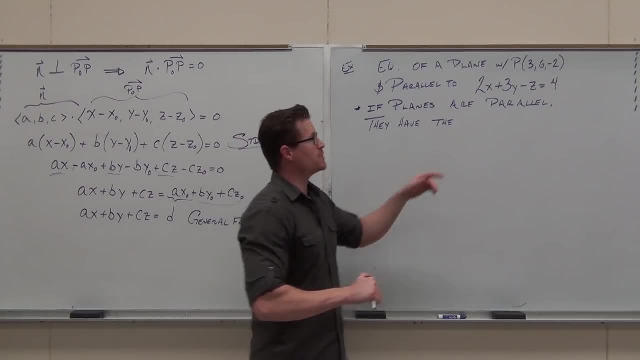 of a plane that's parallel to another plane. if you can find the normal vector to a parallel plane, you have found the normal vector that we are looking for. Does that make sense to you? It's not super hard, but you've got to think like this. 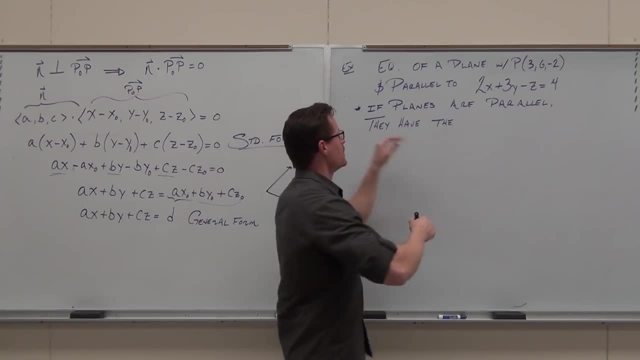 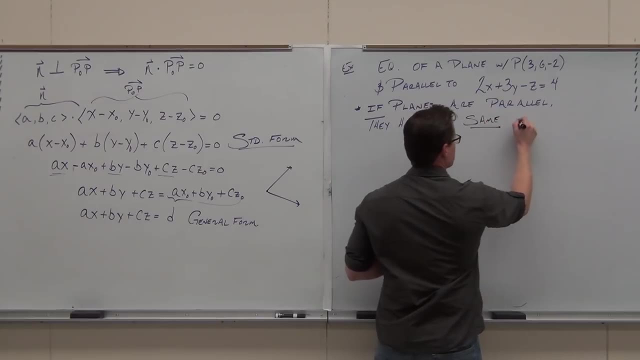 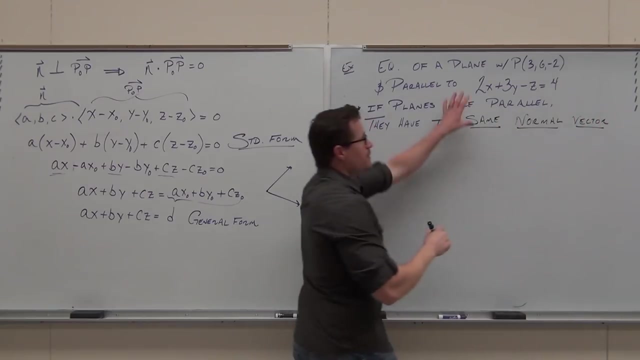 Does that make sense to you? It's not super hard, but you've got to think like this. So if planes are parallel, they have parallel vectors. You've got to find out the same normal vector, And I know you wrote it down. 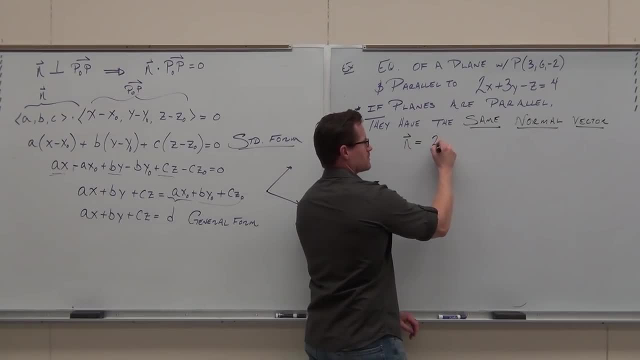 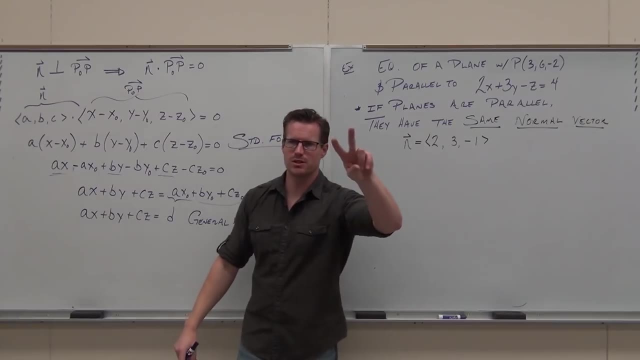 Our normal vector here is: what is it? Two, Two, three, four, Two, three, four. Okay, let's try it again. Come on 20 second recap. There's two things. you need to write the equation of a plane. 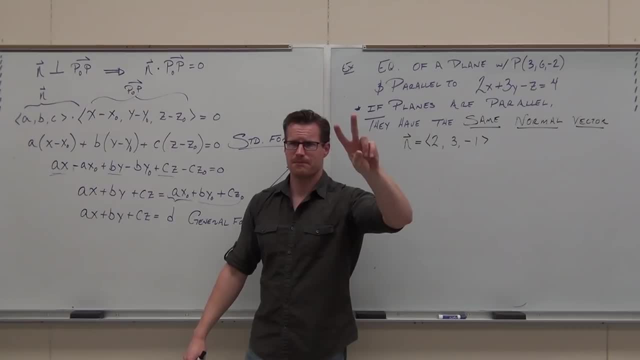 What's one of those things? Three, One, Oh, I'm losing you, Goodness. There's two things. you need to write the equation of a plane, A point. You've got to have a point. Do we have a point? 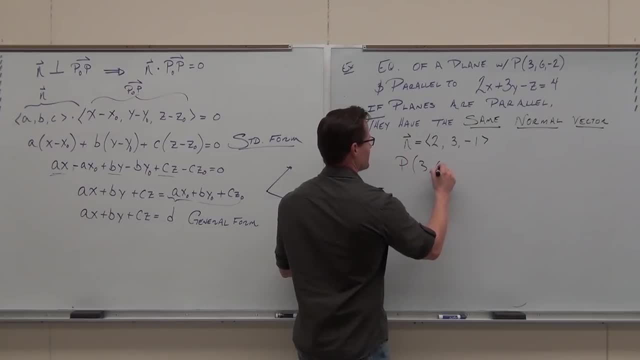 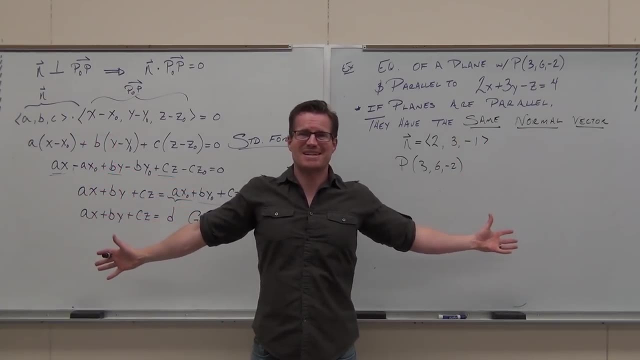 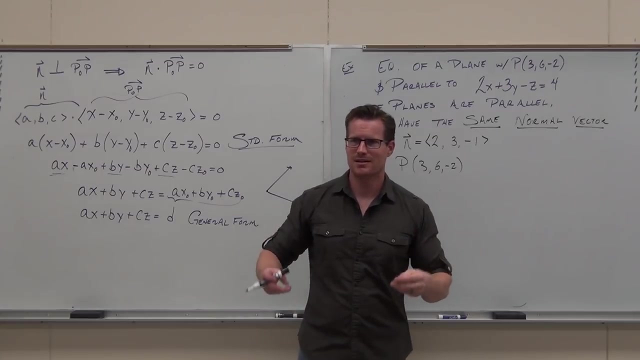 Yes, Do we have a normal vector? How did we find that normal vector A, B, C's man A B C? Easy as one, two, three. Oh, you like what I did there? Now I see. 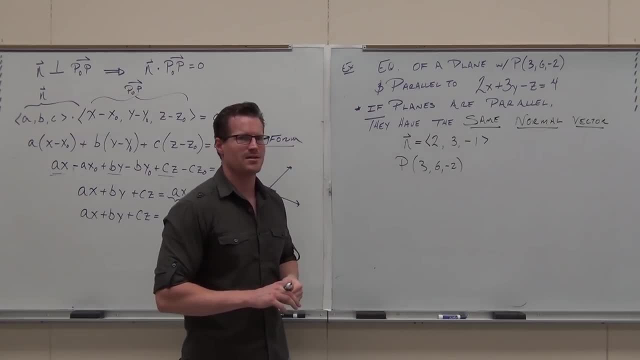 A, B, C. Let's do calculus, you and me now. No, That's how it goes. That's how it goes. I'm pretty sure Michael Jackson told me: I don't think you can anymore. Are you asleep? 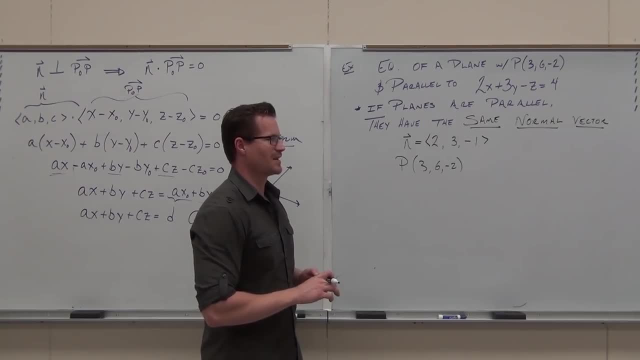 Oh, too soon. I love you, Michael. I'm going to get some negative comments on that one. So listen, if planes are parallel, they have the same normal, or at least scalar Multiple is the same normal. so you use the same freaking one. 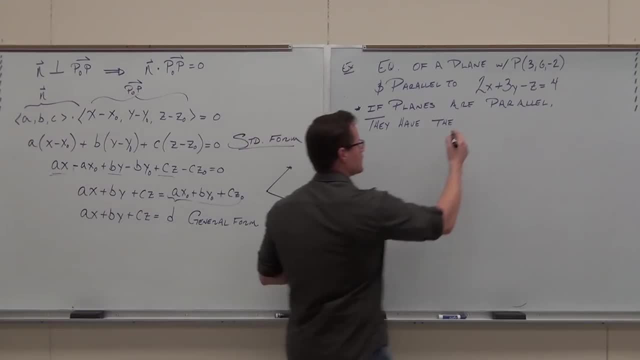 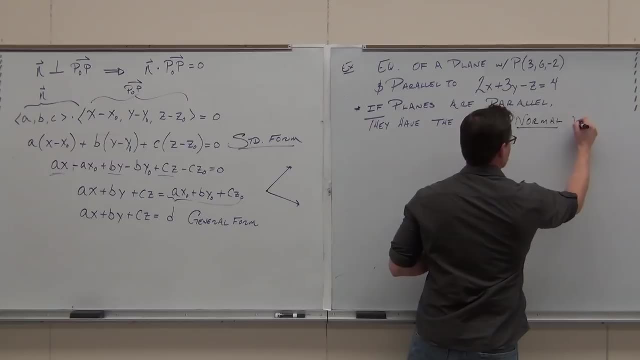 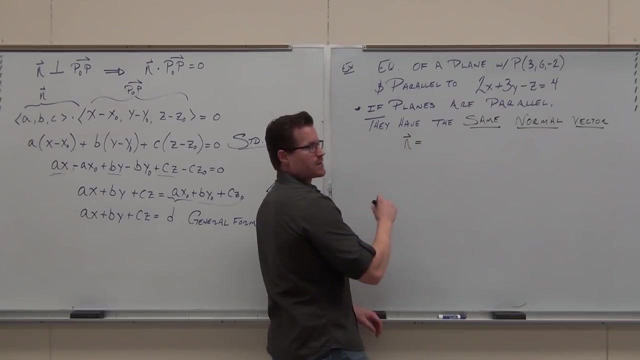 So if planes are parallel, they have the same normal vector, And I know you wrote it down. Our normal vector here is: well, what is it? Two, three, four, five, six, seven, eight, nine, 10,, 11,, 12,. 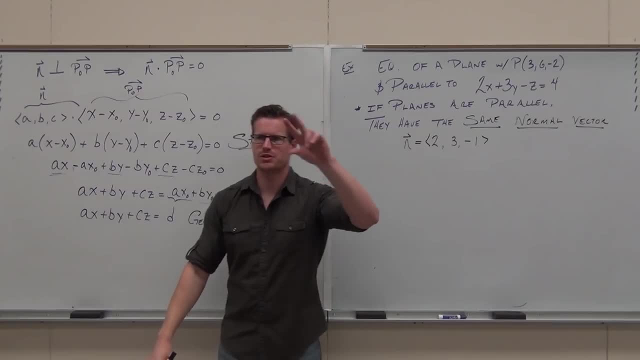 13, 14.. Okay, let's try it again. Come on 20 second recap. There's two things. you need to write the equation of a plane. What's one of those things? A point, I'm losing it. 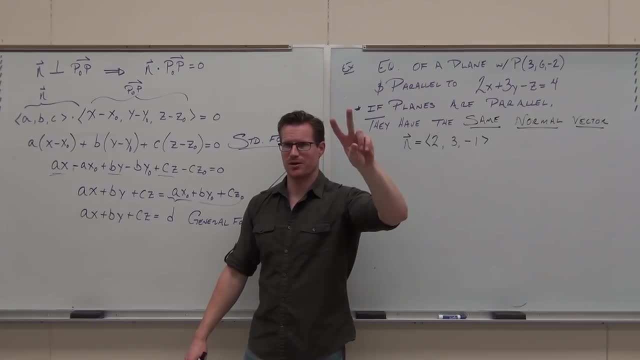 Goodness, There's two things. you need to write the equation of a plane. You can have a point. Do we have a point A? Do we have a normal vector? Yes, How did we find that normal vector A, B, C. 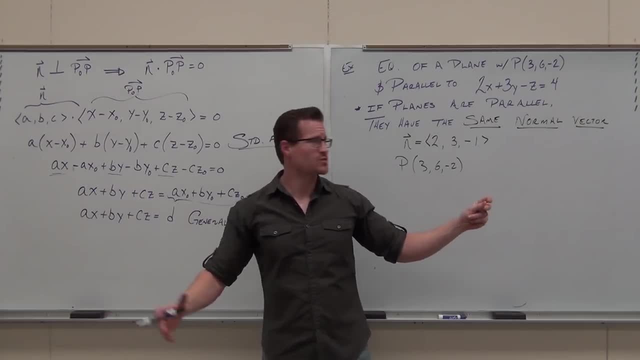 A B C's man A B C. Easy as 1,, 2, 3, 4.. Easy as 1,, 2, 3.. Easy as 1,, 2,, 3, 4.. 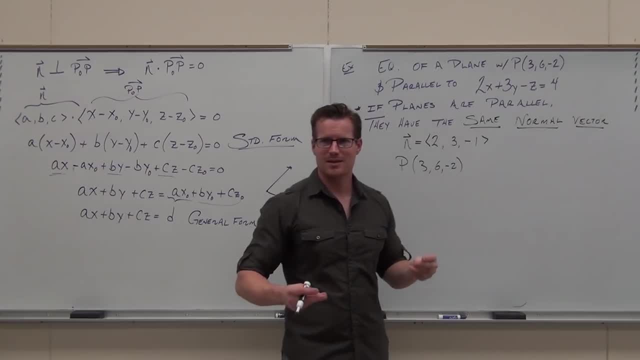 Easy as 1,, 2,, 3, 4.. Oh, you like what I did there. Now I see ABC. let's do calculus, you and me now. No, That's it. That's how it goes. I'm pretty sure Michael Jackson told me. 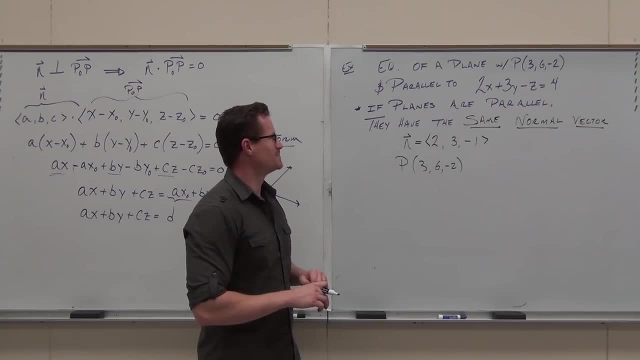 You can't anymore. Oh, too soon. Love you, Michael. I'm going to get some negative comments on that one. So listen, if planes are parallel, they have the same normal, Or at least scalar Multiple is the same normal, so use the same freaking one. 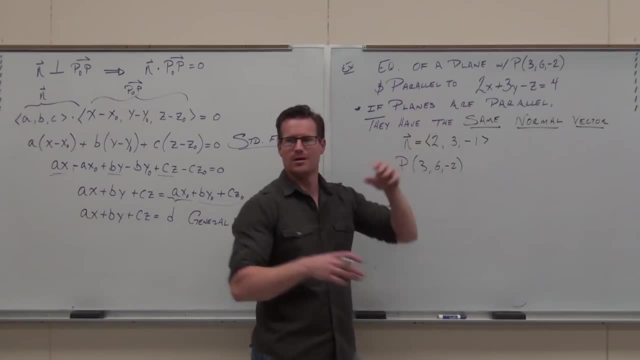 That's fine. So use the same exact normal. So parallel, same normal, Parallel lines, same vector, Parallel planes, same vector. You see the connection. We need a point and a normal. We have a point and a normal And here's how to work with the rest of it. 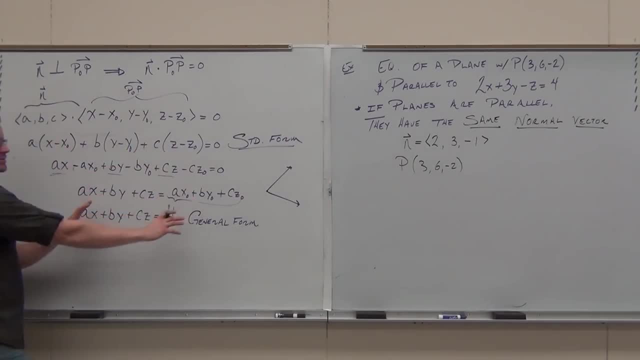 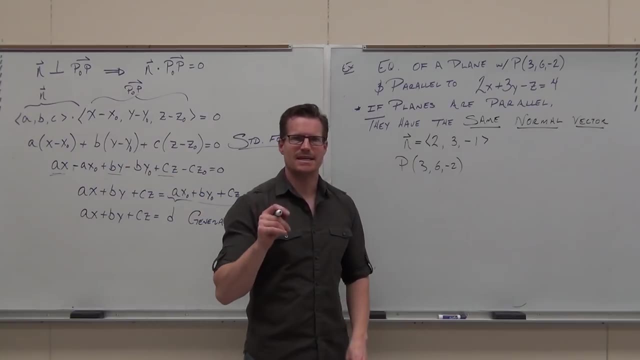 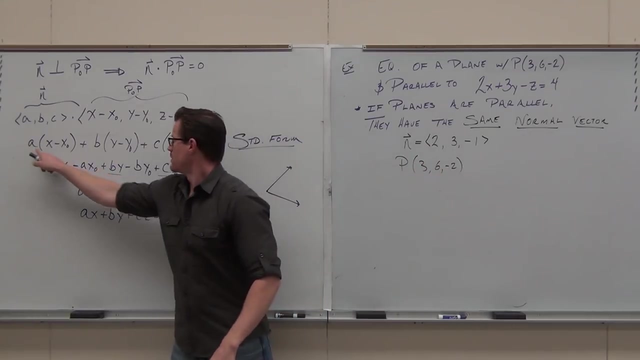 Literally. take these numbers, put them in this spot, Don't try to put it here. Put it here. We use this to get to here. It's easy to get the numbers screwed up. It really is. It's really easy to put these numbers here if you're not paying attention. 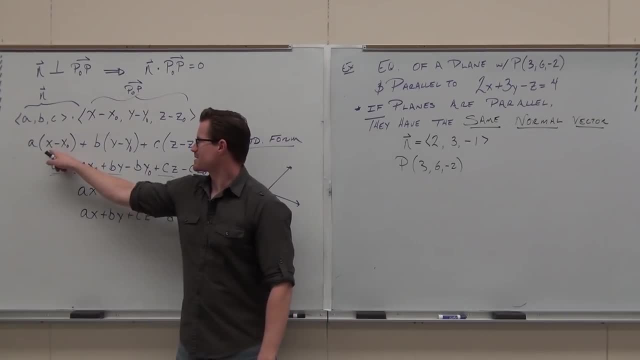 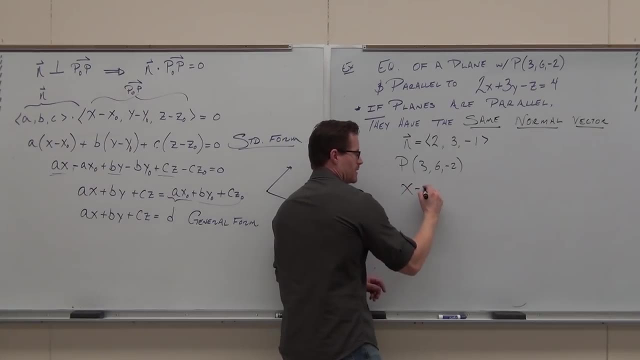 So here's how I always think about it: X's and X coordinates go together. That's what that stands for. So if I build it, I know I have to have an X minus 3, because that's the X point, That's X coordinate at that point. 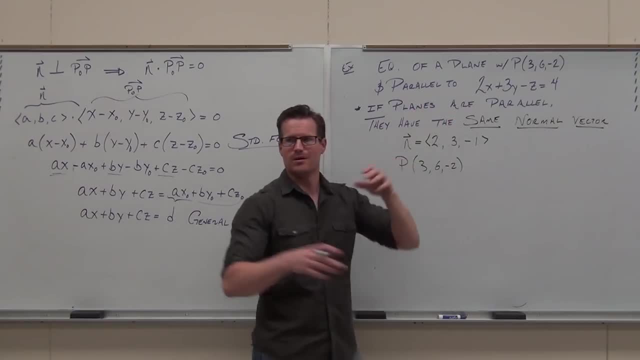 That's fine. So you use the same exact normal. So parallel Same normal, Parallel lines, same vector, Parallel planes, same vector. You see the connection. We need a point and a normal. We have a point and a normal and here's how to work with the rest of it. 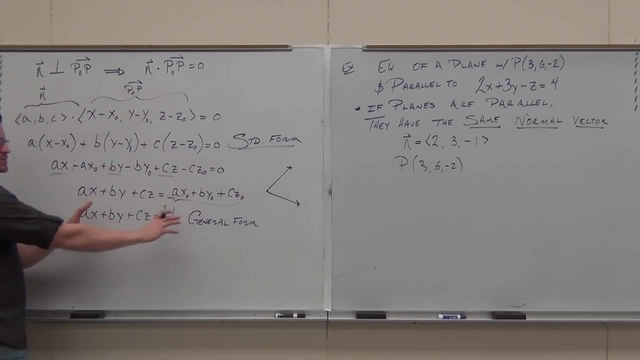 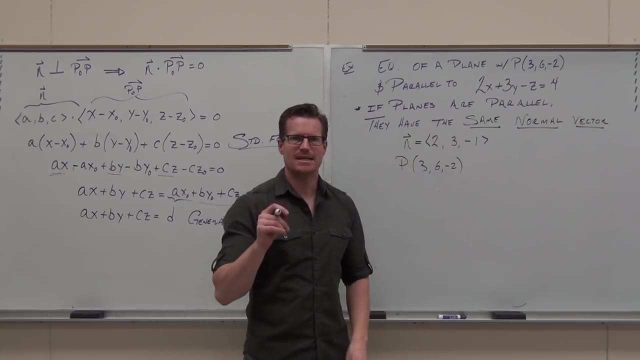 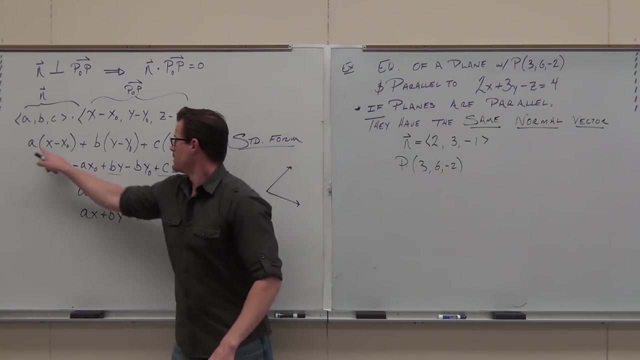 Literally. take these numbers, put them in this spot, Don't try to put it here. Put it here. We use this to get to here. It's easy to get the numbers screwed up. It really is. It's really easy to put these numbers here if you're not paying attention. 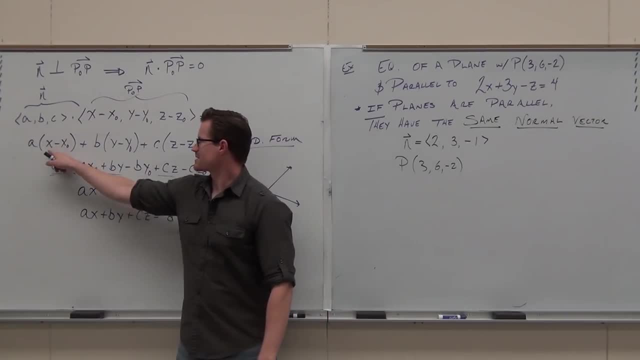 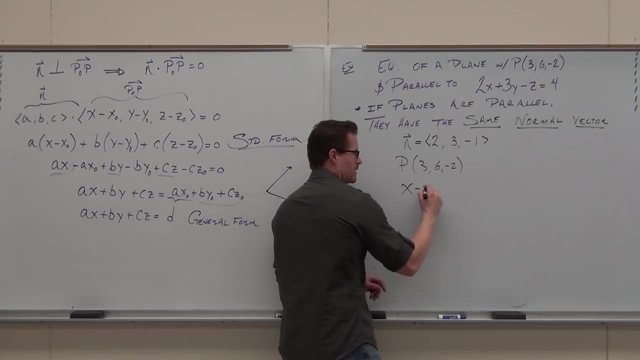 So here, Here's how I always think about it: X's and X coordinates go together. That's what that stands for. So if I build it, I know I have to have an X minus 3, because that's the X point. 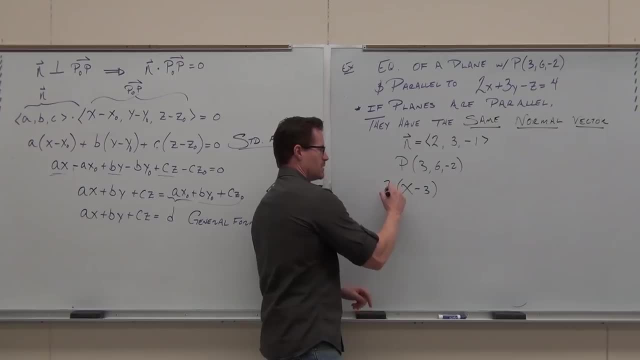 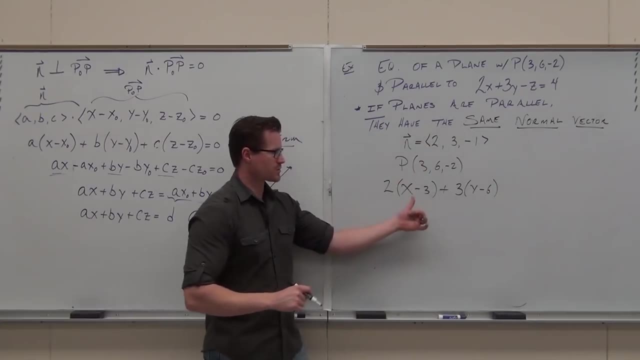 That's X coordinate at that point. And then the vector is what goes on the outside: X minus 3.. I have Y minus 6.. I get the 3 because that's my normal vector. I get the 3 because that's my normal vector. component for Y. 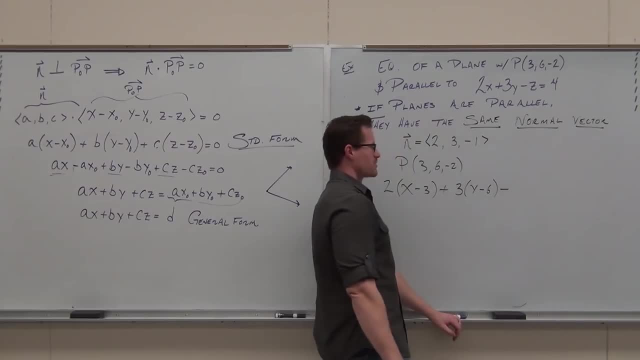 Am I going to have a plus or a minus? Should I do a plus or a minus? Watch your signs. And then Z plus 1, or, sorry, Z plus 2,, Z minus 2.. What's that? one Plus 2.. 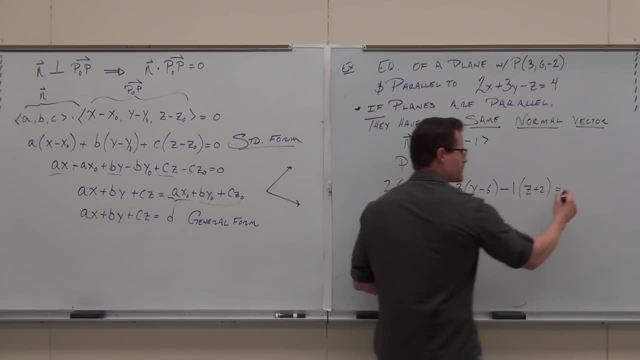 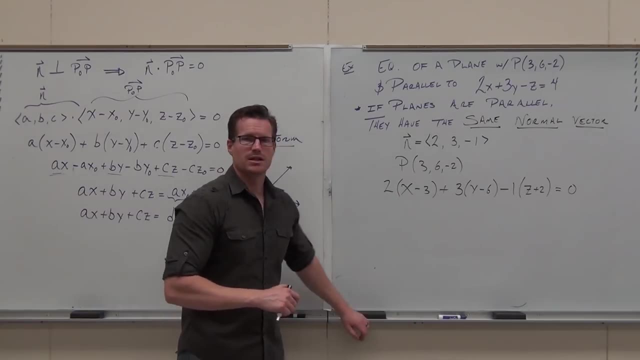 What's it equal? Does it have to equal something? Zero. Nature of the dot, product of perpendicular vectors. give you a zero. That's where it's built off of. Do you leave it like that? No, Heavens, no, Don't leave it like that. 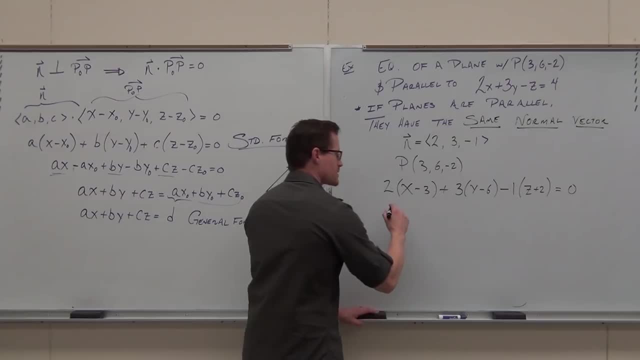 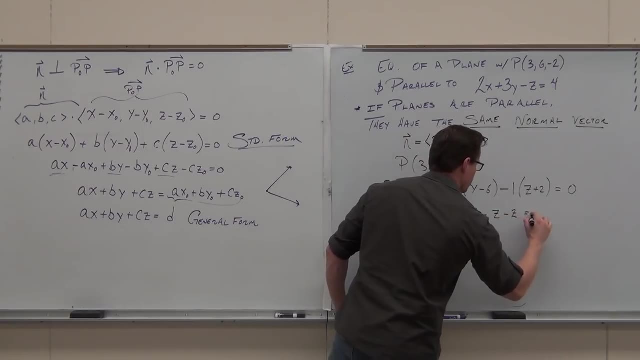 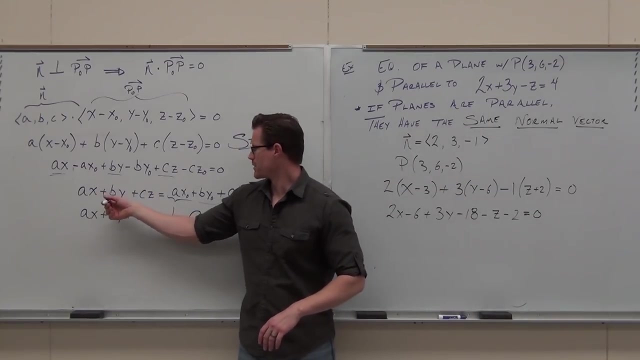 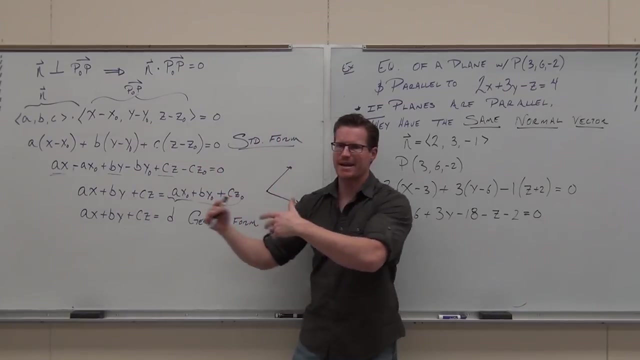 Distribute, get it into this form. So we're going to do it fast and then stop for a while. This is what we did right here, with all this junk hanging out, And then we took all the junk, this stuff, the sub-zeros, and we added it or subtracted it over. 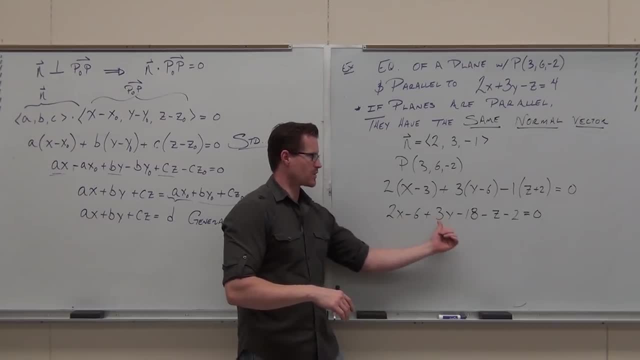 That's what's going on here, Okay. So right, here We have our 2X, we have our 3Y, we've got our minus Z, we've got our negative 6,, our negative 18, and our negative 2.. 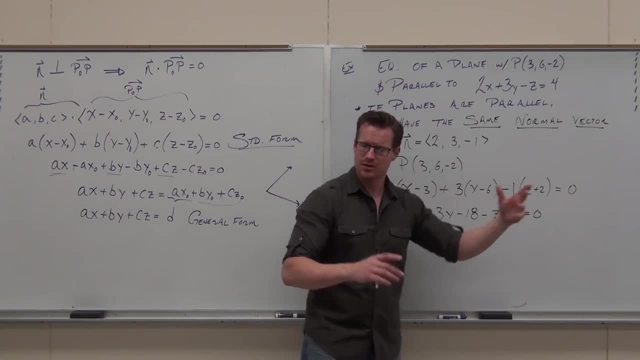 Take those numbers and move them. That's what I want to see. I'm going to do it all at once. I think that we get- let's see- negative 26 over here, So when I add it, it becomes positive 26.. 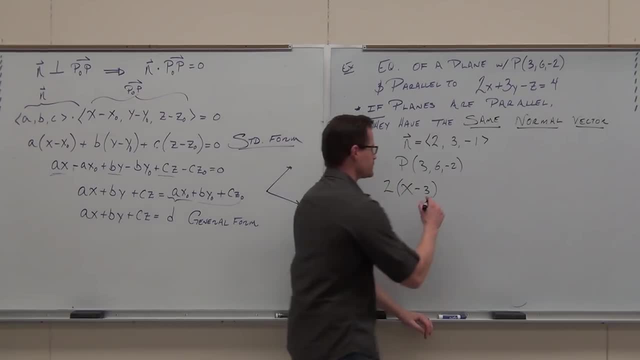 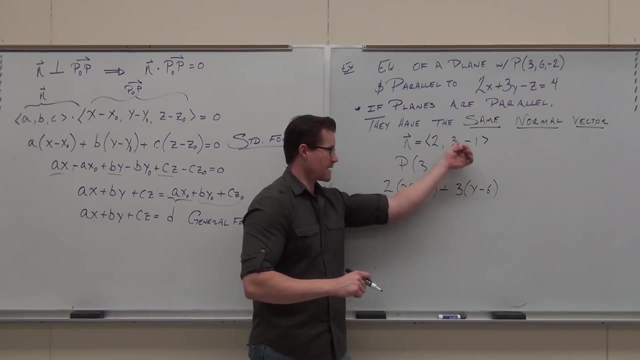 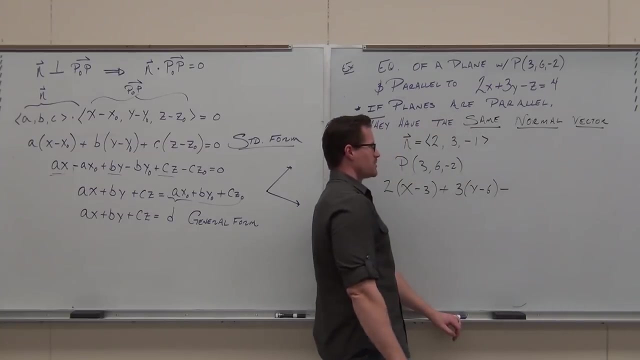 And then the The vector is what goes on the outside: X minus 3.. And I have Y minus 6.. I get the 3 because that's my normal vector component for Y. Am I going to have a plus or a minus? 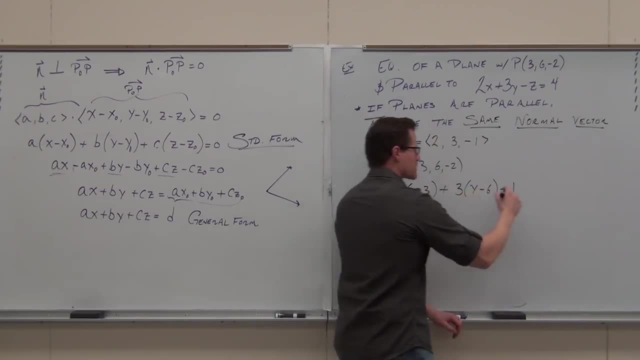 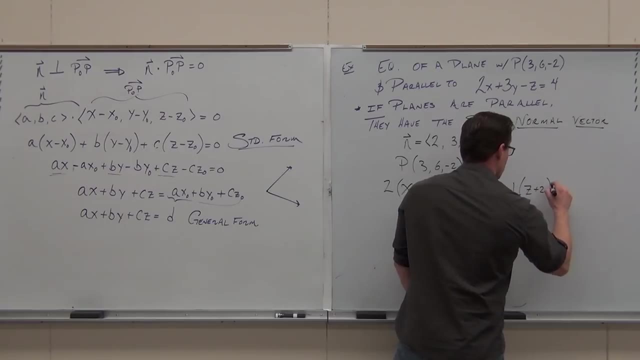 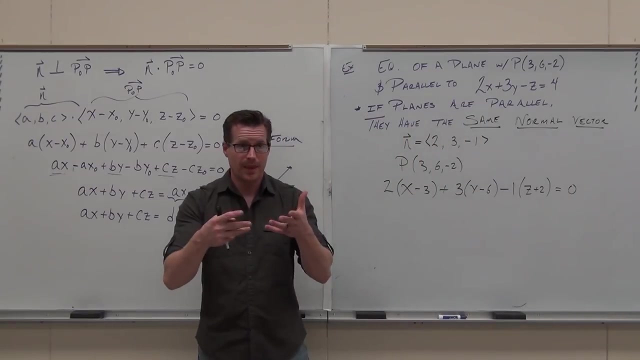 Should I do plus or minus? Watch your signs And then Z plus 1.. Sorry, Z plus 2,, Z minus 2.. What's that one? What's it equal? It's going to equal something. Nature of the dot, product of perpendicular vectors. give you a 0.. 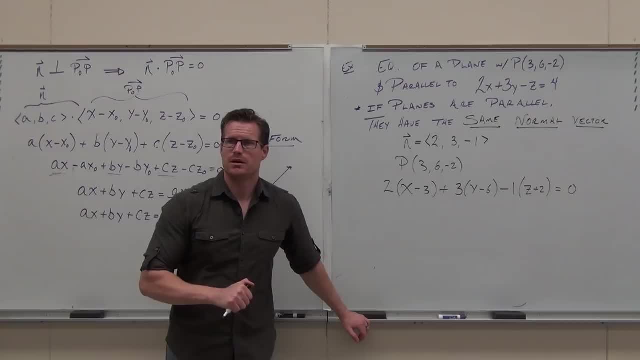 That's where it's built off of. Do you leave it like that? No, Heavens, no, Don't leave it like that. Distribute, get it into this form. So we're going to do it fast and then stop for a while. 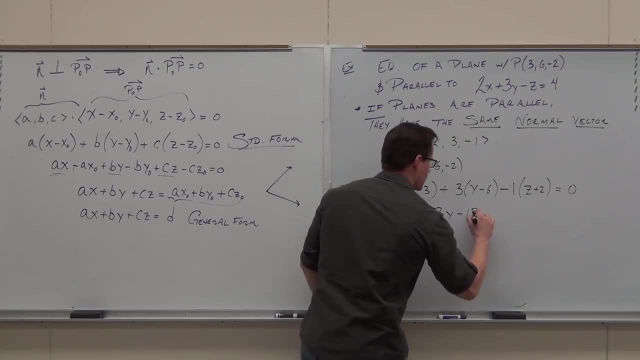 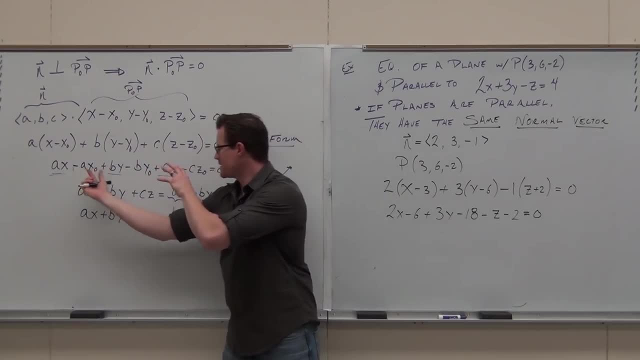 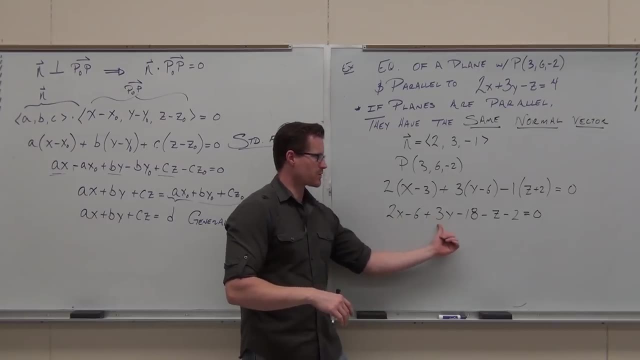 And then we took all the junk, This stuff, the sub-zeros, and we added it or subtracted it over. That's what's going on here. So, right here we have our 2X, we have our 3Y, We got our minus Z, We got our negative 6 and our negative 18 and our negative 2.. 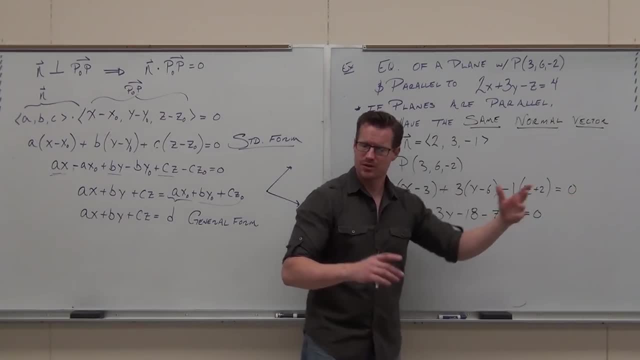 Take those numbers and move it. That's what I want to see. I'm going to do it at once. I think that we get- let's see, Let's see- negative 26 over here. so when I add it, it becomes positive 26.. 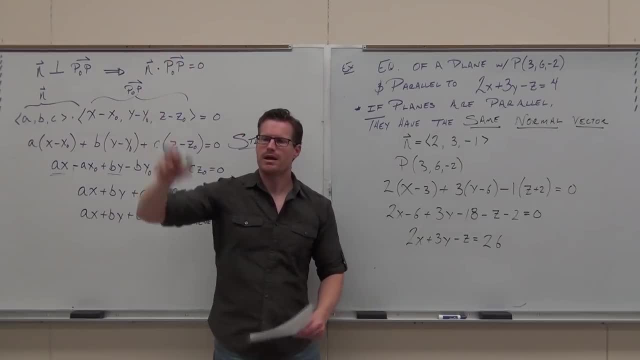 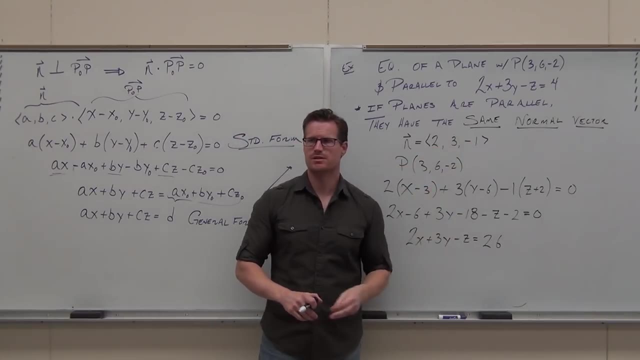 So I think we're okay with that one. Hey, here's a way to check your work. Look here, look at the vector you used for your normal. If you don't have the same exact numbers, you've done something wrong. 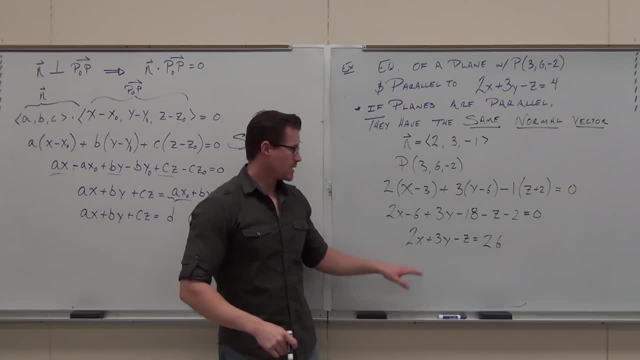 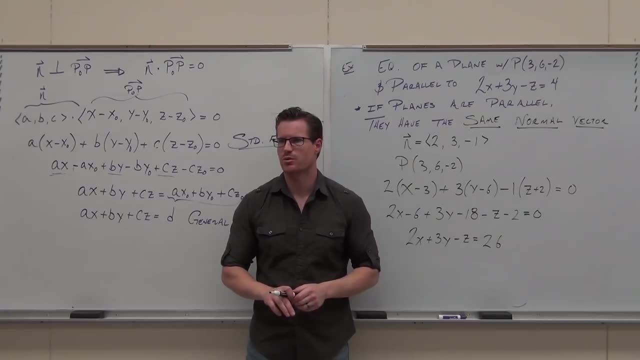 Hey, here's a way to check your work. Look here: Look at the vector You use for your normal. If you don't have the same exact numbers, you've done something wrong. That's how to check your work really fast. 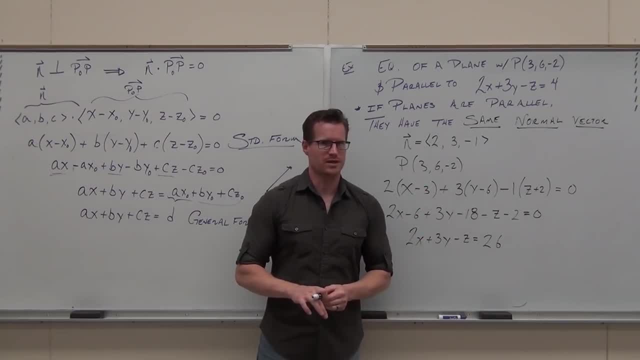 If you have these numbers and these spots, you've done something majorly wrong. Does it make sense to you From here on out? it's going to be a lot of practice, but we're going to take a break for a little bit. 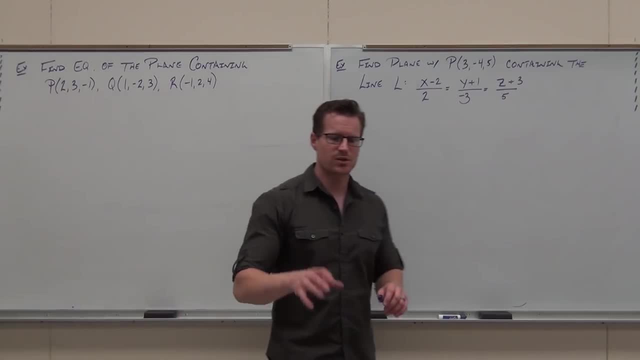 Okay, Hey, our time for a lot of practice, As we were just talking about the two biggest things you need is a point and a normal vector. So in the next examples, that's really all we're going to be talking about- is how to find the point. 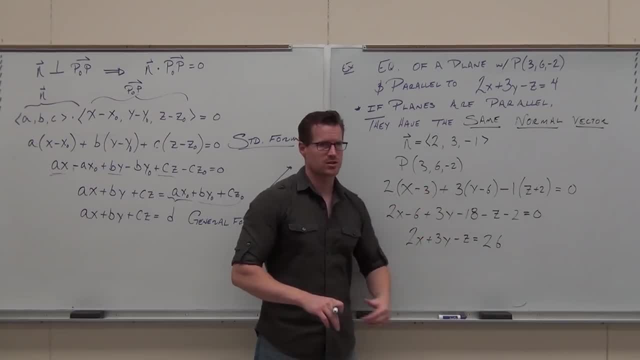 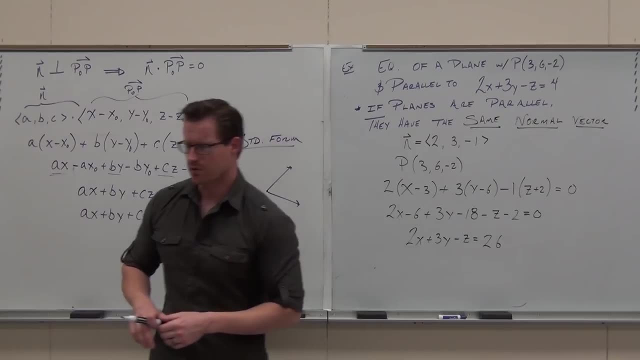 That's how to check your work really fast. If you have these numbers and these spots, you've done something majorly wrong. Did it make sense to you? From here on out, it's going to be a lot of practice, but we're going to take a break for a little bit. 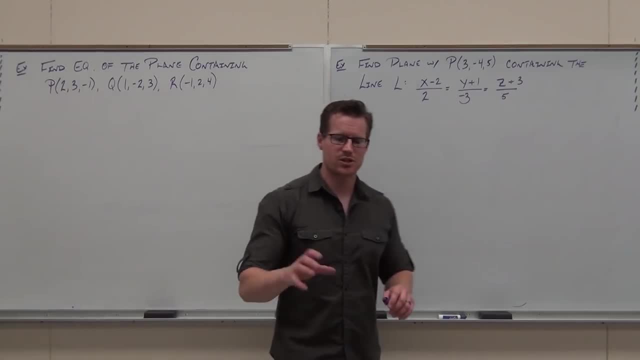 Okay, hey, our time for a lot of practice, As we were just talking about, the two biggest things you need is a point and a normal vector. So in the next examples, that's really all we're going to be talking about. 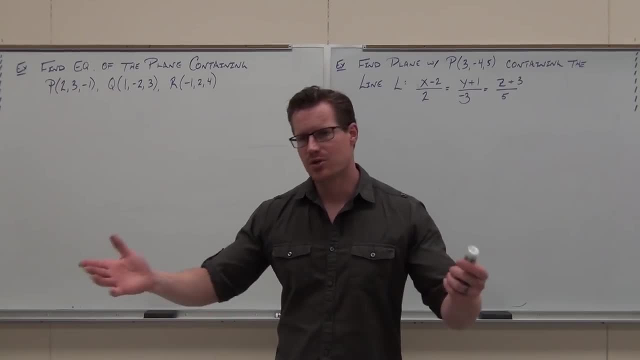 is how to find the point, how to find the normal vector, because if you can find that you have the equation for plane, It's like point slope, It's not bad. So let's take a look at this one. Find the equation of a plane contained in three points. 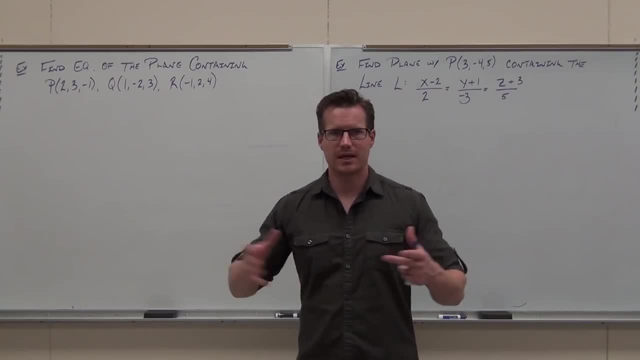 Kind of gave it away last time, but when we talk about a plane contained in three points, the idea is: you need a. what do you need for a plane? Come on, what do you need? Point and normal vector. Do you have a point? 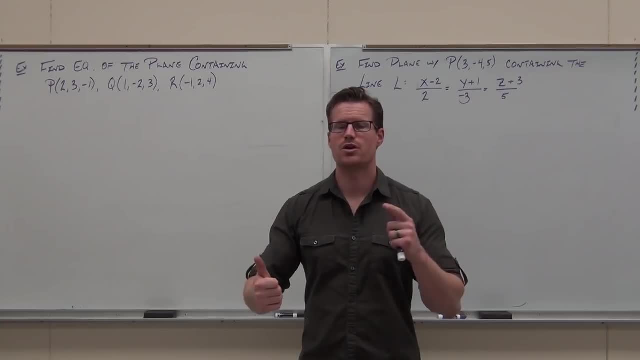 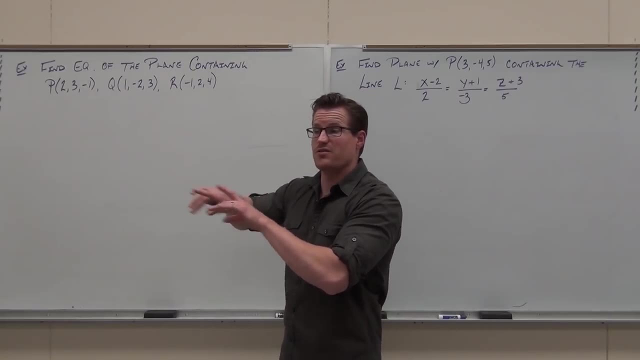 Now you've got three of them. Do you get a normal vector? No, No. Can you find one? Yes, Yeah. So if I give you three points, the idea is let's figure out what the vectors are and connect those three points. 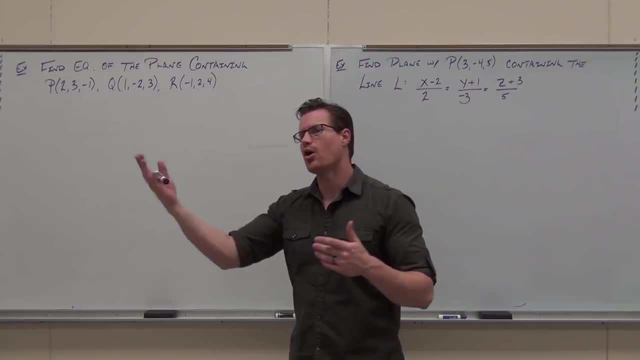 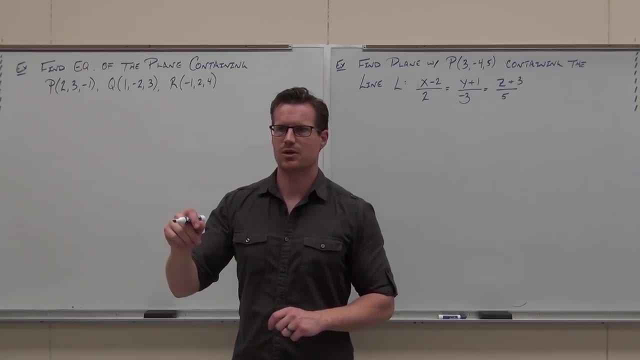 And then if I have two vectors, a cross product always gives us a normal. There's one advice, though: You've got to use the same point twice. So if you're going to go P to Q, you've got to go P to R, because you need that cross product. 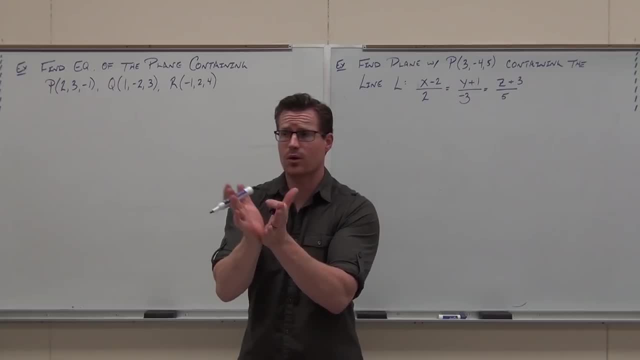 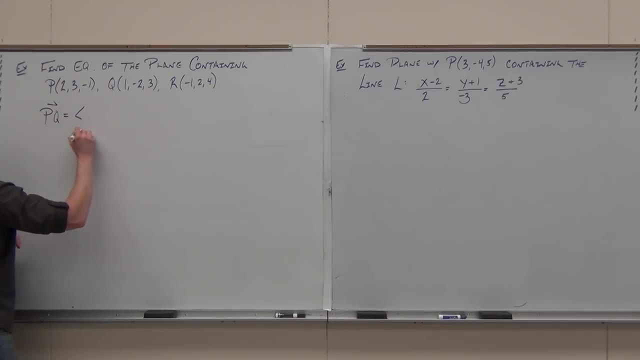 to actually work from that. let's call it a pivot point. okay, from that point, P or Q or R, it doesn't matter, but I'm going to do it this way. So I'm going to find PQ, that vector, from P to Q. 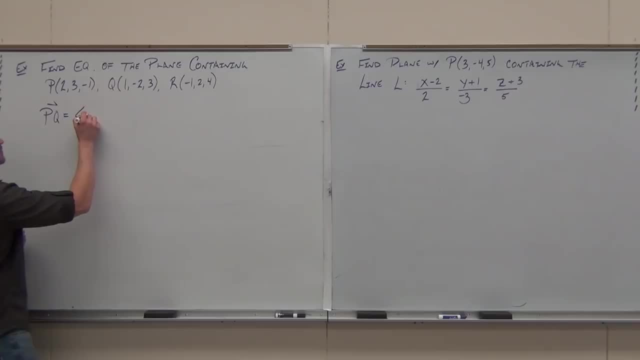 You guys help me out with it. Come on, let's work quickly. but let's work. What is it? One, One, negative five, One. That's the vector from P to Q, for sure, and not if you're okay with that one. 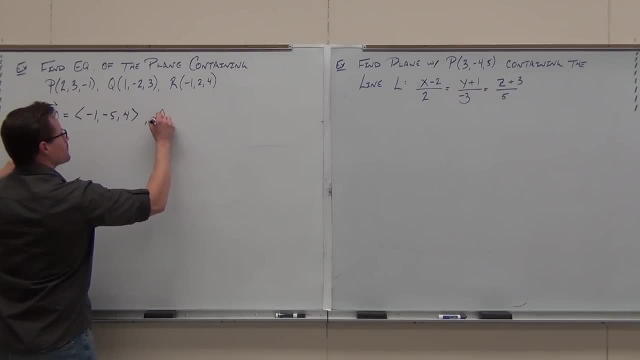 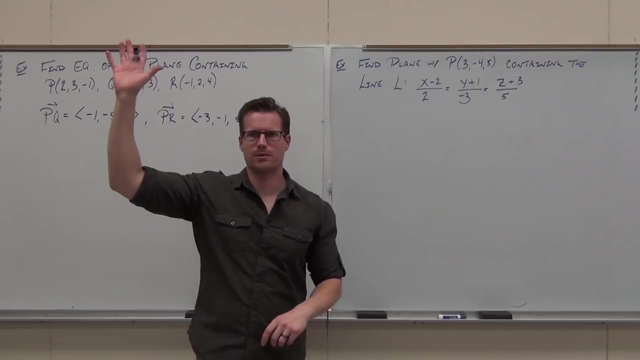 The vector from which should I go? from Q to R, Q to R, P to R, P to R? okay, same one. What's that? Negative three, Negative four? On time, Beautiful. Now, what are those vectors? 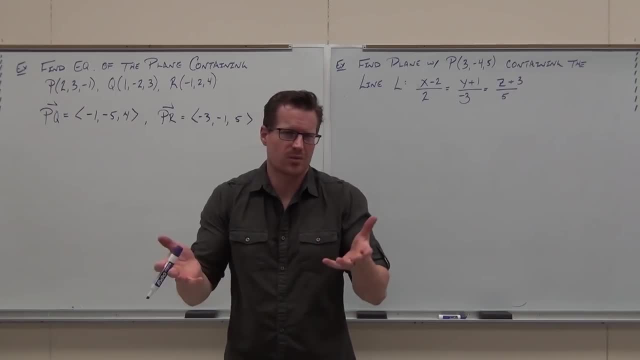 Where are they On the plane? They're in the plane. Yeah, they're on the plane, in the plane. same thing, They're on the plane. Are they a normal vector? No, No, but if I take them and I, what's that thing again. 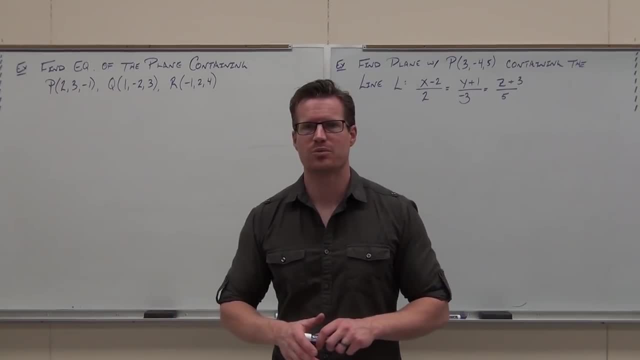 how to find the normal vector, because if you can find that you have the equation of a plane, It's like point slope, It's not bad. So let's take a look at this one. Find the equation of a plane contained in three points. 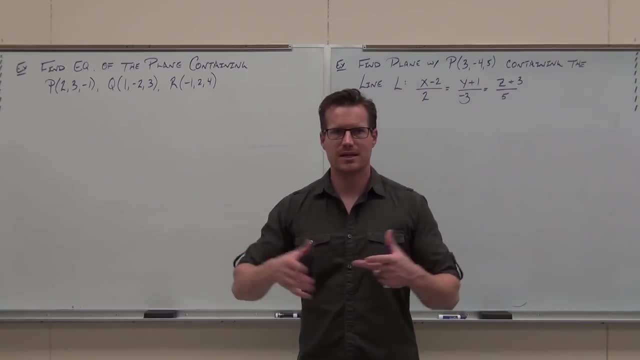 Kind of gave it away last time, but when we talk about a plane contained in three points, the idea is: you need a. what do you need for a plane? Come on, What do you need? Point and normal vector. Do you have a point? 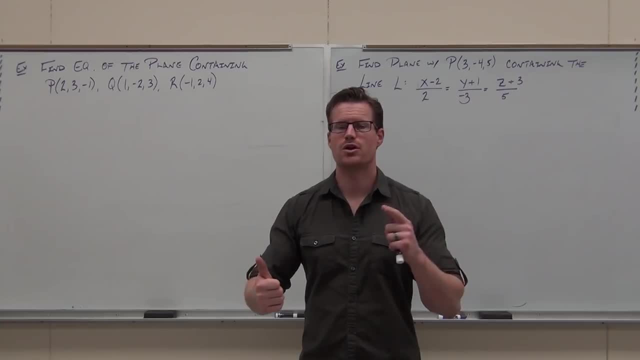 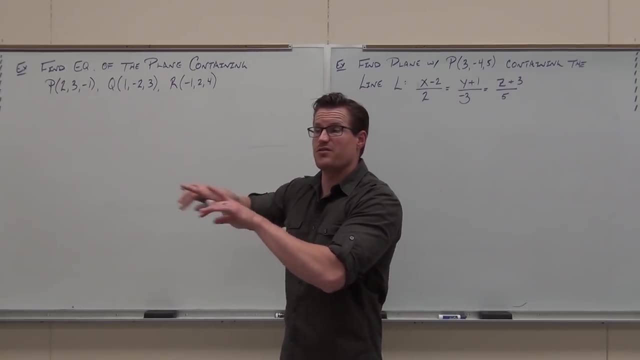 Yes, Now you've got three of them. Do you get a normal vector? No, No, Can you find them? Yes, Yes, Yeah. So if I give you three points, the idea is: let's figure out what the vectors are. 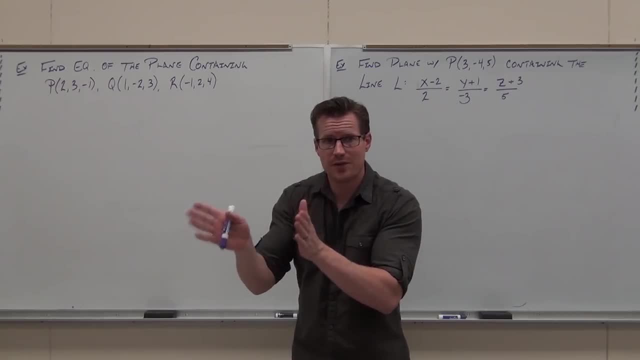 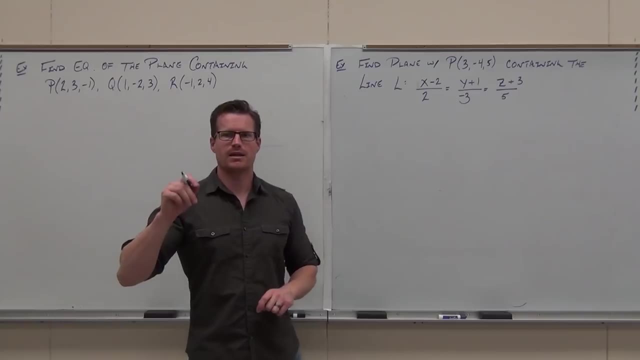 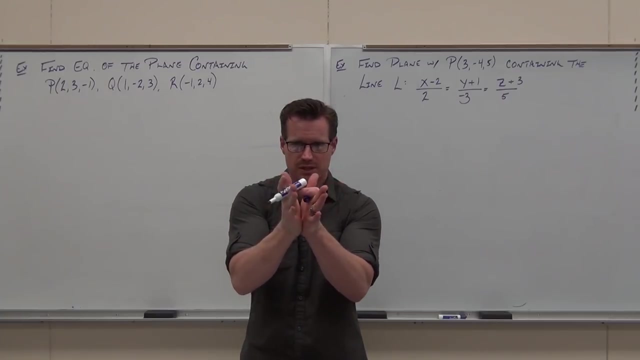 that connect those three points, and then, if I have two vectors, a cross product always gives us a normal. There's one advice, though: You've got to use the same point twice. So if you're going to go P to Q, you've got to go P to R, because you need that cross product. 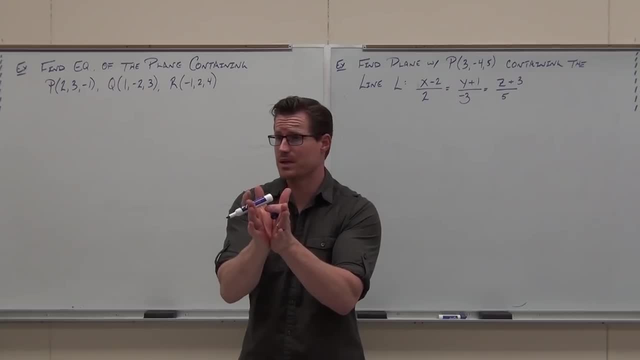 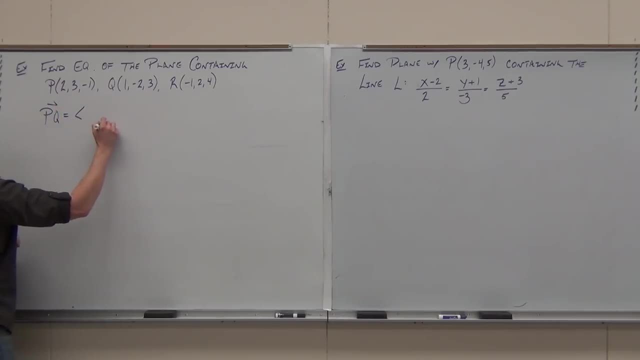 to actually work from that. Let's call it P to R, Let's call it a pivot point. okay, from that point, P or Q or R, it doesn't matter, but I'm going to do it this way. So I'm going to find PQ, that vector, from P to Q. 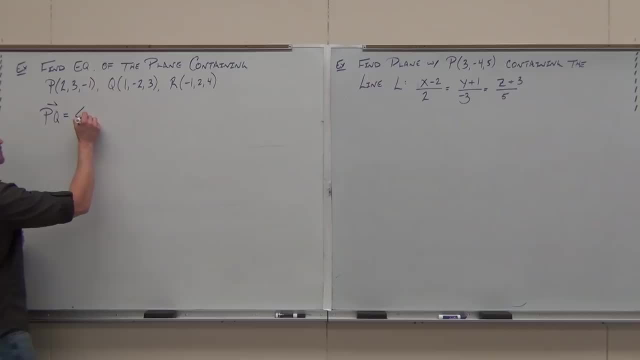 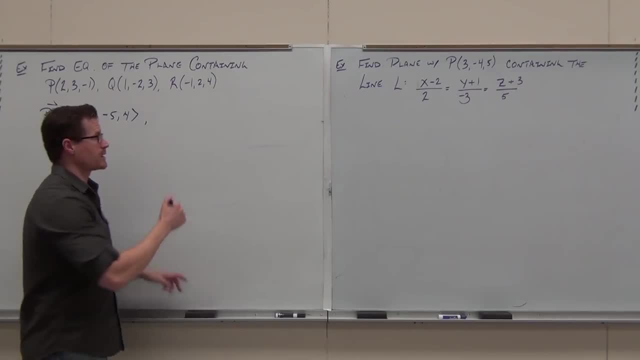 Yes, Q to R, Q to R, P to R, P to R. Okay, same one. What's that Negative? 3. Negative, 4. On time, Beautiful. Now, what are those vectors? Where are they? 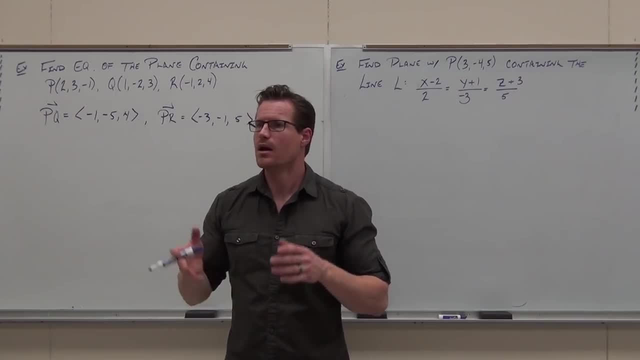 On the plane? They're in the plane. Yeah, they're on the plane. in the plane, something They're on the plane. Okay, are they a normal vector? No, No, but if I take them and I what's that thing again. 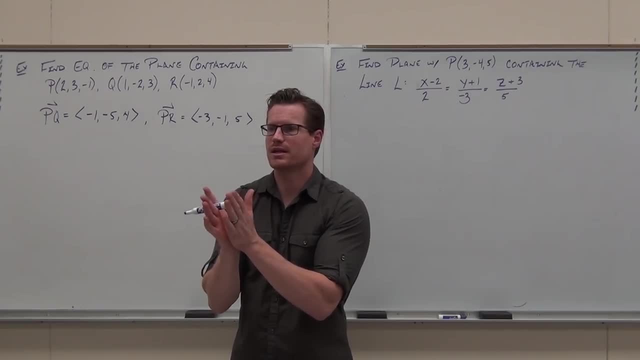 Cross product them. A cross product gives us a vector that's orthogonal to both of them. If it's orthogonal to both of them, they're both in the plane. it's orthogonal to the plane, so it's a normal vector. So let's go ahead, let's find it. 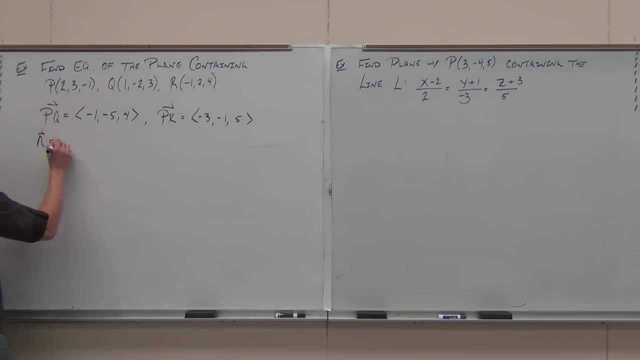 Our normal vector is going to be the cross product of whatever vector connects your, whatever two vectors connect your three points In this case. I can't even write anymore- P, Q and P R. Now here's a good question. 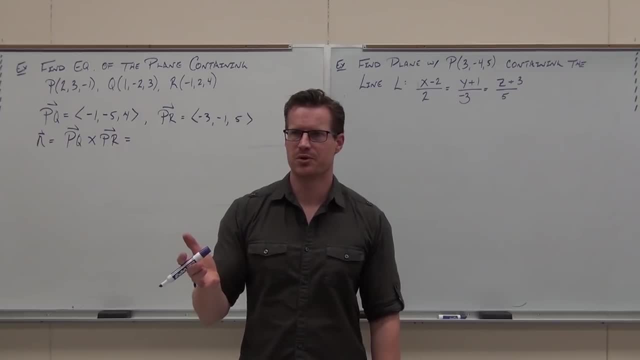 Do you know how to do a cross product? I think I pretty much murdered you with homework enough that you you can do this like in your sleep. I hope I did, unless you, the calculators do it too, I think, so you can do that. 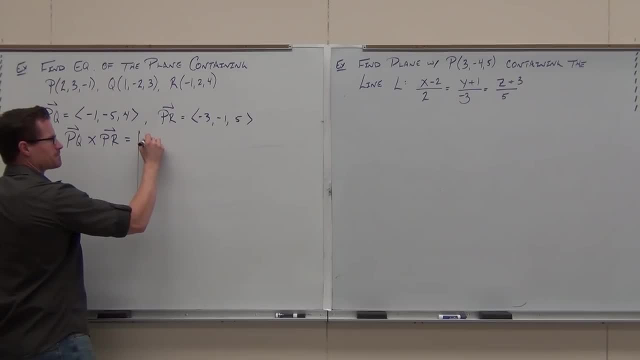 What do you start with? I, I do J, J, A or a, A or K, K, K, F, F. I'm going to ask you a kind of interesting question: Does the order matter? Does the order matter? 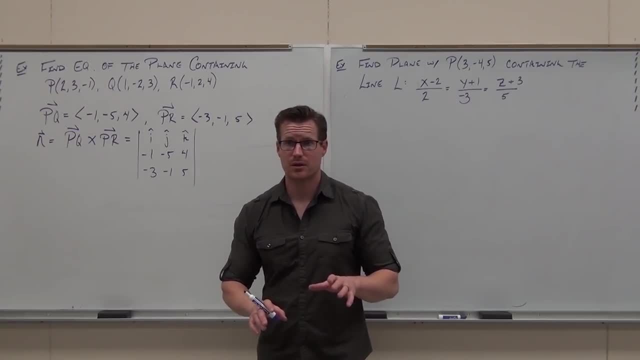 I mean ultimately- I know I'm going to get a different answer, but does the order matter? Would a normal vector going this way be any different than a normal vector going this way? Only by the sign And since, as we can factor out scalar multiples. 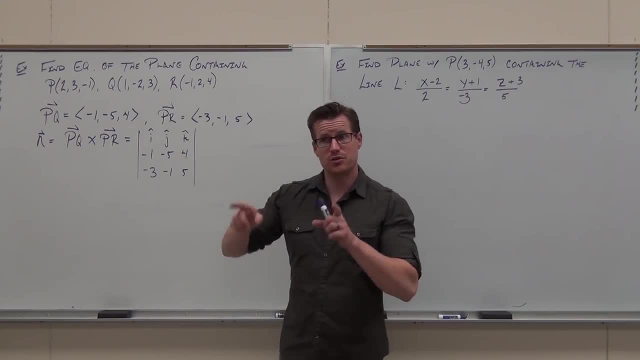 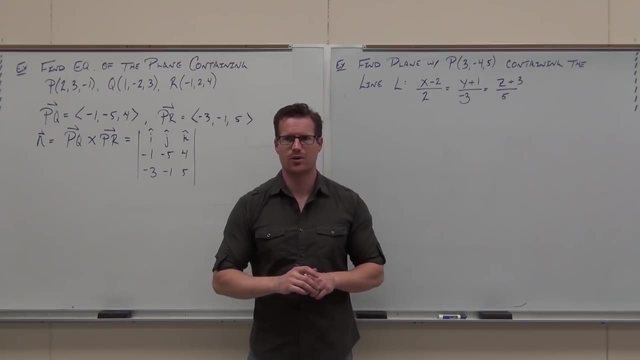 it doesn't really matter. It doesn't matter. It doesn't matter at all. As long as you have two vectors in the plane and you are starting from the same point, cross product them, you're going to find a normal vector. That's all we're looking for. 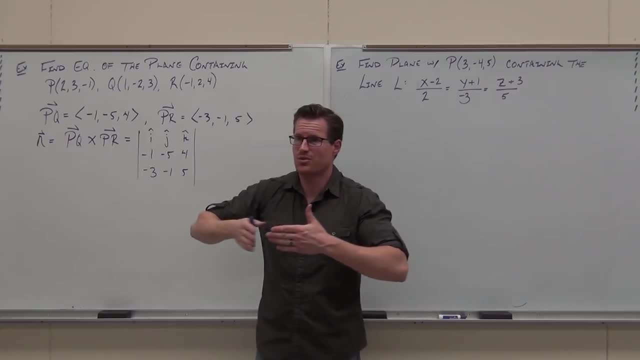 In fact it probably doesn't even matter that you start with the same point, because if you cross product any two vectors in the plane, you're going to get a normal vector. I just like to do it, so the cross product makes a little more sense. 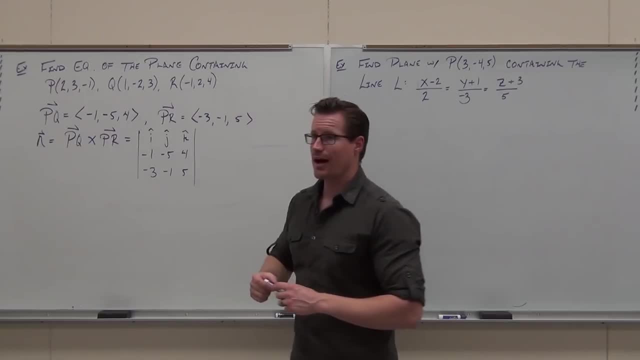 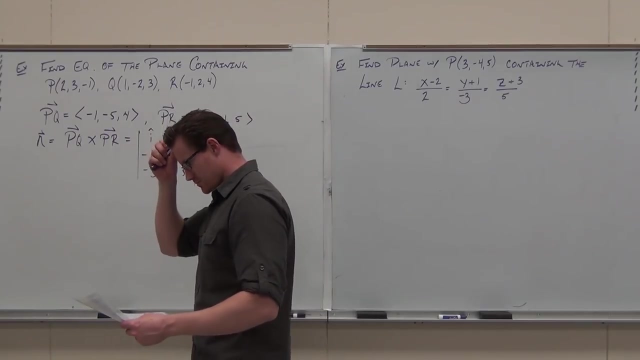 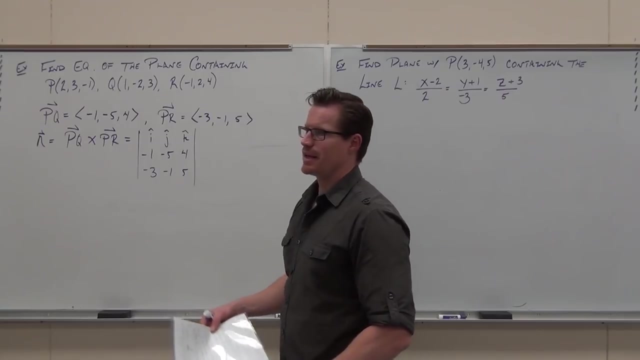 Does that make sense to you? Probably makes sense. I'm hoping that you've been doing as I've been rambling. Have you been doing as I've been? You haven't Darn you. people Do as I ramble. So the idea again, as you're working. 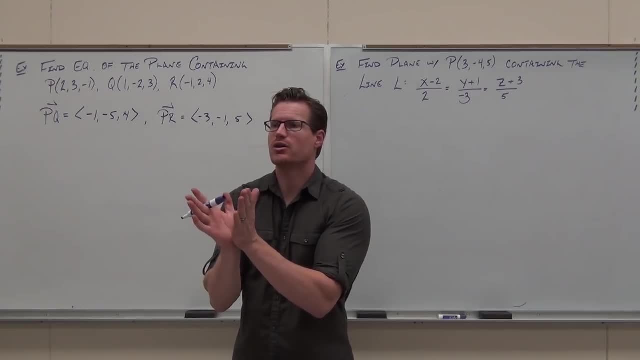 Cross product them. Cross product them. Cross product gives us a vector that's orthogonal to both of them. If it's orthogonal to both of them- and they're both in the plane- it's not orthogonal to the plane, so it's a normal vector. 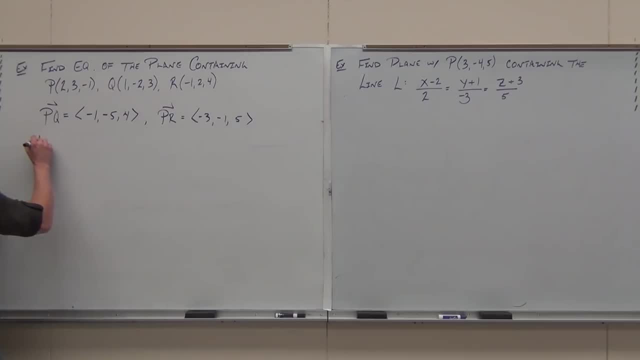 So let's go ahead and let's find it. Our normal vector is going to be the cross product of whatever vector connects your whatever two vectors connect your three points. In this case I can't even write anymore- PQ and PR. Now here's a good question. 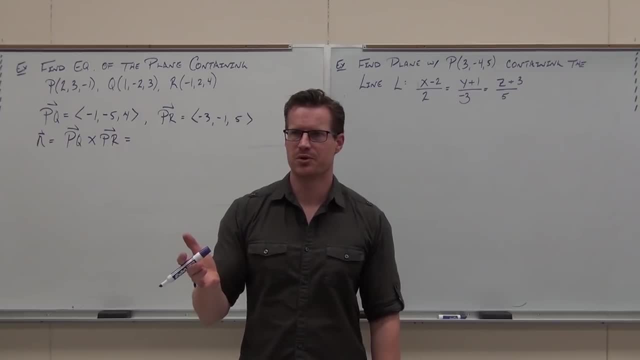 Do you know how to do a cross product? I think I pretty much murdered you with homework enough that you can do this, like in your sleep. I hope I did. Let's see calculators do it too, I think. so you can do that. 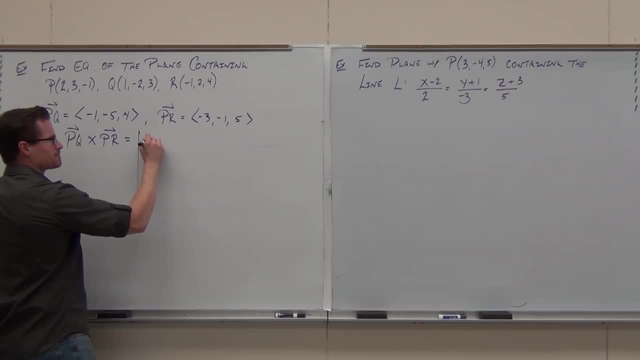 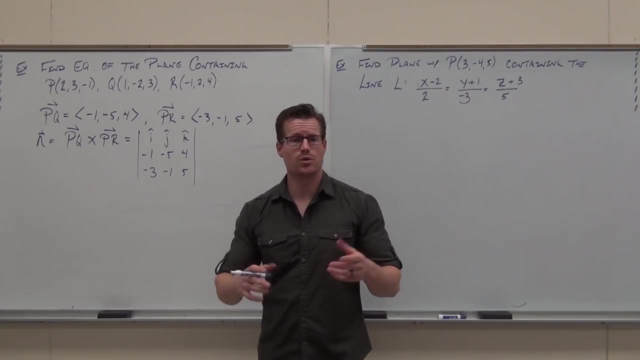 What do you start with? I J S Ste N J S N Fi S I Sil Ja O K P L News. I'm going to ask you kind of an interesting question. Does the order matter? does the order matter? I mean ultimately- I know I'm going to get a different answer, but does the order matter? Would a normal vector going this way be any different than a normal vector going this way? Only by the sign, and since we can factor out square the multiples, it doesn't really matter. 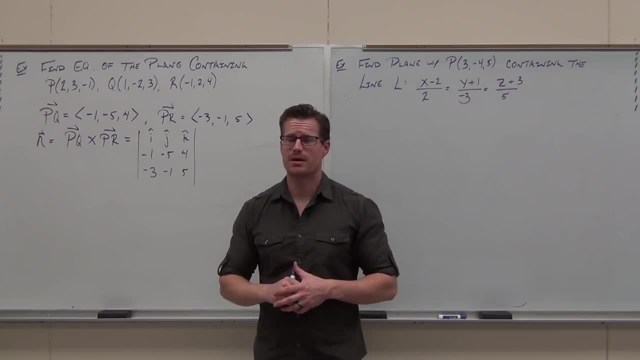 It doesn't matter. it doesn't matter at all as long as you have two vectors in the plane and you are starting from the same point cross while getting red on the side. This really shortens it. This is sure I know, but I think it's beautiful. 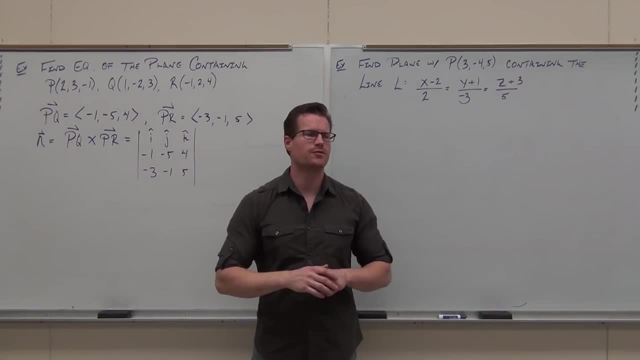 you are starting from the same point. cross product them, You're going to find a normal vector. That's all we're looking for. In fact, it probably doesn't even matter that you start with the same point, because if you cross, product any two vectors, 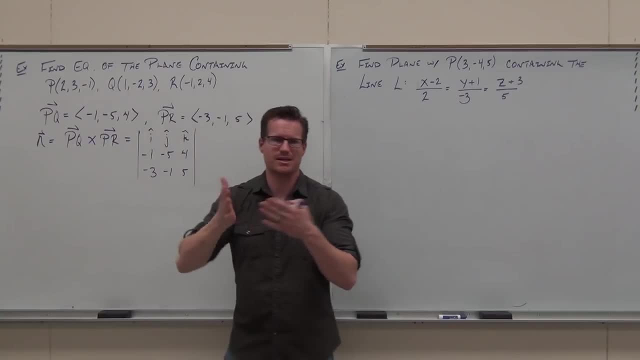 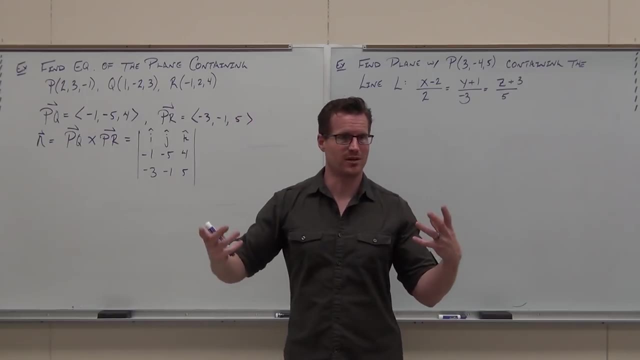 in the plane. you're going to get a normal vector. I just like to do it so the cross product makes a little more sense. Does that make sense to you? Hopefully it makes sense. I'm hoping that you've been doing as I've been rambling. 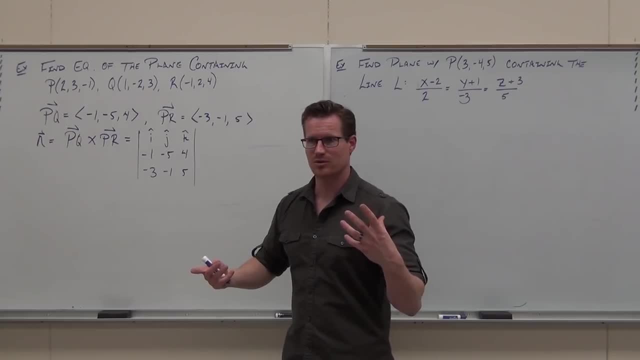 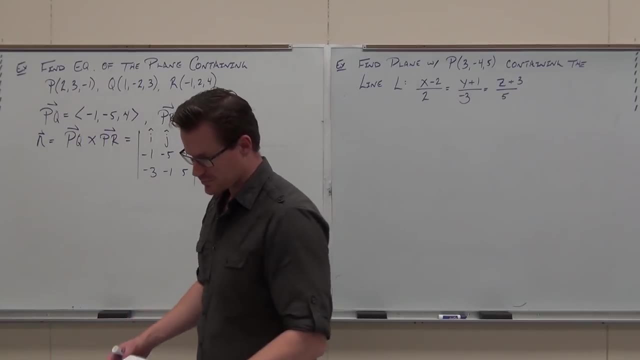 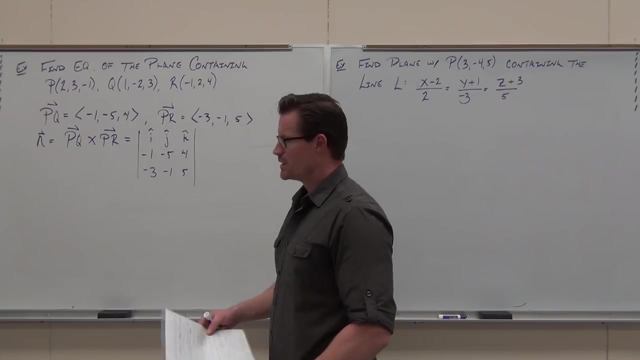 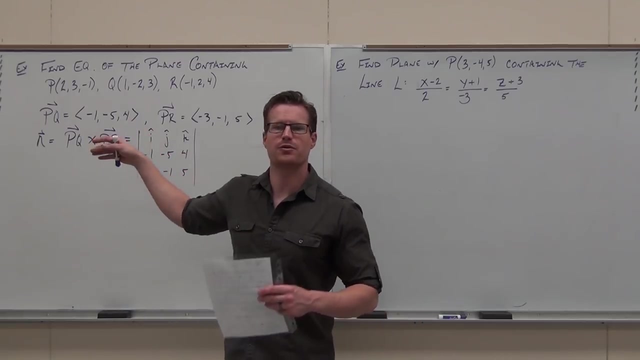 Have you been doing as I've been? You haven't, Darn you. people Do as I ramble. So the idea again: as you're working, because I know it's going to take a little time. as you're working, I don't care about vectors in the plane. 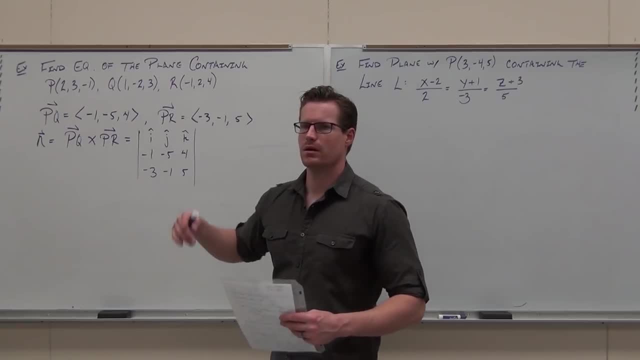 because I know it's going to take a little time as you're working. I don't care about vectors in the plane, for the nature that they're in the plane, That doesn't help me. So that's in the plane, yeah. 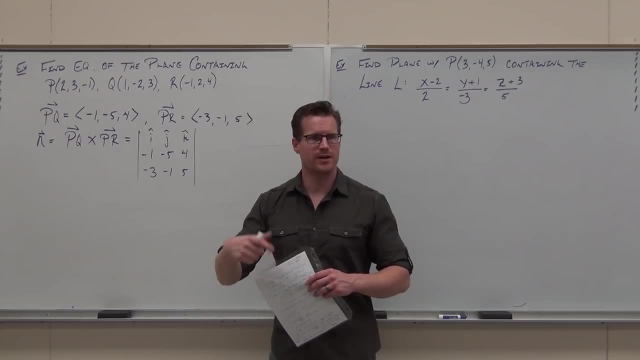 That's in the plane. Yeah, That's not how we define planes. So whenever we find two vectors in the plane, that's great, Cross product them. So when we need a normal, not just a vector, So if I cross product these two vectors. 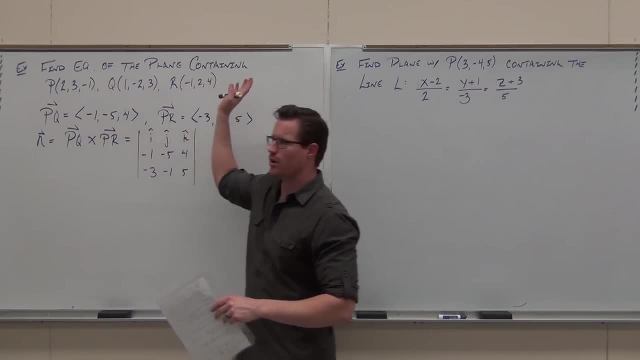 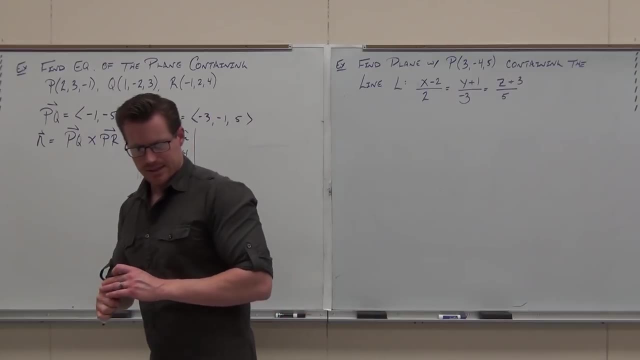 that's what's giving me my normal. Then I'll have a point, any one you want, And I'll have a normal, the thing that we just worked so hard to find, and that's how we define our plane. So let's see. 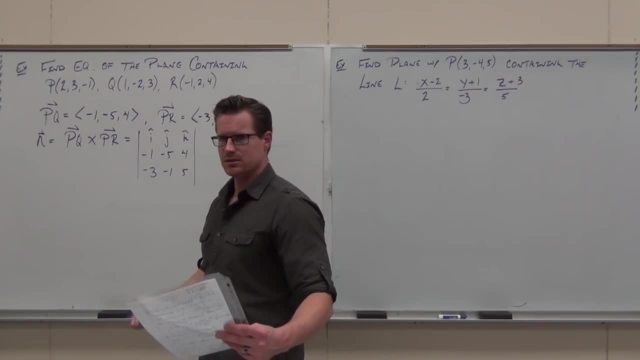 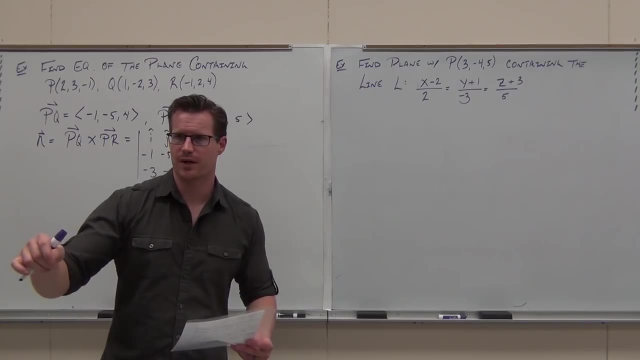 What did you get, Man? what did you get? I'm just going to give you answers from now on. I can't afford to go through all the work like, oh, over and, over and over again. So do you all feel comfortable on finding the cross product? 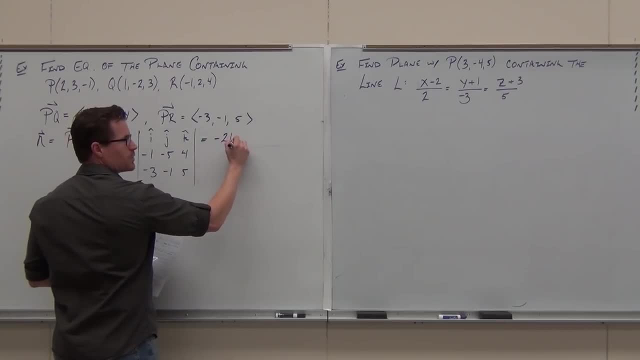 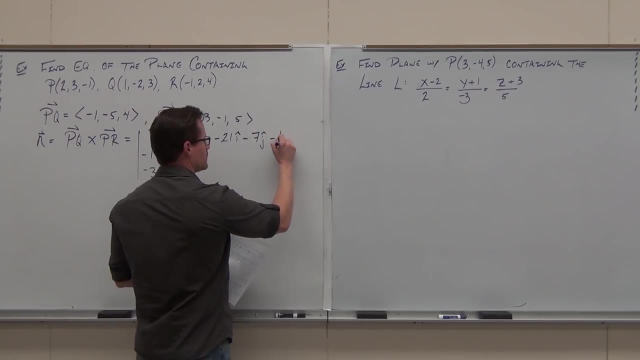 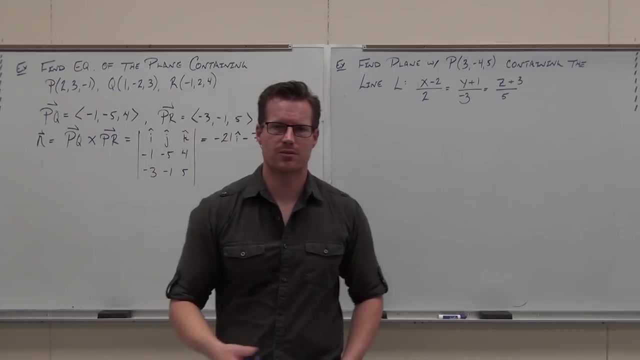 Yes, Okay, what I got out of this was negative 21i minus 7j minus 14k. Did you get the same thing? Yes, I mentioned something earlier. You notice it's going to be a lot of recap, but I mentioned something earlier. 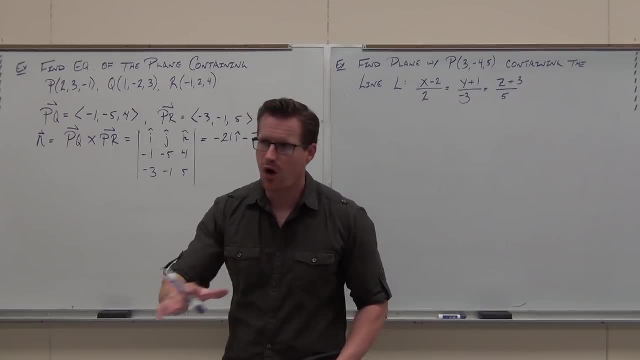 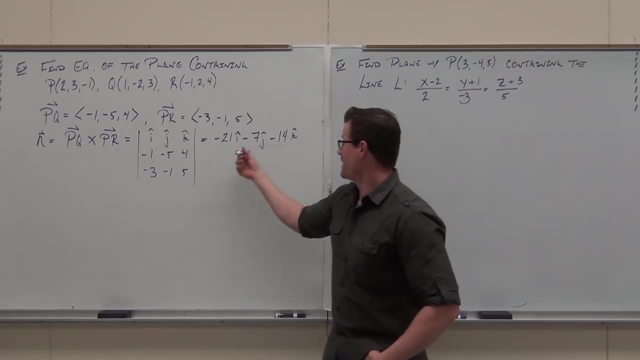 You can manipulate your vectors, as long as they don't- as long as they don't- deal with a distance. This doesn't deal with a distance, It's just a direction. That's nasty, folks, That's nasty. Can you make it look better, more, better? 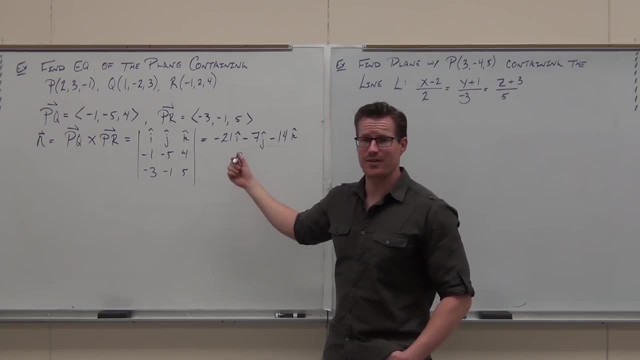 Make it look more better. How are you going to make it look more better? I'd factor the negative, for sure, and the 7.. So, if I do that, what's it doing? Well, it's taking this vector, and it's, it's, it's, it's. 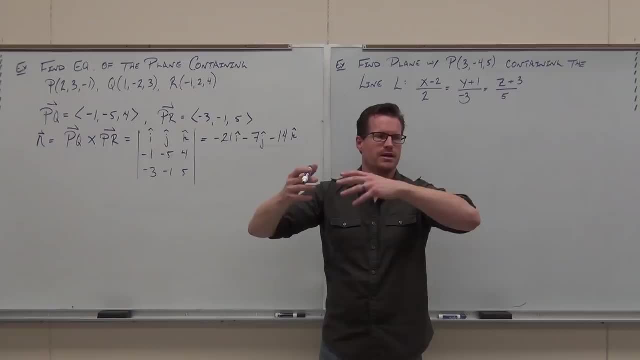 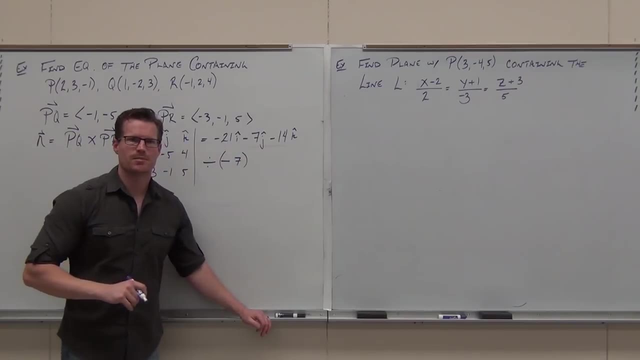 who would have heard? And it's shortening it. Who cares? It's still a normal vector, It's still orthogonal to that plane. Is that logic making sense to you? If you reversed these and did the cross product backwards, it'd be plus, plus, plus. 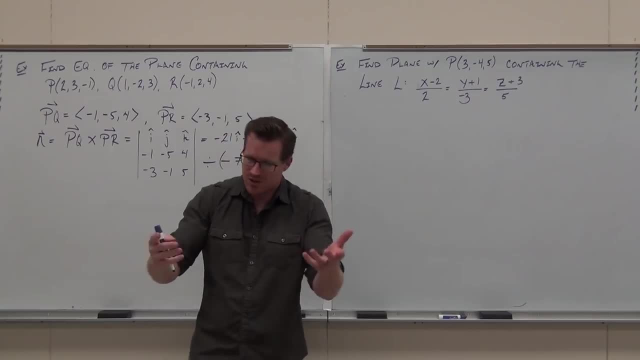 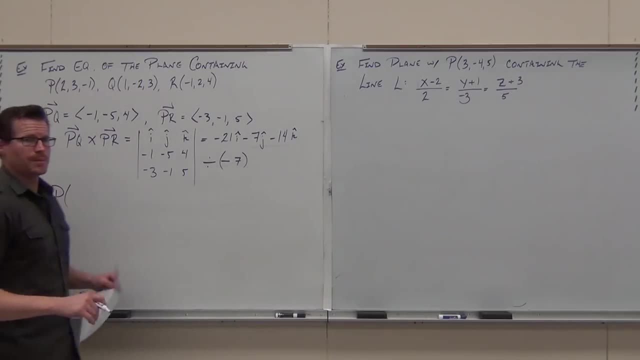 You'd still have to factor out the 7.. But you see, it doesn't matter, You can always change the, the scalar multiple of that. So again, two things we need for a plane order. two things quickly. What are they? 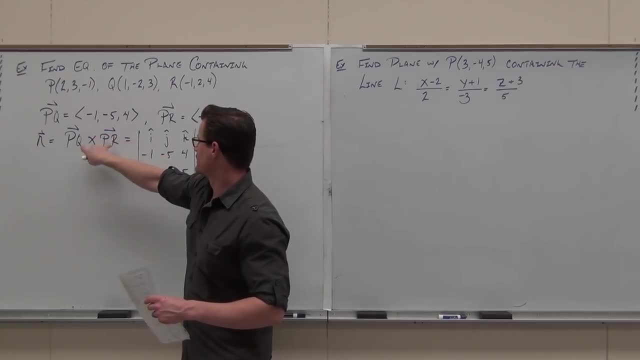 for the nature that they're in the plane. That doesn't help me. So that's in the plane. yeah, That's in the plane. yeah, That's not how we define planes. So whenever we find two vectors in the plane, that's great. 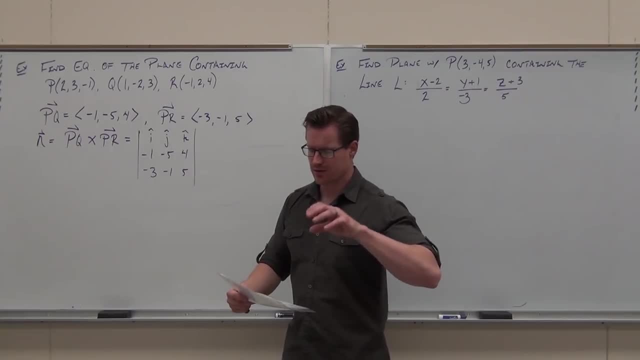 Cross product them. So when we need a normal, not just a normal vector, we need a normal vector, Not just a vector. So if I cross product these two vectors, that's what's giving me my normal- Then I'll have a point, any one you want. 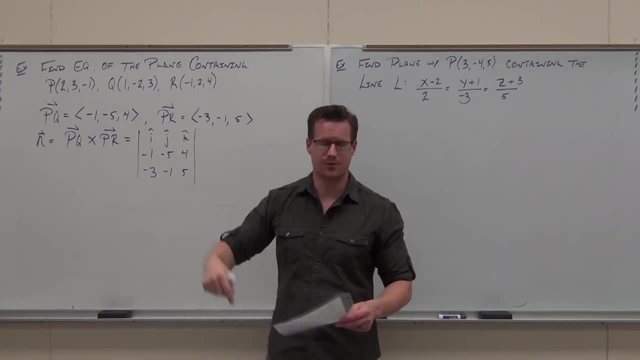 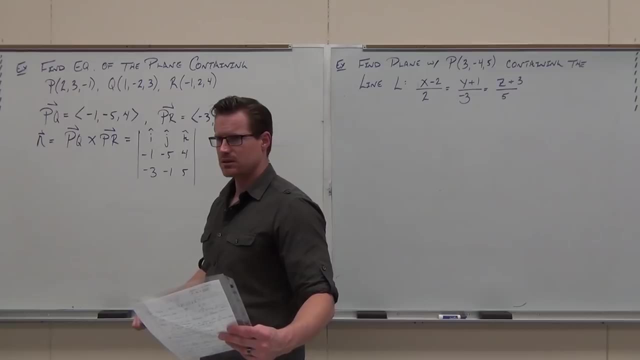 And I'll have a normal, the thing that we just worked so hard to find, and that's how we define our plane. So let's see. What did you get, Man? what did you get? I'm just going to give you answers from now on. 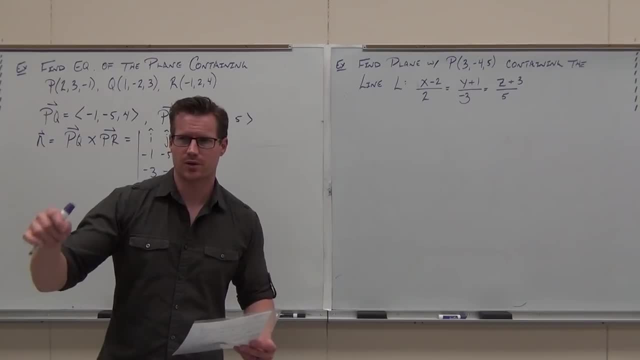 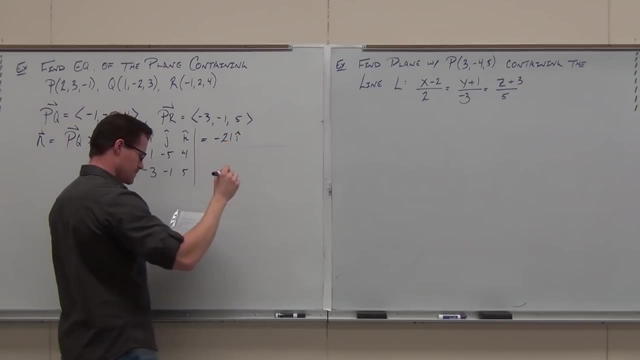 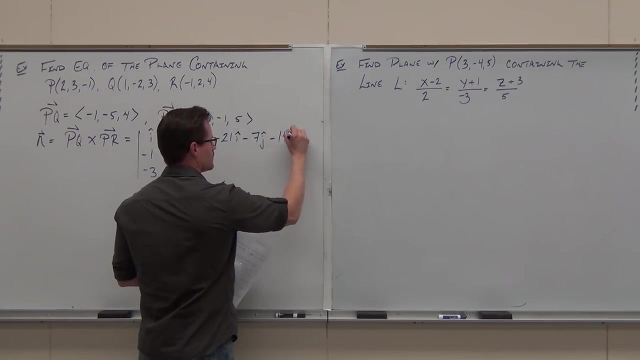 I can't afford to go through all the work like over and over and over again. So do you all feel comfortable on finding the cross product? Yes, Okay, what I got out of this was negative 21i Minus 7j, minus 14k. did you get the same thing? 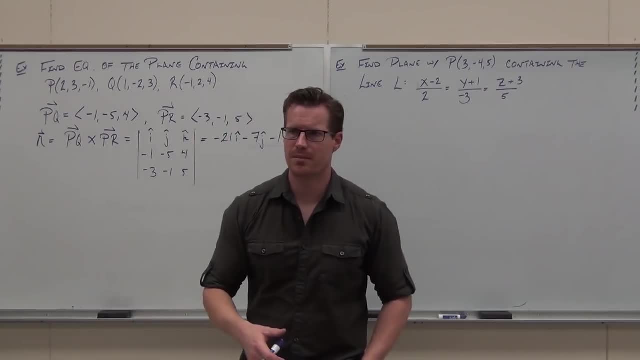 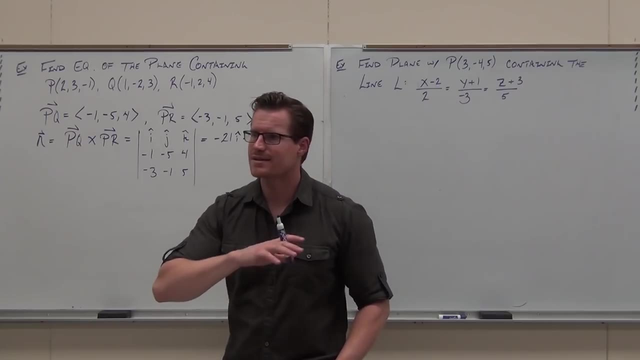 Yes, I mentioned something earlier. You notice it's going to be a lot of recap, but I mentioned something earlier. You can manipulate your vectors as long as they don't deal with a distance. This doesn't deal with a distance, it's just a direction. 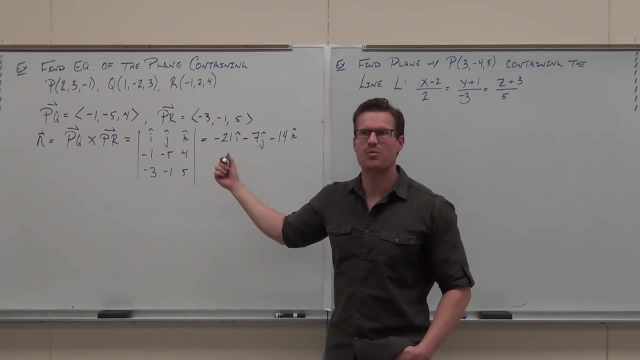 That's nasty folks, that's nasty. Can you make a point? Make it look better, more better. make it look more better. How are you going to make it look more better? I'd factor the negative, for sure, and the 7.. 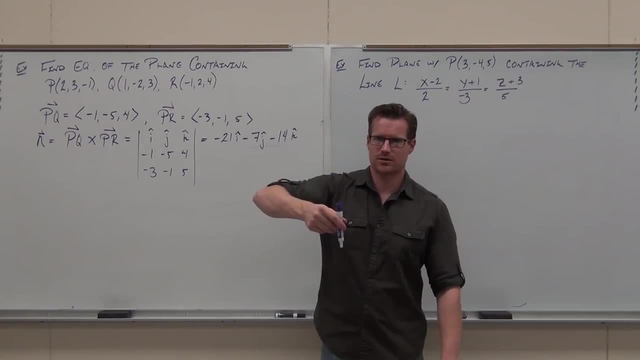 So if I do that, what's it doing? Well, it's taking this vector and it's moving it here and it's shortening it. Who cares? It's still a normal vector, It's still orthogonal to that plane. 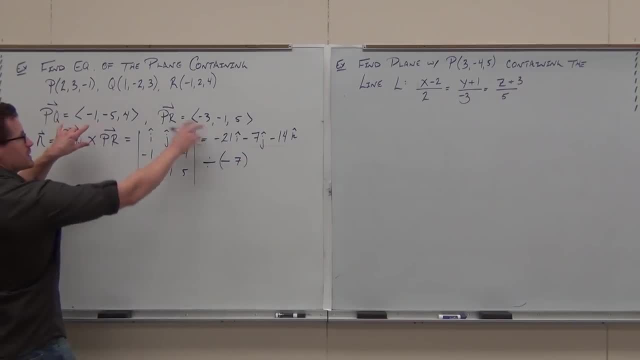 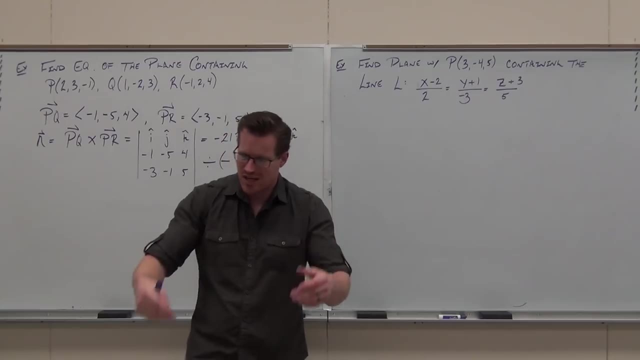 Is that logic making sense to you? If you reversed these and did the cross product backwards, it'd be plus, plus, plus. You'd still have to factor out the 7, but you see, it doesn't matter. You can always change the scale and multiple of that. 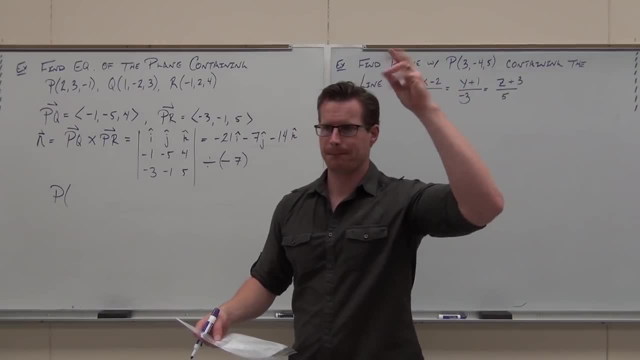 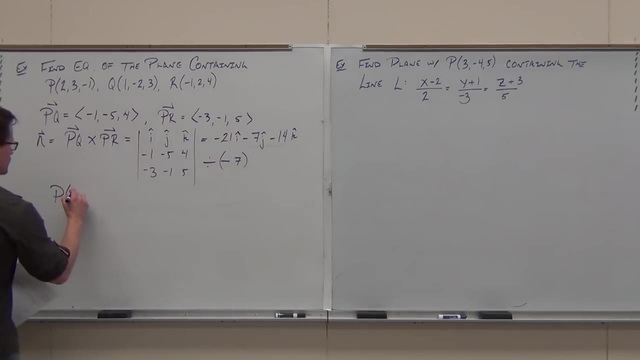 So again, two things we need for a plane order. two things quickly. What are they? Point Point and Normal vector. Do we have a point? Yes, Write down any one you want. I'm going to write down the P. Have we managed to find a normal vector? 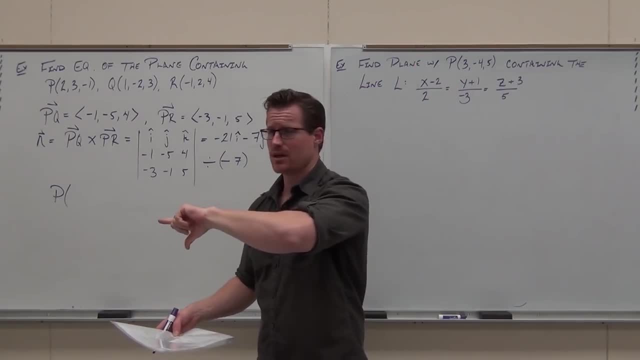 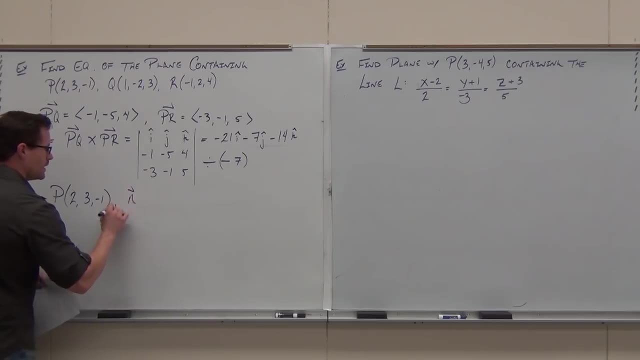 Point Point and Normal vector. Do we have a point? Yes, Write down any one you want. I'm going to write down the P. Have we managed to find a normal vector? Yes, Which one are you going to use? 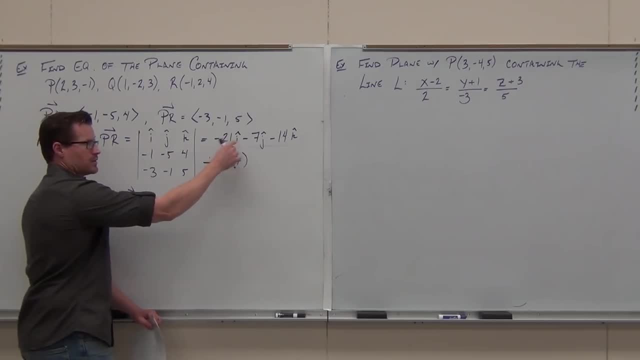 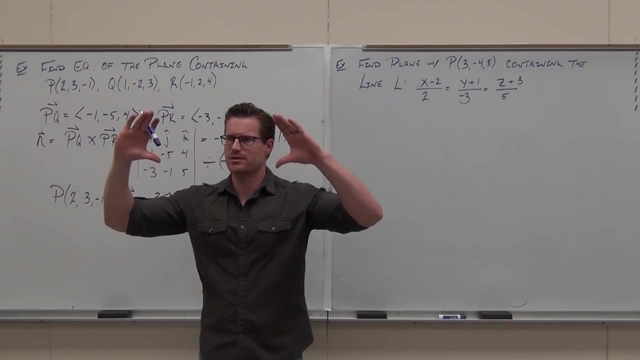 Simplify, Not this one. No, no, no, no. Simplify, You're going to get 3i. 3i plus j plus 2k- Beautiful. Could you change that to the the vector brackets. 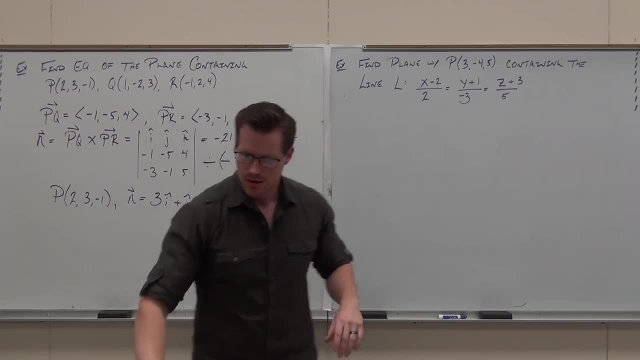 and it'd be just fine. I don't care how you do it, We're going to use both in this class. So from here, we've got a point, We've got a vector. What I want you to do if you haven't done it already. 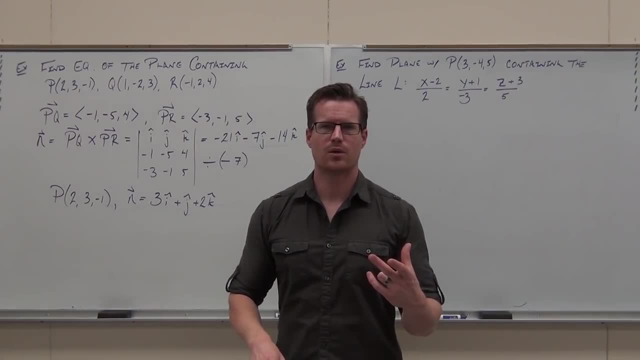 I want you to fill out the formula for a line or a plane. But stop for just a second. I know you've worked. look up here for a minute. Do you see that both formulas have exactly the same junk in them? a point and a vector. 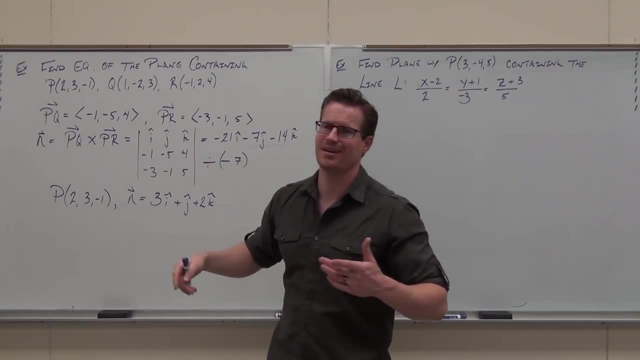 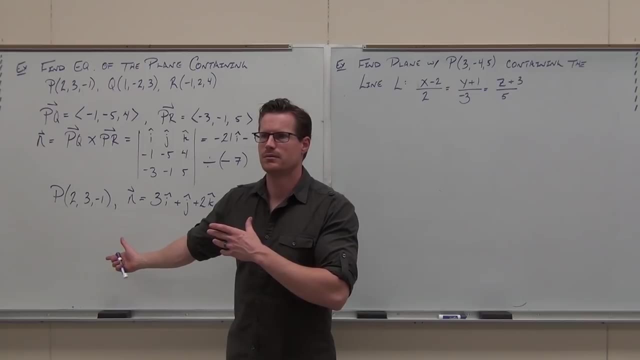 So if you're not really mining your, your P's and Q's- you can- you can put it in the wrong formula really easily. You can go: oh yeah, I'm finding a line, You're not finding a line, You're not finding a line. 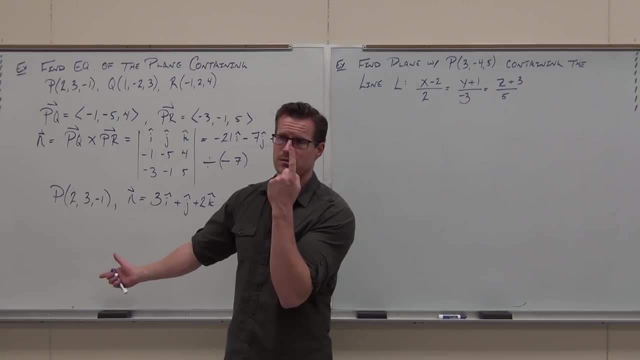 If you did, you'd be finding the line- The line that is perpendicular to a plane- through that point. That's interesting, but it's not what I'm looking for. I want you to define the plane in this case, So use the appropriate formula, even though you have the same. 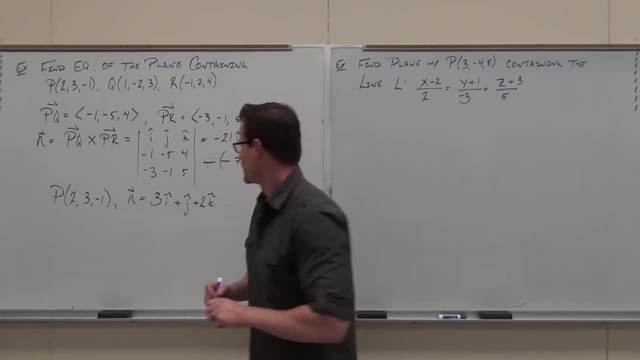 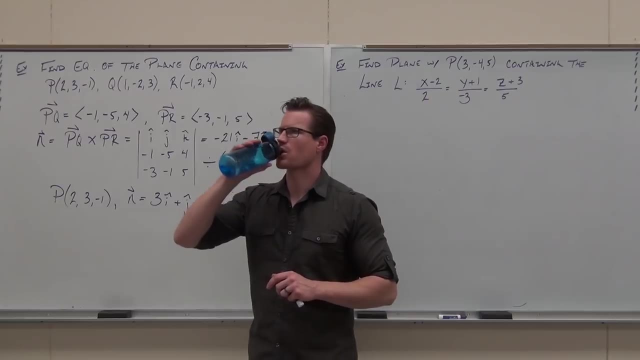 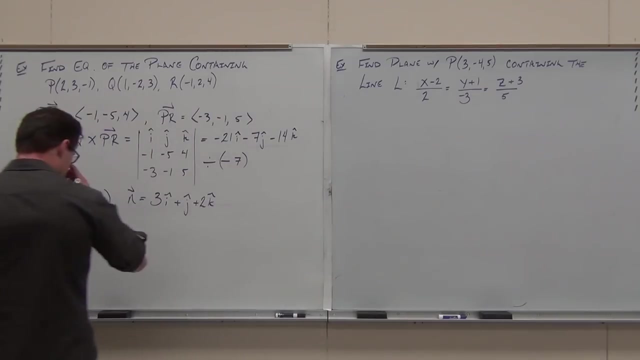 looking stuff. it looks a lot alike. Be careful, okay. So for us, go ahead and figure that one out, and I'm going to give you the answer in just a little bit. I want you to double: go ahead For this negative 7, is that negative or is it positive? 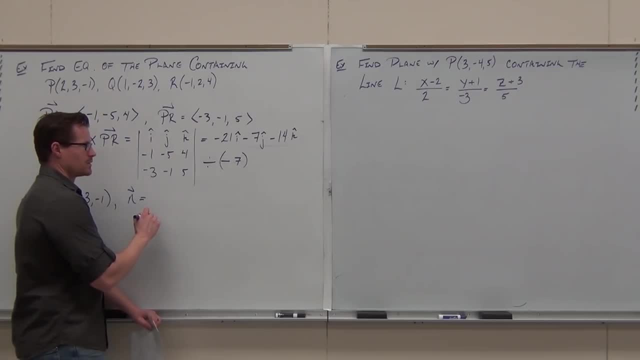 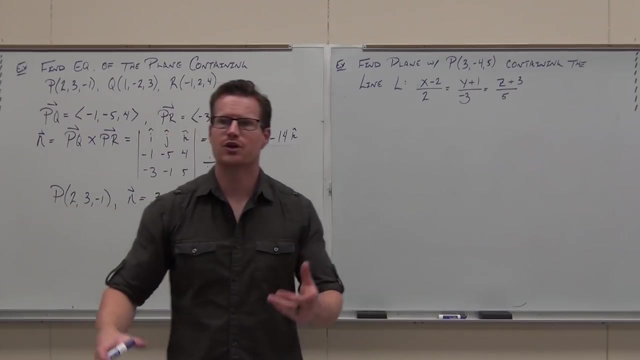 Yes, Which one are you going to use? Some, Not this one. Simplify it: You're going to get 3i, 3i plus j plus 3k. Beautiful. Could you change that to the vector brackets and be just fine? 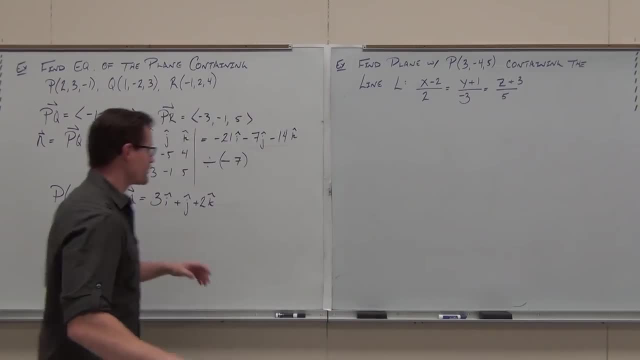 I don't care how you do it, We're going to use both in this class. So from here, we've got a point, We've got a vector. What I want you to do, if you haven't done it already, I want you to fill. 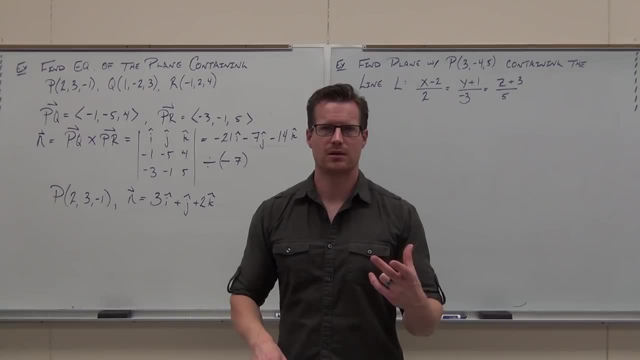 out the formula for a line or a plane Line, But stop there, Line. Stop for just a second. I know you're working. Look up here for a minute. Do you see that both formulas have exactly the same junk in them? a point and a vector. 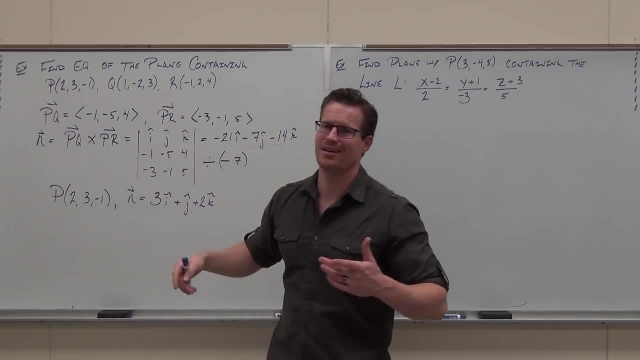 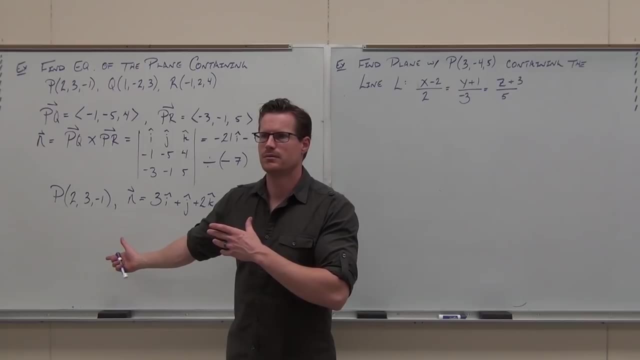 So if you're not really minding your P's and Q's, you can put it in the wrong formula really easily. You can go: oh yeah, I'm finding a line, You're not finding a line, You're not finding a line. 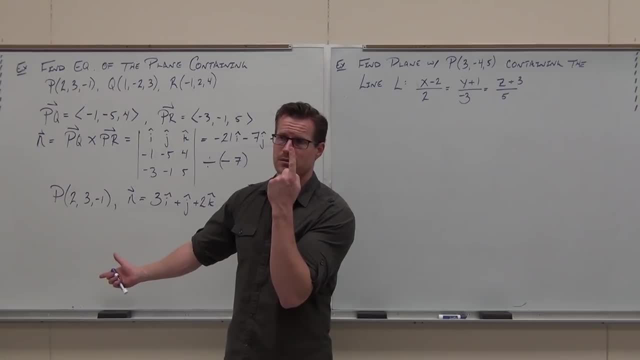 If you did, you'd be finding a line that is perpendicular to a plane through that point. That's interesting, but it's not what I'm looking for. I want you to define a plane in this class In this case, So use the appropriate formula. even though you have the same looking stuff, it looks a lot alike. 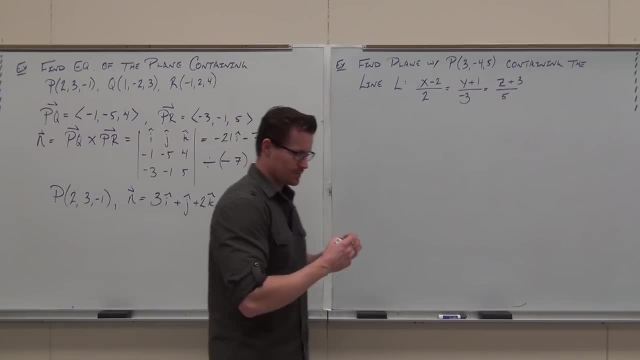 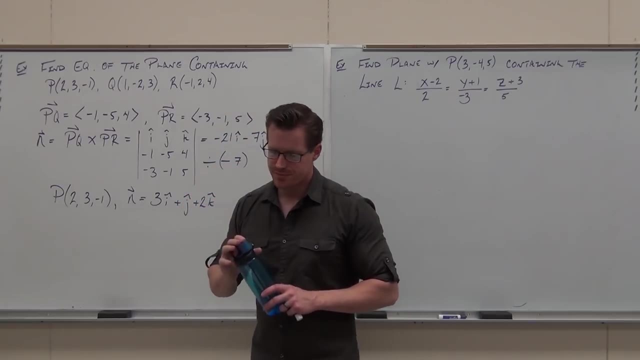 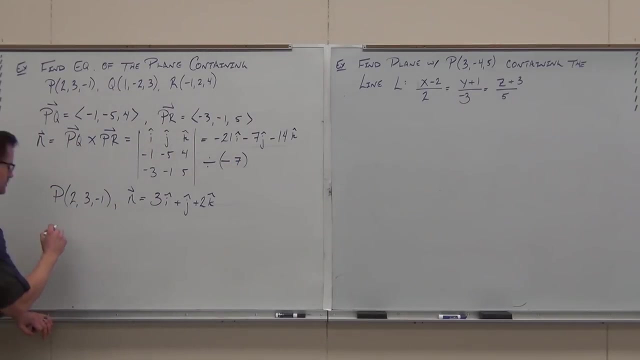 Be careful, okay. So for us go ahead and figure that one out, and I'm going to give you the answer in just a little bit. I want you to double go ahead For this negative 7, is that negative or is it positive? 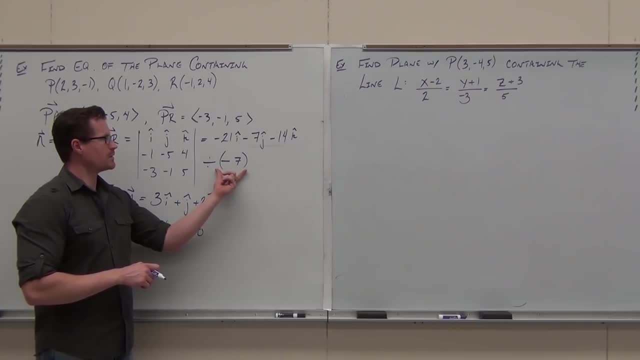 If I divide by negative 7?? Oh no, on the top, is that supposed to be negative or is it positive For this? Yeah, I don't know, Let's find out. Negative 5 plus 12 is 7, but remember there's a minus. 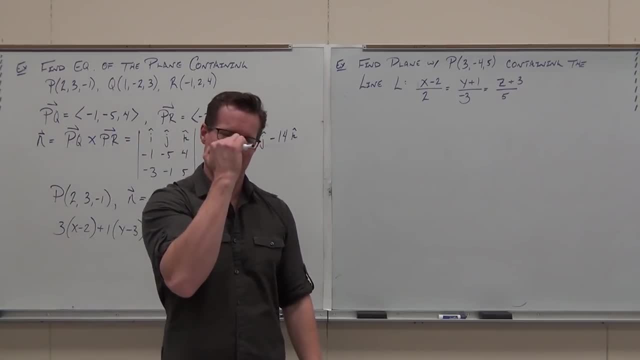 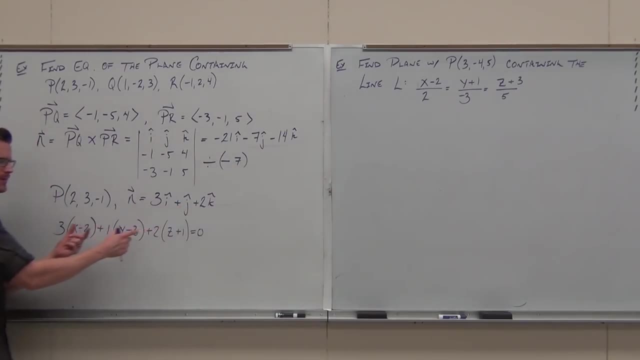 That happens A lot, Remember I did the minus like 14 underlines. Yeah, happens all the time. So we have this. we have our normal vector components here, here and here. We got our coordinates for our point here, here and here. 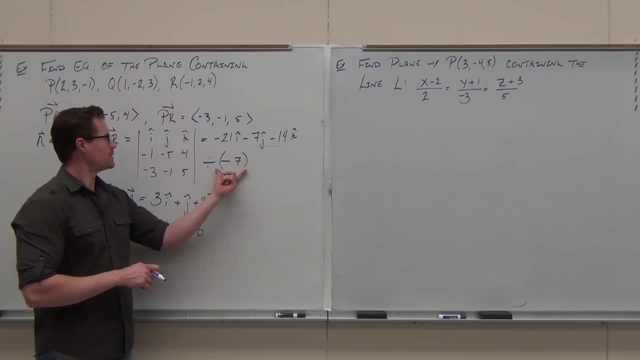 If I divide by negative 7?? Oh no, on the top of, is that supposed to be negative or is it positive For this? Yeah, I don't know, it's hard to negative 5, plus 12 is 7, but remember there's a minus. 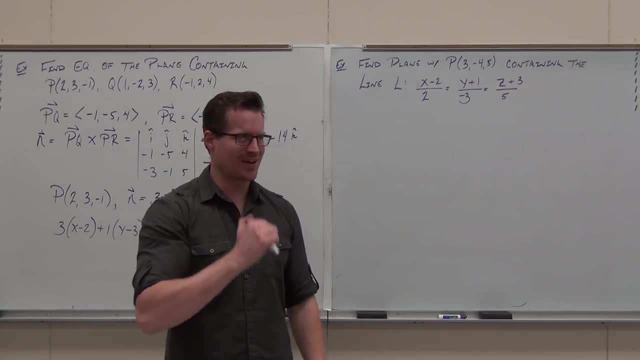 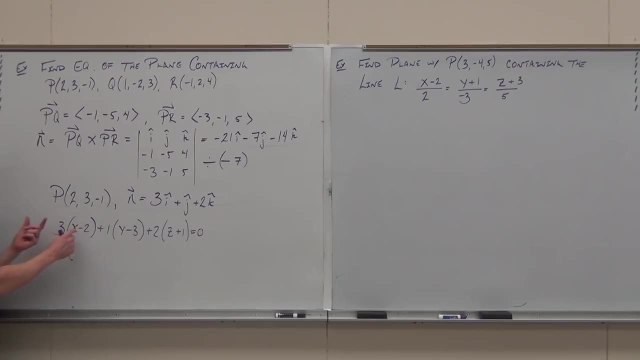 That happens a lot, Remember I did the minus like 14 underlines. Yeah, happens all the time. So we have this, we have our normal vector components here, here and here. We got our coordinates for our point here, here and here. 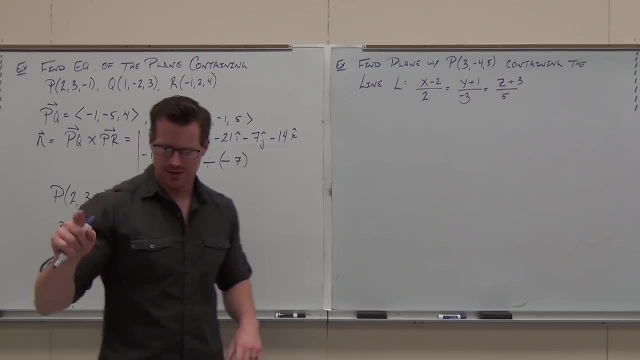 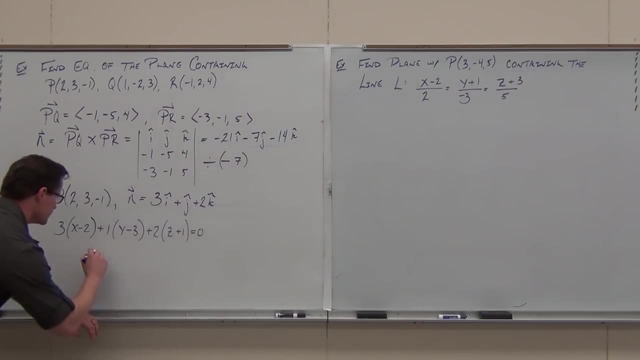 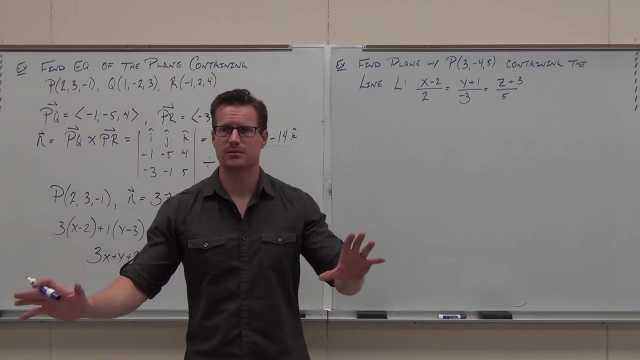 Make sure your signs are okay Distribute. Did you guys do this and get a final answer for me? I got 3x plus y plus 2z equals 7.. Beautiful Ten points on the test, right there. It's very basic, very basic. 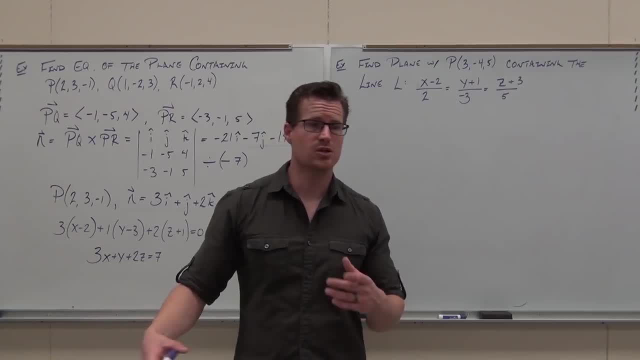 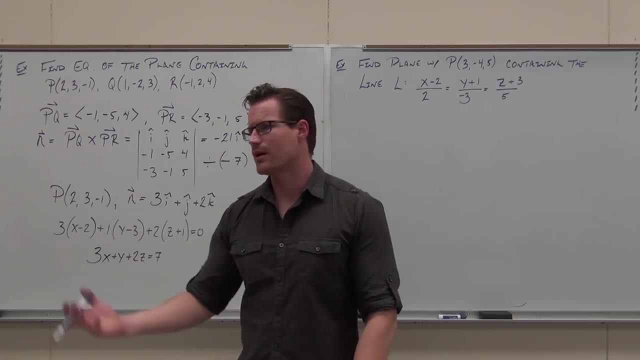 But I'd give you something like this: because it uses the cross product, It uses your understanding of how to do stuff like that. Does that make sense to you? That's how I test you on these things is with composite problems. We don't have enough time for me to test you. 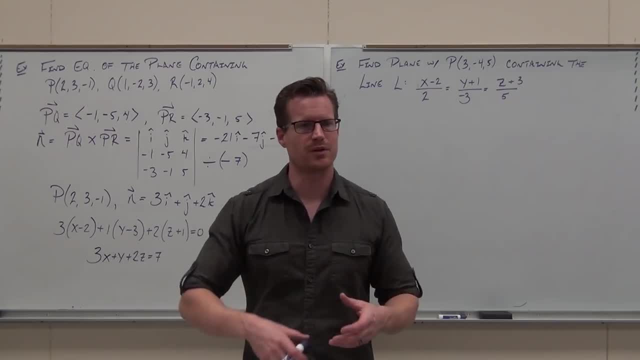 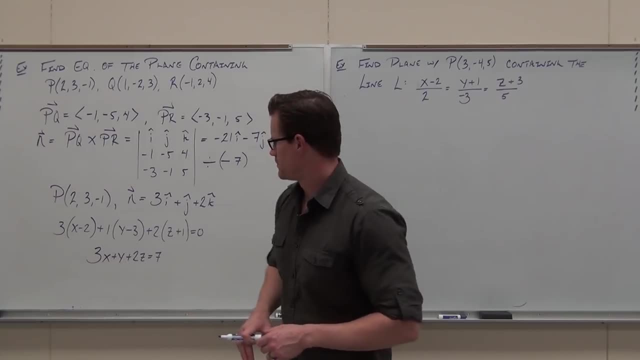 on every little thing. So I make big problems that way. you have to work through me to understand the concept, Do you? How do you check your work? Let's see if it comes up with the right. So I think that's how you check your work. 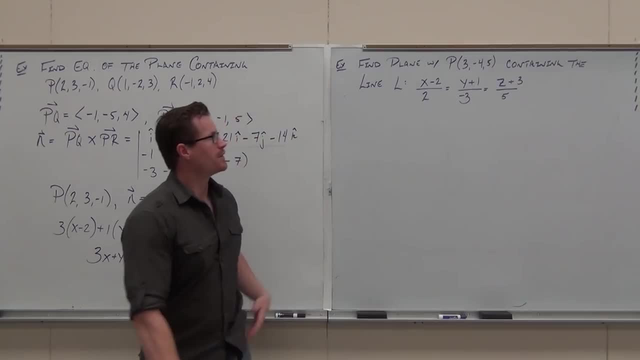 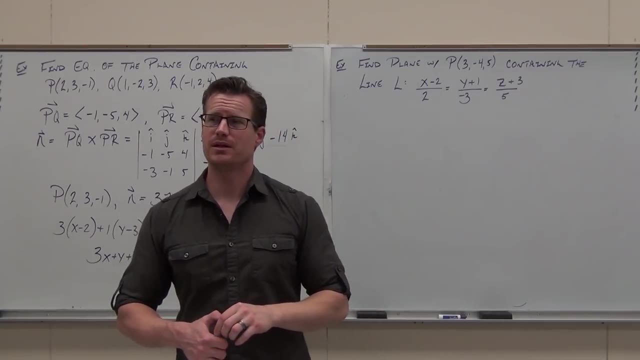 Let's do the next one. I want to find the equation of a plane that has that point in it and contains this line. Now we need a few things, right, We need a few things for a plane. We need a point and we need a normal vector. 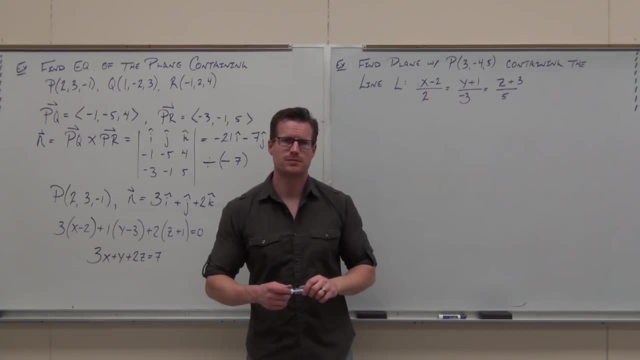 True or false. This has a normal vector in it. No, No, If the plane contains this line. so if this is my plane and I draw my line, tell me what that line is giving me. What do lines have? They have a vector in them. 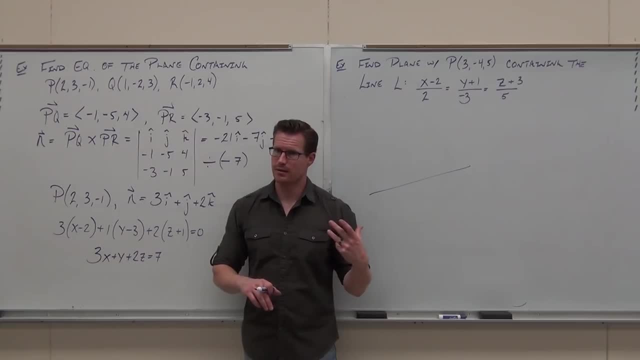 What else do they have? They got a point in there. We got a point on that. So this line gives me really two things. It gives me a vector in the plane. It also gives me another point in that plane. Does that make sense to you? 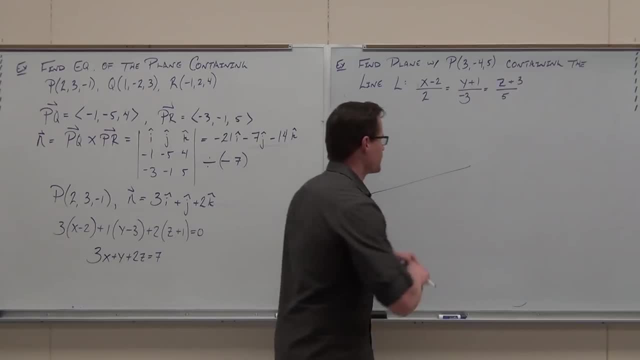 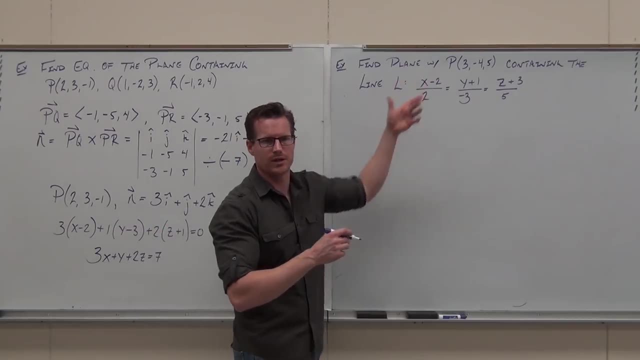 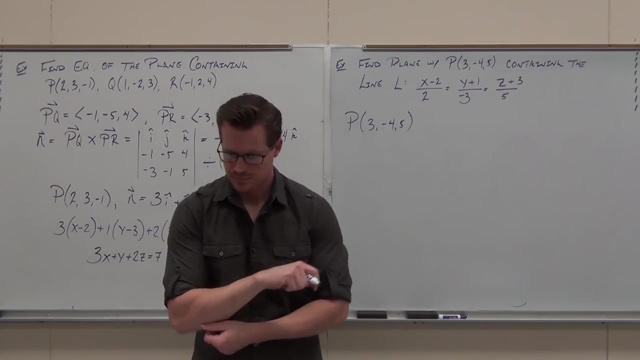 This is a weird problem, So I want to identify everything we get. What do we got going on? What junk do we know about in the plane? Well, I know that there's a point in that plane. I know there's a point in that plane. 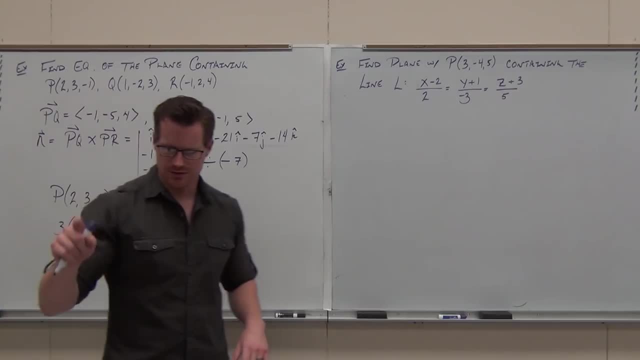 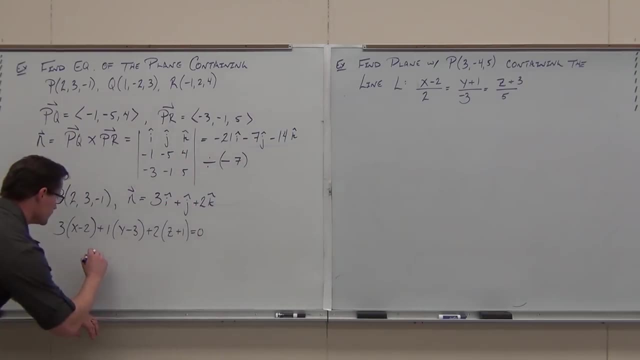 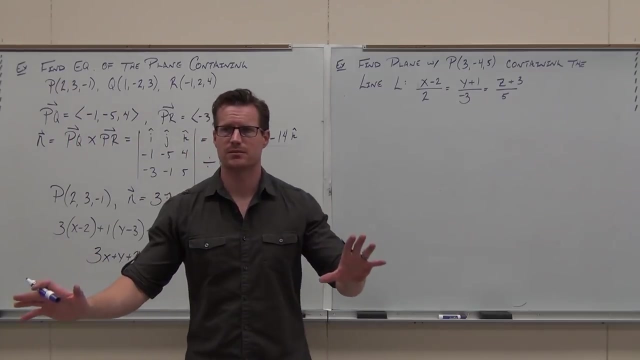 Make sure your signs are okay Distribute. Did you guys do this and get a final answer for me? I got 3x plus y plus 2z. equals Beautiful 10 points in the test right there. Very basic, very basic, but I'd give you something like this: 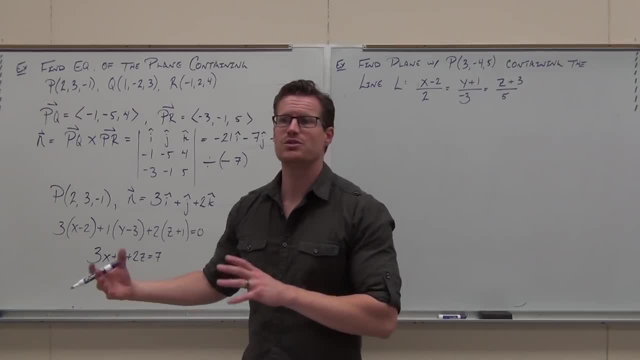 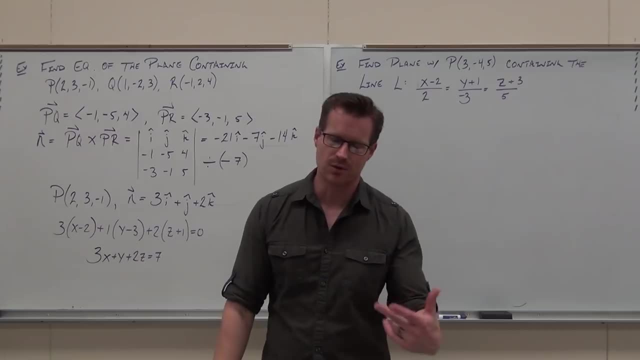 because it uses the cross product. It uses your understanding of how to do stuff like that. Does that make sense to you? That's how I test you on these things is with composite problems. We don't have enough time for me to test you on every little thing. 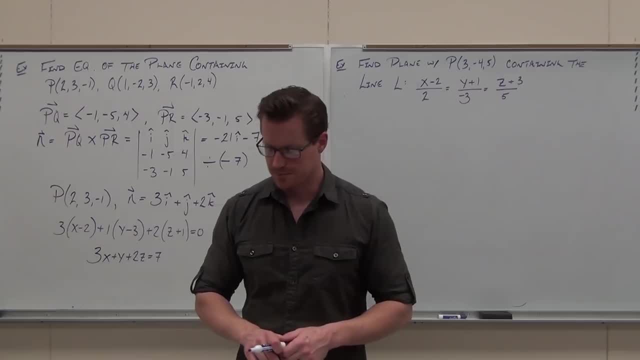 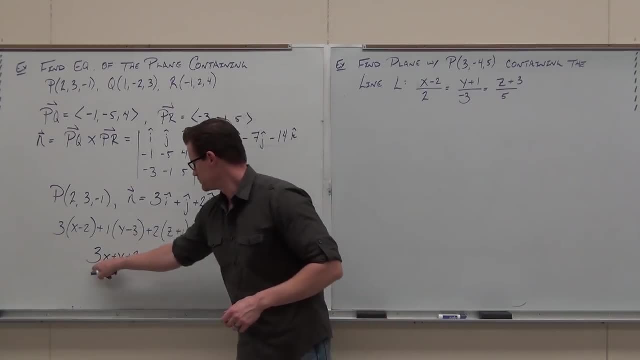 so I make big problems that way. you have to work through me to understand the concept, Do you? How do you check your work? See if it comes up with the right? Yeah, I think you're right, So I think that's how you do it. 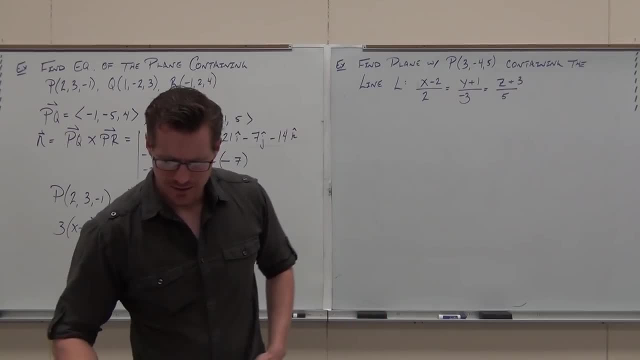 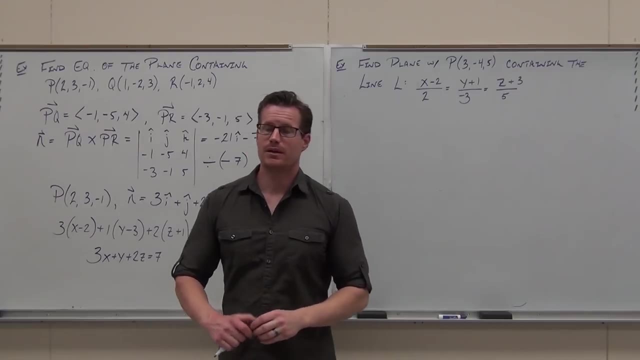 Yeah, I think you're right. Let's do the next one. I want to find the equation of a plane that has that point in it and contains this line. Now we need a few things. right, We need a few things for a plane. 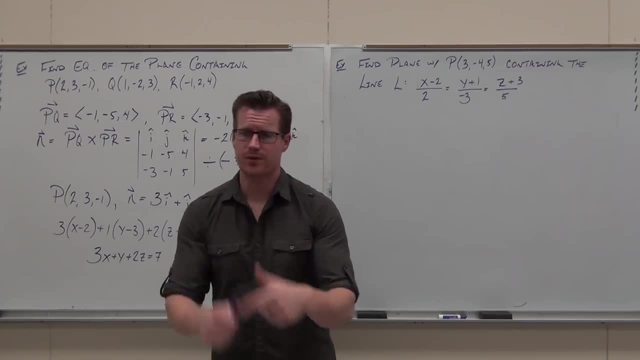 We need a point and we need a normal vector. True or false, This has a normal vector in it. No, No, If the plane contains a line. so if this is my plane, I draw my line. tell me what that line is giving me. 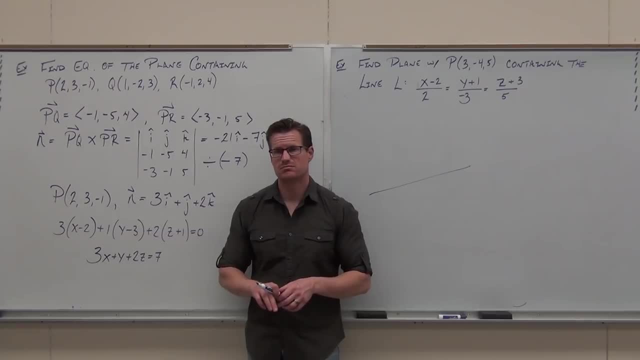 A vector. What do lines have A vector? They have a vector in them. What else do they have A point? They've got a point in there. We've got a point on that. So this line gives me really two things. 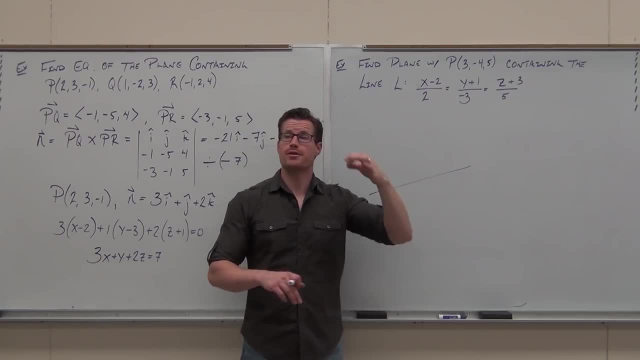 It gives me a vector in the plane. It also gives me another point in that plane. Does that make sense to you? This is a weird problem, So I want to identify everything we've got going on. What junk do we know about in the plane? 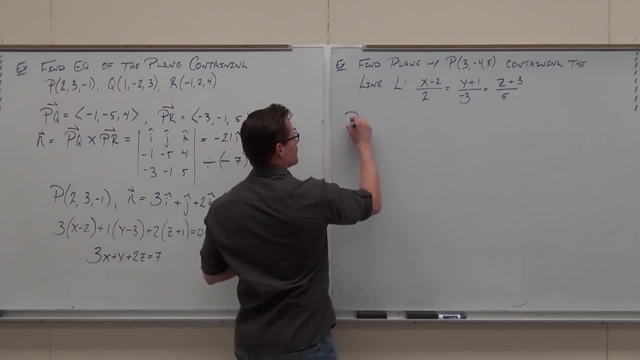 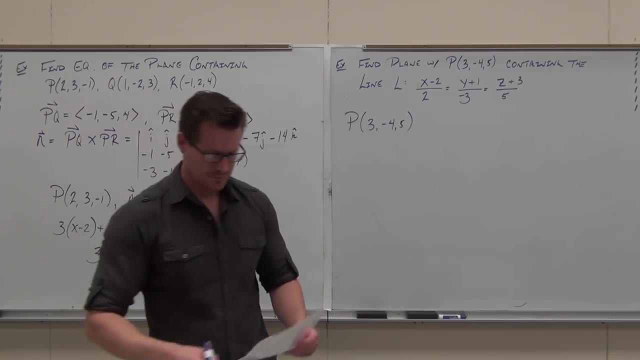 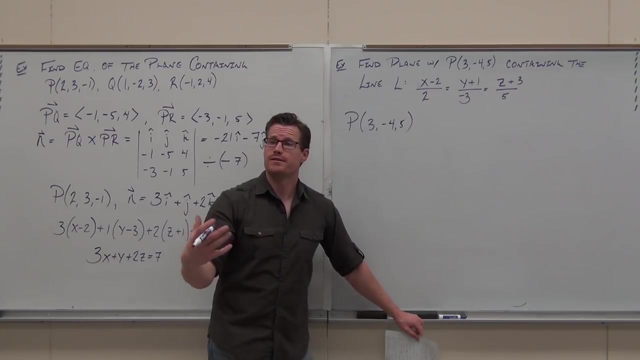 Well, I know that there's a lot of junk in the plane. I know that there's a point in that plane. I know there's a point in that plane. The line also gives me. so if the plane contains a line, that line also gives me a point in. 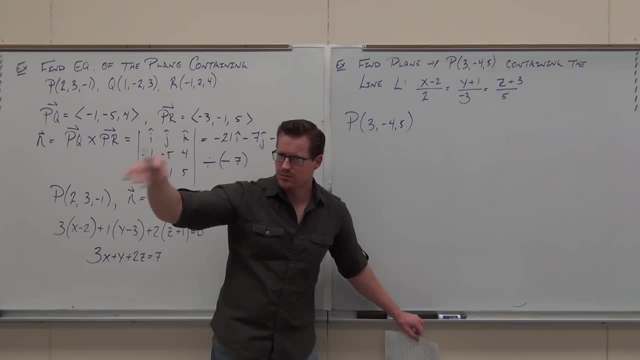 that plane? Not sure. if you follow that logic, The line's in the plane and the point's on the line, The point's on the plane, The point's on the plane. Tell me a point on that line, We'll call it Q. 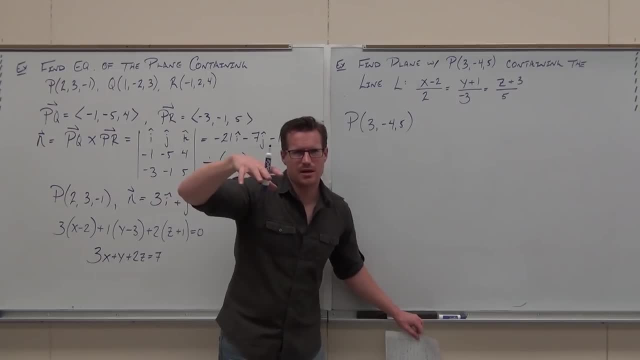 The line also gives me. so if the plane contains a line, that line also gives me a point in that plane. not just if you follow that logic: The line's in the plane and the point's on the line, The point's on the plane. 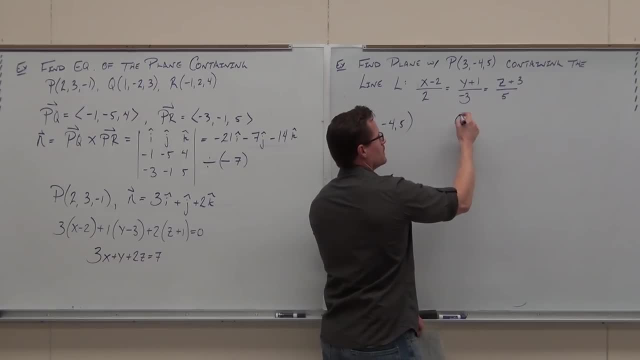 Tell me a point on that line. We'll call it Q Two: Negative one Two. I like the two. Do you see where the two's coming from? Yeah, Negative one. Where's the negative one? Yes, Negative two. 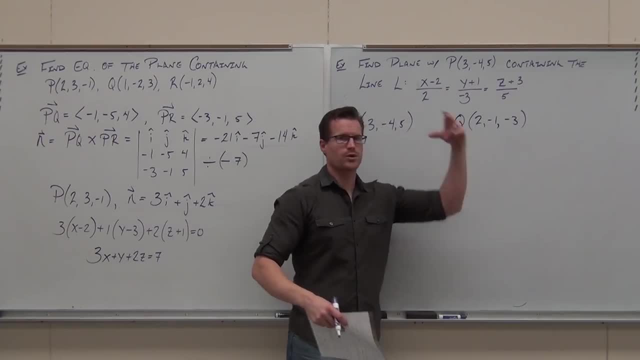 Negative three. That's a point on the line. Therefore it's also in the plane because it's got to be. that line's got to be in the plane. So if you guys feel, okay with it. that's a weird concept. 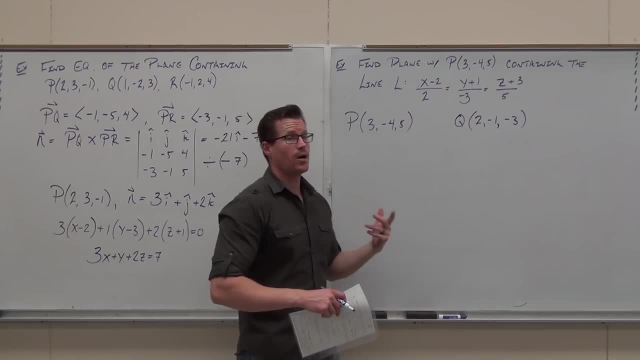 I want to make sure you guys understand, I want to make sure you guys get it. You guys okay with that one. Now, how about this? What else does the line have? Vectors, Vector. So if that line is in the plane, 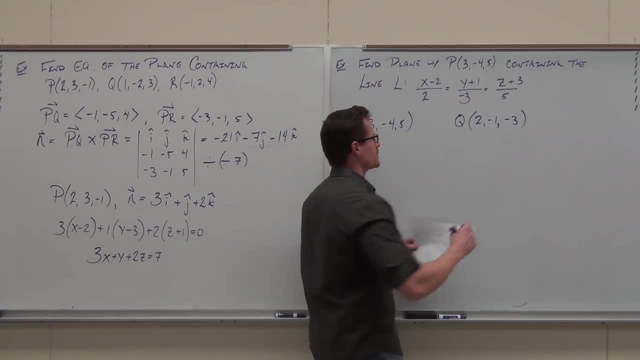 that vector can be thought of as contained in the plane. Let's write the vector. I'm going to call it B. So this is from our line. Our line's got a point. Hey, two negative one. negative three. Our line's got a vector. 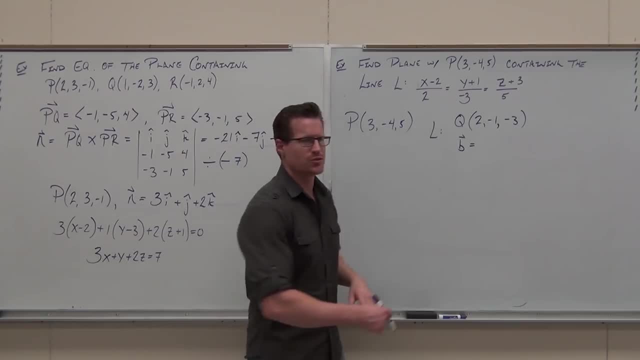 Oh man, You should have known that You should be really good at finding direction vectors at this point. Come on like five seconds. What's the direction vector for that line? Two negative three, five. Use the correct notation. 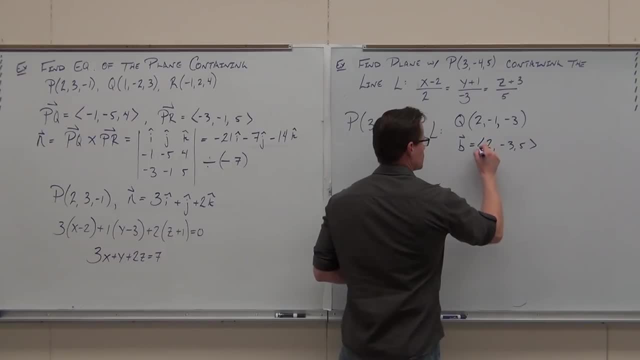 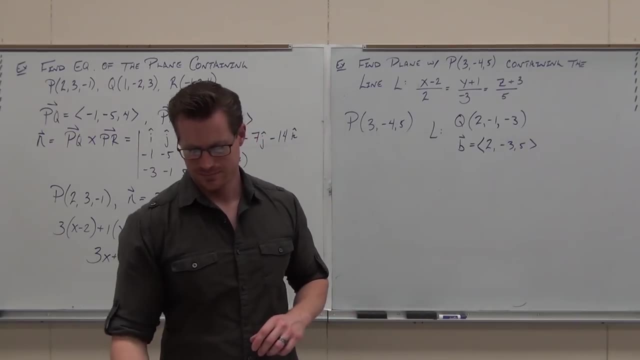 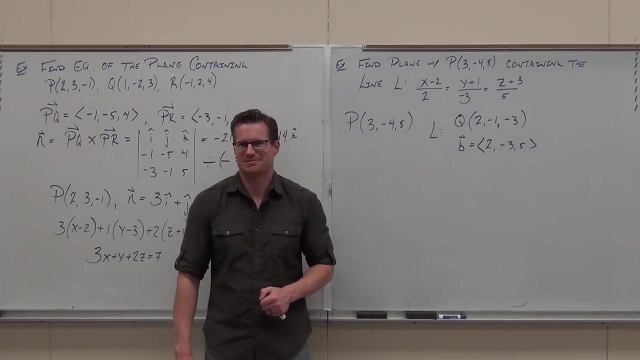 Got to have it correct For P was that given Yup? My daddy always said yup, give it. He wasn't texting. I think it was from California. We talk like that It's because It's cool, Not really. 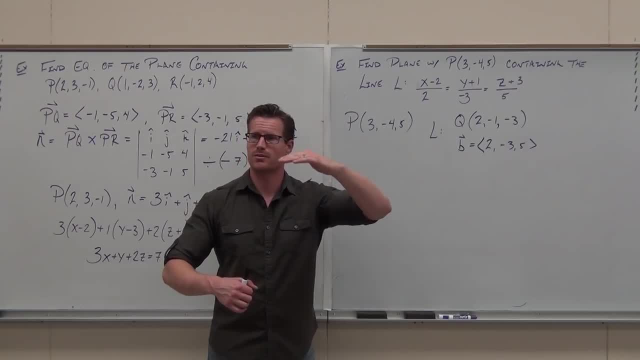 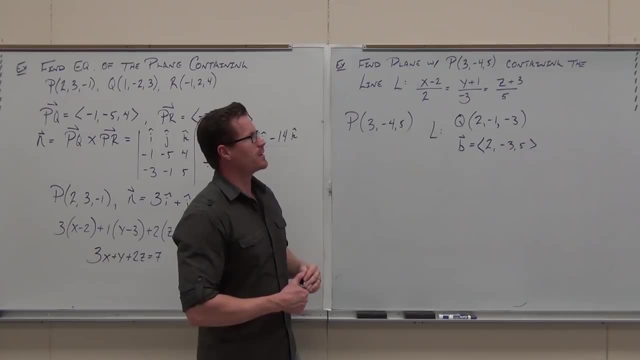 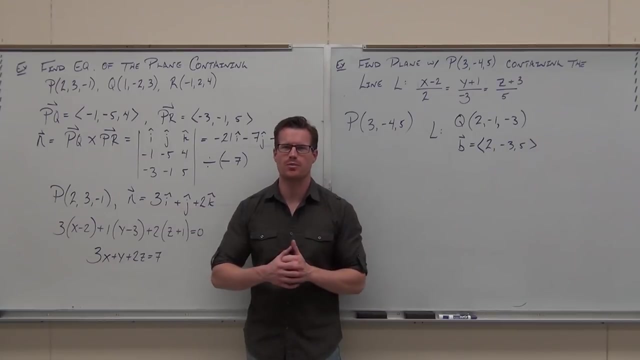 He's a math teacher too. It's a line of dorks like all the way, Like grandfather was a teacher. Yeah, seriously, I don't know A lot. Anyway, the logic is this: Look, you're going to have to find what type of a vector to describe a plane. 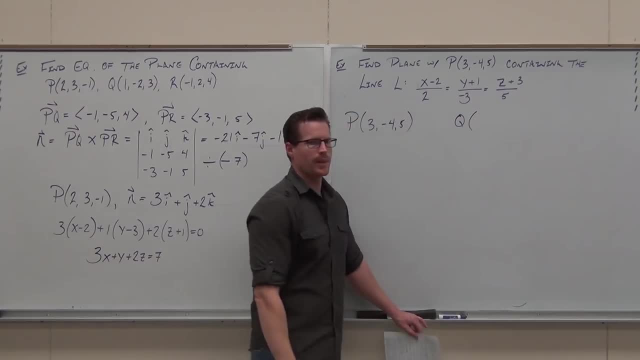 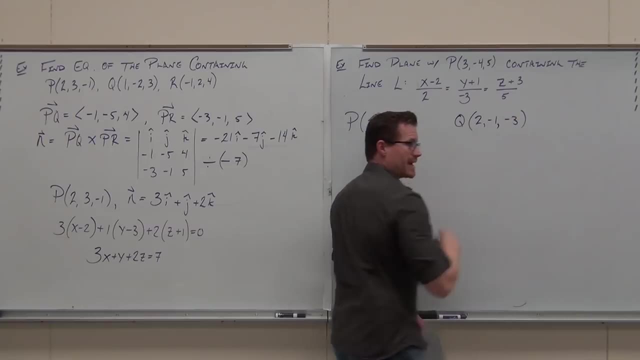 Two. Negative one. Two. I like the two. Do you see where the two's coming from? Yeah, Negative one. Where's it? Negative one. Negative two. Negative three. That's a point on the line. Therefore, it's also in the plane, because it's got to be. that line's got to be in. 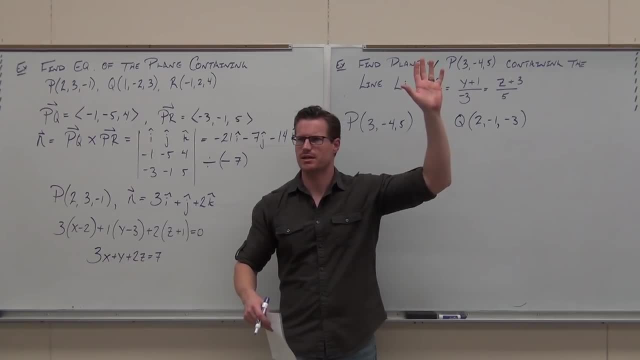 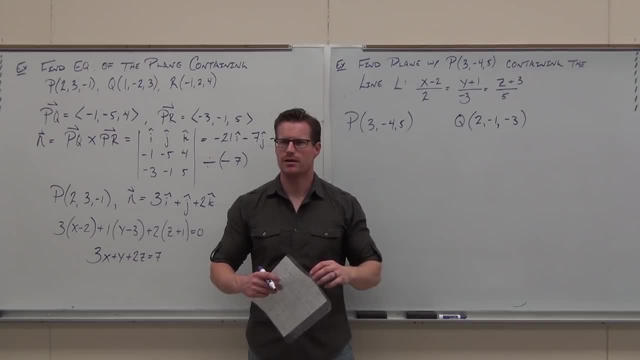 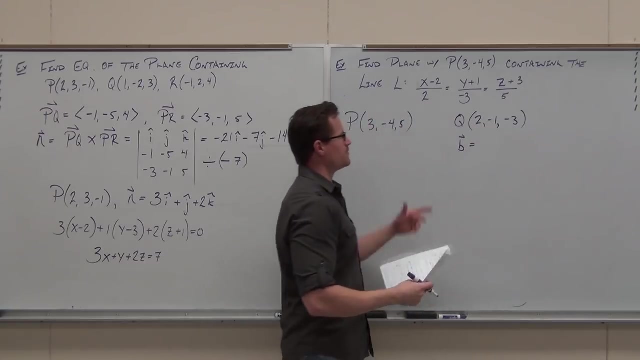 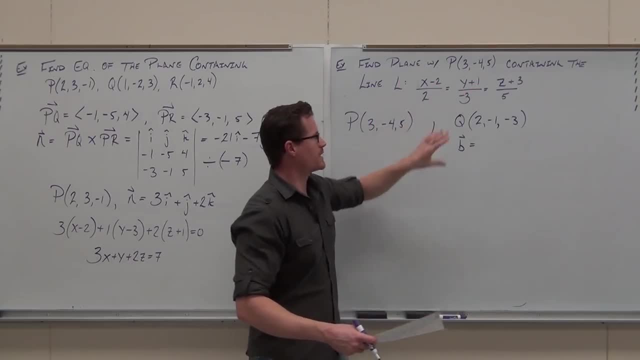 Our line's got a point. Hey, two negative, one negative three. Our line's got a vector. Oh man, you should be really good at finding direction vectors. at this point, Come on like five seconds, What's the direction vector for that line? 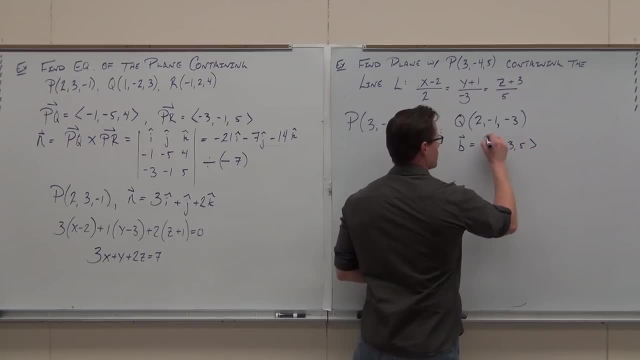 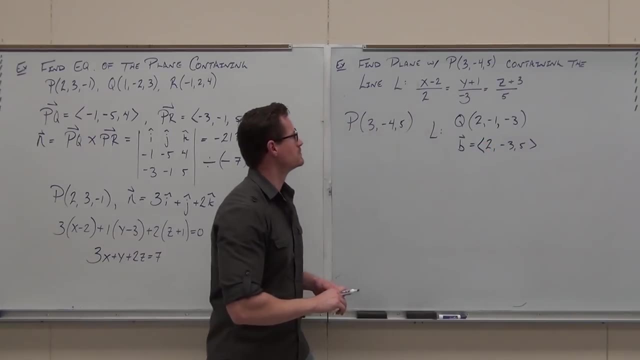 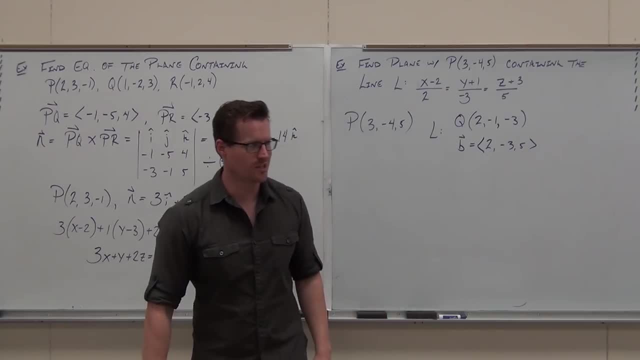 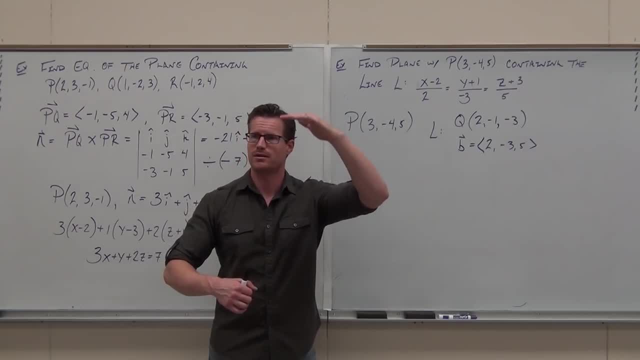 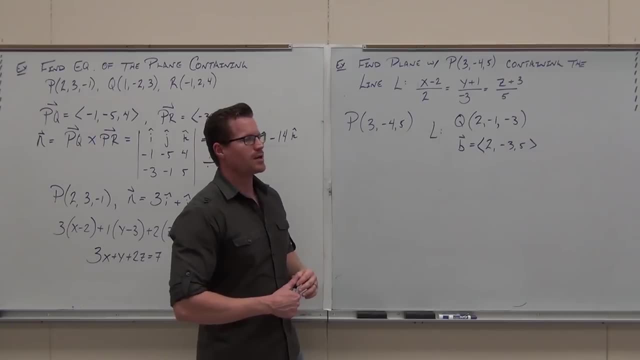 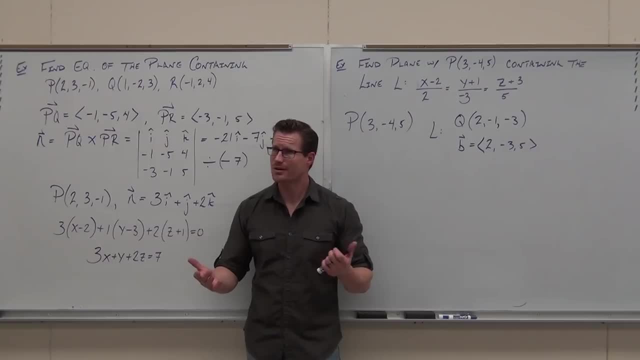 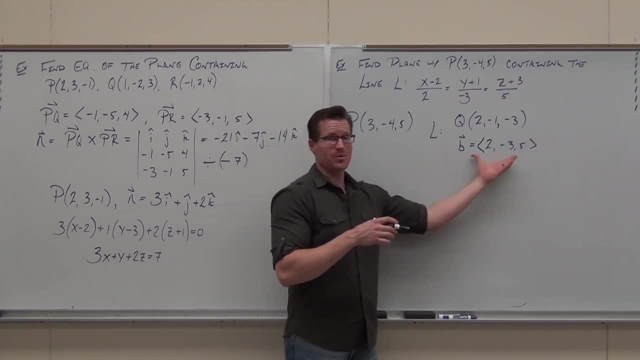 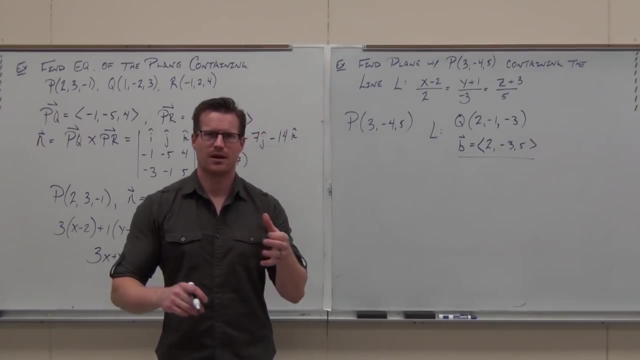 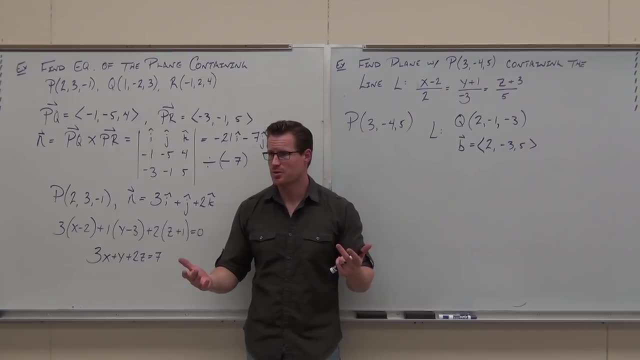 Normal, Normal. If it's not given to you, you're going to be doing a cross product probably, or finding something else from another plane, But right now we go. okay, I don't have anything that's telling me. a normal vector. 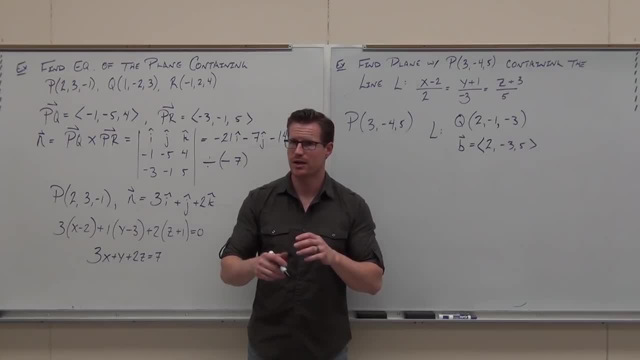 so I'm going to have to have a cross product. Well, in order to find a cross product, how many vectors do you need for a cross product? Two, Do I have one? Yeah, That's in the plane. You guys get what I'm talking about. 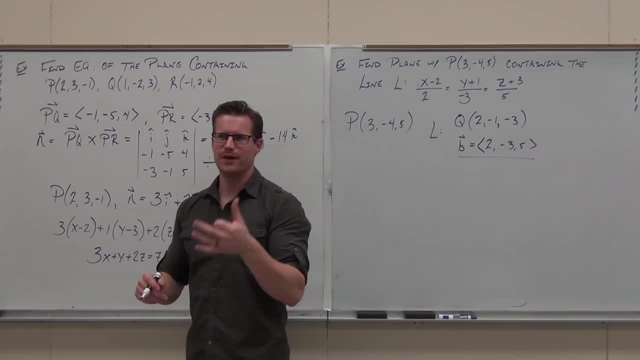 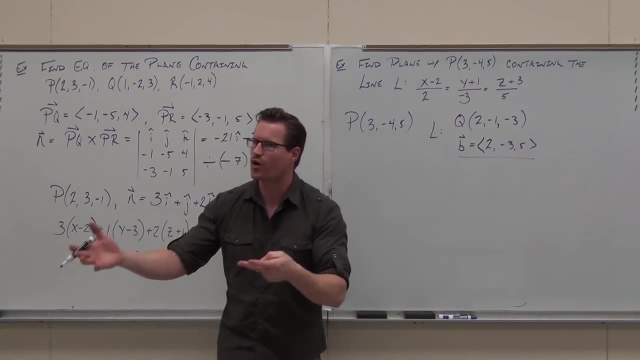 That's in the plane. This is one vector. Can you find another vector in the plane? Yes, Yes, How You can? Yes, because those are both in the plane. See, it's not hard. but do you see how you have to think about these things a little strange. 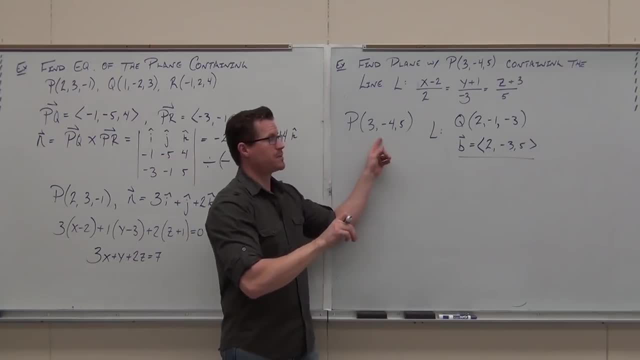 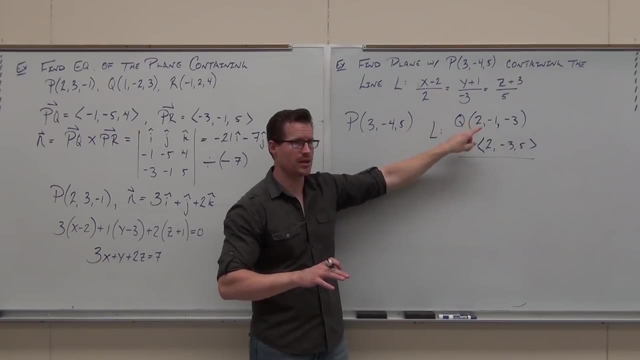 Let me walk you through it, if you didn't catch it the first time. Okay, Check it out. Point P got to be in the plane, Make sense? This line is in the plane, which means that that point is in the plane. 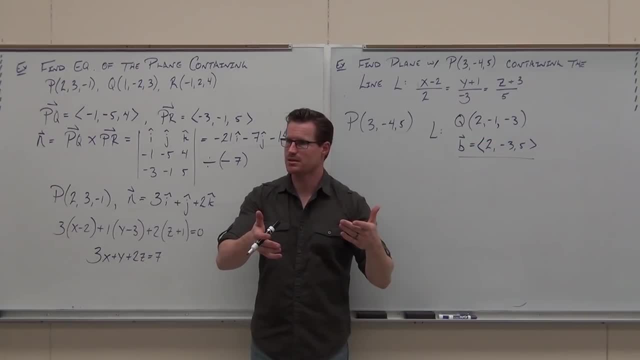 and that vector can be thought of as being in that plane. Does that make sense? So if I have one vector here and I say: well, let's define vector A as P to Q, then I get another vector- Negative 1,, 3, negative 8?. 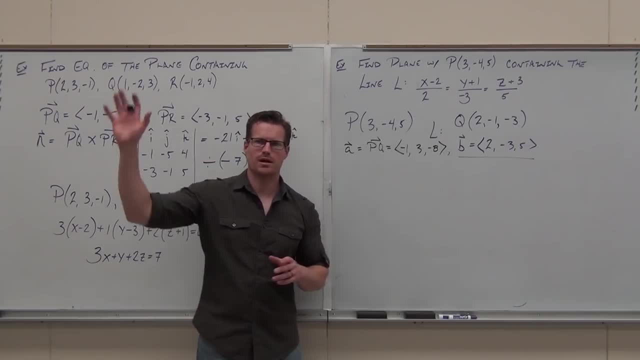 Yes, Cool. So it makes me look good with the thought process so far. So we've had a couple points. Find a vector: We were given a vector in the plane, No problem. Now I have two vectors that are in the plane. 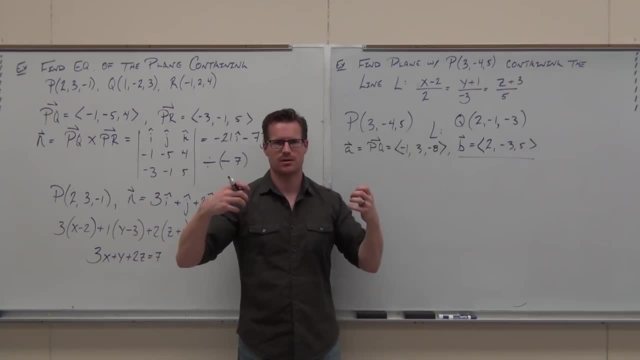 Are you still with me? What is your next step? Find it. I actually have a question about choosing which one should be in front to subtract, because is it the line that? is it the vector? I mean, in this case, is it the line that goes to point B, connected to point Q? 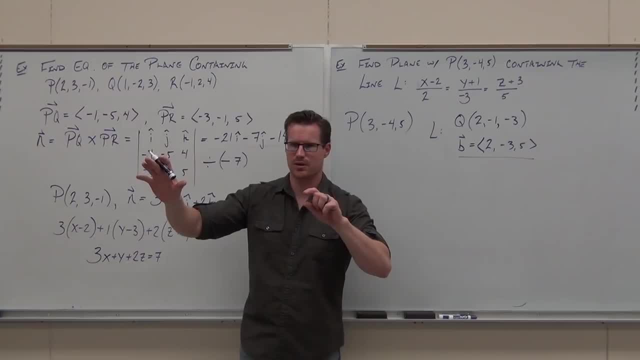 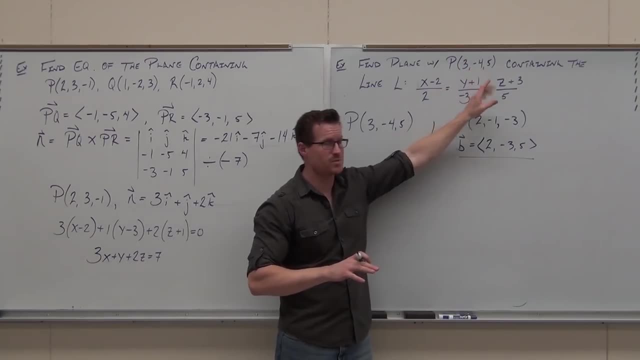 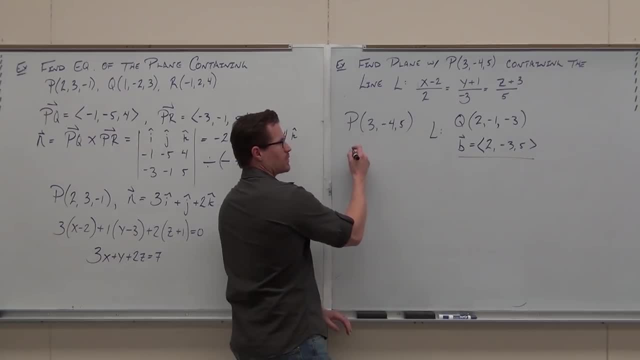 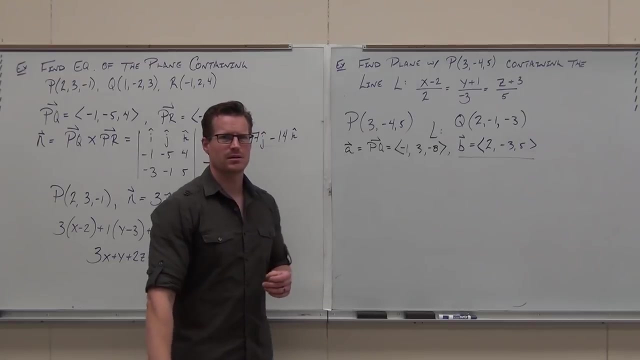 Does that make sense? So if I have one vector here and I say, well, let's define vector A as P to Q, then I get another vector- Negative 1, 3, negative 8? Yes, Cool. So it makes me look good with the thought process so far. 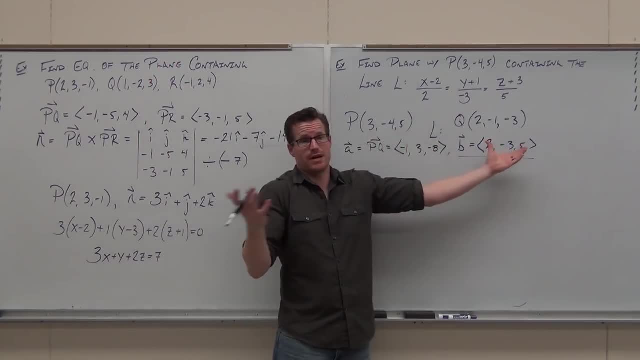 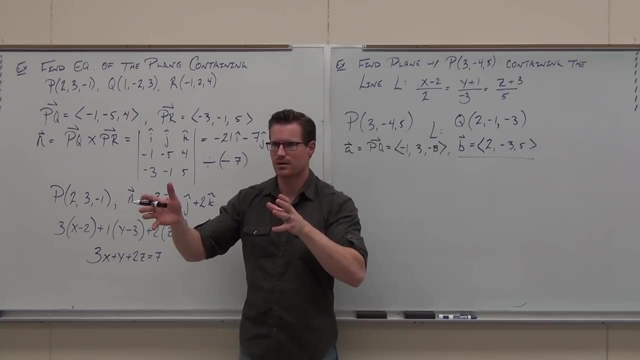 So we've had a couple points. Find a vector. We were given a vector in the plane, No problem. Now I have two vectors that are in the plane. Are you still with me? What is your next step? Cross-pattern- Find it. 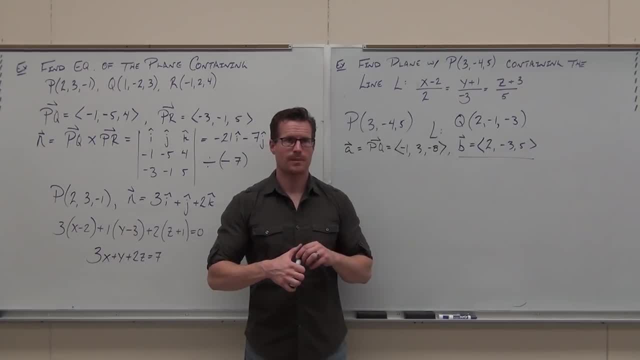 I actually have a question about choosing which one should be in the front to subtract, because isn't the vector being connected to point Q? No, it goes through there, but connected. it's weird, right, Because these vectors are position vectors. They're not connected at all. 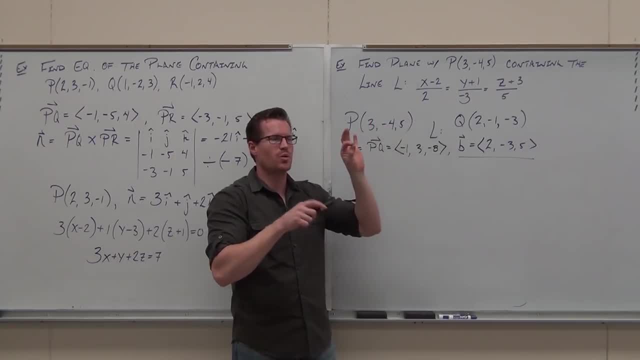 It's a scalar multiple to get up to there. So we think of it more like here's the point and here's the direction you're headed through that point. So it doesn't really matter. It doesn't really matter which one you subtract from which. 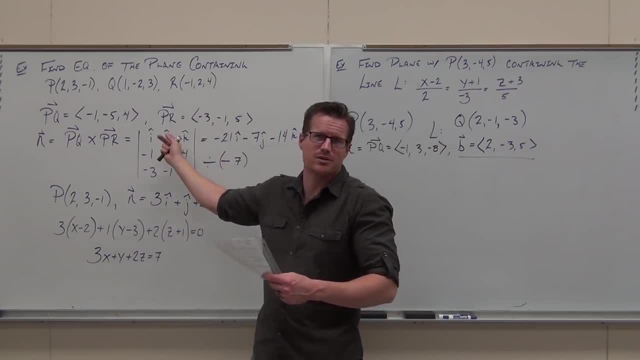 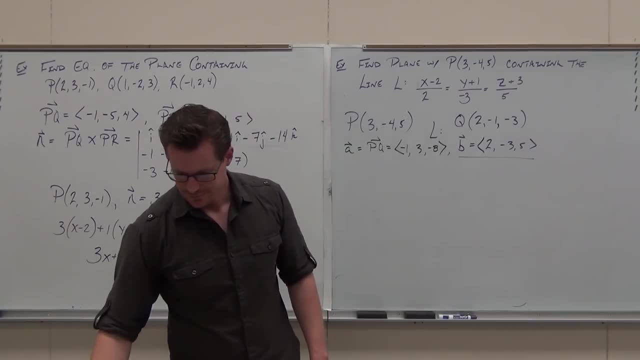 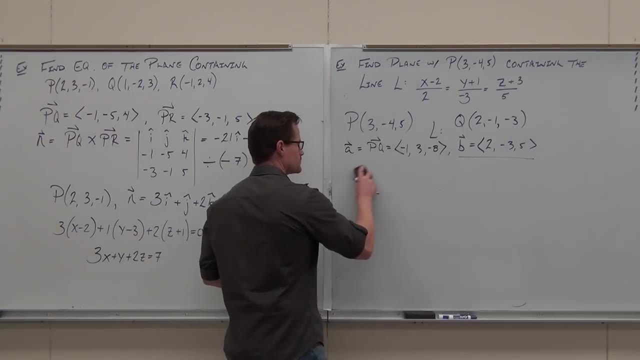 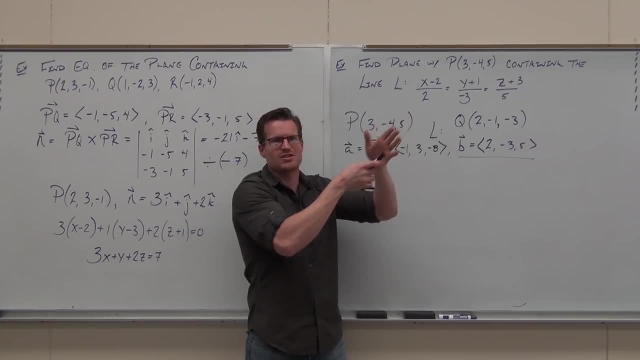 No, It goes through there, But connect. it's weird, right, because these vectors are position vectors. They're not connected at all. It's a scalar multiple to get up to there. So we think of it more like: here's the point. 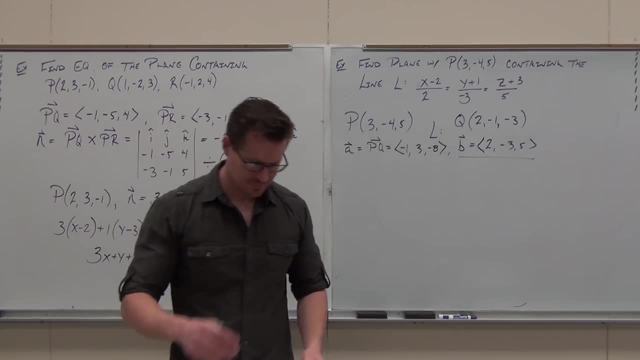 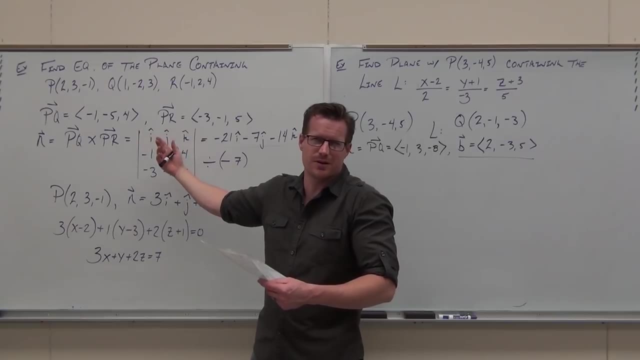 and here's the direction you're headed through that point. So it doesn't really matter. It doesn't really matter which one you subtract from which. We kind of we found that out over here too right, Because even if you cross, product these a little funky. 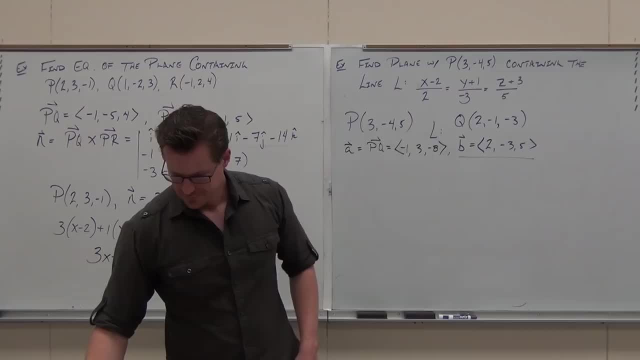 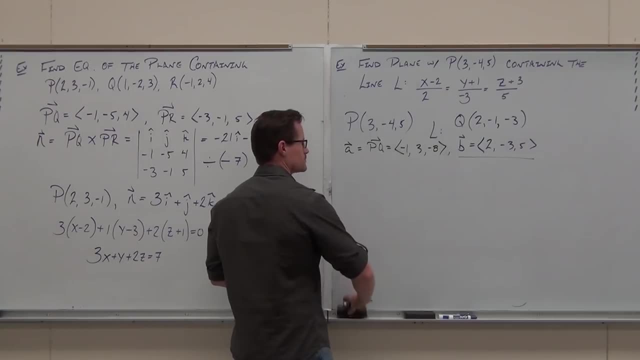 you're still going to find a normal vector. Okay, so point of the plane. yep, check Line of the plane. okay, that has a point, that has a vector. So I've got a vector. I've got another vector. 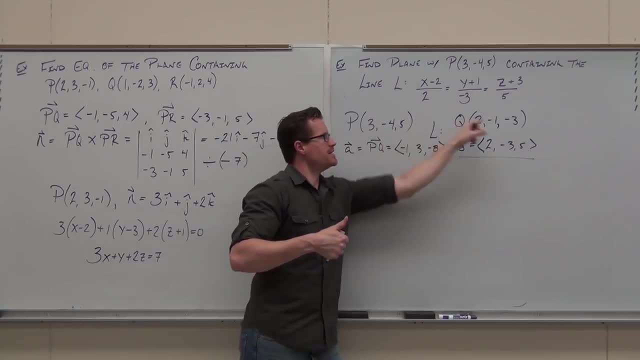 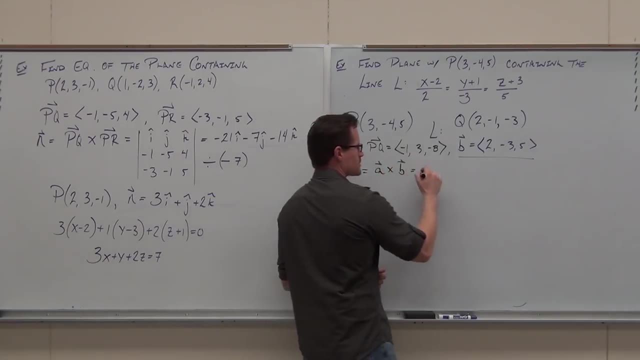 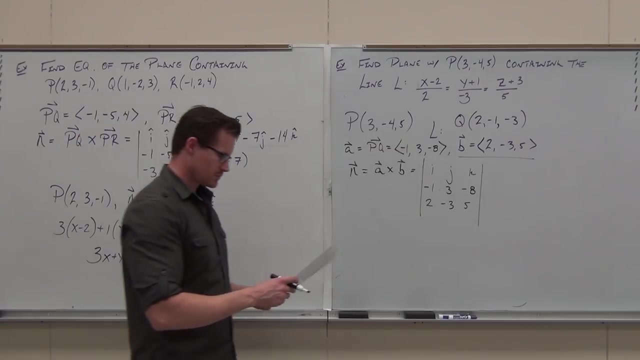 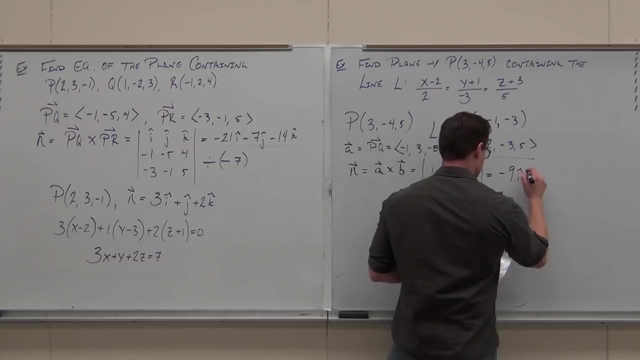 That has a vector. So I've got a vector, I've got another vector. That's two vectors. Let's let our normal be the cross product of the vectors. Let's let our normal be the cross product of the vectors. I want to make sure you get the same thing I'm getting. 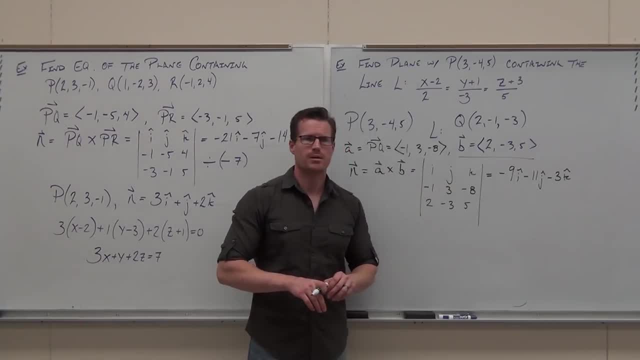 Did you get? if you did it this way, did you get negative 9i minus 11j minus 3k? Did you get that vector? Yes, Yes, What's the first thing you're doing with this nasty vector? Factoring out the negative? 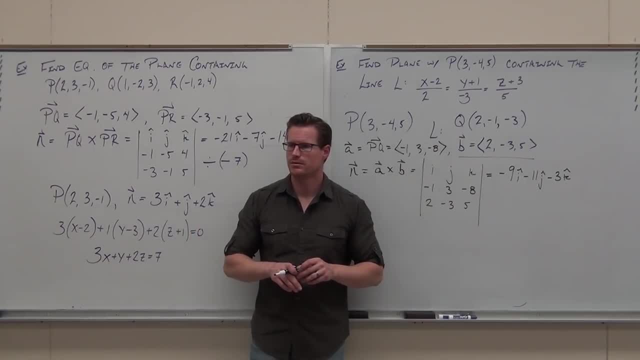 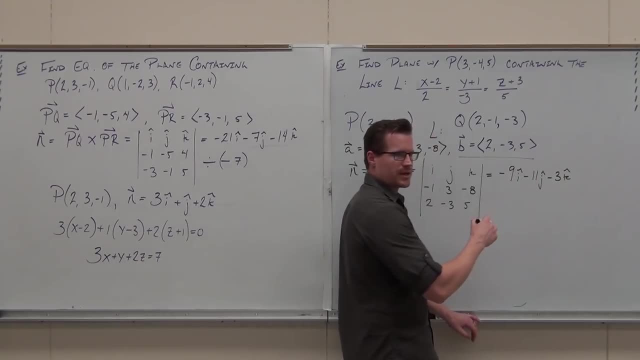 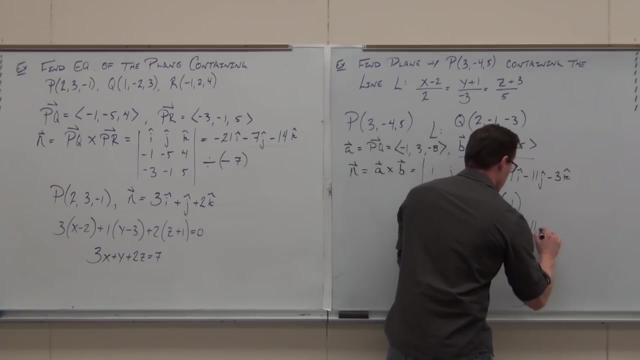 Probably removing what Next parameter? Yeah, factoring out the negative, Because I don't want to deal with all negatives. That's really ugly. So I would multiply or divide by negative 1, whatever you want to do. So I would multiply by negative 1, whatever you want to do. 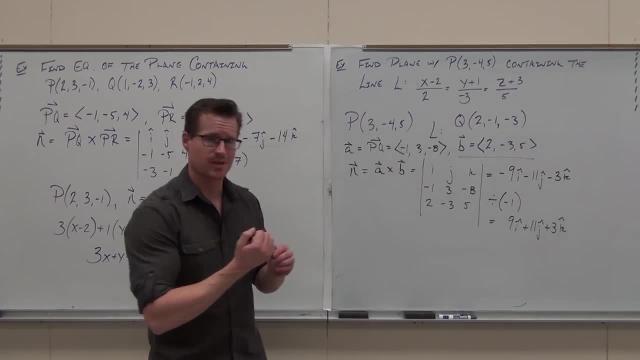 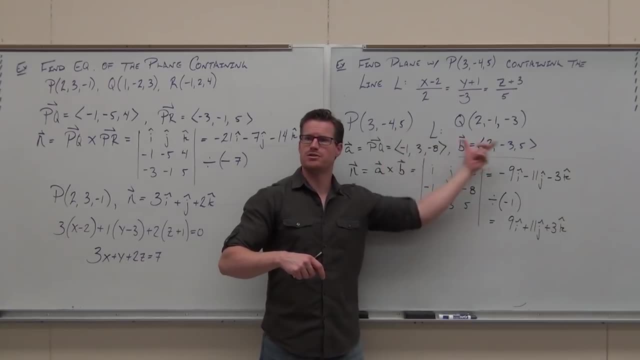 Listen, I told you we're going to move a little quick on this, these topics, because I want to get through a lot of stuff here, but I want to make sure I'm also clear. Are you guys? okay, I'm getting all the way down to at least the idea of you have two vectors. 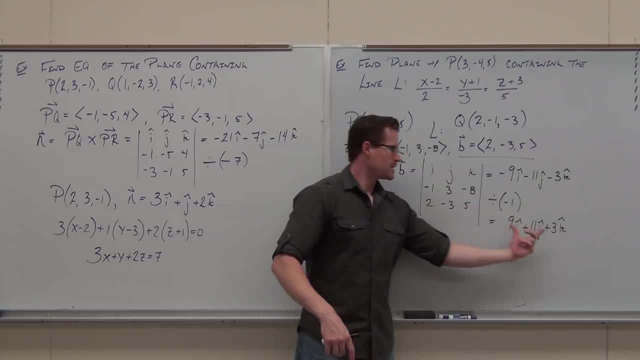 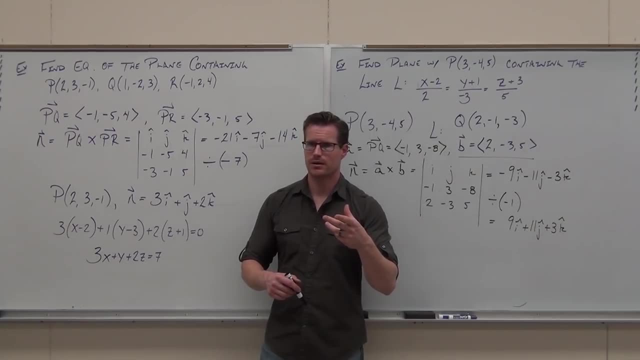 and finding the idea of the cross product. Yes, no, Yes, From here. if you can find your normal vector and you have a point already, can you define the plane? I'm going to leave it to you. Here's the final answer. 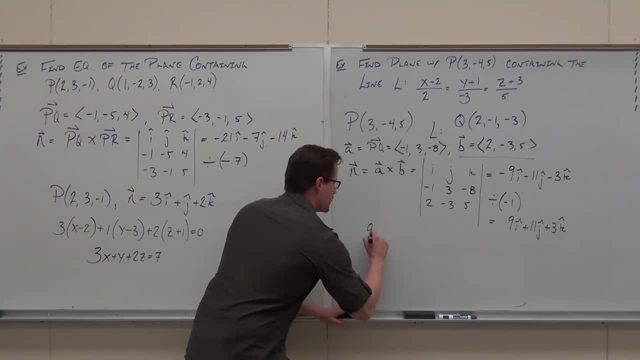 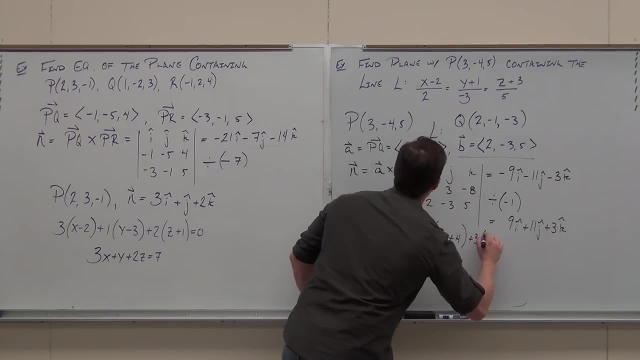 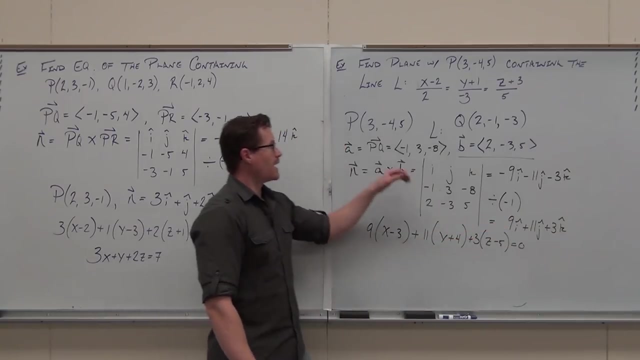 Here's the final answers that we would do. So our plane would be Just using the equation of a plane. we've got my normal vector. Here's 9, 11, 3.. I've got my point Here's: minus 3, plus 4, minus 5.. 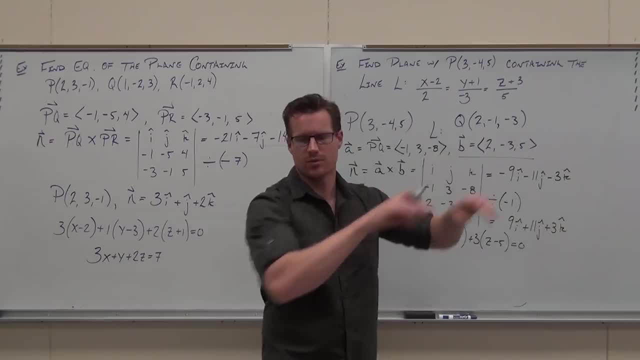 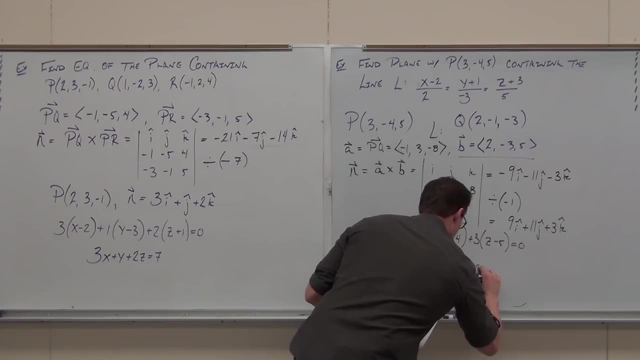 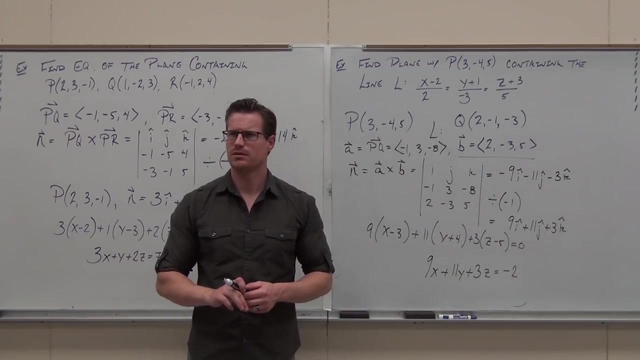 And if we go ahead and distribute and take all of the constants and move them off to the right-hand side, which we're supposed to do, I get negative 2.. Did you get negative 2 as well? Yeah, What did we just find? 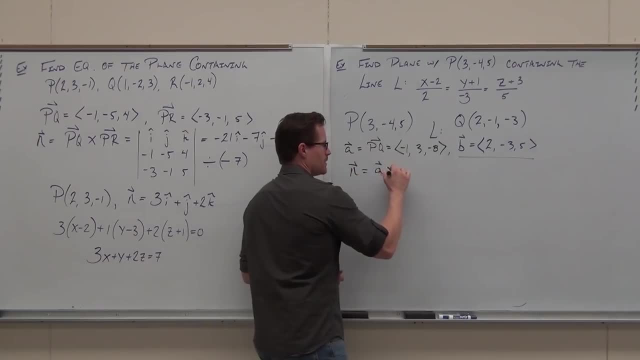 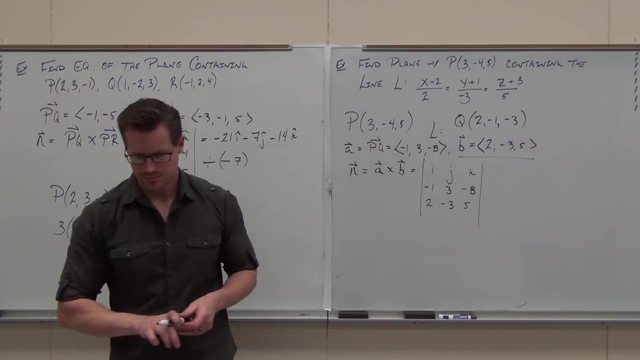 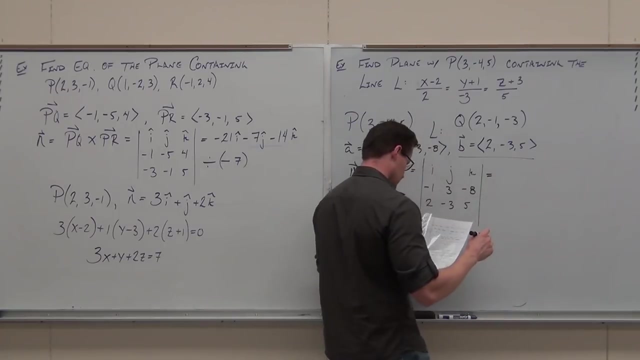 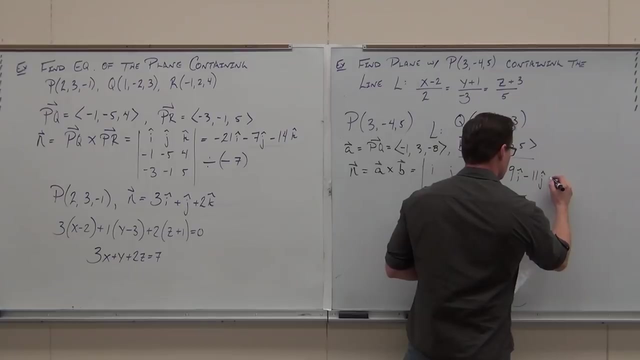 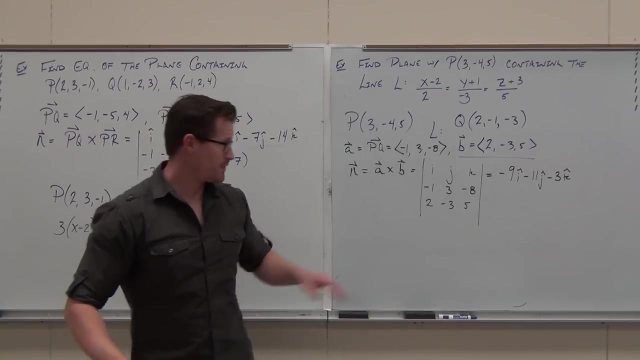 that's two vectors. Let's let our normal be the cross product of the vectors. Oh nastiness, I want to make sure you get the same thing I'm getting. Did you get if you did it this way? did you get negative 9i minus 11j minus 3k? 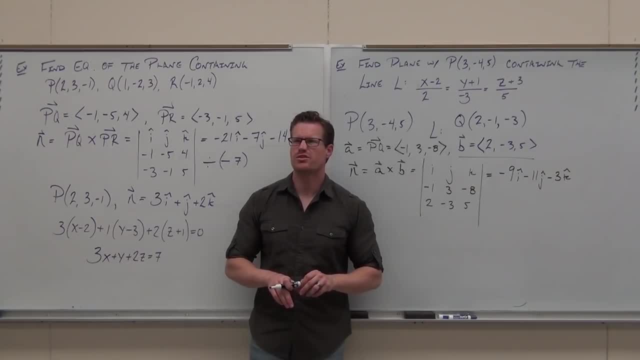 Did you get that vector? Yes, Yes, What's the first thing you're doing with this nasty vector? Factoring out the negative, Probably, removing what Next? Yeah, factoring out the negative, because I don't want to deal with all negatives. that's really ugly. 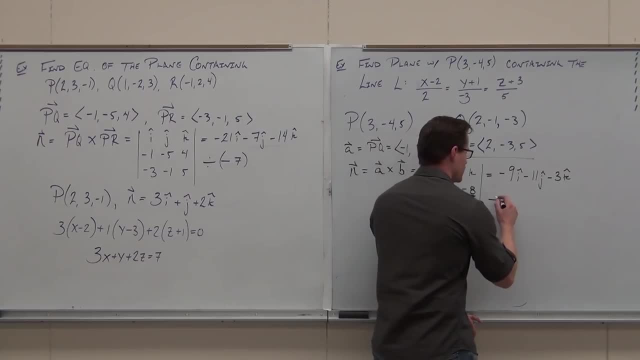 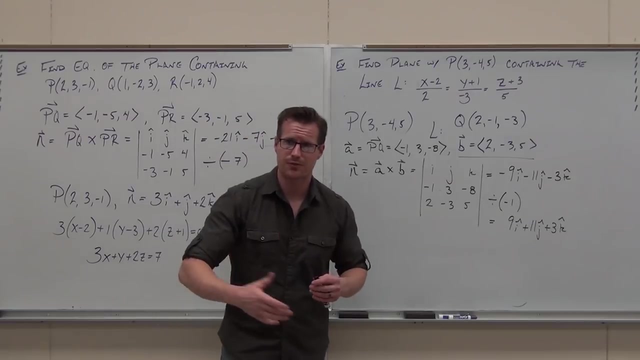 So I would multiply or divide by negative Either one, whatever you want to do. Listen, I told you we're going to move a little quick on this, these topics, because I want to get through a lot of stuff here, but I want to make sure I'm also clear. 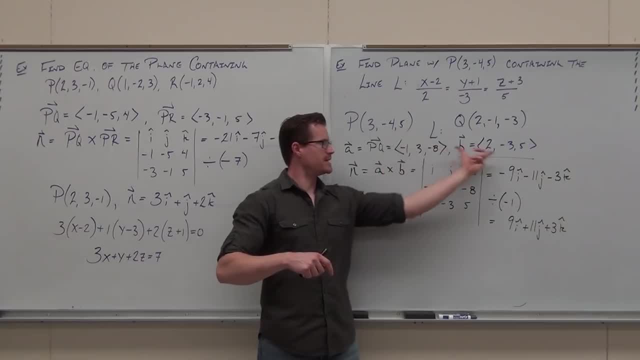 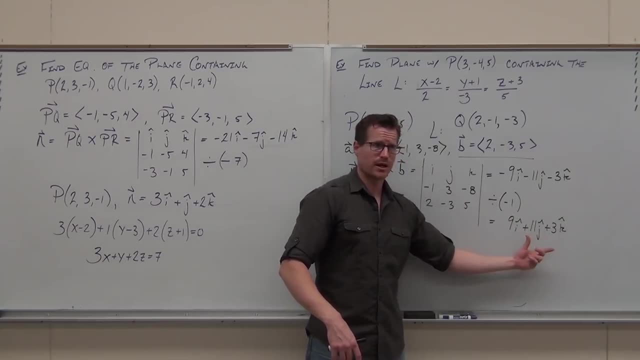 Are you guys? okay, I'm getting all the way down to at least the idea of you have two vectors and finding the idea of the cross product. Yes, no, Yes From here, if you can find your normal vector and you have a point already. 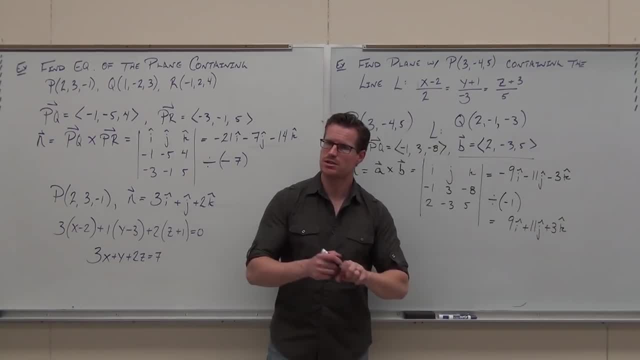 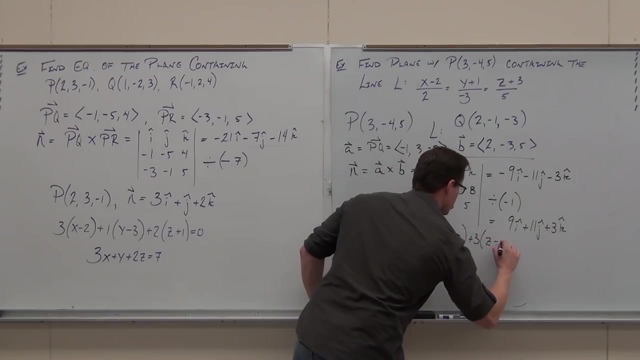 can you just I'm going to leave it to you. Here's the final answers that we would do. So our plane would be Just using the equation of a plane. we've got my normal vector. Here's 9,, 11,, 3.. 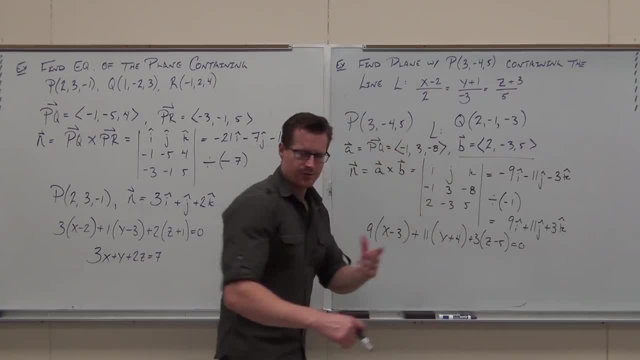 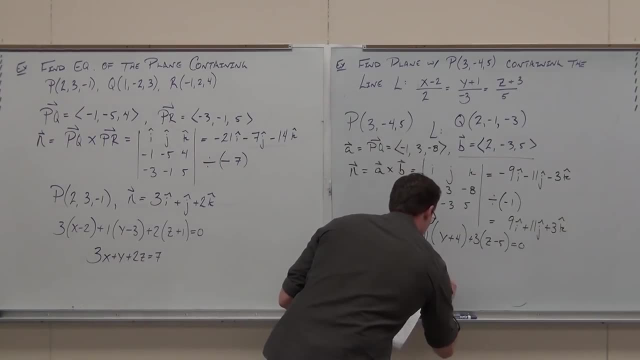 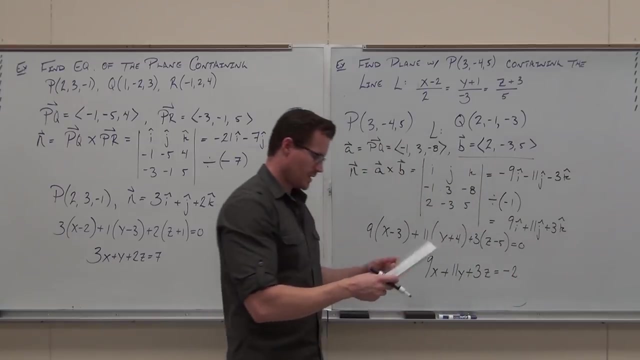 I've got my point. Here's minus 3, plus 4, minus 5.. And if we go ahead and distribute and take all of the constants and move them off to the right-hand side, which we're supposed to do, I get negative 2.. 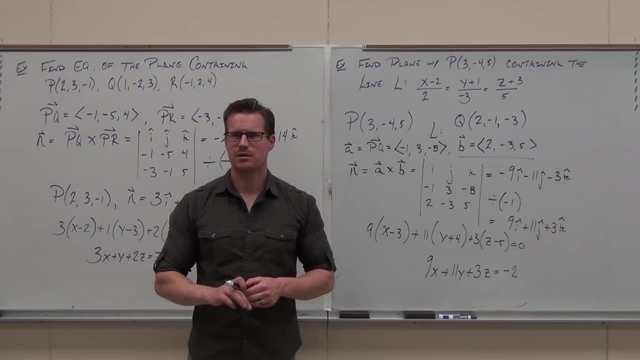 Did you get negative 2 as well? Yeah, What did we just find? Is that a line or is that a plane Plane? It's a plane. It's a plane that contains this point and that line. That's the idea. 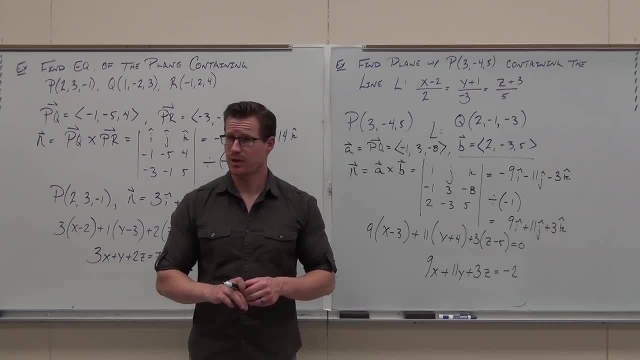 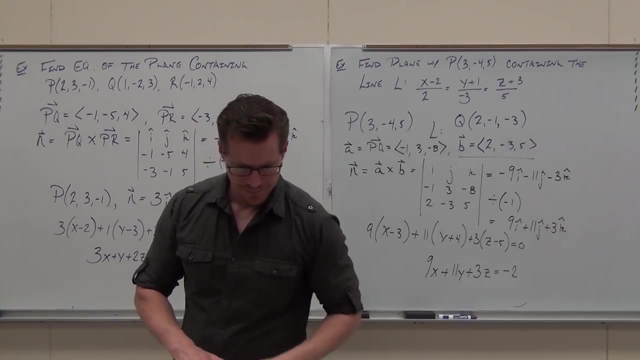 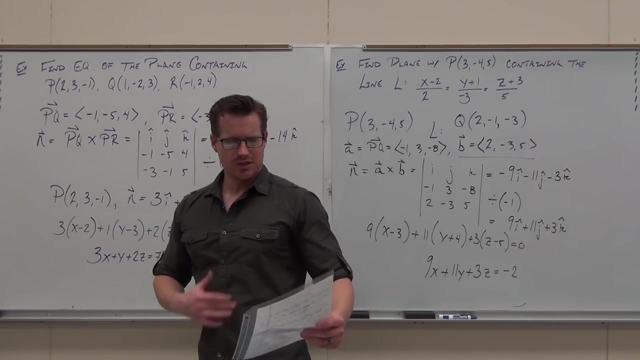 Is that a line or is that a plane Plane? It's a plane. It's a plane that contains this point and that line. That's the idea. Okay, we've got a few more things to do. Next one's a little weird. 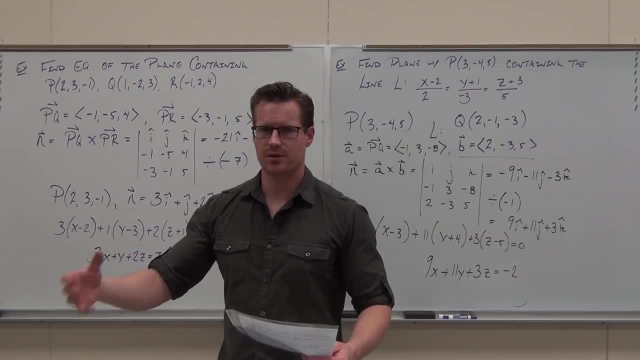 They're all weird. Okay, they're all a little weird. I'm trying to give you the weird ones, so that way I kind of teach you how to think about them. Are you having fun? At least a little bit? Yes, Am I beating your brains into submission, though? 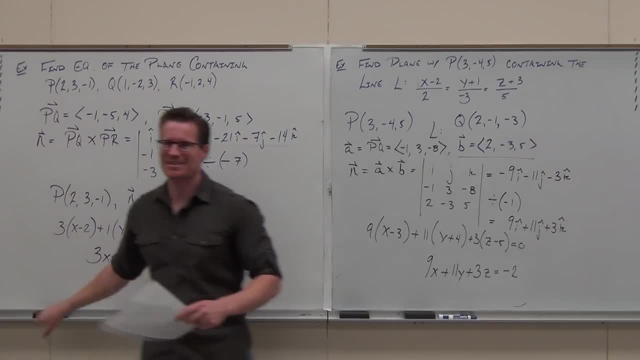 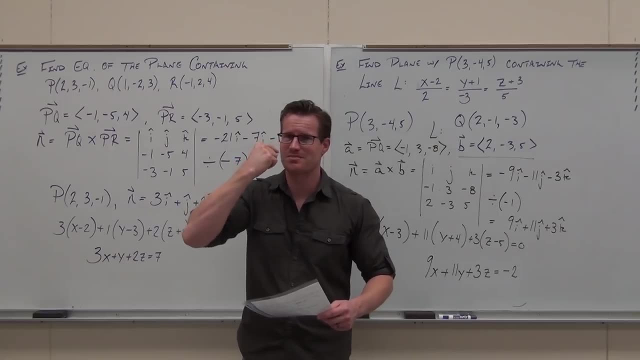 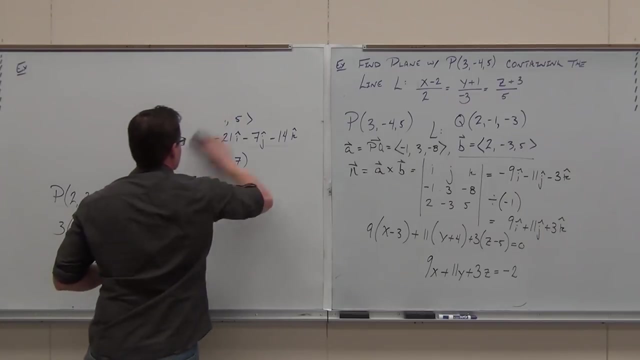 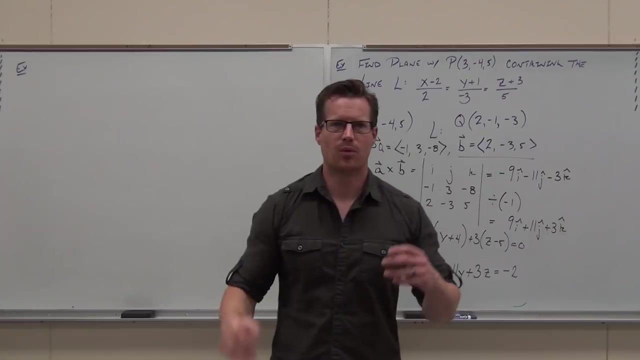 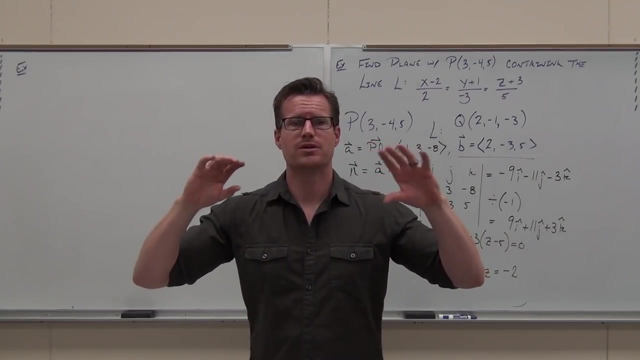 No Good, All right, I love that. Sometimes I look at that and ask that question. you go: Little tears, like little. it's like math tears, I see, like pluses and minuses. Okay, I'm going to give you a little bit of an example of how you do it and then I'm going to give 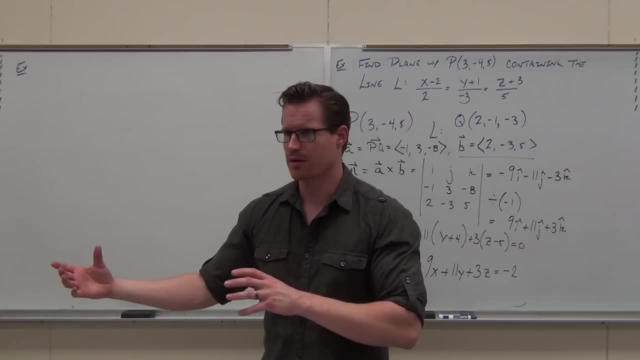 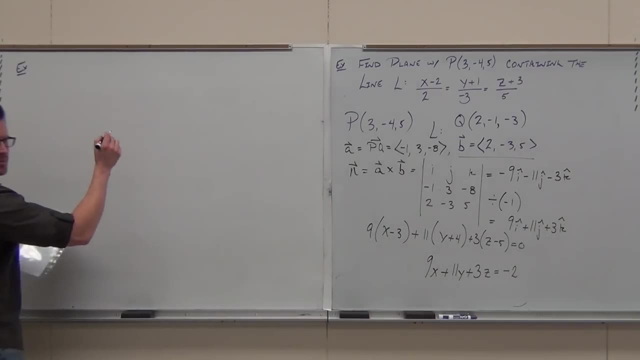 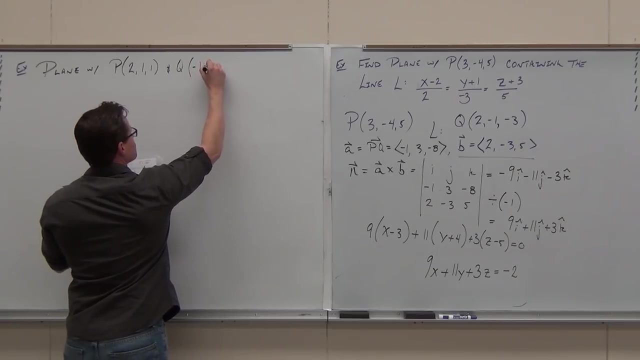 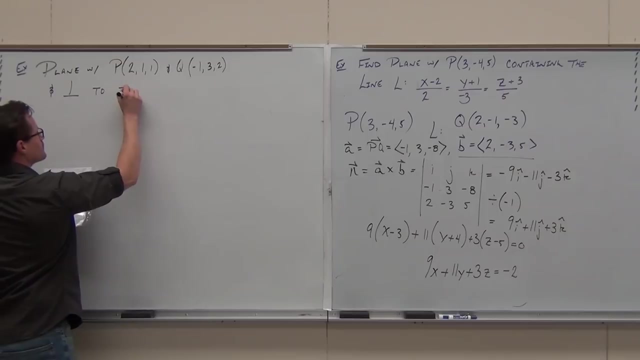 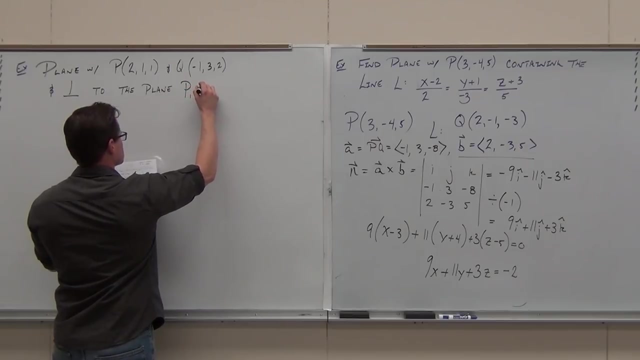 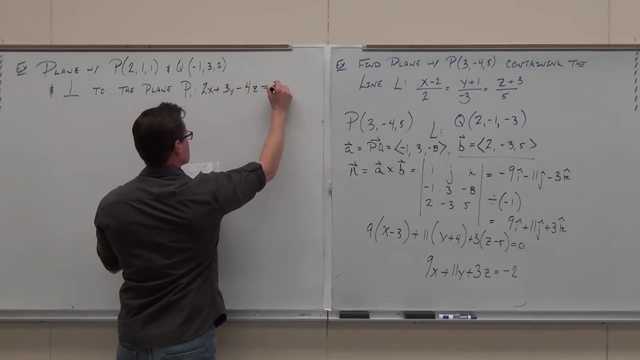 you the answer, But you're expected to be able to go from there. Okay, A lot of it is just thinking about it, Thinking about it, So I want to play with these two points. I'm going to draw this one for you, so you see it. 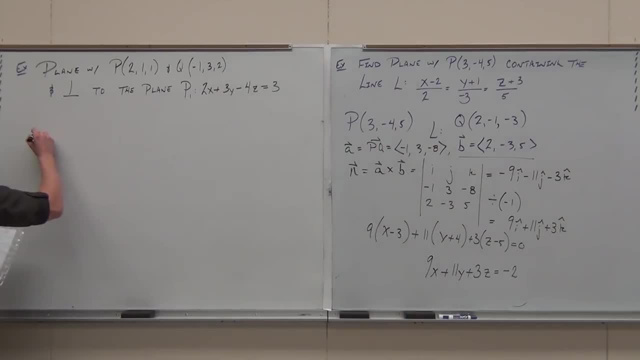 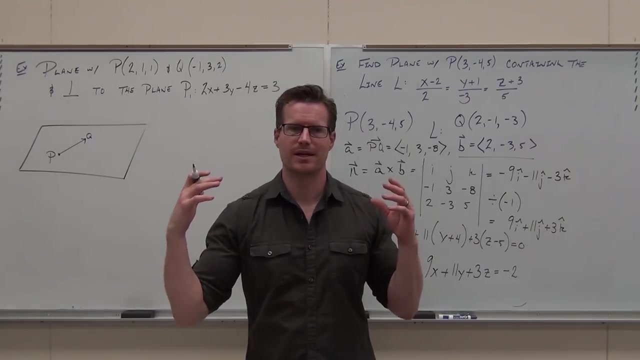 What I want here. I want a plane with two points in it from which I can get a vector Notice, from any two points I can get a vector, so I can automatically get a vector in that plane. That's not the problem. Does that make sense to you? 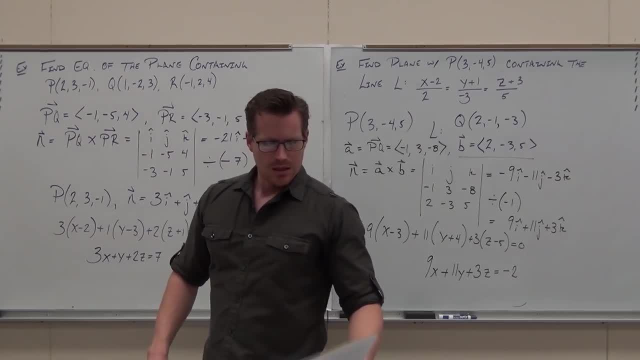 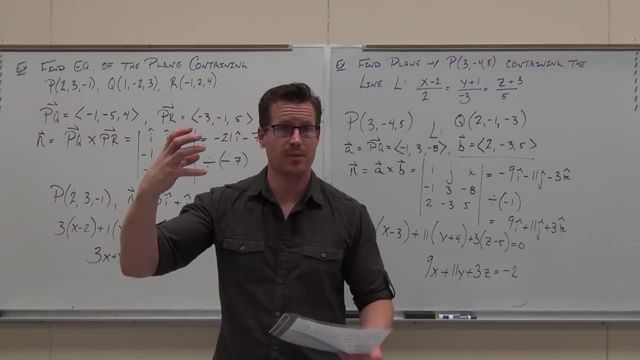 Okay, we've got a few more things to do. Next one's a little weird. They're all weird. Okay, they're all a little weird. I'm trying to give you the weird ones, so that way I kind of teach you how to think about them. 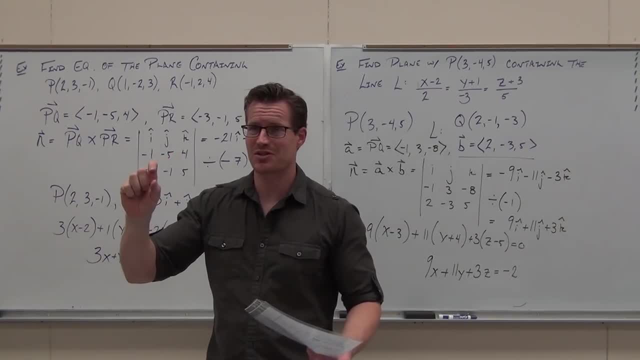 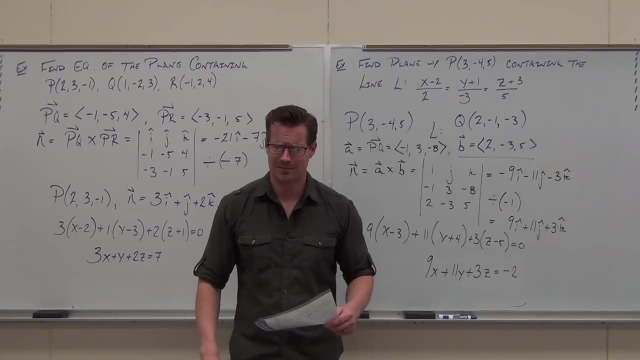 Are you having fun? At least a little bit, Yes, Am I beating your brains into submission though? No, No Good, All right. I love that Sometimes I look out there and ask that question. you go little tears like little tears. 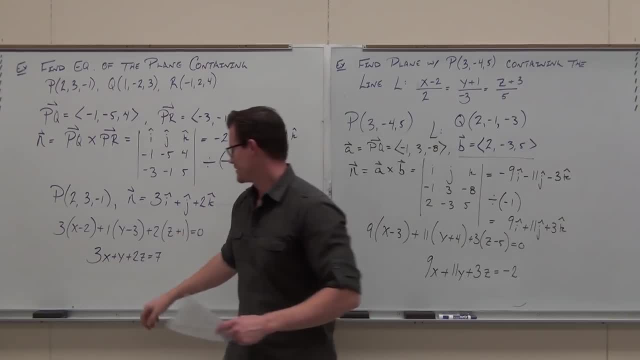 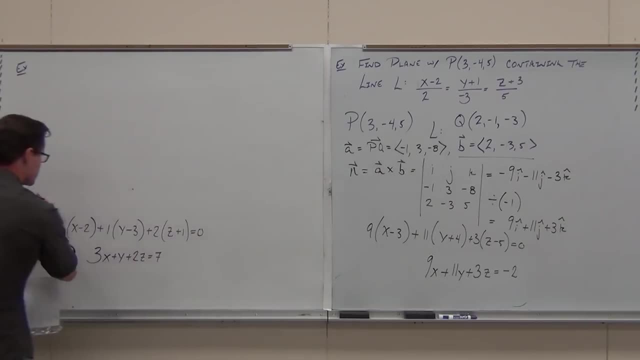 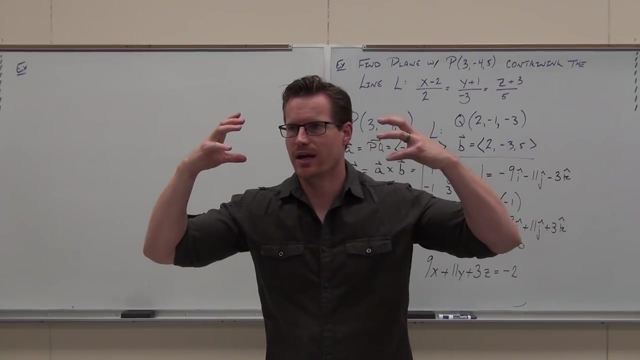 It's like math tears. I see like pluses and minuses. I see like pluses and minuses, Okay, In order, so that I can get more weird ideas in your head, like math weird- okay, not real weird, but like more weird ideas. 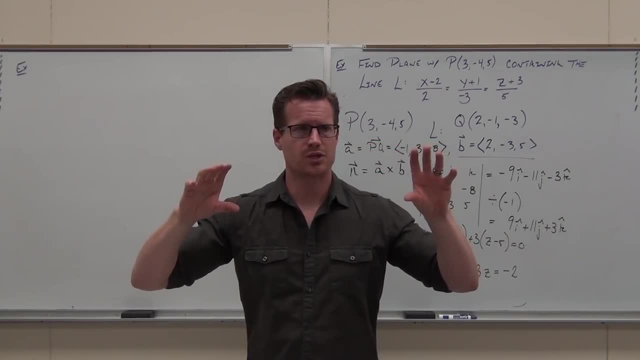 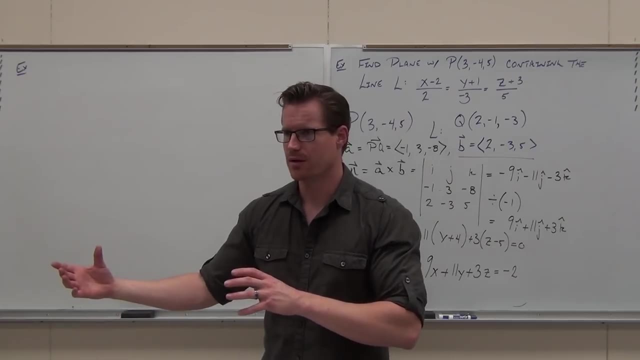 in your head. what I'm going to do is I'm going to give you the example. We're going to talk mostly about the idea of how you do it, and then I'm going to give you the answer, But you're expected to be able to go from there. 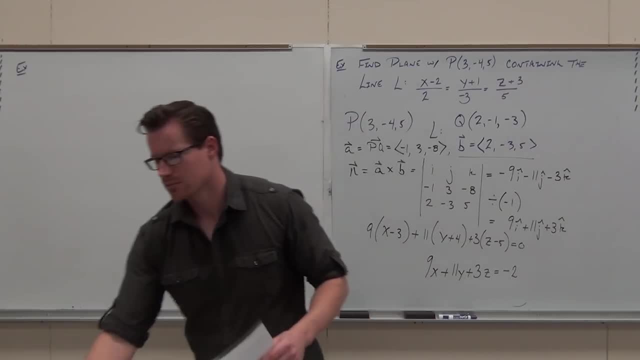 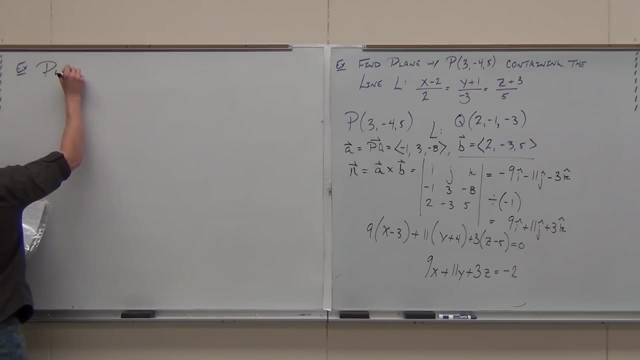 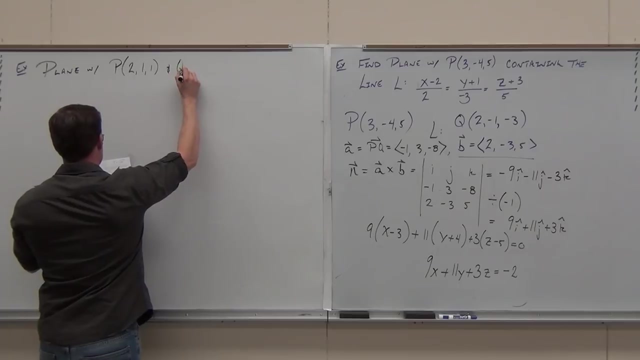 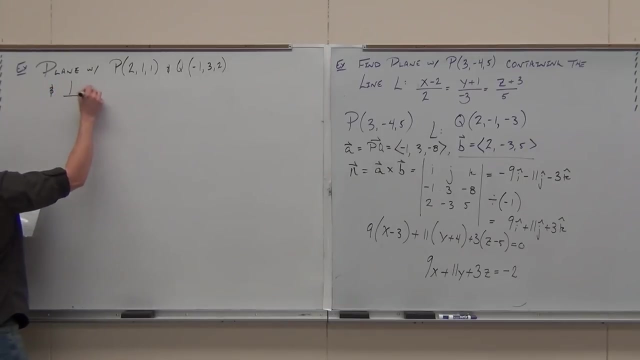 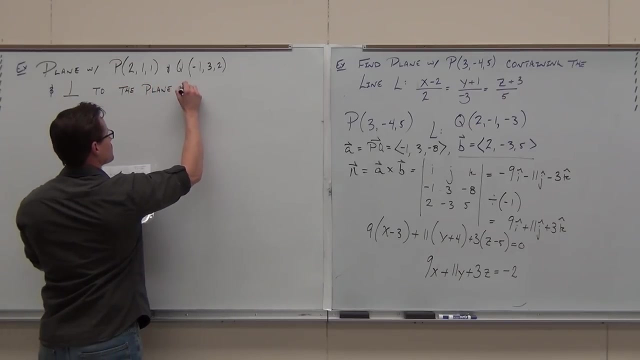 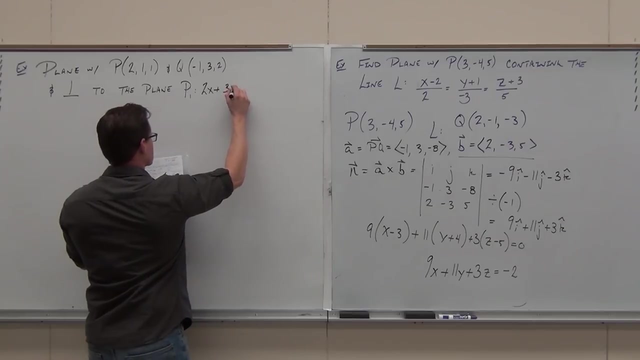 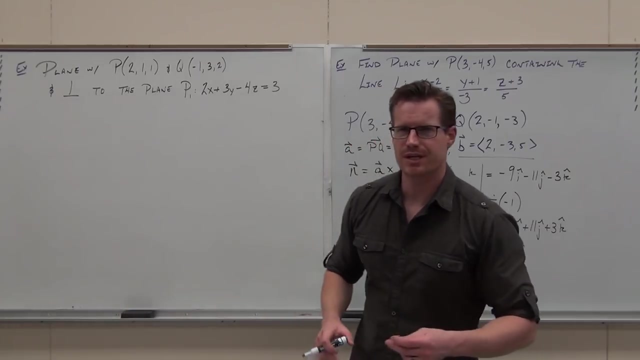 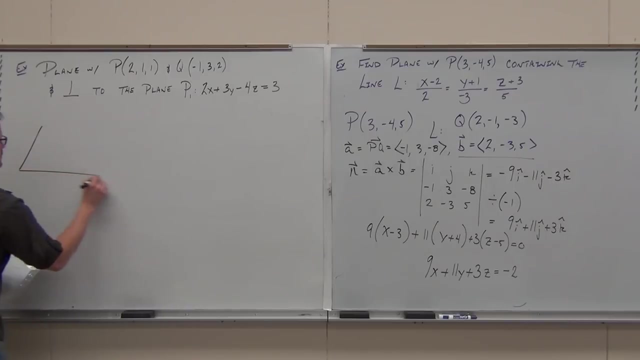 A lot of it is just thinking about it, So I want to play with these two points. I'm going to draw this one for you, so you see it What I want here. I want to play with two points in it From which I can get a vector. 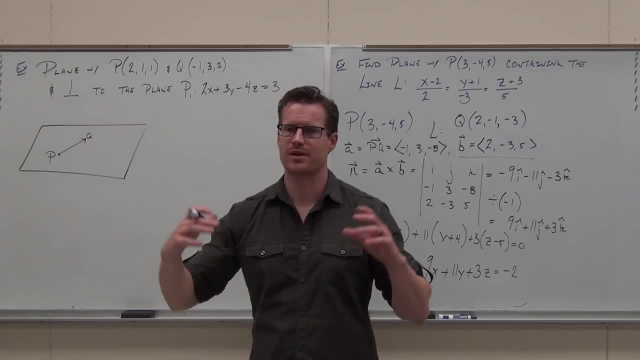 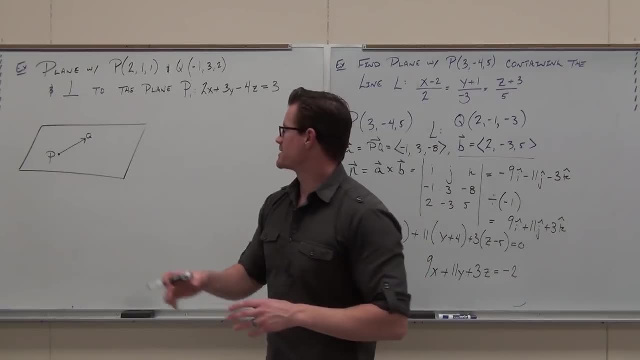 Notice from any two points. I can get a vector, so I can automatically get a vector in that plane. That's not the problem. Does that make sense to you, Are you sure? The problem is: is this one. I also want it perpendicular to this other plane. 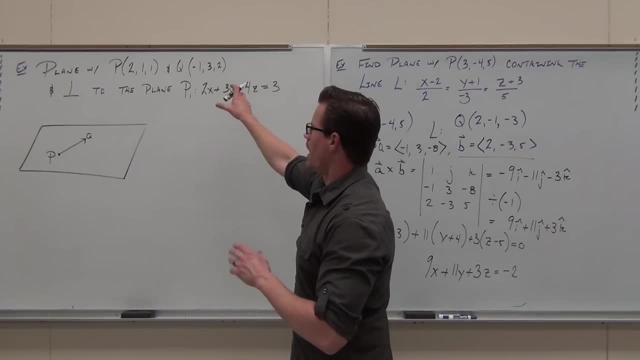 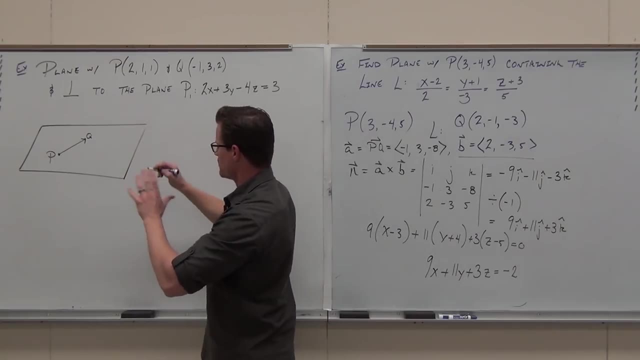 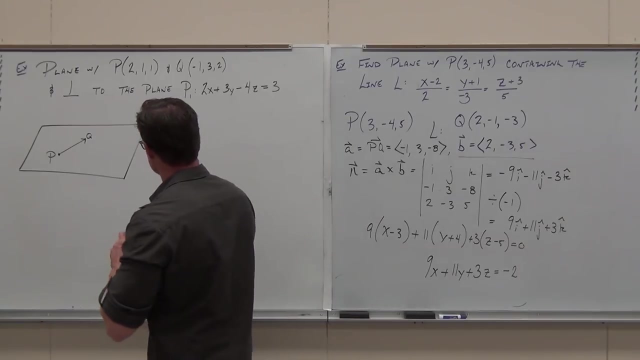 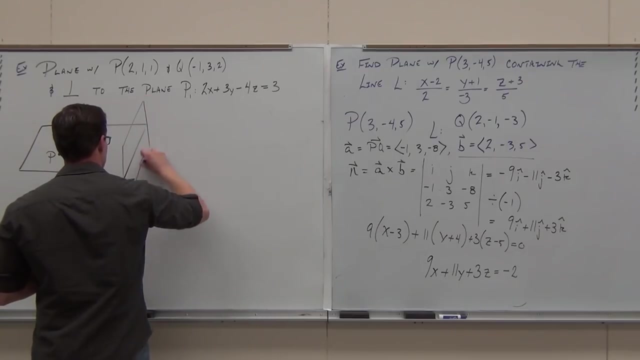 Are you sure? The problem is this one. I also want it perpendicular to this other plane, So I get this plane flying out here that's perpendicular to this plane. So basically, I want I have this. Can you see the picture I'm trying to draw for you? 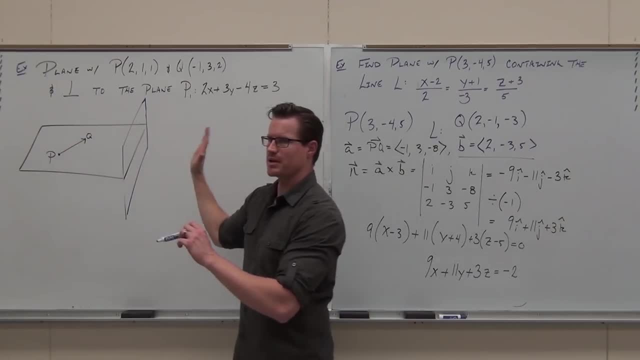 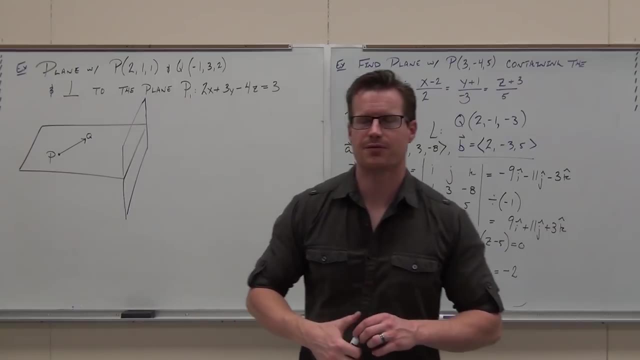 I want you to think of a plane here and a plane that's smashed up against it. Now, here's the point of this: Listen carefully. If you close your ears for a second, you're going to miss it. If you blink, you're going to miss it. 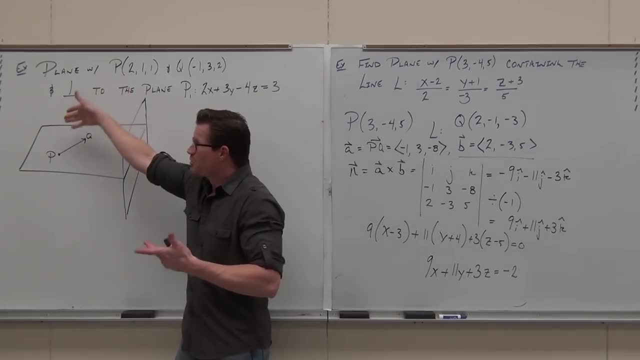 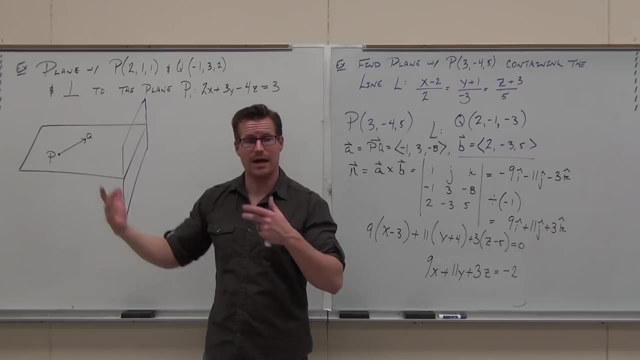 You guys okay on finding that vector. yeah, This one's pretty easy because I got two points- P and Q- You can find a vector. How many vectors do you need in order to find a normal Two? I have one. I'll be able to find one. 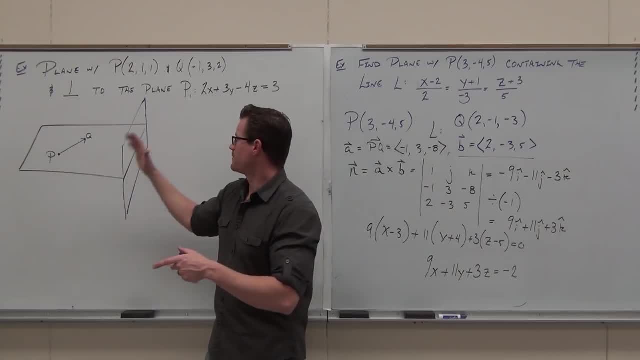 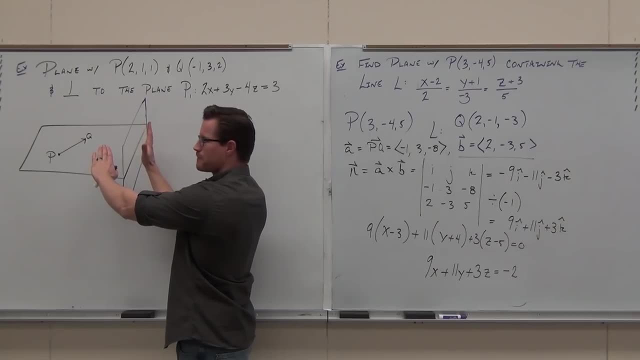 I need another one, but check this out. If this plane- listen carefully- If this plane is perpendicular to this plane, what's the normal of the purple plane got to do, Which means you can fit it in that plane? Does that make sense? 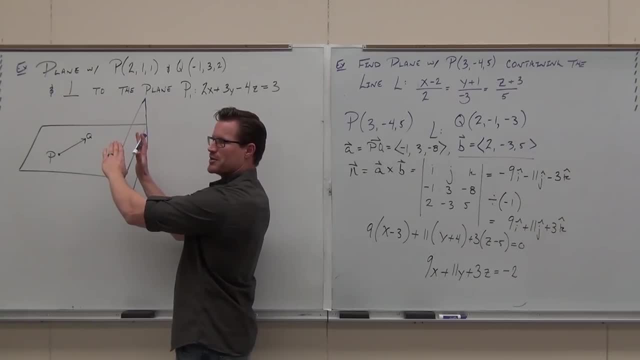 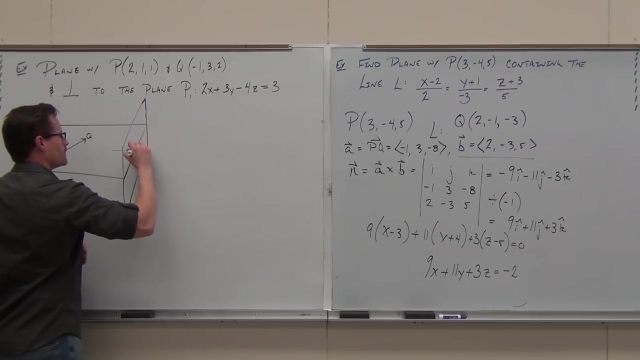 So if the purple plane is perpendicular- purple perpendicular, I say that three times fast to the black plane. the purple plane's got a normal. If it's perpendicular, then the normal to my purple plane has got to be in the black plane. 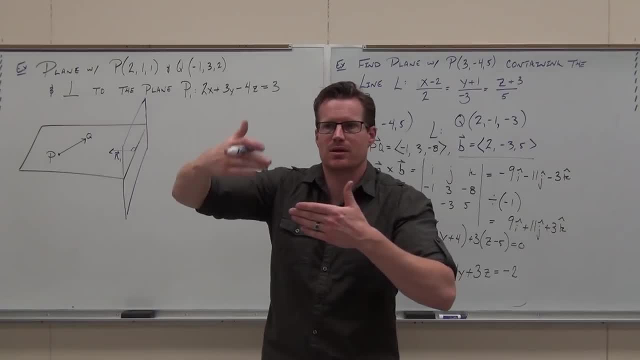 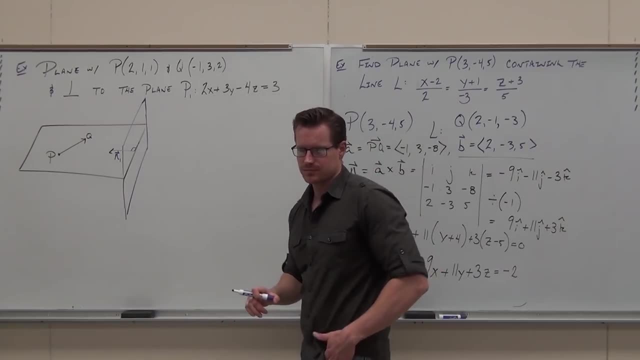 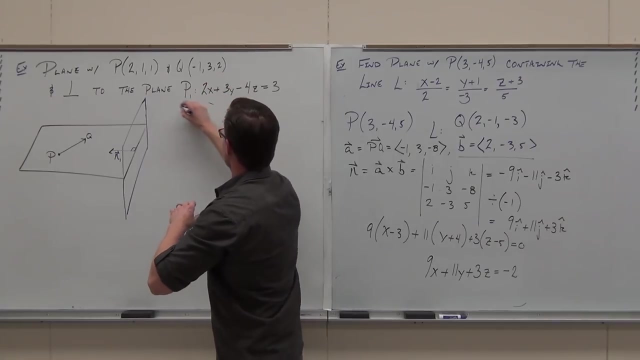 The normal has to be contained in that. Well, it has to be at least parallel to that plane. It's got to be able to be put in that plane. So this whole thing, the perpendicular to the plane. it means that the normal to this plane. 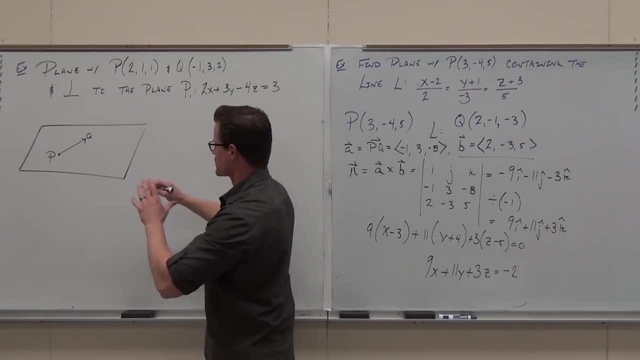 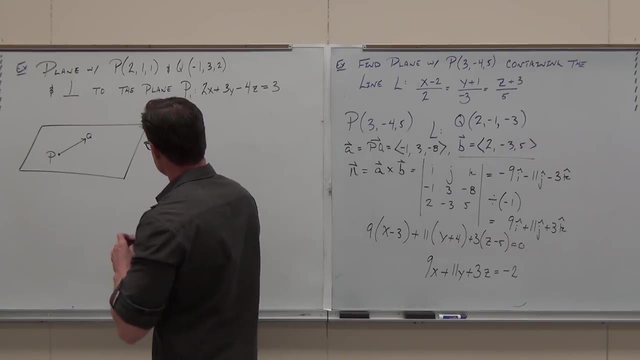 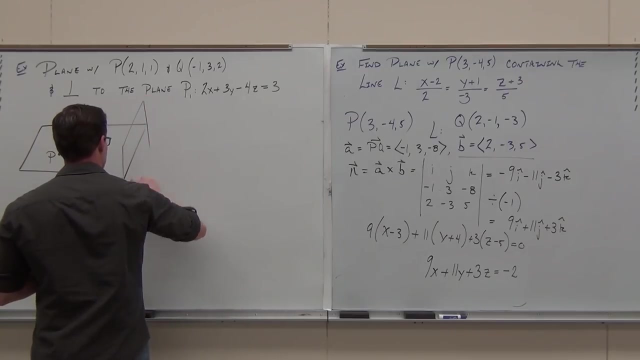 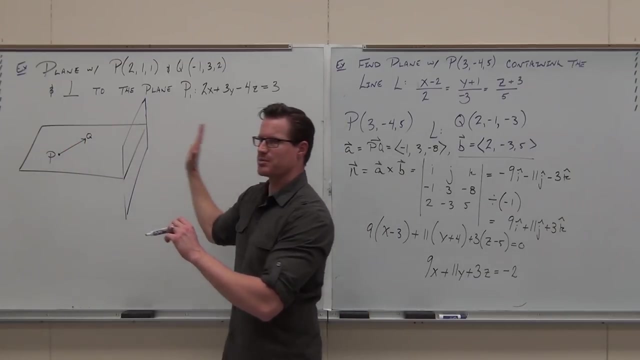 So I get this plane flying out here that's perpendicular to this plane. so basically, I want I have this. Can you see the picture I'm trying to draw for you? I want you to think of a plane here and a plane that's smashed up against it. 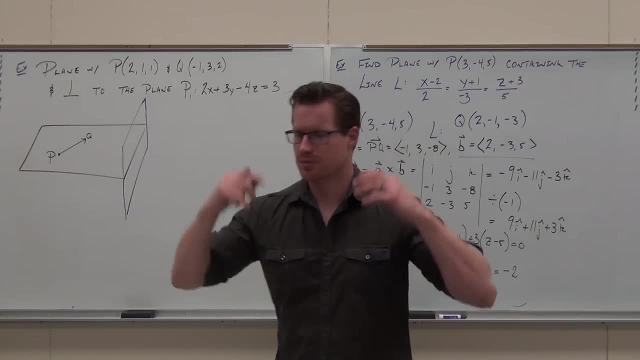 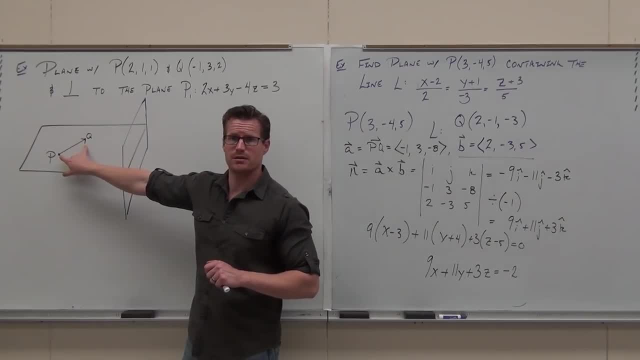 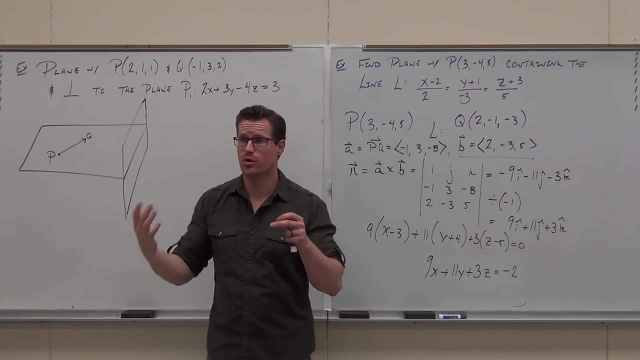 If you blink, you're going to miss it, You guys. okay on finding that vector. yeah, This is pretty easy, because I got two points, P and Q- you can find a vector. How many vectors do you need in order to find a normal? 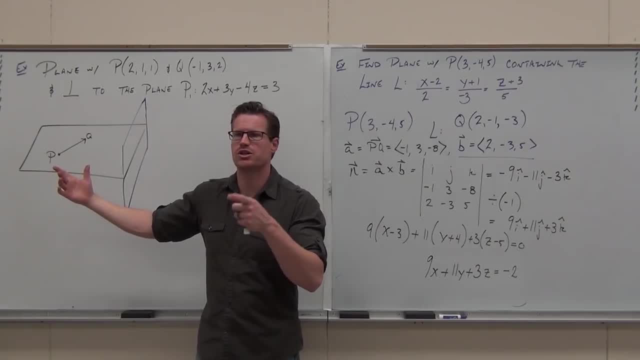 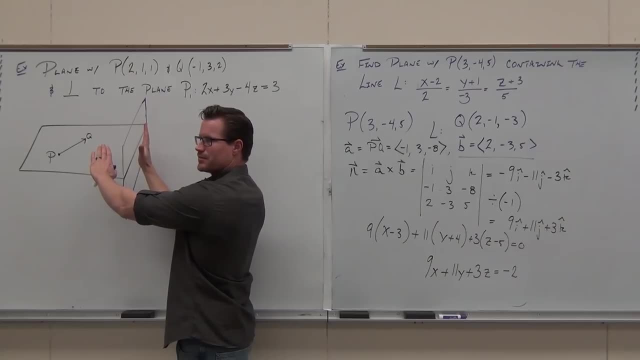 I have one, I'll be able to find one. I need another one, but check this out. If this, listen carefully. If this plane is perpendicular to this plane, what's the normal of the purple plane got to do, Which means you can fit it in that plane? 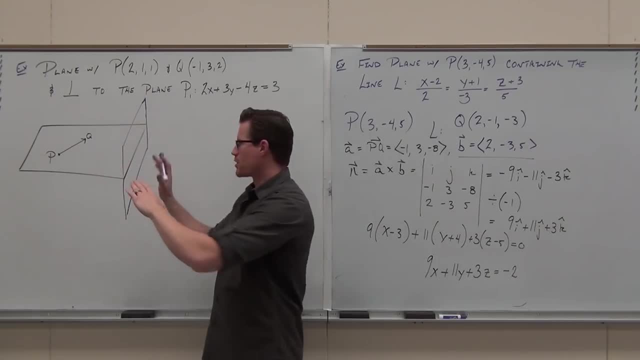 Does that make sense? So if the purple plane is perpendicular- purple perpendicular, I say that three times fast to the black plane. the purple plane's got a normal. If it's perpendicular, then the normal to my purple plane has got to be in the black plane. 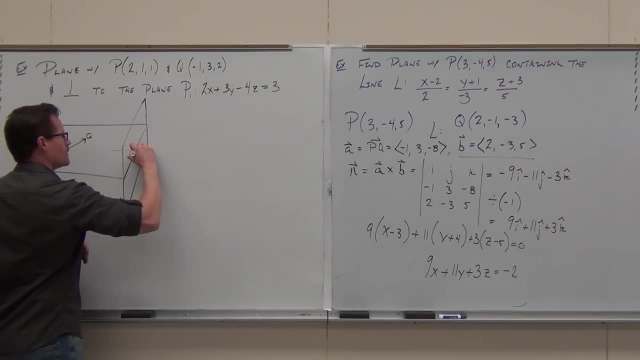 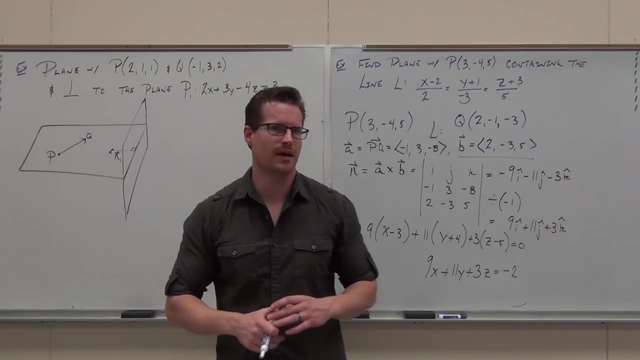 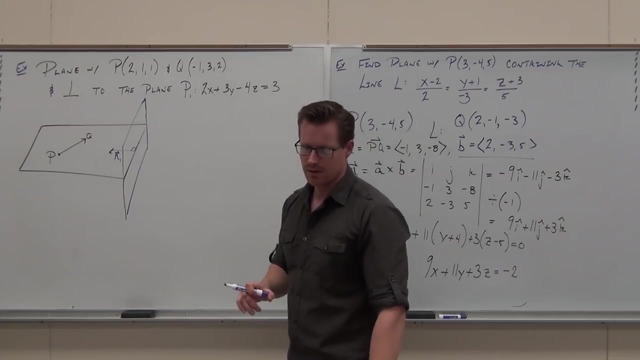 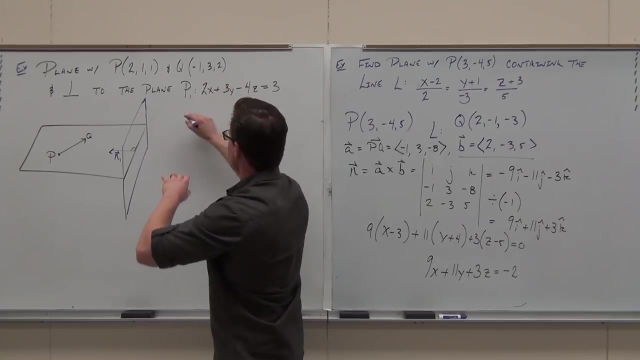 Okay, So if the purple plane is perpendicular to the black plane, the normal has to be contained in that. Well, it has to be at least parallel to that plane. It's got to be able to be put in that plane. So this whole thing, the perpendicular to the plane, 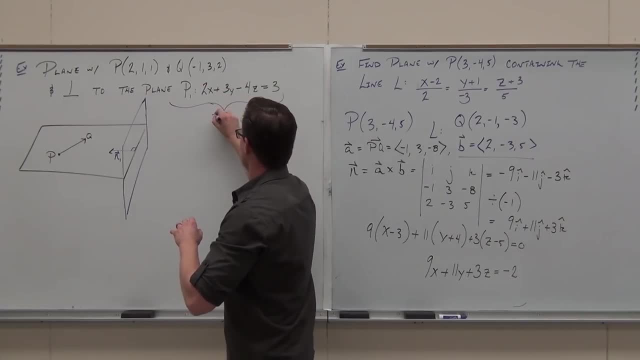 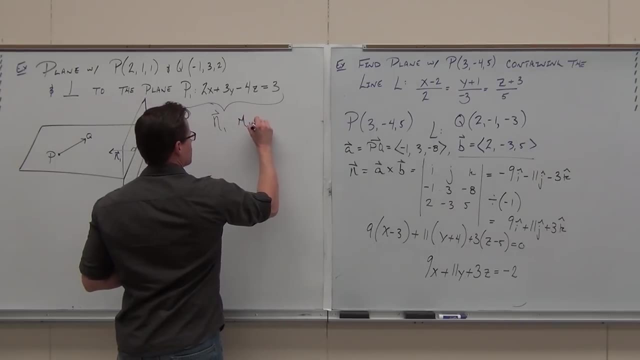 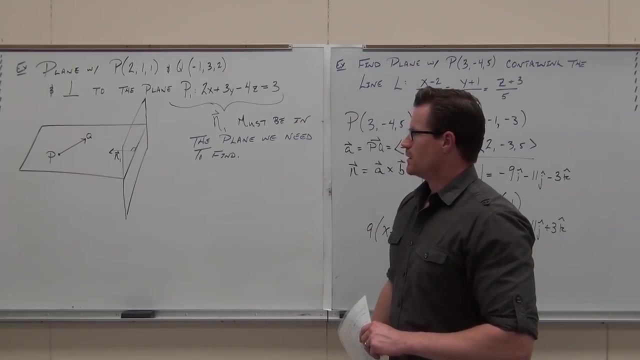 it means that the normal to this plane must be into the one we're trying to find It's got to be, So I'm going to do it on your own. Well, I'm going to have you do it on your own, but here's the idea. 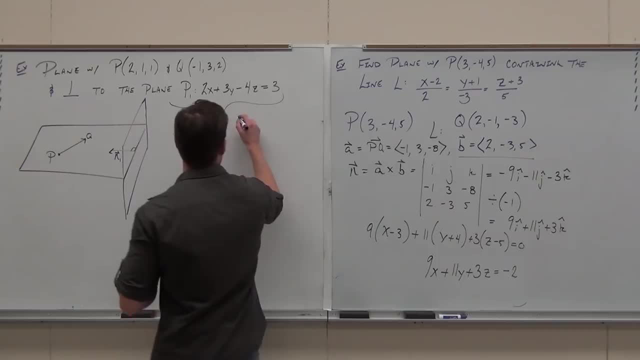 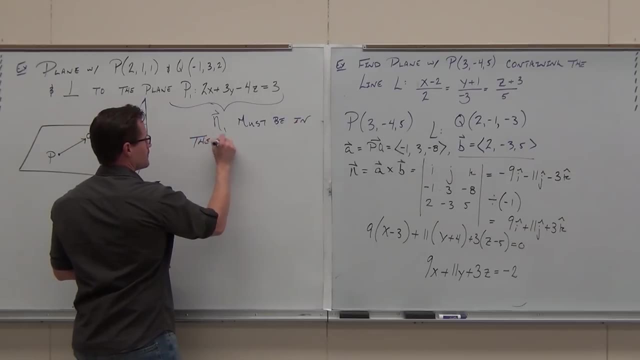 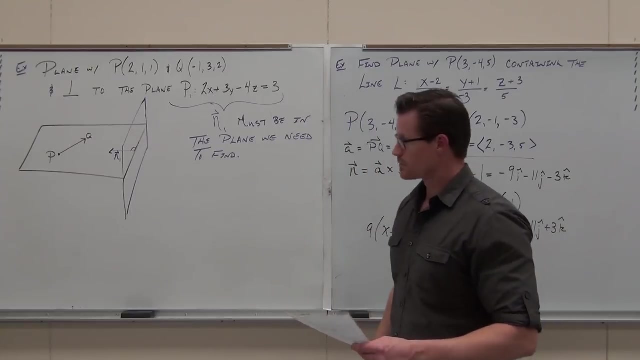 must be into the one we're trying to find. It's got to be. So I'm going to do it on your own. Well, I'm going to have you do it on your own. but here's the idea. Well, I've already given it to you. but the rundown. 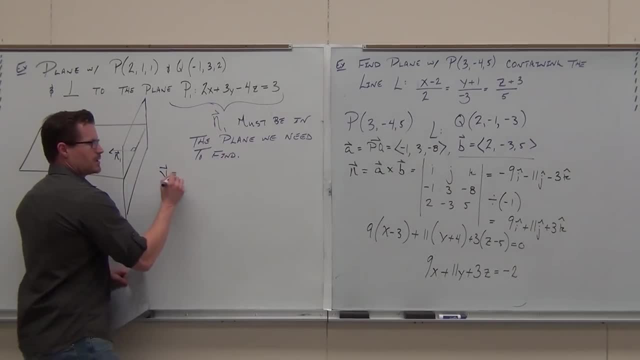 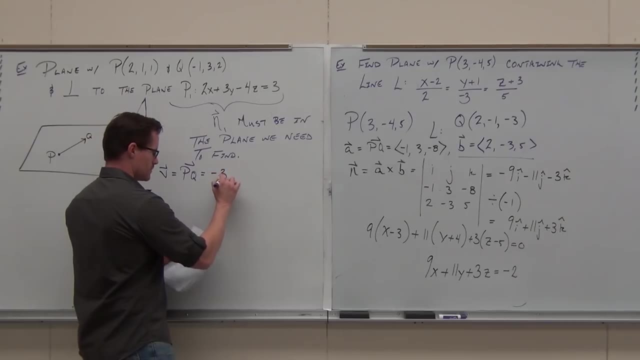 The rundown is number one thing. if we find a vector from P to Q, you need to be able to find that That's the vector from P to Q. You can probably see it right now If we have the normal from that plane. 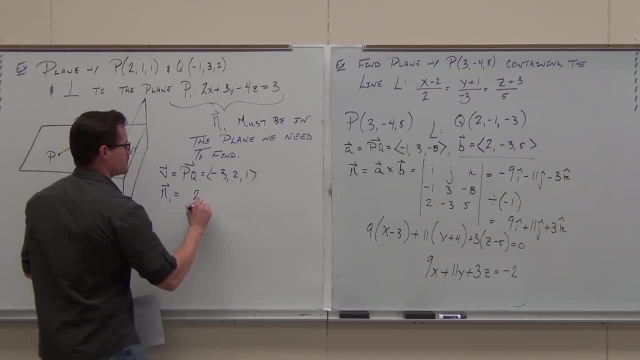 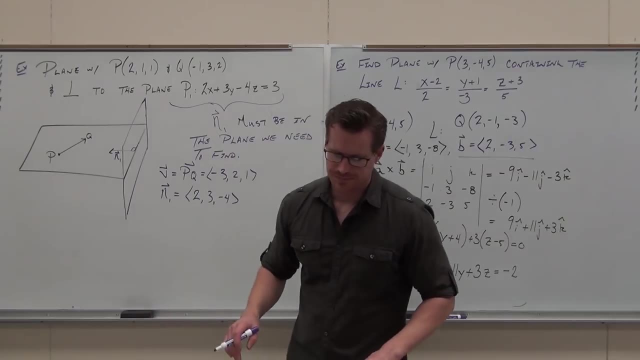 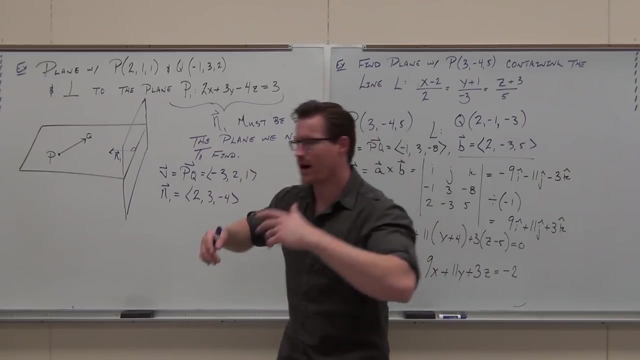 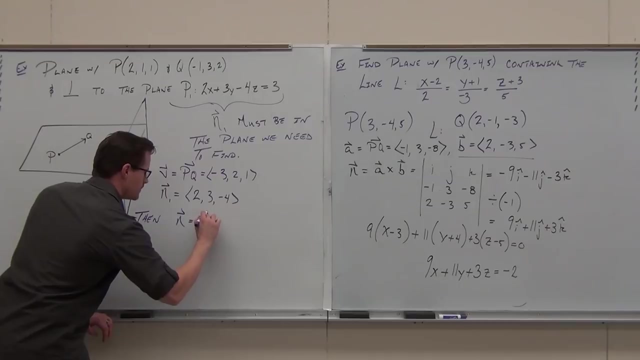 can you find the normal from that plane? I like that. It's pretty easy. If I find the normal from that plane, then, man, the normal for the plane we want to find, it's got to be that normal. It's got to be that normal. 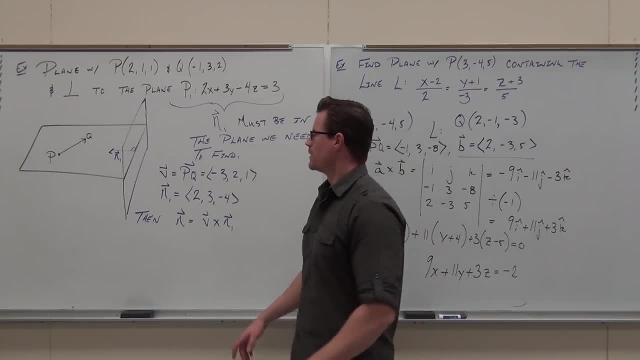 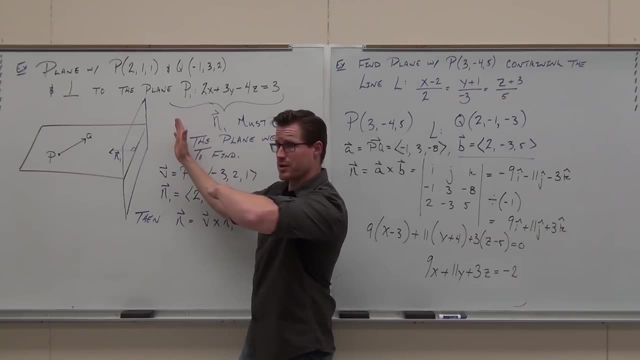 We'll run through it like one more time and then I'm going to give you an answer. Got a couple points. You can find a vector. That's the vector. I've got a plane that's perpendicular. If a plane's perpendicular to another plane, 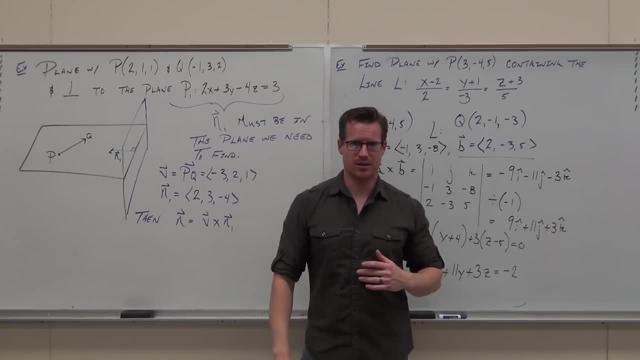 the normal from your perpendicular plane. it's got a line. the plane you're trying to find That gives me one, two vectors, two vectors With any two vectors. you can find a cross product If this vector's in the plane and this vector's in the plane. 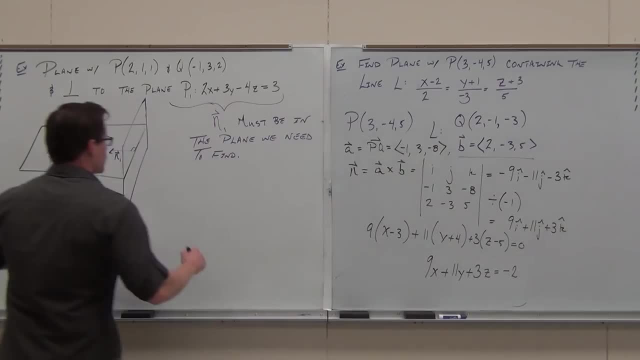 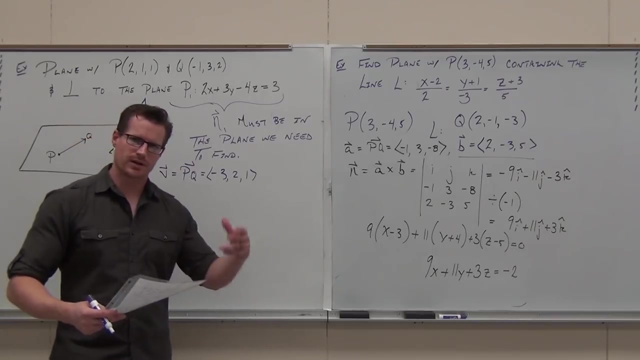 Well, I've already given it to you, but the rundown. The rundown is number one thing. if we find a vector from P to Q, you need to be able to find that. That's the vector from P to Q. You can probably see it right now. 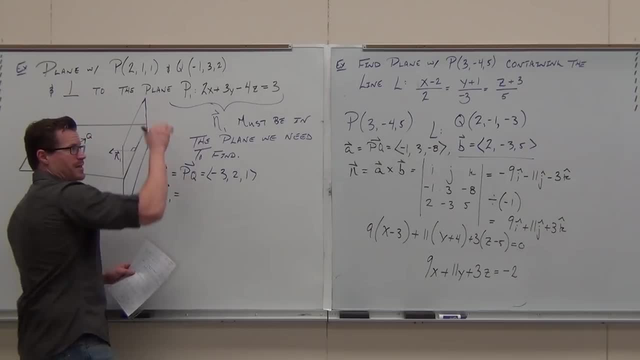 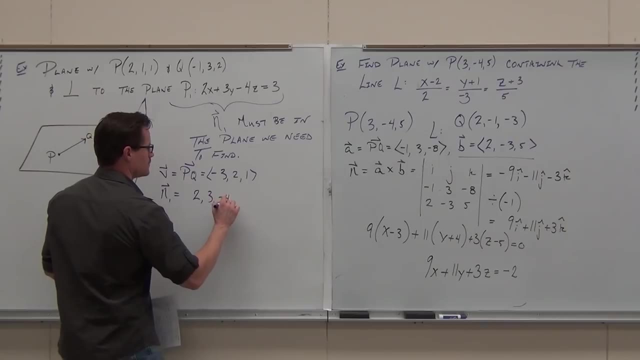 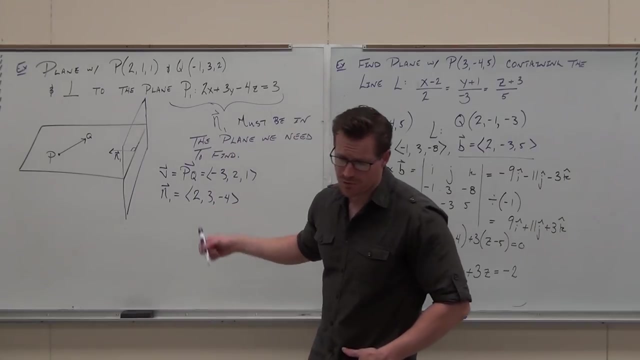 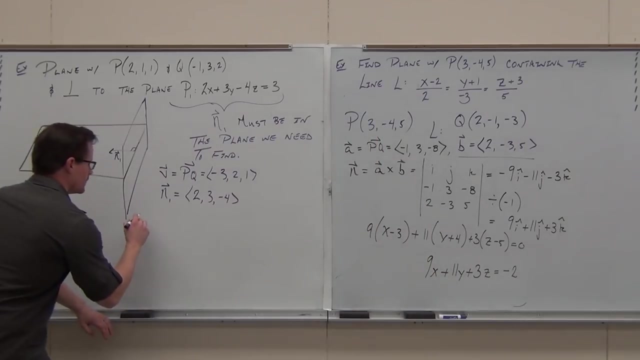 If we have the normal from that plane. can you find the normal from that plane? I can, It's pretty easy. If I find the normal from that plane, then man, the normal for the plane we want to find, it's got to be that normal. 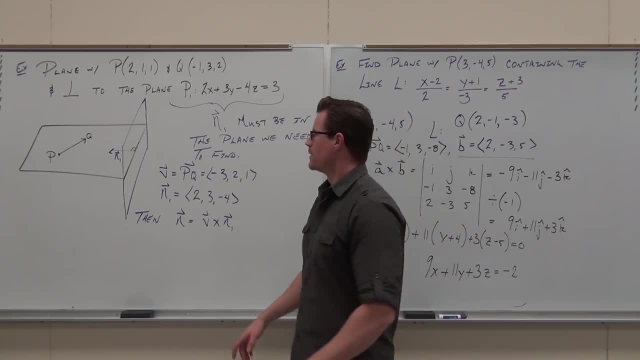 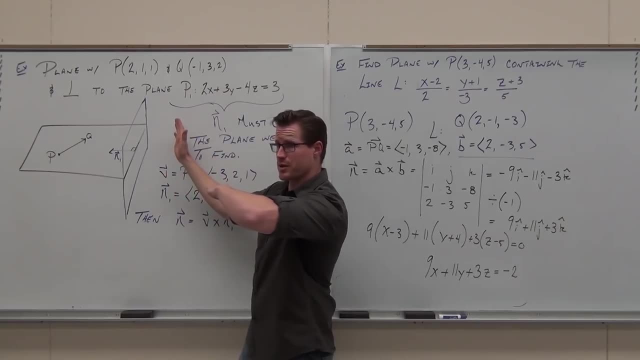 We'll run through it like one more time. then we're going to. I'm going to give you an answer. Got a couple points. You can find a vector. That's the vector. I've got a plane that's perpendicular. If a plane's perpendicular to another plane, 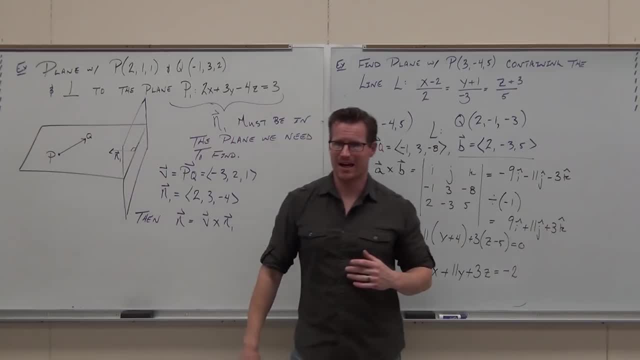 the normal from your perpendicular plane. it's got a line. the plane you're trying to find That gives me one, two vectors, Two vectors With any two vectors. you can find a cross product If this vector's in the plane and this vector's in the plane. 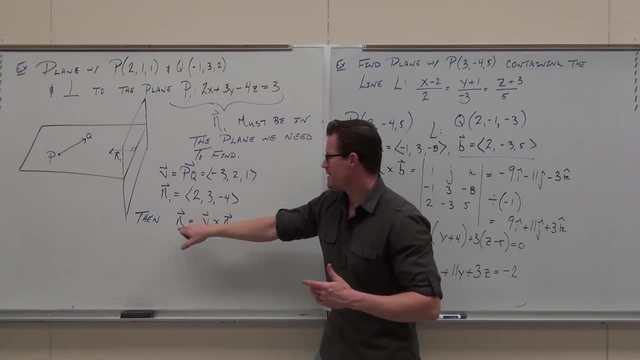 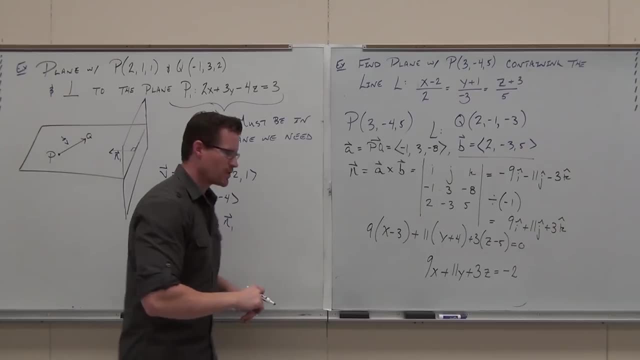 cross product says I get a normal for that plane. That's what this says. Then my normal can be: hey, take V, cross it with N1.. You know how to do a dot product? I'm going to give you the answer. 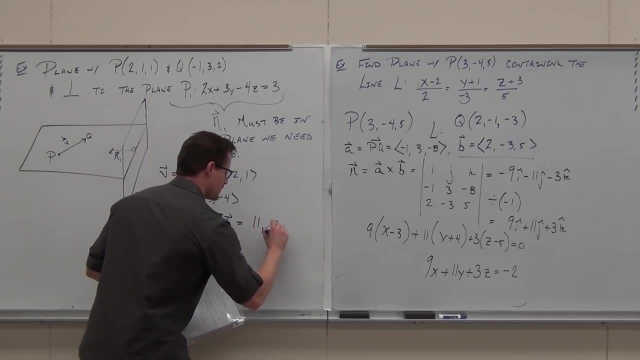 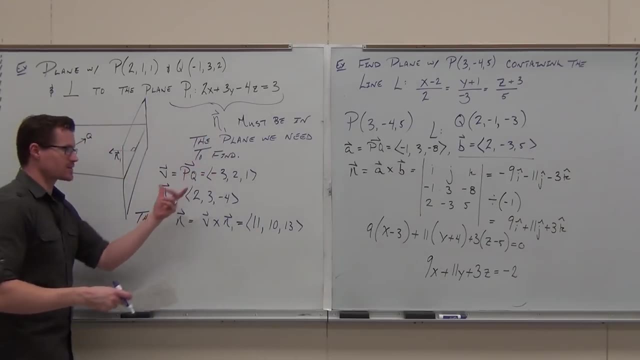 This is 11,, 10,, 13.. Of course, I want you to try this on your own. Walk through it. Make sure you can get this vector. You understand where this is coming from. You get the idea that these two things are in here. 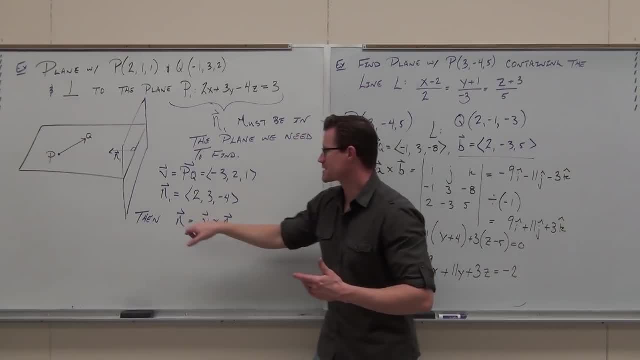 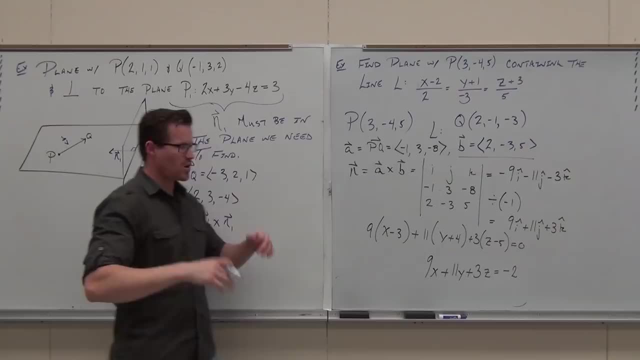 cross product says I get a normal for that plane. That's what this says. Then my normal can be: hey, take V, cross it with N1.. You know how to do a dot product? I'm going to give you the answer. 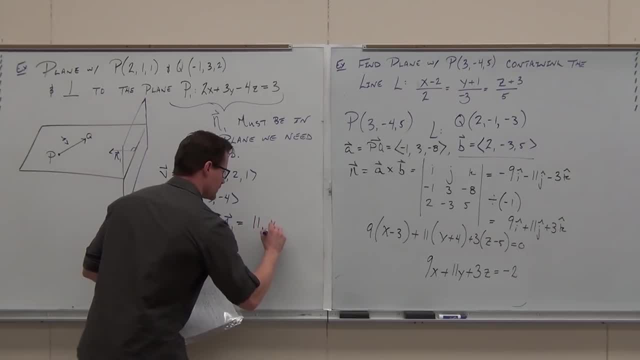 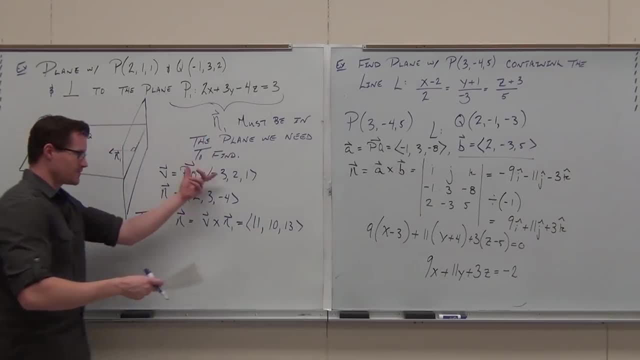 This is 11,, 10,, 13.. Of course, I want you to try this on your own. Walk through it. Make sure you can get this vector. You understand where this is coming from. You get the idea that these two things are in here. 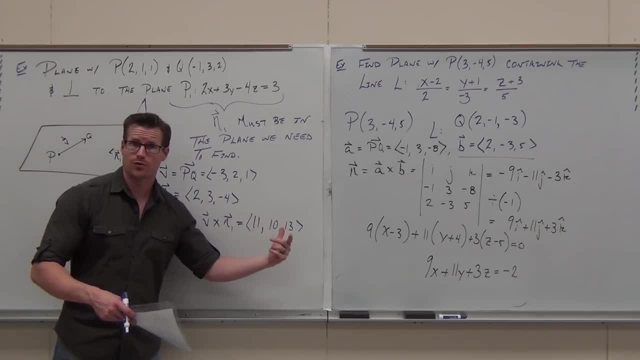 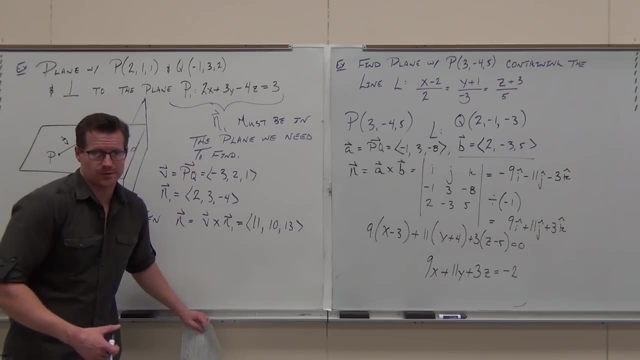 in this plane you're trying to find. Therefore, my cross product is actually going to work for us. This is my normal vector. Now, do I have a point? Yes, Which point do you want to use? Doesn't matter. Do you have a normal vector? 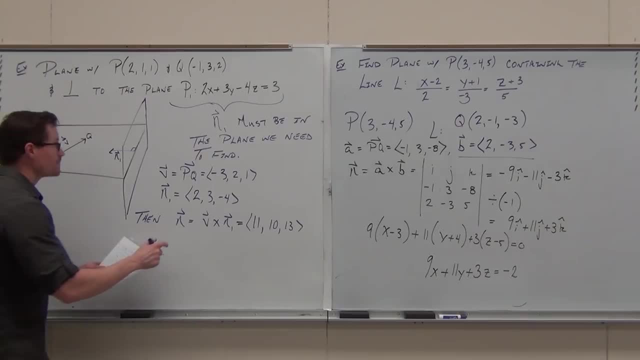 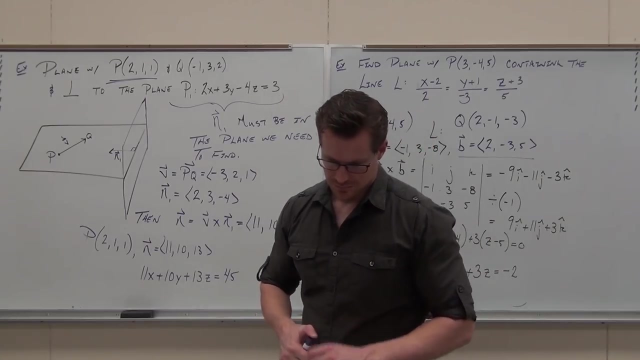 Yes, Now that you did the cross product, yeah, you do. So when I put that all together, I've got point, I've got normal, and all this yields. when I put it together That right there, That's the plane that we would just find. 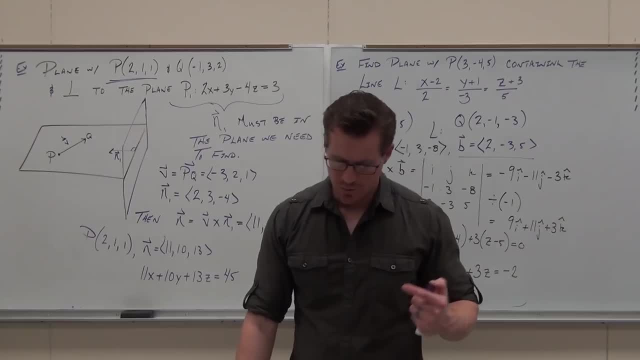 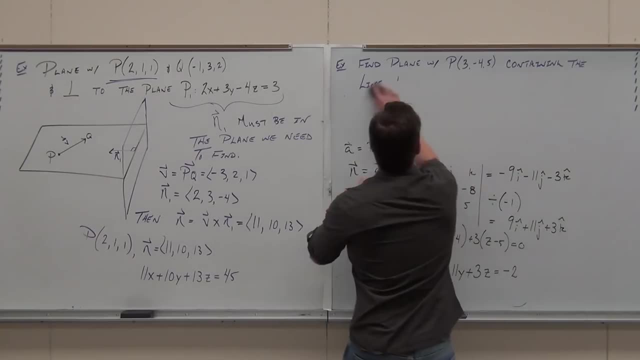 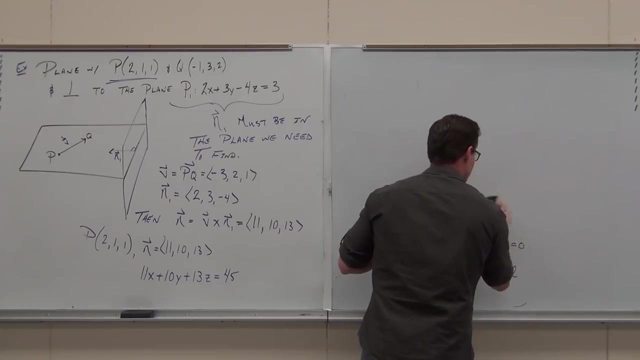 I'm going to make a couple statements. We're going to talk about two more examples and then we're going to call it good. I want you to think of this. We've already spoken of it, but I'm just going to write it down for you. 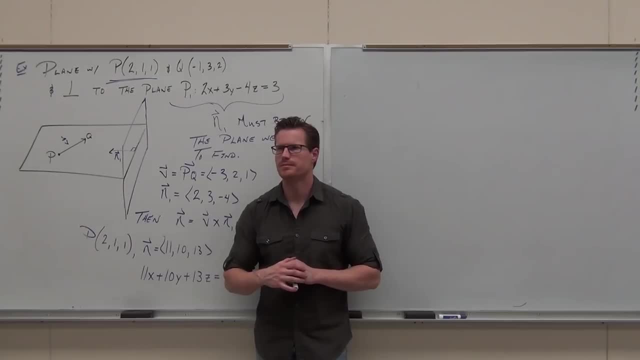 How do you know when planes are parallel, When they're Scalar multiples Planes? What do planes have? You can't just say planes scalar multiples. You're right Part of it. What has to be scalar multiples Spectrum? 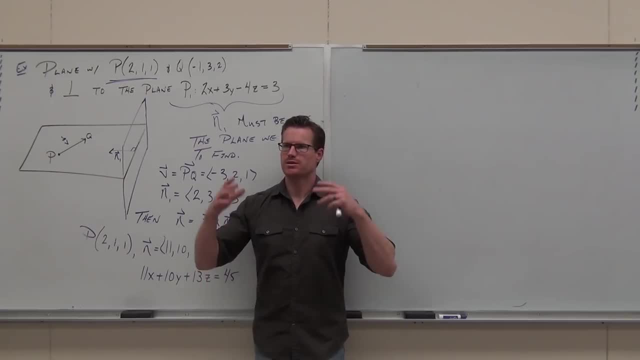 They're vectors. What type of vectors do planes have Normal? So planes are parallel. if their normals are parallel, Does that make sense to you? Planes are perpendicular. if their normals are perpendicular, That's a cool thought. Planes are parallel. 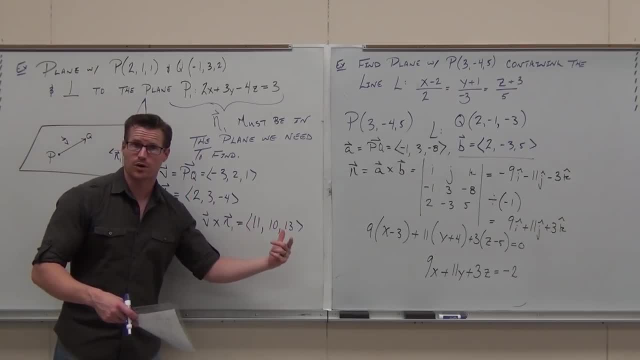 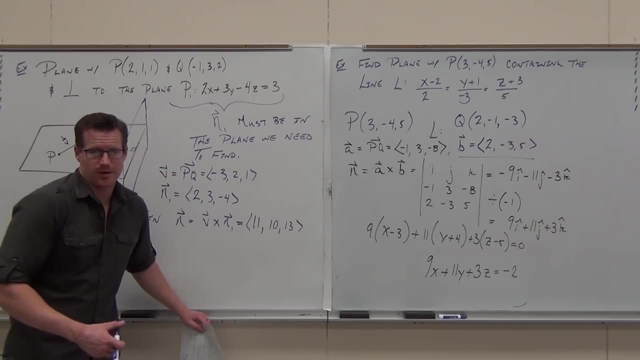 in this plane you're trying to find. Therefore, my cross product is actually going to work for us. This is my normal vector. Now do I have a point? Yes, Which point do you want to use? It doesn't matter. 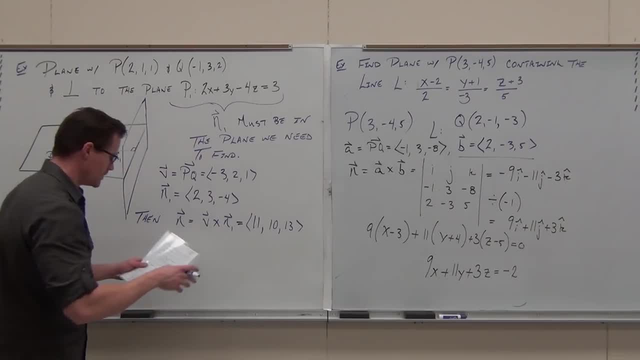 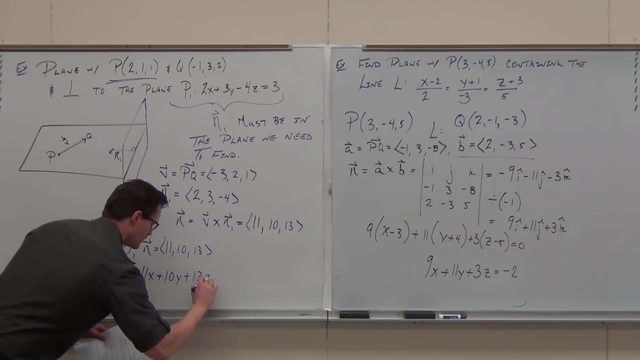 Do you have a normal vector? Yes, Now that you did the cross product, yeah, you do. So when I put that all together, I've got point, I've got normal, And all this yields. when I put it together, That right there. 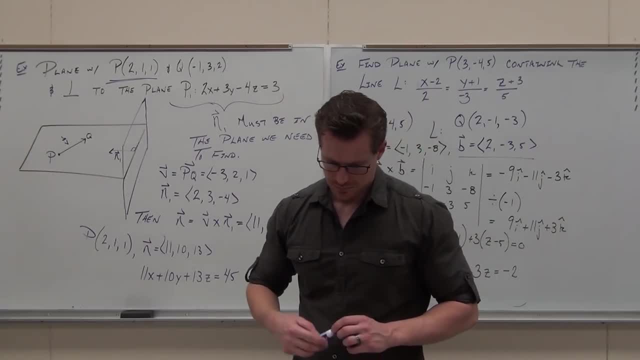 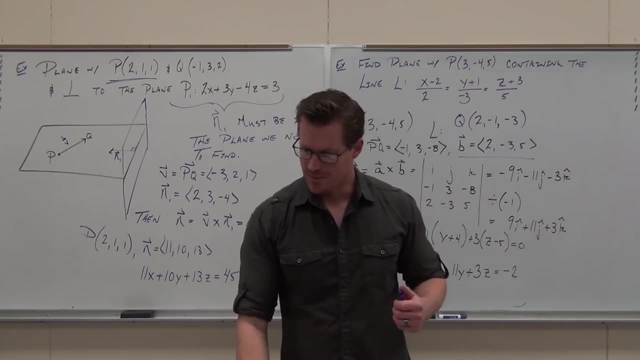 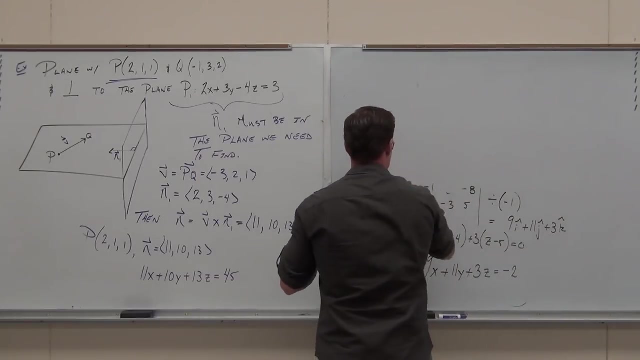 That's the plane that we would just find, that we'd find. I'm going to make a couple statements, We're going to talk about two more examples and then we're going to call it good. I want you to think of this. 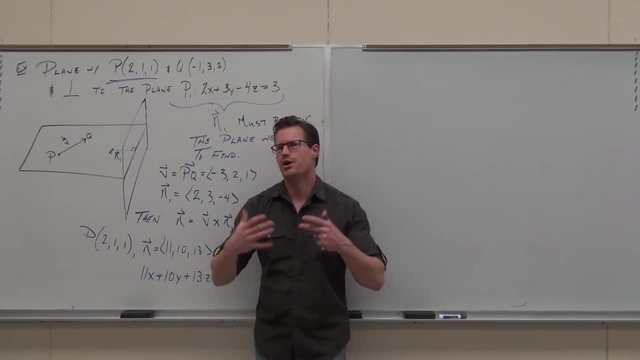 We've already spoken of it, but I'm just going to write it down for you. How do you know when planes are parallel, When they're Scalar multiples Planes? What do planes have? You can't just say planes scalar multiples. 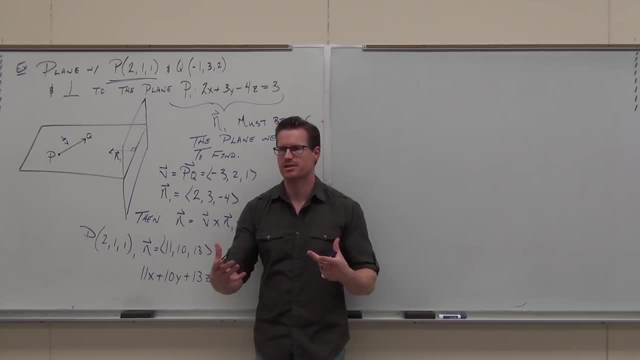 Ah, You're right part of it. What has to be scalar multiple Spectrum? They're vectors. What type of vectors do planes have? So planes are parallel, If their normals are parallel, Does that make sense to you? 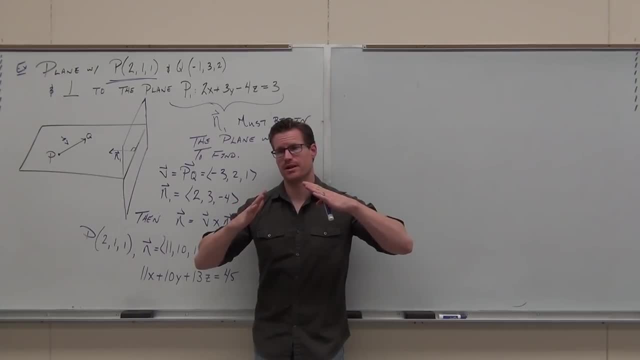 Planes are perpendicular if their normals are perpendicular. That's a cool thought. Planes are perpendicular if their normals are perpendicular. Also, this is a cool one too. It works with the angle properties from geometry. but to find the angle between your planes, 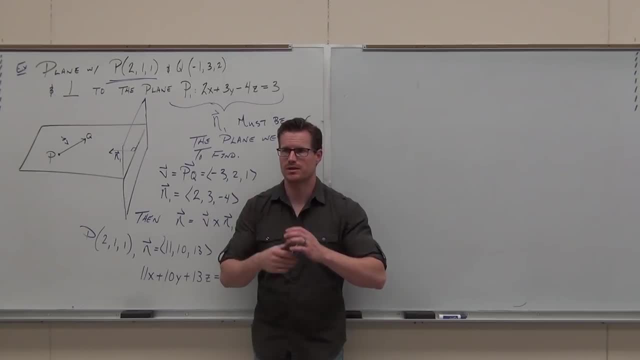 find the angle between the normals, Then you can find the angle between the planes. It's pretty cool too. So those three statements are our next notes. We're going to do Just a couple of examples and we'll be good. 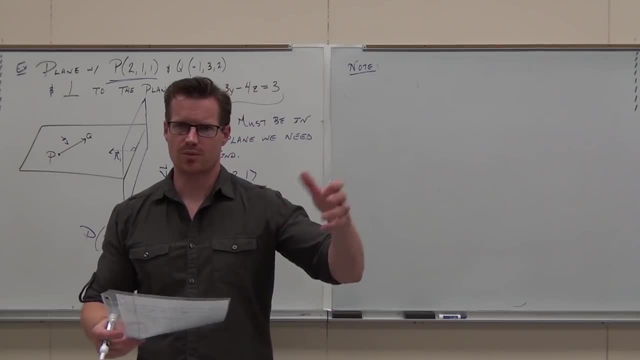 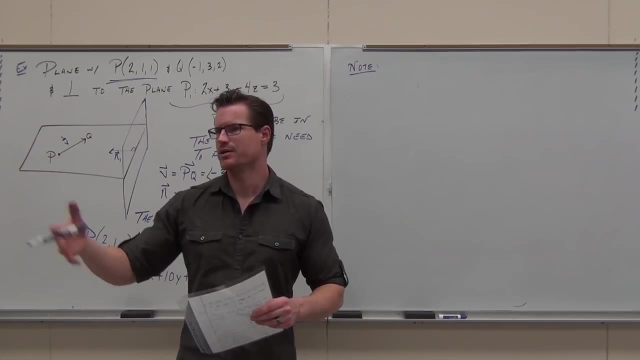 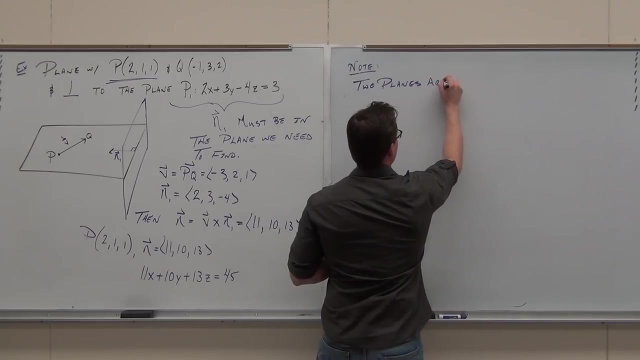 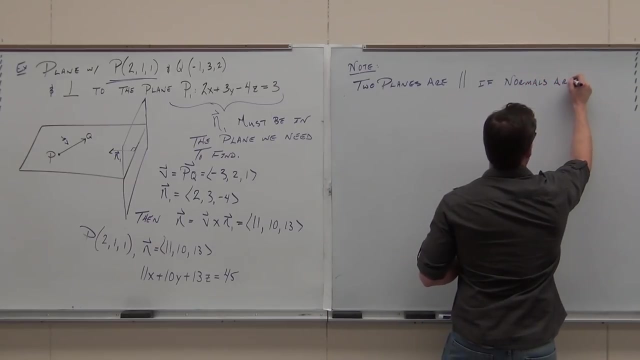 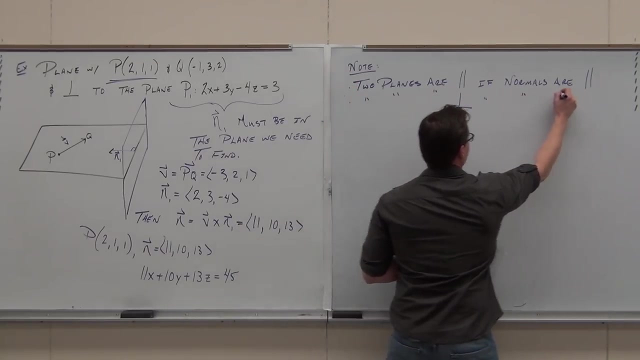 So number one: Two planes are parallel if their norms or normals are parallel. Two planes are perpendicular if their normals are perpendicular And the angle between the planes is the angle between the normals. So Two planes are perpendicular, Which means if a plane is perpendicular, 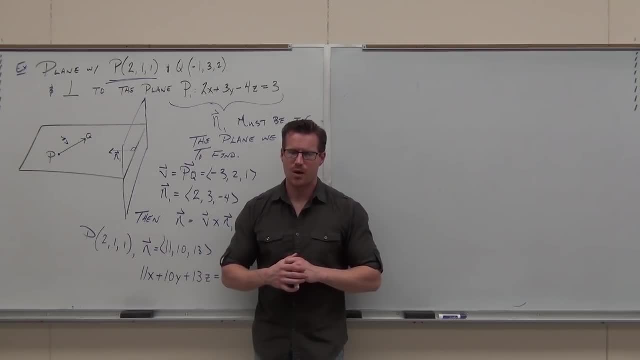 Planes are perpendicular if their normals are perpendicular Also. this is a cool one too. It works with the angle properties from geometry. but to find the angle between your planes, find the angle between the normals and you can find the angle between your planes. 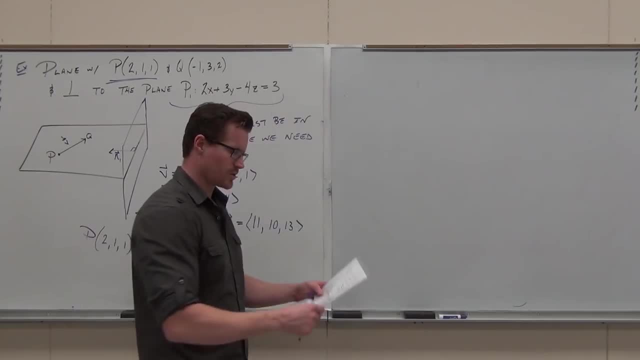 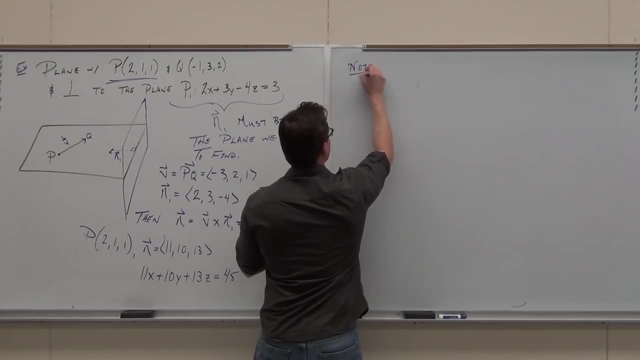 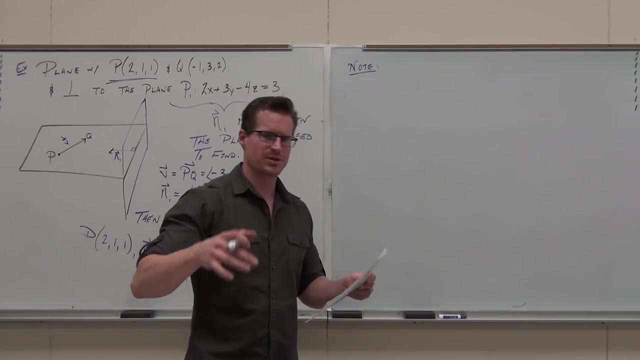 It's pretty cool too. So those three statements are our next notes. We're going to do a couple examples and be good. So number one: Two planes are parallel if their normals are parallel. Two planes are perpendicular if their normals are perpendicular. 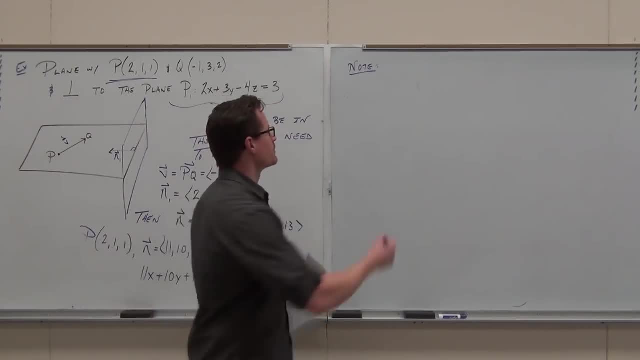 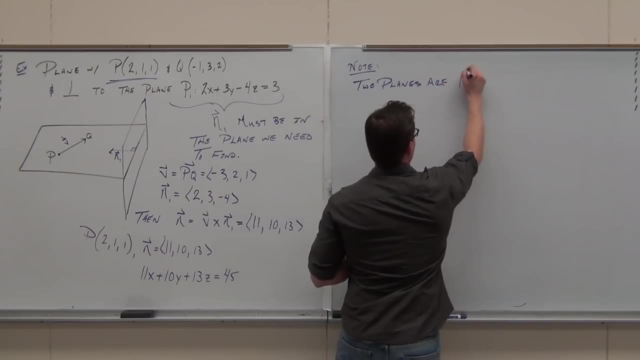 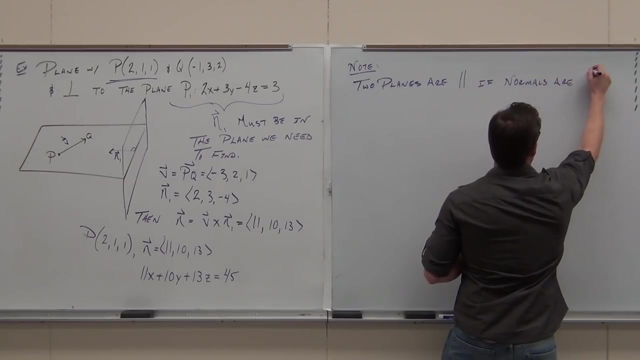 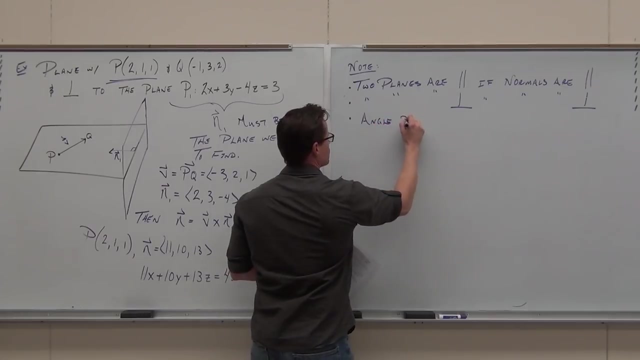 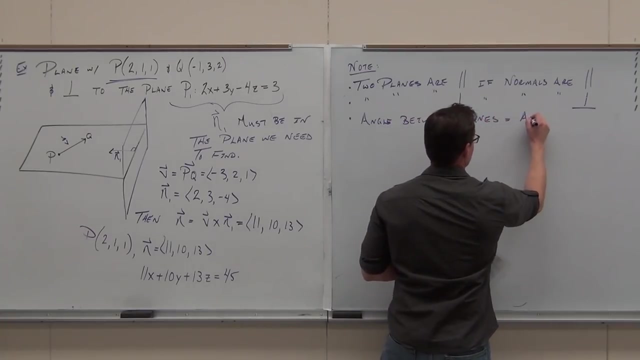 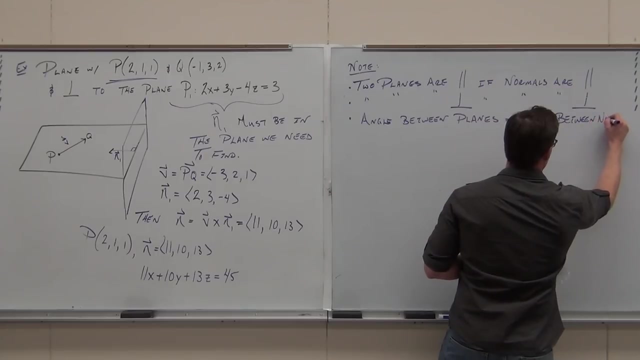 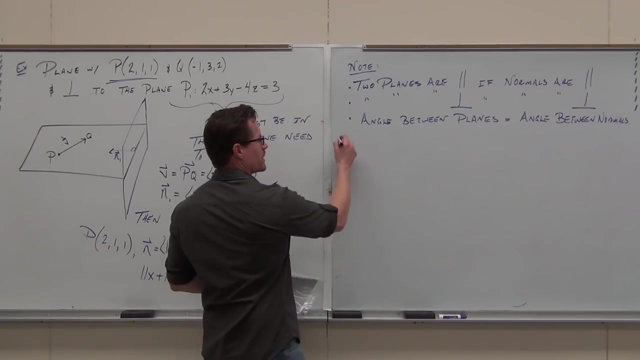 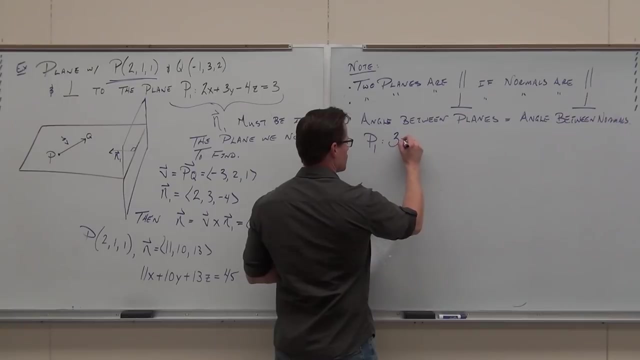 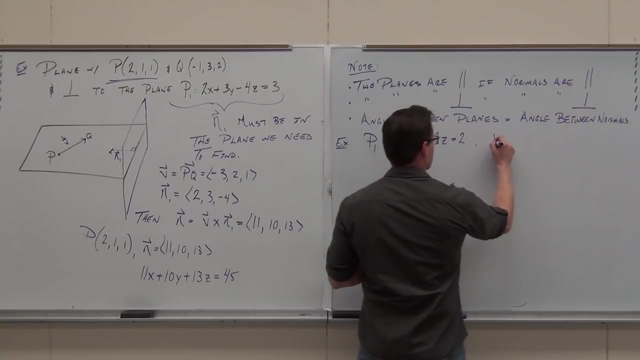 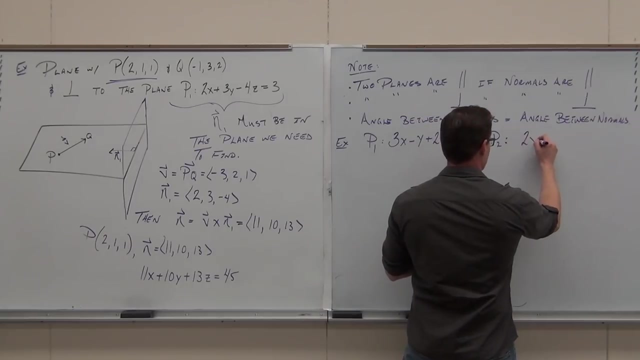 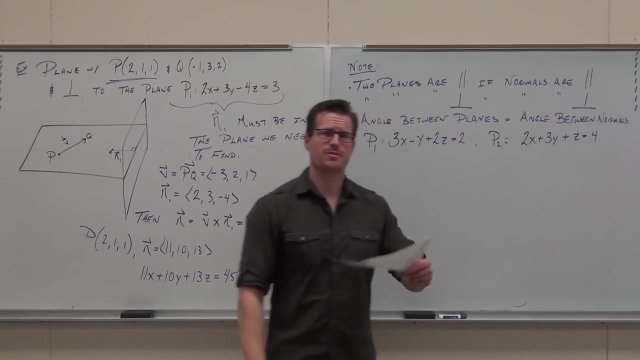 And the angle between the planes is the angle between the normals, And the angle between the planes is the angle between the normals. So let's see if we can describe the relationship here. Here's going to be my test question to you. Okay, 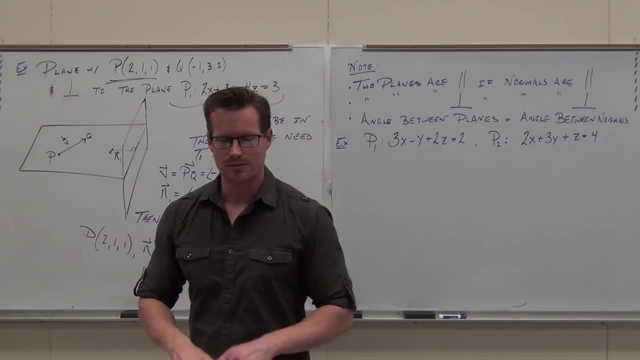 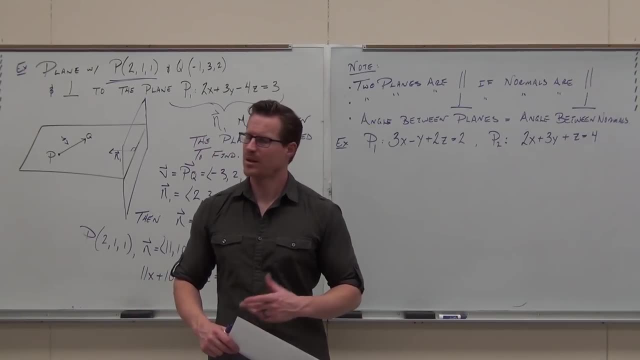 Did you catch that little hand Subtle? The test question is: describe the relationship. Are these planes parallel, perpendicular or neither? If they're neither, find the angle between them. It's pretty straightforward enough, right, if you understand the concept. 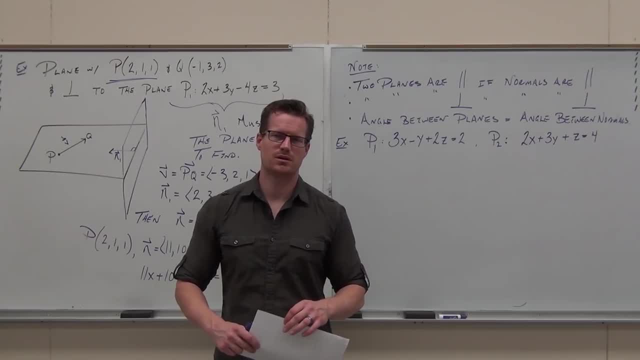 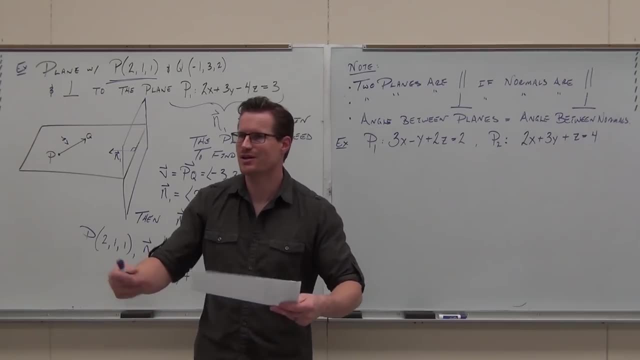 What's your first order of business in doing this problem? What would you do? See if they're parallel, See if what, See if what are parallel. By doing what? What do you need to check? Second, if they're normal. 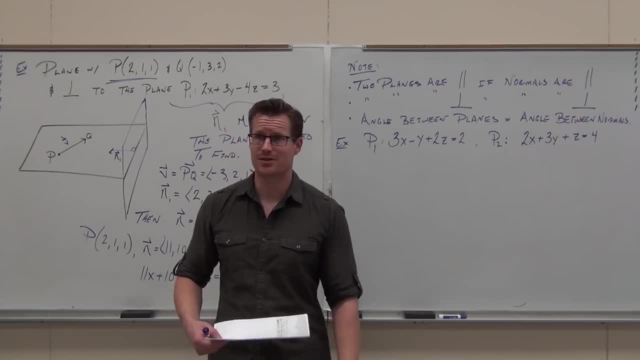 Find the normal vectors. You've got to find the vectors. You've got to at least find the vectors. It's how we're defining these planes, okay. So find the vectors. Do that right now. Find the normal vectors, And then I want you to go through it on your own. 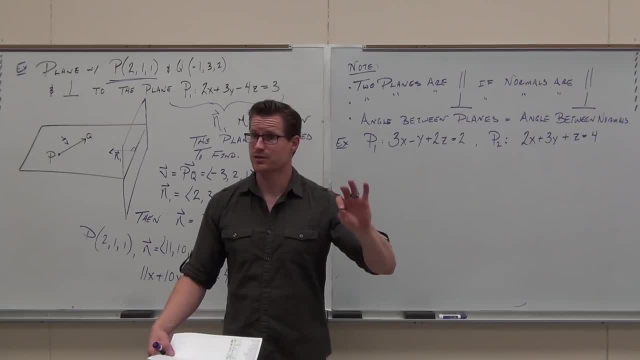 I'm going to go very fast in about a minute, okay, I want you to find the normal vectors first. Determine if they're parallel Scanner multiples. Determine if they're orthogonal Dot product And if they're neither, find the angle between them. 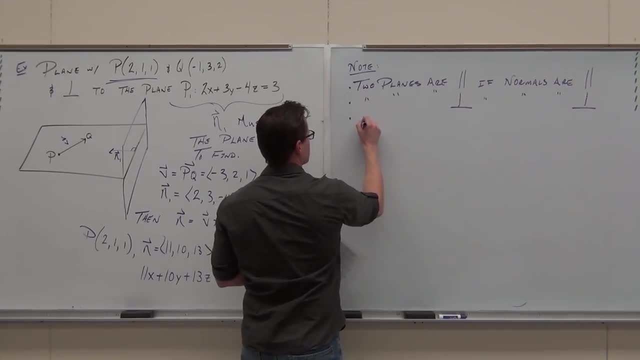 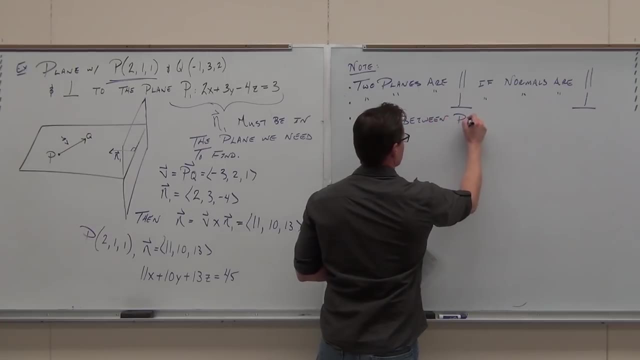 it's going to be very different. Therefore, the flux della are perpendicular to the front. If it's aскихenses are so, Well, it's a straight line here. So two planes are perpendicular if their normals are perpendicular to one another. 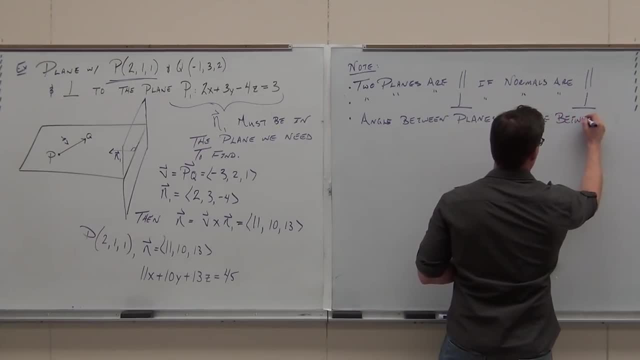 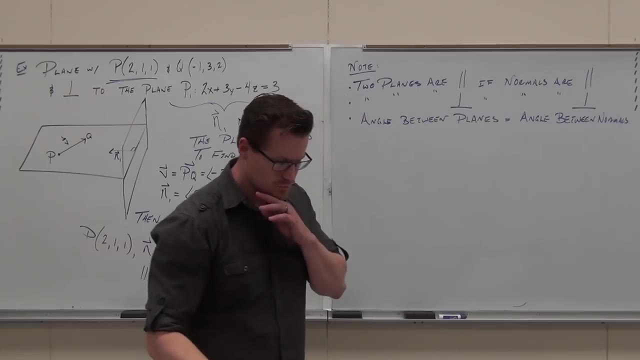 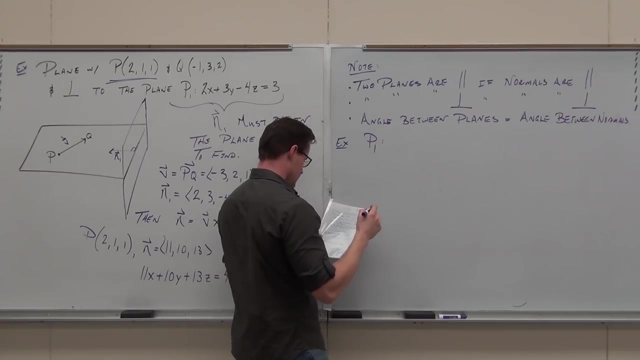 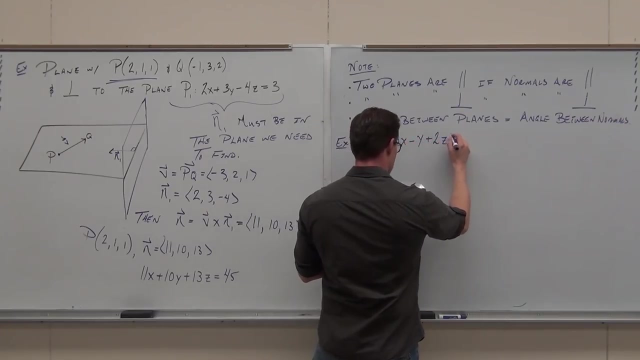 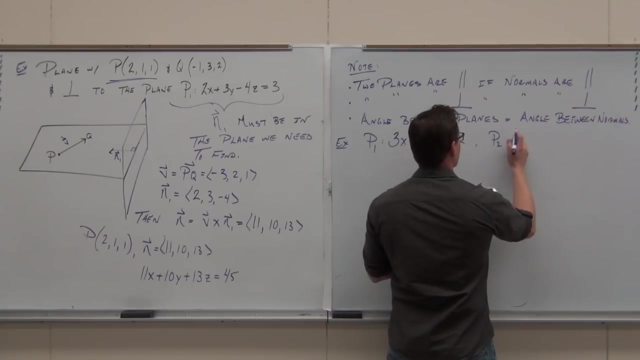 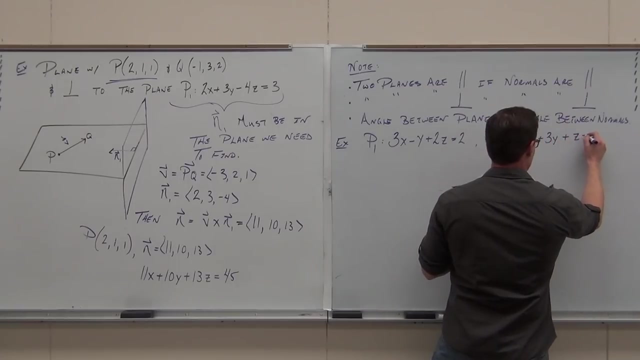 I'll see you in a few minutes. Thanks, Thanks, I Stellen OK, Bye, bye, Bye, bye, Bye, bye. So let's see if we can describe the relationship here. Here's going to be my test question to you: Did you catch that little hand? 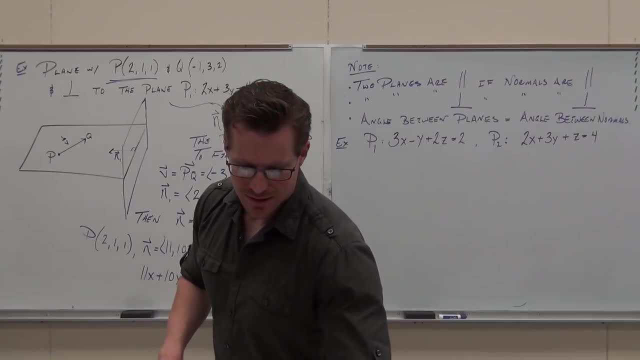 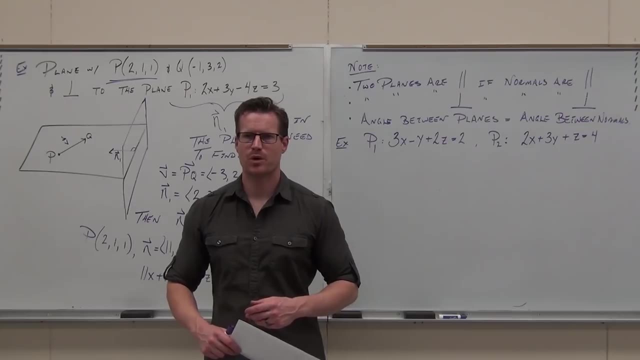 Subtle. The test question is: describe the relationship. Are these planes parallel, perpendicular or neither? If they're, neither, find the angle between them. It's pretty straightforward enough, right? if you understand the concept, What's your favorite? 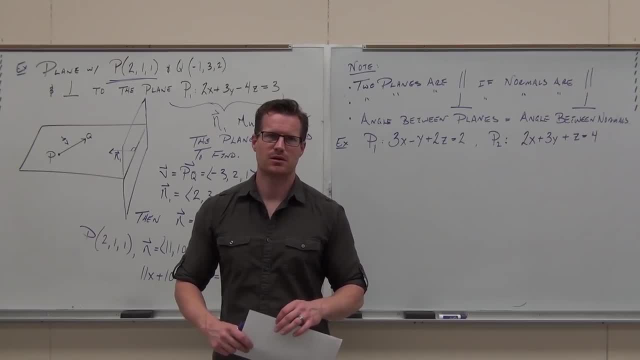 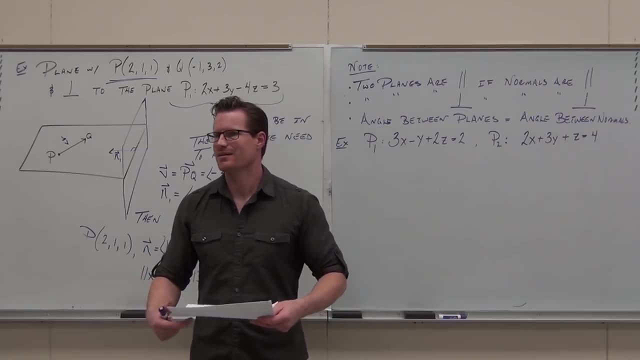 What's the first order of business in doing this problem? What would you do? See if they're parallel, See if what, See if what are parallel. By doing what? What do you need to check? Second, if they're normal. 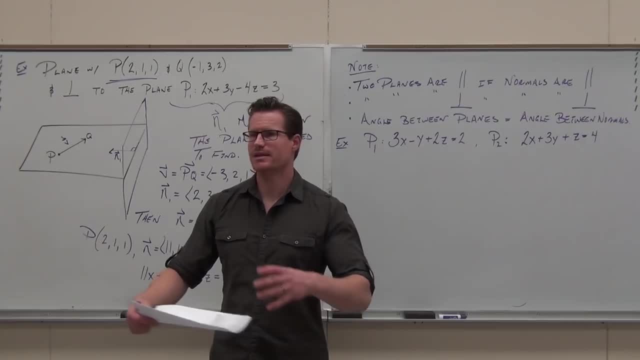 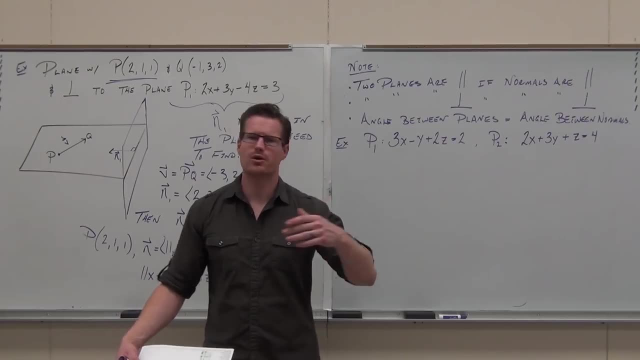 You've got to find the vectors. You've got to at least find the vectors. That's how we're defining these planes, okay. So find the vectors. Do that right now. Find the normal vectors, And then I want you to go through it on your own. 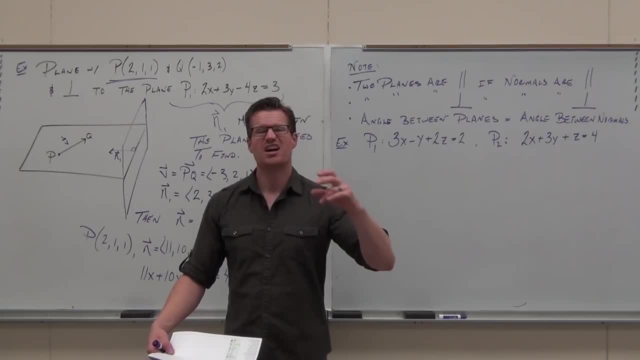 I'm going to go very fast in about a minute. okay, I want you to find the normal vectors first. Determine if they're parallel. Scanner multiplication: I can filter through all of the numbers. Determine if they're orthogonal. Dot product. 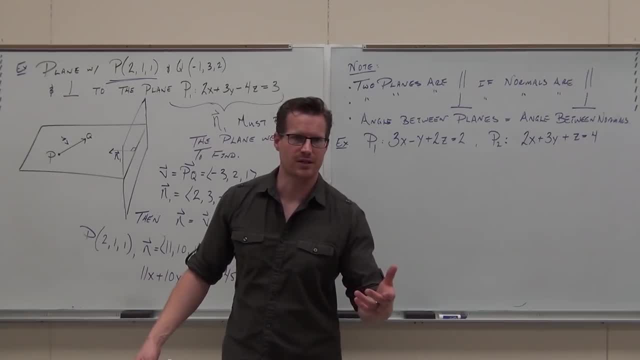 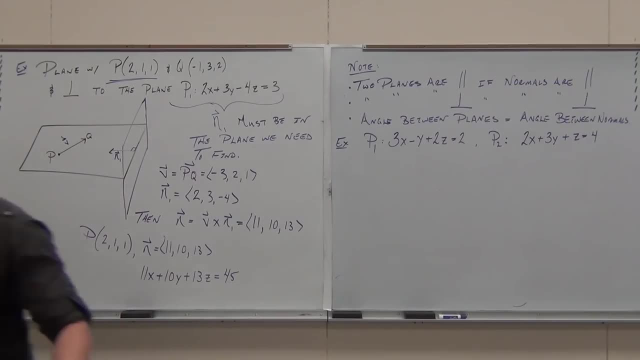 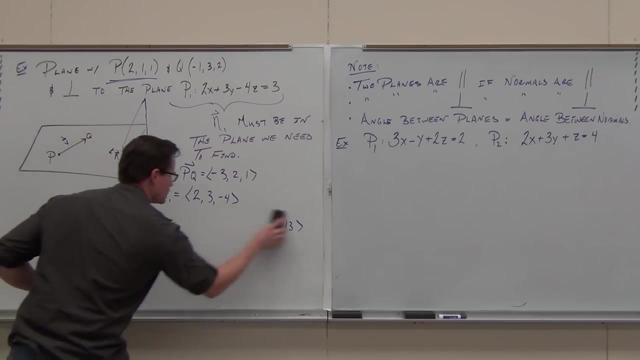 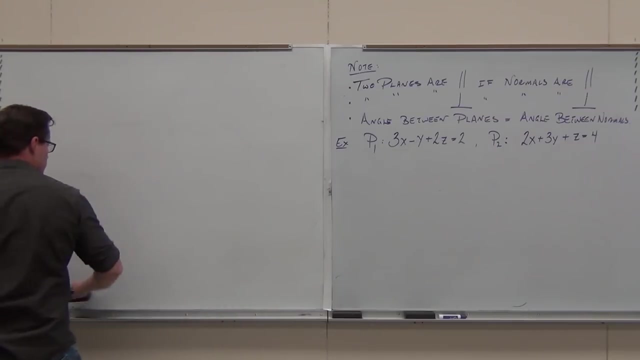 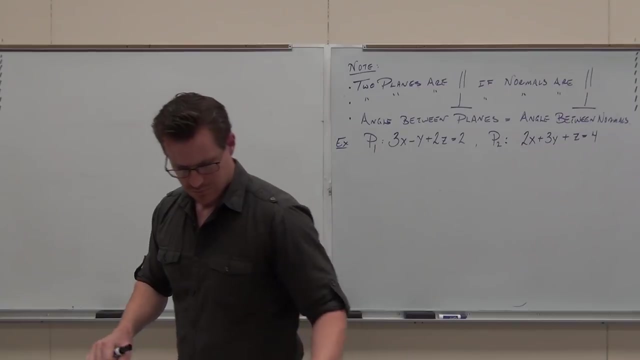 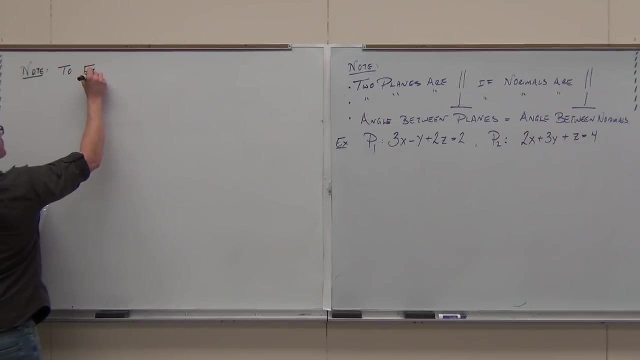 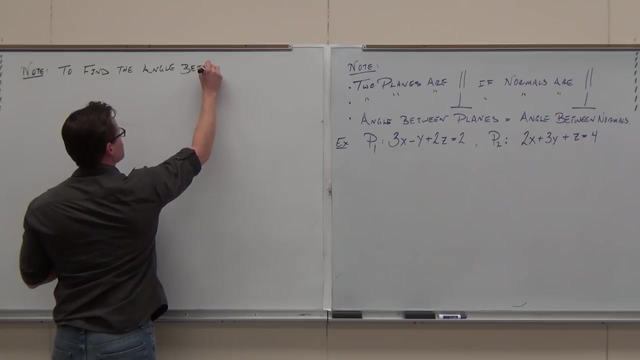 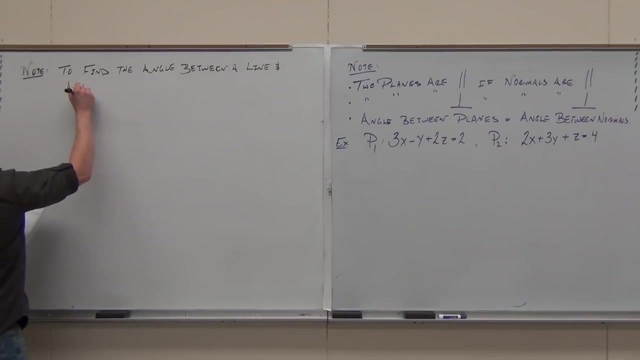 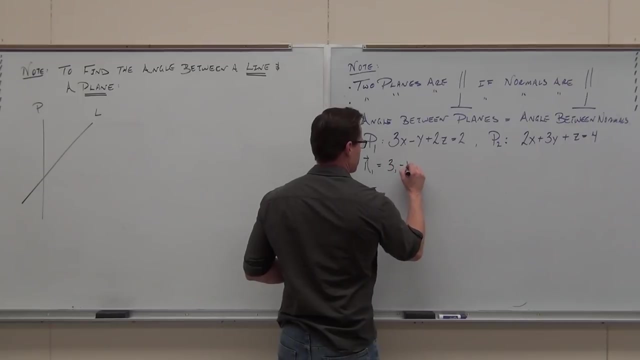 And if they're neither, find the angle between them. If they're perpendicular, that kinds of thing is 90 degrees. If they're parallel, angle is 0. Thank you, Thank you. I got 3, negative 1, 2.. 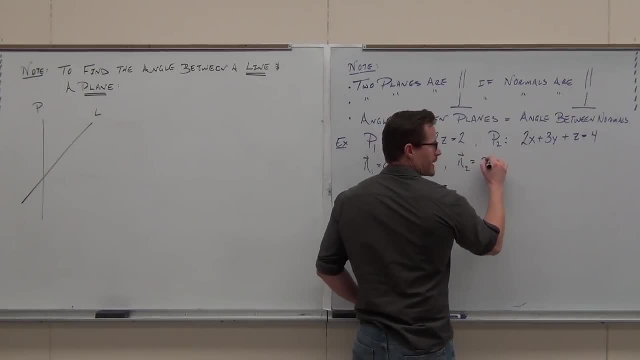 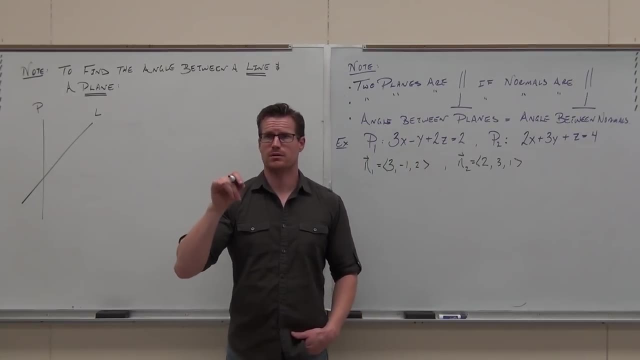 Did you get the same thing? I got Yes. I got 2,, 3, 1.. Did you get the same thing? I got Yes. Are those normals parallel? No, Are the planes parallel? No, No, because the normals are not parallel. 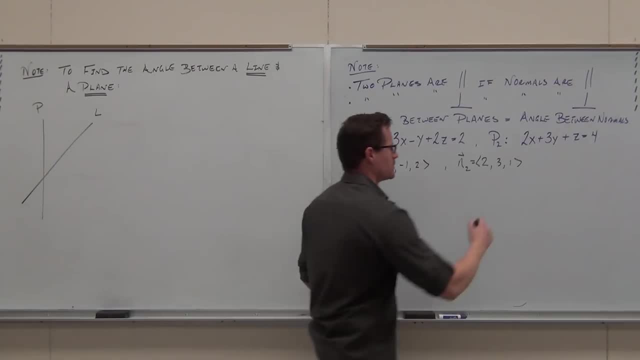 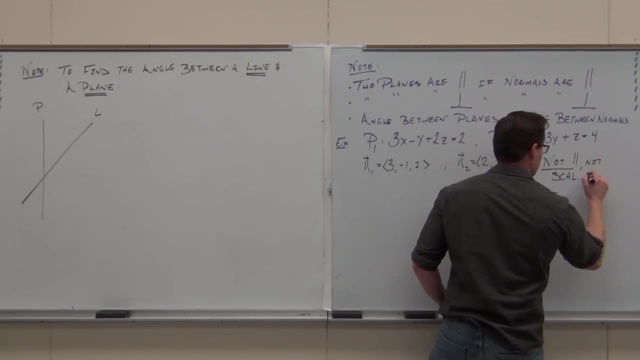 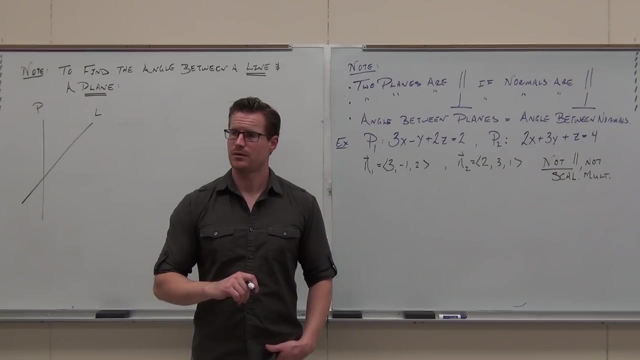 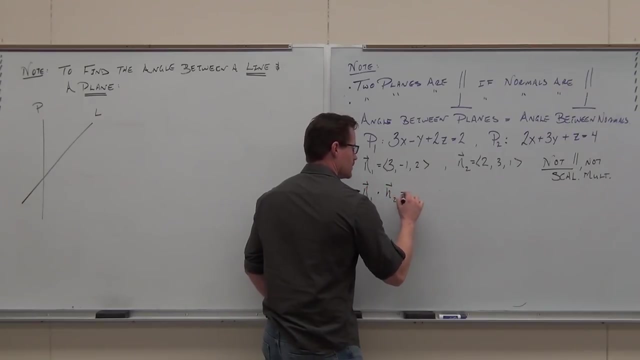 So they're not parallel. because why? How would you state that It's not a scalable problem? Are the planes perpendicular? This is what it would take to figure out. if the. do you remember the dot product? If the dot product is what number, then we have perpendicular. 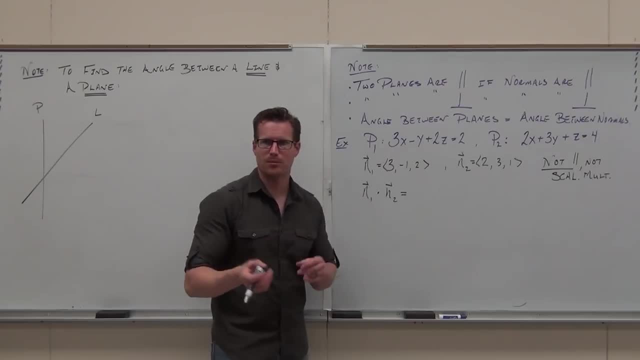 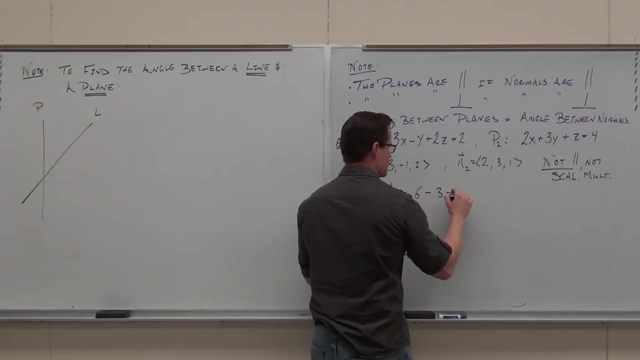 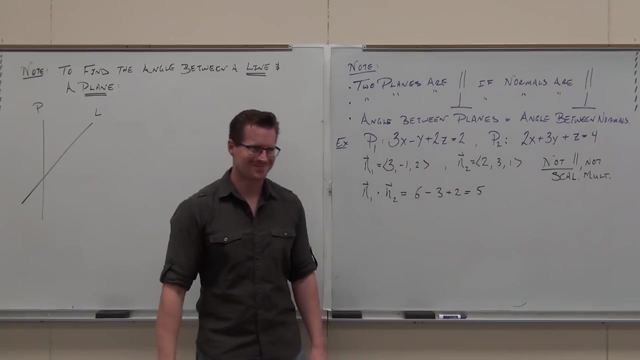 Perfect, that's how you check, So let's, we'll do the. sorry about that. If we do the dot product and it's not 0, then we have not perpendicular, So we'll try it, Not 0.. Did you get not 0?? 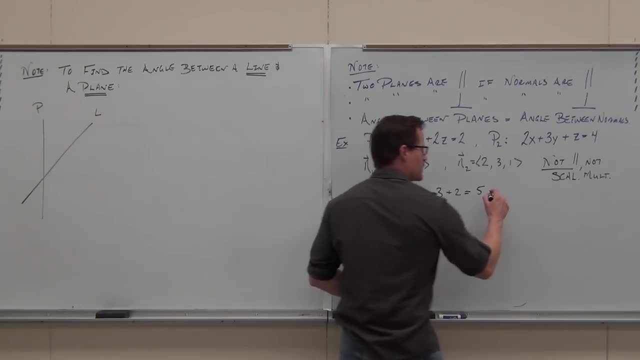 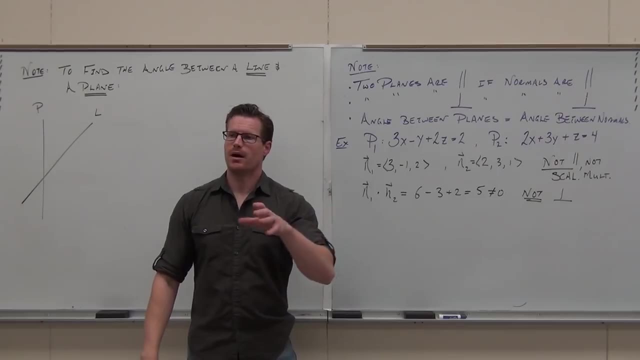 Did you get 5?? It's important. Here's why it's important. So not 0, not perpendicular, But on the, on the test, on your homework, in in real life, you go okay, well look. 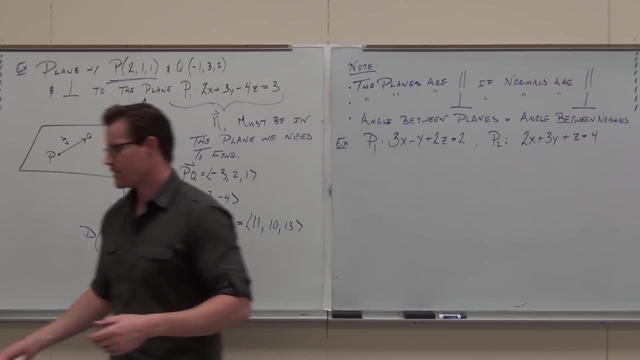 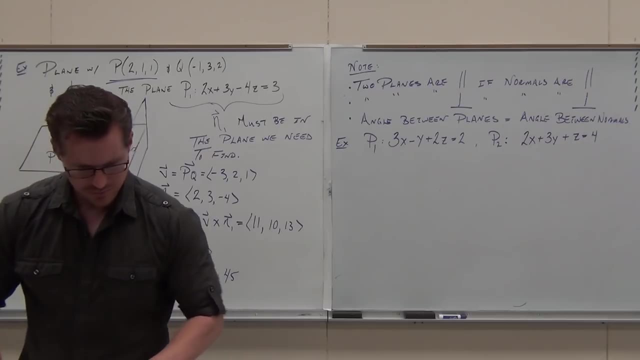 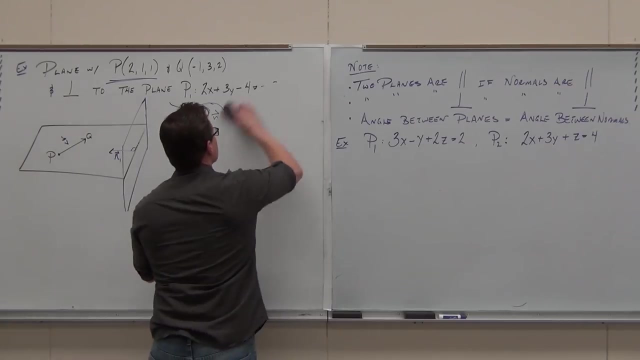 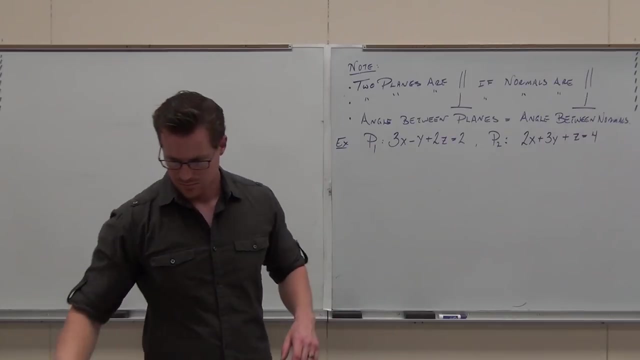 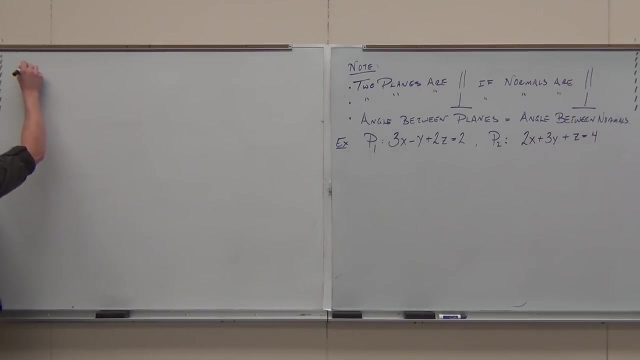 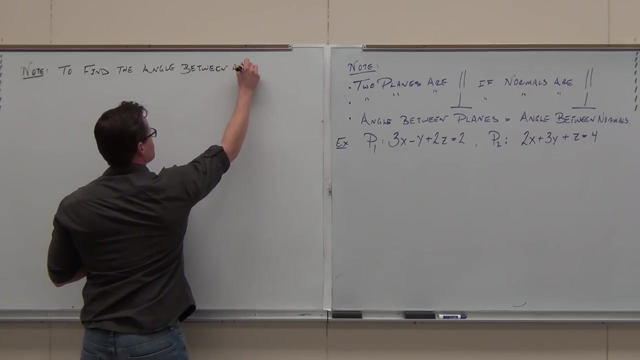 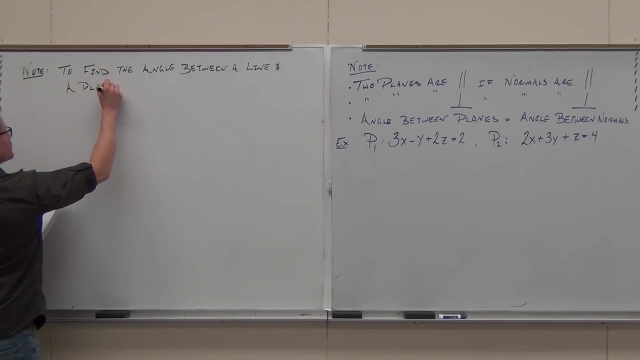 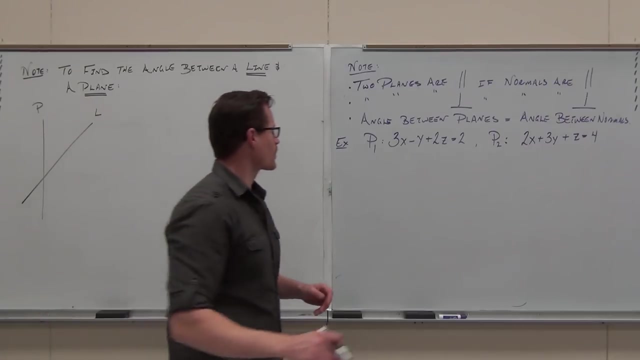 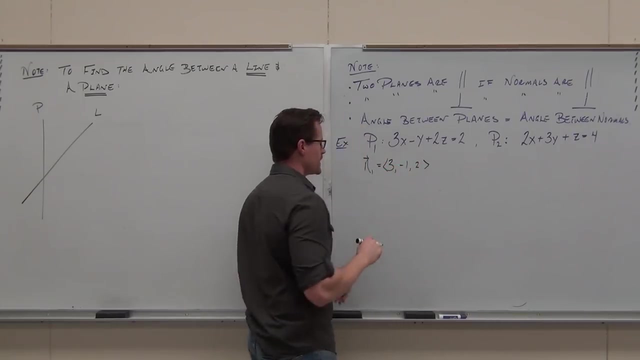 If they're perpendicular, obviously the angle is 90 degrees. If they're parallel, the angle is zero. I got 3, negative 1, 2.. Did you get the same thing I got. 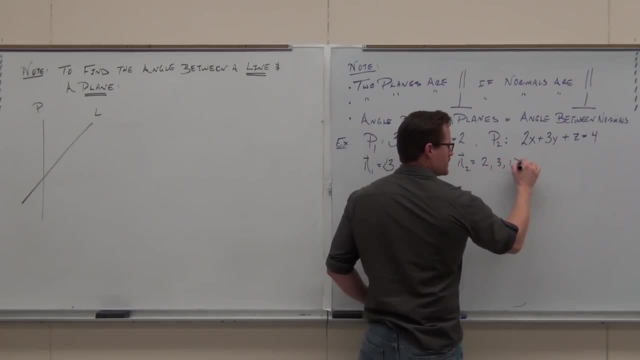 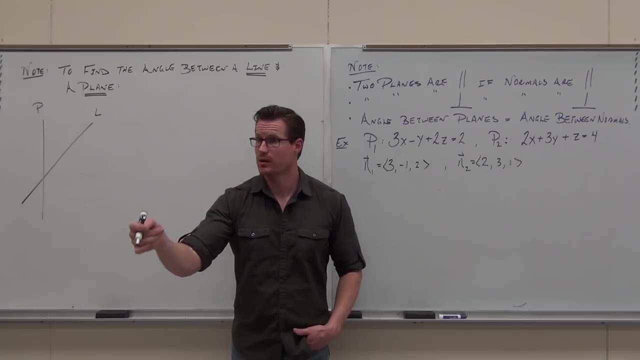 Yes, I got 2,, 3, 1.. Did you get the same thing I got? Are those normals parallel? No, Are the planes parallel? No, No, because the normals are not parallel. So they're not parallel, because why? 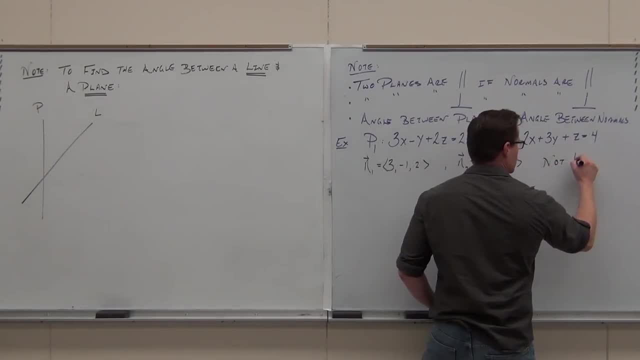 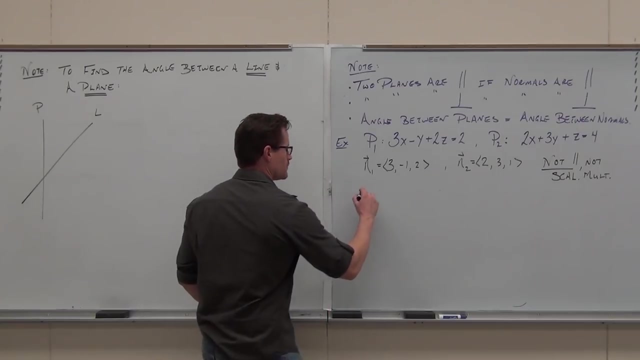 How would you state that? Are the planes perpendicular? No, This is what it would take to figure out. if the, do you remember the dot product? If the dot product is what number, then we have perpendicular. Perfect, that's how you check. 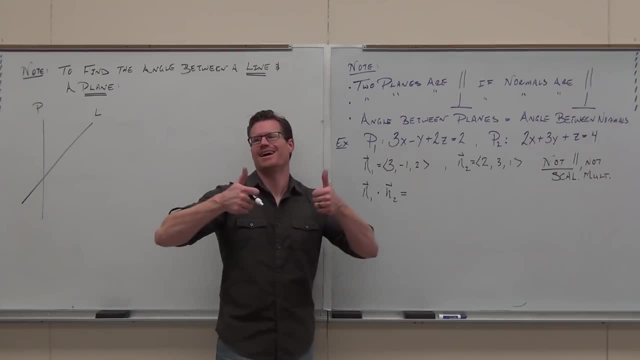 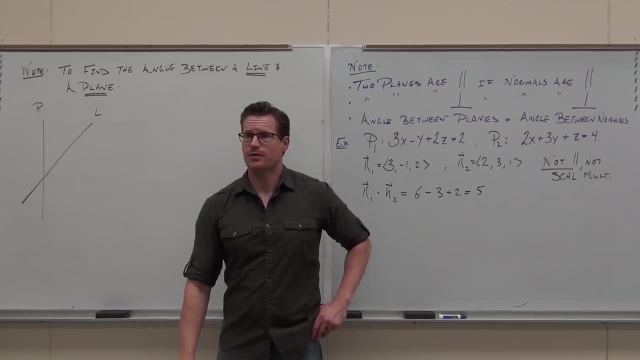 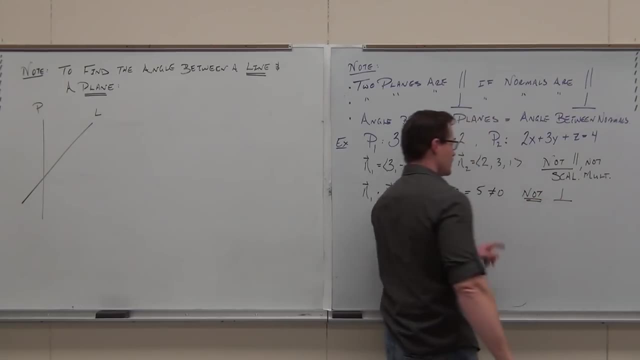 Did you get not 0?? Did you get 5?? Yes, It's important. Here's why it's important. So, not 0, not perpendicular, But on the on the test, on your homework in real life, you go okay. well, look. 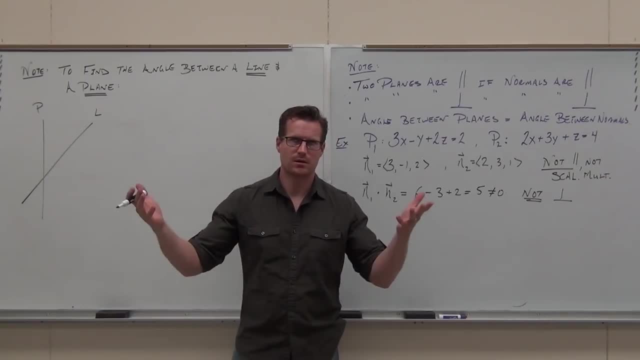 if they're not parallel and they're not perpendicular? what's the angle between them? Can you figure it out? Recall that the cosine of the angle Is that the dot product divided by the magnitudes. Does it make sense on what I'm talking about? 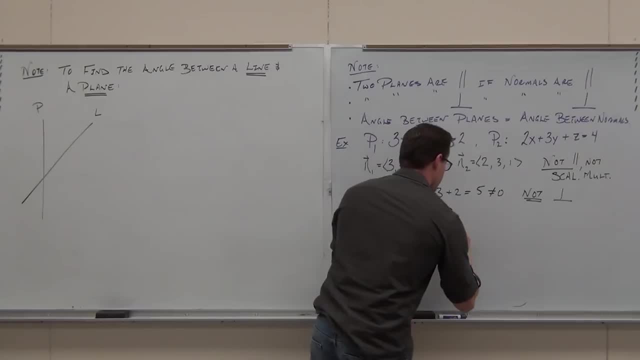 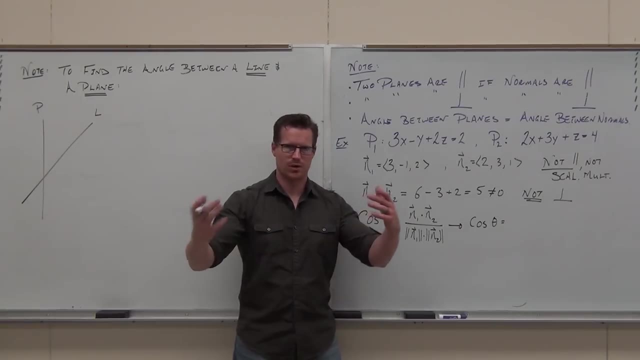 You've seen it before. You've seen it a long long time ago. Would you please just be smart about it. Watch, Please, watch. Watch the rundown. This can be done really, really quick. I don't want you to waste your time on your test because you don't really understand it, okay. 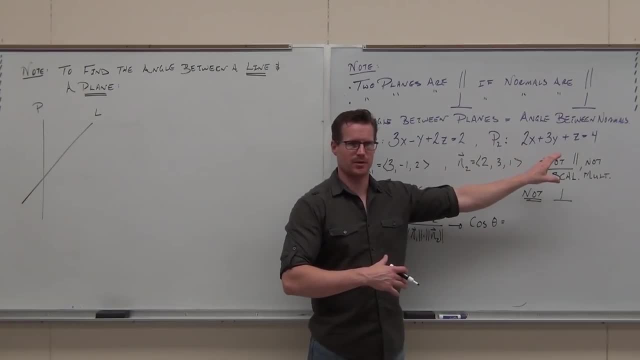 Normals, no problem. Scalar multiples? nope, they're not. they're not parallel. Dot product not 0, not perpendicular. That means that these things meet and they meet at an angle. What's the angle? Well, it's the dot product divided by the magnitudes. 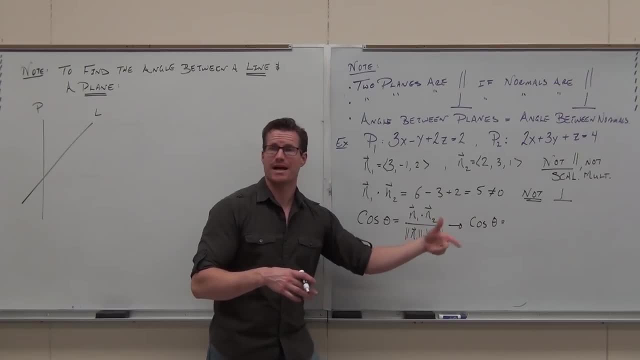 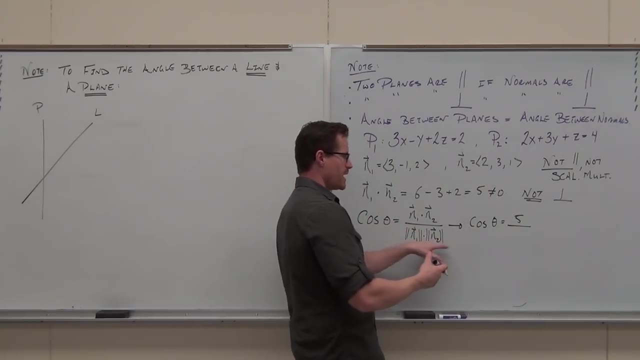 Please use that. You've already figured out the dot product. That's why we actually write it down. So this is 5.. Do you understand where the 5 is coming from? That's the dot product, And then all we've got to do is divide by the magnitudes. 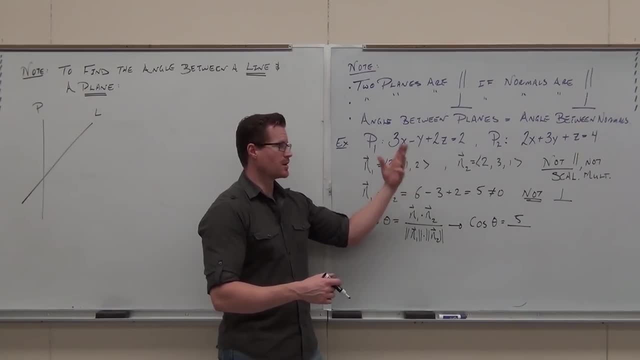 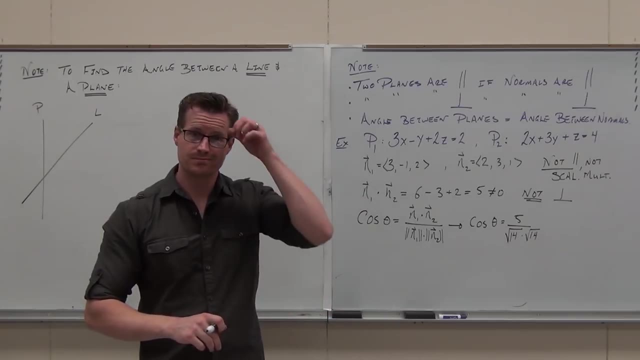 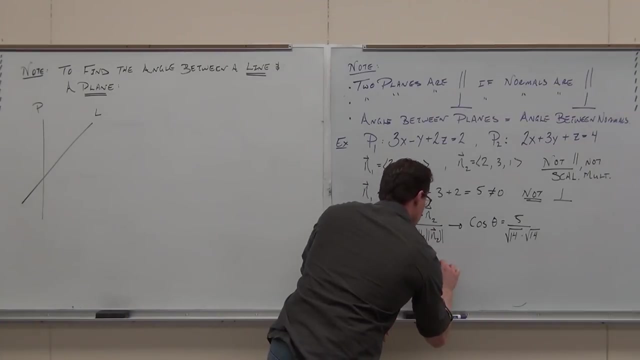 That's. that's pretty easy. This is 9,, 10, square root of 14.. Square root of 14.. Not bad. Angles cosine inverse of 5 fourteenths looks like it's about 69.1 degrees. 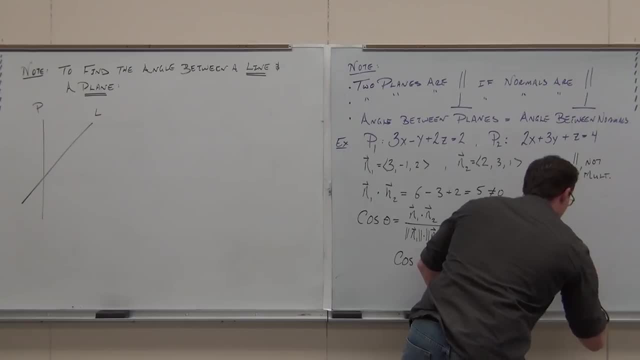 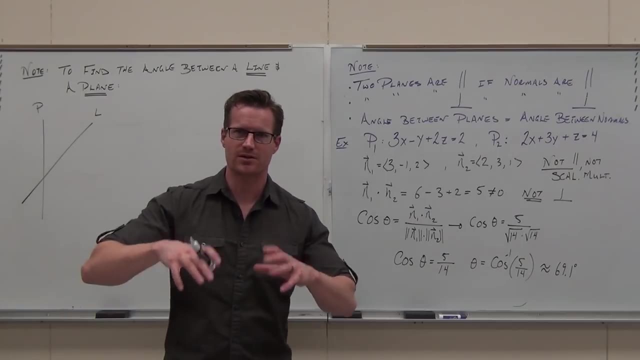 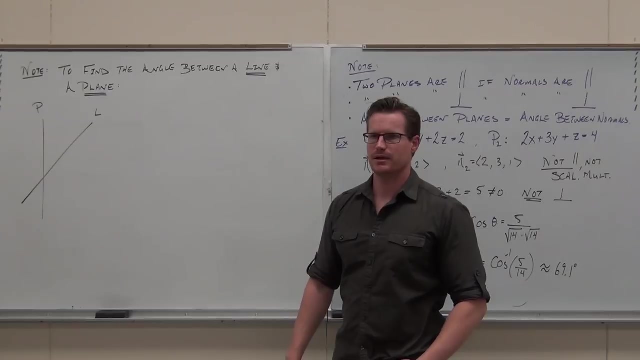 That is my favorite temperature, by the way. I love that temperature. It's so comfortable. It is seriously like right under 70 degrees. beautiful, beautiful weather. How do you find the angle between a line and a plane? I want you to think about this. 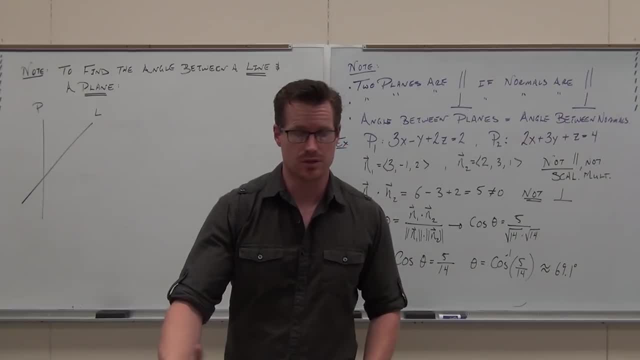 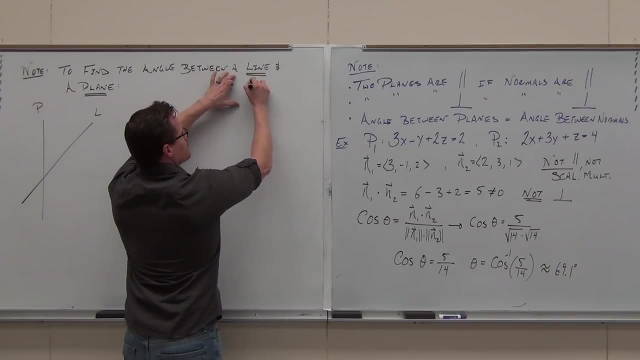 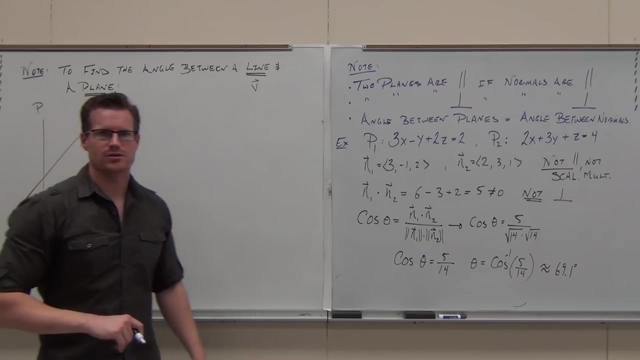 We're not going to actually do an example, but I need you, I need to show it to you. Lines always get direction vectors, no matter what Planes. get normal vectors, no matter what. That's what planes have, That's what lines have. 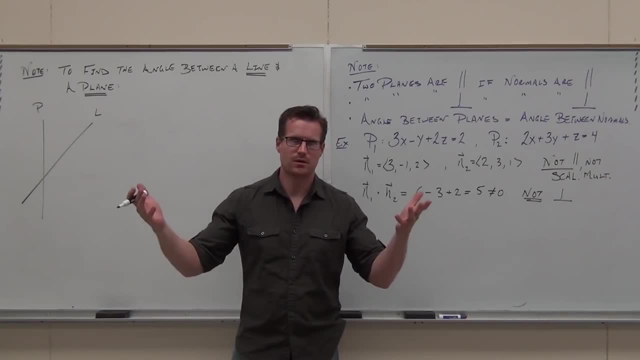 if they're not parallel and they're not perpendicular, what's the problem? What's the angle between them? Can you figure it out? Recall that the cosine of the angle Is that the dot product divided by the magnitudes. Does it make sense on what I'm talking about? 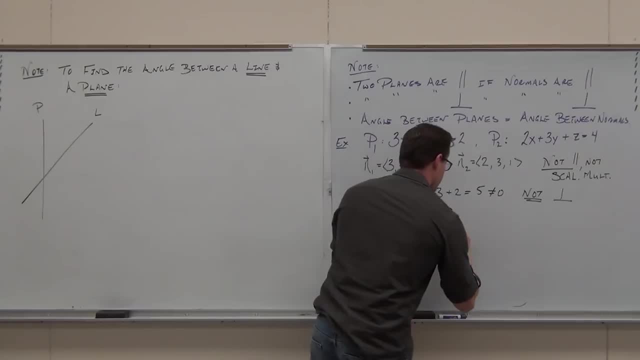 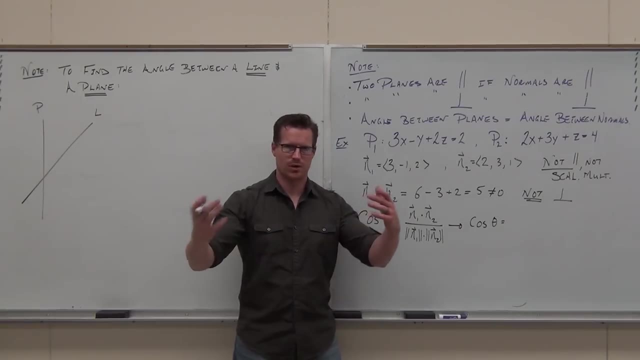 You've seen it before. You've seen it a long long time ago. Would you please just be smart about it. Watch, Please, watch, Watch the rundown. This can be done really, really quick. I don't want you to waste your time on your test. 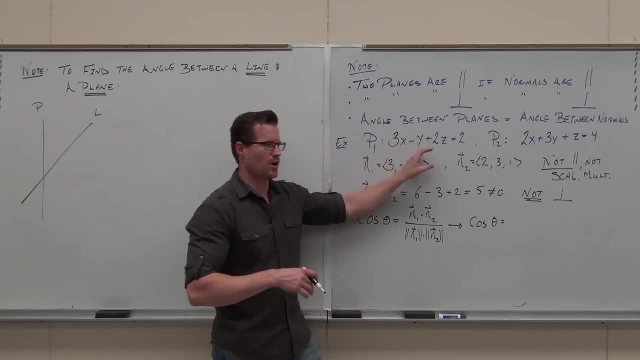 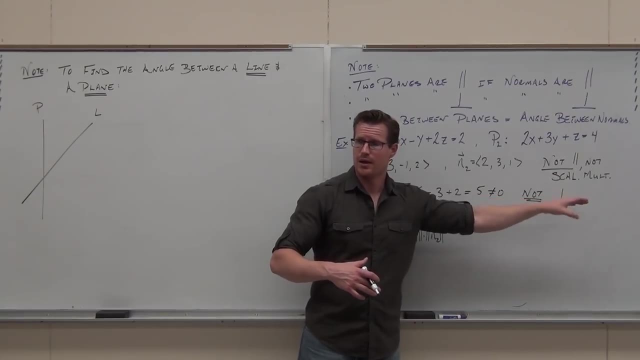 because you don't really understand it. okay, Normals, no problem. Scalar multiples: nope, they're not. they're not parallel, Dot product not 0, not perpendicular. That means that these things meet and they meet at an angle. 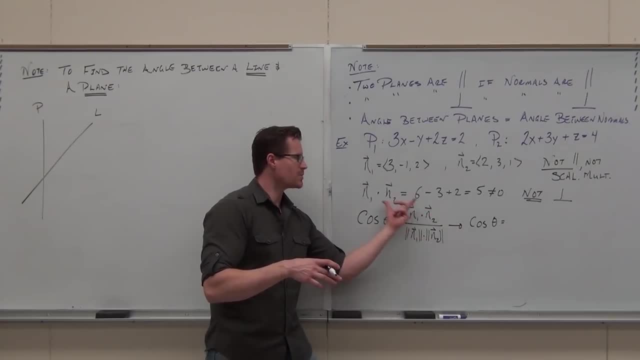 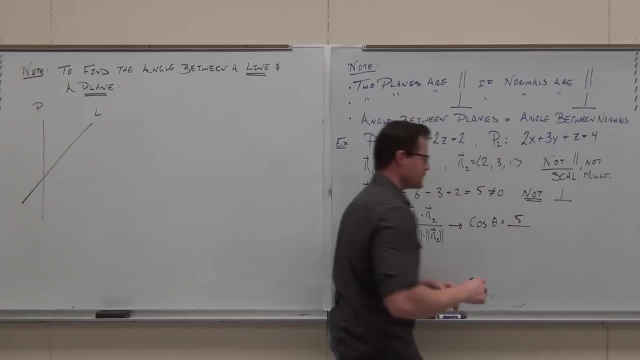 What's the angle? Well, it's the dot product divided by the magnitudes. Please use that. You've already figured out the dot product. That's why we actually write it down. So this is, This is 5.. Do you understand where the 5 is coming from? 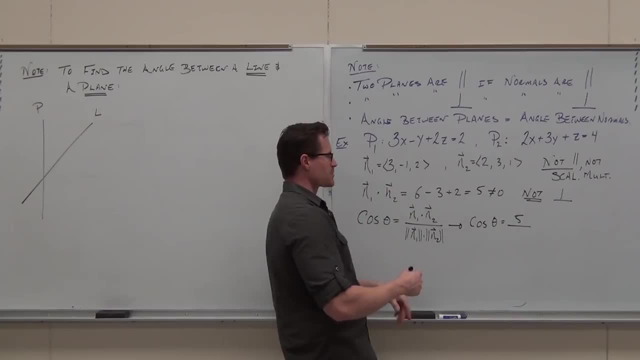 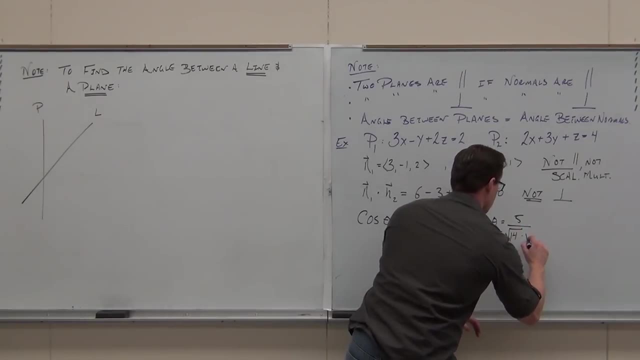 That's the dot product, And then all we've got to do is divide by the magnitudes. That's. that's pretty easy. This is 9, 10,, 12,, 13,. square root of 14.. Square root of 14.. 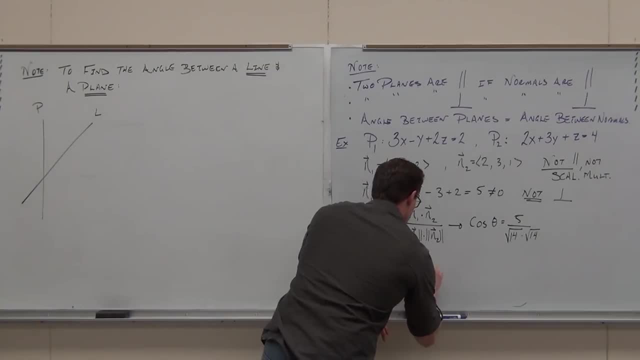 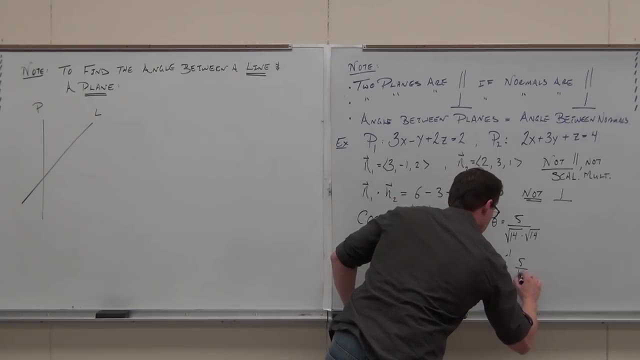 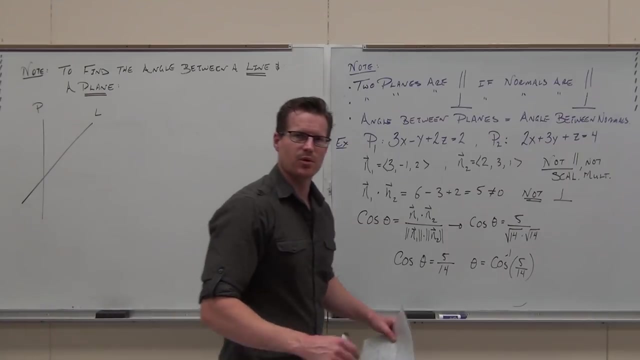 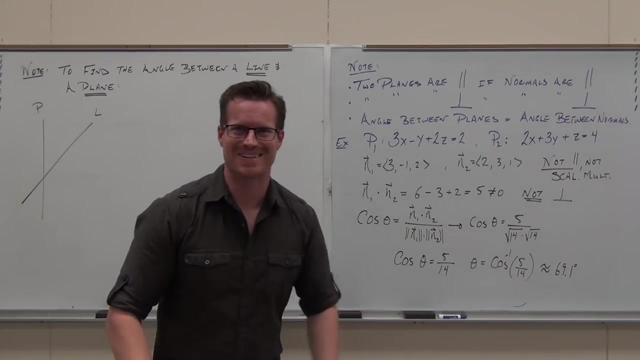 Not bad. Angles cosine inverse of 5 fourteenths Looks like it's about 69.1 degrees. That is my favorite temperature, by the way. I love that temperature. It's so comfortable, It is seriously. 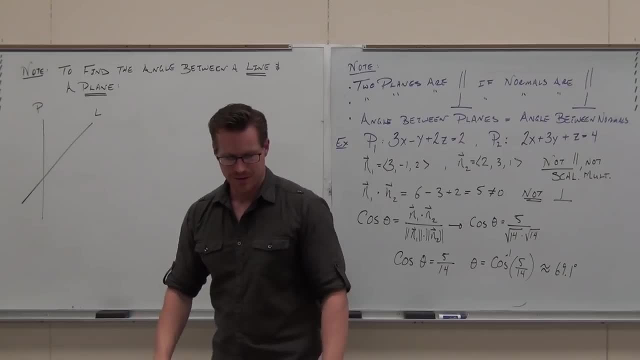 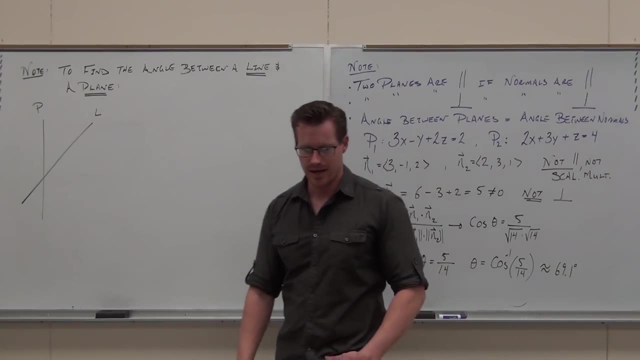 Like right under 70 degrees, beautiful, beautiful weather. How do you find the angle between a line and a plane? I want you to think about this. We're not going to actually do an example, but I need you, I need to show it to you. 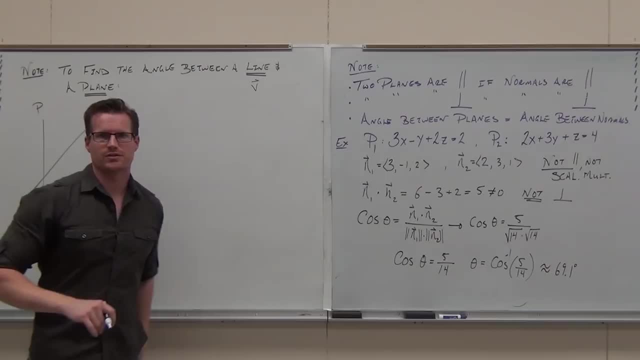 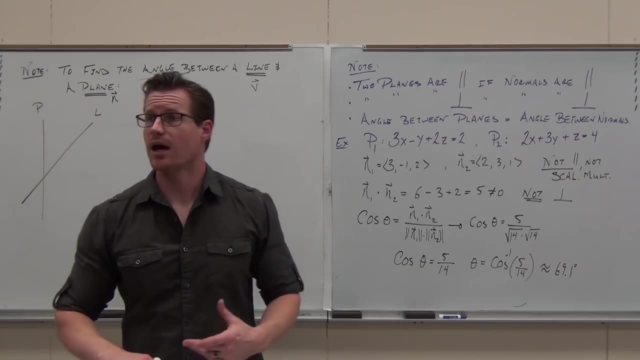 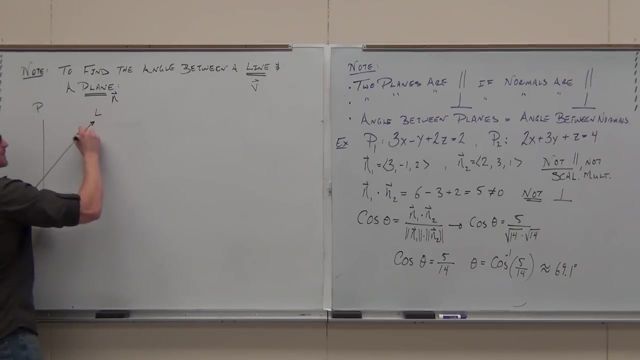 Lines always get direction vectors, no matter what Planes get normal vectors, no matter what. That's what planes have, That's what lines have. So here's the deal. Here's the deal, though. If this is my plane and that's my line, that's my vector. 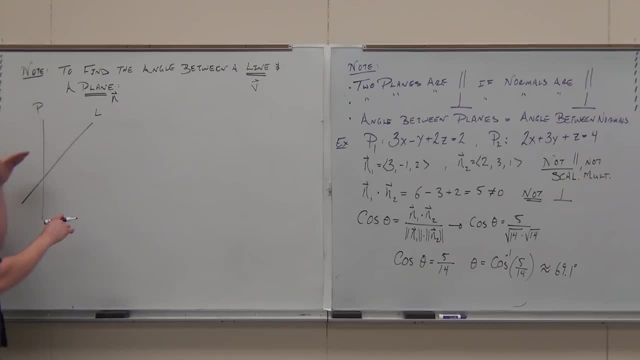 So here's the deal. Here's the deal, though, If this is my plane and that's my, that's my line, that's my vector, but the normal, the normal doesn't go this way, The normal goes this way. 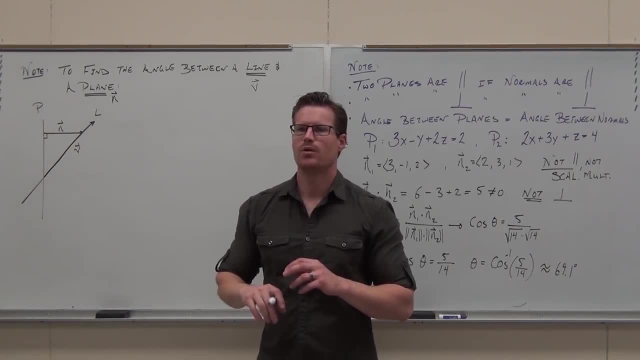 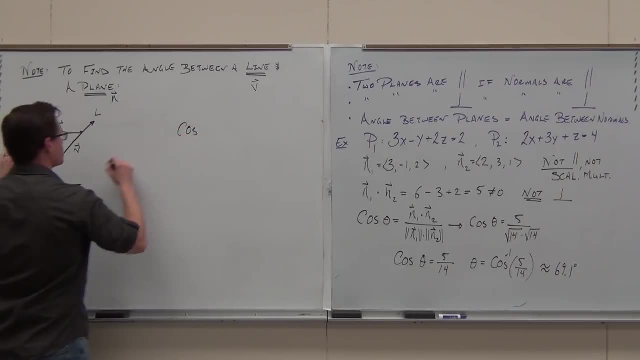 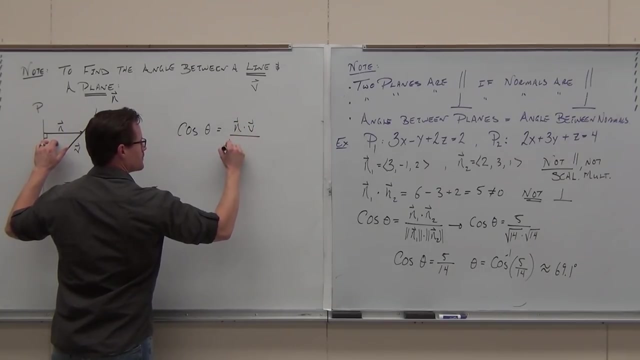 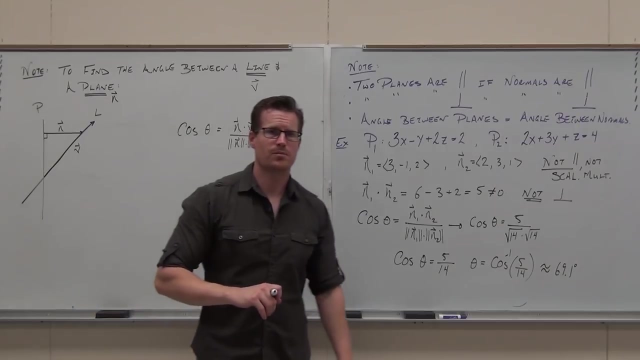 The normal goes that way. Does that make sense to you? Watch carefully so you don't miss it. If I do this, Will it give me the angle here? please watch carefully when you dot, when you do this, when you dot, product divided by the magnitudes, that gives you the cosine of the angle. 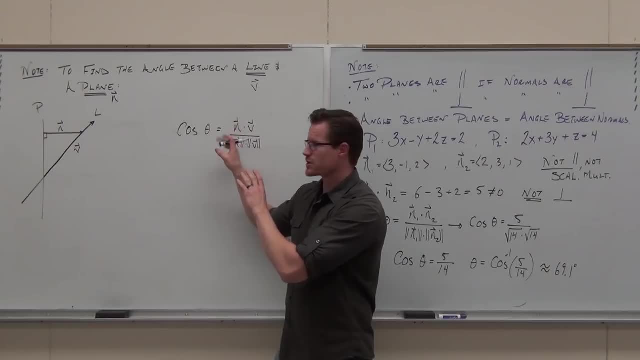 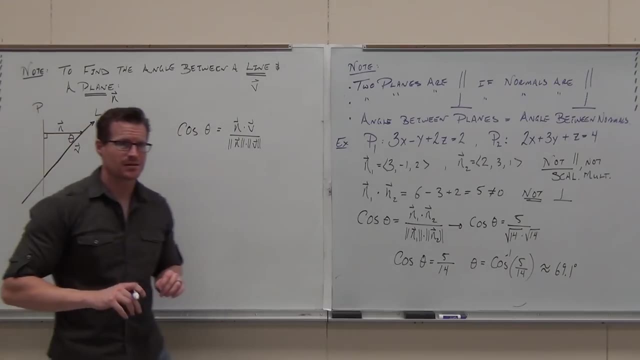 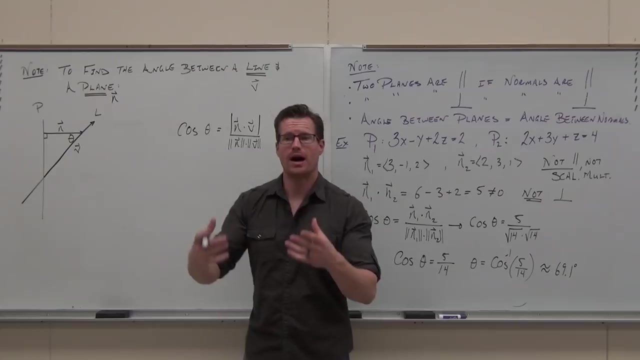 that is between these two vectors. This is not. That is between those two vectors. And in order to figure out the acute one, I do the absolute value to keep it positive, to keep that thing acute. Head nod if you're okay with that one. 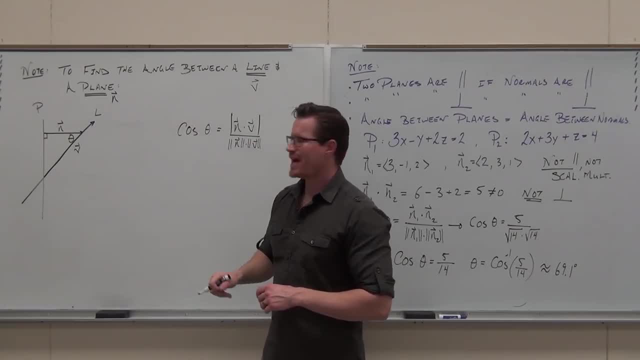 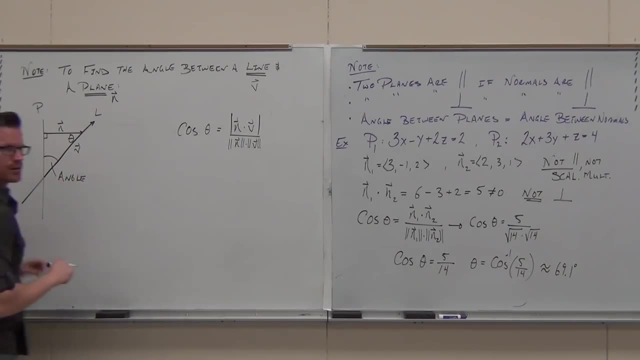 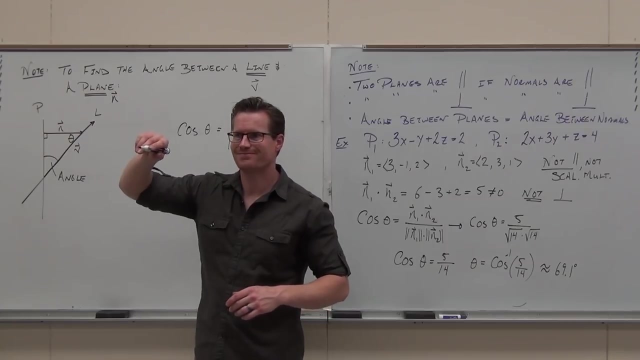 Well, wait a minute. That's not the question. The question is: how do I figure out that angle? Use your, use your geometry. Use your geometry a little bit. How much is all of my 90. 90's already taken up? 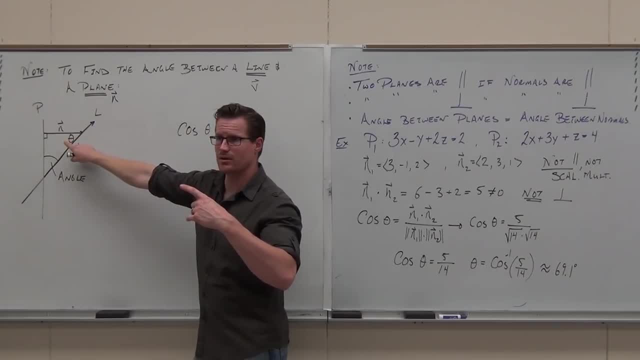 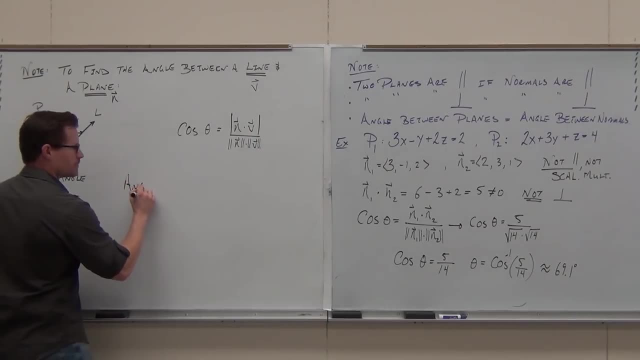 So if I do 90 minus whatever that angle is, then I will have that angle. So in our case, if you ever want to find the angle between a line and a plane, the angle is: hey, take your 90 degrees, subtract cosine inverse of this thing. 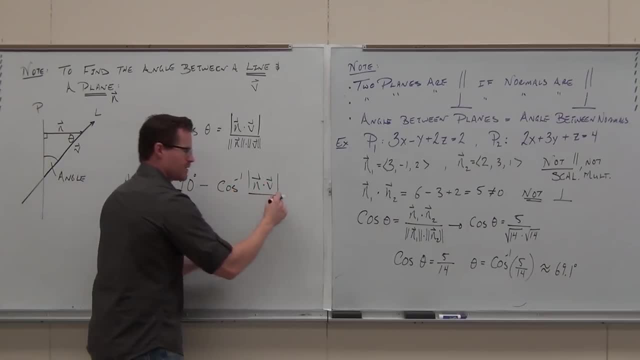 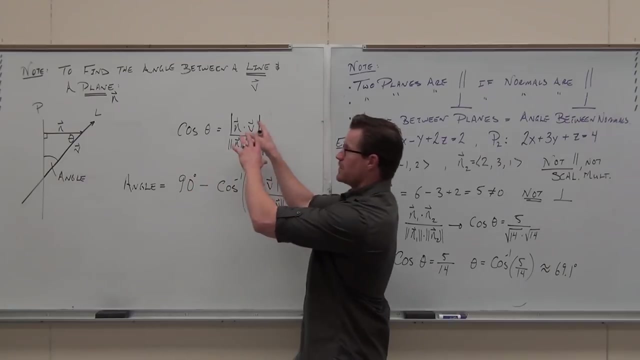 This is to keep it positive. Sorry, keep it positive and make an acute angle. You have to have that because you're subtracting from 90. The idea is, if you do this, you're going to find the angle between the normal and the line, the direction vector. 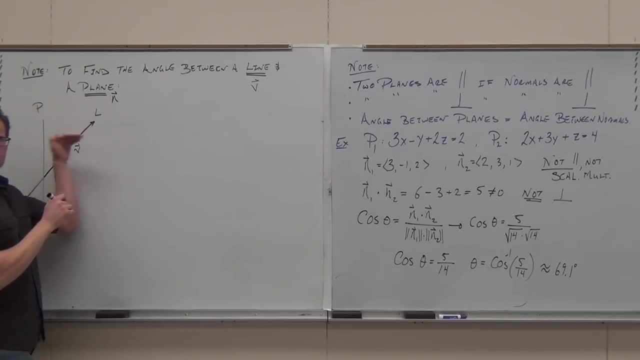 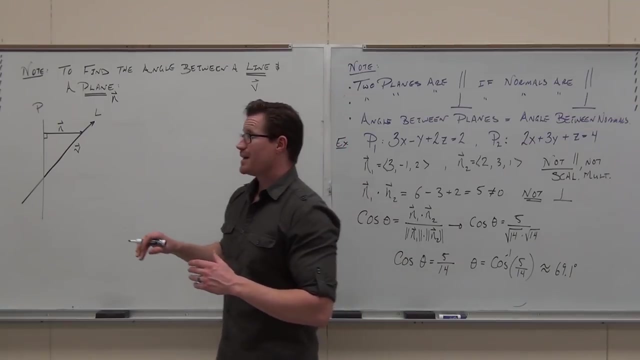 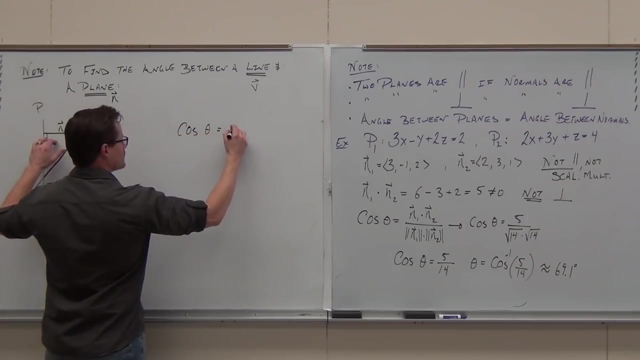 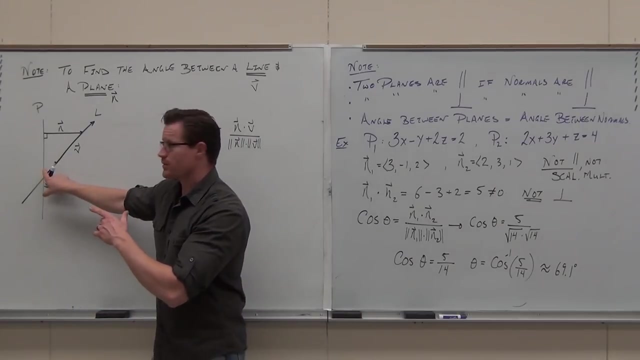 But the normal, the normal doesn't go this way, The normal goes this way, The normal goes that way. Does that make sense to you? Watch carefully so you don't miss it. If I do this, Will it give me the angle here? please watch carefully. 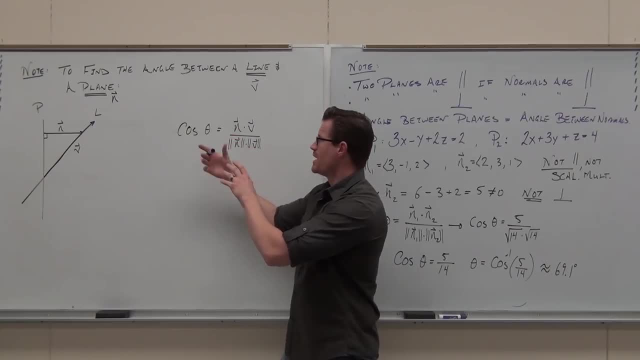 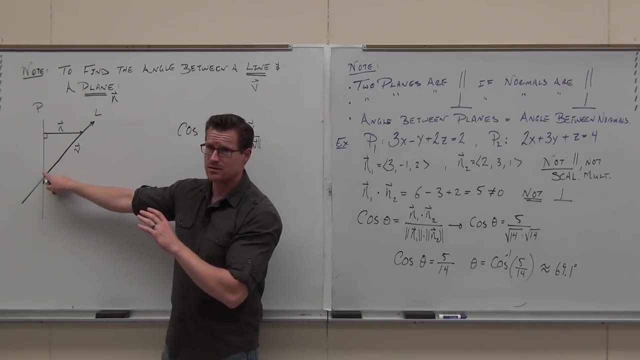 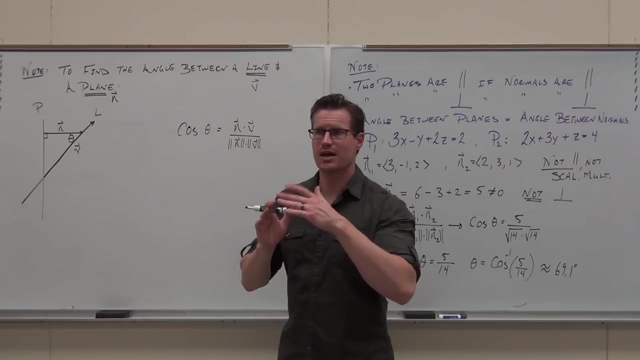 When you dot, when you do this, when you dot product divided by the magnitudes, that gives you the cosine of the angle. that is between these two vectors. This is not between these two vectors. That is between those two vectors. And in order to figure out the acute one, I do the absolute value. 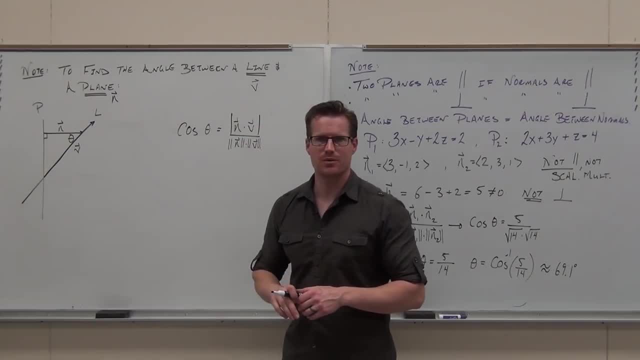 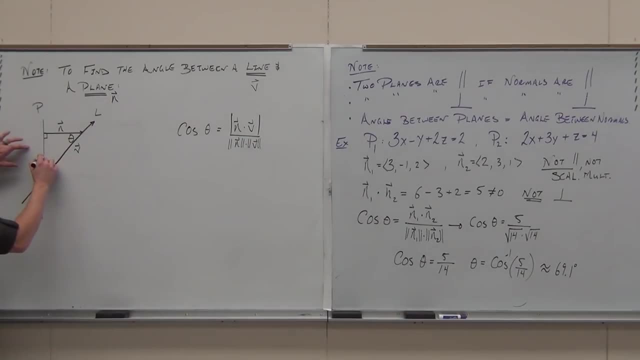 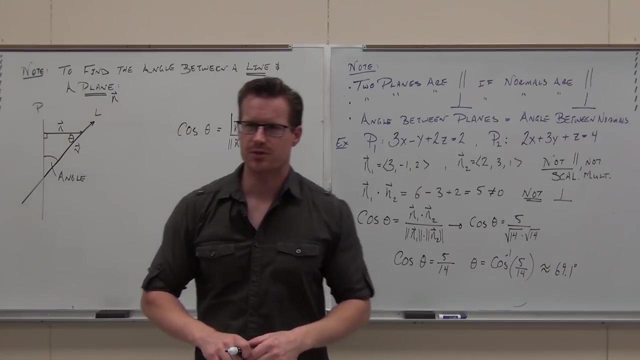 to keep it positive, to keep that thing acute. Head nod if you're okay with that one. Well, wait a minute. That's not the question. The question is: how do I figure out that angle? Use your, use your geometry. 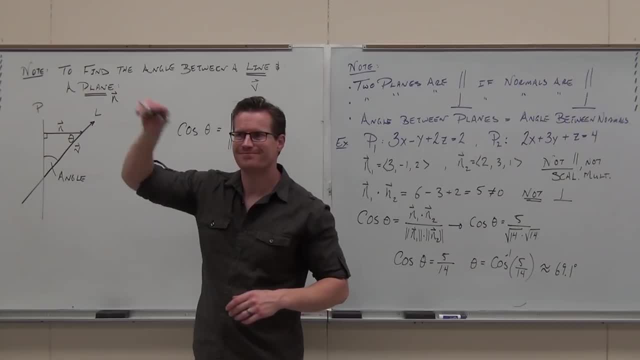 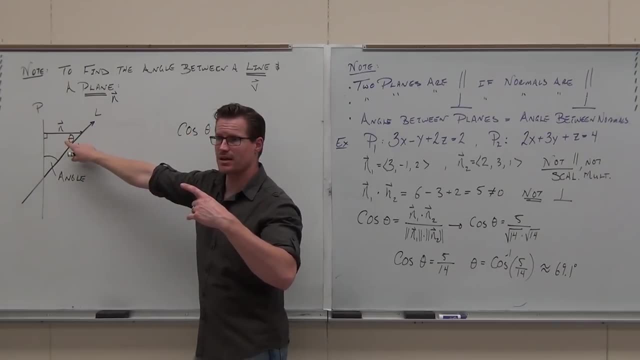 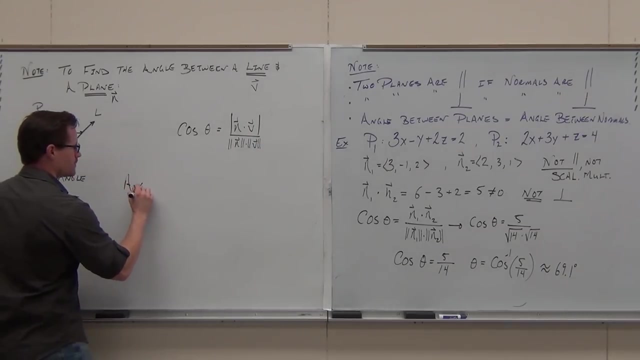 Use your geometry a little bit. How much is all of my One and Ninety's already taken up One? and So if I do 90 minus whatever that angle is, then I will have that angle. So in our case, if you ever want to find the angle between a line, 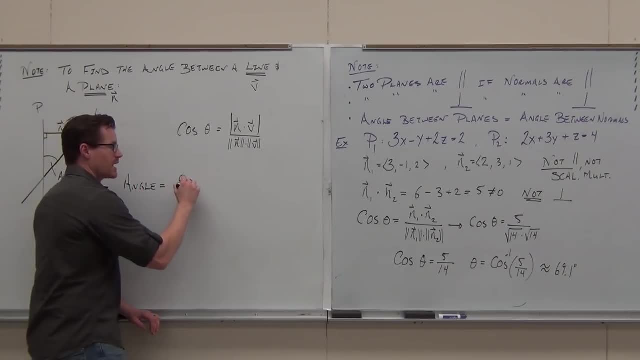 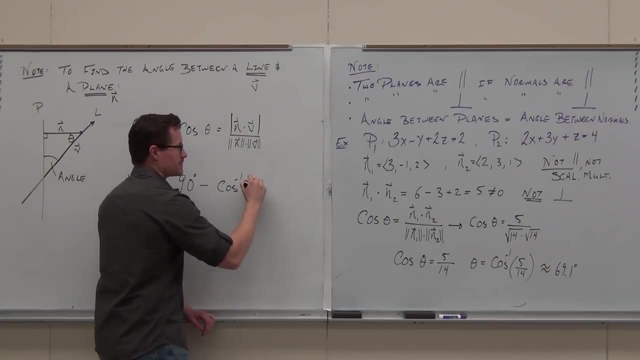 and a plane. the angle is: hey, take your 90 degrees, subtract cosine, inverse of this thing. This is to keep it positive. Sorry, keep it positive and make an acute angle. You have to have that because you're spreading it. 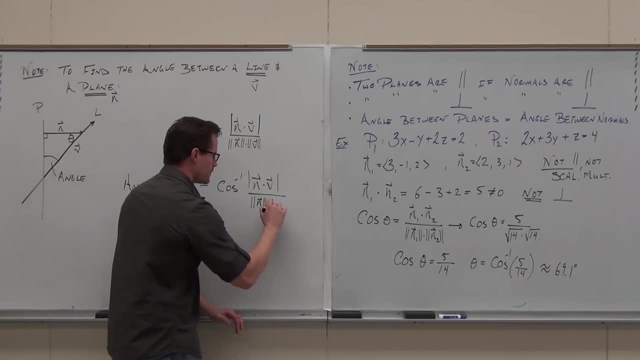 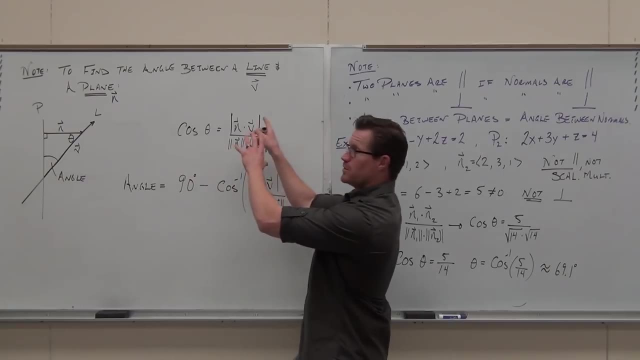 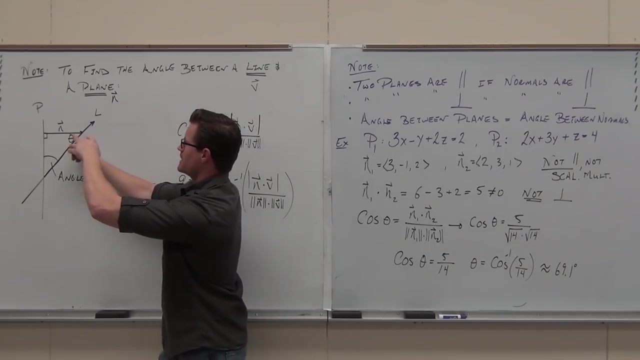 Ninety. The idea is: if you find, if you do this, you're going to find the angle between the normal and the line, the direction vector. If I take 90 minus cosine inverse of that, that scenario, I find that angle. 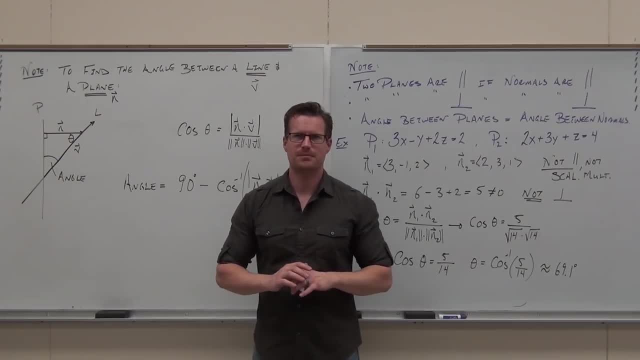 Ninety minus. that gives us the angle between the plane and the line Head. nod, if you're okay with that one. Okay, Last thing, because I know I'm not going to be able to do this. I'm getting tired and I can tell that you're getting tired. 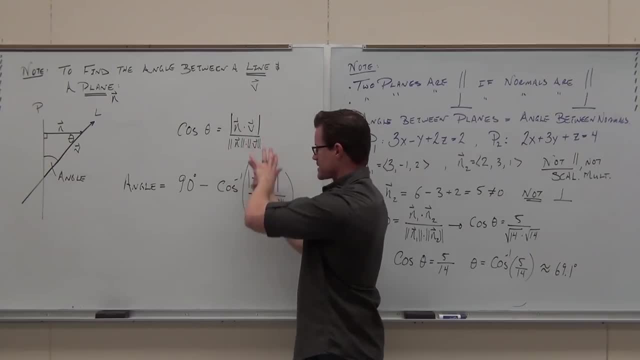 If I take 90 minus cosine, inverse of that, that scenario, I find that angle 90 minus 90 minus 90 minus. that gives us the angle between the plane and the line. And now, if you look here, that one. 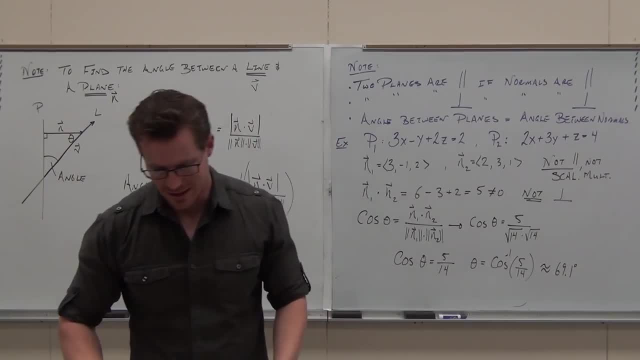 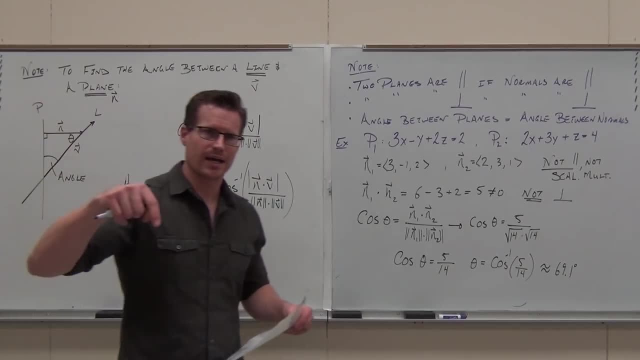 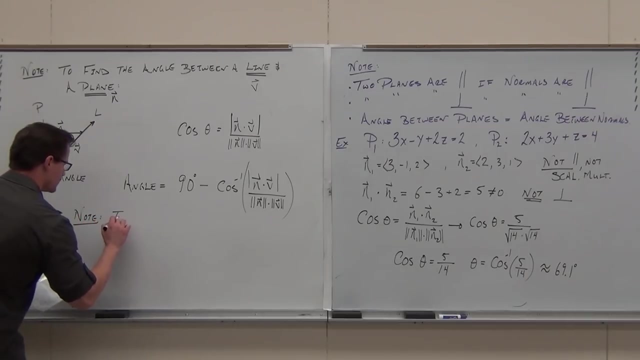 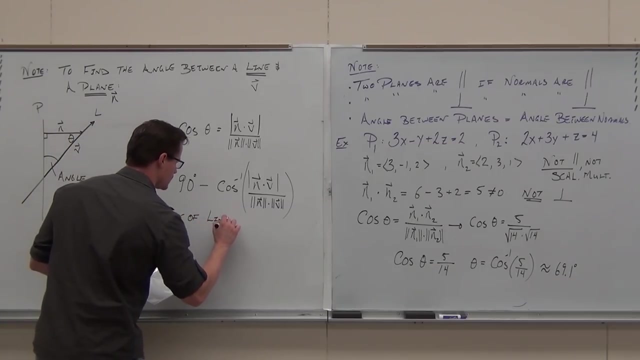 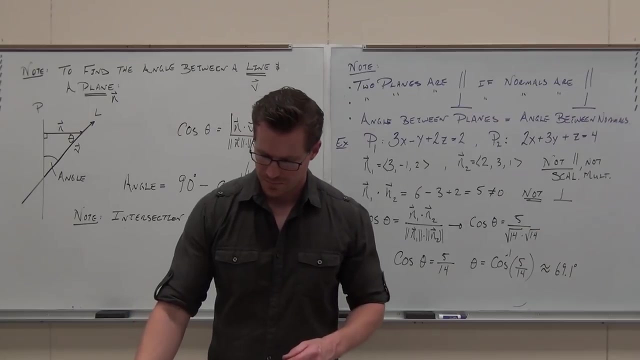 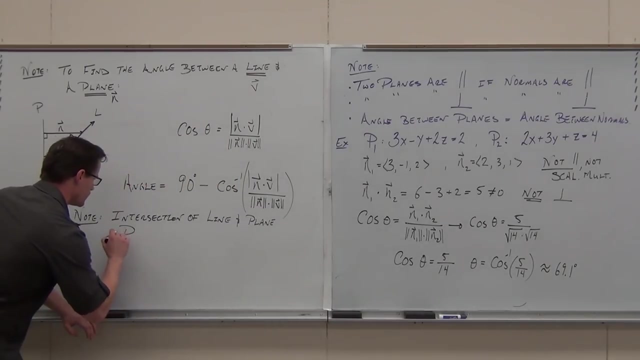 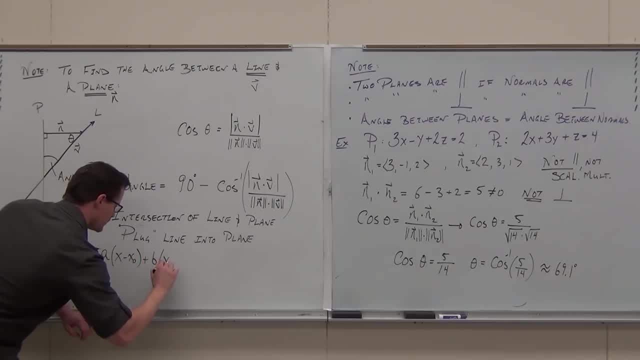 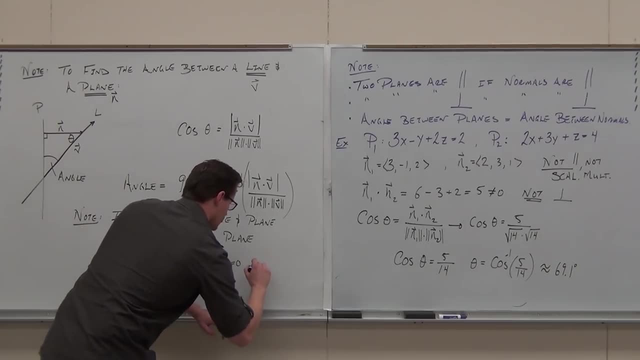 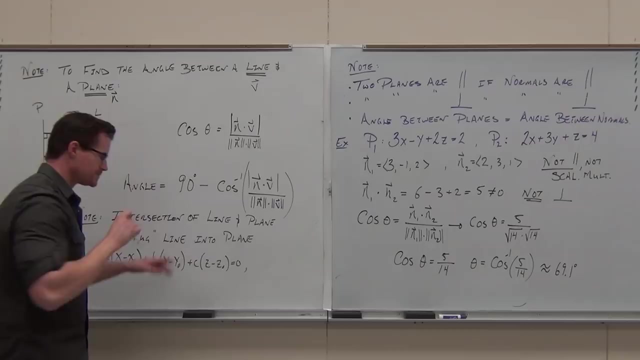 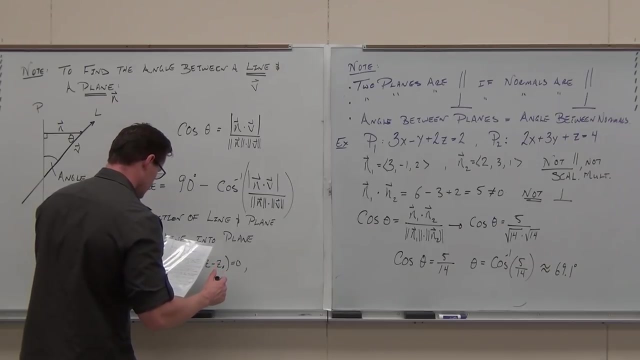 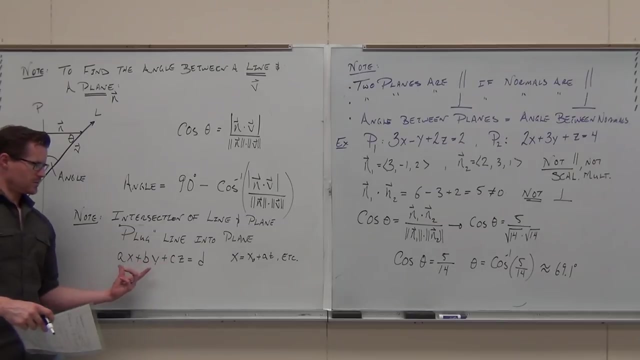 Thank you. Uh, actually this is even easier Here. do this: You got, you got a plane, You got, et cetera. okay, You have X, Y and Z. If you take this stuff, here's your X, same X. 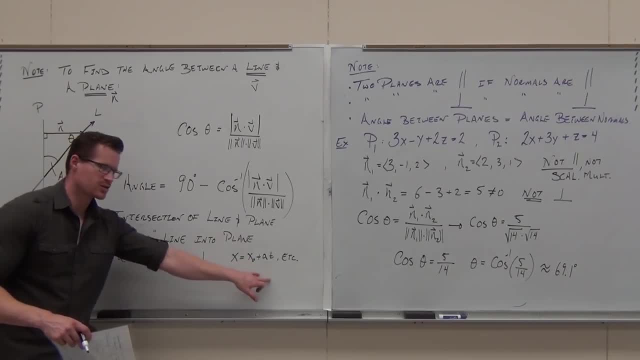 Take this, plug it in for X. Take the next one. plug it in for Y. Take the next one, plug it in for Z. You can easily find the intersection. Do you guys want to do one, or are you okay with it? 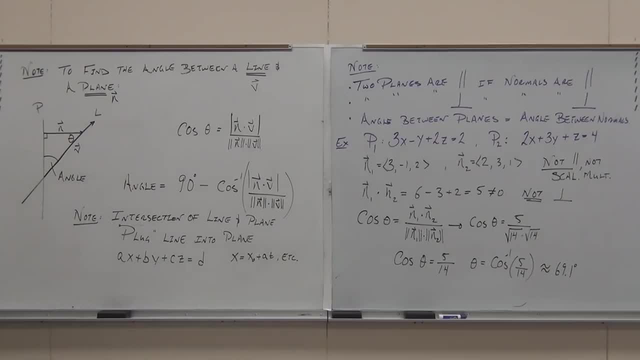 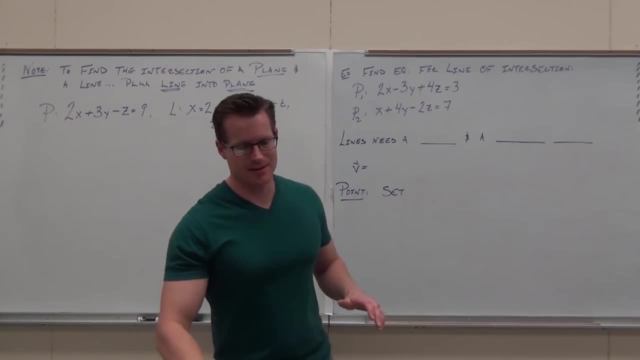 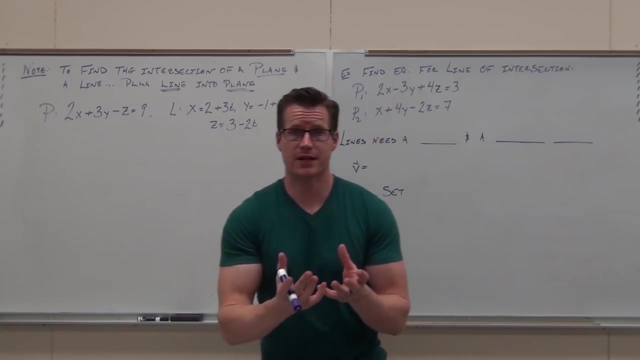 Okay, let's do it next time, all right, Let's do it next time, All right. so back at it. for lines and planes, There was something we stopped on last time: How to find the intersection of a plane and a line. I told you it's very easy. 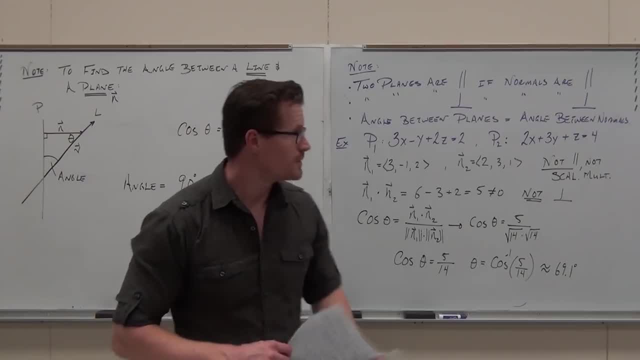 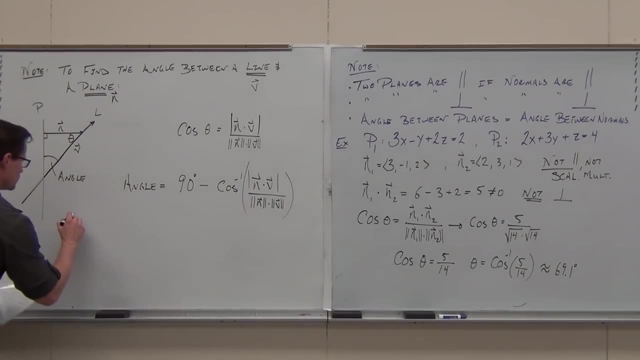 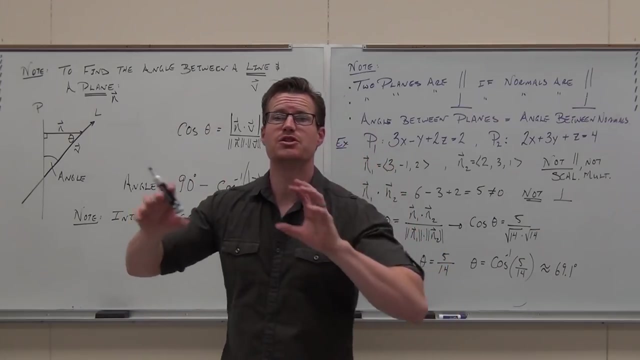 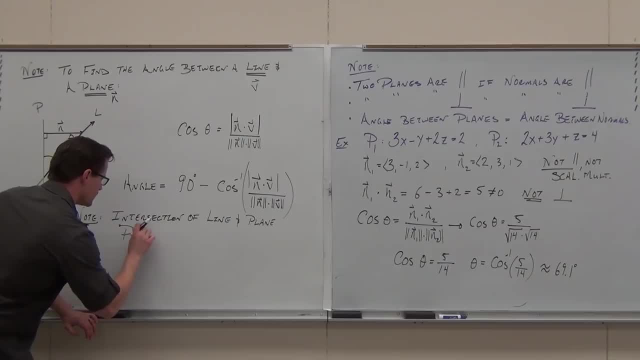 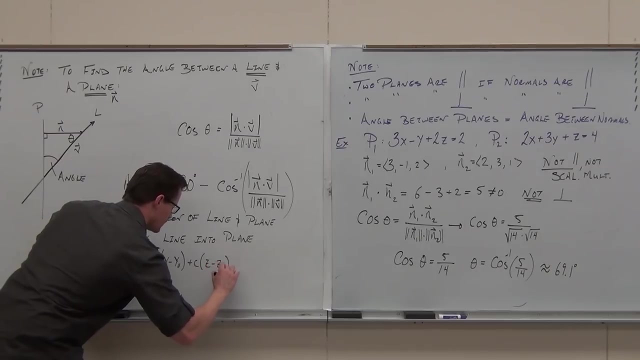 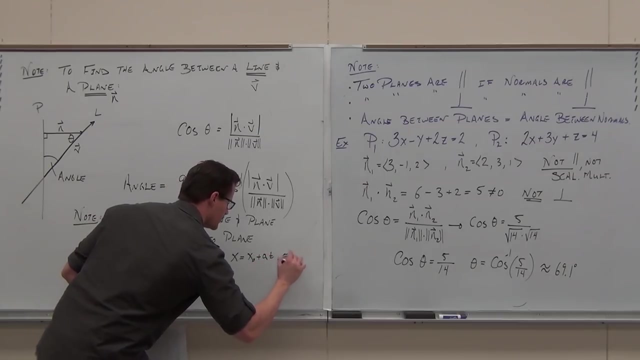 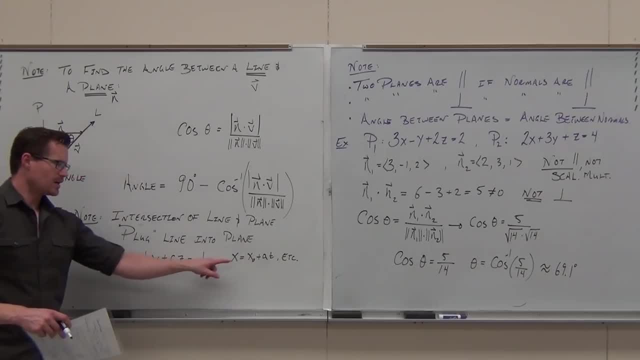 You got, etc. You have x, y and z. If you take this stuff, Here's your x, It's the same x. Take this. Plug it in for x. Take the one. plug it in for y. Take the next one. 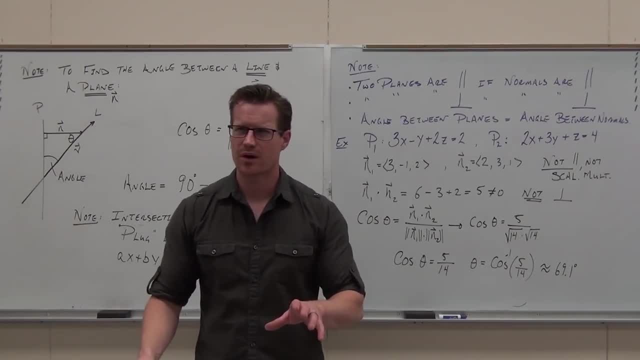 Plug it in for z. You can do a пару efforts. You can hörm is gigak circle easily find the intersection. Do you guys want to do one, or are you okay with it? Okay, let's do it next time. 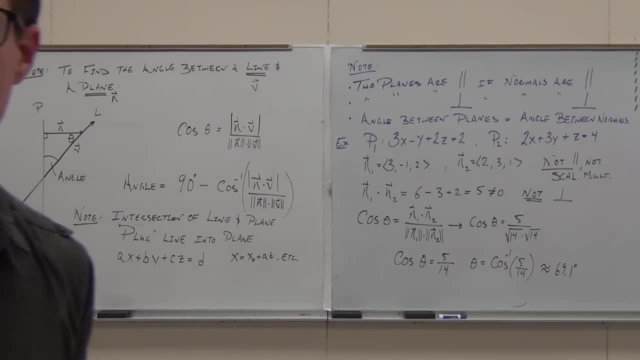 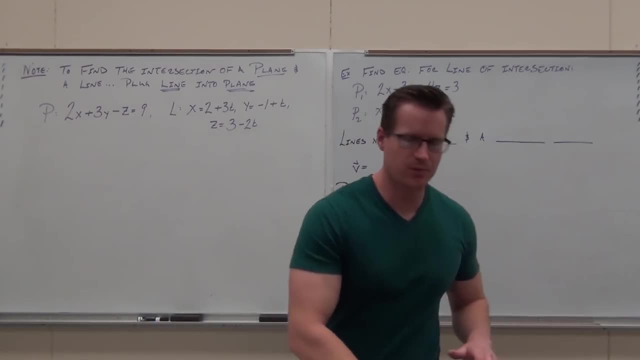 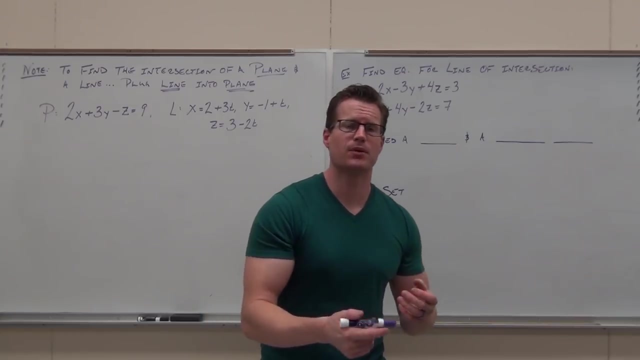 Let's do it next time. Alright, so back at it. for lines and planes. There was something we stopped on last time: How to find the intersection of a plane and a line. I told you it's very easy. We're going to do it with an example. 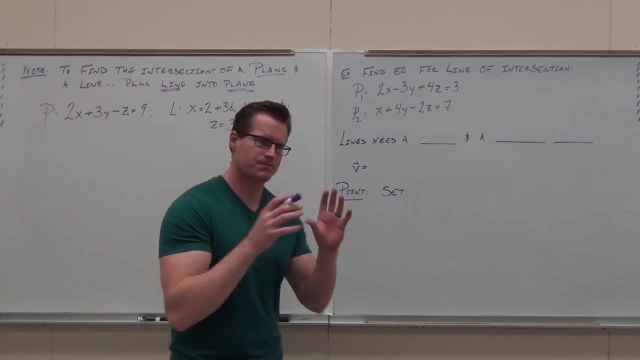 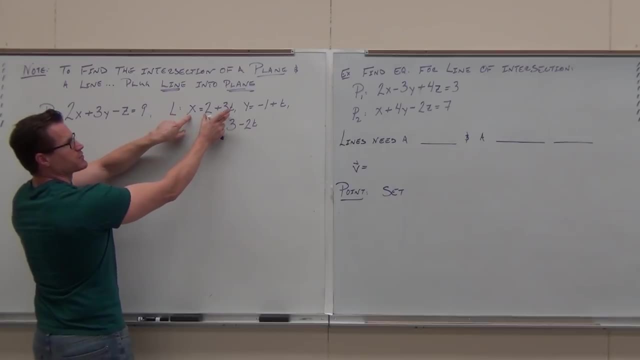 We're going to do it with an example. Here's how you find an intersection of a plane and a line: Literally take the line, plug it into the plane. If we have an expression for X, an expression for Y, an expression for Z and our plane has that, 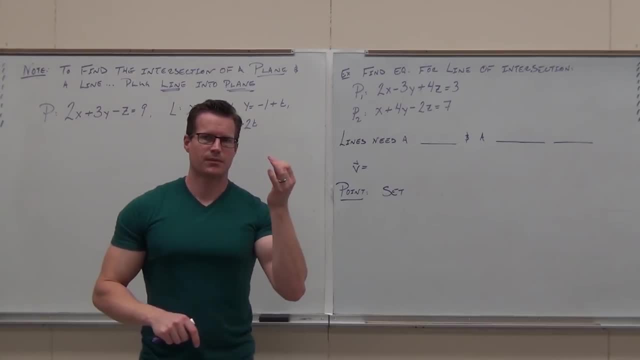 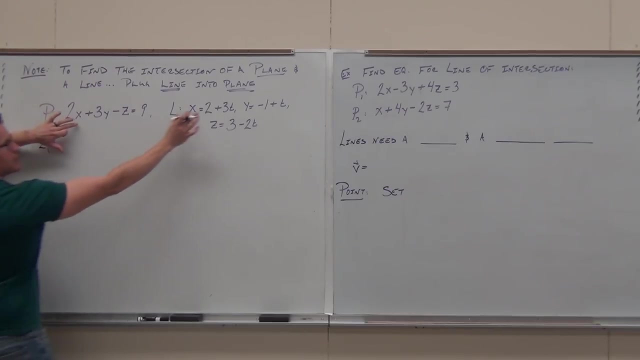 substituting these in will let us solve for T. Taking that T and putting it in for the line will give us a point on the line That will let us solve for the intersection of the plane and the line. So what that would look like, take our plane: X is 2 plus 3T. 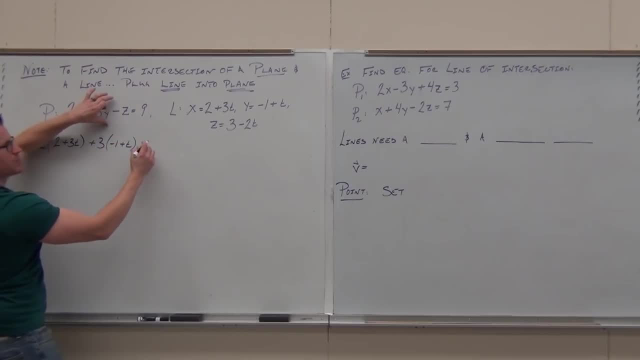 Y negative 1 plus T minus Z. just don't forget parentheses: 3 minus 2T and that still equals 9.. So we're just taking our X coordinates, really equations for those metric, plugging them into our plane. 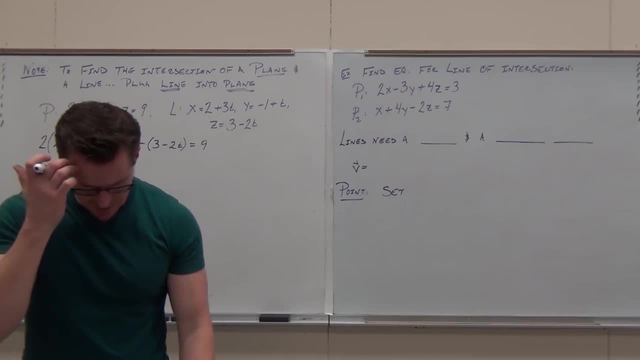 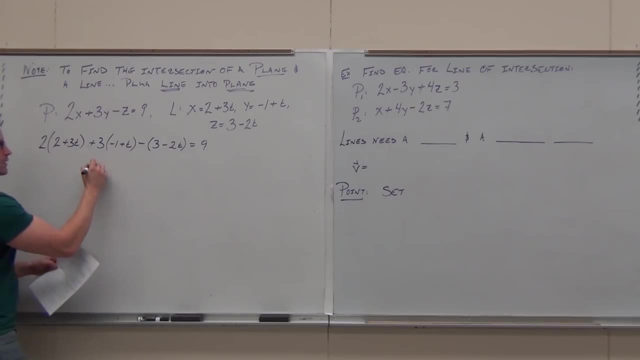 and solving for T. When we do that, I'm sure that you can do this on your own. What we end up getting here. let's see, make sure I'm right. If you solve this, you're going to ultimately- and maybe you can check my work and let me know- 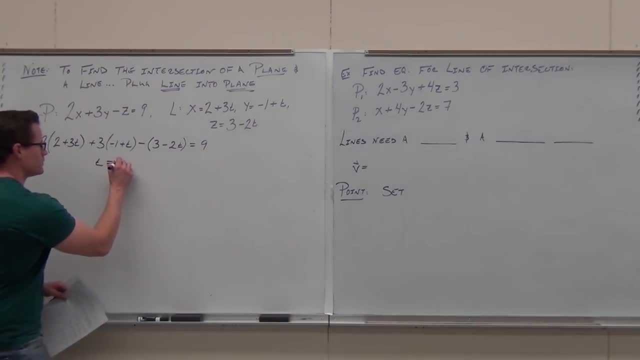 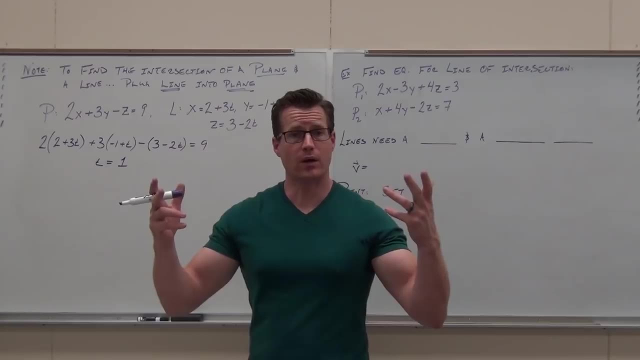 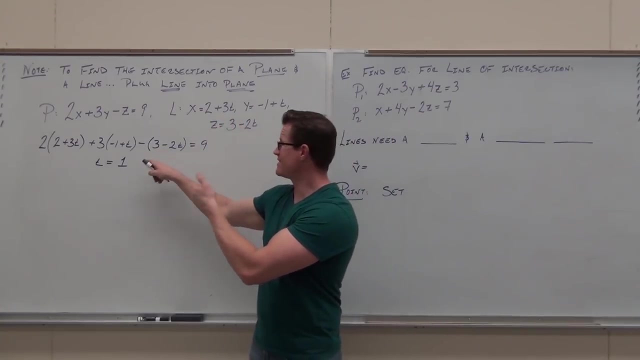 in a couple minutes, if I'm right, you get T equals 1.. Now, T equals 1 is not a point. T equals 1 is more like a time. Well, if we have an equation that translates time into points X, Y and Z, we can take that, put it here. 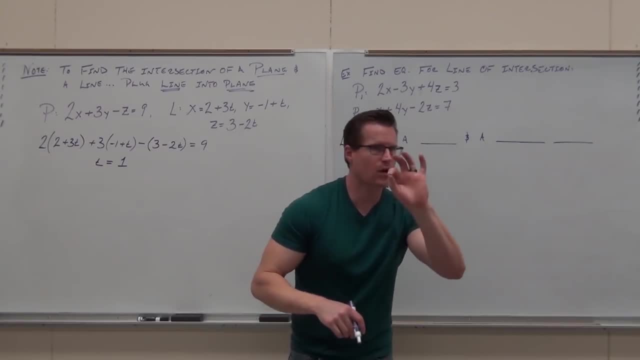 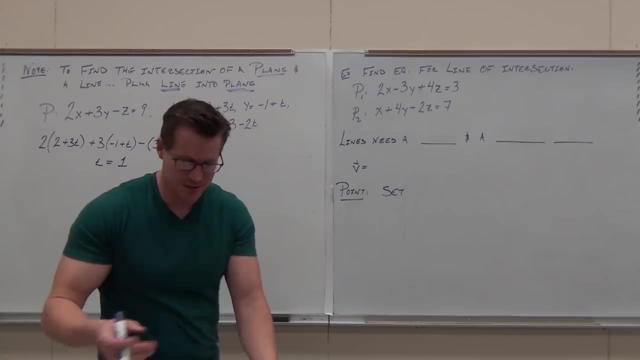 and then you can tell me a point on the line at the place where it crosses the plane. Does that make sense to you? So it's pretty straightforward: Take the line, plug it into the plane, solve for T and then put that back in. 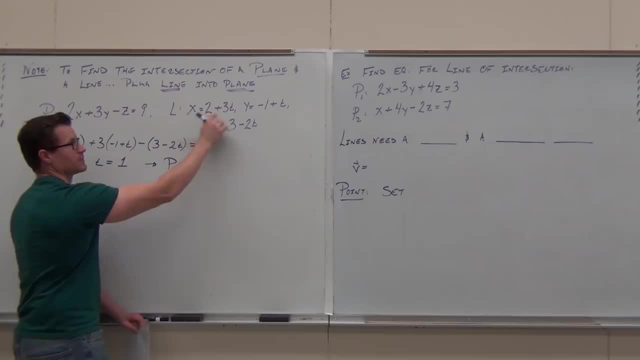 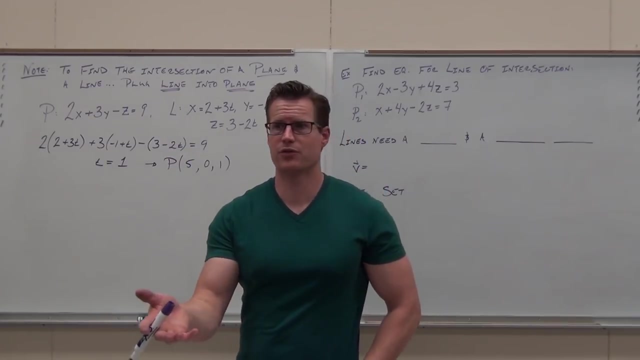 So when we do that, we get this point looks like 5, 0, 1.. That would be the point where that line crosses that particular plane. Are you guys okay on the idea behind it? We're covering more kind of ideas right now. 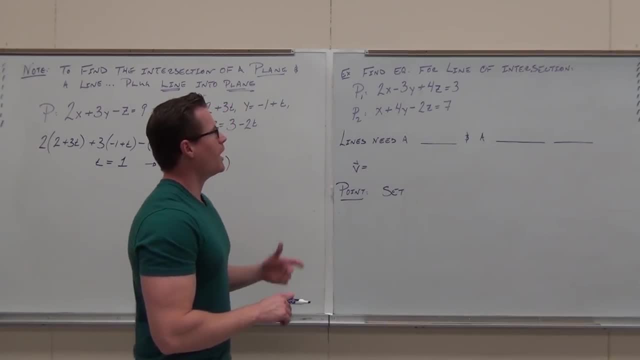 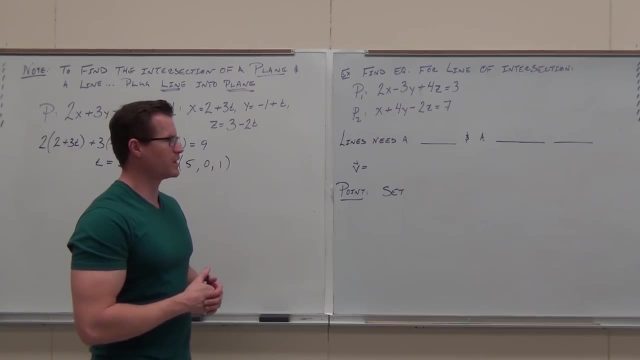 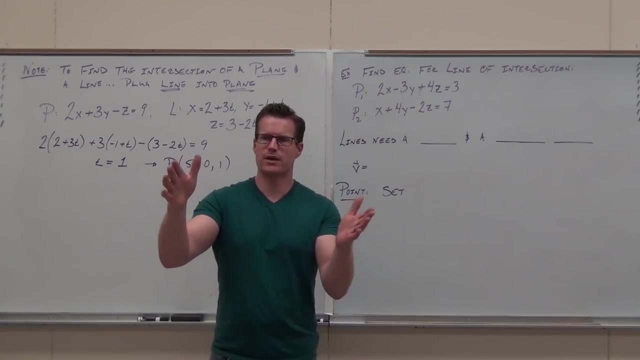 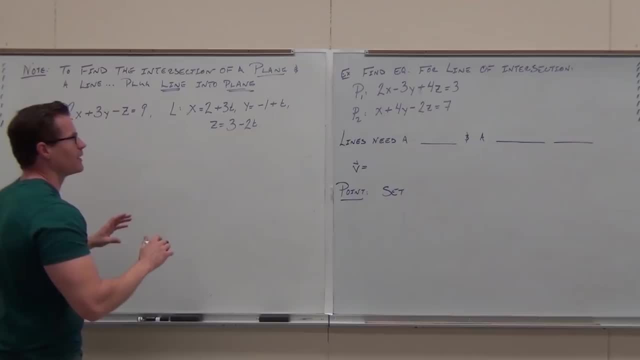 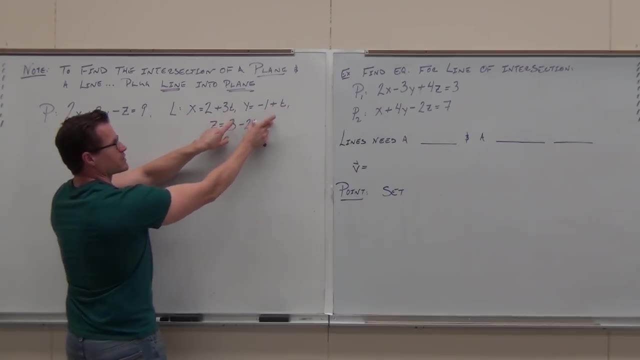 Here's how you find the intersection of a plane and a line: Literally take the line and plug it into the plane. If we have an expression for x, an expression for y, an expression for z and our plane has that, substituting these in. 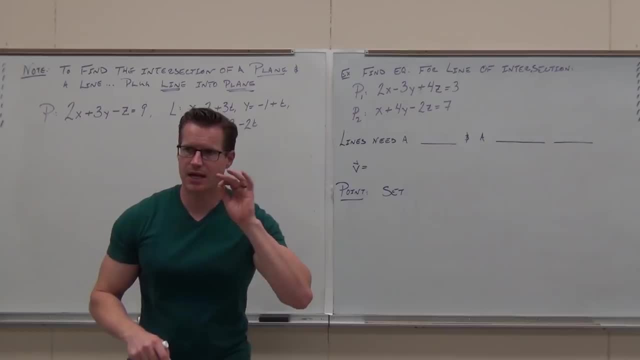 will let us solve for t. Taking that t and putting it in for the line will give us a point on the line That will let us solve for the intersection of the plane and the line. So what that would look like, Take our plane. 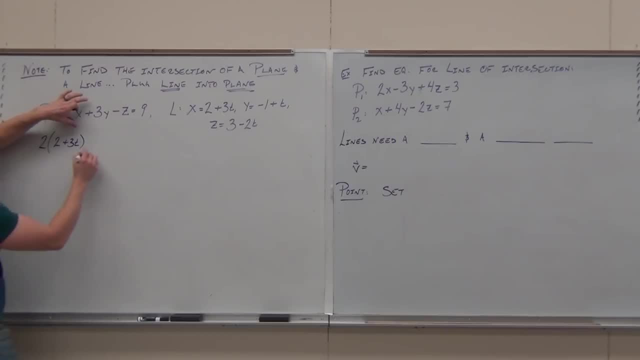 x is 2 plus 3t, y negative 1 plus t Minus z- Just don't forget parentheses- 3 minus 2t And that still equals 9.. So we're just taking our x coordinates, really equations for those. 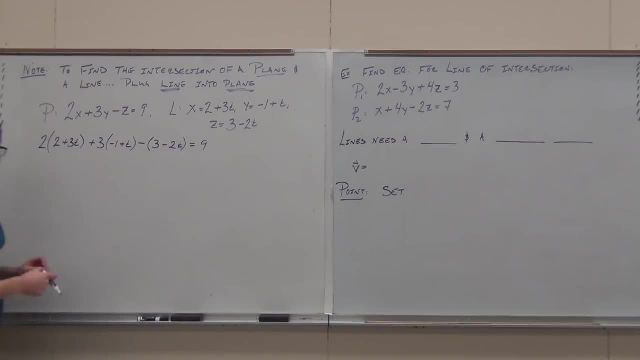 metric, plugging them into our plane and solving, When we do that. I'm sure that you can. you can do this on your own- What we end up getting here. let's see, make sure I'm right. If you solve this, you're going to ultimately- and maybe you can check my work and let me know in a couple minutes if I'm right- 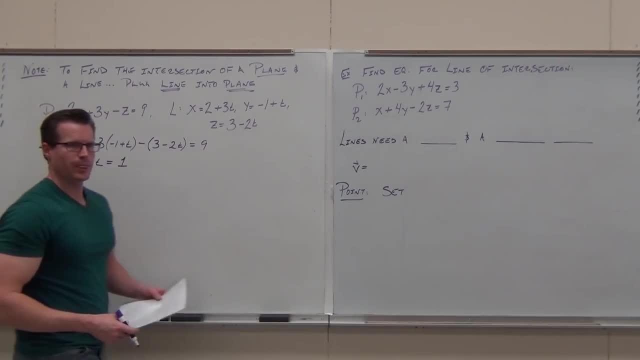 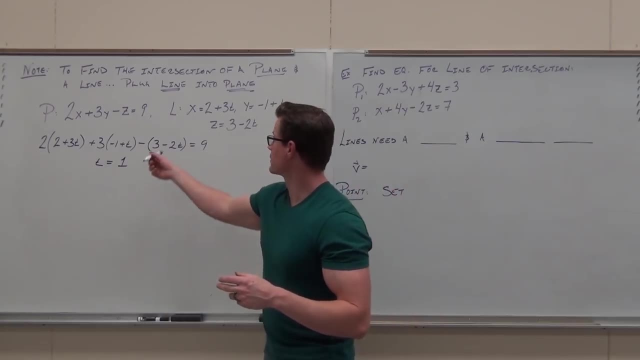 you get t equals 1.. Now, t equals 1 is not a point. t equals 1 is more like a time. Well, if we have an equation that translates time into points x, y and z, we can take that. 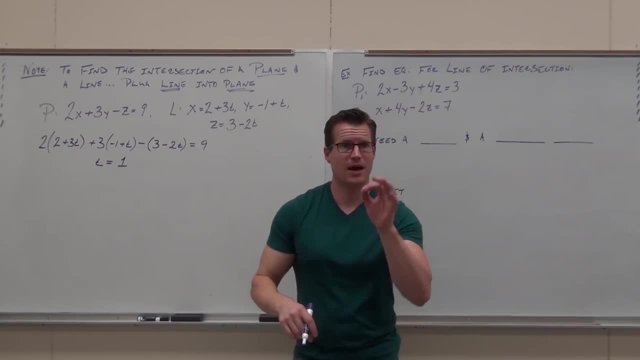 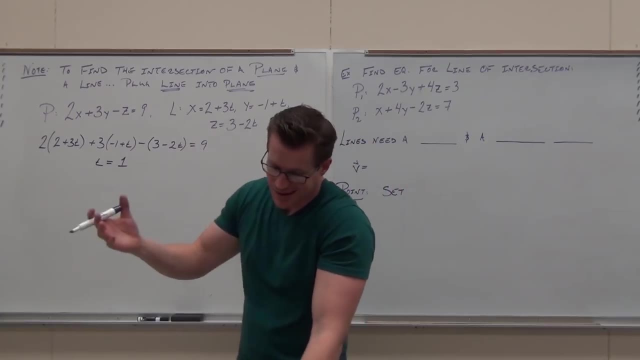 put it here, and then you can tell me a point on the line, at the place of the line, That's the place where it crosses the plane. Does that make sense to you? So it's pretty straightforward: Take the line, plug it into the plane, solve it for t. 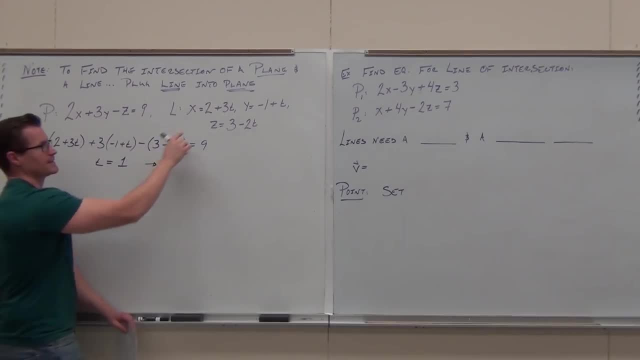 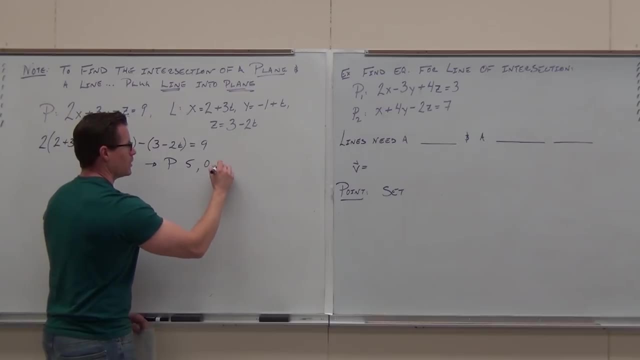 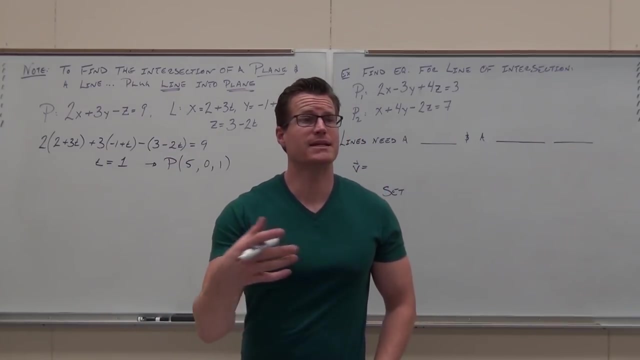 and then put that back in. So when we do that we get this point. It looks like 5, 0, 1.. That would be the point where that line crosses that particular plane. Are you guys okay on the idea behind it? 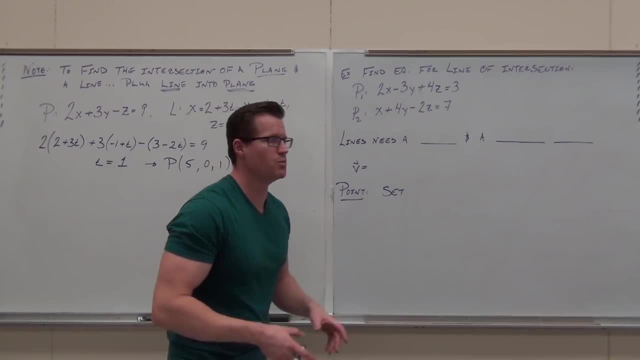 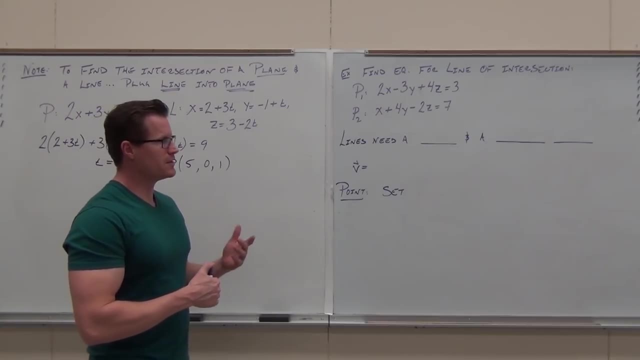 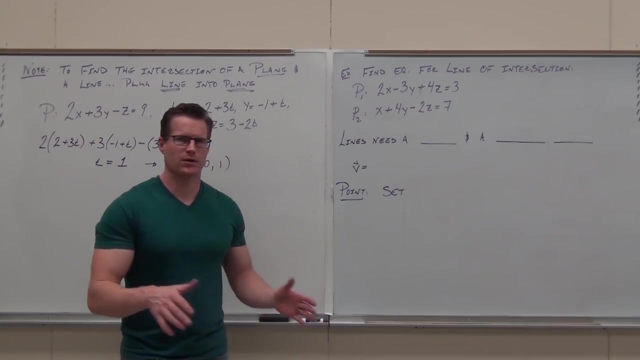 We're covering more kind of ideas right now. This one we're going to thoroughly do, but it's kind of an idea concept. I want to find the equation for a line of intersection between two planes. What- Wait a second If planes aren't parallel? 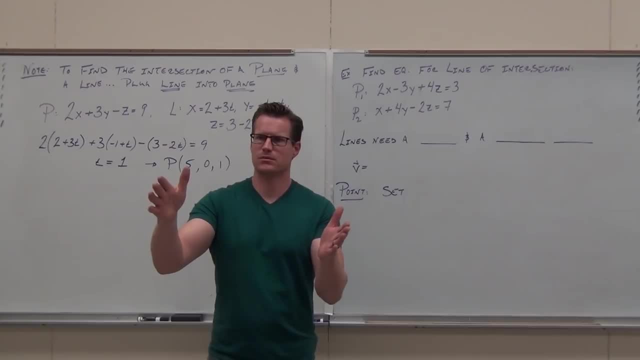 will they cross? No, If planes are not parallel, will they cross? Yes, They're not. like lines, Lines can be skewed, Planes cannot be. Planes go forever. right These sheets If they're somewhere in space and they're not parallel. 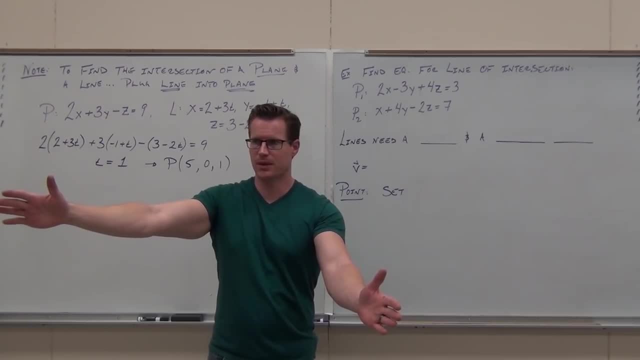 they will cross somewhere. That is going to happen. I want to find- and when they cross they're going to make a line- The crossing of those two planes. just like the xy plane and the yz plane cross, right, They make a line. 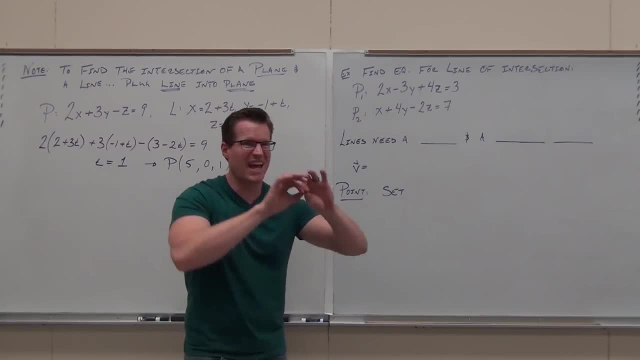 and that line is an axis that we have. So we're going to get kind of an axis, but not along a regular axis, One that goes along whatever. two planes. I tell you These two planes. I don't know if you're okay with that one. 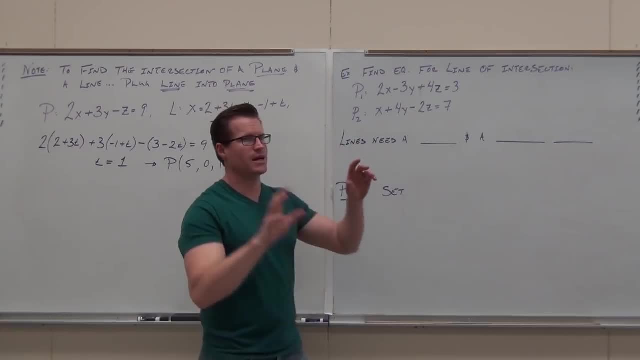 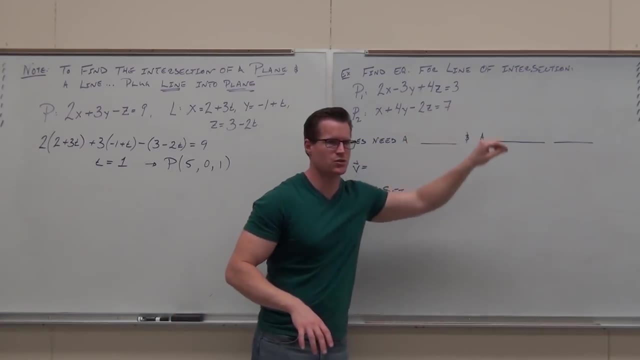 Let's first figure out the relationship of those two planes. Can you find right now- and you should be able to, can you find the normals for those two planes? I'm going to give you 15 seconds. Write down the two normals. 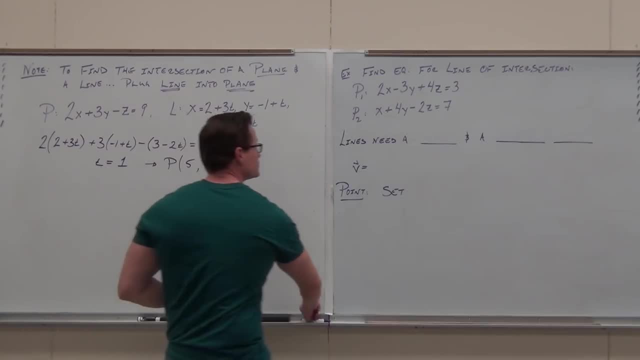 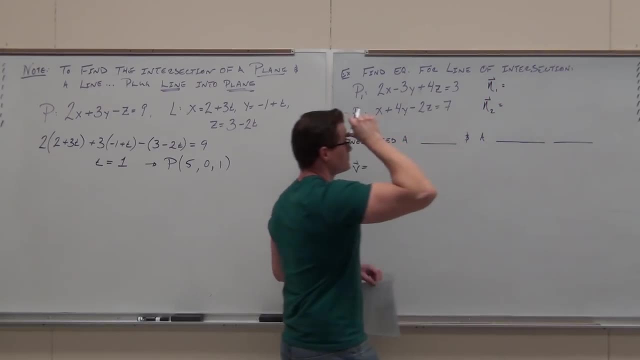 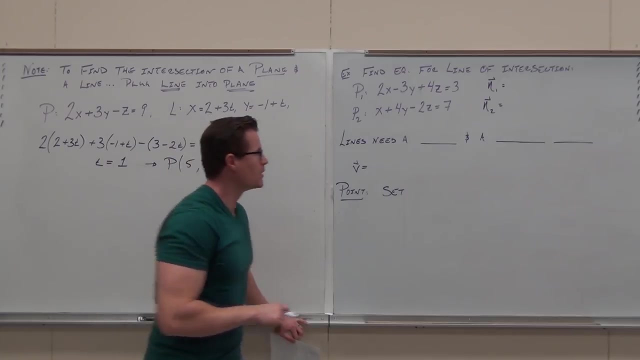 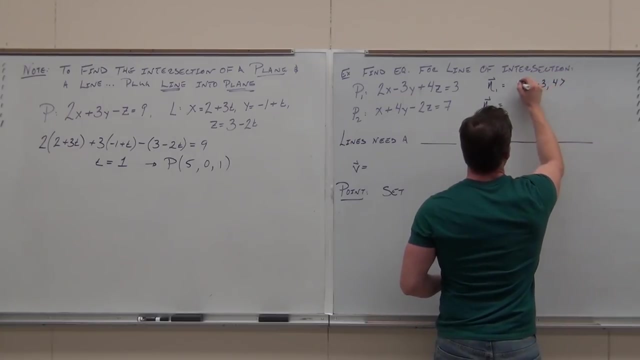 Let's have n1 and n2.. I love planes. I love them because the normals are so nice, So nice to find What's the normal for this one. Let's get a little bit more enthusiasm for that one. Goodness gracious. 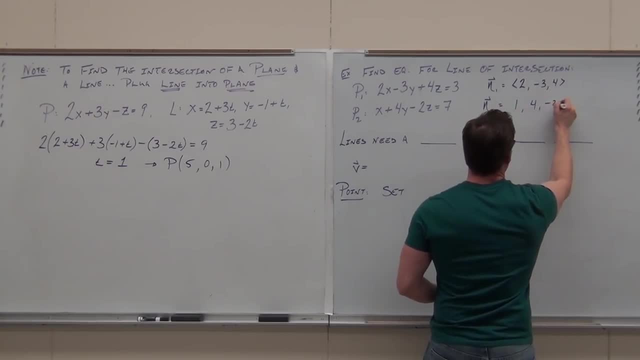 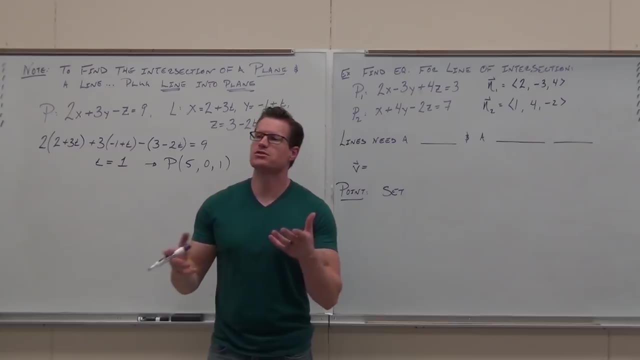 How about this one? What's that one? You don't get to yell at me, Goodness, gracious, Yeah, those are the normals. Okay, let's describe the relationship between the planes. I told you that these planes are going to intersect unless they're parallel. 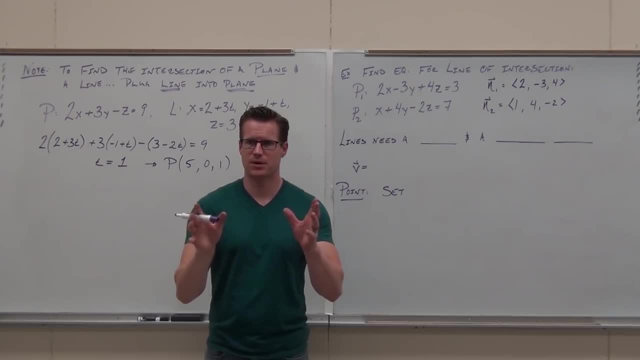 Are the planes parallel? Why not? Because the normals aren't parallel and the relationship between the normals is the relationship between the planes. If they're parallel, the planes are parallel. If they're perpendicular, the planes are perpendicular. These are not parallel. 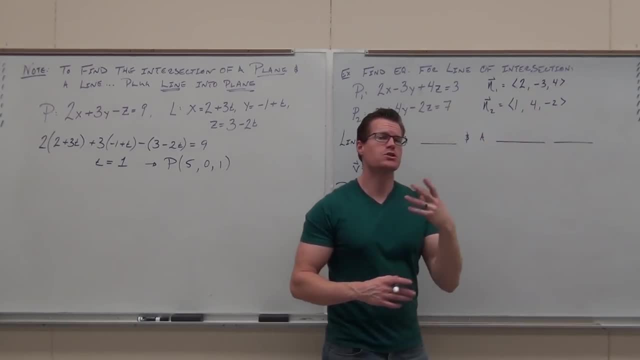 You can tell they're not scalar multiples. They're also not perpendicular. They're not perpendicular because if you did the what product, The dot product, The dot product is not zero. You can do it right now: 2 minus 12 minus 8. 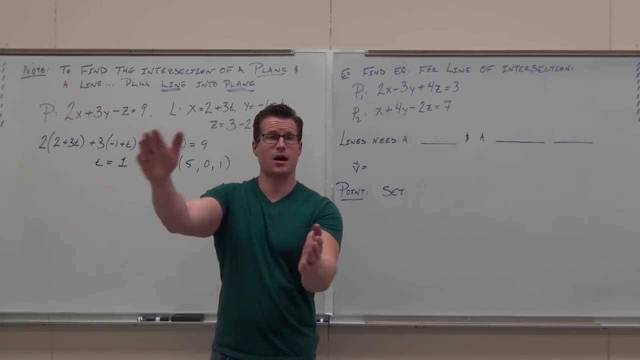 Yes, Yes, They're not like lines. Lines can be skewed, Planes cannot be. Planes go forever. right, These sheets, If they're somewhere in space and they're not parallel, they will cross somewhere. That is going to happen. 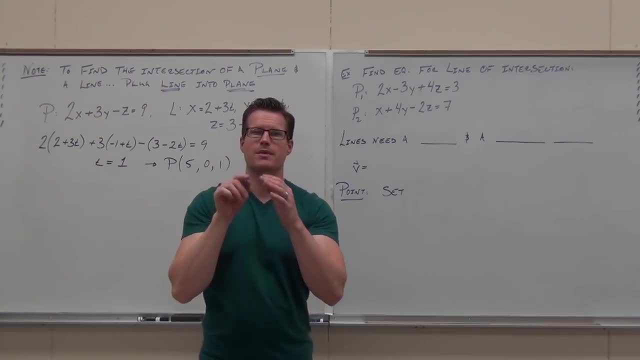 I want to find- and when they cross, they're going to make a line- The crossing of those two planes. just like the XY plane and the YZ plane cross, right, They make a line and that line is an axis that we have. 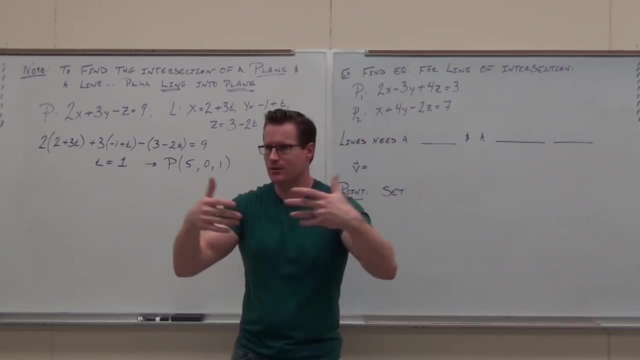 So we're going to get kind of an axis, but not along a regular axis, one that goes along whatever Two planes. I tell you, these two planes, head nod, if you're okay with that one. Well, let's first figure out the relationship of those two planes. 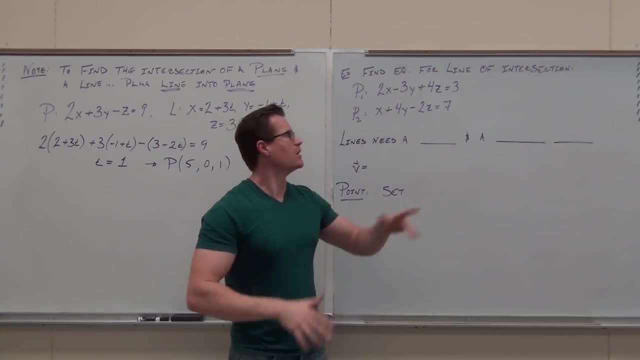 Can you find right now- and you should be able to- can you find? oh, it's good to review the normals for those two planes. I'm going to give you 15 seconds. write down the two normals. Let's have N1 and N2.. 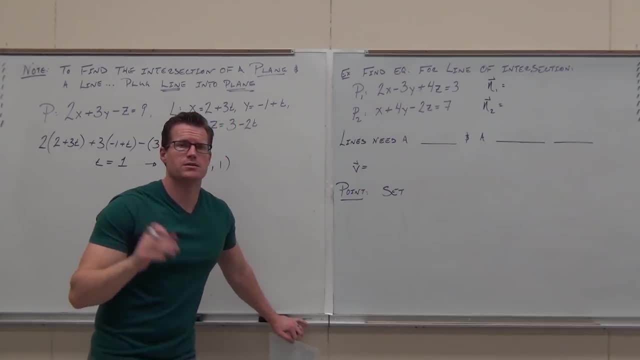 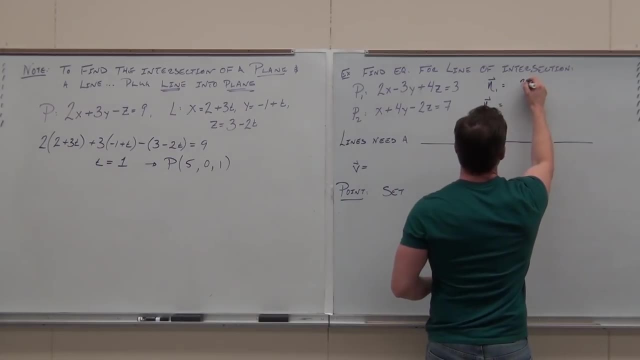 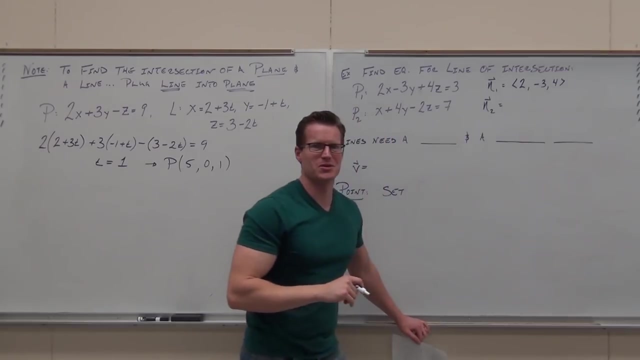 I love planes. I love them because the normals are so nice, so nice to find What's the normal for this one. Let's get a little bit more enthusiasm, because that one, goodness gracious. How about this one? what's that one? 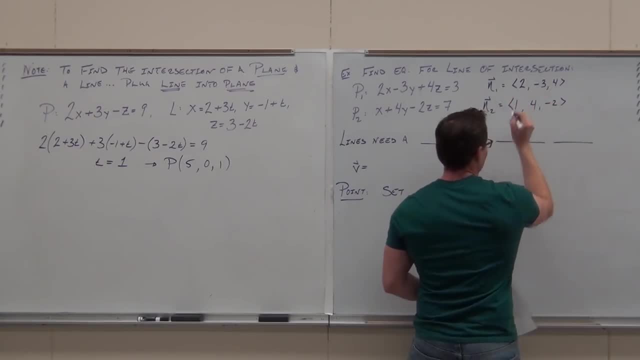 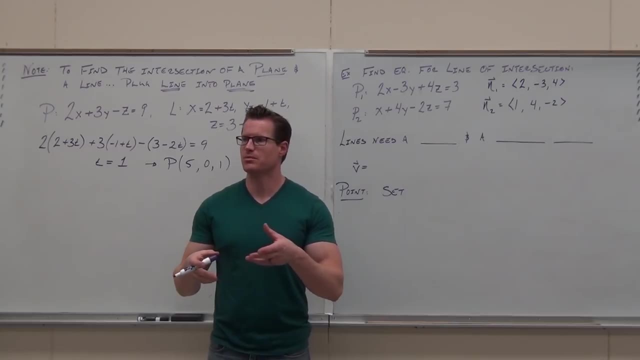 One, four, two and two. You don't get to yell at me, jeez, goodness gracious, Just joking. Yeah, those are the normals. Okay, let's describe the relationship between the planes. I told you that these planes are going to intersect unless they're parallel. 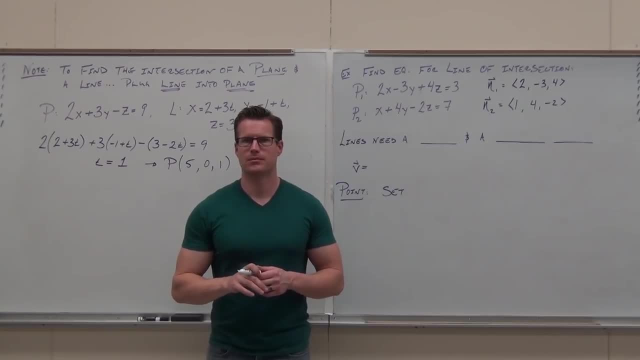 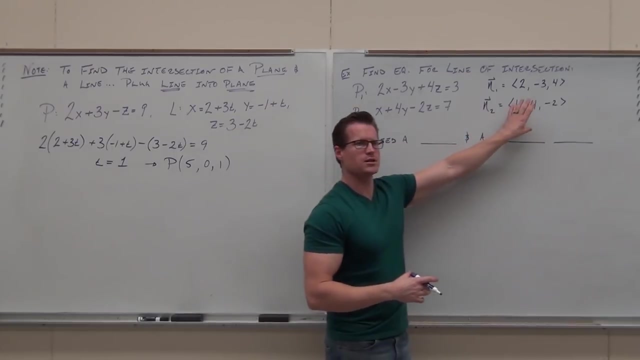 Are the planes parallel? Why not? Because the normals aren't parallel and the relationship between the normals is the relationship between the planes. If they're parallel, the planes are parallel. If they're perpendicular, the planes are perpendicular. These are not parallel. 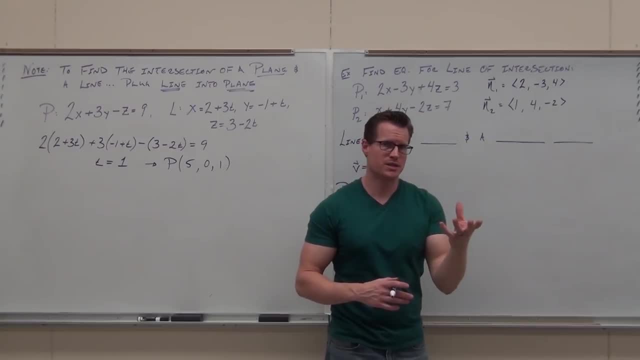 You can tell. they're not scalar multiples, They're also intercalated. They're also not perpendicular. They're not perpendicular because if you did the what product, the dot product, the dot product is not zero. You can do it right now. 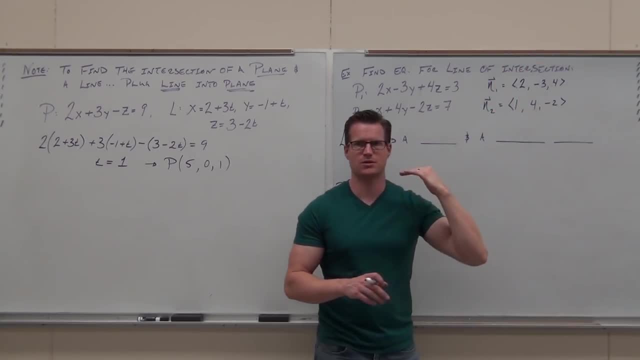 Two minus 12 minus eight, not zero. Does that make sense? So they're not parallel, They're not perpendicular. They will for sure cross because they're not parallel. What I want to do, I want to find the equation of the line of intersection of these two planes. 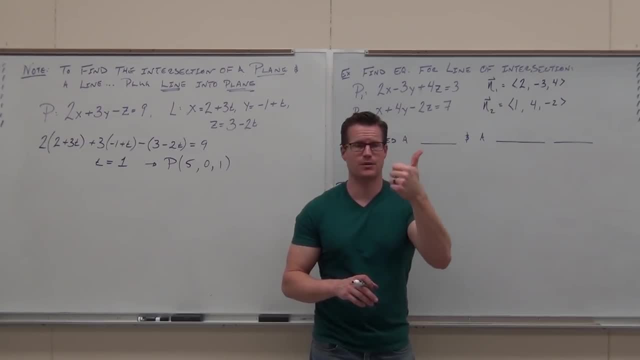 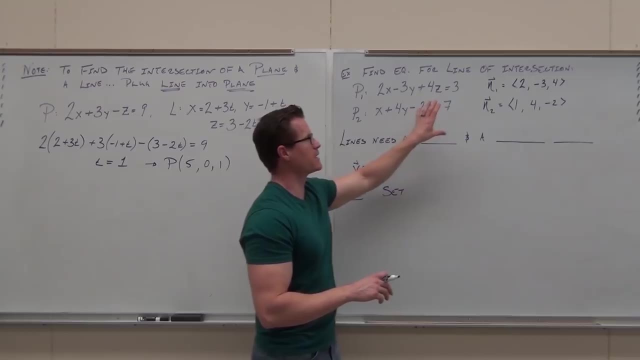 not zero. Does that make sense? So they're not parallel, They're not perpendicular. They will for sure cross because they're not parallel. What I want to do, I want to find the equation of the line of intersection of these two planes. 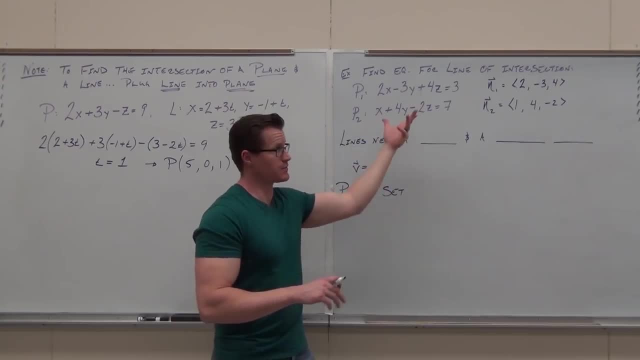 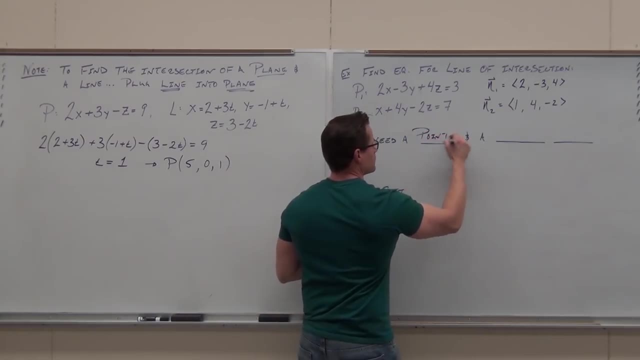 Now, what do lines, lines of intersection even? what do they need? There's two things. lines always need to come on. What do they need? Point Point Vector. We'll talk about the point last, because you're probably going to think it's more difficult. 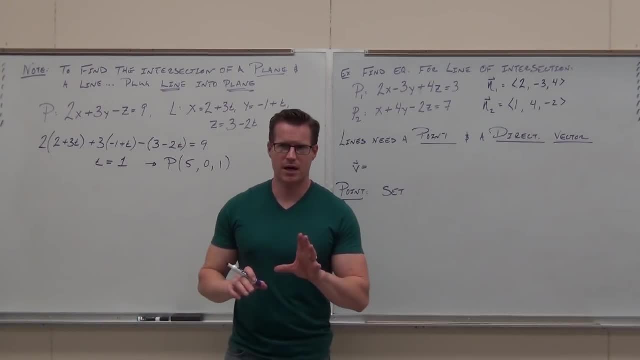 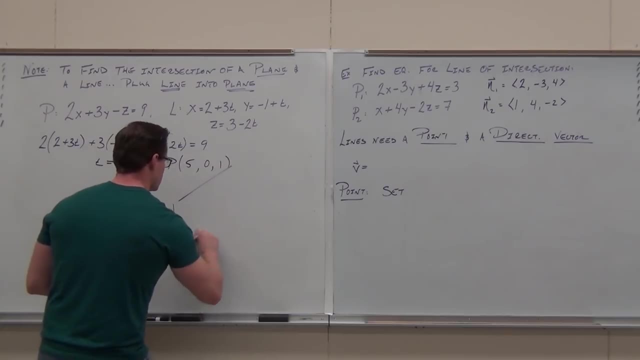 The vector is actually very, very easy. You just need to see it one time and then you'll get it. Check it out. I'm going to draw you a picture over here. Here's a plane. Here's the other plane. Here's the other plane. 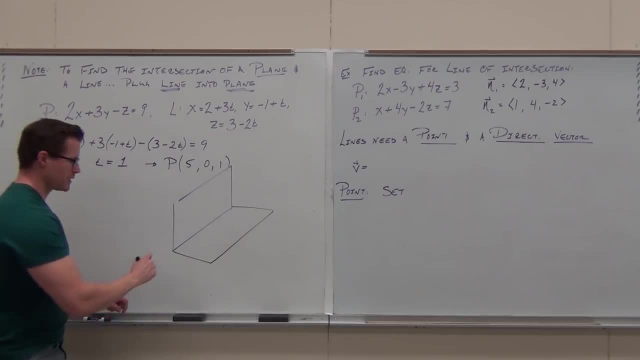 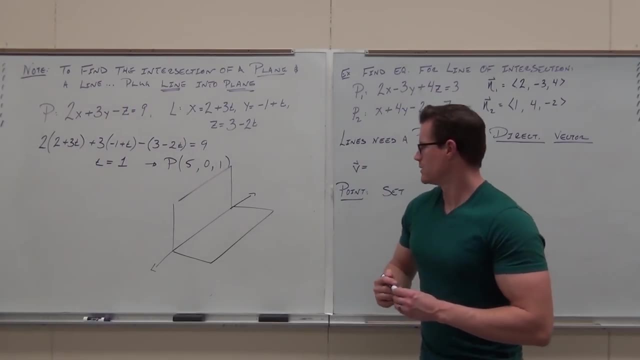 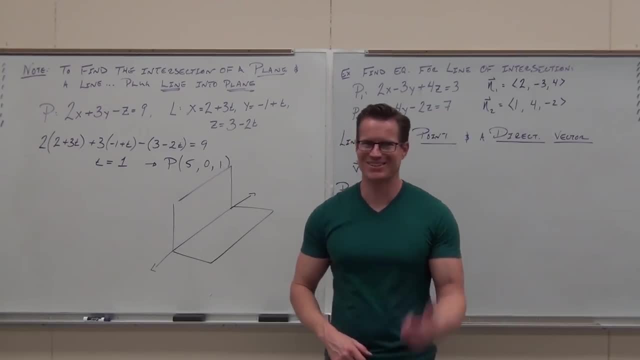 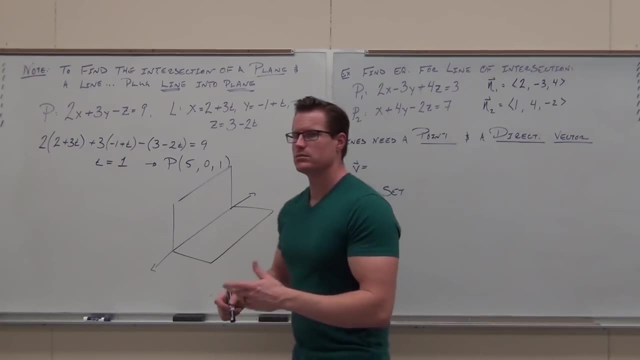 ormol Genius, as all of you. That's exactly right, So good. You are good at this stuff. You are, You are good at this stuff. But they're defined by the normals, The normal vectors. What do normal vectors do with planes? 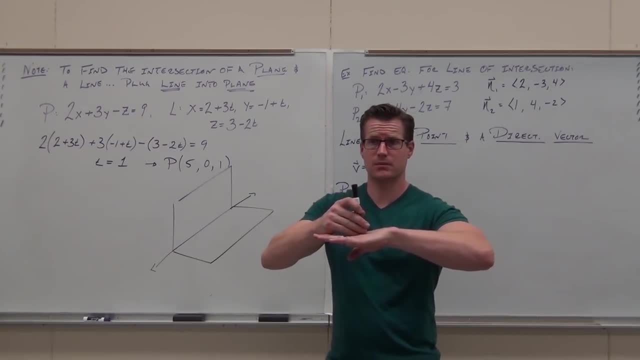 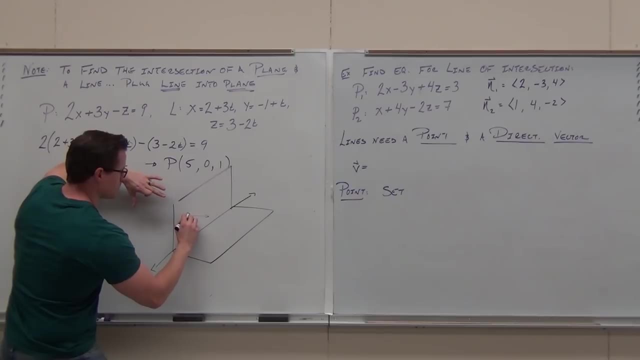 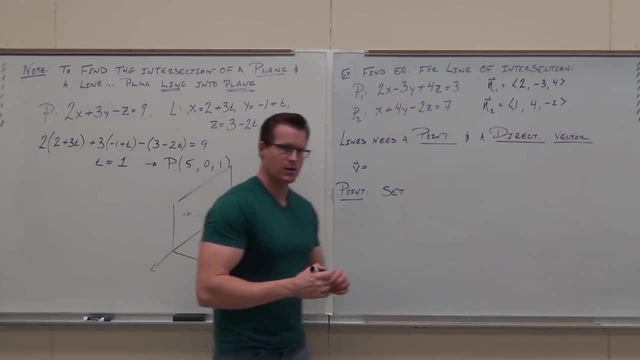 What's the relationship there? Right like that, Which means this normal is coming out, the perpendicular, Correct, And if these are not parallel, this normal coming out the perpendicular, Those vectors are going to meet somewhere, Or the scalar multiples of the vectors. 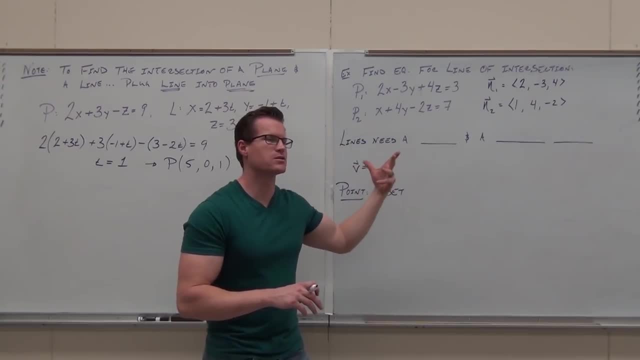 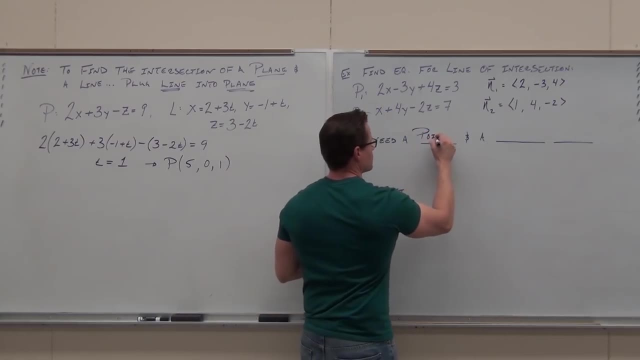 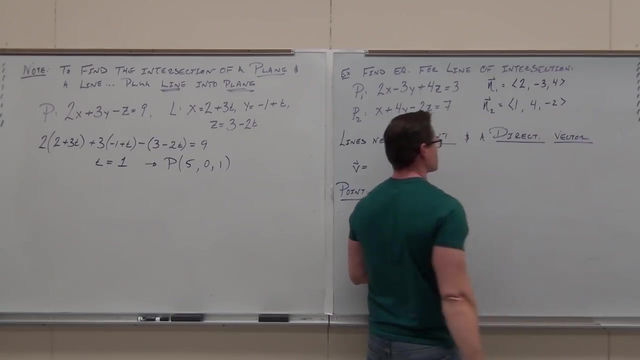 Now let's see. What do lines, lines of intersection even, what do they need? There's two things. lines always need to come on. What do they need? Points, Points, Point. We'll talk about the point last, because you're probably going to think it's more difficult. 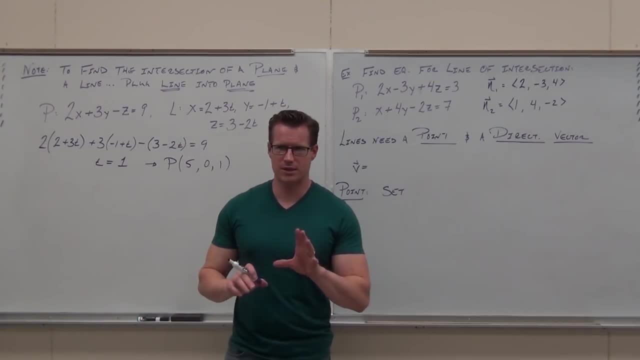 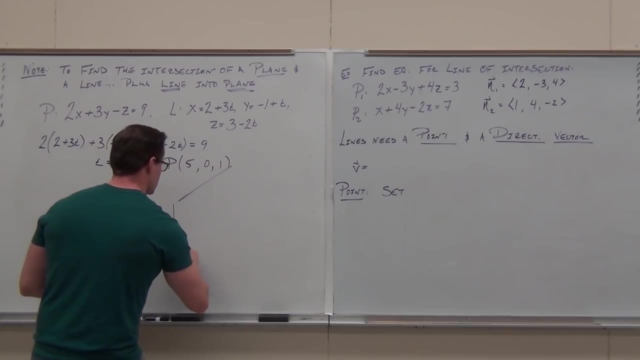 The vector is actually very, very easy. You just need to see it one time and then you'll get it. Check it out. I'm going to draw you a picture over here. Here's a plane. Here's the other plane. 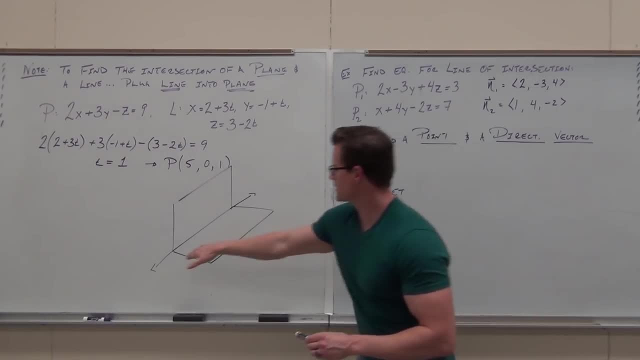 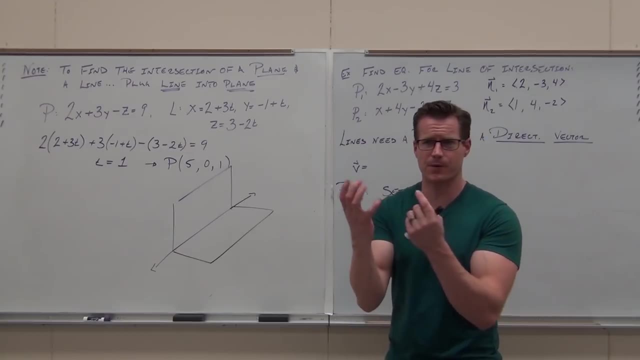 Can you see the line of intersection I'm trying to draw right here? This is the line of intersection. Now we define planes by the. The Starts with an N. Rhymes with or-mal Geniuses, all of you. 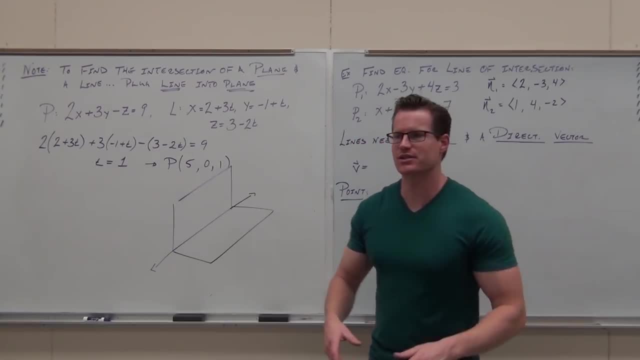 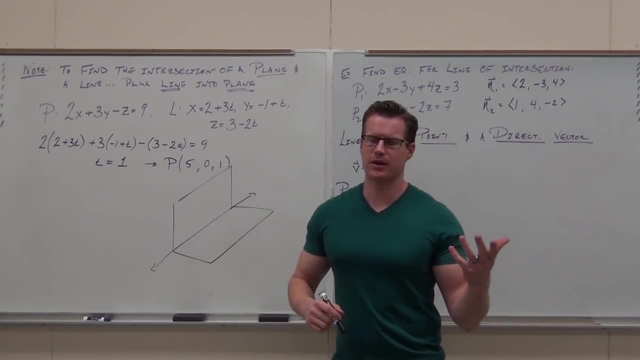 That's exactly right. You're so good at this stuff. You are, You are good at this stuff. But they're defined by the normals. They're normal vectors. What do normal vectors do with planes? What's the relationship there? Right like that. 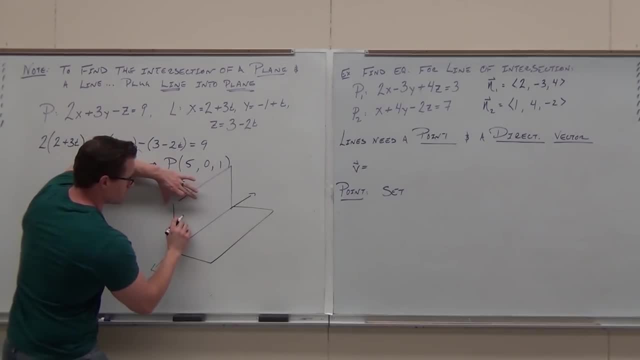 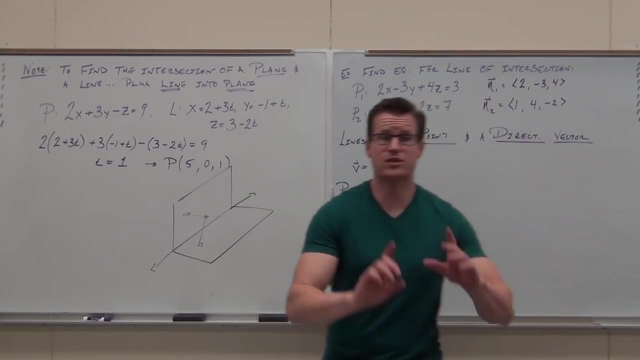 Which means this normal. It's coming out the perpendicular, correct, Yeah Yeah. And if these are not parallel, this also has a normal Coming out the perpendicular: Those vectors are going to meet somewhere, Or the scalar multiples of the vector are going to meet somewhere. 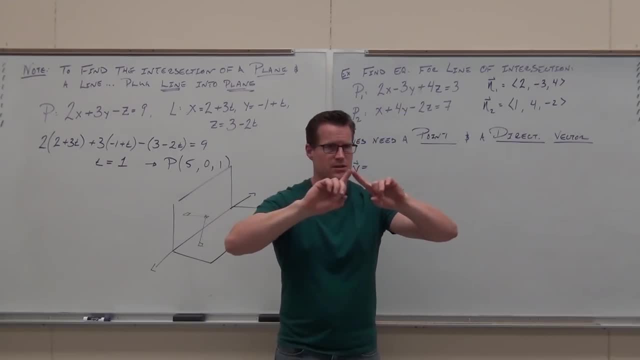 It doesn't really matter if they're scalar multiples. They are going in the same direction. Therefore, they are going to meet somewhere. Two normals of this of these planes are going to meet. Does that make sense? Now, here's the beautiful idea. 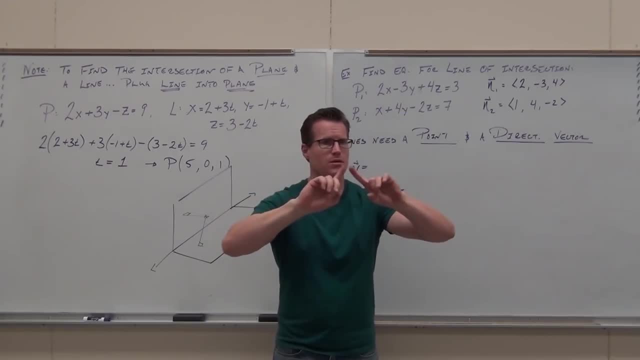 are going to meet somewhere. It doesn't really matter if they're scalar multiples: They are going in the same direction. Therefore, they are going to meet somewhere. Two normals of these planes are going to meet. Does that make sense? Now, here's the beautiful idea. 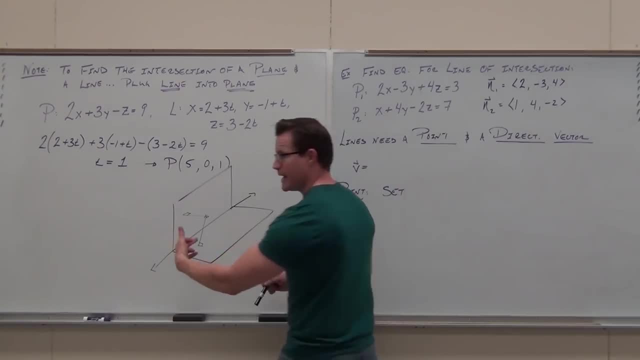 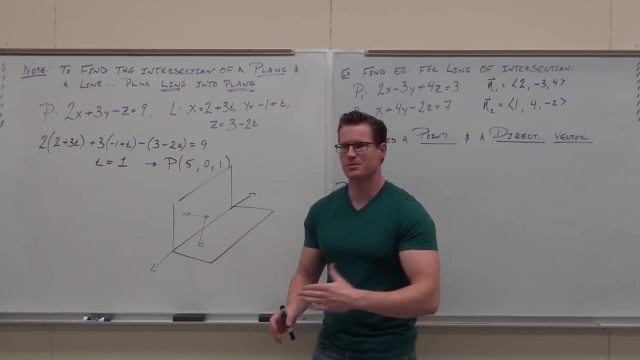 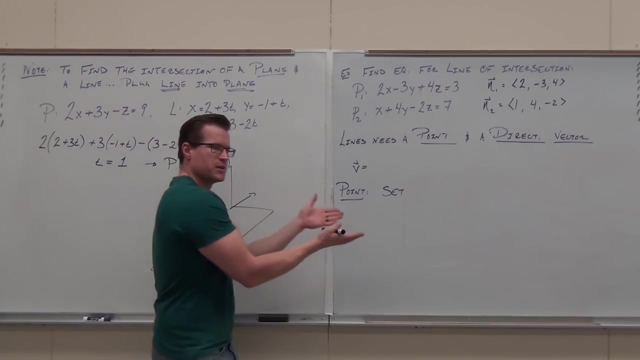 That line, that direction of intersection, has to be orthogonal to both of those normals. Do you see? it Has to be orthogonal to both those normals. So the direction that's going, those planes are meeting Right. They've got normals that are meeting. 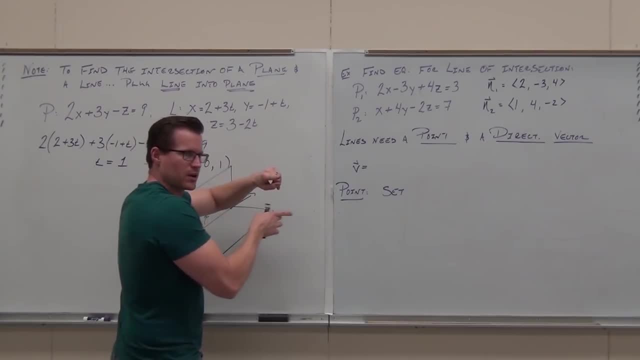 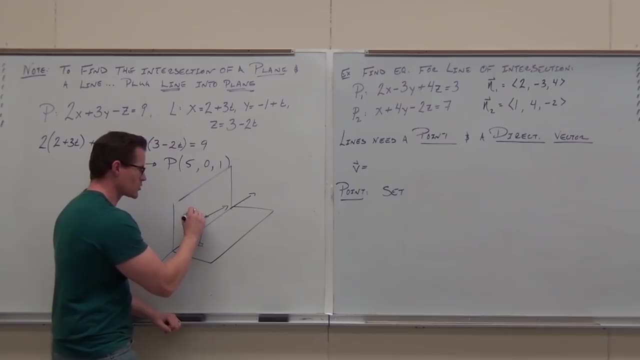 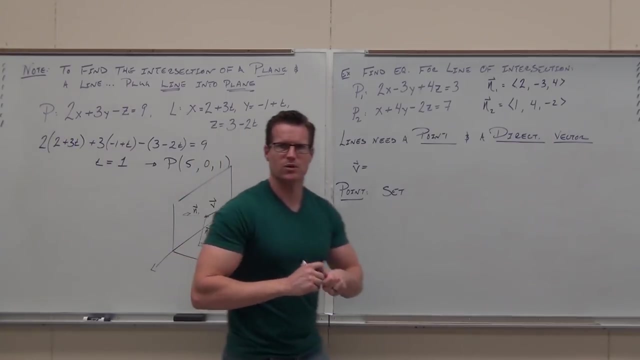 If those planes are like this and the normals are like this, the line is going parallel to whatever is mutually orthogonal to the direction of the normal vectors. How do you find the direction that is mutually orthogonal to two vectors? How do you do it? 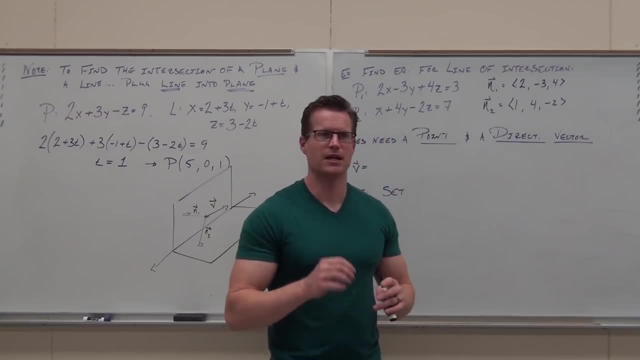 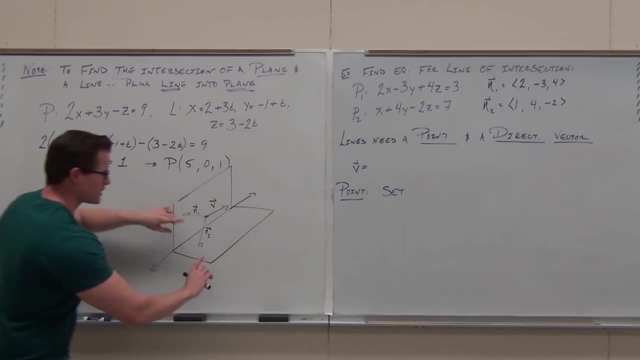 So if you ever want to find the line of intersection or the direction of the line of intersection of two planes, we just have to take our normal vectors, check it out again: Normal one, normal two, they're going to meet. The directional line has to be orthogonal. 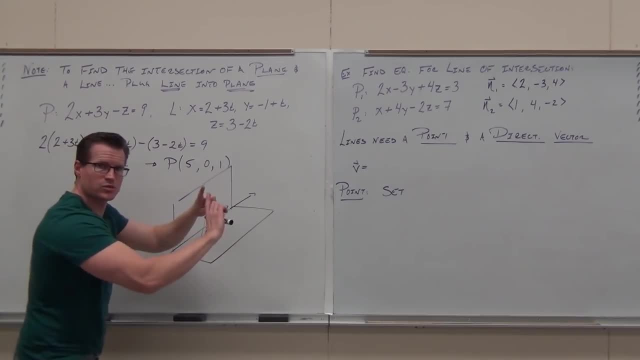 to both of those, Otherwise it would meet and the normals wouldn't make sense anymore. It has to go straight away from it. I need a vector that's in the direction that's mutually orthogonal to both of those vectors, That is, a cross product. 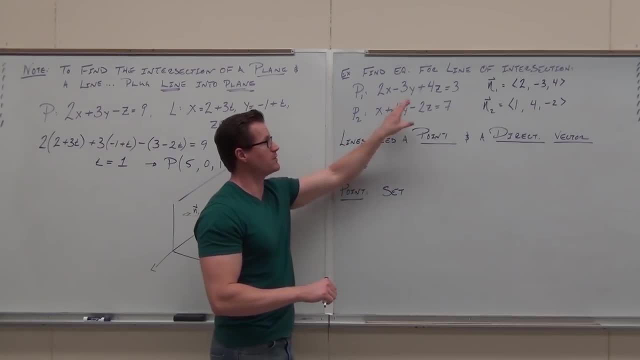 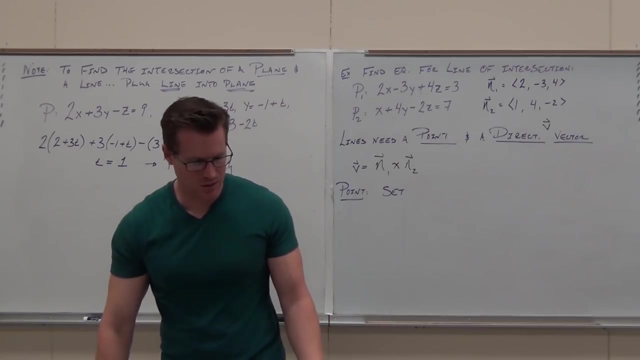 You go: oh, that's sweet. So if I want to find the direction vector of the line of intersection, I take the normals from my two planes and I cross them. Let me ask you something. If I ask you right now to find that hurt when I slammed that down. 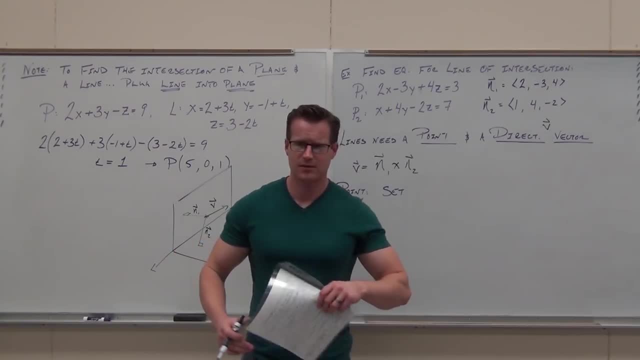 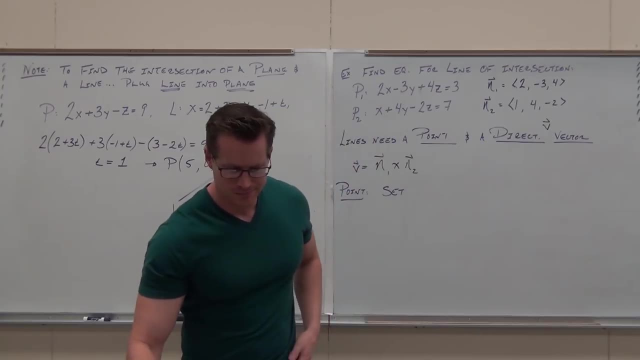 My normal vector made a hurt on my plane. You see that It's like bang It hurt, It's all scarred up. anyway. If I ask you right now to find the cross product, could you do it? Has anyone done it? 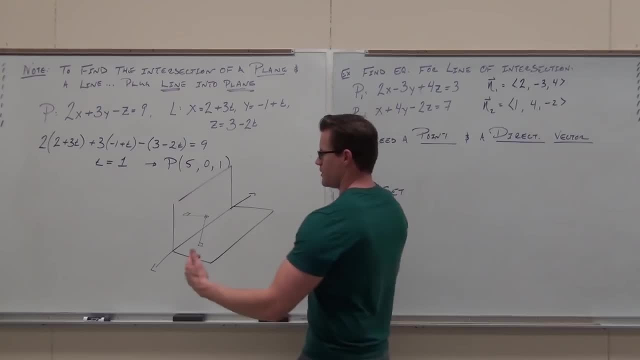 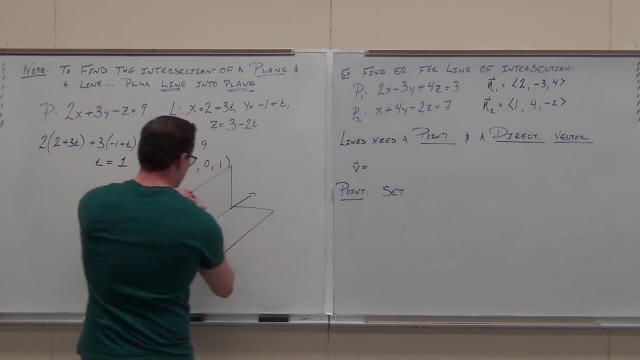 That line, that direction of intersection, has to be orthogonal to both of those normals. Do you see it? It has to be orthogonal to both those normals. So the direction that's going, those planes are meeting right. They've got normals that are meeting. 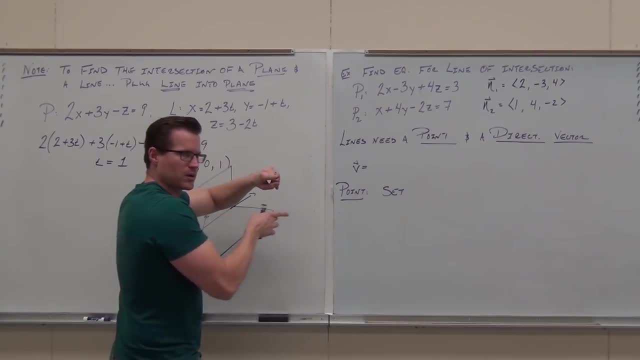 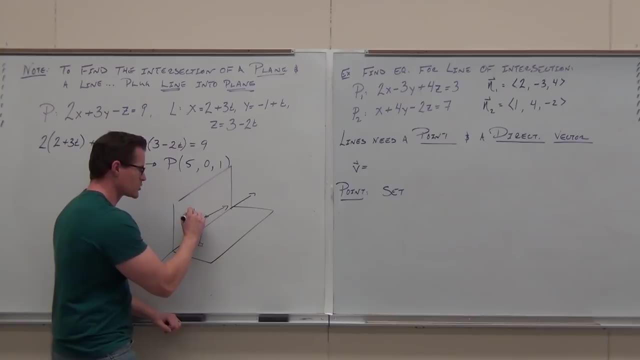 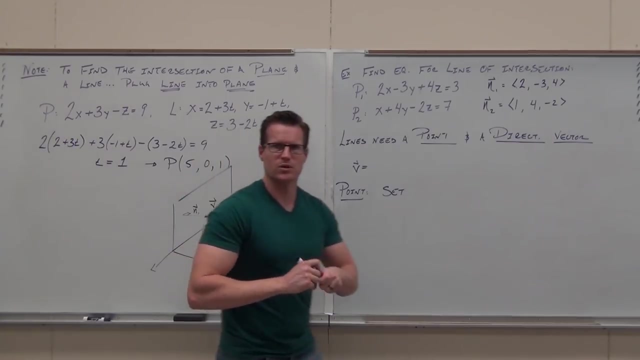 If those planes are like this and the normals are like this, the line is going parallel to whatever is mutually orthogonal to normals. So if you find the line that's going to be orthogonal to the direction of the normal vectors, how do you find the direction that is mutually orthogonal to two vectors? 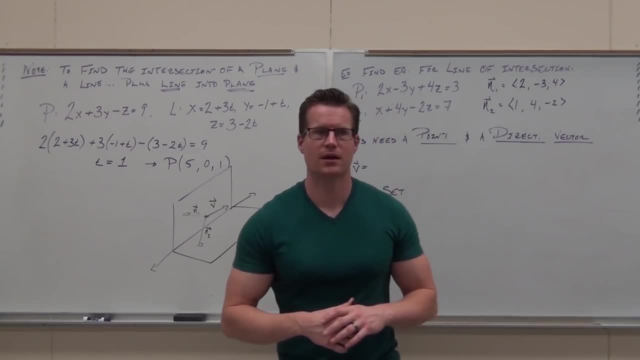 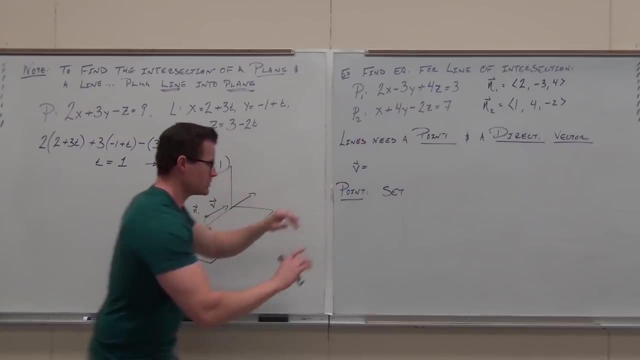 How do you do it? So if you ever want to find the line of intersection or the direction of the line of intersection of two planes, we just have to take our normal vectors, check it out again: Normal one, normal two, they're going to meet. 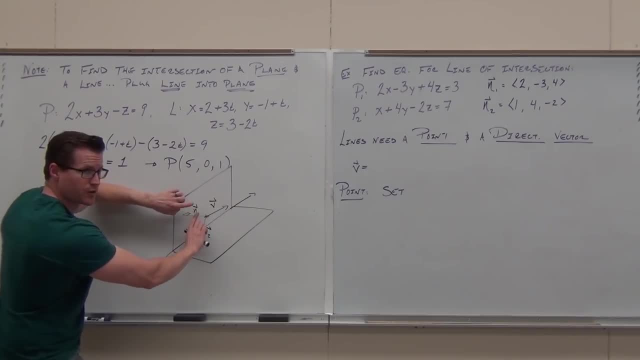 The direction of the line has to be orthogonal to both of those, Otherwise it would meet and the normals wouldn't make sense anymore. It has to go straight away from it, So I need a vector that's in the direction that's mutually orthogonal to both of those vectors. 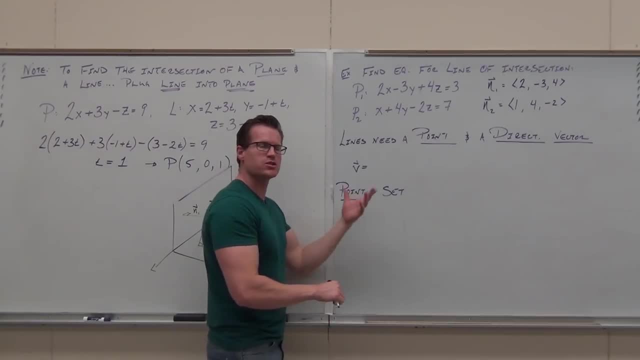 That is a cross product, You go: oh, that's sweet. So if I want to find the direction vector of the line of intersection, I take the normals from my two planes and I cross them. Let me ask you something. If I ask you right now, what would you do? 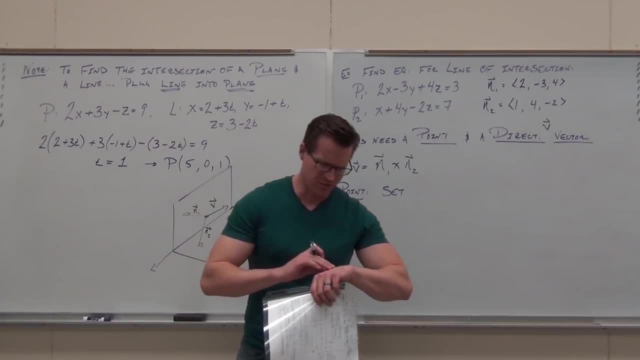 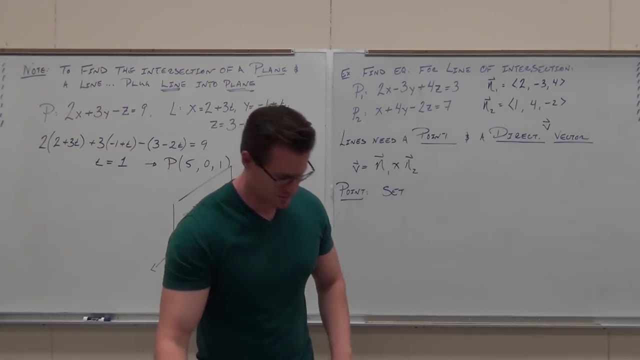 What would you do If I ask you right now to find that hurt? when I slammed it down, My normal vector made a hurt on my plane. You see that It's like bang It hurt. It's all scarred up anyway. 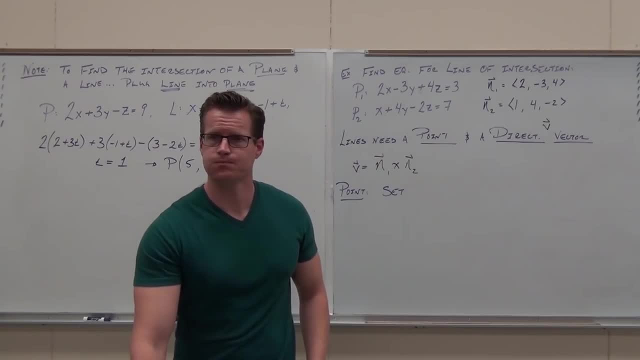 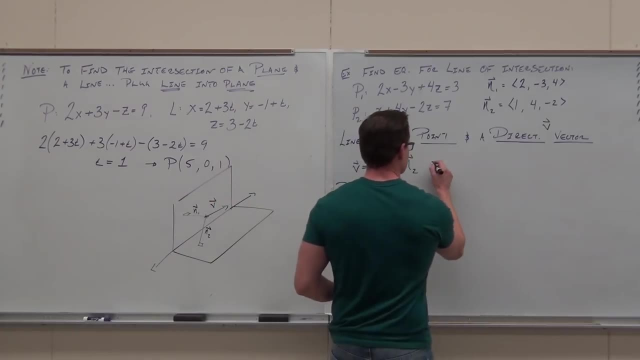 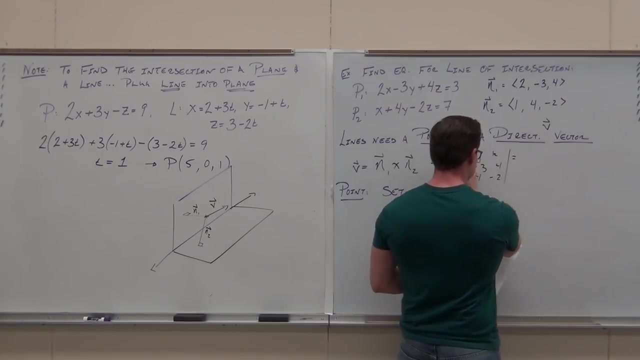 If I ask you right now to find the cross product, could you do it? Yes, Yes, Has anyone done it? Yes, Okay, So you use that one zero. you just now try to find in a like. So. 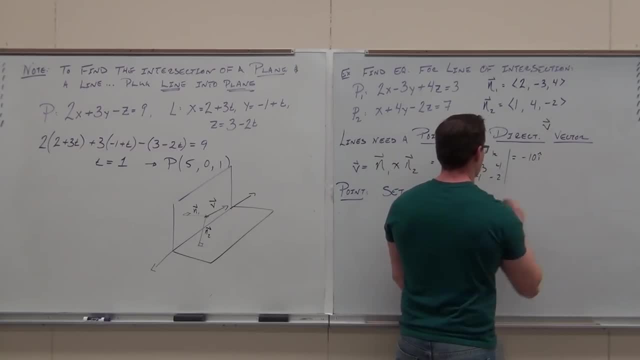 Okay, That's a really good way of finding this. Okay, So yeah, It's easy. Did you see his image there? I'll steal it and give it to him. We've got it now. He'll do it. He'll do it. 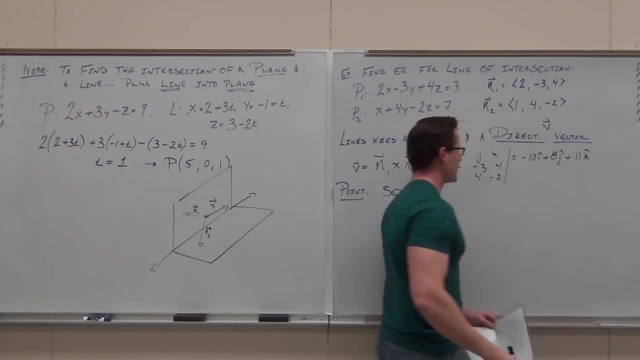 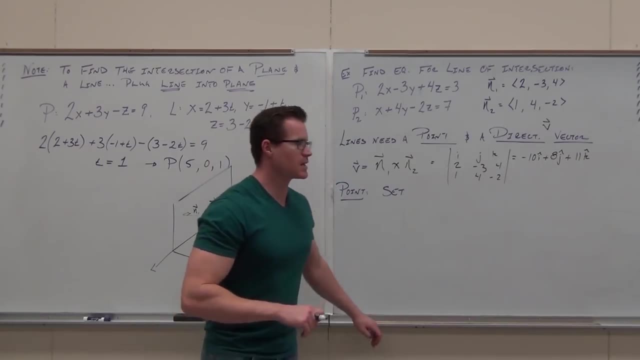 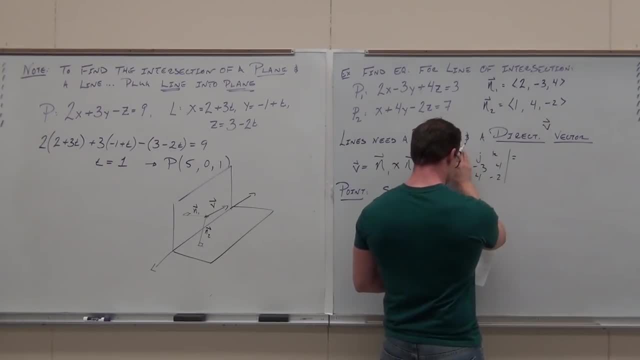 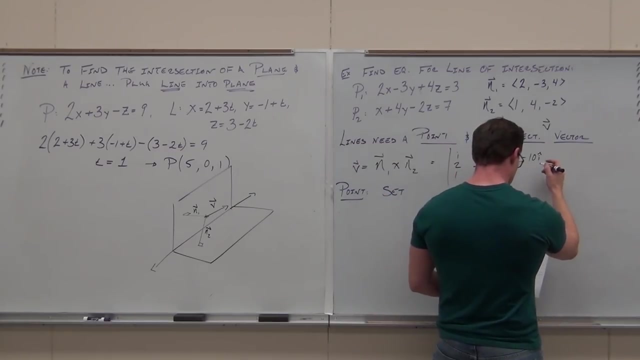 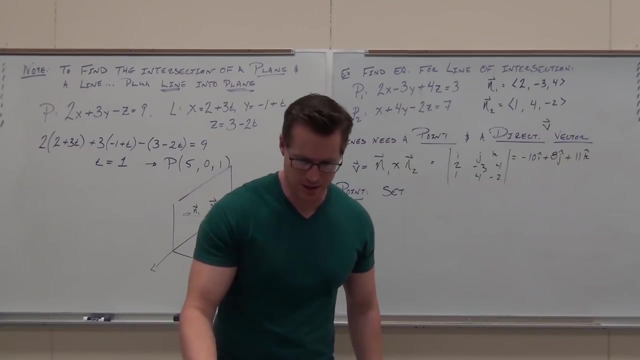 Let me make sure I get that right. I got negative 10i plus 11j plus- sorry- plus 8j plus 11j. Looks like that's what I got here too. Did you guys get the same thing that I got? 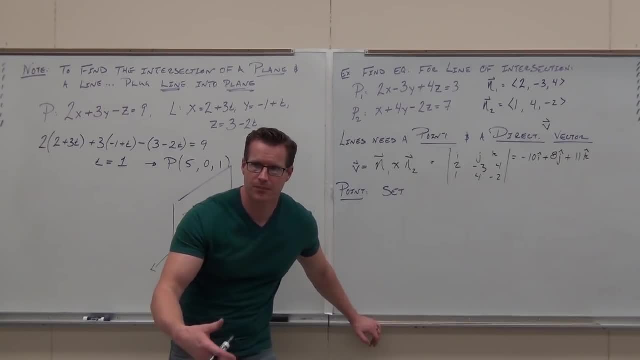 What is it that we just found? The direction vector, The cross product, but it stands for, in this case, the direction vector of our line. Okay, we need two things for a plane: We need a point and a vector, a direction vector. 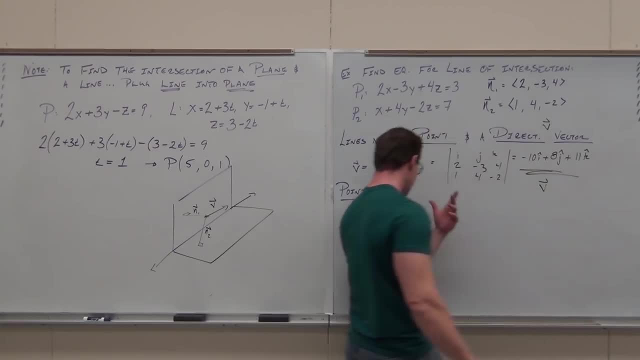 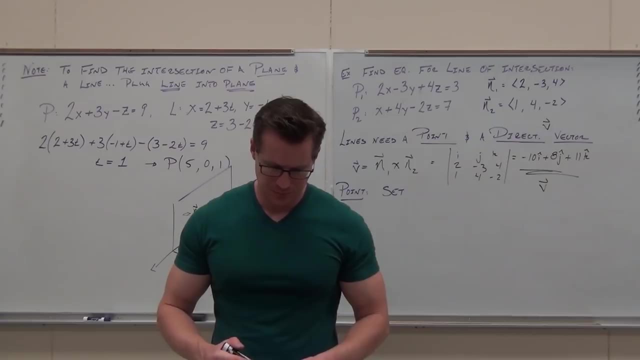 We have that now. This is my v, So that's not bad. Now the point. The point is really interesting. What we do for the point? what we do for the point, set x or y or z, any one that you choose. 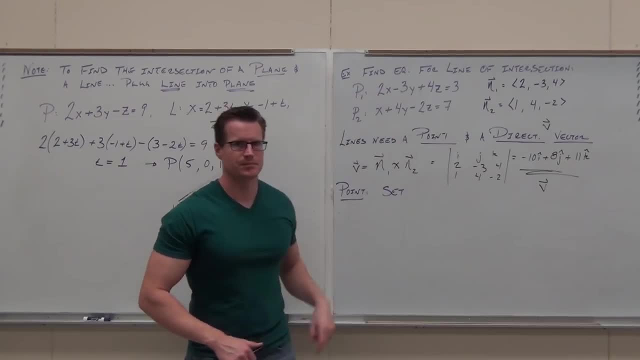 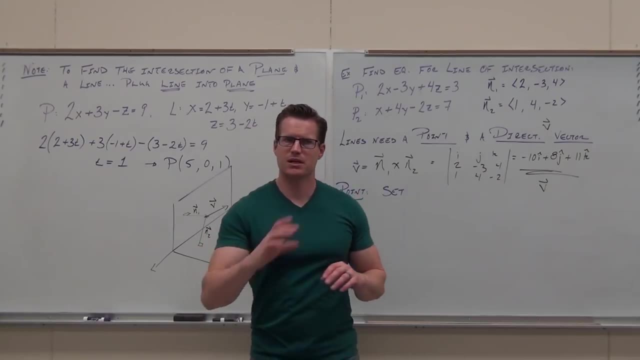 equal to zero in this system. And here's the whole point of this. Here's why it works, because it's not intuitive at first. If you set something equal to zero and you have a system, if you've got a system, that system stands for the intersection. 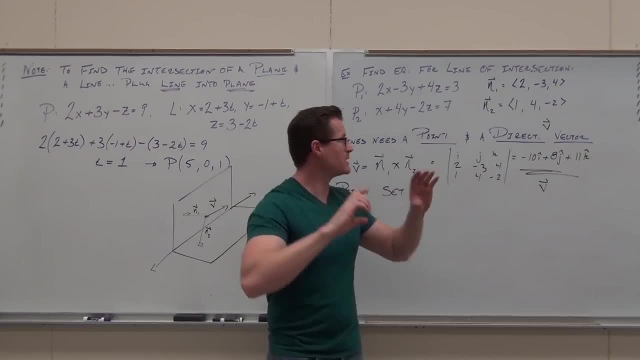 These planes intersect in a line. So if I set something equal to zero in this system, which stands for a line, then what we're going to figure out is where that line crosses the particular plane in space. So if I set y equal to zero, 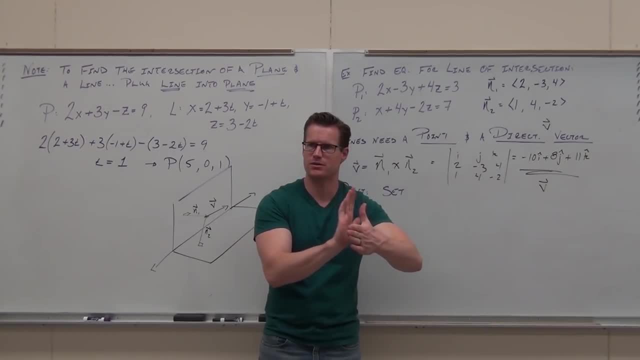 y equal to zero is on the xz plane. Do you guys get it? If I set y equal to zero, I figure out where this system, the line, intersects that plane And that would intersect at a point, And I'm looking for the point. 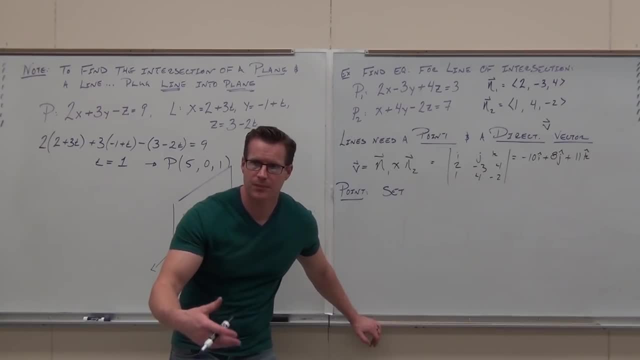 Yes, What is it that we just found? The direction vector Cross product, but it stands for, in this case, the direction vector of our line. Okay, we need two things for a plane: We need a point and a vector, a direction vector. 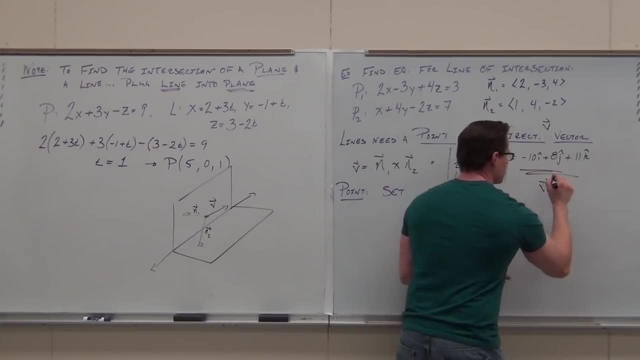 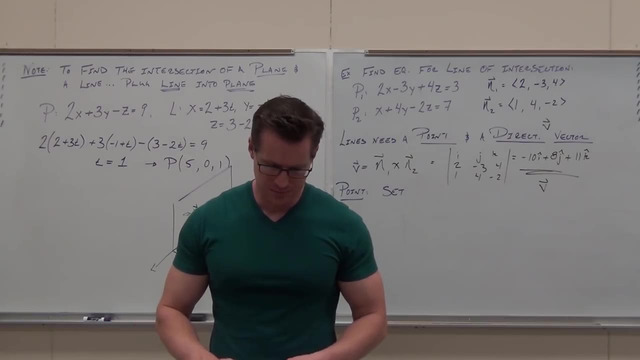 We have that now. This is my v, So that's not bad. Now the point. The point is really interesting. What we do for the point? what we do for the point? set x or y or z- any one that you choose- equal to zero in this system. 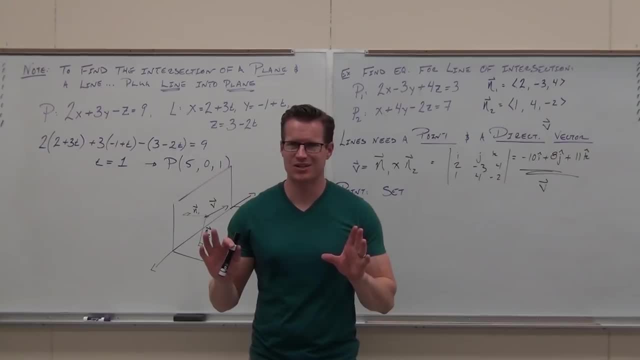 And here's the whole point of this. Here's why it works, because it's not intuitive at first. If you set something equal to zero and you have a system, if you've got a system, that system stands for the intersection. These planes intersect in a line. 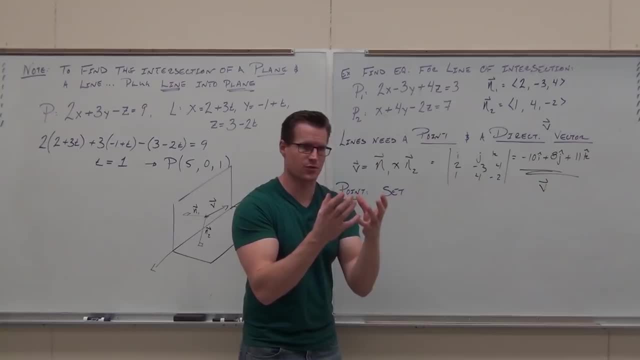 So if I set something equal to zero in this system, which stands for a line, then what we're going to figure out is where that line crosses the particular axis, particular plane in space. So if I set y equal to zero, y equal to zero is: 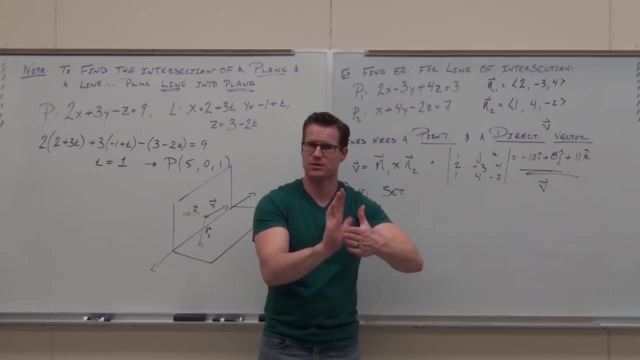 on the xz plane. Do you guys get it? If I set y equal to zero, I figure out where this system, the line, intersects that plane and that would intersect at a point, and I'm looking for the point, Okay. 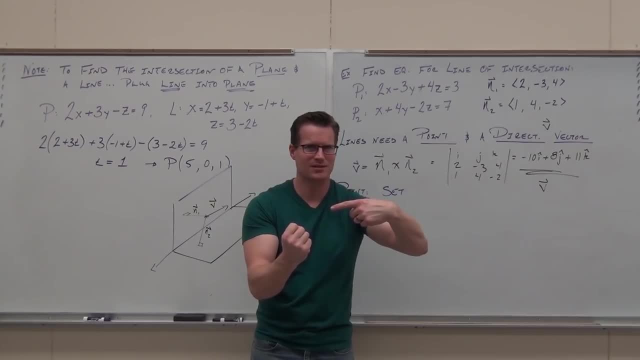 Do you guys get the point? Do you want me to repeat it? Do you understand that where planes meet is a line, So the system is a line? If I set one variable equal to zero, I'm figuring out where the line crosses the plane. 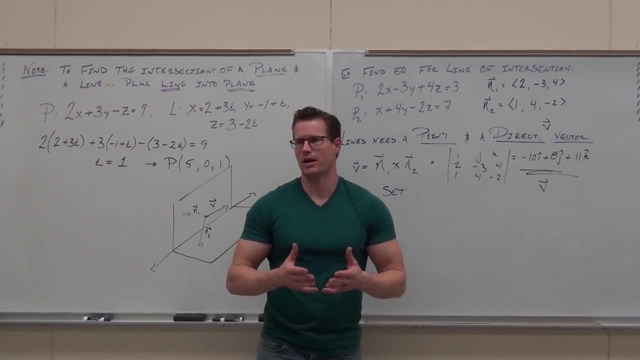 That's it. What plane, It doesn't really matter. So pick y equal to zero. Why, Well, why do I pick y? Because that's nice to deal with and this is not as nice, So I'm picking y equal to zero. 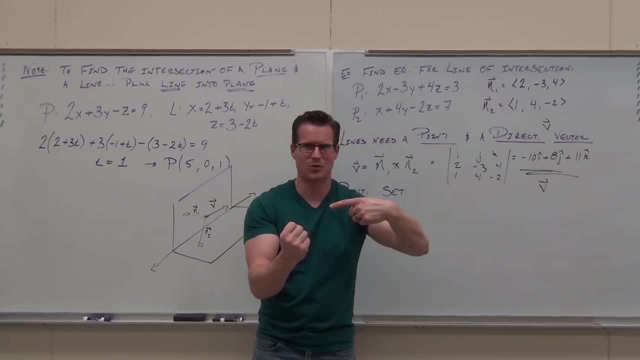 Do you guys get the point? Do you want me to repeat it? Do you understand? Do you understand that where planes meet is a line, So the system is a line. If I set one variable equal to zero, I'm figuring out where the line. 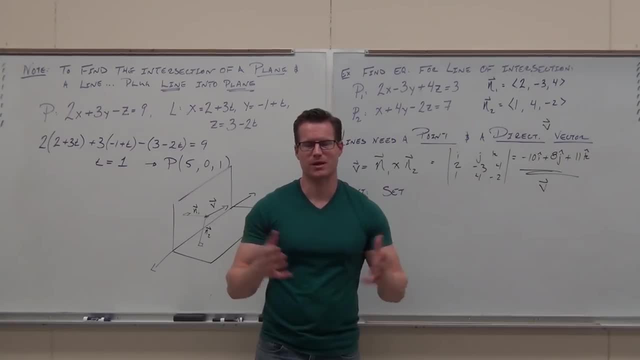 crosses the plane. What plane, It doesn't really matter. So pick y equal to zero. Why? Because that's nice to deal with and this is not as nice. So I'm picking y equal to zero to get rid of that guy. 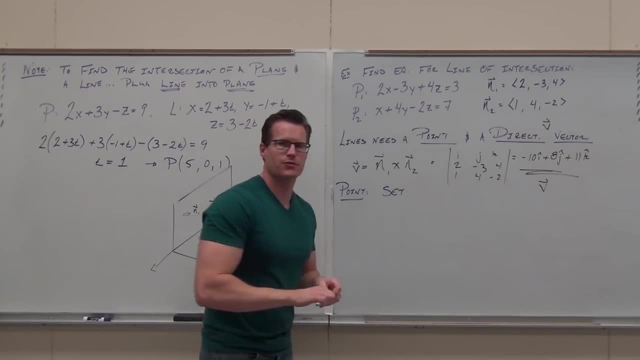 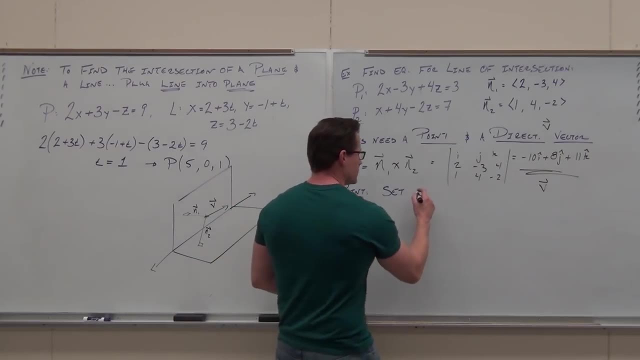 So set y equal to zero or x equal to zero or whichever one you want, Because you'd have a different point for each of the three planes, so you'll get something a little different. It doesn't really matter, You can get different answers here. 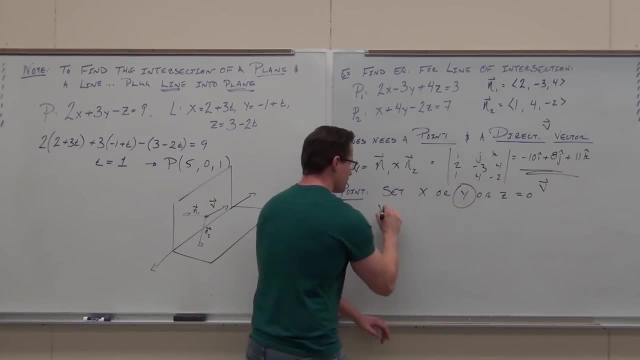 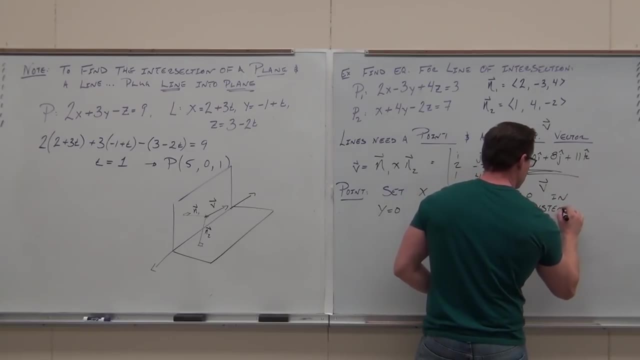 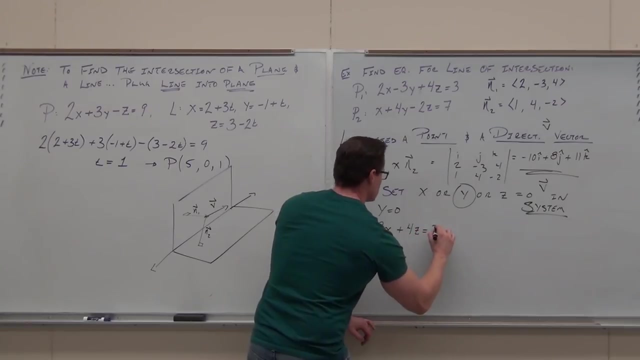 Set x or y or z equal to zero. Me I'm going to pick y In the system. Maybe this will make a little more sense the second time through that I go through it here. Do you know where the y's went? 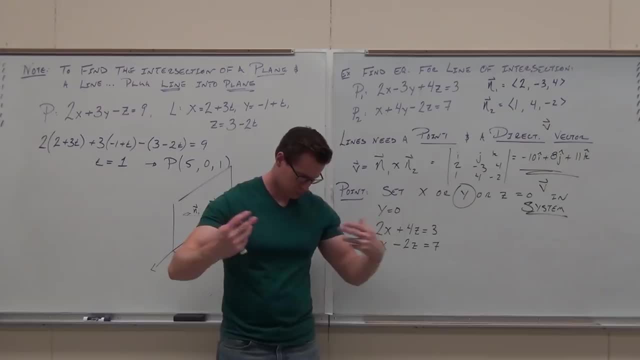 Gone Zeros. What are the only two variables left? x, z. That means it's going to be on the x z plane Where y is zero. you're on the x z plane. We're going to find the point. 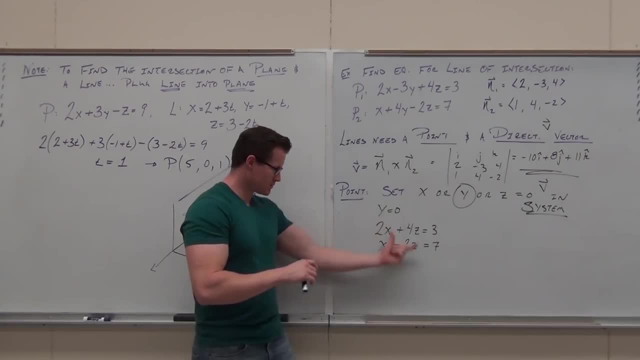 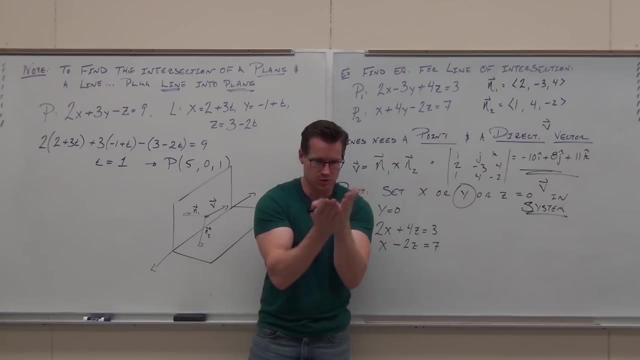 The point is going to be on the x- z plane. You're going to give us a point- x- z. We're going to find the point where this system hits the x- z plane. That's what these variables mean. You've got to know what the variables mean. 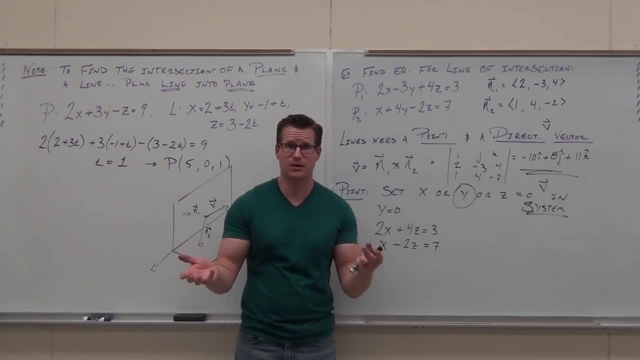 I don't want to just say, hey, this is what you do. I want you to understand it. You guys hopefully now get that when two planes meet, they make a line. If I set one of those variables equal to zero, I'm figuring out where it crosses. 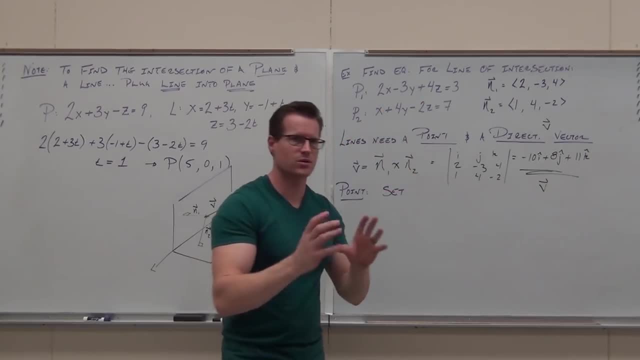 I'm going to pick y equal to zero to get rid of that guy. So set y equal to zero or x equal to zero or z, whichever one you want. It would come out different because you'd have a different point for each of the three planes. 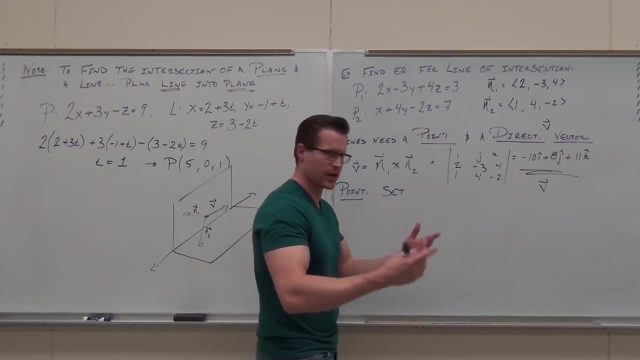 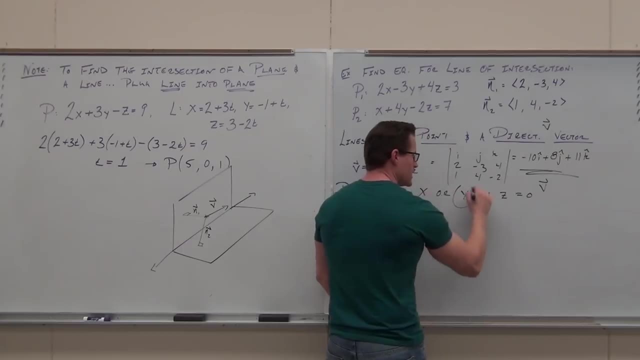 So you'll get something a little different. It doesn't really matter. You can get different answers here. Set x or y or z equal to zero. Me, I'm going to pick y in the system, So I'm going to pick y. 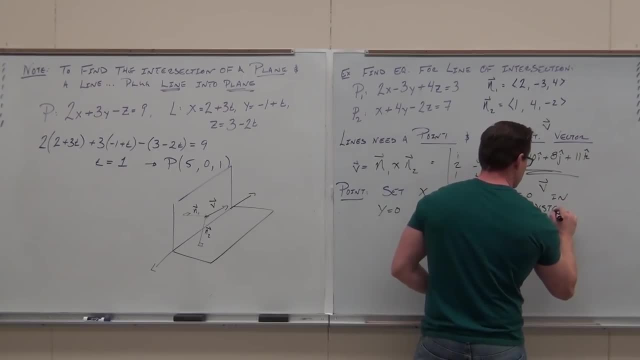 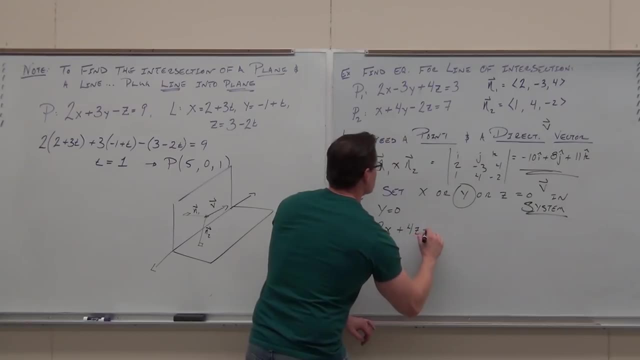 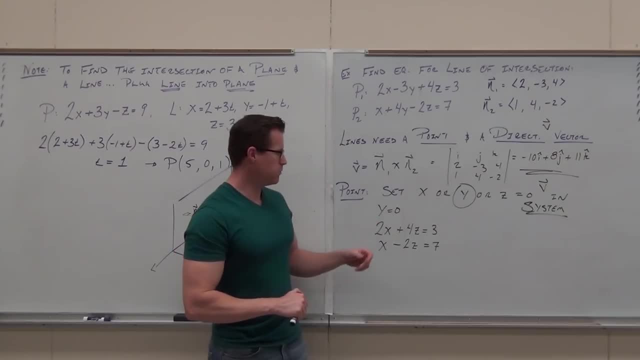 through that. I go through it here. Do you know where the y's went? Gone Zeros, What are the only two variables left? That means it's going to be on the XZ plane where Y is 0,. you're on the XZ plane. 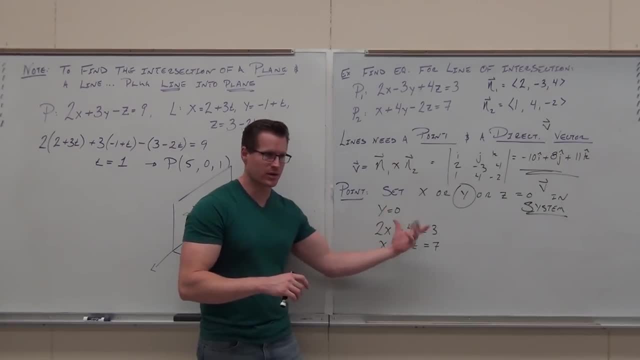 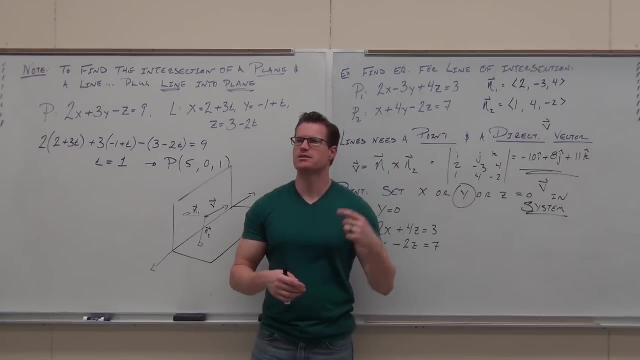 We're going to find the point. The point is going to give us a point: XZ. We're going to find the point where this system- the line of intersection of two planes- hits the XZ plane. That's what these variables mean. 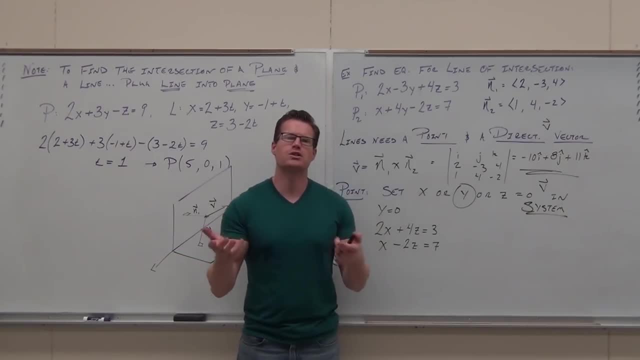 You've got to know what the variables mean. I don't want to just hey, this is what you do. I want you to understand it. You guys hopefully now get that when two planes meet, they make a line. If I set the system which is a line, the intersection. 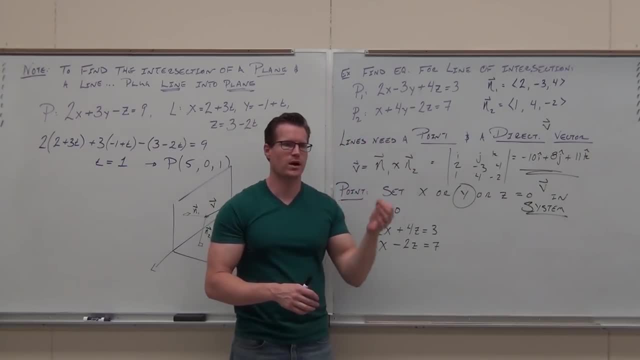 of the system. that's a line. if I set one of those variables equal to 0, I'm figuring out where it crosses the plane of the variables I'm left with. In this case, you go okay. well, I'd probably multiply this by 2.. 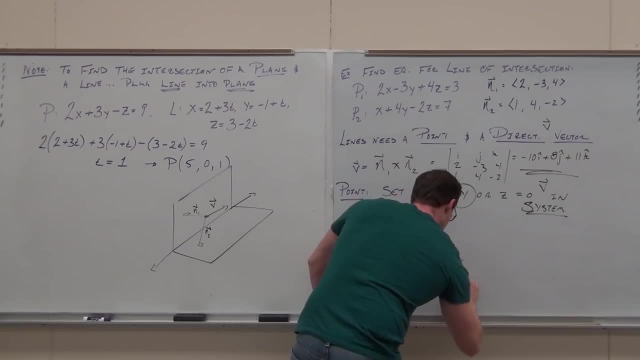 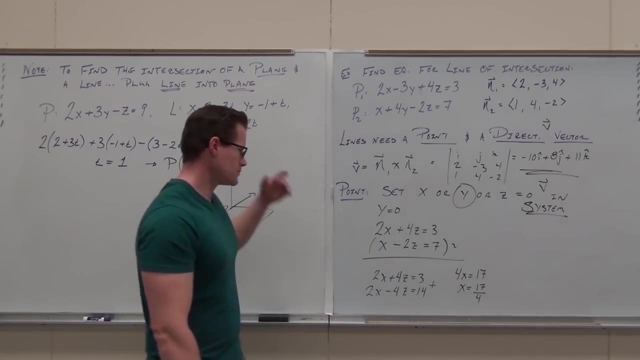 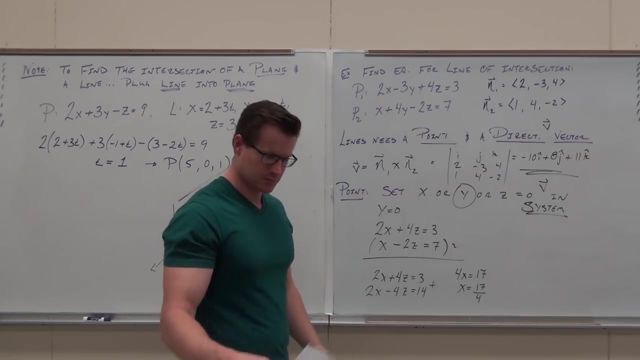 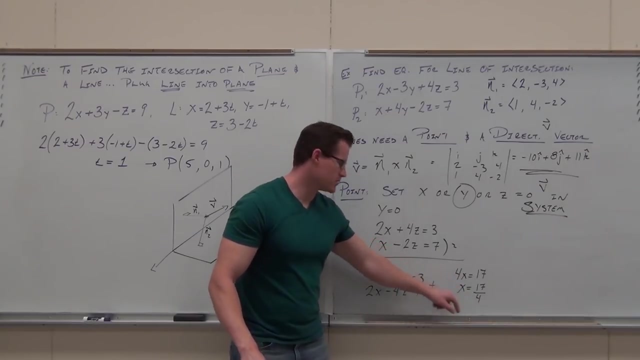 I think I'd add them. I'm not going to show you the rest of the work, but to find the rest of the work, we just take that value, plug it into either one of these equations here and you can solve for your Z, Are you guys okay? 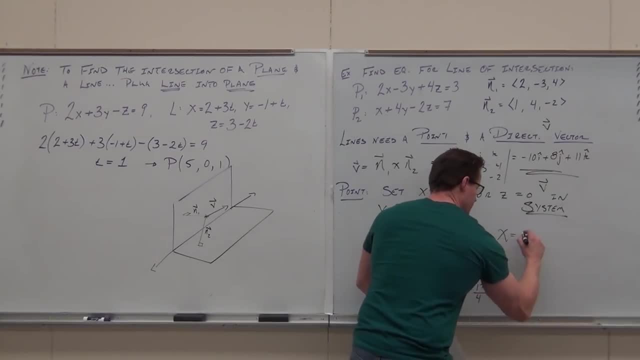 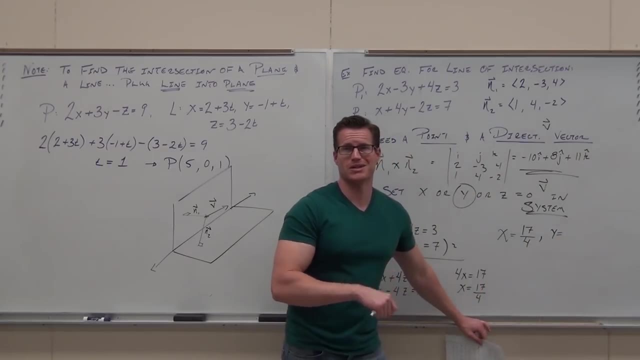 with what I'm talking about, Your X, I'm going to rewrite it. Oh, now let me think about it. What would the Y be Zero? Well, I've set it equal to and Z if you substitute it in. 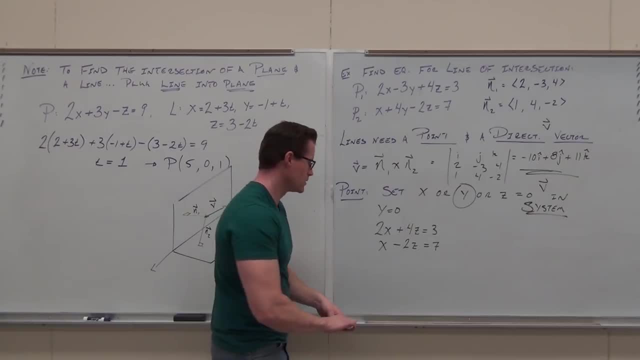 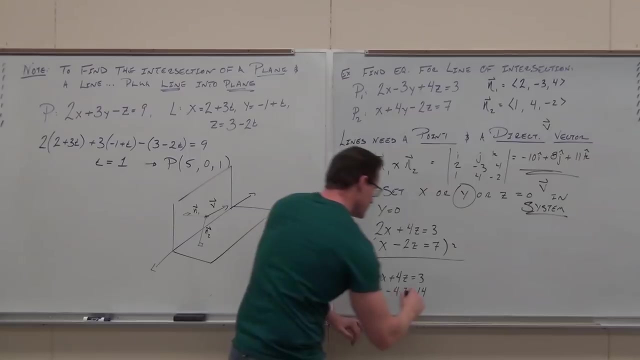 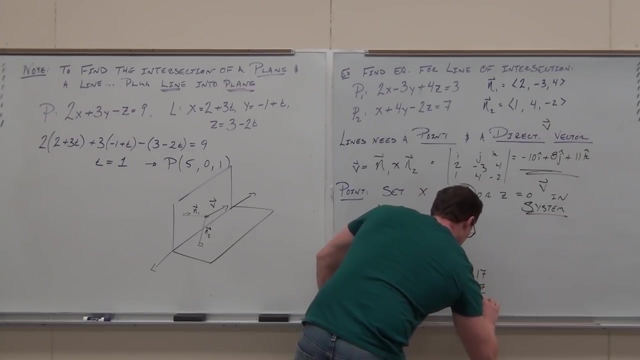 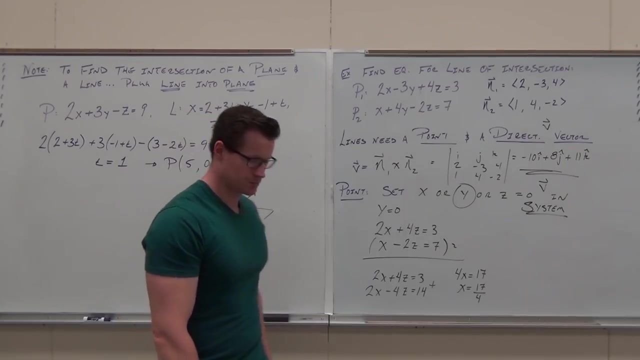 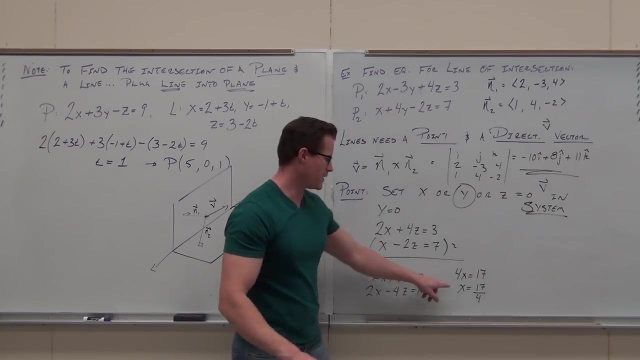 the plane of the variables I'm left with. I'm going to multiply this by two, I think I add them. I'm not going to show you the rest of the work, but to find the rest of the work, we just take that value. 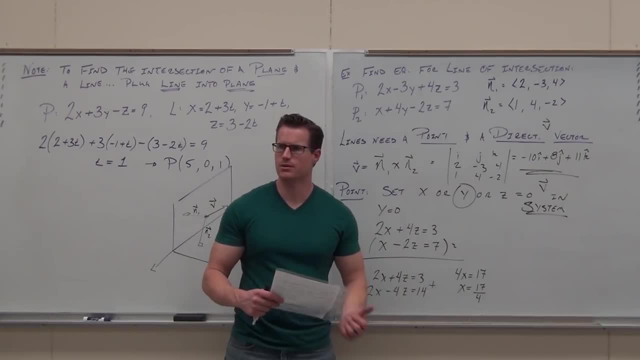 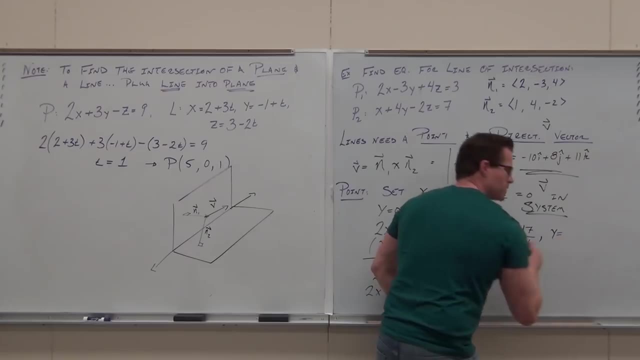 plug it into either one of these equations here and you can solve for your z. Are you guys okay with what I'm talking about? Your x, I'm going to rewrite it. Oh, now let me think about it. What would the y be? 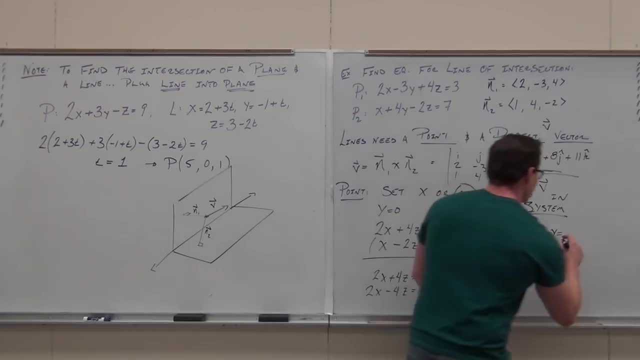 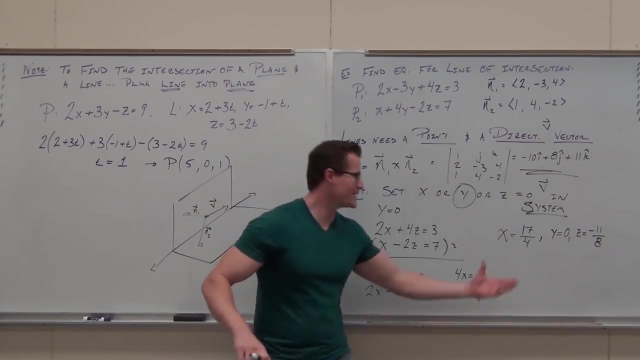 Zero. Well, I've set it equal to And z. if you substitute, in which I want you to try on your own at some point, is negative 11 over 8.. What is that? It's a point. What particular point? 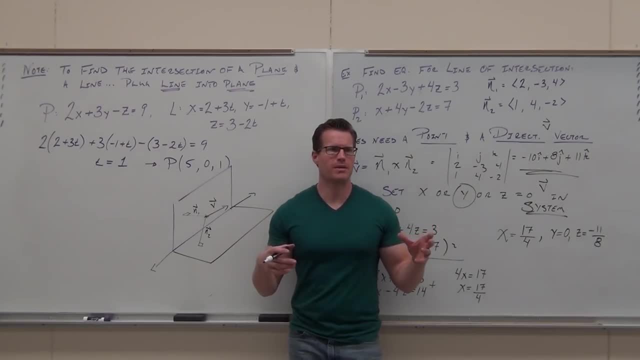 Listen. we just need, please listen, this wasn't supposed to be magic, We just needed any point on that line. Does that make sense? Any point would do. How do you find it? How do you find a plane? Because that's the easiest thing to do right now. 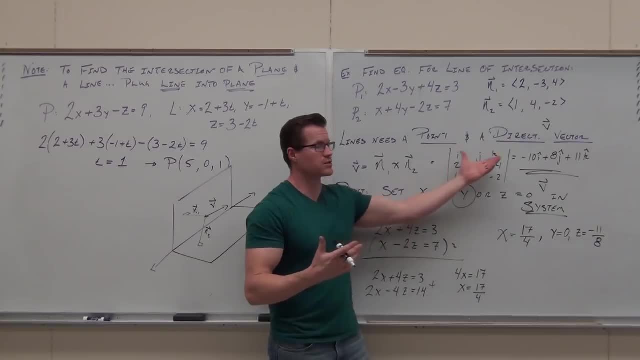 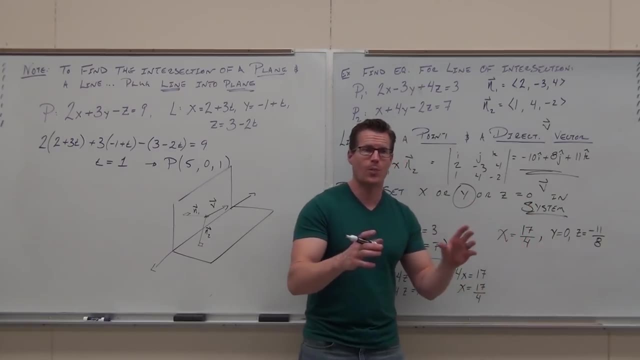 How are you supposed to find a point if you don't know where it crosses anything? All we knew was a vector in the direction. We didn't have a point. So we have to use this sort of system idea to find at least some point. 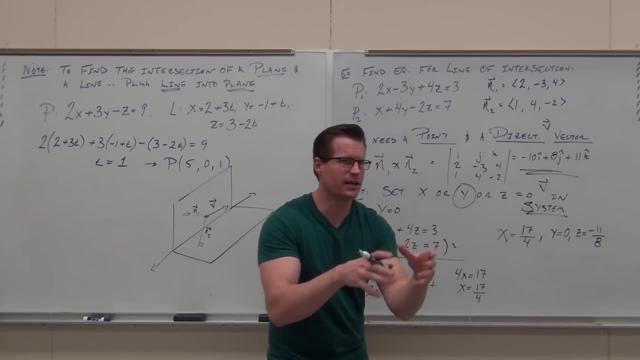 Now do we have a point and a vector. What are we trying to find? again, An equation of a plane or an equation of a line? Let's use the appropriate thing. This is very easy. Let's plug it into a plane. 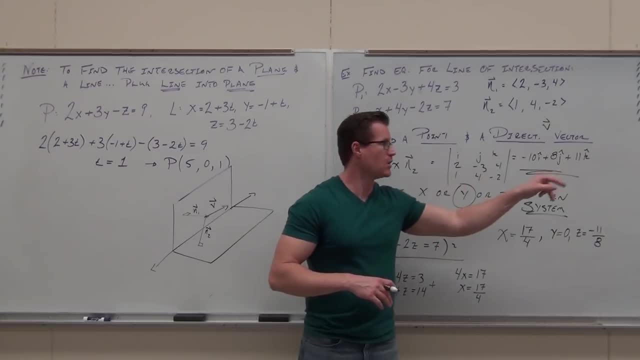 We're not finding a plane folks. We have a direction vector. We've got a point now that it for sure travels through. If we have the line, the line will take the x coordinate. you can call them x sub zeros if you want. 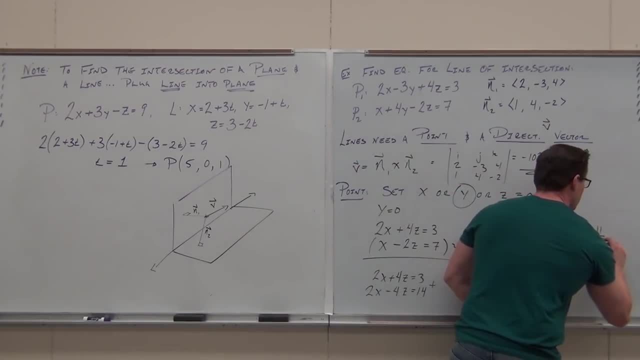 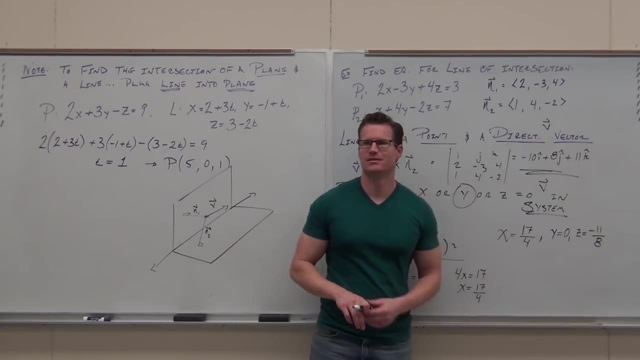 which I want you to try on your own at some point, is negative: 11 over 8.. What is that? It's a point, What particular point? Listen, we just need please listen. This wasn't supposed to be magic. 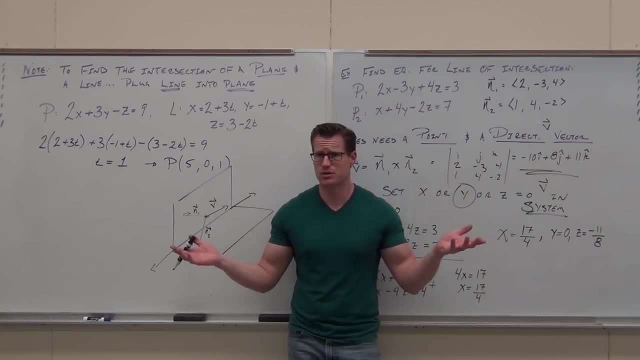 We just needed any point, Any point on that line. Does that make sense? Any point would do. How do you find it? Well, we just wanted to find the point where it crosses a plane, because that's the easiest thing to do right now. 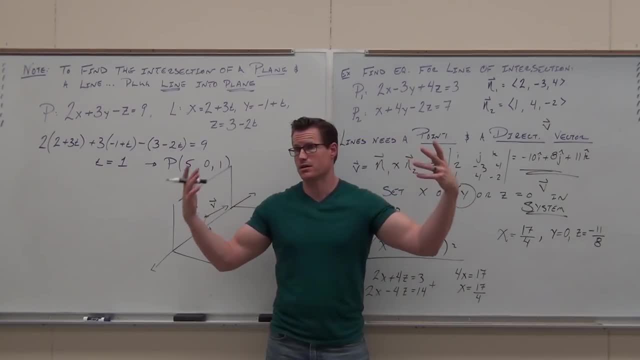 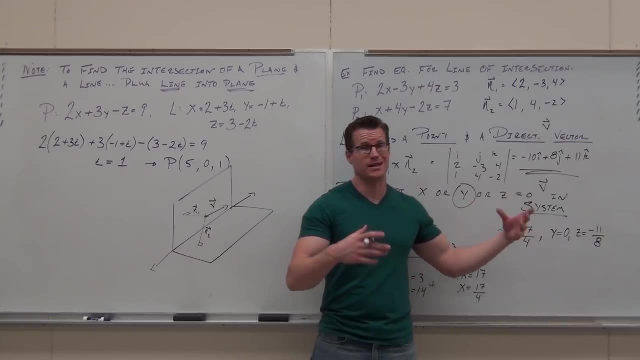 How are you supposed to find a point if you don't know where it crosses anything? All we knew was a vector in the direction. We didn't have a point. so we have to use this sort of system idea to find at least some point. 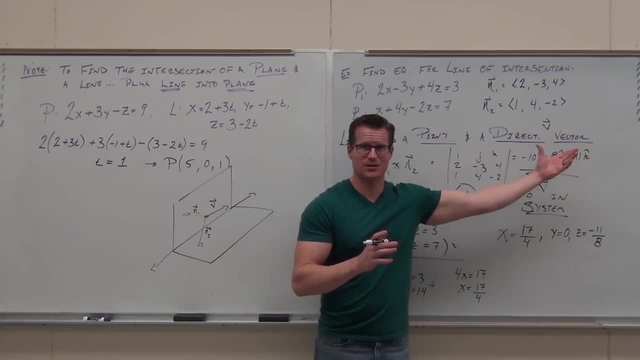 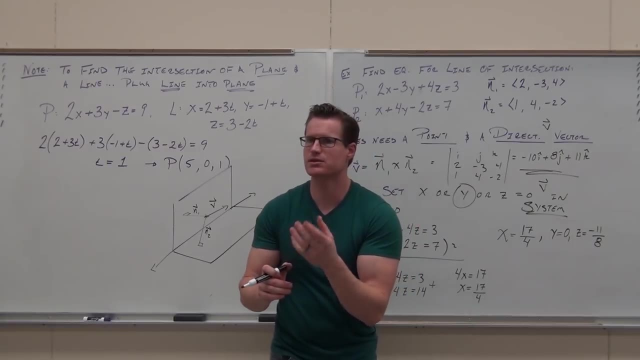 Now do we have a point and a vector. What are we trying to find again? An equation of a plane or an equation of a line? A equation? Let's use the appropriate thing. okay, This is very easy. I talked about it last time. 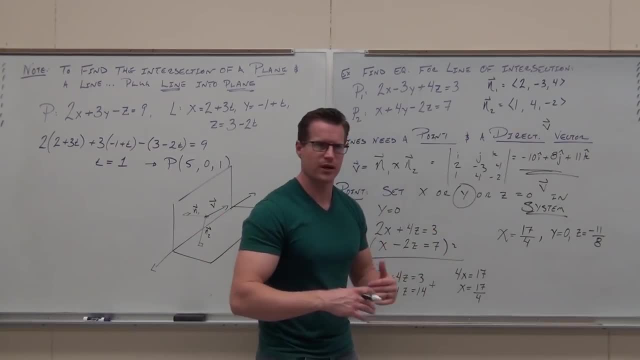 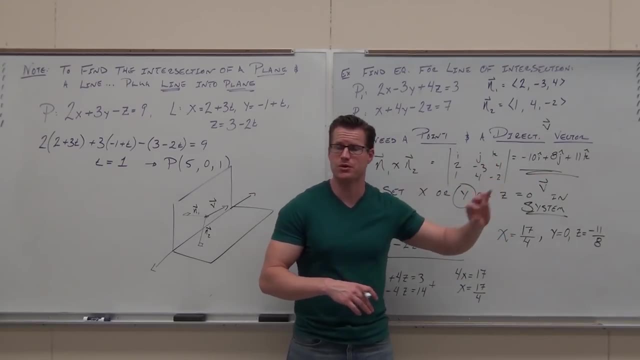 To get confused between these things. you go: oh, that's going to be a plane. We're not finding a plane, folks. We have a direction vector, a direction. We've got a point now that it for sure travels through. 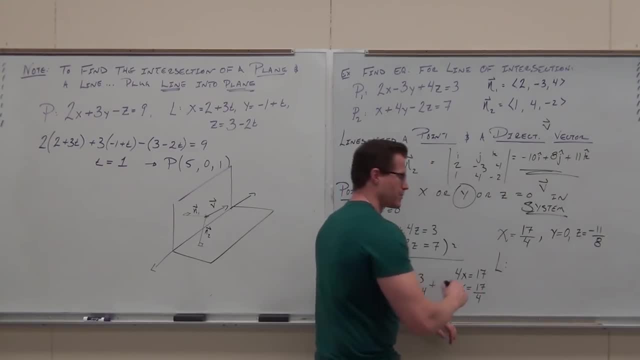 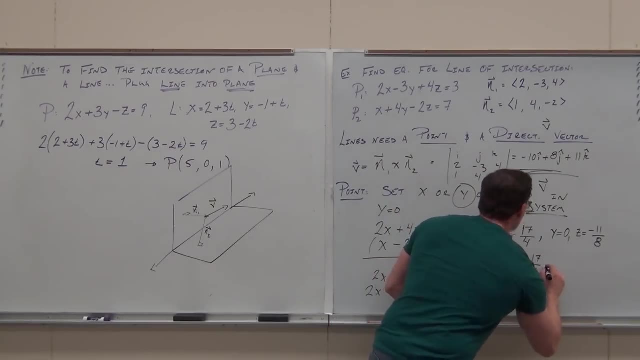 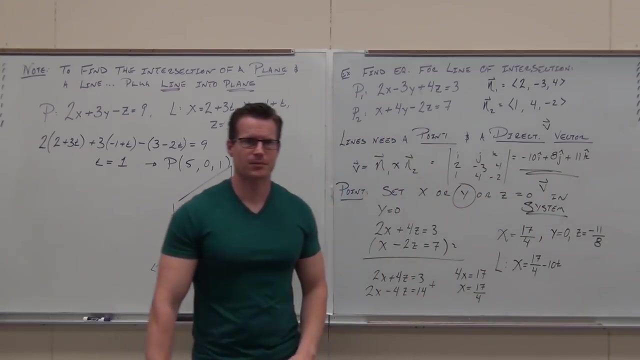 If we have the line, the line will take the x coordinate. You can call them x sub zeros if you want. It will take the direction vector And we'll match them together: x coordinate, x component of the direction vector. That's how the lines work. 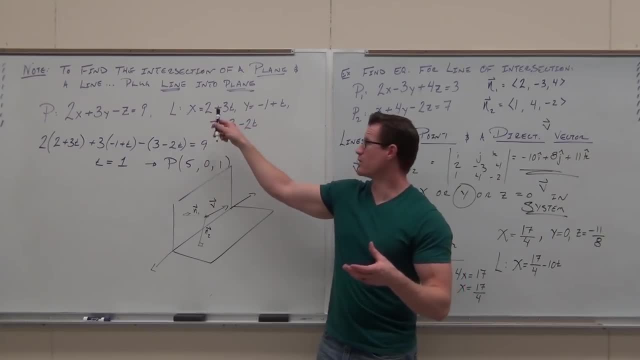 Do you remember the equation of the lines? They look like this stuff right Where. this is your point: x, y, z. This is your direction vector: x, y, z. It's how we made them. Tell me what the y would look like, please. 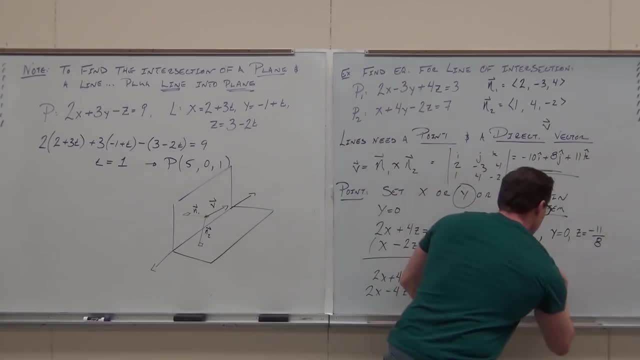 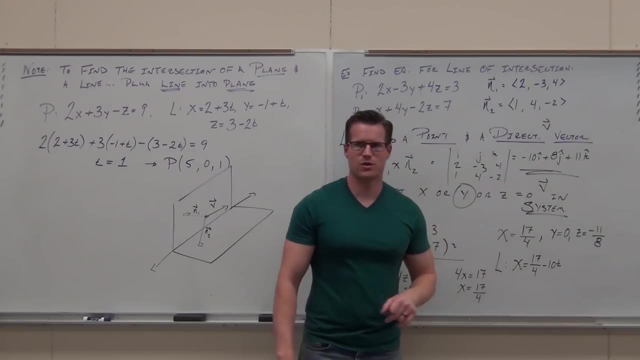 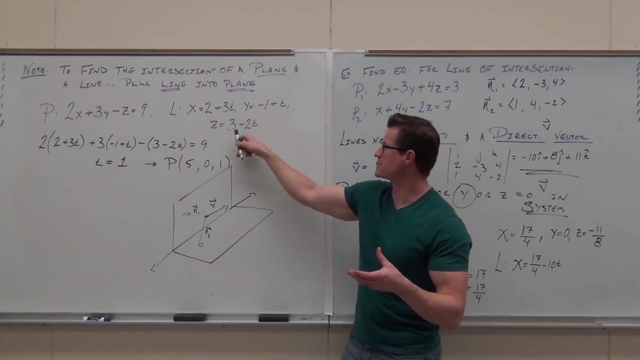 It will take the direction vector and it will match them together. x coordinate the component of the direction vector. that's how the lines work. Do you remember the equation of the lines? They look like this stuff, right Where this is your point: x, y, z. 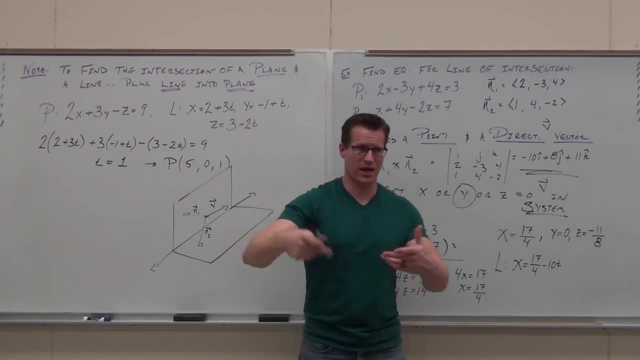 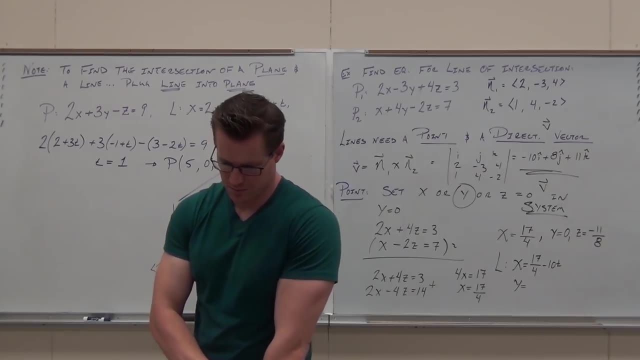 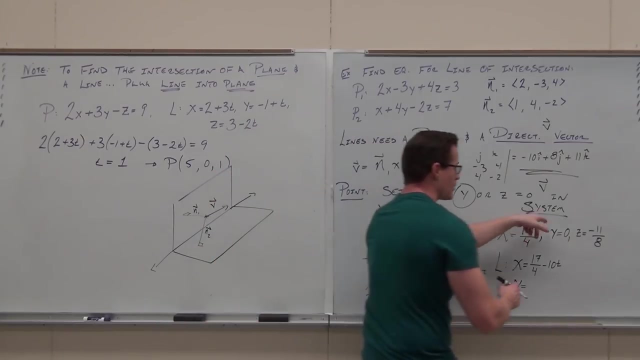 This is your direction. vector x, y, z. It's how we made them. Tell me what the y would look like. please Tell me what the y would look like. Why doesn't it have an actual constant up there? Why doesn't it have that? 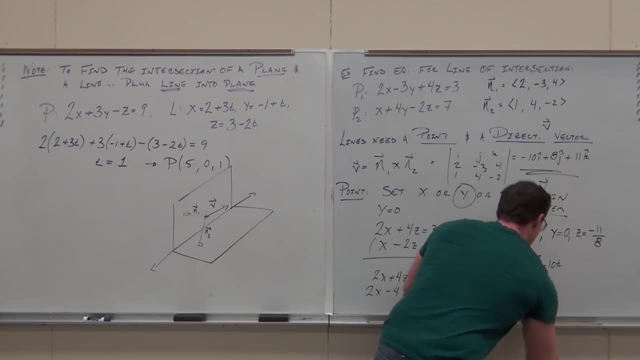 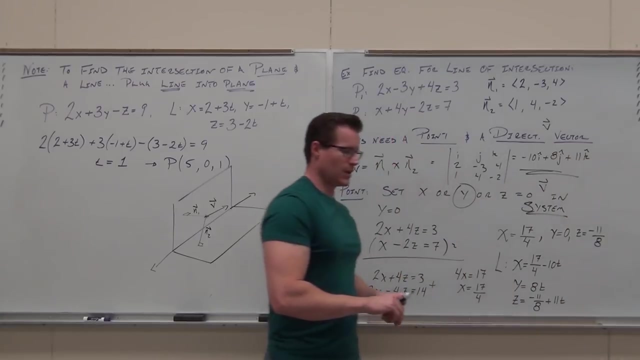 Because we have zero And z. if you want to do that one, what does z start with? Come on quickly. what does z start with? Negative Plus or minus Plus? It's pretty interesting. These planes are going to meet somewhere in space. 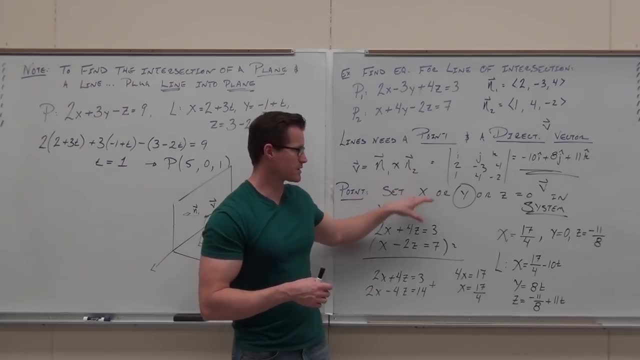 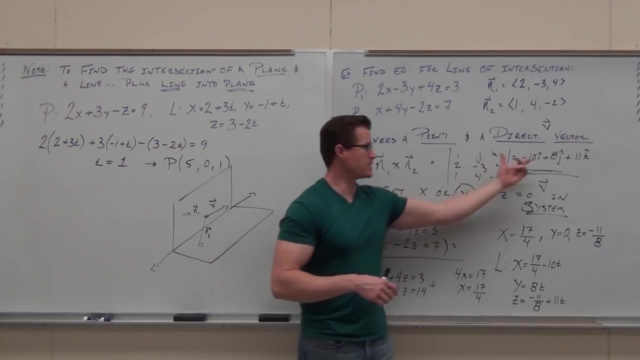 Their meeting is going to be a line. I know that line because I did this system is going to travel through that point on the xz plane. That point and the direction vector which is mutually orthogonal to our normals. we now have an equation of that line. 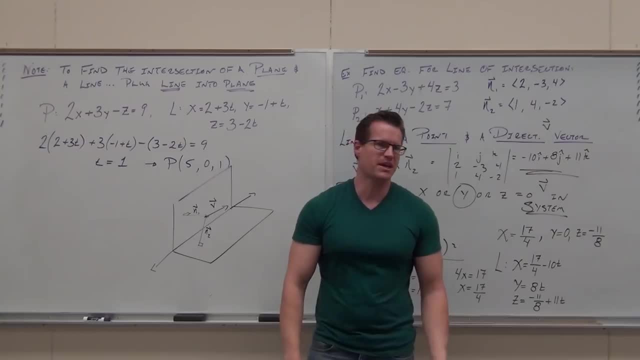 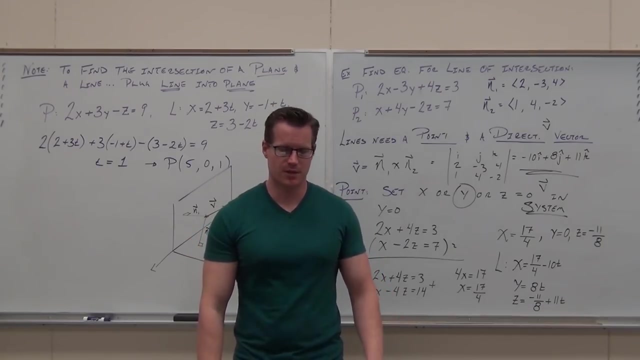 That's pretty cool. We just found out the line that these planes make Pretty neato, Neato, Real neato. I don't care What's it mean to me It's pretty neat if you need to do this stuff on some other topics. 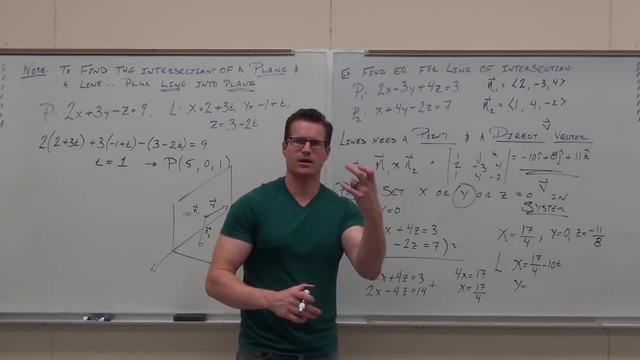 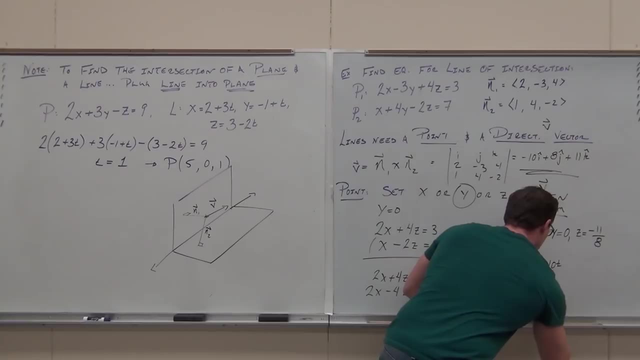 Tell me what the y would look like. Why doesn't it have an actual like constant up there? Why doesn't it have that? Because we have zero, so zero plus 18.. And z. if you want to do that one, what's the z start with? 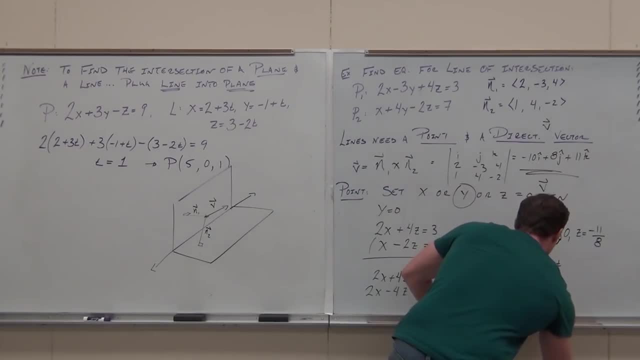 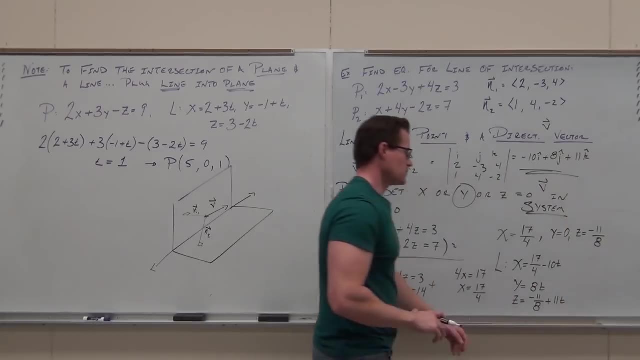 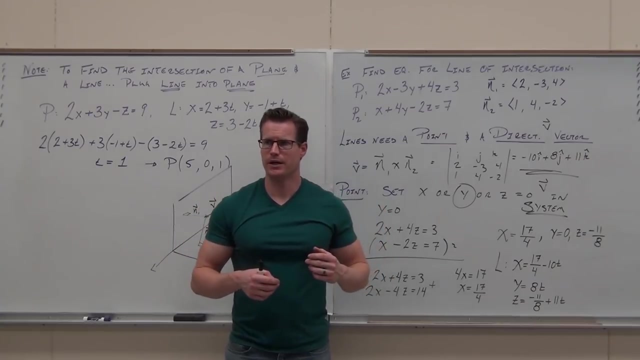 Come on quickly. What's the z start with Plus or minus Plus? It's pretty interesting. These planes are going to meet somewhere in space. Their meeting is going to be a line. I know that line because I did. the system is going to travel. 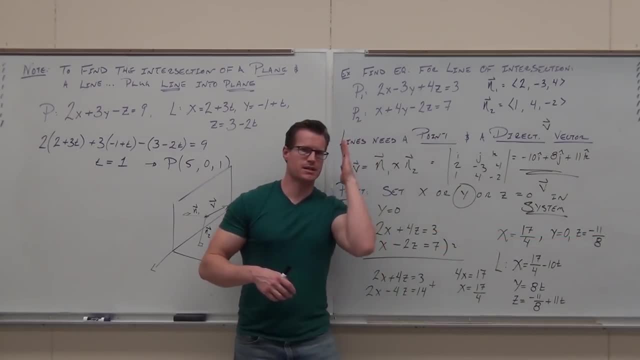 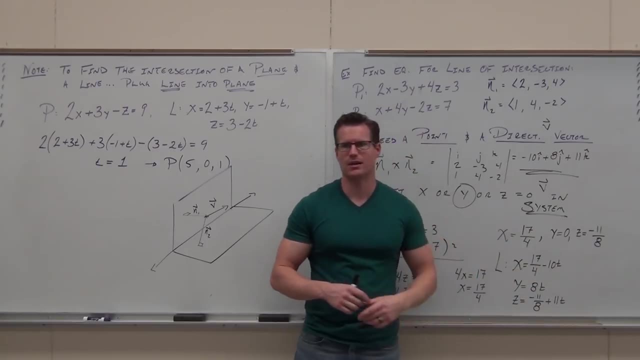 through That point on the x- z plane. using that point and the direction vector, which is mutually orthogonal to our normals, we now have an equation of that line. That's pretty cool. We just found out the line that these planes make. 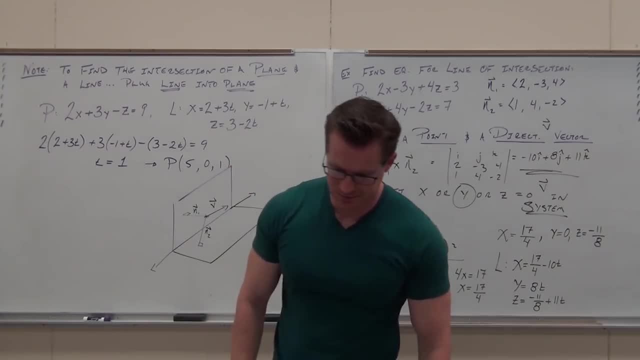 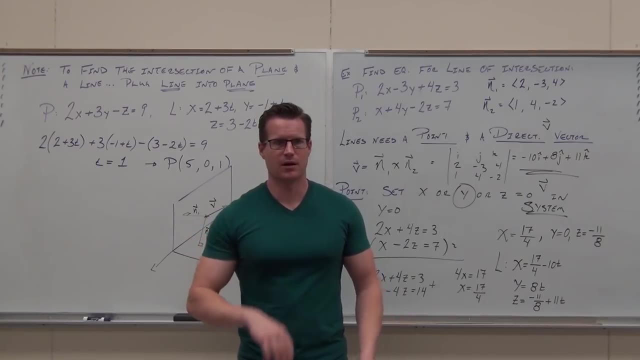 Pretty neato, Neato, Real neato. I don't care What's it mean to me It's pretty neat. if you need to do this stuff on some other topics- We don't have time to cover all of them, but it's pretty neat. 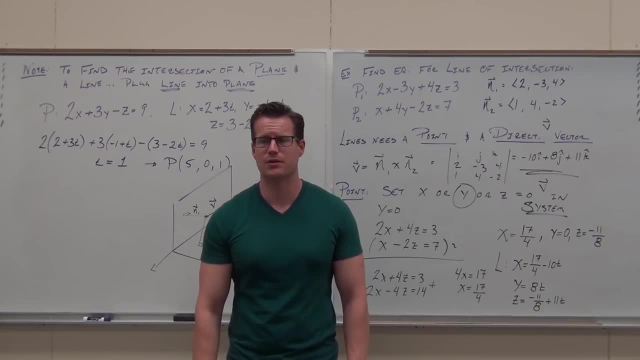 It's pretty interesting. at least that we can even do it is pretty cool, I think. So, if you guys feel okay with the idea, Now is finally our time for distances. I love distances- Finally. We've been talking it up for a while. 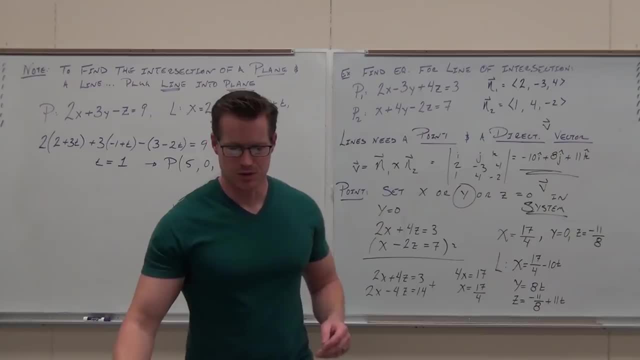 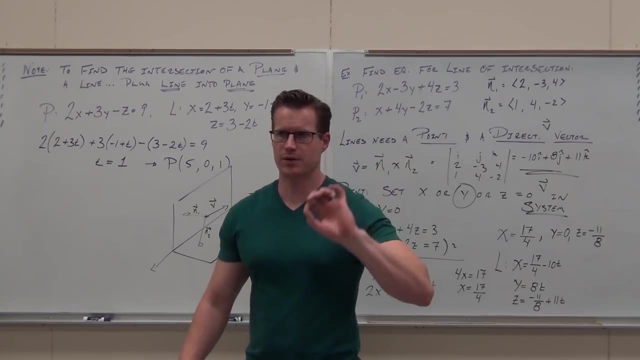 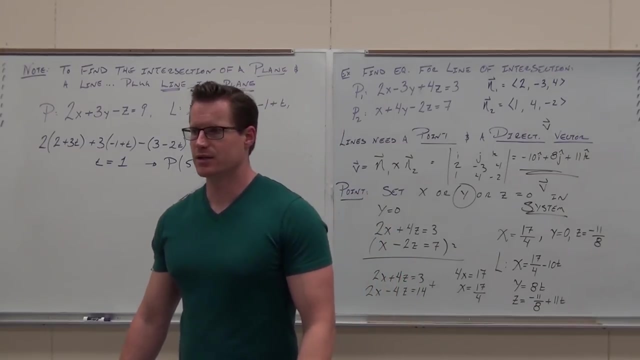 We're going to figure out how to find the distance between a point in a plane, parallel planes, skew lines- and a point in a line. I'm going to have to like warp speed, this stuff. I'd like to prove it to you, but I need your full like cooperation if we're going to do it. okay. 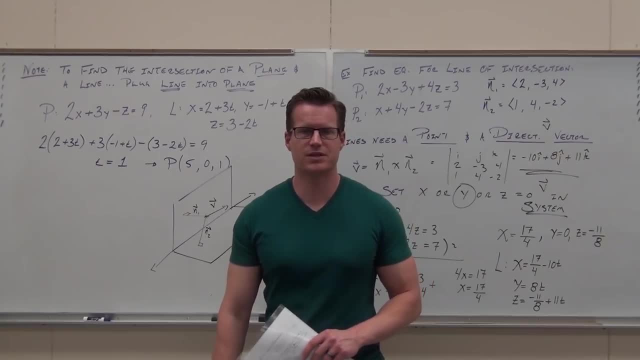 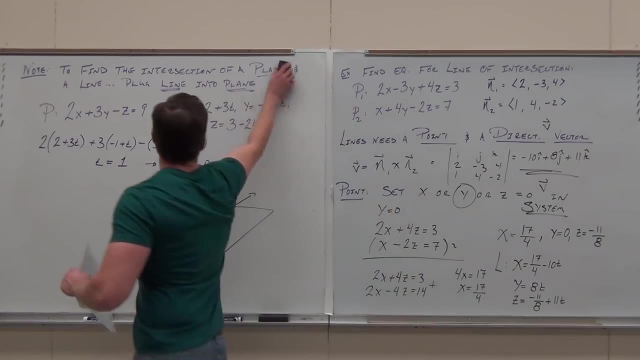 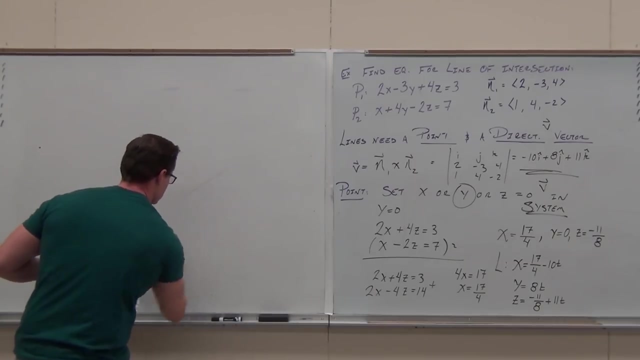 So it's going to be just me talking for a while about proving this stuff. I'm going to go very fast And then I'll show you some examples. We'll do two of them and that will be our whole time. So we're going to find distances of the following: 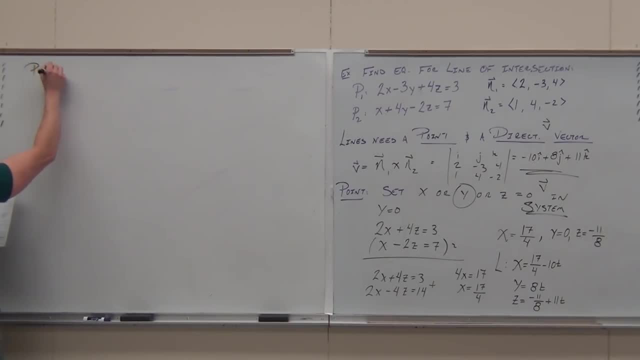 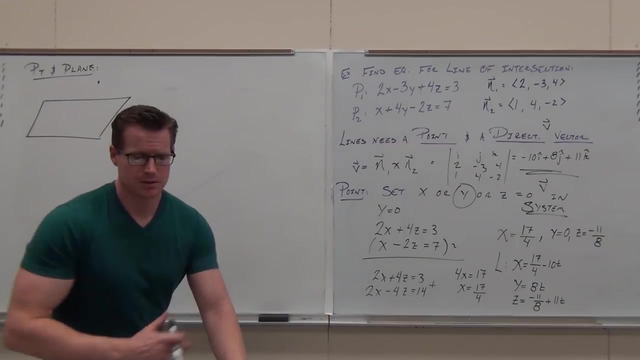 We're going to start with distance between a point and a plane. Here's our idea: Pick a point away from. well, you have a point away from a plane. Somehow we'll call it P1.. Find a point. Find a point on the plane. 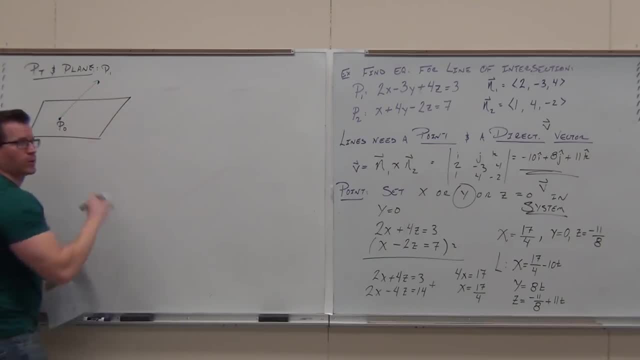 Create a vector. You know what, If you don't want to write this down, I don't care. You don't need to write it down. This is just the proof behind it. okay, You don't need to, unless you want it for future. 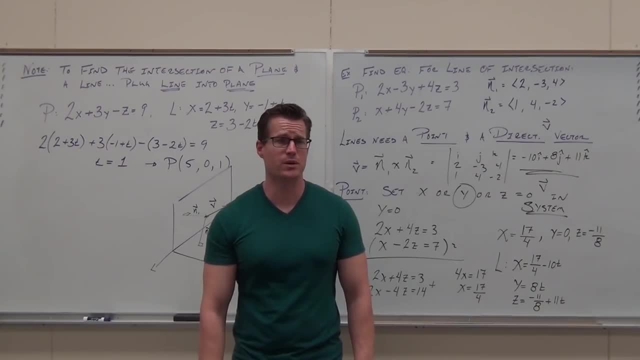 We don't have time to cover all of them, but it's pretty interesting at least that we can even do it. It's pretty cool, I think I like the idea. Now is finally our time for distances. I love distances Finally. 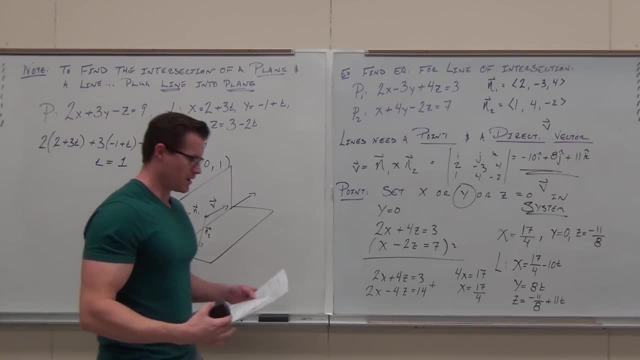 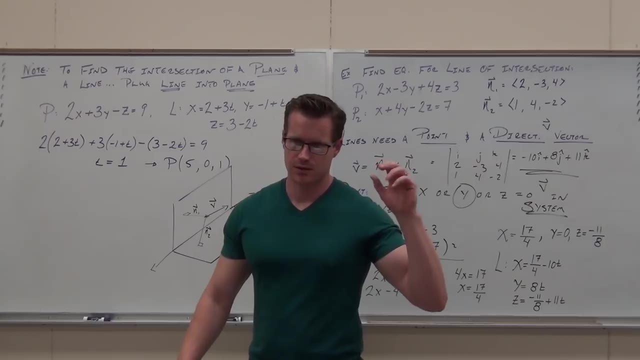 We've been talking it up for a while. We're going to figure out how to find the distance between a point in a plane, parallel planes, skew lines and a point in a line. I'm going to have to warp speed this stuff. 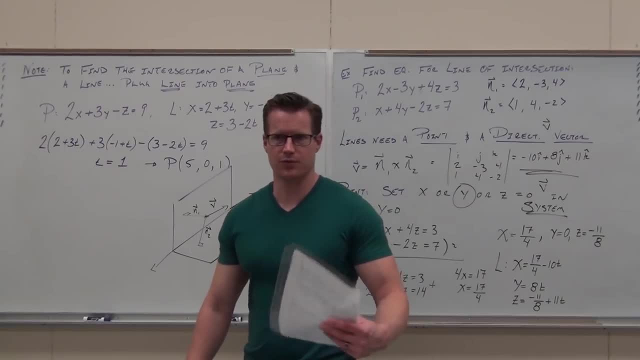 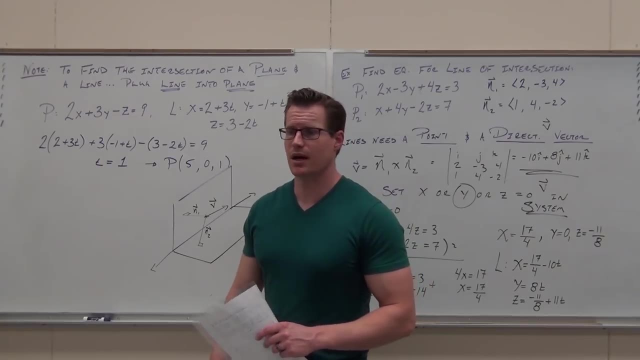 I'd like to prove it to you, but I need your full cooperation if we're going to do it. It's going to be just me talking for a while about proving this stuff. I'm going to go very fast. Then I'll show you some examples. 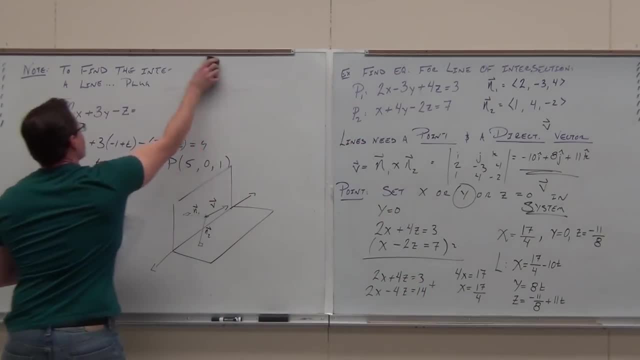 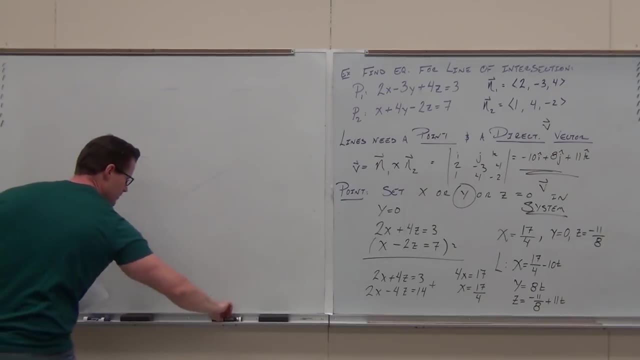 We'll do two of them. That will be our whole time. We're going to find distances of the following things. We're going to start with distance between a point and a plane. Here's your idea. Pick a point away from. Well, you have a point. 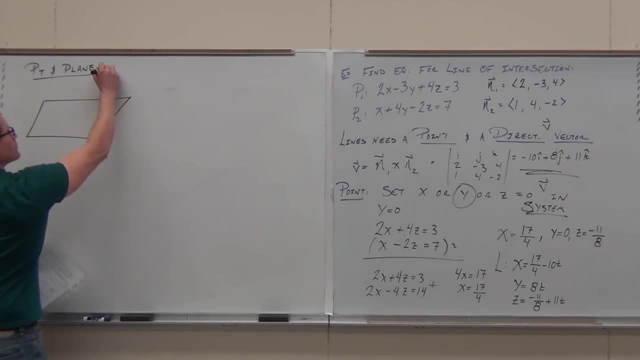 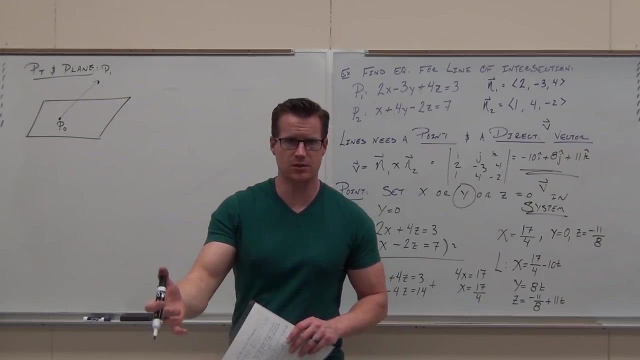 away from a plane- Somehow we'll call it P1,, find a point on the plane, Create a vertical line and a vector. You know what, If you don't want to write this down, I don't care, You don't need to write it down. 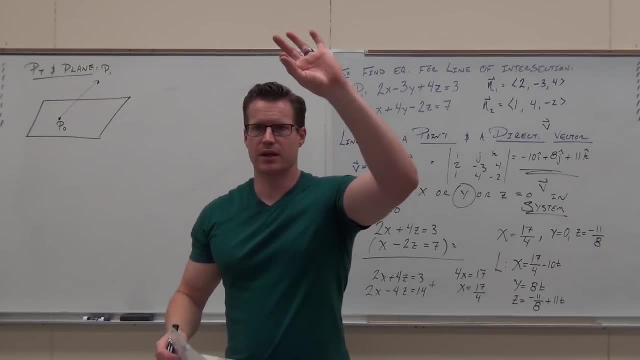 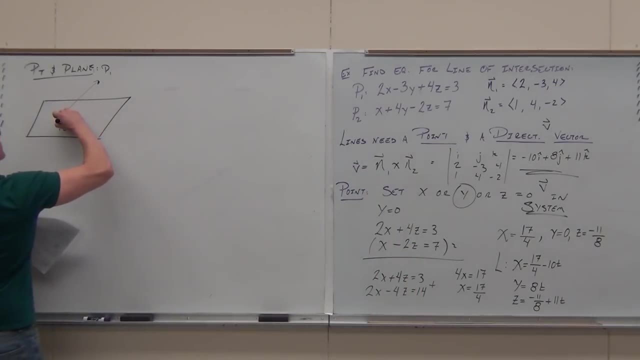 This is just the proof behind it. You don't need to, unless you want it for the future. that's fine. Here's the plan. You're going to have a point that's off the plane and a point that's on the plane. 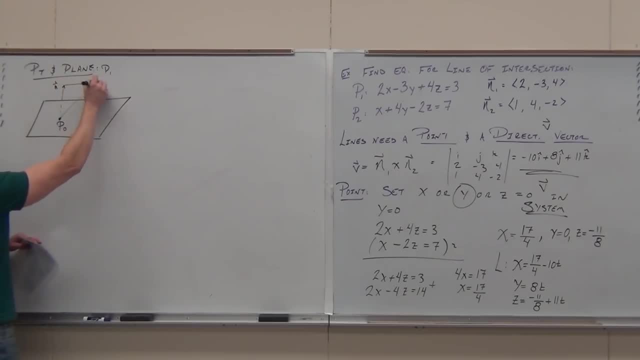 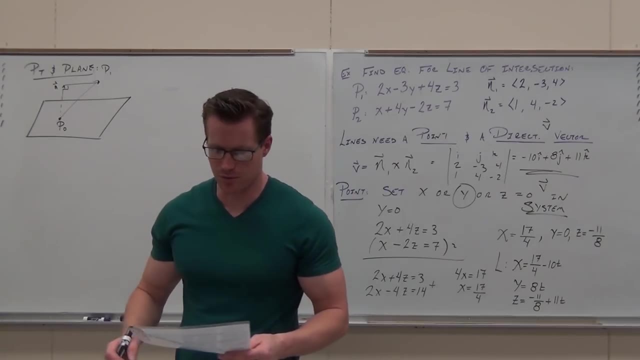 If it's not directly perpendicular, what we're going to do is project it onto the normal. If it's not directly perpendicular, you can project it onto the normal. So this point 1, let's call it x1,, y1,, z1,. 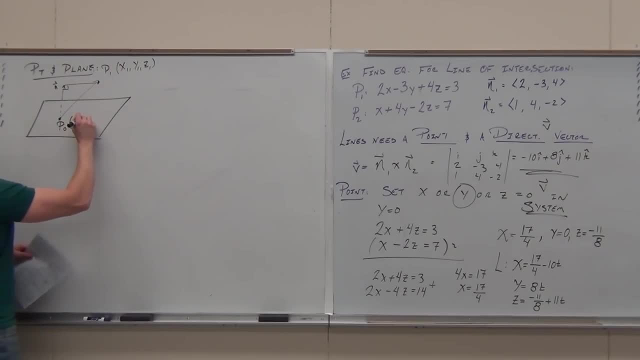 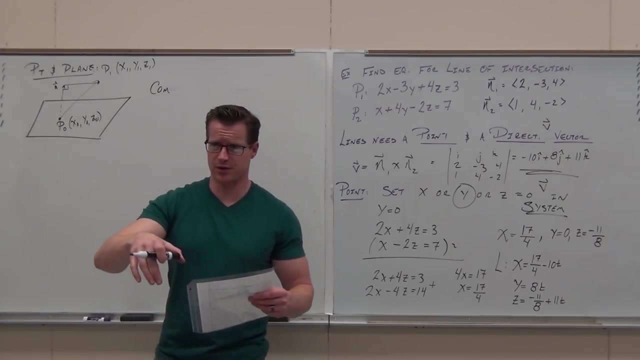 and this point: x0, y0, z0.. If you remember this stuff, component projection. I'm just looking for distance, so I'm not worried about scalar, I'm not worried about vector projection, I'm worried about scalar projection or component projection. 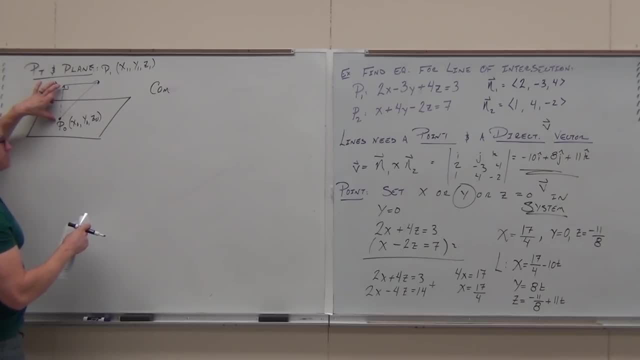 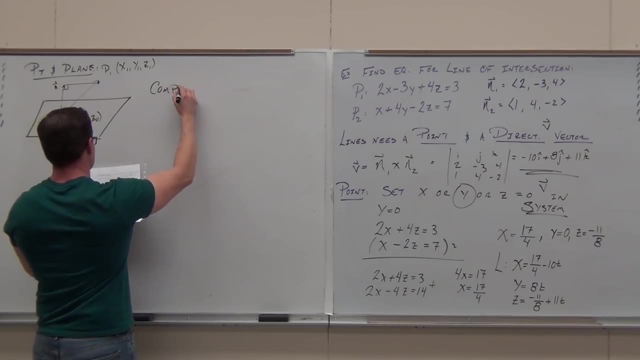 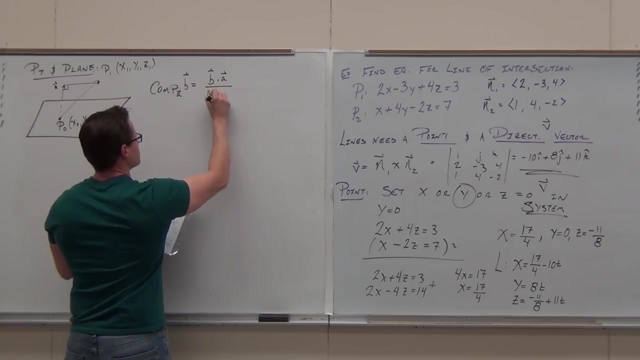 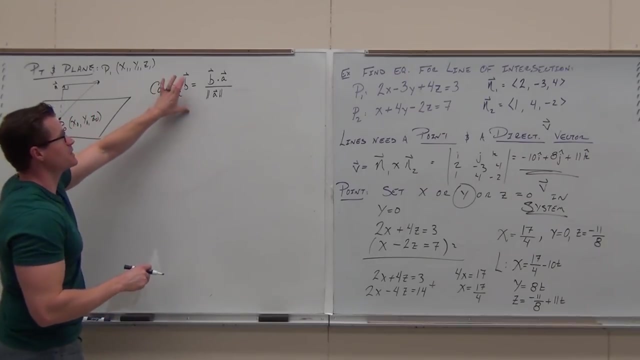 I just want to find the distance man, Verify that. this distance, that projection is that distance. It's the same thing. Do you remember that formula at all? When we want to find the scalar projection of b onto a, we did b first. 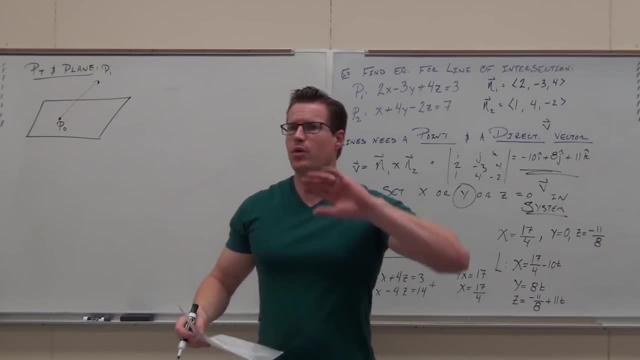 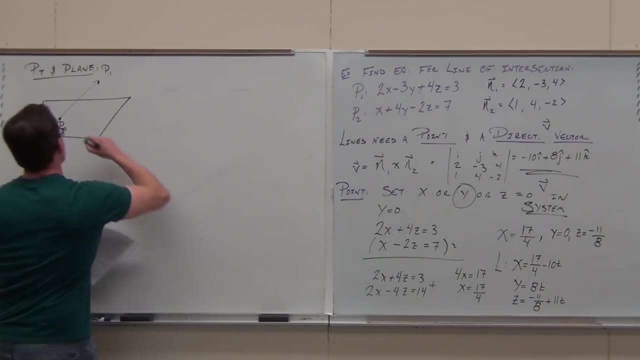 That's fine, But here's the plan. You're going to have a point that's off the plane and a point that's on the plane If it's not directly perpendicular. what we're going to do is we're going to, we're going to project it onto the normal 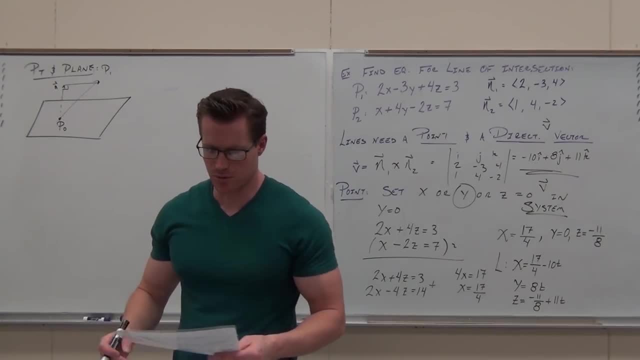 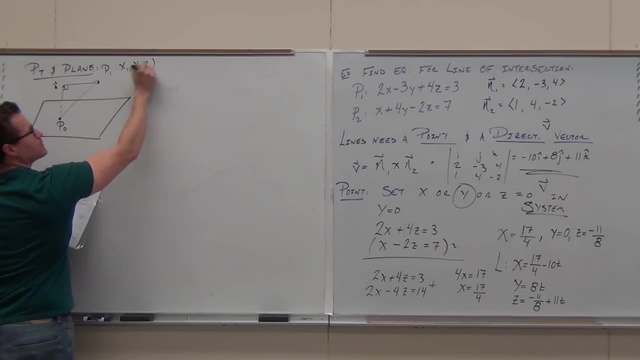 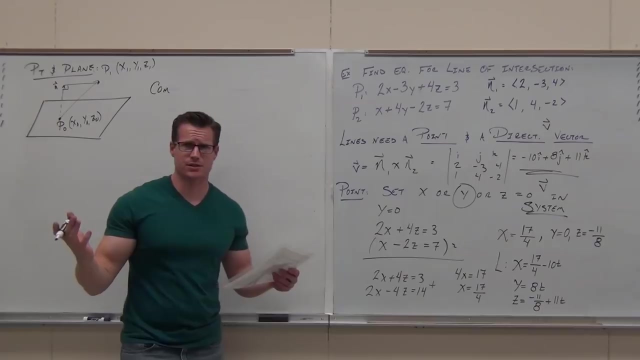 If it's not directly perpendicular, you can project it onto the normal. So this point 1, let's call it X1, Y1, Z1, and this point X0, Y0, Z0,, if you remember this stuff, component projection. I'm just looking for distance, so I'm not worried about 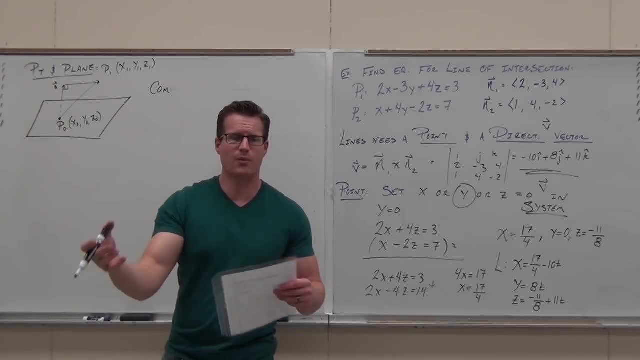 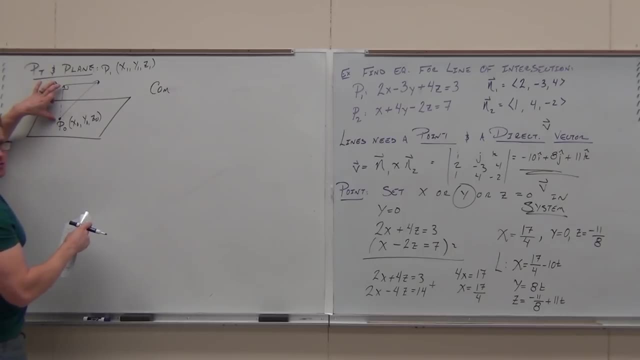 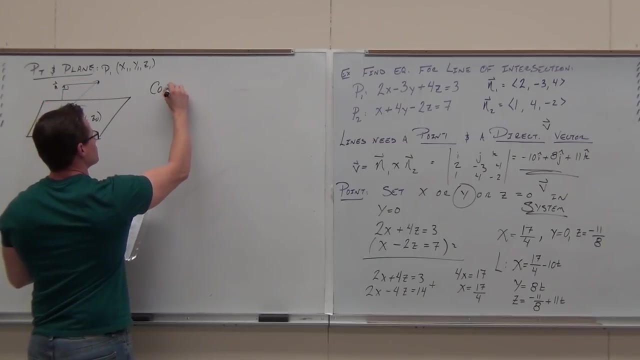 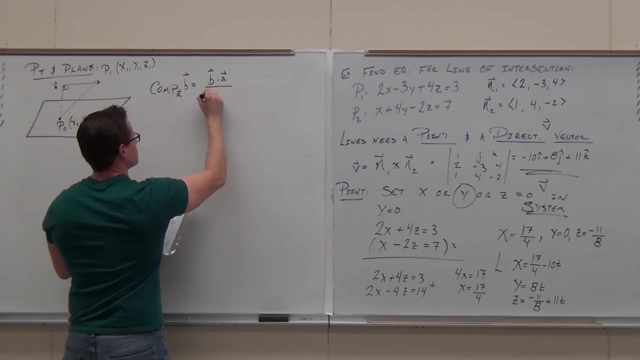 scalar. sorry, I'm not worried about vector projection, I'm worried about scalar projection or component projection. I just want to find the distance. man Verify that. this distance, that projection, is that distance. It's the same thing. Did you remember that formula at all? 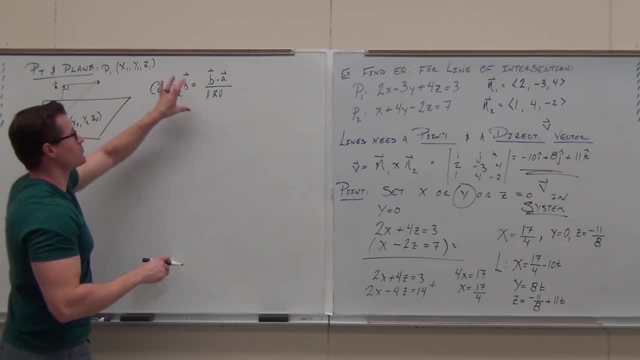 When we want to find the. when we did the scalar projection of B onto A, we did B first dot with A divided by magnitude A, the one you're projecting on. So if I change this to this, if the component projection is the distance, all I got to do 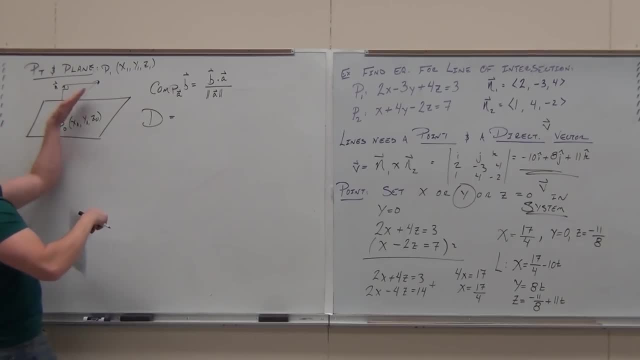 is change the names of my vectors. The one that we're projecting is the B. The one we're projecting is the P0 to P1.. We're projecting that onto the normal and then dividing by the magnitude of the one that we're actually projecting onto the normal. 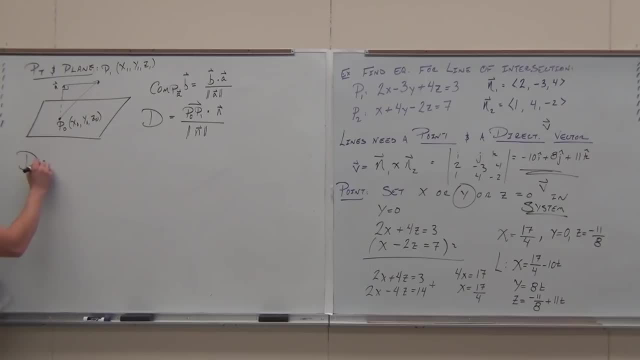 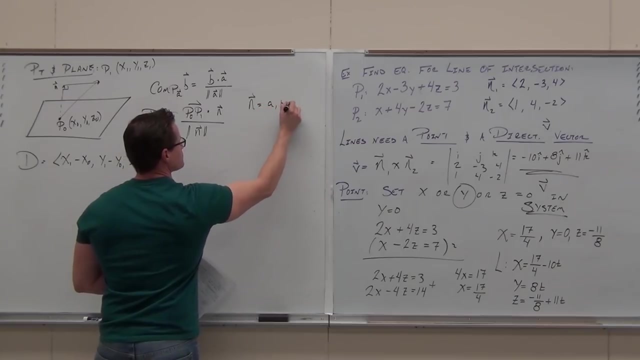 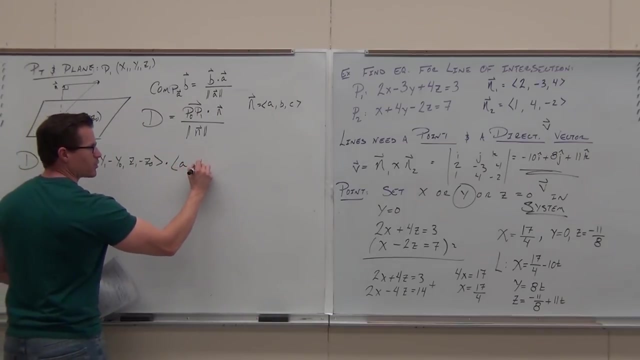 Now, if we do that, if we do that, this right here is that vector dotted with, if I give my normal, our usual, our usual components A, B, C, if I give that, that to my normal, then this is vector P0 to P1.. 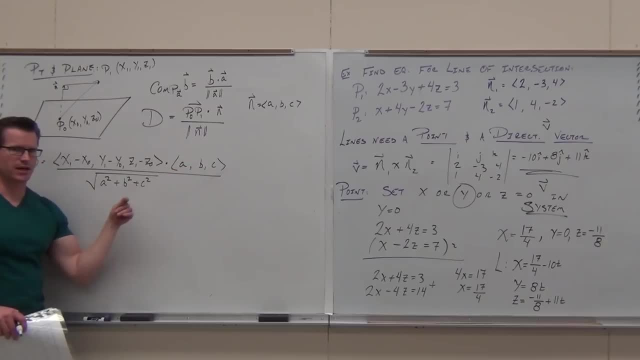 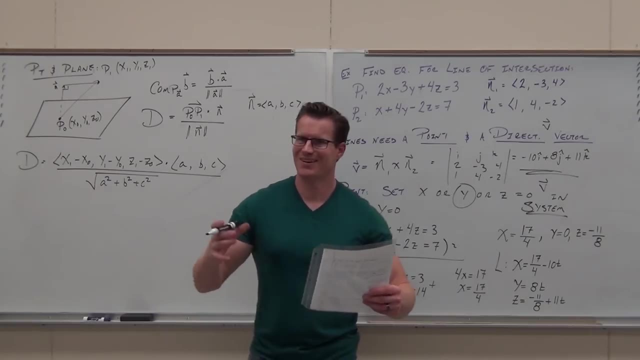 This is vector and the normal. This is the magnitude of vector and the normal Head. nod, if you're okay on the proof so far, This is the cool part. If we did, you're going to miss it. if you blink at it, it's. it's pretty darn neat. 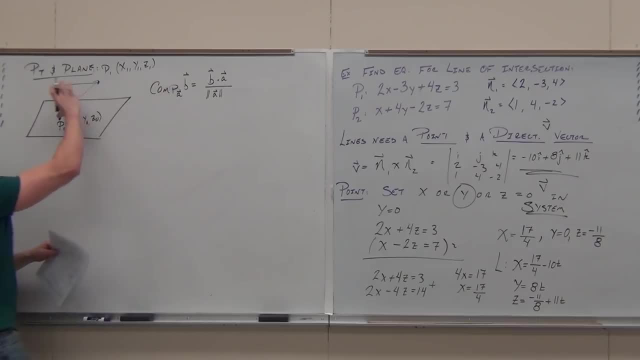 dot with a divided by magnitude of a, the one you're projecting on. So if I change this to this, if the component projection is the distance, all I gotta do is change the names of my vectors. The one that we're projecting is the b. 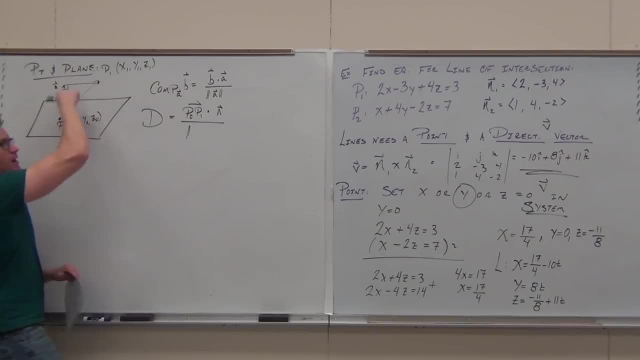 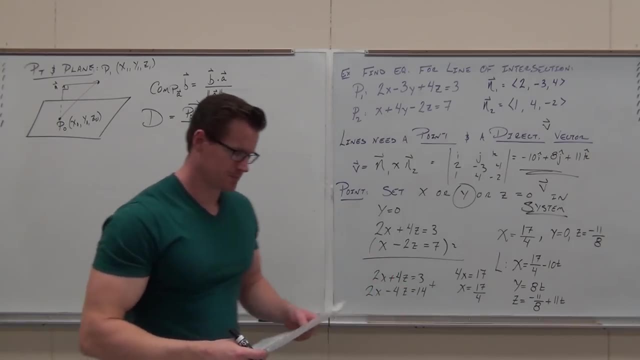 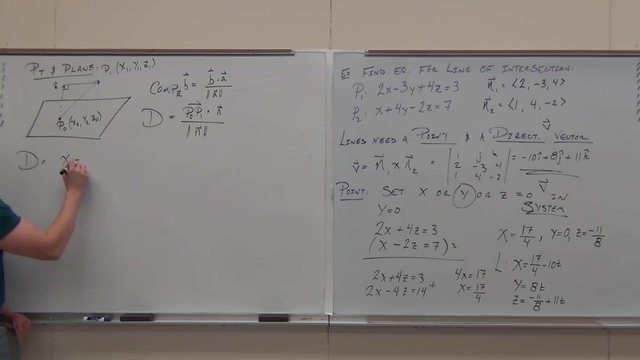 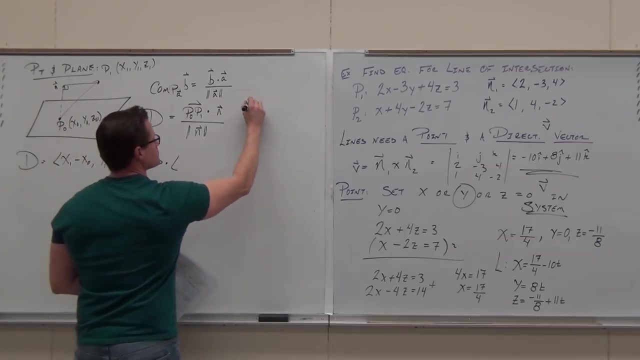 The one we're projecting is the p0 to p1.. And now we project it onto the normal. Now, if we do that, if we do that, this right here is that vector dotted with, if I give my normal, our usual, our usual component's abc. 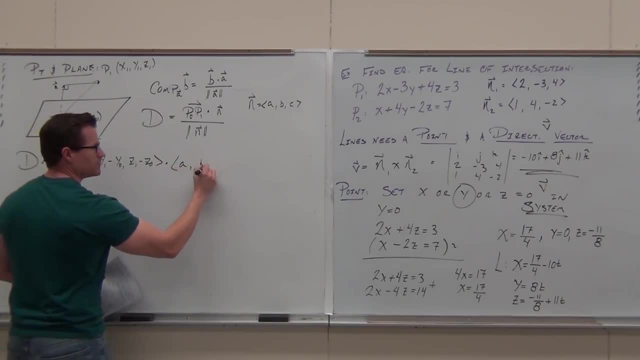 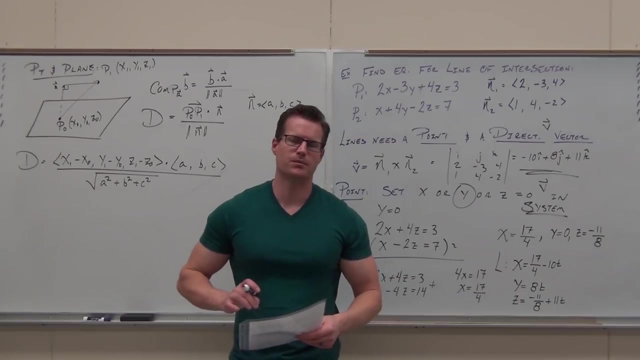 If I give that that to my normal, then this is vector p0 to p1.. This is vector and the normal. This is the magnitude of vector and the normal. This is the cool part, If we you're gonna miss it. 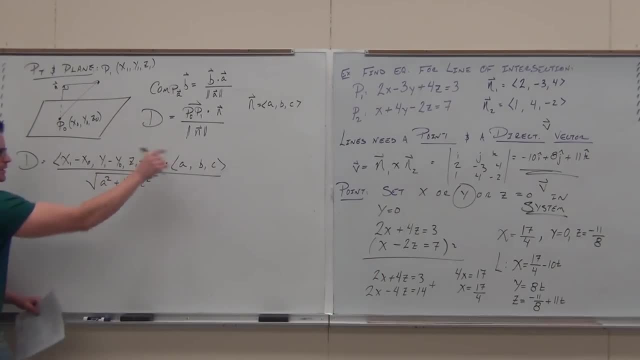 if you blink at it, It's pretty darn neat If you dot product this. I'm gonna do one more thing here. in a second. I'm gonna add some absolute values, because we never want our distances to be negative, So I'm gonna add some absolute values. 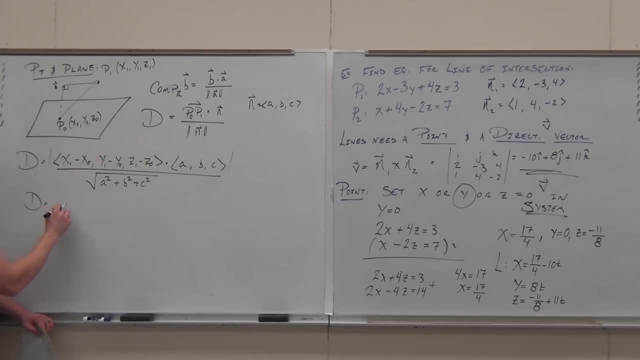 but that's all that's gonna do. So we go: okay, yeah, sure, Then we get: I'm gonna do it kinda fancy-like. Here's what I'm gonna do. just watch carefully so I don't miss you When I dot product. I'm gonna multiply this times this. 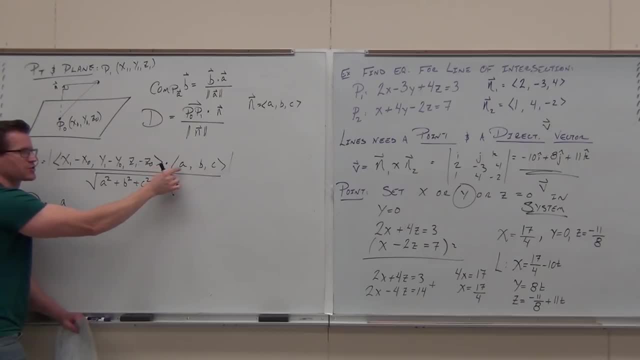 this times this and add them correct, Which means I can distribute this to both of these, this to both of these, this to both of these. Did you catch it? So I'm gonna get ax1,, I'm gonna get by1,. 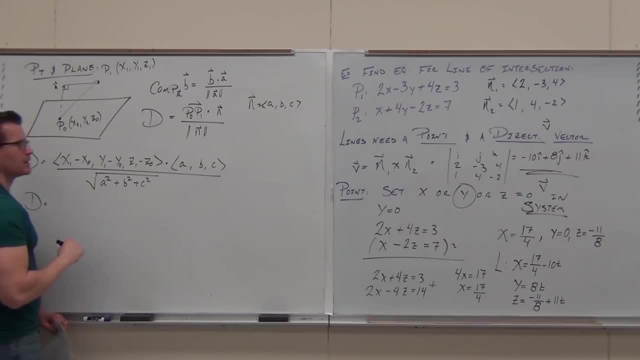 If you dot product this. I'm going to do one more thing here. in a second I'm going to add some absolute values, because we never want our distances to be negative. So I'm going to add some absolute values, but that's all that's going to do. 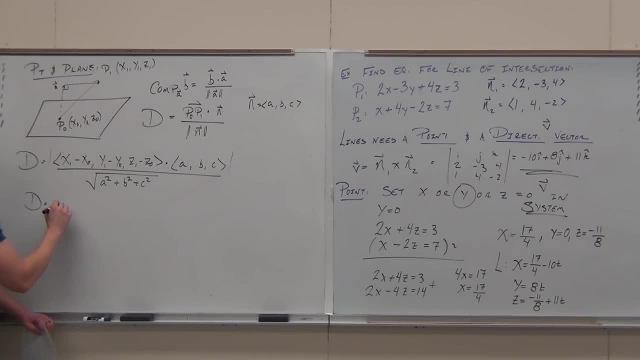 So we go, okay, yeah, sure, Then we get. I'm going to do it kind of fancy like Here's what I'm going to do. Just watch carefully so I don't miss you When I, when I dot product, I'm going to multiply this times this, this times this. 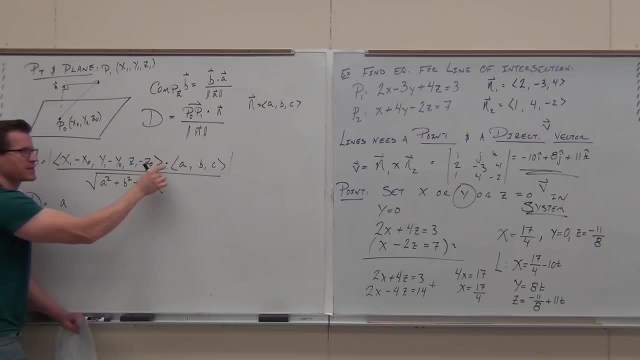 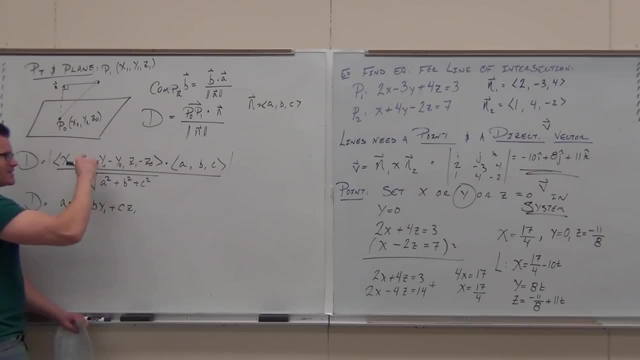 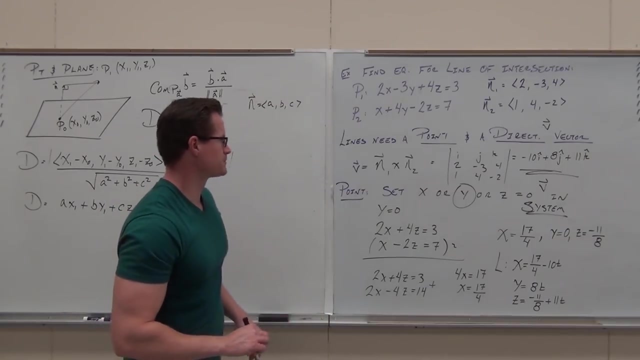 but then I'm going to get this stuff, this, this AX sub 0,, this BY sub 0, and this CZ sub 0.. Now here's the neat thing about this: All this stuff, all that stuff that we, we did, we did before, we called that that letter. 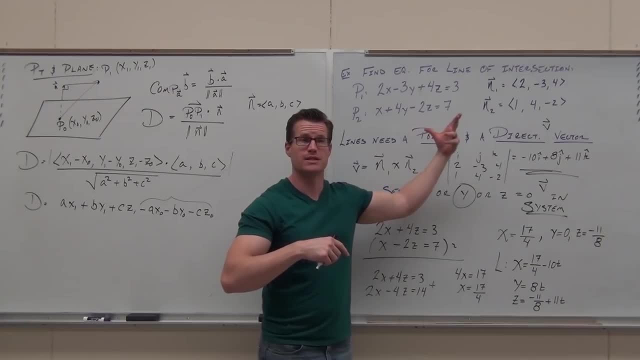 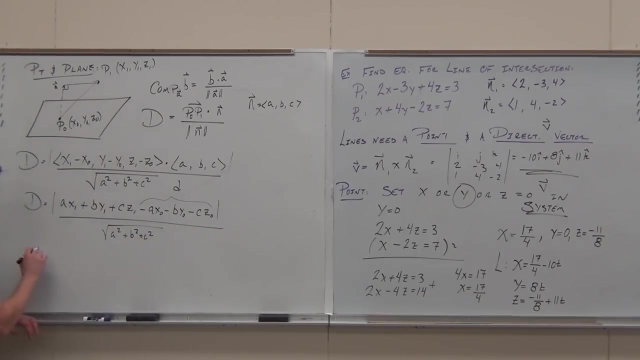 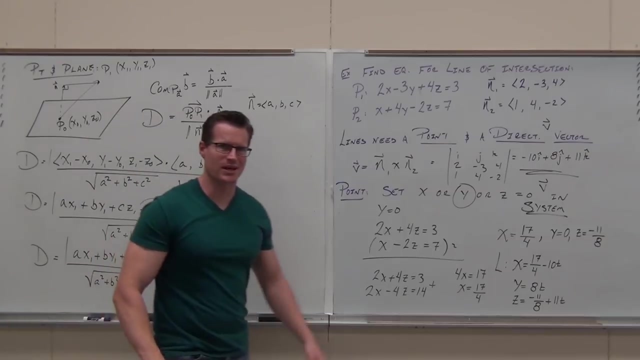 Do you remember distributing it, combining it, adding it over? That was our D, This is all D. So, if I continue, The distance between a point and a plane looks just like this. You go fantastic. What's that? What's that? 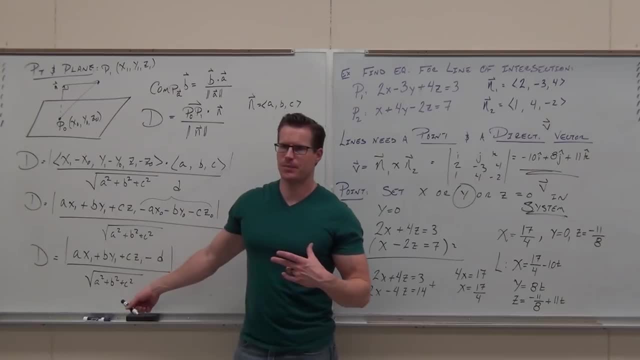 What's that even mean? Firstly, there are no variables. here There are no variables. I want you to look at it real carefully. Where do the A, the B and the C come from? The normal It comes from the plane. 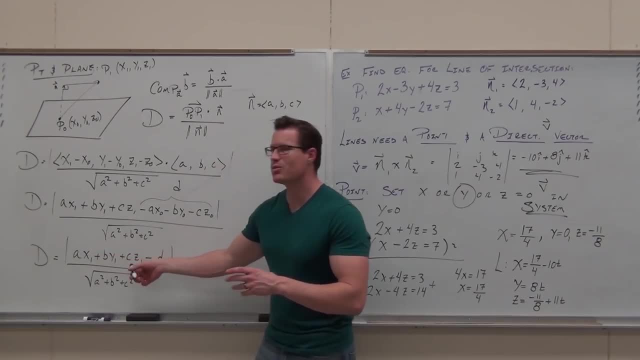 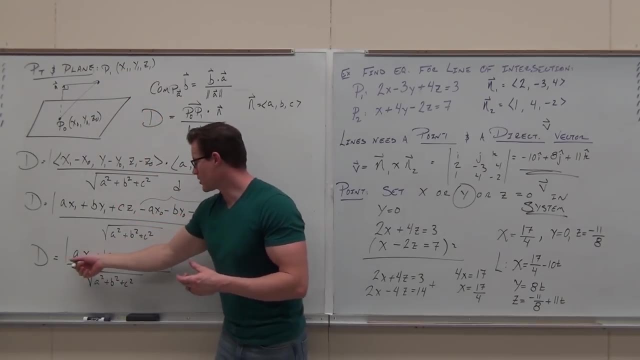 The normal, Same ABC: The X1, the Y1, and the Z1, that is your point off of the plane. That's your X1,, Y1, Z1.. So literally all you got to do: take the normal vector, put the numbers here. 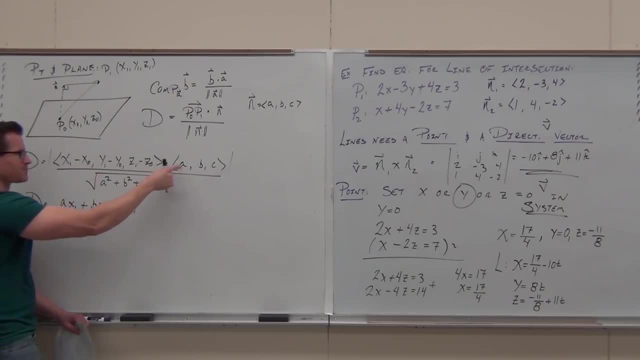 I'm gonna get cz1, but then I'm gonna get this stuff, this ax0,, this by0, and this cz0.. Now here's the neat thing about this: All this stuff, all that stuff that we did, we did before. 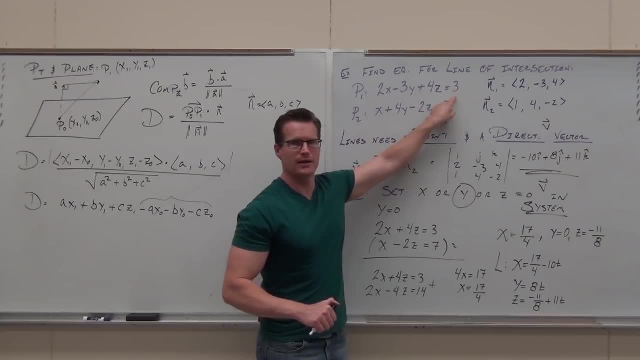 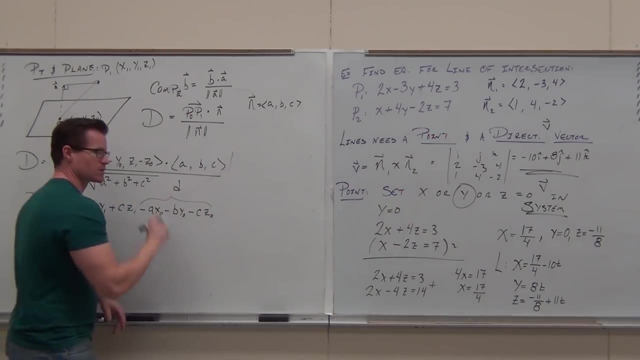 we called that, that letter. Do you remember distributing it, combining it, adding it over? That was our d. This is all d So, if I continue, the distance between a point and a plane looks just like this. Fantastic, What's that? 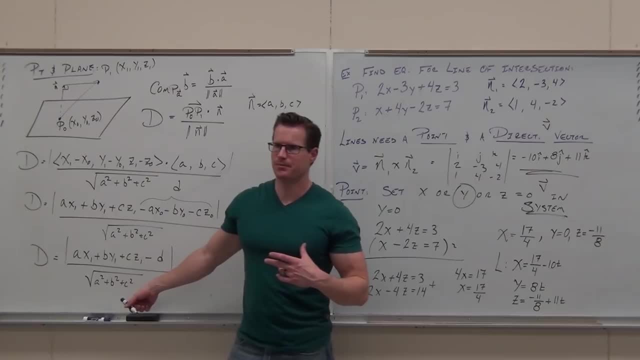 What's that even mean? Firstly, there are no variables here. There are no variables. Where do the a, the b and the c come from? The normal It comes from the plane. The same a, b, c, The x1,, the y1, and the z1,. 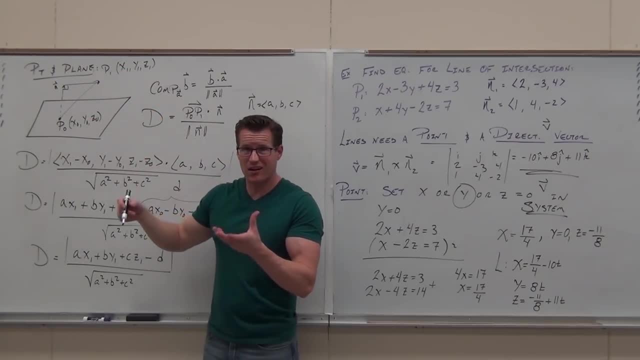 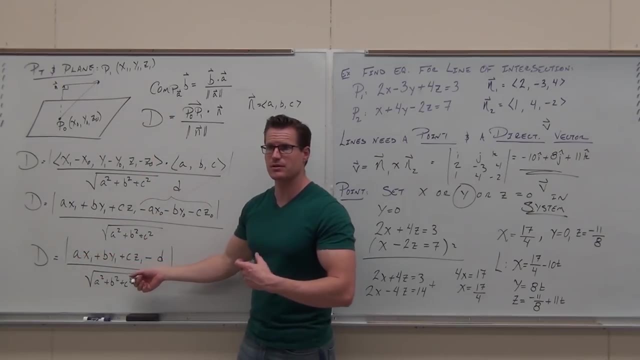 that is your point off of the plane. That's your x1, y1, z1.. So literally all you gotta do: take the normal vector, put the numbers here. Take your x, y and z coordinates, put the numbers here. 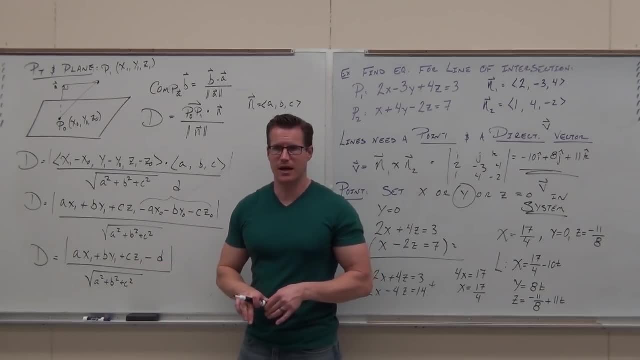 Add them together. subtract the d, take the absolute value, divide by the magnitude of the normal vector. That's how you figure out the point and the plane. Does that make sense to you? Okay, I want to try one. You know what? 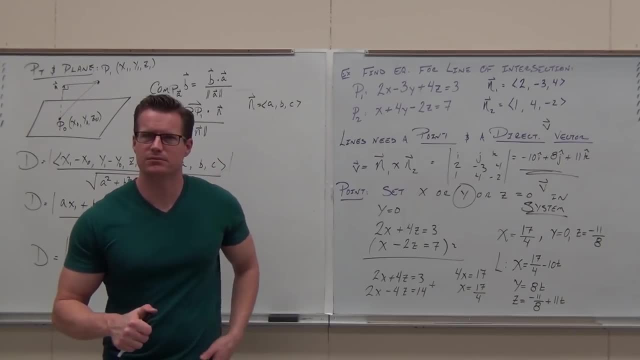 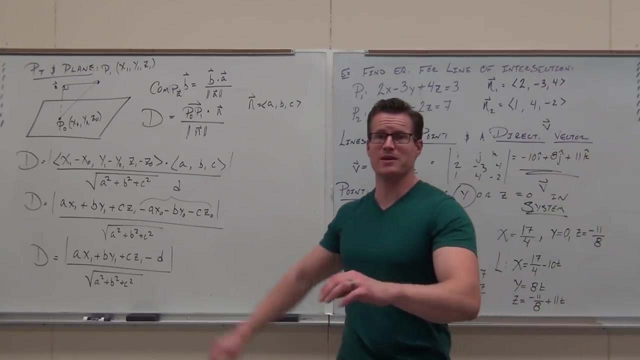 I'm sorry. Do you want to try one? Can I give you the other ones first? Can we do that? You want to try one, Do you care? Do you want more candy? If I hit you in the face, don't sue me. 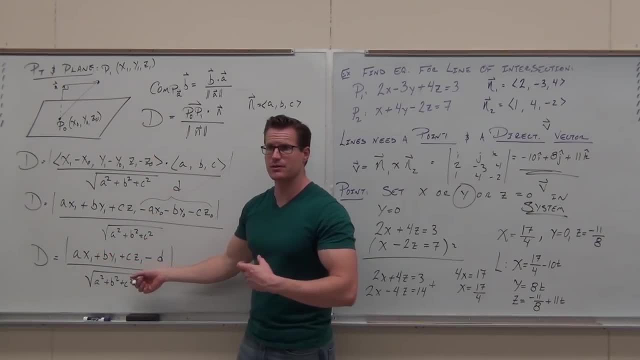 Take your X, Y and Z coordinates, put the numbers here, Add them together. Subtract the D, Take the absolute value, divide by the magnitude of the normal vector. That's how you figure out how to find the distance between a point and a plane. 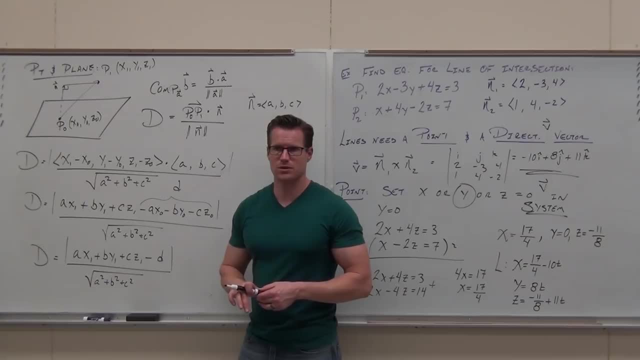 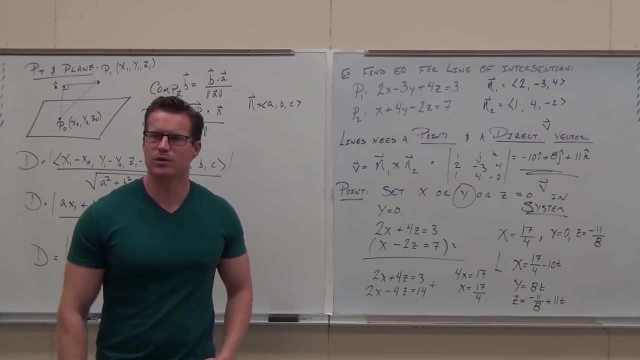 That's how you figure out how to find the distance between a point and a plane. Does that make sense to you? Yes, Okay, I want to try one. You know what? I'm sorry. Do you want to try one, Or can I give you the other ones first? 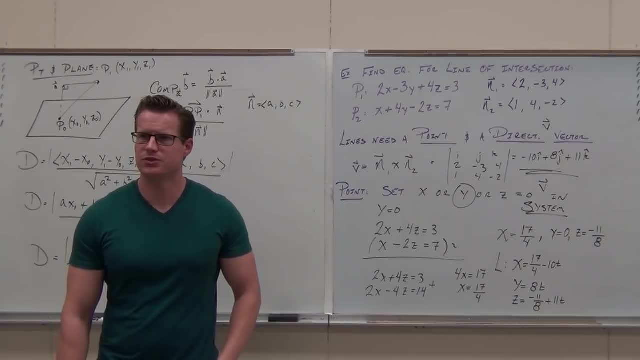 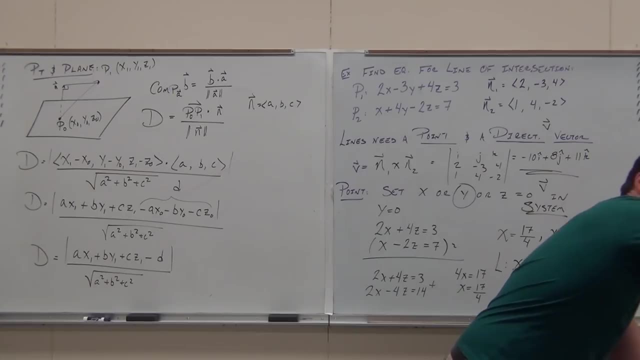 Can we do that? Yeah, let's do that. You want to try one, Do you care? Do you want more candy? Do you want more candy? If I hit you in the face, don't say it. Say it to me. 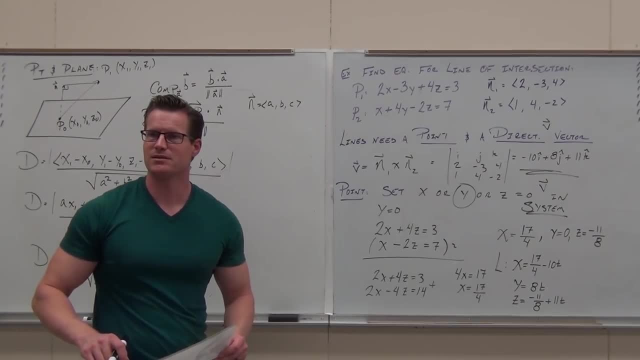 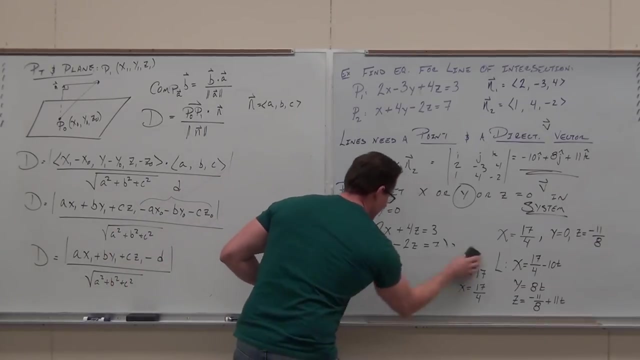 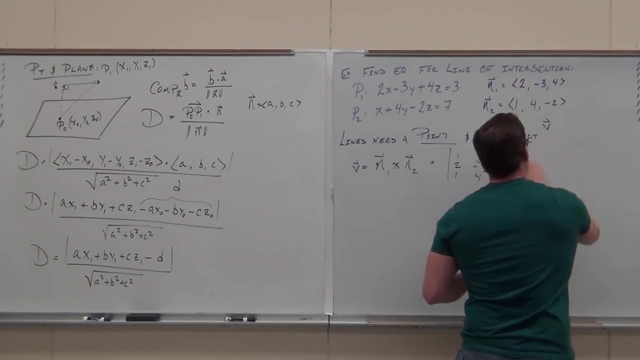 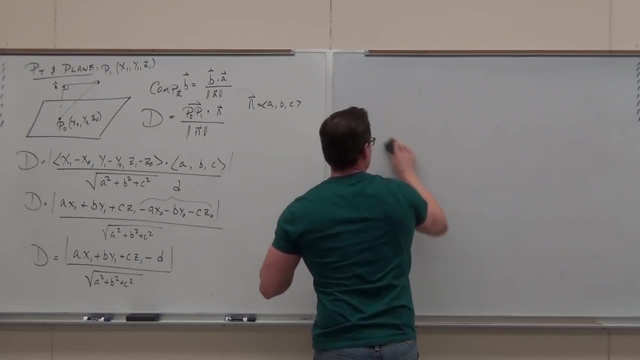 Nice. You said yes, That's why it was a good throw Right to you. You literally could have just. You know what. You want to try that Neither. I don't want to hit you in the face Now. there's something interesting that we're going to talk about here. 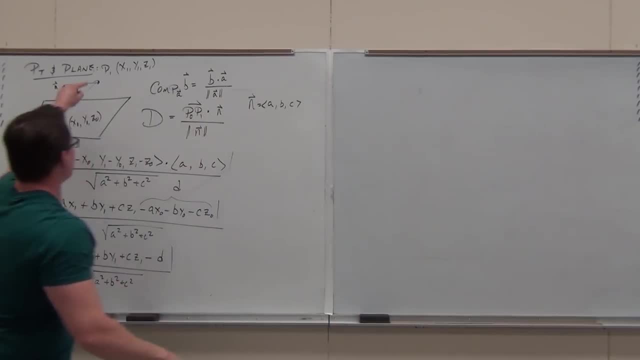 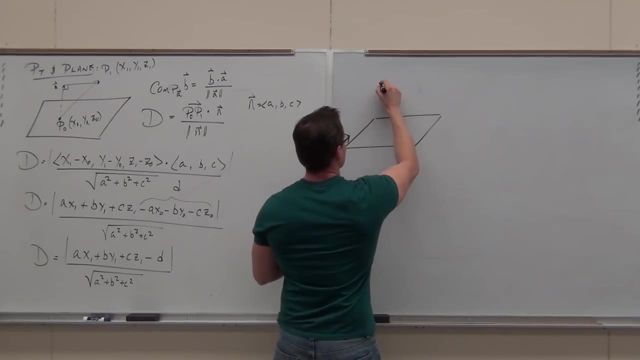 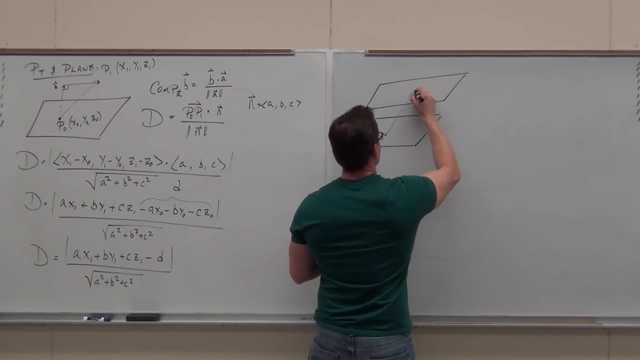 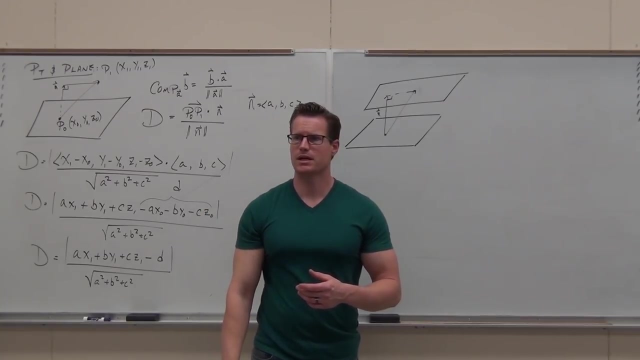 What if that point were contained in another plane? Do you see the picture I'm trying to draw? The point's contained in another plane. What if that happens? Furthermore, what if the planes were parallel? Now, I'm not going to ask you. hey, find the distance between two planes if they're not parallel. 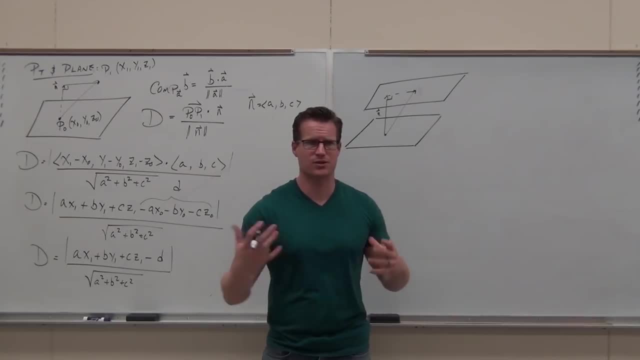 You know why? Because there is none, Because they're going to meet. We just did that problem. intersection of two planes. It's a line, There is no distance They actually cross. But if the plane is parallel it's not parallel. 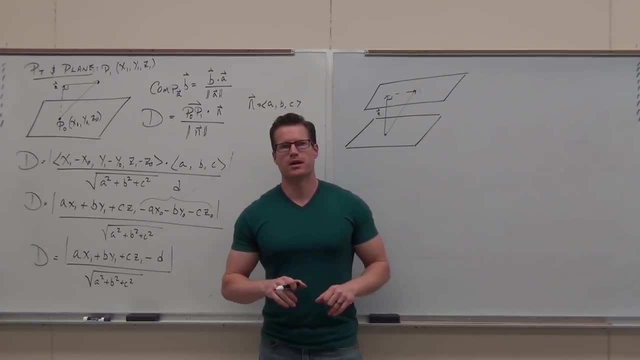 If the planes are parallel, true or false. If the planes are parallel, they have the same normal vector, True, True, Yes, Okay, If the planes are parallel, they have the same normal vector. then when I move this, when I move this over, we have the same normal vector. a lot of cool stuff happens. 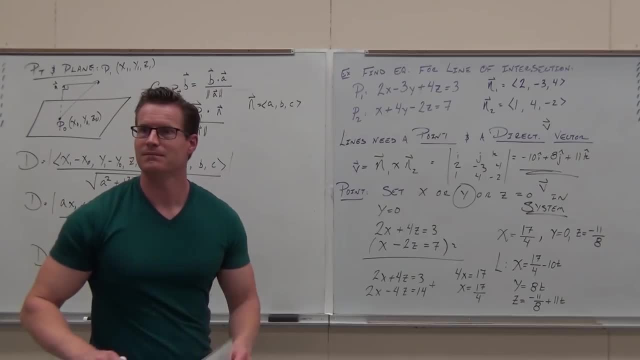 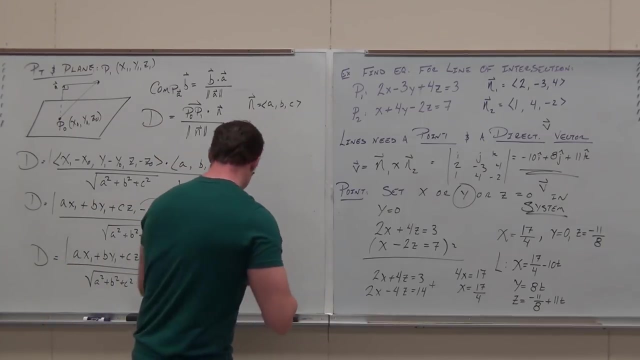 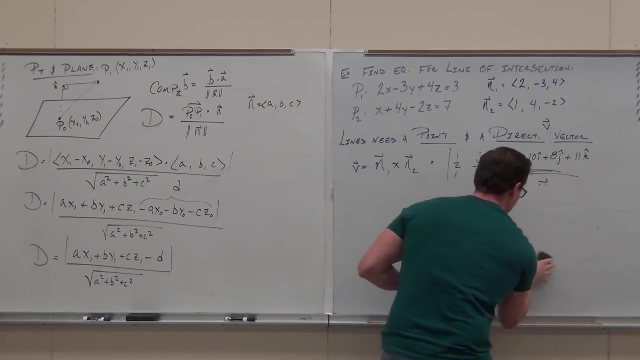 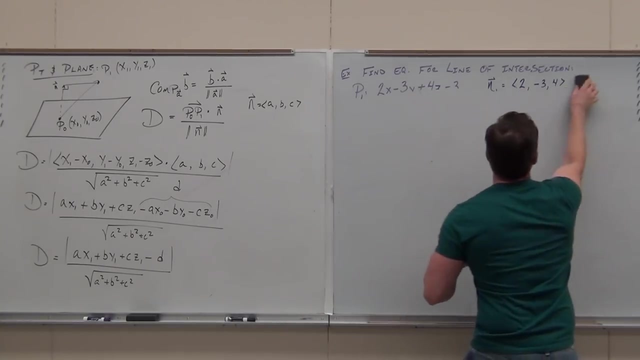 Cool, Nice. You said yes, That's why it was a good throw Right to you. You literally could have just. You want to try that. I don't want to hit you in the face Now. there's something interesting that we're going to talk about here. 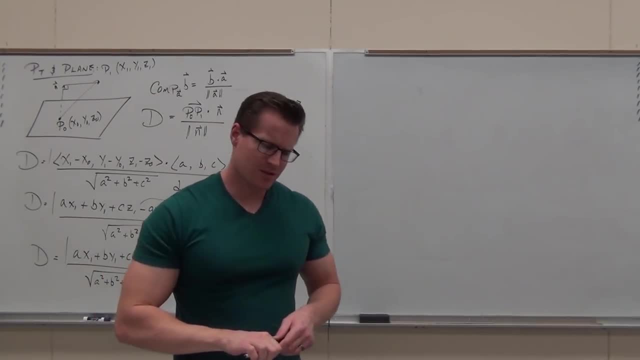 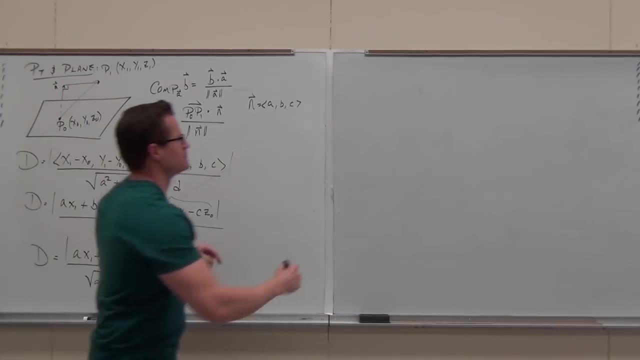 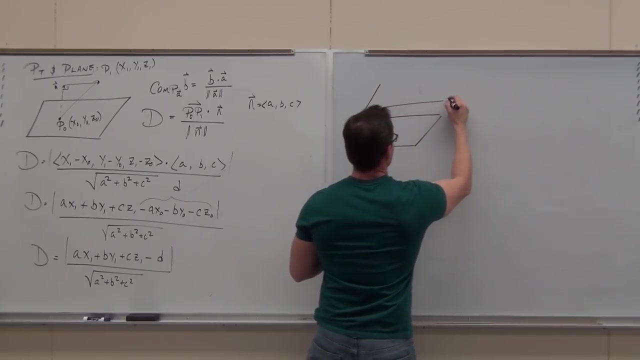 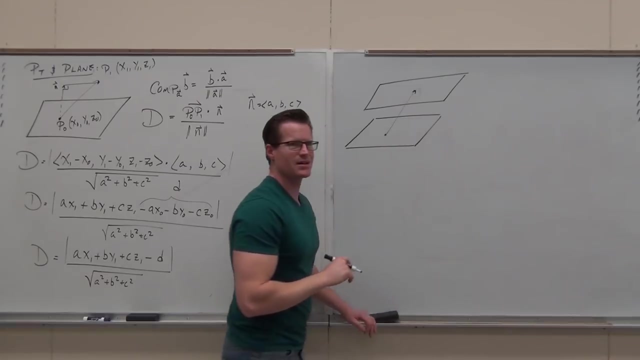 What if? What if that point, What if that point were contained in another plane? Do you see the picture I'm trying to draw? The point's contained in another plane. What if that happens? Furthermore, what if the planes were? 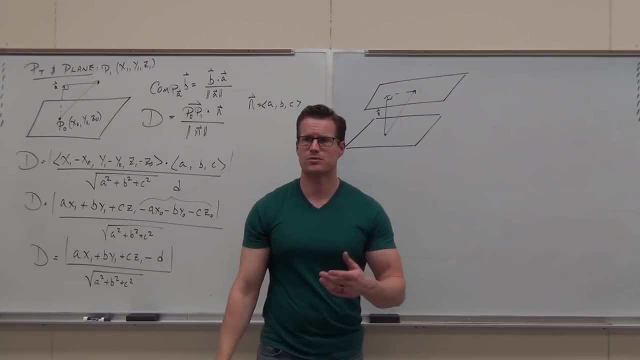 Okay, What if the planes were parallel? Now I'm not going to ask you. hey, find the distance between two planes if they're not parallel. You know why? Because there is none, Because they're going to meet. We just did that problem. 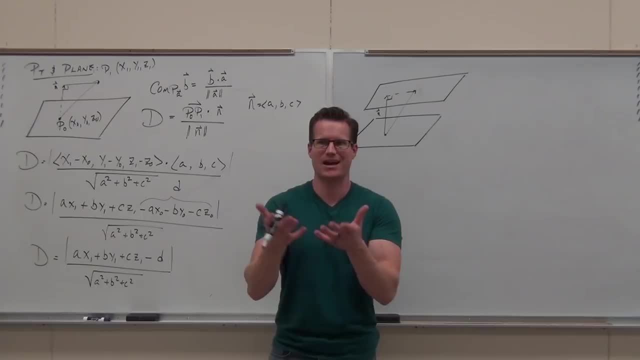 intersection of two planes. It's a line. There is no distance, True or false. But if the planes are parallel, True or false. If the planes are parallel, they have the same normal vector. Yes, Okay, If the planes are parallel. 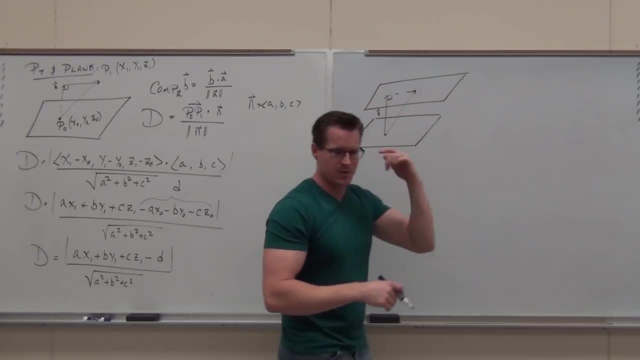 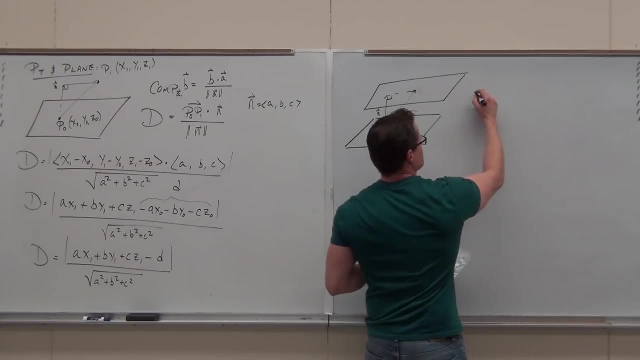 they have the same normal vector, then when I move this, When I move this over, we have the same normal vector. a lot of cool stuff happens. In fact, if we have that same normal vector, the distance between parallel planes is the same. 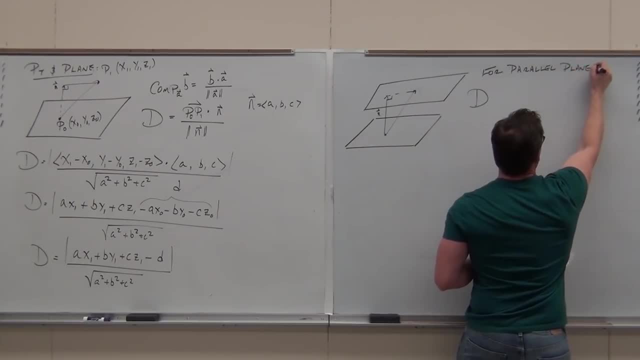 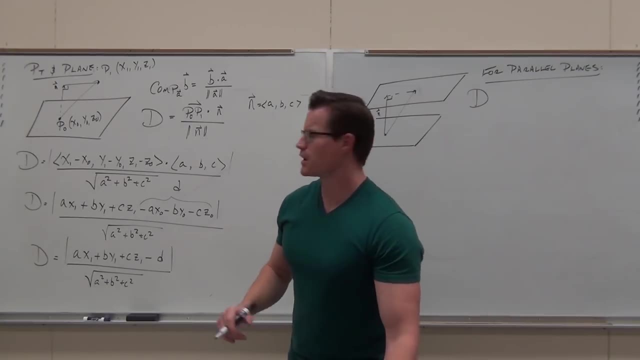 Distance between parallel planes. Distance between parallel planes, Distance between parallel planes. If I give you two planes and they have the same normal vector, a lot of the things here, because you have the same a, b and c, simplify out. 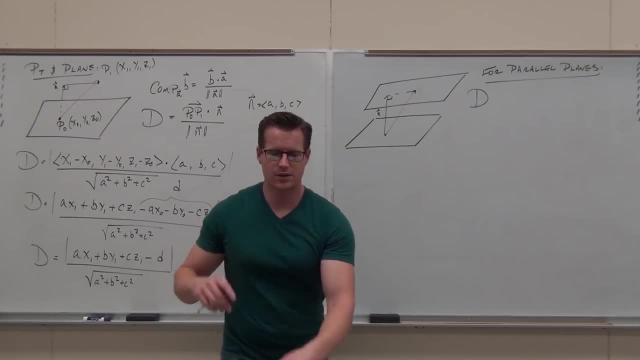 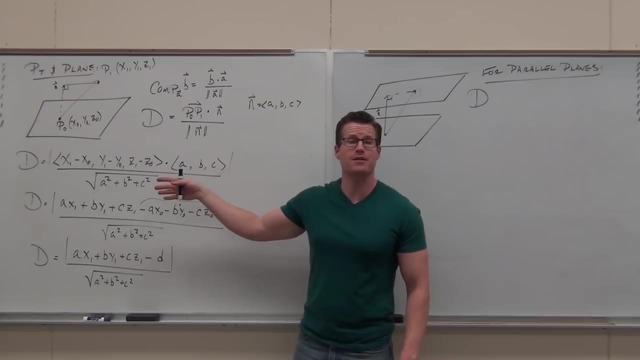 They are gone. They're not going to be there anymore. What's going to happen is that we end up with only two different d's. Verify: that's the only thing in planes that can possibly be different if we have like ax plus. 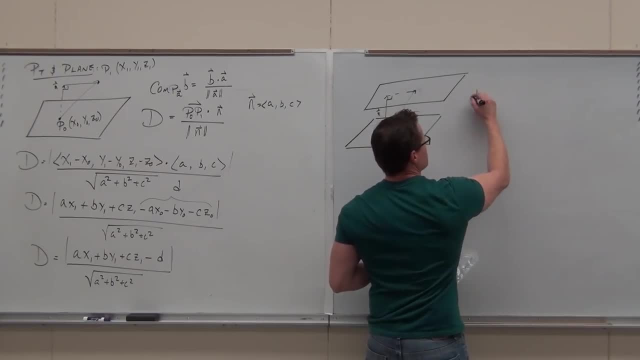 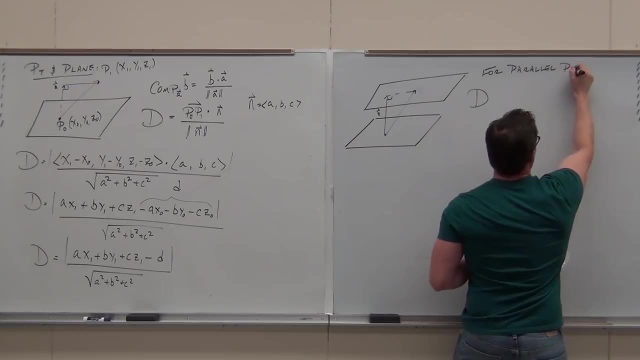 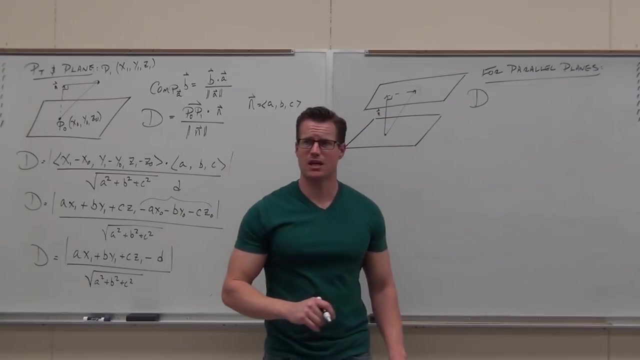 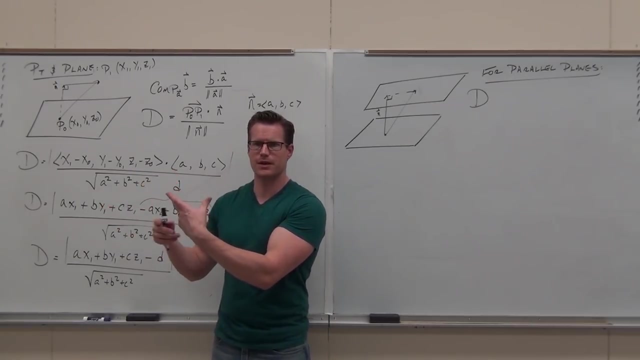 In fact, if we have that same normal vector, the distance between parallel planes, if I give you two planes and they have the same normal vector, a lot of the things here, because you have the same A, B and C. simplify out, they are gone. 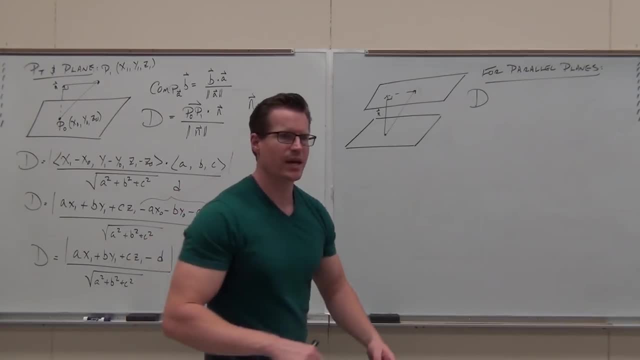 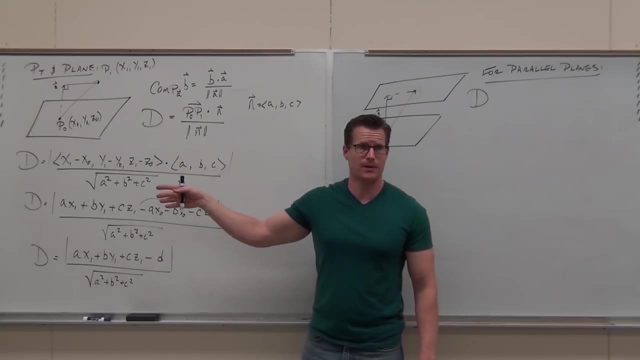 They're not going to be there anymore. What's going to happen is that we end up with only two different Ds. Verify: that's the only thing in planes that could possibly be different if they're parallel, If we have like. oh, this is a plane. 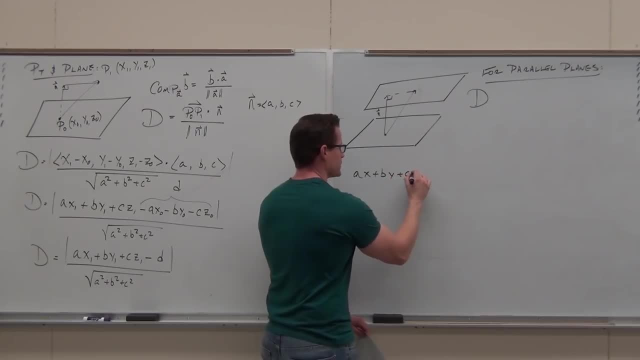 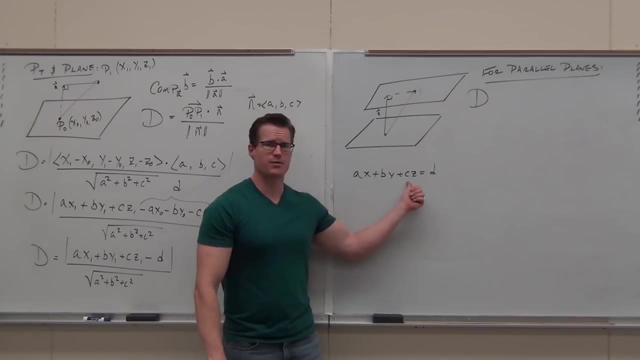 This is a plane. This is a plane. AX plus CZ equals D. If we have that, I say: hey, here's two planes and they're parallel. Are these numbers the same for parallel planes? Yes, Yes, Are these numbers necessarily the same? 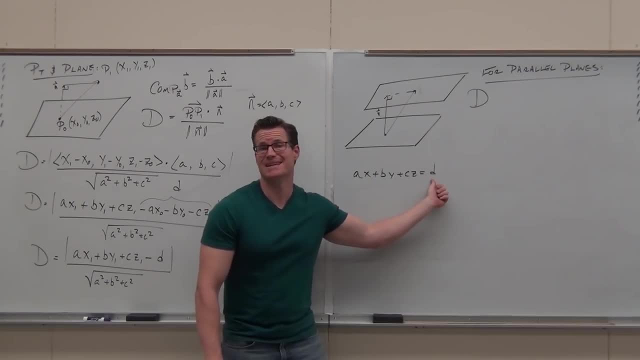 No, No. That's the only thing that could possibly be different And the only way that we get that different number is with that point. A different point gives us the different number. That's why that point in the normal vector to find a plane. 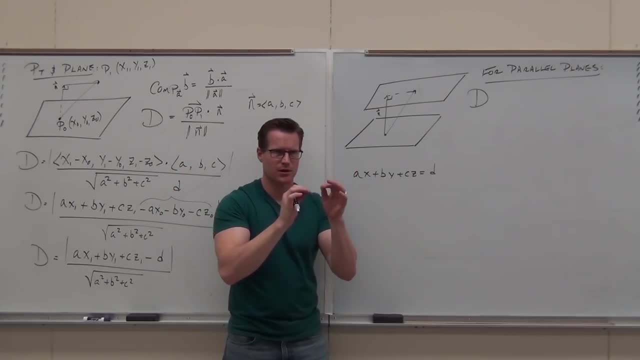 So if we have the same normal, the point is the only thing that's different. That point: when we distribute all of this, this stuff here, that point A, this, this, this and this, that's what gives us the D. 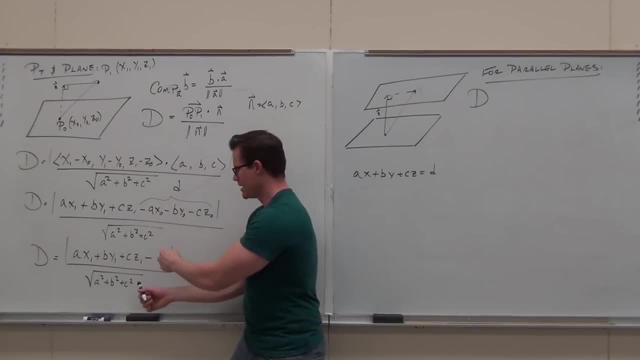 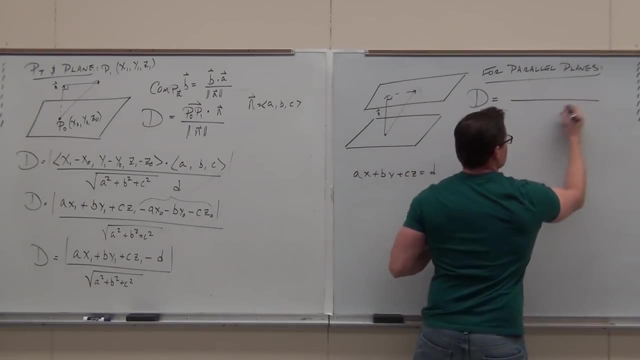 They're the same normal. All of this stuff disappears, except the two Ds. So if I want to find the distance between parallel planes, it ends up being this: You still have a normal, It's a common normal. It's still an absolute value. 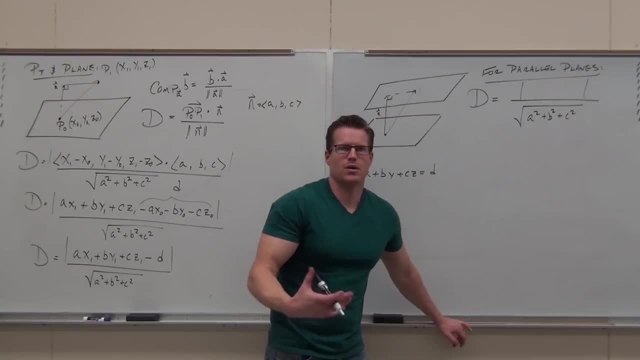 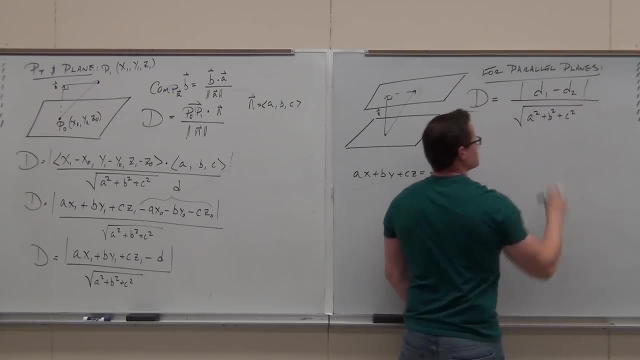 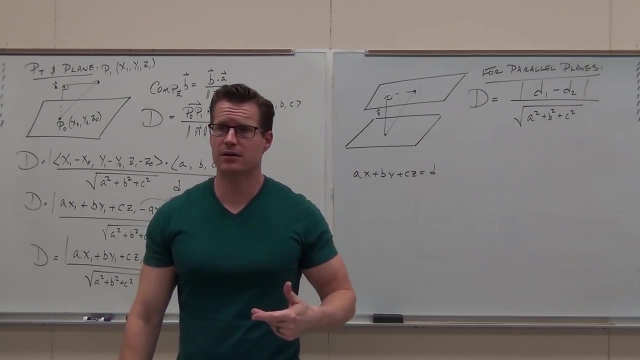 I want a positive. But the only problem- not problem the great part about it- the only difference between the planes is the Ds. Take the Ds, subtract them, find the absolute value of that divide by the magnitude, For instance. just so I can give you at least something. 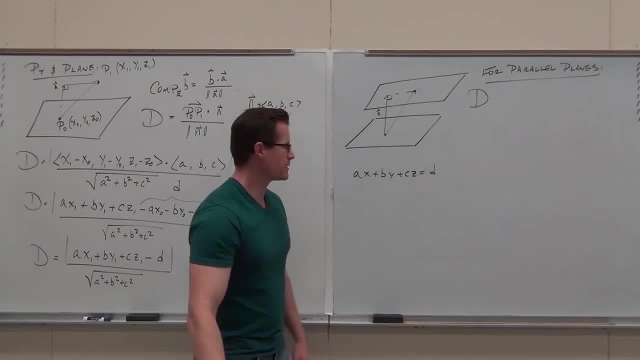 and cz equals d. If we have that, I say, hey, here's two planes and they're parallel. Are these numbers the same for parallel planes? Yes, Are these numbers necessarily the same? No, That's the only thing that can possibly be different. 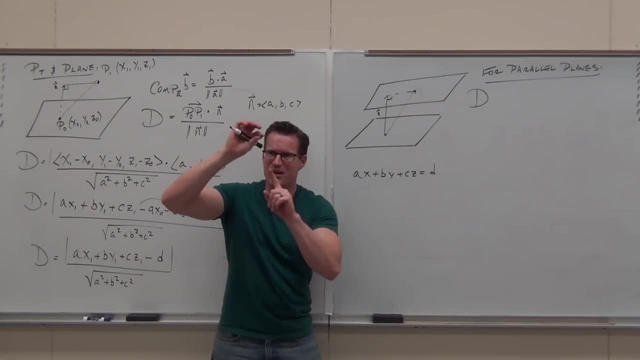 And the only way that we get that different number is with that point. A different point gives us the different number. That's why that point in the normal vector is different. That point when we distribute all of this stuff here, that point. 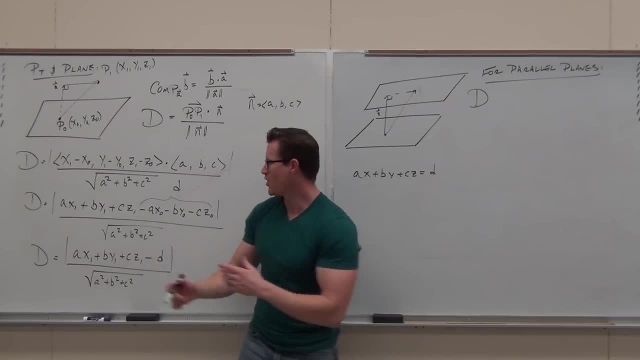 a this, this, this and this. that's what gives us the d. They're the same normal. All of this stuff disappears, except the two d's. So if I want to find the distance between parallel planes, it ends up being this: 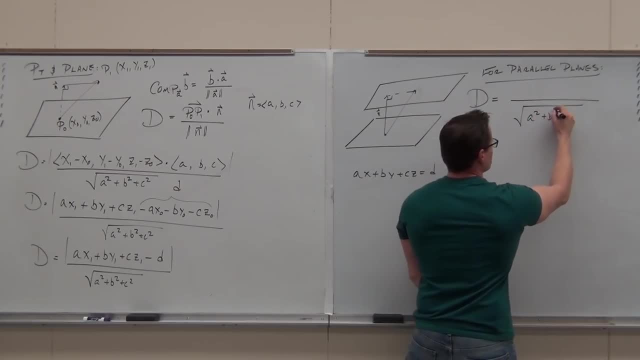 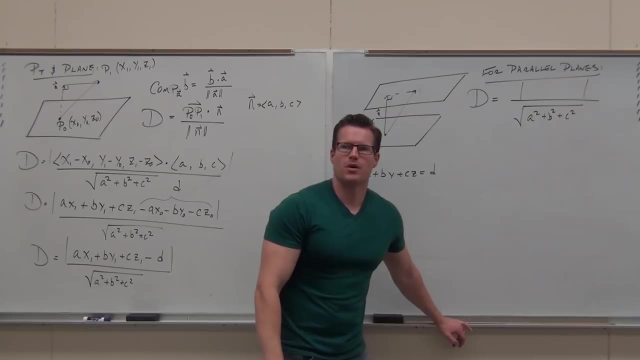 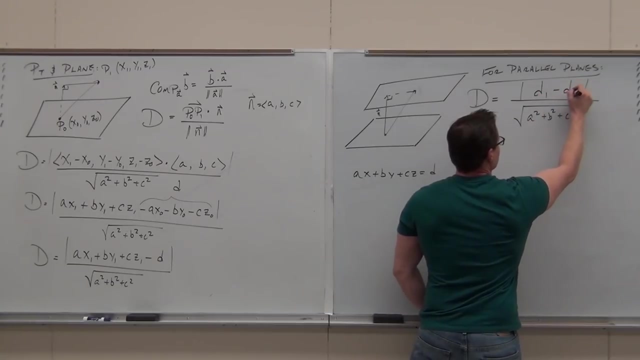 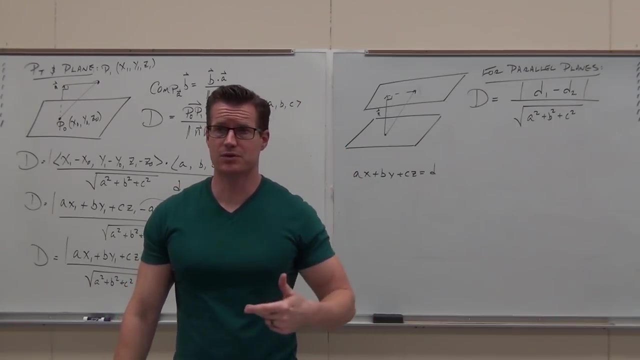 You still have a normal. It's a common normal. It's still an absolute value. I want a positive, But the great part about it, the only difference between the planes, is the d's. Take the d's, subtract them, find the absolute value of that. 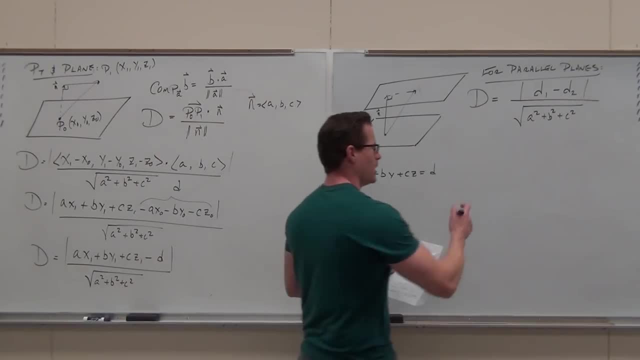 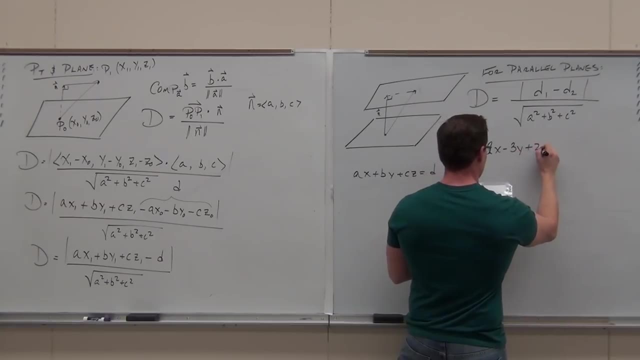 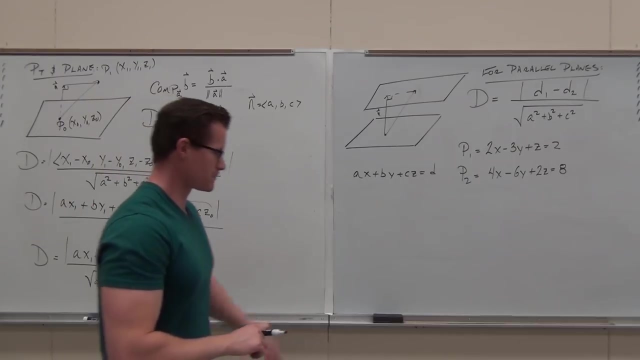 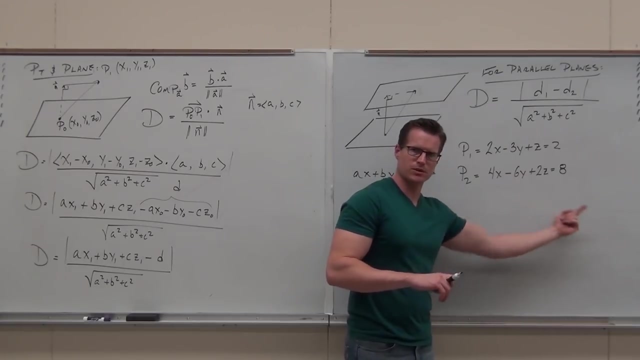 divide by the magnitude, For instance. just so I can give you at least something. I'm glad I'm doing this one too, because this is useful. This is not good, This is. don't give me things like this, don't deal with things like this. 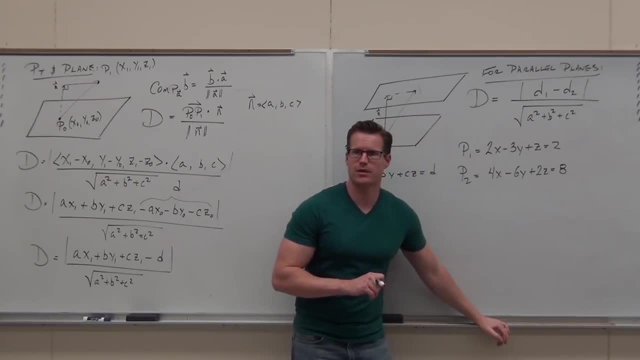 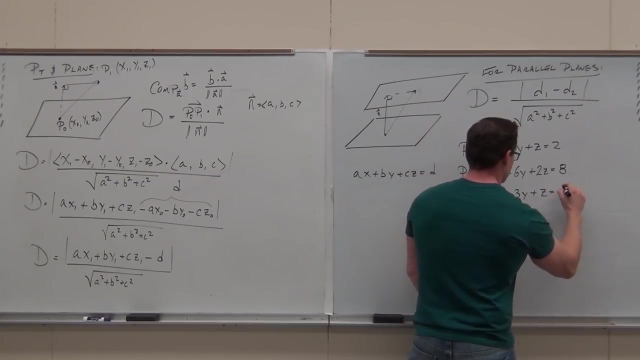 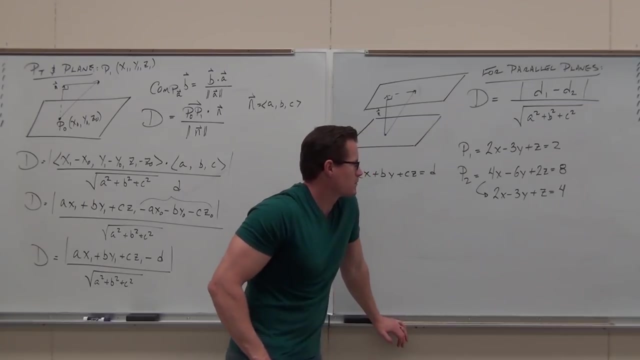 don't let this be. this shall not pass Right here. you can't divide a vector enough, and you should. So when you can divide everything by two, like in this case, do it True or false? Those are parallel. 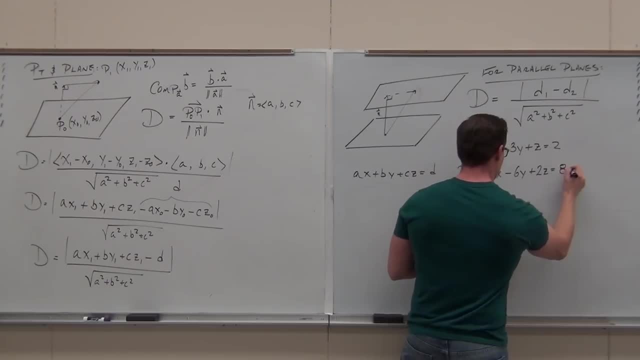 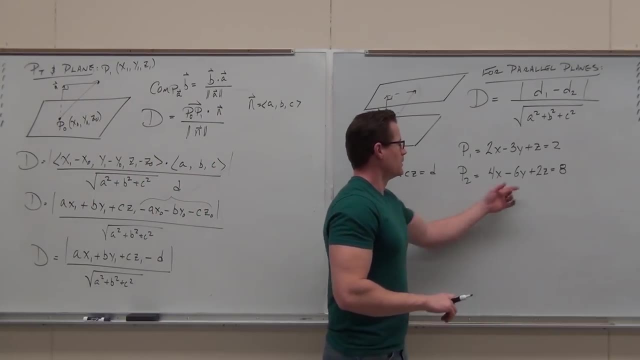 I'm glad I'm doing this one too, because this is useful. This is not good. This is: don't give me things like this. don't deal with things like this. don't let this be. this shall not pass Right here. do you see the problem with that? 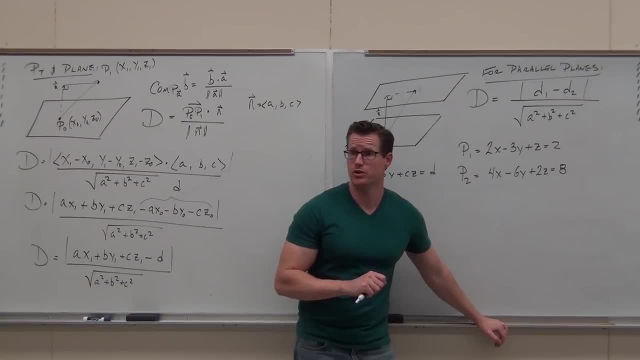 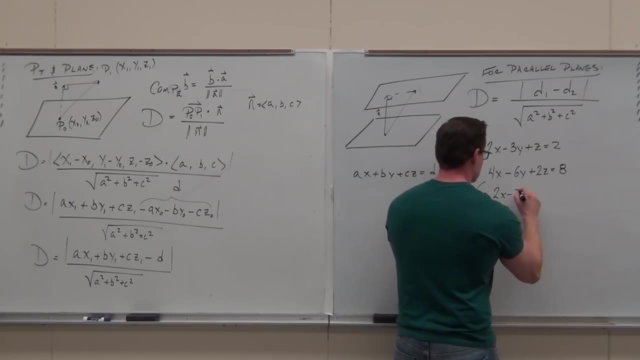 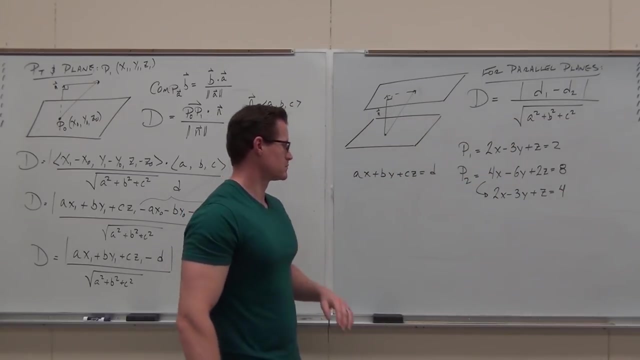 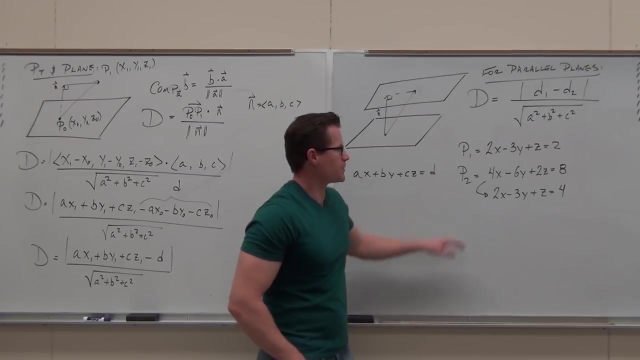 Someone didn't simplify their vector enough, and you should. So when you can divide everything by two, like in this case, do it True or false? Those are parallel. True If those are vectors, don't they both have the vector notation above the variable names? 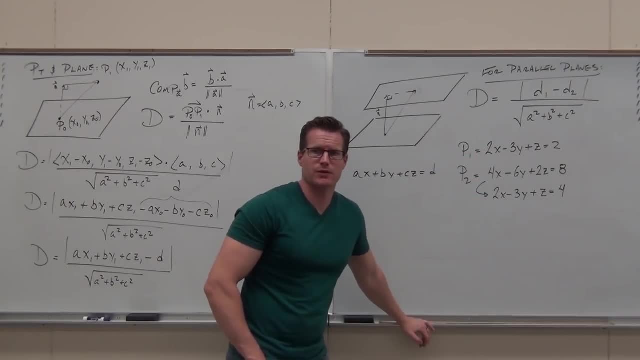 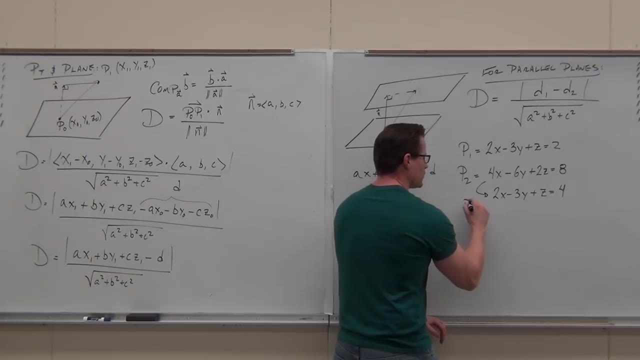 These ones? No, Those are planes. Okay, So, not vectors, just planes. What is the joint common? whatever you want to call that, what is the normal vector for this here? Two, three, four, five, six, seven, eight, nine, 10,, 11,, 12,, 13,, 14,, 15,, 16,, 17,, 18,, 19,, 20,, 21.. 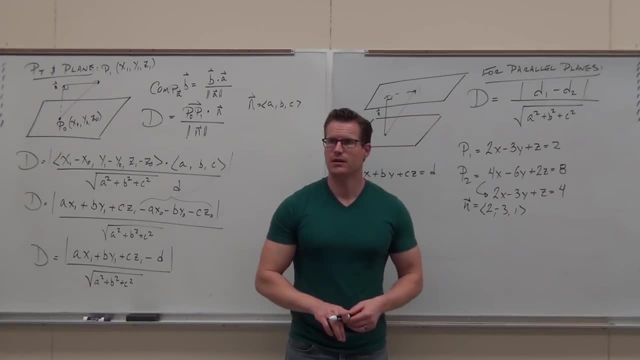 My notation keeps that's the normal vector right there. They share the same normal vector. They have to because they are parallel. They are parallel because they share the same normal vector And not if you give it that one. As soon as you simplify this, you can find the distance between these parallel planes. 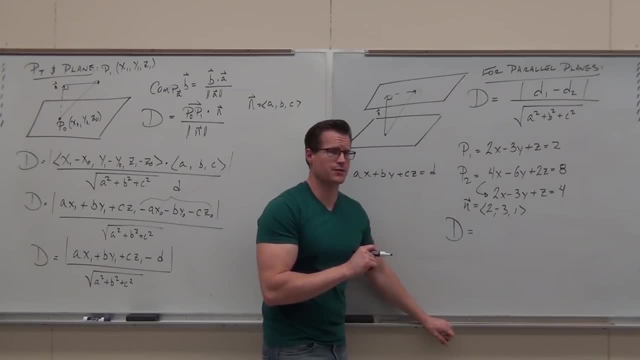 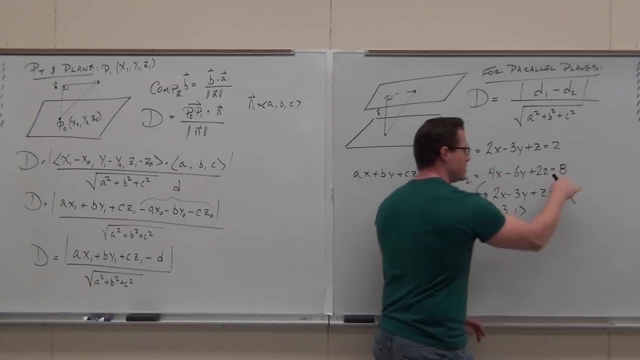 And it's very, very fast and very, very easy. Just don't use that, That number. you have to use a simplified one. So, as soon as you do it, this is the D. that's not the D. So we have our normal vector. 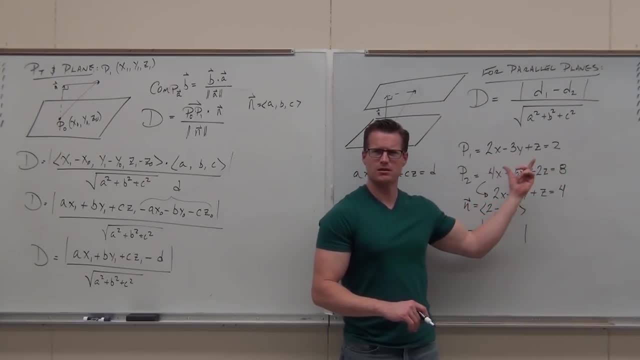 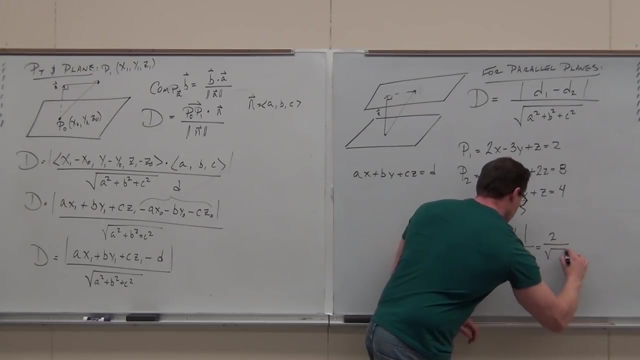 We've got our what's our. what's our D for for the first plane. What's our D? Two, Two, Two. What's our D for the second plane? Four, Four. That's the distance between those planes. 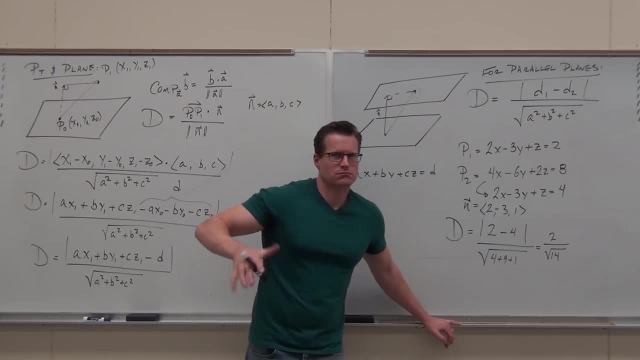 Yeah, square root of 14.. Are you guys okay with that one? Yeah, Proved it, but I want to make sure you see where the numbers are coming from, If you have to find distance between planes, and you know they're parallel, hey. 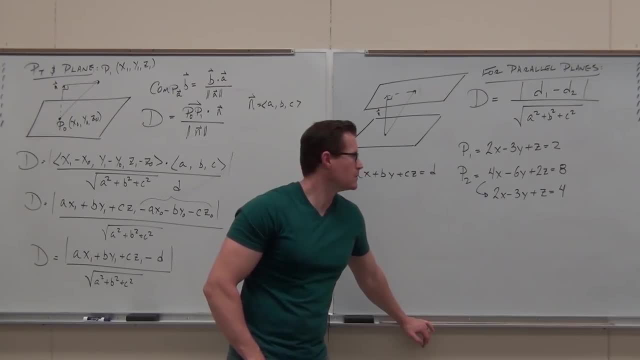 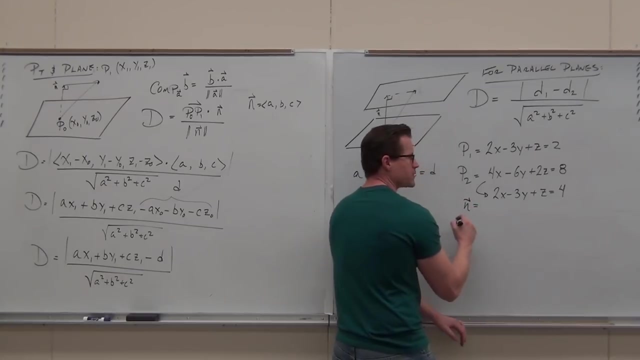 True, If those are vectors, do you have variable names? These ones, No. those are planes. So not vectors, just planes. What is the joint common? whatever you want to call that, what is the normal vector for this here? 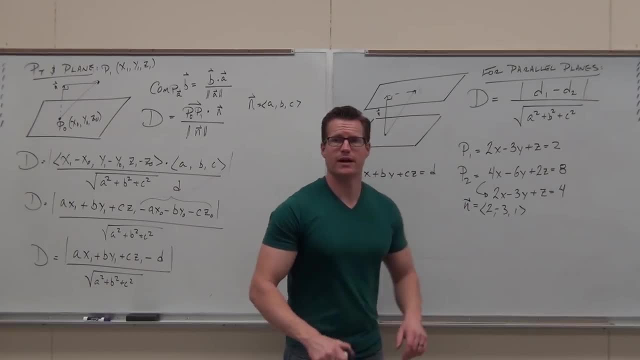 Got my notation pp's. That's the normal vector right there. They share the same normal vector. They have to because they are parallel. They share the same normal vector. As soon as you simplify this, you can find the distance between these parallel planes. 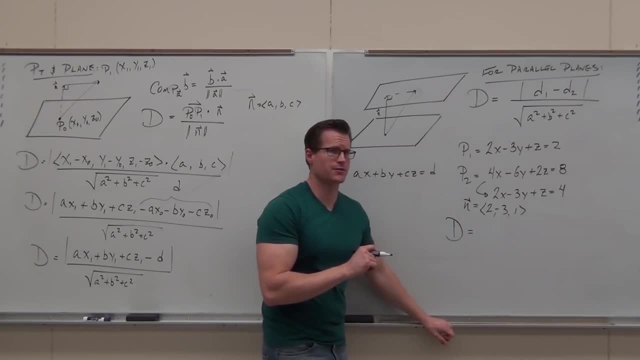 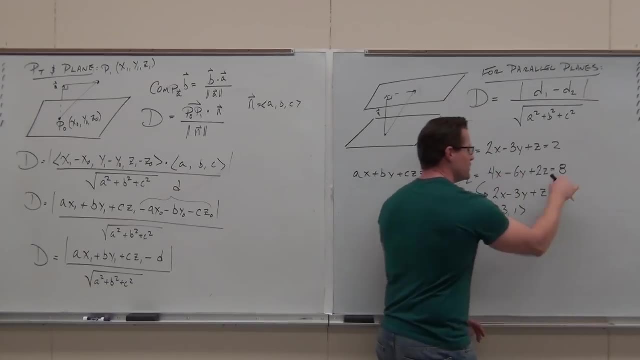 and it's very, very fast and very, very easy. Just don't use that number. You have to use a simplified one. So, as soon as you do it, this is the d. that's not the d. So we have our normal vector. 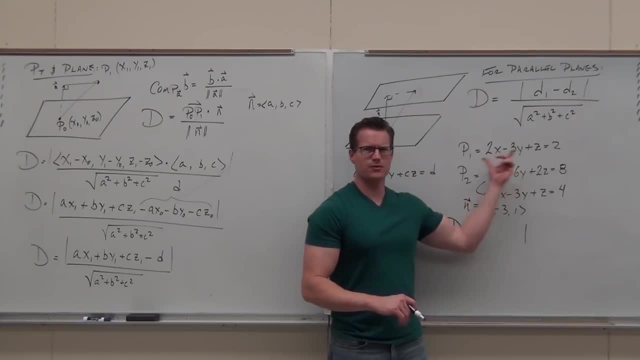 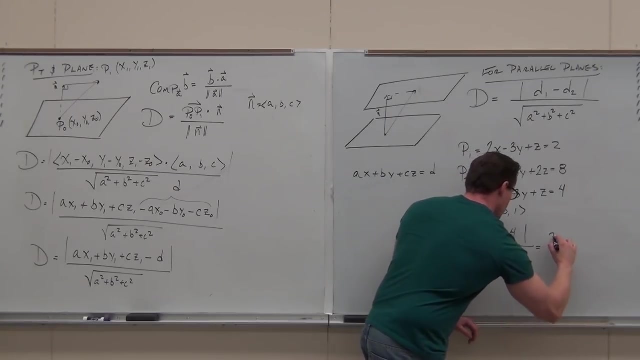 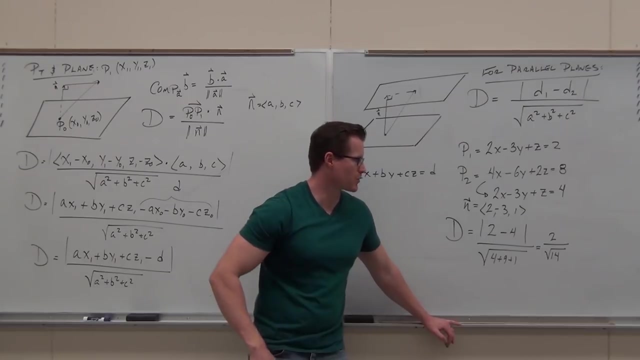 we've got our. what's our d for the first plane? What's our d? 2. What's our d for the second plane, 4. That's the distance between those planes. Are you guys okay with that? one Proved it, but I want to make sure. 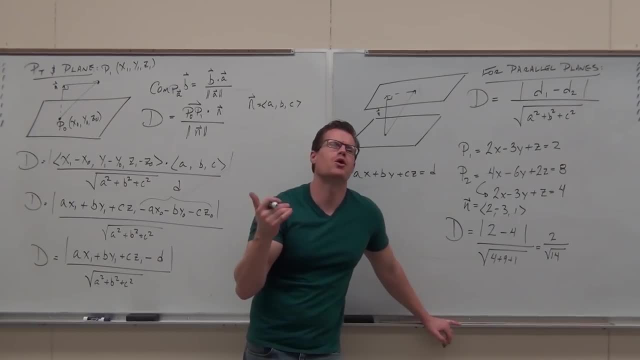 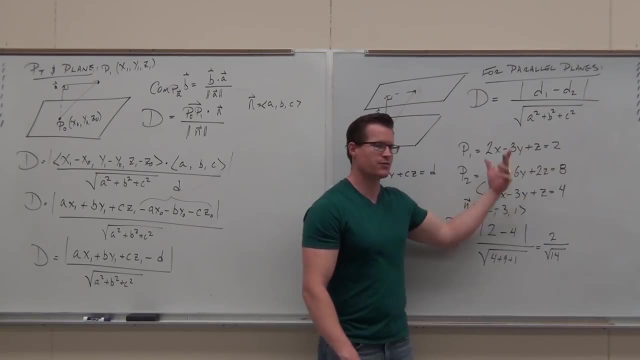 you see where the numbers are coming from. If you have to find distance between planes that are parallel, hey, take these two d's, subtract them, whatever order, It doesn't matter. Absolute value says it doesn't matter. Subtract them. divide by the magnitude. 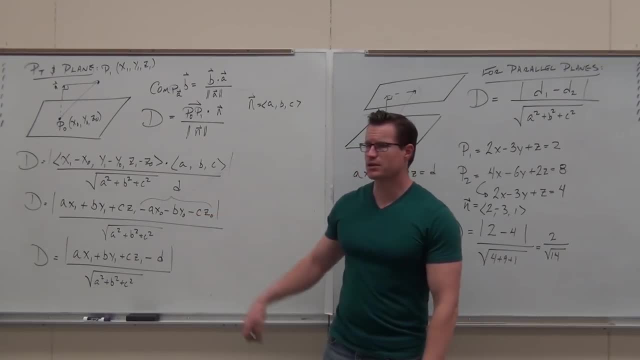 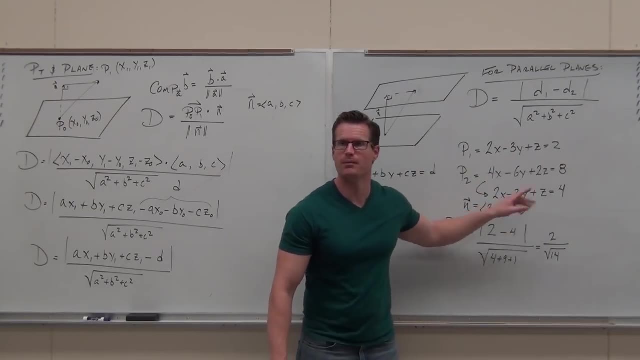 of the normal vector and you're good to go. I want to go back to this for just a second, just to prove it by an example. What if you didn't know they were parallel? You freaking should, But if you didn't? 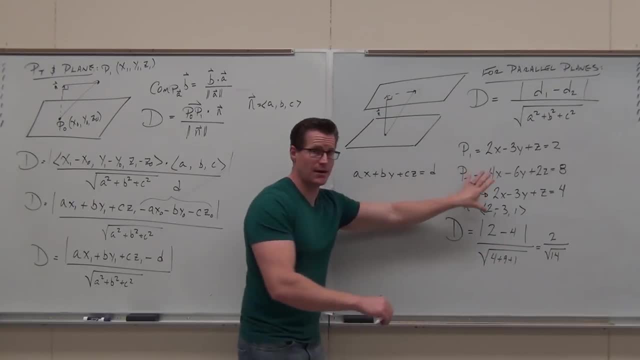 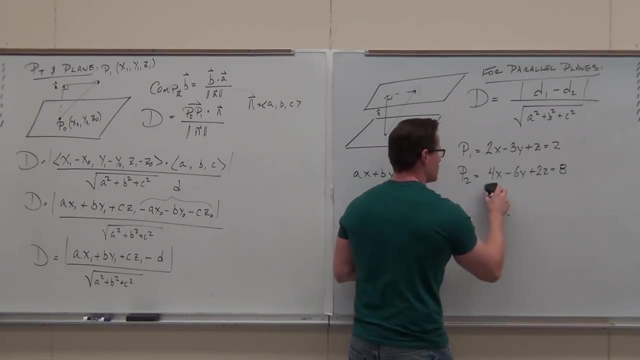 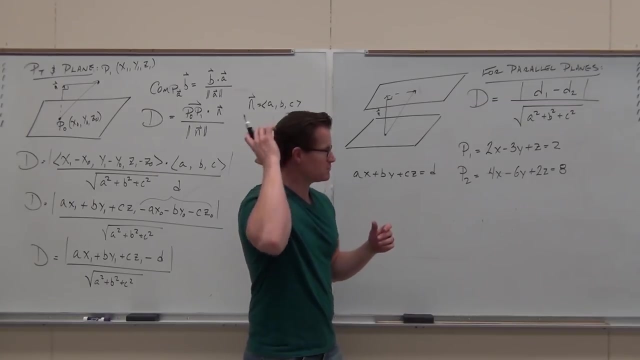 if you didn't know. do you have this down? Can I erase it? Remember, 2 over root 14, okay, So let's say you didn't know, You go. if I don't know they're parallel, well, you should. 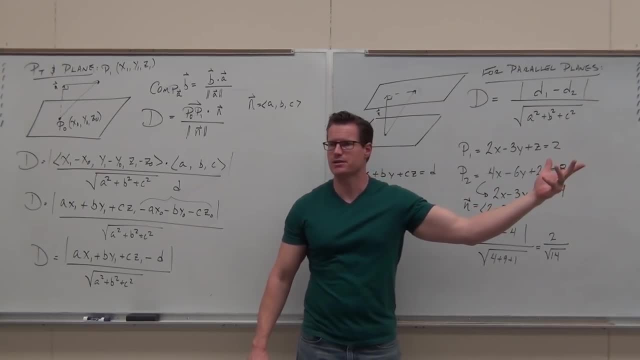 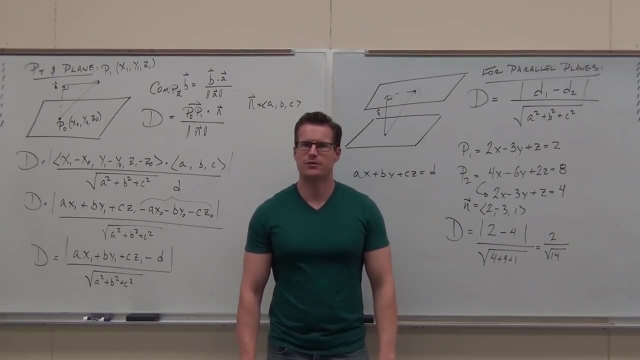 take these two D's, subtract them whatever order, it doesn't matter. Absolute value says it doesn't matter. Subtract them, divide by the magnitude of the common vector and you normal vector and you're good to go. Head nod if you're okay with that one. 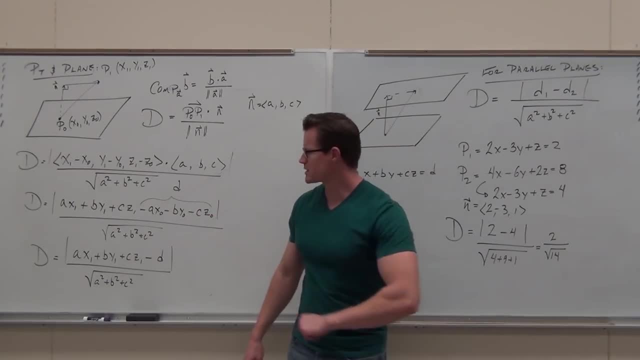 I want to go back to this. I want to go back to this for just a second, just to prove it. just to prove it by an example. What if you didn't know they were parallel? Freaking should, okay, But if you didn't, if you didn't know, then you'd find a point on this plane. 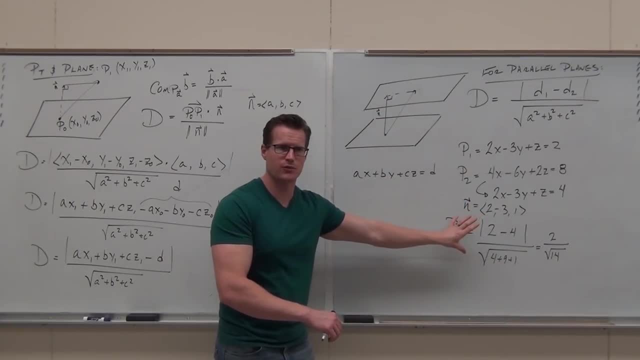 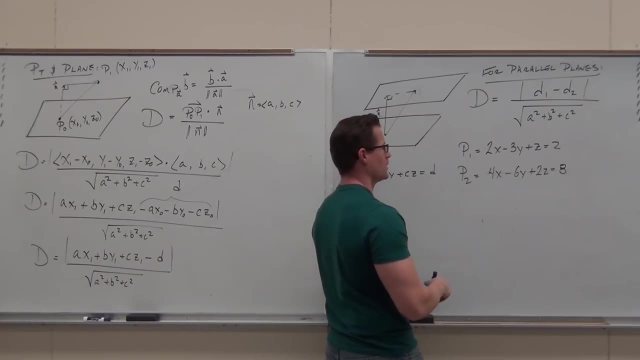 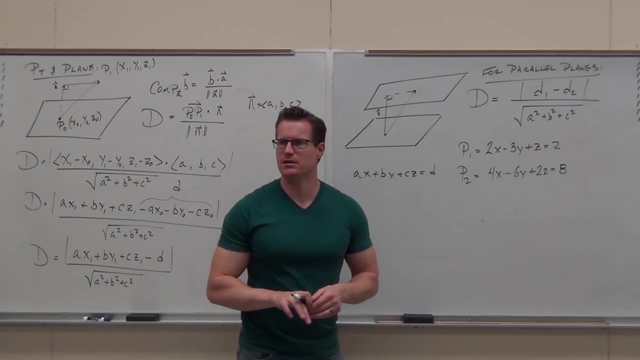 So do you have this down? Can I erase it? Remember: 2 over root 14, okay, So let's say you didn't know, You go. if I don't know they're parallel, well, You should. but if you didn't, then you had to. you should check, but if you didn't. 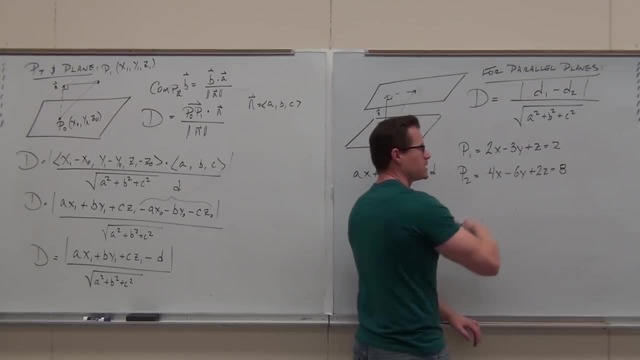 I'll find a point on it, because I wouldn't be able to do it that way. To find a point on a plane, any point on a plane, you can set two variables equal to zero and find out where it crosses an axis. Planes will cross the axis unless it's parallel to the axis. 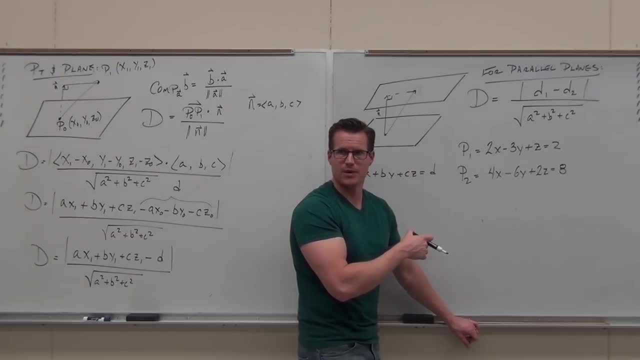 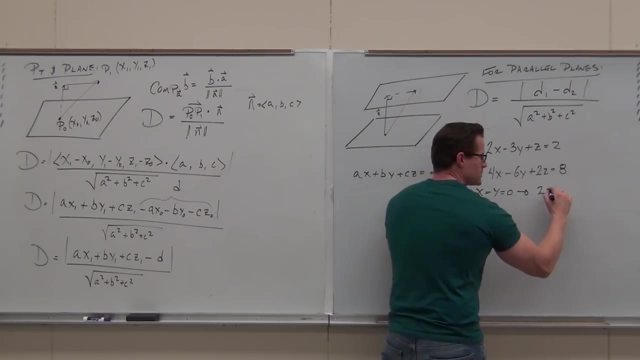 If it's parallel to the axis, you wouldn't have that variable. Any time you have a variable, you have to cross that axis. This stuff should be ringing a bell. so if I set x equal to y equal to zero, I get 2z equals 8 or z equals 4.. 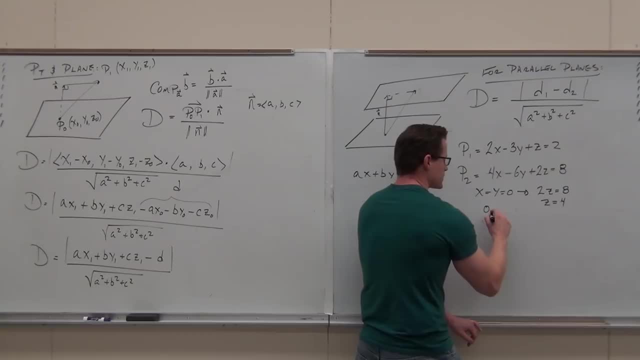 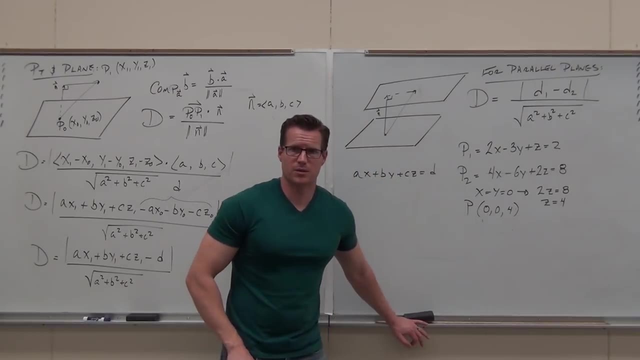 I get z equals 4.. There's a point there. It's 0, 0, 4.. That is a point on plane number 2.. That is a point on plane number 2.. It's actually the point where plane number 2 crosses the z axis. 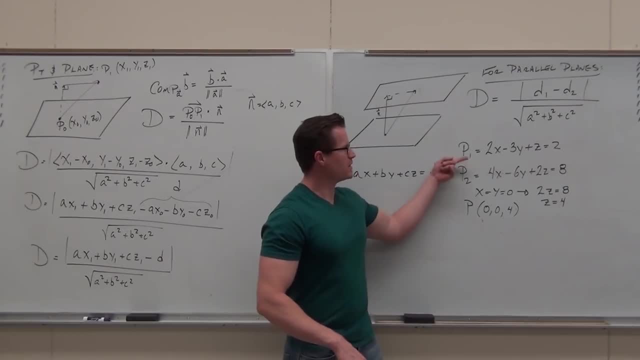 That's what's going on. If I said: how far is this point from that plane? Here's how you do it. It's right here. So if you didn't know they were parallel, If they were parallel, you have this as your back-end plane. 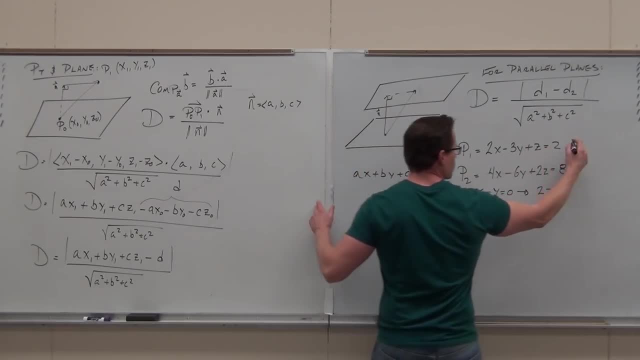 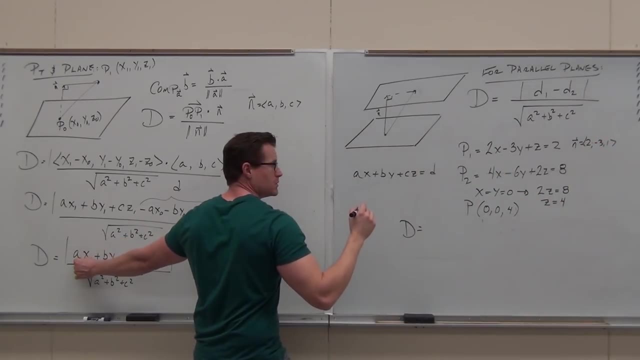 I want to show you so you see where it works. Here's our normal. We put 2, negative, 3,, 1, and 2.. Here we put 0,, 0, and 4.. Do you see where those numbers are coming from? 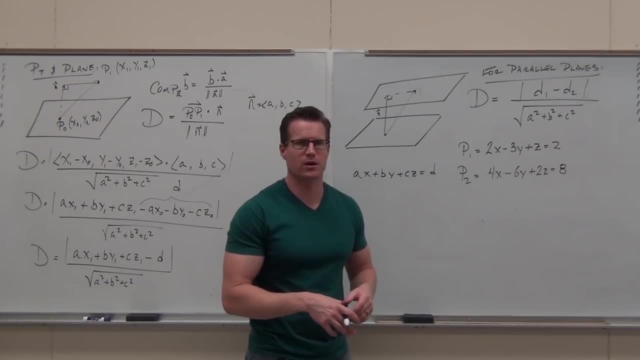 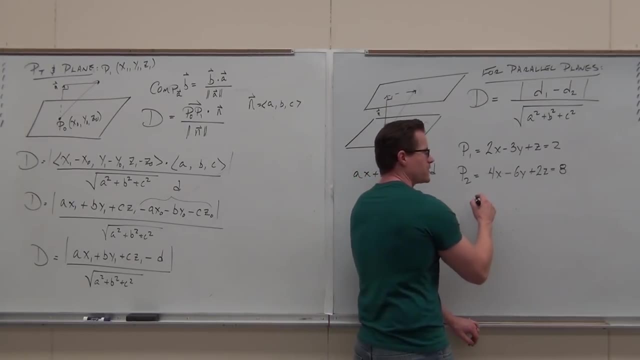 But if you didn't, you should check. I'll find a point on it. To find a point on a plane, any point on a plane- you can set two variables- x equal to 0, and find out where it crosses an axis. 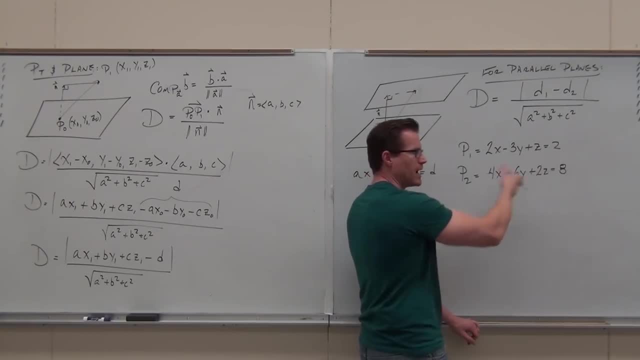 Planes will cross the axis unless it's parallel to the axis. If it's parallel to the axis, you wouldn't have that variable. Anytime you have a variable, you have to cross that axis. The sub should be ringing a bell. 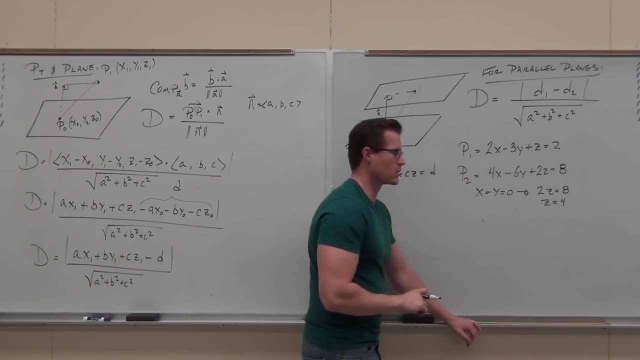 So if I set x equal to y equal to 0,, I get 2z equals 8, or z equals 4. I get z equals 4.. There's a point there. It's 0, 0, 4.. 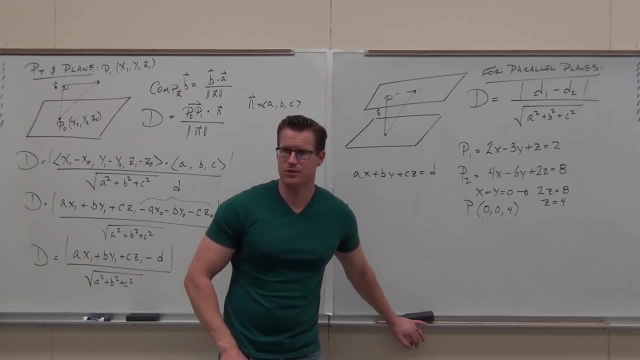 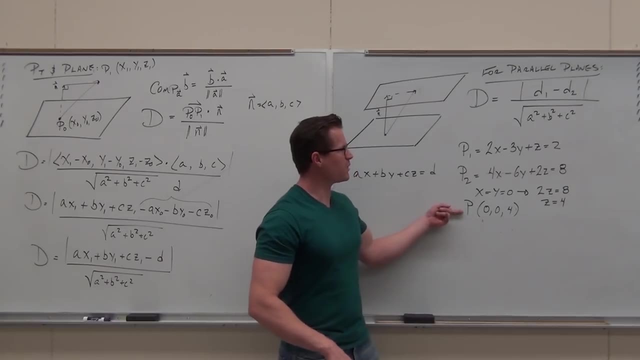 There's a point on plane number 2.. That is a point on plane number 2.. It's actually the point where plane number 2 crosses the z axis. That's what's going on. If I said: how far is this point from that plane? 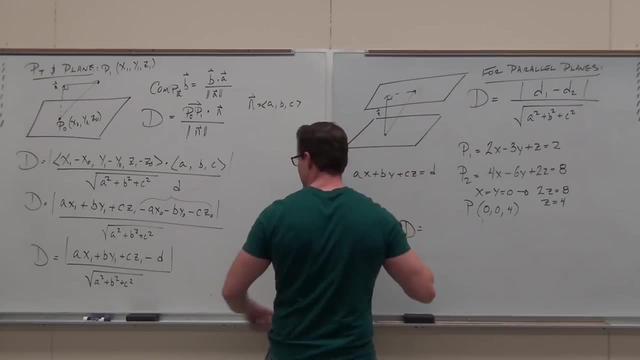 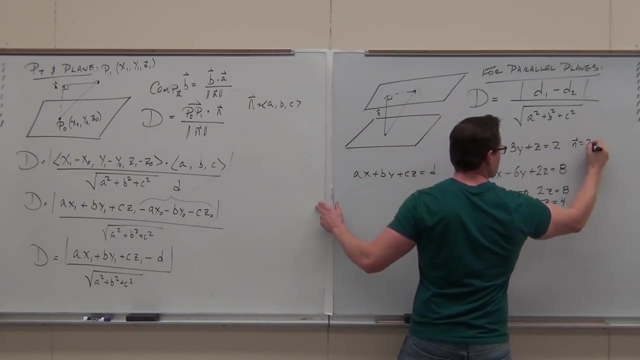 Here's how you do it. It's right here. So if you didn't know they were parallel. you have this as your back-end plan. I want to show you so you see where it works. Here's our normal. We put 2. 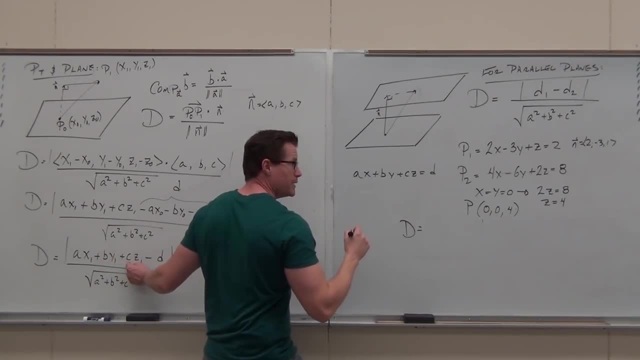 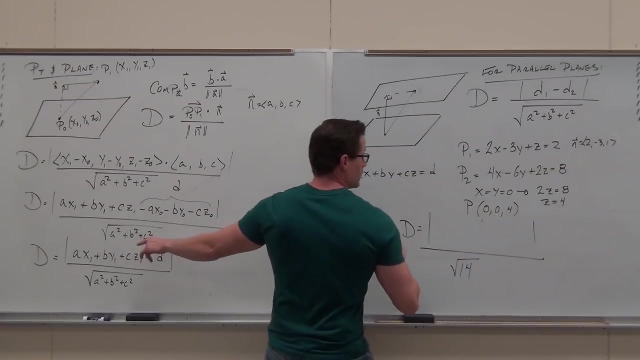 made of 3, 1 and 2. Here we put 0,, 0, and 4.. Do you see where those numbers are coming from? Square root of 14,, because I already did it. What is it again? 2 times 0.. 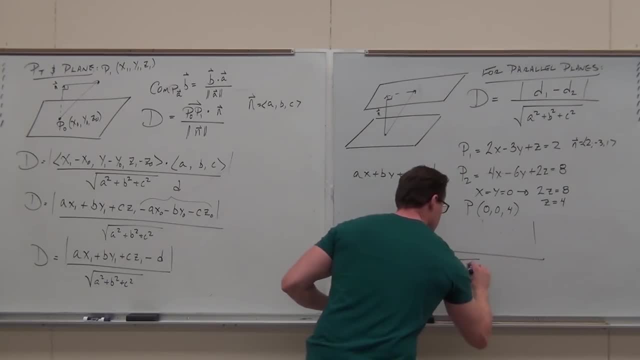 Okay, Okay. so I'm going to ask it by square root of 14, because I already did it. I'm going to ask it by square root of 14 because I already did it. What is it again? 2 times 0.. 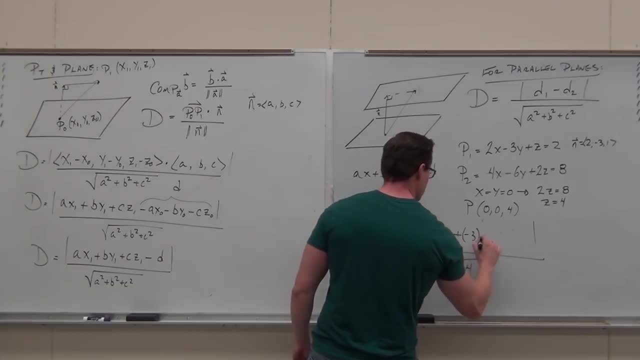 Plus Negative 3 times 1.. Negative 3 times 1.. Plus 1 times 4.. How much 1 times 4.. Uh-huh, Do you see where the 1 times 4 is coming from? 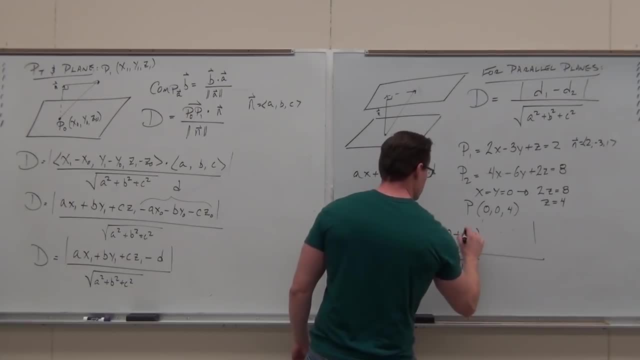 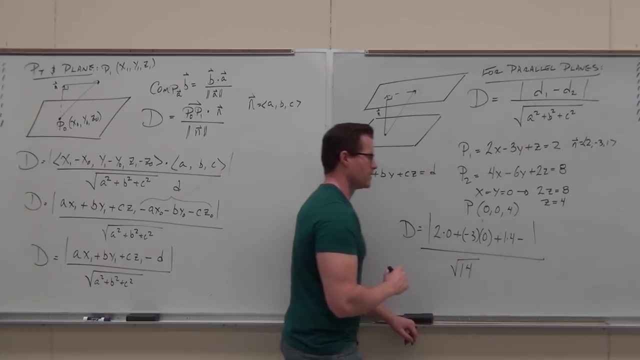 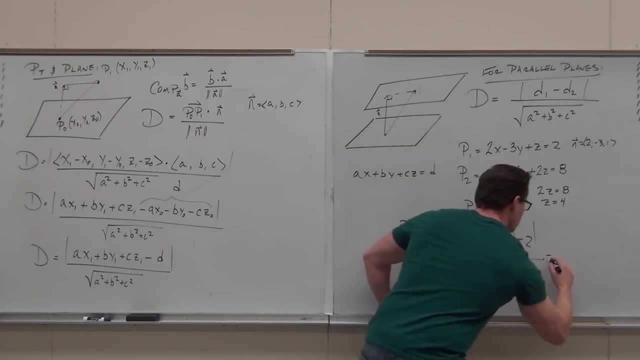 Plus Plus How much? 1 times 4.. Uh-huh, Do you see where the 1 times 4 is coming from? Is it minus 0, 0,? That's how you find the distance between any point in a plane. 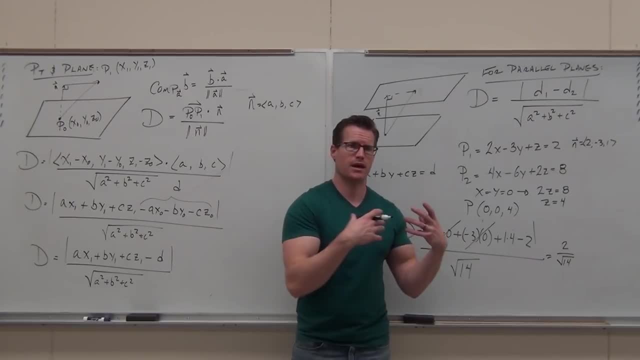 You literally plug in x, y, z coordinates and the x- y, z components of the normal vector divide by the magnitude of the normal. That's all there is to it. It works out the same Why? Because those planes were parallel. 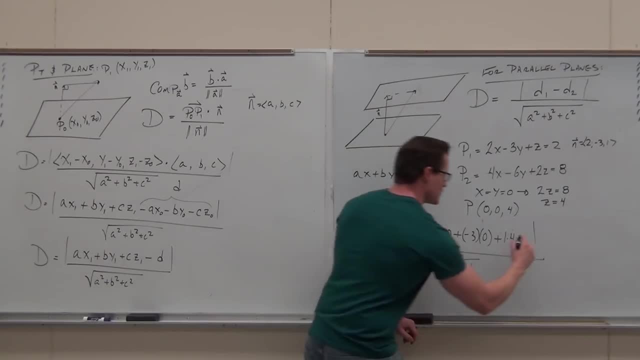 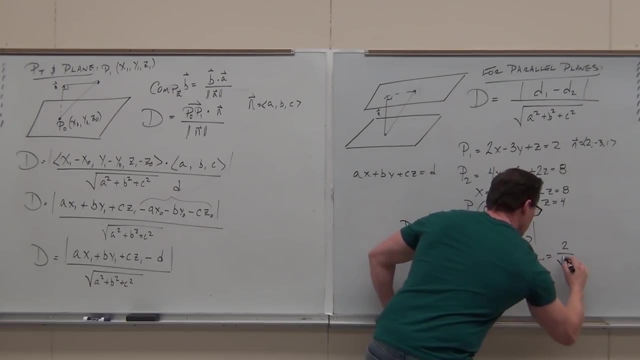 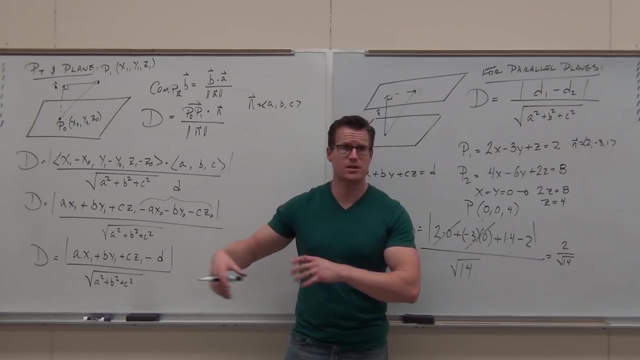 Yeah, Is it minus 0, 0.. That's how you find the distance between any point in a plane. You literally plug in x, y, z coordinates and the x, y, z components of the normal vector Divide by the magnitude of the normal. 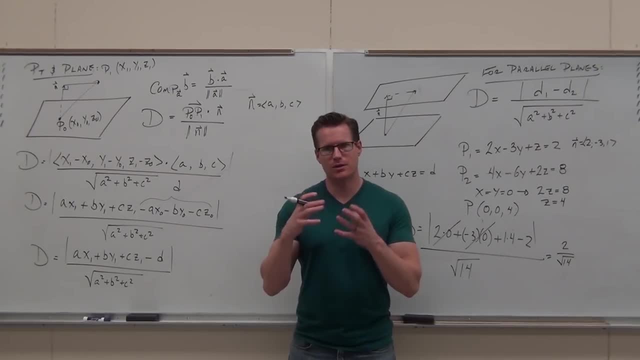 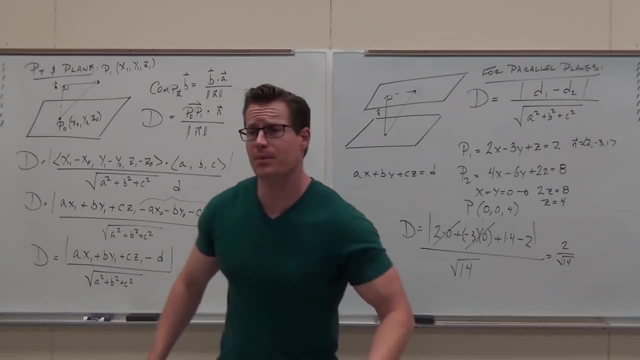 That's all there is to. it Works out the same. Why? Because those planes were parallel. That's why We've got two more things to do and then we're going to be done. We're so close. I want to wrap it up. 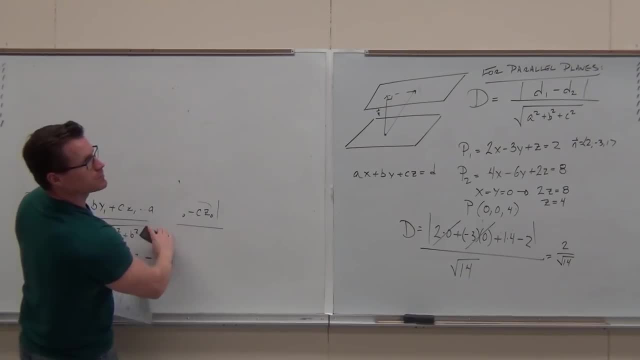 I want to give you the idea for skew lines. Here's just the idea for skew lines. Distance between skew lines. Show me with your hands what skew lines look like. Can you do that? What is skew? What do skew lines look like? 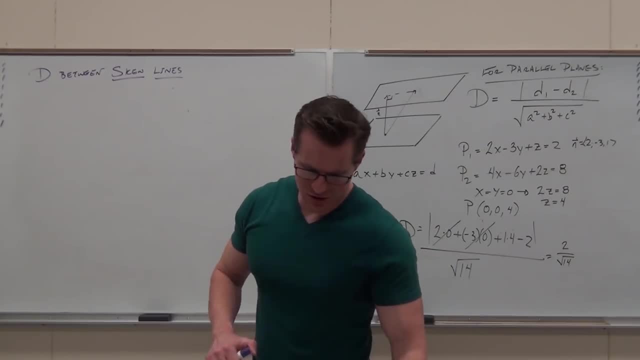 Yeah, don't throw gang signs at me. okay, Skew lines don't meet in space, but they're not parallel. So here's the idea: If lines are skew, they have to be contained by planes which are parallel. You have to be able to find parallel planes which contain those skew lines. 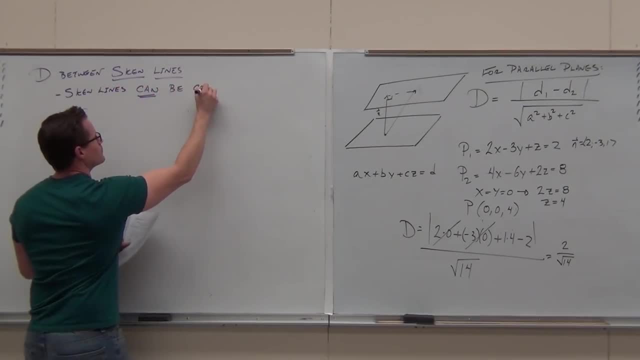 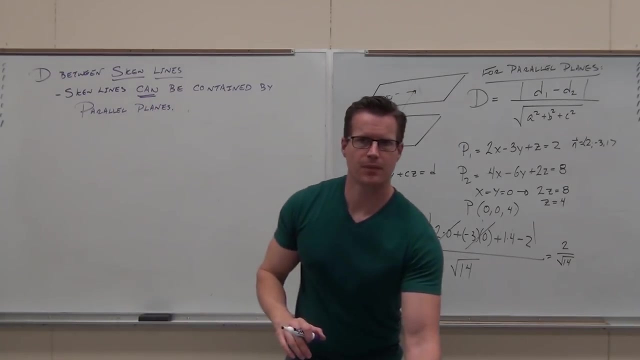 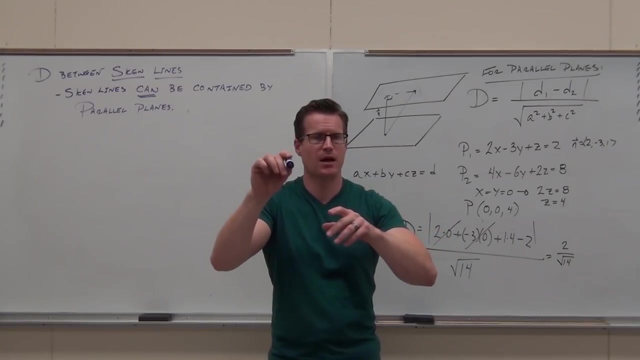 Did you catch that? There's an infinite number of planes that can contain a line. You have one line. There's billions of planes that can contain that, But as soon as I have another skew line, I pick one here and one here that are parallel. 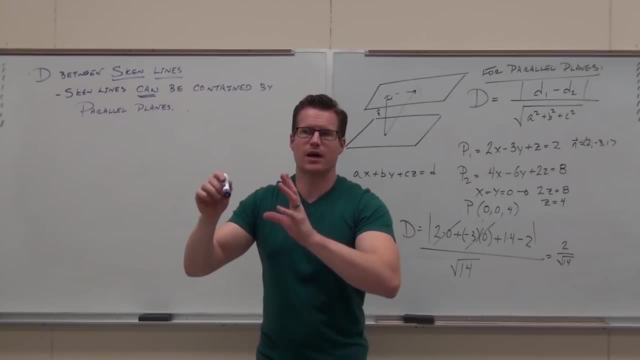 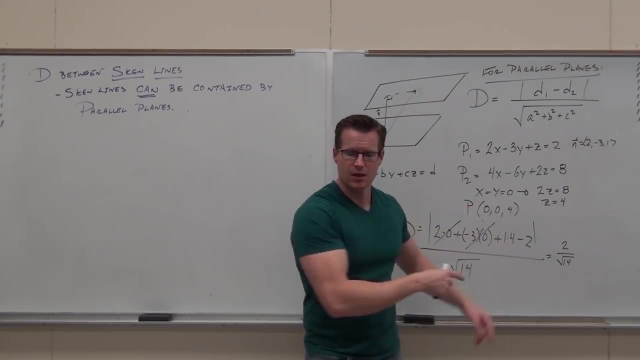 Does that make sense to you? I do that, Okay, so the idea is, define those parallel planes, then use that distance between parallel planes How we can, how we can, and that'll be the shortest distance. So how we can do that. lines have direction vectors. 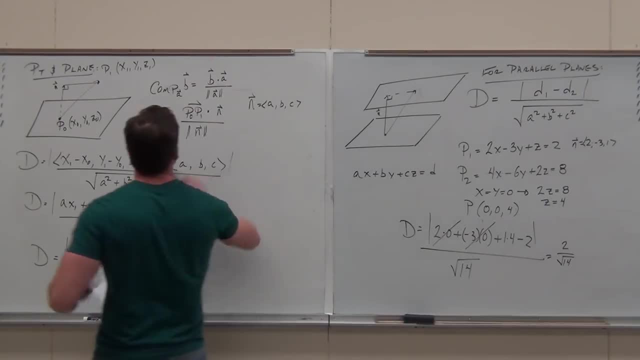 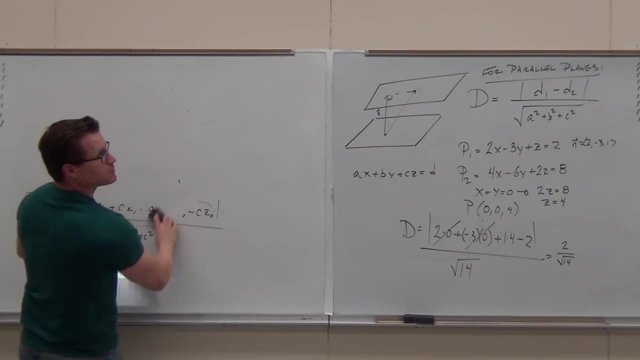 That's why We've got 2 more things to do, and then we're going to be done. We're so close. I want to wrap it up. I want to give you the idea for skew lines. Here's just the idea for skew lines. 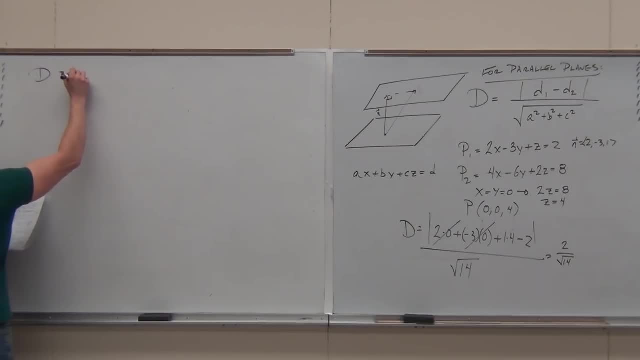 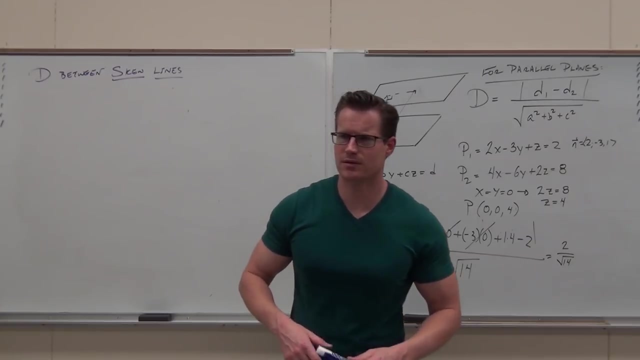 Distance between skew lines. Show me with your hands what skew lines look like. Can you do that? What do skew lines look like? Yeah, Don't throw gang signs at me. okay, Skew lines don't meet in space, but they're not parallel. 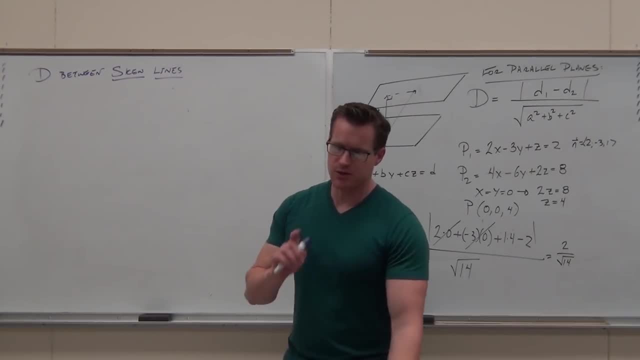 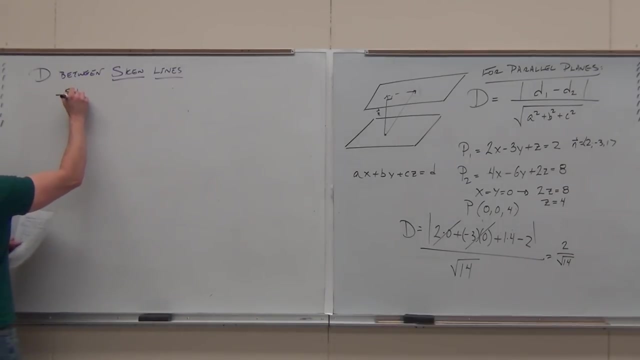 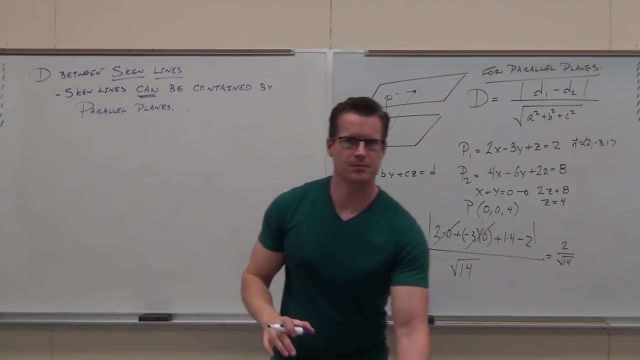 So here's the idea: If lines are skew, they have to be contained by planes which are parallel. You have to be able to find parallel planes which contain those skew lines. Did you catch that There's an infinite number of planes that can contain a line? 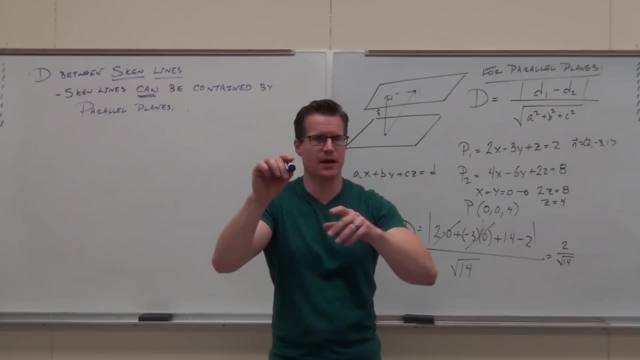 You have one line, there's billions of planes that can contain that. But as soon as I have another skew line, I pick one here and one here that are parallel. Does that make sense? I do that. So the idea is define those parallel planes. 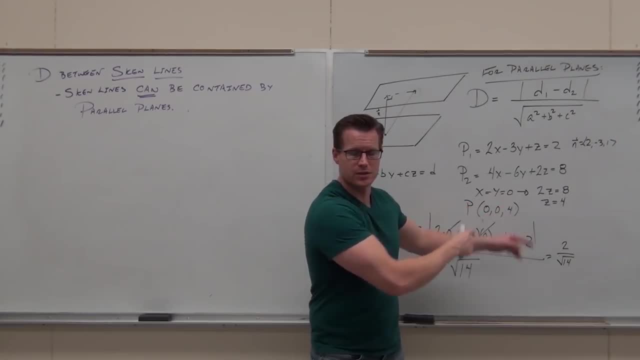 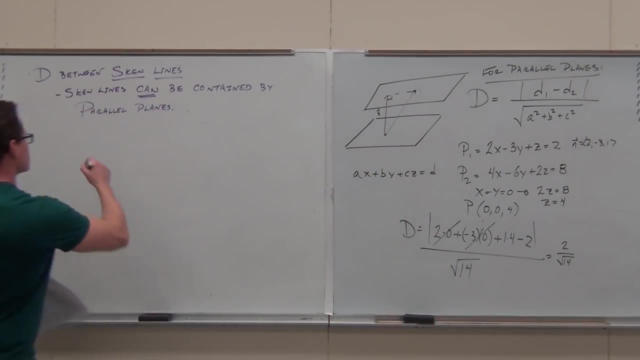 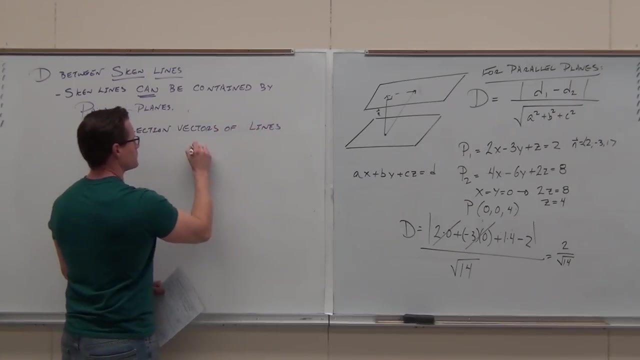 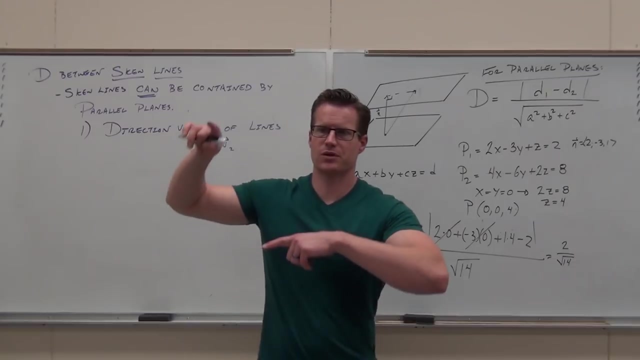 then use that Distance between parallel planes And that will be the shortest distance. So how we can do that, Lines have direction vectors. So what you would do first you'd find the direction vectors of your lines If those direction vectors are in planes that are parallel. 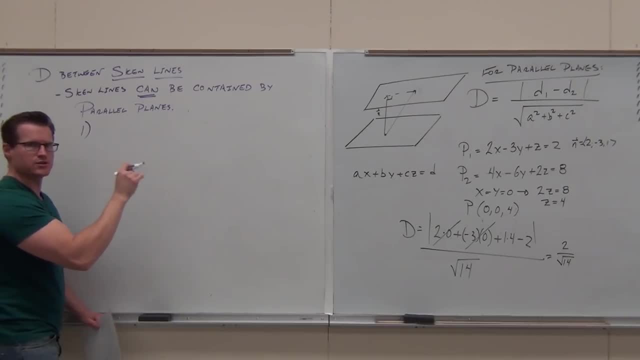 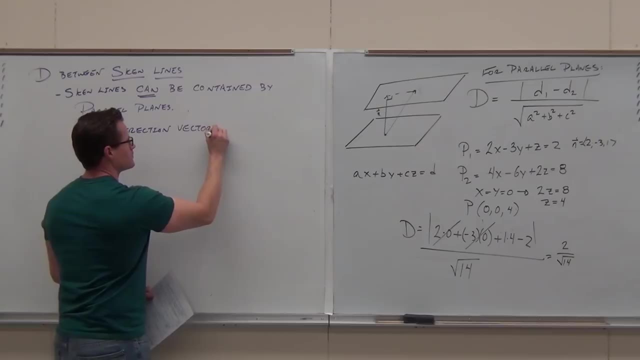 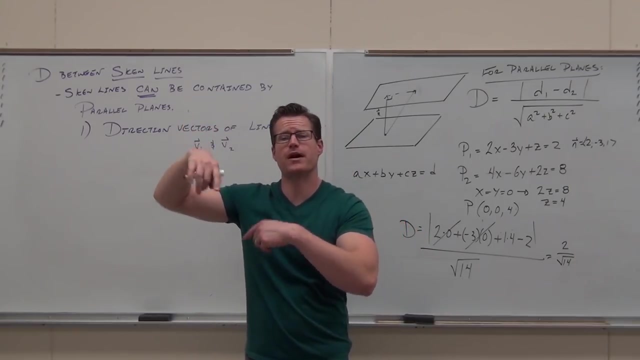 So what you would do: first you'd find the direction vectors of your lines. If those direction vectors are in planes that are parallel, they will have a common normal. You find the normal between those vectors. That'll be the normal of the plane. 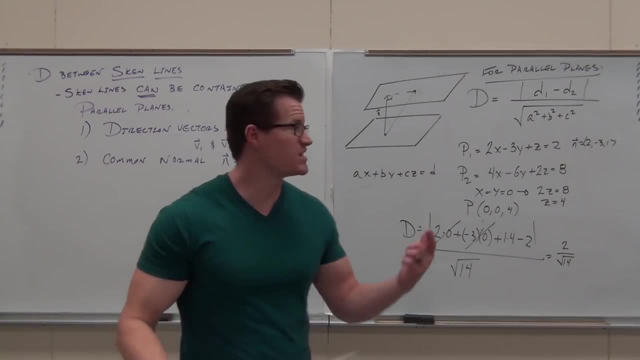 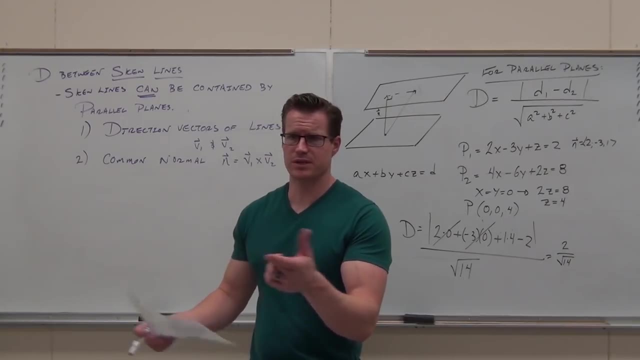 Every line is given. we've had some lines that are parallel. I'll have one right now, But every line is given to you with at least one point, correct? Yep? You just plug in: t equals zero, you get a point. 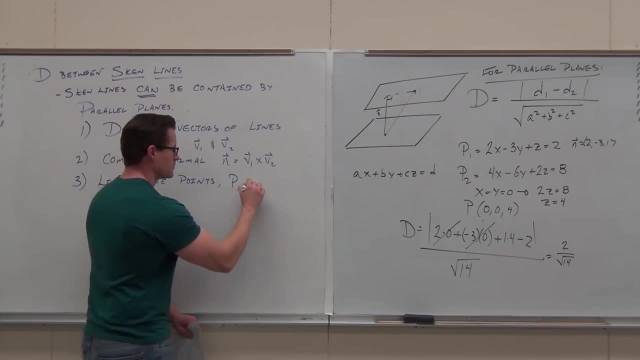 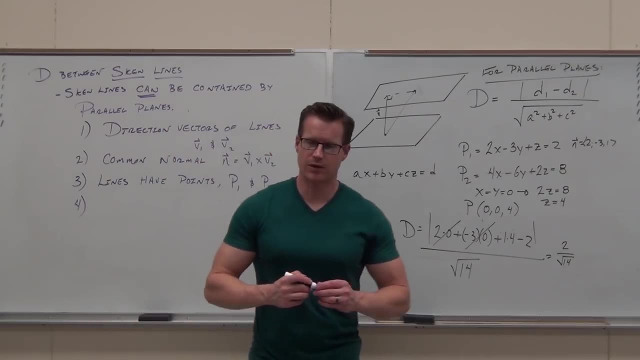 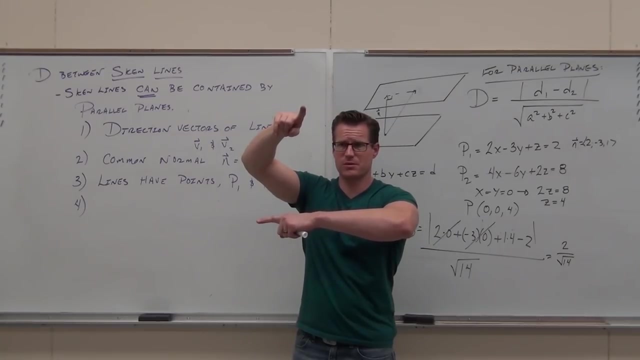 Lines have points. Two lines, two points. I know that's a lot at one time. If you've got lines like this, they've got direction vectors like this. consider them to be contained in parallel planes. Planes need a normal. 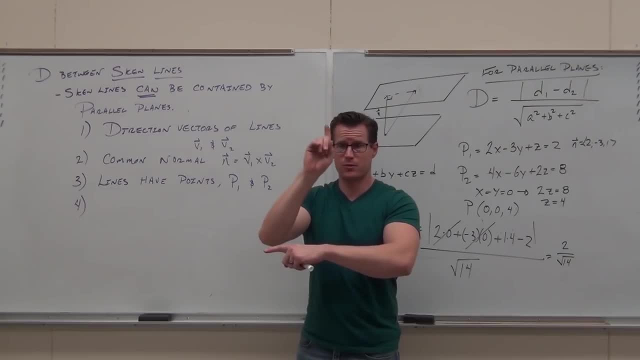 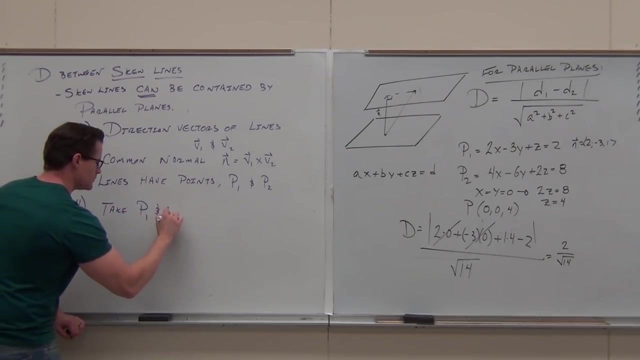 Cross them to find your normal. Now you have a normal for both planes. Lines have points. Take the normal with each independent point. find the equation of the planes. Lines have points. Take the normal with each independent point. Take the normal with each independent point. 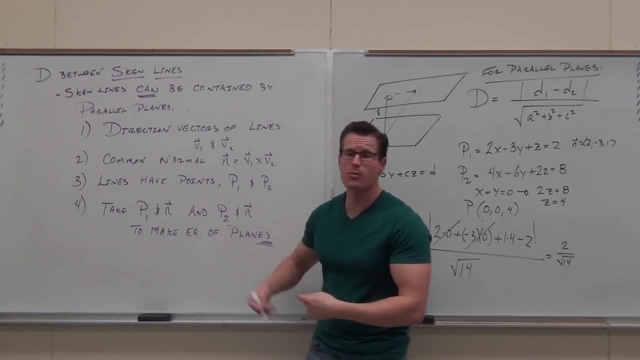 Those planes will be parallel. They have the same normal. They can't be anything other than parallel. So when you find those two planes that are parallel, you have the equation right. Those equations are going to have some D's in them. 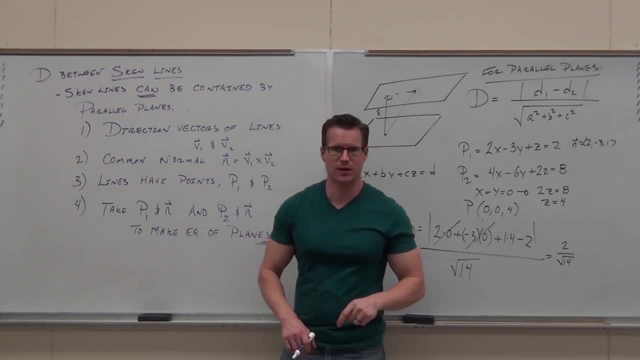 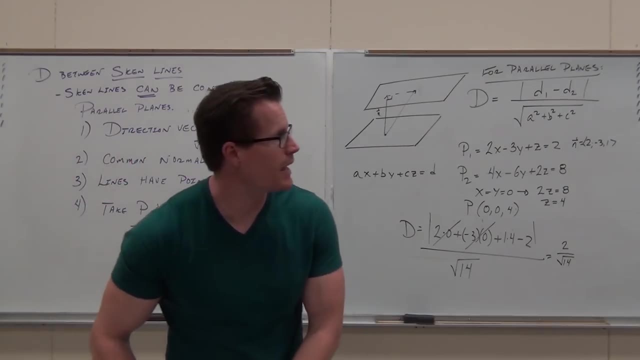 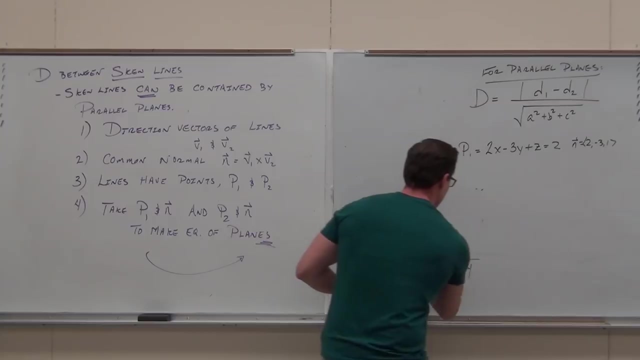 Take the D's, take the common normal distance between parallel planes. So, after this stuff, distance between parallel planes. That's the idea on how you would do it. The last thing that we're going to do, We're going to do how to find the distance between a line and a point. 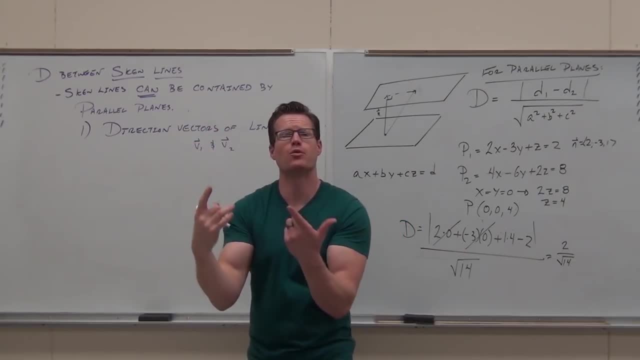 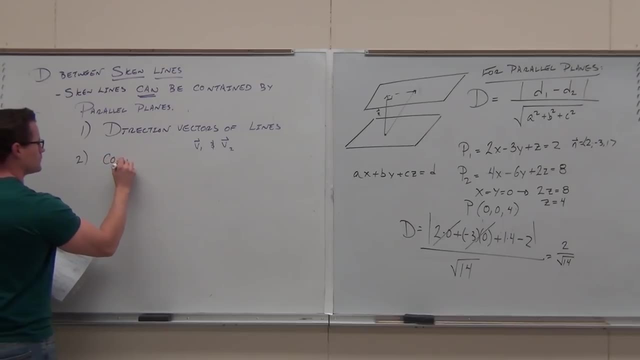 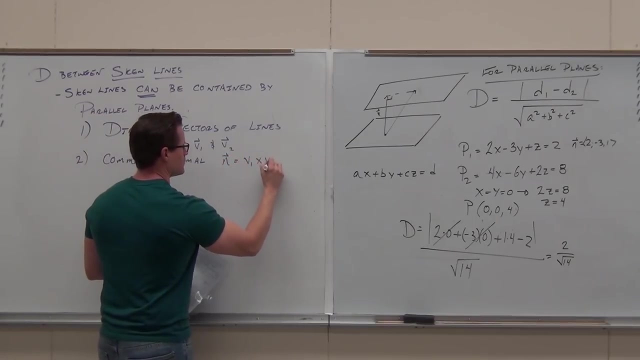 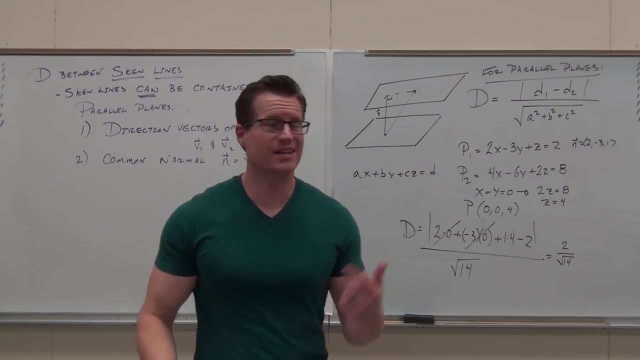 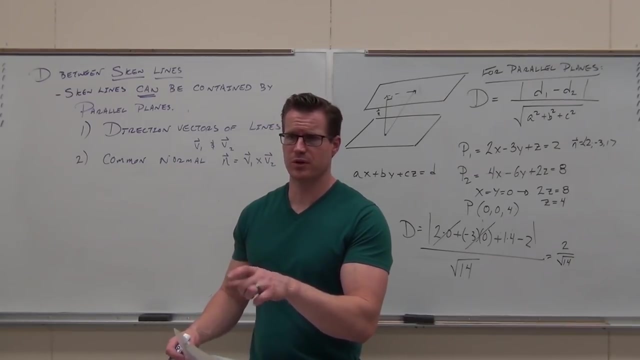 they will have a common normal. You find the normal between those vectors. That will be the normal of the plane. Every line is given. we've had some lines in parallel, but every line is given to you with at least one point. If you just plug in, t equals zero. 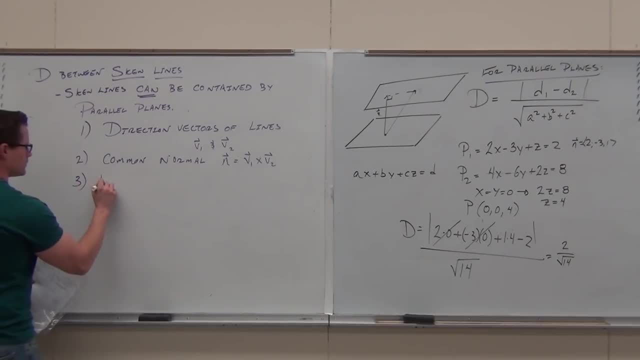 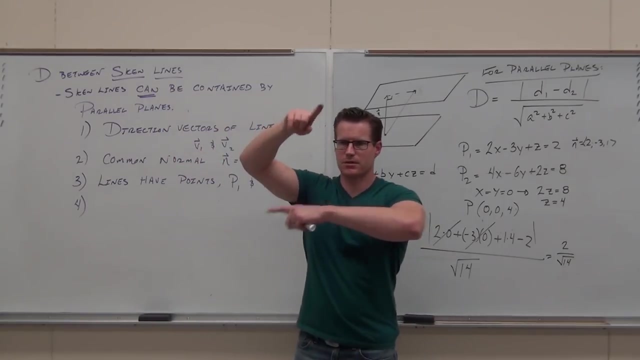 you get a point. Lines have points. Two lines, two points. I know that's a lot at one time. If you've got lines like this, They've got direction vectors like this. Consider them to be contained in parallel planes. Planes need a normal. 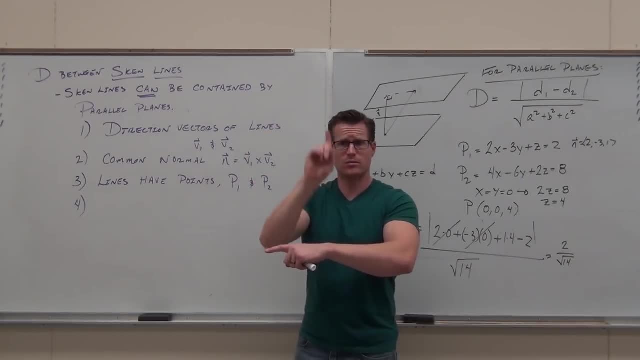 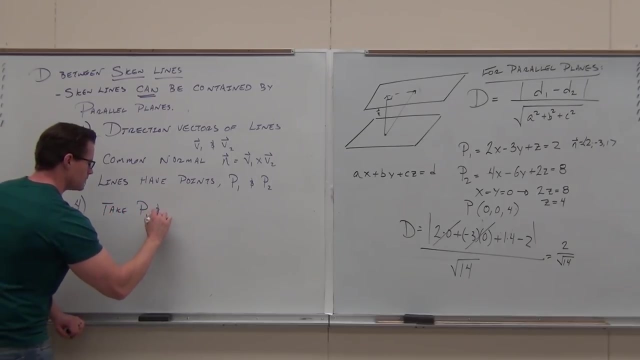 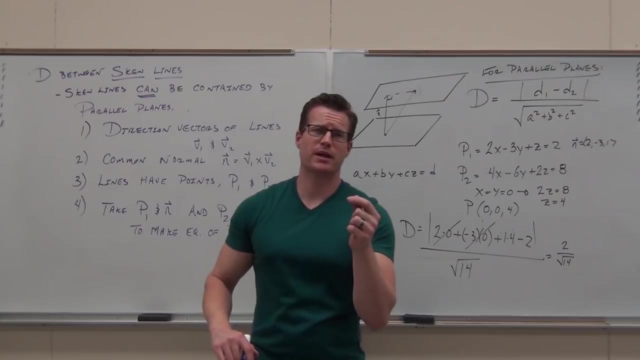 Cross them to find your normal. Now you have a normal for both planes. Lines have points. Take the normal with each independent point. find the equation for planes, Two of them. Those planes will be parallel. They have the same normal. They can't be anything other than parallel. 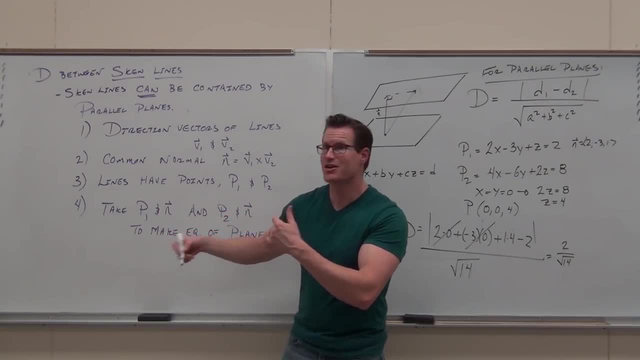 So when you find those two planes that are parallel, you have the equation right. Those equations are going to have some d's in them. Take the d's, take the common normal distance between parallel planes. So after this stuff, distance between parallel planes. 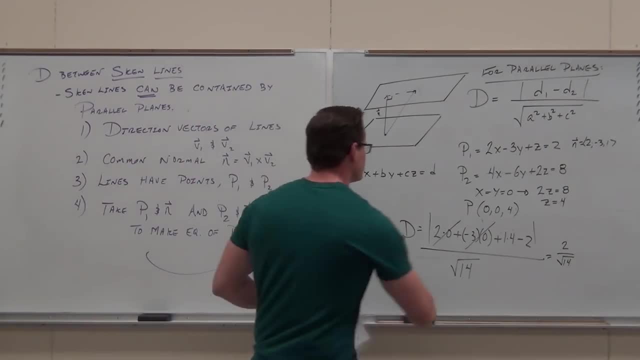 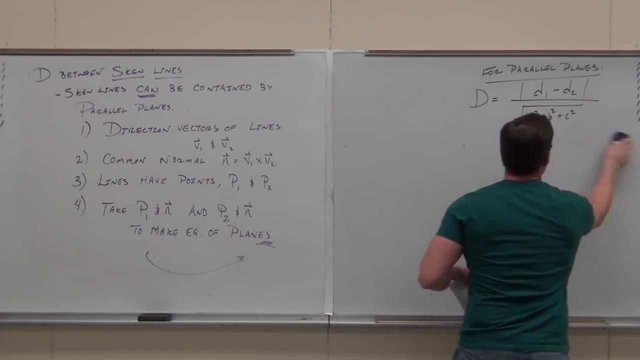 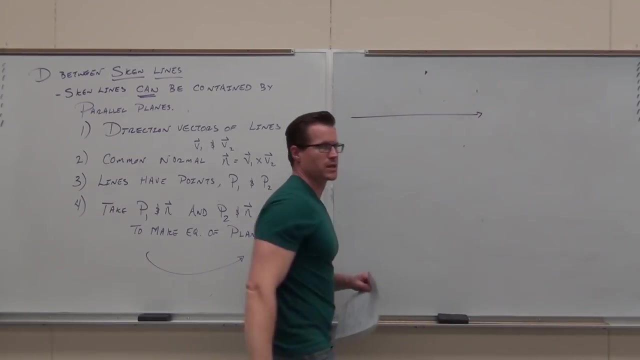 That's the idea on how you would do it. The last thing that we're going to do. How to find the distance between a line and a point Doesn't seem so hard, but consider that the line is going through space And you go. How do I do that? 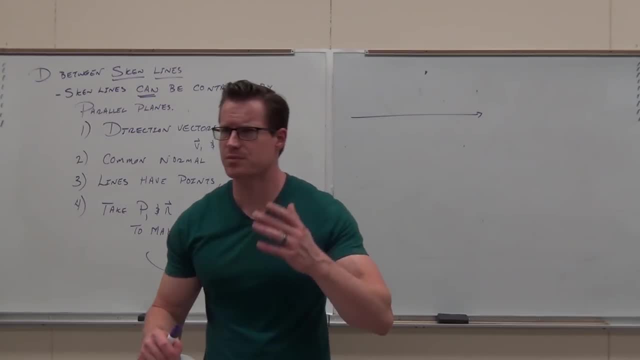 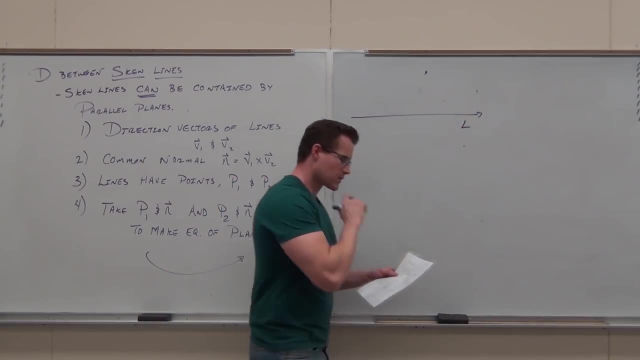 It doesn't seem so hard. but consider that the line's going through space And you go. how do I do that? Here's the idea. If that's our line, then we're going to do the same thing. Number one thing I want to do: I want to put a point on the line. 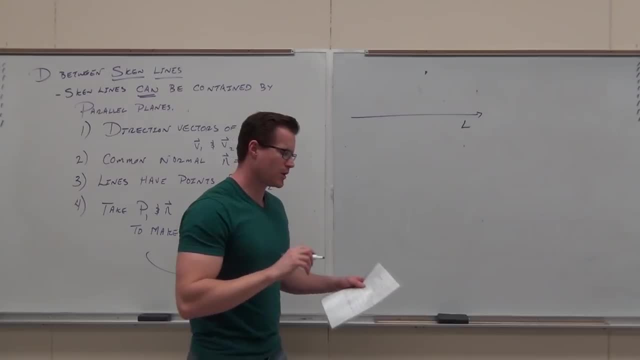 Here's the idea. If that's our line, the number one thing I want to do. I want to put a point on the line. We'll call it Q. I want to find a vector. I don't know where that point is going to be. 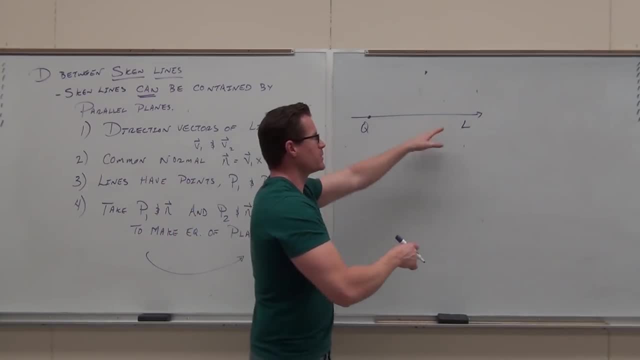 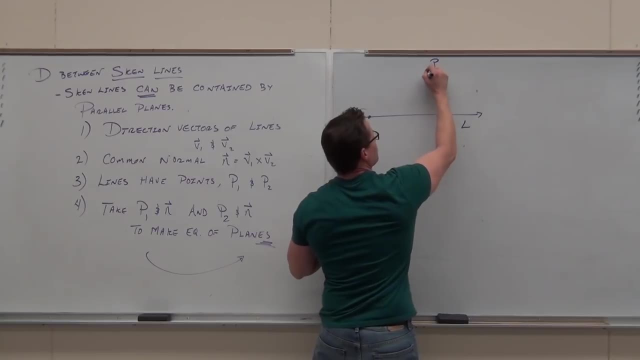 and I can't just say it's right under P because I don't know where that's at. So I need to put some point on the line and the point's typically given on the equation of a line, It's given to you And I have a point P out here on space. 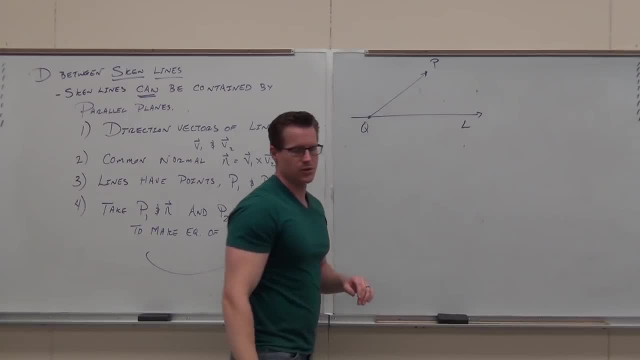 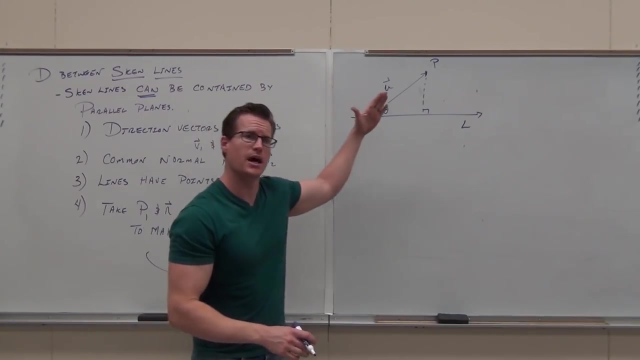 off of the line. Create a vector from Q to P- Let's call that U, And I want to find this. Keep in mind: there's going to be an angle between any vector off of the line and the vector of the line itself. Let me go through it real quick. 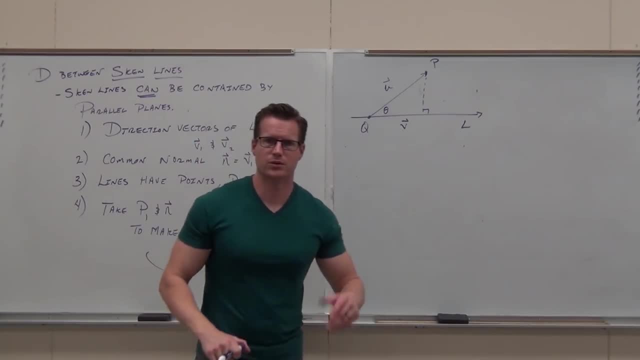 We'll do our example okay, So check it out. I get a point not on the line. If it's not on the line, I can find a point on the line Q and a direct vector to P Head down. if you're okay with that one. 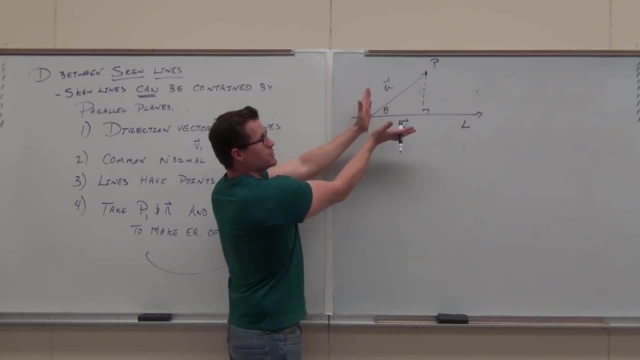 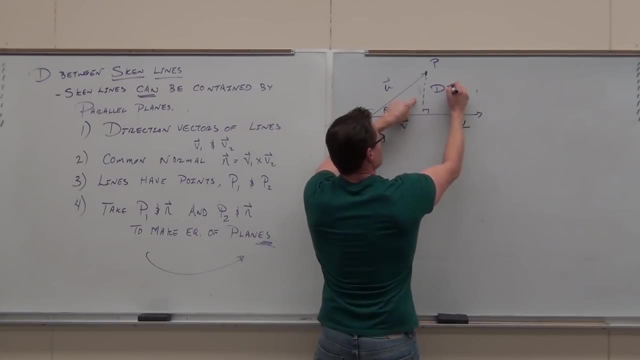 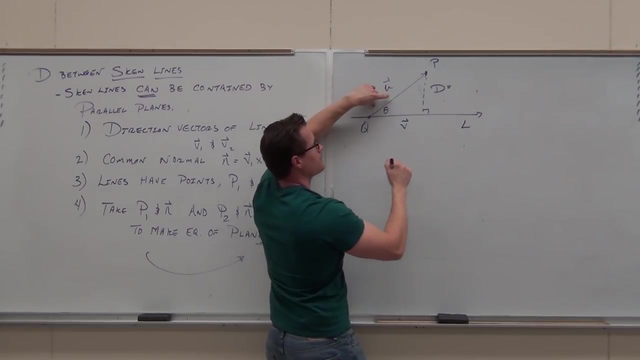 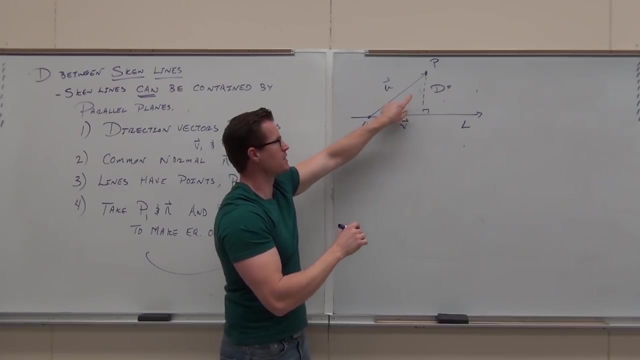 Lines also have vectors. Any two non-parallel vectors have an angle between them. If you use sine, this distance of the line, this distance is, let's see, sine would be opposite over hypotenuse. so if I solve for this, it's going to be. 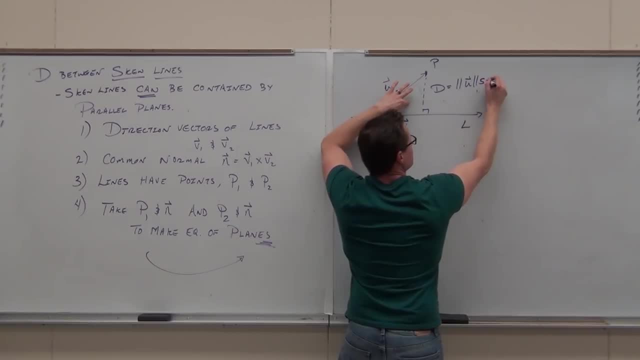 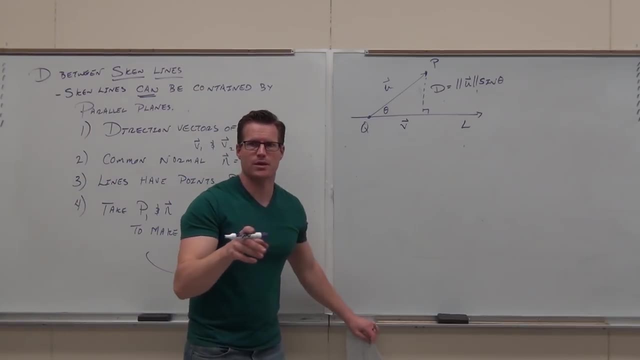 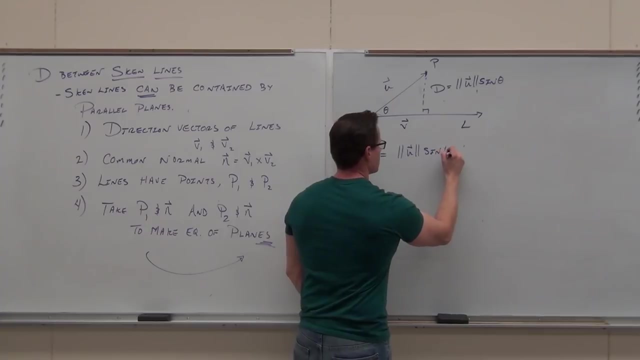 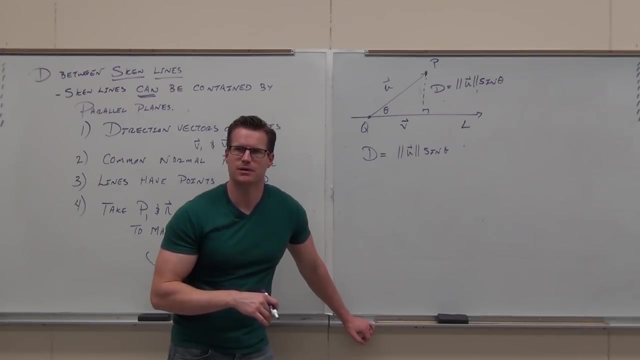 hypotenuse sine beta. You guys? okay with that? Here's some math magic. We're going to invent some stuff Right now. what I'm going to do is I'm going to multiply both sides by the magnitude of vector V. Magnitudes are scalars, right? 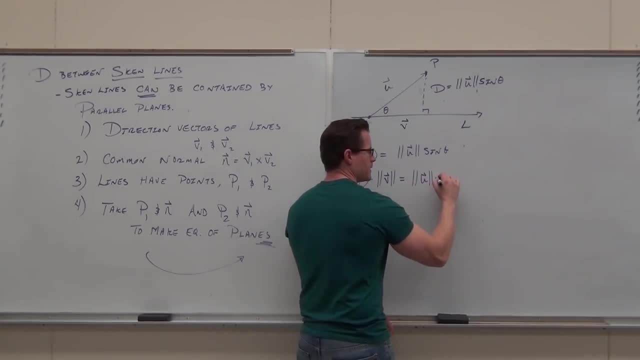 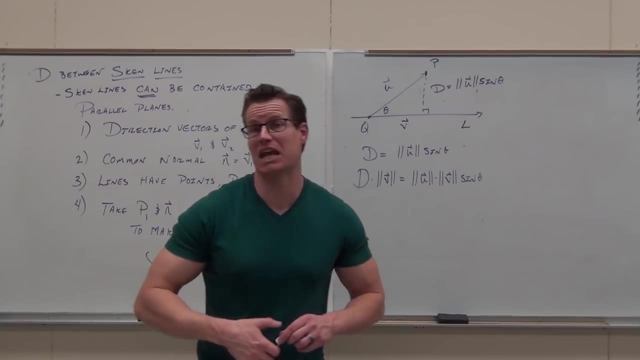 So I can multiply both sides by this scalar and still consider it to be equal. And you go what, Leonard? You're crazy man. You got too much candy, Which is why I'm talking very fast, But that's okay. I don't get it very often. 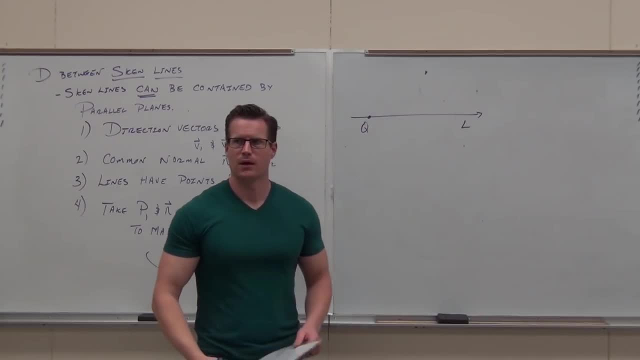 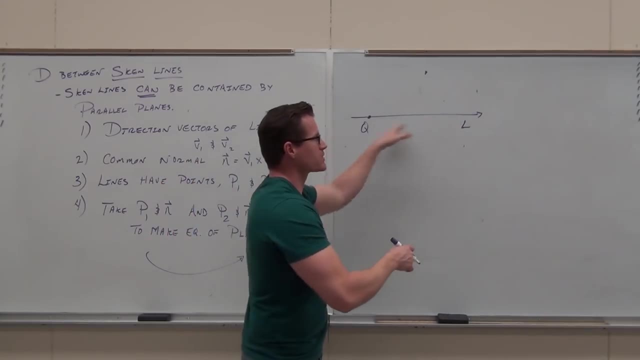 We'll call it Q. I want to find a vector. I don't know where that point's going to be and I can't just say it's right under P, because I don't know where that's at. So I need to put some point on the line and the point's typically given. 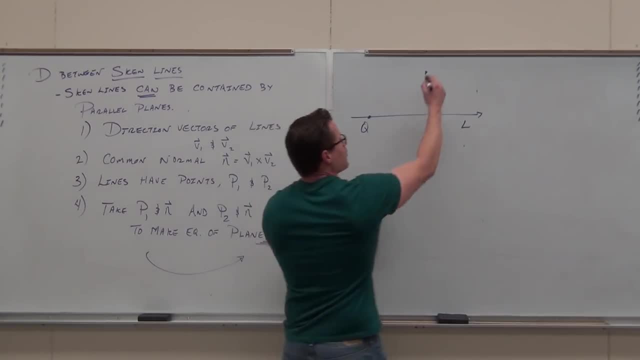 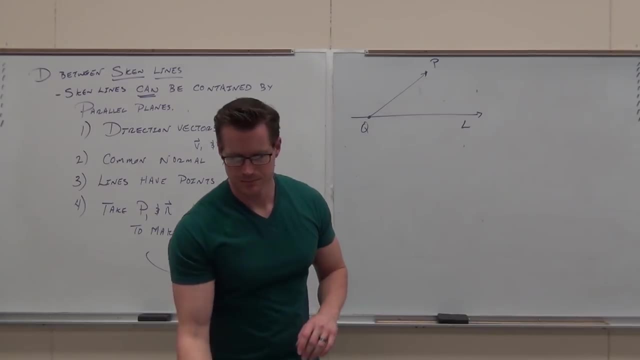 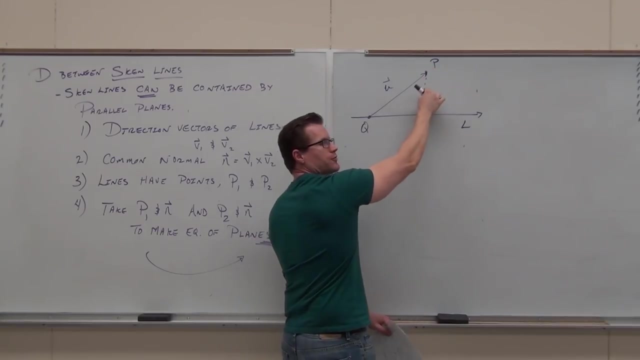 on the equation of a line. right, It's given to you And I have a point P up here on space, off the line. Create a vector from Q to P, Let's call that U, And I want to find this. Keep in mind: there's going to be an angle between any vector off of the line. 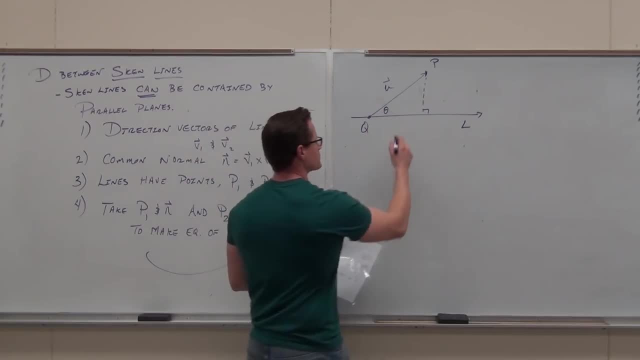 and the vector of the line itself. Let me go through it real quick. We'll do our example, okay, So check it out. I get a point not on the line. If it's not on the line, I can find a point on the line Q and a vector, 2P. 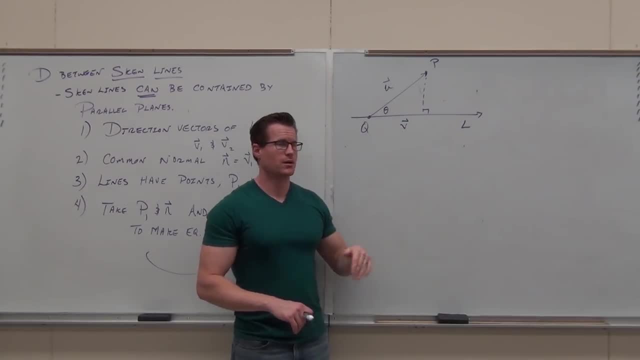 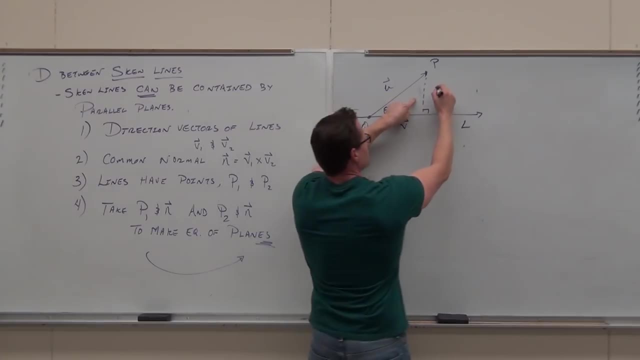 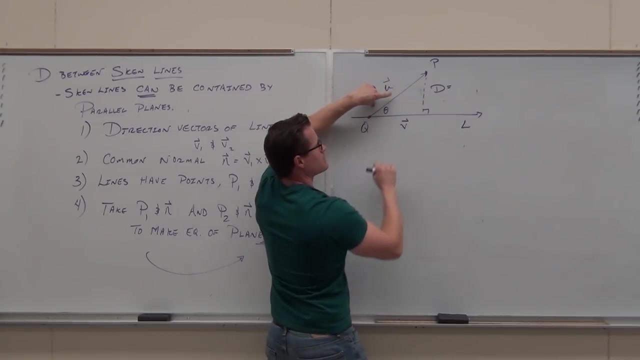 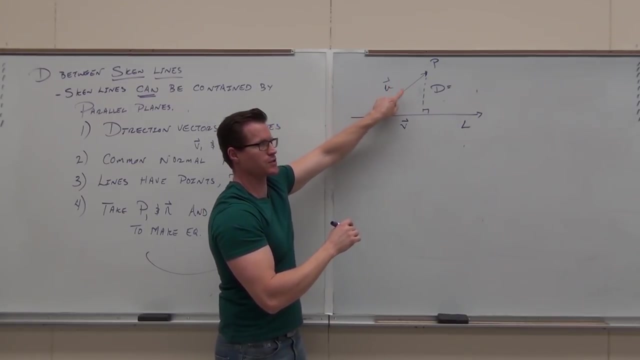 Head down, if you're okay with that. one Lines also have vectors. Any two non-parallel vectors have an angle between them. If you use sine, this distance is, let's see. sine would be opposite over hypotenuse. So if I solve for this, it's going to be hypotenuse. 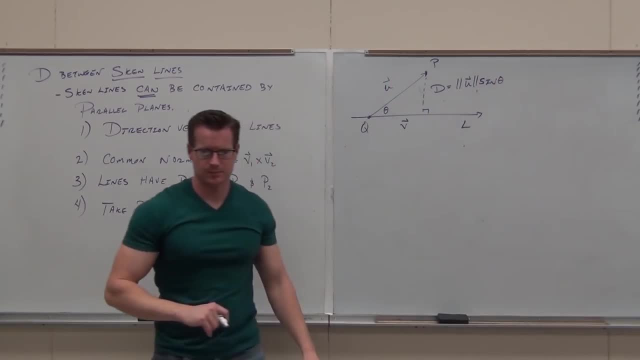 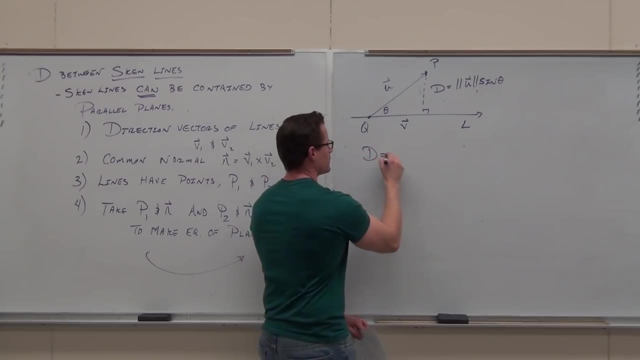 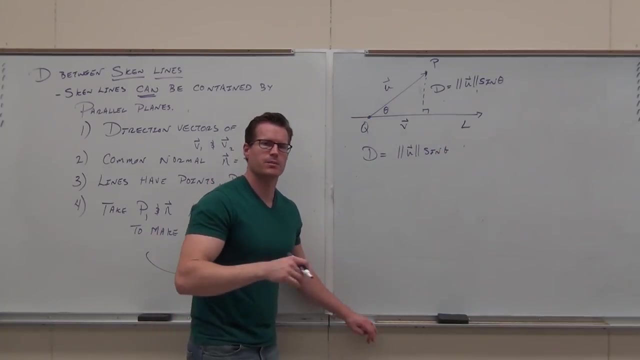 So if I solve for this, it's going to be hypotenuse Sine beta. You guys, okay with that? Here's some math magic. We're going to invent some stuff. Right now, what I'm going to do is I'm going to multiply both sides by the magnitude of vector V. 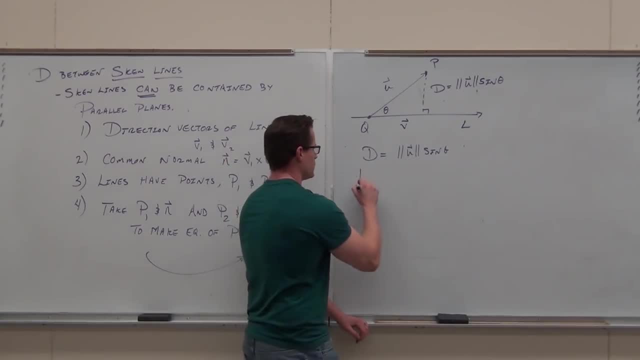 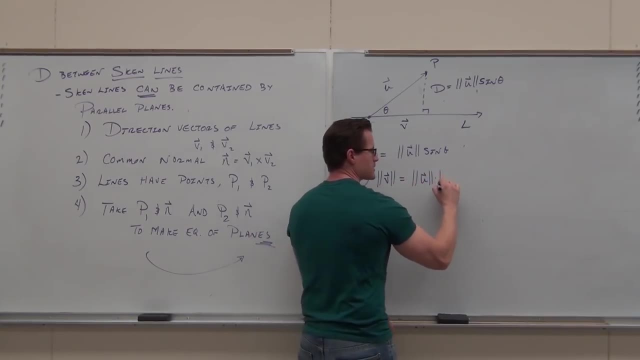 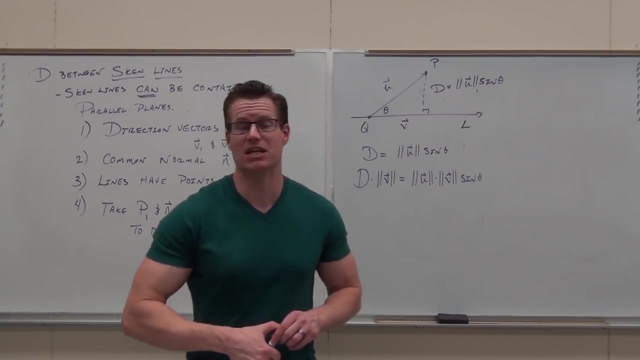 Magnitudes are scalars, right, So I can multiply both sides. I can multiply both sides by the scalar and still consider it to be equal, and you go one letter. you're crazy man, you've got too much candy. 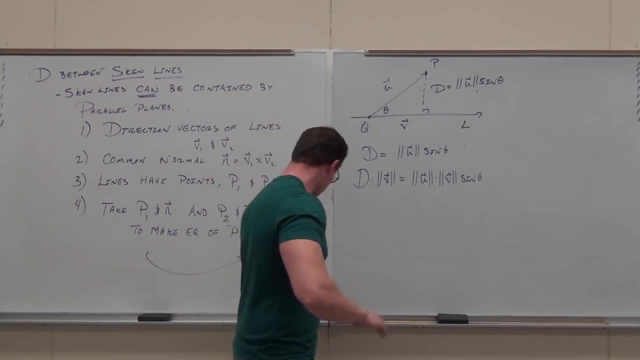 I have had some candy today, which is why I'm talking very fast, But that's okay. I don't get it very often. So what? Why would we do it? If you look at that, that should be really, really, really familiar. 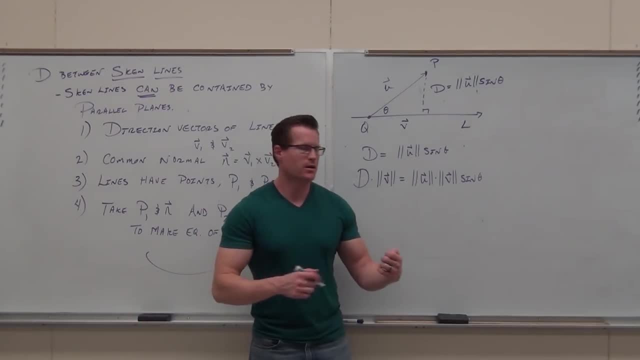 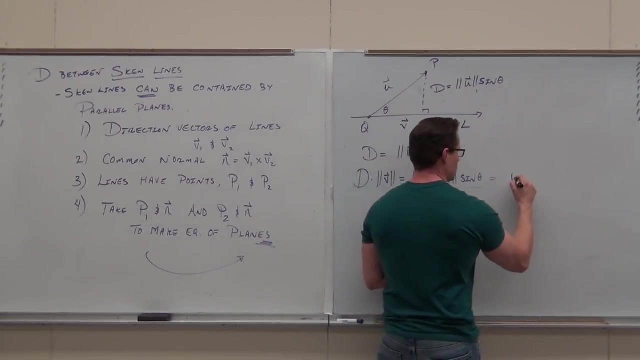 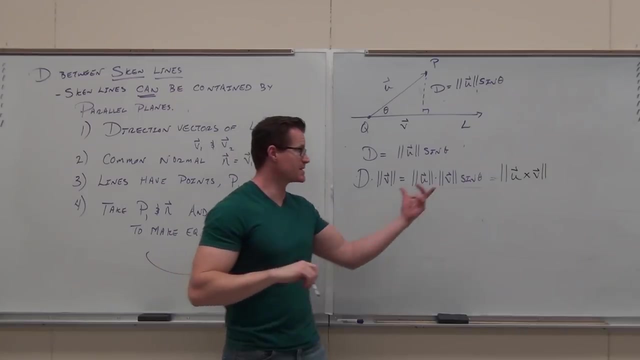 So what? Why would we do it? If you look at that, that should be really, really, really familiar. Not just the cross product, Very close The magnitude of the cross product. This is not a vector, So it cannot be a vector. 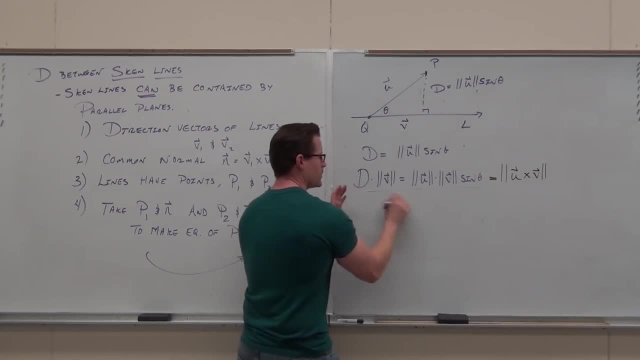 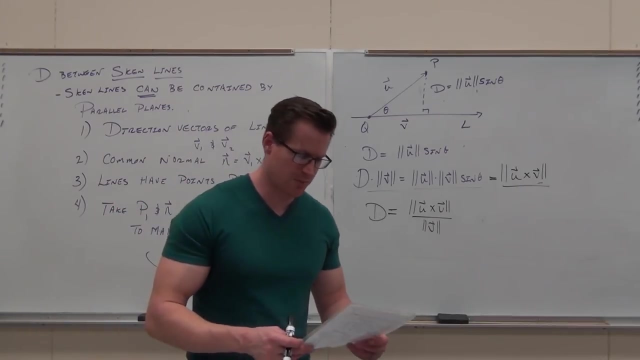 So it can't be the cross product, but it's the magnitude of the cross product. If I divide both sides by the magnitude of V, the distance between a line and a point is this: I would like to give you an example, since this recording device 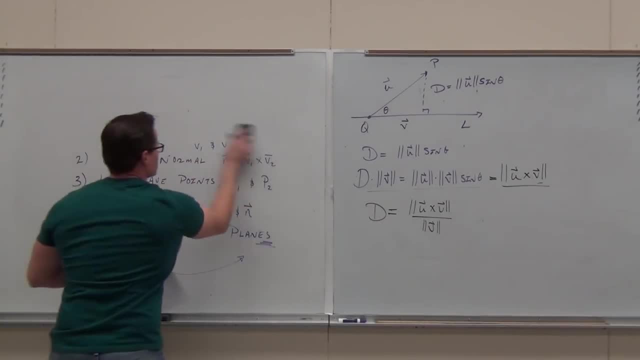 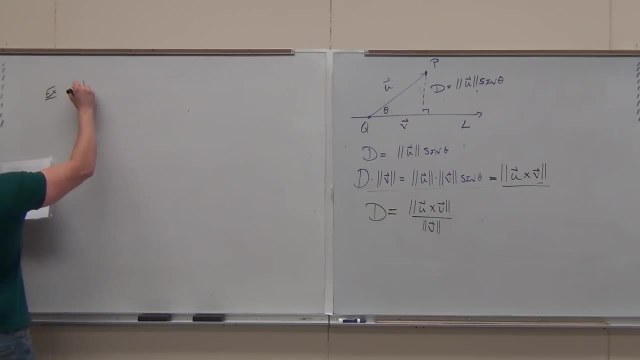 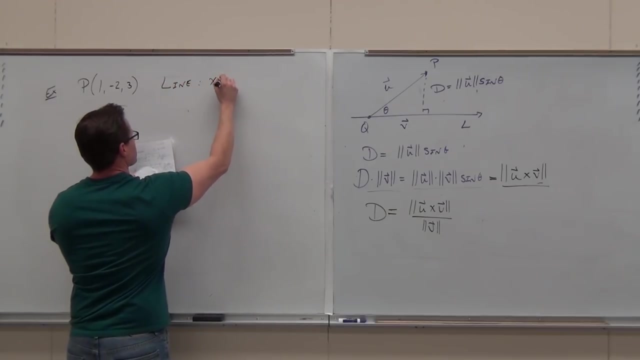 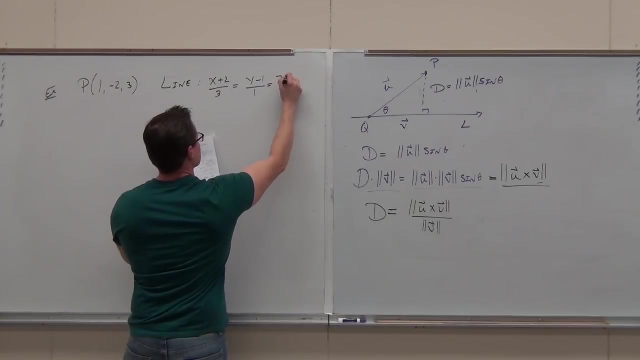 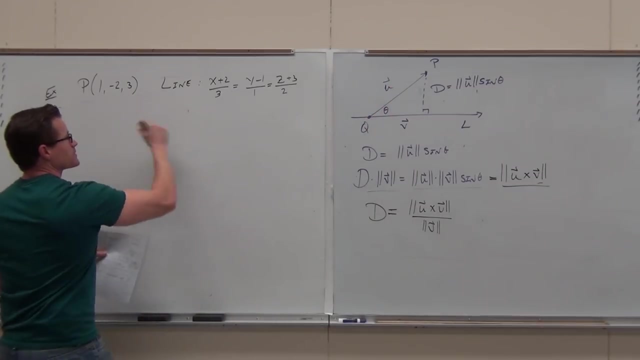 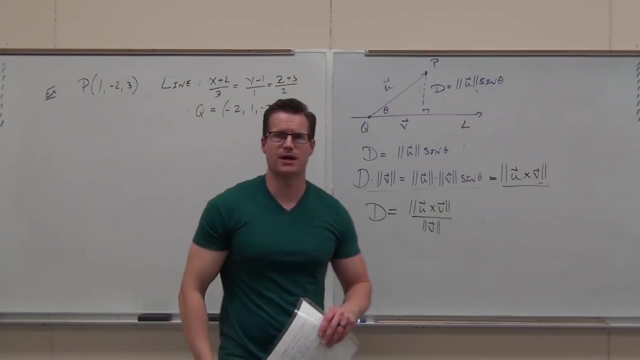 is going to stop in four minutes. Here's the things we need. We need a vector from P to Q. We need a vector from the line to this point. This point Q would be- I know I'm moving fast, but you can follow me on the point from that line. 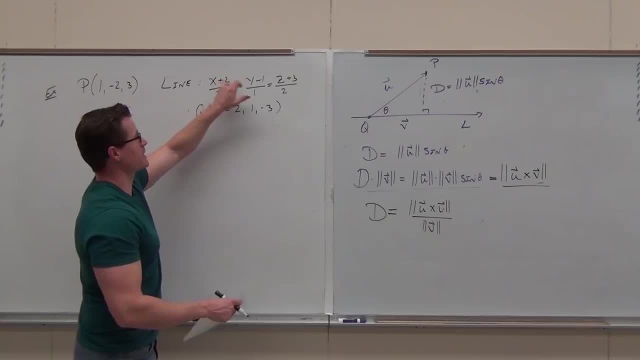 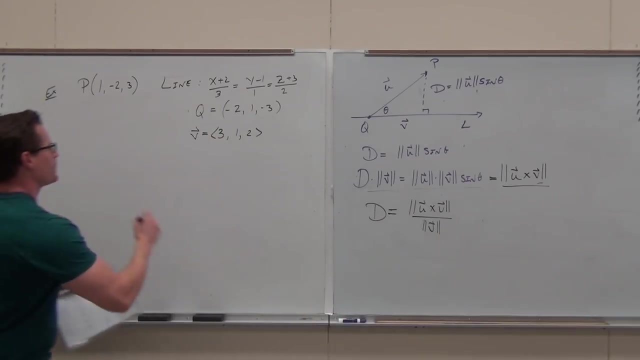 It's pretty easy to find a point on a line With symmetric. it's just: We get. We also need a vector. The vector is really easy. I love vectors from that form of a line. You just read the denominator, That's the vector. 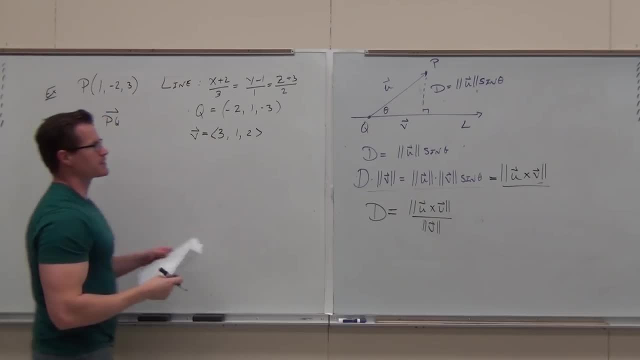 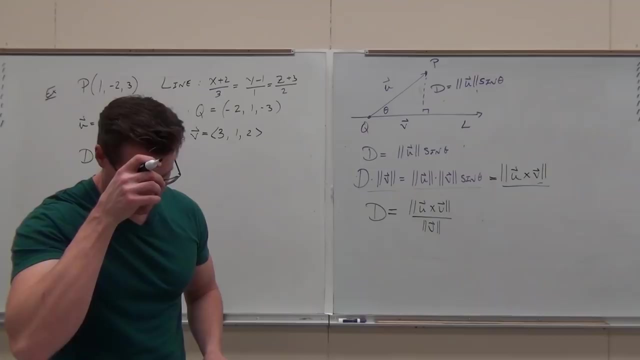 We also need a vector from Q to P or P to Q, it doesn't matter, That'll work. Then we can find our distance. Distance is simply U cross V, magnitude divided by magnitude of V, This V. There's one thing I want you to not do, though. 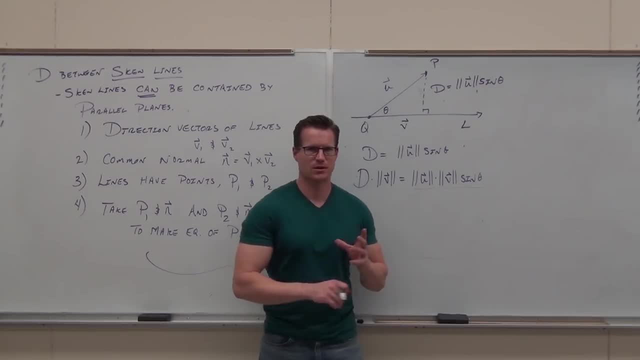 Not just the cross product- Very close: The magnitude of the cross product. The cross product has to. this is not a vector, This is a number, So it cannot be a vector, So it can't be the cross product, but it's the magnitude of the cross product. 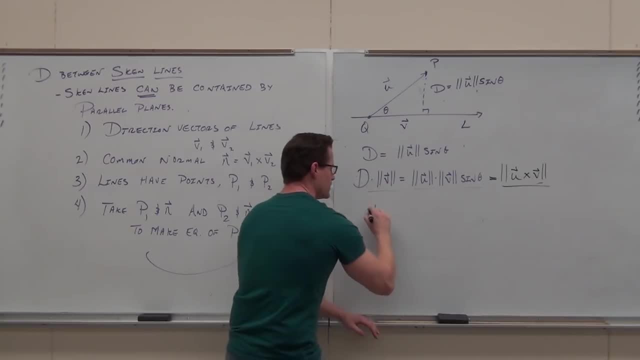 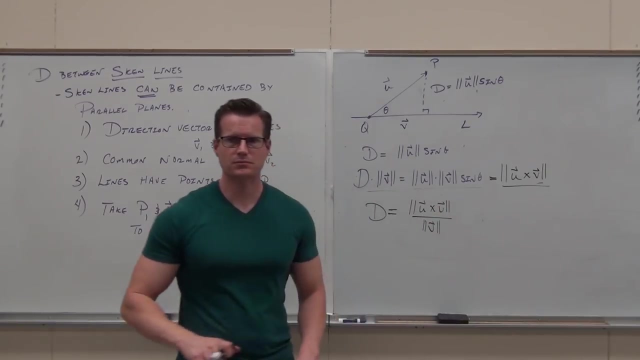 If I divide both sides by the magnitude of V, the distance between a line and a point, I would like to give you an example, since this recording device is going to stop in four minutes. so we're going to stop in four minutes. 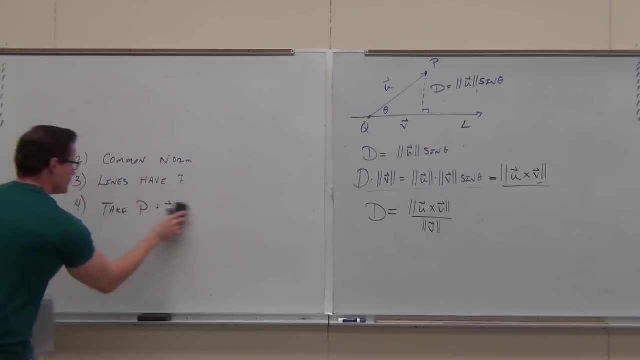 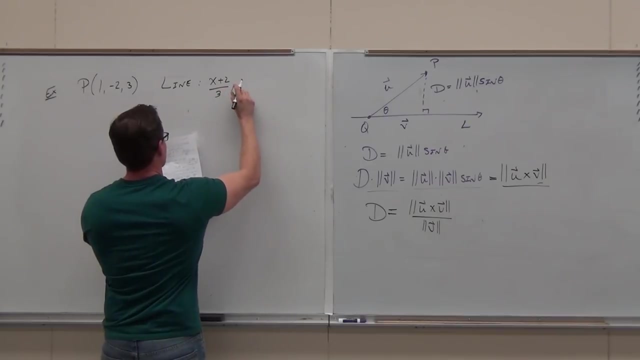 Here's the things we need. We need a vector from P to Q. We need a vector from the line to this point. 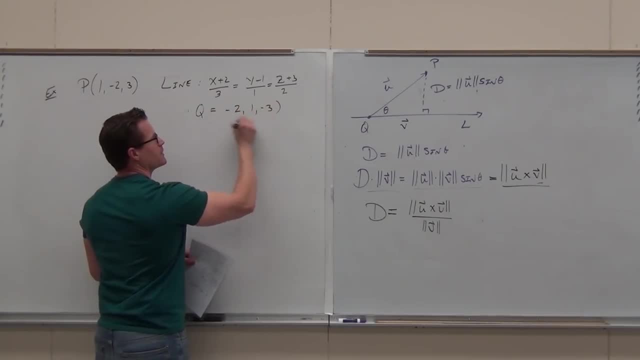 This point Q would be negative 2, 1, negative 3.. I know I'm moving fast, but you can follow me on the point from that line. It's pretty easy to find a point on a line. It's with symmetric, it's just negative, positive, negative. 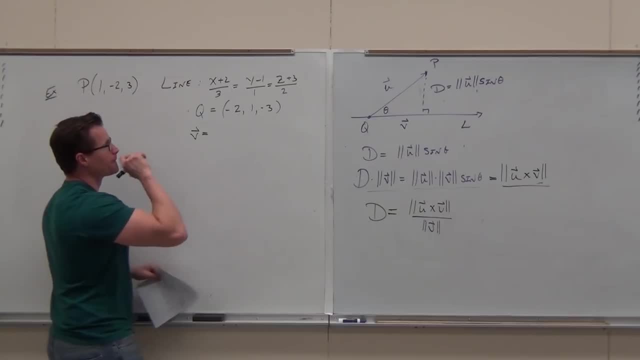 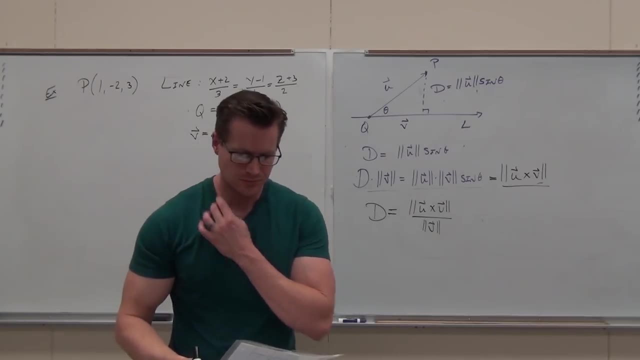 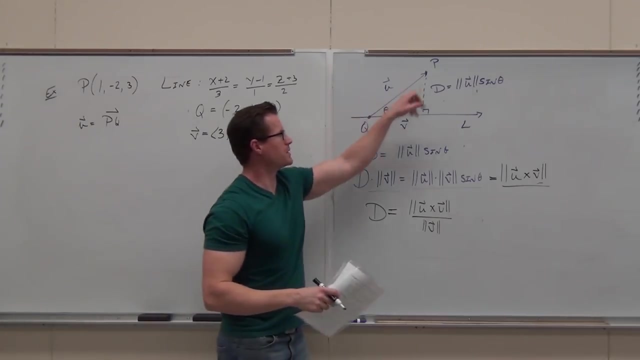 We get 2,, 1,, 3.. We also need a vector. The vector is really easy. I love vectors from that form of a line. You just read the denominator. That's the vector. We need a. we also need a vector from Q to P. 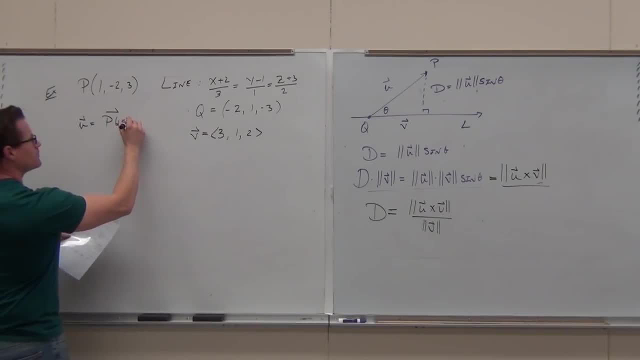 or P to Q, doesn't matter. We need a vector from Q to P or P to Q doesn't matter, And then we can find our distance. Our distance is simply U cross V, magnitude divided by magnitude of V, this V. 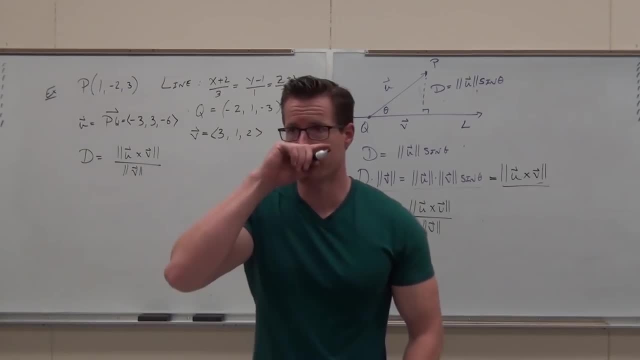 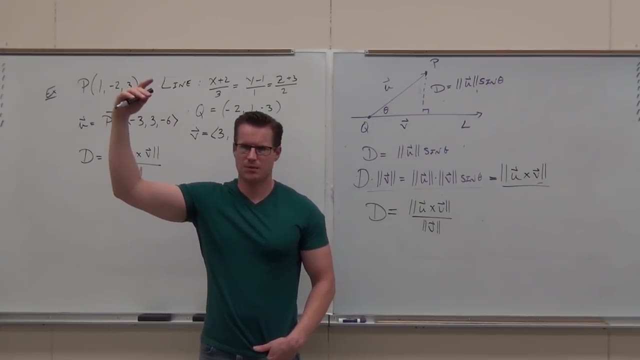